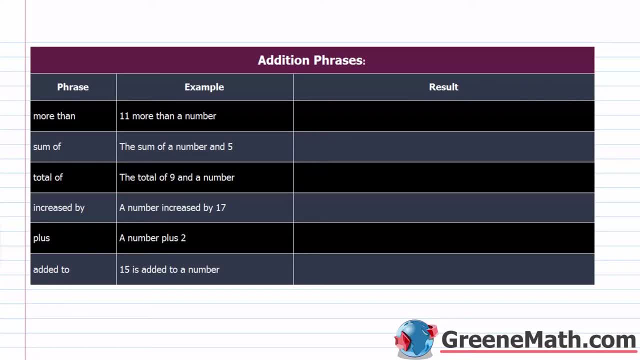 going to start today by looking at some common addition phrases. So first we have for a phrase: more than so more than is telling us we need to add. So, as an example, we have eleven more than a number. Now, anytime I see a number or the number, I can replace it with a variable. 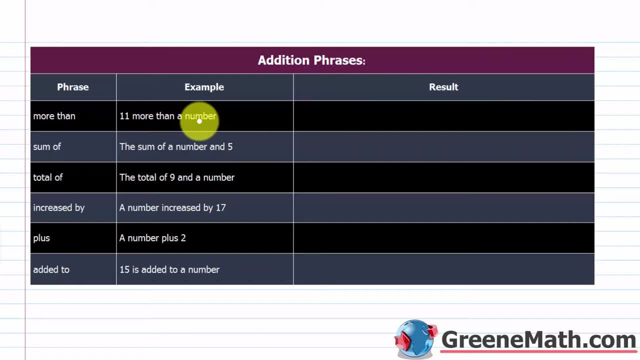 like x or y or z, whatever you want to use. I'm just going to use x. One strategy is just to kind of line out where you see a number and just put a variable. I'm just going to put x there And if I read it now it says 11 more than x. Well, that just means, if I 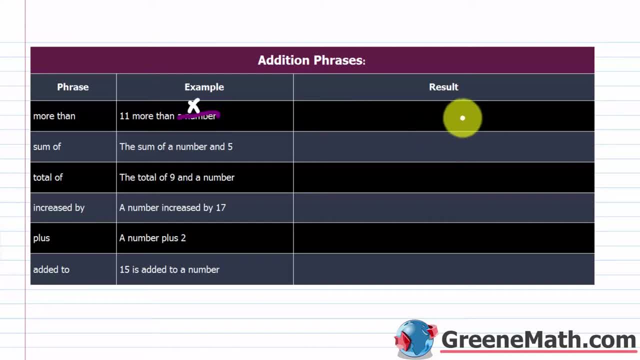 had x. I want 11 more than that. So that can be represented with x plus 11, right? This is 11 more than x. Then you have sum of, So the sum of a number and 5.. So again, when 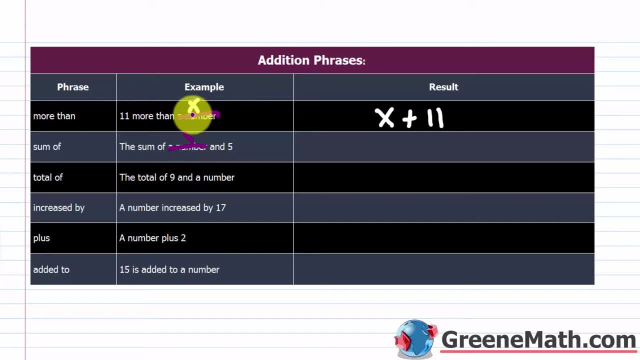 I see a number. I'm just going to line that out and put x. Let me kind of change my ink here. So the sum of x and 5, that's just x plus 5.. Then next we have total of, So the. 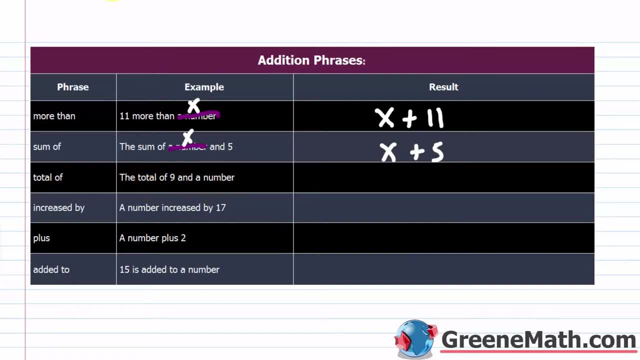 total of 9 and a number. So let me line this out and let me put x here. So now we have the total of Of 9 and x. So that just tells me I have x plus 9 or 9 plus x. So next we have increased. 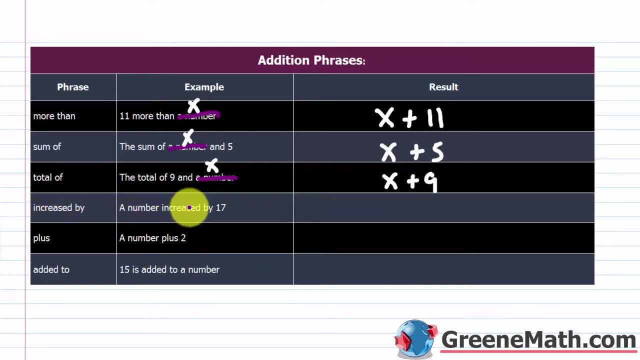 by. And then we have, for our example, a number increased by 17. So where I see a number, I'm going to cross that out. Just put x. So if x is increased by 17,, it's just x plus. 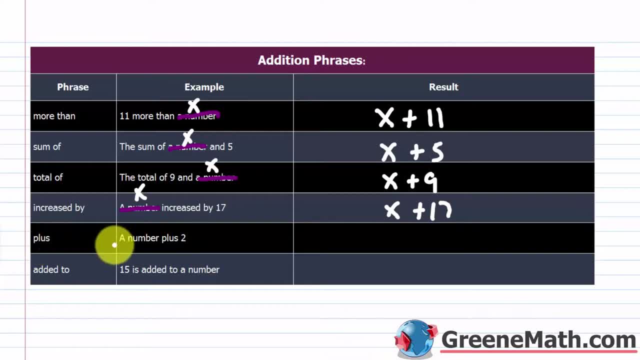 17. Then we have plus A number plus 2. So again, let's line this out on a number, Let's put x here, And it says x plus 2.. It's just x plus 2. Very straightforward. Then, lastly, we have added to, And then we 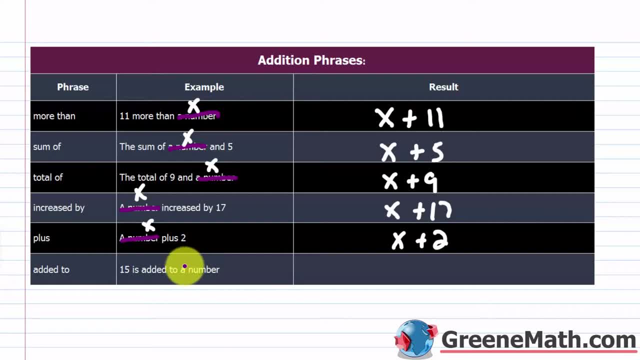 see 15 is added to a number. Let me line this out where it says a number. Let me put x here. So 15 is added to x, So we have x plus 15.. OK, So it's very easy when you're working with addition, because addition is commutative. 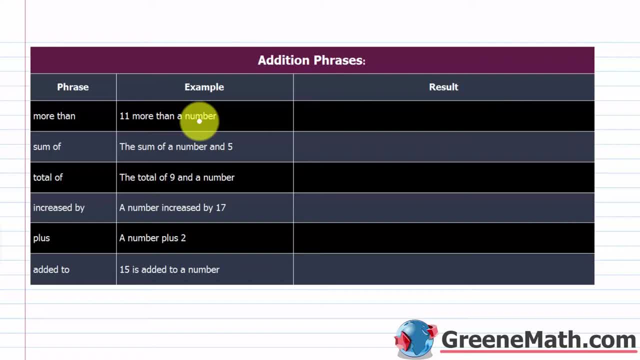 y or z, whatever you want to use. I'm just going to use x. One strategy is just to kind of line out where you see a number and just put a variable. I'm just going to put x there And if I read it, 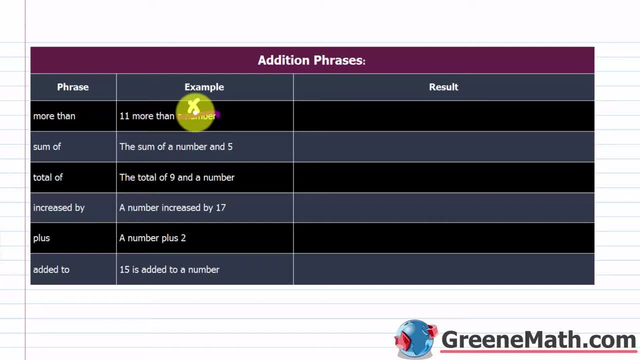 now it says 11 more than x. Well, that just means if I had x, I want 11 more than that. So that can be represented with x plus 11, right, This is 11 more than x. Then you have. 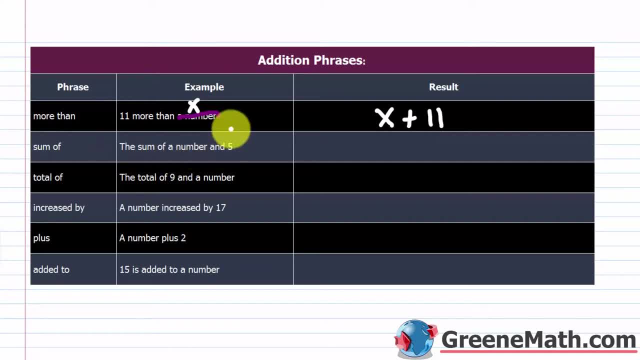 sum of, So the sum of a number and 5.. So again, when I see a number, I'm just going to line that out and put x- Let me kind of change my ink here. So the sum of x and 5, that's just x plus 5.. 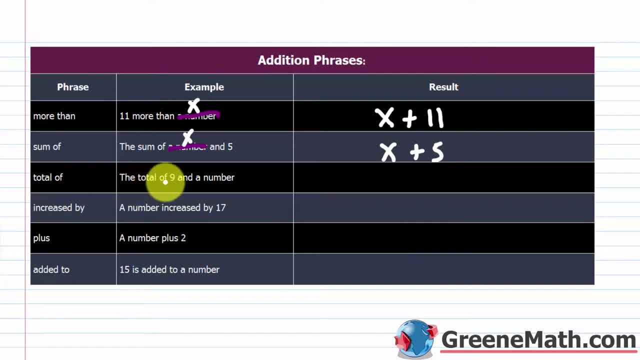 Then next we have total of, So the total of 9 and a number. So let me line this out And let me put x here. So now we have the total of 9 and x. So that just tells me I have x plus 9. 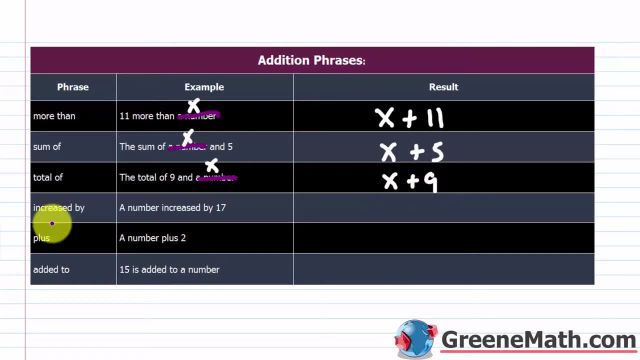 or 9 plus x. So next we have increased by, And then we have, for our example, a number increased by 17.. So where I see a number, I'm going to cross that out. Just put x. So 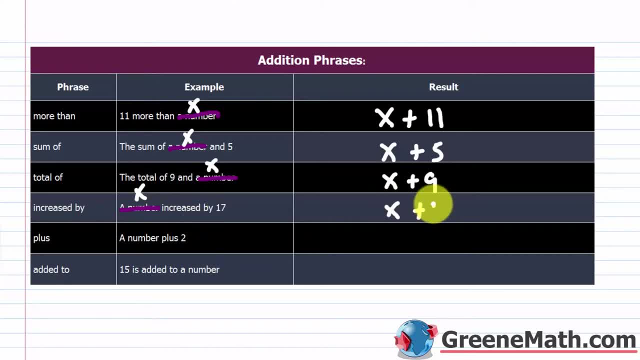 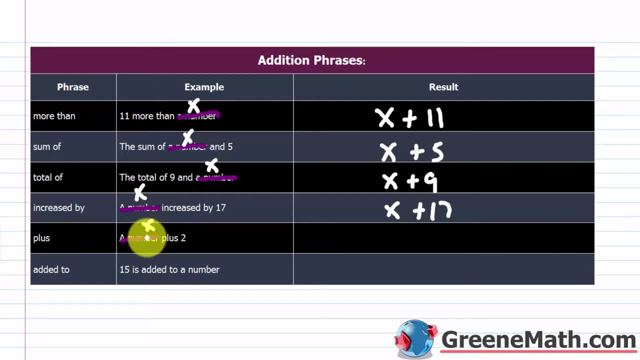 Let's line this out on a number. Let's put x here, And it says x plus 2.. It's just x plus 2. Very straightforward. Then, lastly, we have added to, And then we see 15 is added to a number. 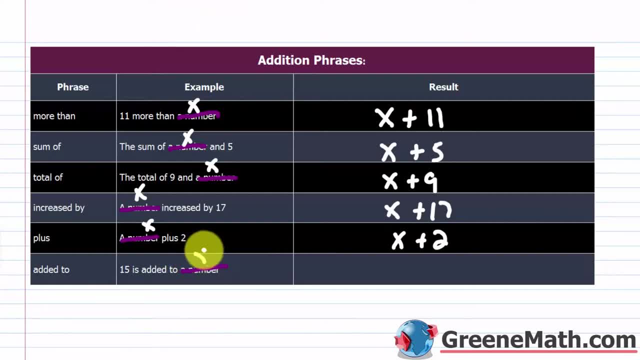 Let me line this out. where it says a number, Let me put x here. So 15 is added to x, So we have x plus 15.. Okay, So it's very easy when you're working with addition, because addition is commutative, The order that you add in does not affect. 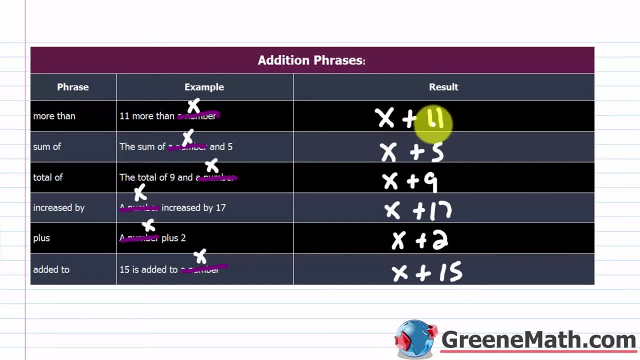 the result. So in this case, where we have x plus 11, I could reorder that and say 11 plus x. It doesn't change anything. Same thing here: x plus 5 could be 5 plus x. x plus 9 could be 9. 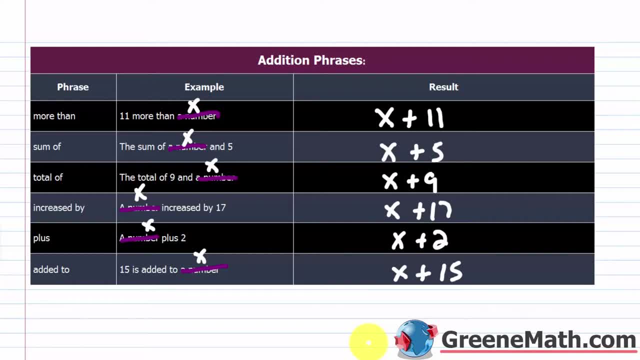 The order that you add in does not affect the result. So in this case, where we have x plus 11.. I could reorder that and say 11 plus x. It doesn't change anything. Same thing here: X plus 5 could be 5 plus x, X plus 9 could be 9 plus x. You know so on and so forth. 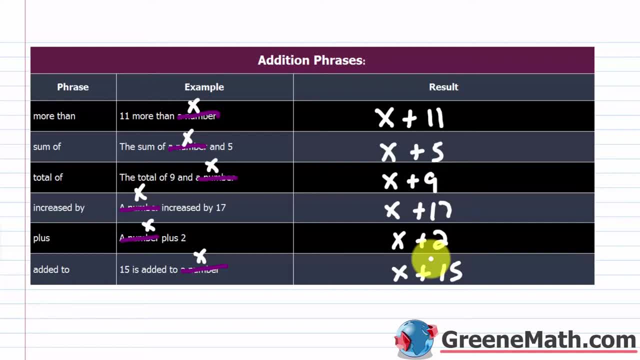 So with addition and also multiplication they're commutative. The order does not matter. With subtraction and division the order does matter. So we've got to pay closer attention to the way things are worded when we work with subtraction and division. So let's look. 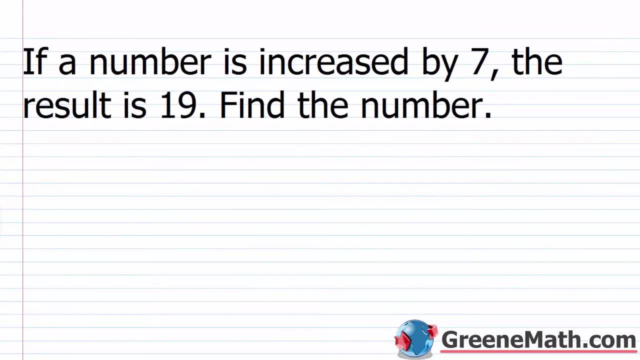 at an example of some addition phrases, And we have this sample problem here. So if a number is increased by 7, the result is 19.. Find the number. So again, if I see something like a number or if I see the number, I'm 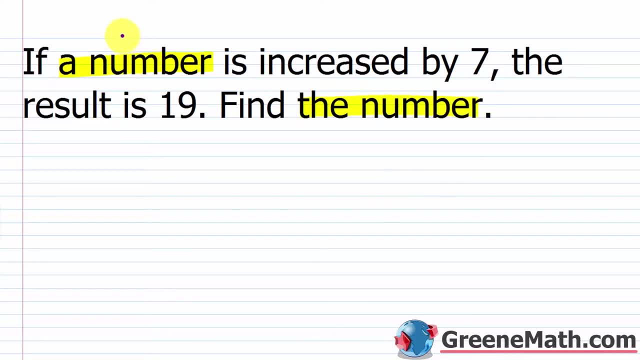 just going to replace it with a variable, So I'm going to use x, but again, you can use whatever you want. I'm just going to put that in each place And down here I can even specify that I'm going to let my variable x be equal to the. 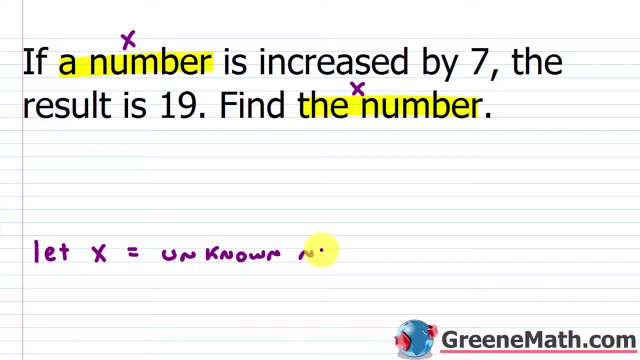 unknown. There, Huh, number, Let me make that e a little bit better. Okay, so what am I saying here? If x- let me write that down- is increased by, we know this is a key phrase. that means plus. So x, plus we have our. 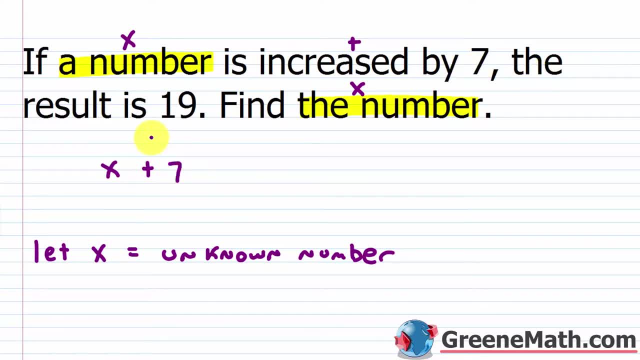 number seven. It says: the result here is 19.. So when you see is in this context, here it means equals. Okay, so we're going to put equals here and then we have 19. So, once again, if x is, 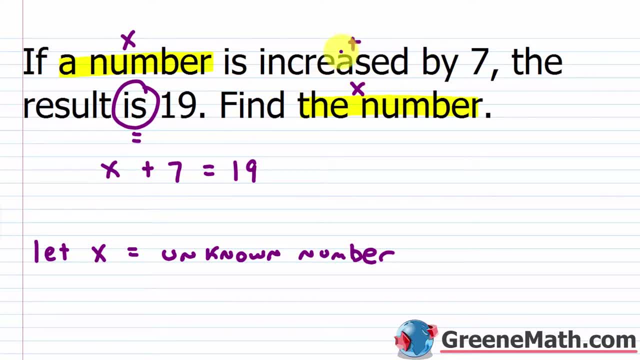 increased by. we have our x here. increased by again means plus. then we have seven, seven's here. The result is that means equals. and then we have our 19,. so our 19 is here. So we want to. 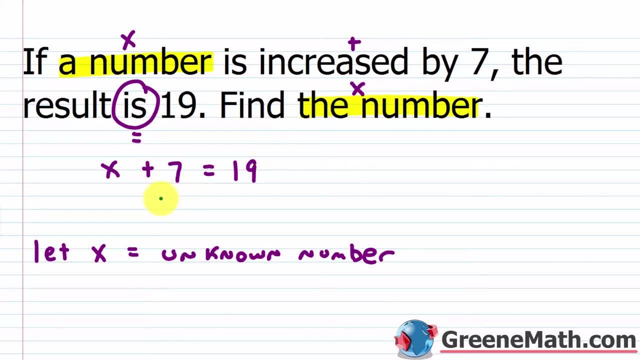 find x and all we need to do is just solve this guy. So I'm going to subtract seven away from each side of the equation and that's going to give me that x is equal to 12.. You can read back through the problem and determine if you got the right answer right If 12 is increased by seven. 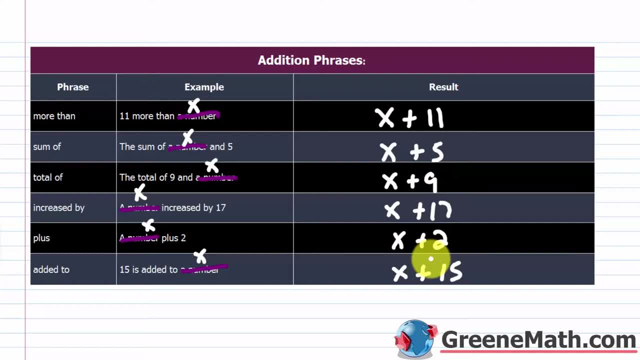 plus x, You know so on and so forth. So with addition and also multiplication they're commutative. The order does not matter. With subtraction and division the order does matter. So we've got to pay closer attention to the way things are worded when we work with. 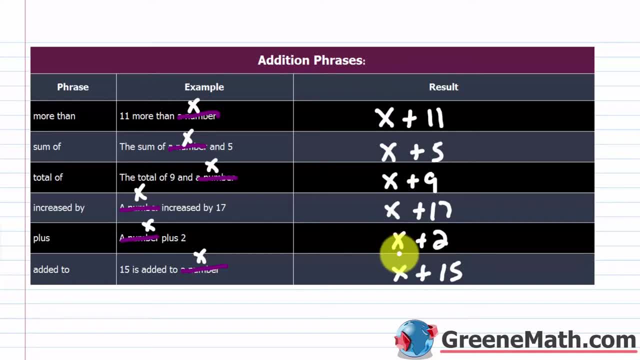 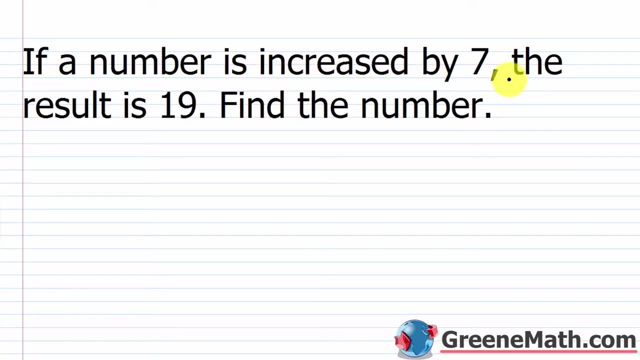 subtraction and division. So let's look at an example of some addition phrases And we have this sample problem here. So if a number is increased by 7, the result is 19.. Find the number. So again, if I see something, 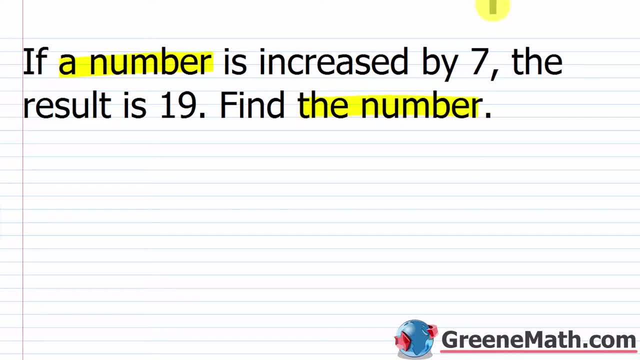 like a number, or if I see the number, I'm just going to replace it with a variable. So I'm going to use x, But again, you can use whatever you want. So I'm just going to put that in each. 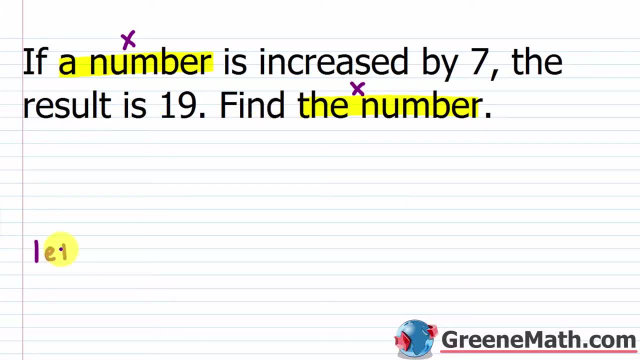 place. And down here I can even specify that I'm going to let my variable x be equal to the unknown number. Let me make that e a little bit better, Okay. So what am I saying here? If x- let me write that down- is increased by, we know this is a key phrase. that means plus. So x, plus. 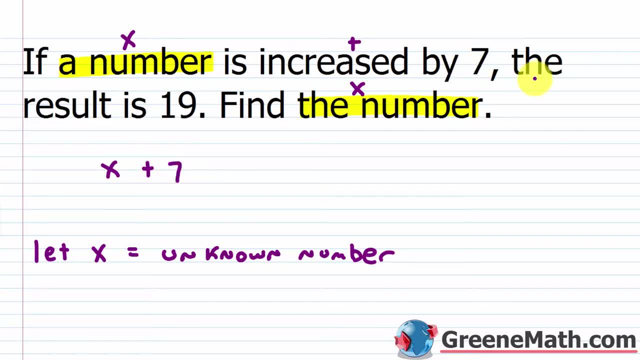 we have our number 7. It says: the result here is 19. So when you see, is in this context, here it means equals. Okay, So we're going to put equals here, And then we have 19. So, once again, if x is increased by, 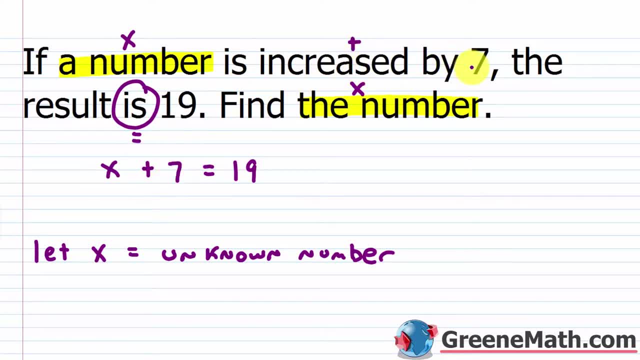 we have our x here. Increased by again means plus. Then we have 7. 7's here. The result is that means equals. And then we have our 19. So our 19 is here. So we want to find x And all. 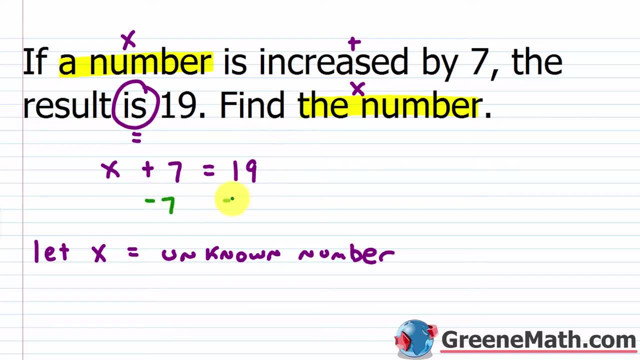 we need to do is just solve this guy. So I'm going to subtract 7 away from each side of the equation And that's going to give me that x is equal to 12.. And you can read back through the equation and determine if you got the right answer. Right, If 12 is increased by 7, the result 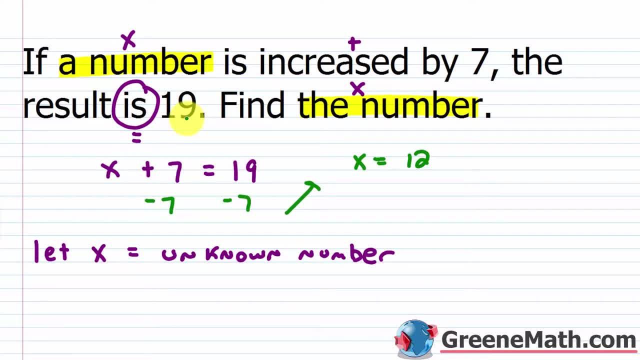 is 19.. Well, yeah, that's true. 12 plus 7, or 12 increased by 7, is 19.. So if we want to find the number, the number is just 12.. Okay, Let's take a look at another one. So if a number is added to, 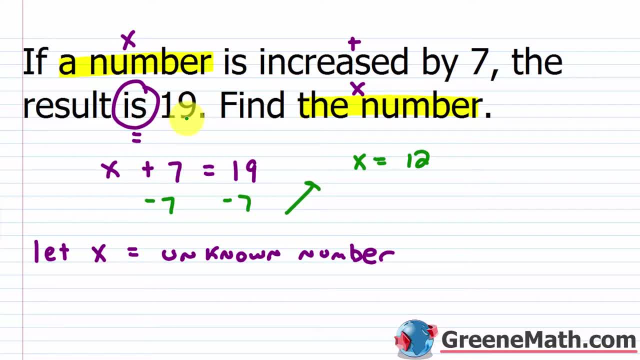 the result is 19.. Well, yeah, that's true. 12 plus seven, or 12 increased by seven, is 19.. So if we want to find the number, the number is just 12.. Okay, let's take a look at another one. So if a? 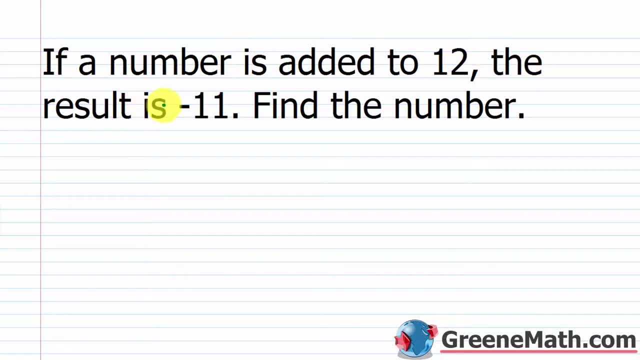 number is added to 12,. the result is negative 11.. We want to find the number. So, again, if I see a number or I see the number, I'm just going to replace that with a variable and I'm going to 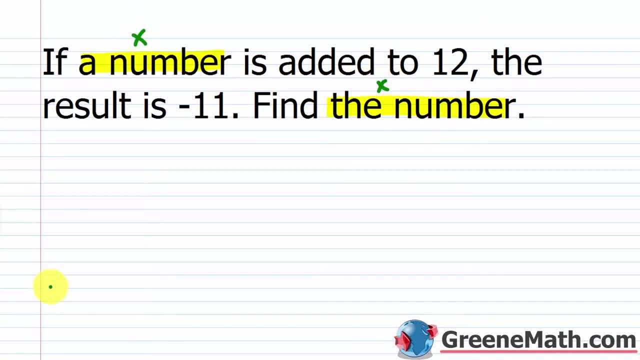 use x Again. I can label this down here and just say that we're going to let x be equal to the unknown number. Okay, just for clarity. And again, if x. so I'm going to read it like that. So if x. 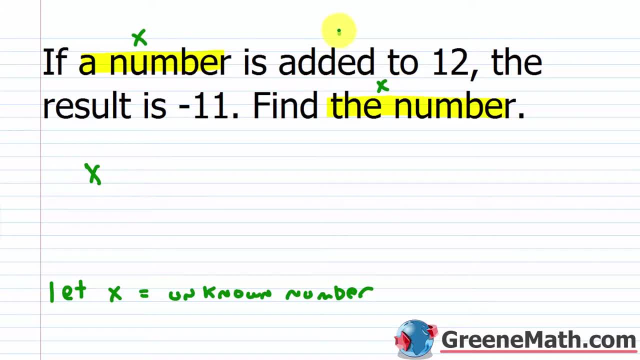 is added to 12,, so is added to just means plus, so x plus and then 12.. The result is okay. in this context, this means equals. then we have negative 11.. Okay, so if x is added to 12,, so x plus 12, the result is: or the result equals negative 11.. So that's how we got. 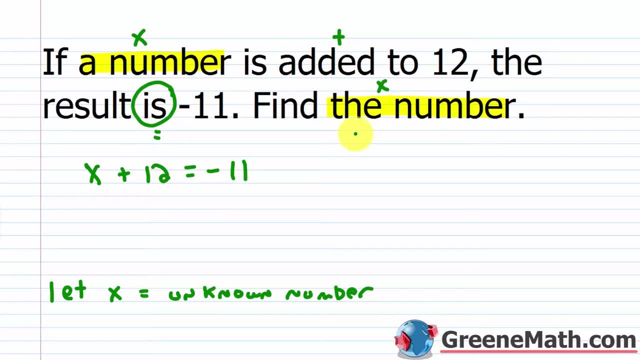 our equation, Then we want to find x or find the number. So again, I just want to solve this guy. Let me subtract 12 away from each side of the equation. I would have that x is equal to negative 23.. Right, And again, reading back through the problem, 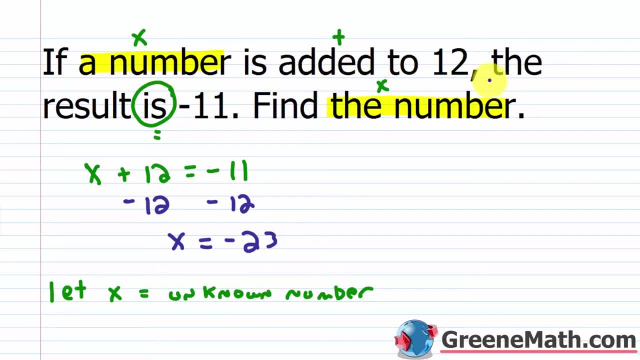 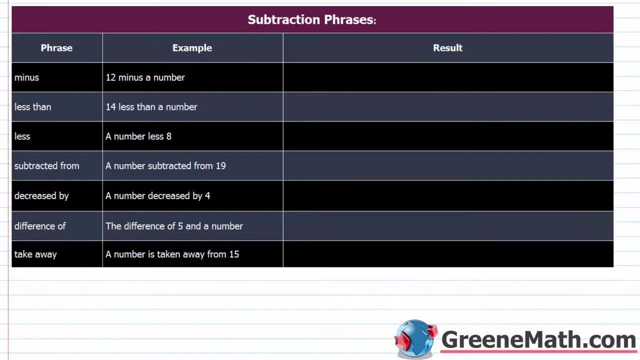 if negative 23 is added to 12,, the result is negative 11.. That is true, right? So our number here is negative 23.. Okay, this is what we're looking for. All right, let's look at some subtraction phrases. Again, you've got to pay close attention with subtraction, because it's 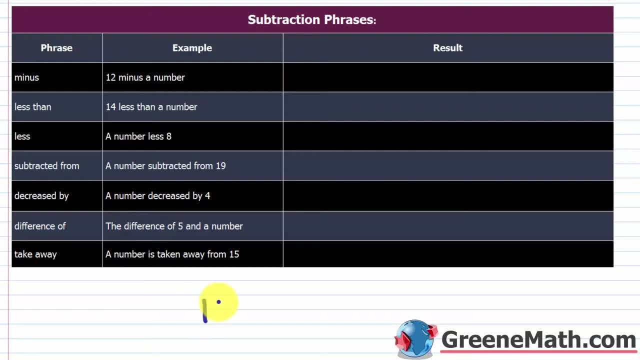 not commutative, Right? If I have something like 10 minus five, this is not equal to five minus 10.. I can't switch the order there like I can with addition, right? If I had 10 plus five, that is equal to five plus 10.. With addition I can change the order, with subtraction I cannot. 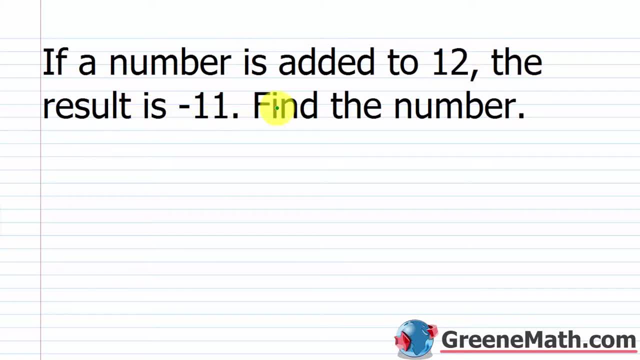 12,. the result is negative 11.. We want to find the number. So, again, if I see a number or I see the number, I'm just going to replace that with a variable and I'm going to use x And again. 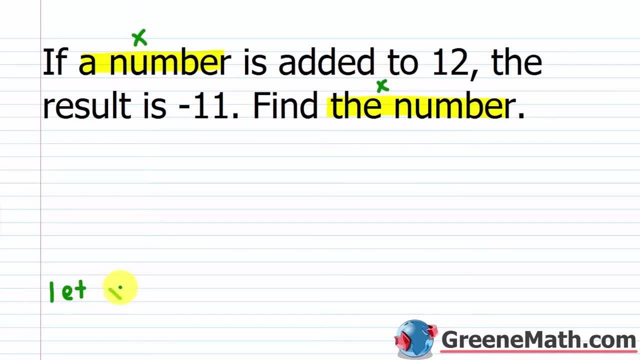 I can label this down here and just say that we're going to let x be equal to the unknown number. Okay, Just for clarity. And again, if x, so I'm going to read it like that. So if x is added to 12. So is added to just means plus. So x plus and then 12.. The result is: 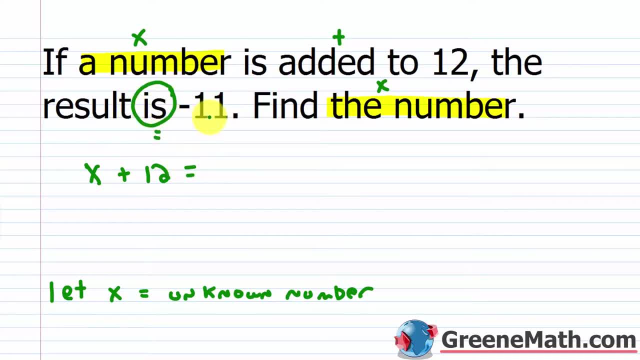 okay, in this context this means equals. Then we have negative 11.. Okay, So if x is added to 12, so x plus 12, the result is: or the result equals negative 11.. So that's how we got our equation. 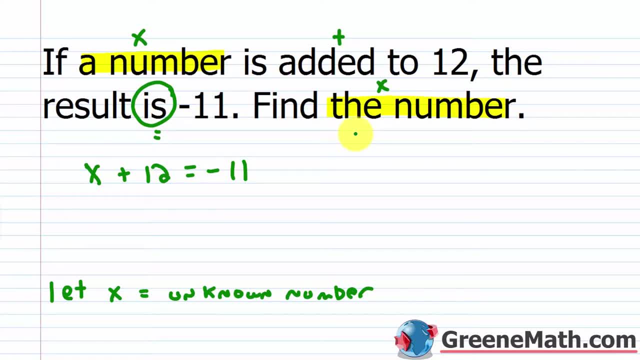 Then we want to find x or find the number. So again, I just want to solve this guy. Let me subtract 12 away from each side of the equation. I would have that x is equal to negative 23.. Right, And again reading back through the problem, if negative 23,. 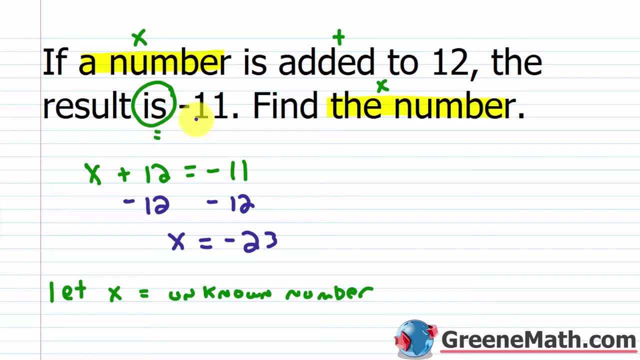 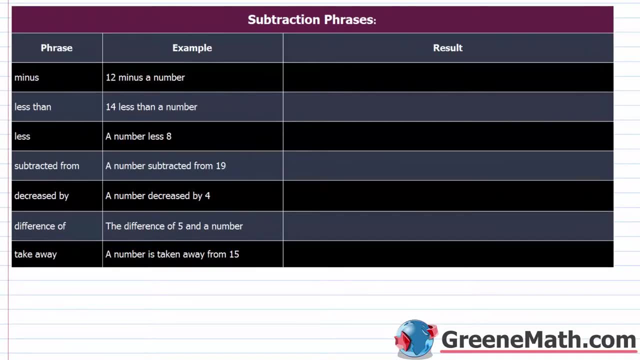 is added to 12,, the result is negative 11.. That is true, Right? So our number here is negative 23.. Okay, This is what we're looking for. All right, Let's look at some subtraction phrases. Again, you've got to pay close attention with subtraction, because it's not commutative. 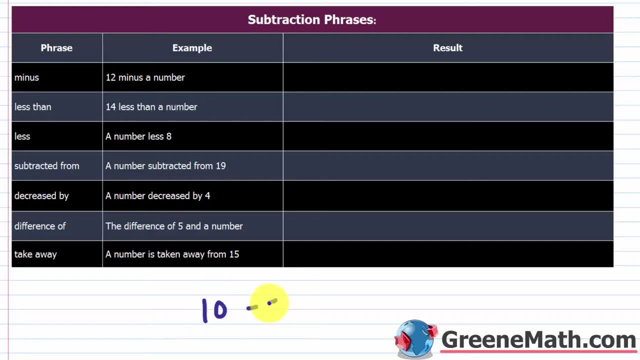 Right. If I have something like 10 minus 5, this is not equal to 5 minus 10.. I can't switch the order there like I can with addition. Right, If I had 10 plus 5, that is equal to 5 plus 10.. 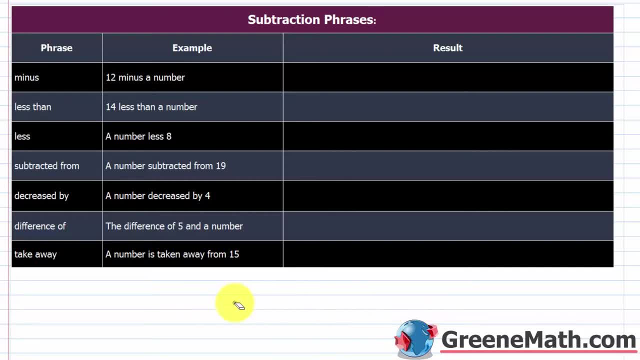 With addition I can change the order. With subtraction I cannot. Okay, So one of the phrases is minus. Okay, We all know minus means subtraction, Something like 12 minus a number. So I'm starting with 12 and I'm subtracting away a number. So again, every time I see a number, 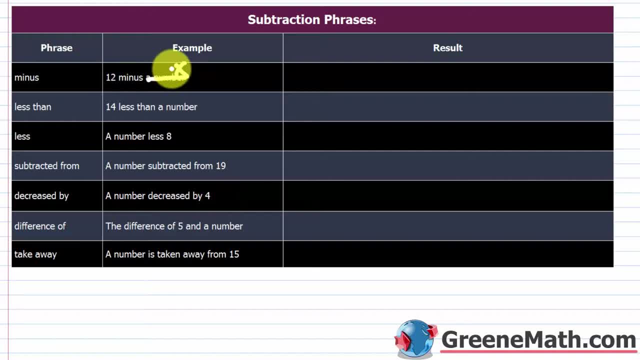 I can line that out and just put x. So 12 minus x is 12 minus x. Again, if you put x minus 12 there, it's not correct, Right? This would This would be wrong. This would be wrong. Okay, So you've got to make sure you go in the correct. 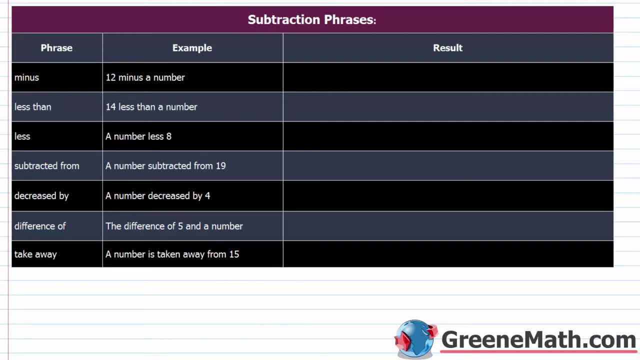 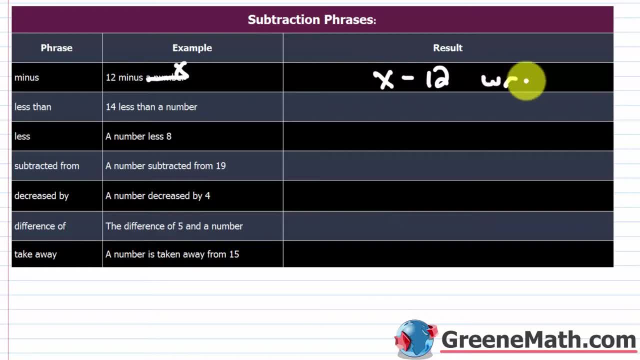 It's not correct, right? This would be wrong. This would be wrong. Okay, so you've got to make sure you go in the correct order- 12 is what I'm starting with- And then minus my variable x or my unknown number, then we have less than So 14, less than a number. Okay, let me line this out and put: 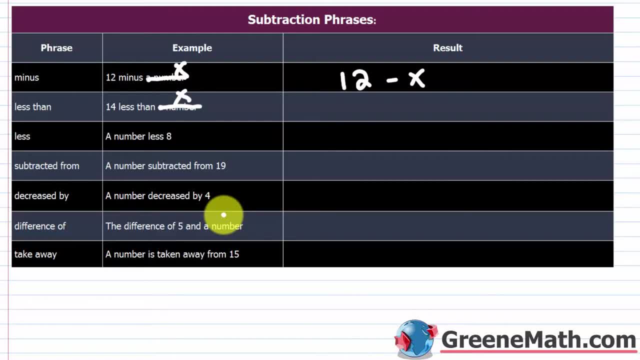 x here. So again, very important to interpret this correctly: We want 14 less than x. So that means we want 14 less than that. So I'm going to subtract away 14.. So this translates into x minus 14, not 14 minus x. Okay, Next, we have less, So a number less eight. Okay, Again, a number I'm. 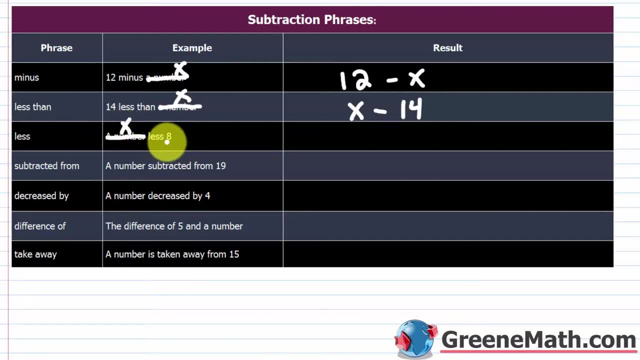 going to cross that out and put x, So x less eight. That means I'm starting with x And I'm taking away eight from that. Okay, Another one is subtracted from, So again a number subtracted from 19.. Let me line this out: and put x, So we have x subtracted from 19.. So pay attention there. 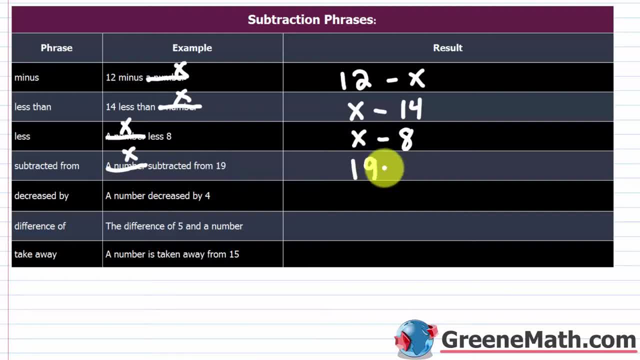 It's subtracted from 19.. So I'm starting with 19. And I'm subtracting away x. Okay, so this is 19 minus x. Then we have decreased by, So a number decreased by four. So let's line out a number. 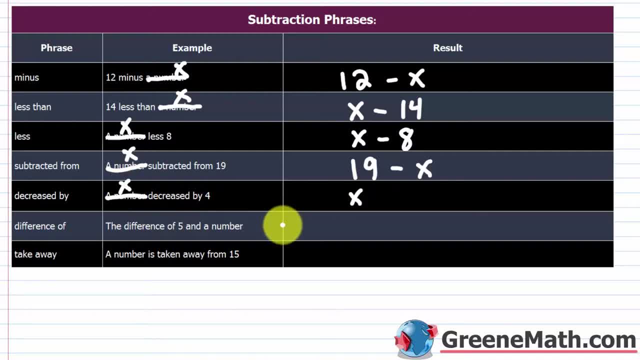 and put x. So if x is decreased by four it's just x minus four. Then we have difference of, So the difference of five and a number. So you've got to go in order here. Remember, when we talk about the difference, that's a result of subtraction, So the difference of five. 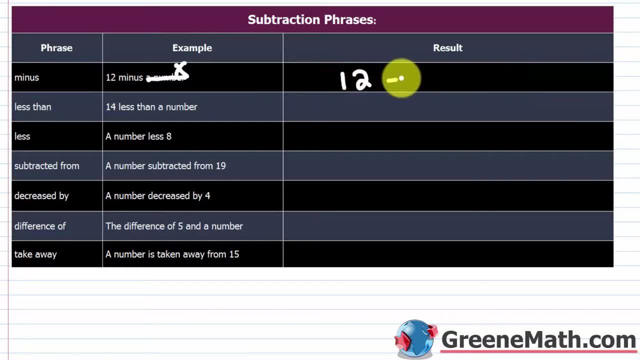 order. 12 is what I'm starting with, and then minus my variable x or my unknown number, Then we have less, than So 14 less than a number. Okay, Let me line this out and put x here. So again, very important to interpret this correctly- We want 14 less than x. So 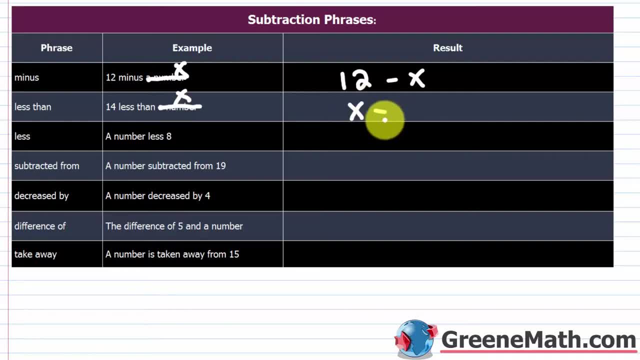 that means I'm starting with x and I want 14, less than that, So I'm going to subtract away 14.. So this translates into x minus 14, not 14 minus x. Okay, Next, we have less, So a number less 8.. Okay, Again, a number. I'm going to cross that out and 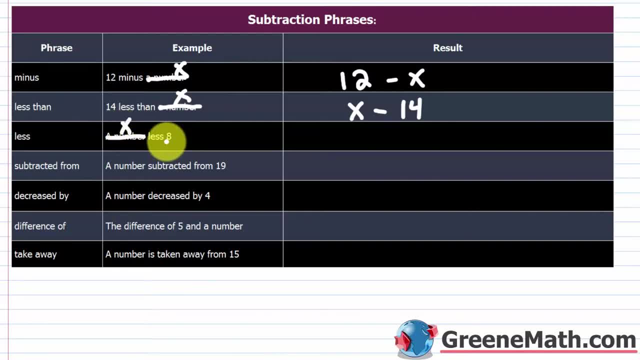 put x, So x less 8.. That means I'm starting with x and I'm taking away 8 from that. Okay, Another one is subtracted from, So again a number subtracted from 19.. So I'm starting with 19 and I'm subtracting away x. Okay, So this is 19 minus x. Then we 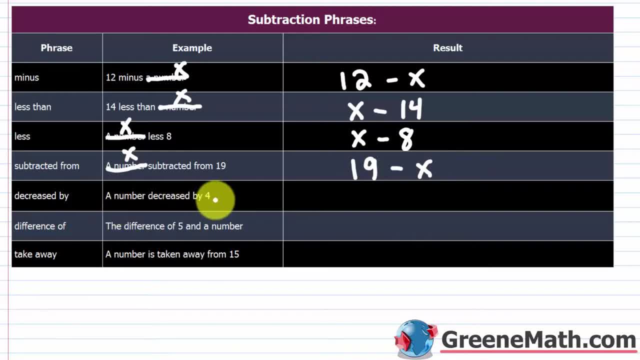 have decreased by So a number decreased by 4.. So let's line out a number and put x, So x is decreased by 4.. It's just x minus 4.. Then we have difference of, So the difference of. 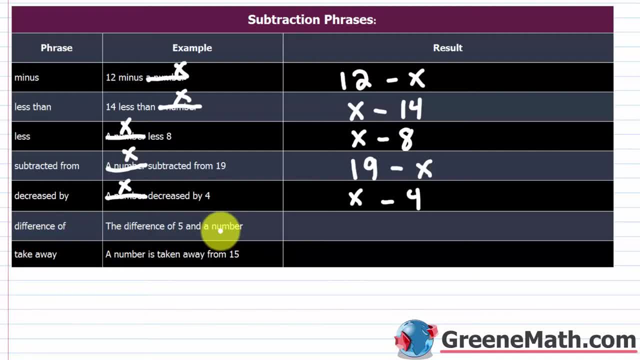 five and a number. so you've got to go in order here. remember, when we talk about the difference, that's a result of subtraction. so the difference of five- five is going to go first- and a number- let me line this out and put x. the difference of five and x would be five minus x. if it said: 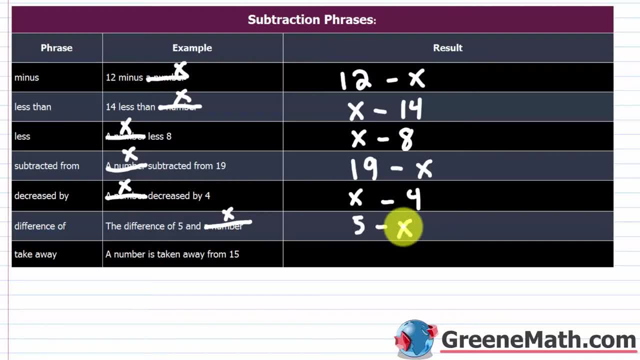 the difference of x and five, that would be x minus five. so you've got to go in order. then we have takeaway, so a number is taken away from 15. so again for a number, i'm just going to put x. so x is taken away from okay, it's taken away from 15. so 15 starts out, and then we take. 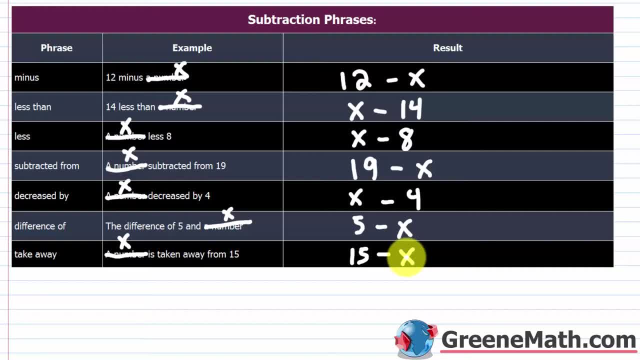 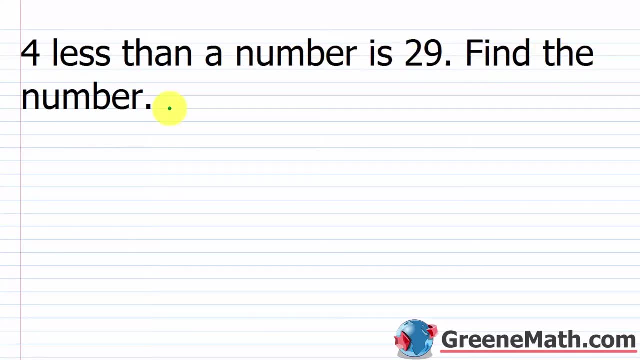 away our x. okay, so again with subtraction. the order matters, so you've got to correctly interpret these, otherwise you will not get the right answer. so let's look at some examples. all right, so we have that four letters less than a number is 29,. find the number. So again, wherever I see a number or the number, 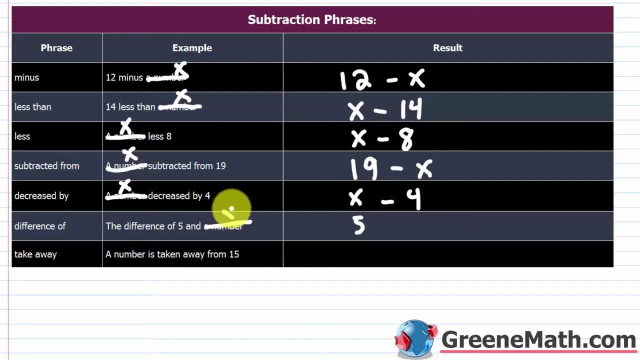 five is going to go first, And a number. let me line this out: and put x, The difference of five and x will be five minus x. If it said the difference of x and five, that would be x minus five. So you've got to go in order. Then we have takeaway. So a number. 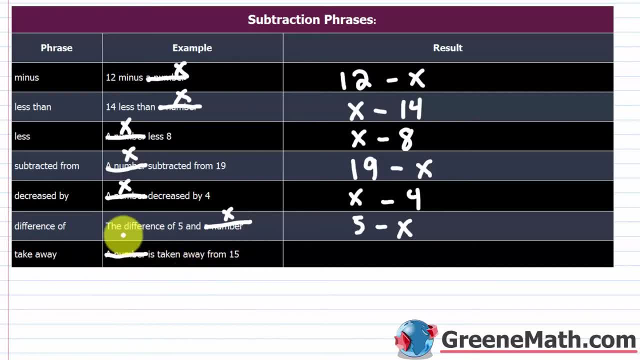 is taken away from 15.. So again, for a number, I'm just going to put x, So x is taken away from. okay, it's taken away from 15.. So 15 starts out, and then we take away our x. Okay, So again. 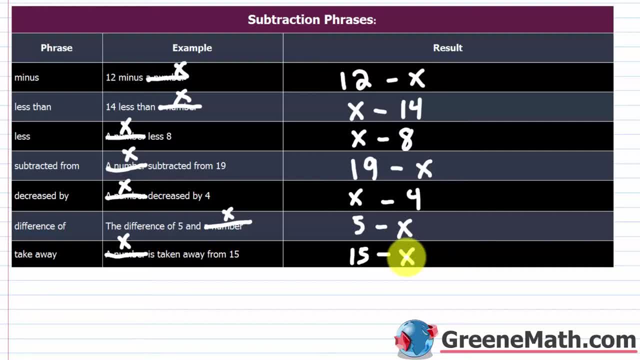 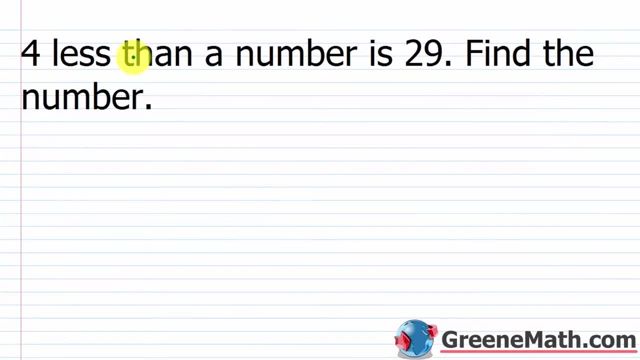 with subtraction. the order matters, So you've got to correctly interpret these, Otherwise you will not get the right answer. So let's look at some examples. All right, so we have that. four less than a number is 29.. Find the number. 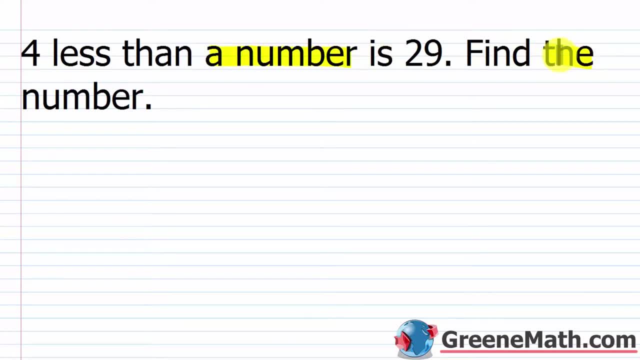 So, again, wherever I see a number or the number, I'm just going to replace that with a variable. Again, I'm going to use x And again, for the sake of completeness, I'm just going to say we're going to let x be equal to our unknown number. Okay, So four less than x, right, Think? 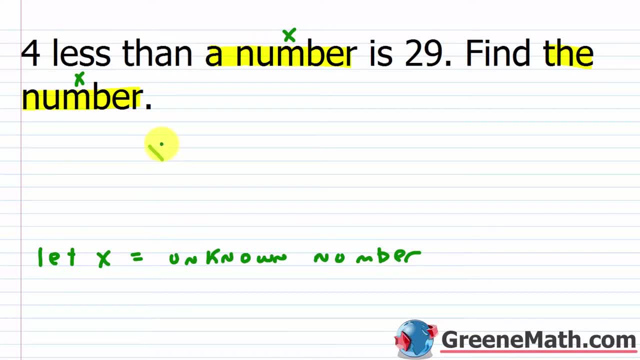 about that. That means I have x and I want four less than that, So x minus four. Then we have is, and this copy is going to be x minus four. So x minus four is going to be x minus four, So x minus. 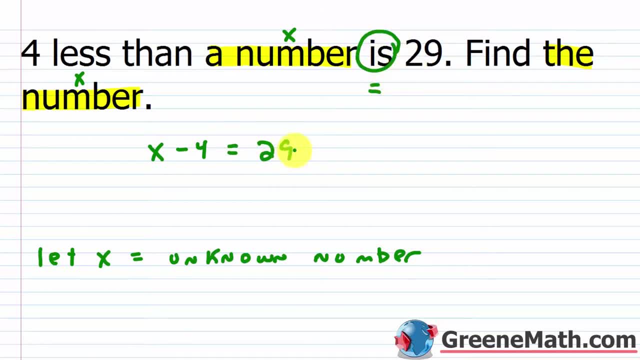 x is 23.. So 5 plus x minus x minus four is x minus four. So x minus x minus x, that's almost thirty-nine. Yeah, So x is write. so if, if x is a number less than x, then x squared down. We create a comma for that. 1. 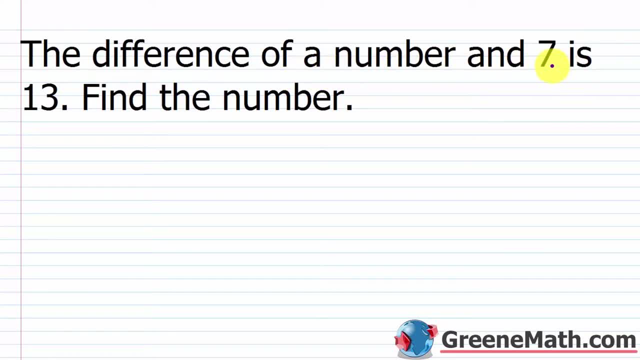 times two square root: one square root 12, 금. We can write it for a comma. Hey, I have a number less than x and I'm looking for a comm같. stayed between x and 23.. So if x is phonetictonics, in this case, instead of two over 30, is going to end wa. 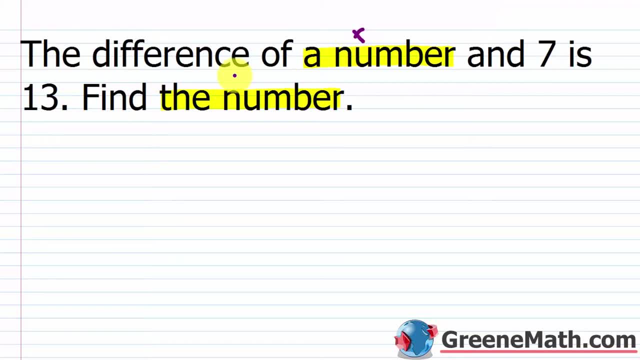 ed sec. So 4 less than x times three, and then 29.. variable. So we'll use x again And again. for completeness, I'm just going to say that we're going to let x be equal to our unknown number. Okay, so what can we say here? the difference of 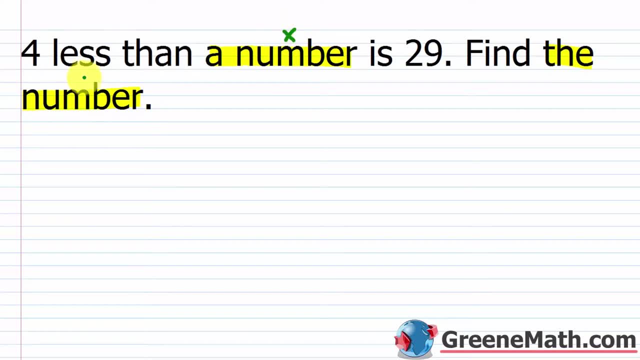 I'm just going to replace that with a variable. Again, I'm going to use x And again, for the sake of completeness, I'm just going to say we're going to let x be equal to our unknown number. Okay, so four less than x, right? Think about that. That means I have x and I want four less. 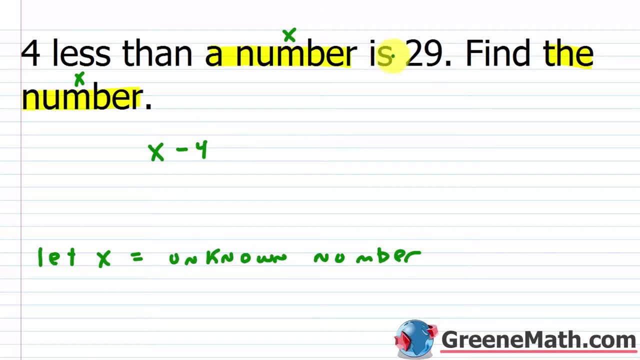 than that. So x minus four, then we have is- in this context that means equals, and then 29.. So to find the number, I would just add four to both sides of the equation. Now we get that x is equal to 33.. Right, So if I had four less than 33, that would be 29.. So the number is 33.. All right, 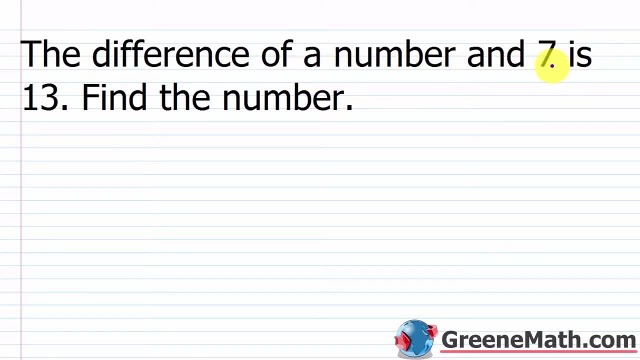 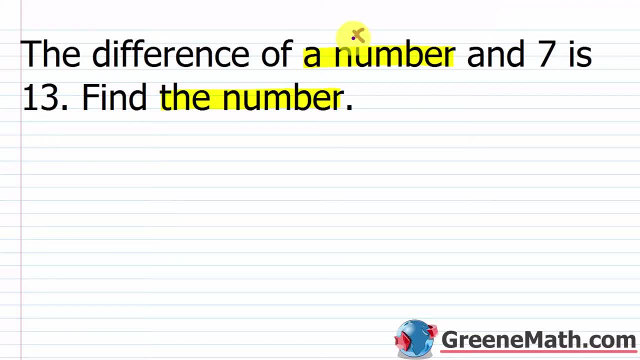 I'm just going to replace that with a variable, So we'll use x again And again. for completeness, I'm just going to say that we're going to let x be equal to our unknown number. Okay, so what can we say here? The difference of we have x and seven, So the difference of x and 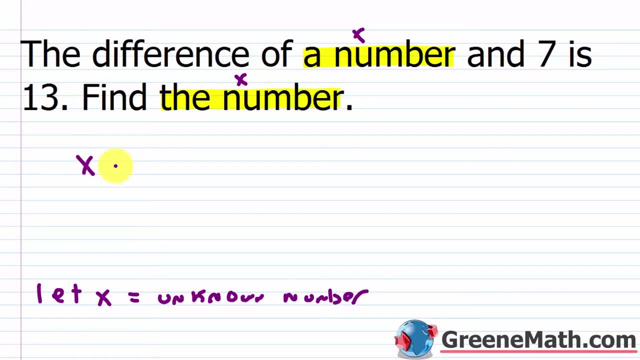 seven. x comes first. So we'd have x, And then we have minus. we've got our seven, And then we've got our is okay, this means equal to x. And then we have minus. we've got our seven, And then we've 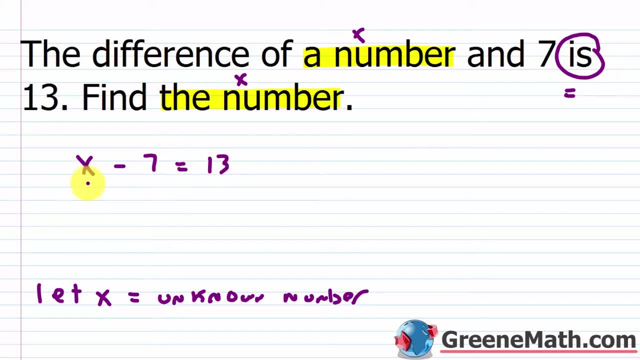 equals and then we have 13.. So essentially we have x minus 7 equals 13.. To solve this for x, we add 7 to both sides of the equation. We get x is equal to 20.. So the difference of 20 and 7. 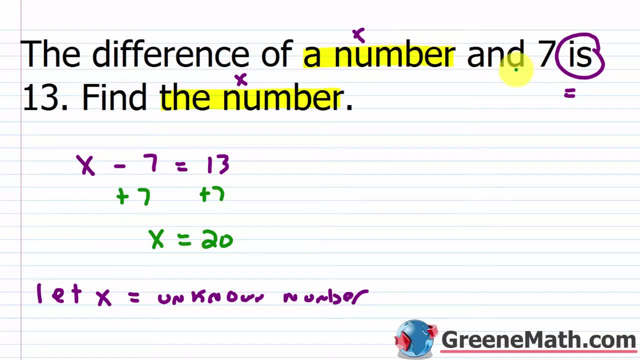 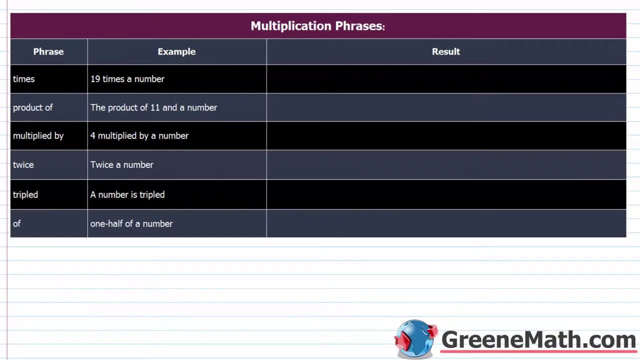 is going to be 13.. That's correct, right? 20 minus 7 is 13.. So we can say our unknown number here is 20.. All right, let's take a look at some multiplication phrases. So we have times. 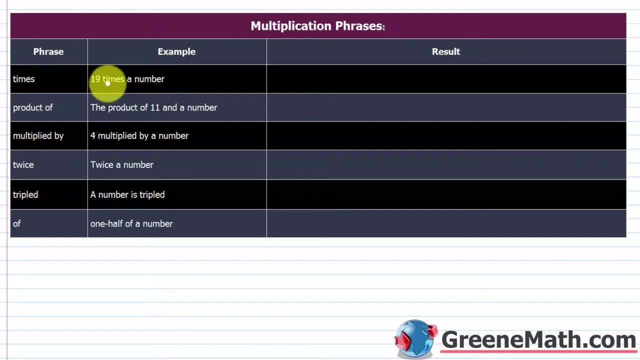 We all know that times means multiplication, So 19 times a number. Again, I can mark out a number and put x 19 times x is just 19x. or you can put 19 times x, like this. whatever you want to do, 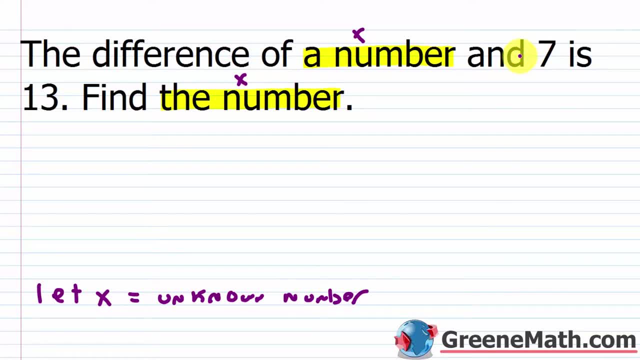 we have x and seven, So the difference of x and seven, x comes first, So we'd have x, And then we have minus. we've got our seven And then we've got our is okay, this means equals. and then we. 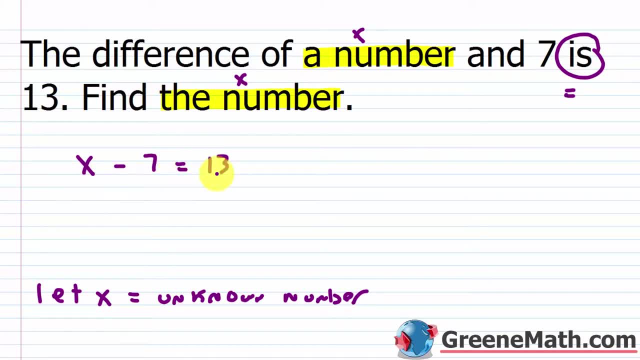 have 13.. So essentially we have x minus seven equals 13.. To solve this for x, we add seven to both sides of the equation. we get x is equal to 20.. So the difference of 20 and seven is going to. 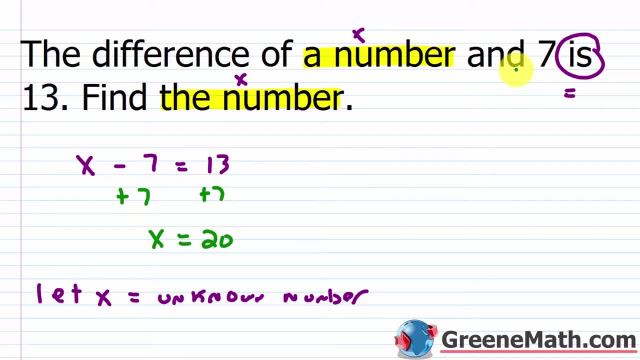 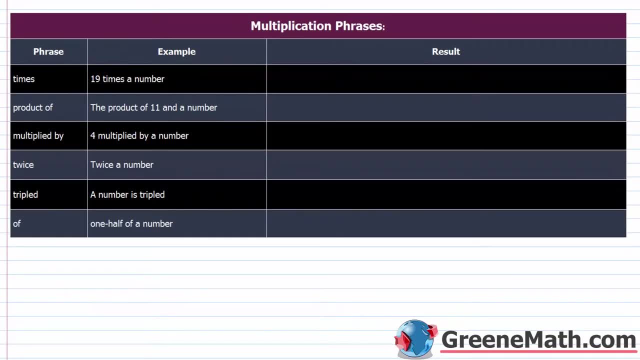 be 13.. That's correct, right. 20 minus seven is 13.. So we can say our unknown number here is 20.. All right, let's take a look at some multiplication phrases. So we have times. we all know that times means multiplication. So 19 times a number. 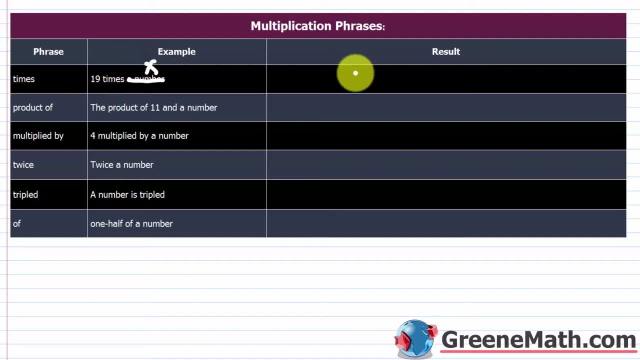 again, I can mark out a number and put x 19 times x is just 19x. where you put 19 times x like this, whatever you want to do, then the product of- we know the product is a result of multiplying two. 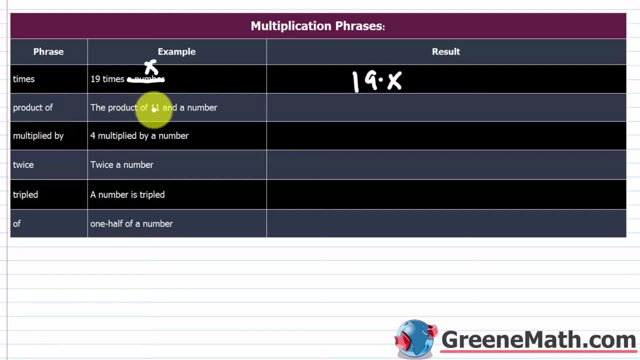 or more numbers together. So the product of 11 and a number. So again we can mark out a number and put x. So the product of 11 and x is again just 11 times x. then multiplied by four, multiplied by x is four times x, And then twice. we know that's like doubling something or multiplying by. 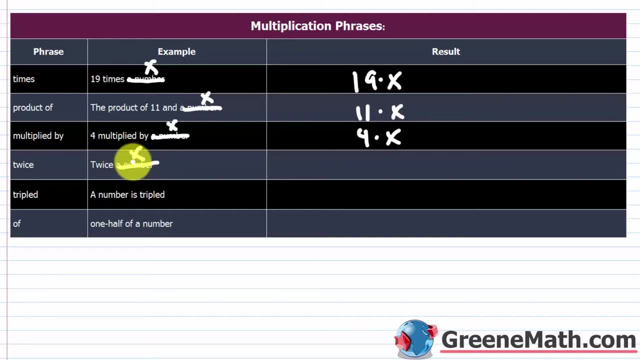 two, So twice a number. So if we put twice x, that's just two times x Tripled, a number is tripled. we know, if we multiply by three we're tripling something, So we can mark out a number. 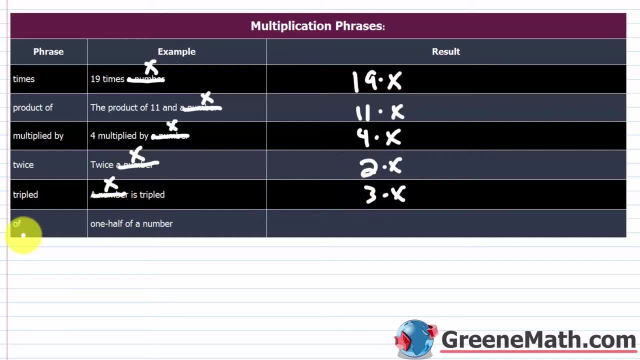 and put x. x is tripled, that's three times x. And then of here we have one half of a number. So again, mark out a number and put x. Generally you're going to use of when you're working with fractions, you want a fractional. 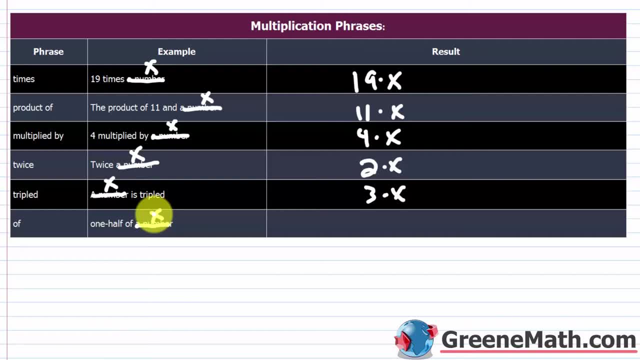 amount of something. So I want three fourths of something, five sixths of something or, in this case, one half of something. So one half of x is one half times x. Now again, with multiplication it's commutative right. The order that I multiply in does not affect my result. So let's look at: 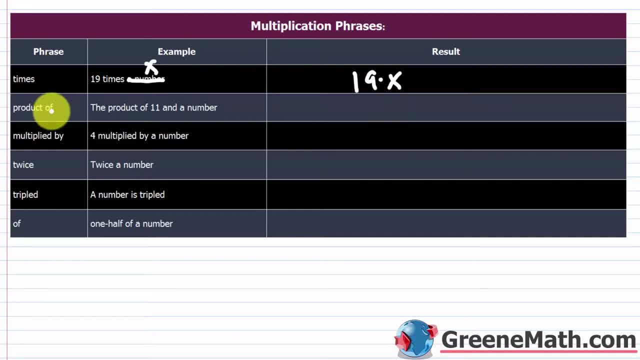 Then the product of. We know the product is a result of multiplying two or more numbers together, So the product of 11 and a number. So again we can mark out a number and put x. So the product of 11 and x is again. 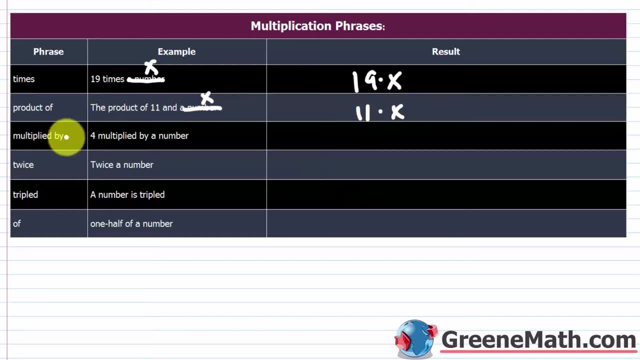 just 11 times x, then multiplied by 4, multiplied by a number. mark out a number and put x, 4 multiplied by x is 4 times x, and then twice. we know that's like doubling something or multiplying by 2, so twice a number. so if we put twice x, that's just 2 times x. tripled, a number is tripled. we. 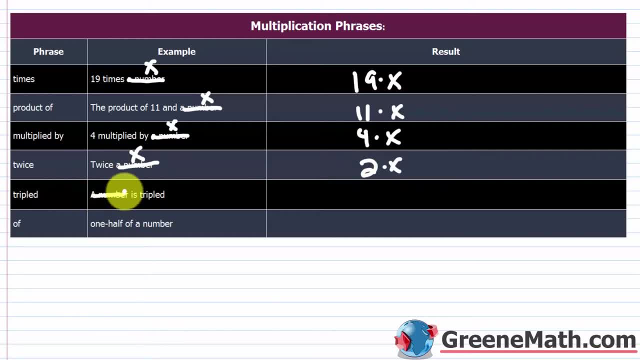 know, if we multiply by 3, we're tripling something. so we can mark out a number and put x. x is tripled, that's 3 times x. and then of here we have one half of a number. so you can mark out a number and put x generally you're going to use of when you're working with fractions. you want a fractional. 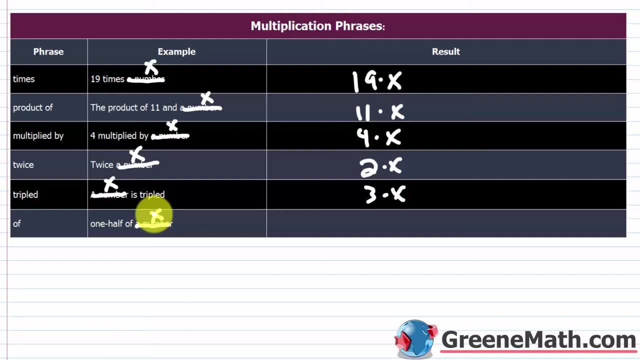 amount of something. so i want three-fourths of something, five-sixths of something or in this case, one-half of something. so one-half of x is one-half times x. now again, with multiplication it's commutative right. the order that i multiply in does not affect my result. 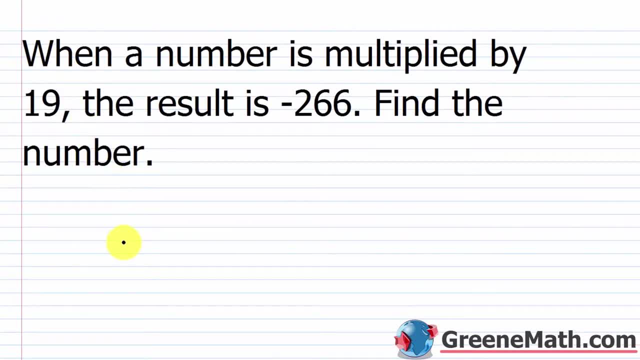 So let's look at some examples. So when a number is multiplied by 19,, the result is negative: 266.. Find the number. So, again, when a number- and here we have the number- I'm going to replace that with x. So let's put an x here. 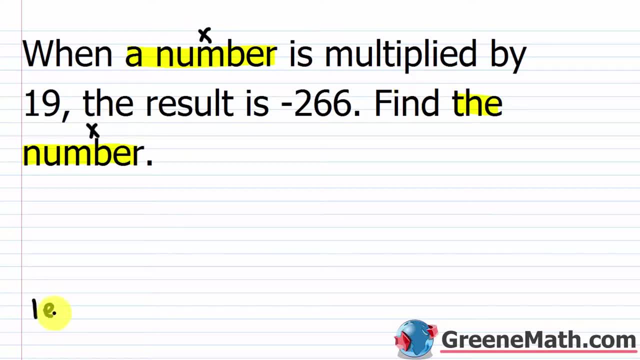 and let's put an x here And again for completeness, I'm just going to say: let x be equal to my unknown again, my unknown number. Okay, so when x is multiplied by 19,. so that's just 19x. 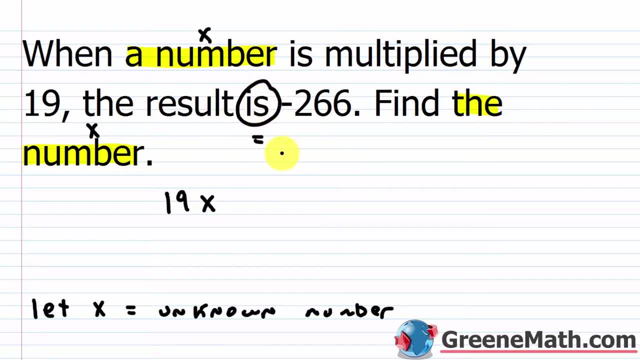 the result is again- this guy right here is just going to be- equals negative 266.. So this tells me I have 19x, that's equal to negative 266.. I can solve this very easily. I can divide both sides by 19, and I'm going to get. 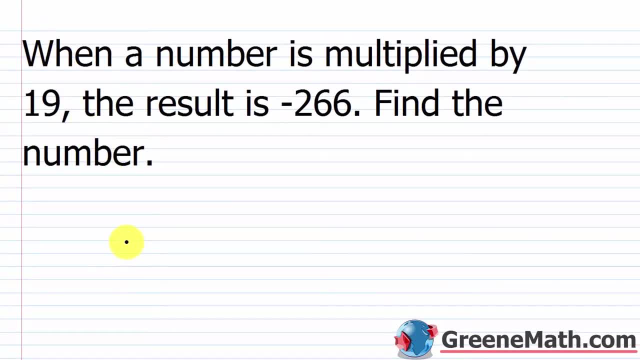 some examples. So when a number is multiplied by 19, the result is negative 266.. Find the number. So again, when a number- and here we have the number- I'm going to replace that with x. So let's put an x here, and let's put an x here And again. for completeness, I'm just going to say: 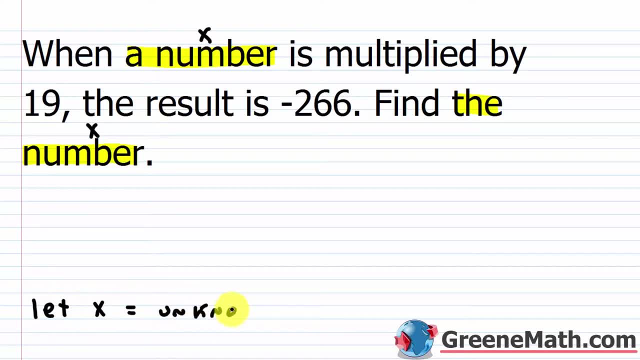 let x be equal to my unknown- again my unknown number. Okay, So when x is multiplied by 19,, so that's just 19x, the result is again this guy right here is just going to be- equals negative- 266. 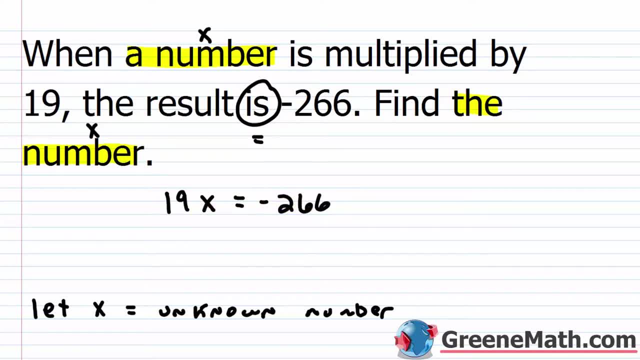 So this tells me I have 19x. that's equal to negative 266.. I can solve this very easily. I can divide both sides by 19.. And I'm going to get that x is equal to negative 14.. So again find the number. It's going to be negative 14, because when negative 14 is multiplied, 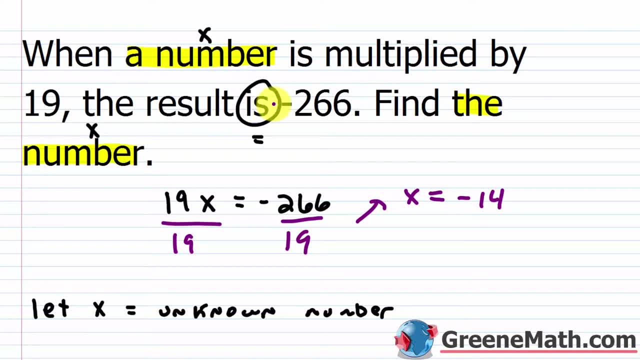 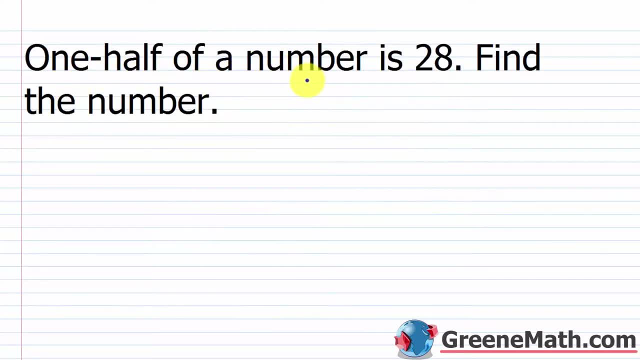 by 19,. the result is negative 266.. That's true. So negative 14 is my unknown number here. All right, Now we're saying that one half of a number is 28.. Find the number. So again a number and the number. I'm just going to replace that with. 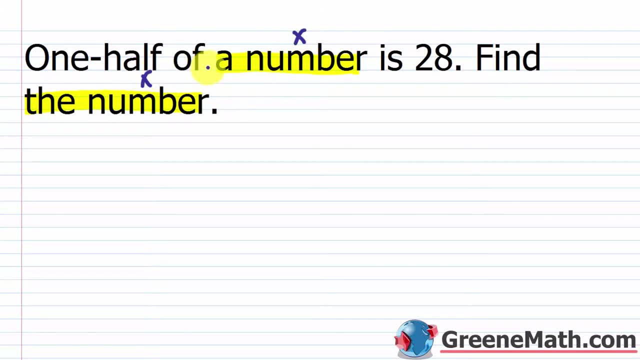 a variable like x. So one half of x would just be one half x. And then we're saying, is okay, this is going to be equals. And then we have 28.. So find the number. All I've got to do is solve. 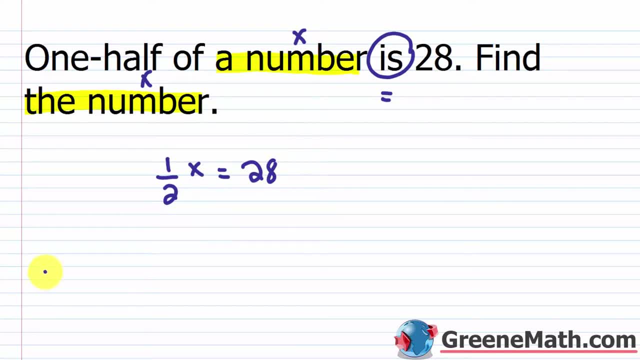 this equation, But let me write this right here and say that we're going to again let x be equal to our unknown number. Again, this is just for the sake of completeness. So let's put an x here and this, And to multiply both sides by 2 here would give me a solution for my equation. I can multiply. 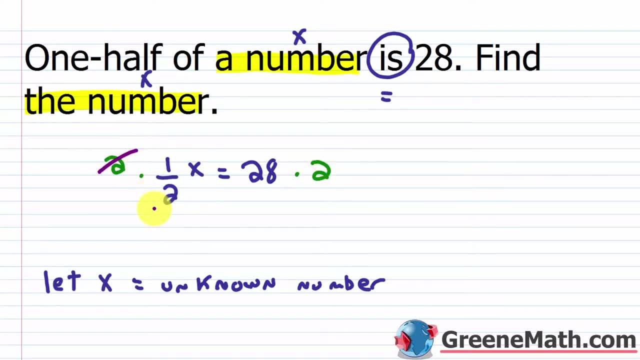 this side by 2 and this side by 2.. This guy here would cancel I'd have. x is equal to 28 times 2 is going to be 56. So that's my unknown number right. One half of 56 is 28.. That's correct. 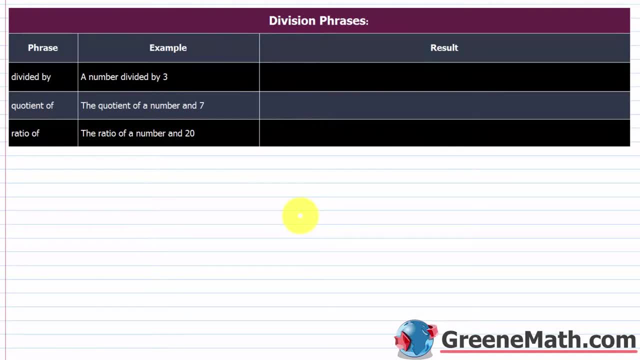 All right. So we also have some division phrases. We want to remember that division is not commutative. The order that we divide in is going to change the result, right? So something like divided by: and then we have a number divided by 3. So again, I'm just going to line out a number and put x. 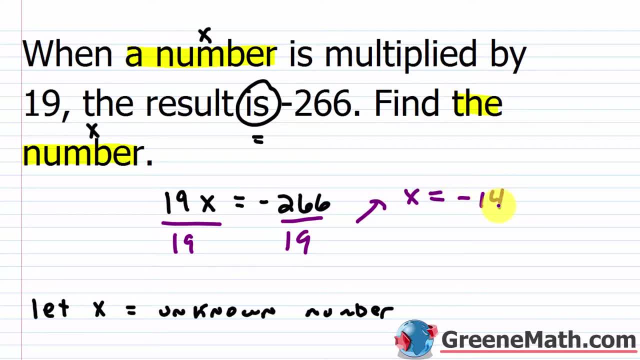 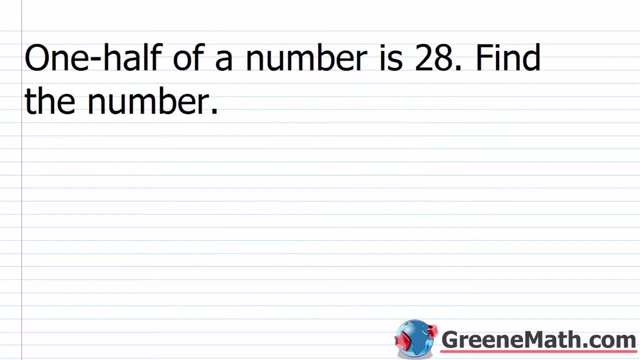 that x is equal to negative 14.. So again, find the number. It's going to be negative 14, because when negative 14 is multiplied by 19, the result is negative 266.. That's true. So negative 14 is my unknown number here. Alright, now we're saying that. 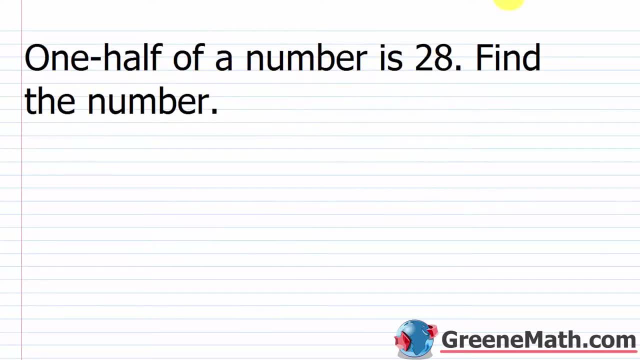 one half of a number is 28.. Find the number. So again a number and the number. I'm just going to replace that with a variable like x. So one half of x would just be one half x. And then we're saying: is okay, this is going to be. 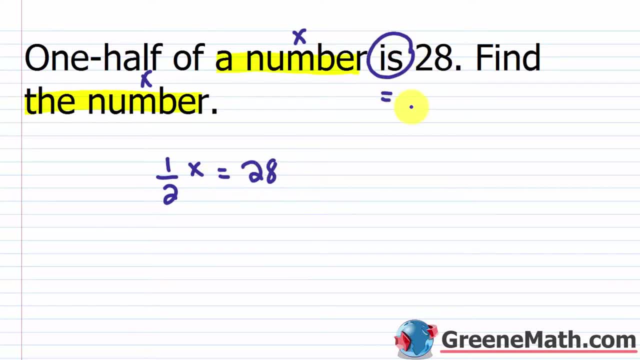 equals, And then we have 28.. So find the number. All I've got to do is solve this equation, But let me write this right here and say that we're going to again: let x be equal to our unknown number. 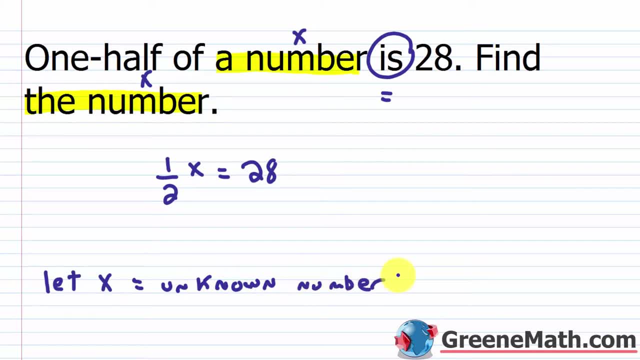 Again, this is just for the sake of completeness, And to multiply both sides by 2 here would give me a solution for my equation. I can multiply this side by 2 and this side by 2.. This guy here would cancel. I'd have x is equal to. 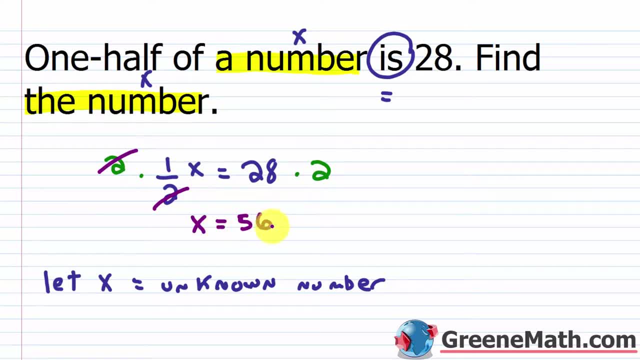 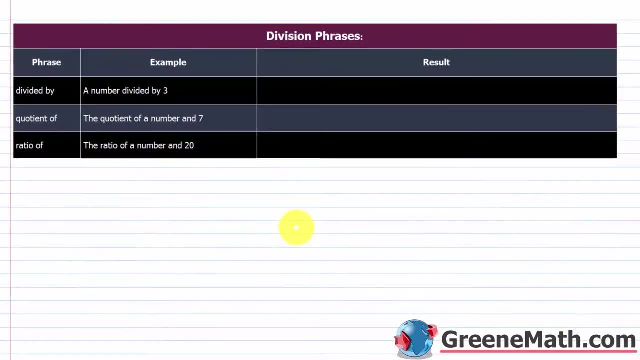 28 times 2 is going to be 56. So that's my unknown number. Alright, one half of 56. Is 28.. That's correct, Alright. so we also have some division phrases. We want to remember that division. 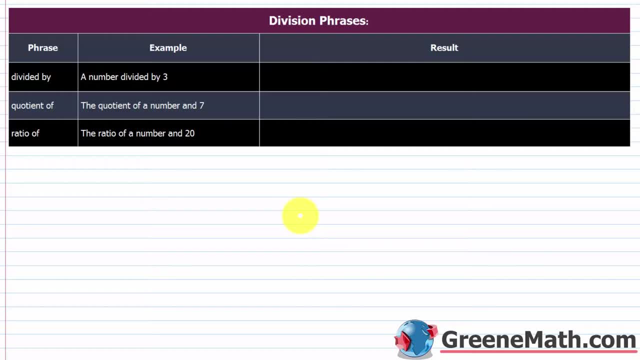 is not commutative, So the order that we divide in is going to change the result. So something like divided by, and then we have a number divided by 3.. So again, I'm just going to line out a number and put x. 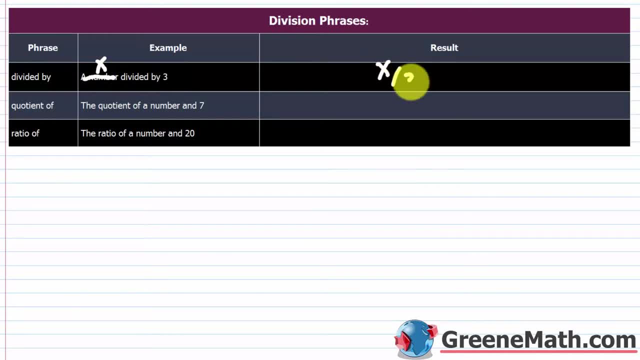 If that's divided by 3, we would have x over 3.. x divided by 3.. So essentially, x goes in the numerator- It's your dividend- And 3 goes in the denominator- It's your divisor. So x divided by 3 would be x over 3.. 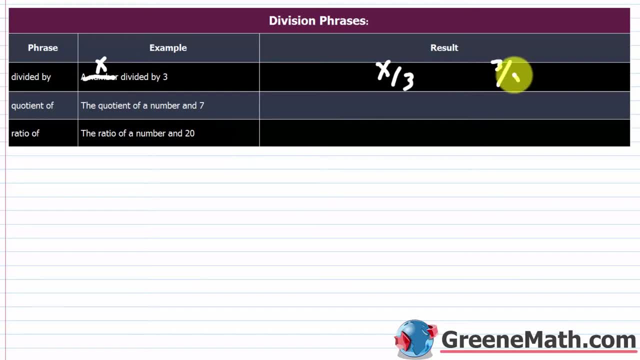 It would be wrong if you put 3 over x, If I put 3 over x, that would be incorrect. So again, the order matters here. Then we have quotient of, So the quotient of a number, and 7.. I'm just going to line out this part that says a number and put x, So the 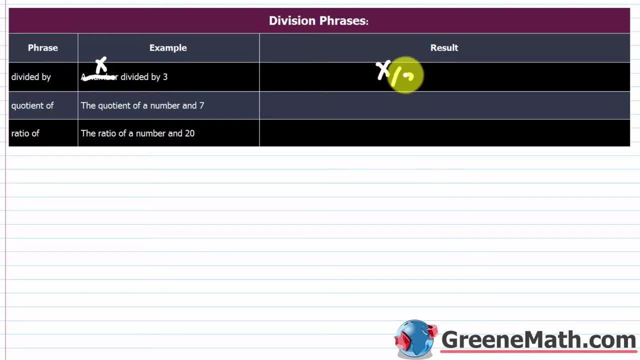 If that's divided by 3, we would have x over 3, right x divided by 3.. So essentially, x goes in the numerator, It's your dividend, And 3 goes in the denominator, It's your divisor right. So x. 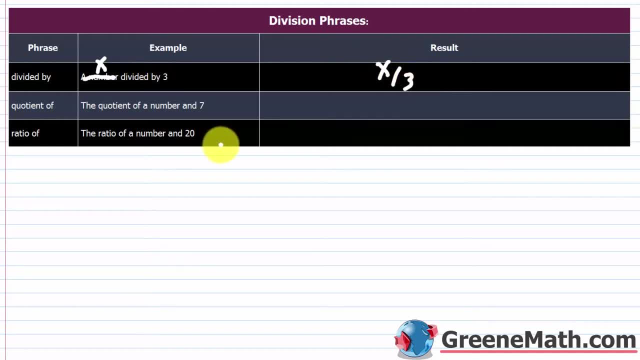 divided by 3 would be x over 3.. It would be wrong if you put 3 over x, right? If I put 3 over x, that would be incorrect. So if I put 3 over x, that would be incorrect. So if I put 3 over x. 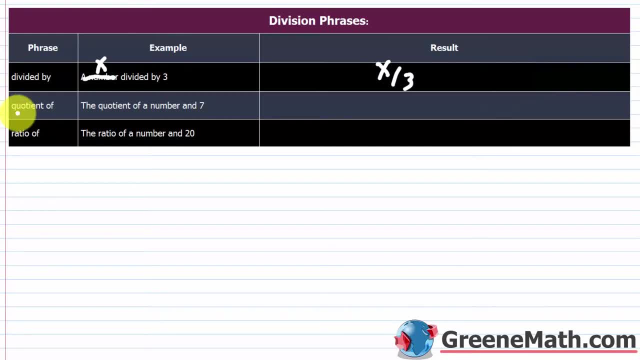 that would be incorrect. So again, the order matters here. Then we have quotient of, So the quotient of a number, and 7, it's going to line out this part that says a number and put x, So the quotient of x and 7 would be x over 7, okay. Then we have ratio of, the ratio of a number. 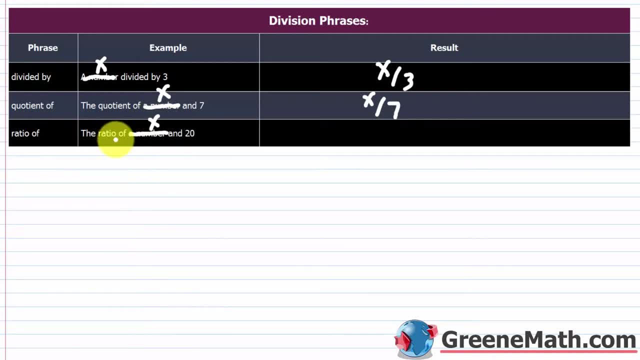 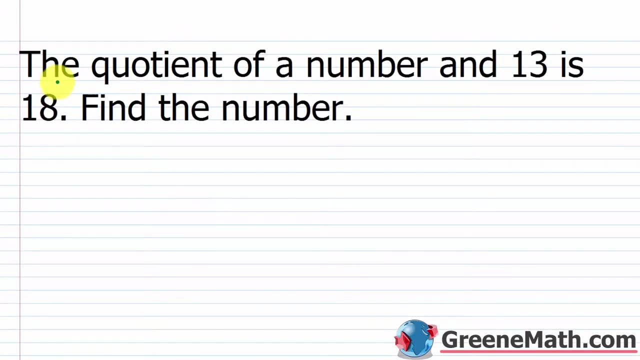 and 20.. Again, just going to line out a number and put x, So the ratio of x and 20 would just be x over 20.. All right, So let's look at a few problems with division. So we have the quotient of a number. 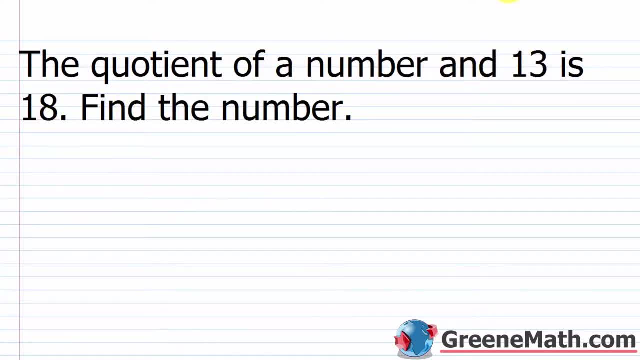 and 13 is 18.. Find the number. So again, wherever I see a number or the number, I'm just going to replace this with our variable x. And again, for completeness, I'm just going to say down here: we want to let x be equal to our unknown number. So the quotient of x and 13,, that's just x over. 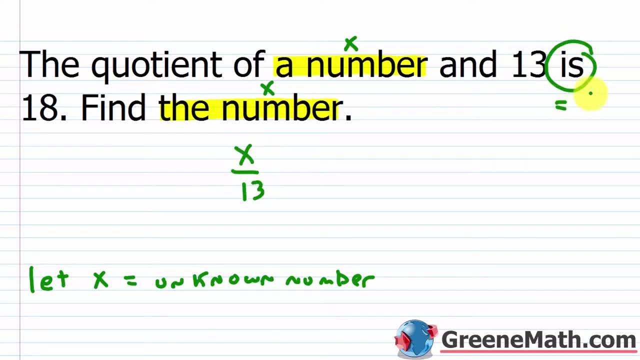 13. Then we have is right- In this context it means equals- Then we have 18.. So to find the number, let's just solve the equation. We'll multiply both sides by 13, and we'll get what. 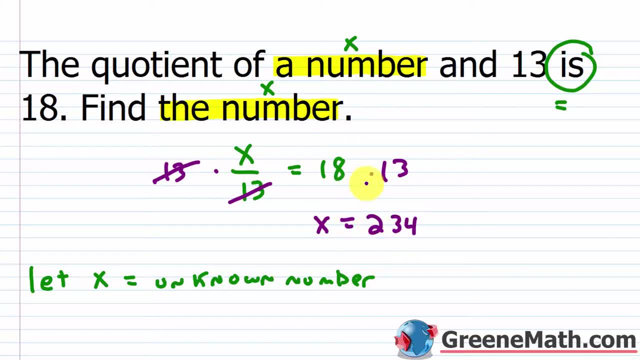 This cancels, We'll get. x is equal to 234, right, 18 times 13 is 234.. So when we say find the number, the number is going to be 234, because the quotient of 234 and 13 is 18.. Right, Now we have a number. 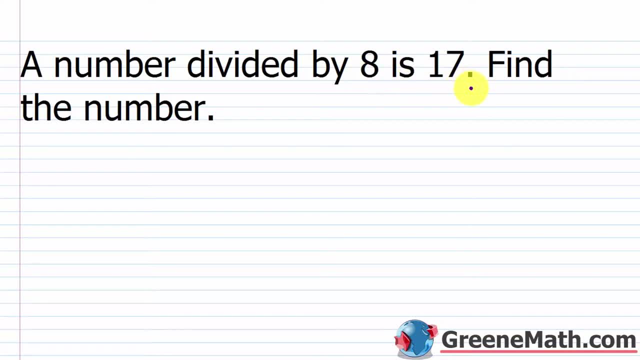 divided by 8 is 17.. Find the number. So again for a number or for the number, I'm just going to put x. So x divided by 8.. So x divided by 8 is again: this means equals. So we have equals. 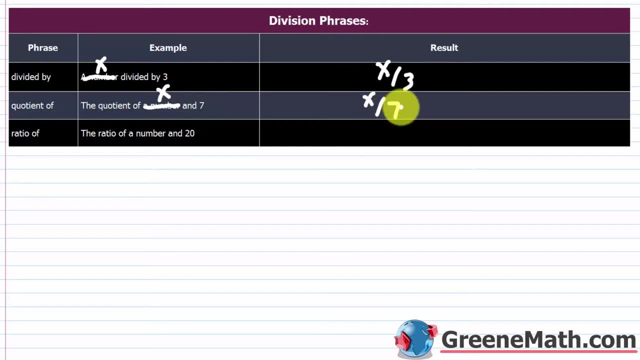 quotient of x and 7 would be x over 7.. Then we have ratio of The ratio of a number and 20.. Again, just going to line out a number and put x. So the ratio of x and 20 would just be x over 20.. 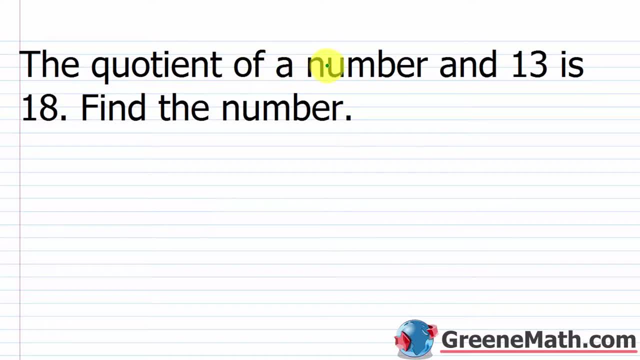 Alright, so let's look at a few problems with division. So we have the quotient of a number and 13 is 18.. Find the number. So, again, wherever I see a number or the number, I'm just going to replace this with our variable. 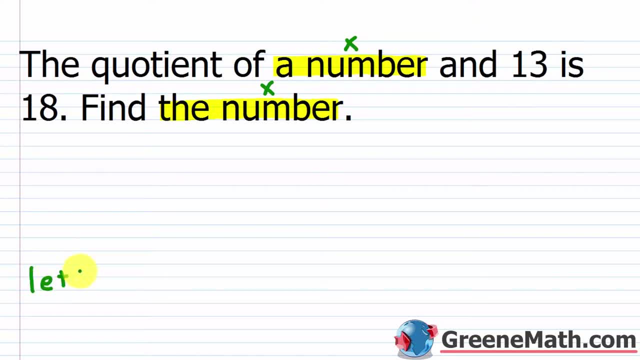 x. And again, for completeness, I'm just going to say down here: we want to let x be equal to our unknown number, So the quotient of x and 13. That's just x over 13. Then we have is. In this context, it means: 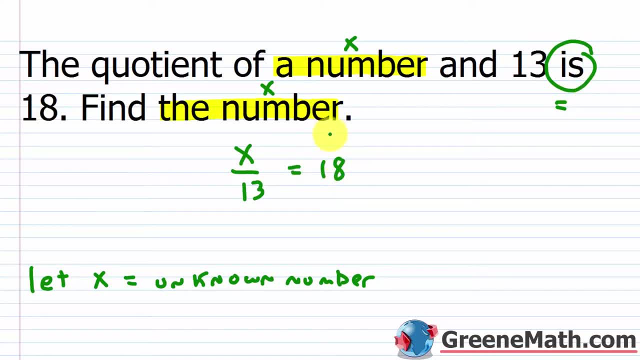 equals, Then we have 18.. So to find the number, let's just solve the equation. We'll multiply both sides by 13 and we'll get what This cancels. We'll get. x is equal to 234.. 18 times 13 is 234.. So when we say find 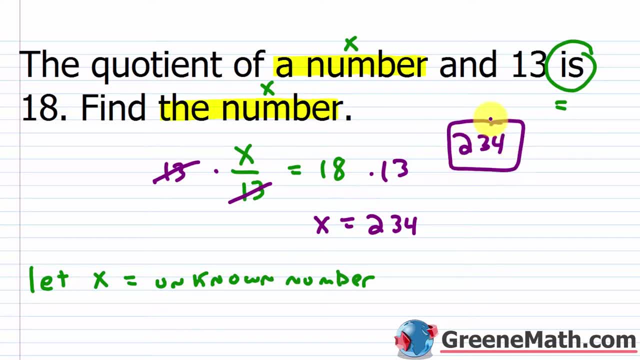 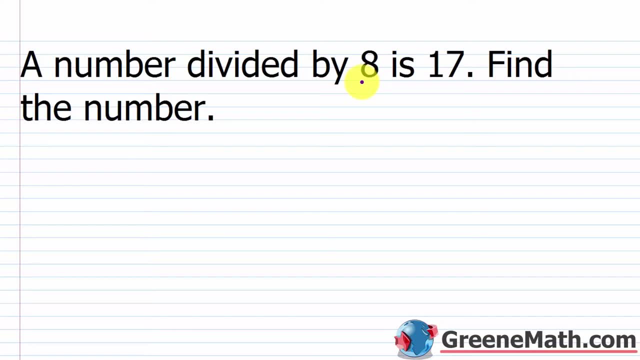 the number. the number is going to be 234, because the quotient of 234 and 13 is 18.. Alright, now we have a number divided by 8 is 17.. Find the number. So, again for a number or for the number, I'm just going to put my variable x. 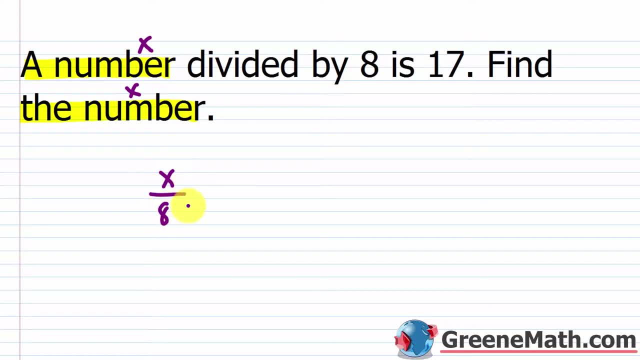 So x divided by 8.. So x divided by 8 is again: this means equals. So we have equals, Then we have 17.. Again, find the number. or find x. Let me write down here that we're going to let x be. 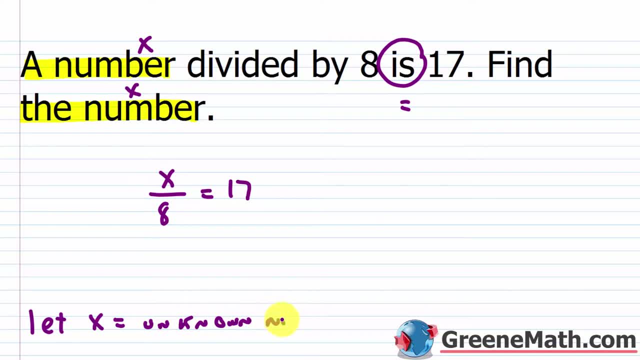 equal to our unknown number. Again, just for completeness And so to solve the equation here, I'm just going to multiply both sides by 8.. 17 times 8 is 136. So these guys cancel. You get x equals 136.. So that's going to be my. 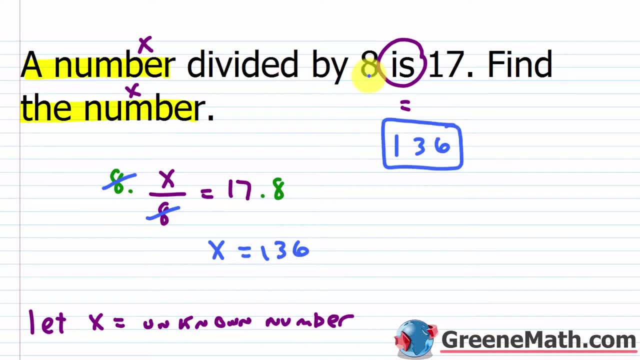 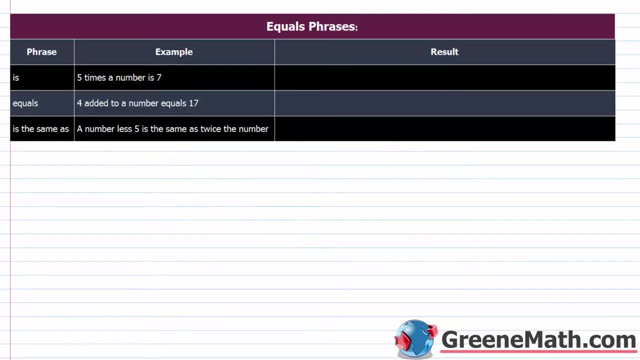 unknown number. Again, if 136 is divided by 8, the result is 17.. So 136 again is the number For all the problems we looked at. we used is for equals, but there's other things you can see, So it's basically any. 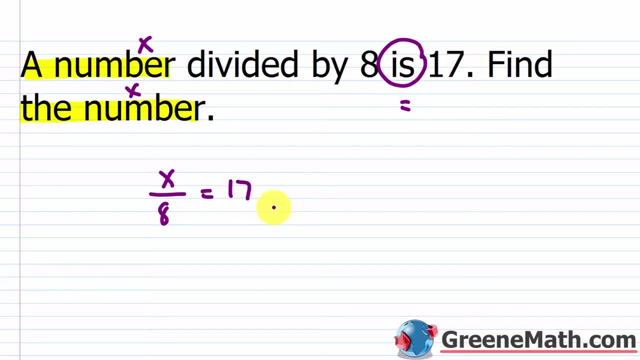 and then we have 17.. Again, find the number. or find x. Let me write down here that we're going to let x be equal to our unknown number. Again, just for completeness, And so to solve the equation here, I'm just going to multiply both sides by 8.. 17 times 8 is 136.. So these guys cancel. 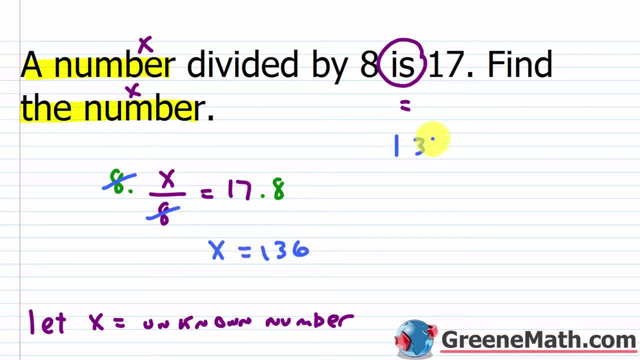 You get: x equals 136. So that's going to be my unknown number. Again, if 136 is divided by 8, the result is 17.. So 136, again, is the number For all the problems we looked at. we used is: 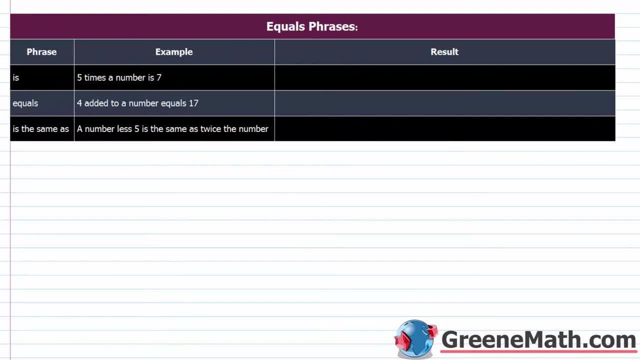 for equals. but there's other things you can see, So it's basically any phrase that implies sameness. So some examples would be: again we use is. So 5 times a number is 7.. So again, if you line this out and you put x here, 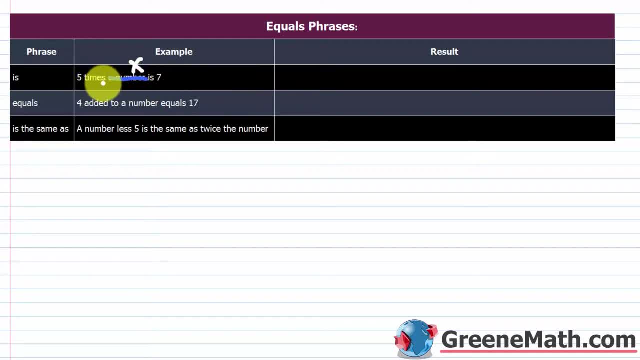 5 times x is okay, that is means equals. So 5 times x is or equals 7.. Then here we just have the word equals, So 4 added to a number equals 17.. So that's pretty straightforward. Line out your unknown number and put x, 4 added to x, which is x plus 4,. 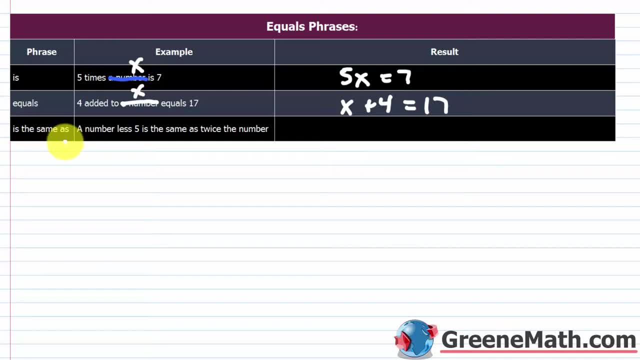 equals 17.. Then we have: is the same as. So a number less 5 is the same as twice the number. So let's line this part out here and put x. Let's line out this part here and put x. So x less 5, that's x minus 5, is the same as Okay. 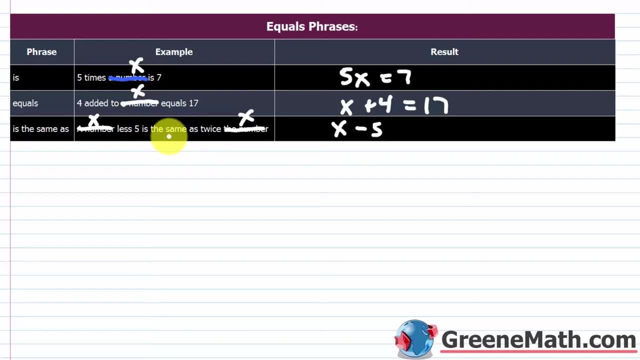 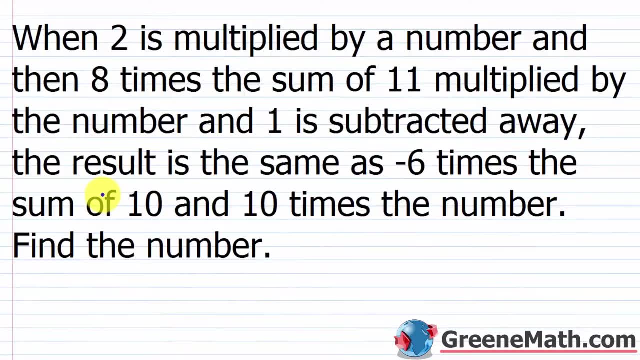 that's basically us saying equals- right, It's implying sameness, So is the same as is equals. And then we have twice x, So 2 times x. All right, let's go ahead and take a look at two examples that kind of tie everything together And in the next lesson we'll start looking at. 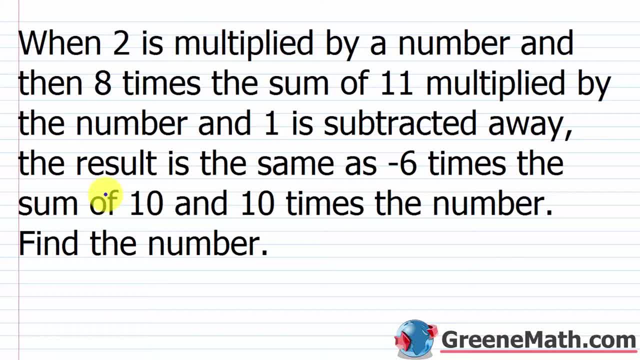 some common application problems again that deal with linear equations in one variable. So when 2 is multiplied by a number, and then 8 times the sum of 11 multiplied by the number and 1 is subtracted away, the result is the same as negative 6 times the sum of 10 and 10. 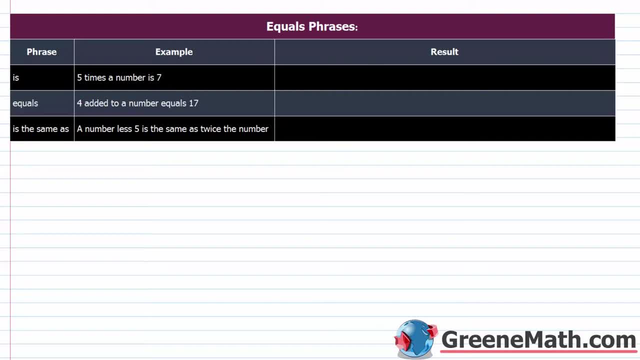 phrase that implies sameness. Okay. so some examples would be. again we use is: So 5 times a number is 7.. So again, if you line this out and you put x here 5 times x is okay. that is means equals. So 5 times x. 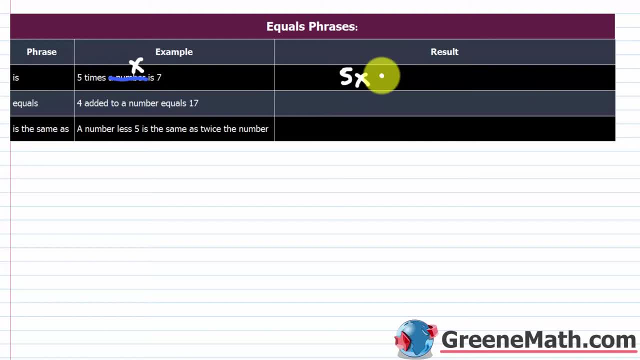 is or equals 7.. Then here we just have the word equals. So 4 added to unknown number equals 17.. So that's pretty straightforward. Line out your unknown number and put x, 4 added to x, which is x plus 4, equals 17.. Then we have: is the 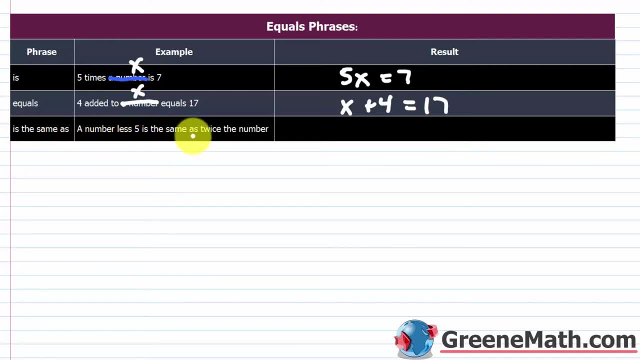 same as. So a number less 5 is the same as twice the number. So let's line this part out here and put x. Let's line out this part here and put x. So x less 5, that's x minus 5, is the same as: Okay, that's basically us. 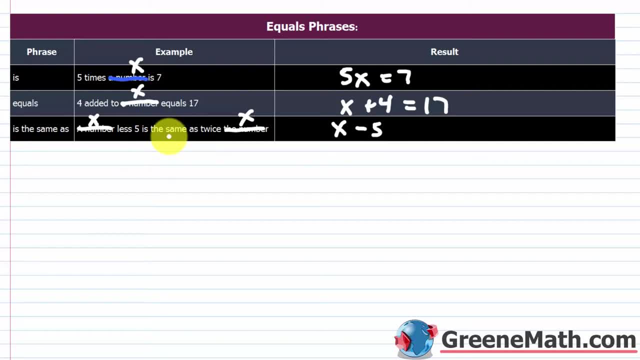 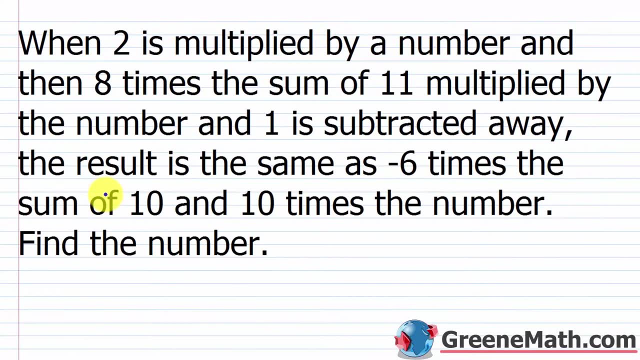 saying equals, right, It's implying sameness, So is the same as is equals. And then we have twice x, So 2 times x. Well, let's go ahead and take a look at two examples that kind of tie everything together, And in the next lesson we'll 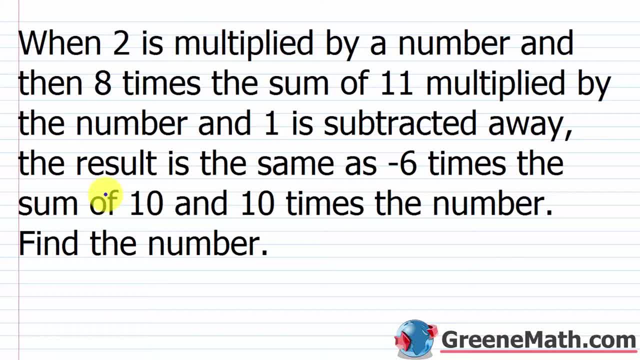 start looking at some common application problems again that deal with linear equations in one variable. So when 2 is multiplied by a number, and then 8 times the sum of 11 multiplied by the number and 1 is subtracted away, the result. 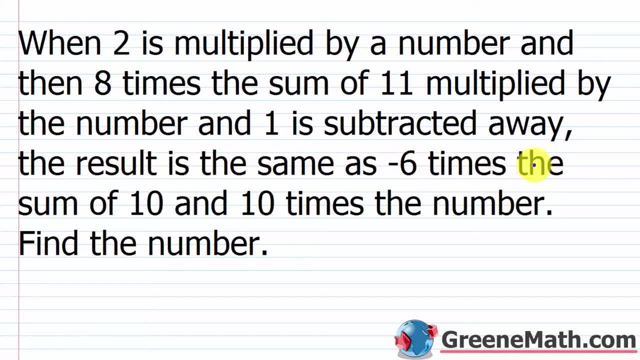 is the same as negative, 6 times the sum of 10 and 10 times the number, Find the number. So this is a lot more complex than the little simple ones we looked at earlier. We're just kind of putting things together, So let's go through And again. 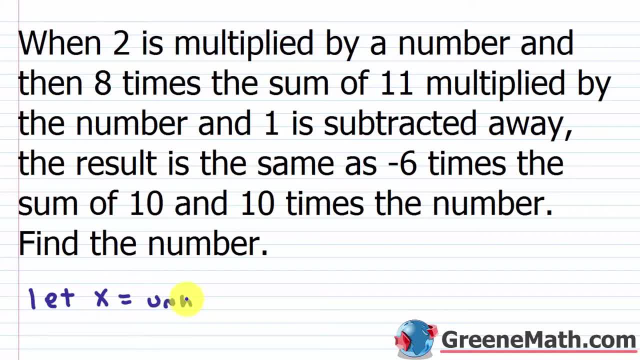 I'm just going to let x be equal to my unknown number here. So I'm going to highlight everywhere I see a number and just put x there. So everywhere I see a number or the number. So let's read back through. When 2 is multiplied by x and 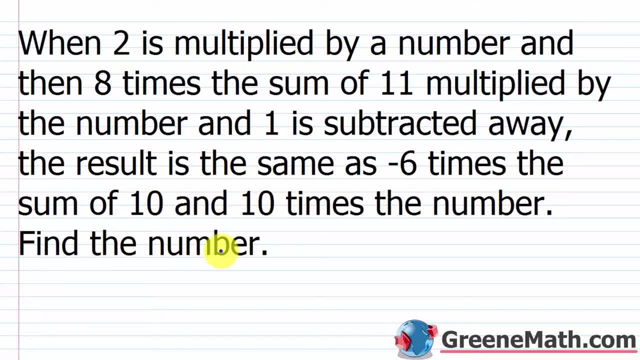 times the number, Find the number. So this is a lot more complex than the little simple ones we looked at earlier. We're just kind of putting things together, So let's go through and again, I'm just going to let x be equal to my unknown number here. So I'm going to highlight everywhere: 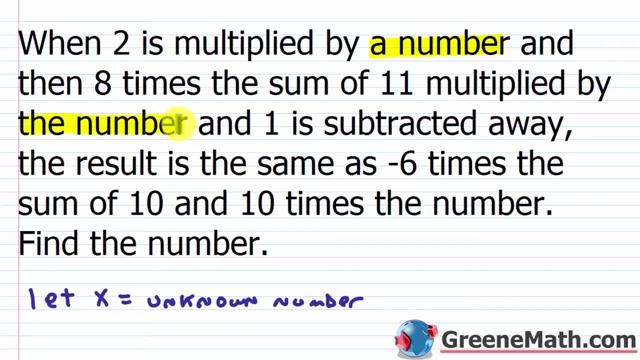 I see a number and just put x there. So everywhere I see a number or the number. So let's read back through. When 2 is multiplied by x, and then 8 times the sum of 11 multiplied by x and 1 is subtracted away, the result is the same as. 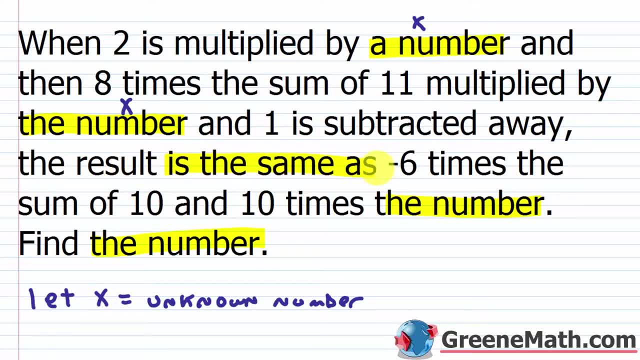 So we know this part right here where we say: is the same as that's going to be, equals negative 6 times the sum of 10 and 10 times again for the number I'm going to put x, and then find the number I'm going to put x here. All right. so let's read back through this now. 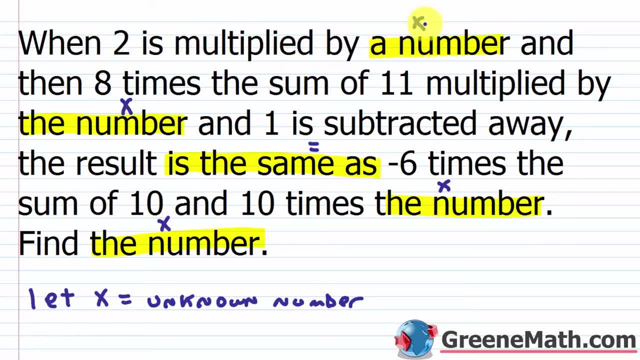 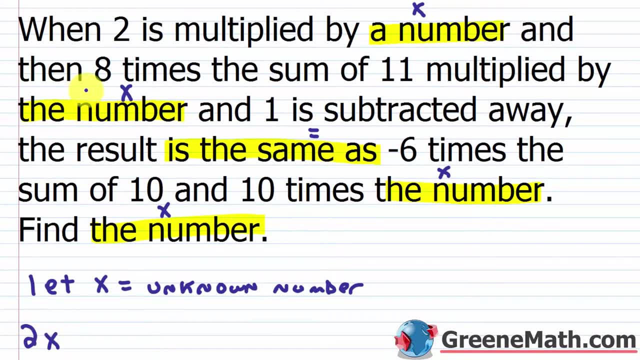 So we have when 2 is multiplied by our number x- so I'm going to put 2x- Then we have, and then So, and then means afterwards We have 8 times the sum of So whenever you have the sum of in this type of problem, 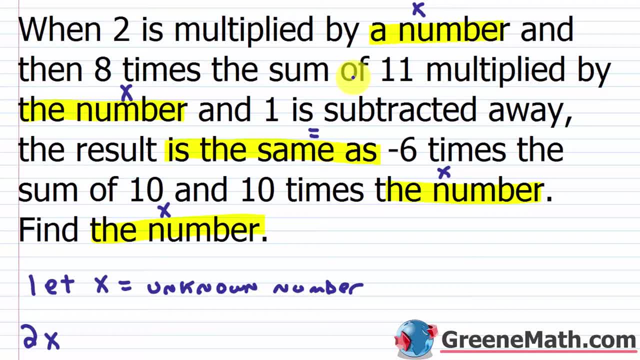 you're going to multiply 8 by a set of parentheses. okay, because you're going to have a sum. So I'm going to put 8 out here times a set of parentheses. I don't know what's going to go inside yet, but I'm just going to set that up. So 8 times the sum of, you've got 11 multiplied by. 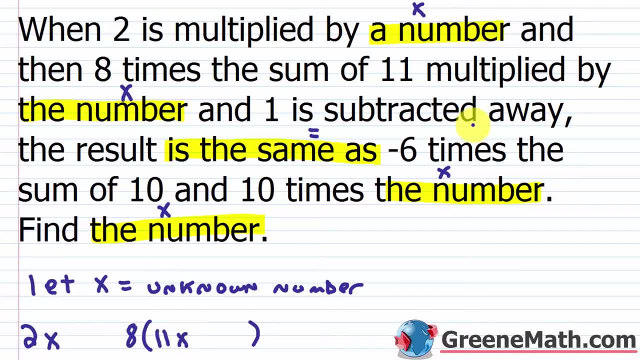 our x, So we've got 11x, and then and 1.. So and 1.. And now it says, is subtracted away. So this was subtracted away from our 2x. So let's just read through this part again. 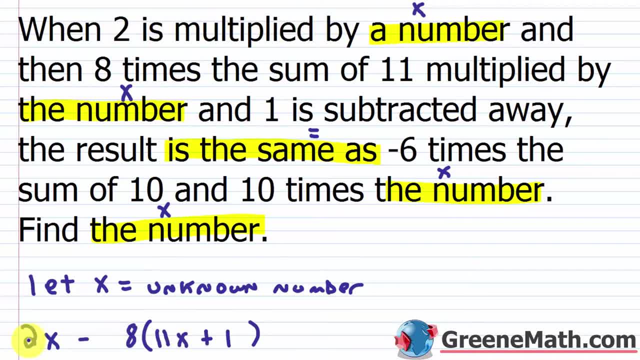 and make sure we got it. So when 2 is multiplied by x, we have our 2x, And then 8 times the sum of 11 multiplied by x and 1 is subtracted away. So 8 times the sum of, we have 11x and 1.. 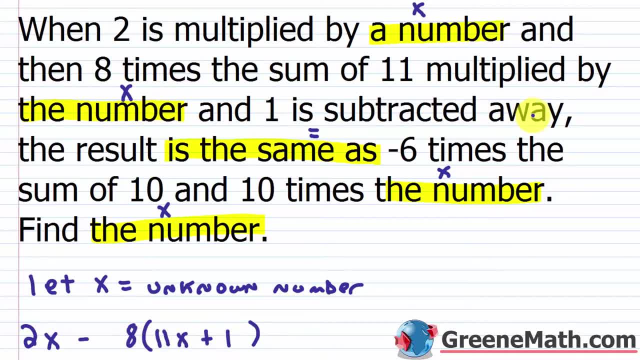 So 8 times the sum of 11x and 1. That's what we have here, and again that's subtracted away. So that's why we have minus 8 times the quantity 11x plus 1. Then we have: 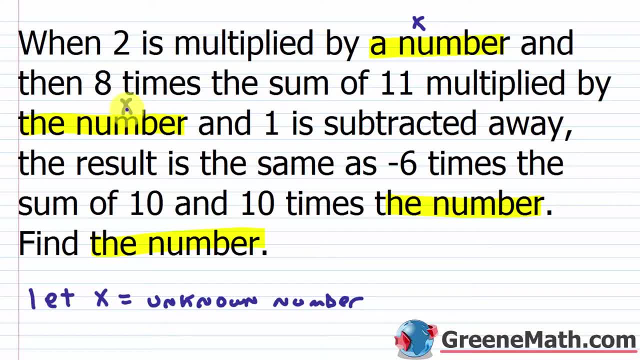 then 8 times the sum of 11, multiplied by x and 1 is subtracted away, the result is the same as. So we know this part right here where we say: is the same as, that's going to be equals negative, 6 times the sum of 10 and 10 times again for. 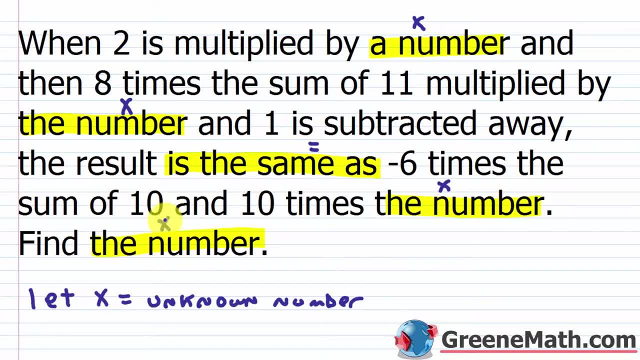 the number. I'm going to put x, And then find the number I'm going to put x here. All right, so let's read back through this now. So we have when 2 is multiplied by, and then we have our number x. So I'm going to put 2x, Then we have, and then 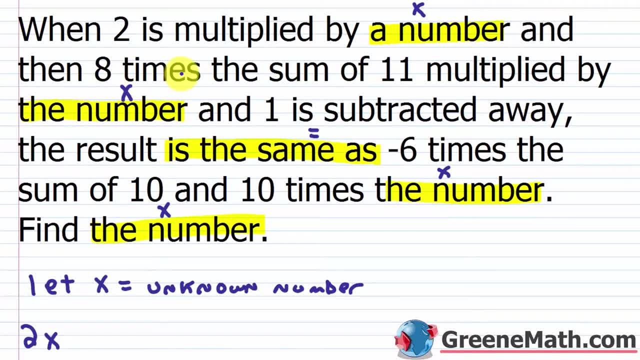 So, and then means afterwards We have 8 times the sum of. So whenever you have the sum of in this type of problem, you're going to multiply 8 by a set of parentheses. okay, because you're going to have a sum, So I'm going to put 8 out here. 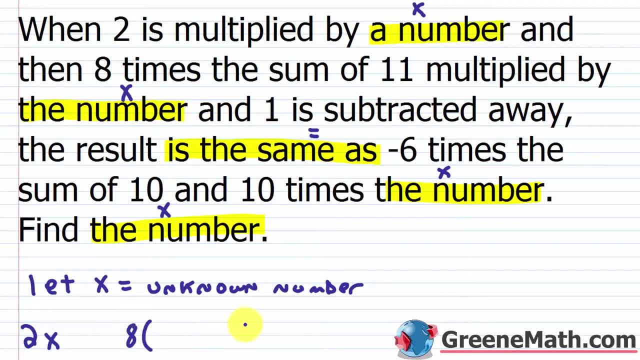 times a set of parentheses. I don't know what's going to go inside yet, but I'm just going to set that up. So 8 times the sum of you've got 11 multiplied by our x, So we've got 11x And 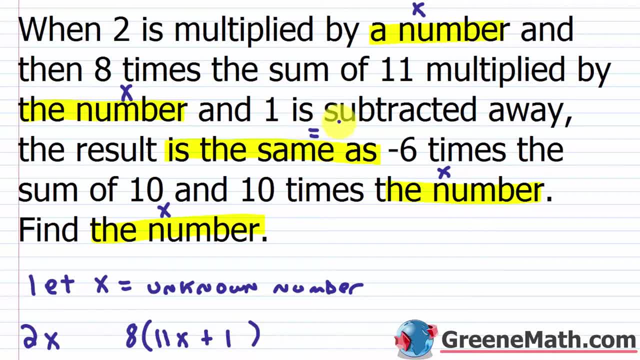 then and 1.. So and 1.. And now it says is subtracted away. So this was subtracted away from our 2x. So let's just read through this part again and make sure we got it. So when 2 is multiplied by, 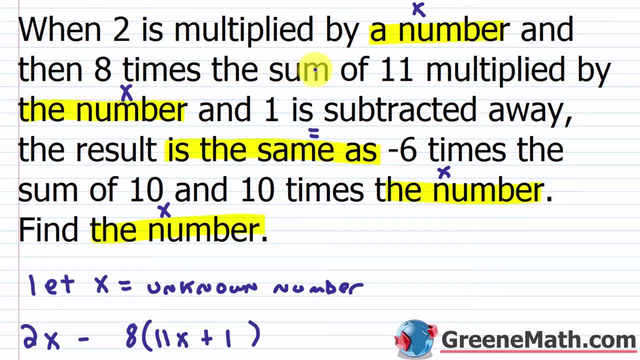 x, we have our 2x, And then 8 times the sum of 11 multiplied by x and 1 is subtracted away, So 8 times the sum of, and then we have 11x and 1.. So 8 times the sum of 11x and 1.. That's what. 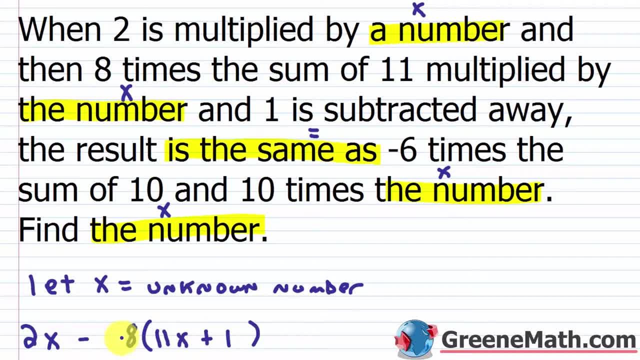 we have here And again that's subtracted away. So that's why we have minus 8 times the quantity, 11x plus 1. Then we have the result is the same as: So we know this is equals. Then we have negative 6 times the sum. of So again I want to put: 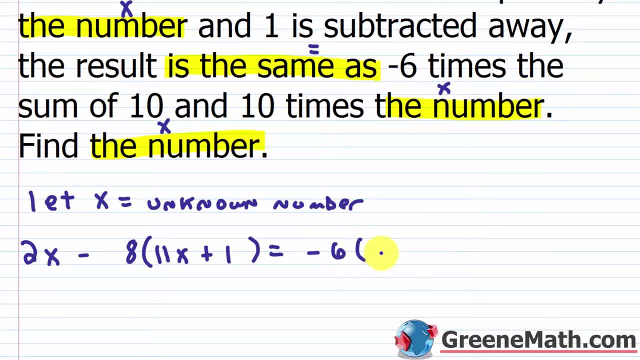 negative 6. here, If I have times the sum of something, I'm going to use parentheses. So then we have 10 and 10 times x, So 10 times the negative 6.. And going to use a spice, I'm going to use. 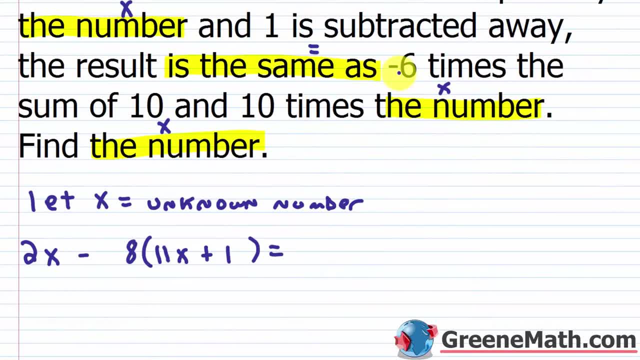 result is the same as. So we know this is equals. Then we have negative six times the sum of. So again I want to put negative six here. If I have times the sum of something, I'm going to use parentheses. So then we have 10 and 10 times x, So 10 plus 10x, And this is basically going to be. 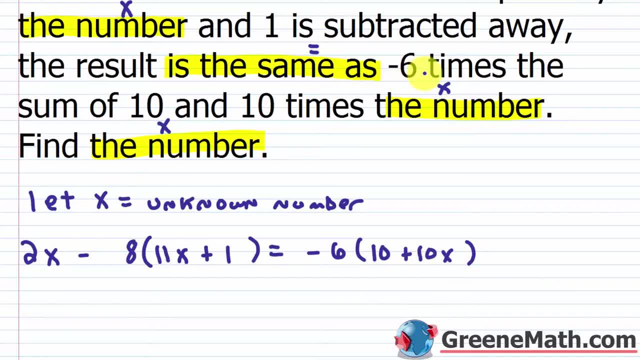 our equation right. So again to go through this part, again we have negative six times the sum of, So negative six times the sum of 10 and 10 times x, So negative six times the quantity 10 plus 10x. 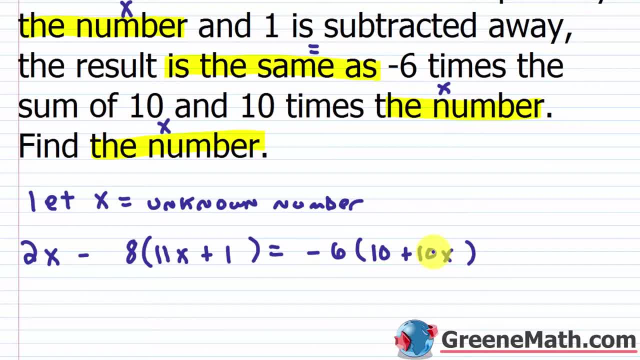 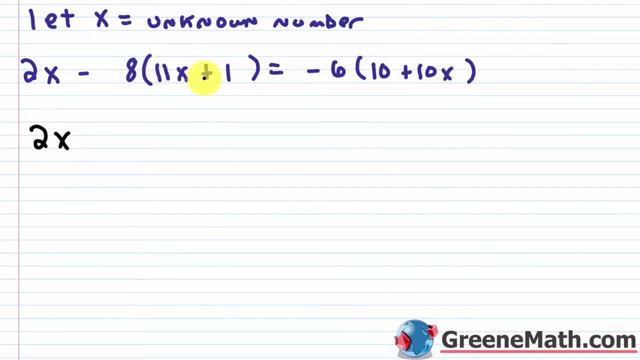 is what that translates to. Okay, let's go ahead and solve this equation. So I'm going to have my 2x here And then I'm going to distribute the negative eight to each term. So you would have minus 88x and then minus eight. This equals I'm going to distribute the negative six to each term. 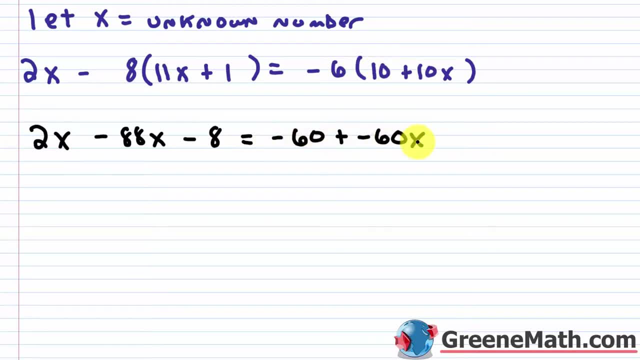 So negative 60 plus negative 60x. On the left I can clean up because 2x minus 88x would be negative 86x. Then you have: minus eight is equal to negative 60 plus negative 60x. So you can just put minus 60x, whatever you want to do. 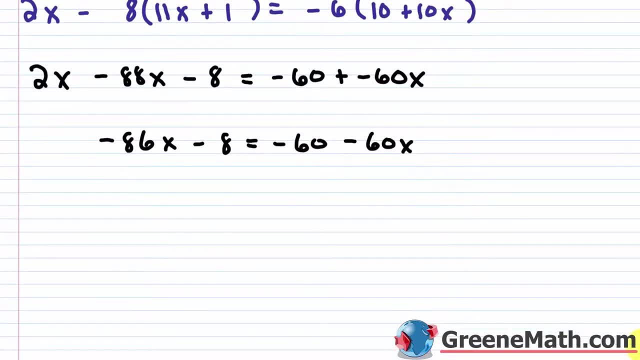 It doesn't matter, Let me kind of get some room going here. So let's go ahead and add 60x to each side of the equation. Let's add eight to each side of the equation. So we know that this is going to. 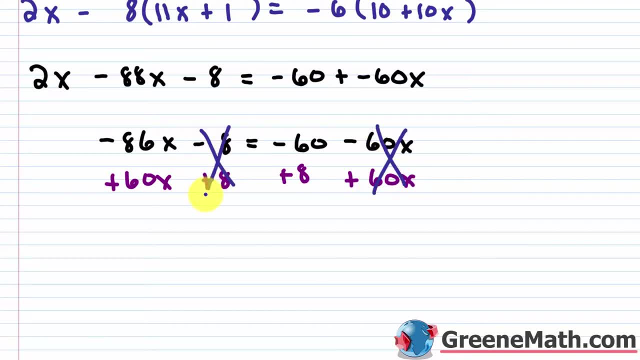 cancel here And this is going to cancel here. Negative 86x plus 60x is negative 26x, And this equals negative 60 plus eight is going to be negative 52. Now if I divide both sides of the equation by negative 26,, I'm going to get that. 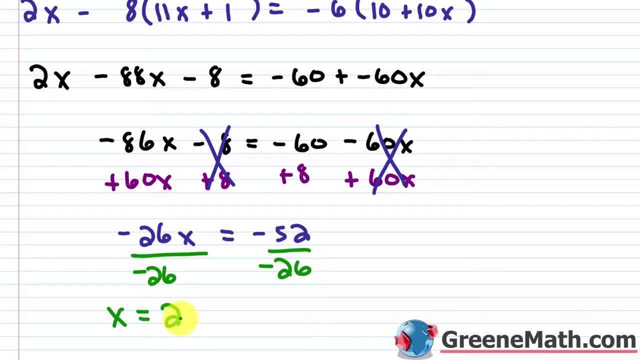 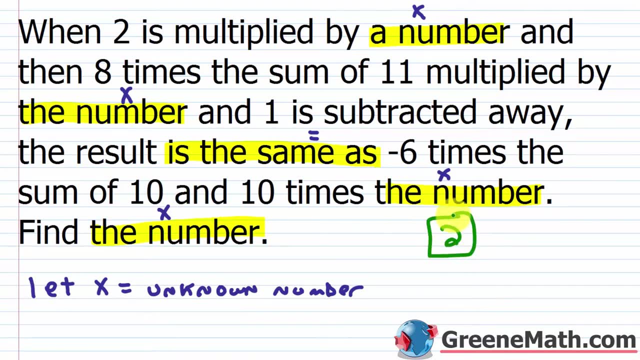 x is equal to positive two. Okay, so two is my unknown number. So let's go back up, Let's write this as our unknown number And let's check this. So when two is multiplied by two, so two times two. 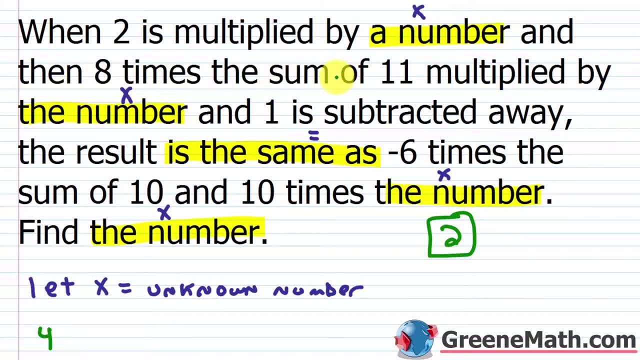 is four, And then eight times the sum of 11 multiplied by two and one. So we're going to have eight multiplied by the sum of 11 times two, which is 22. And one. So 22 plus one is 23.. 23 times. 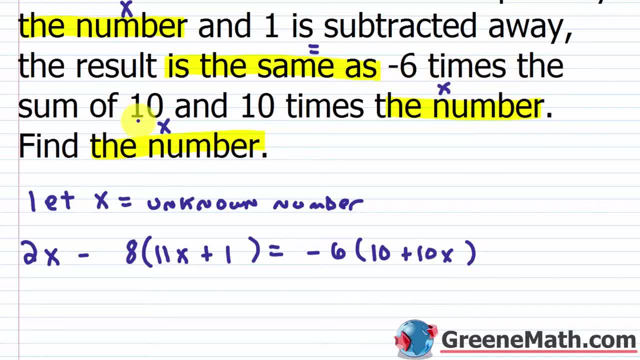 1. So that's subtracted away from 11 time. So I'm going to draw out like this And I'm going to write: represent anti-12 times 10 times. provided for x, I'm going to put 1 plus 7 times 8 timesazzle, which is reflect for degrees worth. 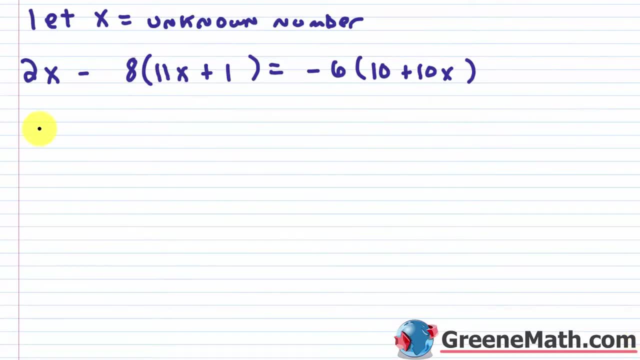 8. And subtract out all effectively, all effectively, all effectively from our automatically. We're going to call this, we're going to do aession here to do function And we're going to worried it. We're going to do function with. 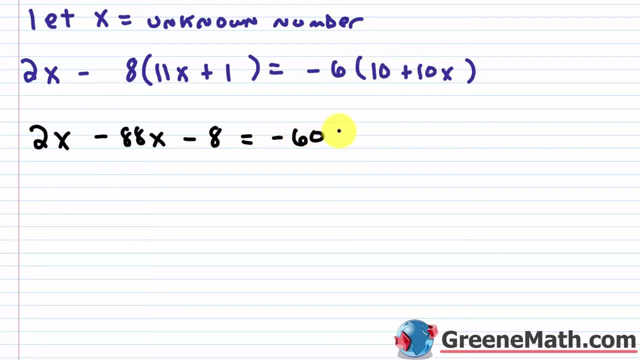 the power of 1 and scratch that when x get toambt And we're going to distribute the negative 60 each term, So negative 60 plus negative 60x. On the left side I can clean up, because 2x minus 88x would be negative 86x. Then you have minus 8 is equal to negative. 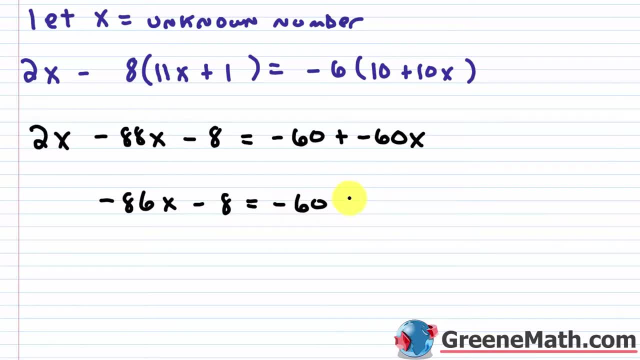 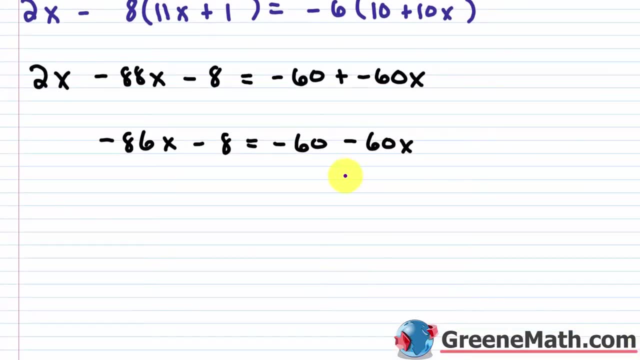 60 plus negative 60x, So you can just put minus 60x. whatever you want to do, It doesn't matter. Let me kind of get some room going here, So let's go ahead and add 60x to each side of the equation. 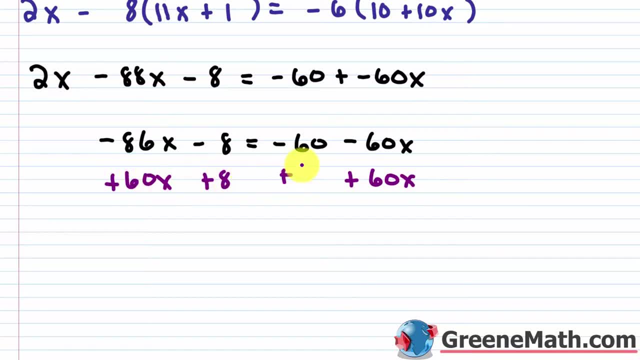 Let's add 8 to each side of the equation, So we know that this is going to cancel here and this is going to cancel here. Negative 86x plus 60x is negative 26x, And this equals negative 60 plus 8 is going to be negative 52.. Now, if I divide both sides of the equation by, 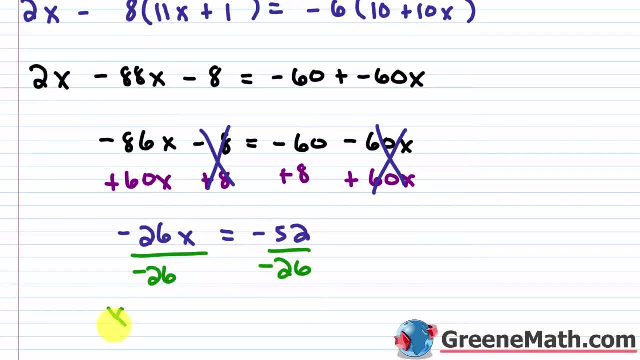 negative 26,. I'm going to get that x is equal to positive 2.. So 2 is my unknown number. So let's go ahead and add 8 to each side of the equation. So we know that this is going to cancel. 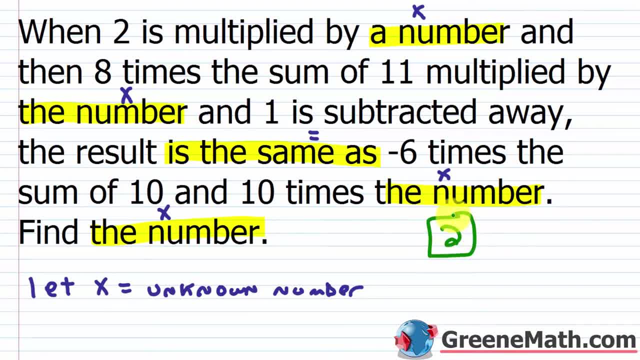 here. So let's go back up, Let's write this as our unknown number and let's check this. So when 2 is multiplied by 2, so 2 times 2 is 4, and then 8 times the sum of 11 multiplied by 2. 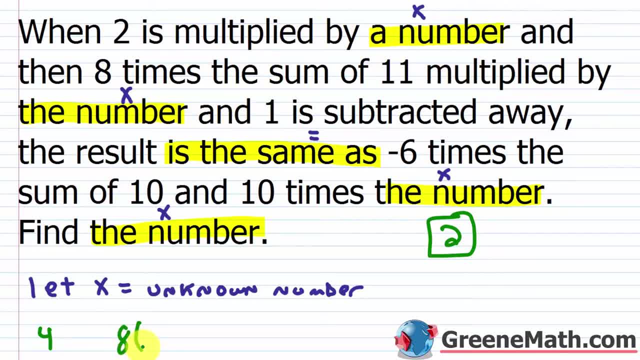 and 1.. So we're going to have 8 multiplied by the sum of 11 times 2, which is 22, and 1.. So 22 plus 1 is 23.. 23 times 8 is 184.. So we'd have 184 here. 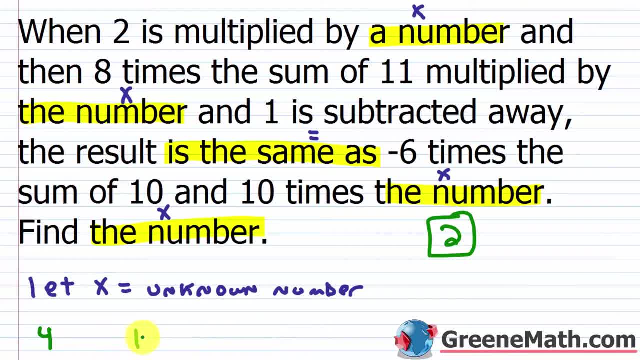 eight is 184. So we'd have 184. Now it says that this is subtracted away. So four minus 184 is going to be negative, negative 184. And it says the result is the same as. so we're going to put equals here. you've got negative six. 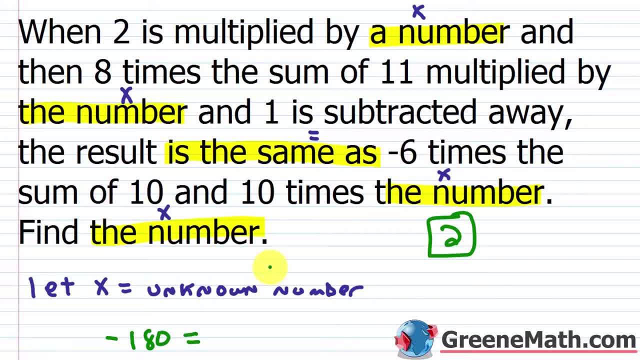 times the sum of you've got your 10 and 10 times x. And again x is two. So you'd have negative six times the sum of you would have 10 plus 10 times two is 20.. So 10 plus 20 is 30. So you'd have. 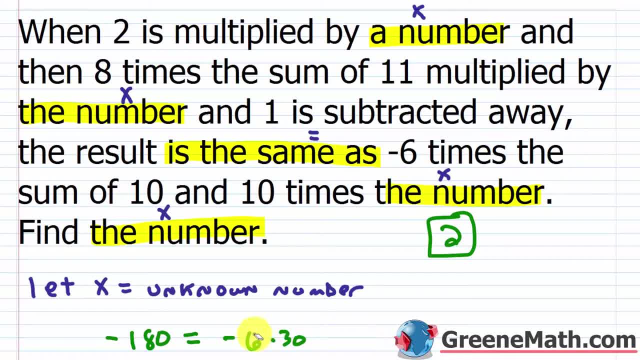 negative six times 30, which is negative 180.. So the same value is on the left. So you'd have the numbers on the left as we have on the right. both are similar values. So two is our correct solution, right? that's going to be our unknown number. Alright, so I'll say we got one more of. 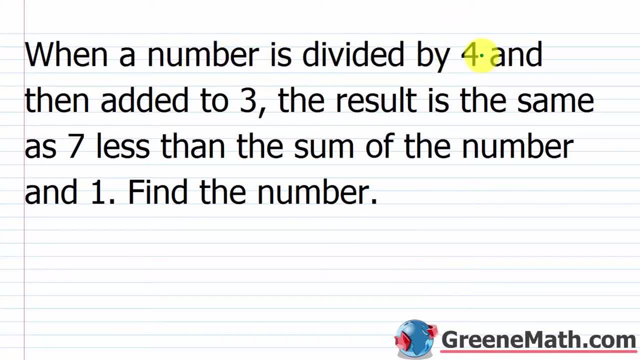 these So we have, when a number is divided by four and then added to three, the result is the same as seven less than the sum of the number and one then find the number. So again, wherever I see a number, So where we see a number here, and then If I put x in each place And then the number, 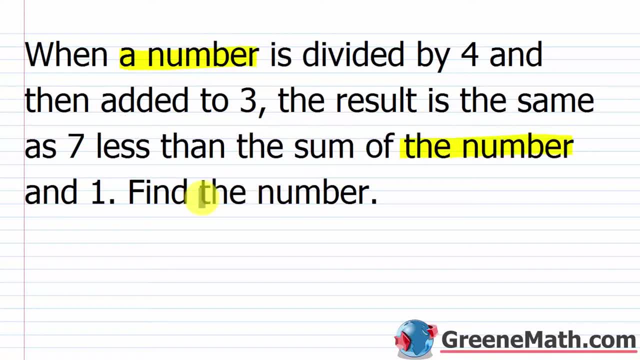 here, and then the number here, And then the number here, is going to put x in each place And then again, for completeness, I'm just going to say we're going to let x be equal to our unknown, our unknown number. okay, 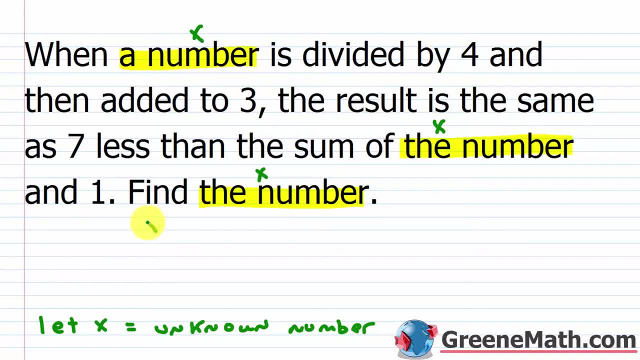 So, reading back through now, when x is divided by 4, so that's x over 4, and then add it to 3, so then just plus 3, the result is the same as. so that means equals right. 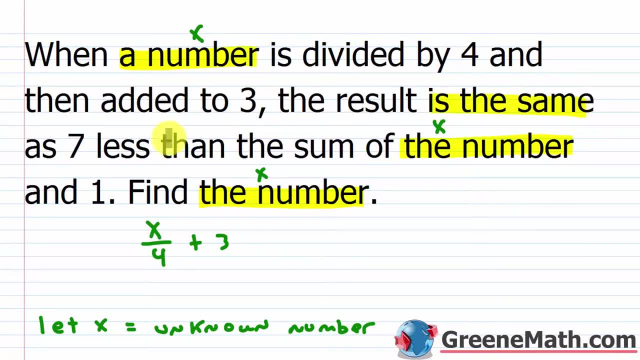 So I can just kind of highlight this, where it says is the same as- and I can just put equals there, so this will be equals here- It says 7 less than 7 less than the sum of x and 1.. So we want the sum of x and 1, which is x plus 1, and then we want 7 less than that. 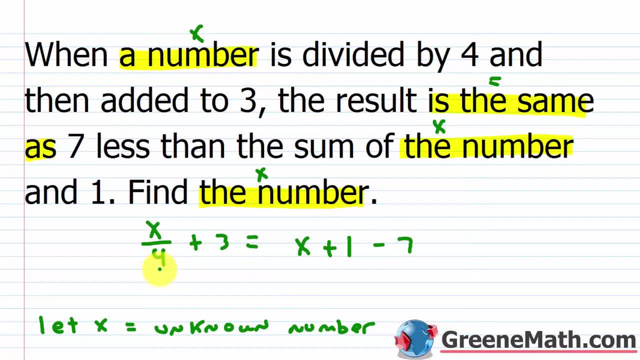 so just subtract 7 away from that and this will be our equation. okay, So let's copy this and we'll just come down here to a fresh page. so we're not in the way of everything, And what I'm going to do is just kind of click. 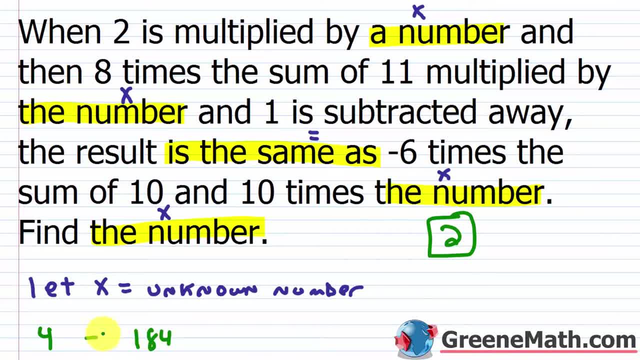 Now it says that this is subtracted away, So 4 minus 184 is going to be negative, negative 180. And it says the result is the same as. So we're going to put equals here. You've got negative 6 times the sum of, You've got your 10 and 10 times x, And again x is 2.. 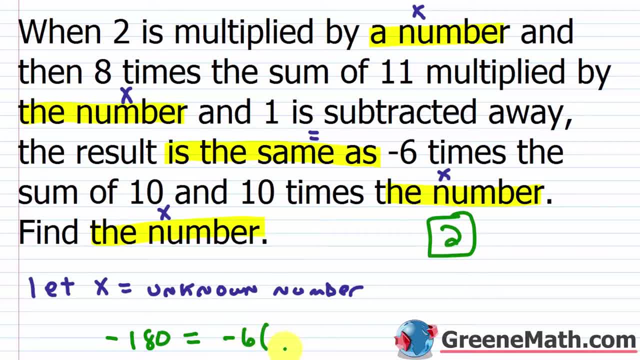 So you'd have negative 6 times the sum of You would have: 10 plus 10 times 2 is 20.. So 10 plus 20 is 30. So you'd have negative 6 times 30, which is negative 180.. So the same. 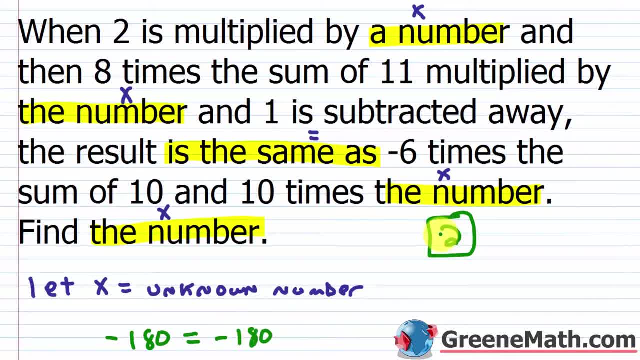 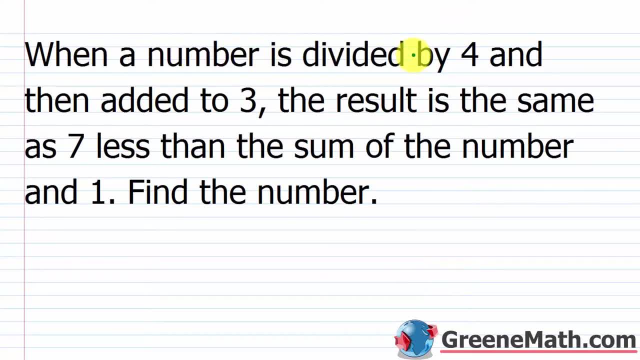 value is on the left as we have on the right, So 2 is our correct solution here. That's going to be our unknown number, So let's take a look at one more of these. So we have. when a number is divided by 4 and then added to 3, the result is the same as 7 less than the sum of the number. and 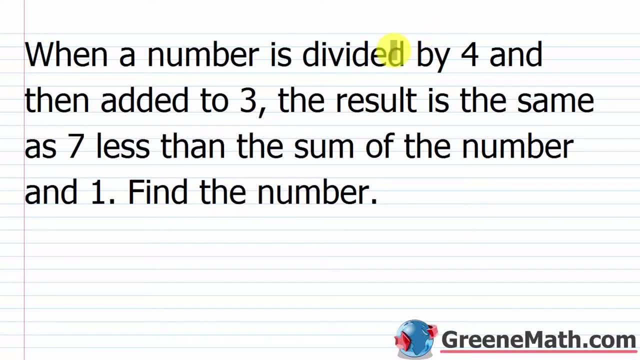 1. Then find the number, So again wherever I see a number. so where we see a number here, and then the number here, and then the number here. I'm just going to put x in each place And then again for completeness. 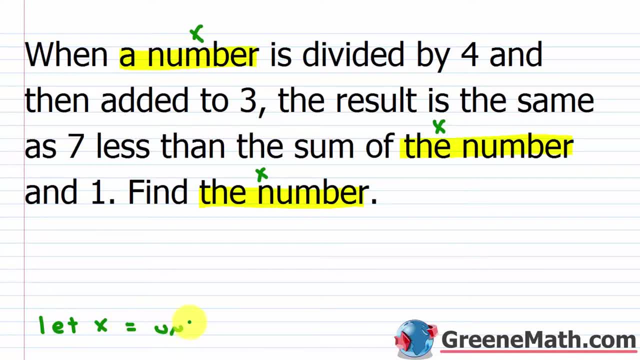 I'm just going to say we're going to let x be equal to our unknown, our unknown number. OK, so reading back through now, when x is divided by 4, so that's x over 4, and then added to 3.. 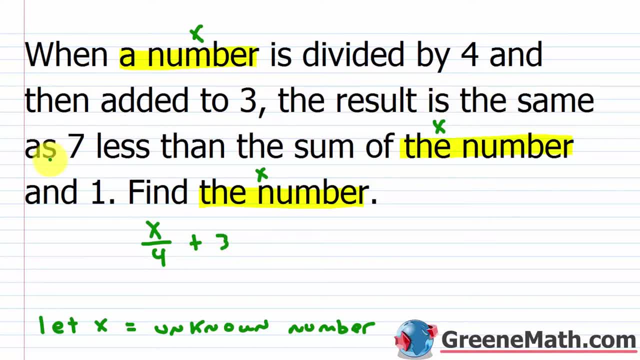 That's just plus 3.. The result is the same as. So that means equals, right? So I can just kind of highlight this. where it says is the same as- And I can just put equals there, So this will be equals. here It says 7 less than 7 less than the sum of x and 1.. So we want the sum of x and 1, which is x. 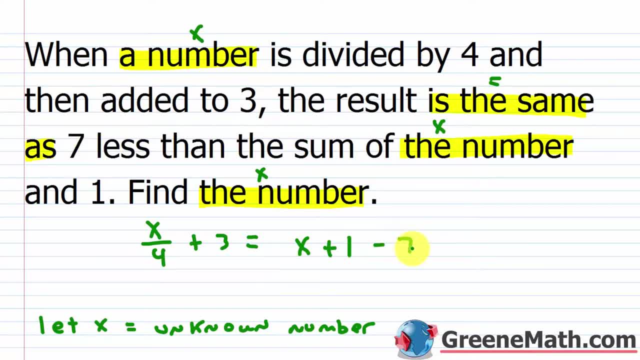 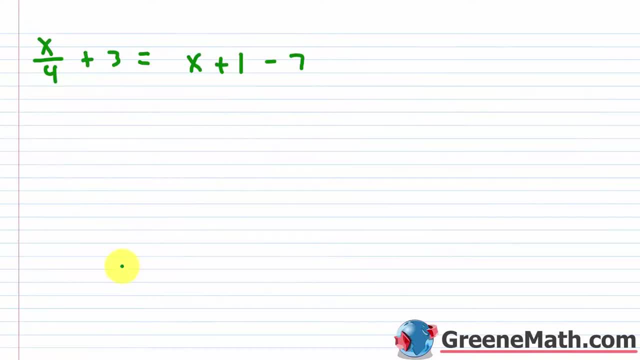 plus 1.. And then we want 7 less than So just subtract 7 away from that And this will be our equation. OK, so let's copy this And we'll just come down here to a fresh page, so we're not in the way of everything. 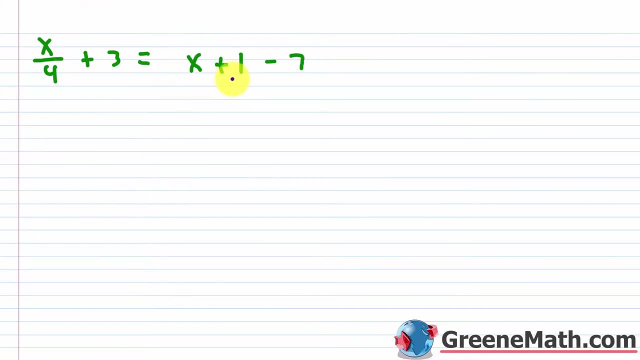 And what I'm going to do is just kind of clean up first. So I'm going to add 1 and negative 7.. 1 plus negative 7 or 1 minus 7 is going to be negative 6. So I would have x over 4 plus 3. 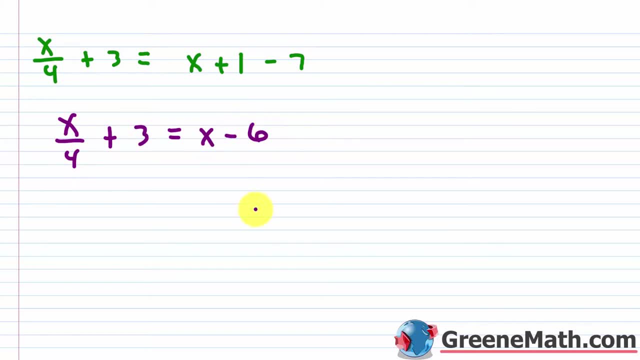 equals x minus 6.. And I can subtract 3 away from each side of the equation. Kind of make that a little better And let me go ahead and cancel this. So we have x over 4.. 1 minus 7 is equal to x minus. if we have negative 6 minus another 3, or negative 6 plus negative 3.. 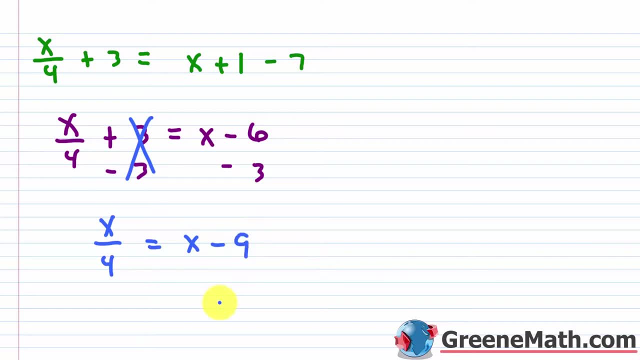 You're going to get negative 9.. So this is x minus 9.. And then now I can clear this denominator here by multiplying both sides of the equation by 4.. So these would cancel. I just have x on the left. On the right you'd have 4 times the quantity x minus 9.. So that's 4x minus 36.. OK, So to solve. 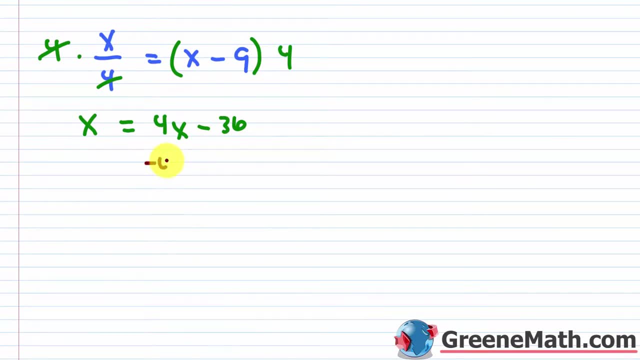 this equation: we're going to have x minus 9.. And then we're going to have x minus 9 plus 9.. So that's 4x minus 36.. guy for x. what I'm going to do is I'm going to subtract 4x away from each side of the equation. 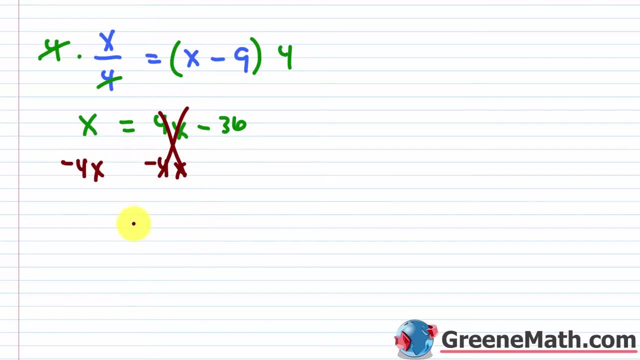 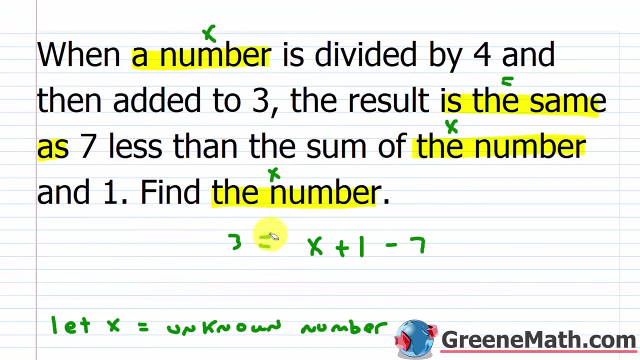 so that's going to cancel x minus 4x is going to be negative 3x and this equals negative 36. so now we can divide both sides of the equation by negative 3 and we're going to get that x is equal to 12. so let's go back up. so we're going to say that our unknown number is 12, so 12. 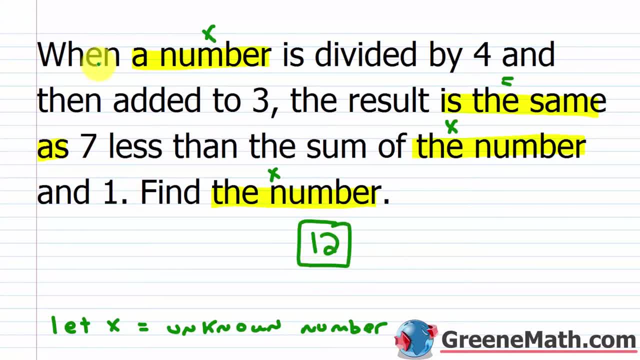 okay. so let's check when 12 is divided by 4, that would give me 3, right? 12 divided by 4 is 3, and then added to 3. so 3 plus 3 would be 6. we say the result is the same as or equal to. 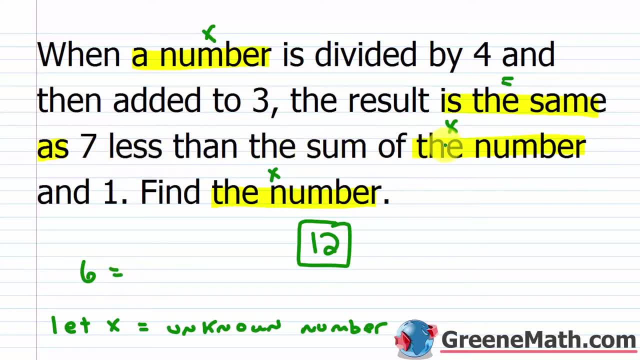 7 less than the sum of, you'd have x as representing the number. so 12 and 1. so the sum of 12 and 1 is 13, and if I had 7 less than that I would have 6. so again, same value on the left as you have. 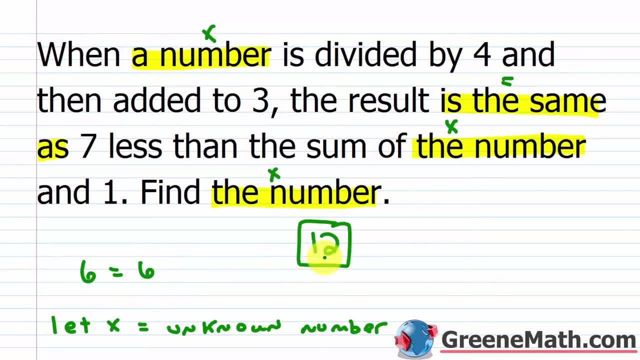 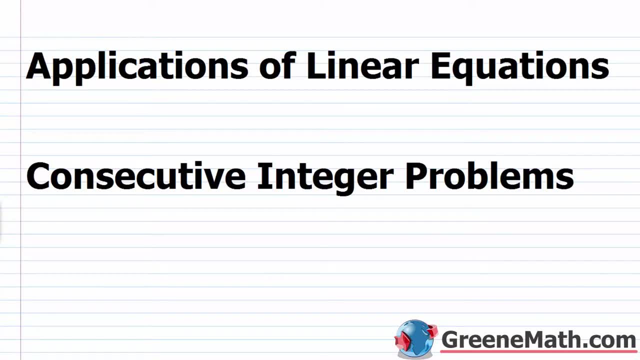 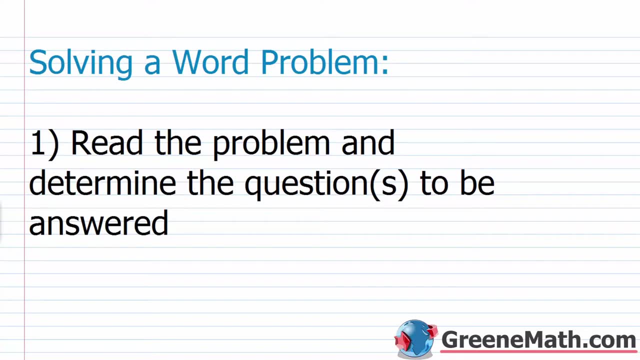 on the right, so you can say that 12 is in fact the correct solution. that's your unknown number. in this lesson, we want to review applications of linear equations and talk about consecutive integer problems. all right, so once again, when we have an application problem that involves setting, 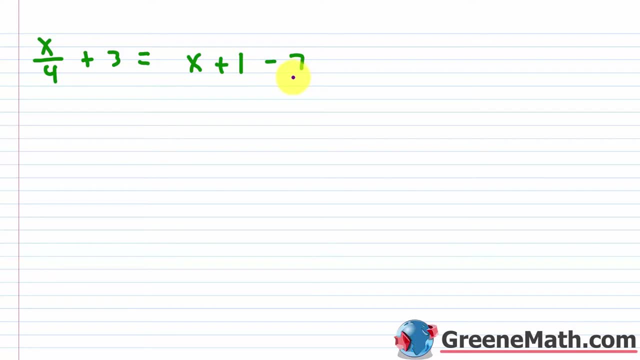 I'm going to clean up first. So I'm going to add 1 and negative 7.. 1 plus negative 7 or 1 minus 7 is going to be negative 6.. So I would have x over 4 plus 3 equals x minus 6.. 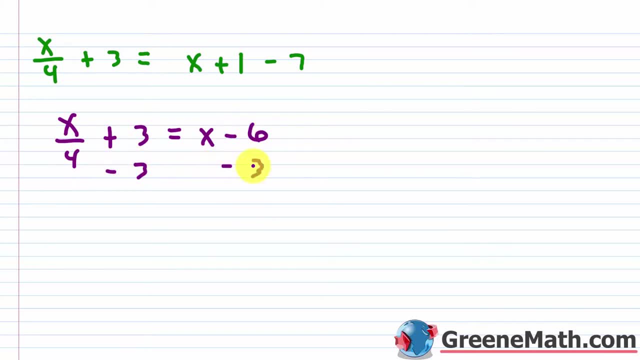 And I can subtract 3 away from each side of the equation. kind of make that a little better And let me go ahead and cancel this. So we have x over 4 is equal to x minus. If we have negative 6 minus 6.. 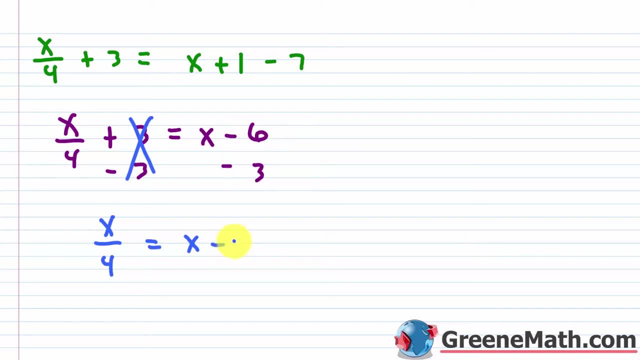 This is another 3, or negative 6 plus negative 3,, you're going to get negative 9.. So this is x minus 9.. And then now I can clear this denominator here by multiplying both sides of the equation by 4.. 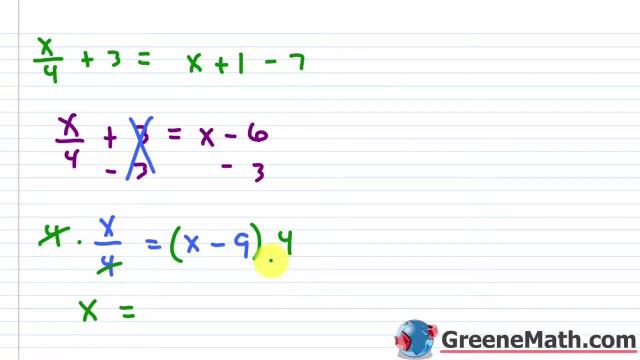 So these would cancel. I just have x on the left. On the right you'd have 4 times the quantity x minus 9, so that's 4x minus 36, okay, So to solve this guy for x, what I'm going to do is I'm going to subtract 4x away from 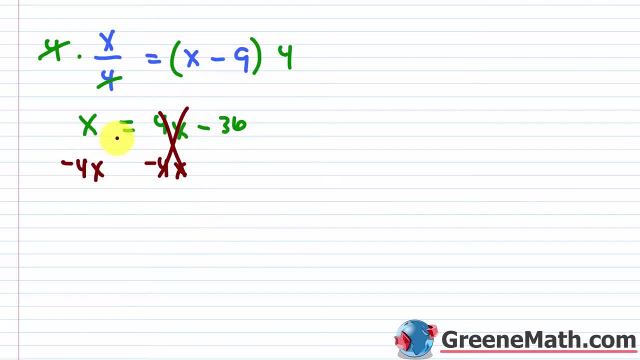 each side of the equation. So that's going to cancel. x minus 4x is going to be negative 3x and this equals negative 36.. So now we can divide both sides of the equation by negative 3, and we're going to get that. 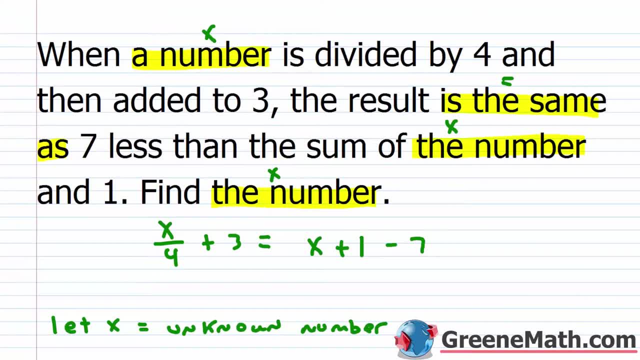 x is equal to 12.. So let's go back up. So we're going to say that our unknown number is 12.. So 12. Okay, So let's check When 12 is divided by 4, that would give me 3,, right? 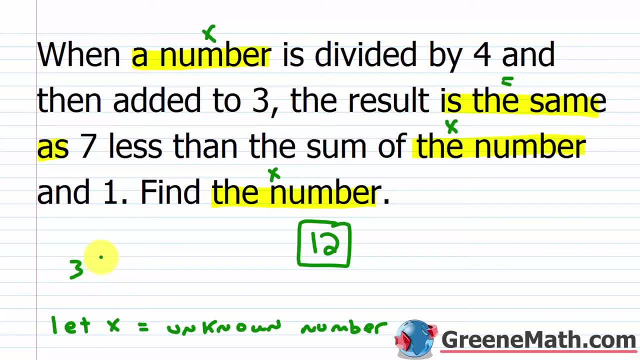 12 divided by 4 is 3.. And then add it to 3.. So 3 plus 3 would be 6.. We say the result is the same as, or equal to, 7 less than the sum of you'd have x as. 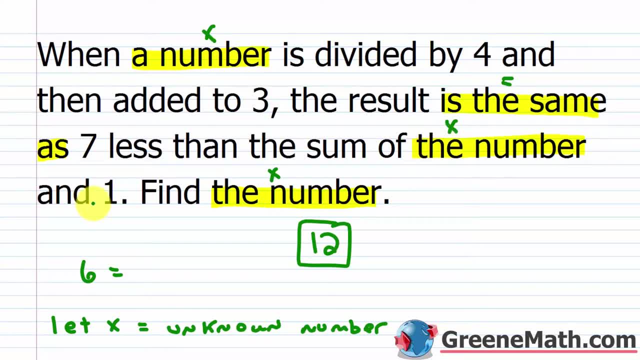 representing the number. so 12 and 1.. So the sum of 12 and 1 is 13,, and if I had 7 less than that, I would have 6.. So again, same value on the left as you have on the right. 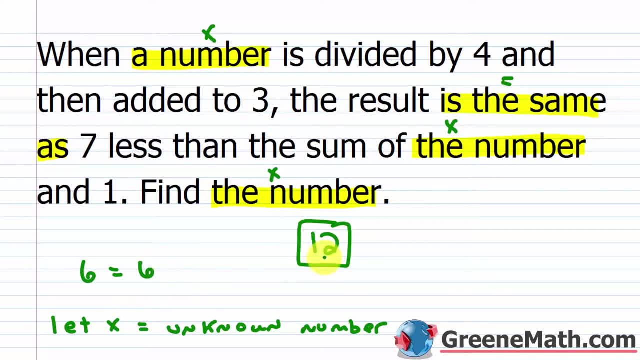 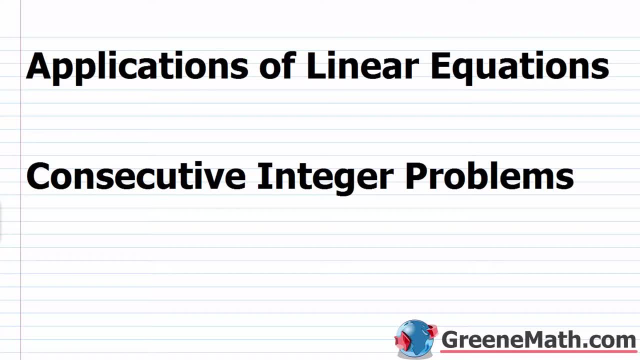 So you can say that 12 is in fact the correct solution. That's your unknown number. In this lesson we want to review applications of linear equations and talk about how to solve them, and talk about consecutive integer problems. All right, So once again, when we have an application problem that involves setting up and solving 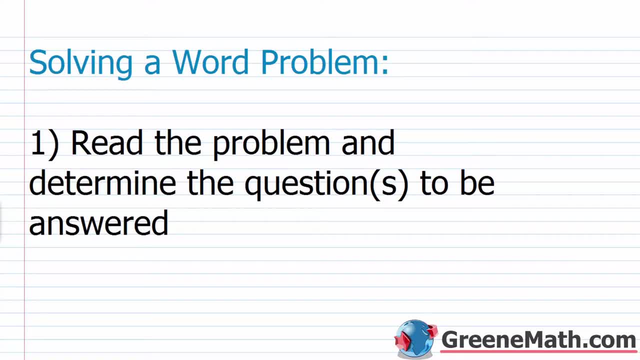 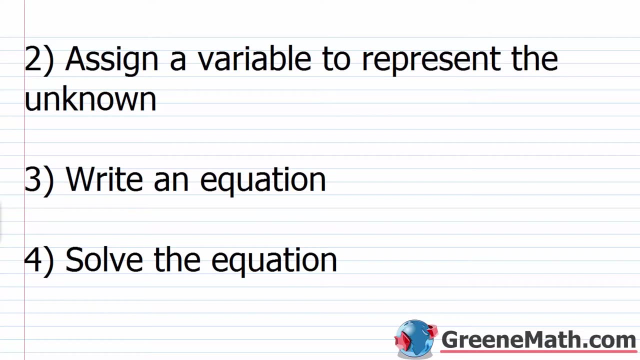 up and solving a linear equation in one variable. we have a little six-step procedure we can use. so for solving a word problem, the first thing we want to do is read the problem and determine the question, or get questions to be answered. then we want to assign a variable to represent the unknown and then in these type of problems we can always. 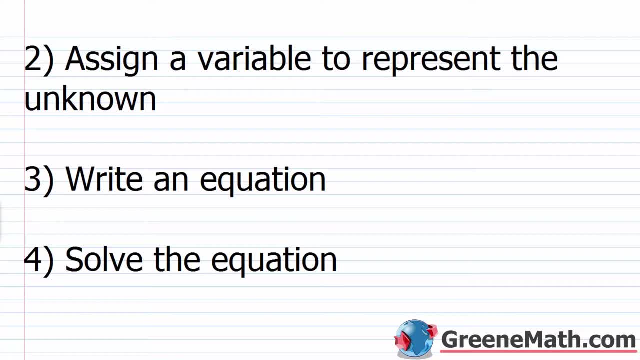 express any other unknowns in terms of this original variable, then we're going to write an equation. this will be based on the situation given. we're going to solve the equation, then we're going to write the answer in terms of the question or, again, the questions being asked. 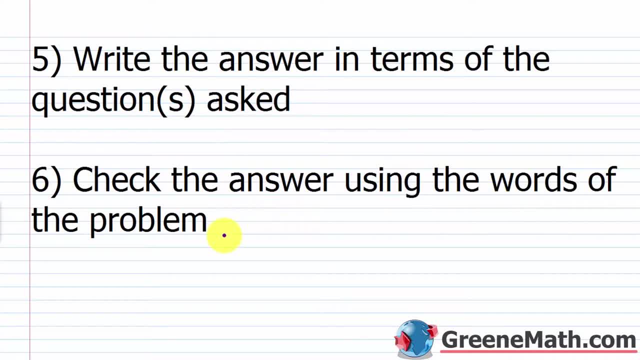 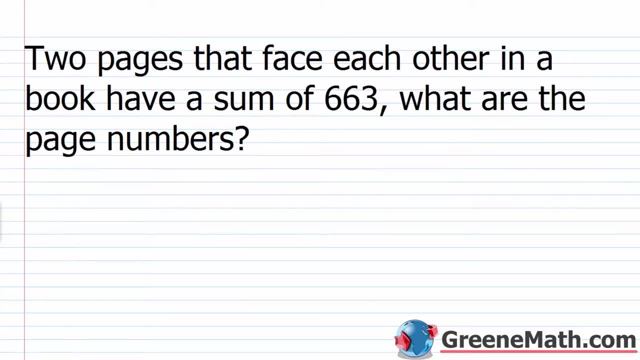 then, lastly, we're going to check the answer using the words of the problem. we always want to make sure that our answer is reasonable. all right, so let's just jump in and look at a problem. these problems are very easy to understand and solve, so you really shouldn't. 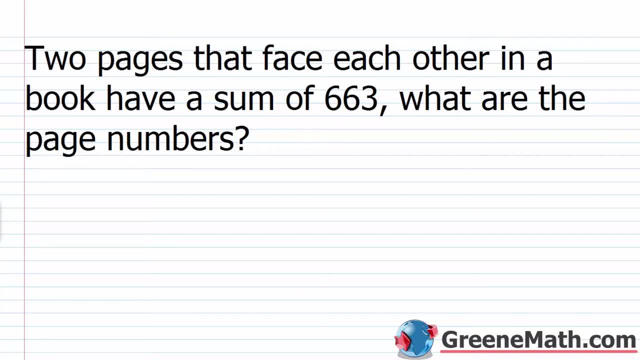 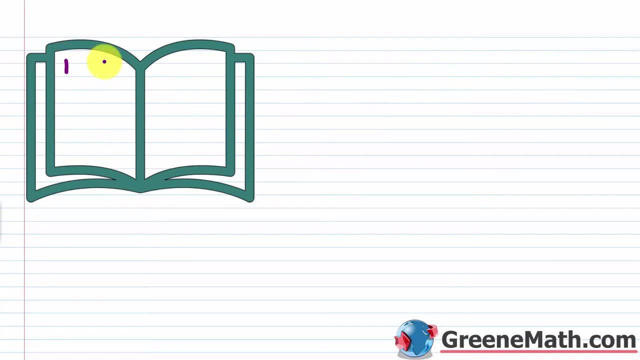 have too much of an issue with them. so two pages that face each other in a book have a sum of 663. what are the page numbers? so to get an idea of what's going on here, if you think about a book and you think about two pages that face each other, you could say this page is one and this page is two. 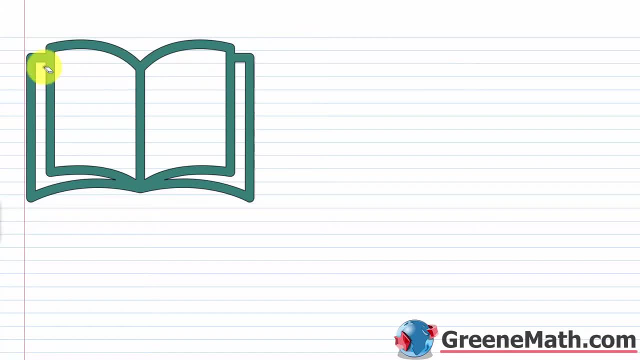 right, they're going to differ by one. or you could say that this page is, let's say, 500 and this page is 501. you know something like that. so we know that the smaller page could be represented with a variable like X. so let's let X be equal to the smaller page. okay, let me make that better, okay. 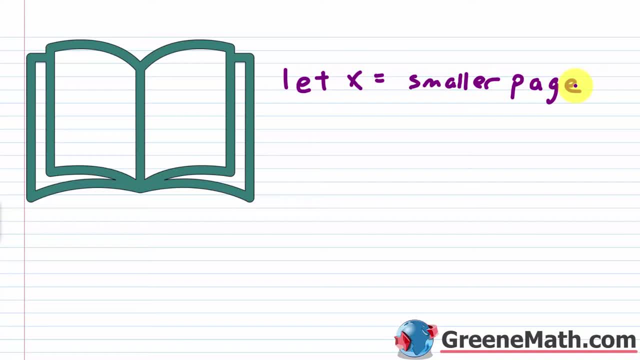 so then, what can we say about the larger page? well, it's just one more right. in the instance where we had one and two, one was the smaller, two is the larger, it's just a different of one. okay. so what I can say is that we could say then: X plus one is the larger. okay, the larger. 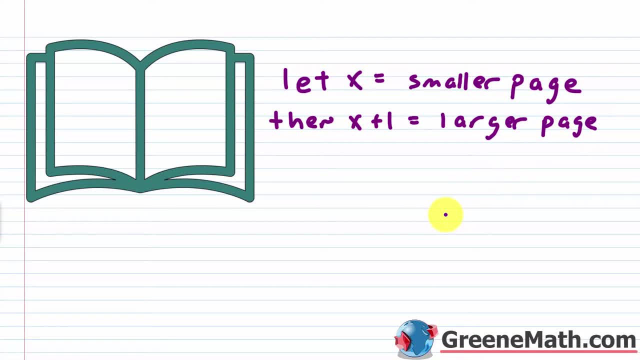 page. okay, so what we're told is that the sum of the pages is 663. so it's very easy to solve this. I just take my smaller page, which is X, and I add it to my larger page, which is X plus one, and this equals six hundred sixty-three. okay, so what we're told is that the sum of the pages is 663, so it's. 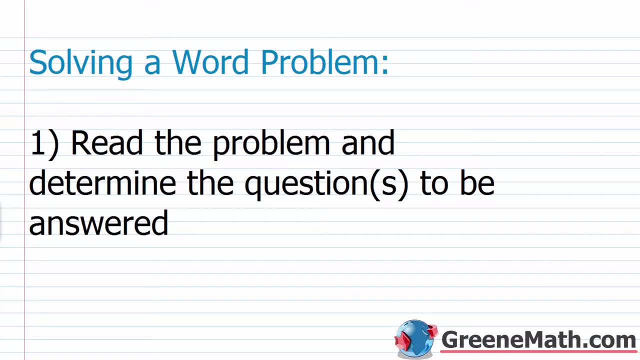 a linear equation in one variable. we have a little six-step procedure we can use. So for solving a word problem. the first thing we want to do is read the problem and determine the question, or get questions to be answered. Then we want to assign a variable to represent the unknown. 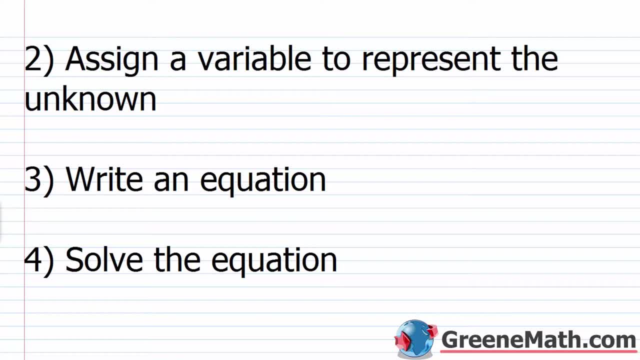 And then in these type of problems, we can always express any other unknowns in terms of this original variable. Then we're going to write an equation. This will be based on the situation given. We're going to solve the equation and we're going to write the answer in terms of the 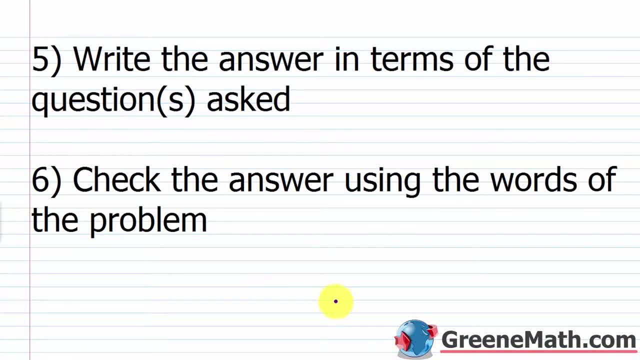 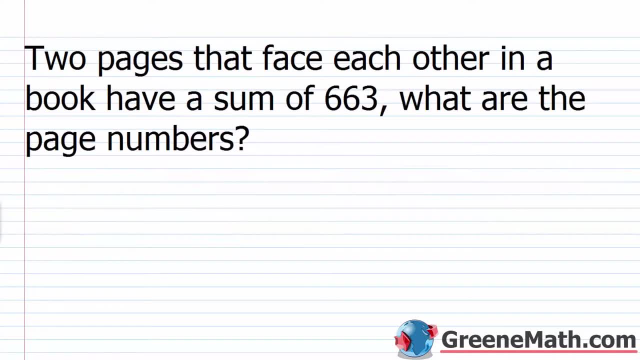 question, or again the questions being asked. Then, lastly, we're going to check the answer using the words of the problem. We always want to make sure that our answer is reasonable. All right, So let's just jump in and look at a problem. 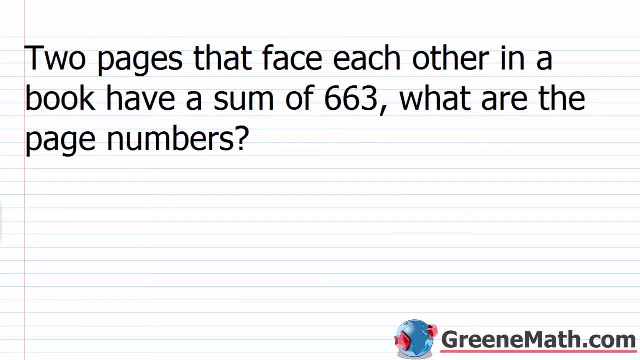 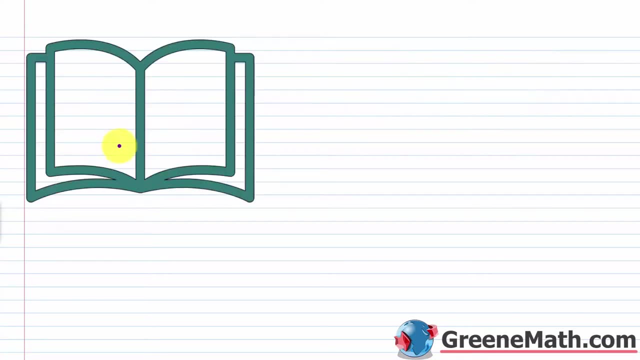 These problems are very easy to understand and solve, so you really shouldn't have too much of an issue with them. So two pages that face each other in a book. They have a sum of 663.. What are the page numbers? So to get an idea of what's going on here, if you think about a book and you think about 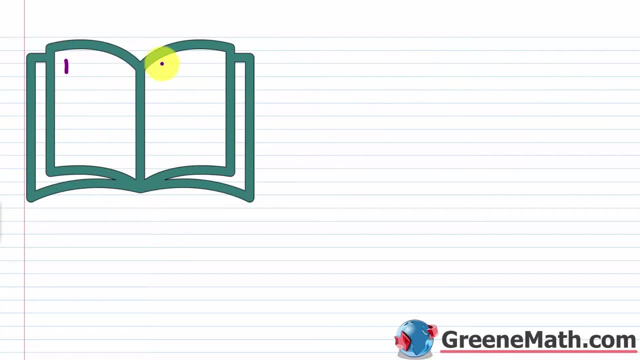 two pages that face each other. you could say: this page is 1 and this page is 2. They're going to differ by 1.. Or you could say that this page is, let's say, 500, and this page is 501, something. 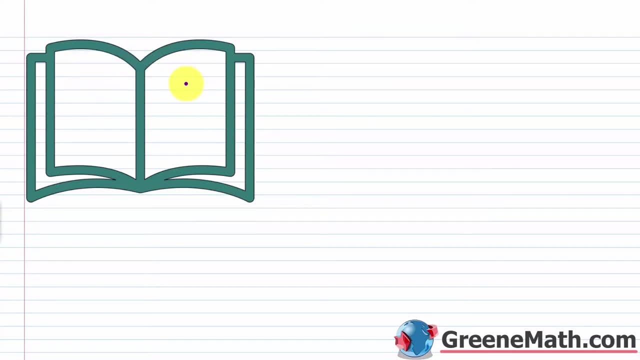 like that. So we know that the smaller page could be represented with a variable like x. So let's let x- So this is going to be an x- will be equal to this smaller page, And let me make that better. So then, what can we say about the larger page? 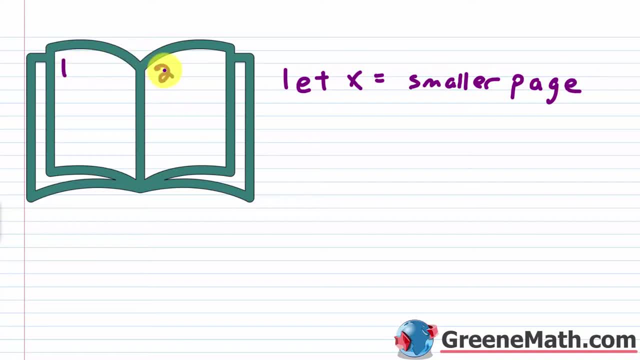 Well, it's just one more. In the instance where we had 1 and 2,, 1 was the smaller, 2 was the larger. It's just the difference of 1.. So what I can say is that we could say then x plus 1 is the larger. 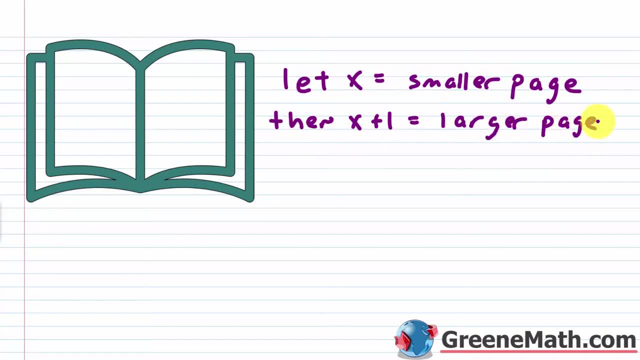 Okay, the larger page. okay, so what we're told is that the sum of the pages is 663. so it's very easy to solve this: I just take my smaller page, which is X, and I add it to my larger page, which is X plus 1, and this equals 663. okay, so all I got to do 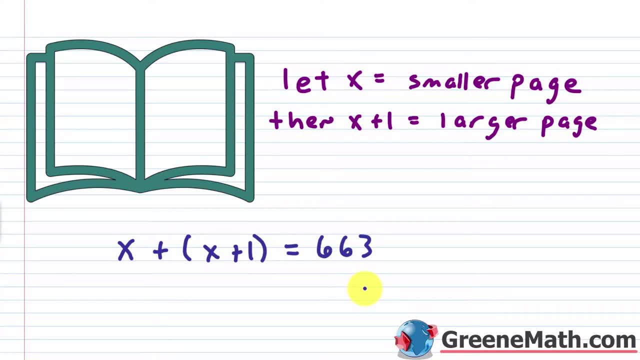 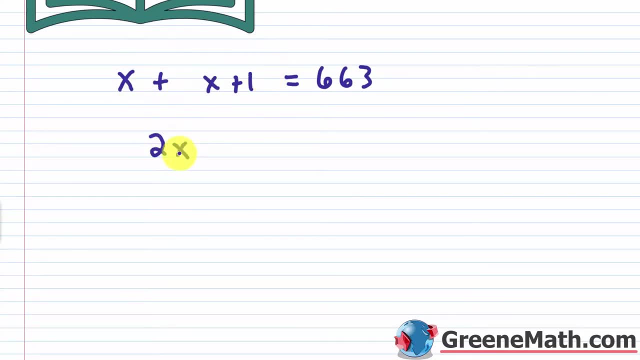 okay, so all I got to do now is just solve my equation very, very easy. so if I just remove the parentheses here, because I don't really need them, X plus X is 2x, and then plus one equals 663, let's go ahead and subtract one away from each side of the equation. we know this will cancel, and. 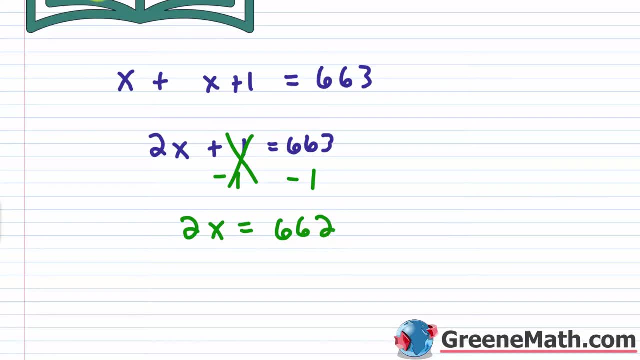 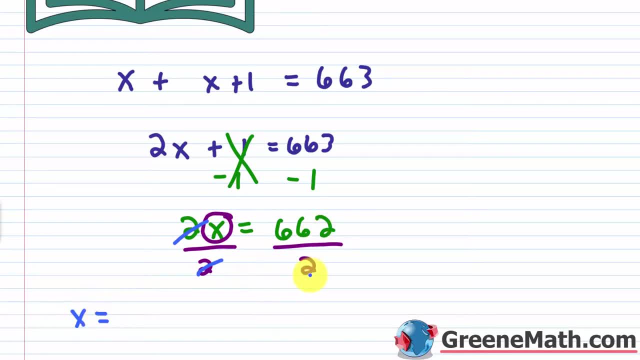 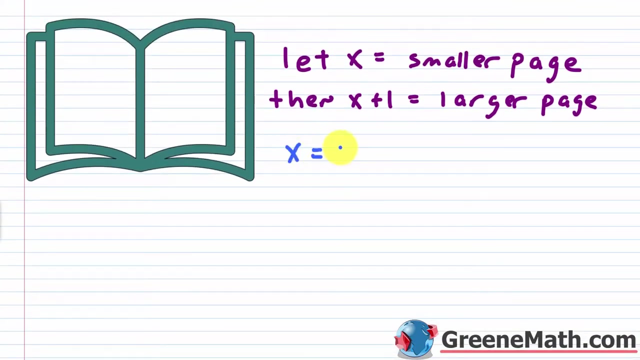 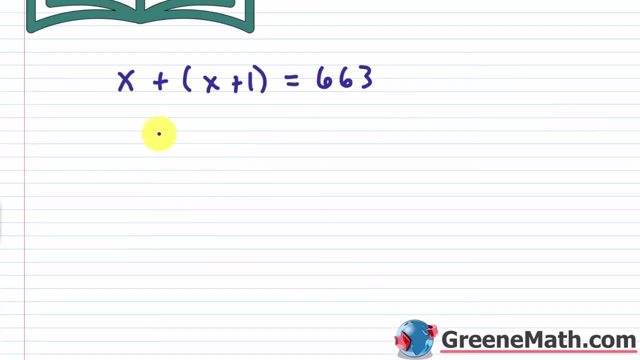 now is just solve my equation very, very easy. so if I just remove the parentheses here because I don't really need them, X plus X is 2x, and then plus 1 equals 663. let's go ahead and subtract 1 away from each side of the equation. we know this. 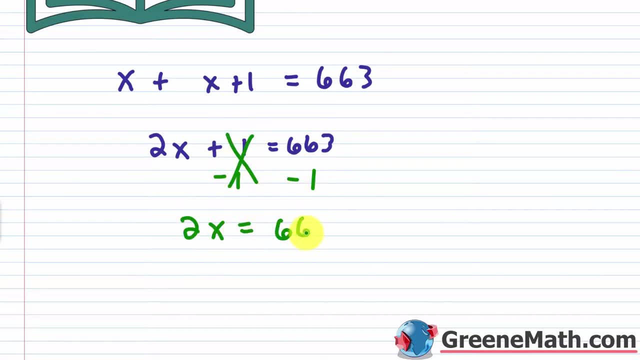 will cancel and you'll have: 2x is equal to 662. let's now divide both sides of the equation by 2 so that we can isolate the variable X. so we know that this will cancel. with this, and I'm going to end up with: X is equal to 662 divided by 2 is: 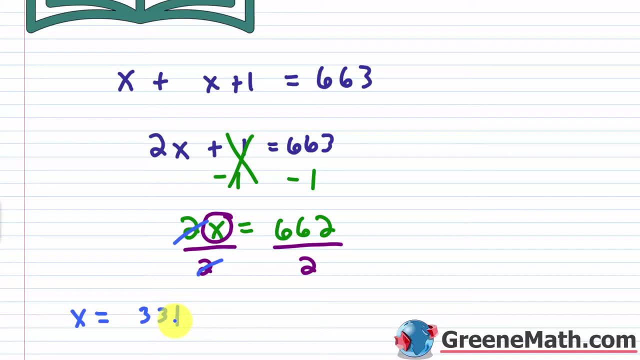 300, 363, 363, 331. okay, so again, when you work with a word problem, you can't just say X equals 331 and turn in the test. right, you got to make sense of it. so let's erase all this. I'll show you in our little picture what's going on. alright, so we come back. 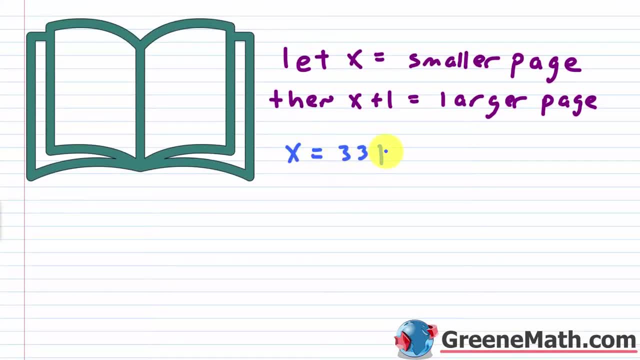 up here again. we said X was equal to 331. this is the smaller page. so in our book we could say: this page here is 331, and then the next page, the page that faces that one, is going to be 332. okay, and you could check. that is the smaller page, 331. well, if 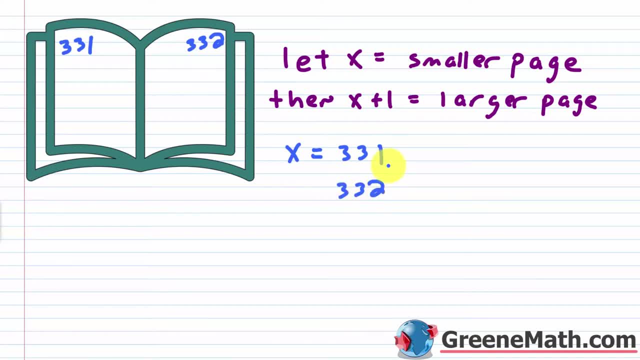 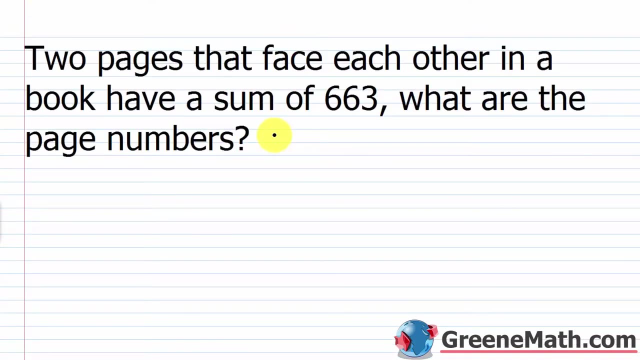 the larger page is 332. if you sum those two amounts together you do get 663, okay, so everything is consistent with what we're told in the problem. so let's go back up again. what are the page numbers? so to answer that question, we could say: 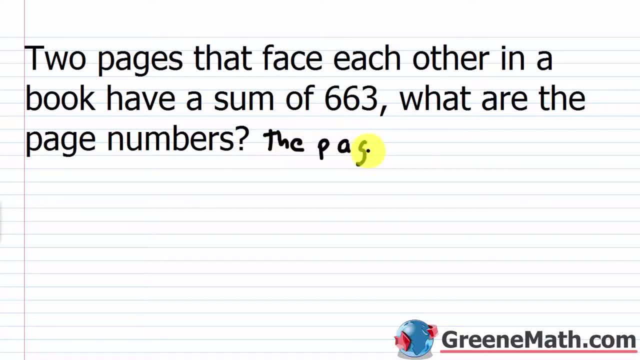 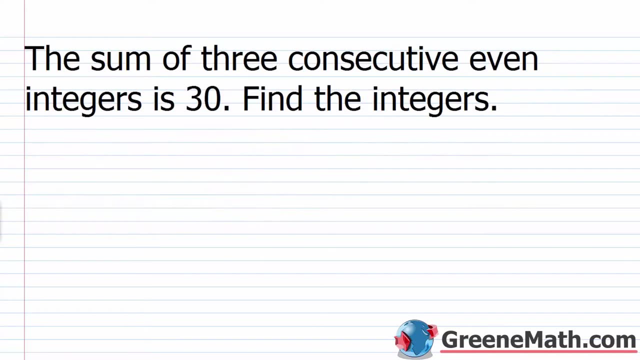 the page numbers, you are again 331 and 332. okay, nice and simple. all right, let's take a look at another one. so the sum of three consecutive even integers is 30, find the integers. so in this particular case, you've got to understand what it means by saying consecutive even integers. so, with 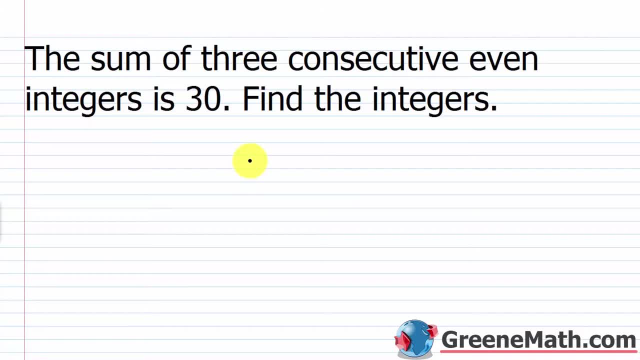 that we're talking about again, even numbers are numbers that are divisible by two, right? so this is 0, 2, 4, 6, 8, 10, 12, things like that. so if I want consecutive even integers, it could be 2, 4, 6, 8, 10, something like that it could. 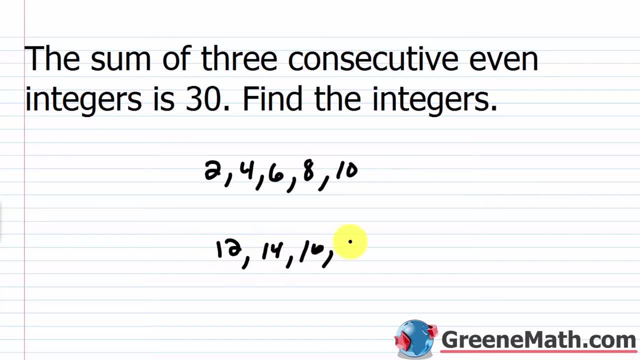 be starting at 12, so 12, 14, 16, 18, whatever number you start at, you're just increasing by 2 each time to get to the next even integer. okay, so if I want three consecutive even integers, I can let the smallest just be X. so let X be equal to the smallest even integer. okay, I make 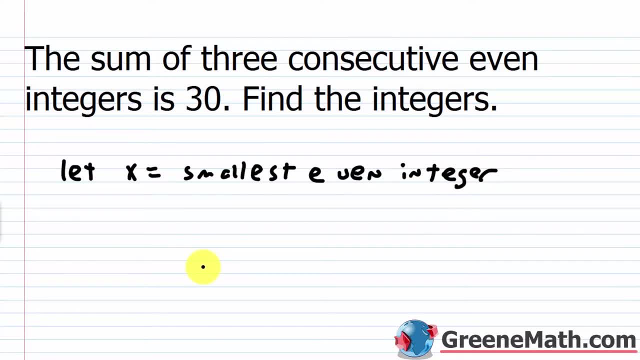 these E's a little better. so what can we say about the middle one? right, we have a smallest, we have a middle one and we have a largest. well, again, I'm just increasing by 2. if I started at 2 and I went to 4, I'm increasing by 2, right then? 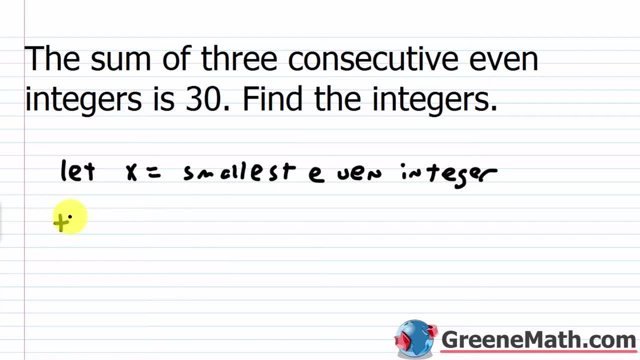 if I go to 6, I'm increasing by 2 again. so we can say then X plus 2 is our middle even integer. okay, let me make that better. and then what we could say then if I add another 2, so X plus 2. 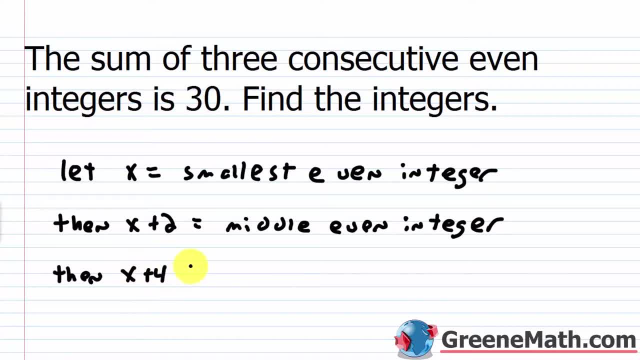 plus another 2 would be X plus 4. so X plus 4 would be the largest, even integer. okay, let me make these better. so we're told the sum is 30. right, it's right here. so all we really have to do is take X, which is the. 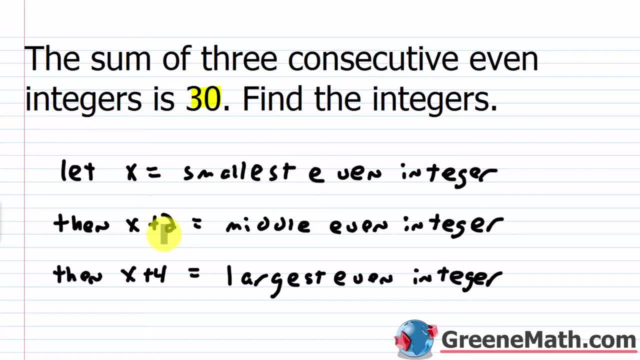 smallest even integer. add it to X plus 2, which is the middle even integer, and add that to X plus 4, which is the largest even integer, and set that to 30. solve that equation and we'll be good to go. so we have X plus X plus 2 plus X plus 4. you can wrap these in parentheses to kind of separate. 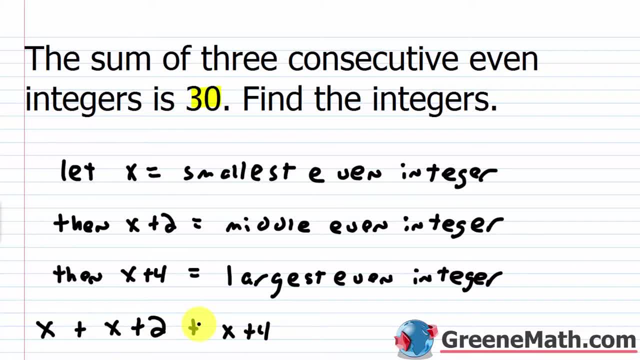 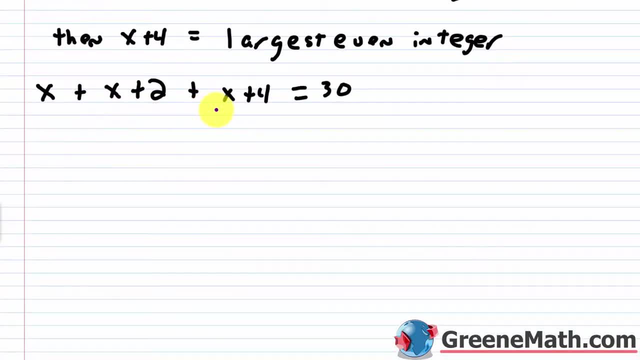 them if you want, but it really serves no purpose, so I'm not going to do that. and this is equal to 30. so let's solve this guy real quick. we'll have our answer. so X plus X plus X is 3, X, and then 2 plus 4, 6. so 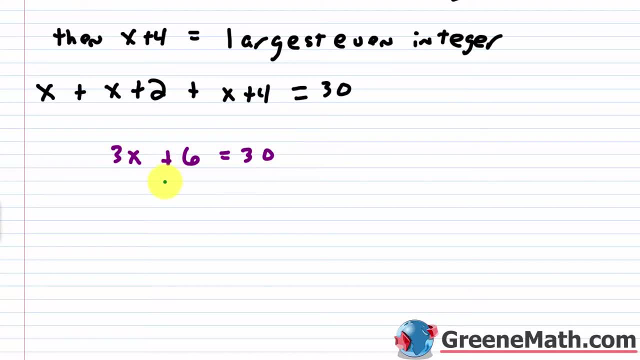 plus 6, this equals 30. let's go ahead and subtract 6 away from each side of the equation and this is going to cancel. we're going to have 3. X is equal to 30 minus 6 is 24, and then I want X by itself. 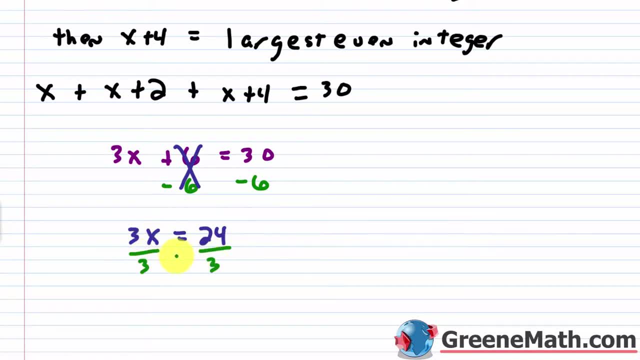 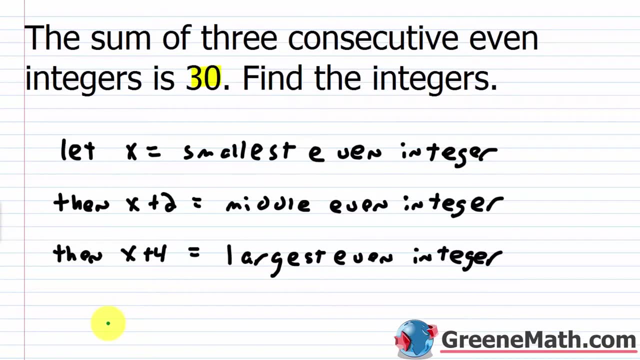 so let's divide both sides of the equation by 3 and we'll get what this cancels. with this you've got: X is equal to 8. okay, so let's erase everything again. the smallest even integer was represented with X, so we know that's 8. so then the next even integer would be what we add 2 to that, so we get 10 and then add: 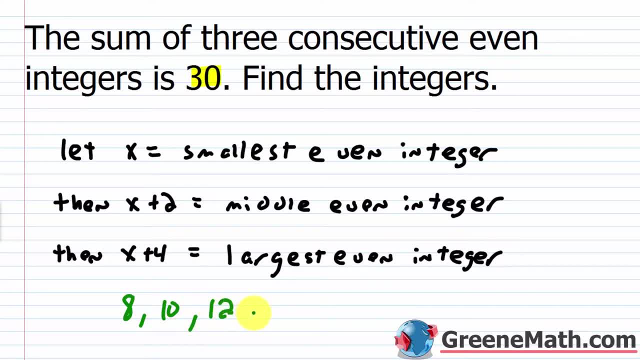 2 to that to get to the largest, and that would be 12. okay, so the integers would be 8, 10 and 12. is that consistent with the problem? 8 plus 10 is 18, and then 18 plus 12 is 30, so we're basically good. 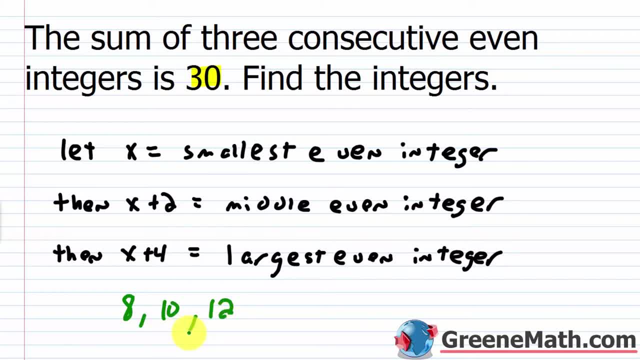 to go right there. all even numbers and they're in a consecutive sequence. so I can just say: find the integers, the integers are, the integers are, we'll say, 8, 10 and 12.. all right, let's take a look at another one, and this one kind of trips students up, so you just want to pay close attention. 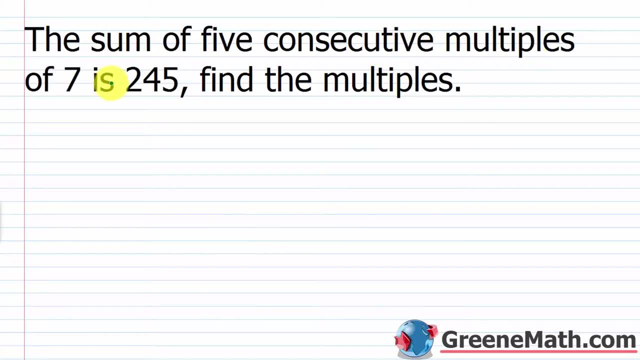 here. so the sum of five consecutive multiples of seven is 245. find the multiples, so the idea here. if you don't remember what a multiple is from pre-algebra, just note that there's multiple definitions of this. but essentially if I take the number seven and I multiply it by an integer, so by 1 or 2, or it could be negative 7 or whatever I want to multiply- 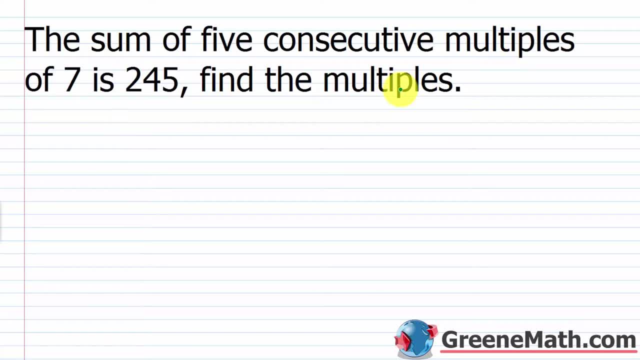 it by as long as it's an integer, the result there is a multiple of 7. so generally in pre-algebra or a lower level algebra course, you kind of restrict this to multiplying the number, which in this case is 7, by whole numbers which are 1 or larger, right? so I would say multiples of 7, you'd have 7 times. 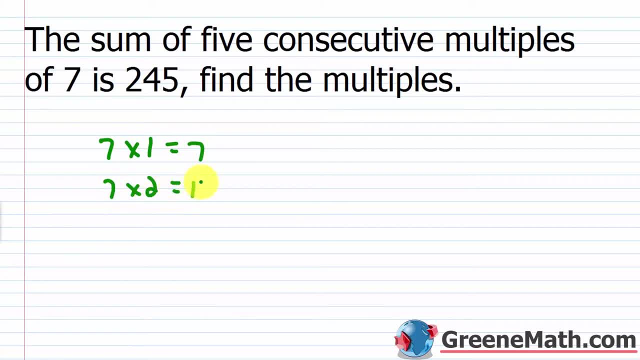 1 is 7, then 7 times 2 is 14, then 7 times 3 is 21, right, so on and so forth. so if I start with 7, then I increase by 7, I get to 14, increased by 7, I get to 21, you know, so on and so forth. so I go 28. 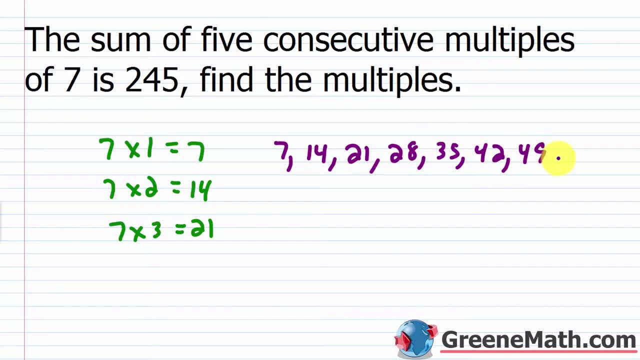 35, 42, 49, right. this would continue forever. now, in this particular case, all we need to understand is that each time I go to the next multiple in the sequence, I just add 7, right? so to get from 7 to 7, I get to 1.. 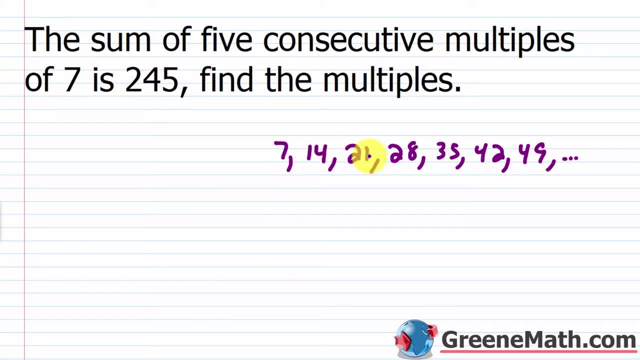 7 to 14, I add 7.. To get from 14 to 21,, I add 7.. So if the sum of 5 consecutive multiples of 7 is 245, the first multiple could just be x. So let's say, let x be. you say this is the smallest, or the 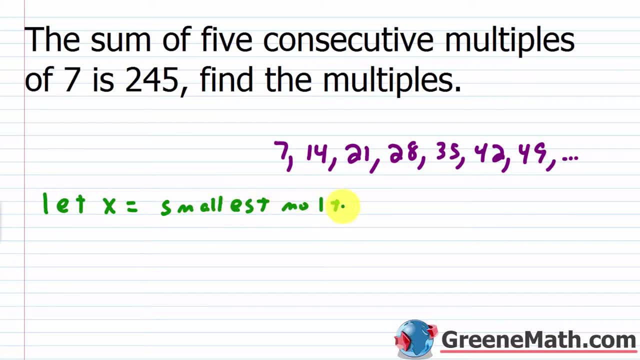 first multiple, You'd say of 7.. So then each time I increase to the next multiple, I'm just going to add 7, right? just to follow this pattern. So we could say then: x plus 7 is what It's the. 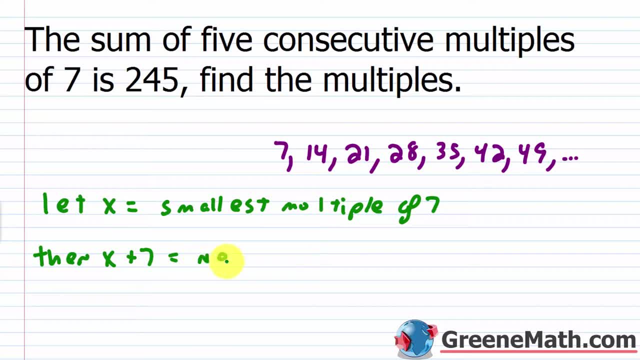 next number in the sequence, So we would say the next largest, Okay, And then, following this pattern, you're just going to keep adding 7.. So we could say then: x plus 7 plus 7 or x plus 14 would be what, It would be, your next largest. 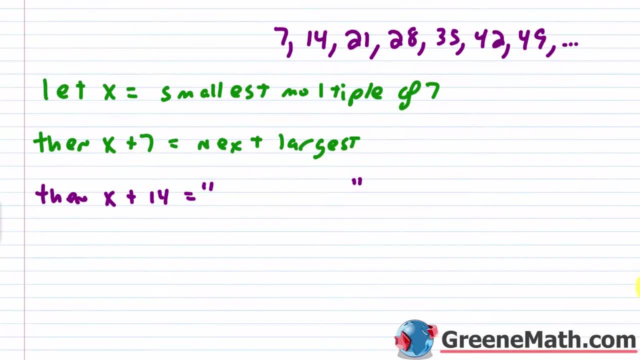 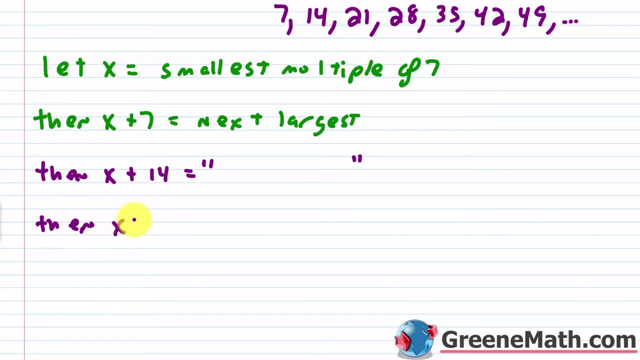 So you just keep going Until you have 5 of these guys. So we would say: then let me make that e better. You'd have x plus 14 plus 7, which is x plus 21, is again the next largest. So you have 1,, 2,, 3,. 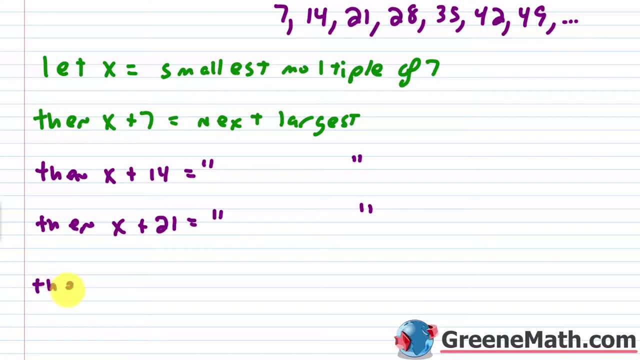 4.. You need one more. So then we could say x plus 28 is now going to be your largest. Let me write that out. So this would be your largest, And I'll be specific here and say multiple Of 7.. Okay, So now, what do we want to do? We're told the sum of these guys is 245. 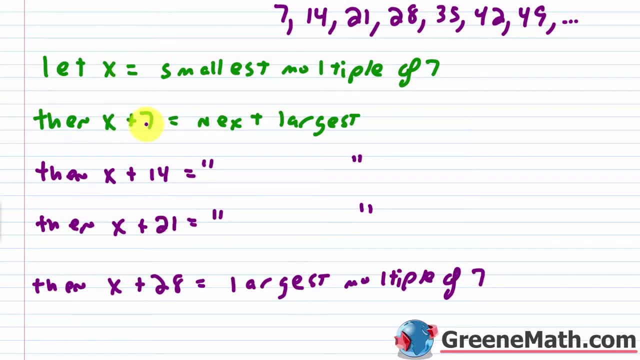 So essentially what I got to do is just take x plus x plus 7 plus x plus 14 plus x plus 21 plus x plus 28 and just set it equal to 245.. Solve that for x and I'll have my answer, Okay. 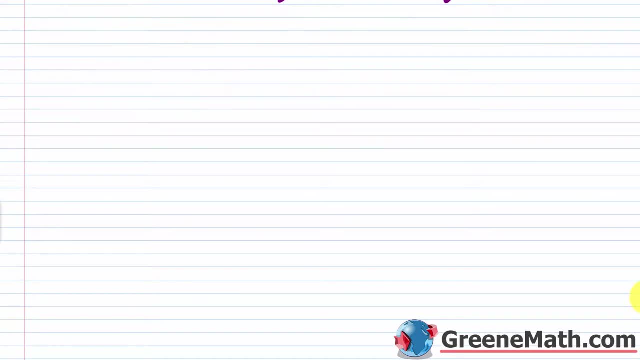 Pretty easy overall. So again I have x plus the next guy in the sequence is x plus 7, plus the next guy in the sequence is x plus 14, plus the next guy is x plus 21.. And then, lastly, 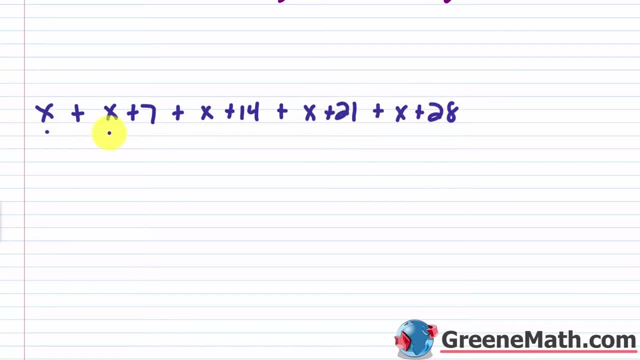 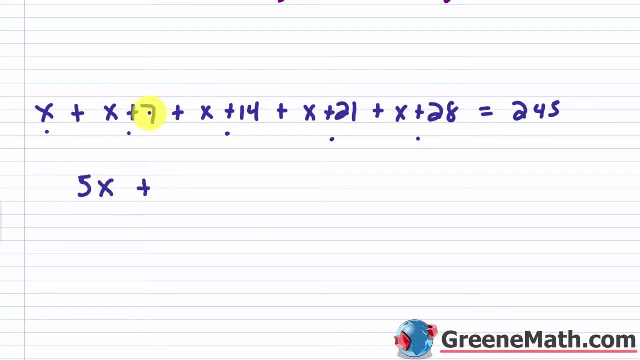 So it's 5x, And then plus, you've got 7 plus 14, plus 21, plus 28,, which is 7.. Okay, So then this equals 245.. If I want to solve this for x, I'm going to subtract 70 away from. 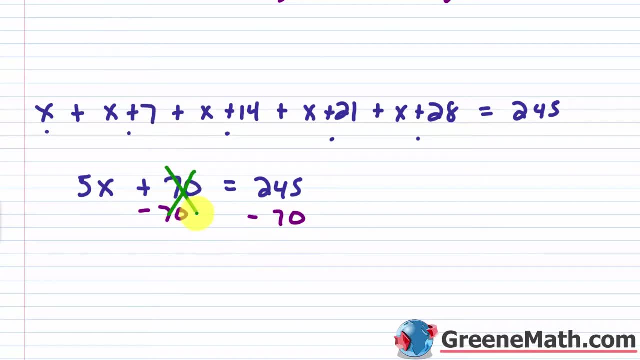 both sides of the equation. So this guy is going to cancel, You'll have: 5x is equal to 245 minus 70 is going to give me 175.. And now what we can do is divide both sides of the equation by 5.. 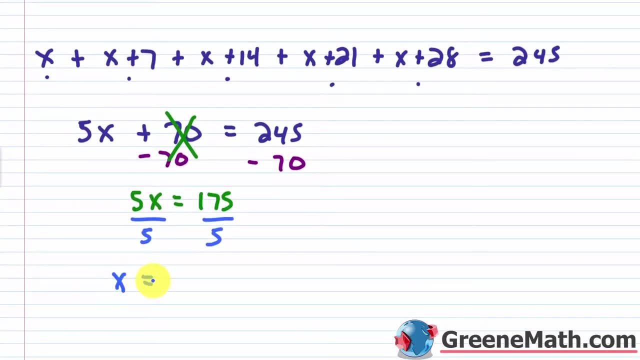 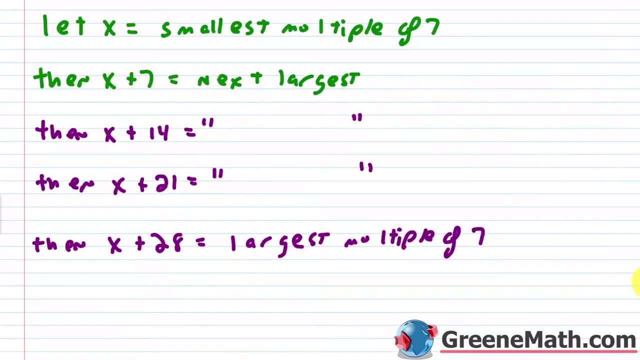 So we can isolate x and we'll get that x is equal to 175. divided by 5 is 35.. Okay, So let's make sense of this. So x is 35.. Let's go back. So we said x was the smallest multiple of 7.. So the next largest would be plus 7.. 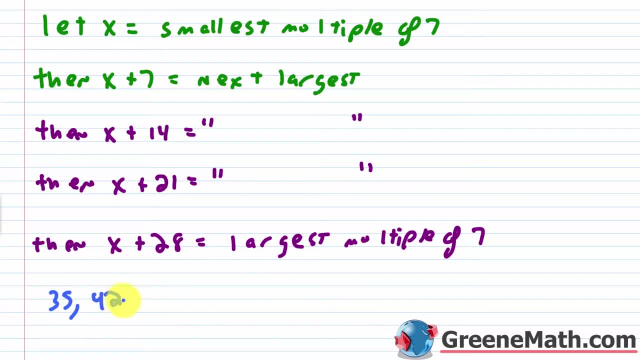 So we would get 35.. Add 7,, you would get 42. Again, keep adding 7.. So you get to 49. You would get to 56. And then, finally, you would get to 63. So these are your multiples of 7.. So let's erase this, All right. So let's say the multiples. 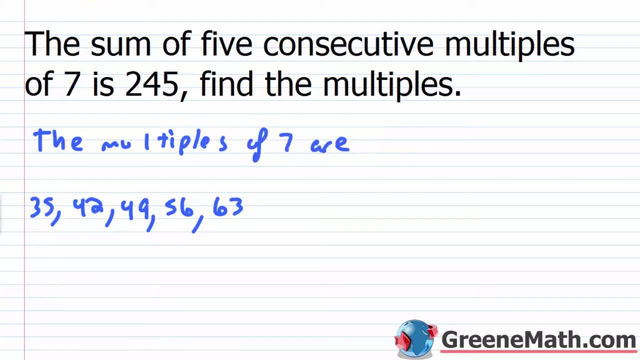 of 7 are again. you have 35,, 35,, 42,, 49,, 56, and 63. Now, if you sum these, you get 245,. right, We know that they're multiples of 7.. That's very easy to see. But if we sum these, do we get 245?? Well, 35 plus. 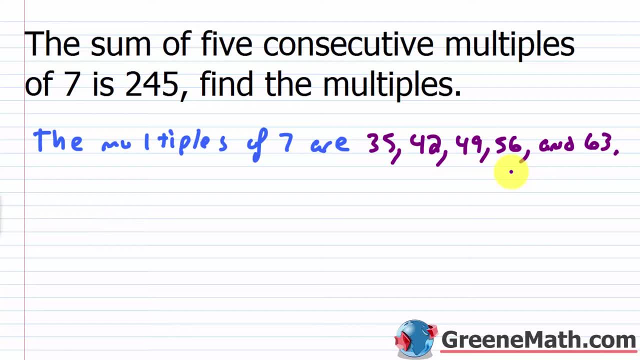 42 is 77. Then if I add 49, I get 126.. Then if I add 56, I get 182. Then finally, if I add 63, I do get 245.. So when I sum these numbers I do get 245.. So my solution here is correct. 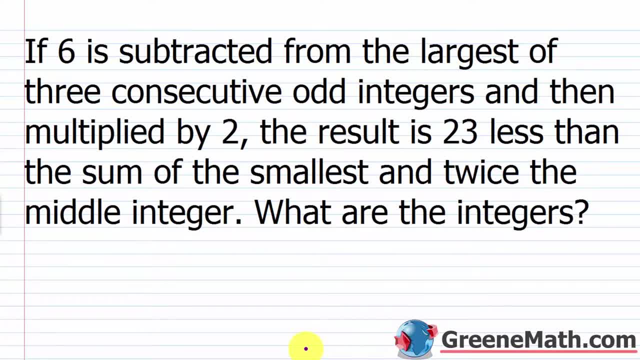 All right, Let's take a look at one more problem. So if 6 is subtracted from the largest of three consecutive odd integers and then multiplied by 2,, the result is 23 less than the sum of the smallest and twice the middle integer. What are the integers? So, when you get a problem like this, 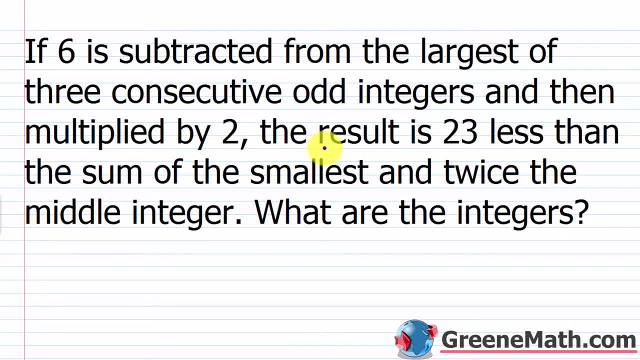 you just have to stop and go step by step, okay, If you try to go too fast you might miss a part. This is one of the ones that's just meant to kind of confuse you. So the first thing is it says consecutive odd integers. Think about the fact that if you have 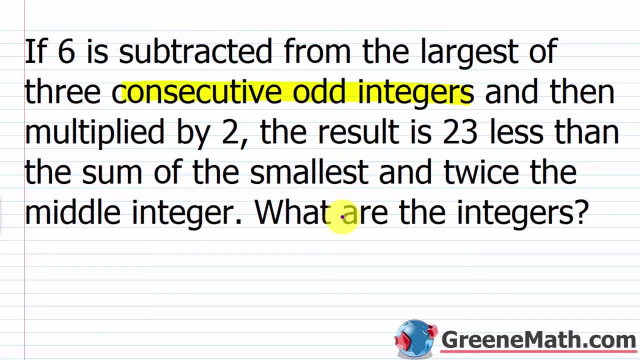 consecutive even integers: it's 2,, 4,, 6,, 8,, 10, right, So on and so forth. Odd integers are integers that are not divisible by 2.. So if they're consecutive, it's going to differ by 2.. 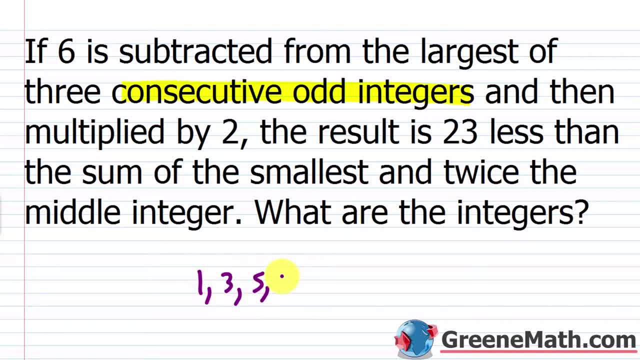 So something like 1,, 3,, 5,, 7, 9.. I'm just increasing by 2 once I start with an odd integer. So to kind of model this: let's let x be the smallest odd integer And then we can say that x plus 2 is going to be the middle one. So this is the middle. 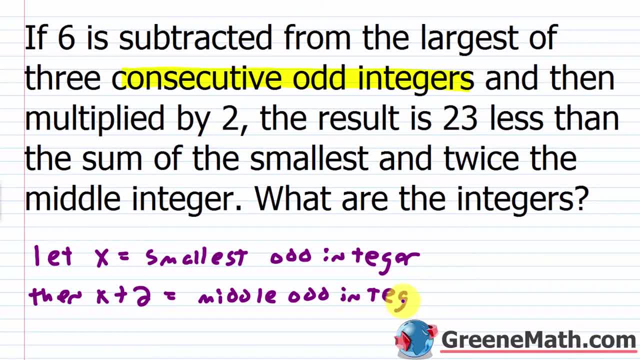 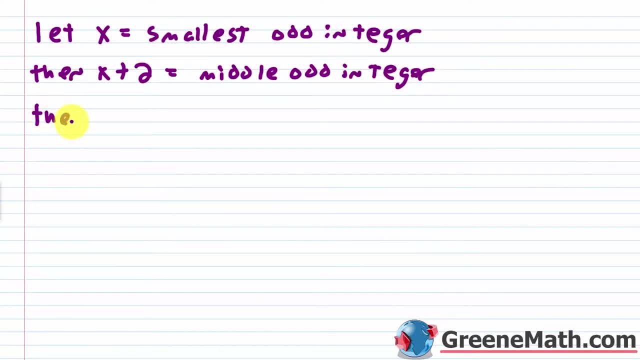 odd integer. I'm going to run out of room, So let's take this to another page, and so we can also say: then x plus two plus two, which would be x plus four, is the largest. okay, the largest odd integer, okay. so now that we've modeled the odd integers, that sequence, let's go. 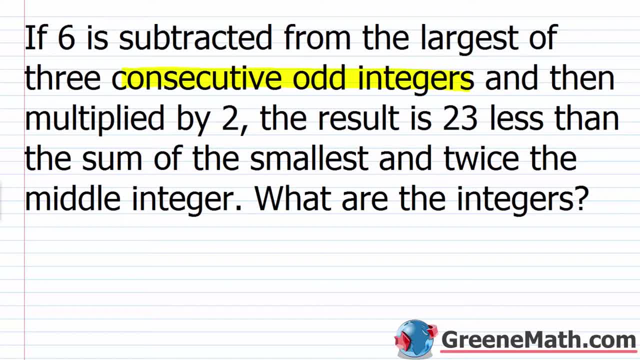 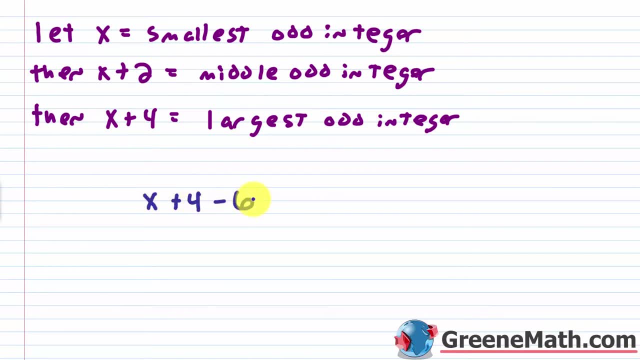 back up and let's think about what it's saying. if six is subtracted from the largest of three consecutive odd integers, okay. so six is subtracted away from the largest. so the largest we said was x plus four. so six subtracted away, we'd have x plus four minus six, which would translate into: 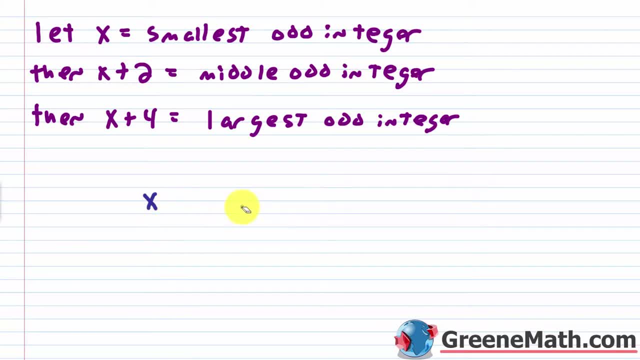 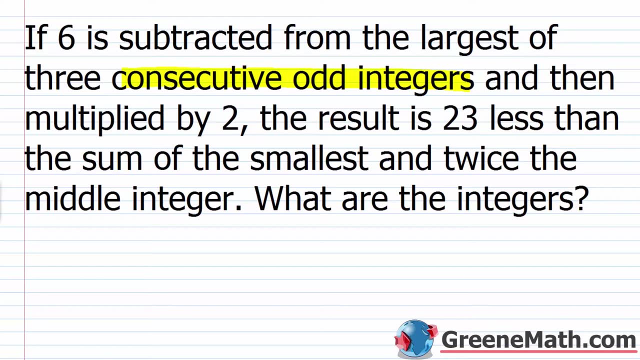 x minus two. okay, so let's just write that, so let's put this as x minus two, and it says again: if six is subtracted away from the largest of three consecutive odd integers, which we've already done- and then okay, so, and then so it's done, after the fact, multiplied by two: 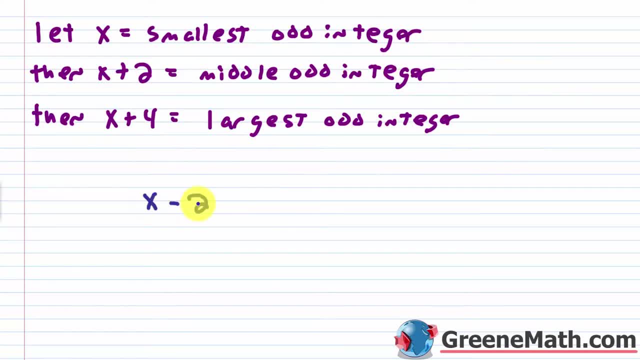 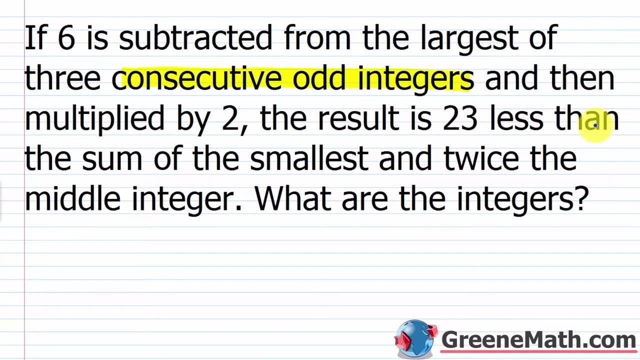 okay. so we're going to multiply this guy by two. this is a quantity. x minus two is a quantity. so i've got to multiply the quantity x minus two by two. then it says the result is: so that always means equals. so again, the result is you have 23 less than the sum of the smallest and 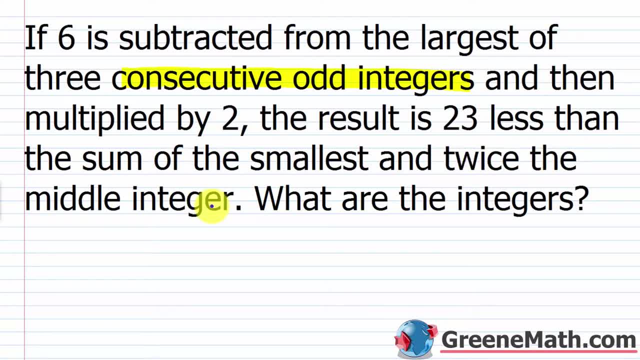 twice the middle integer. okay, so this is a lot to unpack. so we know that we're subtracting 23 away from something because it says the result is 23 less than so let's go back and do that again. so we're going to multiply this guy by two. so we're going to 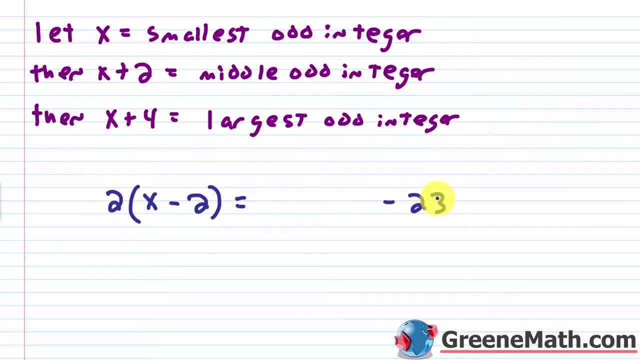 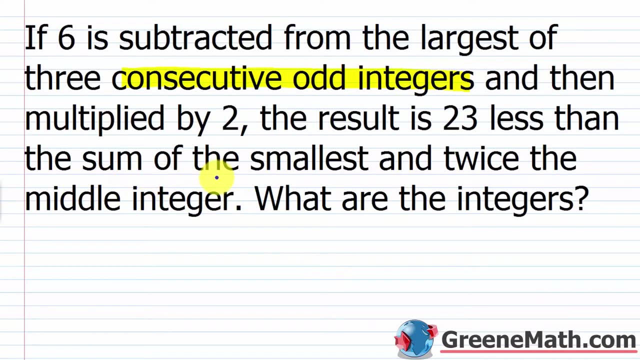 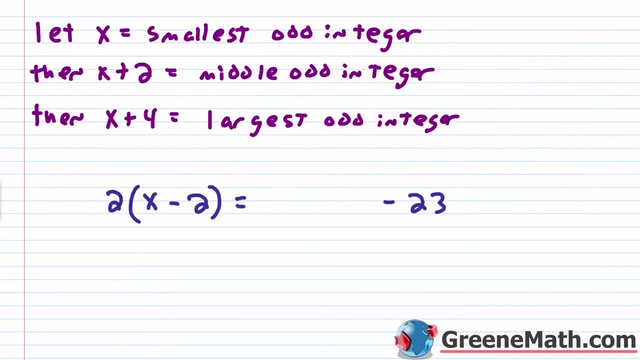 go back here. i'm just going to put minus 23 out here because we're going to do something and then we're going to subtract 23 away. now it says the sum of the smallest, which we said, was x and twice the middle integer. the smallest, which we said, was x and twice the middle integer we want. 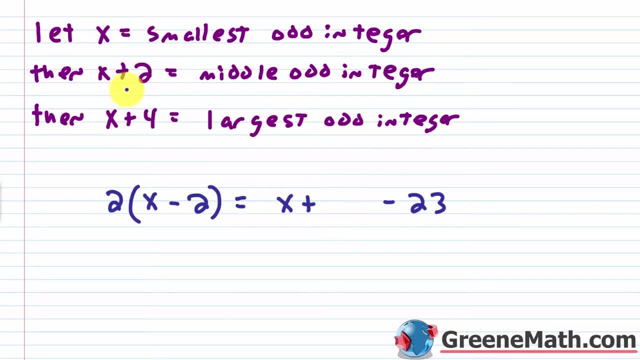 that sum, the middle integer is x plus two. so again, i've got to use some parentheses here, so we kind of drag this over. so two times this quantity x plus two, okay, so let's read through this again and make sure we understand where this came from. so again, if six is subtracted from the largest of three consecutive, 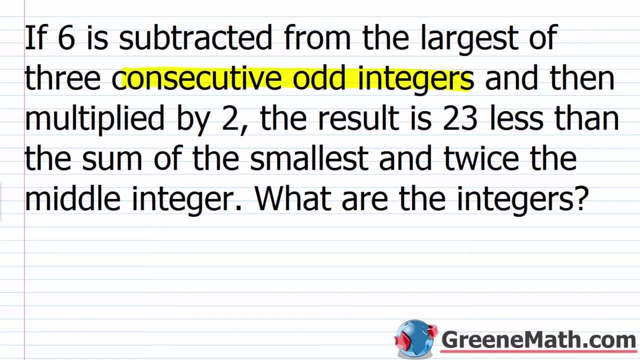 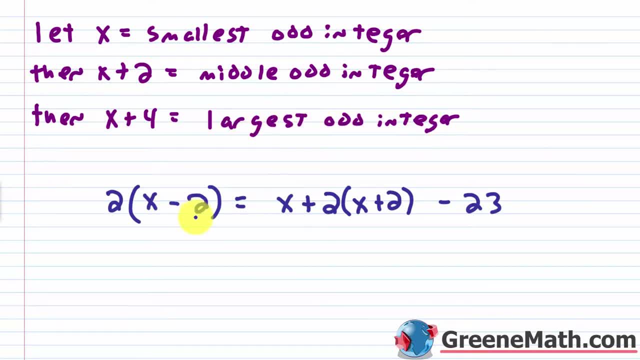 odd integers and then multiplied by two. so essentially we started with the x plus four is the largest odd integer. we subtracted away six. that's how we got x minus two, and then we multiplied by two to get the left side. then it tells us the result is: 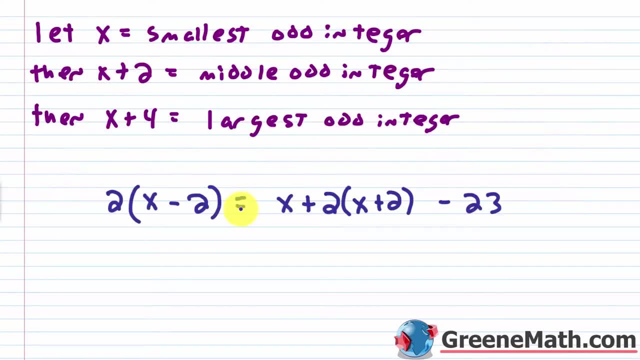 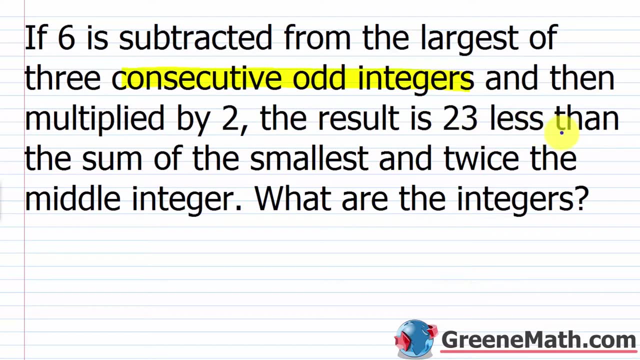 so that's where we got our equal sign from. if you say the result is, you're basically saying is equal to. so on the right side we have that it's 23 less than the sum of the smallest, which are represented with x and twice the middle integer. now the middle integer is x plus two, so twice the middle integer. 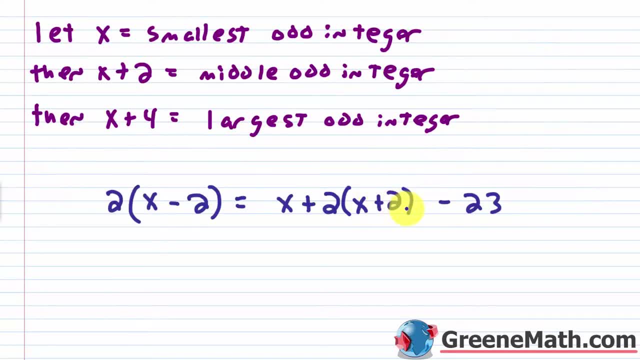 is two times the quantity x plus two. so that's where you got this: from the sum of the smallest integer, which is x, and twice the middle integer, which is x plus two. so that's where you got this middle integer, which is two times x plus two. so we sum those two together and then we need to. 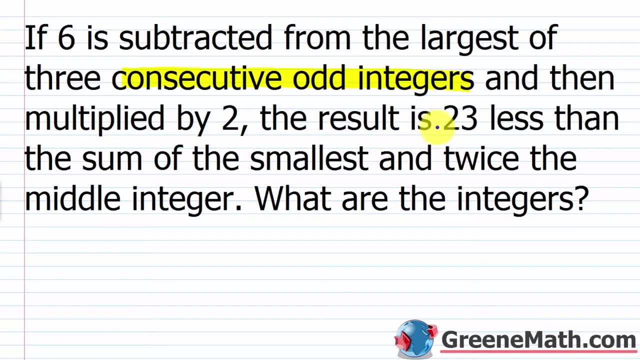 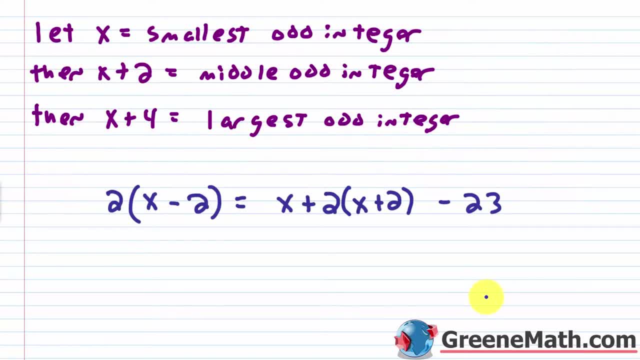 subtract 23 away from that, because it says the result is 23 less than okay. so now that we have this set up again, these are kind of a pain to get to this point, but once you have it it's pretty easy. you're solving an equation. so clean up: on the left: two times x is 2x, then minus two times two. 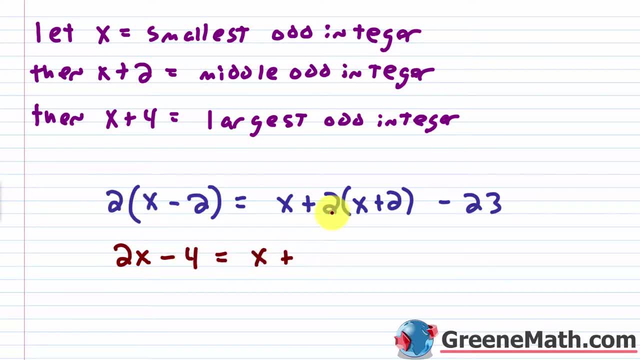 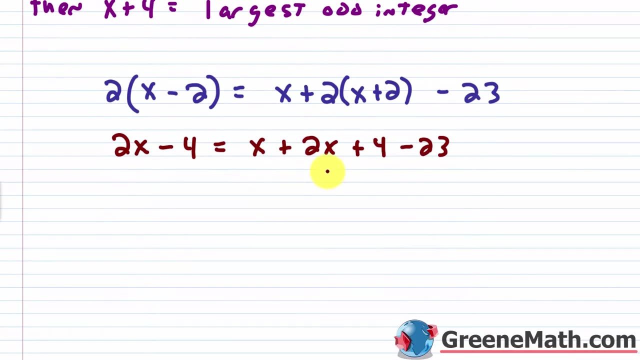 is four is equals. you have x plus two times x is 2x, and then plus two times two is four, and then minus 23. okay, so let's think about this on the left side, nothing i can do on the right side. i can take x and add to 2x. that would give me 3x, and then 4 minus 23 is negative. 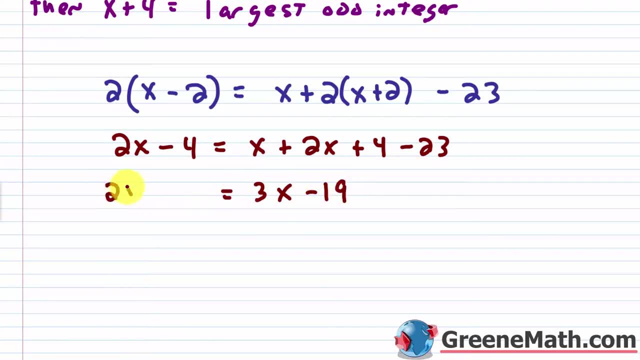 19 again over here. i'm just going to write 2x minus 4. nothing's going to change. i'm going to subtract 3x away from each side of the equation. i'm going to add 4 to each side of the equation. so what's going to happen is: 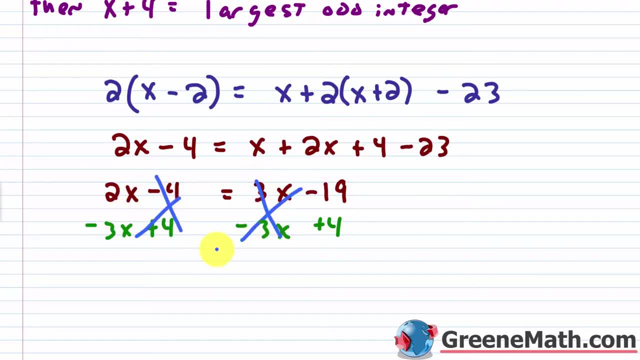 this guy right here is going to cancel, and this guy is going to cancel. 2x minus 3x is negative x and this equals negative 19 plus 4 is going to be negative 15. now to get x by itself. i can multiply both sides by negative 1 or divide both sides by negative 1, makes no difference, you're going to get. 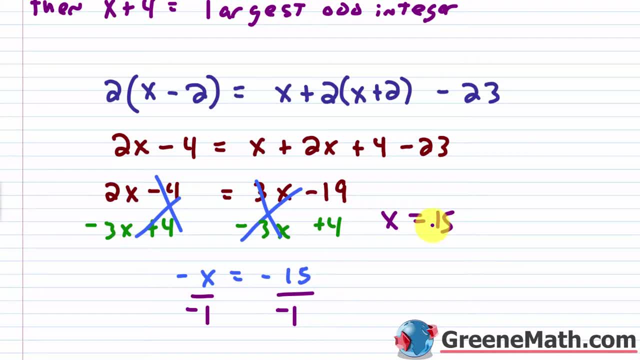 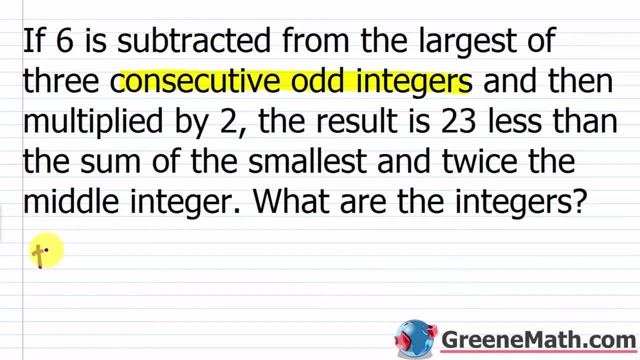 that x is equal to 15. okay, so let's erase all this. so remember, x was the smallest odd integer. so if we go back up, what are the integers? we'll say the integers are- let me make the e better- so we have 15, the next one would be 17, right, if it's consecutive odd integers and then the last. 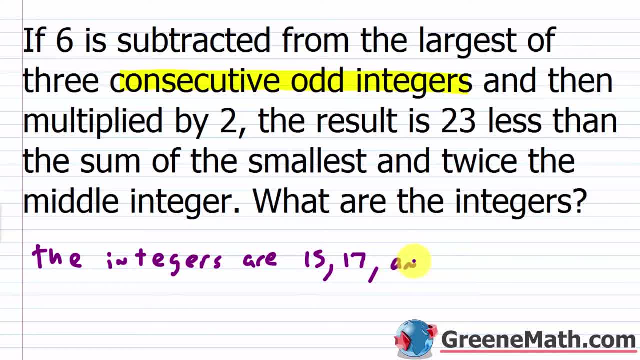 one would be 19. let me put: and 19 here and 19, okay. does this make mathematical sense? normally with these problems you just get a straight sum, so it's very easy to check, but this one you have to do a little bit of work. so if 6 is subtracted from the largest, 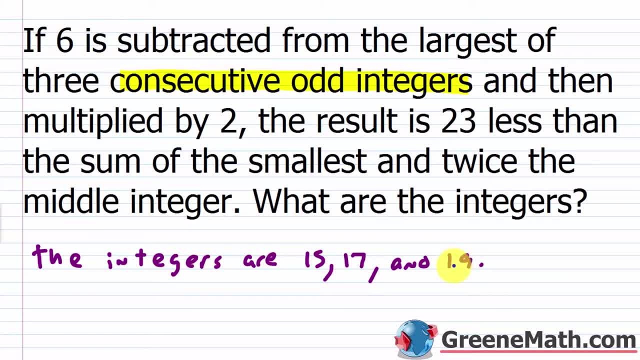 of three consecutive odd integers, so the largest is 19. if i take 6 away, i'd have 13.. then it tells us, and then, multiplied by 2.. so 13 multiplied by 2 is 26.. so this is 26 and it says the result is: so this is equal to: so we have 23 less than the sum of the. 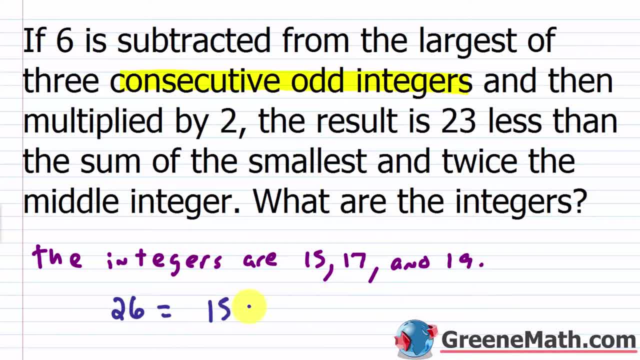 smallest. so the smallest is what? it's 15 plus twice the middle integer. the middle integer is 17.. so if i take 2 and multiply it by 17, i get 34.. and again it's 23 less than this. so i'm going to subtract 23 away from this sum. so 15 plus 34. 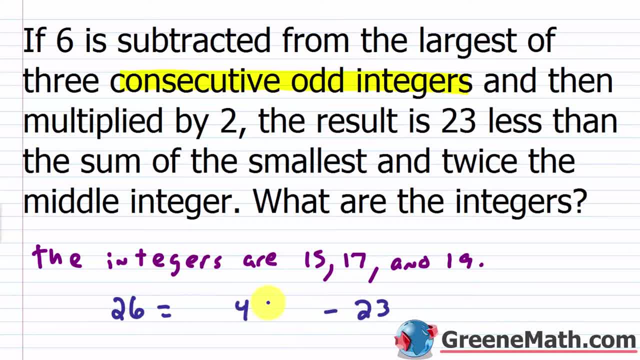 is 49. so you would have 49 minus 23, which is 26. right, you end up with the same value on the left as you do on the right. so we've successfully completed checking this guy. right. we can say our answer is correct. the integers are going to be 15, 17 and 19.. in this lesson we want to review: 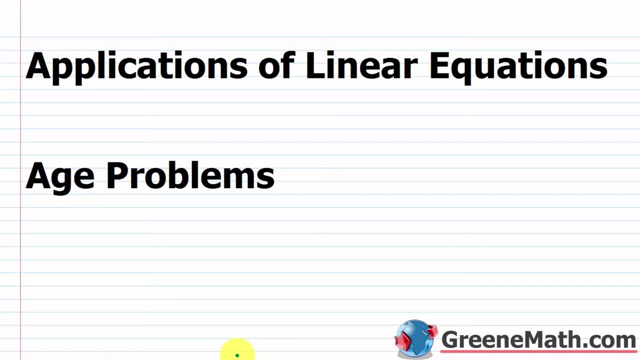 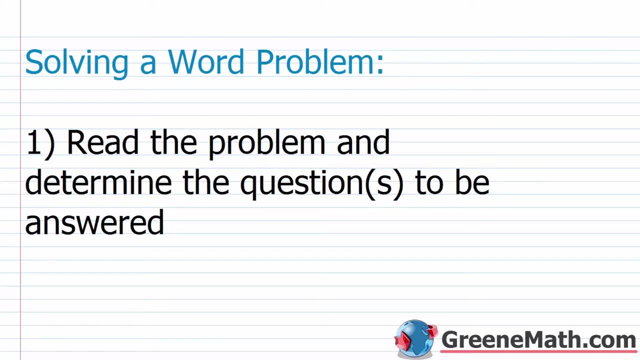 applications of linear equations and look at some examples of age problems. so again, whenever we're working with an application problem that involves a linear equation in one variable, we can use our little six step procedure. so for solving a word problem we have that. we want to read the problem and again determine the question or questions to be. 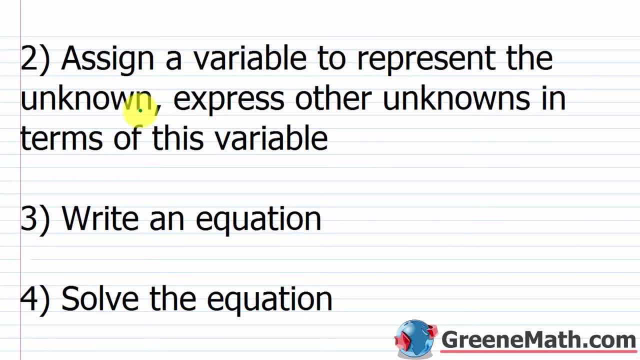 answered, then we want to assign a variable to represent the unknown with these problems. we're going to express other unknowns in terms of this variable, then we're going to write an equation- this is based on the situation given to us in our problem- and then we're going to solve. 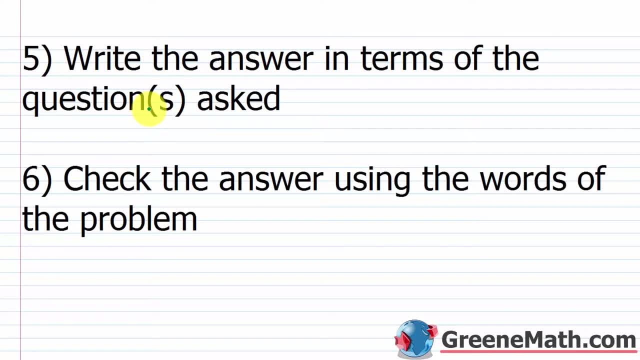 the equation, then we're going to write the answer in terms of the question or again questions asked, and then, lastly, we're going to check the answer using the words of the problem. we always want to make sure the answer is reasonable. so for age, word problems, this is: 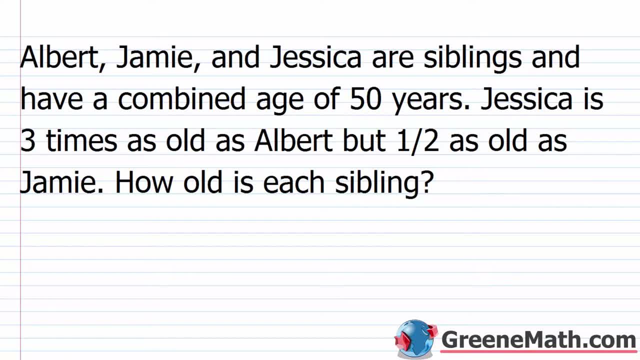 another extremely common type of word problem. in algebra, this type of problem is generally going to give us the sum of the ages of family members, friends or some group of associated people, and then we'll start with that group and why. we're going to make that pretty simple to understand. 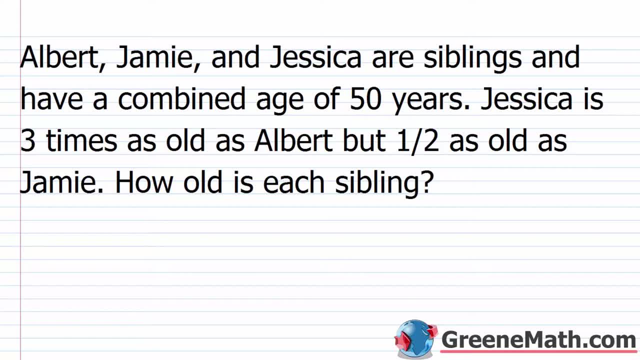 going to ask us to find their individual ages. now, it doesn't always set up this way, but that's the most common scenario. all right, so let's take a look at the first example. so we have that albert, jamie and jessica are siblings and have a combined age of 50 years, so jessica is three times as old. 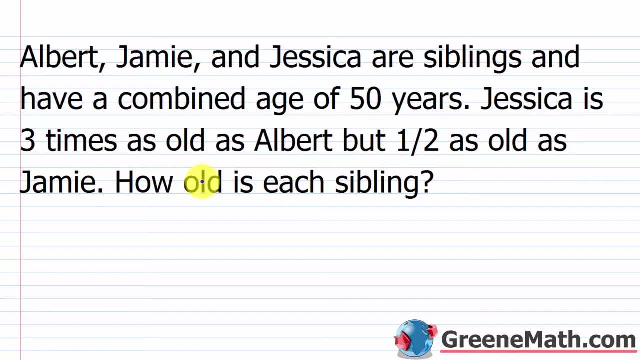 as albert, but half as old as jamie. how old is each sibling? so this is our main question here, right, how old is each sibling? so we need to find out how old is jamie, how old is albert and how old is jessica. okay, so we are only given the fact that they have a combined age of 50 years and we've 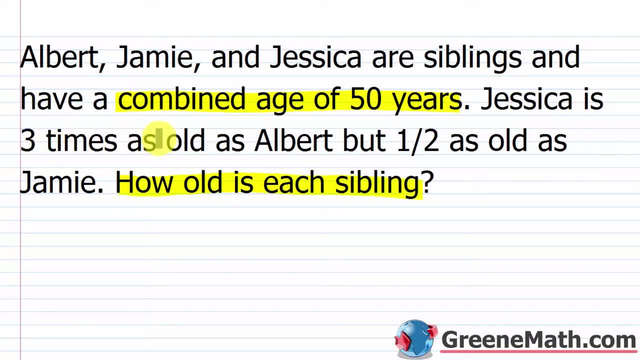 given some comparisons here. it tells us jessica is three times as old as albert, but half as old as jamie. so to solve this- we know what we're trying to find- let's assign a variable. let's let x be equal to. since jessica is involved in both comparisons, let's let x be equal to jessica's age. 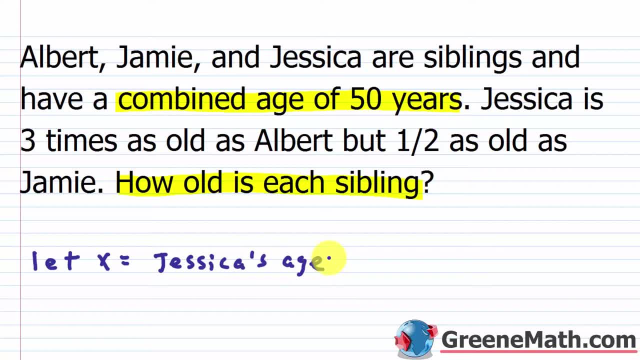 now, what can we say about albert's age? and what can we say about jamie's age? we're told here, specifically, that jessica is three times as old as albert. so if jessica is three times as old as albert, that means albert is one-third the age of jessica. so then, x which? 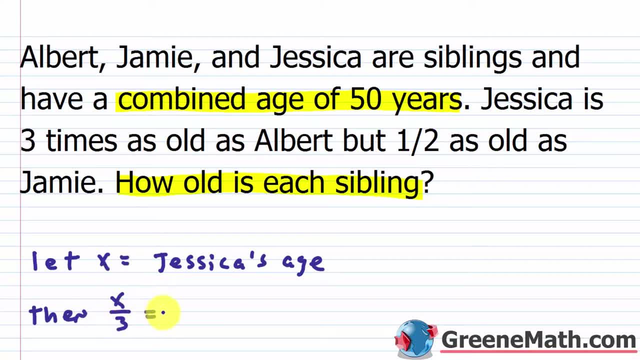 is jessica's age. over three would be equal to albert's age. now we're also told that she's half as old as jamie. so jessica is half the age of jamie. that means jamie is two times as old as jessica. so i can say then two times x. again, x is jessica's. 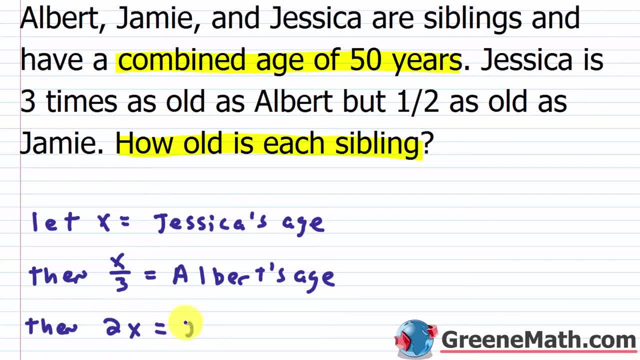 age. so two times that would be jamie's age. okay, so this is jamie's age. now we have everything set up here, we have everything modeled. how do we get an equation going so we can get a solution? well, essentially we have a combined age of 50 years, so i can take jessica's age, which is x. 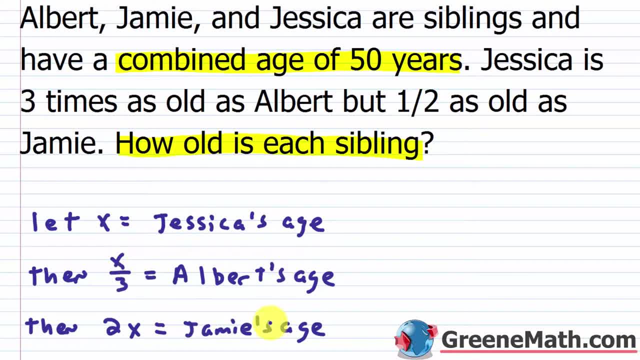 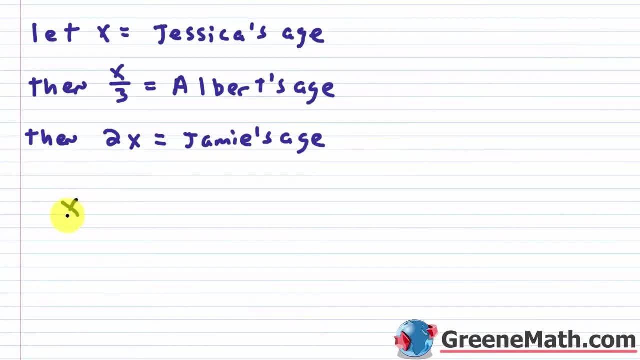 add that to albert's age, which is x over 3, and add that to jamie's age, which is 2x, and i can set that equal to 50. right, their combined age. so let's go ahead and set that up so we would have x plus x over 3, plus 2x is equal to 50.. what i can do to clear this? 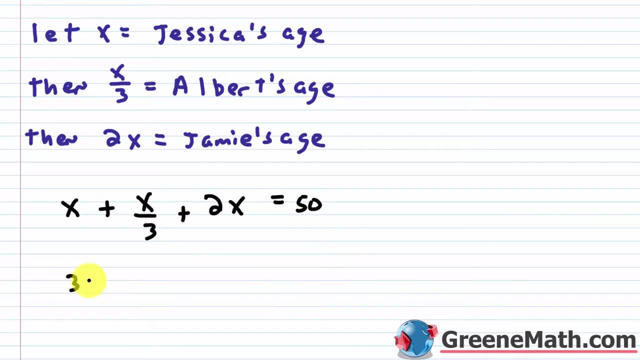 denominator is: multiply everything by 3, so i would have 3x plus. if i multiply x over 3 by 3, i would have x, and then plus 2x times 3 is 6x and this equals 15 times 3 is 150.. okay, so basically i 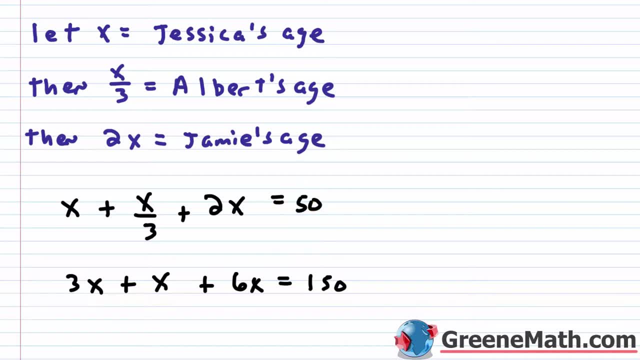 just multiplied both sides of the equation by 3 again, so i can clear this denominator here. so now 3x plus x is 4x, plus 6x is 10x. so you get 10x is equal to 150.. let's divide. 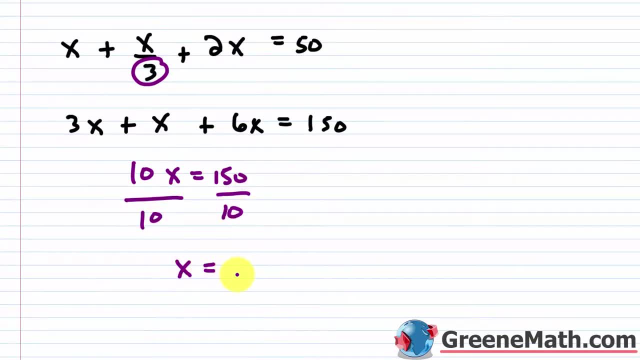 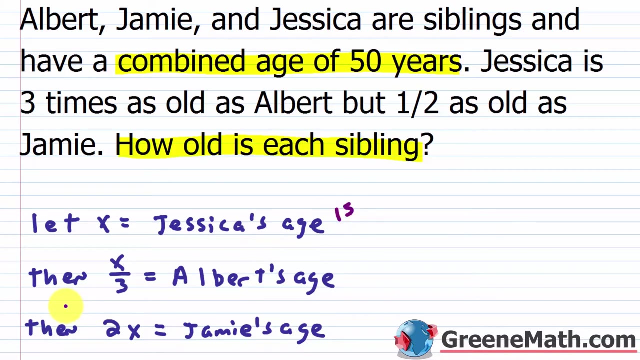 both sides of the equation by 10. we get that x is equal to 50. so if x was jessica's age, that tells me jessica is 15 years old. so let's go back up. so again, x is 15, so jessica is 15. and then we know: 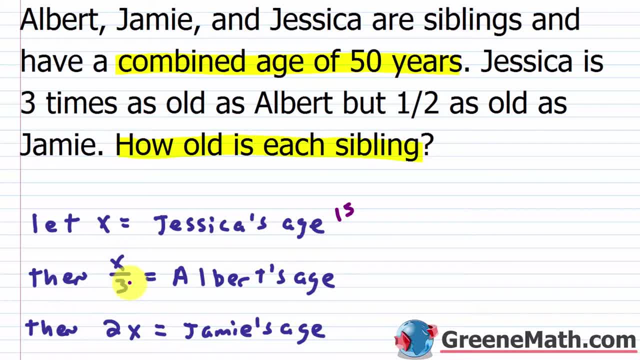 that albert is a third of the age of jessica, right, it's 15 over 3, which is 5.. and then jamie is twice the age of jessica, so it's 2 times 15 or 30.. so to answer this question, we can say that jessica 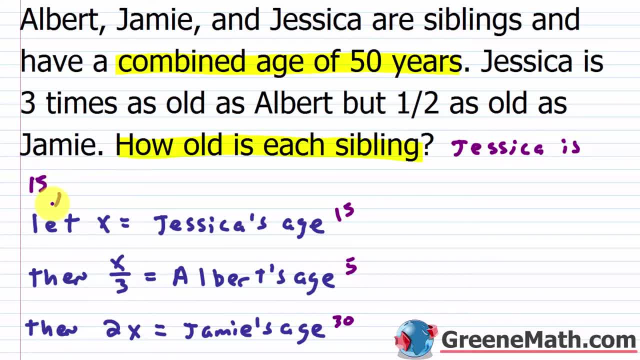 is 15, and then when we do the sum, we'll say jessica is 15.. and then we'll take the upper number and we'll give this a zero comma. we'll say albert is five and we'll say jamie is 30.. okay, now you can check this to make sure it makes sense. so again, albert, jamie and jessica. 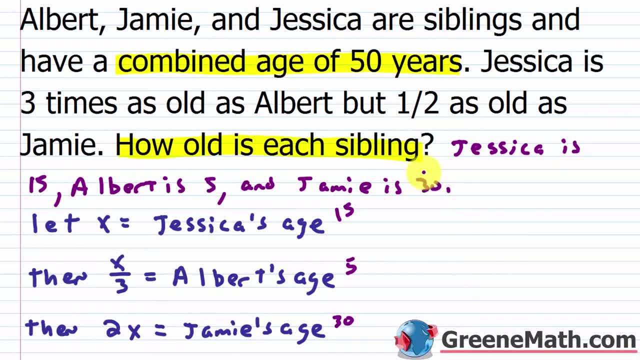 are siblings and have a combined age of 50 years. so is 15 plus 5 plus 30, 50. yes, 15 plus times as old as albert. so jessica is 15, albert is 5, 15 is 5 times 3.. so we're good to go there. 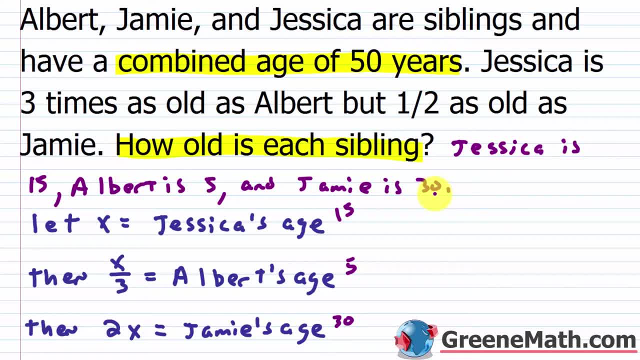 and then half as old as jamie. 30 is jamie's age. again, jessica is 15. 15 is half of 30, so you're good to go there. so this checks out: jessica again is 15, albert is 5 and jamie is 30.. all right, let's. 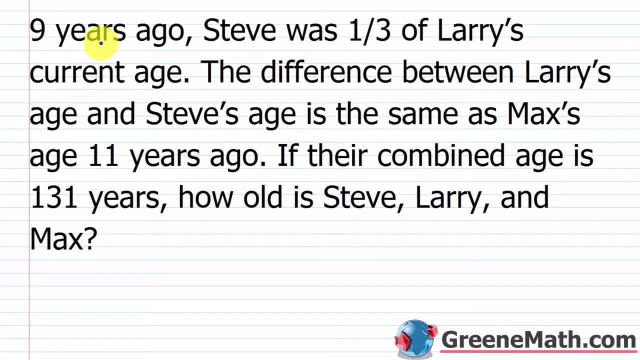 take a look at one that's a little bit more challenging. so we have that. nine years ago, steve was one third of larry's current age. the difference between larry's age and steve's age is the same as max's age 11 years ago. if their combined age is 131 years, how old is steve larry? 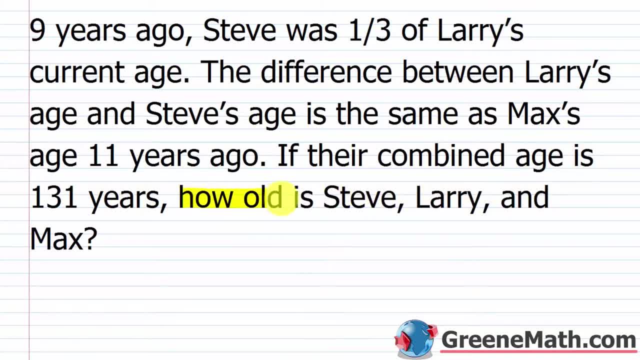 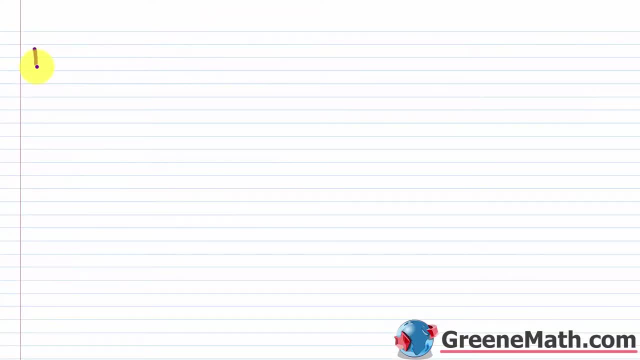 and max. so we want to find out how old is steve, larry and again max. so i'm going to jump right in and let a variable like x represent the current age of larry. okay, so let me go down here. so we have lots of room. so let's let x've got lots of room, so let's let x. you can see some different. 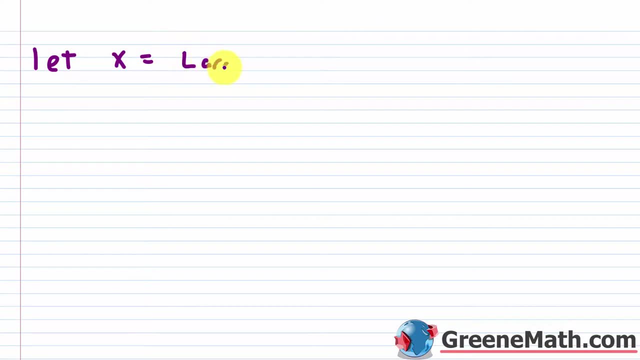 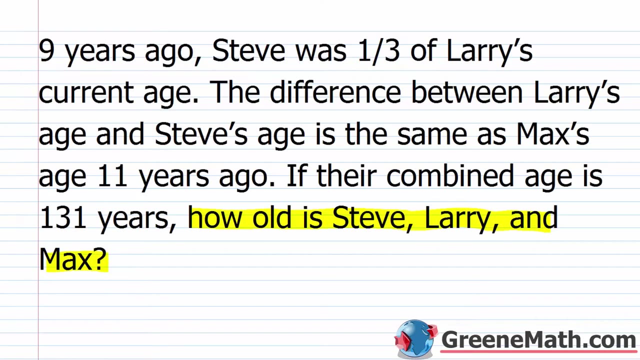 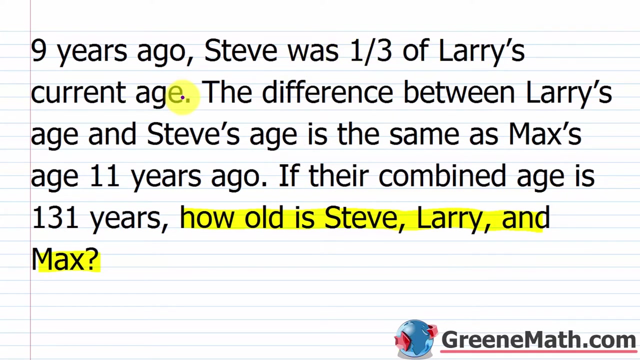 numbers. a gets in other numbers here in the left-hand corner: individuals. this explains how be equal to Larry's current age. Now what can we say about Steve? Well, it says specifically that Steve was one-third of Larry's current age nine years ago. okay, So I have to think about the. 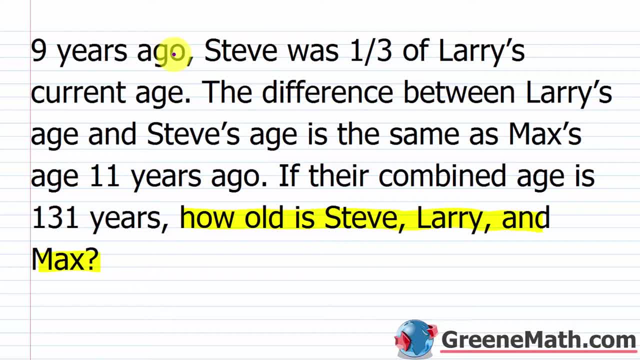 fact that one-third of Larry's current age is one-third X, but this is Steve's age nine years ago. So I've got to add nine on top of that to get back to our present day in time. So for Steve's, 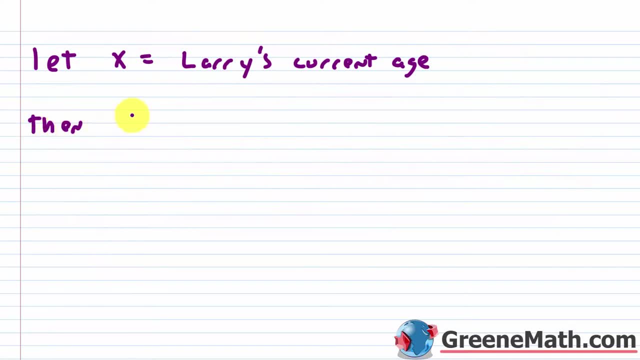 age. we could say then one-third X, so one-third of Larry's current age. then plus nine, right? Because this part right here is Steve's age nine years ago. So I've got to add nine to that to get his current age. So this would be Steve's current. 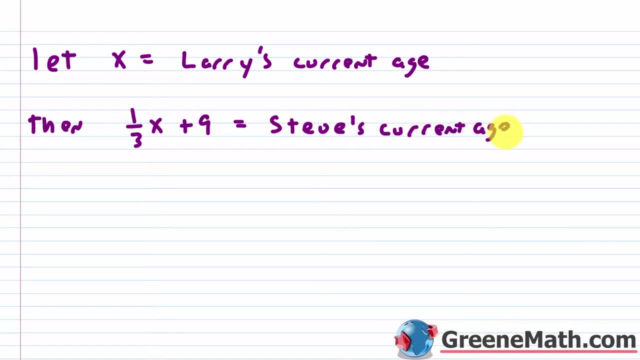 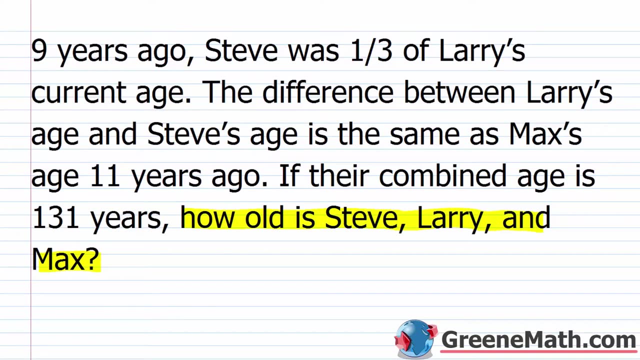 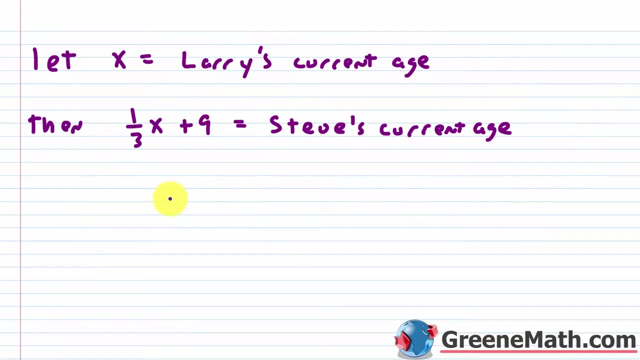 age. Now let's think about Max now. So it tells us that the difference between Larry's age and Steve's age is the same as Max's age 11 years ago. okay, So the difference between Larry's current age, which is X, and Steve's current age, which, again, is this one-third X plus nine. 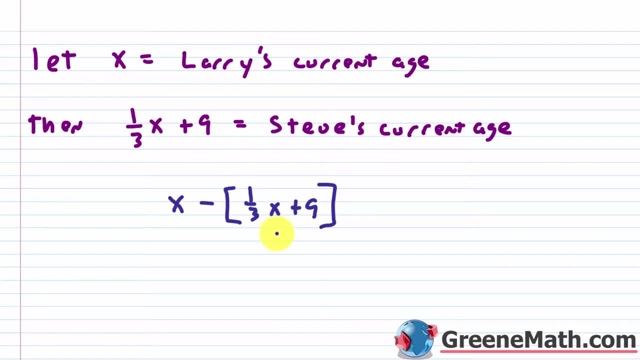 Notice that I'm using brackets here because I've got to subtract the whole thing away. This is the same as Max's age 11 years ago, So to get his current age, I've got to add 11 to this amount. okay, So this would be then. 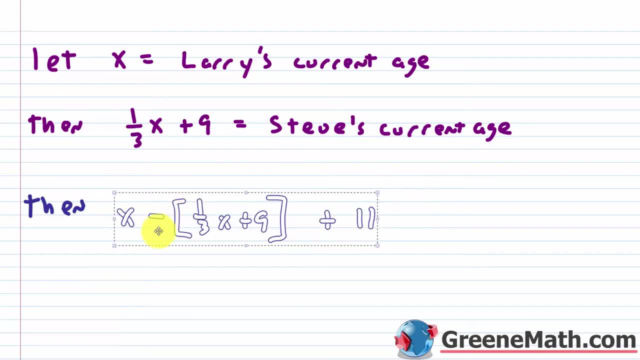 we'll say: this guy right here, let me just kind of slide this down. we'll say: this is Max's current age. okay, And I might run out of room, so let me make that a little bit better. So Max's. 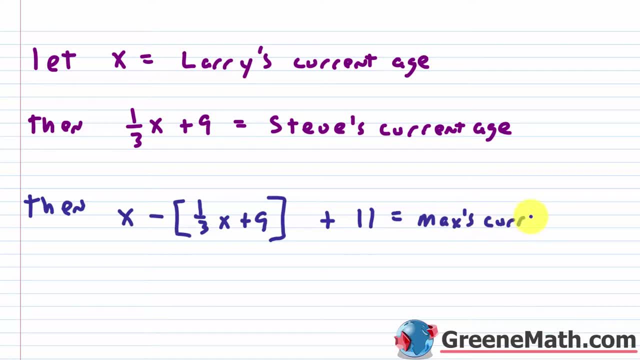 current age. okay, So now it also tells us in the problem that their combined age is 131 years. So essentially, just like I did in the last problem, I can sum the ages and set it to 131,. 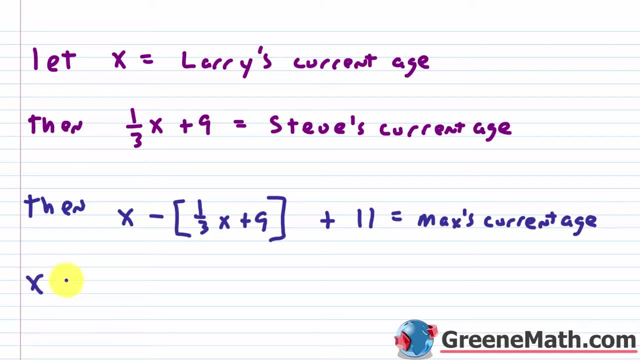 and I'll get a solution. So I would have X, which is Larry's age, plus one-third X plus nine, which is Steve's current age, and then plus you have X, minus- you have this inside of brackets- one-third X. 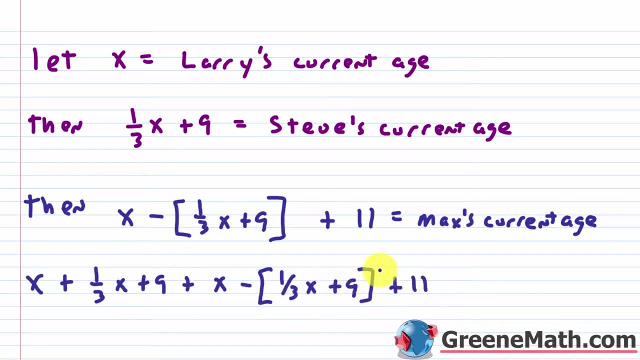 plus nine, and then plus 11,, which again is Max's current age. This is all equal to 131.. So let me copy this. We're going to go down to a fresh sheet of paper, So let me just kind of clean this up. 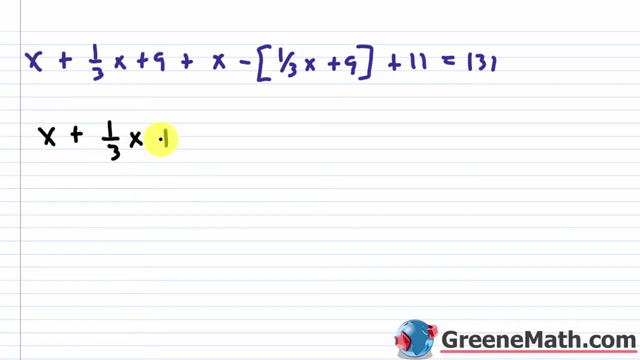 We have X plus one-third X plus nine plus X. Use your distributive property here, So you'll have minus one-third X, then minus nine, then plus 11, and this equals 131.. Now, what do you notice here? 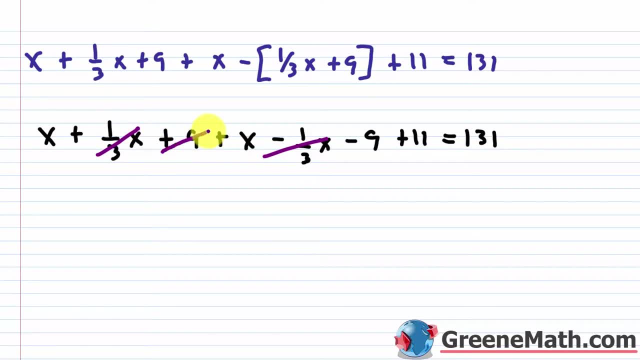 One-third X minus a third X, that's gone. Nine minus nine: that's gone. X plus X is 2X, and then plus 11 equals 131.. If I subtract 11 away from each side of the equation, I'm going to get that 2X is equal to 120.. 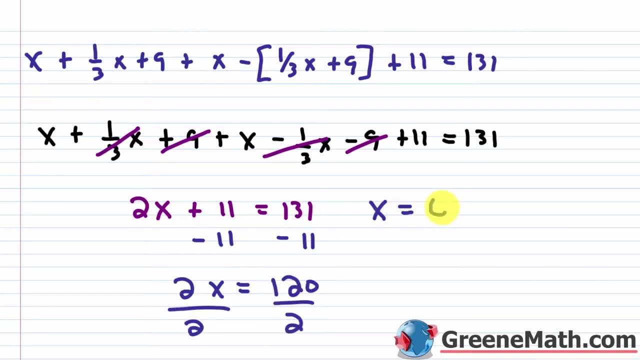 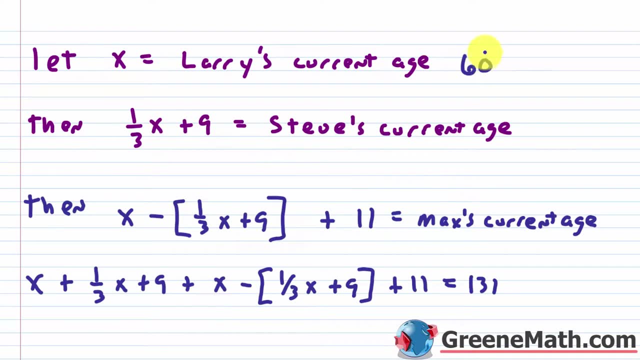 Divide both sides of the equation by two and we're going to get that X is equal to 60. So, remember, X was Larry's current age, So Larry is 60. So Larry is 60.. We can say that, Steve, again, he's one-third times 60,, which is 20, plus nine, which is 29.. 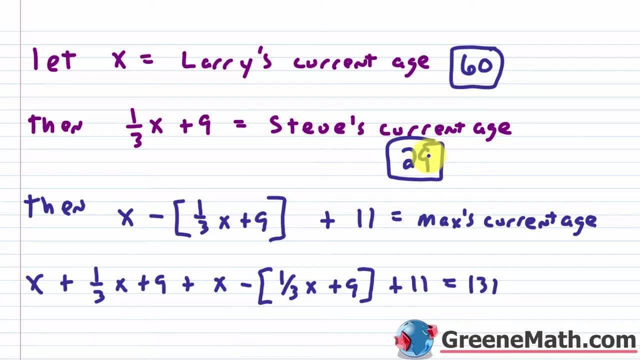 And then for Max, we basically have 60 minus 29,, which is 31,, and then plus 11,, which is 42. So his is going to be 42.. All right, let's go back up. So let's write our answer here. 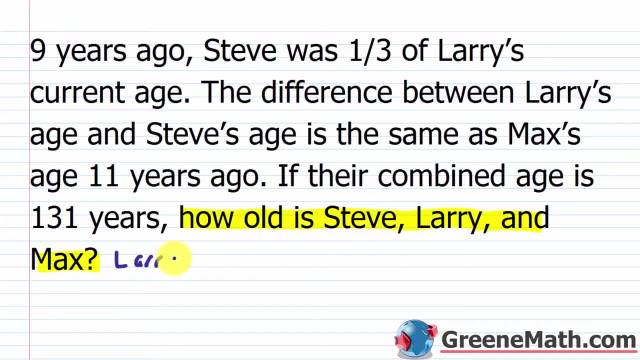 Again, Larry is 60. So Larry is 60. Then we can say: Steve, Steve is 29, and Max is 42. Again we can check this. So it says nine years ago Steve was one-third of Larry's current age. 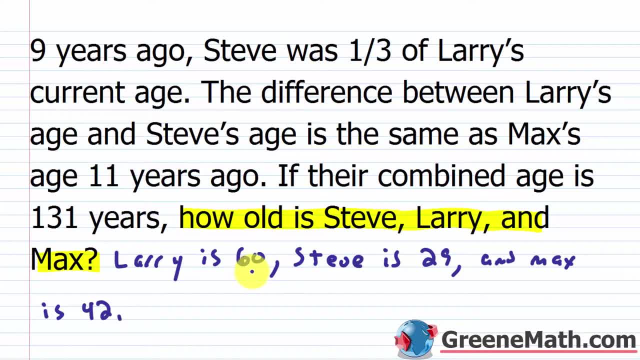 So if we go nine years ago, Larry's current age is 60.. So a third of that is 20,. okay, So Steve is 29.. Nine years ago he would have been 20, and that is one-third of Larry's current age, which again is 60.. 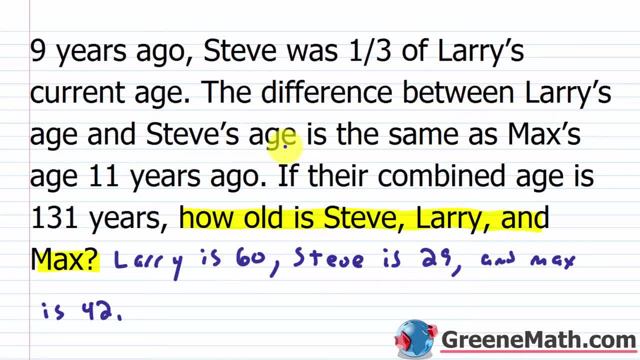 Then it says The difference between Larry's age and Steve's age, the difference between 60 and 29,, is 31.. And it says This is the same as Max's age 11 years ago. Well, again, Max is 42.. 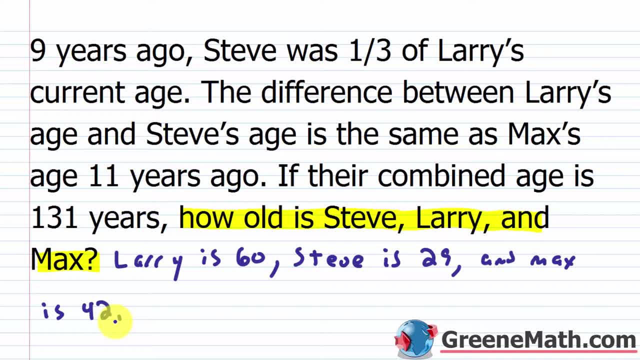 11 years ago he would have been 31.. So that checks out as well. Then it says their combined age is 131. Well, 60 plus 29 is 89. Then if I add 42, I do get 131. 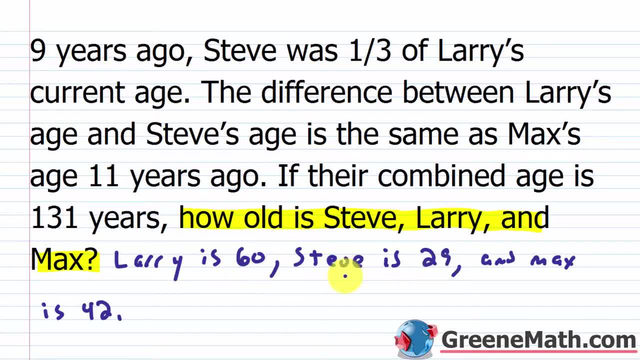 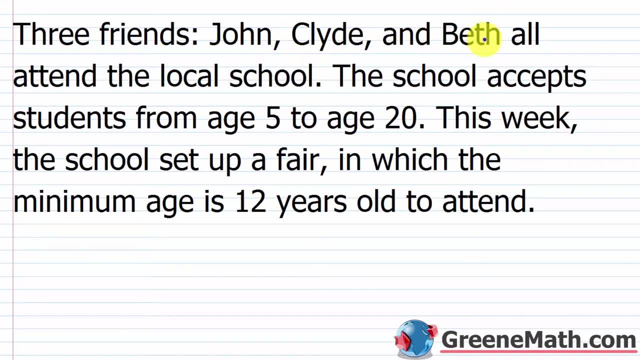 So everything checks out here. We can say that Larry is 60.. Steve is 29.. And again Max is 42.. All right, let's take a look at one more. So we have three friends, John, Clyde and Beth. all attend the local school. 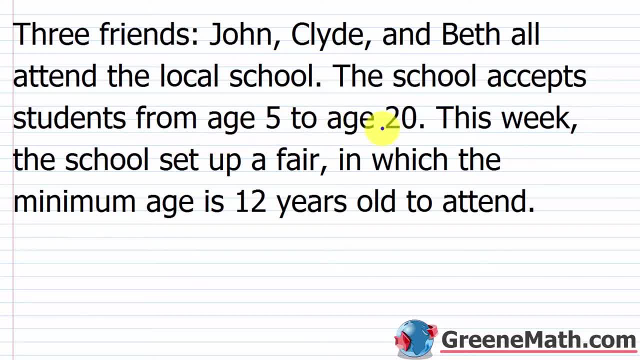 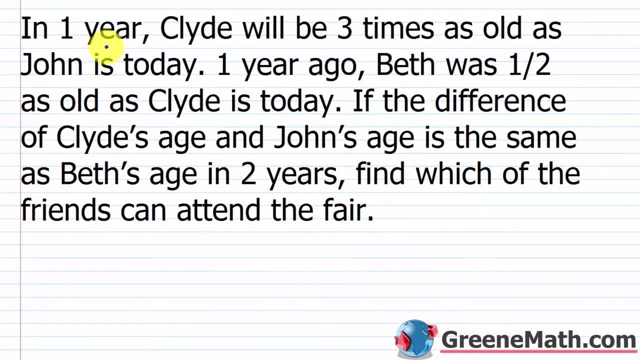 The school accepts students from age 5 to age 20.. This week the school set up a fair in which the minimum age is 12 years old to attend. So now we're told, in one year Clyde will be three times as old as John is today. 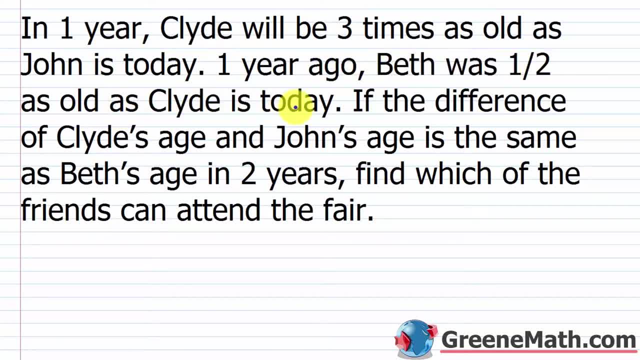 And then one year ago, Beth was one-half as old as Clyde is today. If the difference of Clyde's age and John's age is the same as Beth's age in two years, find which of the friends can attend the fair, okay. 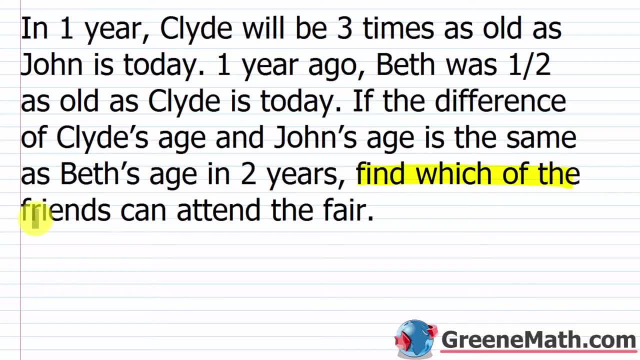 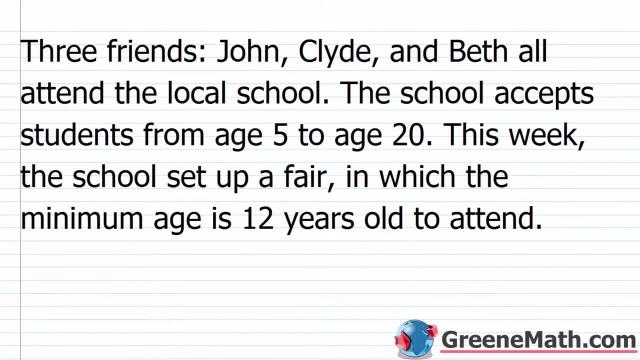 So we're trying to find which of the friends so we have- Beth, Clyde and John- can attend the fair. Remember, it tells us that you can only attend the fair if you're at least 12 years old, right? 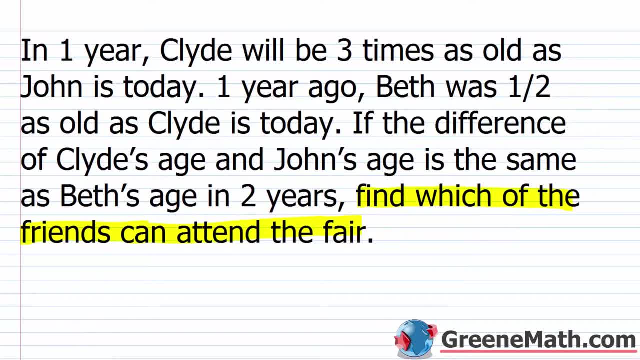 You need to be 12 years old to attend. So we're trying to find out which of these individuals are at least 12, right, Because if you're 12, you can go to the fair. If you're older than 12, you can go to the fair. 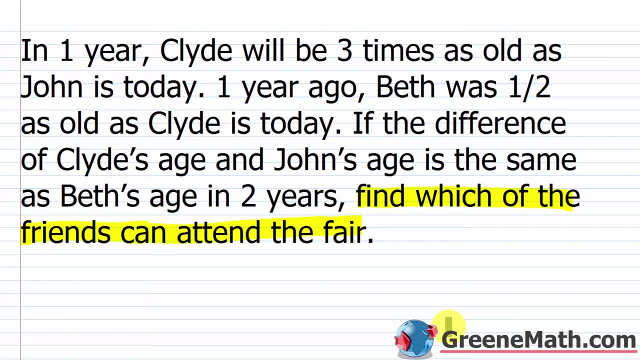 And if you're less than 12, you can't go to the fair. So let's think about a variable to represent one of their ages And then we can go through a model- the rest of the ages, based on that variable. So it tells us that, again, in one year, Clyde will be three times as old as John is today. 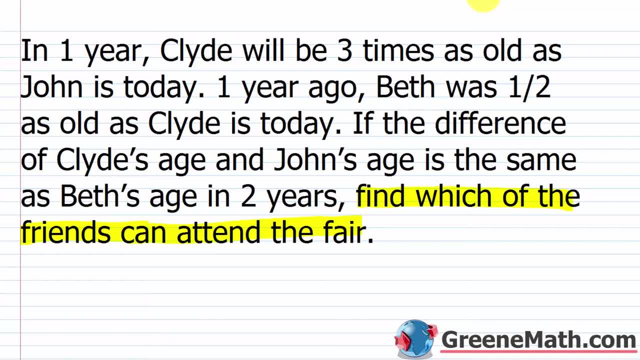 And it tells us one year ago, Beth was one-half as old as Clyde is today. So since Clyde is involved in both comparisons there, let's just go ahead and let X be Clyde's current age. Let's do this on a fresh note. 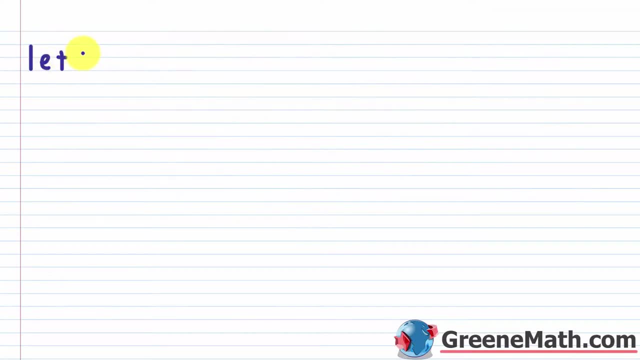 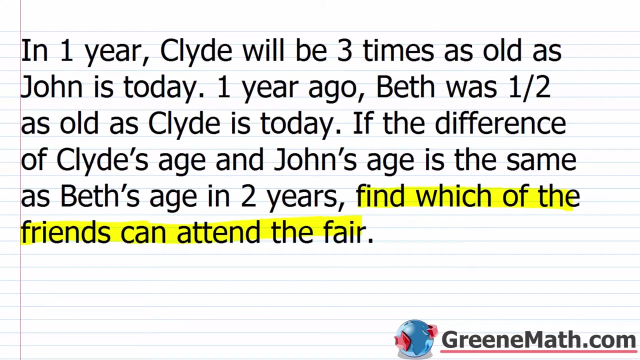 So let's let X be equal to Clyde's current age. Okay, So what can we say about John's age? Well, it says, in one year Clyde will be three times as old as John is today. So that means, if I take Clyde's current age, which is X, and I add one to it, right, because it's in one year. 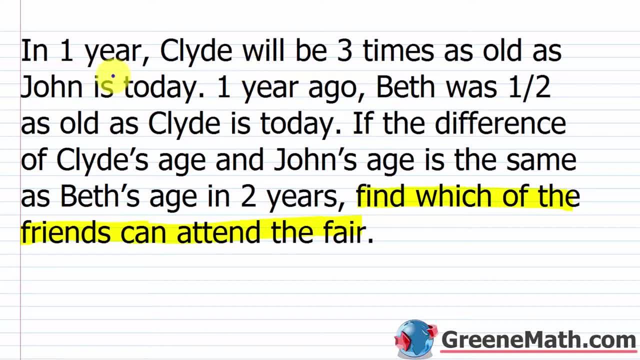 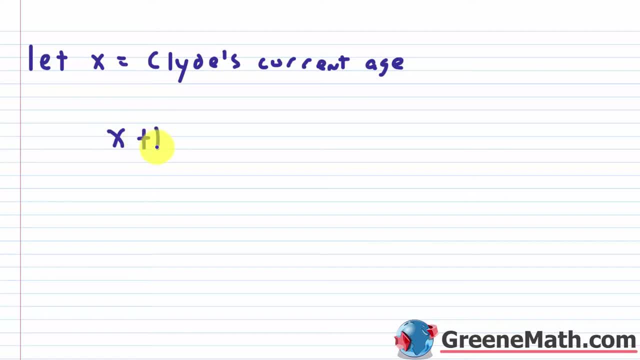 that amount, X plus one, would be three times the age of John, right? So X plus one? X plus one is three times the age of John. So I can just divide by three to get John's current age. 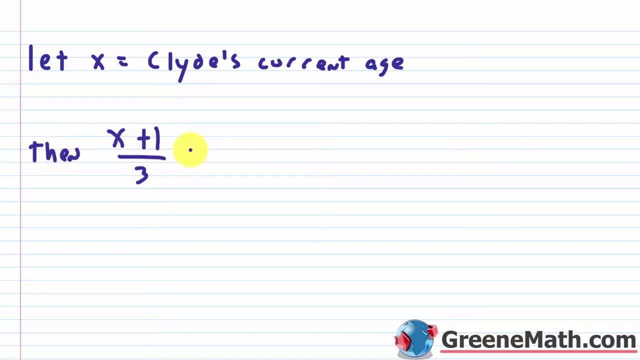 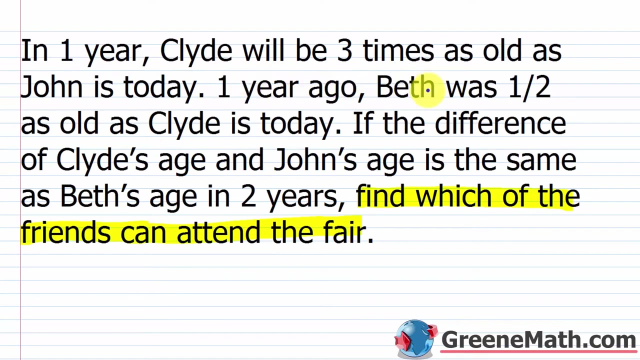 So we can say then: X plus one over three is John's current age. Okay, So what can I say about Beth, Beth's current age. So, if we think about this, one year ago Beth was half as old as Clyde is today. 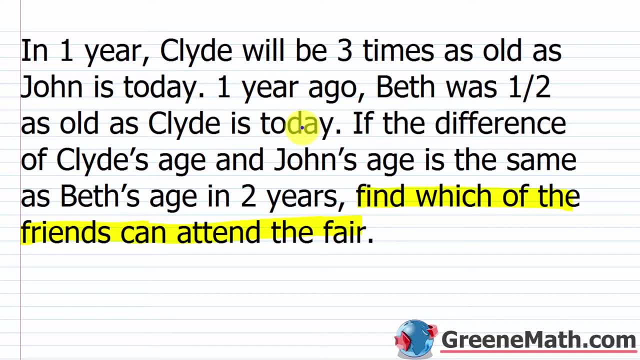 So half of Clyde's age today is one half times again. Clyde's age is represented with X, so it's one half X. Now this is Beth's age, not today, but a year ago. Okay, A year ago she was half as old as Clyde. 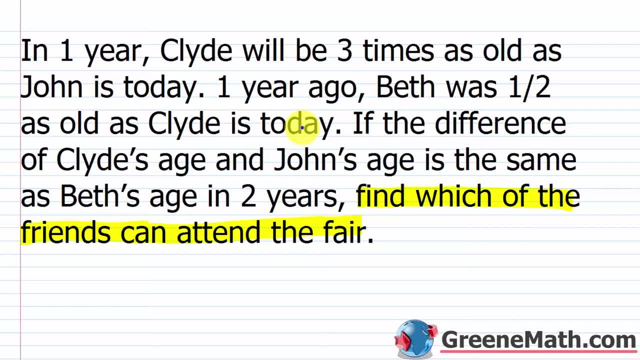 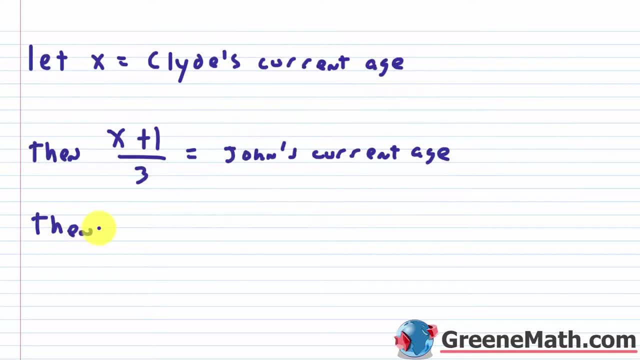 So if I think about one half X, that's Beth's age one year ago. If I add one to that, that's Beth's current age. So we would say that Then X over two, which again is her age a year ago, then plus one would be her current age. 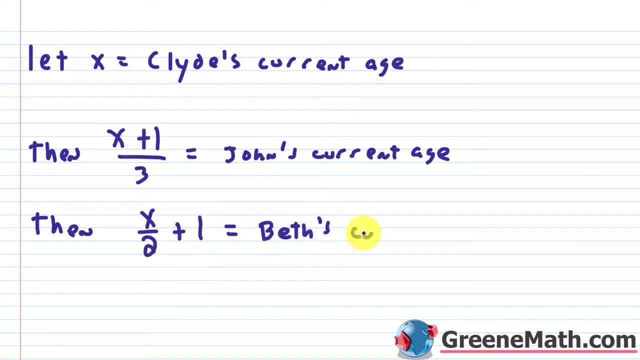 So this would be Beth's current age. So in most of these problems you're given a sum right of all the ages, but in this case you're not. You have to use something else to get your equation, and it's this sentence right here. So if the difference of Clyde's age and John's age is the same as Beth's age in two years, So the difference of Clyde's age and John's age would be Clyde's age minus John's age. So let's set that up first. 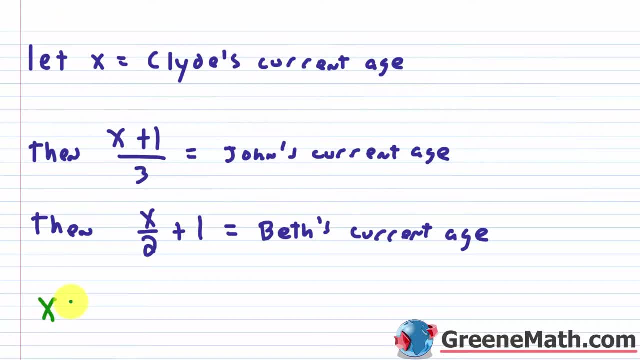 So Clyde's age is X, so this is X, and then, minus John's age, is X plus one over three. Now I'm subtracting this whole thing away, so let me just put it in brackets so we don't make a sign mistake. 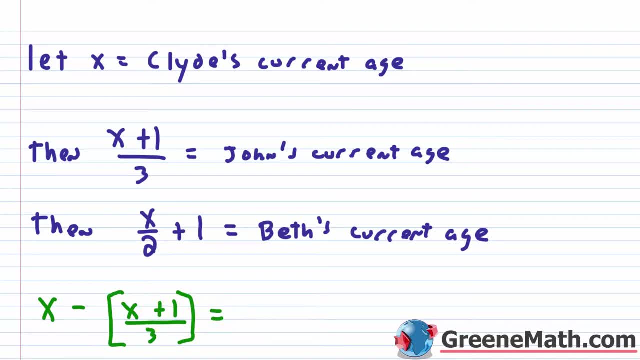 And then we're saying is the same as. so that's equals. Here we're told Beth's age in two years. So her current age is X over two plus one. So X over two plus one In two more years. you would just add another two to this amount. 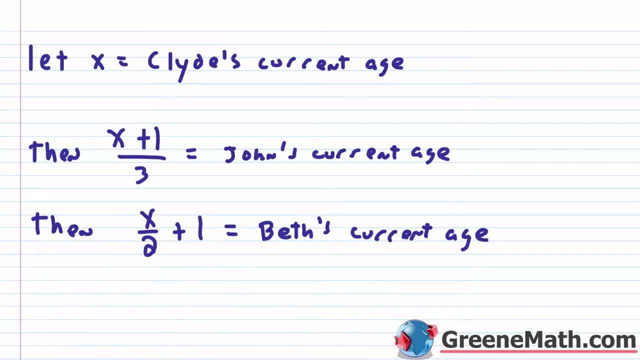 So let's copy this. We're just going to take it to a fresh sheet of paper and we can solve this guy. So we have X and then you have your minus here. You can distribute this. You can go ahead and set this up as X over three plus one over three. 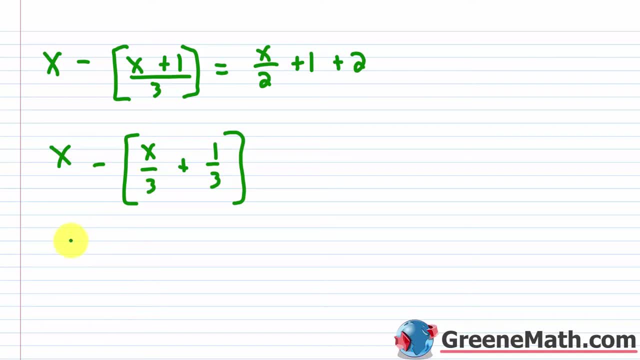 And then if I had a minus out in front of that, then I would have what I would have: X minus X, So X over three and then minus one third. okay, Then this would be equal to- let me just kind of drag this back up. 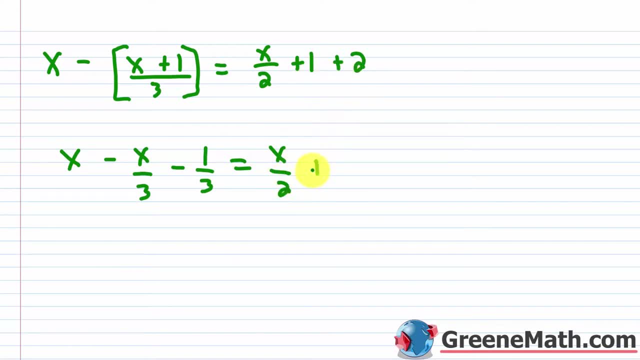 You have your X over two. One plus two is three, so plus three. Now, if I want, I can multiply both sides of the equation by six. right That would be the LCD. So if I did that I would have six X minus. 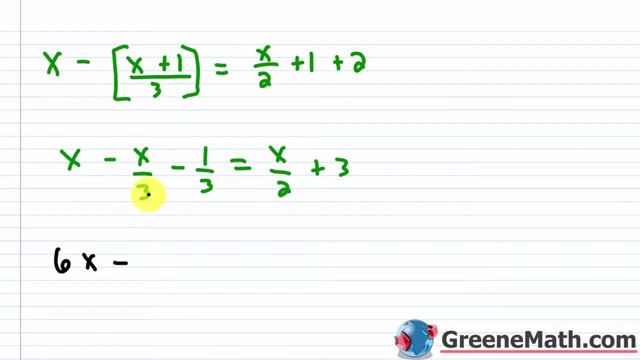 If I have six times X over three, the six would cancel the three and give me a two. So this would be two X then minus. If I have six times one third, that's two. This equals, if I have X over two times six. again six divided by two would be three. 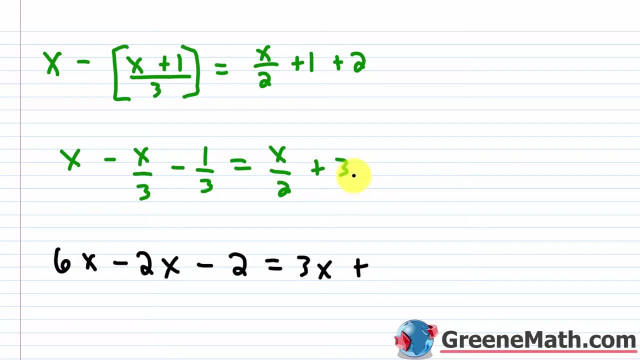 Three times X is three X, and then plus six times three is 18.. Okay, So now here on the left I have six X minus two X, which is four X, and then minus two equals three X plus 18.. 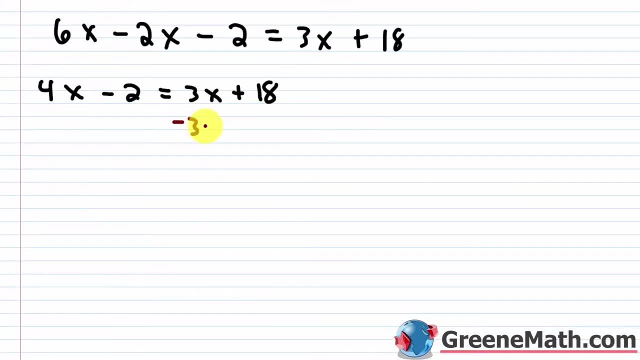 Let me scroll down and get some room going. So now I can subtract three X away from each side of the equation, So this is going to cancel. I can add two to both sides of the equation- This is going to cancel. 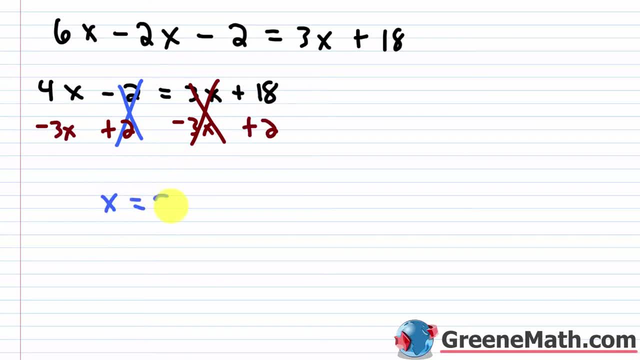 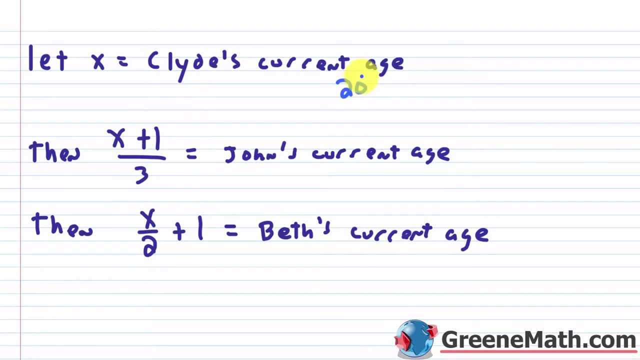 Four X minus three, X is X, and this is equal to 18 plus two, which is 20.. So X is equal to 20.. Now, X was Clyde's current age, So he's 20.. John's current age was what? 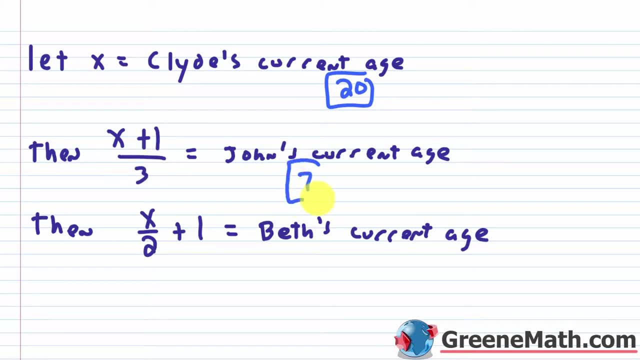 It's 20 plus one, which is 21,, divided by three, which is seven. Beth's current age is 20, divided by two, which is 10, plus one, which is 11.. So it doesn't ask for their ages. 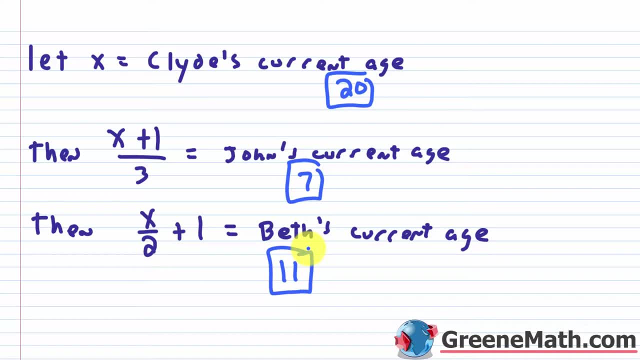 It wants us to find out who can attend the fair. So we know that Clyde is the only one that can attend the fair because the minimum age is 12.. Right, Beth can't go because she's 11, and John can't go because he is seven. 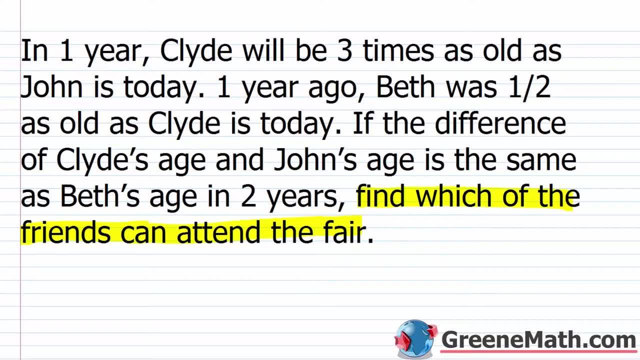 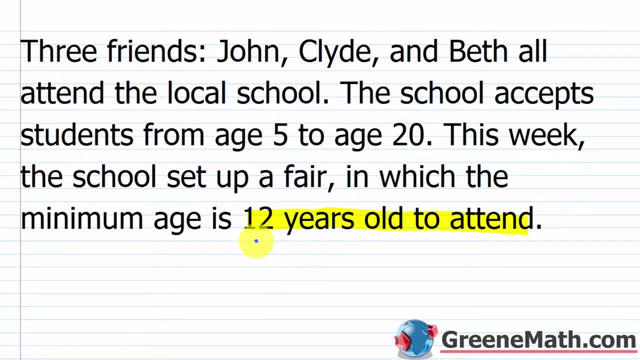 So only Clyde can attend. So that's the only information we need to know. It's again, find which of the friends can attend the fair. and once more, you can only attend if you're 12 or older, Right? 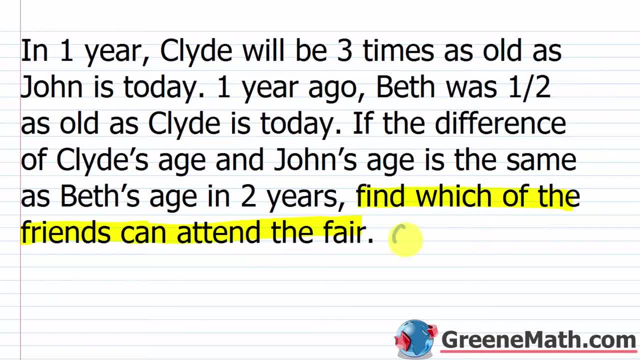 So let's go back down and say that only Clyde Can attend the fair. Okay, Now if we think about this, we can go back and check. So in one year Clyde will be three times as old as John is today. 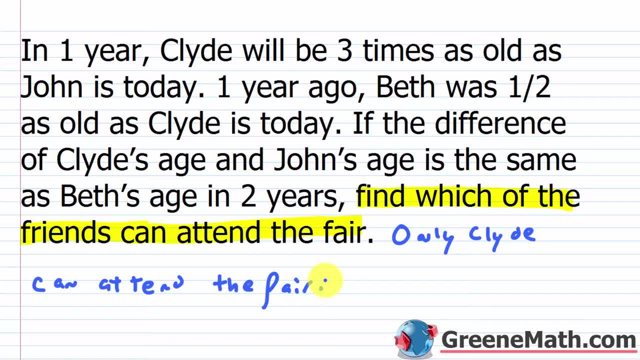 We said that Clyde was 20.. We said John was seven. So in one year Clyde will be what He'll be: 21.. And that is three times as old as John is. He'll be 21.. He'll be 20.. 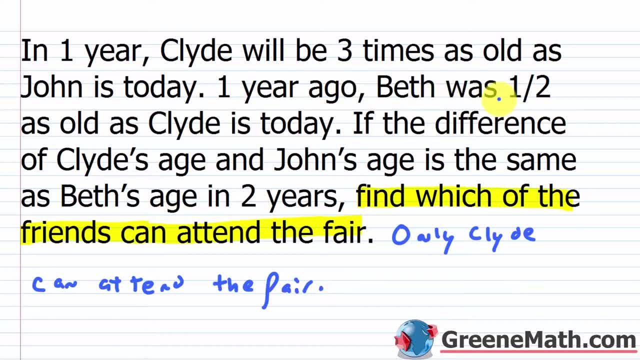 And that is three times as old as John is today, because John is seven. So that checks out. Then it says: one year ago Beth was one half as old as Clyde is today. So a year ago Beth would have been 10 years old, and that is half as old as Clyde is today. 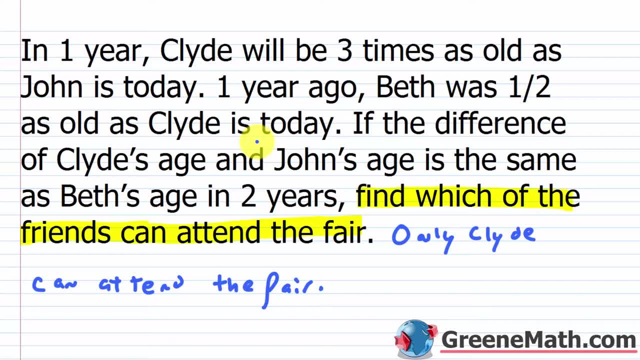 because he is 20.. Okay, So that checks out. Then it says if the difference of Clyde's age and John's age, So the difference between 20 and seven Clyde's age and John's age, is 13.. 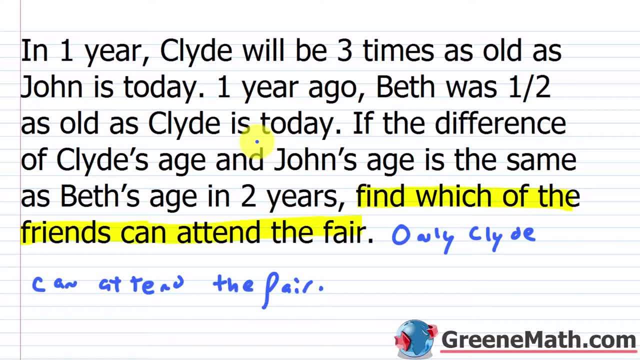 That is the same as Beth's age in two years. She's currently 11.. In two years she's going to be 13.. So that all checks itself out. So our answer here is correct: Only Clyde can attend the fair because, again, he's the only one that's at least 12 years. 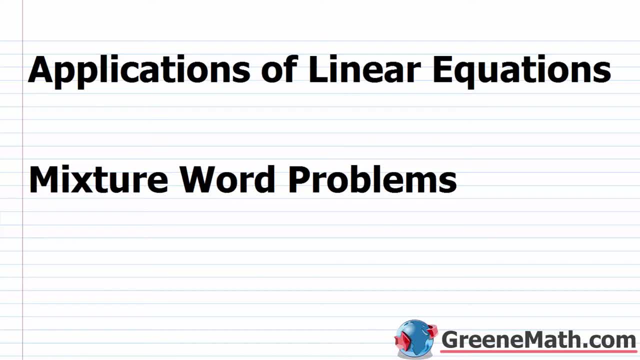 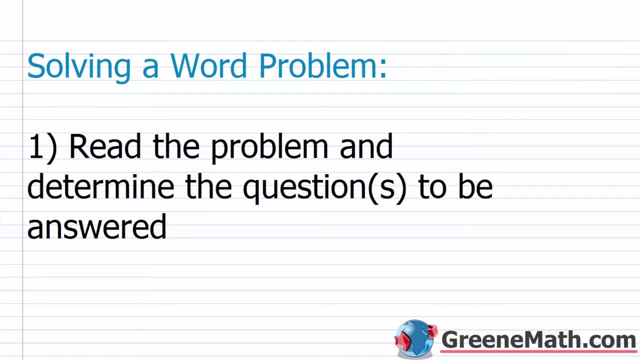 old. In this lesson we want to review applications of linear equations. We're going to look at mixture word problems. So again, when we're working with applications of linear equations, we have a little six-step procedure that we can use. 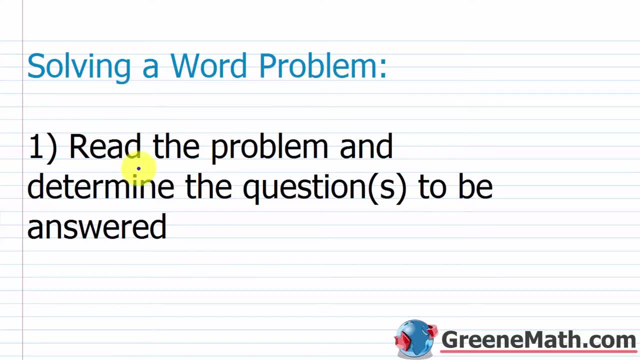 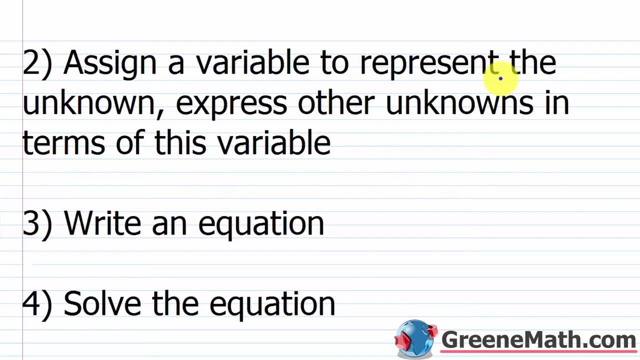 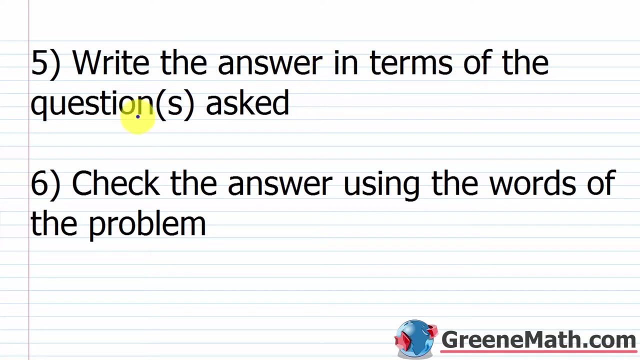 So for solving a word problem, we have, as our first step, we want to read the problem and determine the question Or again questions to solve. Okay, So we're going to write the answer in terms of the question or again questions being. 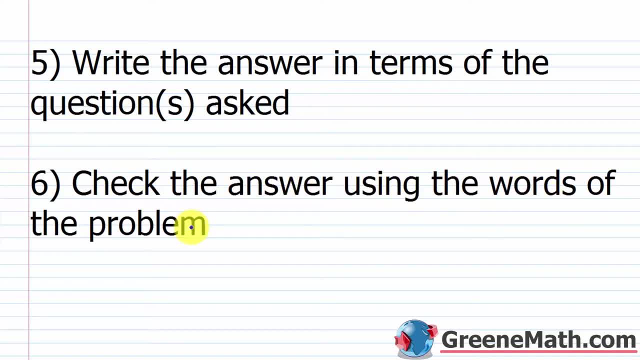 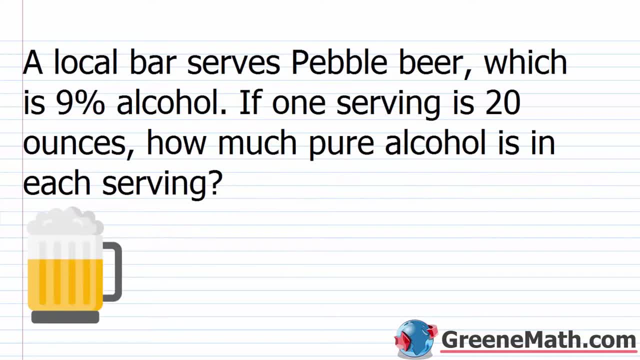 asked. Then, lastly, we're going to check the answer using the words of the problem. This one right here, number six. the last step is very important. You want to make sure your answer is reasonable. So, of all the word problem types that we have, we're going to write the answer in terms: 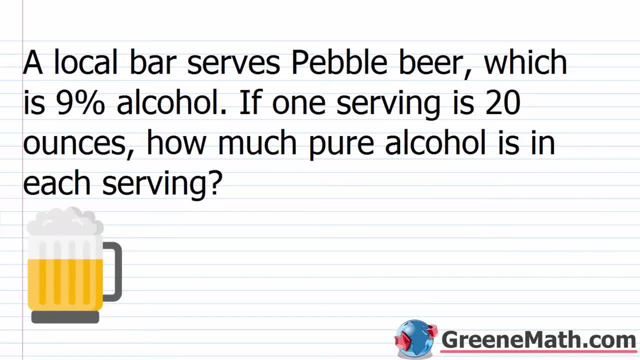 of the question, So we're going to write the answer in terms of the word. problem types that we encounter in elementary algebra courses. Usually mixture problems give students the most trouble, right when you're in that section on applications of linear equations. 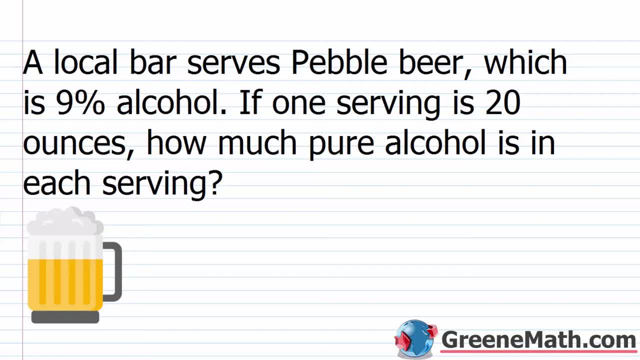 The key to understanding mixture problems is understanding how to find the pure amount of a substance in a mixture. To accomplish this task, we can multiply the rate of concentration as a decimal by the amount of the solution. Okay, This will give us the pure amount of a substance in a mixture. 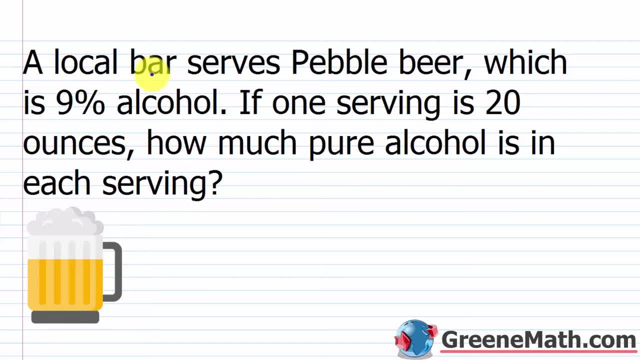 So let's look at a simple example. Okay, Let's look at a simple example. So a local bar serves pebble beer, which is nine percent alcohol. So I'm just going to highlight this because they gave us a percentage. so nine percent. 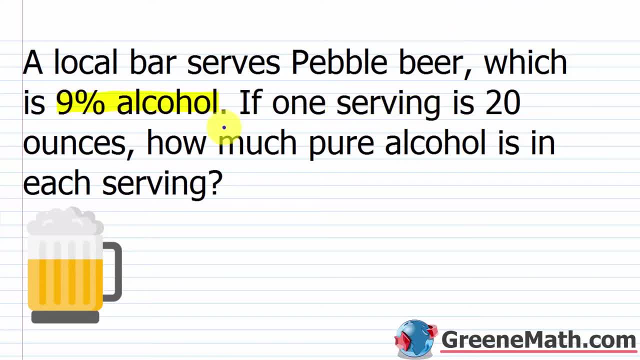 alcohol. If one serving is 20 ounces- let me just highlight that. so it's 20 ounces- how much pure alcohol is in each serving? So obviously, this is what we want to answer here: How much pure alcohol is in each serving. 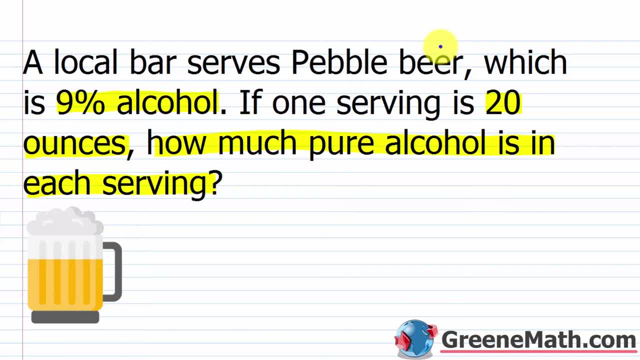 So all I need to do is take the amount of one serving, which is 20 ounces- Forget about the ounces part for a minute, just the number 20, and it's nine percent alcohol. Okay, So all I need to do is multiply the 20 by nine percent as a decimal, which is .09.. 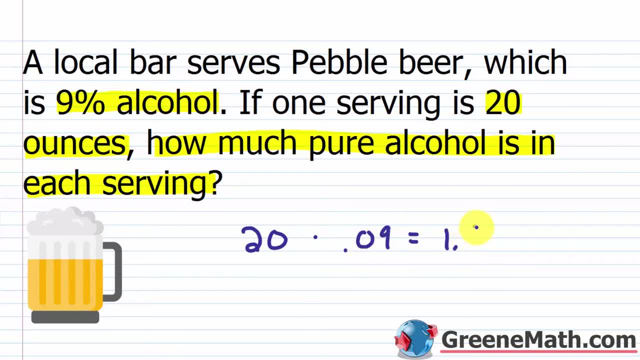 If I do that calculation, I'm going to get 1.8.. Okay, So what this tells me is that this pebble beer here is going to be 1.8 ounces of pure alcohol. So let me erase this and I'll write a nice little sentence. 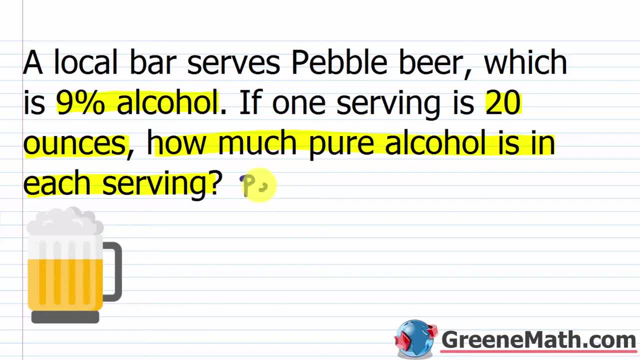 And we'll say that pebble beer has 1.8 ounces of pure alcohol per serving. Okay, So a very simple example, Just something we need to understand. We need to understand how to find the pure amount of something in a mixture or substance. 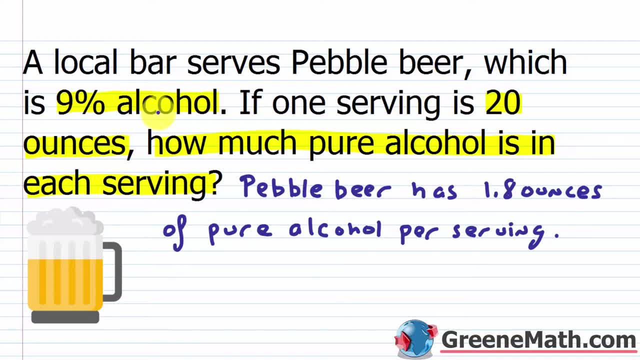 So in this case we have a beer. It's nine percent alcohol. We want to know the pure amount of alcohol in the full serving, which is 20 ounces. Again, we take the rate of concentration, which is .09, as a decimal. 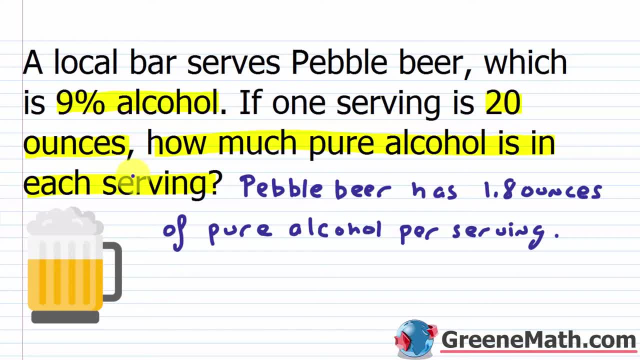 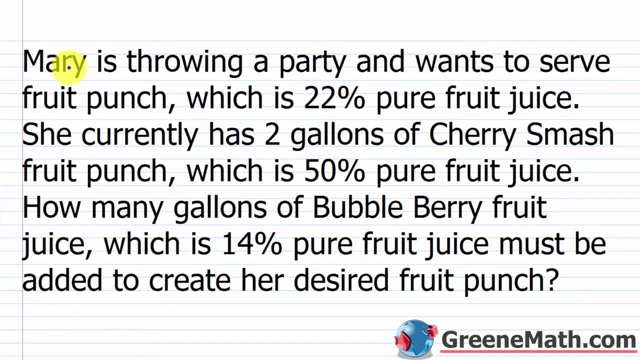 We multiply it by that serving, which is 20 ounces, and that tells us we have 1.8 ounces of pure alcohol in each serving. All right, Let's look at a typical word problem now. So we have that. Mary is throwing a party. 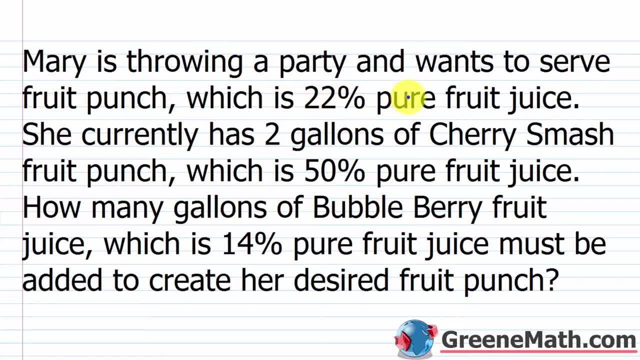 She's throwing a party and wants to serve fruit punch which is 22 percent pure fruit juice. She currently has two gallons of cherry smash fruit punch, which is 50 percent pure fruit juice. How many gallons of bubble berry fruit juice, which is 14 percent pure fruit juice, must? 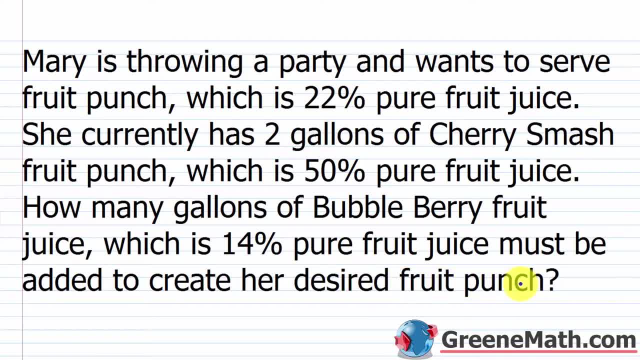 be added to create her desired fruit punch. So understand what we're trying to find here. We're trying to find out how many gallons of this bubble berry fruit juice, which again is 14 percent pure fruit juice, That's got to be added to create her desired fruit punch. and again her desired fruit punch. 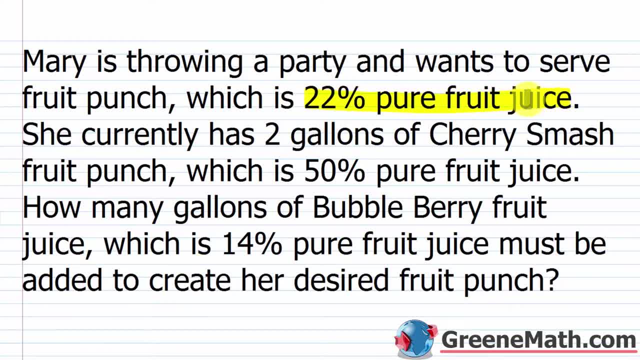 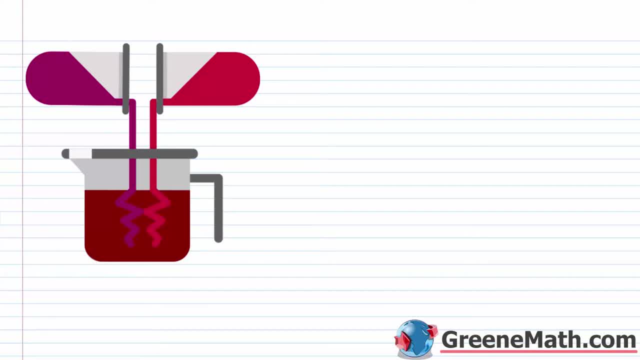 is 22 percent pure fruit juice. Okay, That's what we want. So let's get a little idea of what's going on. She has these two fruit punches that she's mixing together: One is the cherry smash and the other is the bubble berry. 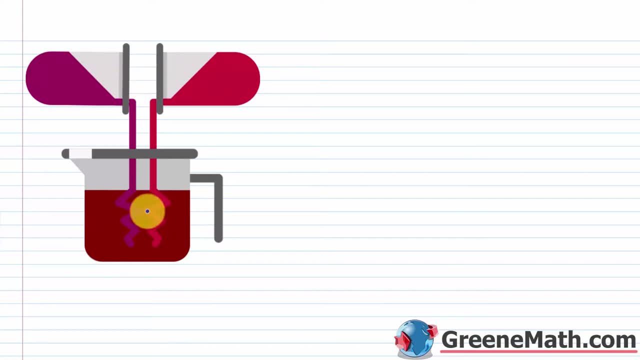 Okay, So you can see that little image here. So she's mixing them together to get this final mixture here and the final mixture is going to be 22 percent pure fruit juice. Okay, So that's the goal. So let's let a variable like X be equal to the amount of the bubble berry fruit punch. 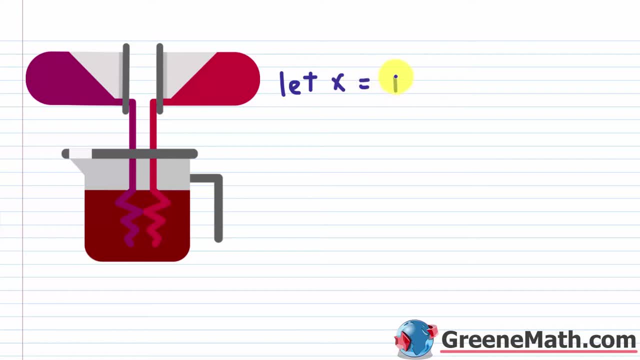 in gallons. Okay. So that's the amount she's going to use in gallons. So we'll say the amount. let me kind of erase that. So we'll say the amount of the bubble berry fruit punch in gallons Okay. 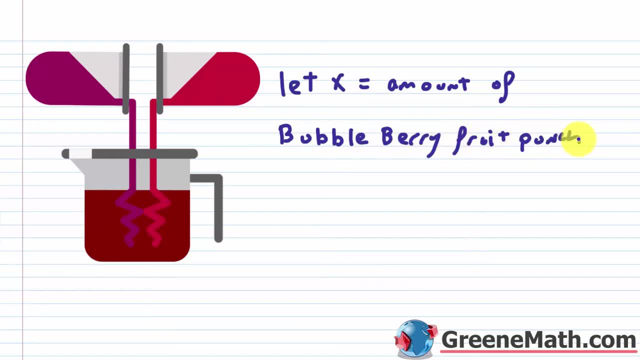 fruit punch used, And this is going to be in gallons. Okay, In gallons, All right. So once we know that X is representing the amount of bubble berry fruit punch used in gallons, what else do we need? Well, we already know the amount of cherry smash, It tells us. 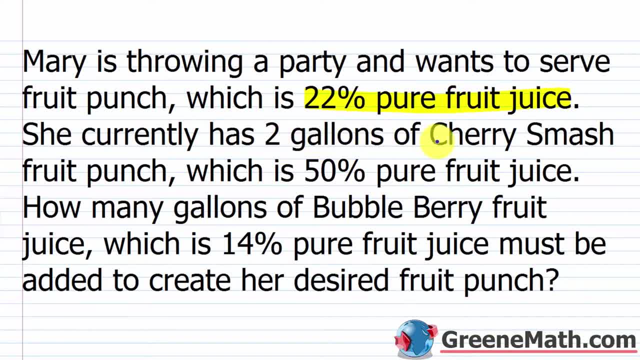 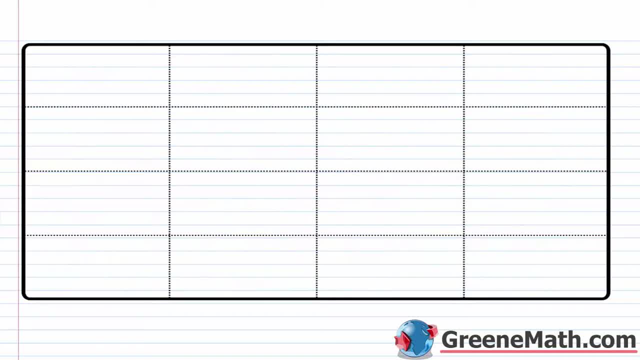 that in the problem, It tells us that she has two gallons of cherry smash. Okay, So let's go down to a little table and organize this information. So for our table up here, we're going to put the gallons. So this is going to be the gallons. This is going to be our concentration percentage as a 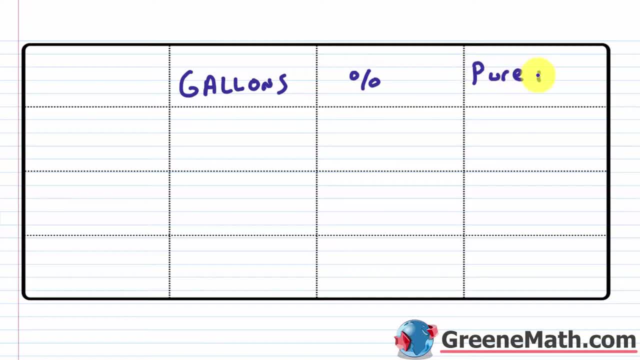 decimal, And this amount right here is going to be our pure fruit juice. Okay, Then, for our products over here, we're going to have the cherry smash and we're going to have the bubble berry. Okay, So those two products. Now it tells us in the problem. 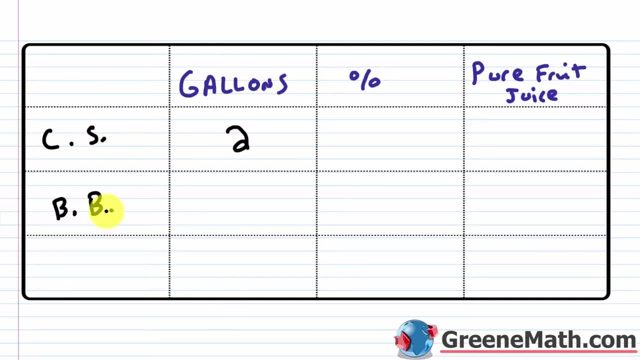 the number of gallons of the cherry smash is going to be two. And then we said the number of gallons of bubble berry that we're going to use is going to be represented with our variable X. What is the percentage of pure fruit juice in cherry smash? So let's go back up. So cherry. 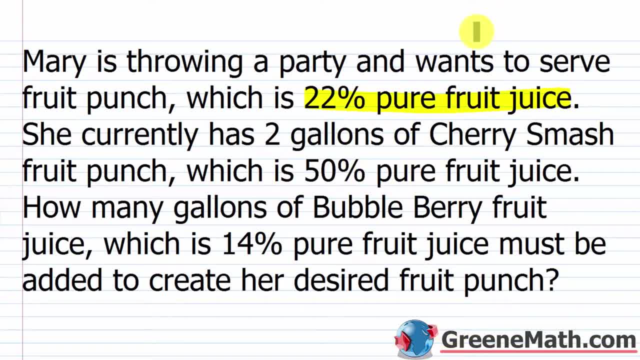 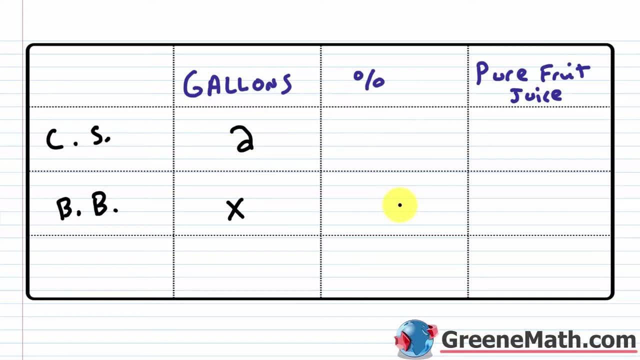 smash, it tells us, is 50% pure fruit juice- 50% pure fruit juice, Whereas bubble berry is 14% pure fruit juice. Okay, So let's fill this part in. So cherry smash again is 50% fruit juice, So as a decimal, that's 0.5.. Okay, Bubble berry is 14% pure fruit juice, So as a 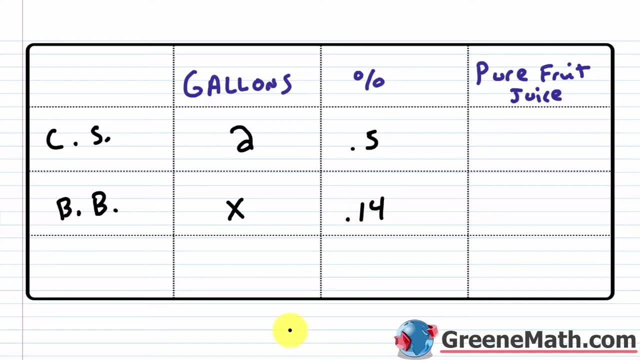 decimal, that's 0.14.. Now, as we just saw in our simple example a minute ago, all we need to do to get the amount of pure fruit juice here is multiply across. So for cherry smash, if I have two gallons, 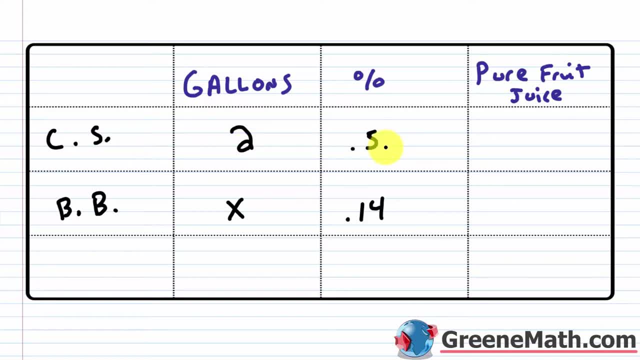 of my fruit punch, and it's 50% pure fruit juice. the amount of pure fruit juice in gallons there is going to be two times 0.5, or one. Okay, Then for the bubble berry. I just got to multiply across. 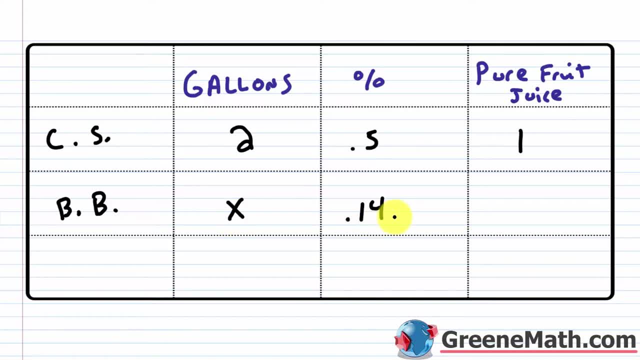 again. So I have X gallons. It's 0.14 or 14% pure fruit juice. So the amount of pure fruit juice there is 0.14 times X. Okay, And again, this is in gallons. Now we have this final row here. 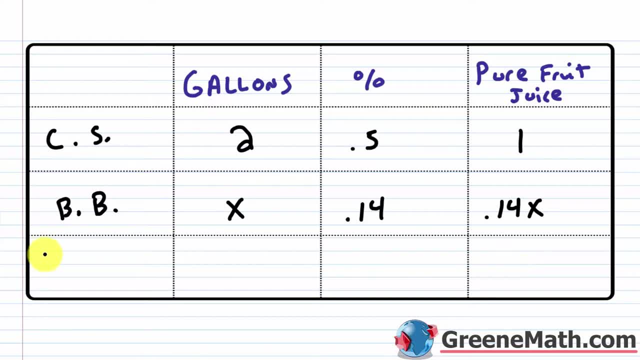 that represents our mixture, our desired mixture, So we'll say this is our final mixture. Okay, So the number of gallons will be what? Well, we only have gallons coming from two sources, right? We have the cherry smash and the bubble berry, So I can just add these. 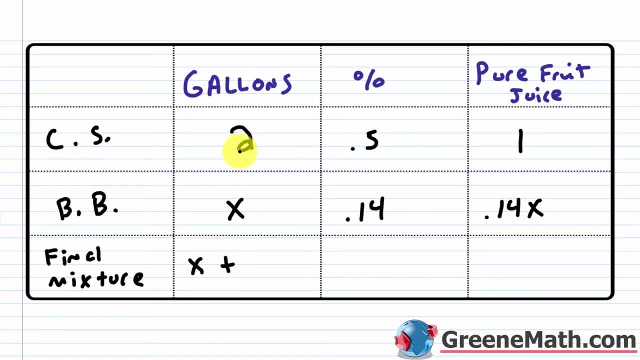 I would have X gallons coming from the bubble berry, then plus two gallons coming from the cherry smash. Now the percentage is given to us in the problem. It tells us that the final mixture again is 22% pure fruit juice. So this has to be 0.22.. And so the pure fruit juice in gallons. 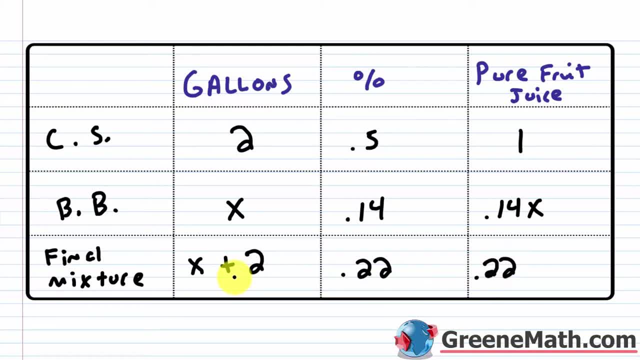 would be what? It would be 0.22 times this quantity of X plus two. All right, So let's stop here. From this point, it's very easy to set up an equation. We know that the amount of pure fruit juice in gallons in the final mixture comes from two sources. It comes from this source, right? 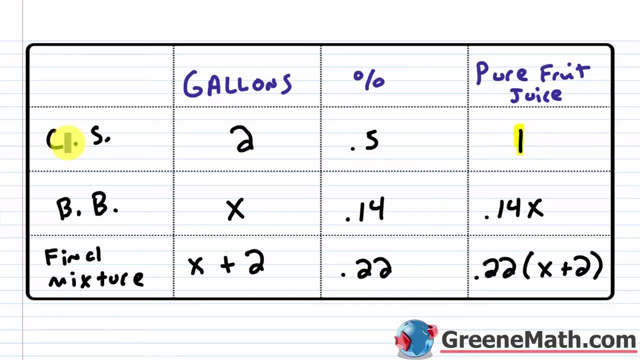 here You've got one gallon coming from your cherry smash and then you've got 0.14, X gallons coming from your bubble berry. That has to be equal to the pure fruit juice in gallons. in the final mixture, This 0.22 times the quantity X plus two. So that's where we're going to get our. 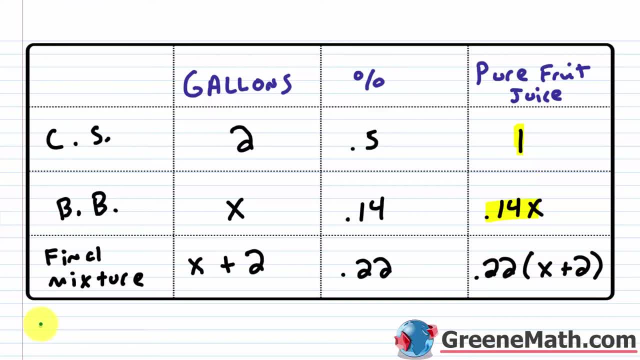 equation. We're just going to set this up, So we will have one again: the amount of pure fruit juice in gallons from cherry smash, plus you're going to have your 0.14 X, which again is the amount of gallons of pure fruit juice in the bubble berry, And we're going to set this equal. 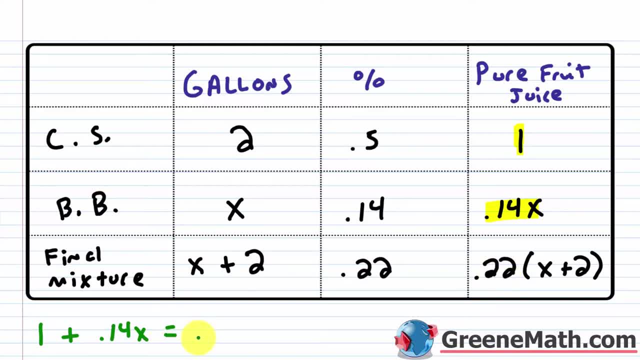 to the amount of pure fruit juice in the final mixture, which is 0.22 times the quantity X plus two. Okay, So once we've set this up, we're going to set this equal to the amount of pure fruit juice in the 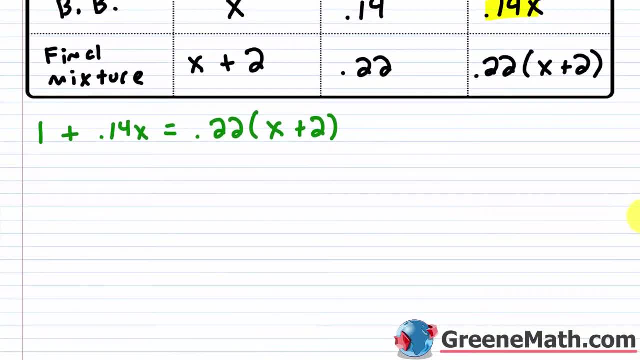 final mixture. So once we've set up an equation, it's very easy. So you have your one. plus 0.14 X is equal to use our distributive property. we'll have 0.22 X and then plus two times 0.22 is 0.44.. 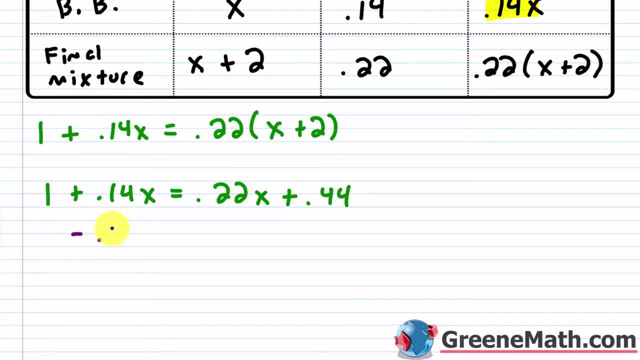 And then to solve this guy, I'm just going to go ahead and subtract 0.14 X away from each side of the equation And I'm going to subtract 0.44 away from each side of the equation. And what's that? 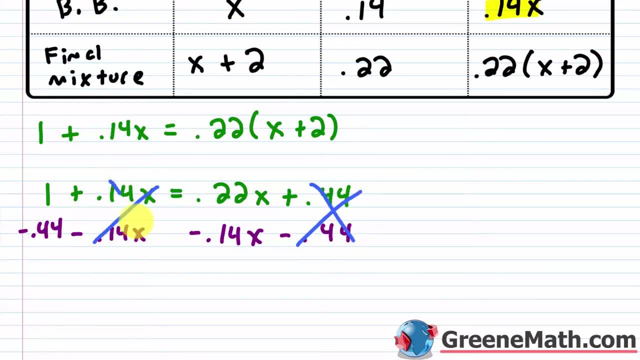 going to give me. So we know that this would cancel. We know that this would cancel. So one minus 0.44 is 0.56.. So the left side is 0.56.. This is equal to 0.22 minus 0.14 is 0.08.. And then times X. If we finish this. 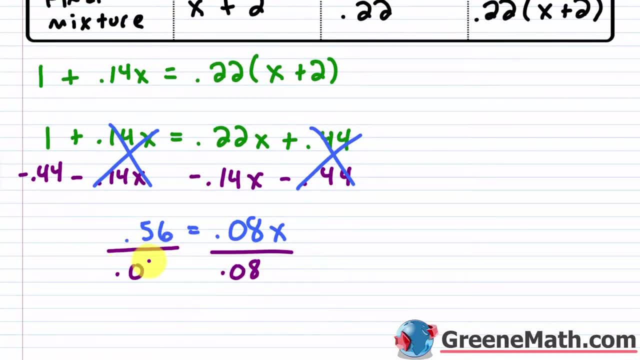 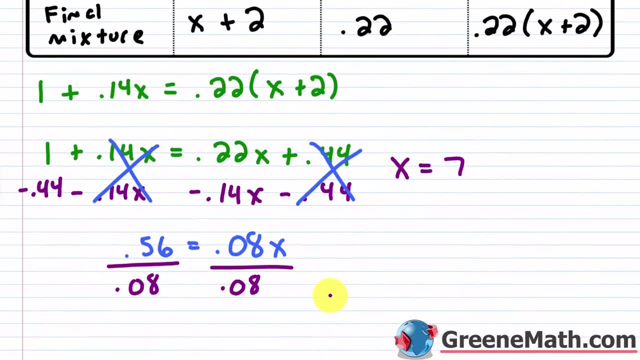 up by dividing both sides by 0.08, we're going to get seven. Okay, so X here is going to be equal to seven. Now let's make sense of this. We said that X was the amount of pure fruit juice in the 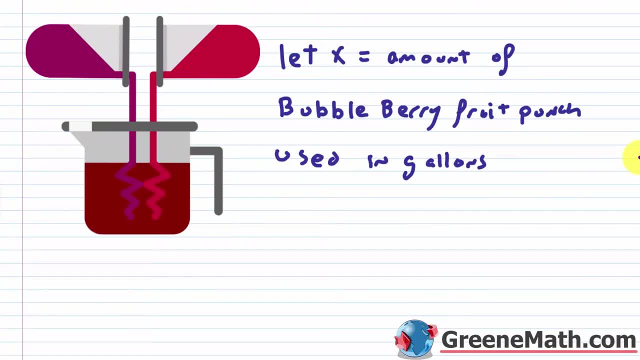 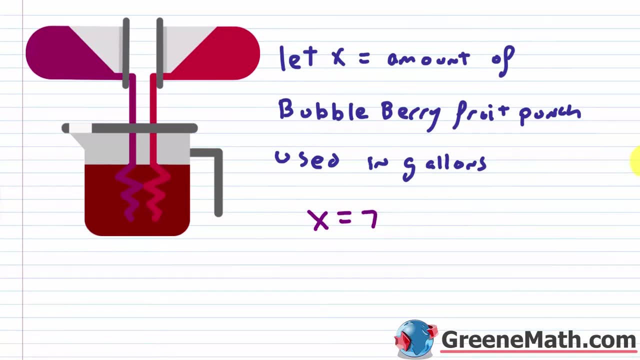 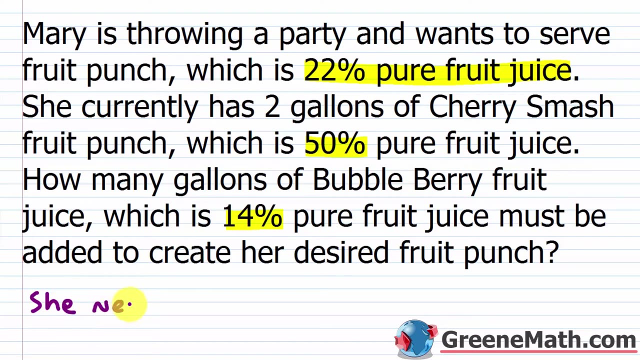 amount of bubbleberry fruit punch used in gallons. So we know that X is equal to seven, So she needs to use seven gallons of bubbleberry fruit punch. Okay, so let's go back up and let's answer our question. So we'll just say that she needs to use seven gallons of bubbleberry. 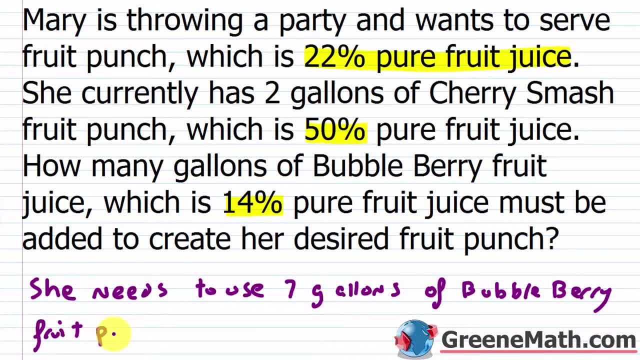 fruit punch. Now let's check this, Let's make sure the answer is reasonable. She's throwing a party and wants to serve fruit punch which, again, is 22% pure fruit juice. She currently has two gallons of cherry smash fruit punch, which is 50% pure fruit juice, And again it asks how many. 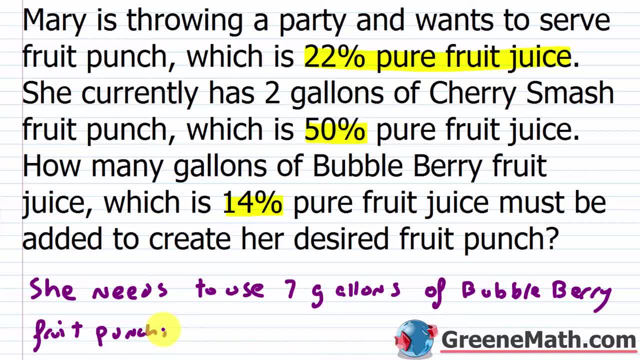 gallons of bubbleberry fruit juice, which is 14% pure fruit juice, must be added to create her desired fruit punch. We know if she's using seven gallons of bubbleberry fruit juice, she's going to use seven gallons of bubbleberry fruit punch and it's 14% pure fruit juice, then essentially she's 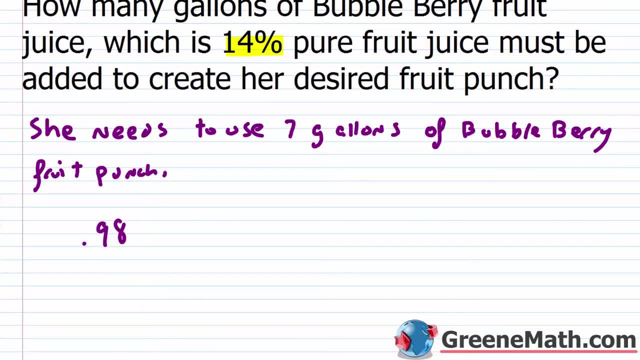 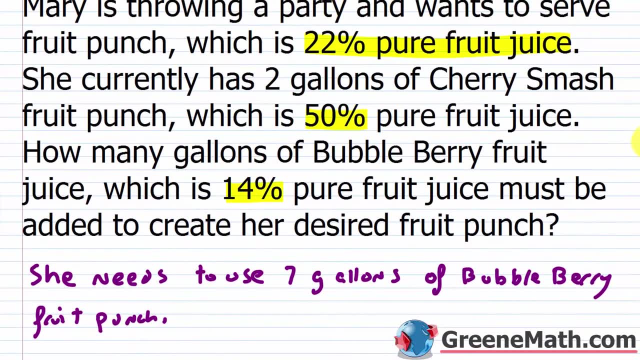 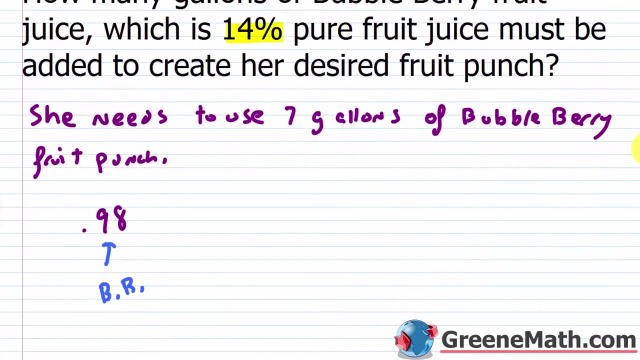 getting 0.98 gallons of pure fruit juice from the bubbleberry. So this comes from the bubbleberry. Now we're told again in the problem directly that she's using two gallons of the cherry smash and it's 50% pure fruit juice. So two gallons times 0.5 is again one, So add that to one. 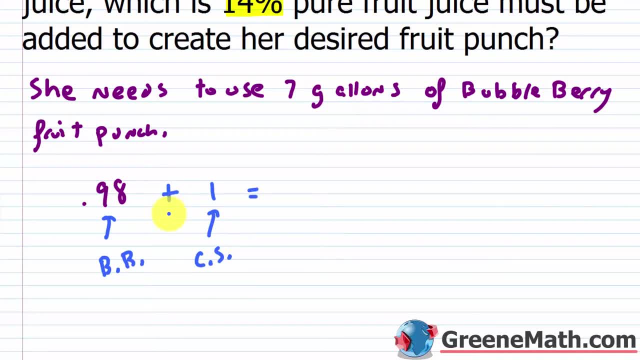 This is from the cherry smash, So this amount should be equal. this one plus 0.98, which is 1.98, should be equal to the amount of pure fruit juice in the final mixture. So in the final mixture she's going to have seven gallons. 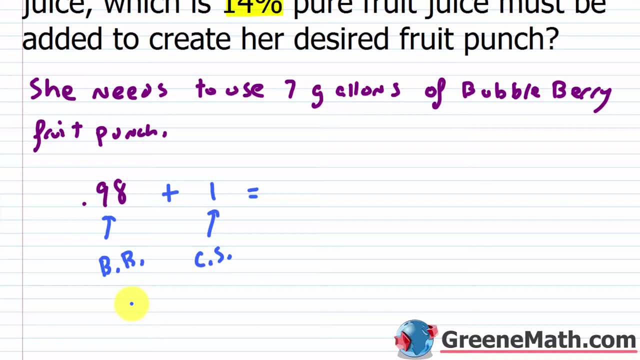 of bubbleberry plus two gallons of cherry smash, So that's nine gallons, And again it's 22% pure fruit juice, and nine times 0.22 is 1.98.. So we're good to go right. This is your final mixture. 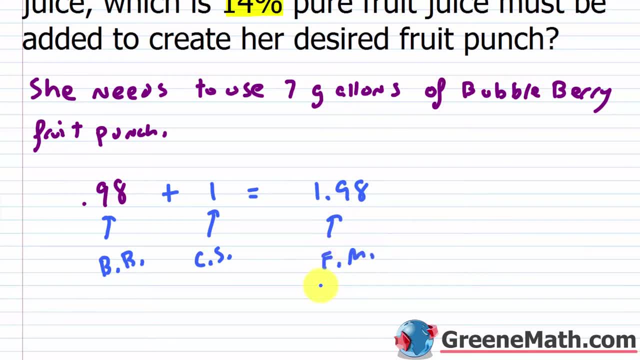 You basically have said that the amount of pure fruit juice coming from the bubbleberry and the cherry smash is equal to the amount of pure fruit juice in the final mixture, and it is 22% pure fruit juice. So we're good to go. She needs to use seven gallons of bubbleberry fruit punch. 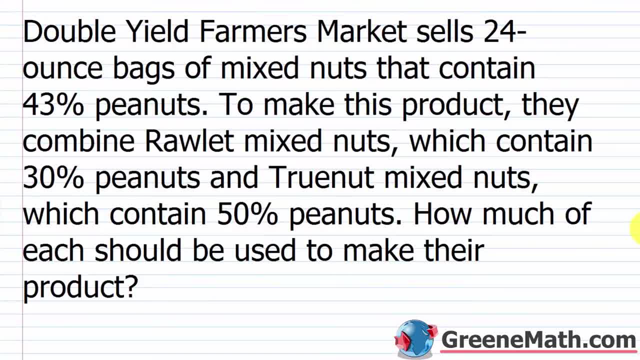 to make her desired fruit punch mixture. All right, let's take a look at another one. So Double Yield. Farmer's Market sells 24 ounce bags of mixed nuts that contain 43% peanuts. To make this product, they combine raw lit mixed nuts, which contain 30% peanuts. 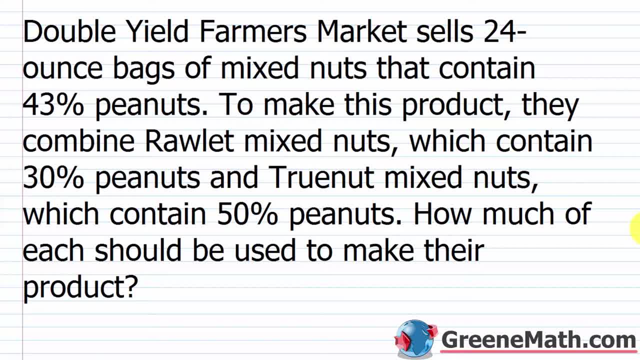 and true nut mixed nuts which contain 50% peanuts, How much of each should be used to make their product? So again, another straightforward kind of question: how much of each? So we're saying how much of the raw lit mixed nuts and how much of the true nut mixed nuts. 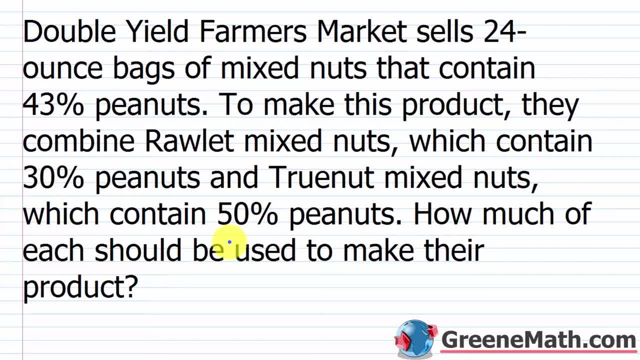 should be used to make their product, which again is a 24 ounce bag of mixed nuts that contains 43% peanuts. Okay, So in this case, we don't know an amount for either, right, So we have to kind of get that. 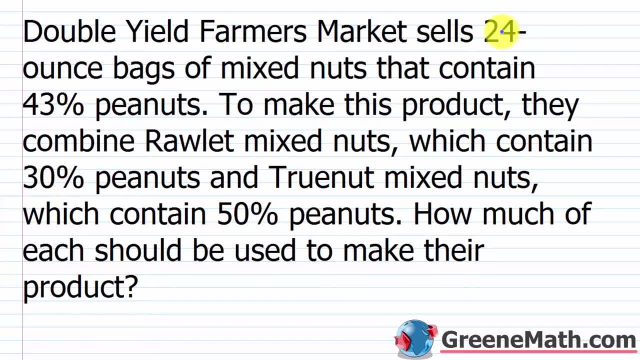 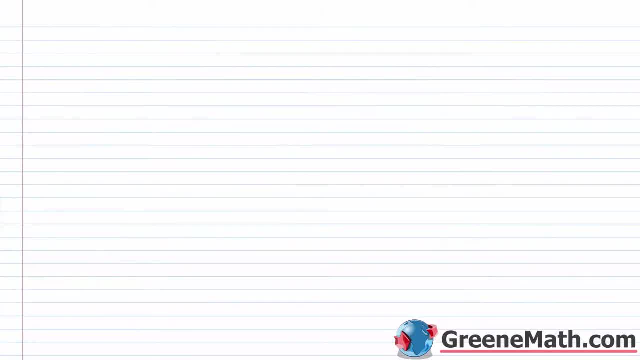 We're working with ounces. So the total amount in the final mixture that they sell is 24 ounces. So let's use that information to create a variable. So let's let X be equal to the amount in ounces of we'll just go ahead and say raw lit. 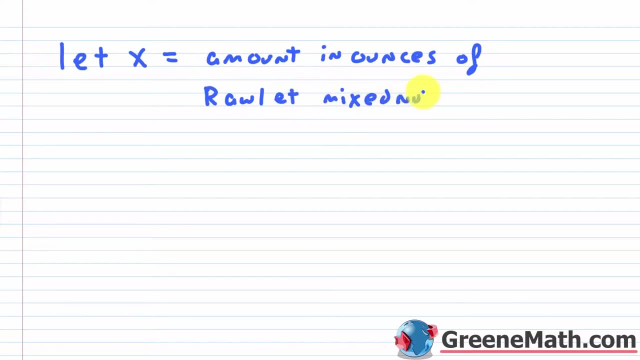 mixed nuts used. Okay Now, because the total mixture in the end is 24 ounces. we know that if we subtract away X again, the amount in ounces of raw lit mixed nuts used what's going to happen is 24 minus X can represent the amount of the true nuts mixed. 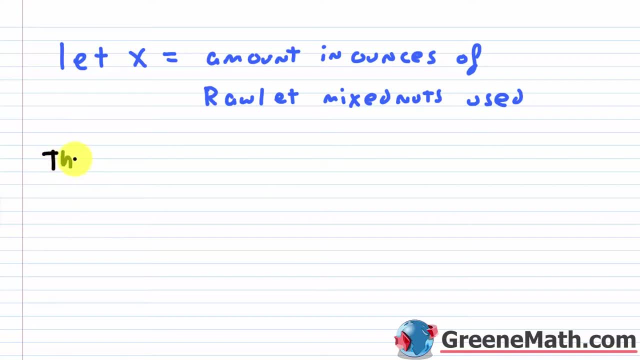 nuts that's going to be used, right? So if we put, then we'll say 24, again the total amount of ounces of the final mixture Minus X, which is the amount in ounces of raw lit mixed nuts used. So this is going to be equal to: 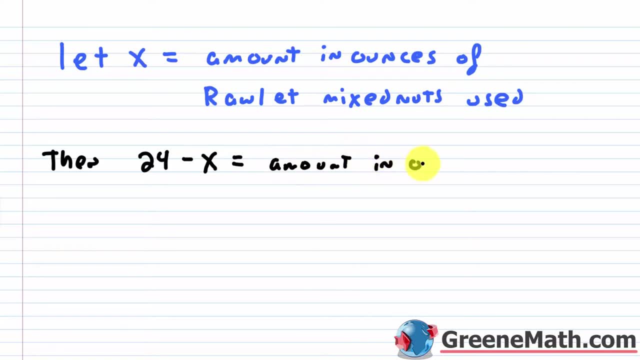 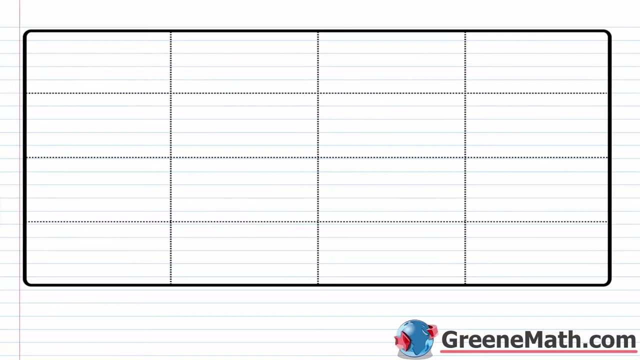 the amount in ounces of the true nut, the true nut mixed nuts used. Okay, So once we've kind of modeled this, we can go down to the little table and set things up just like we did in the last example. So on the left, let me put the name: So you have your raw lit, you have your raw lit mixed nuts. 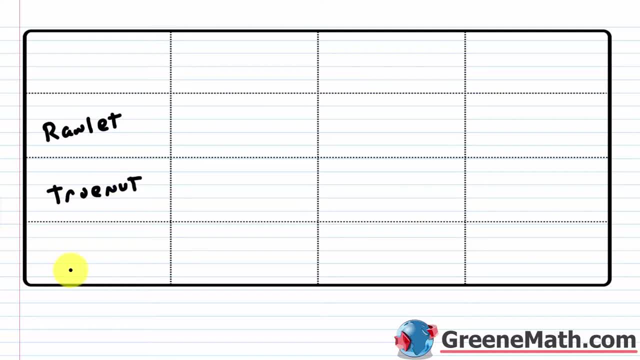 you have your true nuts and we're going to have a final product. So we'll have a final. you can say final mixture or final product. Okay, Let me make that a little better. So again, final mixture. So up here we'll have our ounces. 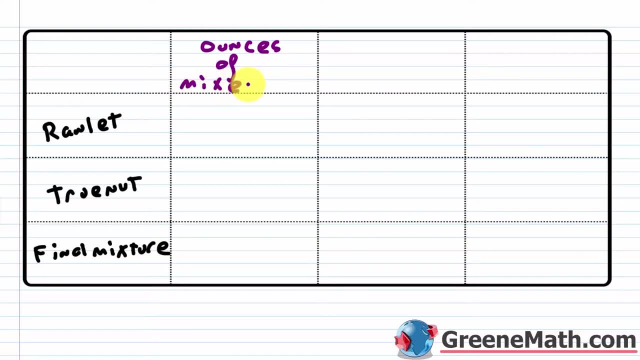 This is what our raw lit mix nut on is going to look like: to be我們本not. we know what this mean. We're going to have an ounce, and this is pure nuts in ounces, And then we're going to have our 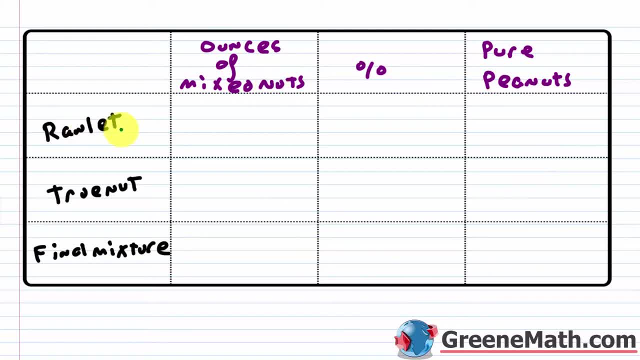 concentration percentage of peanuts. So this is our mixture per teacher. So we can be divided between pure nuts and ounces and we know that we represent our viens as the percentage of our mixed nuts for the final mixture. we know it's 24. okay, that's given to us in the problem. now the percentages. 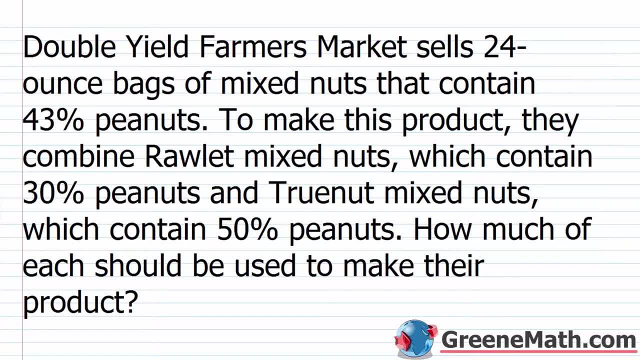 let's go back up. we're told that the final mixture is 43, so this would be 43 or 0.43 as a decimal. then we're told that raw lit mixed nuts has 30 peanuts and true nut has 50 peanuts. so let's go. 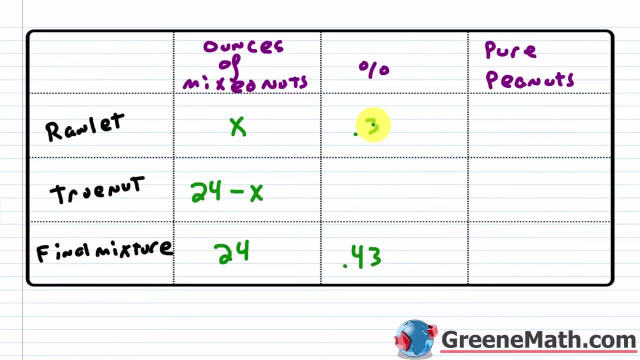 back down. so raw lit is 30, so 0.3 as a decimal. true nut is 50, so 0.5 as a decimal. and again, to get the amount of pure peanuts, we just multiply across if it's 30 peanuts and it's. 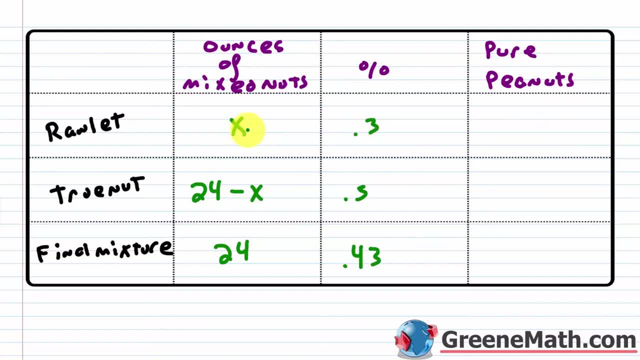 x. number of ounces, the ounces of pure peanuts would be 0.3 times x. again, if it's 50 peanuts and there's 24 minus x ounces, the pure peanuts would be 0.5 times the quantity, 24 minus x. and then for the final mixture, if it's 43 percent peanuts and there's 24 ounces of mixed nuts, well, 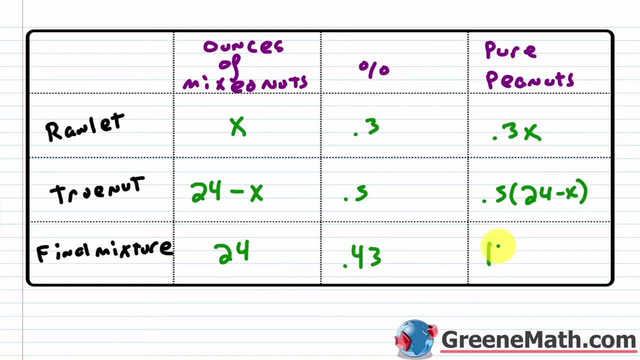 i can multiply 0.43 times 24.. to give me 10.32, this is the amount in ounces of pure peanuts in the final mixture. now again, we can set up an equation in the same way that we did in the last problem. we basically think about: 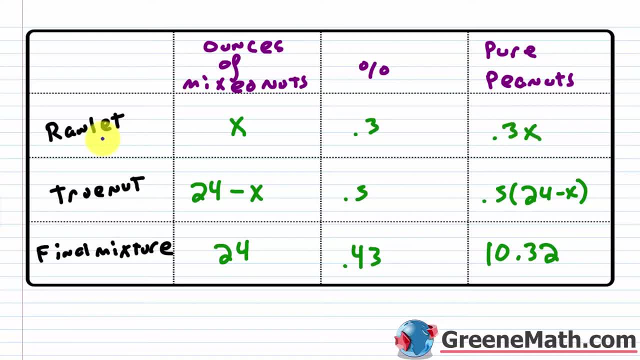 the fact that the amount of pure peanuts coming from the raw lit mixed nuts plus the amount of pure peanuts coming from the true nut mixed nuts has to be equal to the amount of pure peanuts in the final mixture. so all i've got to do is take this 0.3 x and add it to my 0.5 times the. 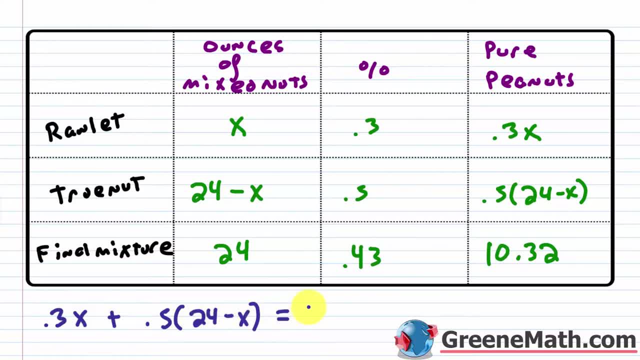 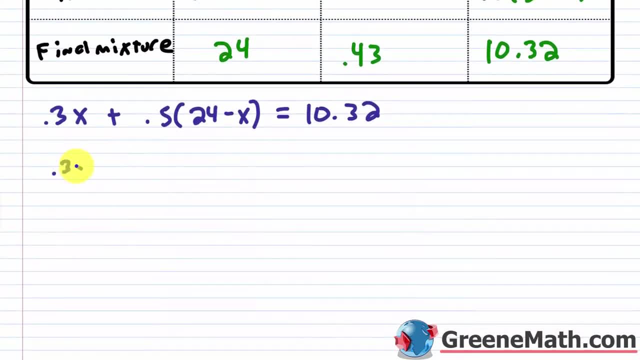 quantity 24 minus x, and then set this equal to my 10.32. so let's solve this and we'll be good to go. so we have our 0.3 x plus 0.5 times 24 is 12. then minus, you have 0.5 times x, which is 0.5 x. 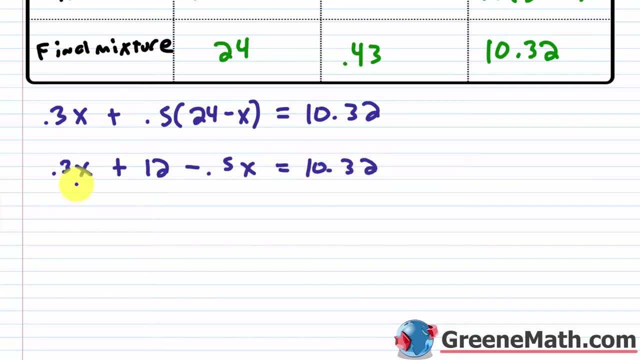 this equals 10.32. 0.3 x minus 0.5 x is going to give us a negative 0.2 x. then you have your plus. let's go ahead and subtract 12 away from each side of the equation and this is going to cancel. 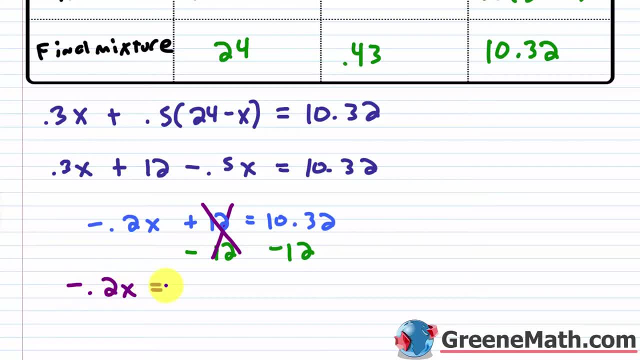 you have your negative 0.2. x is equal to: if i do 10.32 minus 12, i get negative 1.68, so negative 1.68. as a final step, let's divide both sides by negative 0.2 and then this cancels with this. 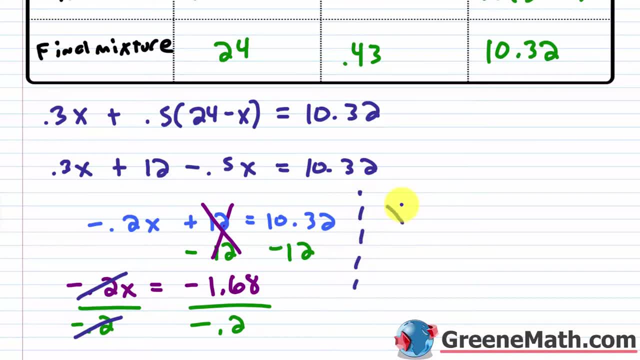 we'll have that. let me kind of make a border here. we'll have that. x is equal to negative. 1.68 divided by 2.2 is going to be 8.4. okay, so 8.4. so let's go back up. so this is going to be 8.4, and then 24. 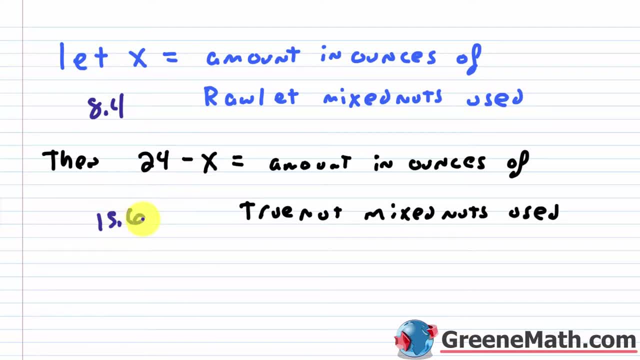 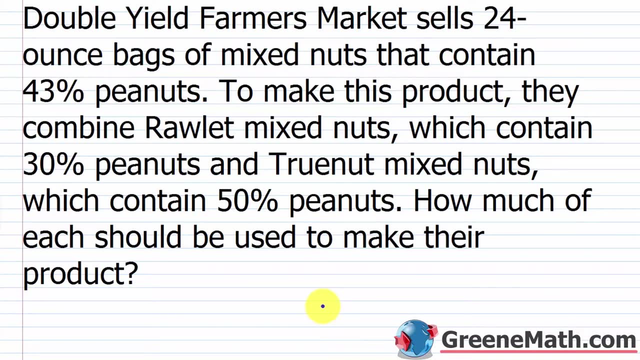 minus 8.4 or 15.6 is going to be the amount in ounces of true nut mix nuts used. so let's go back up. we'll make a nice little sentence here. we'll say that they should use 8.4 ounces of rawlet. 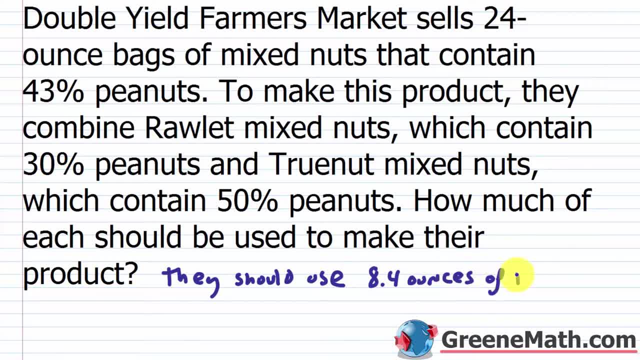 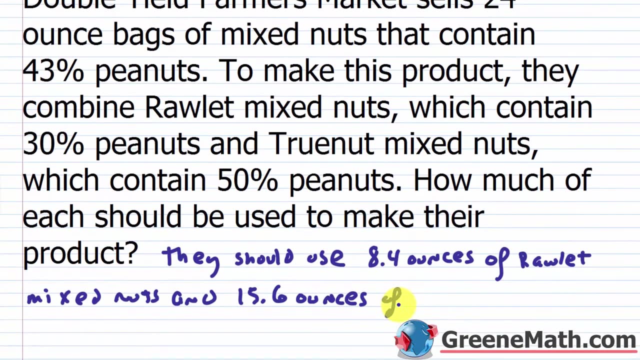 make that better. again, mix nuts and you have 15.6 ounces of true nut mix nuts. so true nut mixed nuts nuts, okay. so again, they should use 8.4 ounces of rawlet mixed nuts and 15.6 ounces of true nut mixed. 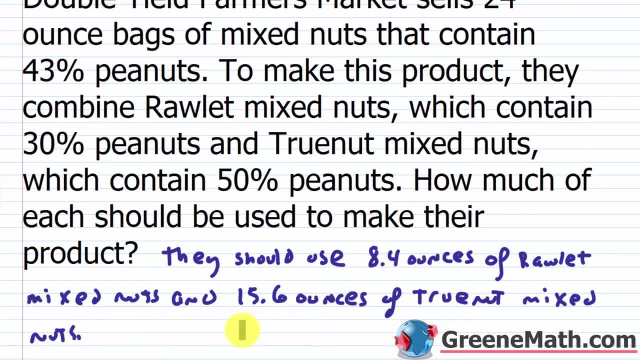 nuts. all right. so to check this, the first thing you want to do is make sure that the a number of ounces coming from rawlet mixed nuts and the number of ounces coming from the true nut mixed nuts match up. so you've got 8.4 ounces coming from rawlet mixed nuts and 15.6 ounces coming from the true nut mixed nuts. that does give you 24 ounces. okay, 15.6 plus 8.4 ounces of true nut mixed nuts. 8.4 would give you 24. so you're good to go there if again we have a 24 ounce bag, that's 43 peanuts. 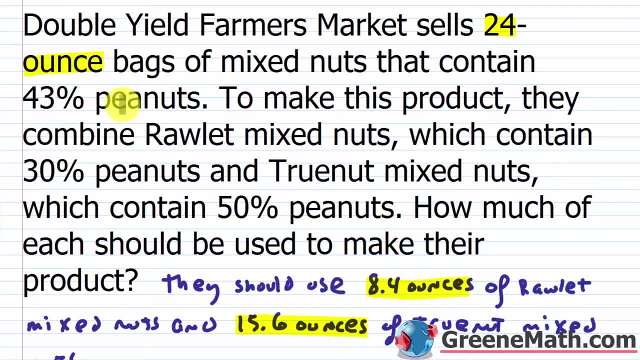 we know there's 10.32 ounces of pure peanuts in that product. now this comes from what? it comes from the rawlet mixed nuts, which is 30 peanuts. so 8.4 times 0.3 is going to give us 2.52. 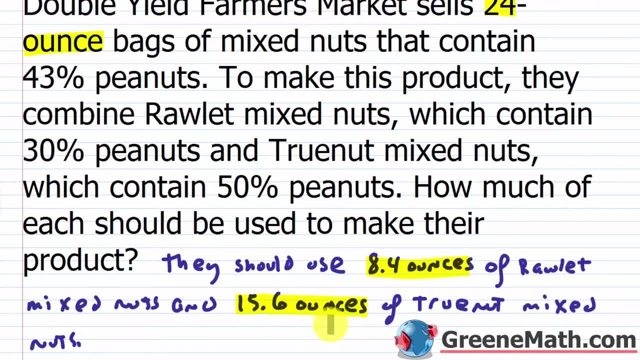 and then it also comes from 15.6 ounces of true nut, mixed nuts, which is 50 percent peanuts. so 15.6 times 0.5 is 7.8. so if you take the 7.8, the amount of pure peanuts coming from true nut. 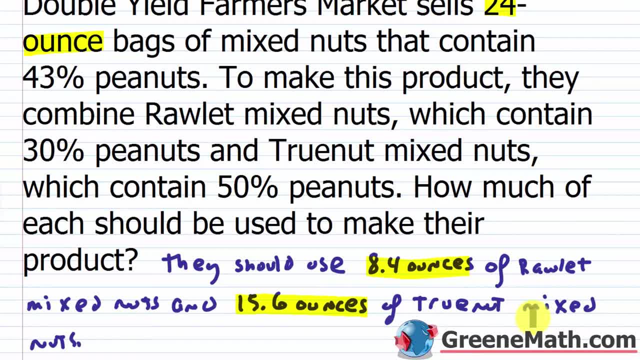 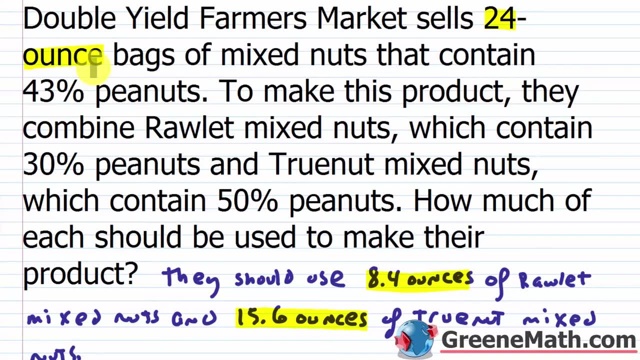 mixed nuts and you add that to the 2.52- again the number of ounces of pure peanuts from the raw mixed nuts, you do get your 10.32, or again the number of ounces of pure peanuts in your final product for the double yield farmers market. so we can say our answer here is correct again. 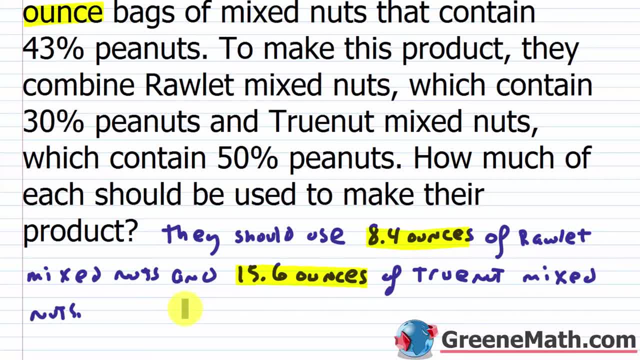 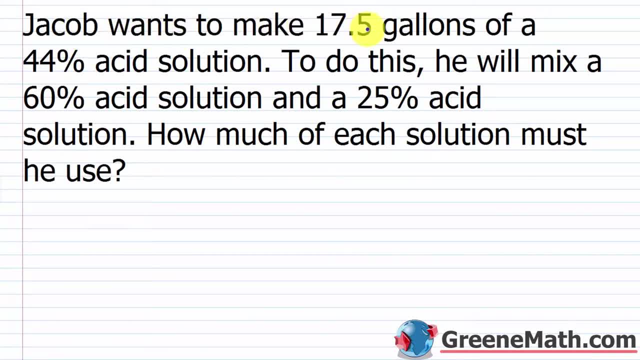 they should use 8.4 ounces of raw mixed nuts and 15.6 ounces of true nut mixed nuts. all right, let's take a look at one more of these. so jacob wants to make 17.5 gallons of a 44 acid solution to do. 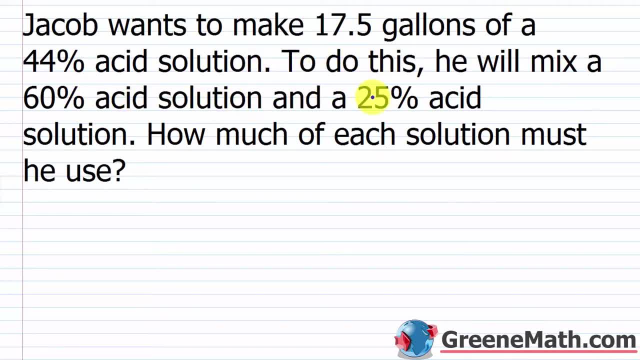 this: he will mix a 60 acid solution and a 25 acid solution. how much of each solution must he use? again, very simple problem. the key to understanding this here again is to think about the final mixture. it's 17.4 gallons of a 44 acid solution. so basically we have 17.5 gallons, 44 of it is pure acid. now 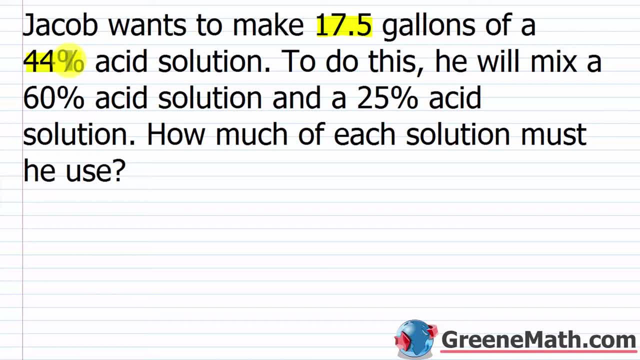 this can only come from what two sources. here we've got a certain number of gallons which is unknown at this point, of a 60 acid solution, and then a certain number of gallons, again unknown at this point, of a 25 acid solution. now, if we let a variable like x, 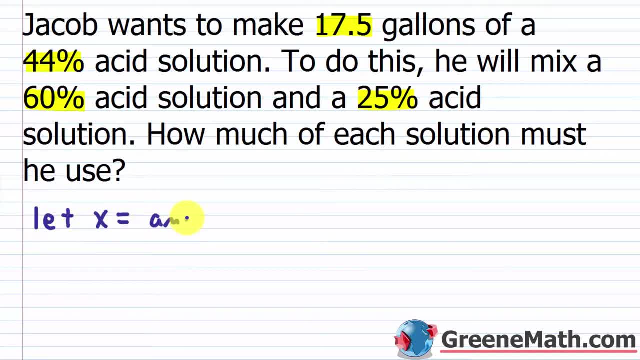 be equal to the amount of pure acid solution. we're going to get a certain number of gallons. if we look at this wishing up here on my data, I get the holders, so we're going to get the total amount in gallons of the 60 acid solution that we're going to use. then what can we say? 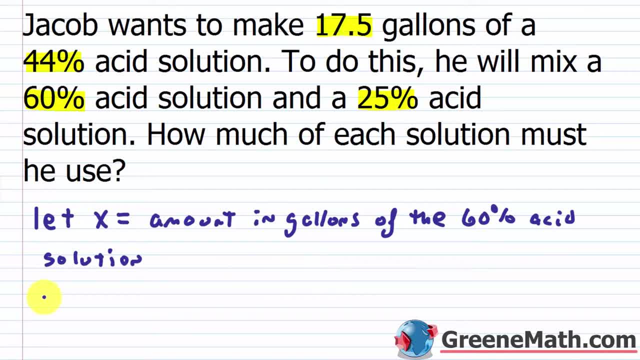 about the amount of the 25 acid solution we're going to use. again, the total amount in gallons is 17.5. so we could say then 17.5 again the total amount in gallons of the final solution, minus an absolute number of gallons: 10, 7 chasing lipline, descending każm proposal: using how much cars a don'tuna want to do this. total amount in gallons of the 65來說. all have to do is see how much you can use this. so 1 million chaud fully дляchair primeッ to 들어가sm can use again: total amount in gallons of the 16.5. so we have to denote per 100 analytical. 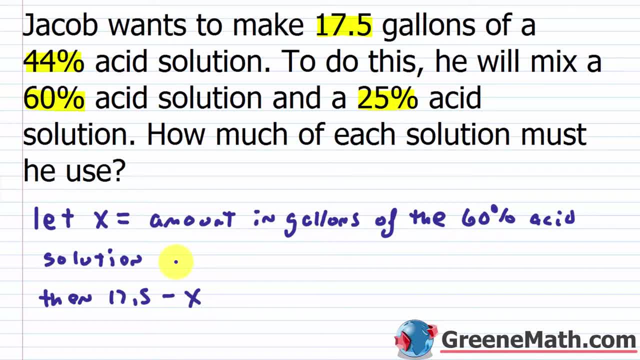 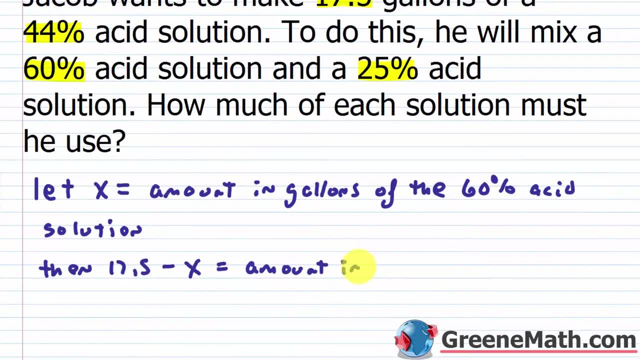 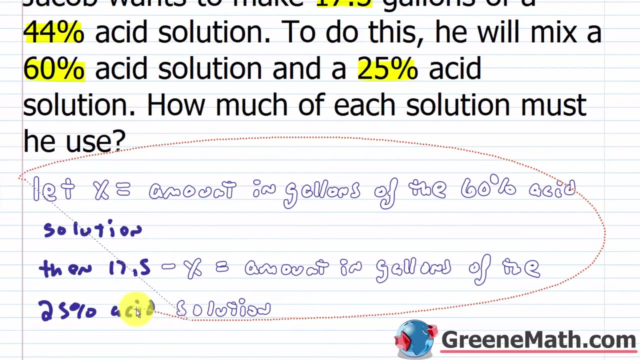 x again, the amount in gallons of the 60 acid solution we're going to use this is going to be equal to the amount in gallons of the 25 acid solution. let me just drag this to another page. so it's nice and clean, so let's go down to a little. 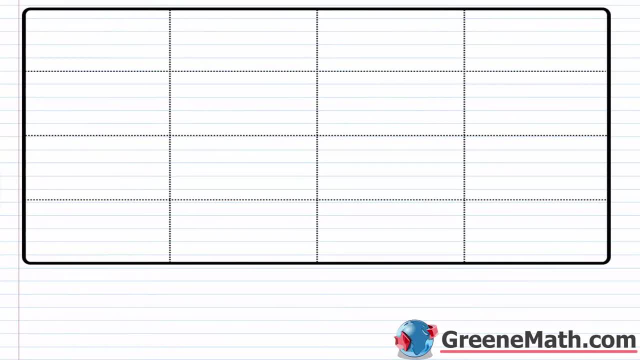 table real quick and let's kind of set this up. so we know that we want to have gallons of the acid solution, so this is gallons, right here. we know we want a percentage concentration basically of acid and then we're going to have the amount of pure acid. 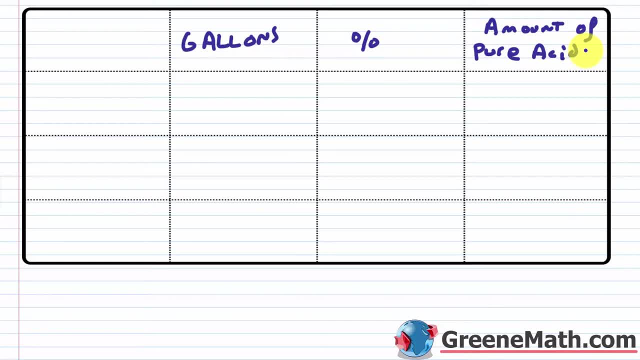 okay, and of course this is going to be in gallons. now we have our 60 acid solution, we have our 25 percent acid solution and then we have our final mixture. okay, so the number of gallons for the final mixture is given to us as 17.5 in the problem. 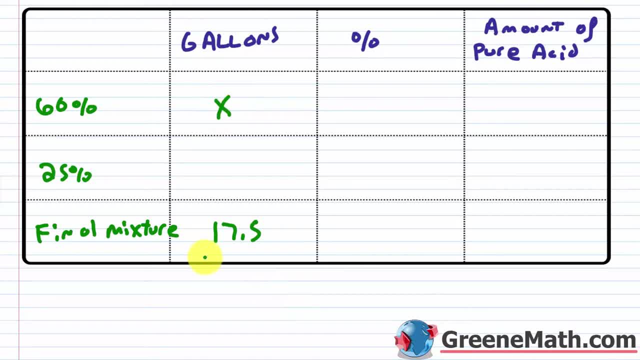 we assigned our variable x to represent the amount of gallons for the 60 acid solution. let me make that clear because it looks like 66. and then we said that 17.5. again the amount in gallons of the final mixture, minus x the amount of gallons for the 60. 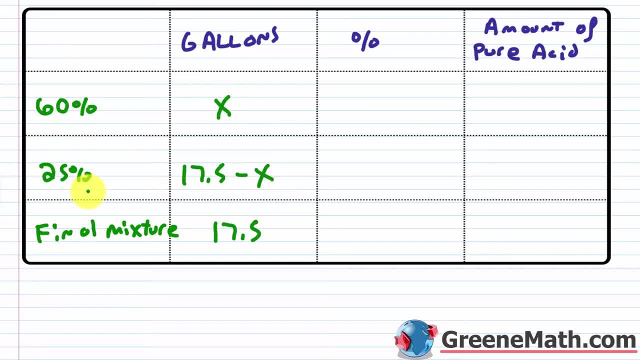 acid solution that we're using is going to be the amount of the 25 acid solution that we're going to use. okay, so we have the number of gallons modeled for each. the percentage is very easy because it's off to the left, right, so this one right here is going to be 0.6, as 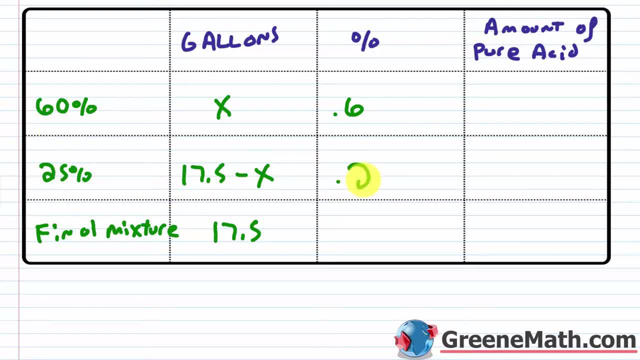 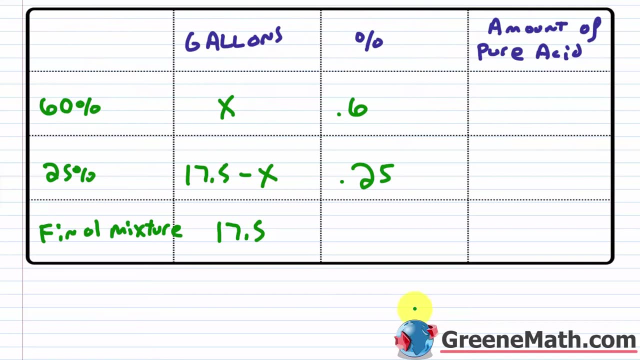 a decimal right, that's 60 percent, and this one right here would be 0.25 as a decimal, that's 25 percent. so the final mixture we are told is 44 percent. again, jacob wants to make 17.5 gallons of a 44 acid solution. so as a decimal, 44 is 0.44. so to get the amount of pure acid in gallons for, 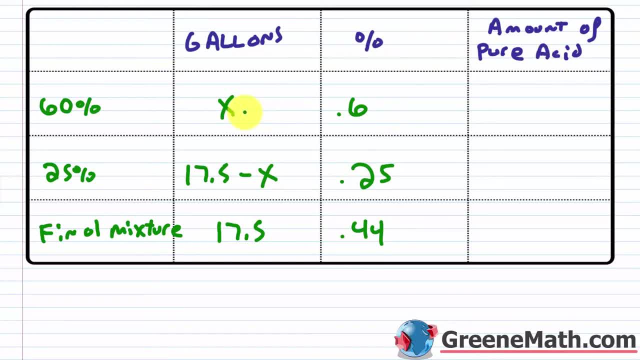 each. i would just multiply across. so i have x gallons and it's 60 percent pure acid. so 0.6 times x is 0.6 x. i have 17.5 minus x gallons: it's 25 pure acid. so 0.25 times the quantity 17.5 minus x. 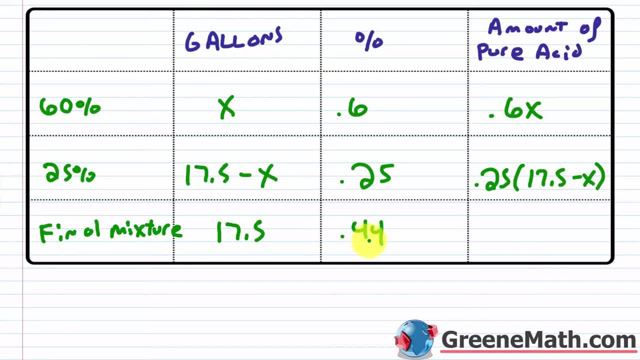 and then my final mixture is 44 acid and it's 17.5 gallons. if we multiply those together you get 7.7. so this is the amount of pure acid in the final mixture: it's 7.7 gallons. now for our equation. 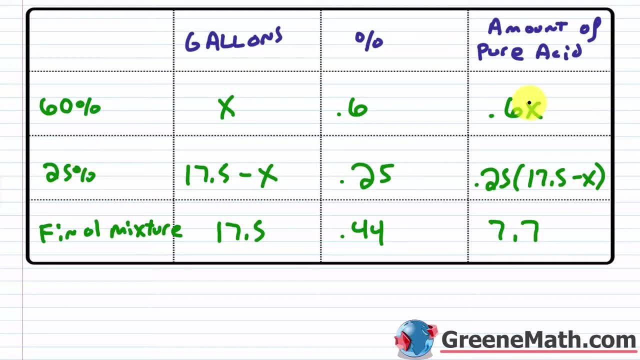 again, we use a similar format. we think about the amount of pure acid coming from the 60 acid solution, which is 0.6 x, plus the amount of pure acid coming from the 25 acid solution, which is 0.25 times the quantity 17.5. 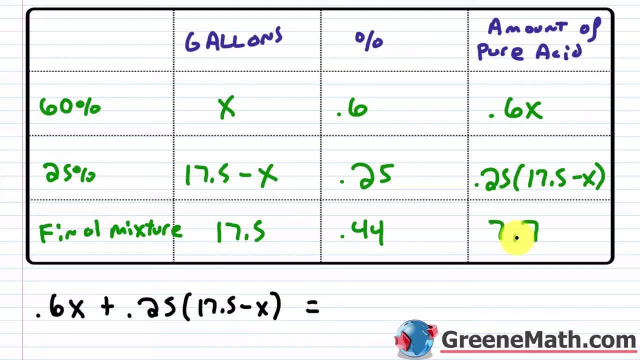 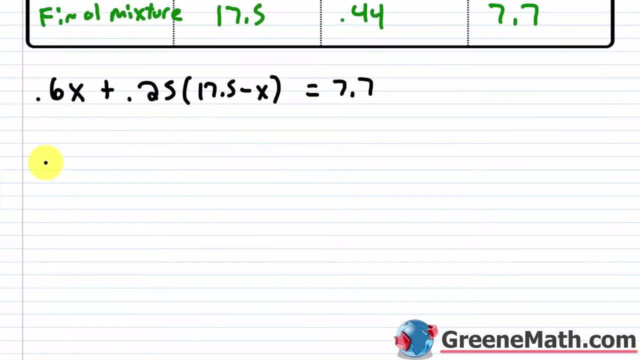 minus x. this has to be equal to the amount of pure acid in the final mixture, right? so 7.7. okay, so let's solve this equation. we'll be good to go. so we have that: 0.6 x plus 0.25 times 17.5 is 4.375. 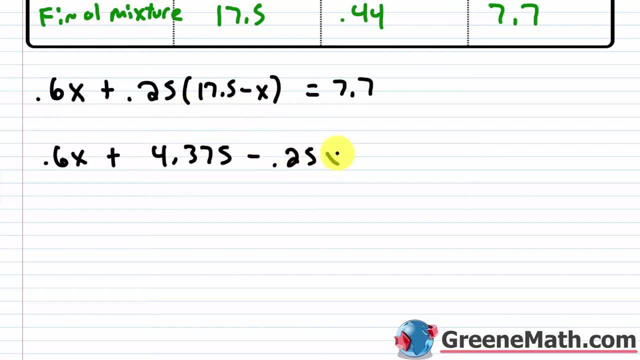 and then minus 0.25 times x is 0.25 x, and this equals 7.7. okay, so let's clean up on the left: 0.6 x minus 0.25 x is 0.25x, 0.35x, So 0.35x. And then if I subtract 4.375 away from each side, what will I get? Well, 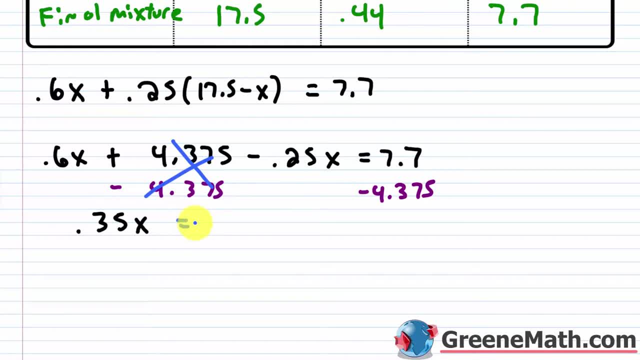 we know this would cancel. So we'll say this is equal to 7.7 minus 4.375 is 3.325.. All right, So to finish this up, let's divide both sides of the equation by 0.35.. So we'll. 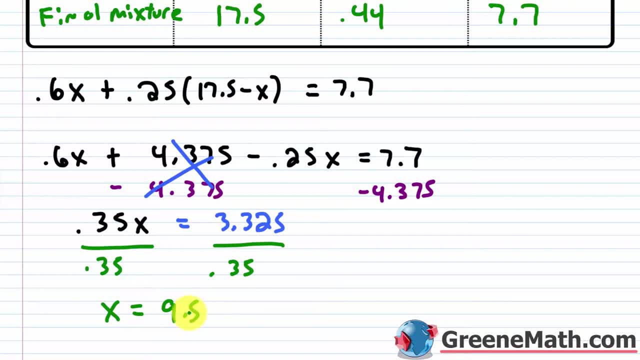 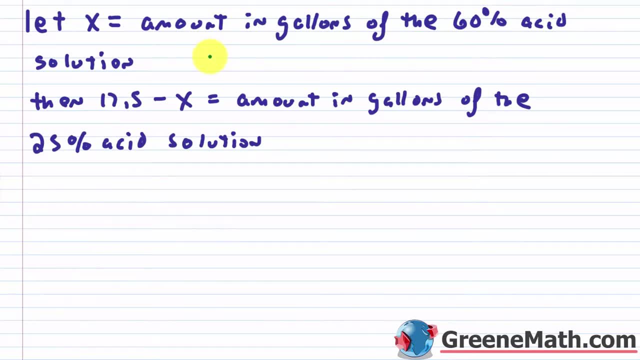 get. x is equal to 9.5.. Okay, So let's go back up. So again, we said that x was the amount in gallons of the 60% acid solution, So this is going to be 9.5.. And then 17.5. 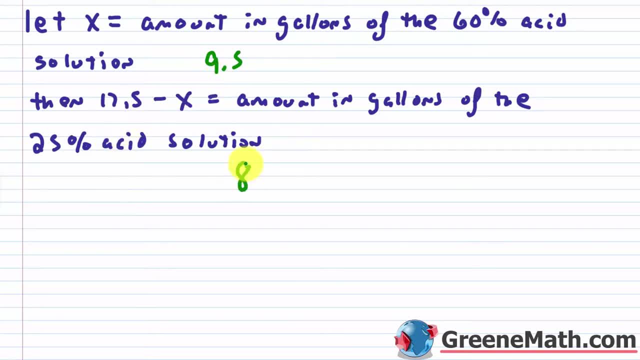 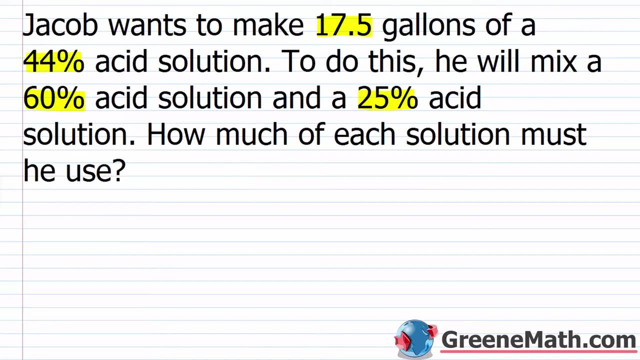 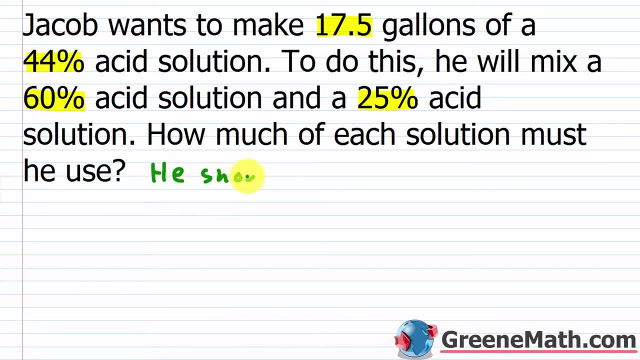 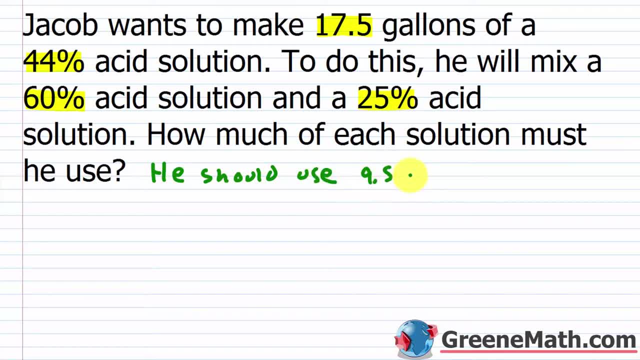 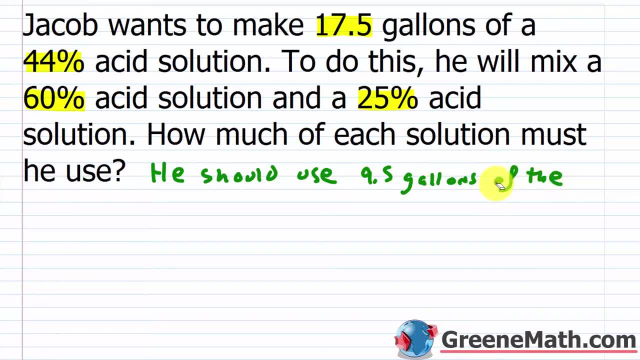 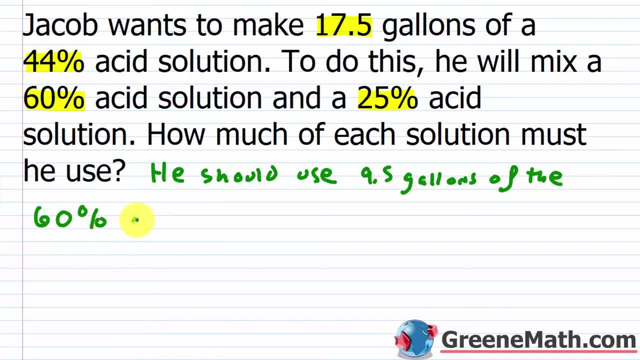 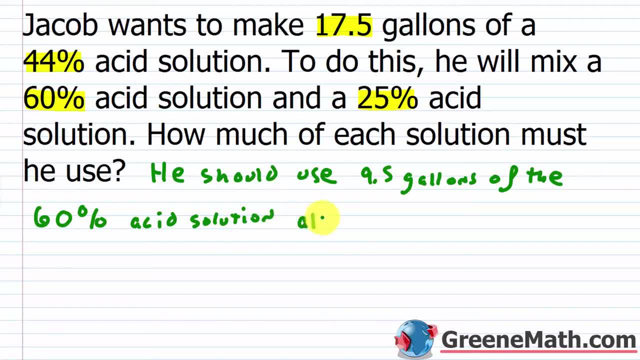 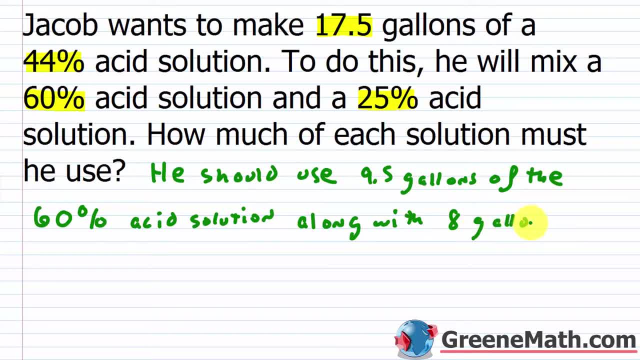 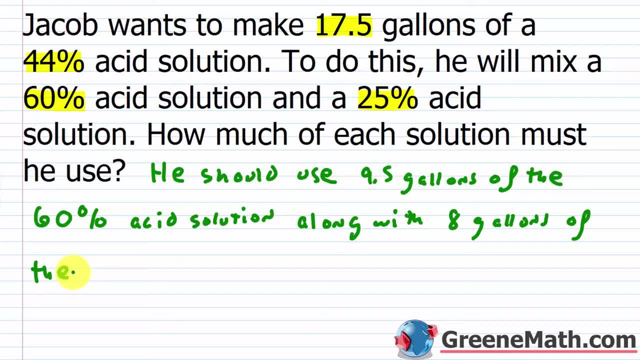 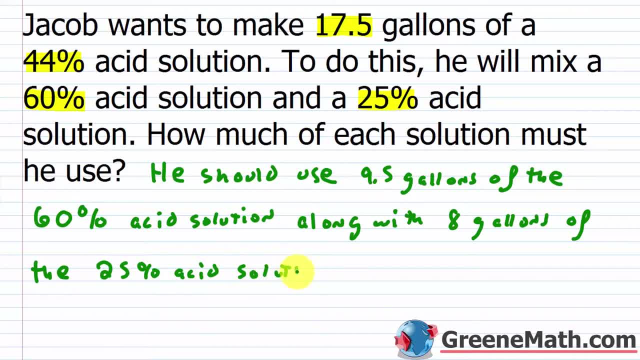 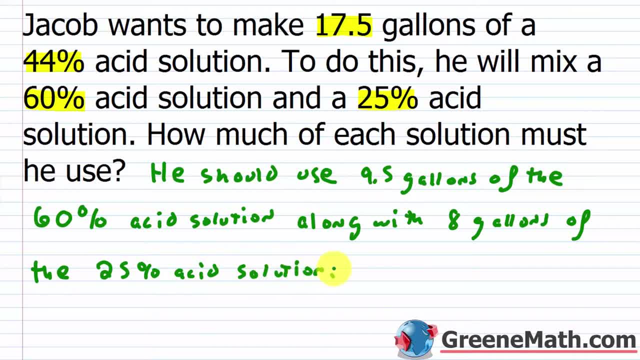 again very easy to check. First, you would say, is 9.5 plus 8, the gallons coming from each source. if you add those together, is that 17.5, right? The number of gallons in the final mixture that he has? Well, yes, it is right. 9.5 plus 8 is 17.5.. So that. 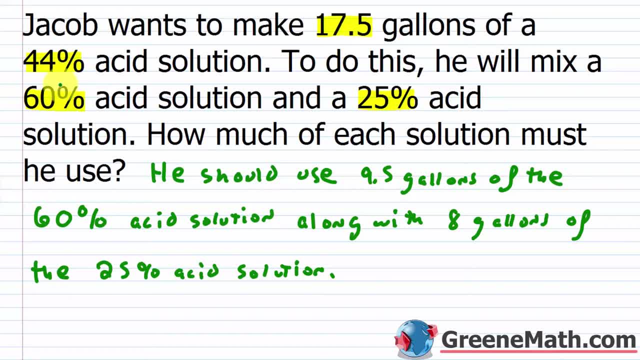 part checks out. All right Now next, remember he has 7.7 gallons of pure acid in the final solution. that came from multiplying 17.5, the number of gallons in the final mixture times 0.44.. Again, that's the number of gallons in the final mixture. So that's. 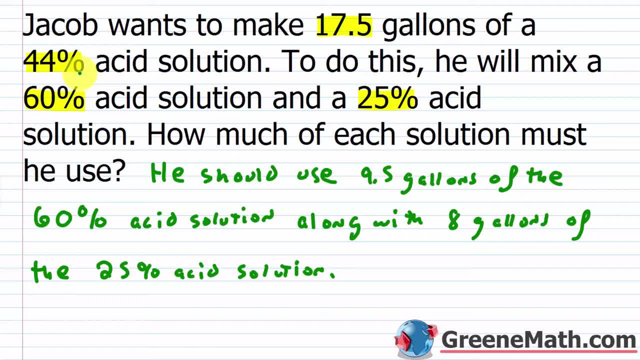 7.7 gallons of pure acid in the final mixture. So that comes from two sources. From one source he has 9.5 gallons, that's 60% acid. So that would be 5.7, 5.7 gallons of pure acid Then. 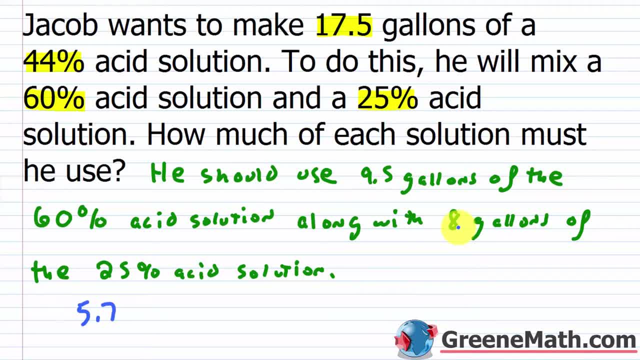 lastly, he has 8 gallons. that's 25% acid. So 8 times 0.25 is 2.. So if you add 2 to 5.7, you do get 7.7, right? So you've checked the amount of pure acid in the final mixture. 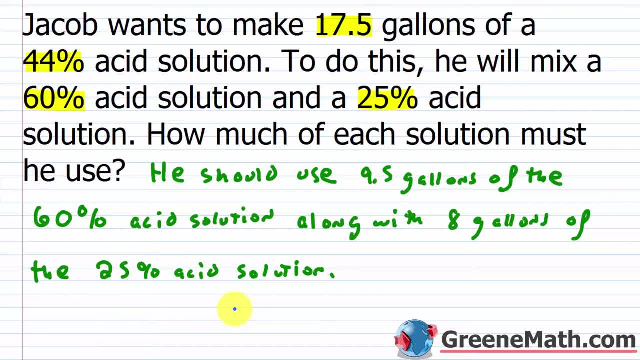 That matches up And you've checked the number of gallons of the final mixture. That matches up, So we can say our solution here is correct. He should use 9.5 gallons of the 60% acid solution along with 8 gallons of the 25% acid solution. In this lesson we want to 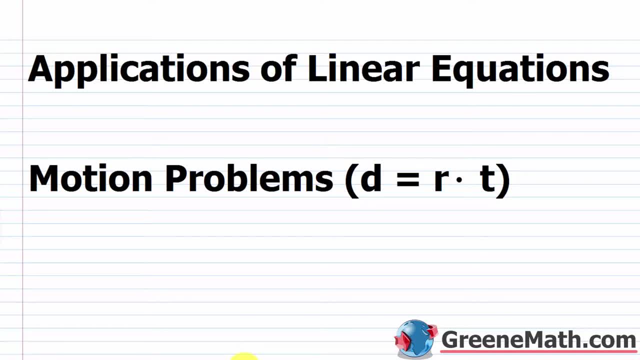 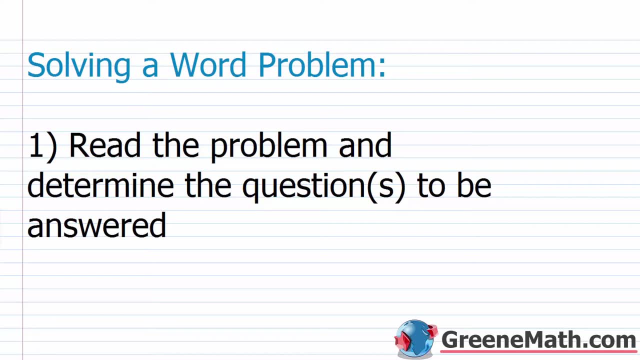 review applications of linear equations And, specifically, we're going to look at motion word problems. All right, So let's just go through our procedure real quick on how to solve a word problem. This is just a general guideline, something you can use as your. 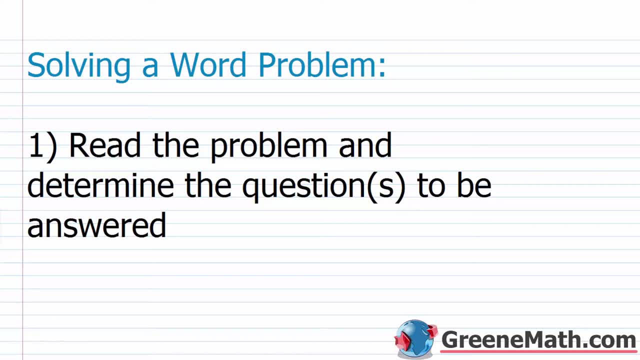 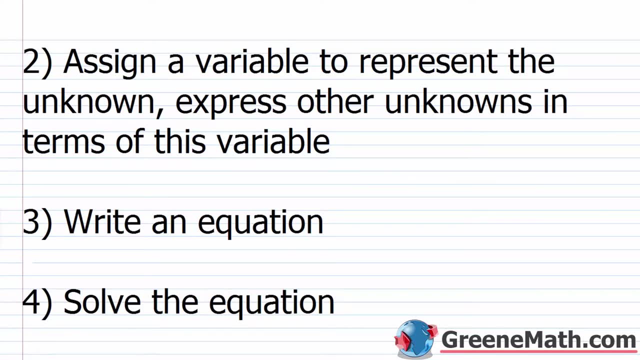 problem. So the first thing is just to read the problem and determine the question or, in some cases, questions to be answered. The next thing is to assign a variable to represent the unknown, Express other unknowns in terms of this variable. Then we want to write an. 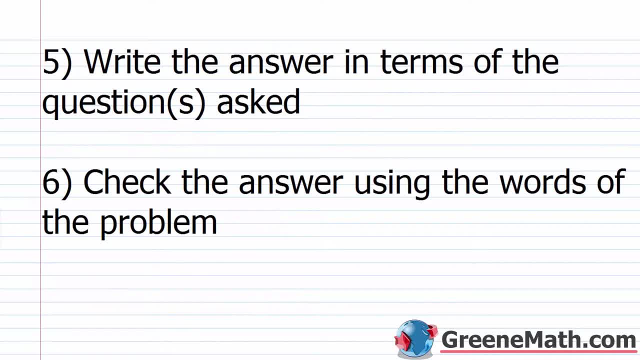 equation, Then we're going to solve the equation, Then we're going to write the answer in terms of the question or the questions being asked And then, lastly, we're going to check the answer using the words of the problem. All right, So for motion, word problems a lot. 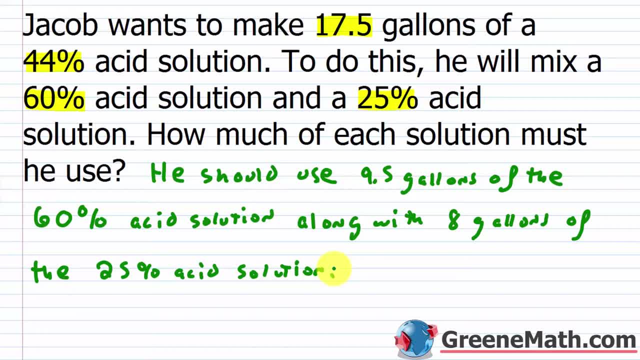 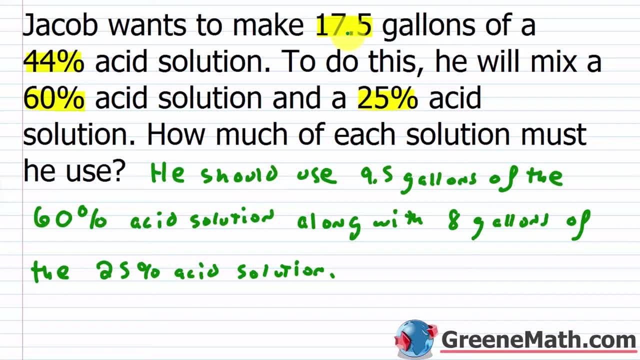 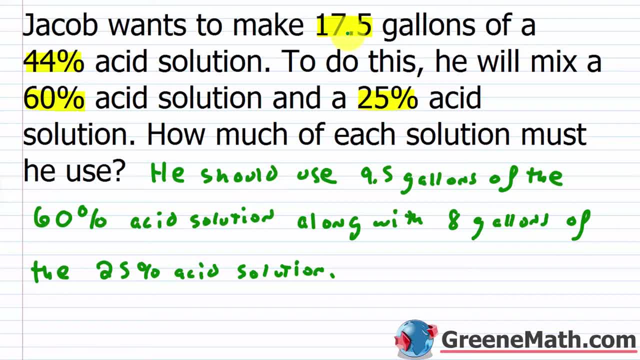 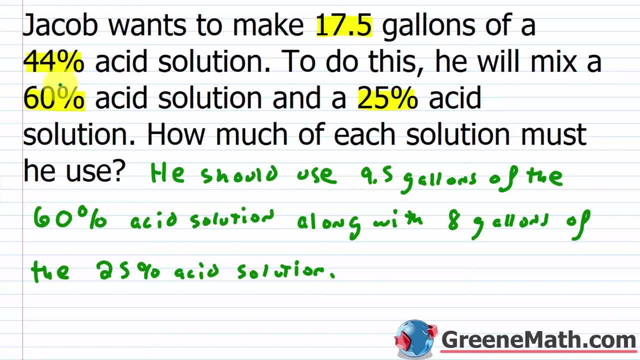 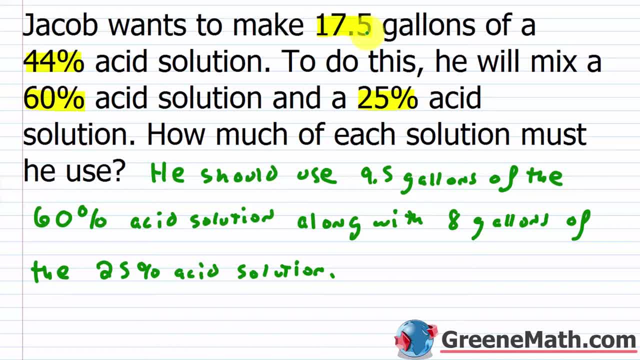 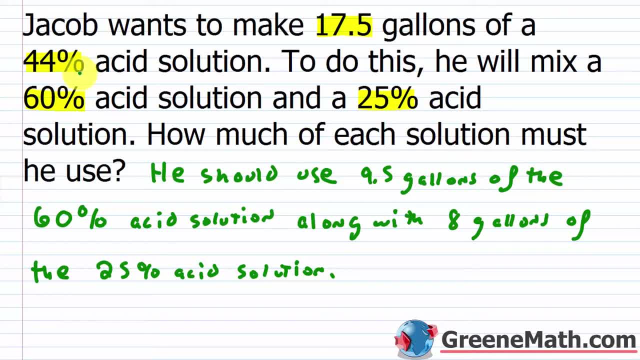 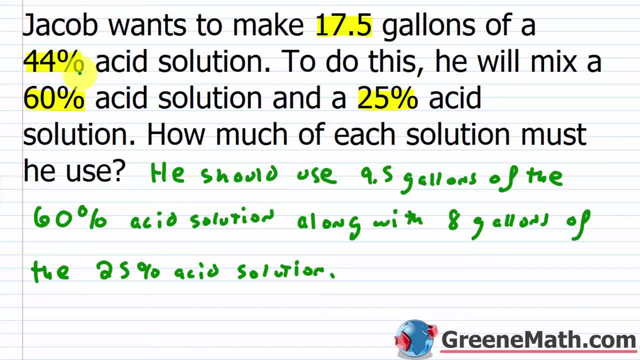 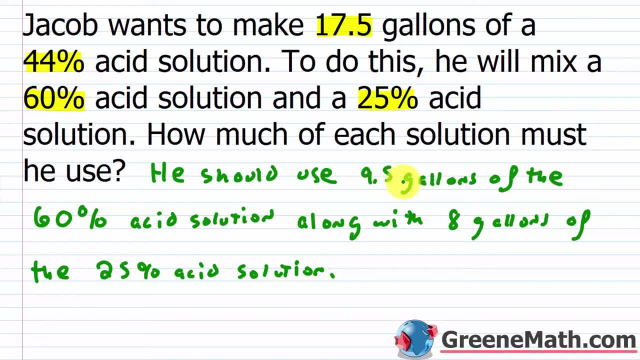 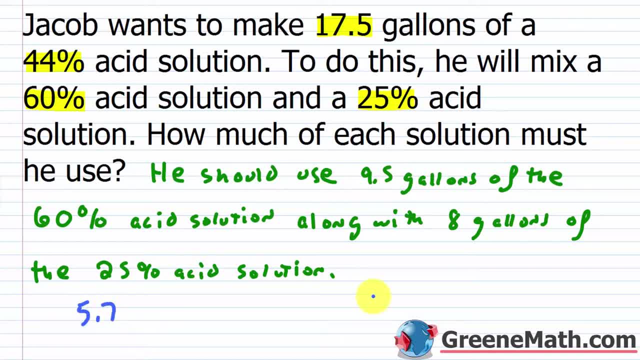 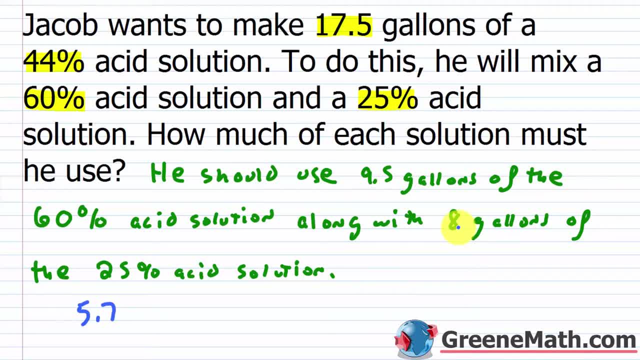 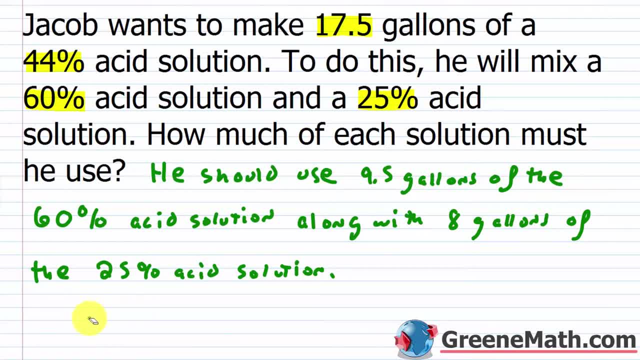 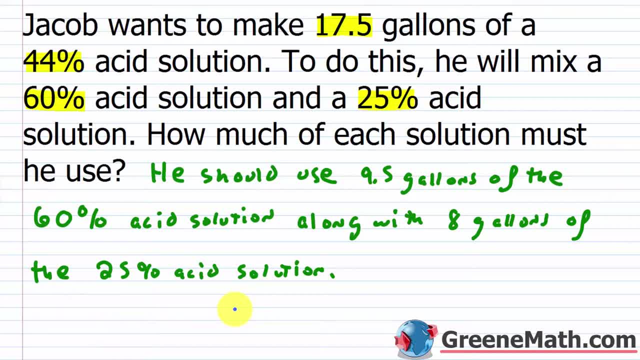 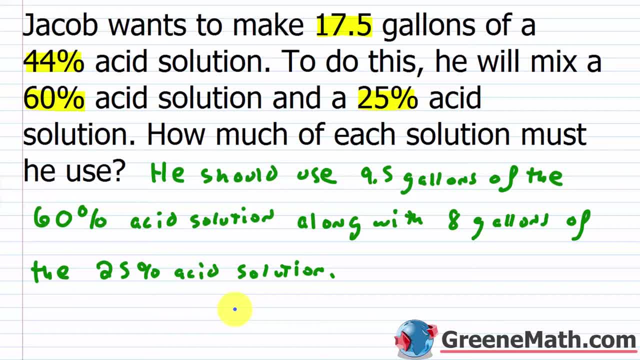 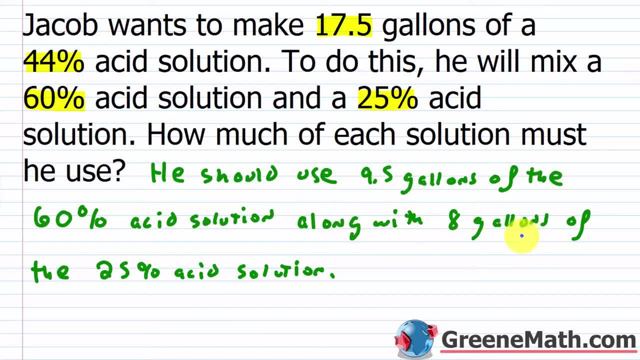 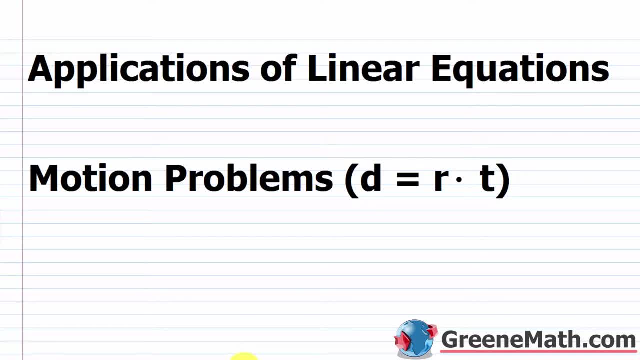 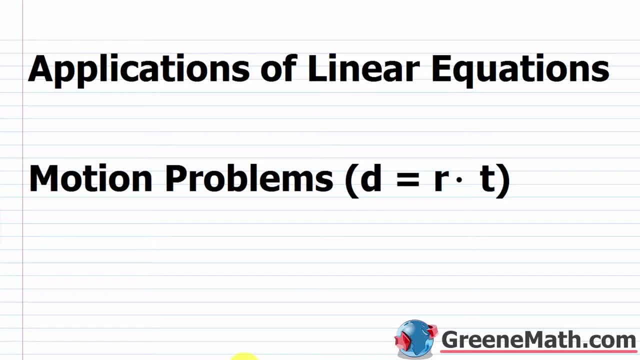 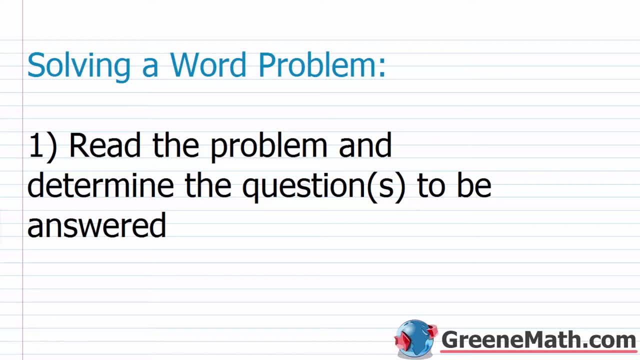 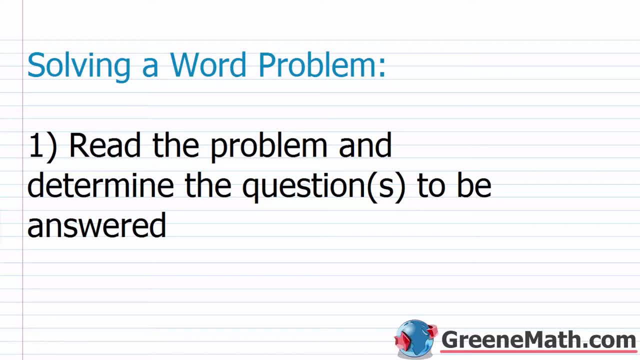 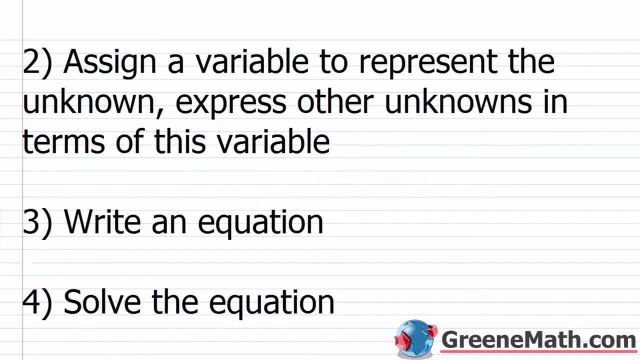 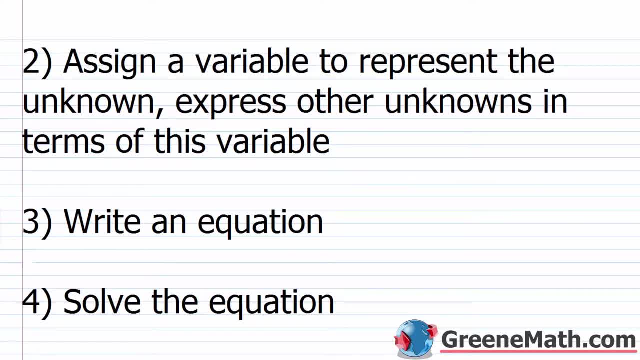 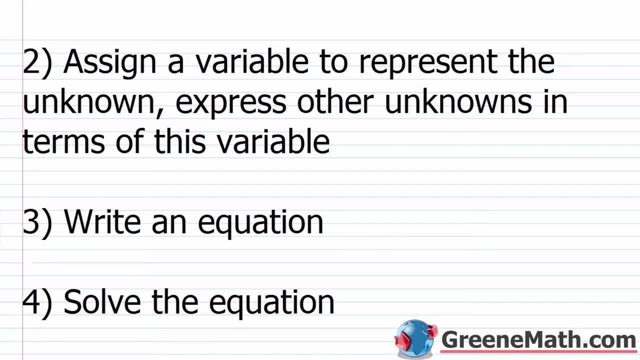 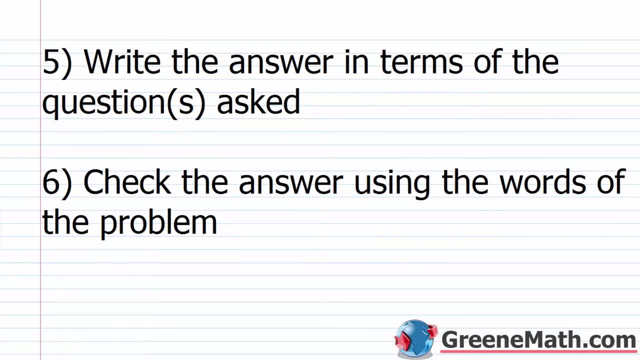 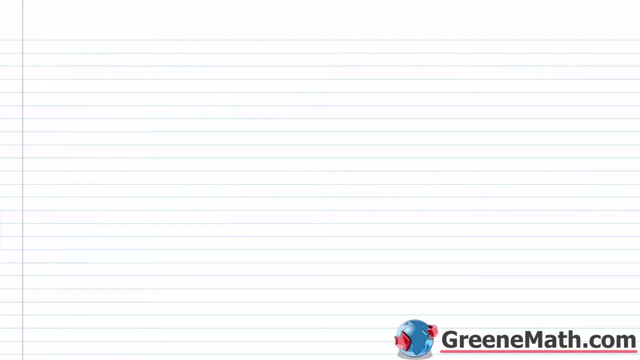 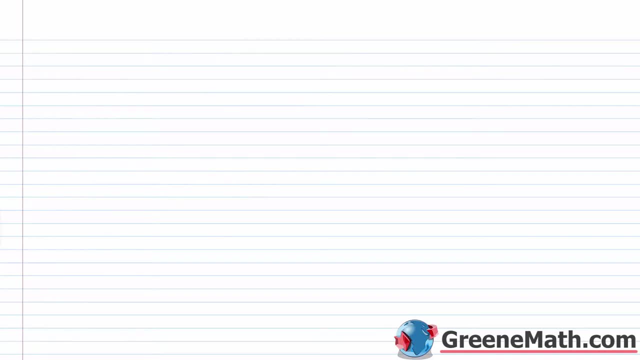 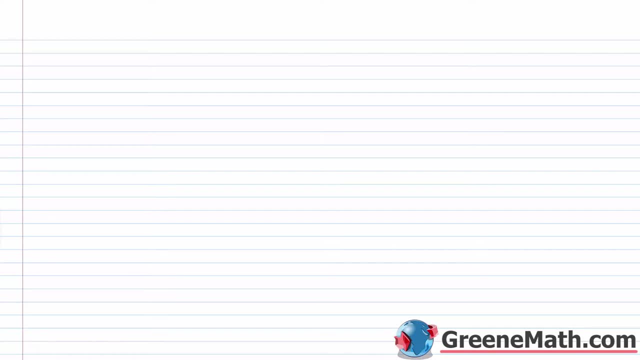 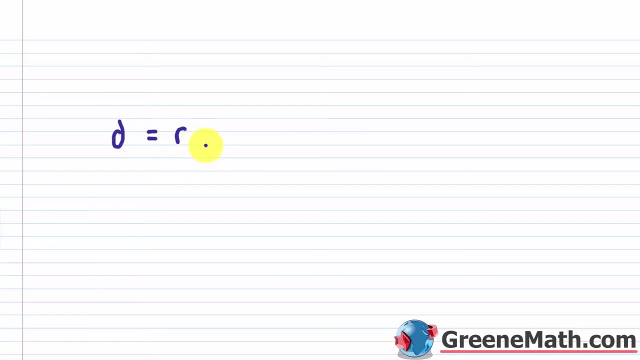 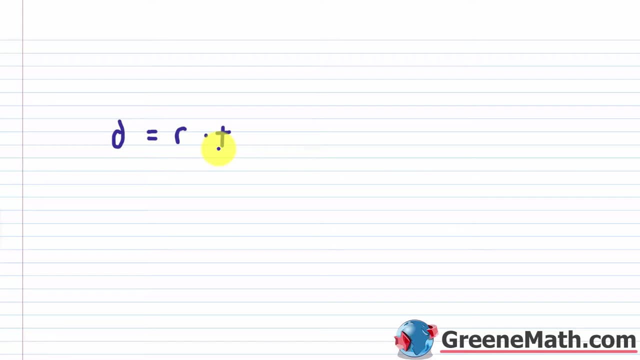 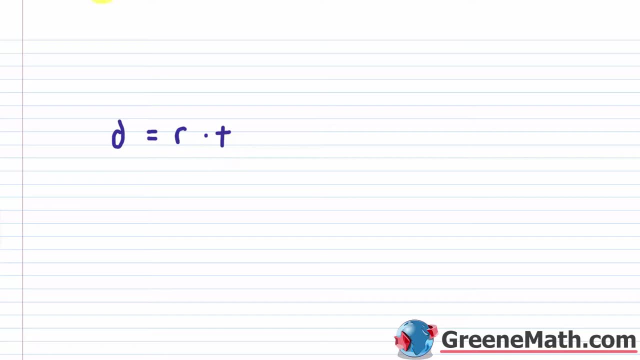 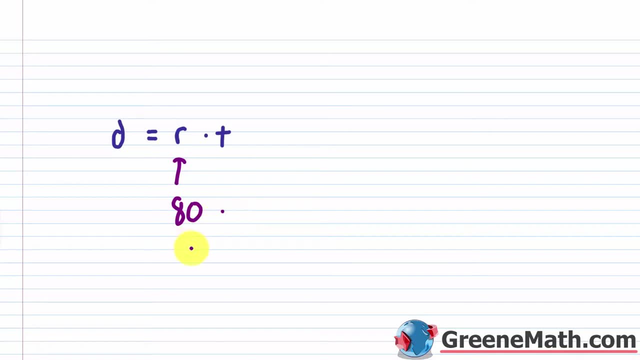 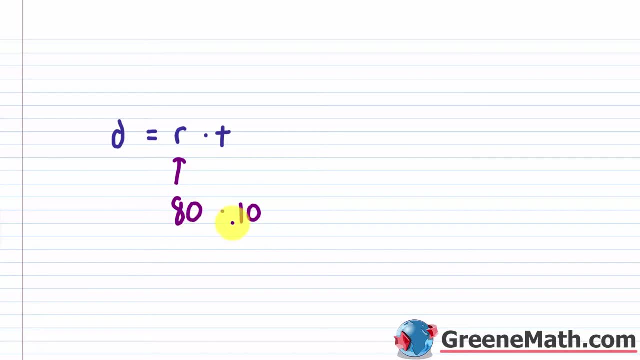 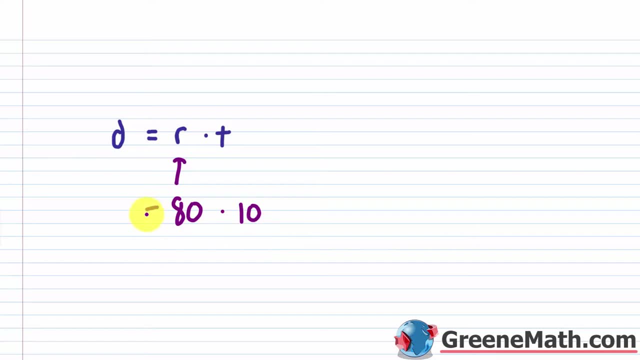 80.. The amount of time is 10.. 80 times 10 is 800. So your distance is 800 miles. Okay, So it's a very intuitive formula, something you can kind of work out in your head, If you just kind of can't. 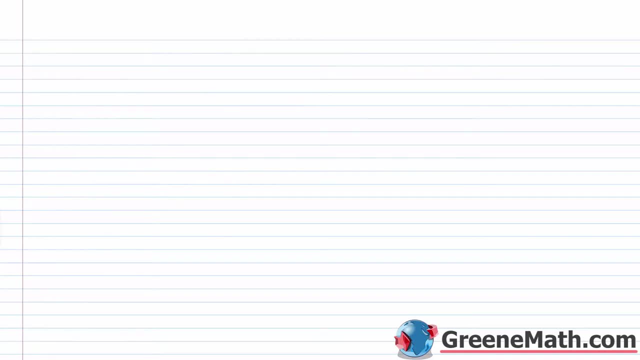 of people take lower level algebra courses Got a lot of experience with these. It's a very common type of word problem. They rely on the understanding of the formula. D or distance is equal to R for rate of speed times, T the time traveled. It's a very intuitive formula. 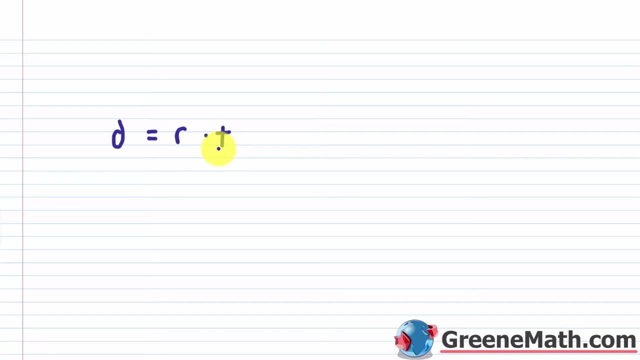 Think about being on a road trip and let's say your rate of speed is 80 miles per hour. So let's say this is 80 miles per hour and I'll just write 80. And then you do this for, let's say, 10 hours. 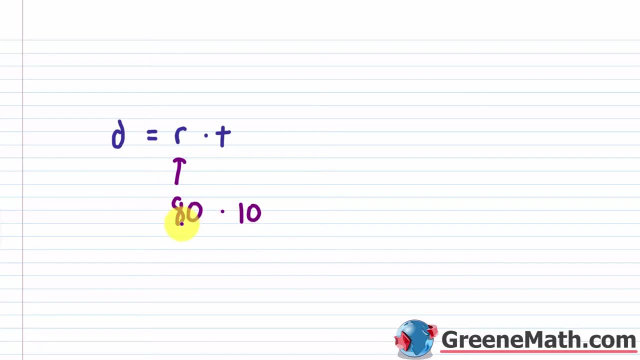 How far did you go in terms of miles? Well, you just multiply. The rate of speed is 80.. The amount of time is 10.. 80 times 10 is 800.. So your distance is 800 miles. Okay, So it's. 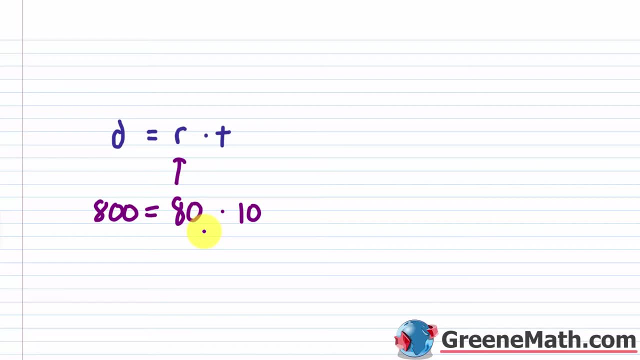 a very intuitive formula, something you can kind of work out in your head. If you just kind of can't remember the distance formula, think about being on a road trip and saying, okay, if I'm going at this rate of speed for this amount of time, well, I can multiply. 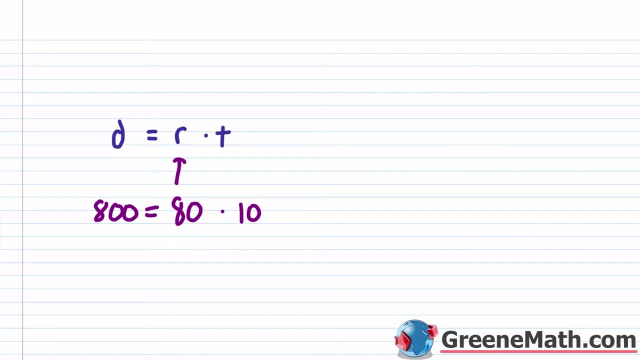 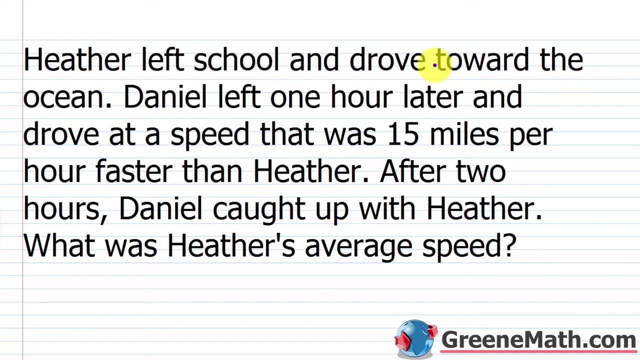 those two numbers together to get my distance. All right, Let's look at our first example. So we have that. Heather left school and drove toward the ocean. Daniel left one hour later and drove at a speed that was 15 miles per hour faster than Heather. After two hours, Daniel caught up with Heather. What was Heather's? 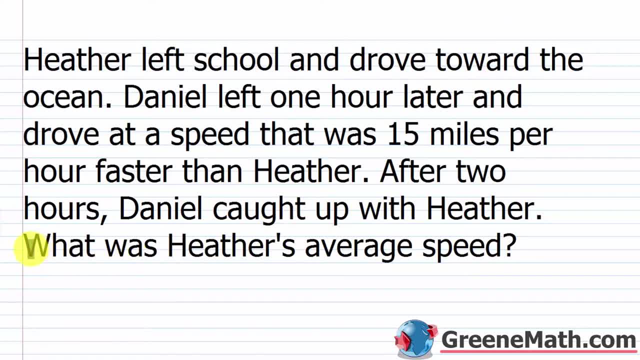 average speed. So this is what we need to answer here: What was Heather's average speed? That's the key. Take the second to look at the problem and understand the question that you're being asked. That's where a lot of students really, you know they read the problem. They don't really. 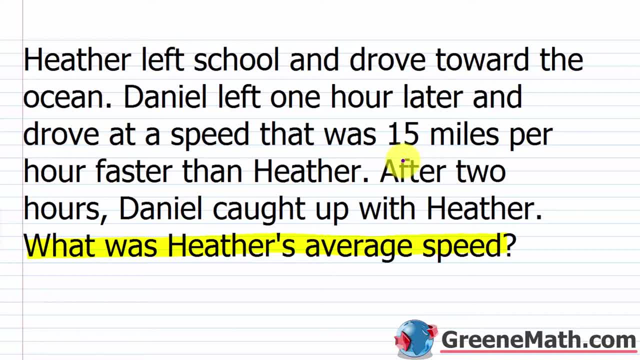 understand what they're being asked. So they're like: what do I do? Okay, That's what you've got to understand. What was Heather's average speed? So now we're ready to kind of go through the problem, And the first thing that I'm going to do is just let a variable you can 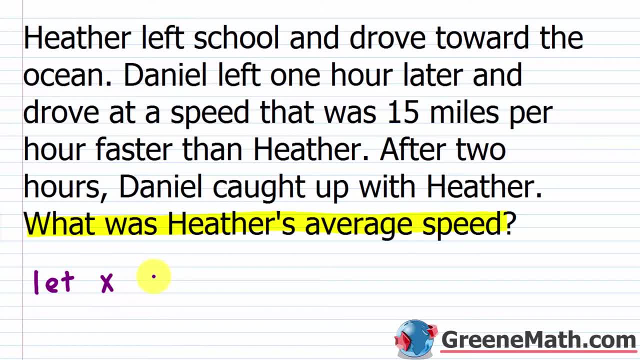 let it be X, or it could be Y or Z. whatever you want to use, Doesn't matter. So let X be equal to. what am I looking for? I'm looking for Heather's average speed, So let's let X be equal to Heather's average speed. 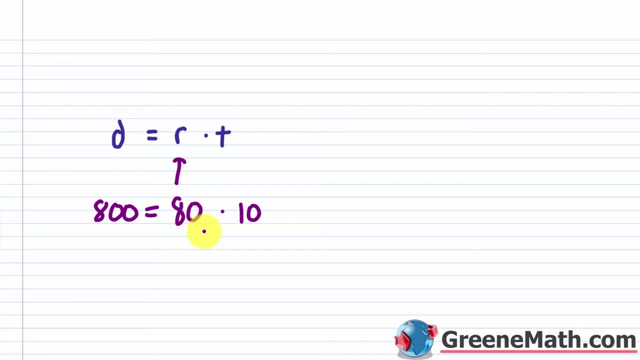 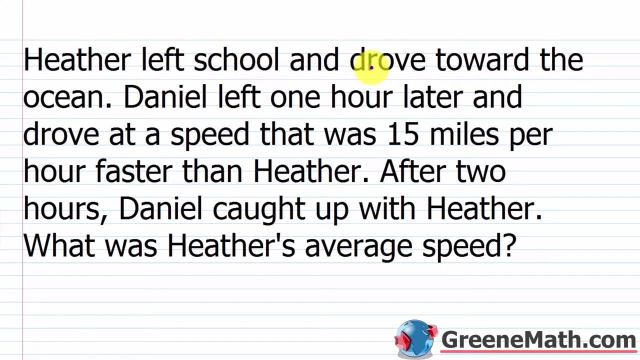 remember the distance formula. think about being on a road trip and saying, okay, if I'm going at this rate of speed for this amount of time, well, I can multiply those two numbers together to get my distance. All right, Let's look at our first example. So we have that Heather left school and 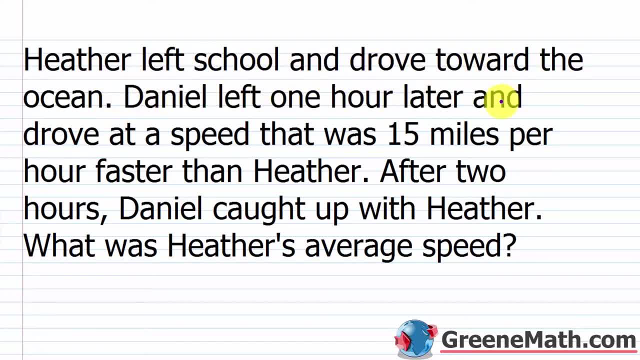 drove toward the ocean. Daniel left one hour later and drove at a speed that was 15 miles per hour faster than Heather. After two hours, Daniel caught up with Heather. What was Heather's average speed? So this is what we need to answer here: What was Heather's average speed? That's the key. 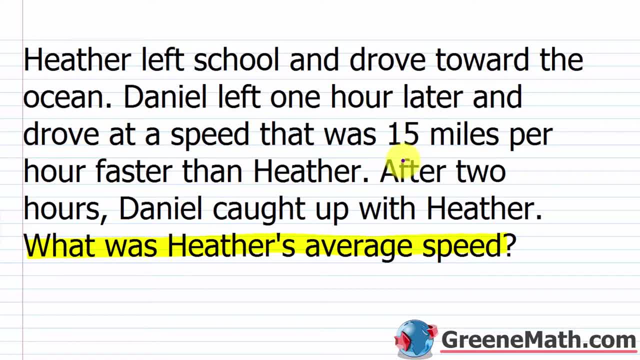 Take the second to look at the problem and understand the question that you're being asked. That's where a lot of students really, you know they read the problem. They don't really understand what they're being asked, So they're like: what do I do? Okay, That's what you've got to understand. What was Heather's? 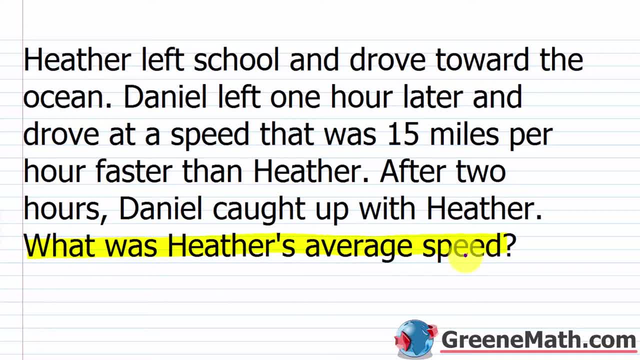 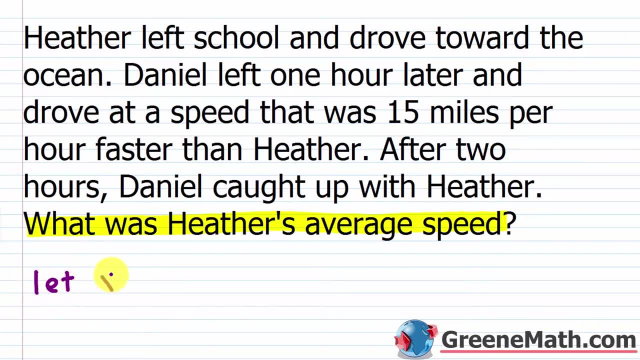 average speed. So now we're ready to kind of go through the problem, And the first thing that I'm going to do is just let a variable- you can let it be X, or it could be Y or Z, whatever you want to use, It doesn't matter. So let X be equal to. what am I looking for? I'm looking for Heather's. average speed, So let's let X be equal to X. I'm looking for Heather's average speed, So let's let X be equal to X. So let's let X be equal to X. I'm looking for Heather's average speed, So let's let 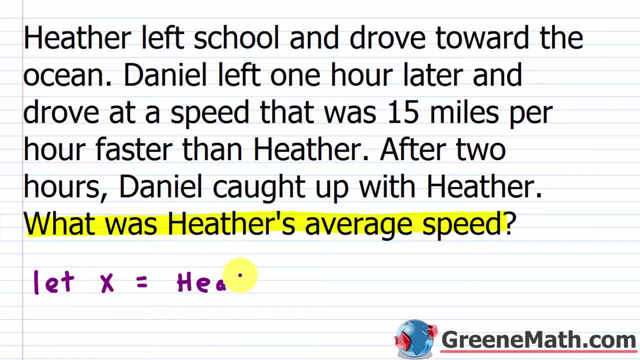 X be equal to Heather's average speed. okay, And this is going to be in terms of miles per hour, because that's what we're working with in the problem. Now we need to model other unknowns in terms of this variable X. 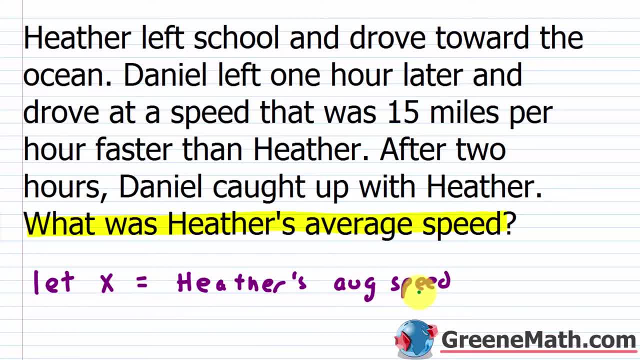 So we have Heather's average speed modeled, but we don't have Daniel's average speed modeled. Well, Daniel, it tells us in the problem that he's driving 15 miles per hour faster than Heather. okay, Well, if Heather's average speed is X? 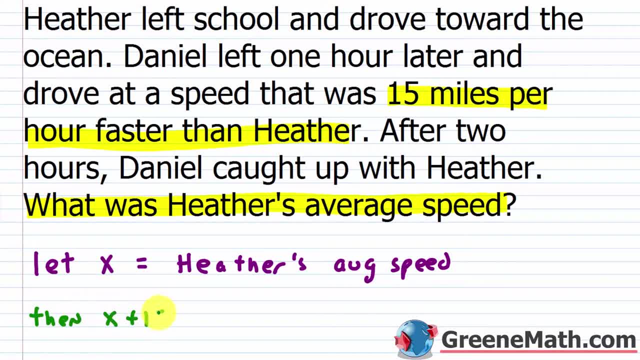 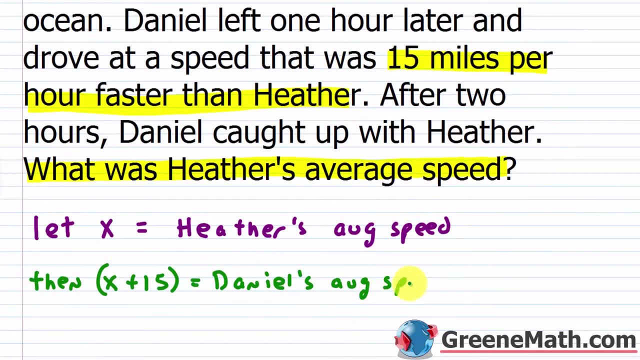 then we can say that X plus 15, okay, that amount there is going to be Daniel's average speed. okay, So this is Daniel's average speed. okay, Let me make those a little bit better. All right, so with this information, 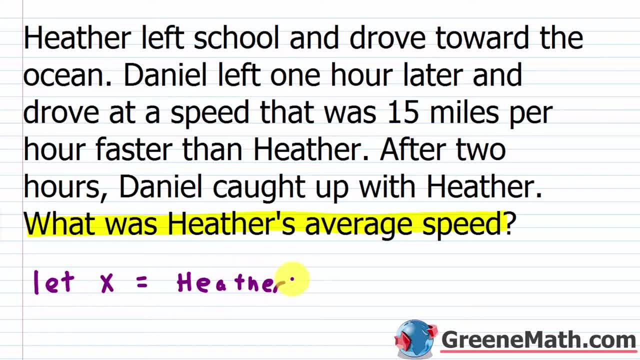 Okay, Okay, So we're going to have Heather's average speed Okay, And this is going to be in terms of miles per hour, because that's what we're working with in the problem. Now we need to model other unknowns in terms of this variable X. So we have Heather's average speed modeled. 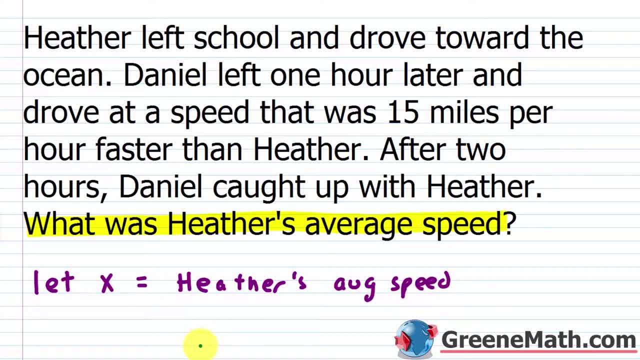 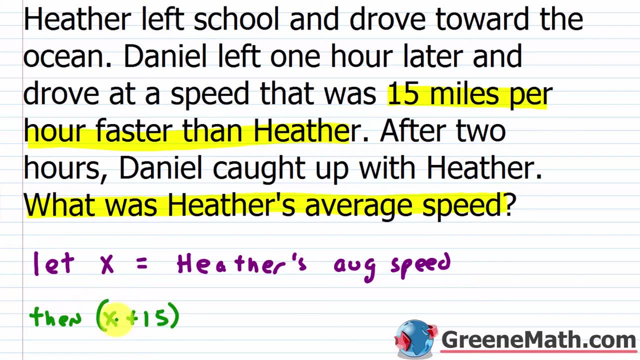 but we don't have Daniel's average speed modeled Well. Daniel, it tells us in the problem that he's driving 15 miles per hour faster than Heather. Okay, Well, if Heather's average speed is X, then Then we can say that X plus 15, okay that. 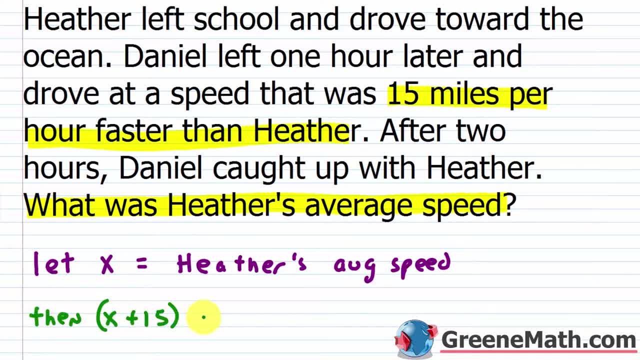 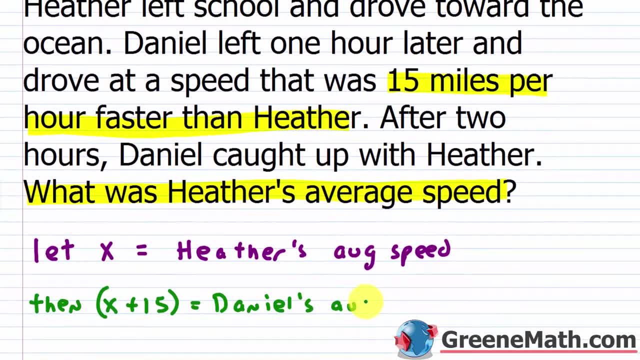 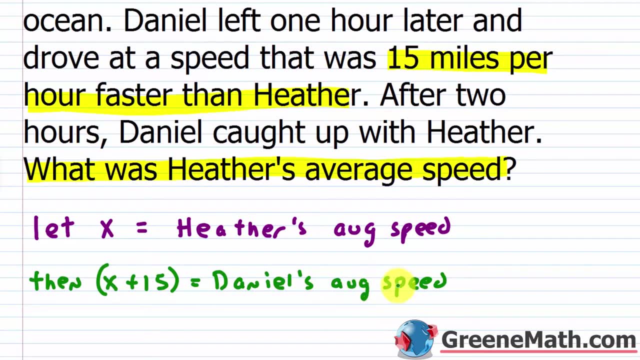 amount there is going to be Daniel's average speed. Okay, So this is Daniel's average speed. Okay, We're going to make those a little bit better. All right, So with this information, we can take this to a table. Okay, And I'm going. 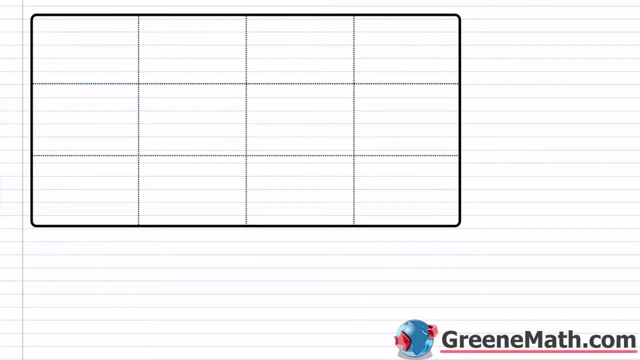 going to show you this table real quick. This is something you can use to kind of organize your thoughts, Okay, So in this case I'm going to put the names on the left, So I can just kind of put it as the names if I want, and that's going to go down like this. So let's put H for Heather and 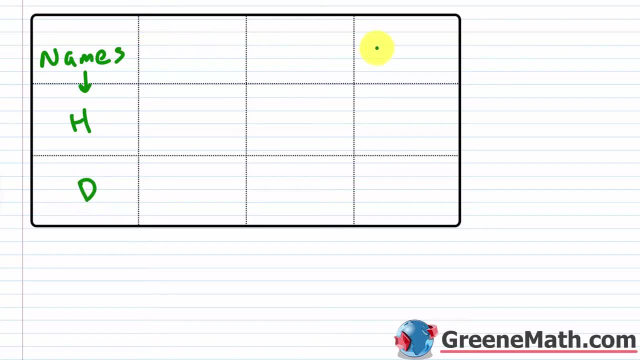 let's put D for Daniel, to the right here in the top. I'm going to put D for the distance. This is equal to my R, which is the rate of speed multiplied by my T, which is the amount of time it traveled. So we already know for Heather, her rate is X and for Daniel, his rate is X plus 15.. 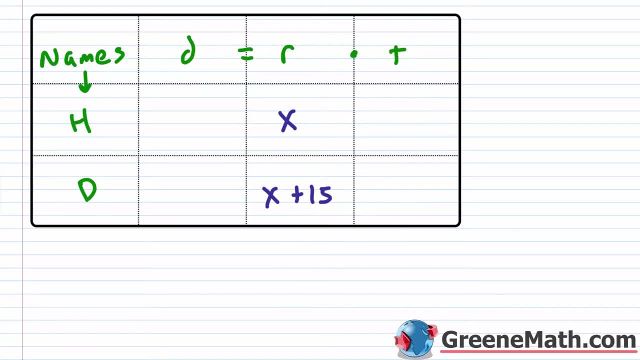 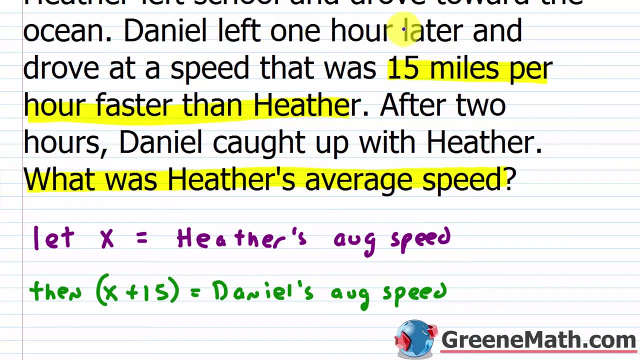 Okay, What about the time? Let's go back up and see if we can figure that out. So it tells us in the problem specifically that Daniel left one hour later- Okay, So he drives for an hour less than Heather does when they catch up, Okay, Or when they're at the same point. So it says: 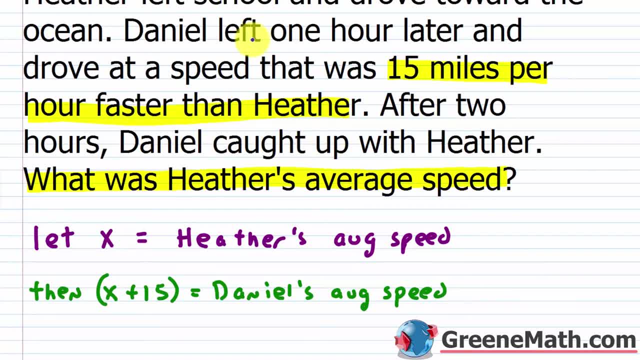 after two hours Daniel caught up, And it also says he left one hour later. Okay, So that means that Daniel was driving for two hours, because it says, specifically after two hours Daniel caught up. And it tells us also that, again because Daniel left one hour later than Heather, that 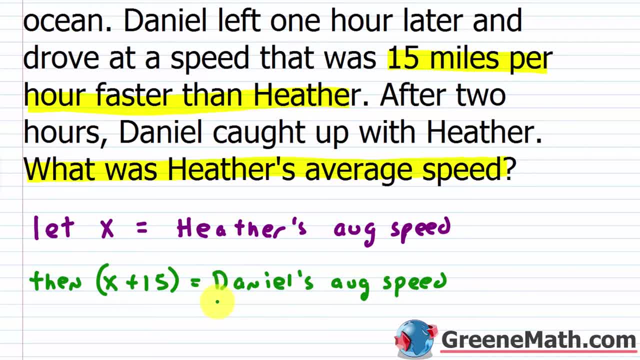 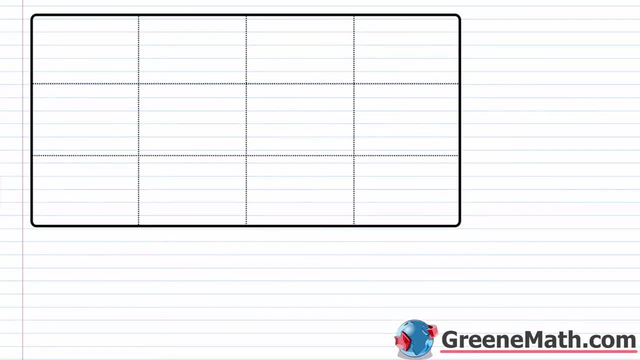 we can take this to a. we can take this to a table, okay, And I'm going to show you this table real quick. This is something you can use to kind of organize your thoughts, okay. So in this case, I'm going to put the names on the left. 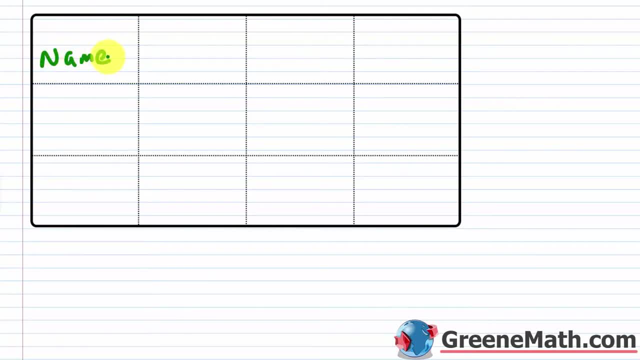 So I can just kind of put it as the names, if I want, and that's going to go down like this. So let's put H for Heather and let's put D for Daniel. To the right here in the top I'm going to put D for the distance. 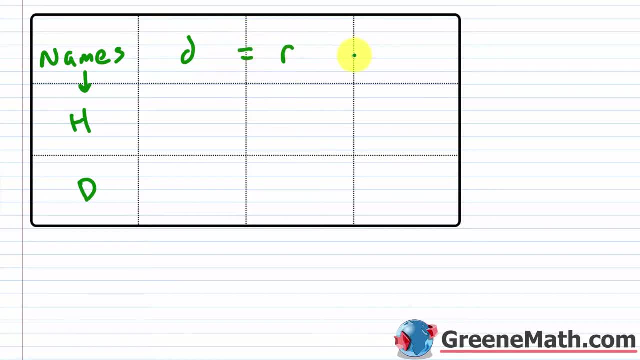 This is equal to my R, which is the rate of speed, multiplied by my T, which is the amount of time traveled. So we already know: for Heather, her rate is X And for Daniel, his rate is X plus 15, okay. 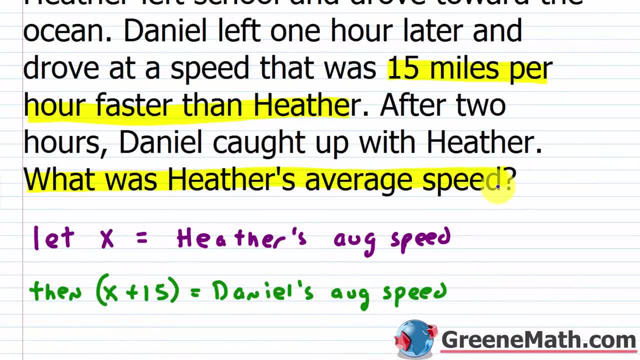 What about the time? Let's go back up and see if we can figure that out. So it tells us in the problem specifically that Daniel left one hour later, okay, So he drives for an hour less than Heather does when they catch up, okay, or when they're at the same point. 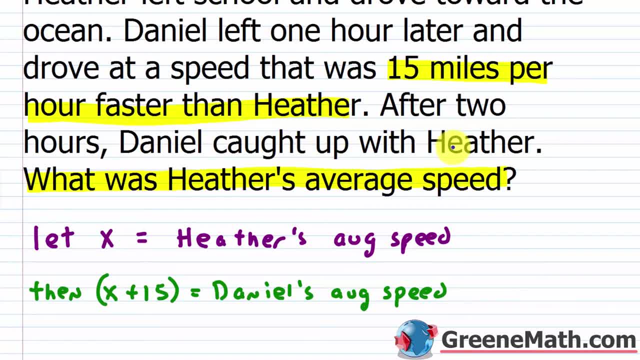 So it says after two hours, Daniel caught up, and it also says he left one hour later. okay, So that means that Daniel was driving for two hours, because it says specifically after two hours Daniel caught up, And it tells us also that again. 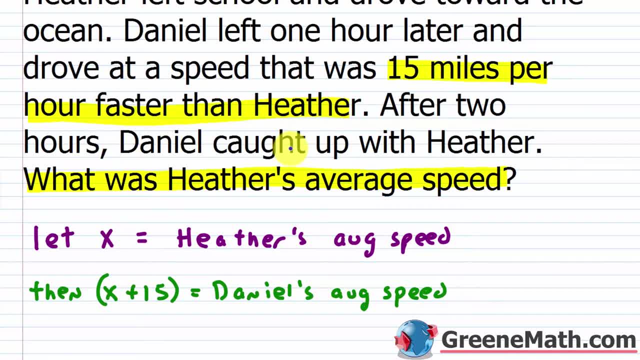 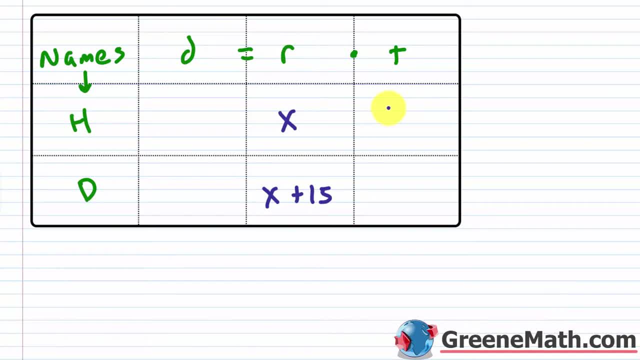 because Daniel left one hour later than Heather, that Heather was driving for an hour more, so she was driving for three hours. So I can fill this out and say Heather was driving for three hours, Daniel was driving for two. Now I can get the distance by multiplying these two together, okay. 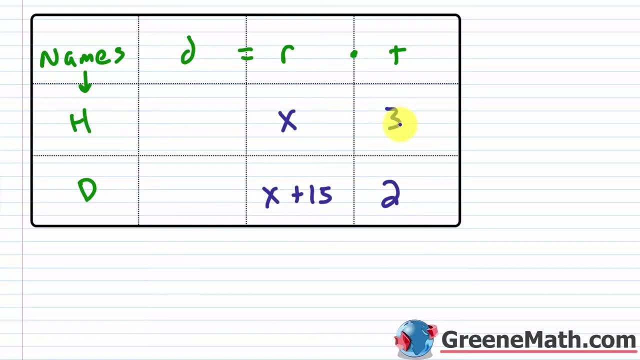 So in other words, the distance that Heather travels is the amount of time she travels for times the rate of speed that she travels at. So three times X is 3X. That's my distance for Heather, Two times the quantity X plus 15. 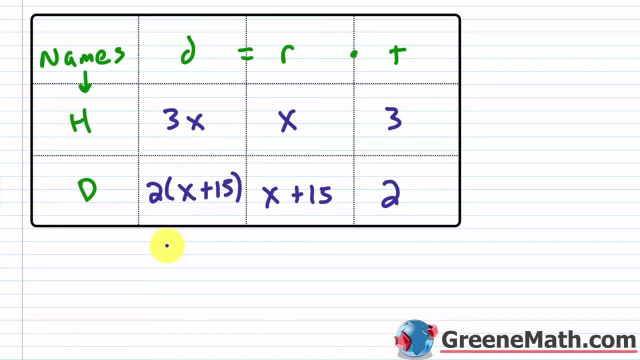 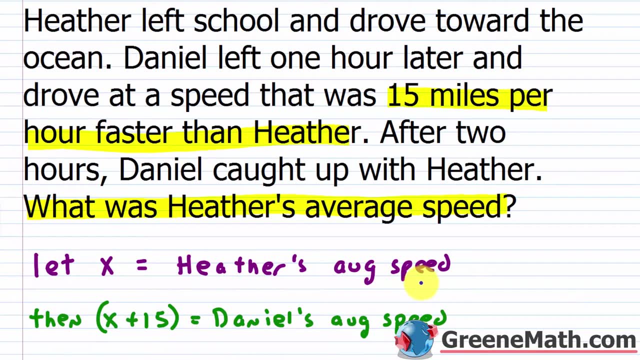 is my distance for Daniel. Now let's go back up and see how we can figure out an equation If we think about this. remember they leave from the same point. Heather left school and drove toward the ocean. Daniel left one hour later, okay. 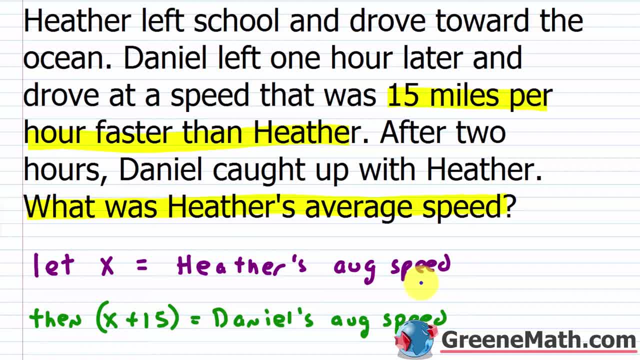 So he's leaving from the same point. Now they catch up, meaning they go to the same point when they're caught up. okay, So they leave from the same point, they go to the same point. So that means that Heather and Daniel drive the same distance. 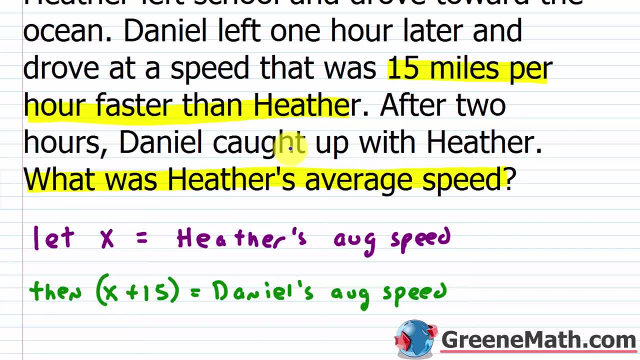 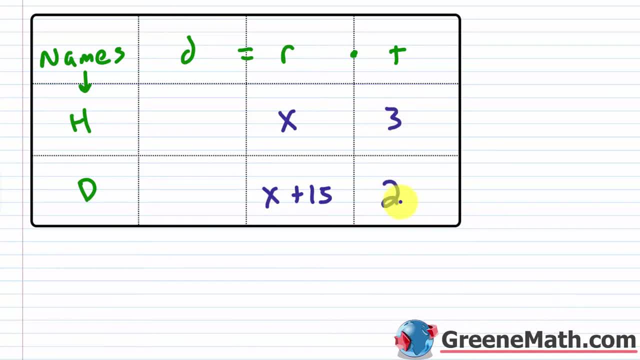 Heather was driving for an hour more, So she was driving for three hours. So I can fill this out and say Heather was driving for three hours, Daniel was driving for two. Now I can get the distance by multiplying, Okay. So in other words, the distance that Heather travels is the amount of time she travels for. 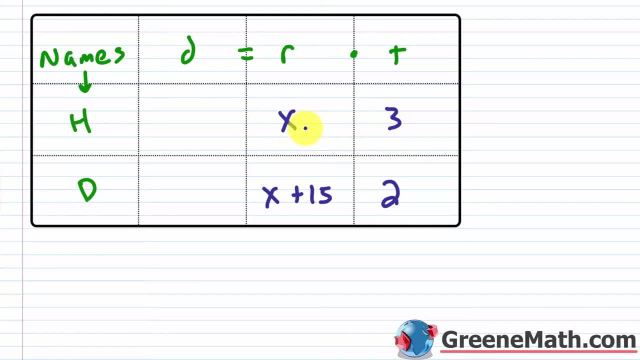 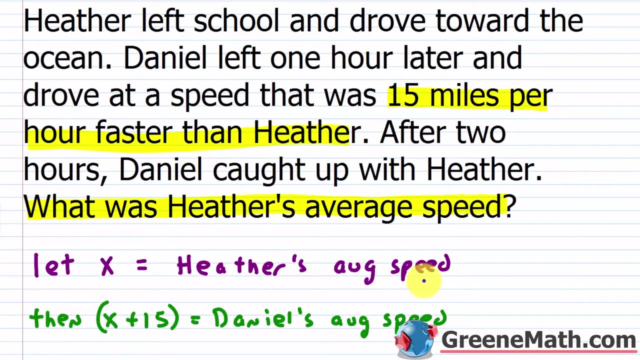 times the rate of speed that she travels at. So three times X is three X, That's my distance for Heather. Two times the quantity X plus 15 is my distance for Daniel. Now let's go back up and see how we can figure out an equation. If we think about this, remember they leave from the same. 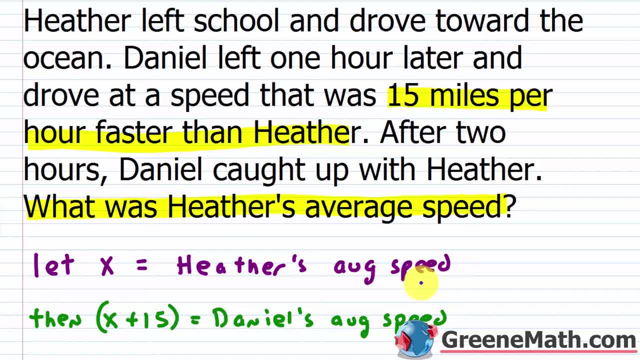 point. Heather left school and drove toward the ocean. Daniel left one hour later. Okay, So he's leaving from the same point. Now they catch up, meaning they go to the same point when they're caught up. Okay, So they leave. 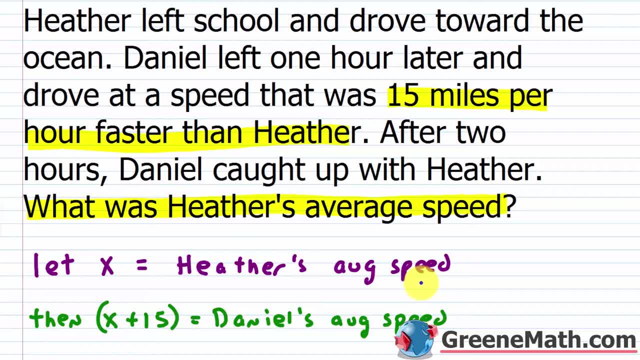 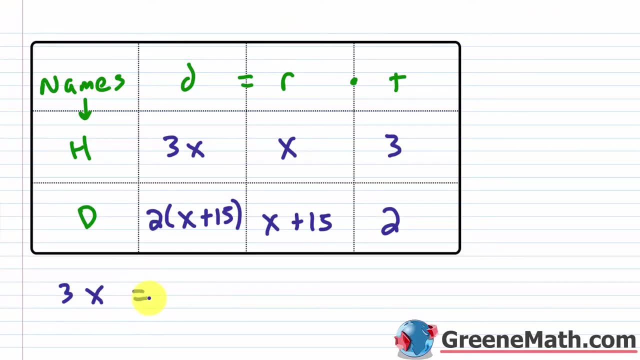 from the same point. They go to the same point. So that means that Heather and Daniel drive the same distance. They do it at a different amount of time, but they drive the same distance. So what I can say here is that the distance for Heather, which is three X, is going to be equal. 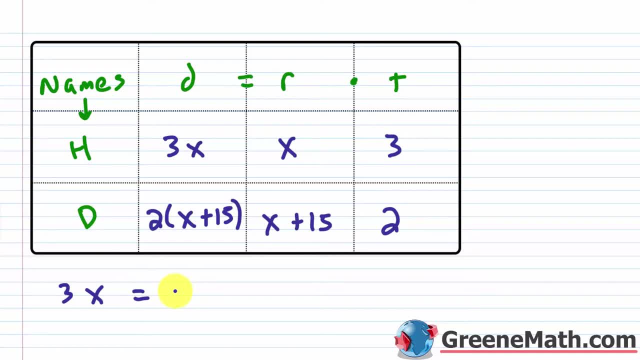 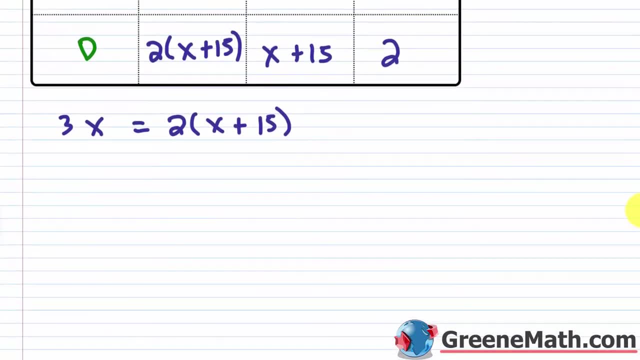 or the same as the distance for Heather. So that's going to be equal or the same as the distance for Daniel, which is two times the quantity X plus 15.. So once we've set this up, it's basically a breeze. from here, We would use our distributive property on the right. This is two X plus 30.. 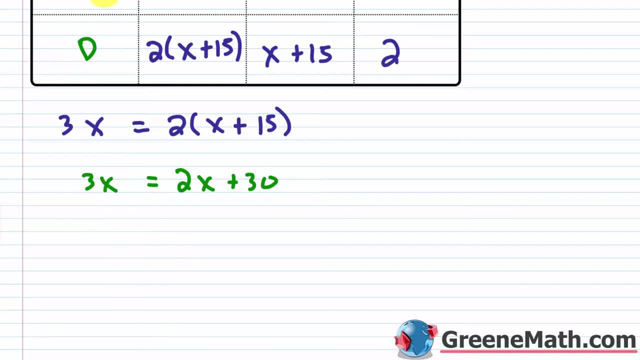 On the left, we still just have three X. Let me go ahead and subtract two X away from each side of the equation. This is going to cancel. I'll have that X is equal to third. Okay, So this is another big problem. 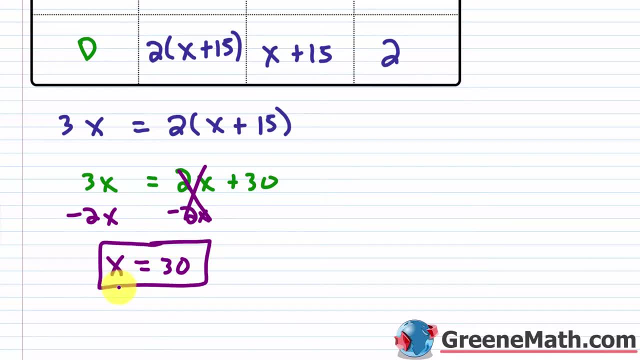 a lot of students get x equals 30 and they stop right. We're used to just saying, hey, this is my answer. x equals 30. With word problems you've got to go back up and make sense of your answer. So x equals 30 tells me that Heather's average speed was 30 miles per hour. 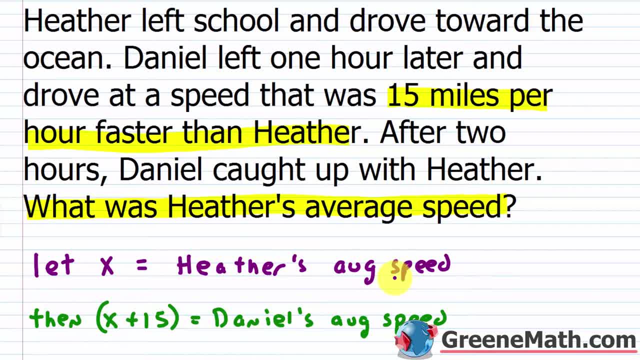 okay, And it also tells me that Daniel's average speed was 45 miles per hour, because his is expressed as x, which is 30 plus 15.. 30 plus 15 is 45. So let's erase this And say what was Heather's average speed. We can say Heather's. 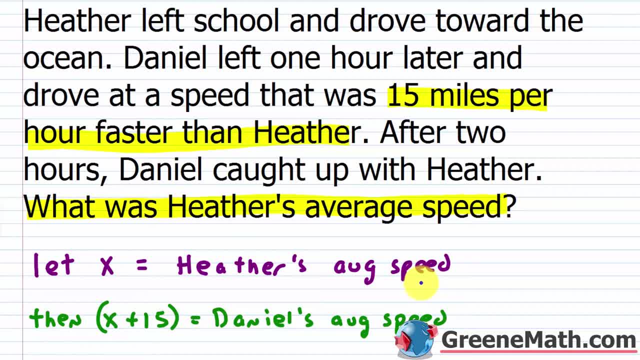 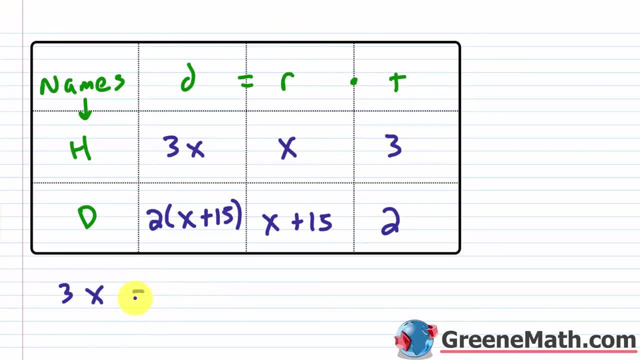 They do it at a different amount of time, but they drive the same distance. So what I can say here is that the distance for Heather, which is 3X, is going to be equal or the same as the distance for Daniel, which is two times the quantity X plus 15.. 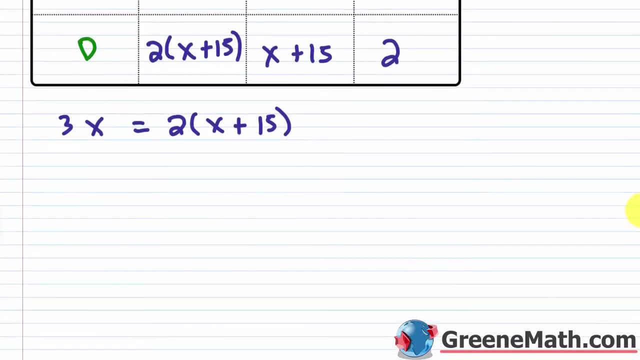 So once we've set this up, it's basically a breeze from here. We would use our distributive property. on the right, This is 2X plus 30. On the left, we still just have 3X. Let me go ahead and subtract 2X away. 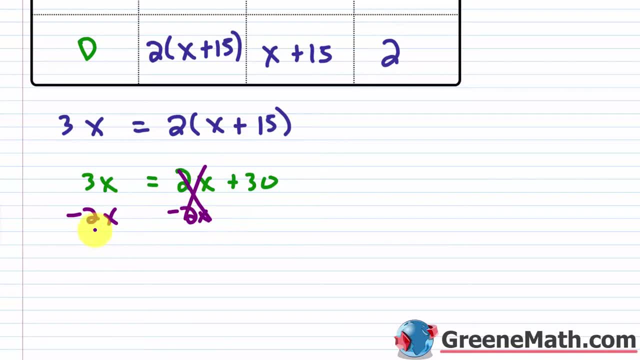 from each side of the equation. This is going to cancel. I'll have that X is equal to 30.. Okay, so this is another big problem. A lot of students get X equals 30 and they stop right. We're used to just saying: 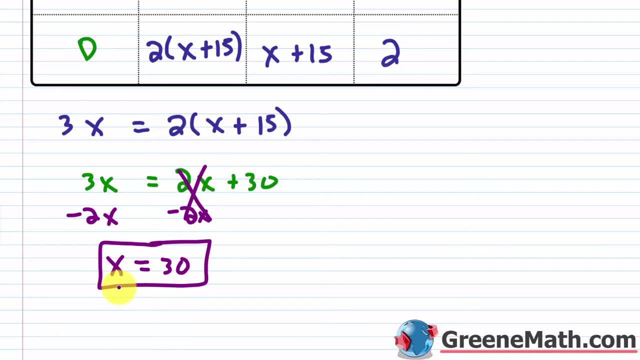 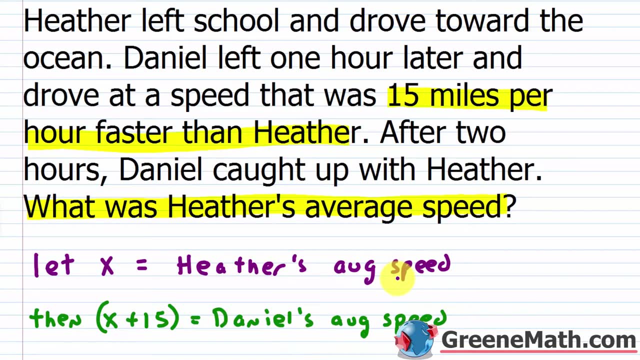 hey, this is my answer. X equals 30.. With word problems, you've got to go back up and make sense of your answer. So X equals 30 tells me that Heather's average speed was 30 miles per hour. okay, 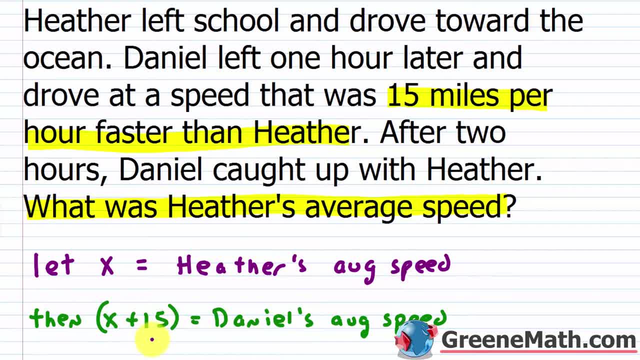 And it also tells me that Daniel's average speed was 45 miles per hour, because his is expressed as X, which is 30 plus 15. 30 plus 15 is 45. So let's erase this and say what was Heather's average speed. 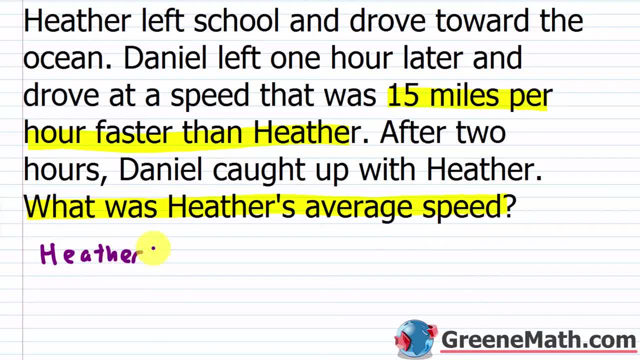 We can say Heather's average speed was 30 miles per hour. okay, And you can check this pretty easily. You can say: are the distances equal? Well, if Heather drives at 30 miles per hour for three hours, she's going to go 90 miles right. 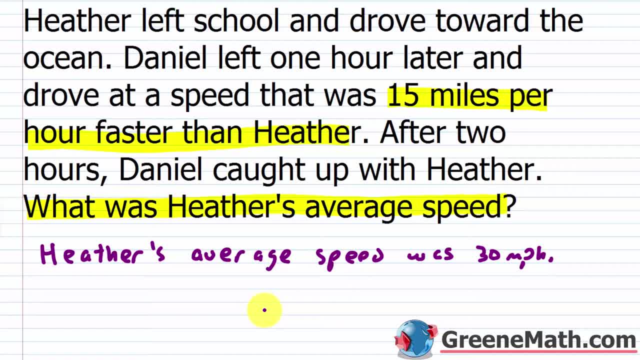 Again, distance equals rate of speed, which is 30 times time traveled, which is three. 30 times three is 90. So when you think about the units, it's going to be 90 miles For Daniel. he drives for only two hours. 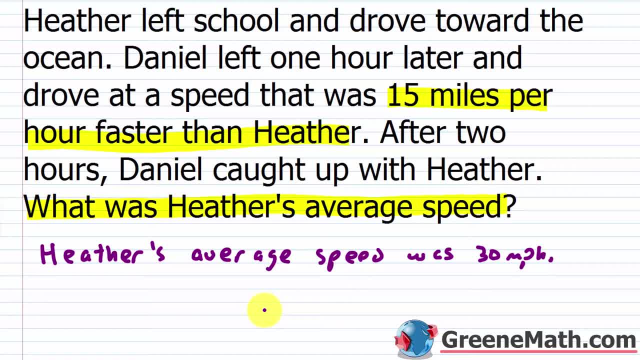 but he does it at 45 miles per hour. Two times 45 is also 90. So you can say this is the correct answer. Heather's average speed was 30 miles per hour. And again, although it doesn't ask for it in the problem, 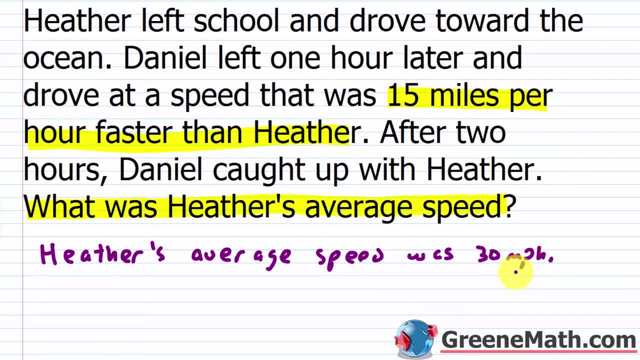 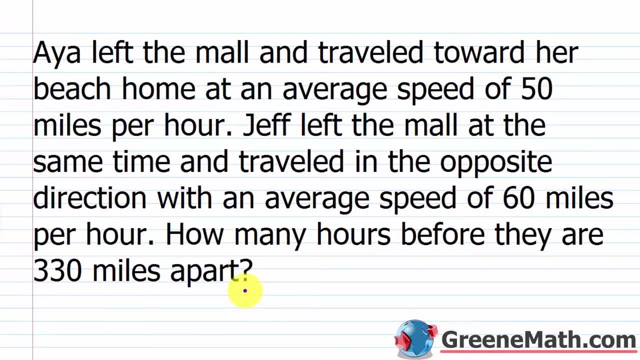 we can say Daniel's average speed was 45 miles per hour. All right, let's look at another one. So we have that. Aya left the mall and traveled toward her beach home at an average speed of 50 miles per hour. Jeff left the mall at the same time. 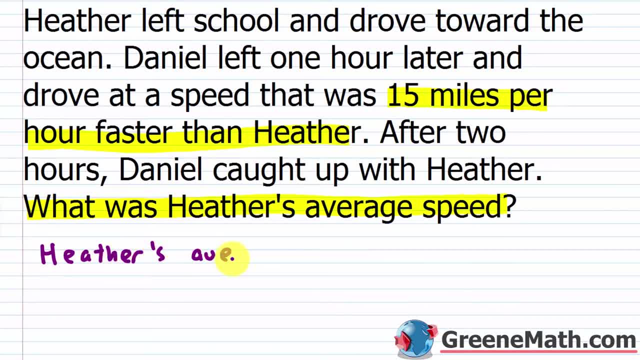 average speed was 30 miles per hour. okay, And you can check this pretty easily. You can say: are the distances equal? Well, if Heather drives at 30 miles per hour for three hours, she's going to go 90 miles right Again. 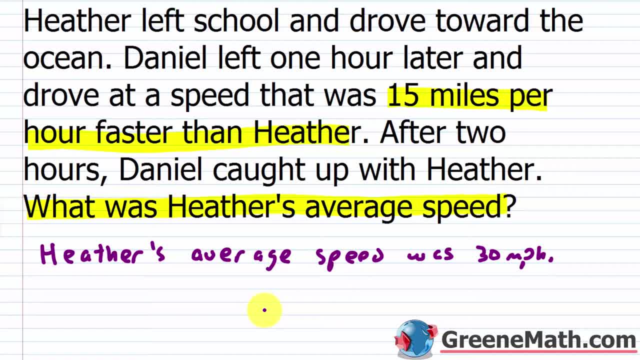 distance equals 30 miles per hour. So if Heather drives at 30 miles per hour for three hours, distance equals rate of speed, which is 30 times time traveled, which is three. 30 times three is 90. So when you think about the units, it's going to be 90 miles For Daniel, he drives for only two. 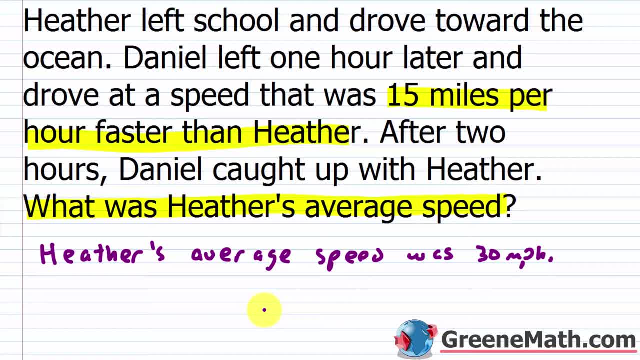 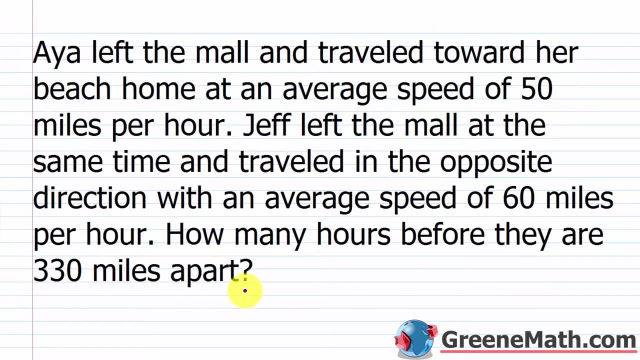 hours, but he does it at 45 miles per hour. Two times 45 is also 90. So you can say this is the correct answer. Heather's average speed was 30 miles per hour And again, although it doesn't ask for it in the problem, we can say Daniel's average speed was 45 miles per hour. All right, 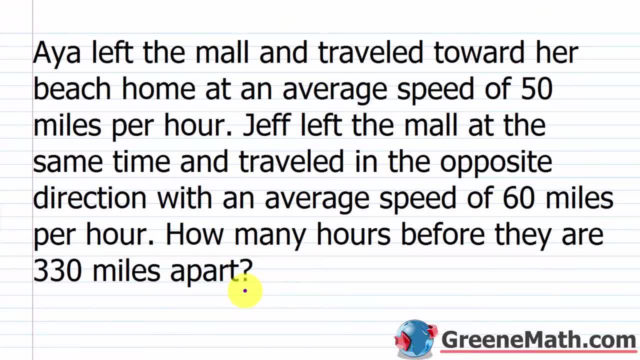 let's look at the next question. So let's say that Heather left the mall and traveled toward her beach home at an average speed of 50 miles per hour. Jeff left the mall at the same time and traveled in the opposite direction with an average speed of 60 miles per hour. 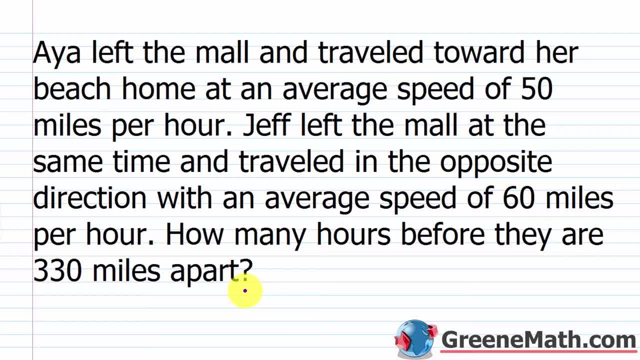 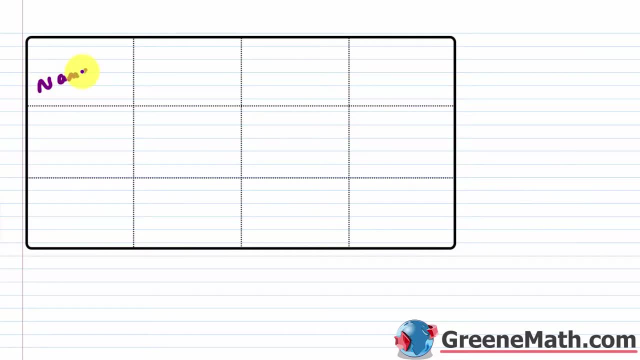 How many hours before they are 330 miles apart. So this is what we need to answer: How many hours before they are 330 miles apart. So let's label our kind of table down here So we have our names going down. Let me make that a little bit better. So we have Aya and we have Jeff. Okay, And then 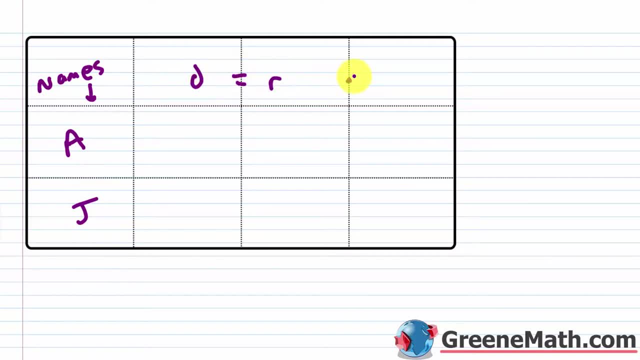 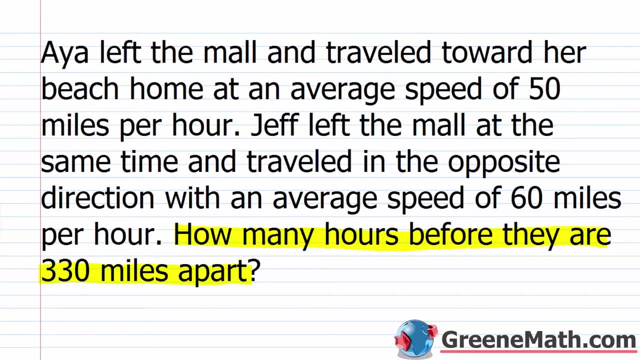 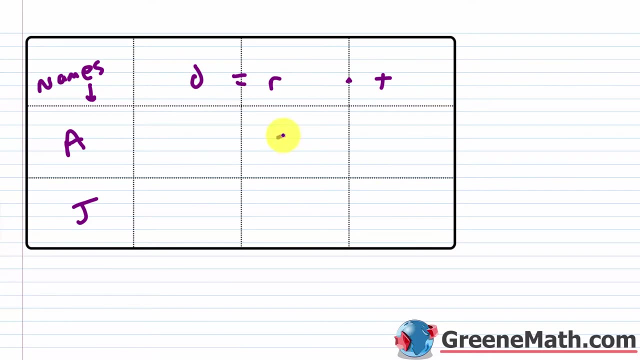 for this part. right here we have: our distance is equal to rate times time. Okay, So what are we given in the problem? We're told that Aya's average speed is 50 miles per hour and Jeff's average speed is 60 miles per hour. So for Aya, the rate of speed is 50.. For Jeff, it's 60. 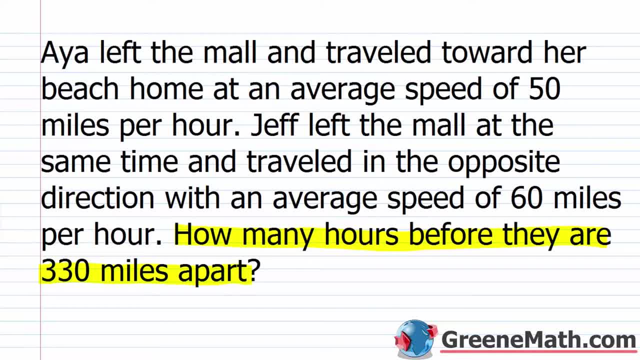 Do we know the time in each case? No, we're not, given that Okay, And in fact, what we need to find is how many hours before. they are 330 miles apart, meaning they start at one point and one drives in one direction, another drives in the opposite direction, And we want to know how long. 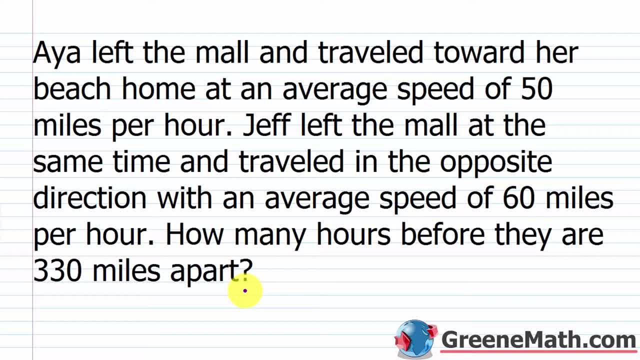 and traveled in the opposite direction with an average speed of 60 miles per hour. How many hours before they are 330 miles apart. So this is what we need to answer: How many hours before they are 330 miles apart. So let's label our kind of table down here. 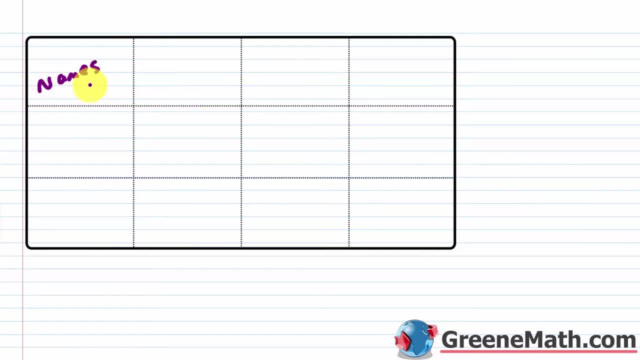 So we have our names Going down. Let me make that a little bit better. So we have Aya and we have Jeff, okay, And then for this part right here we have: our distance is equal to rate times time. Okay, so what are we given in the problem? 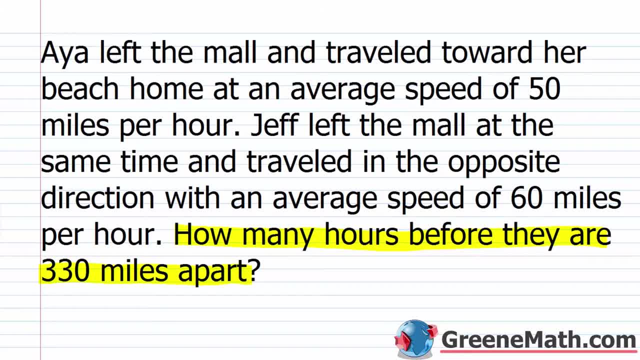 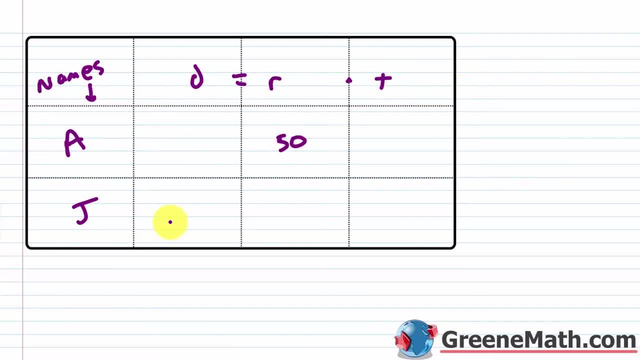 We're told that Aya's average speed is 50 miles per hour and Jeff's average speed is 60 miles per hour. So for Aya the rate of speed is 50.. For Jeff it's 60. Do we know the time in each case? 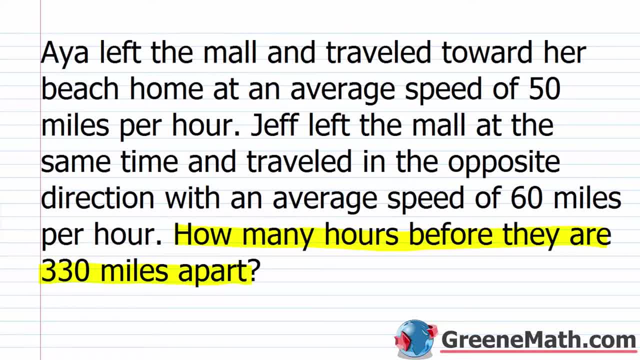 No, we're not given that okay, And in fact, what we need to find is how many hours before. they are 330 miles apart, Meaning they start at one point and one drives in one direction, another drives in the opposite direction. 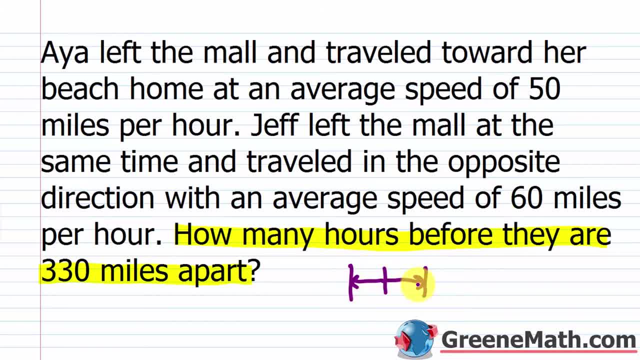 And we want to know how long before. kind of, the distance between them is 330 miles, okay, So let me make that better. So what we want to do is let a variable like X be equal to the amount of hours that they're each traveling for. 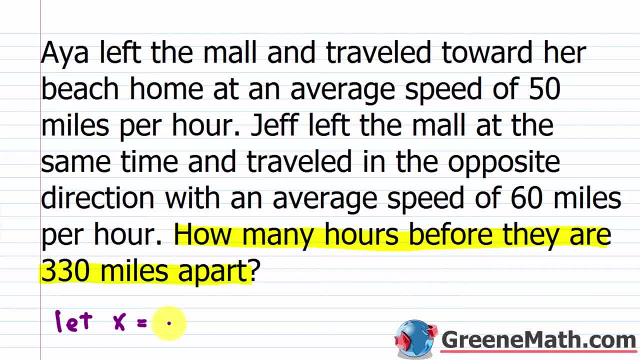 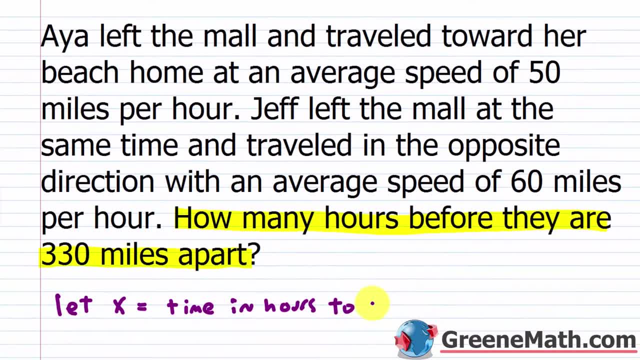 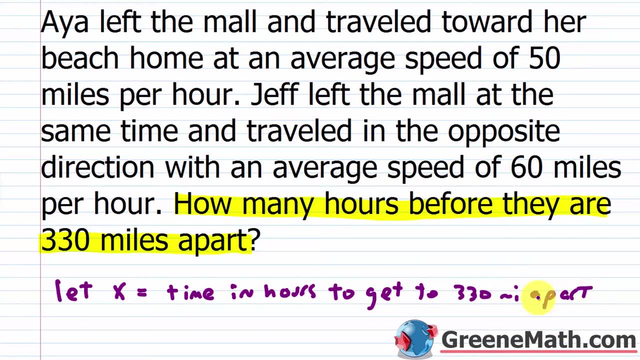 before they are 330 miles apart. So time in hours we could say to get to 330 miles apart. Okay, let me make that a little bit better. So each of them are going to drive for that amount of time, So we can go down here. 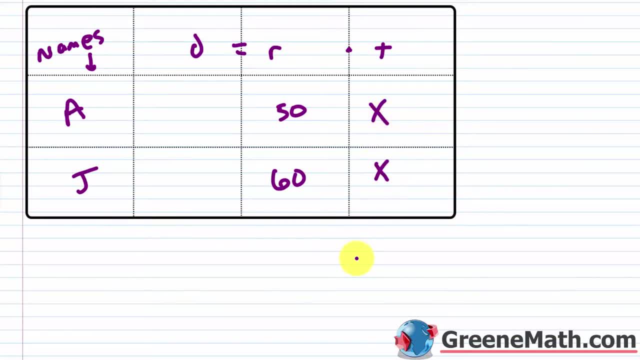 and we could say that this is X and this is X. Now, the distance that Aya travels is 50 times X or 50X. The distance that Jeff travels is 60 times X or 60X. In the last problem we set the distances equal to each other. 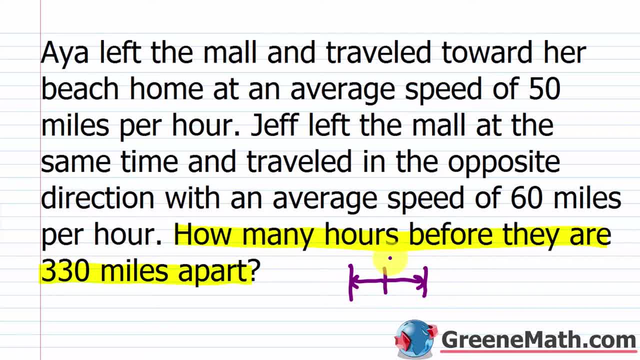 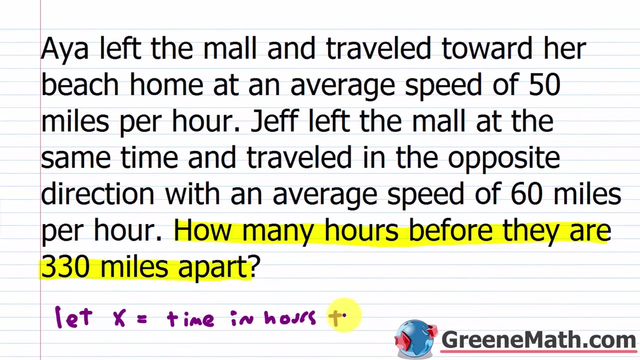 before, kind of the distance between them is 330 miles. Okay, So let me make that better. So what we want to do is let a variable like X be equal to the amount of hours that they're each traveling for before they are 330 miles apart. So time in hours we could say to get to 330 miles. 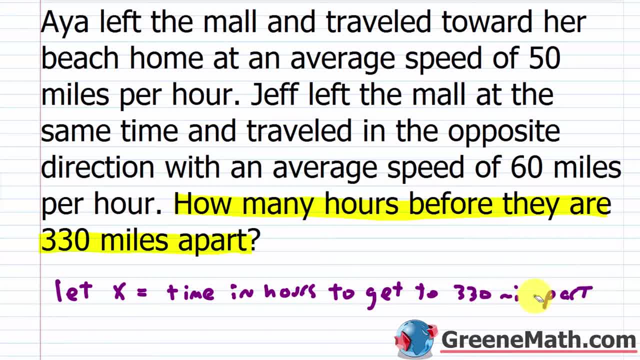 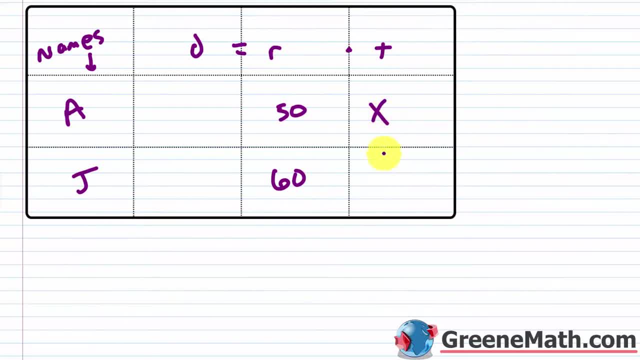 apart. Okay, Let me make that a little bit better. So each of them are going to drive for that amount of time, So we can go down here and we can say that this is X and this is X. Now the distance that Aya travels is 50 times X or 50. 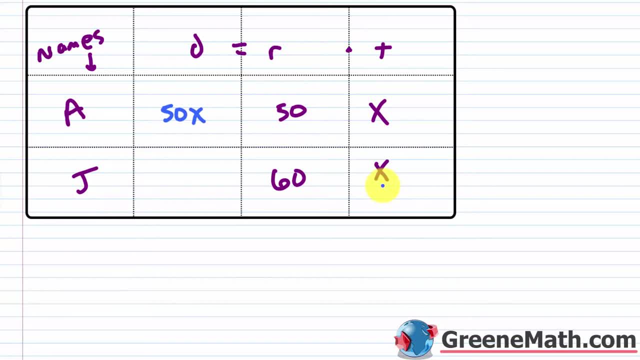 X. The distance that Jeff travels is 60 times X or 60 X. In the last problem we set the distances equal to each other, but that's not going to work here, because what we're saying is that the sum of travels is going to be 330 miles. right, 50 X plus 60 X needs to be 330 miles. Okay, So if we solve, 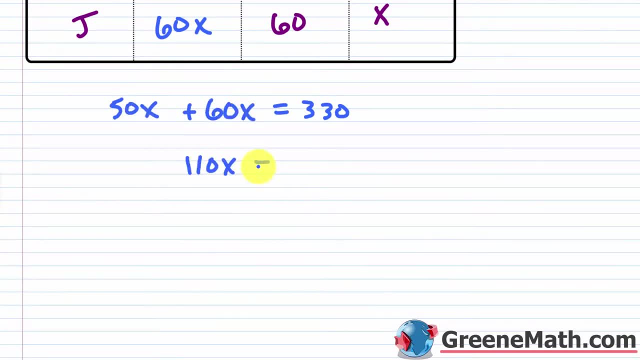 this: 50 X plus 60 X is 110 X, and this equals 330.. We divide both sides of the equation by 110.. We're going to get that X is equal to three. All right, So let's erase this And let's say: 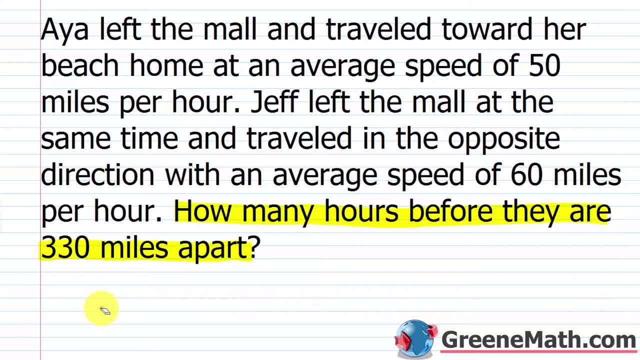 since X was three and X represents the amount of hours that they're traveling for for them to get to 330 miles apart. we'll just say it takes three hours for them- meaning Aya and Jeff- for them to be 330 miles apart. 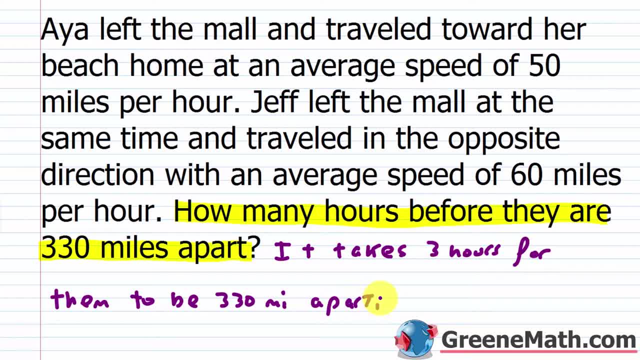 Okay, And that would be your answer there And you can think about why that makes sense. If Aya drives at a speed of 50 miles per hour for three hours, she's basically going- let's say, from this point to here she's going 150 miles, Okay. 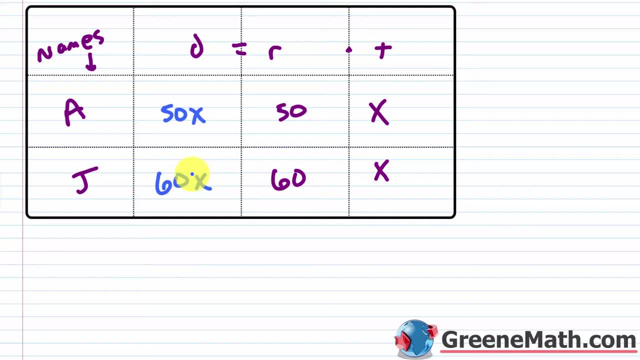 But that's not going to work here, because what we're saying is that the sum of the distances- the amount that Aya travels plus the amount that Jeff travels- is going to be 330 miles. right, 50X plus 60X needs to be 330 miles, okay. 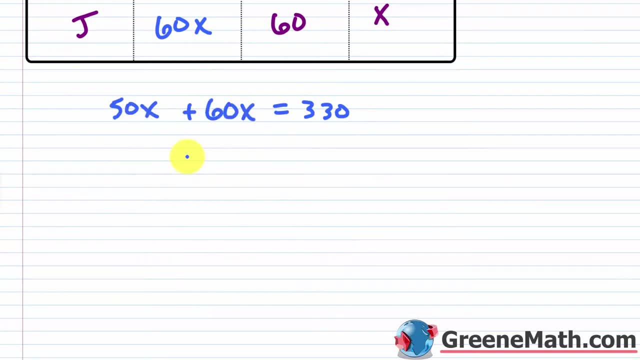 So if we solve this, 50X plus 60X is 110X and this equals 330.. We divide both sides of the equation by 110.. We're going to get that X is equal to 3.. All right, so let's erase this. 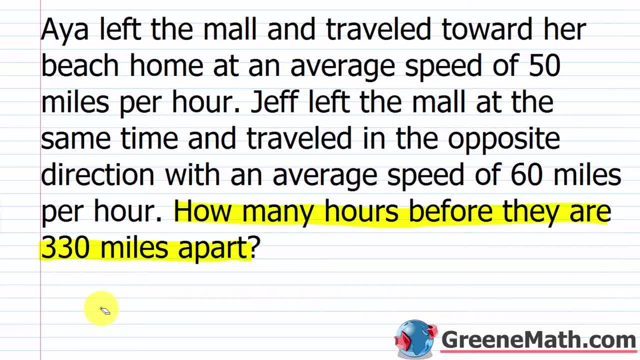 And let's say, since X was 3, and X represents the amount of hours for them to get to 330 miles apart, we'll just say it takes three hours for them, meaning Aya and Jeff- for them to be 330 miles apart. 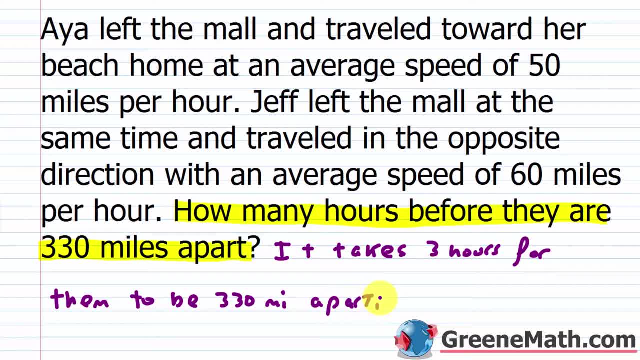 Okay, And that would be your answer there And you can think about why that makes sense. If Aya drives at a speed of 50 miles per hour for three hours she's basically going, let's say, from this point to here. 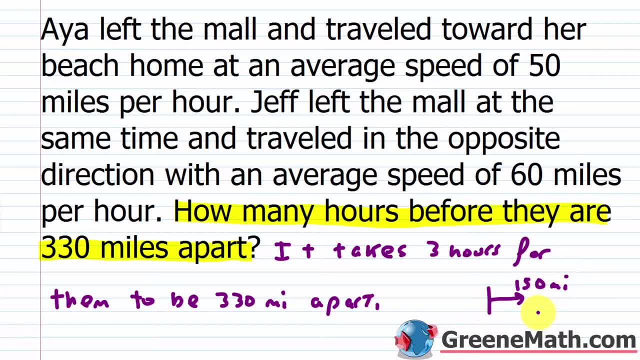 she's going 150 miles. okay, If Jeff goes the opposite direction, he starts here and goes this way. well, he's going to go a little bit further because he's going faster: 60 miles an hour times three hours would be 180 miles. 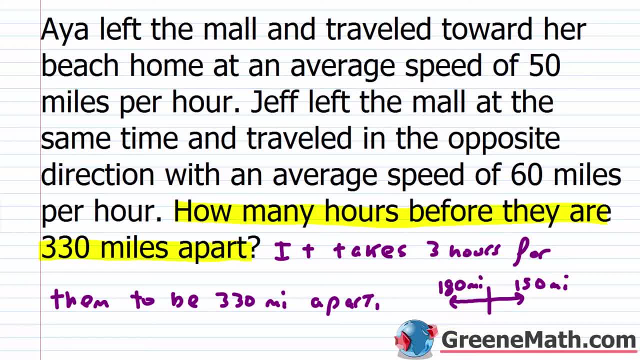 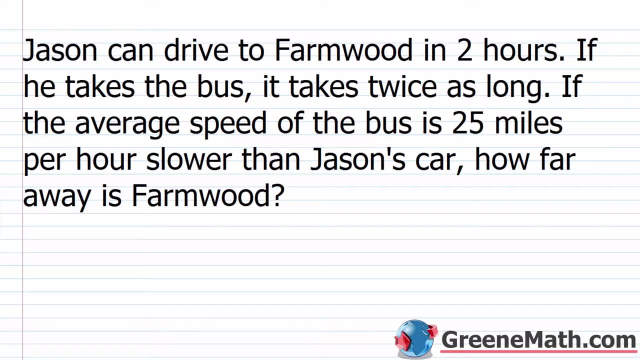 Okay, So the distance between them now, from here, where Jeff is, to here where Aya is, is 180 plus 150, which is going to be 330.. All right, let's look at one more. So Jason can drive to Farmwood in two hours. 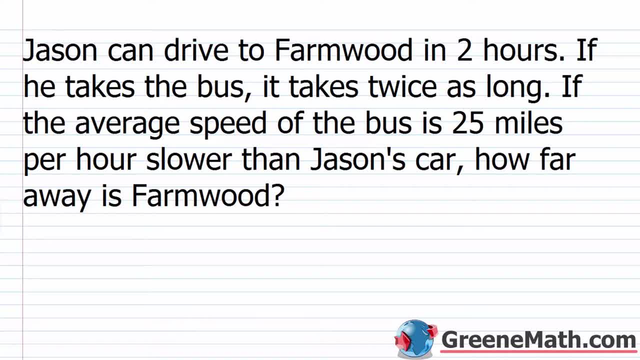 If he takes the bus, it takes twice as long. If the average speed of the bus is 25 miles per hour slower than Jason's car. how far away is Farmwood? Okay, So what are we asking? We're asking for how far away is Farmwood? 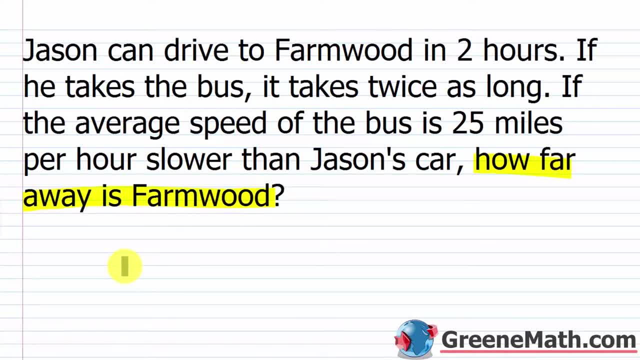 meaning? what is the distance from wherever Jason starts to? you know, drive to Farmwood, Okay, Well, we know that there's two situations: There's one where he takes a car and there's another where he takes a bus. So let's go down here. 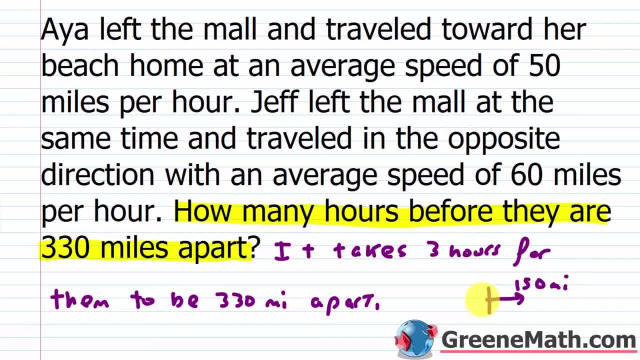 If Jeff goes the opposite direction, he starts here and goes this way. Well, he's going to go a little bit further because he's going faster. 60 miles an hour times three hours would be 180 miles. Okay, So the distance between them now, from here, where Jeff is, to here, where Aya is, 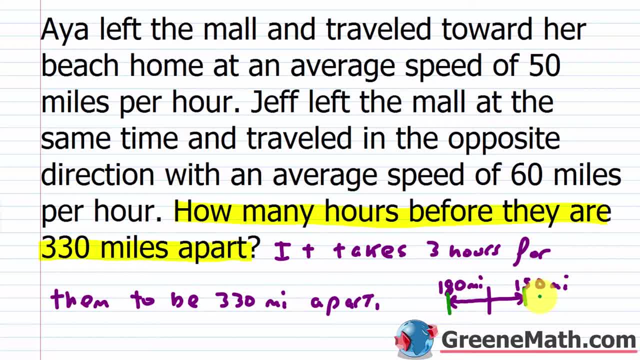 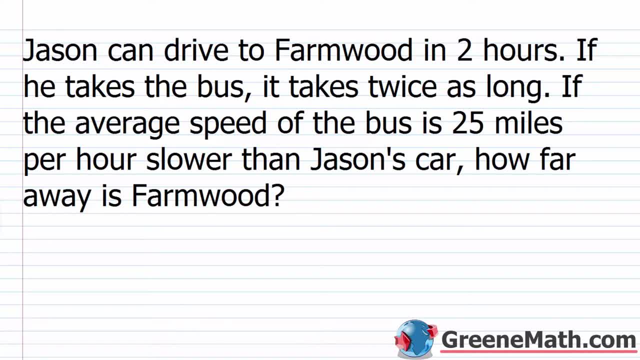 is 180 plus 150, which is going to be 330.. All right, Let's look at one more. So Jason can drive to Farmwood in two hours If he takes the bus. it takes twice as long If the average speed of. 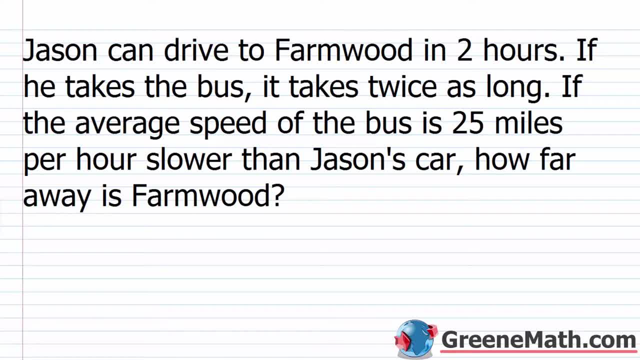 the bus is 25 miles per hour slower than Jason's car. how far away is Farmwood? Okay, So what are we asking? We're asking for how far away is Farmwood, meaning, what is the distance from wherever Jason starts to Farmwood? Okay, So what are we asking? We're asking for how far away is. 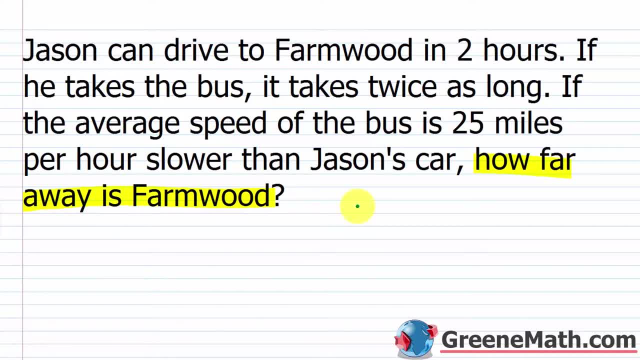 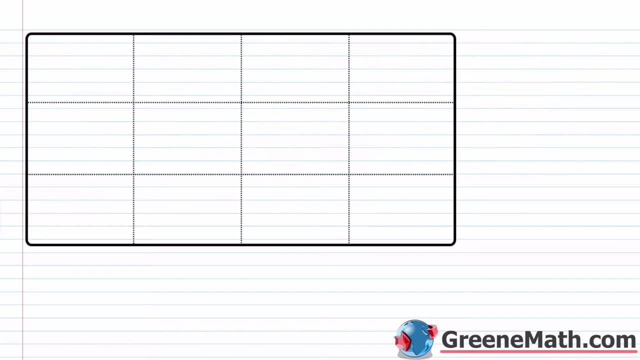 Jason to Farmwood. Okay, Well, we know that there's two situations: There's one where he takes a car and there's another where he takes a bus. So let's go down here So to start filling in the table. we'd have one scenario which is a car and another which is a bus. So this just 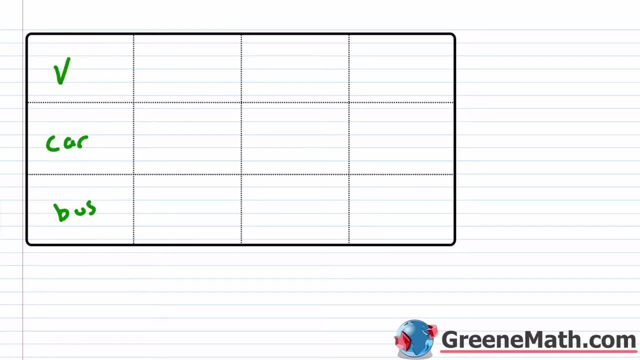 represents the vehicle. So I just put V for that. Again, we're still going to have our. D for distance is equal to R for rate of speed times, T for time traveled. So let's go back up. We're totally going to have our. D for distance is equal to R for rate of speed times, T for time traveled. 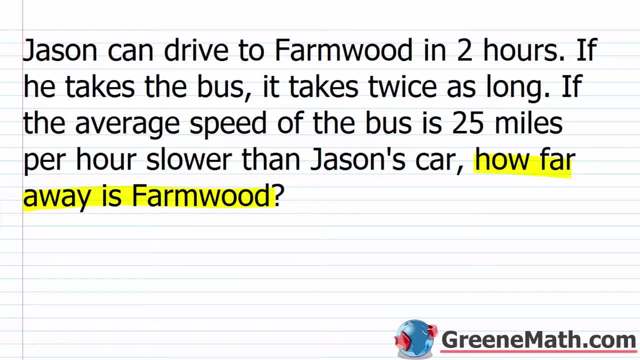 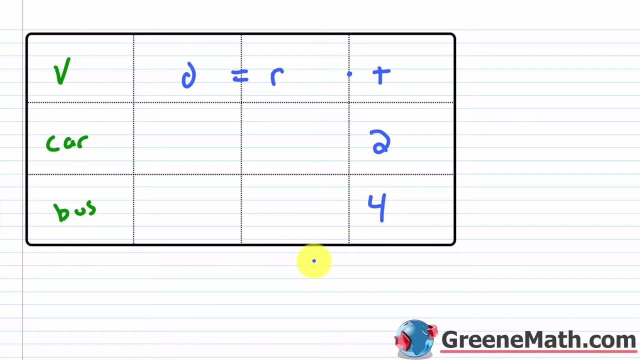 Okay. So we're only told that Jason can drive to Farmwood in two hours. So by car the trip takes two hours. So the time by car we're going to put two there And then if he takes the bus it takes twice as long. So two times two would be four. So if he takes the bus it's four hours. 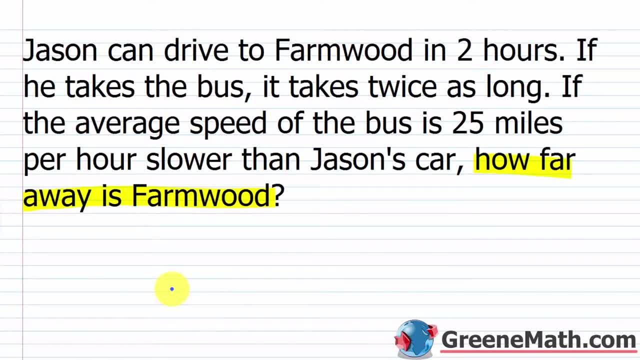 Now, in terms of the rate of speed, we're not given that. We're only told that the speed of the bus is 25 miles per hour slower than Jason's car. Okay, So let's say that Jason's let a variable like X be equal to the car's average speed, And again, this is in miles per. 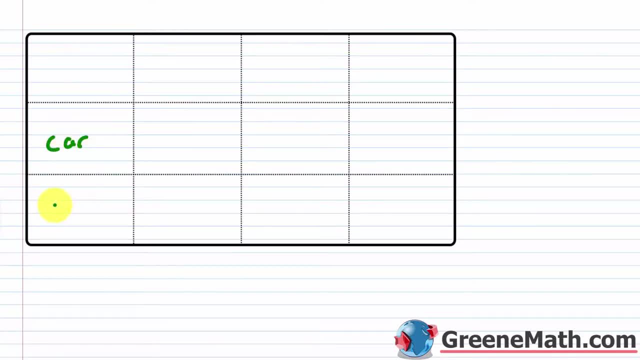 So to start filling in the table, we'd have one scenario which is a car and another which is a bus. So this just represents the vehicle. So I just put V for that. Again, we're still going to have our D, for distance is equal to R for rate of speed. 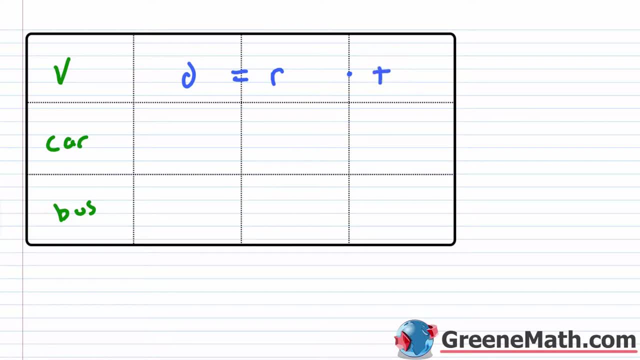 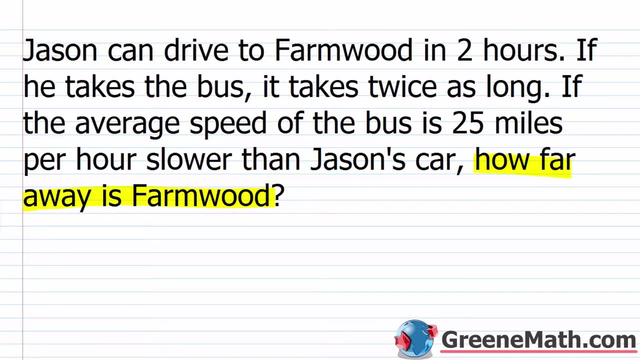 times T for time traveled. So let's go back up. We're told that Jason can drive to Farmwood in two hours. So by car the trip takes two hours. So the time by car we're going to put two there. 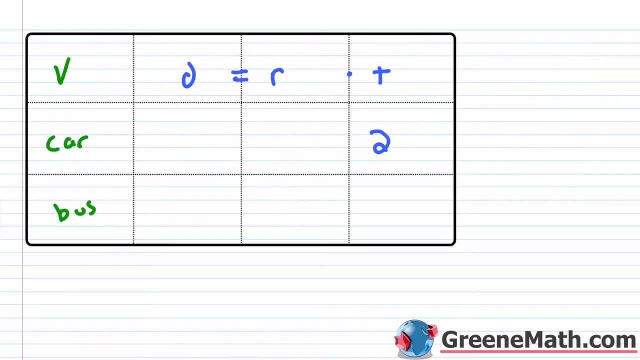 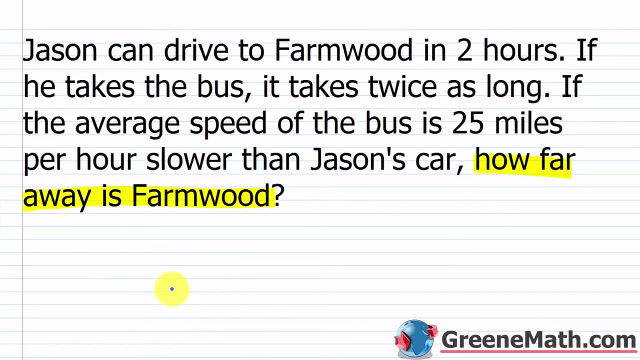 And then if he takes the bus, it takes twice as long. So two times two would be four. So if he takes the bus, it's four hours. Now, in terms of the rate of speed, we're not given that, We're only told that the speed of the bus is 25 miles per hour slower than Jason's car. 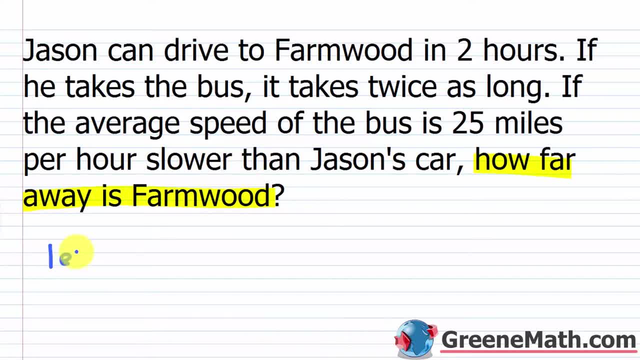 Okay. So let's let a variable like X be equal to the car's average speed, And again, this is in miles per hour. Now we can model the speed of the bus based on this right, If X is the car's average speed. 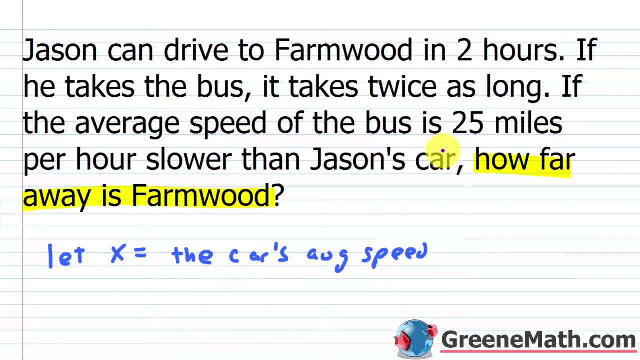 since the bus is going 25 miles per hour slower than the car, we can say X minus 25 can represent the bus's average speed, So we'll say the average speed of the bus. Okay, All right, So X is the car's average speed. 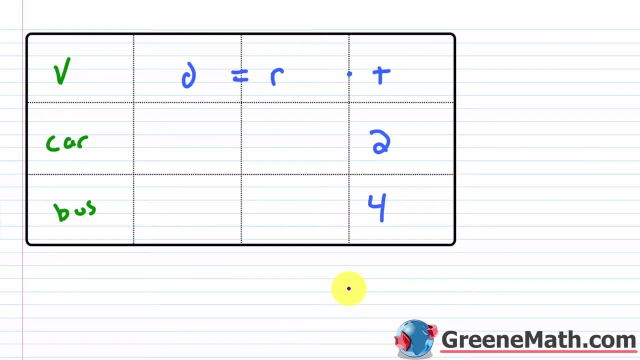 X minus 25 is the average speed of the bus. So rate of speed for the car is X, Rate of speed for the bus is X minus 25.. Now we know for distance we multiply. So two times X is two X. 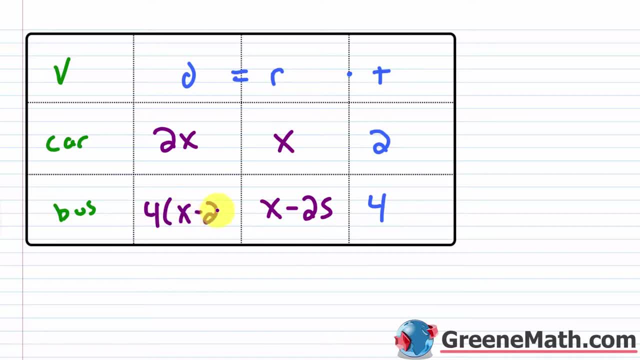 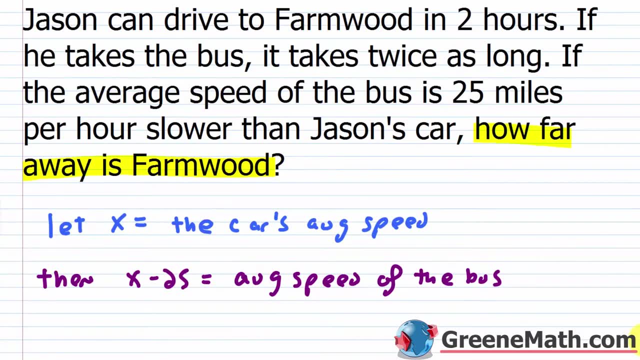 And over here we'd have four times the quantity X minus 25.. Okay, Now we know that the distance is equal, right? Jason can drive to Farmwood in two hours. If he takes the bus, it takes twice as long. 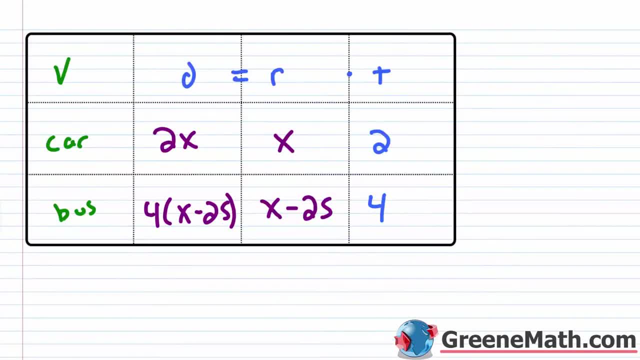 So the distance is going to be the same. So to solve this one, I can just set this distance that he travels by car of two X, equal to the distance of the bus, which is four times the quantity X minus 25.. All right, 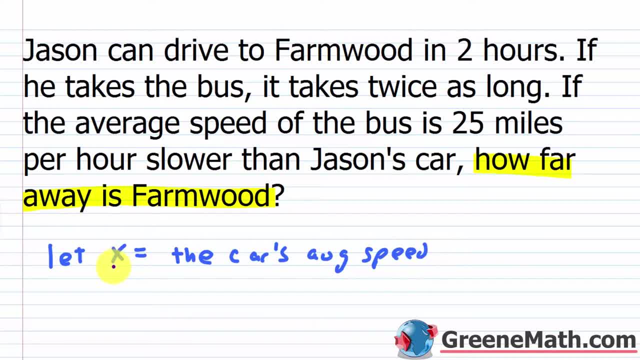 hour. Now we can model the speed of the bus based on this right. If X is the car's average speed, since the bus is going 25 miles per hour slower than the car, we can say X minus 25 can represent the bus's average speed. So we'll say: 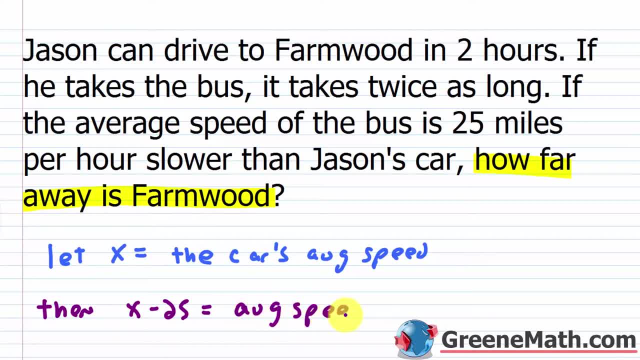 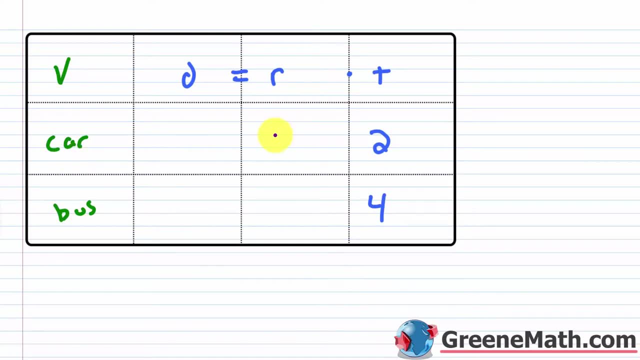 the average speed of the bus. Okay, All right. So X is the car's average speed, X minus 25 is the average speed of the bus. So rate of speed for the car is X. Rate of speed for the bus is X minus 25.. Now we know. for distance we multiply. So two times X is two X, And over here we'd have 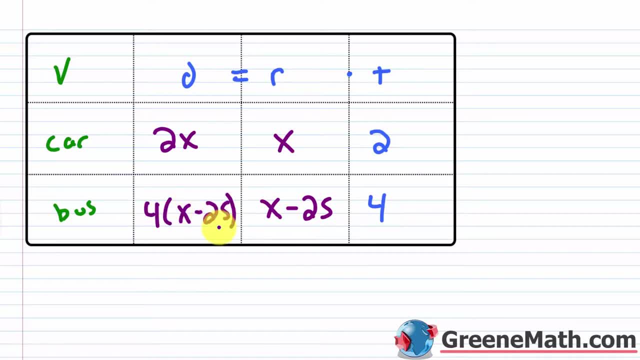 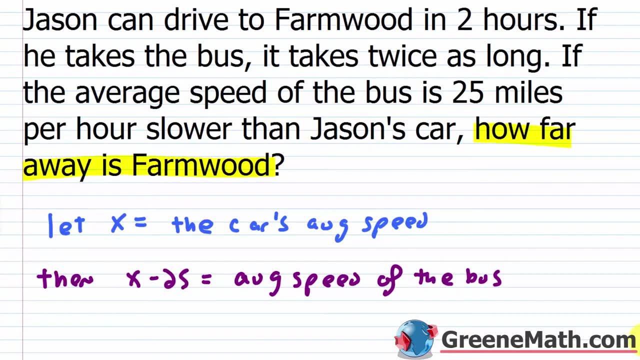 four times the quantity X minus 25.. Okay, Now we know that the distance is equal, right? Jason can drive to Farmwood in two hours. If he takes the bus, it takes twice as long. So the distance is going to be the same. So to solve, 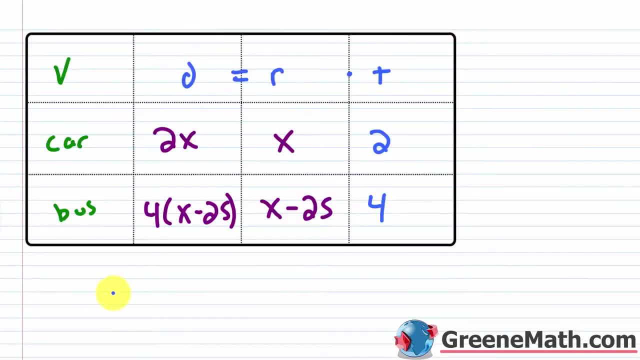 this one. I can just set this distance that he travels by car of two X equal to the distance of the bus, which is four times the quantity X minus 25.. All right, So let's scroll down, get some room going. So we have two X on the left is equal to four times. 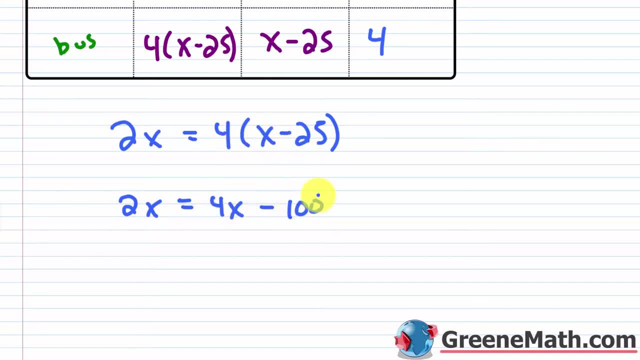 X is four X, And then minus four times 25 is 100. Let's go ahead and subtract four X away from each side of the equation. That cancels Two X minus four X is negative two X. This equals negative 100.. Let's go ahead and divide both sides by negative two And we're going to get that X. 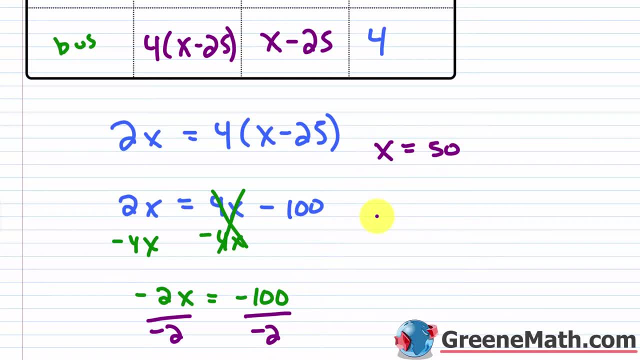 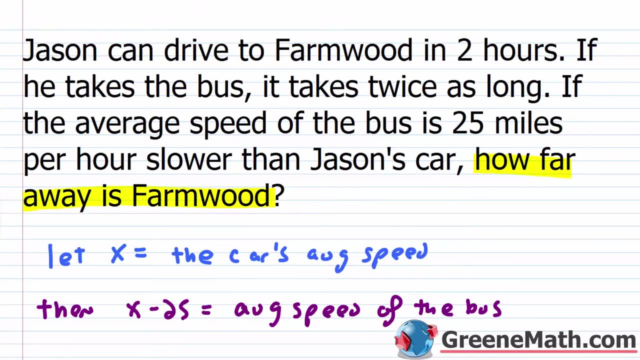 is equal to 50. Okay, So what does that mean? X equals 50.. We won't stop there, We've got to go back up. So X is the car's average speed. So that means the car was traveling at 50 miles per hour. 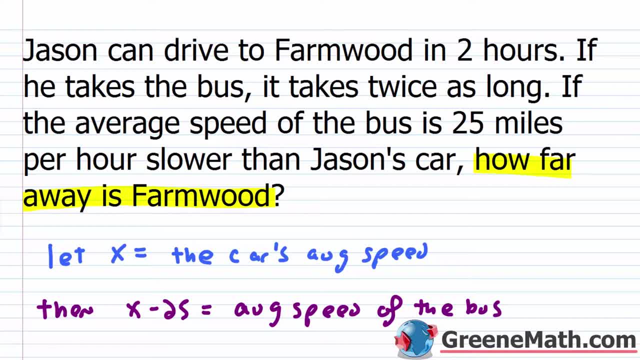 Okay, The average speed of the bus is 50 minus 25 or 25 miles per hour. That still doesn't answer the question. It didn't ask what was the speed of Jason's car. It asked how far away is Farmwood. 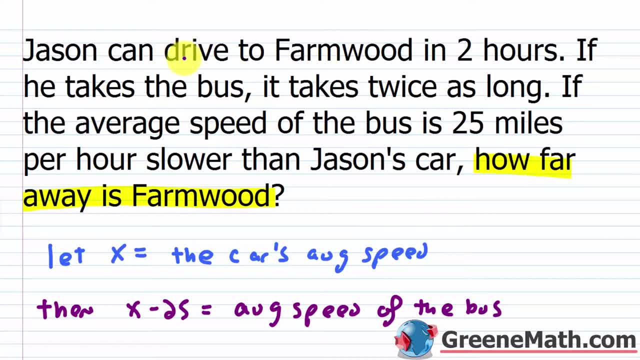 Well, all we have to do now is say: since Jason can drive to Farmwood in two hours, and he's driving at 50 miles per hour- 50 times two is 100. So that means Farmwood is a hundred miles away. So Farmwood. 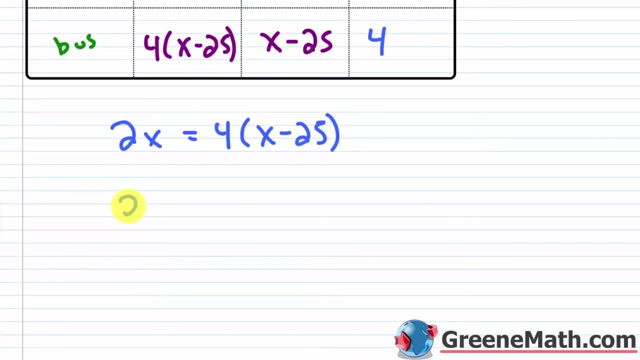 So let's scroll down, get some room going. So we have two: X on the left is equal to four times X is four X, and then minus four times 25 is a hundred. Let's go ahead and subtract four X away from each side of the equation. 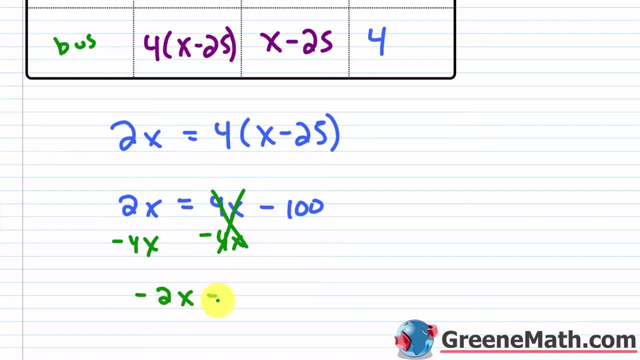 that cancels two X minus four. X is negative two X, This equals negative 100.. Let's go ahead and divide both sides by negative two And we're going to get that X is equal to 50.. Okay, So what does that mean? 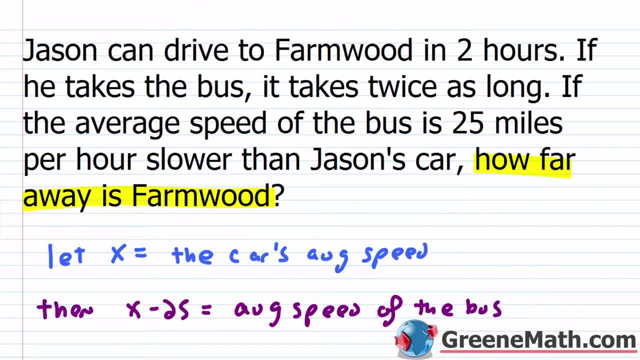 X equals 50, won't stop there, We've got to go back up. So X is the car's average speed. So that means the car was traveling at 50 miles an hour. Okay, the average speed of the bus is 50 minus 25 or 25 miles per hour. 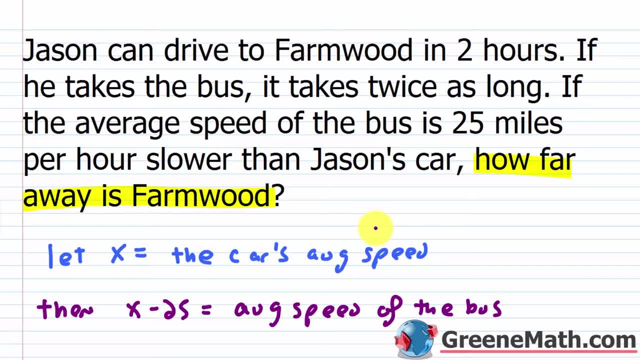 That still doesn't answer the question. It didn't ask What was the speed of Jason's car and asked how far away is Farmwood. Well, all we have to do now is say, since Jason can drive to Farmwood in two hours, and he's driving at 50 miles per hour, 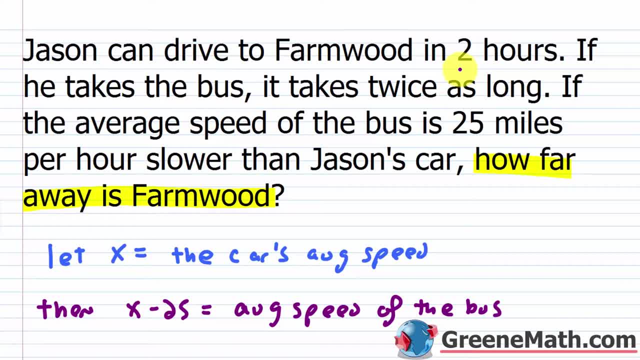 50 times two is 100. That means Farmwood is a hundred miles away. So Farmwood is 100 miles away. Let me erase all this. Okay, you can check that pretty easily Again, if he can drive to Farmwood in two hours and he's going at 50 miles per hour. 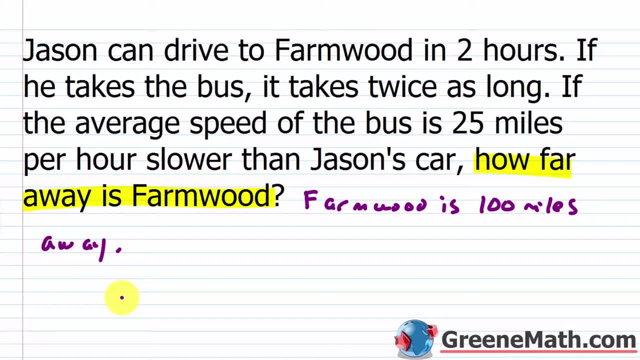 that's a hundred miles. If the bus is 25 miles per hour slower than the car, 50 minus 25 is 25.. It takes him twice as long. It takes him four hours. 25 times four is also a hundred. 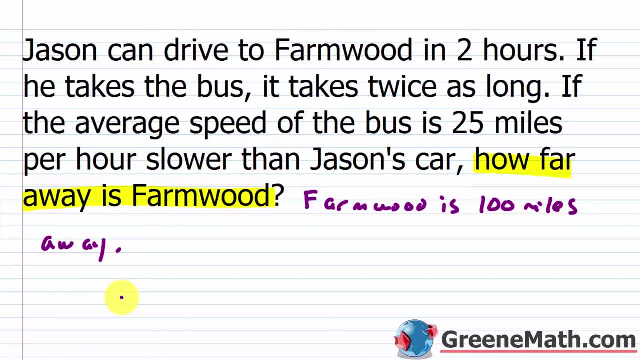 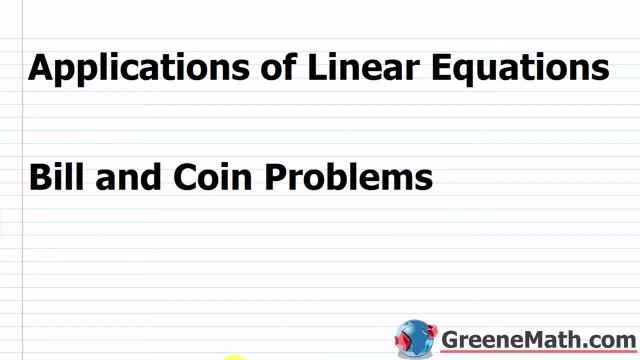 So either way, he's going a hundred miles. So that's consistent with our problem, right? Farmwood is a hundred miles away. in this lesson We want to review applications of linear equations and look at bill and coin problems, All right. 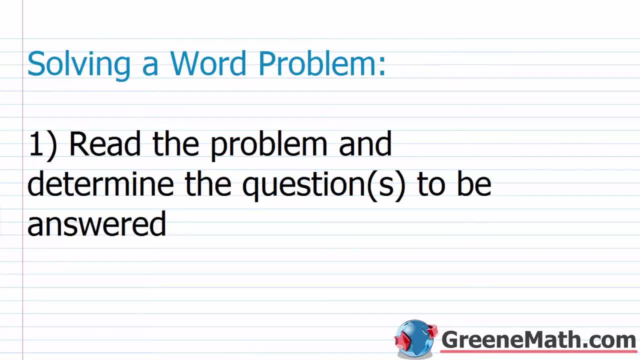 So again, if we're solving application problems that involve a linear equation in one variable, we can use our little six-step procedure. So again, for solving a word problem, we want to read the problem and determine the question or questions to be answered. 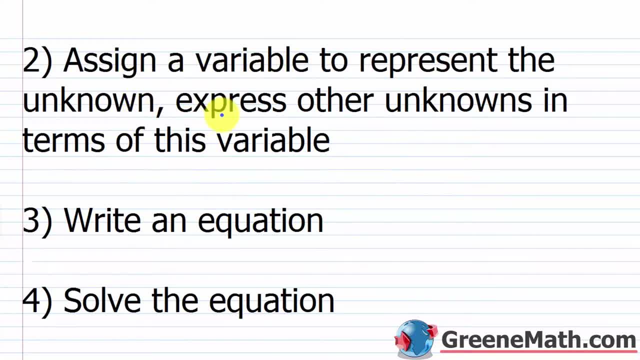 Then we want to assign a variable to To represent the unknown. We want to express other unknowns in terms of this variable. Then we want to write an equation, again based on the situation given in our problem. Then we're going to solve the equation. 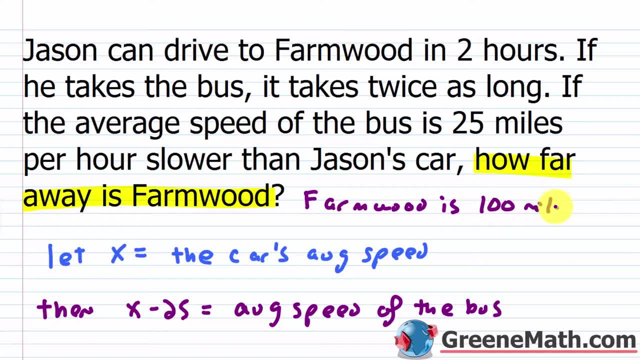 is 100 miles away. Let me erase all this. Okay, You can check that pretty easily Again. if he can drive to Farmwood in two hours and he's going at 50 miles per hour, that's a hundred miles. If the bus is 25 miles per hour slower. 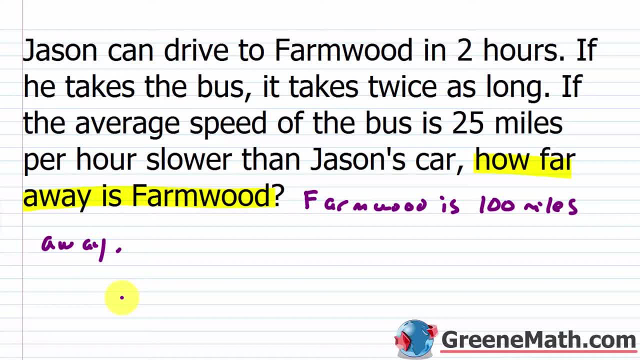 than the car. 50 minus 25 is 25.. It takes him twice as long. It takes him four hours. 25 times four is also a hundred. So either way he's going a hundred miles. So that's consistent with our problem, right? Farmwood is a hundred miles away. 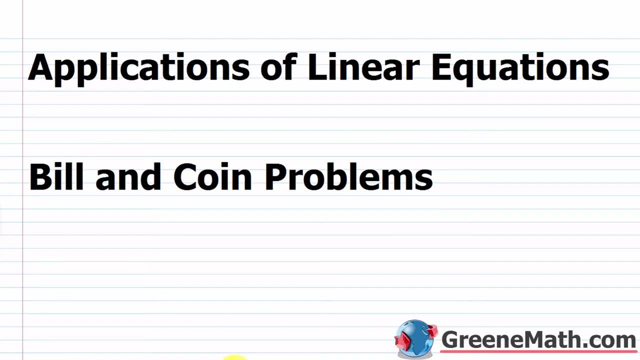 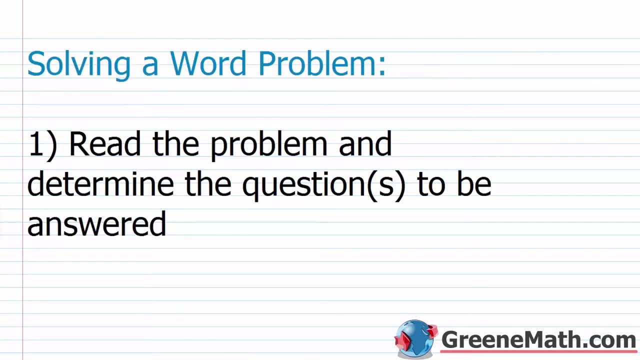 In this lesson we want to review applications of linear equations and look at bill and coin problems. All right. So, again, if we're solving application problems that involve a linear equation in one variable, we can use our little six step procedure. So, again, for solving a word problem, we want to read the problem and determine the question. 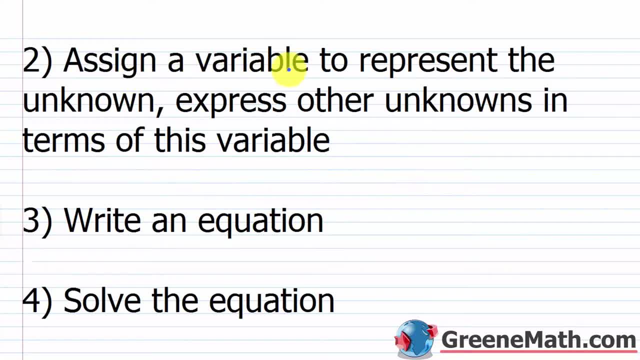 or questions to be answered. Then we want to assign a variable to represent the unknown, Express other unknowns in terms of this variable. Then we want to write an equation, again based on the situation given in our problem. Then we're going to solve the equation, Then we're. 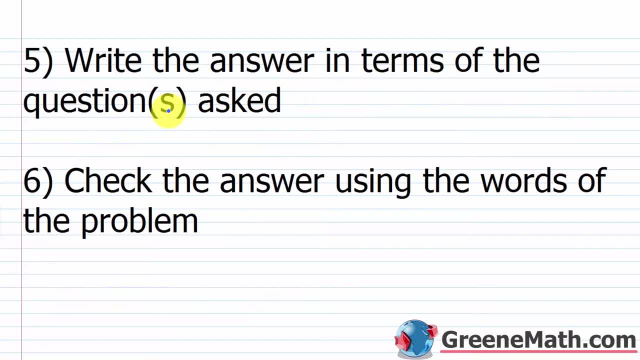 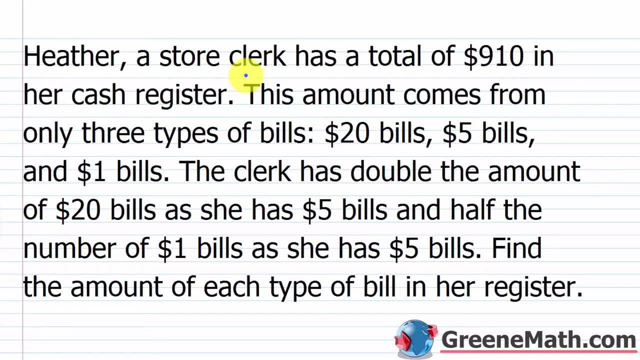 going to write the answer in terms of the question or again questions asked And, lastly, we're going to check the answer using the words of the problem. We just want to make sure our answer is reasonable. So another very common problem type that occurs when we're solving applications of: 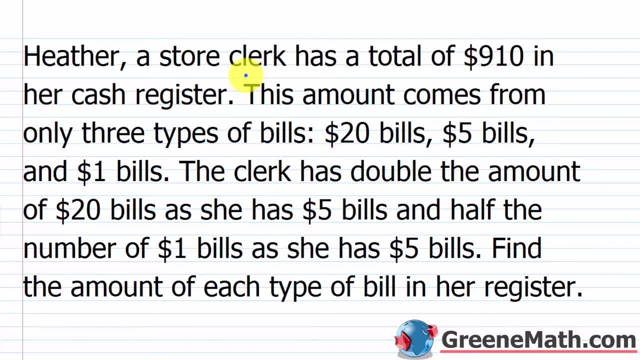 linear equations involves denominations of money. Okay, So these might be referred to as dollar word problems. You might hear them called coin word problems. just based on the situation given, Okay, And essentially all you're doing here, you're normally given a value for all of. 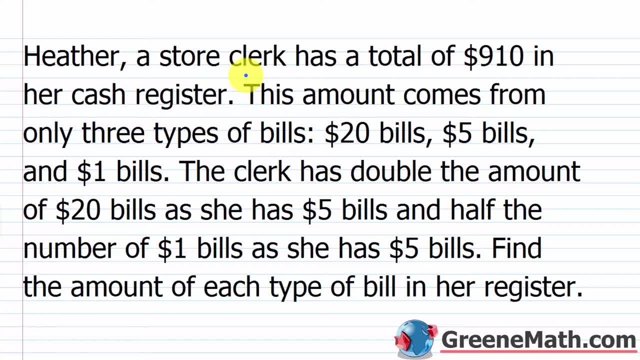 the coins or all of the bills, and you need to find the individual amounts. So how many of you know this type of coin do you have, or how much of this type of bill do you have? you know, so on and so forth. So let's jump in and look at the first example. 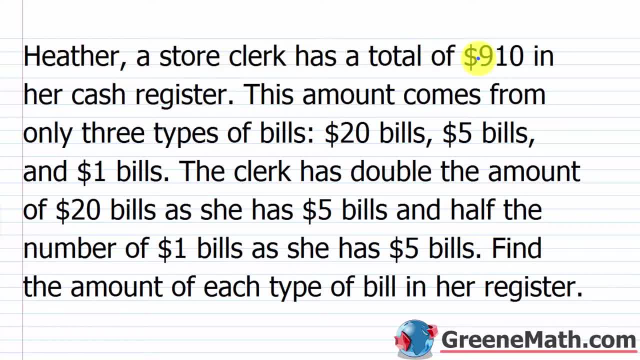 So we have Heather. a store clerk has a total of $910 in her cash register. This amount comes from only three types of bills: $20 bills, $5 bills and $1 bills. Now it says the clerk has doubled the amount of $20 bills, as she has. 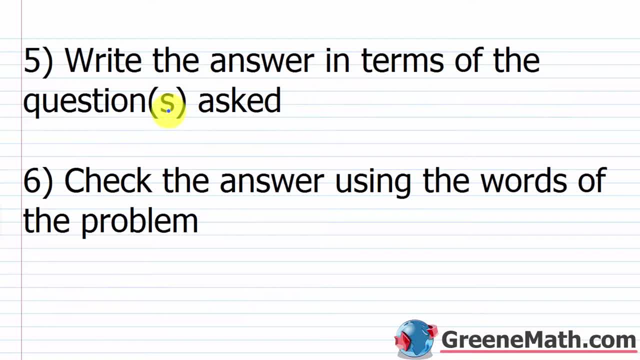 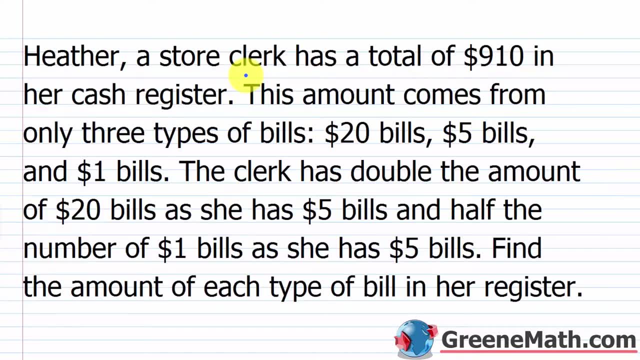 Then we're going to write the answer in terms of the question or again questions asked And lastly, we're going to check the answer using the words of the problem. We just want to make sure our answer is reasonable. So another very common problem type that occurs when we're solving applications of linear equations involves denominations of. 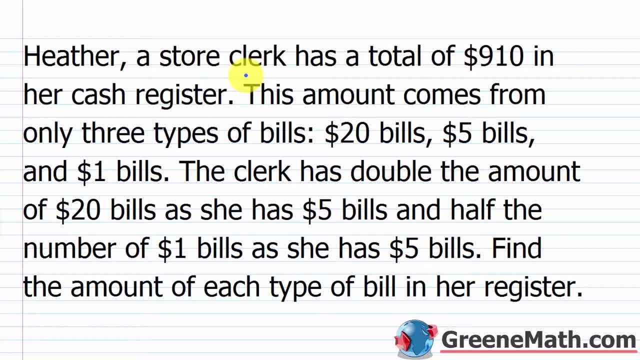 money Okay, so these might be referred to as dollar word problems. You might hear them called coin word problems, just based on the situation given Okay, and essentially all you're doing here. You're normally given a value for all of the coins or all of the bills and you need to find the individual amounts. 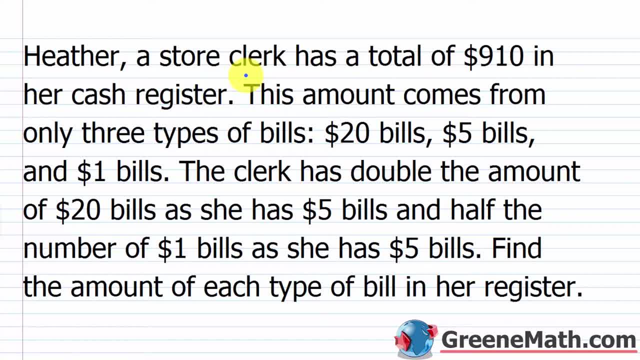 So how many of you know, this type of coin do you have? or how much of this type of bill do you have? you know, so on and so forth. So let's jump in and look at the first example. So we have Heather. 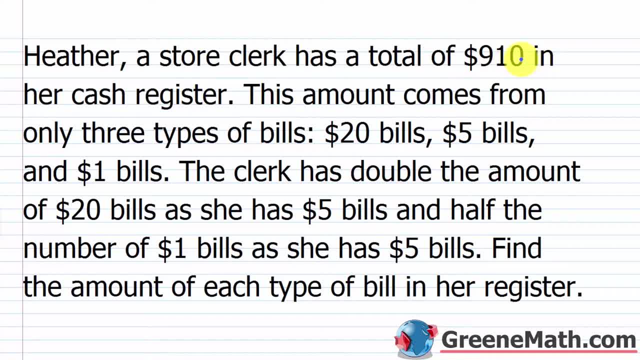 A store clerk has a total of $910 in her cash register. This amount comes from only three types of bills: $20 bills, $5 bills and $1 bills. Now it says the clerk has double the amount of $20 bills, as she has $5 bills, and half the number of $1 bills, as she has $5 bills. 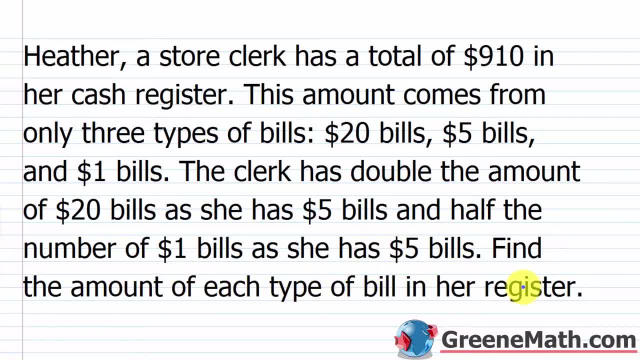 Find the amount of each type of bill in her register. So this is a very, very straightforward Problem. We just need to find, as it says here, the amount of each type of bill in her register, So how many $5 bills, how many $1 bills and how many $20 bills, and again. 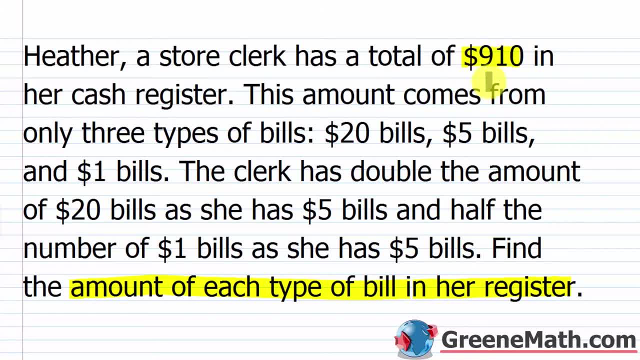 this is based on the fact that there's a total value of $910 in the register. Okay, so let's let a variable be equal to one of our unknowns. since the $5 bill is involved in both comparisons, Let's let X be equal to that. 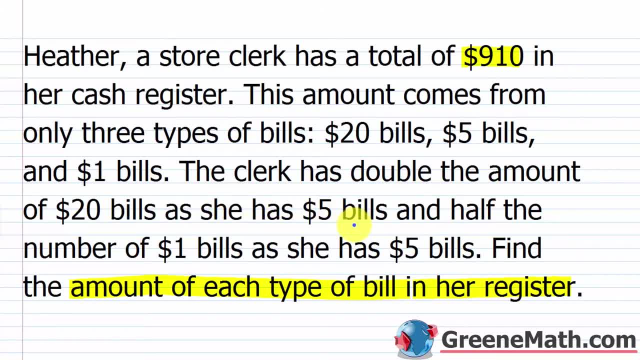 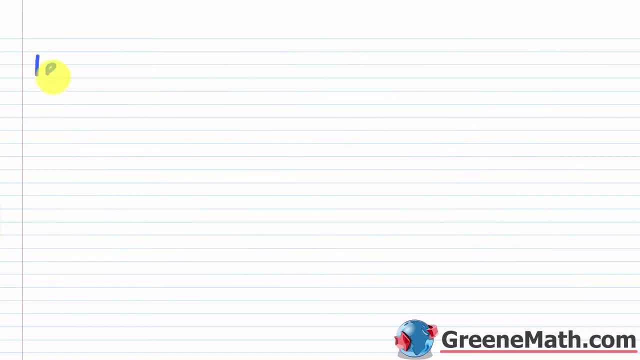 right, Because it says the clerk has double the amount of $20 bills, as she has $5 bills, and half the number of $1 bills, as she has $5 bills. So let's let X be equal to the amount, or you could say the number of $5 bills in her register. 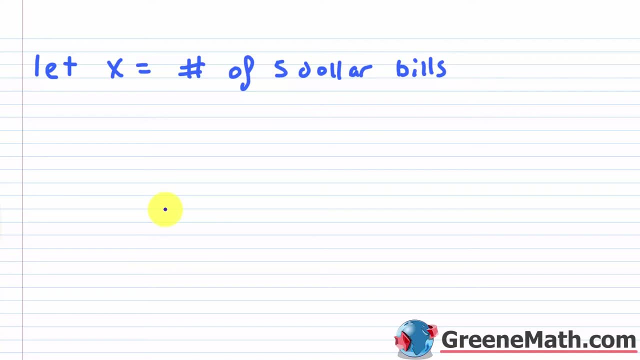 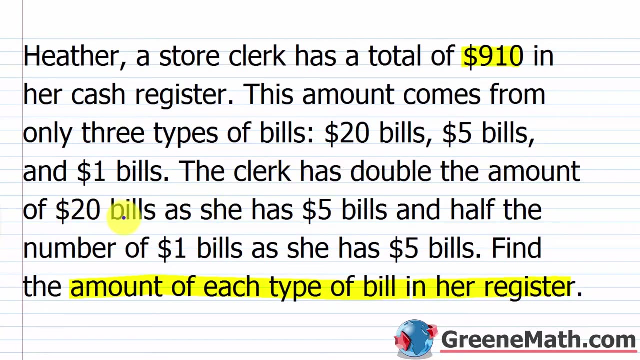 All right. So what can we say about the number of $20 bills and the number of $1 bills? So if we go back up, it says here specifically, the clerk has double the amount of $20 bills as she has $5 bills. 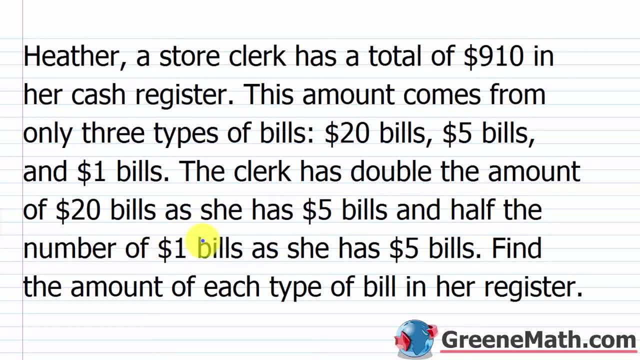 $5 bills and half the number of $1 bills, as she has $5 bills. Find the amount of each type of bill in her register. So this is a very, very straightforward problem. We just need to find, as it says here, the amount of each type of bill in her register. So how many $5 bills? 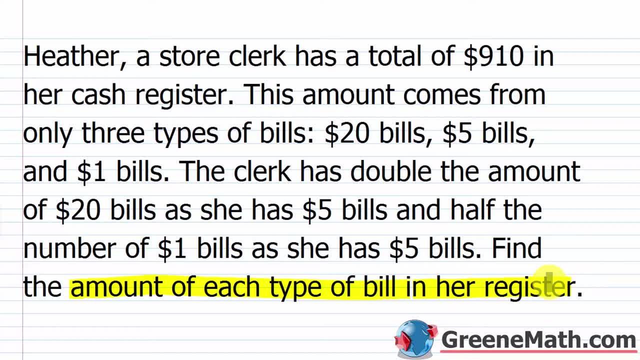 how many $1 bills and how many $20 bills. And again, this is based on the fact that there's a total value of $910 in the register. Okay, So let's let a variable be equal to one of our unknowns. Since the $5 bill is involved in both comparisons, let's let X be equal to that. 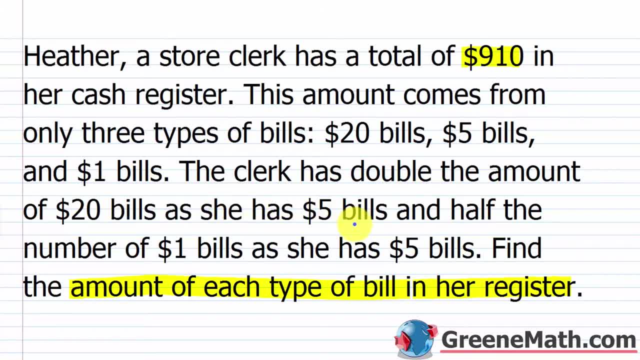 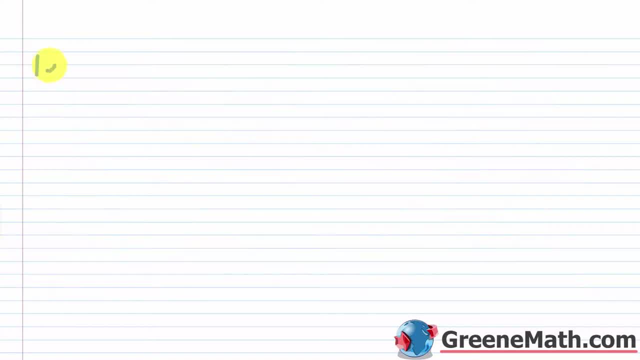 right, Because it says the clerk has doubled the amount of $20 bills, as she has $5 bills, and half the number of $1 bills, as she has $5 bills. So let's let X be equal to the amount, or you could say the number of $5 bills in her register. All right, So what can we say? 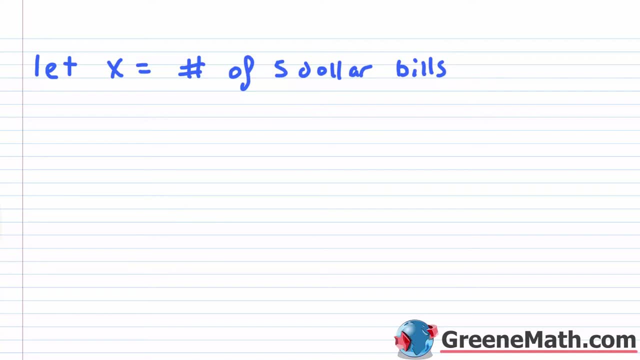 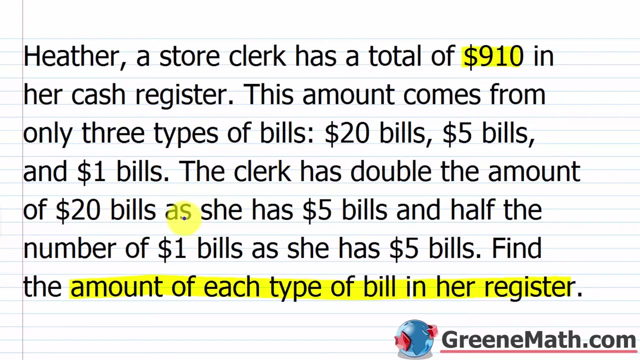 about the number of $20 bills and the number of $1 bills. So if we go back up, it says: here specifically, the clerk has doubled the amount of $20 bills as she has $5 bills. So let's let X be equal to the amount of $20 bills, as she has $5 bills. So if I take the number of $5 bills, 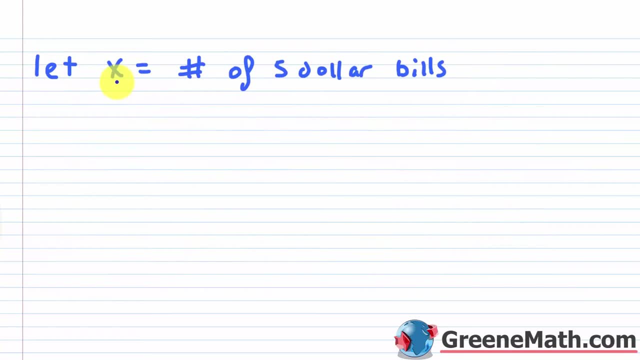 which we modeled as X, and I double that, or if I multiply it by two, that would give me 2X and that would be the number of $20 bills that she's going to have, Let's put. then we'll put our 2X is equal to the number of $20 bills. Okay, So we go back up for the number of. 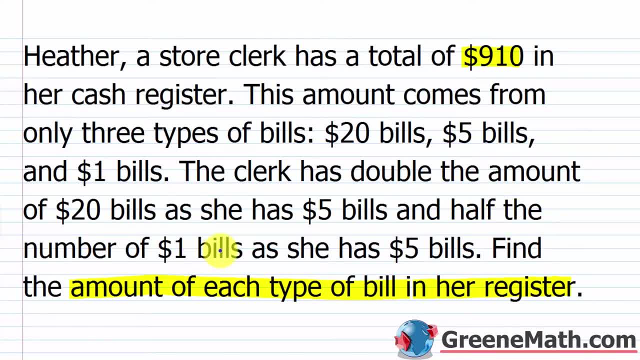 $1 bills. It says half the amount of $1 bills, as she has $5 bills. So let's let X be equal to the number of $1 bills, as she has $5 bills. So if I take half of X or just one half X, that's going. 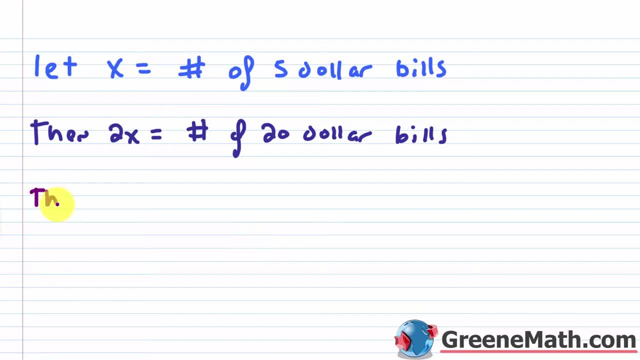 to represent the number of $1 bills. So we'll say then again, we're going to do one half times X, equal to X over two. whatever you want to do is equal to the number of $1.. Let me make that. 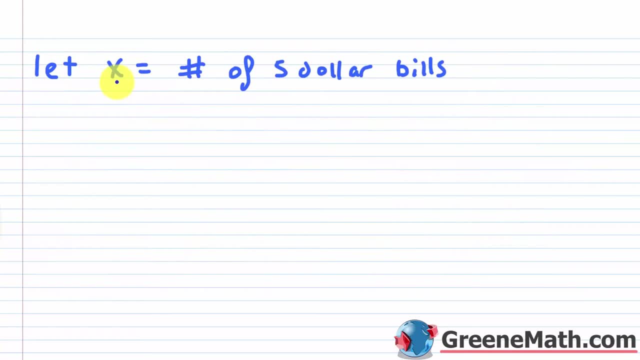 So if I take the number of $5 bills, which we modeled as X, and I double that, or if I multiply it by 2, that would give me 2x and that would be the number of $20 bills that she's going to have. 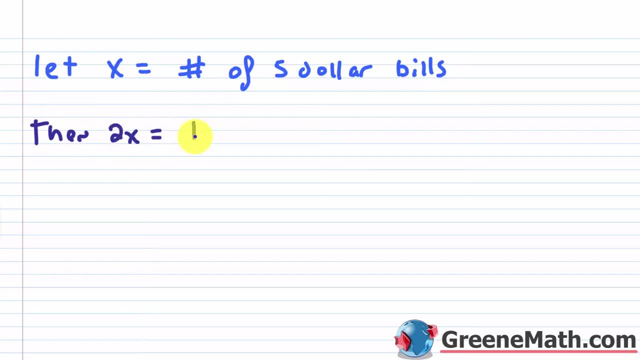 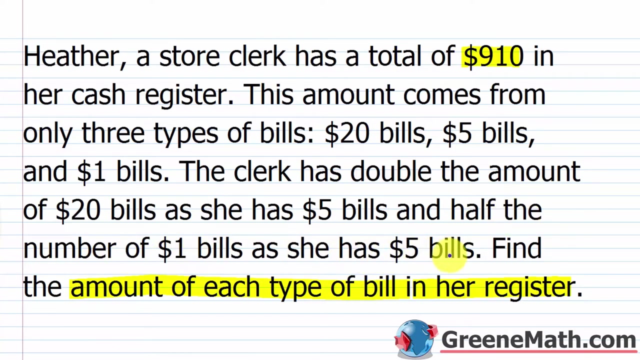 Let's put. then we'll put: our 2x is equal to the number of $20 bills. Okay, so we go back up For the number of $1 bills. It says half the number of $1 bills, as she has $5 bills. 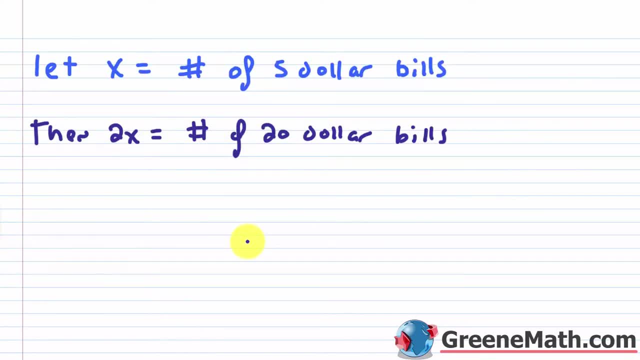 So if I take half of X or just one half X, that's going to represent the number of $1 bills. So we'll say then again we're going to do one half times X, equal to X over to whatever you want to do is equal to the number of $1. 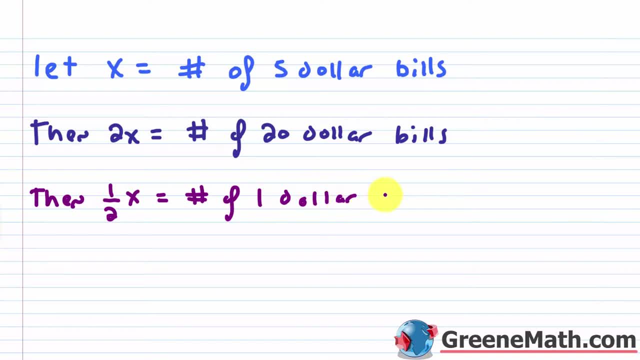 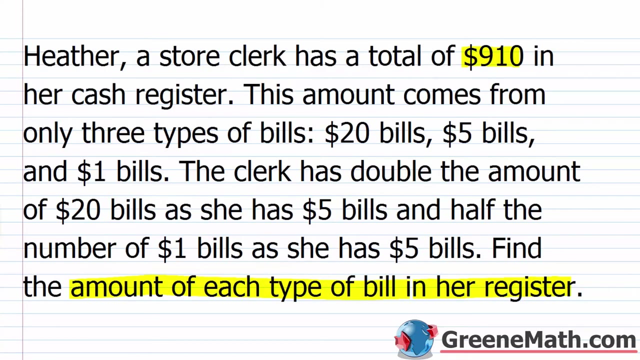 Let me make that better Again: $1 bills. Okay, so how do we get an equation going? We've modeled all of our kind of unknowns, but we need an equation to get a solution. So let's go back up Now. 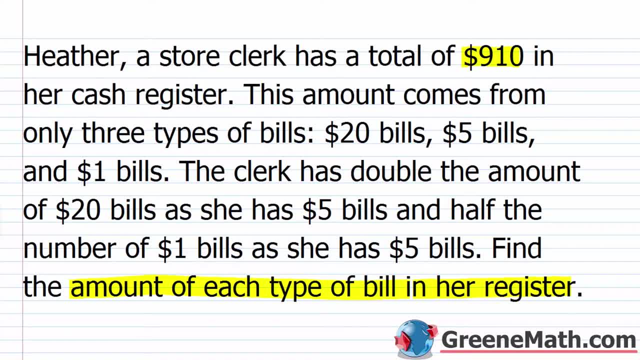 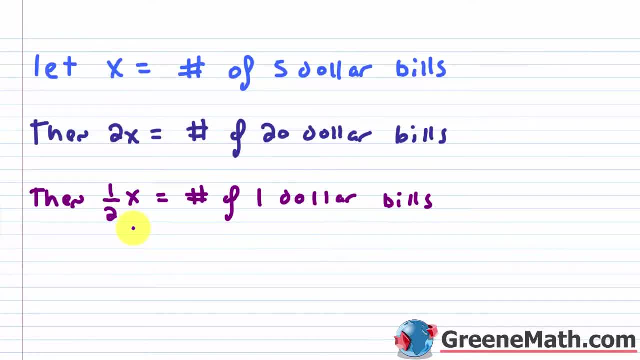 It says: a store clerk has a total of $910 in her cash register, where the problem comes in a lot of students at this point They're used to kind of summing what they have and setting it equal to that value. So you see a lot of people do this. 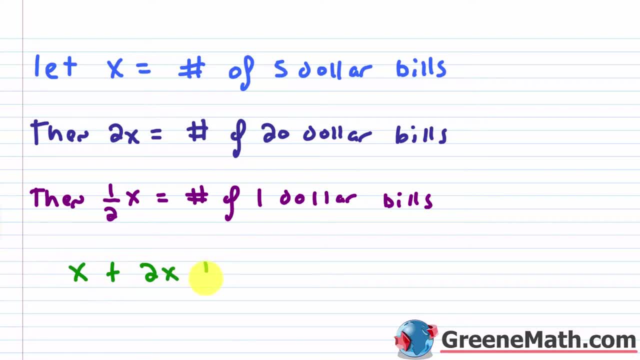 They'll go Okay. X plus 2x plus 1x, X plus 1 half X is equal to 910.. This is not the correct equation. Why is that the case? Well, what I have on the left here is going to be the total amount of bills that she has right between the $5 bills, the $20 bills and the $1 bills. 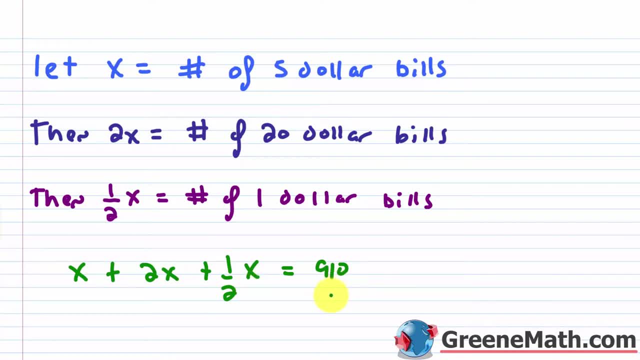 What I have on the right is a value. Okay, so it's not the same. These two would not be equal. So suppose you had six $20 bills in your wallet or purse. How would you find the value there? You wouldn't say you just have six bills. 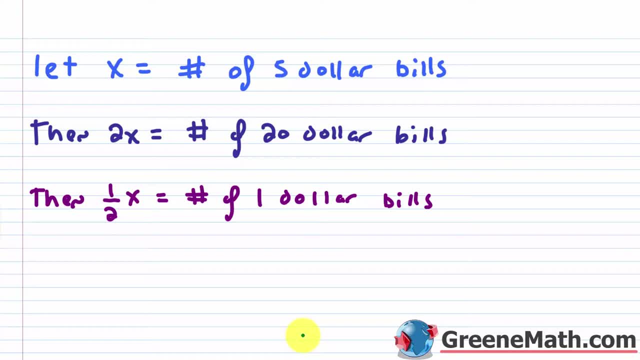 You would say that you have six times 20, or $120.. Okay, it's another words going to be found by multiplying the quantity of bills, which is 6, by the value of each bill, which is 20, which gives us 120. 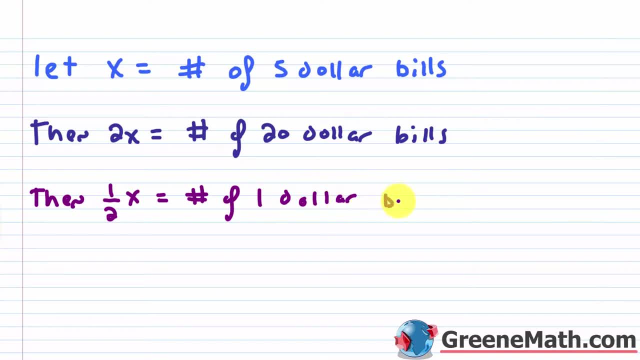 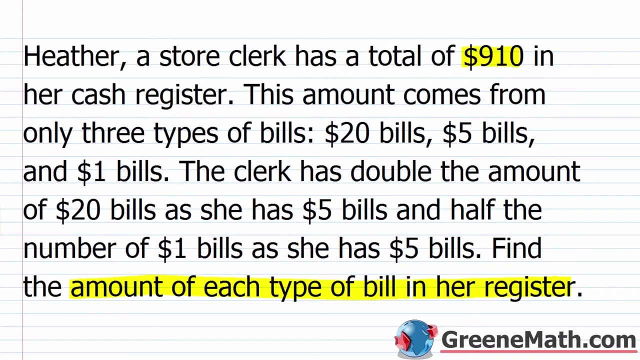 better Again: $1 bills, Okay, So how do we get an equation going? We've modeled all of our kind of unknowns, but we need an equation to get a solution. So let's go back up Now. it says a store clerk has 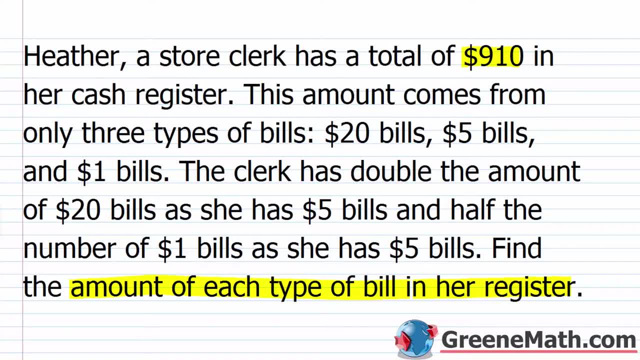 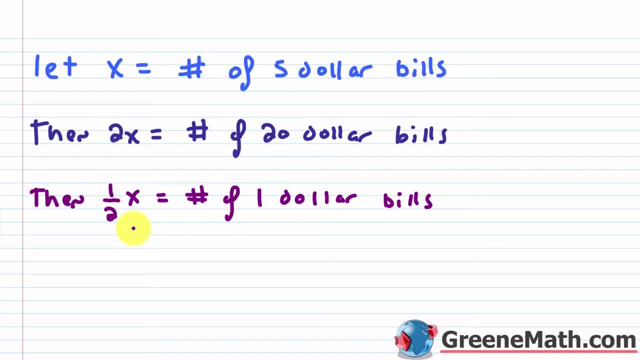 a total of $910 in her cash register, Where the problem comes in. a lot of students at this point they're used to kind of summing what they have and setting it equal to that value. So you see a lot of people do this. They'll go okay. X plus 2X plus one half X is equal to 910. 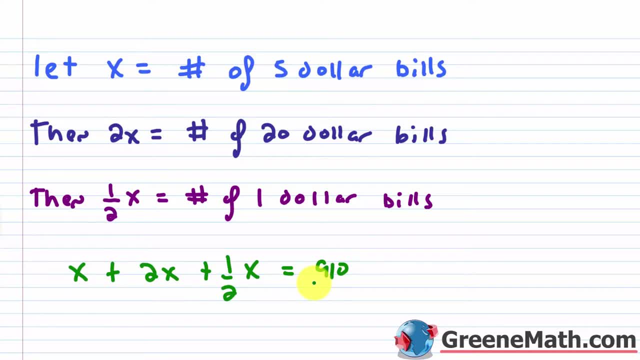 This is not the correct equation. Why is that the case? Well, what I have on the left here is going to be the total amount of bills that she has right Between the $5 bills, the $20 bills and the $1 bills. What I have on the right is a value. Okay, So it's not the same. 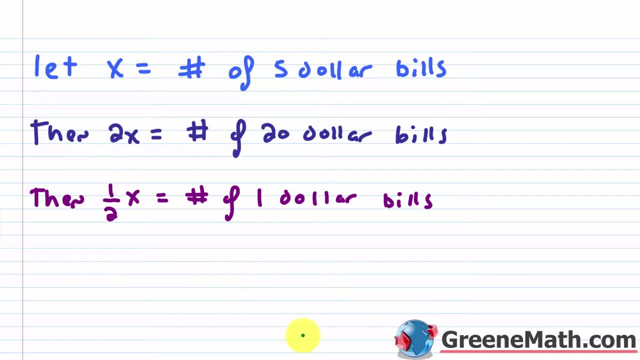 These two would not be equal. So suppose you had six $20 bills in your wallet or purse, How would you find the value there? You wouldn't say you just have six bills. You would say that you have six times 20 or $120. 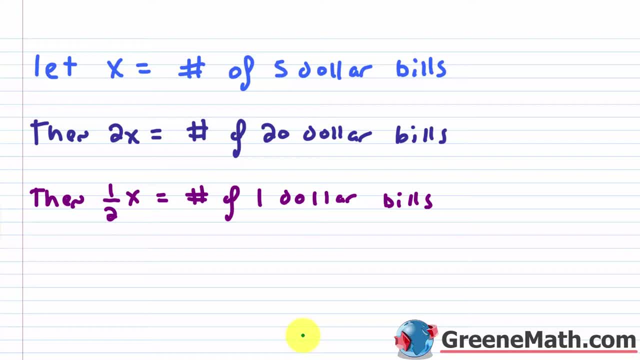 Okay, It's. another word's going to be found by multiplying the quantity of bills, which is six, by the value of each bill, which is 20, which gives us 120,. right, That's how we got the value. So we're going to basically do the same thing To get our 910 total value. 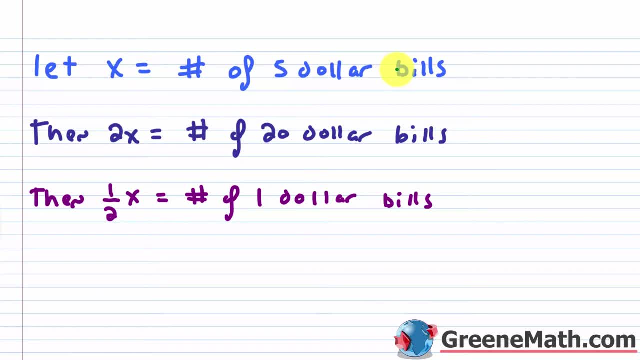 we need to take the number of $5 bills and multiply it by five, plus the number of $20 bills, multiply it by 20, plus the number of $1 bills and multiply it by one. So let's do this with a nice little table. Let's go down here. 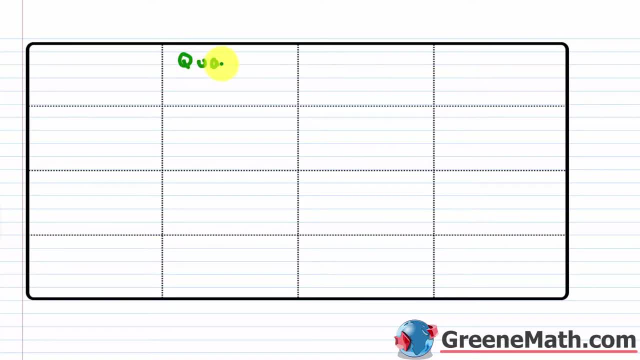 And, essentially, what I'm going to have here is the quantity of bills, And what I'm going to have here is the value per bill, And what I'm going to have here is the total value. Okay, Pretty straightforward. So we have our $20 bills. Let's just label this as 20.. 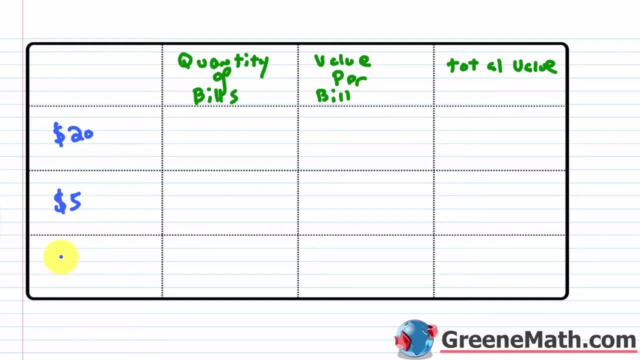 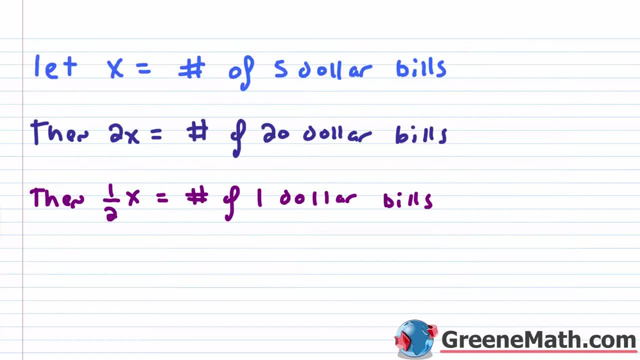 And we have our $5 bills, We'll label that as 5.. And we have our $1 bills. Just label that as 1.. So the quantity of bills: again, if I go back up, I know that the $5 bills are labeled with X. 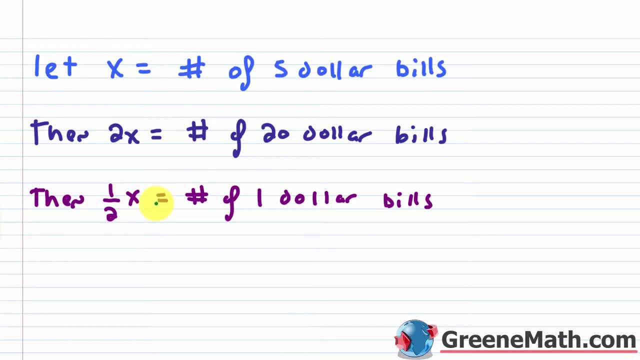 Right, That's how we got the value, So we're going to basically do the same thing. to get our 910 total value, We need to take the number of $5 bills and multiply it by 5, plus the number of $20 bills multiplied by 20.. 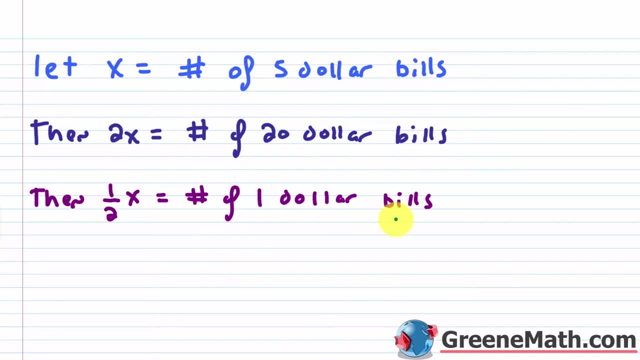 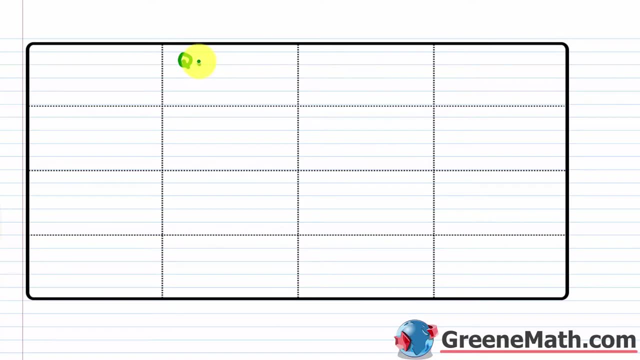 Plus the number of $1 bills and multiply it by 1.. So let's do this with a nice little table, Let's go down here And essentially what I'm going to have here is the quantity Of bills, And what I'm going to have here is the value per bill. 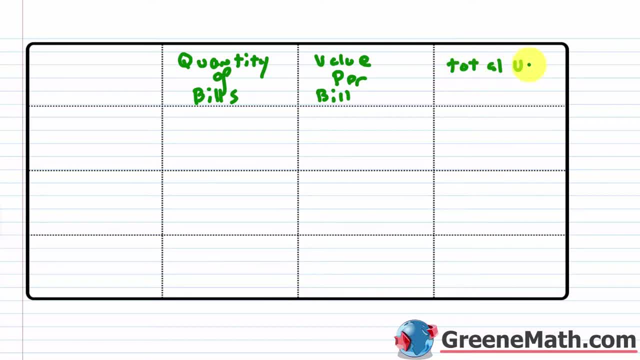 And what I'm going to have here is the total value. Okay, pretty straightforward. So we have our $20 bills- Let's just label this as 20.. And we have our $5 bills- Label that as 5.. And we have our $1 bills. 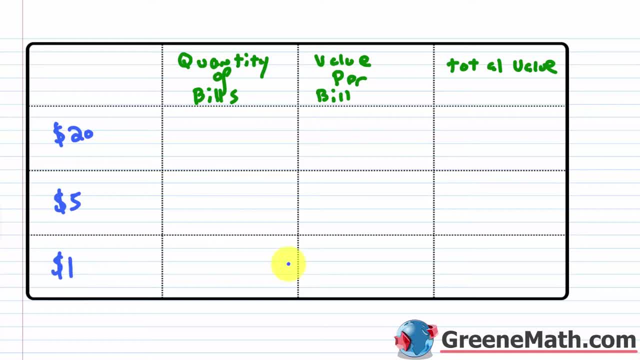 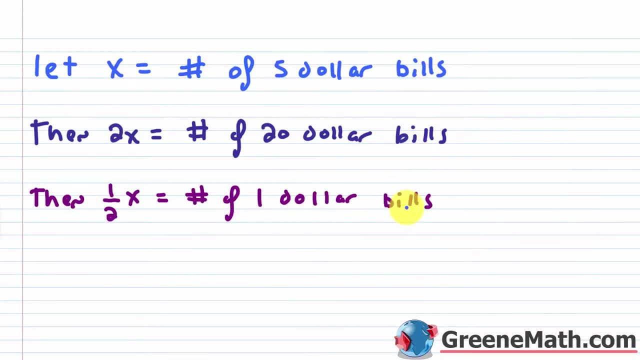 Just label that as 1.. So the quantity of bills. Again, if I go back up, I know that the $5 bills are labeled with X, The $20 bills are labeled with 2X and the $1 bills are labeled with 1 half X. 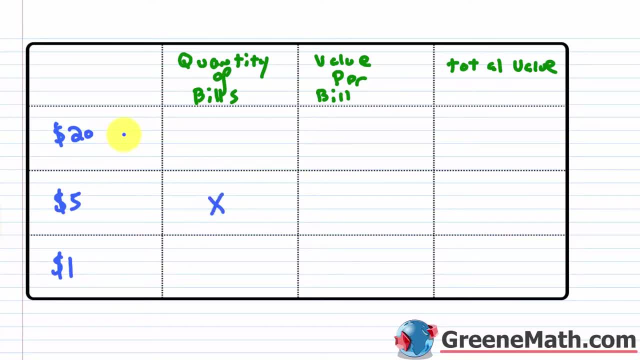 So the quantity of bills: for the $5 bills It's X, For the $20 bills it's 2X And for the $1 bills it's 1 half X, Or again you can do X over 2.. 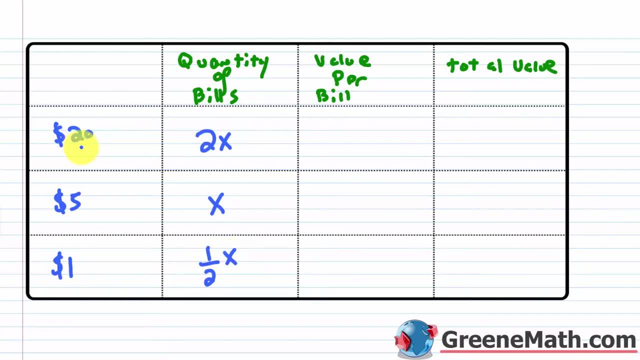 Now the value per bill. That's pretty easy. Just look all the way to the left. This one's going to be 20.. This one's going to be 5. And this one's going to be 1.. Okay, that's pretty straightforward. 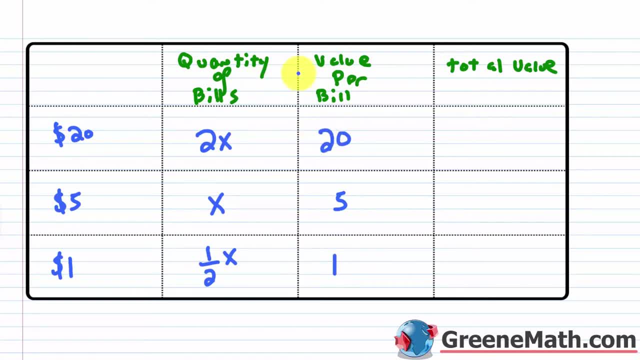 Then to get the total value, I just multiply across right, This times this will be equal to this. Okay, So 2X times 20 would be 40X, X times 5 would be 5X, And then 1 half X times 1 would be 1 half X. 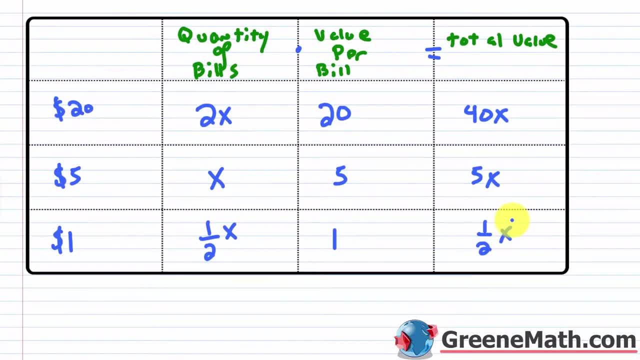 So now I have something that I can set up an equation with. I have the total value of the 20s, which is 40X, Plus the total value of the 5s, which is 5X, Plus the total value of the 1s, which is 1 half X. 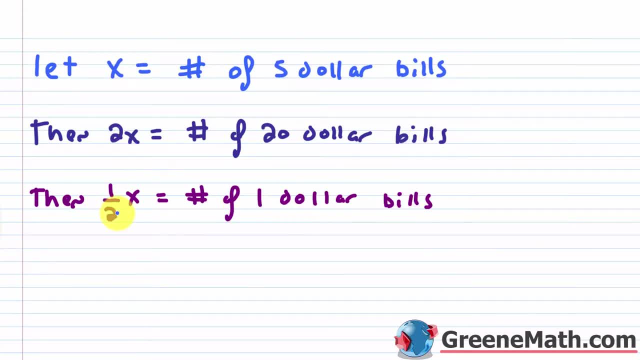 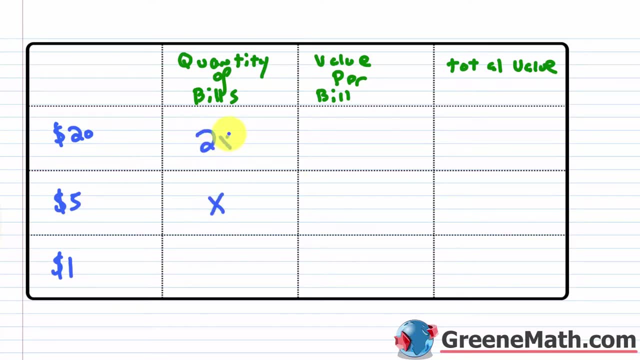 the $20 bills are labeled with 2X and the $1 bills are labeled with 1 half X. So the quantity of bills: for the $5 bills it's X, For the $20 bills it's 2X And for the $1 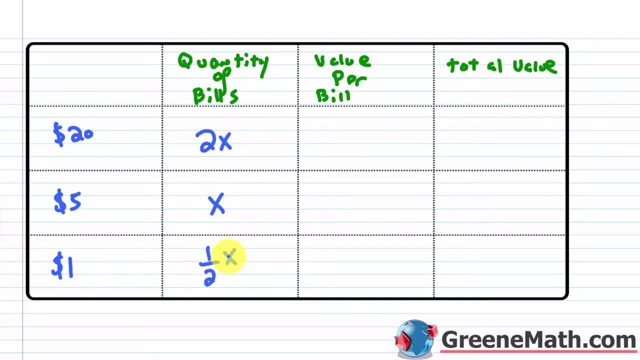 bills. it's 1 half X, Or again you can do X over 2.. Okay, So we're going to have our $20 bills and we're going to have our $1 bills and we're going to. That's pretty easy. Just look all the way to the left. This one's going to be 20.. This one's going. 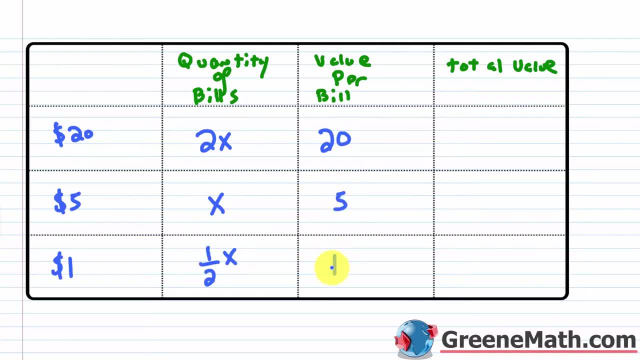 to be 5.. And this one's going to be 1.. Okay, That's pretty straightforward. Then, to get the total value, I just multiply across right. This times this will be equal to this. Okay, So 2X times 20 would be 40X, X times 5 would be 5X, And then 1 half X times 1 would be 1 half X. 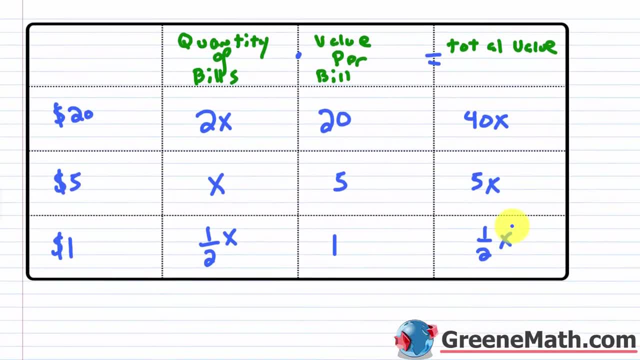 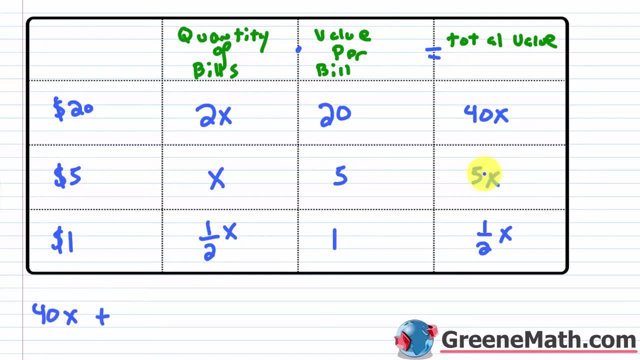 So now I have something that I can set up an equation with. I have the total value of $20.. The value of the 20s, which is 40X plus the total value of the 5s, which is 5X plus the total value. 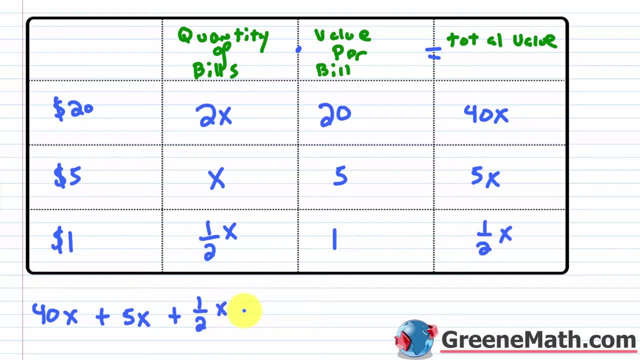 of the 1s, which is 1 half X, And this is equal to again, the 910, that amount of dollars which is the total value in her cash register. Okay, So you've got to go through and make this setup here. 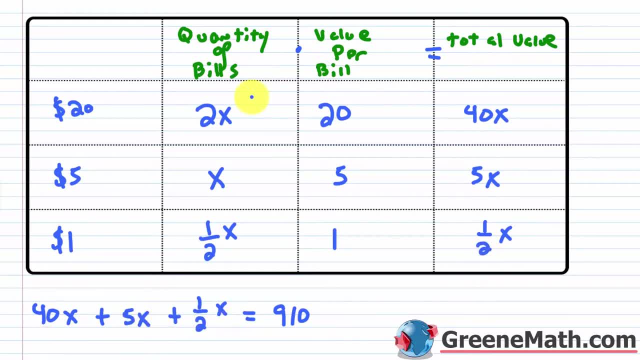 Otherwise, you're not going to get the right answer by just going through and saying, okay, I have 2X plus X plus 1 half X and setting That's a 910, because you're not setting a value equal to a value. Okay, That doesn't work. 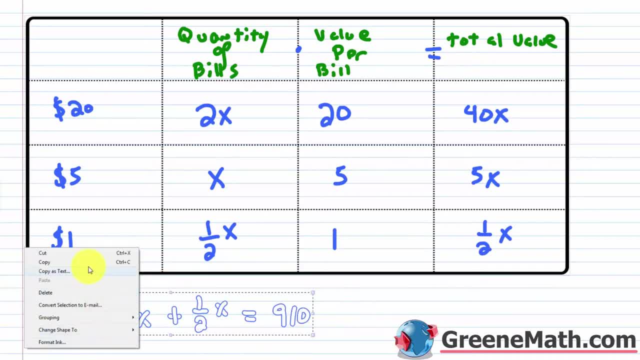 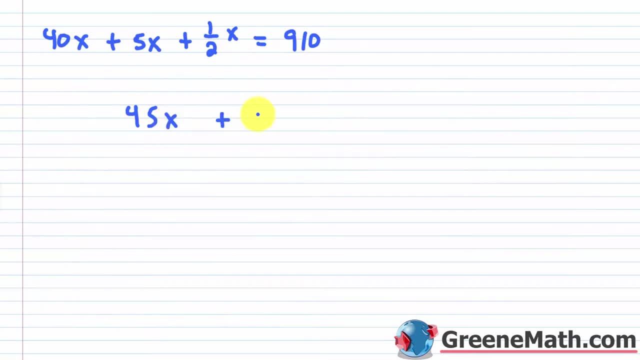 So let's go ahead and solve this guy. I'm just going to copy this and go to a fresh sheet. All right, So what I can do, 40X plus 5X is 45X. Then plus 1 half X equals 910.. I want to clear that denominator. Let's multiply both sides of. 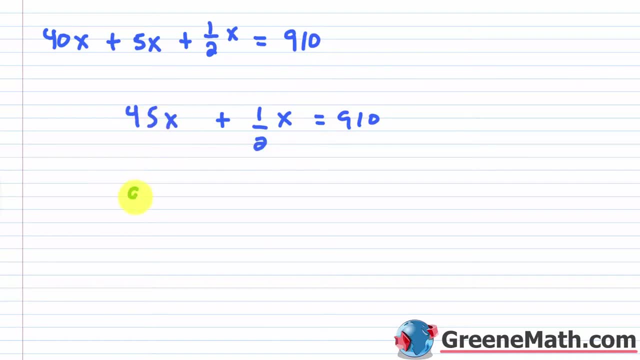 the equation by 2.. So the 45X. if I multiply that by 2, I get 90X. And plus 1 half X times 2 would be just X, And this equals 910 times 2 would be 1,820.. And now 90X plus X would just be 91X. 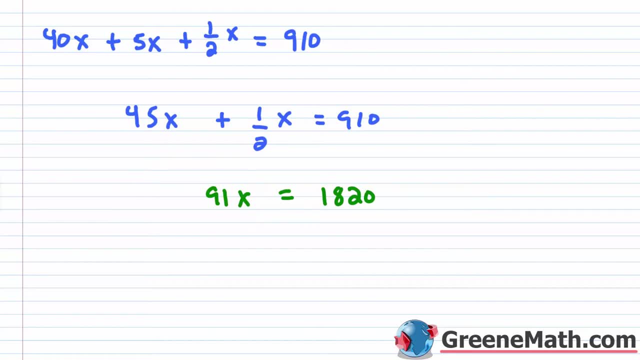 So let's write this as 91X. To get X by itself, I divide both sides of the equation by 91. And we're going to find that X is equal to 20.. Okay, So again we're not done, We have to go. 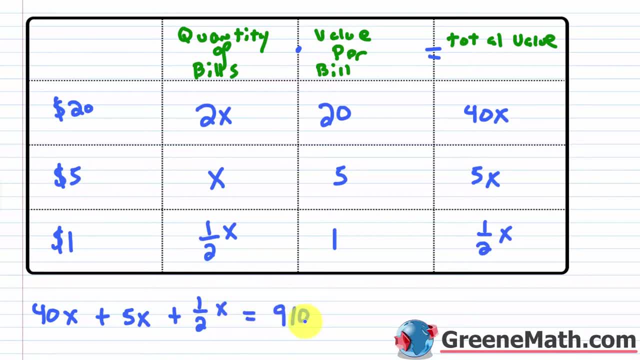 And this is equal to, again, the 910.. That amount of dollars, which is the total value in her cash register. Okay, I'm going to go through and make this set up here, Otherwise you're not going to get the right answer by just going through and saying: 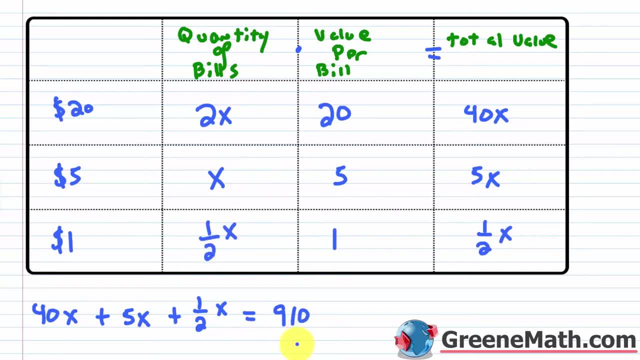 okay, I have 2X plus X plus 1 half X and setting that to 910.. Because you're not setting a value equal to a value. Okay, that doesn't work. So let's go ahead and solve this guy. I'm just going to copy this and go to a fresh sheet. 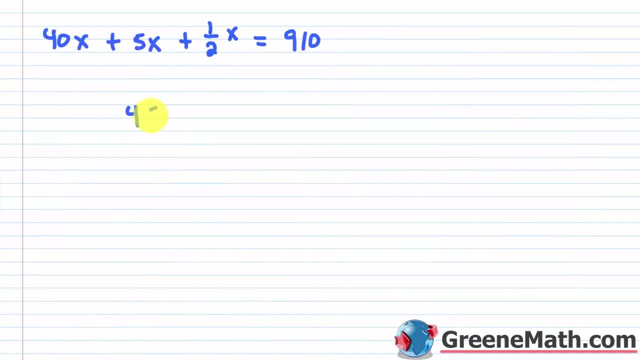 All right. So what I can do, 40X plus 5X is 45X. Then plus 1 half X equals 910.. I want to clear that denominator. Let's multiply both sides The equation by 2.. So the 45X. if I multiply that by 2, I get 90X. 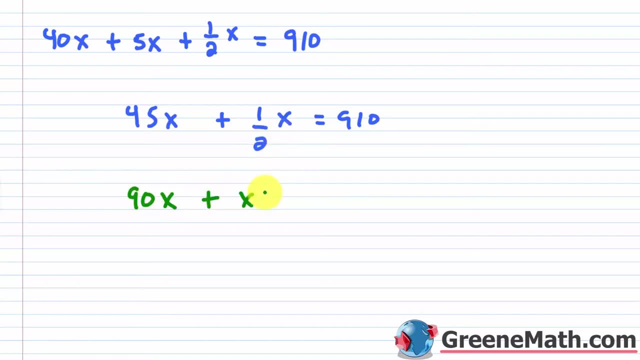 And plus 1 half X times 2 would be just X. And this equals 910 times 2 would be 1820.. And now 90X plus X would just be 91X. So let's write this as 91X. 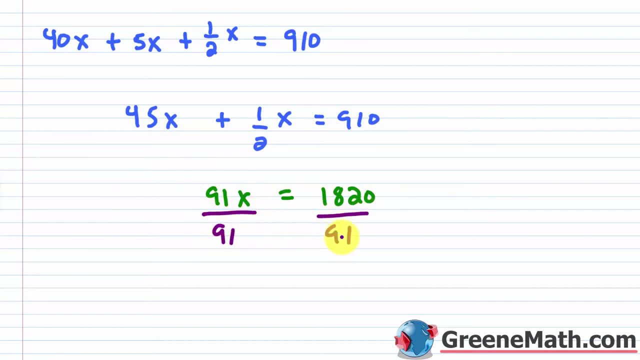 To get X by itself, I divide both sides of the equation by 91. And we're going to find that X is equal to 20.. Okay, So again we're not done. We have to go back And make sense of this. 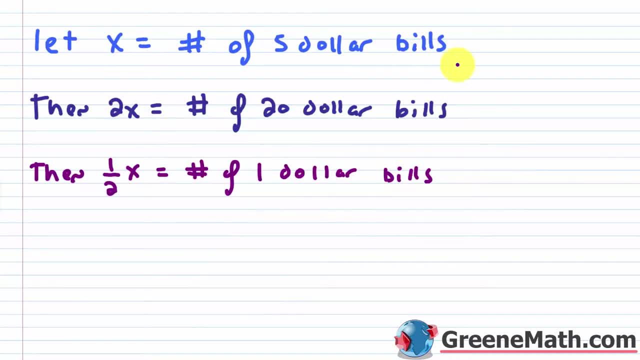 So X equals 20.. So X was the number of $5 bills, So that's going to be 20.. Then 2X is the number of $20 bills. 2 times 20 is 40. Then 1 half X is going to be the number of $1 bills. 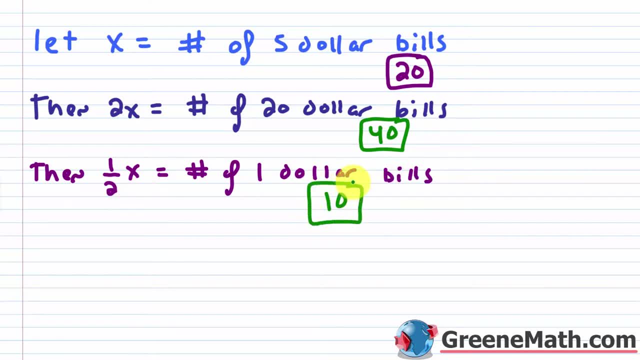 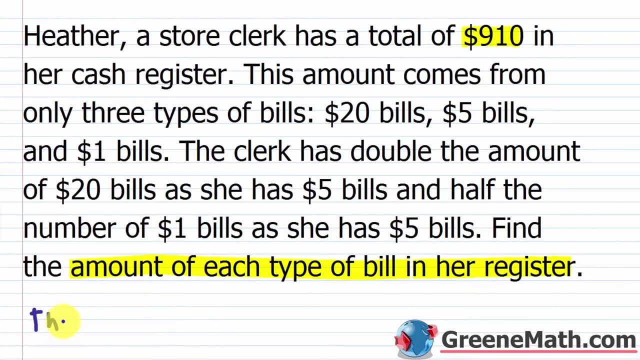 So 1 half times 20 is 10.. Okay, so let's go back up and write our answer. So what we're going to say is that there are there are 20 $5 bills And then you have 40 $20 bills. 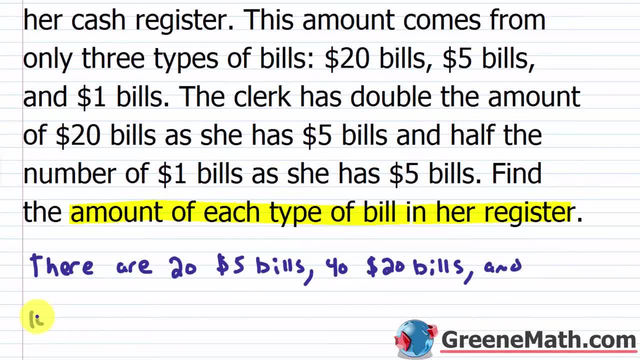 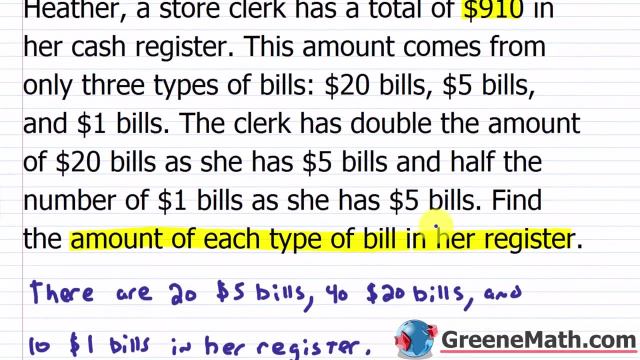 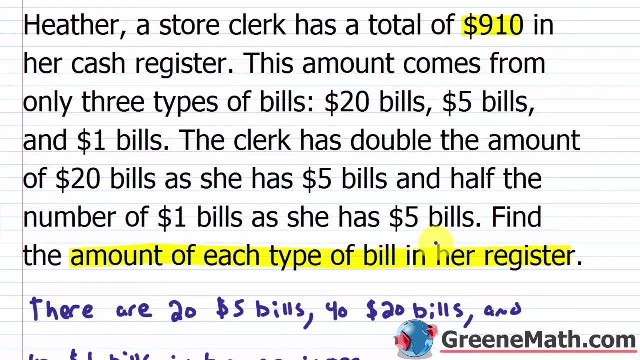 And you're going to have 10 $1 bills In her. let me make that better Register, All right, so let's check this and make sure it makes logical sense. So it tells us that again, she has a total value of $910 in her cash register. 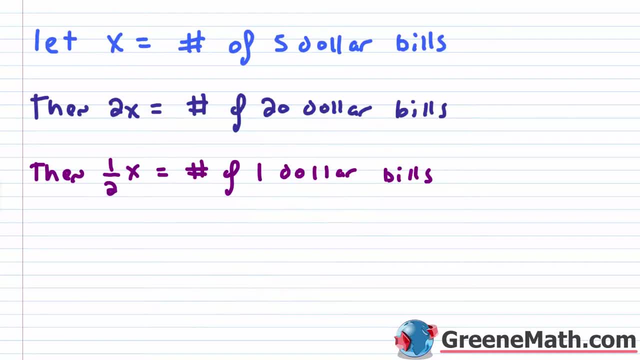 back and make sense of this. So X equals 20.. So X was the number of $5 bills, So that's going to be 20.. Then 2X is the number of $20 bills. 2 times 20 is 40. Then 1 half X is going to be the number of $1. 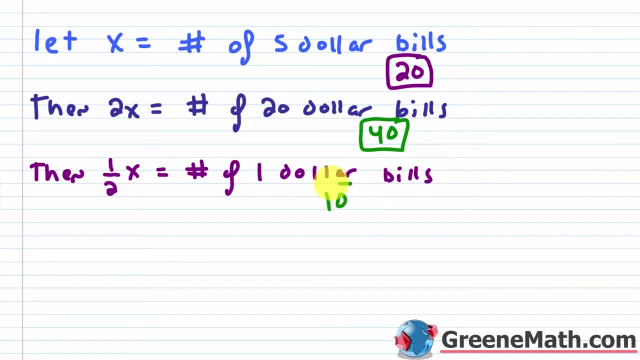 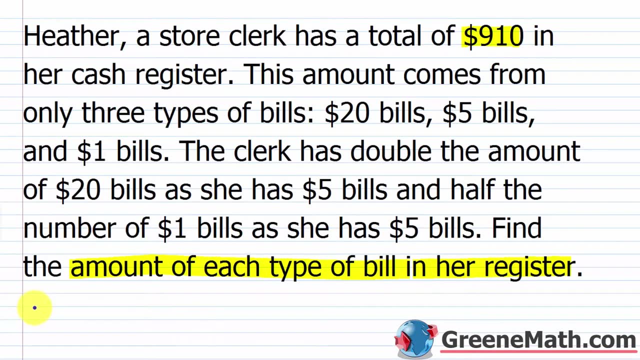 bills. So 1 half times 20 is 10.. Okay, So let's go back up and write our answer. So what we're going to say is that there are there are 20 $5 bills And then you have 40 $20 bills. 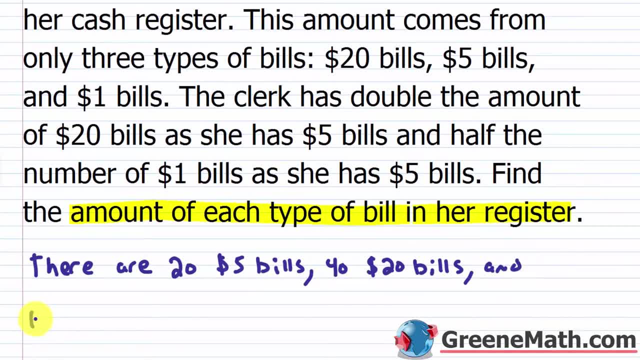 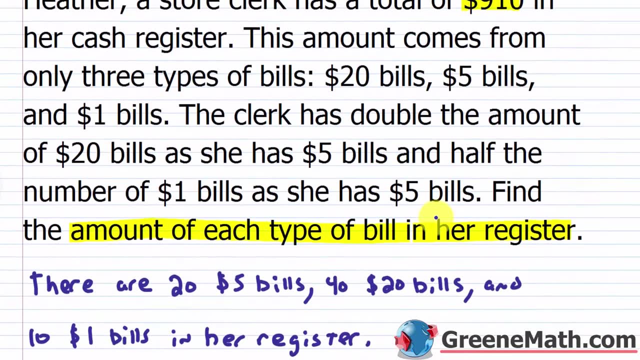 And you're going to have 10 $1 bills in her. let me make that better register, All right, So let's check this and make sure it makes logical sense. So it tells us that again, she has a total value of. 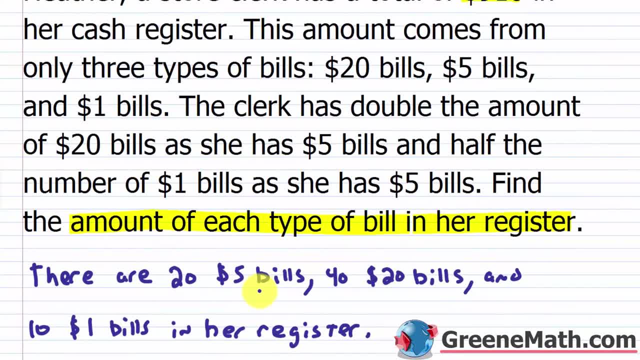 $910 in her cash register. So $25 bills is $100.. Let me just line this up and put this as a hundred: 40 $20 bills is $800 and 10 $1 bills is $10.. So some of those amounts- 100 plus 800 plus 10- is 910. 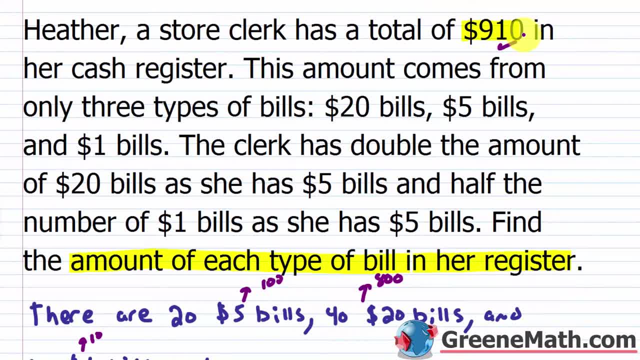 So this part to check. okay, that works out. It says this amount comes from three types of bills: $20 bills, $5 bills and $1 bills. Good to go there. The clerk has double the amount of $20 bills. 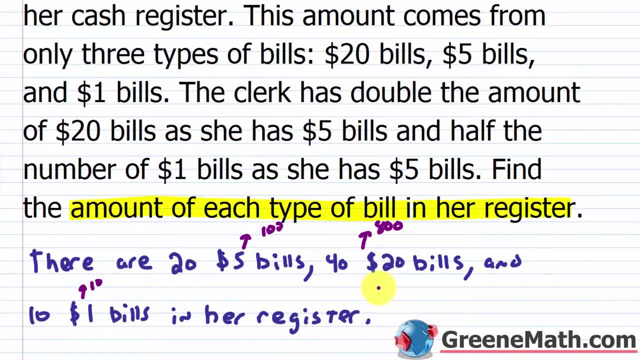 She has $5 bills bills again. she has 25s and she has 40 20s. so we're good there. and then it says she has half the number of one dollar bills, that she has five dollar bills. you've got again 25s and you've got. 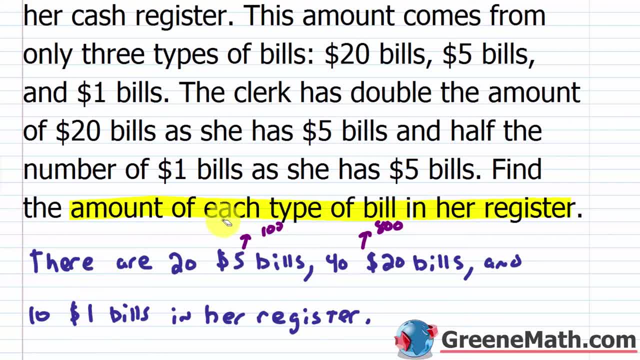 10 ones. so good to go there. so everything checks itself out. we can say our answer here is correct. we'll go ahead and just state this again: there are 25 dollar bills, 40 20 dollar bills and 10 one dollar bills in her register. all right, let's take a look at another one again. these are pretty. 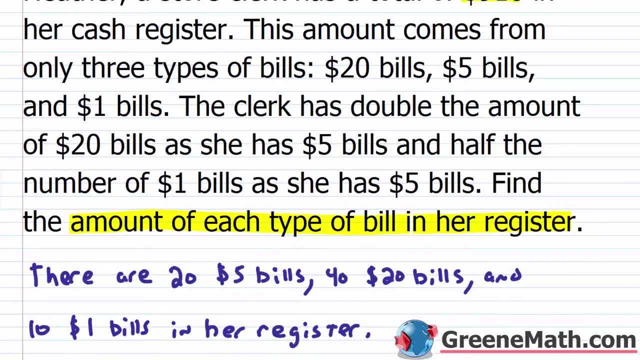 So $25 bills is $100.. Let me just line this up and put this as 100.. 40 $20 bills is $800.. And 10 $1 bills is $10.. So sum those amounts 100 plus 800 plus 10 is 910. 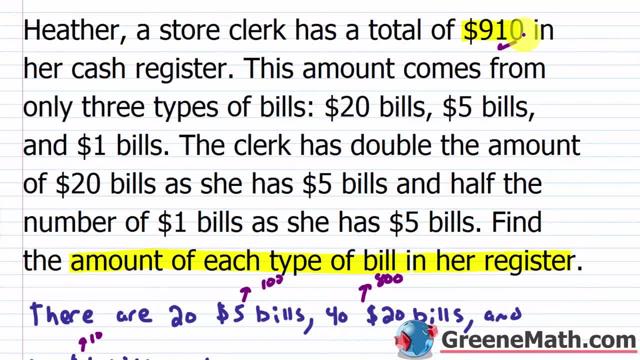 So this part's a check. Okay, that works out. It says this amount comes from three types of bills: $20 bills, $5 bills and $1 bills. Good to go there. The clerk has double the amount of $20 bills as she has $5 bills. 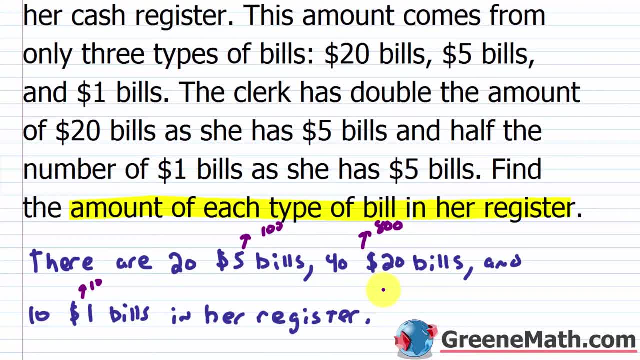 Again she has 25s and she has 40 20s. So we're good there. And then it says she has half the number of $1 bills. as she has $5 bills, You've got again 25s and you've got 10 ones. 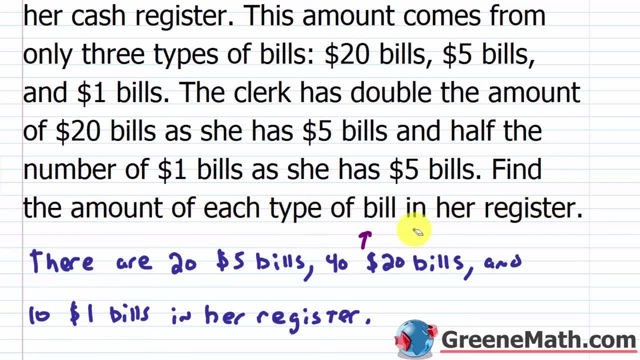 So good to go there. So everything checks itself out. We can say: our answer here is correct. We'll go ahead and just state this again: There are 25 $1 bills, 40 $20 bills And 10 $1 bills in her register. 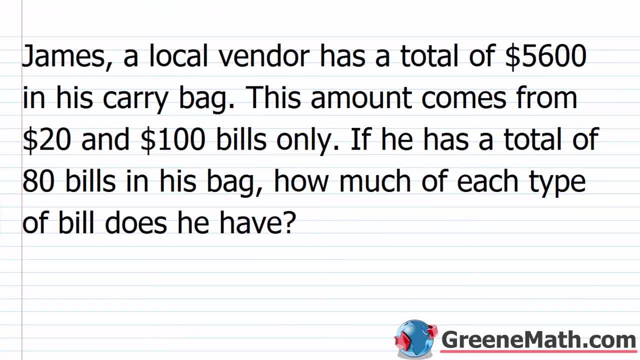 All right, let's take a look at another one. Again, these are pretty easy overall. So James, a local vendor, has a total of $5,600 in his carry bag. This amount comes from $20 and $100 bills only. 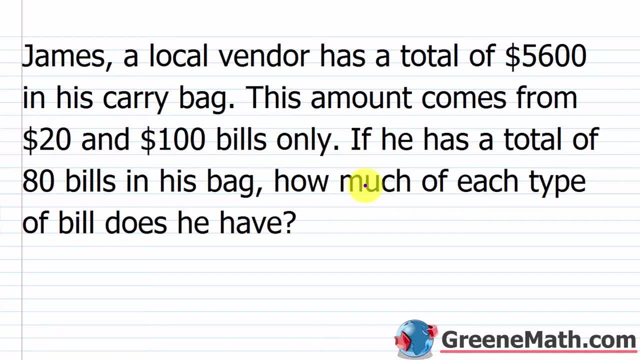 If he has a total of 80 bills in his bag, how much of each type of bill does he have? So, in other words, what we're trying to find here, it says how much of each bill does he have. Well, we want to know how much of the $20 bills does he have and how much of the $100 bills does he have? 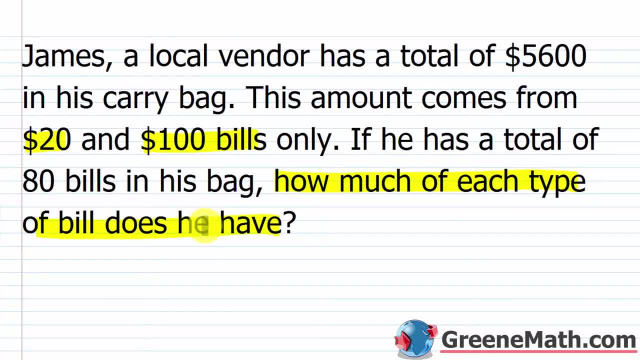 Because, again, he only has those two types of bills in the bag. And again, another thing to highlight here is that he has a total of $5,600 and there's only 80 bills in the bag. Okay, so let's let a variable represent one of the unknowns. 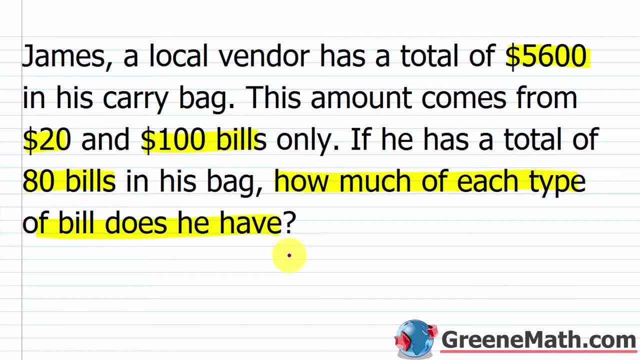 It could be the $20 bills or it could be the $100 bills. The key to understanding this problem is knowing that if he has a total of 80 bills in the bag, whatever I let x represent, then 80 minus x is going to represent the other one. 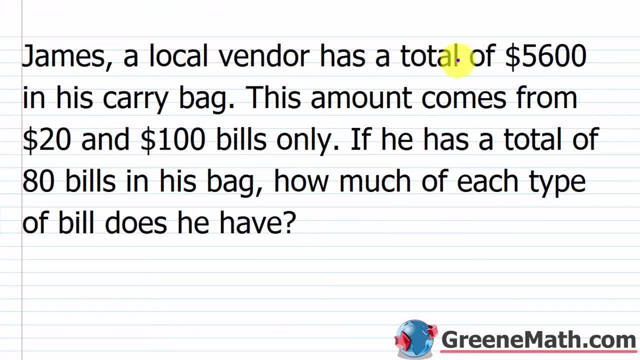 easy overall. so james, a local vendor, has a total of 5600 in his carry bag. this amount comes from 20 and 100 bills only. if he has a total of 80 bills in his bag, how much of each type of bill does he have? so, in other words, what we're trying to find here, it says how much of each bill does. 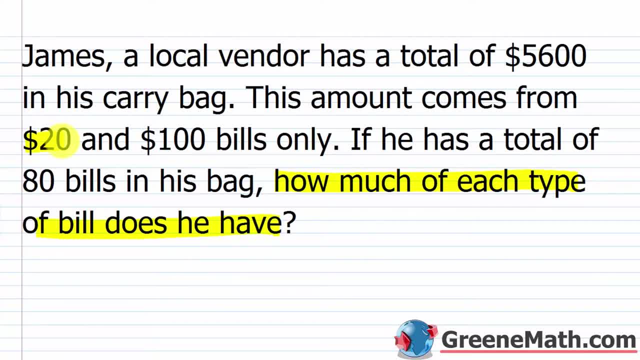 he have. we want to know how much of the 20 bills does he have and how much of the hundred dollar bills does he have, you to know how much of each bill does he have, because, again, he only has those two types of bills in the bag. and again, another thing to highlight here is that he has a total of 5600 and there's 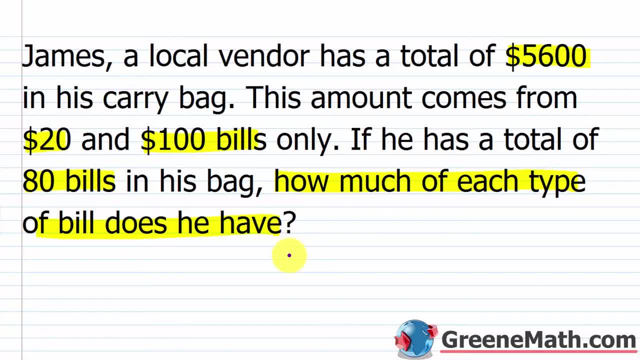 only 80 bills in the bag. okay, so let's let a variable represent one of the unknowns. it could be the 20 bills, or it could be the hundred dollar bills. the key to understanding this problem is knowing that if he has a total of 80 bills in the bag, whatever i let x represent, then 80 minus x is. 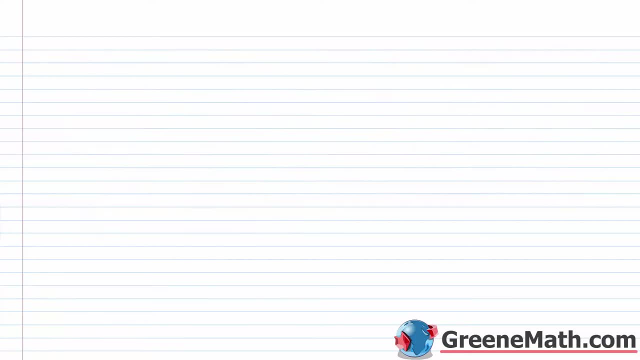 going to represent the other one. so in other words, if i let x be equal to the number of 20 bills, then because again there's only 80 bills in the bag, it has to be true that we could say 80. the total number of bills minus acts. the number of twenty dollar bills has to be: 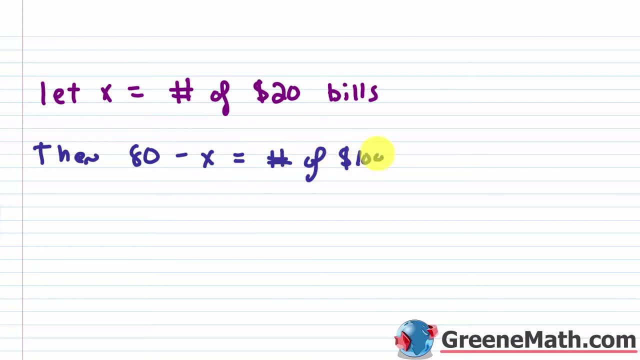 equal to the number of 100 dollars. bisher aabicannesantas nesse severi was actually important information, since in a theirضobarwahl one hundred dollars because两ahrobanoff was initially the one bill that baseball and make this a little bit better. Okay, So now that we have both of our unknowns, kind of modeled. 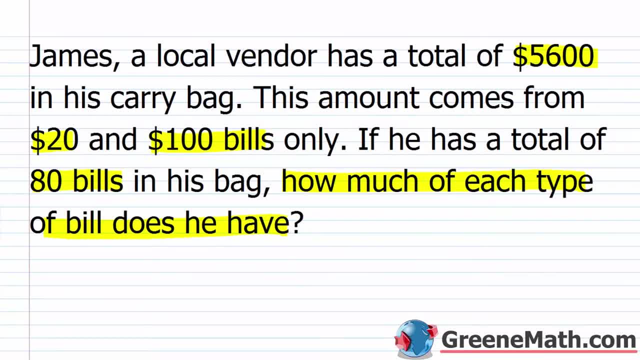 let's think about how we can get an equation going. So again, just like with the last problem, we're given a value, okay, But we've modeled things as kind of an amount of bills that we have. So we have to again go through, set up a little table and relate the values. 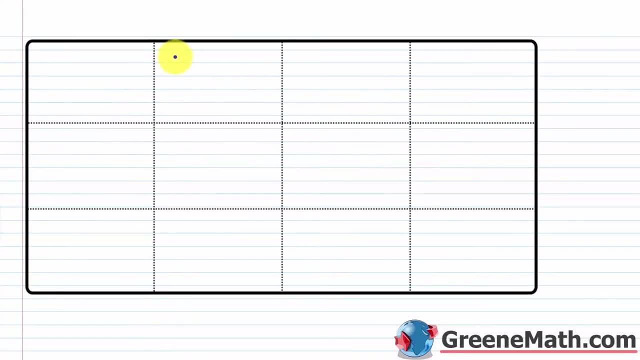 So let's go down here And again, I'm going to say I have quantity of bills, I'm going to say value per bill And I'm going to say total value. Again, if I take the quantity of bills times the value per bill, I will get the total value. 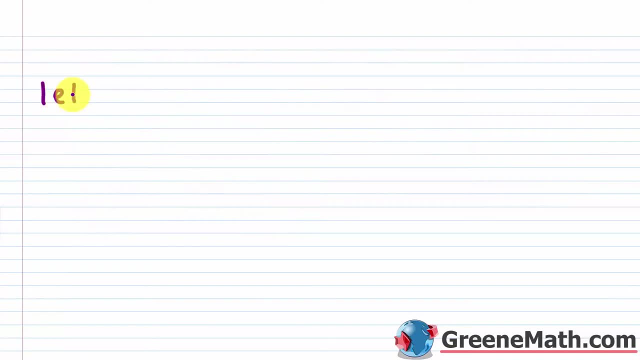 So, in other words, if I let x be equal to the number of $20 bills, then, because again there's only 80 bills in the bag, it has to be true that we could say 80, the total number of bills minus x the number of $20 bills. 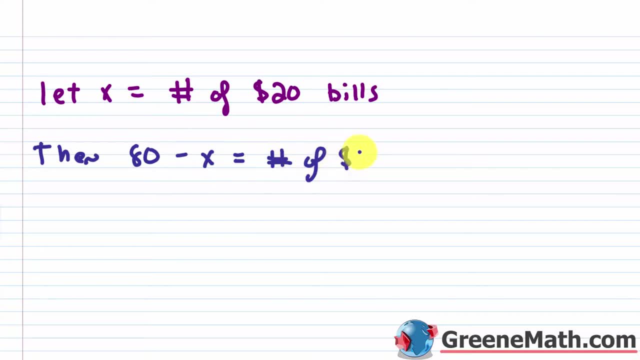 has to be equal to 80.. It has to be equal to the number of $100 bills. okay, Let me make this a little bit better. Okay, so now that we have both of our unknowns kind of modeled, let's think about how we can get an equation going. 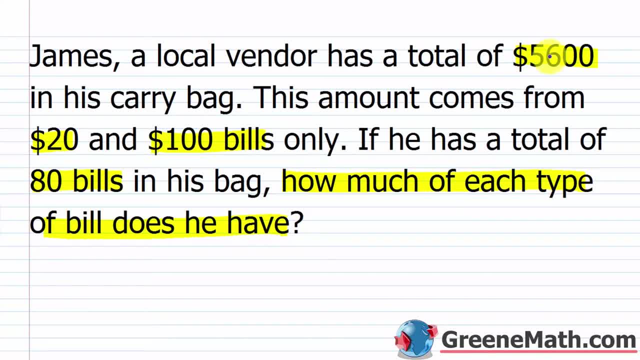 So again, just like with the last problem, we're given a value, okay, But we've modeled things as kind of an amount of bills that we have. So we have to again go through, set up a little table and relate the values. 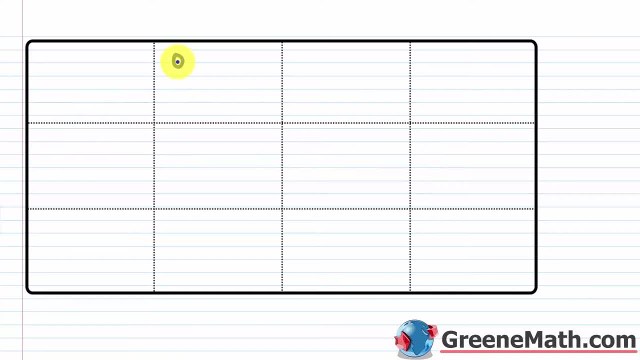 So let's go down here And again, I'm going to say I have quantity of bills, I'm going to say value per bill And I'm going to say total value. Again, if I take the quantity of bills times the value per bill, I will get the total value. 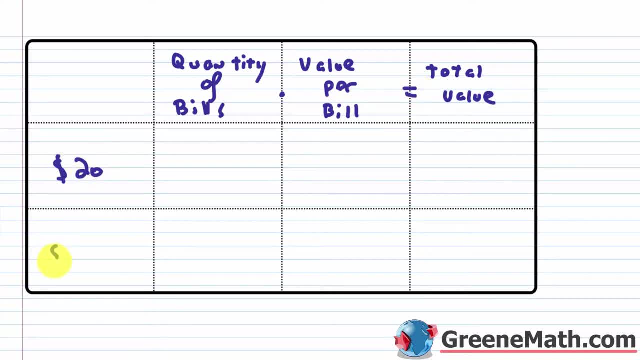 So here I'm going to have my $20 bills And here I'm going to have my $100 bills. So we said that the quantity of bills for 20s, we represented that with x, And the quantity of bills for 100s, we represented that with 80 minus x. 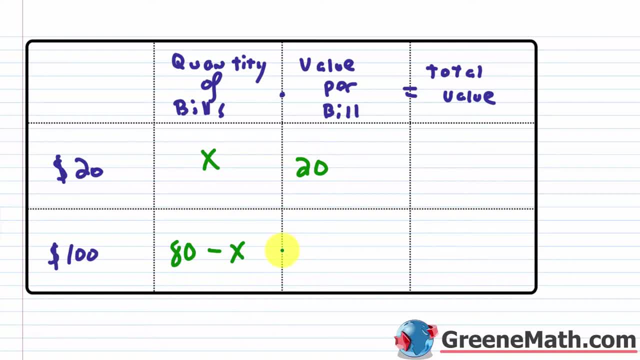 Now the value per bill for 20 we know is 20.. We know the value per bill for 100 is 100. And we just multiply across So to get the total value for the $20 bills it would be x times 20, or 20x. 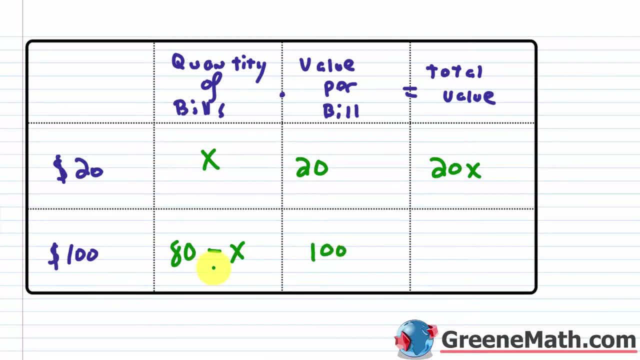 To get the total value for the $100 bills, it would be 100 times 80 minus x, So 100 times the quantity. Remember you're multiplying by the whole thing: 80 minus x. Okay, So now we have the total value of the 20s and the total value of the 100s. 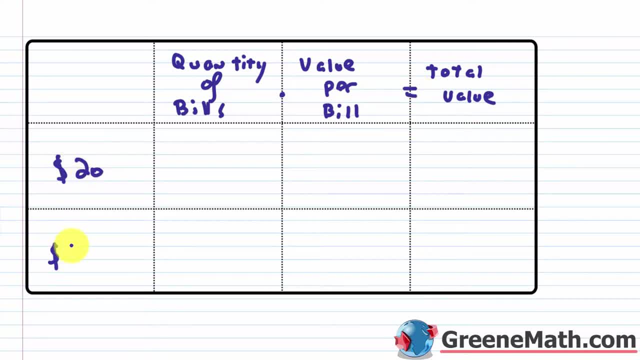 So here I'm going to have my $20 bills and here I'm gonna have my $100 bills. So we said that the quantity of bills for 20s- we represented that with x- and the quantity of bills for 100s. 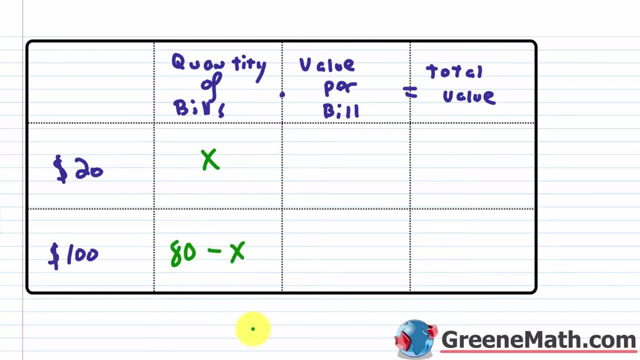 we represented that with 80 minus x. Now the value per bill for 20 we know is 20.. We know the value per bill for 100 is 100. We just multiply across So to get the total value for the $20 bills. 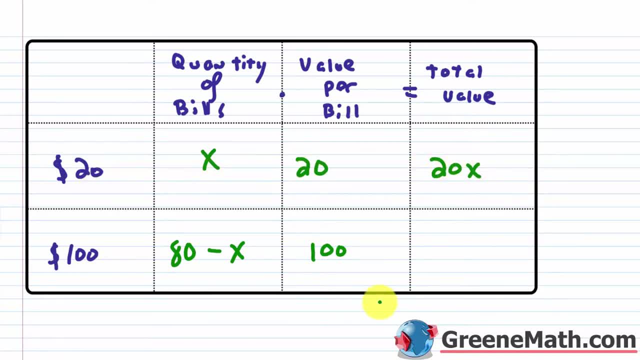 it would be x times 20 or 20x To get the total value for the $100 bills. it would be 100 times 80 minus x, So 100 times the quantity. remember you're multiplying by the whole thing: 80 minus x. 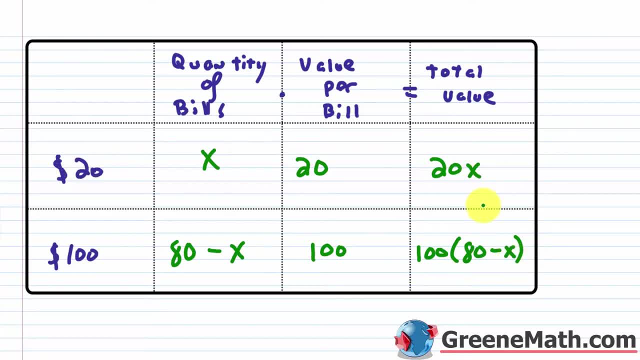 Okay, so now we have the total value of the 20s and the total value of the 100s and we can sum those amounts and set it equal to the total amount that he has, which is $5,600.. So, in other words, I would have 20x. 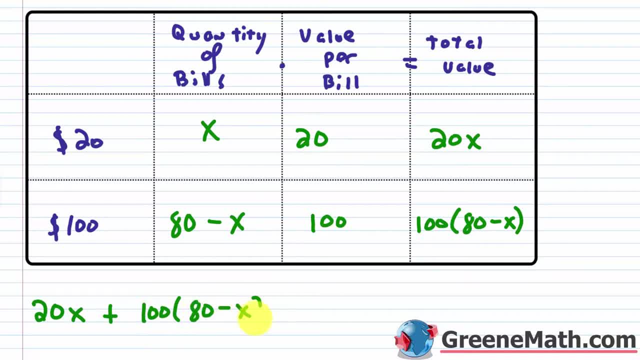 plus 100 times the quantity 80 minus x, And again this is set equal to the total value of his carryback, Which is $5,600.. So let's copy this and go to a fresh sheet. So on the left I have my 20x. 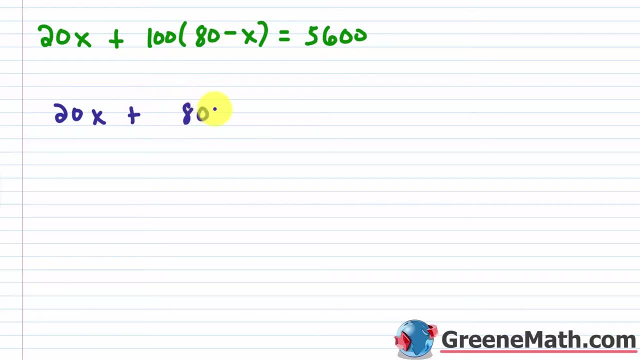 And then plus, you've got 100 times 80,, which is gonna be 8,000.. Then minus 100 times x is 100x, And this equals 5,600.. So 20x minus 100x is negative 80x. 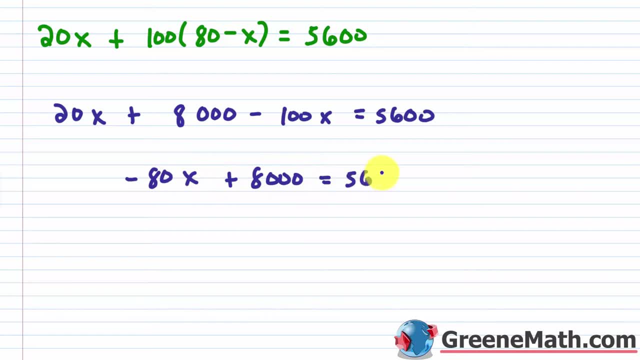 Then again you have plus 8,000.. This equals 5,600.. And now I'm gonna subtract it. I'm gonna subtract 8,000 away from each side of the equation, So I'm gonna have negative. 80x is equal to. 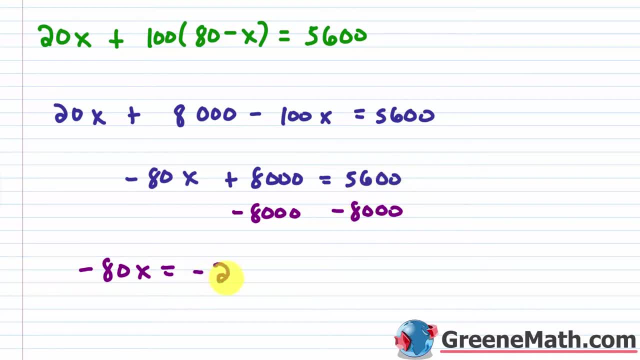 if I have 5,600 minus 8,000, that's gonna be negative 2,400.. To get x by itself, I'm gonna divide both sides of the equation by negative 80. So we know these cancel and you're gonna get that x is equal to 30.. 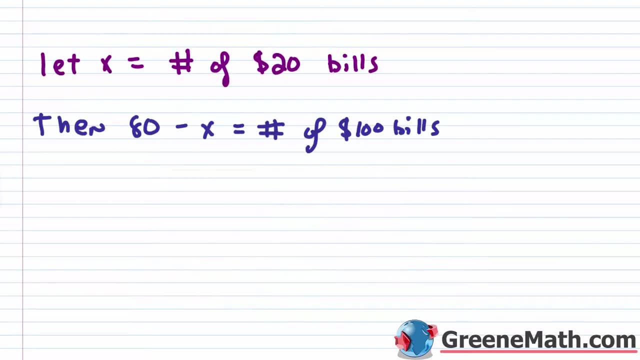 Okay, so let's take this result here back up Again. we said x was the number of $20 bills, so this is gonna be 30.. We said 80 minus x, or 80 minus 30, or 50,. 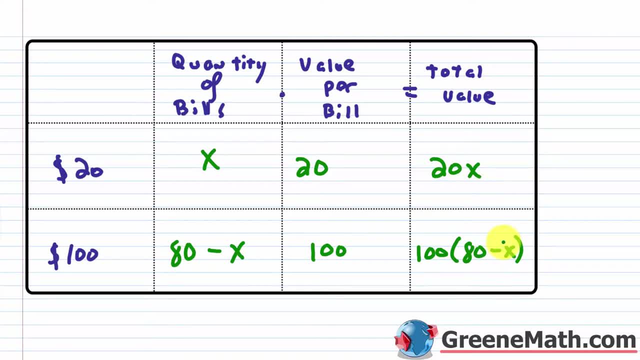 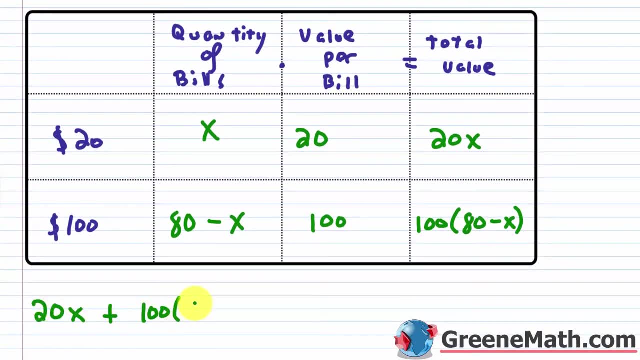 And we can sum those amounts and set it equal to the total amount that he has, which is $5,600.. So in other words, I would have 20x plus 100 times the quantity 80 minus x And again this is set equal to the total value of his carry bag, which is $5,600. 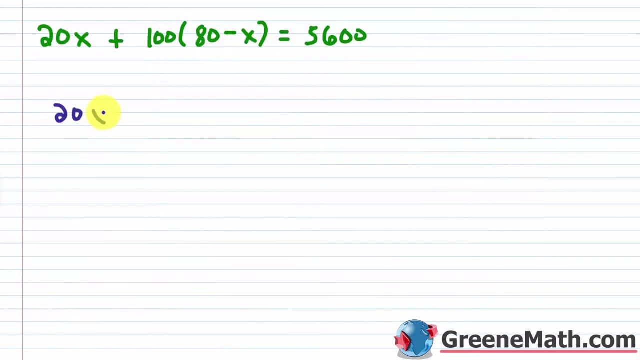 So let's copy this and go to a fresh sheet. So on the left I have my 20x, And then plus you've got 100 times 80, which is going to be 8,000.. Then minus 100 times x is 100x. 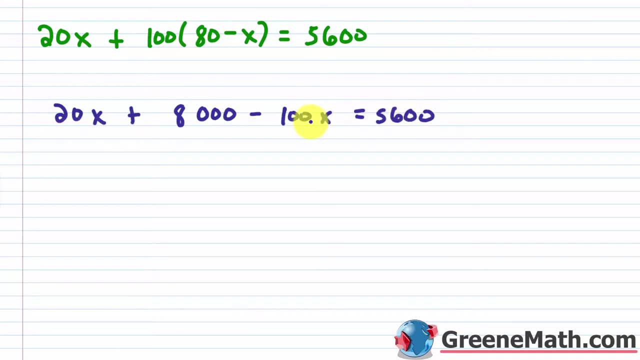 And this equals 5,600.. So 20x minus 100x is negative 80x, And then again you have plus 8,000. This equals 5,600.. And now I'm going to subtract 8,000 away from each side of the equation. 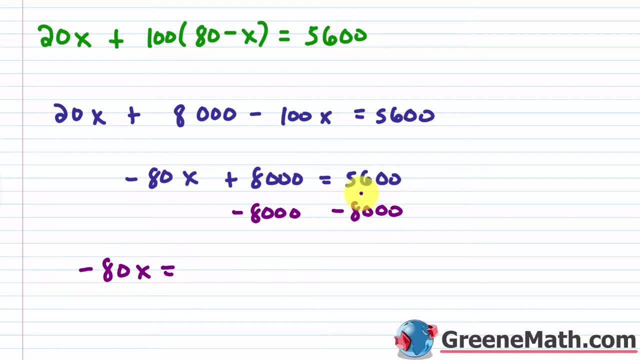 So I'm going to have negative 80x is equal to: If I have 5,600 minus 8,000, that's going to be negative 2,400.. To get x by itself, I'm going to divide both sides of the equation by negative 80.. 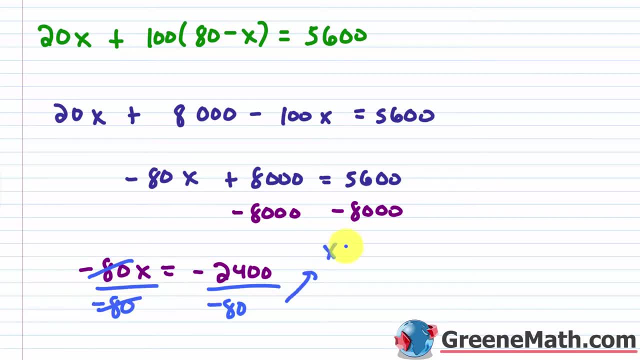 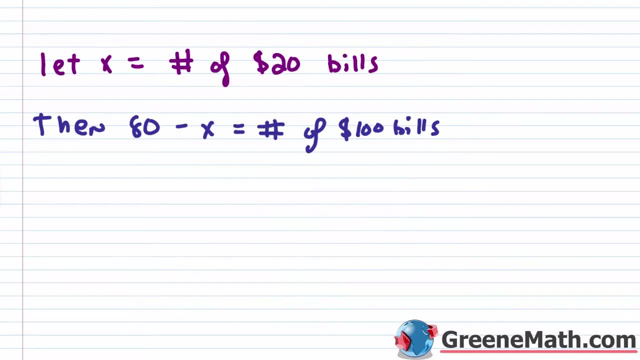 So we know these cancel. You're going to get that x is equal to 30.. Okay, So let's take this result here. back up Again. we said x is the number of $20 bills, So this is going to be 30.. 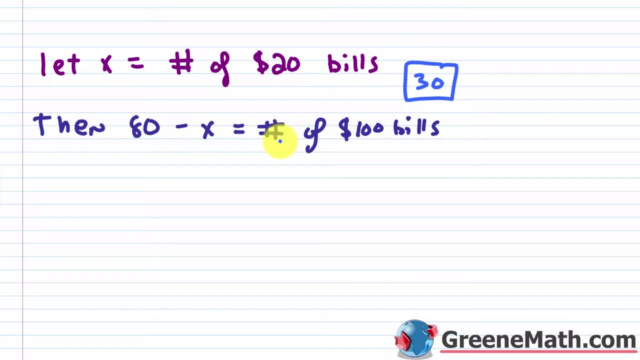 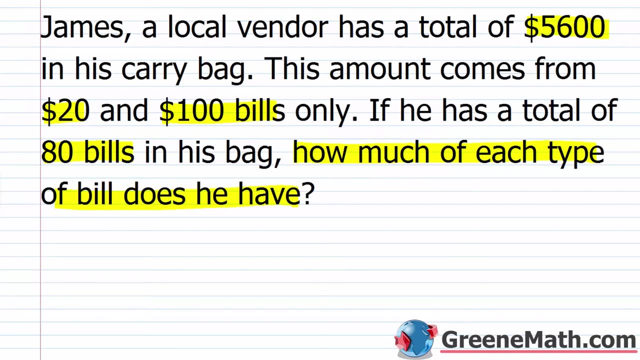 We said 80 minus x or 80 minus 30 or 50 is the number of $100 bills. Okay, so we have our solution. Let's go back up And now let's answer this guy So we can say: there are. 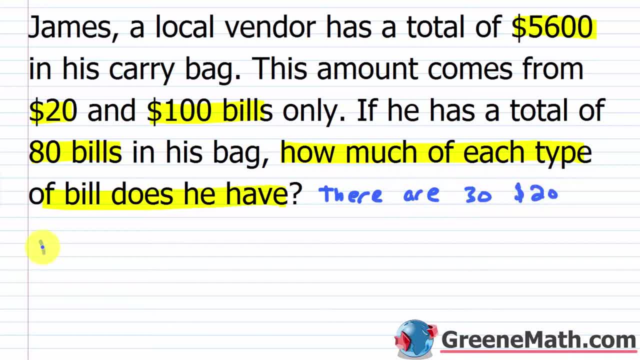 Again, 30 $20 bills And 50 $100 bills. To check this is very easy. You'd want to make sure the value works out. So 30 times 20 is 600.. So the value from the 20s is 600. 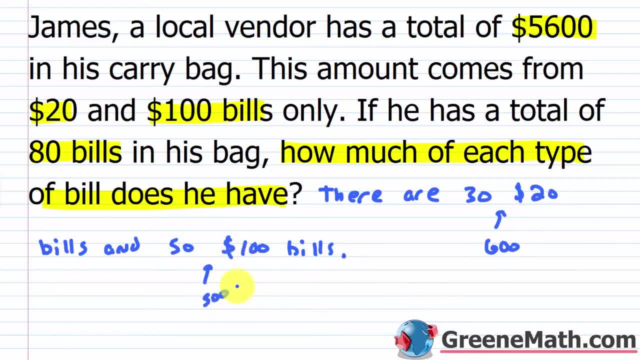 And then 50 times 100 is 5,000.. Okay, so the value from the $100 bills is 5,000.. 5,000 plus 600 is 5,600.. So you're good to go there. Now. the next thing you want to check is: does the amount of bills from the 20s plus the amount of bills from the 100s give me 80 bills, which is what's in his back? 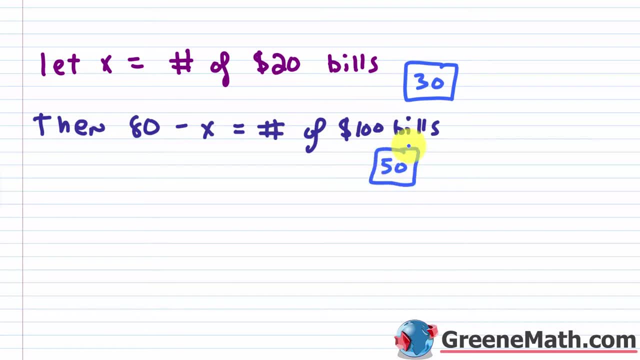 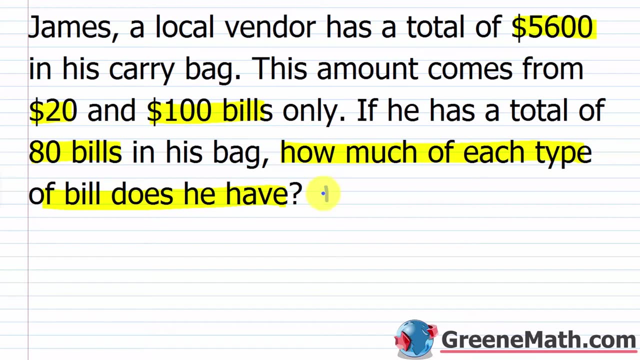 is the number of $100 bills. Okay, so we have our solution. Let's go back up and now let's answer this guy, So we can say there are again 30 $20 bills and 50 $100 bills. 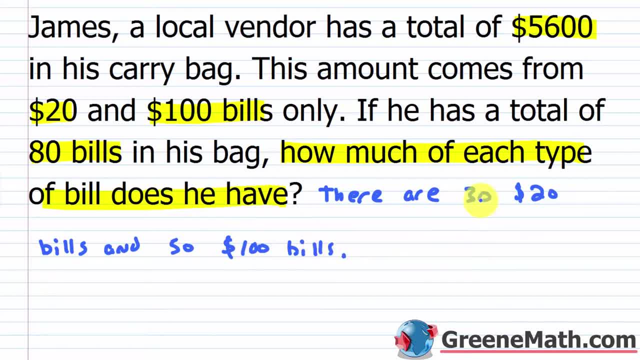 To check. this is very easy. You wanna make sure the value works out. So 30 times 20 is 600, so the value from the 20s is 600, and then 50 times 100 is 5,000.. 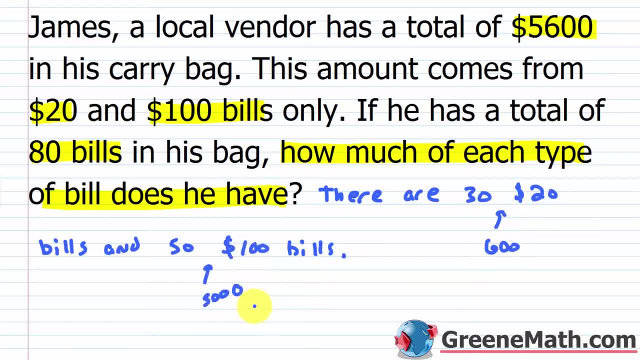 Okay, so the value from the $100 bills is 5,000.. 5,000 is plus 600 is 5,600, so you're good to go there. Now. the next thing you wanna check is: does the amount of bills from the 20s? 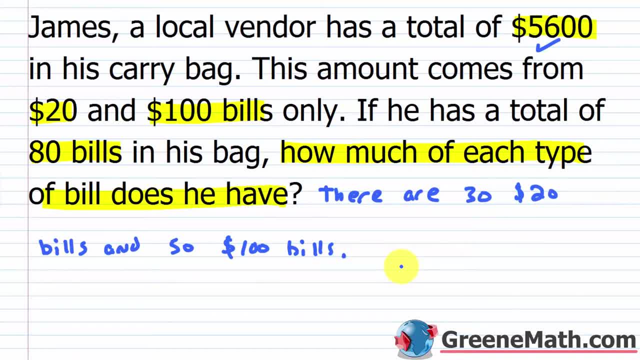 plus the amount of bills from the 100s and 600 fit in this equation, give me 80 bills, which is what's in his bag. So there's 30, 20s and 50 100s. 30 plus 50 is 80. So 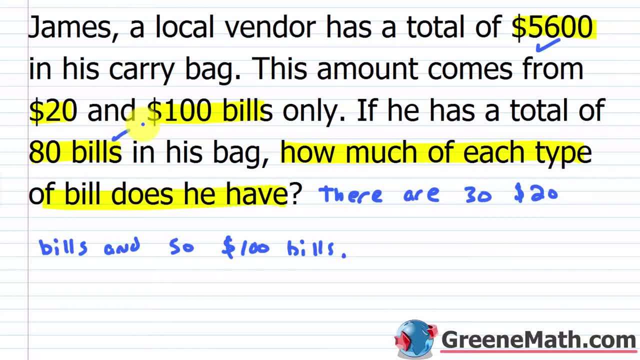 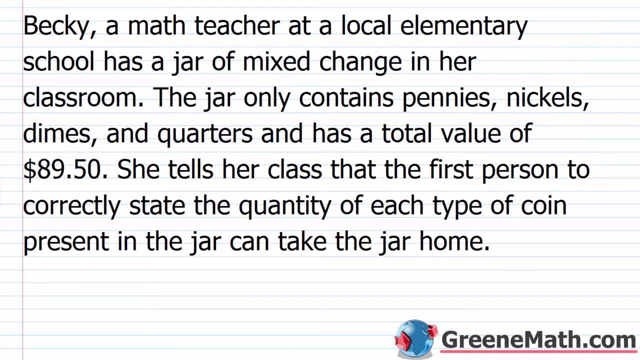 you're good to go there as well. So, again, our answer is that there are 30 $20 bills and 50 $100 bills. All right, let's take a look at one more problem, And this is one that's going to be a. 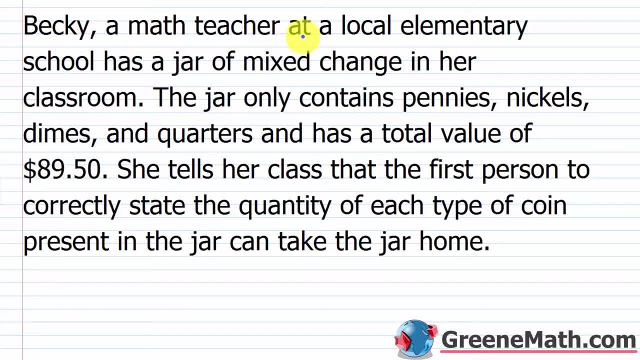 little bit tedious. So we have Becky. a math teacher at a local elementary school has a jar of mixed change in her classroom. The jar only contains pennies, nickels, dimes and quarters and has a total value of $89.50.. She tells her class that the first person to correctly state 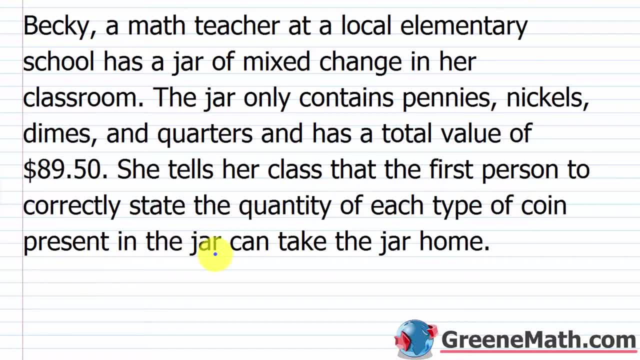 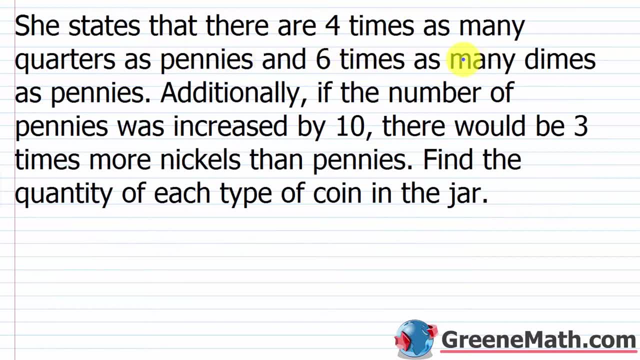 the quantity of each type of coin present in the jar, can take the jar home. Now she states that there are four times as many quarters as pennies and six times as many dimes as pennies. Additionally, if the number of pennies was increased by 10, there would be three times more. 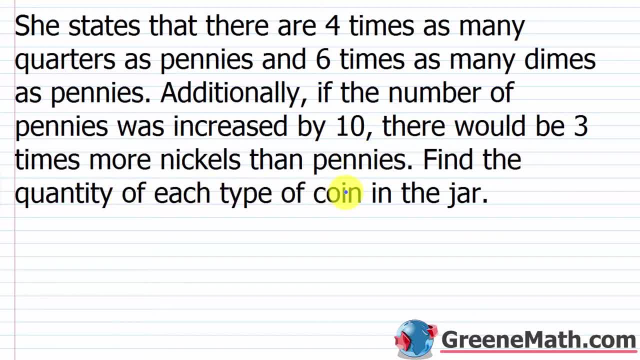 nickels than pennies. Find the quantity of each type of coin in the jar. So this one is tedious because you have four coins involved. You have pennies, nickels, dimes and quarters. So that's the unknown. here, Again, we're trying to find the quantity of each type of coin in the jar. So how? 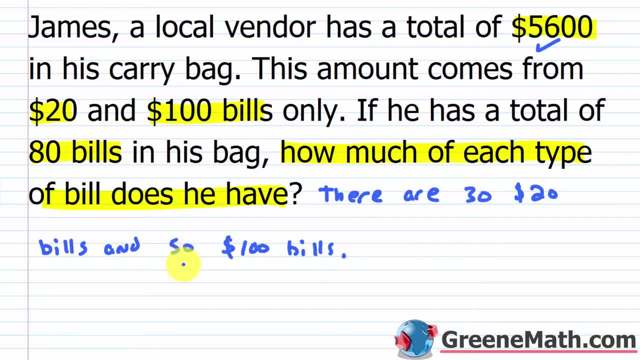 So there's 30 20s and 50 100s. 30 plus 50 is 80.. So you're good to go there as well. So again, our answer is that there are 30 $20 bills and 50 $100 bills. 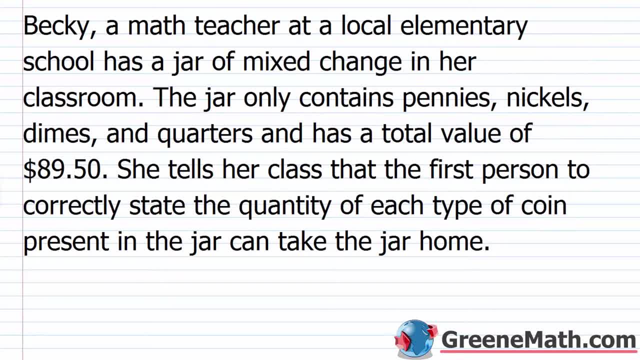 All right, let's take a look at one more problem, And this is one that's going to be a little bit tedious. So we have Becky. She's a math teacher at a local elementary school, has a jar of mixed change in her classroom. 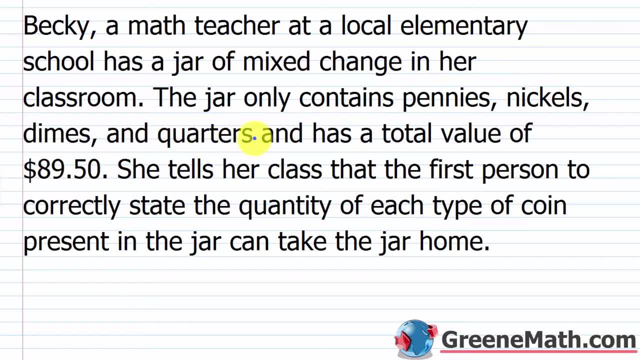 The jar only contains pennies, nickels, dimes and quarters and has a total value of $89.50.. She tells her class that the first person to correctly state the quantity of each type of coin present in the jar can take the jar home. 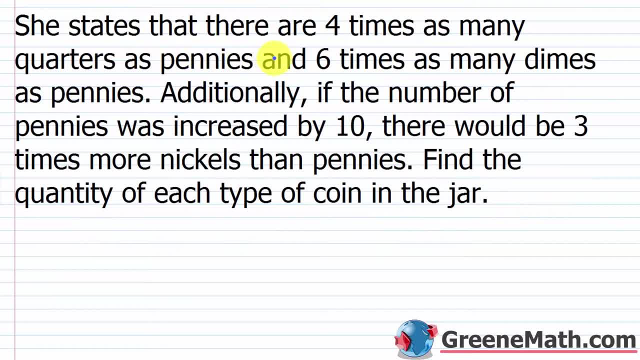 Now she states that there are four times as many quarters as pennies and six times as many dimes as pennies. Additionally, if the number of pennies was increased by 10, there would be three times more nickels than pennies. 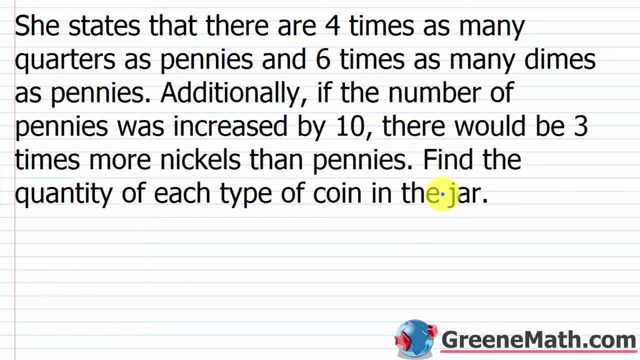 Find the quantity of each type of coin in the jar. So this one is tedious because you have four coins involved. You have pennies, nickels, dimes and quarters. So that's the unknown. here Again, we're trying to find the quantity of each type of coin in the jar. 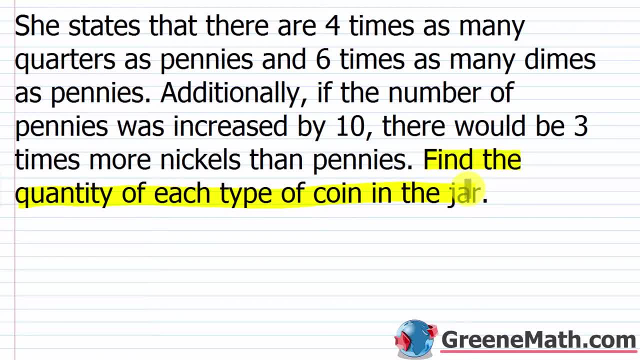 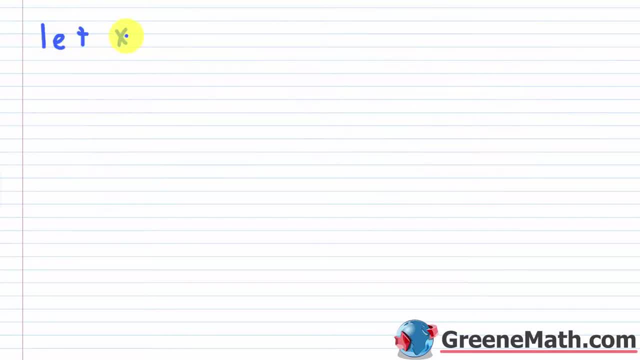 So how many pennies, how many nickels, how many dimes, how many quarters? So let's start out by just modeling our unknowns. So let X be equal to the number of pennies. We're going to do that because it's involved in all the comparisons. 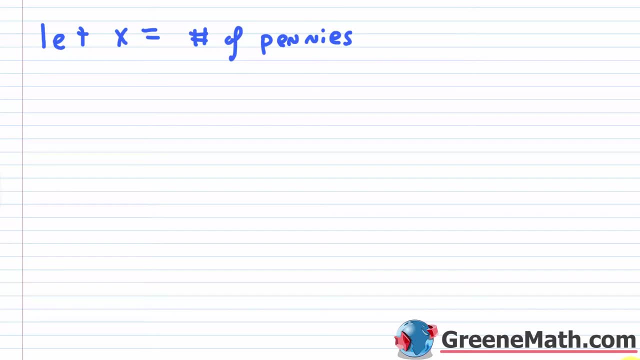 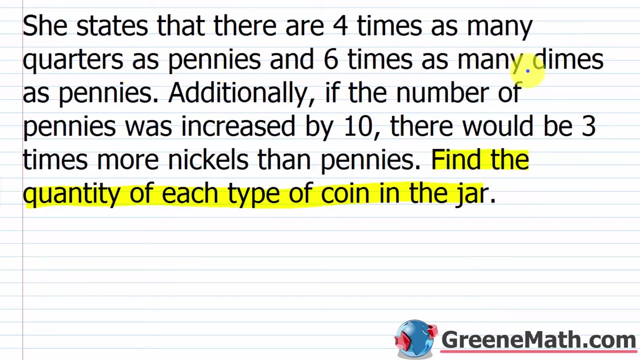 So it's just easier if you do that. So what can we say about the number of nickels, the number of quarters and the number of dimes? So it tells us, to start, that there are four times as many quarters as pennies and six times as many dimes as pennies. 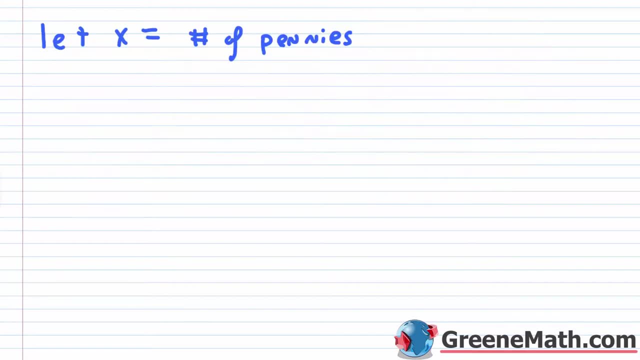 So if there's four times as many quarters as pennies, that means we could say then four X or four times the number of pennies, which is X is equal to the number of quarters. Then we can also say again, since it told us that there are six times as many dimes as pennies: 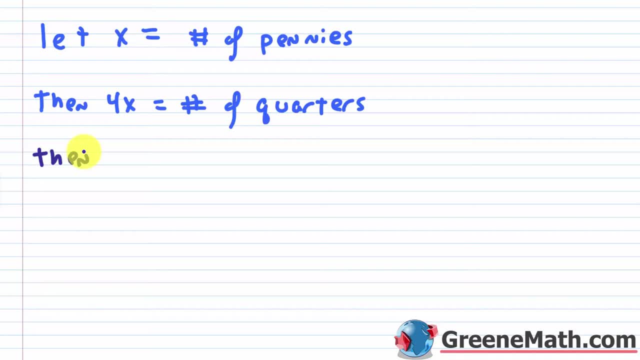 well, if there's X number of pennies, six times that amount would be six X. So that's going to be my number of dimes. So six X is equal to the number of dimes. Okay, so what can we say about the nickels? 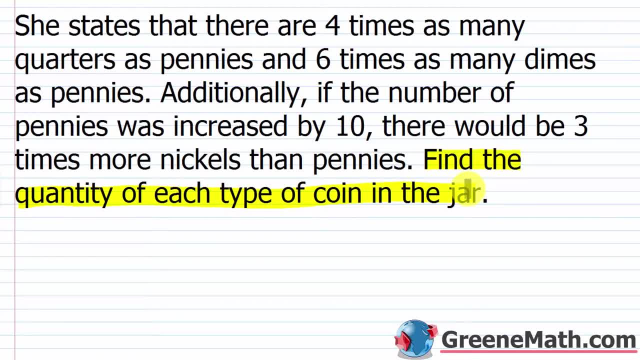 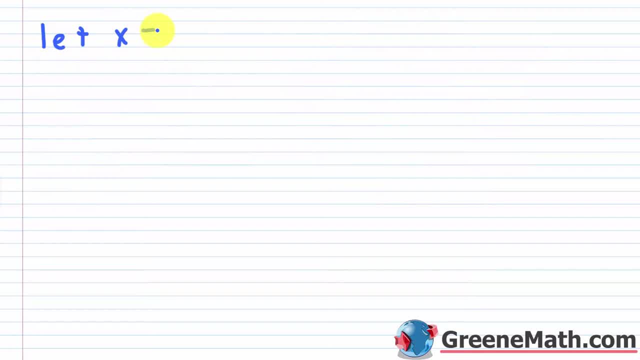 many pennies, how many nickels, how many dimes, how many quarters? So let's start out by just modeling our unknowns. So let's let x be equal to the number of pennies, And we're going to do that because it's involved in all the comparisons. So it's just 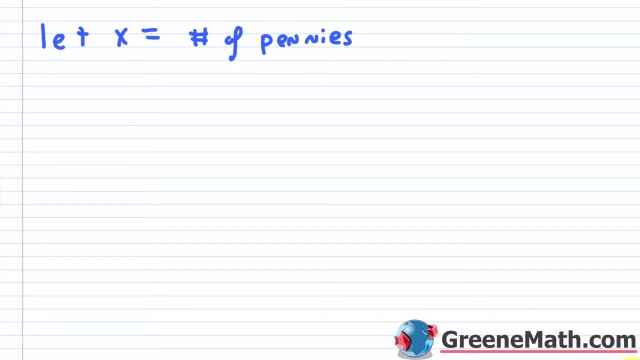 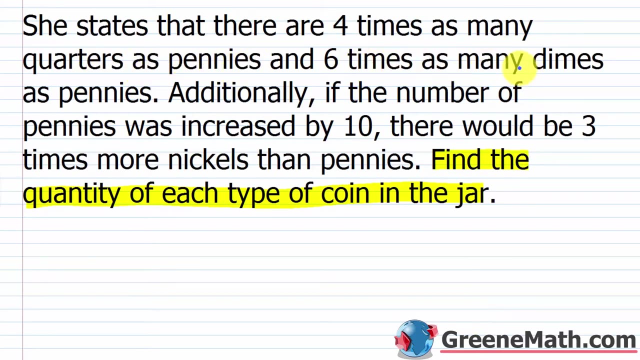 easier if you do that. So what can we say about the number of nickels, the number of quarters and the number of dimes? So it tells us, to start, that there are four times as many quarters as pennies and six times as many dimes as pennies. So if there's four times as many quarters as 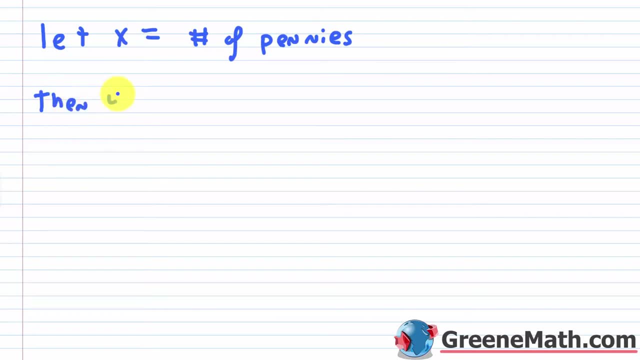 pennies. that means we could say then 4x, or four times the number of pennies, which is x is equal to the number of quarters. Then we can also say again, since it told us that there are six times as many dimes as pennies, well, if there's x number of pennies, six times that amount would be. 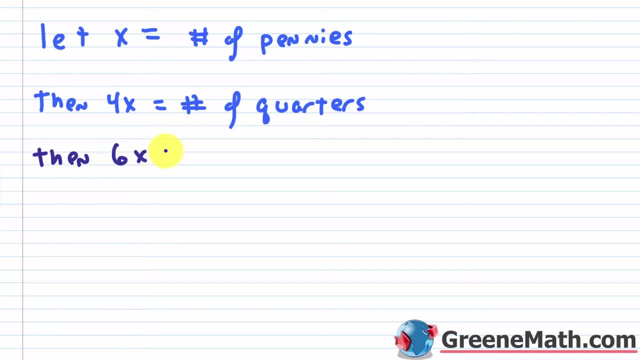 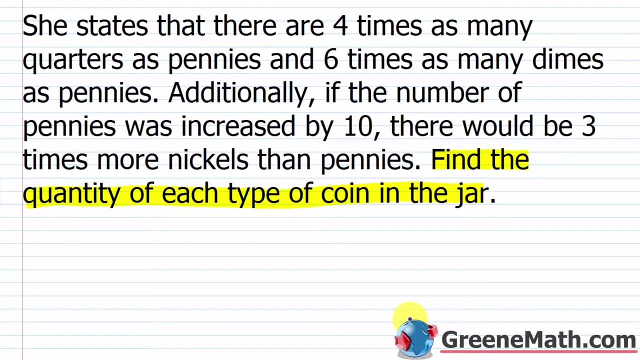 6x. So that's going to be my number of dimes. So 6x is equal to the number of dimes. Okay, so what can we say about the nickels? So what can we say about the nickels? So then it tells us if the number of pennies was increased. 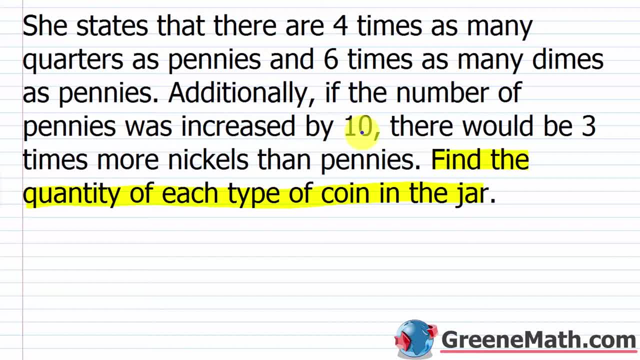 by 10.. So I have x number of pennies. If I increased it by 10, that would be x plus 10. There would be three times more nickels than pennies. So in other words, if I increase the number of pennies by 10, again, if I take x the number of pennies, I add 10 to it, If I multiply. 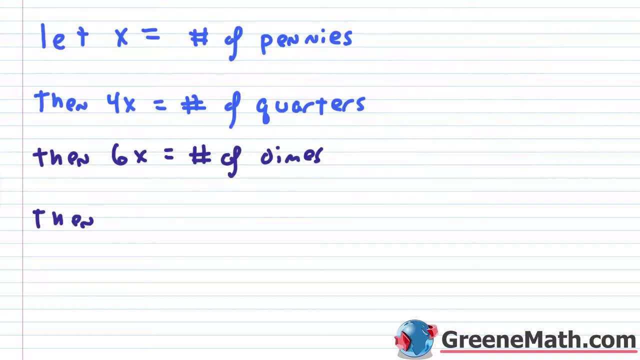 that amount by three, that's how many nickels I would have. Again, if I multiply three times the quantity x plus 10, this would be equal to the number of nickels. Okay, so now that we have everything modeled again, we're told the total value of: 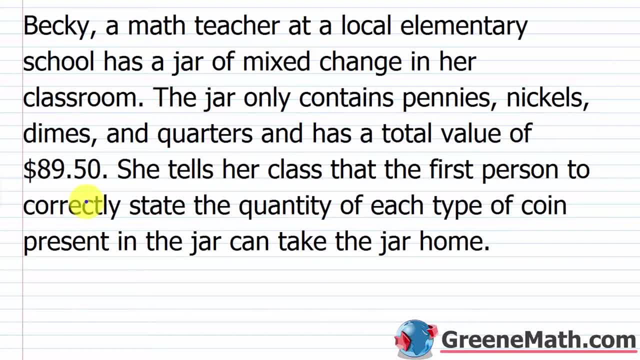 all the coins in our jar At the start of the problem. that's going to be $89.50.. So again we got to think about the value of each coin. We're going to sum the values of all the coins and that should be equal to $89.50.. So let's use a little table. 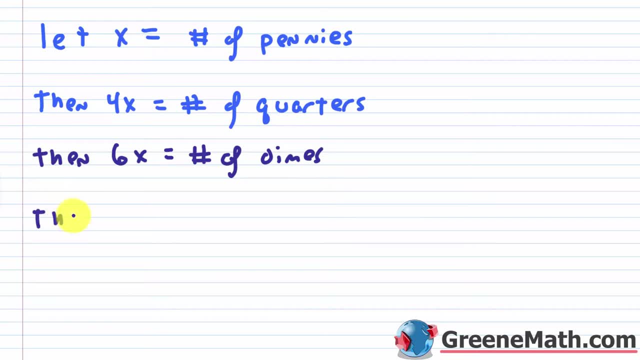 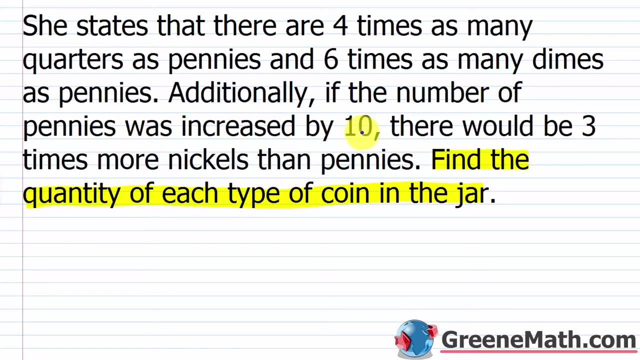 So what can we say about the nickels? So then it tells us if the number of pennies was increased by 10, so I have X number of pennies. if I increased it by 10, that would be X plus 10,. 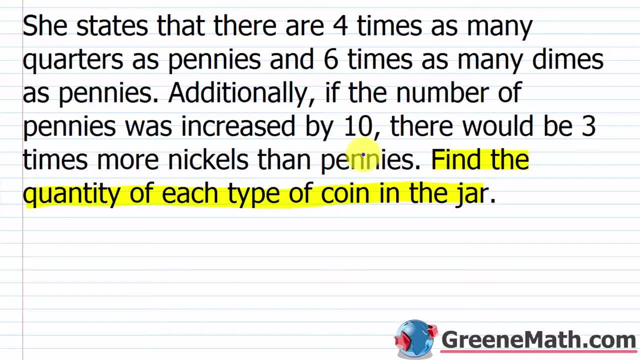 there would be three times more nickels than pennies. So in other words, if I increase the number of pennies by 10, again if I take X the number of pennies, I add 10 to it. if I multiply that amount by 3, that's how many nickels I would have. 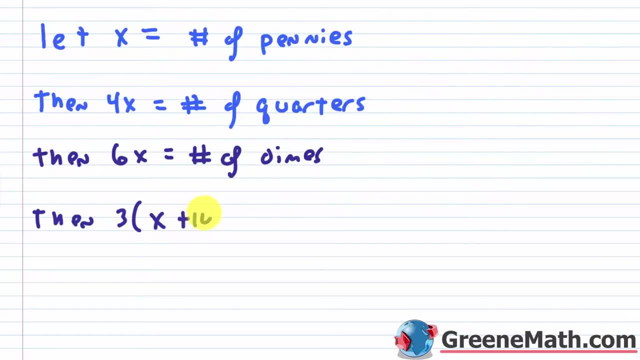 So again, if I multiply 3 times the quantity X plus 10,, this would be equal to the number of nickels. Okay, so now that we have everything modeled again, we're told the total value of all the coins in our jar. 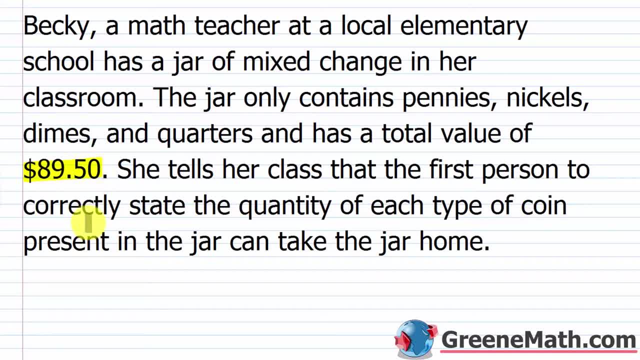 At the start of the problem. that's going to be $89.50.. So again we got to think about the value of each coin. We're going to sum the values of all the coins And that should be equal to $89.50. 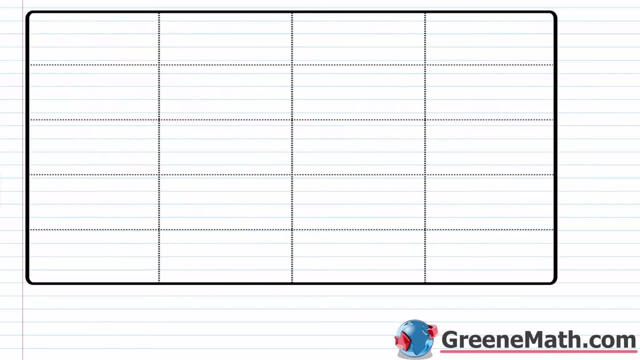 So let's use a little table, Alright? so let's set this up in the normal way, So we have our quantity of coins And then we have our value per coin, And then we have our total value. Okay, let me make that better. 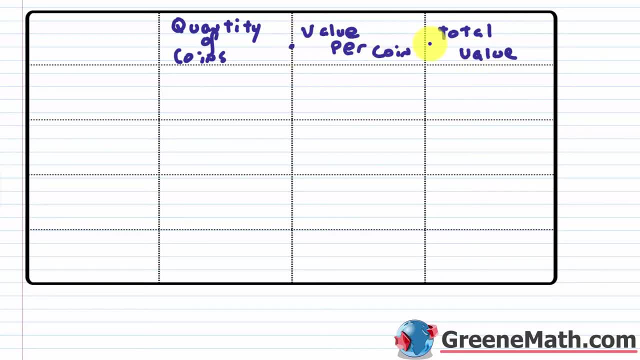 And again, if I multiply the quantity of coins by the value per coin, I'm going to get the total value for that set of coins. So again, I have pennies which I'm just going to put a P for, or you could put 0.01.. 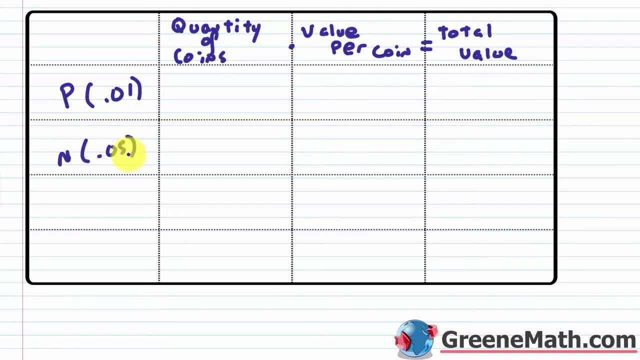 I have nickels which I'm going to put an N and I'll just put 0.05.. I have dimes which I'll put a D for And then 0.1 or 0.10.. I don't know if you want that. 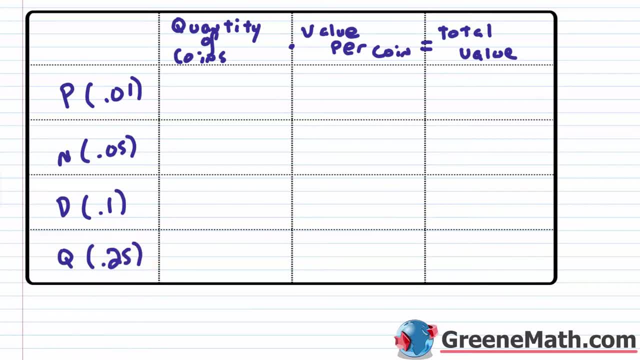 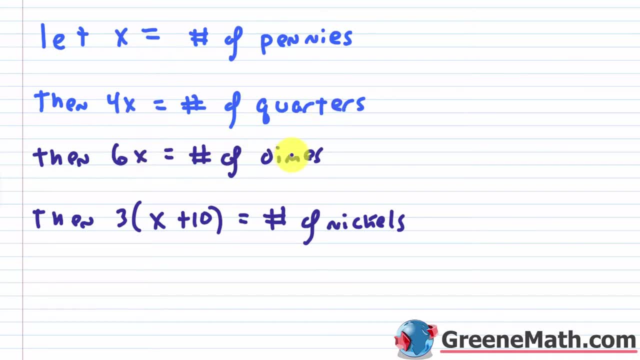 And then I have quarters, which I'll put a Q for, And this is 0.25.. So quantity of coins: If we go back up again, X is the number of pennies, 4X is the number of quarters, 6X is the number of dimes and 3 times the quantity X plus 10 is the number of nickels. 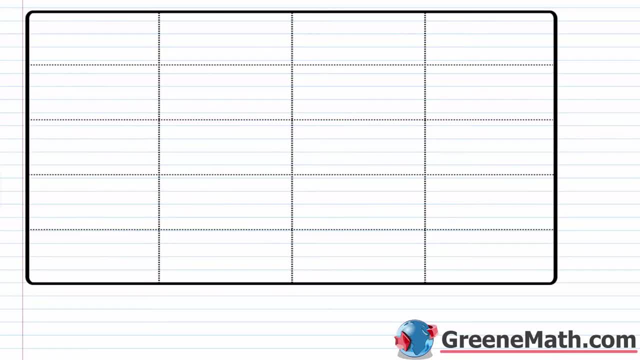 All right. so let's set this up in the normal way. So we have our quantity of coins And then we have our value per coin, And then we have our total value. Okay, let me make that better. And again, if I multiply the quantity of coins by the value per, 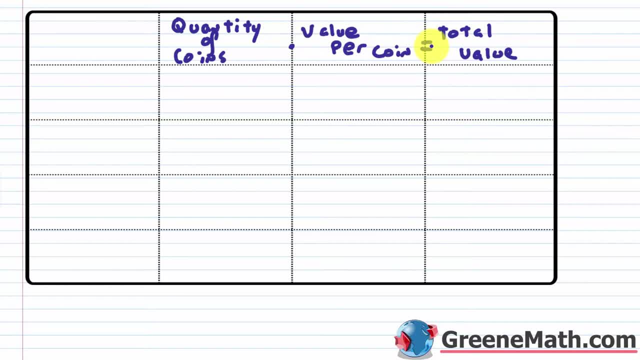 coin, I'm going to get the total value for that set of coins. So again, I have pennies which I'm just going to put a P for where you could put 0.01.. I have nickels which I'm going to put an. 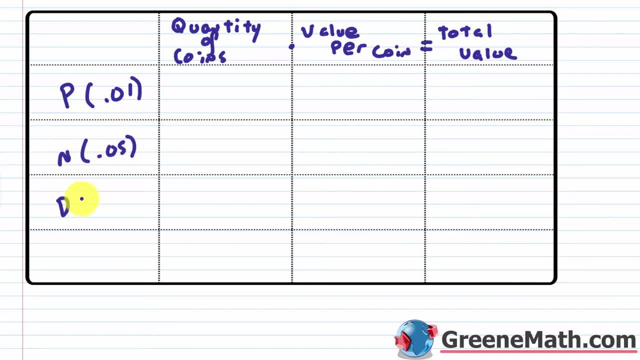 N and I'll just put 0.05.. I have dimes which I'll put a D for, and then 0.1 or 0.10, if you want that, And then I have quarters, which I'll put a Q for, and this is 0.25.. 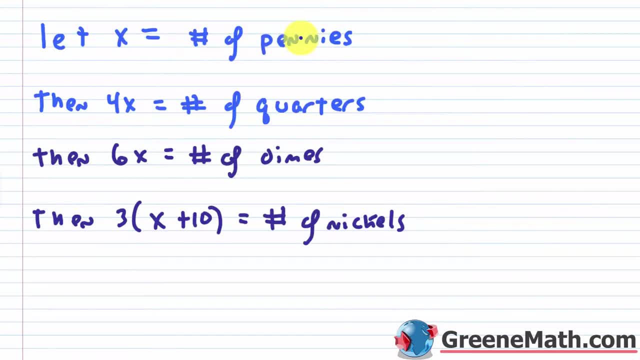 So quantity of coins, If we go back up again, X is the number of pennies, 4X is the number of quarters, 6X is the number of dimes and 3 times the quantity X plus 10 is the number of nickels. 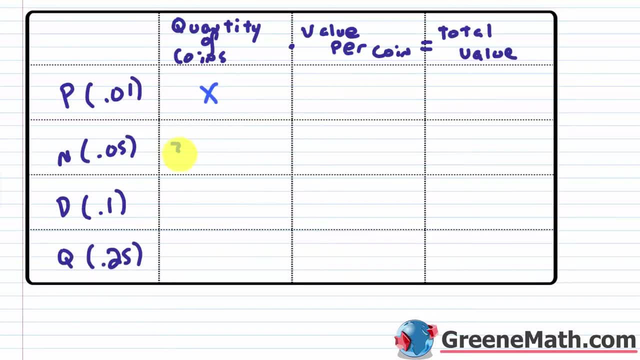 So for pennies this was X. For nickels this was 3 times the quantity X plus 10.. For dimes this was 6X And for quarters this was 4X. Now the value per coin is pretty simple: For pennies it's 0.01.. For nickels it's 0.05.. 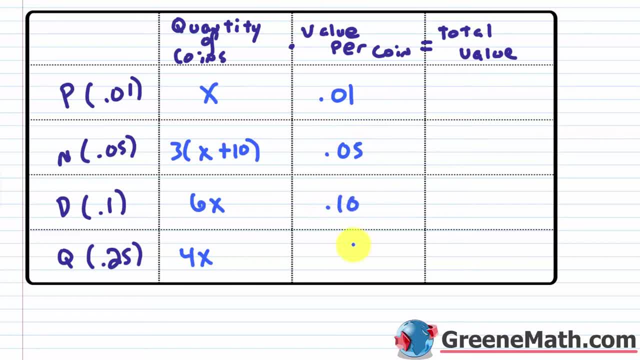 For dimes it's 0.15.. For quarters it's 0.25.. So again the total value I just multiply across. So for pennies it's X times 0.01 or 0.01X. For nickels it's 0.05 times 3, which is 0.15,. 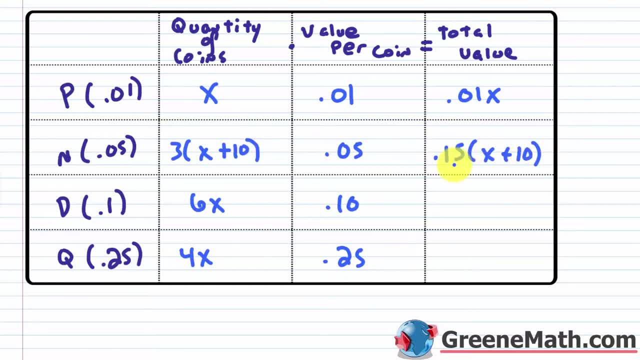 then times the quantity X plus 10.. Now you can simplify this here, or you can wait till later. Let's just simplify it here: 0.15 times X is 0.15X, and then 0.15 times 10,. 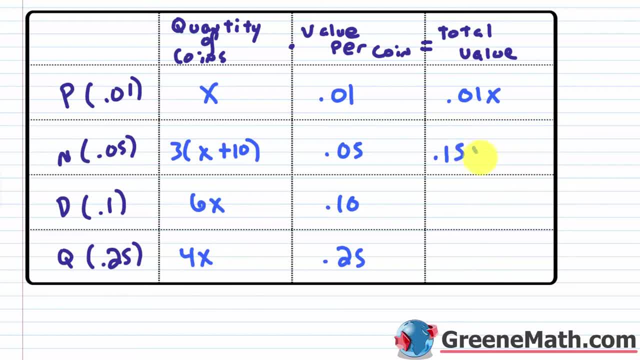 is 1.5.. So let's put 0.15X plus 1.5.. And then for dimes it's 6X times 0.1. So that's 0.6X. And then for quarters it's 4X times 0.25, which is 1X or just X. Okay, So if we sum these total, 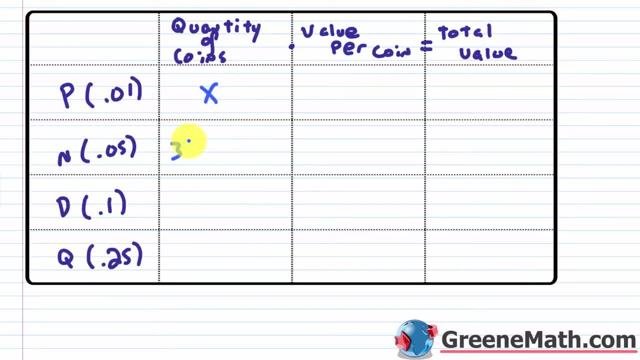 So for pennies this was X, For nickels this was 3 times the quantity X plus 10.. For dimes this was 6X And for quarters this was 4X. Now the value per coin is pretty simple. 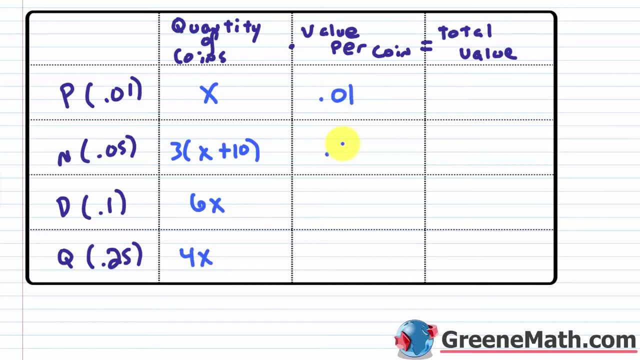 For pennies it's 0.01.. For nickels it's 0.05.. For dimes it's 0.1, or you can put 0.10, whatever you want to do. And then for quarters it's 0.25.. 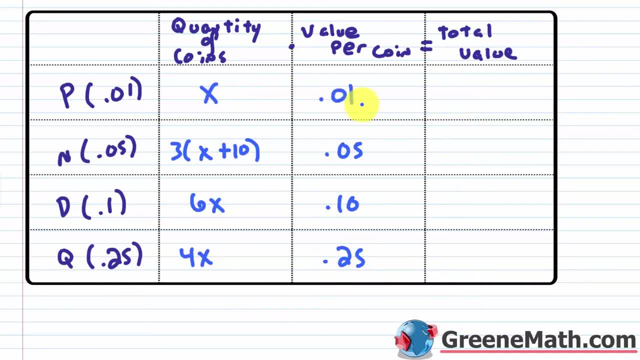 So again the total value I just multiply across. So for pennies it's X times 0.01 or 0.01X. For nickels it's 0.05 times 3, which is 0.15, then times the quantity X plus 10.. 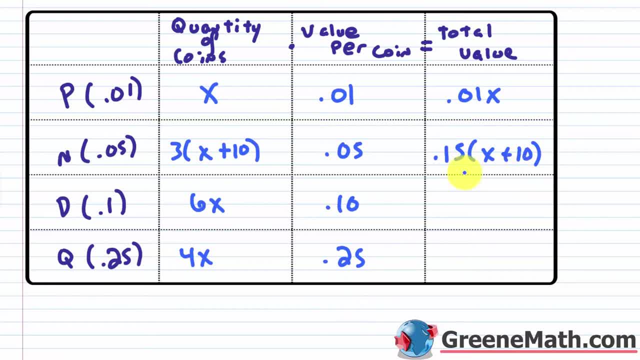 Now. you can simplify this here, or you can wait till later. Let's just simplify it here: 0.15 times X is 0.15X, and then 0.15 times 10 is 1.5.. So let's put 0.15X plus 1.5. 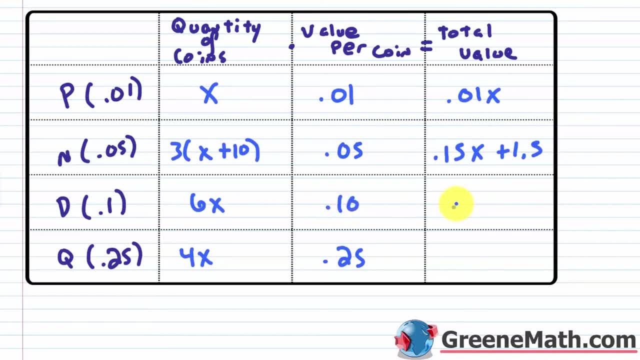 And then for dimes it's 6X times 0.1, so that's 0.6X. And then for quarters it's 4X times 0.25, which is 1X or just X. 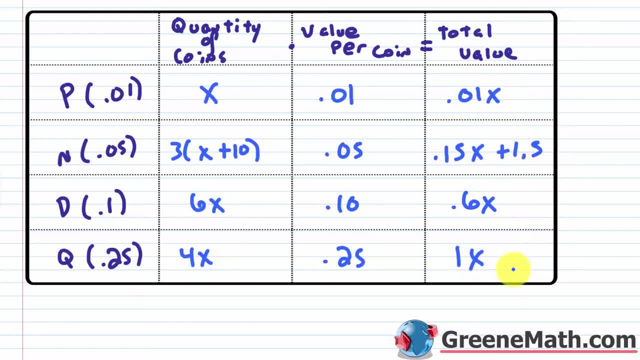 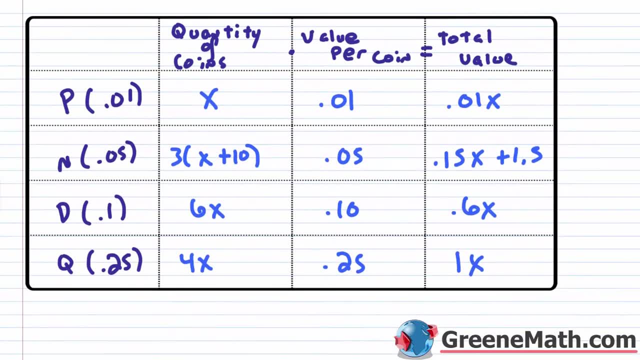 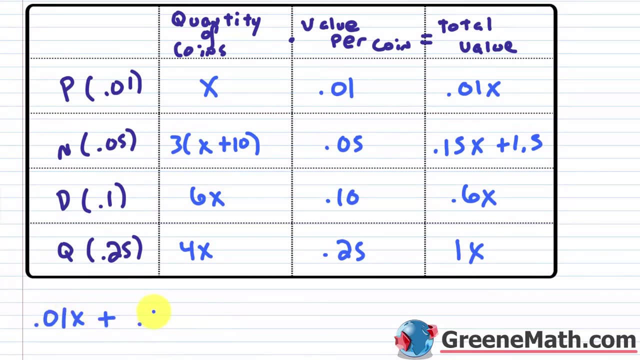 Okay. So if we sum these total values for each, then what we're going to get is a value that is equal to $89.50.. So, in other words, if I take 0.01X, the value of all pennies, and if I add it to 0.15X plus 1.5,. 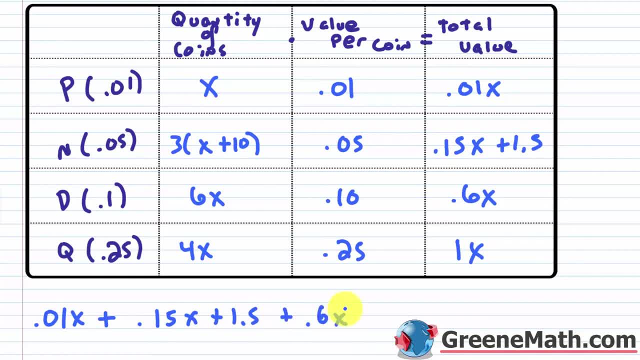 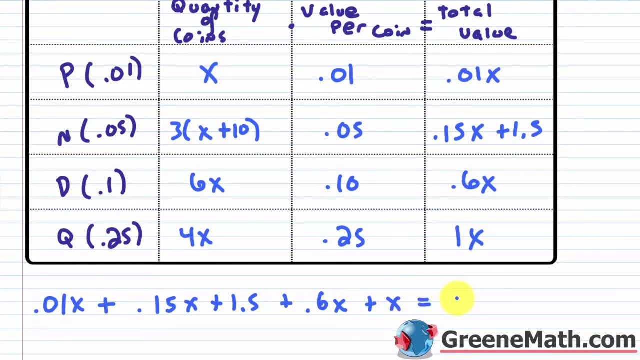 the value of all nickels, and I add it to 0.6X the value of all dimes, and I add it to 1X the value of all quarters. I'm just going to write X. This is equal to, again, the total value of the jar, which is $89.50.. 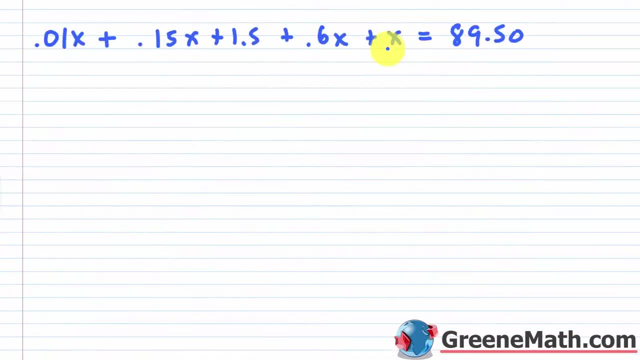 Okay, So let's copy this and go to a fresh sheet. So 0.01 plus 0.15 is 0.16.. If I add 0.6 to that, I get 0.76.. And then if I add another 1,- again, this is an implied coefficient of 1,- then I get 1.76.. 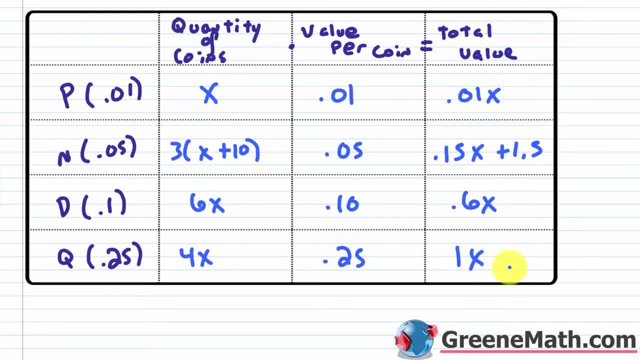 values for each, then what we're going to get is a value that is equal to $89.50.. So, in other words, if I take 0.15X plus 1.5X, then what we're going to get is a value that is equal to $89.50.. 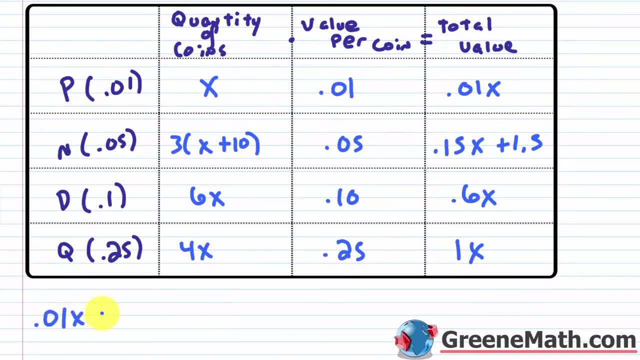 So if I take 0.01X, the value of all pennies, and if I add it to 0.15X plus 1.5,, the value of all nickels, and I add it to 0.6X, the value of all dimes, and I add it to 1X, the value of all, 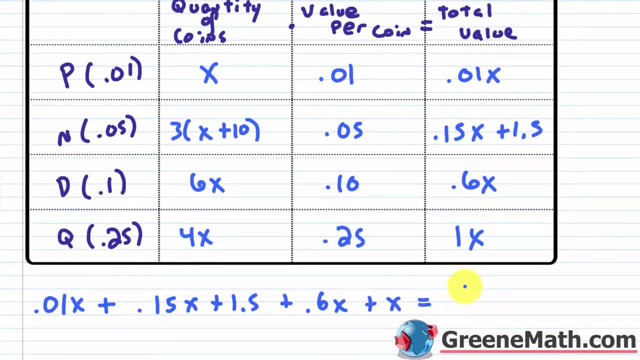 quarters. I'm just going to write X. this is equal to, again, the total value of the jar, which is $89.50.. Okay, So let's copy this and go to a fresh sheet. So 0.01 plus 0.15,. 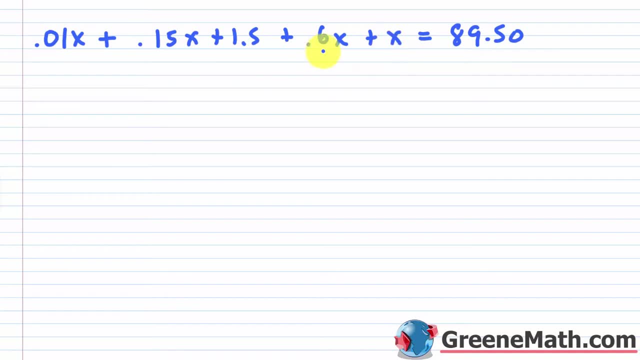 is 0.16.. If I add 0.6 to that, I get 0.76.. And then if I add another 1,- again, this is an implied coefficient of 1, then I get 1.76.. So the left side would be 1.76X. And then, don't forget, 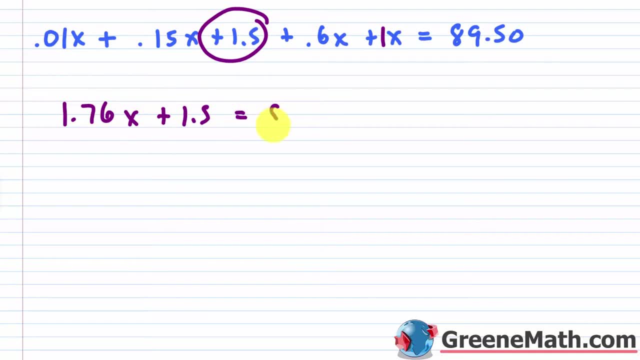 about this guy. So plus 1.5, this equals 89.50, or just 89.5, if you want. Now, if I subtract this 1.5 away from each side of the equation, this will cancel. Here you have: 1.76X is equal to 89.5. minus 1.5 is 88.. Now to get X by itself, I'm going to 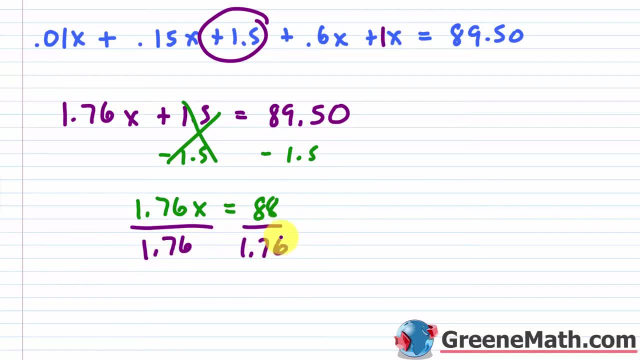 divide both sides by 1.76.. So we know that this is going to cancel and you'll have that X is equal to 88, divided by 1.76 is 50. So this is our answer here, But again we've got to go back and 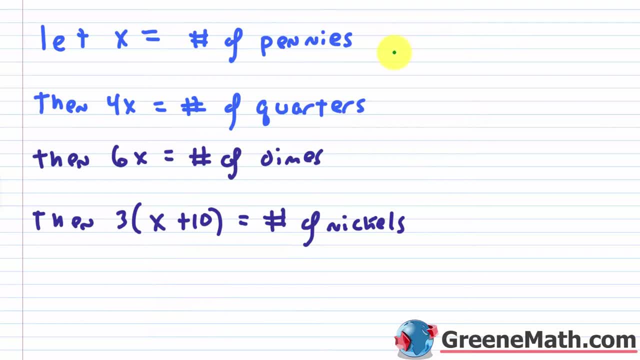 make sense of it. All right. So we know that X represents the number of pennies, And again we found that X was 50. So there are 50 pennies. Then 4 times X is the number of quarters. Again X is 50.. 4 times 50 is 200.. So there's going to be. 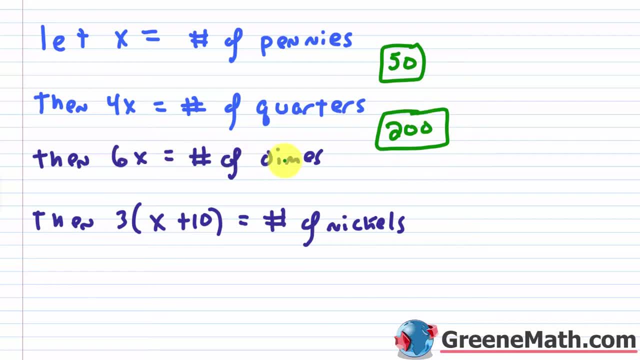 200 quarters. Then 6X is the number of dimes. Again X is 50.. 6 times 50 is 300. So there's 300 dimes. And then, lastly, 3 times the quantity X plus 10 is the number of nickels. So X again. 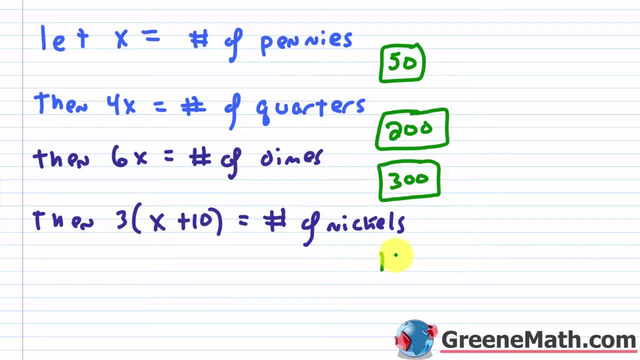 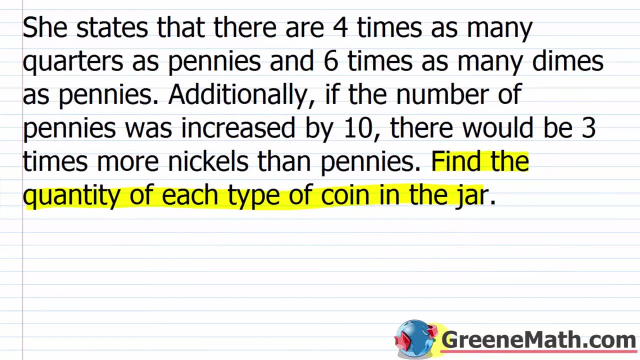 is 50.. 50 plus 10 is 60.. 60 times 3 is 180.. So there's 180 nickels. So let's go ahead and write our answer. So find the quantity of each type of coin in the jar. We can say that. 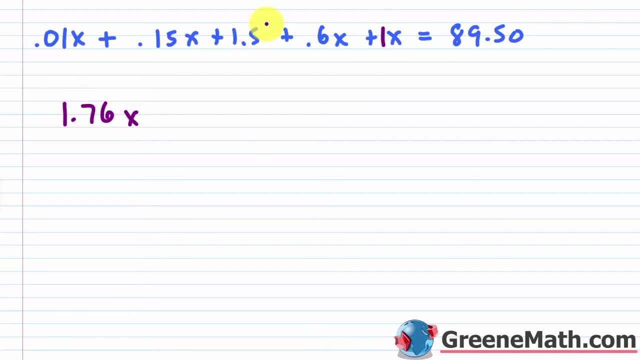 So the left side would be 1.76X, And then don't forget about this guy. So plus 1.5, this equals 89.50, which is 89.5, if you want. Now, if I subtract this 1.5 away from each side of the equation, this will cancel here. 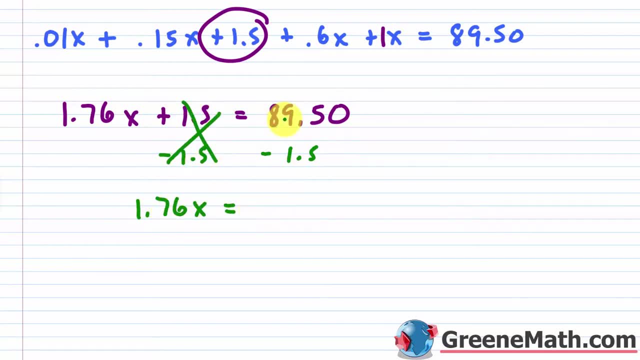 You have: 1.76X is equal to 89.5, minus 1.5 is 88.. Now to get X by itself, I'm going to divide both sides by 1.76.. So we know that this is going to cancel and you'll have that X is equal to 88. divided by 1.76 is 50.. 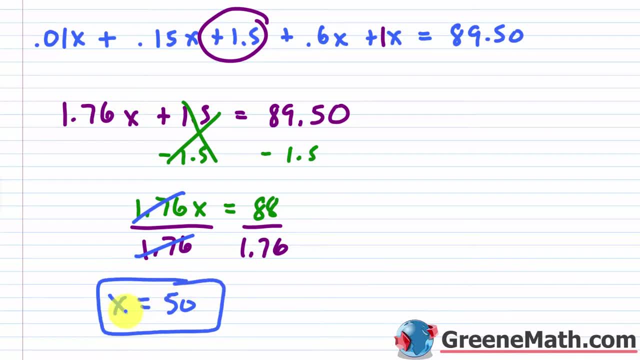 So this is our answer here, But again we've got to go back and make sense of it. All right, so we know that X represents the number of pennies, And again we found that X was 50. So there are 50 pennies. 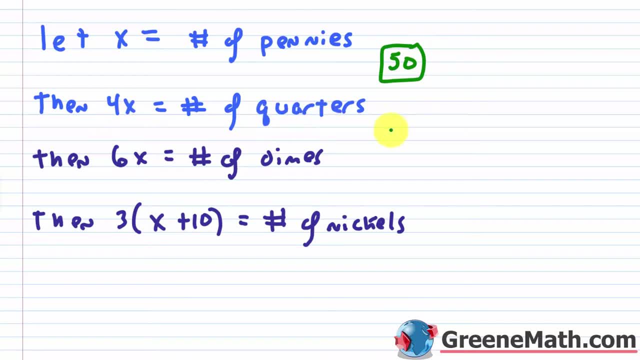 Then 4 times X is the number of quarters, Again X is 50.. 4 times 50 is 200.. So there's going to be 200 quarters. Then 6X is the number of dimes, Again X is 50.. 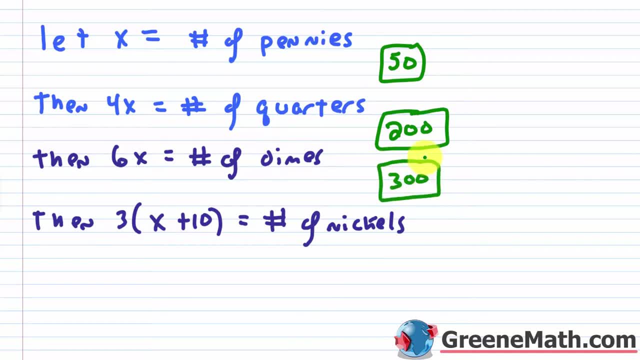 6 times 50 is 300.. So there's 300 dimes. And then lastly, 3 times the quantity X plus 10 is the number of nickels. So X again is 50.. 50 plus 10 is 60.. 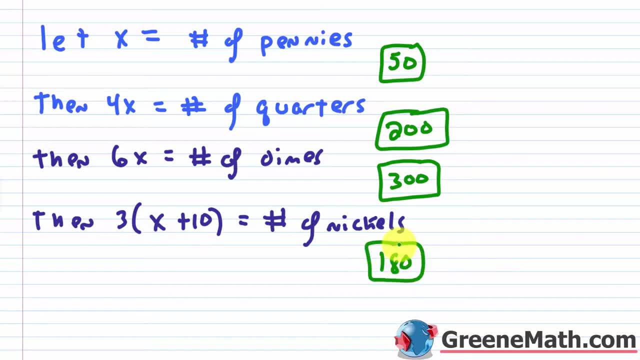 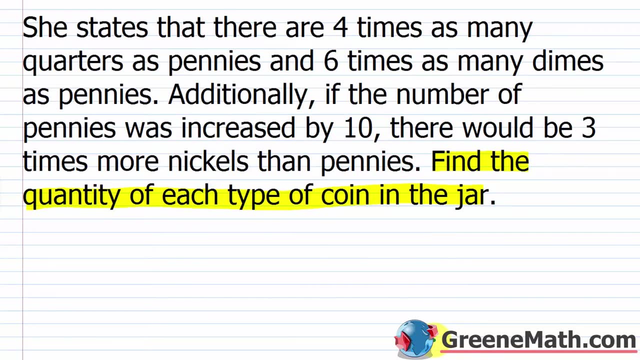 60 times 3 is 180.. So there's 180 nickels. So let's go ahead and write our answer. So find the quantity of each type of coin in the jar. We can say that there are 50 pennies, 180 nickels, 300 dimes. 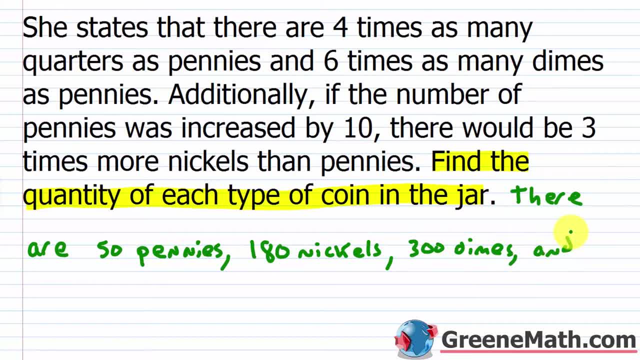 And then, lastly, we'll say: and there's 200 quarters, 200 quarters, We can say in her jar. Okay, So there are 50 pennies, 180 nickels, 300 dimes and 200 quarters in her jar. 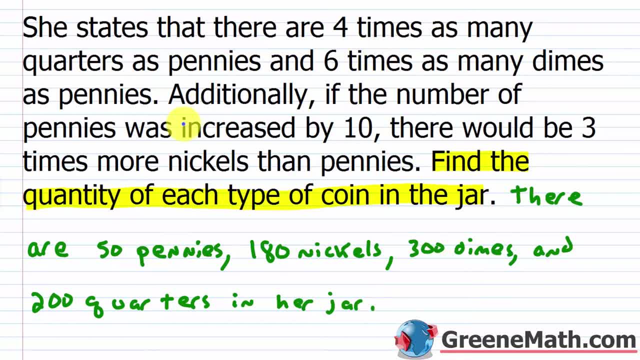 So let's check this. So it tells us there are 4 times as many quarters as pennies. You've got 50 pennies and 200 quarters, So that checks out. So I'll just put a check there. Then we're told there are 6 times as many dimes as pennies. 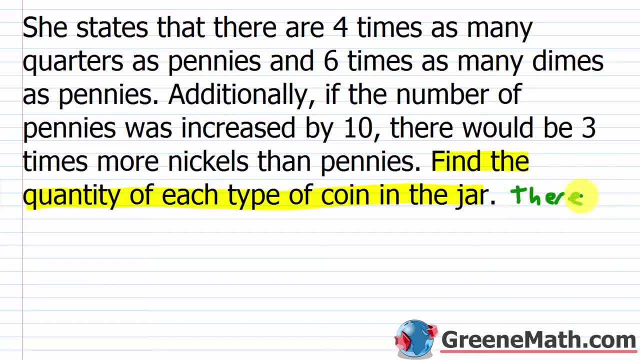 there are 50 pennies, 180 nickels, 300 dimes. And then lastly we'll say: and there's 200 quarters, 200 quarters, We could say in her jar. Okay, So there are 50 pennies, 180 nickels, 300 dimes and 200 quarters in her jar. 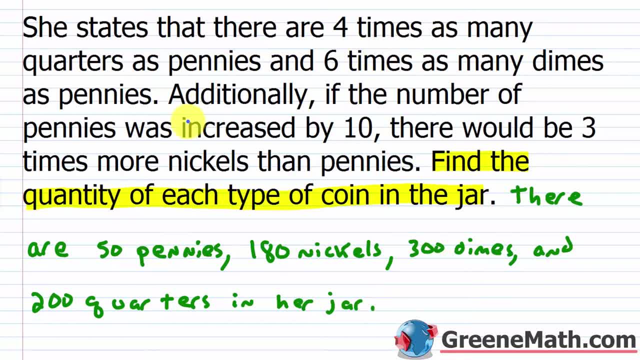 So let's check this. So it tells us there are 4 times as many quarters as pennies. You've got 50 pennies and 200 quarters. So that checks out. So I'll just put a check there. Then we're told there are 6 times as many dimes as pennies. You've got 300 dimes and 50 pennies. 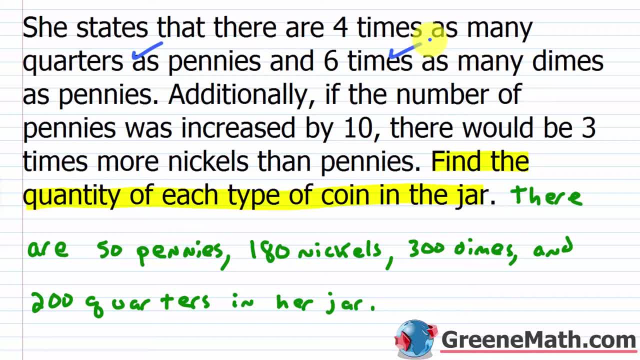 So that checks out right. 300 is 6 times 50. And then, additionally, if the number of pennies was increased by 50, then we're told that there are 4 times as many quarters as pennies, So that: 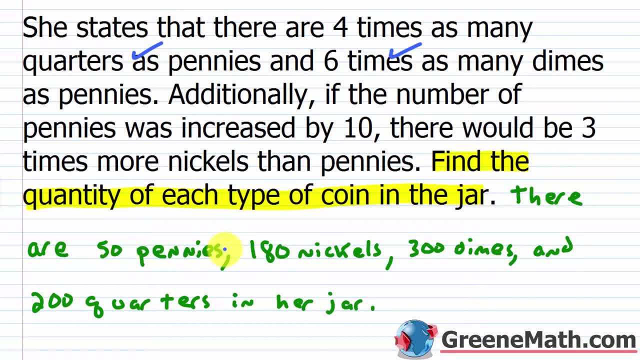 tells us there are 6 times as many quarters as pennies. So that's what this tells us. So if we went from 50 to 60, there would be 3 times more nickels than pennies. Well yeah, If I had 60 pennies, I have 180 nickels. 60 times 3 is 180. So we're good to go there. 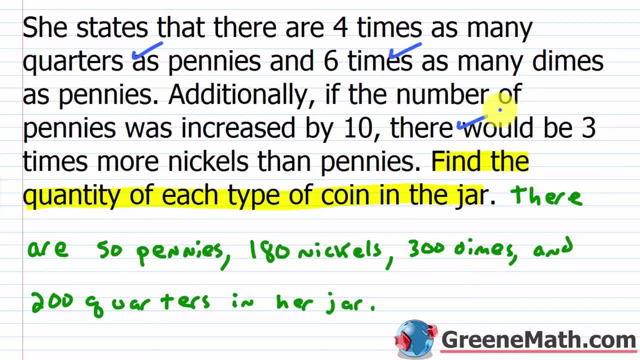 as well. Now, the last thing to check is the value. If I have 50 pennies, that's .5 or 50 cents. If I have 180 nickels, that's 180 times .05.. It's basically $9.. If I have 300. 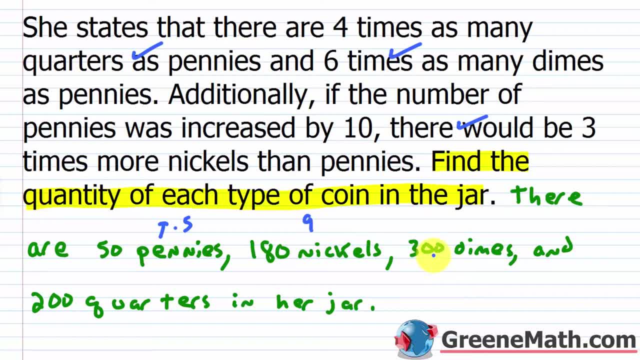 dimes, it's basically $9.. And if I have 100 nickels, that's 180 times .05.. It's basically 300 times 0.1,. that's going to be $30.. And then if she has 200 quarters, that's 200 times 0.25,. 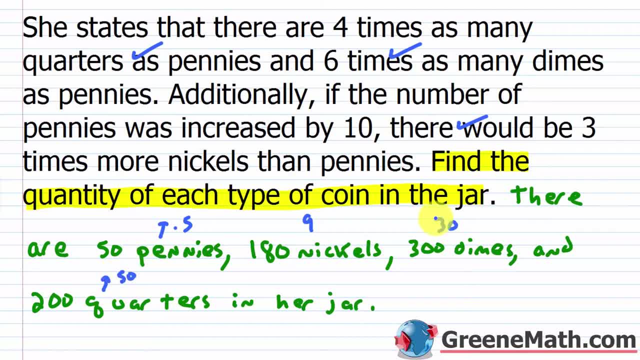 which is going to be 50.. Okay, So 50 plus 30 is 80.. 80 plus nine is 89 plus 50 cents is going to be $89 and 50 cents. So we're good to go on our value, right? If we add everything up, we do get. 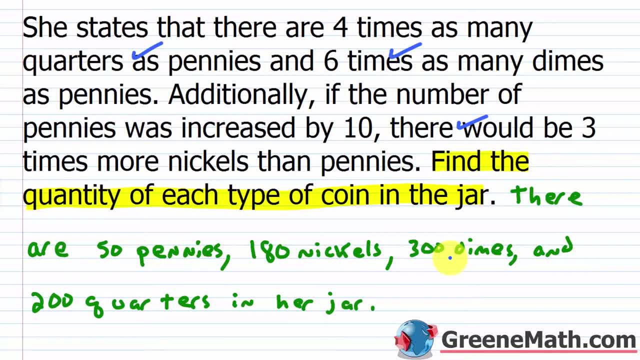 $89 and 50 cents, which again is what it told us in the problem. So we can say our answer here is correct. There are 50 pennies, 180 nickels, 300 dimes and 200 quarters in her jar In this lesson. 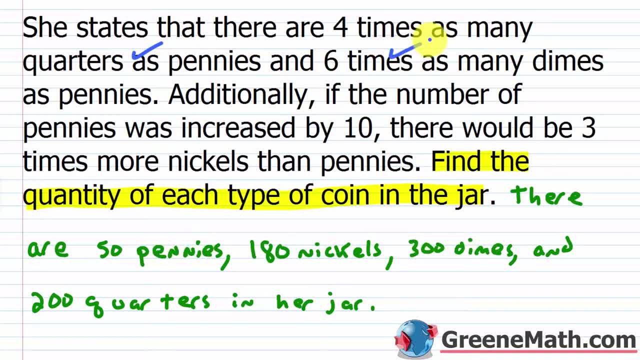 You've got 300 dimes and 50 pennies. So that checks out Right. 300 is 6 times 50. And then, additionally, if the number of pennies was increased by 10. So if we went from 50 to 60, there would be 3 times more nickels than pennies. 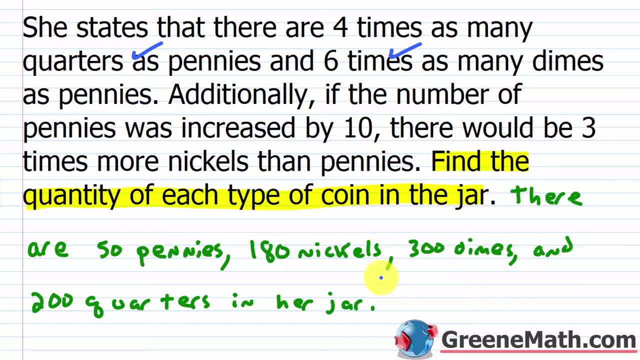 Well, yeah, if I had 60 pennies, I have 180 nickels. 60 times 3 is 180.. So we're good to go there as well. Now, the last thing to check is the value. If I have 50 pennies, that's 0.5 or 50 cents. 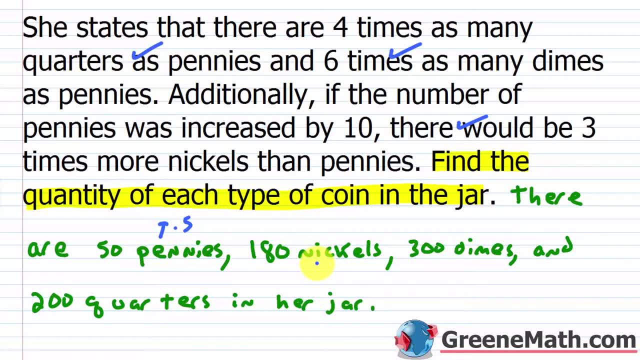 If I have 180 nickels, that's 180 nickels, That's 180 times 0.05.. It's basically $9.. If I have 300 dimes, it's basically 300 times 0.1.. That's going to be $30.. 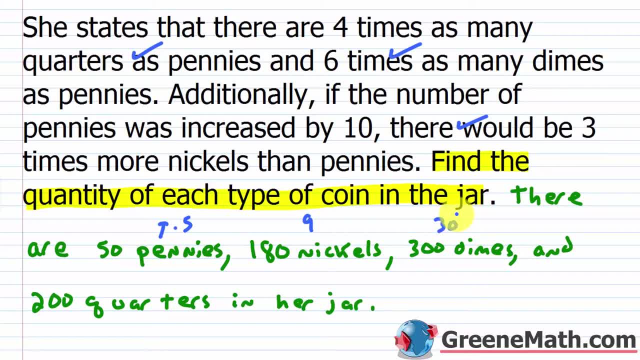 And then if she has 200 quarters, that's 200 times 0.25, which is going to be 50.. Okay, So 50 plus 30 is 80.. 80 plus 9 is 89.. Plus 50 cents is going to be $89.50. 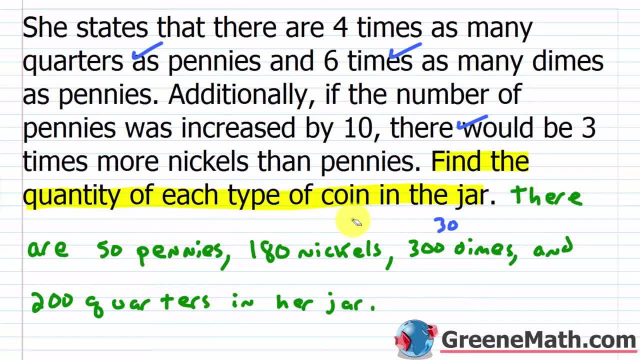 So we're good to go on our value Right. So if we add everything up we do get $89.50, which again is what it told us in the problem. So we can say our answer here is correct. There are 50 pennies, 180 nickels, 300 dimes and 200 quarters in her jar. 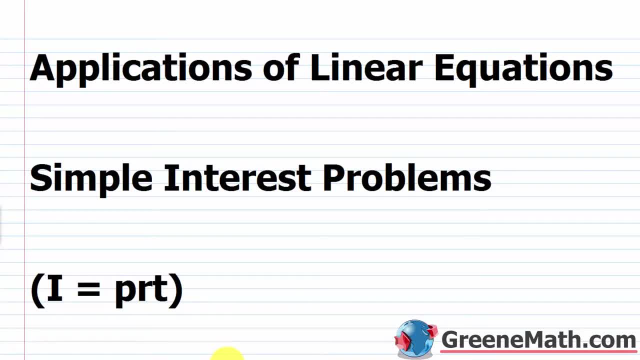 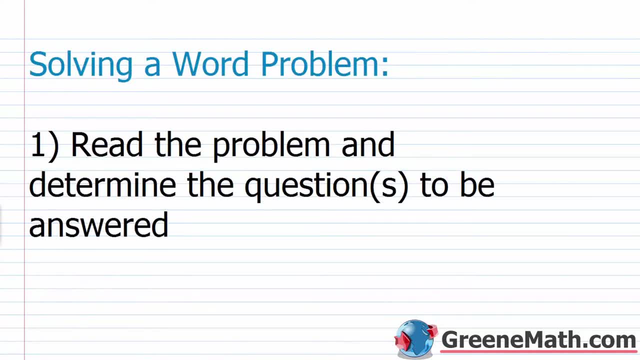 In this lesson we want to review applications of linear equations and look at some simple interest problems. So again, when we're solving applications of linear equation problems, we can use this little six-step procedure to help us out. So for solving a word problem, we have that. we want to read the problem and determine the question or, again, questions to be answered. 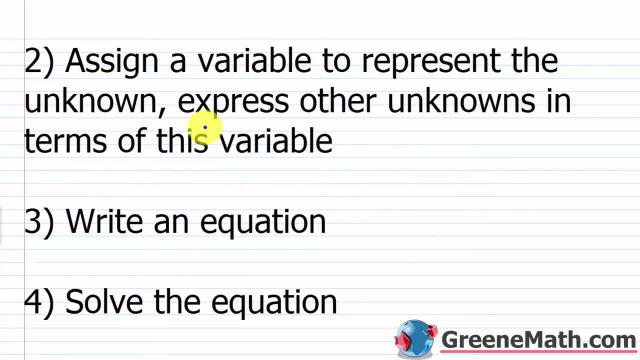 We want to assign a variable to represent the unknown And then, with these type of problems, you're going to be able to express other unknowns in terms of this variable. Then we're going to write an equation, We're going to solve the equation. 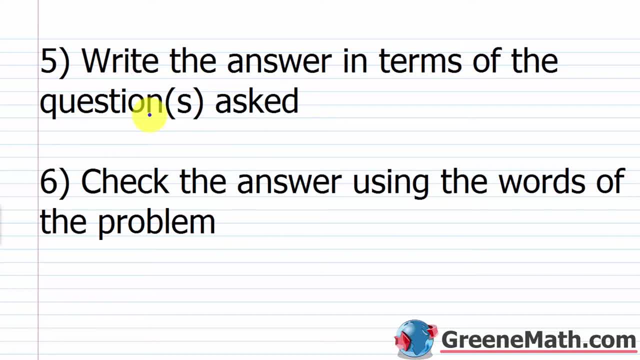 We're going to write the answer in terms of the question or questions asked And then we're going to check the answer using the words of the problem. So this part, right here. the last part. Just make sure your answer is reasonable, All right. 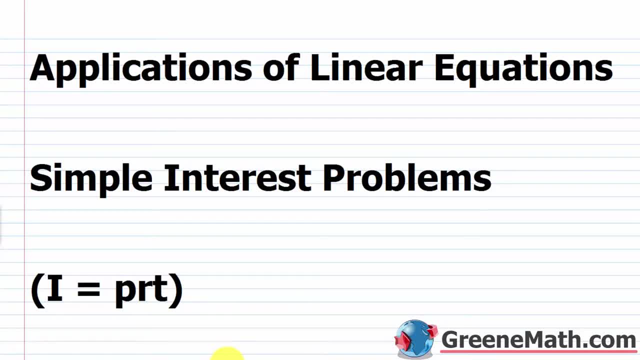 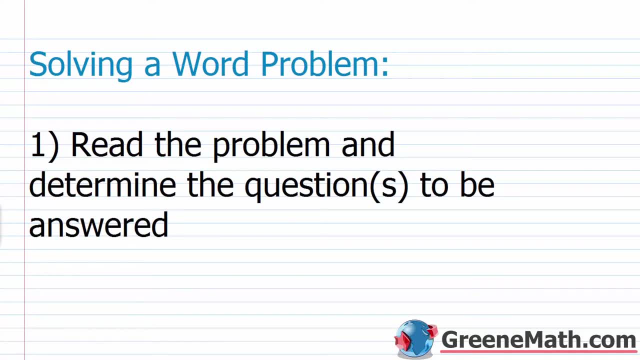 we want to review applications of linear equations and look at some simple interest problems. So again, when we're solving applications of linear equation problems, we can use this little six-step procedure to help us out. So for solving a word problem, we have that. we want to read the problem. 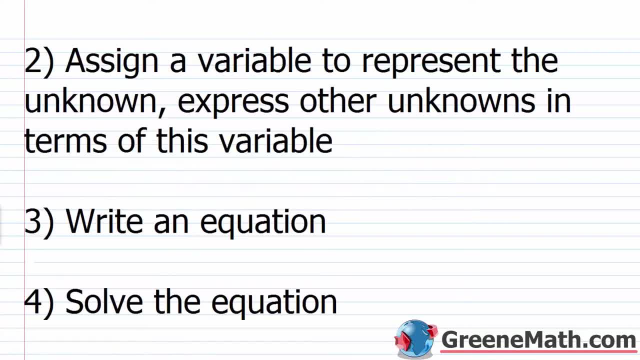 and determine the question or, again, questions to be answered. We want to assign a variable to represent the answer. So we want to assign a variable to represent the answer. So we want to the unknown, And then, with these type of problems, you're going to be able to express other unknowns. 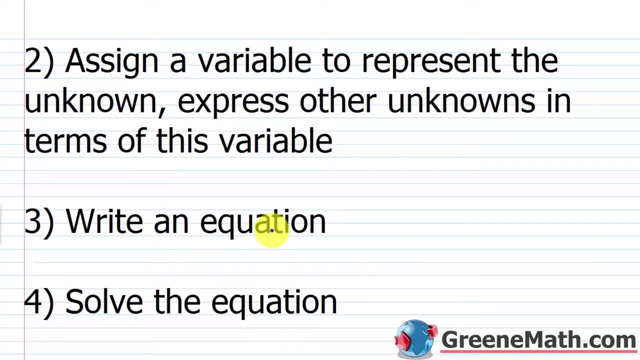 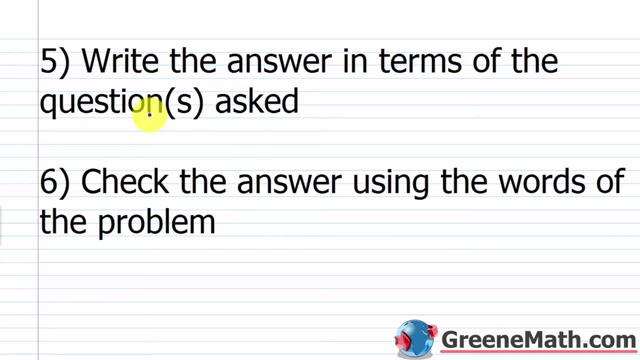 in terms of this variable, Then we're going to write an equation, We're going to solve the equation, We're going to write the answer in terms of the question or questions asked And then we're going to check the answer using the words of the problem. So this part, right here. the last part. 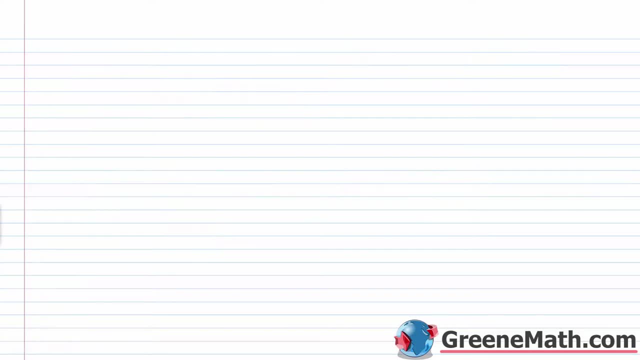 just make sure your answer is reasonable. All right, So for today's problems we're going to be using the simple interest formula. So the simple interest formula goes like this: We have I, which is the amount of simple interest earned, is equal to P, which is the principal or amount. 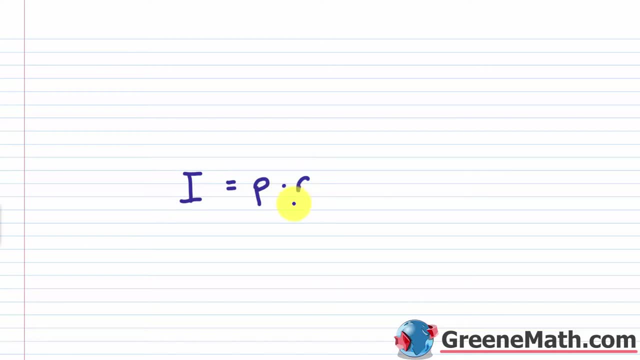 invested. times R, which is the rate as a decimal, times T, which is the time which is generally given to us in years, But it could be months, it could be weeks, it could be whatever they give to you, Okay, But generally it's going to be years. Now, one thing we need to understand before we 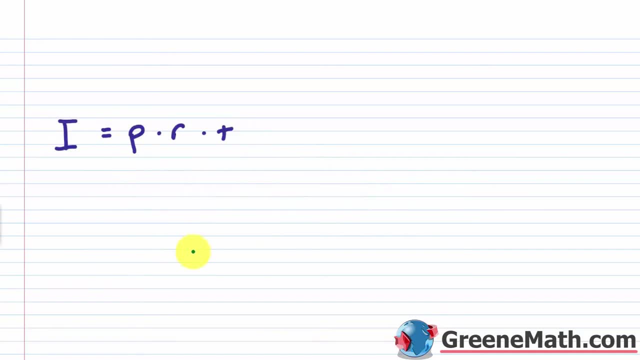 move on is kind of the difference between simple interest and compound interest. We will look at examples that deal with compound interest later on in the course. We need to kind of build some concepts before we deal with that, But right now we'll be dealing with just simple. 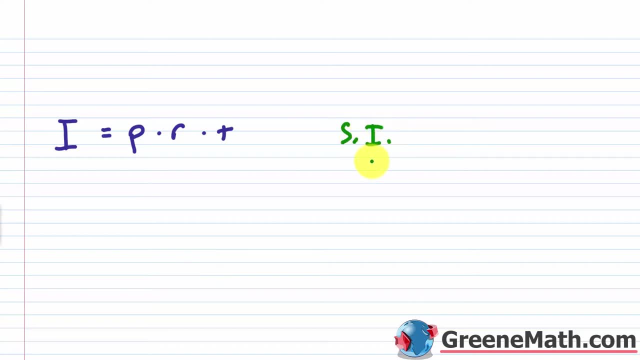 interest. So with simple interest, I only earn interest on the principal or the original amount invested. With compound interest, I earn interest on interest. So let's look at a very simple example. Let's say that my original amount that I invest is $1,000.. Okay, So this is my account. 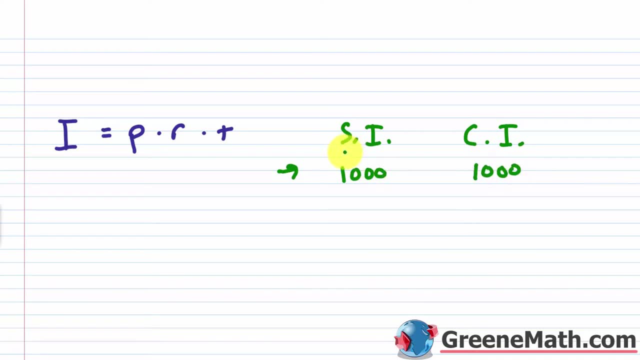 balance with each of these. Okay, So one is a savings account with simple interest, One's a compound interest And let's say each of them pays me 10%. Okay, So it's 10% in each case. So no difference At the end of year one. let's just assume they hold the money for a year And at the 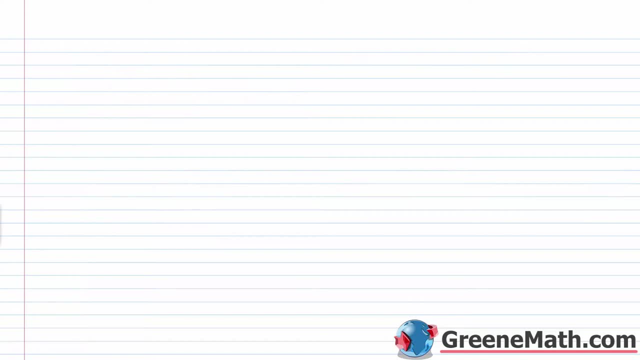 So for today's problems we're going to be using the simple interest formula. So the simple interest formula goes like this: We have: I, which is the amount of simple interest earned, is equal to P, which is the principal or amount invested, times R, which is the rate as a decimal, times T, which is the time which is generally given to us in years. 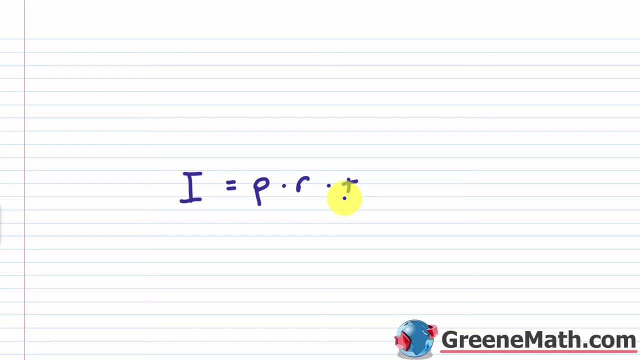 But it could be months, It could be weeks, It could be whatever they give to you Okay, But generally it's going to be years. Now one thing we need to understand before we move on Is kind of the difference between simple interest and compound interest. 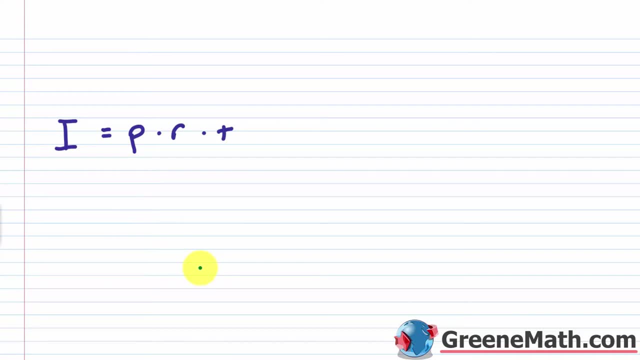 We will look at examples that deal with compound interest later on in the course. We need to kind of build some concepts before we deal with that, But right now we'll be dealing with just simple interest. So with simple interest I only earn interest on the principal or the original amount invested. 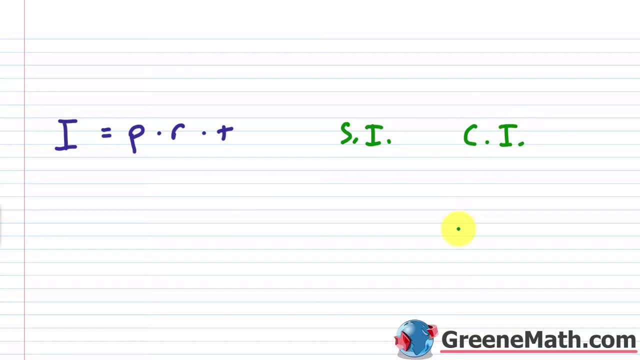 With compound interest, I earn interest on interest. So let's look at a very simple example. Let's say that my original amount that I invested Is $1,000.. Okay, So this is my account balance with each of these. Okay. 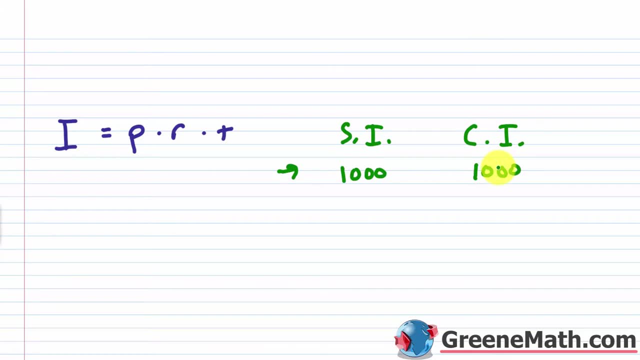 So one is a savings account with simple interest, One is a savings account with compound interest, And let's say each of them pays me 10%. Okay, So it's 10% in each case. So no difference At the end of year one. let's just assume they hold the money for a year. 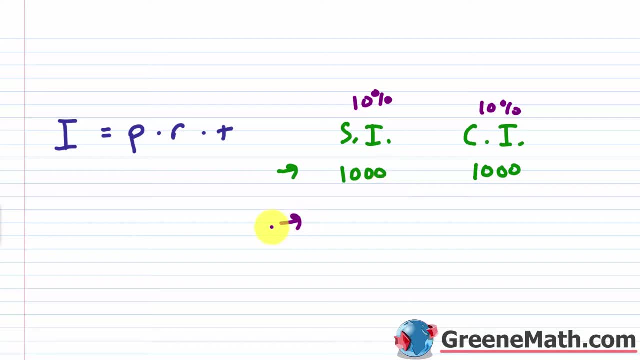 And at the end of the year they give us our interest payment. So at the end of year one- then this guy right here- 10% of $1,000 is $100. So my balance is $1,100.. Same thing when it's compounding. 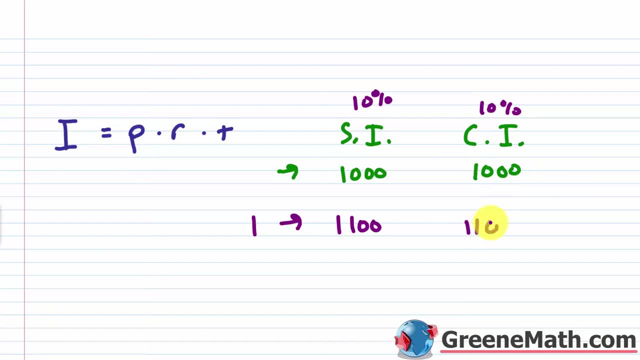 I didn't get any interest dropped in there yet, So it's still $1,100.. Now, at the end of year two, what's going to happen is I'm going to have a difference, Right, Because this guy, I- just get paid on the original amount that I invested, which is $1,000. 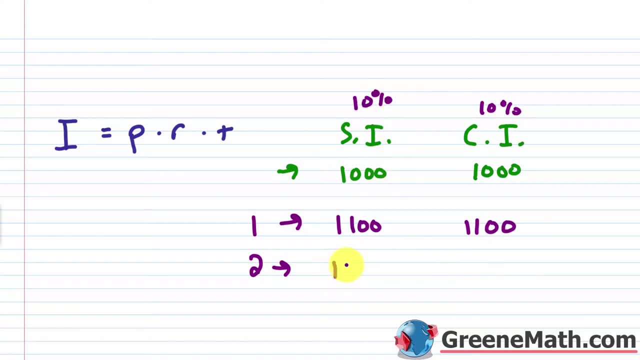 So I get my 10% again, which is just $100.. So this guy is going to go to $1,200.. Okay, So that's where it is. with simple interest, With compound interest, they're now going to say, okay, you get 10% of the balance. 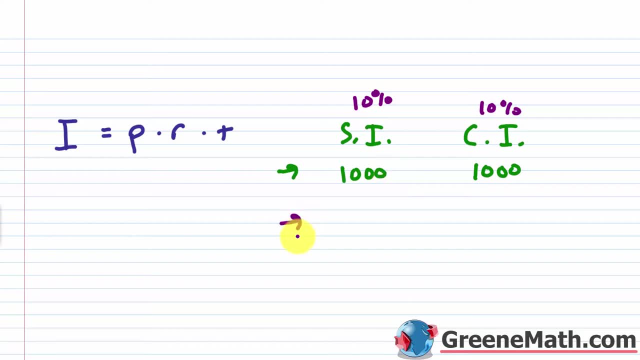 end of the year they give us our interest payment, So at the end of year one. then this guy right here: 10% of a thousand is a hundred, So my balance is $1,100.. Same thing when it's compounding. I. 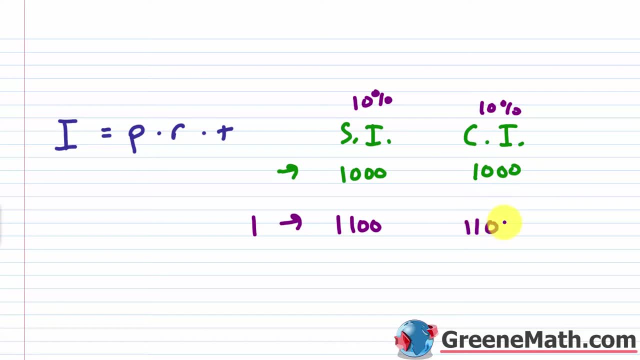 didn't get any interest dropped in there yet, So it's still $1,100.. Now, at the end of year two, what's going to happen is I'm going to have a difference, right, Because this guy just get paid on the original amount that I invested, which is a thousand. So I get my 10% again, which is just. 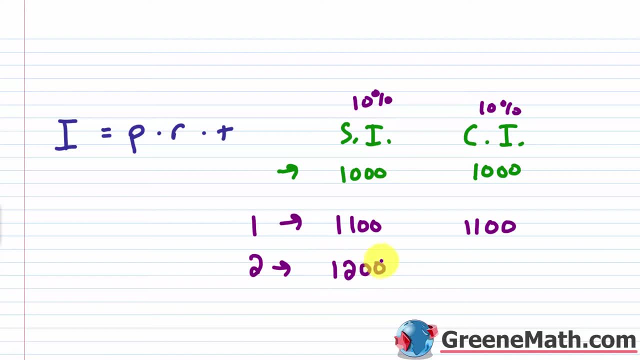 $100.. So this guy's going to go to 1200.. Okay, So that's where it is with simple interest. With compound interest, they're now going to say, okay, you get 10% of the balance, So the balance is. 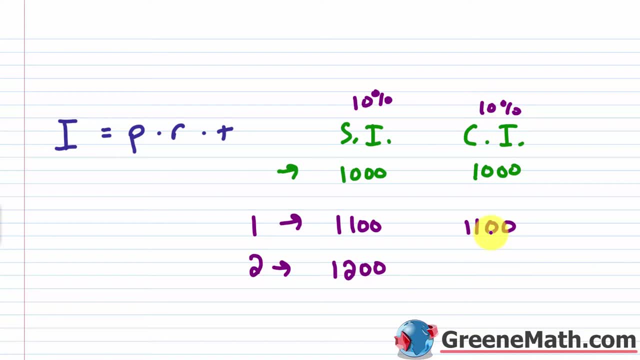 $1,100. So I'm going to get 10% of that, which is $110.. So I'm going to get $1,210 as a balance. So the difference here is that I have 1200 from simple interest or $1,210 with compound interest. 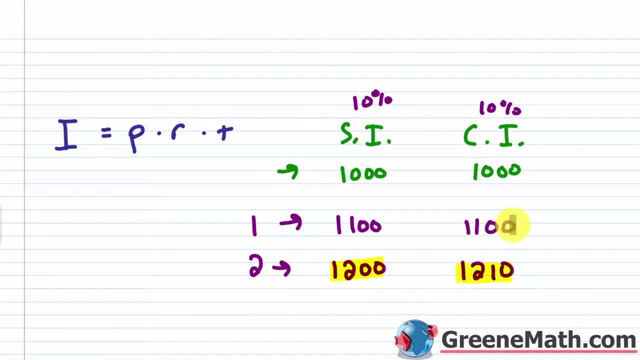 because my interest that was earned, which was a hundred dollars at that point, earned interest of 10%. Okay, A hundred dollars, 10% of that is 10 bucks. So that's where you're going to get the difference in the account balance. Okay, So simple interest. you only earn interest on the original. 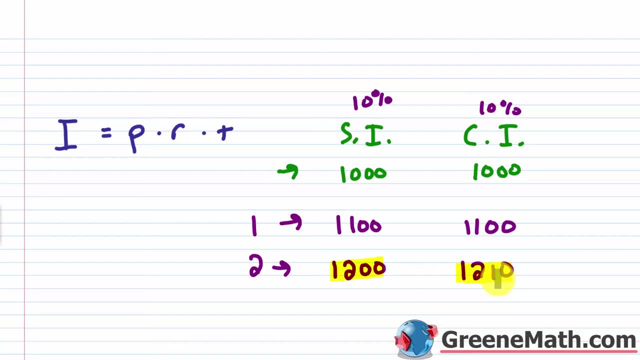 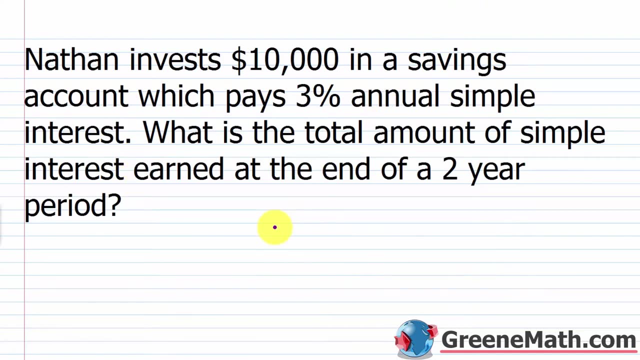 amount invested, Compound interest, you earn interest on the full balance, or you could say 10% of that. So let's look at a simple example here, just to kind of get our feet wet, And then we'll look at two kind of typical problems that you'd see. So Nathan invests $10,000 in a savings. 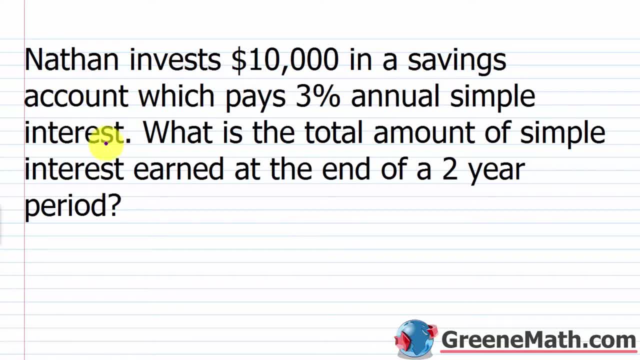 account which pays 3% annual simple interest. What is the total amount of simple interest earned at the end of a two-year period? So again, for this guy right here, you can almost do this mentally. You can say what This is. I simple interest earned equals P, which is the principal. 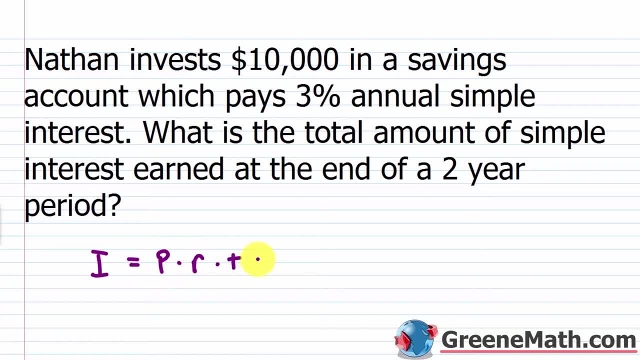 times R the rate as a decimal. times T the time, in this case in years. Mentally I can say: okay, $10,000 times 3% as a decimal is 0.03.. So if you do that, 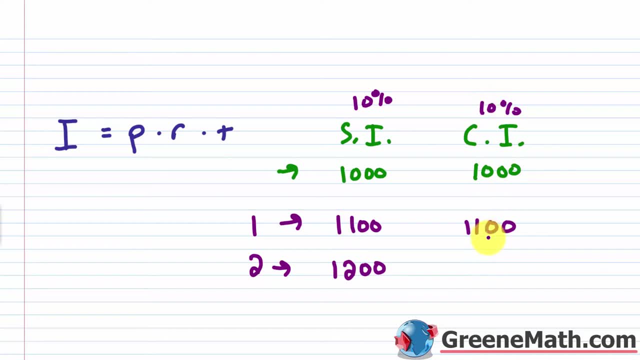 So the balance is $1,100.. So I'm going to get 10% of that, which is $110.. So I'm going to get $1,210 as a balance. Okay, So the difference here is that I have $1,200 from simple interest or $1,210 with compound interest. 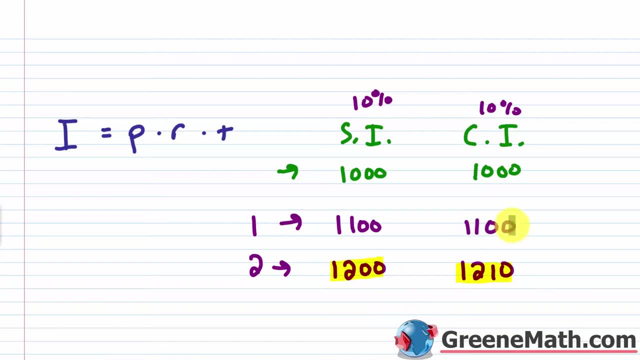 Because my interest that was earned, which was $100 at that point, earned interest of 10%. Okay, $100, 10% of that is $10. So that's where you're going to get the difference in balance. That's where you're going to get the difference in the account balance. 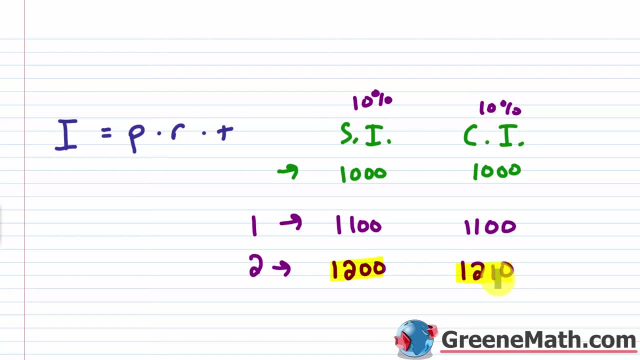 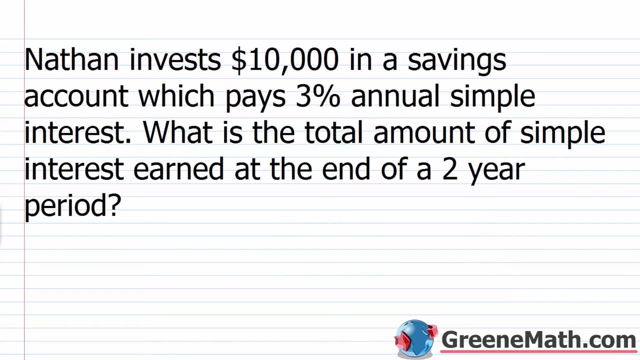 Okay, So simple interest: you only earn interest on the original amount invested. Compound interest, you earn interest on the full balance. Or you could say you earn interest on your interest, All right. So let's look at a simple example here, just to kind of get our feet wet. 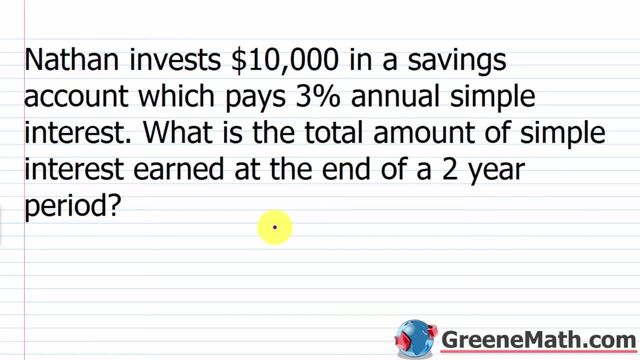 And then we'll look at two kind of typical problems that you'd see. So Nathan invests $10,000 in a savings account which pays 3% annual simple interest. What is the total amount of simple interest earned at the end of a two-year period? 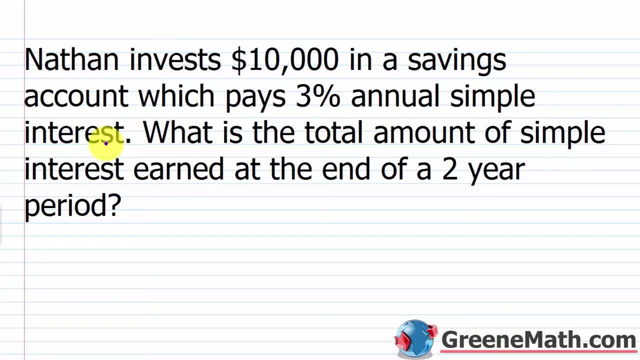 So again, for this guy right here, you can almost do this mentally. You can say what This is I simple: interest earned equals P, which is the principal. times R, the rate as a decimal times T, the time, in this case in years. 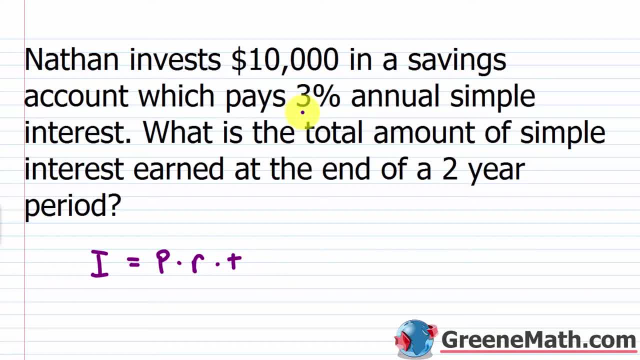 Mentally I can say: okay, $10,000 times 3% as a decimal is 0.03.. So if you do that, 10,000 times 0.03 is 300.. And so it's basically $300 a year for two years. 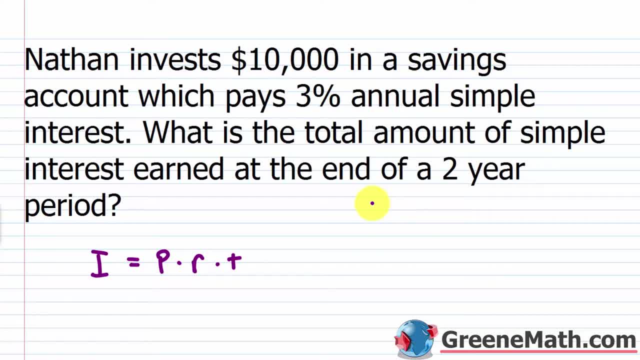 300 times 2 is 600. So he would earn $600 for the two-year period. But to plug it into the formula, to kind of make it official, you would substitute in a 10,000 for P, because that's your principal or amount invested. 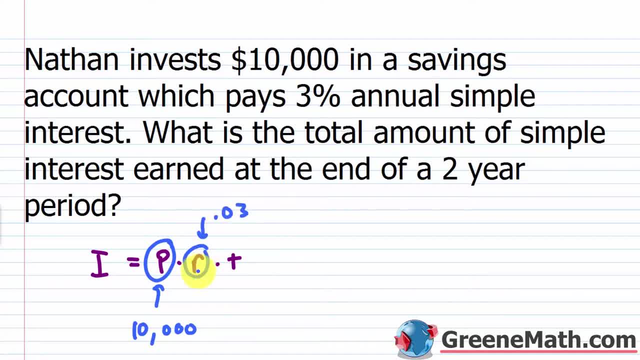 You would substitute in a 0.03 for your rate- It's always as a decimal- And you would substitute in a 2 for the time period. In this case that stands for two years. So again, make sure that the rate is in terms of years if you're dealing with years. 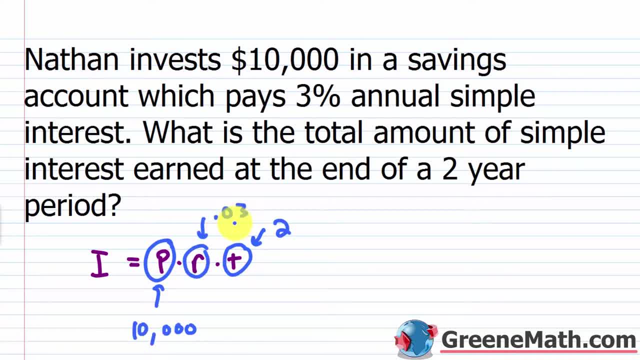 So we have 10,000 times 0.03, which is 300, times 2,, which is 600.. So you can say that your I or your simple interest earned is 600.. And again we can answer this. 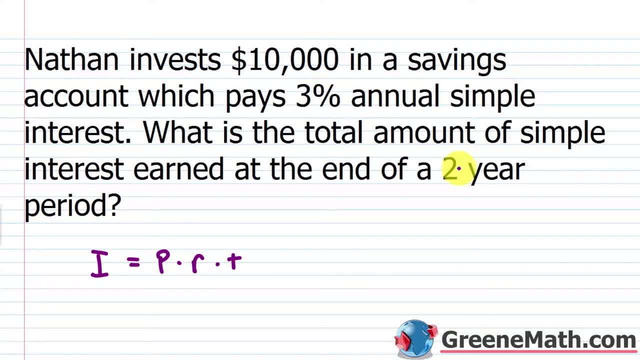 10,000 times 0.03 is 300. And so it's basically $300 a year for two years. 300 times two is 600. So he would earn $600 for the two-year period. But to plug it into the formula to kind of make: 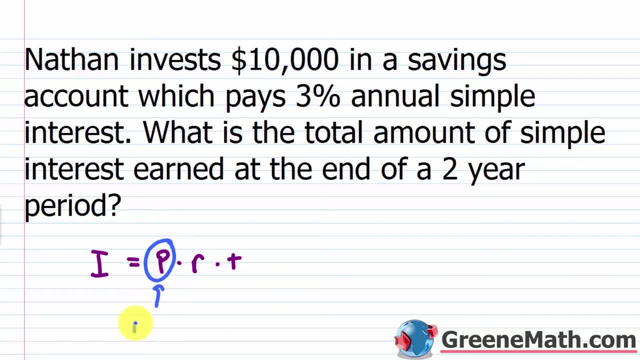 it official. you would substitute in a 10,000 for P, because that's your principal, or amount invested. You would substitute in a 0.03, which is the principal, and you would substitute in a 0.03, for your rate- Okay, It's always as a decimal- And you would substitute in a two for the time. 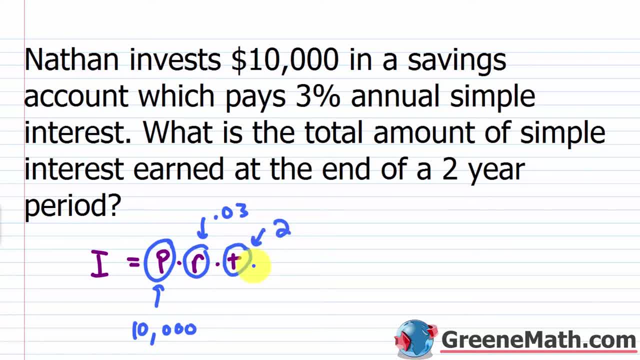 period. In this case, that stands for two years. Okay, So again, make sure that the rate is in terms of years, if you're dealing with years. Okay, So we have 10,000 times 0.03, which is 300. 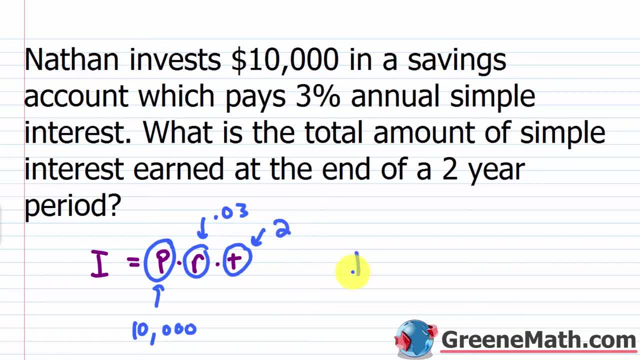 times two, which is 600.. So you can say that your I or your simple interest earned is 600.. And again, we can answer this. Let me just erase everything. We have our answer now. We'll make a nice little sentence and say that, Nathan. 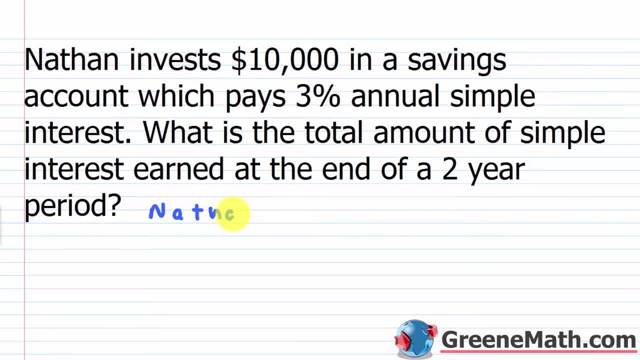 earned $600 at the end of two years. Okay, And lots of different sentences that you can construct to answer this. You're just looking for something that addresses what they asked. Okay, So it says: what is the total amount of simple interest earned as a total amount of simple interest earned, And you can say: 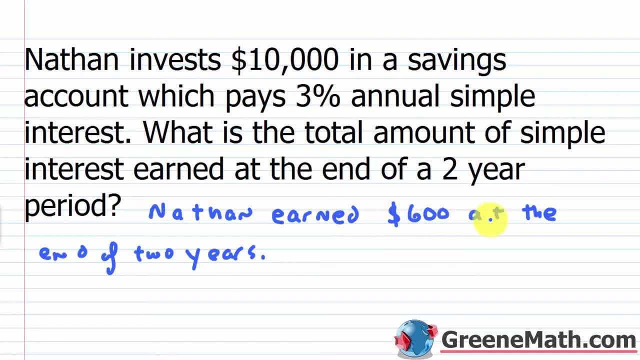 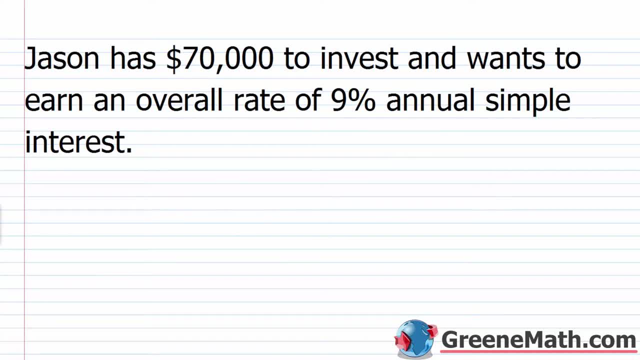 at the end of a two-year period. And we just said Nathan earned $600 at the end of two years. Perfectly acceptable. Okay, Let's look at a typical problem now, One where we'd have to set up kind of our full array of steps. So Jason has $70,000 to invest and wants to earn an overall. 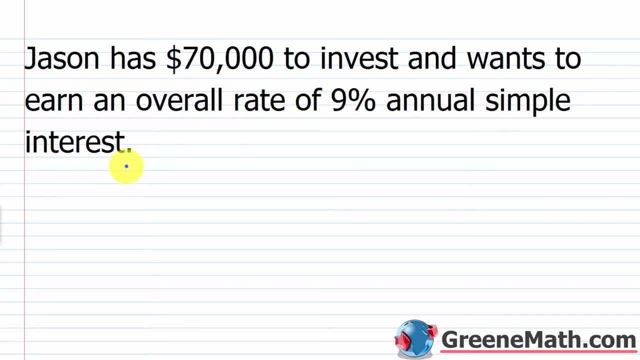 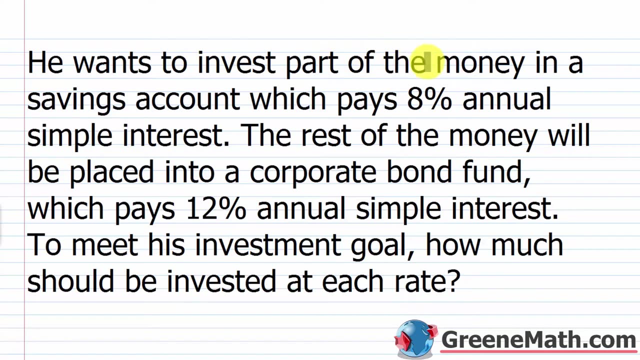 rate of 9% annual simple interest. So he has $70,000 to invest and he wants to earn an overall rate of 9% annual simple interest. Okay, Let's go down and look at the next part. So he wants to invest part of the money in a savings. 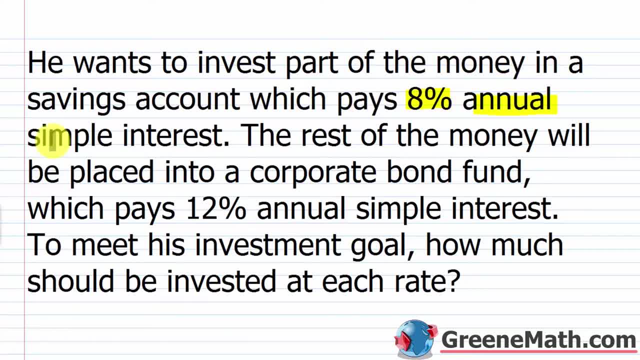 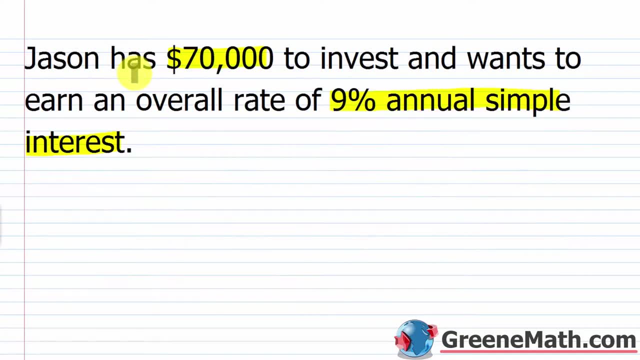 account which pays 8% annual simple interest. The rest of the money will be placed in a corporate bond fund which pays 12% annual simple interest. Then here's the question to meet his investment goal, which again was up here. He has $70,000 to invest and wants to earn an overall rate of 9%. 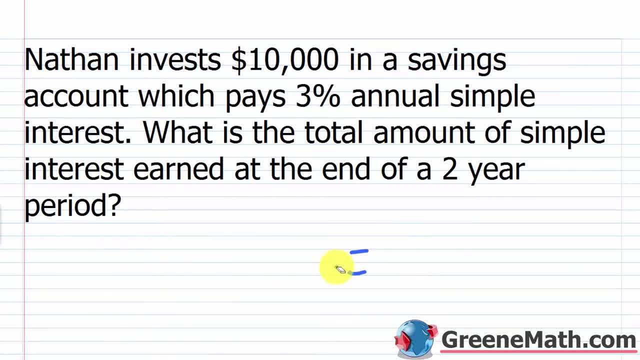 Let me just erase everything. We have our answer now. We'll make a nice little sentence and say that Nathan earned $600 at the end of two years. Okay, and lots of different sentences that you can construct to answer this. You're just looking for something that addresses what they asked. 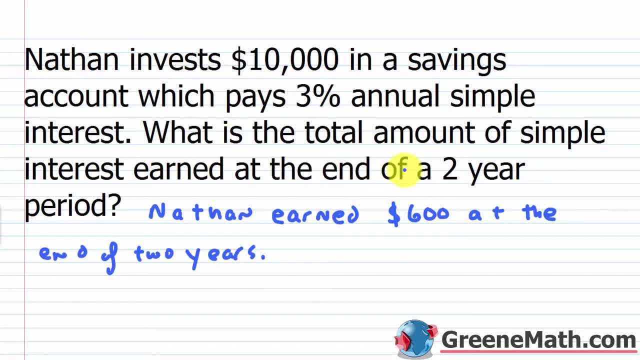 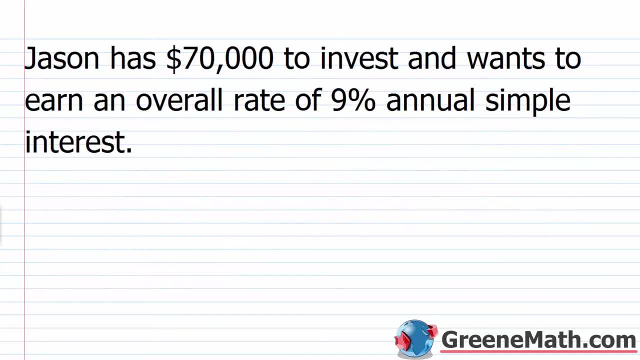 Okay. so it says what is the total amount of simple interest earned at the end of a two-year period? And we just said Nathan earned $600 at the end of two years. Perfectly acceptable. Okay, let's look at a typical problem now. 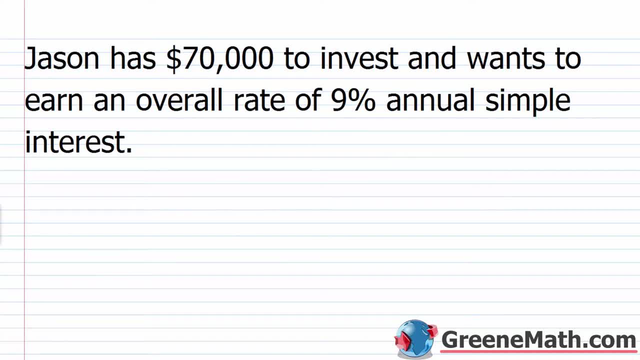 One where we have to set up, kind of our full array of steps. Okay, So Jason has $70,000 to invest and wants to earn an overall rate of 9% annual simple interest. So he has $70,000 to invest and he wants to earn an overall rate of 9% annual simple interest. 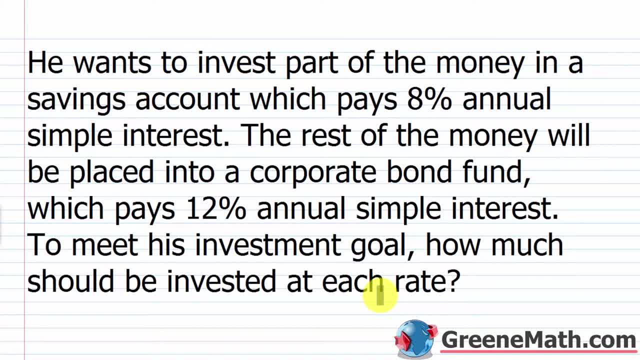 Okay, Let's go down and look at the next part. So he wants to invest part of the money in a savings account which pays 8% annual simple interest. The rest of the money will be placed in a corporate bond fund which pays 12% annual simple interest. 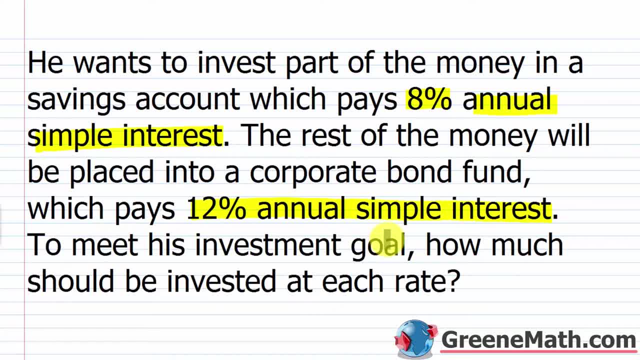 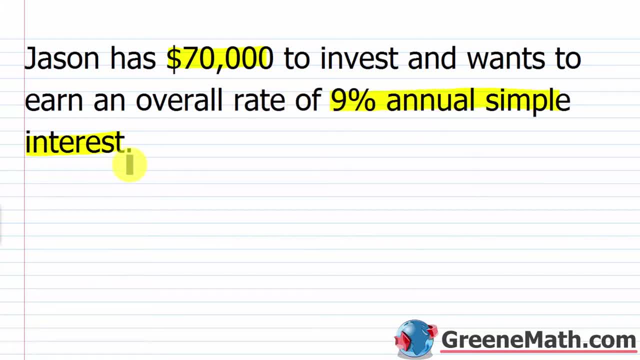 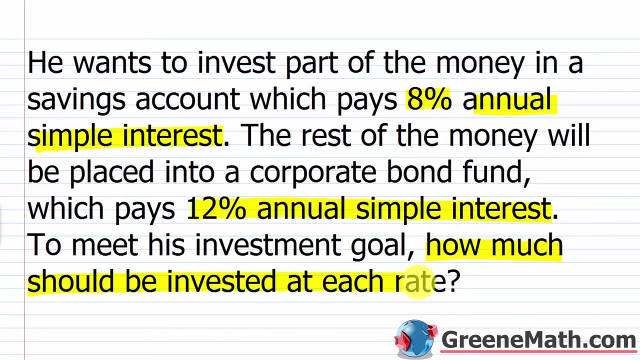 Then here's the question: To meet his investment goal, which again was up here, He has $70,000 to invest and wants to earn an overall rate of 9% annual simple interest. That's the investment goal. So to meet his investment goal, how much should be invested at each rate? 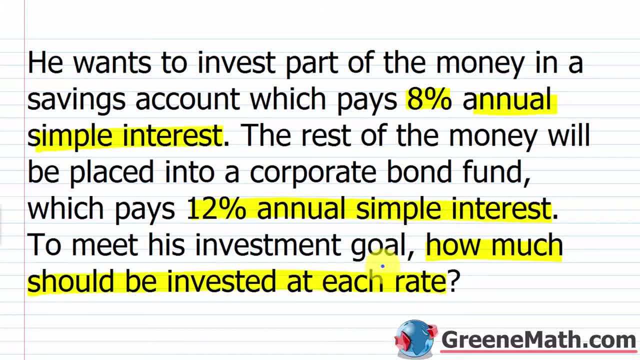 So to earn 9% on $70,000.. Okay, So he has $70,000.. How much should he put in the savings account and how much should he put in the corporate bond fund? All right, So we've read the problem. 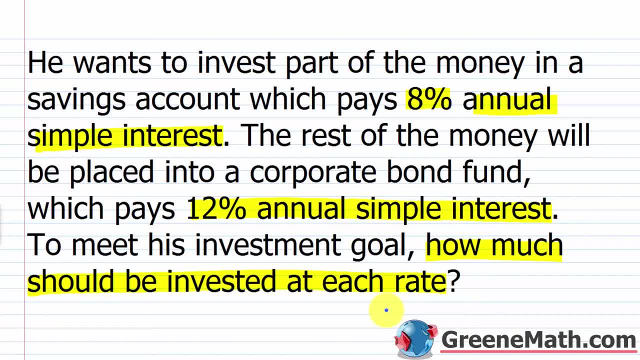 We understand what we need to do. Let's let a variable like X be equal to the amount he invests in one of these guys. It doesn't matter which one you choose. You can say X is the amount he invests in the savings account, or you can say X is the amount he invests in the corporate bond fund. 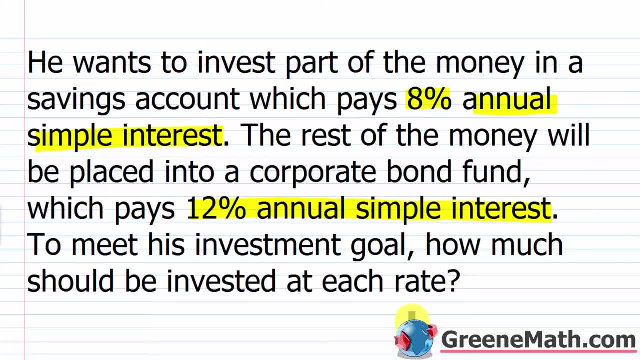 annual simple interest. That's the investment goal. He has $70,000 to invest and wants to earn an overall rate of 9% annual simple interest. That's the investment goal. so to meet his investment goal, how much should be invested at each rate? so to earn nine percent? 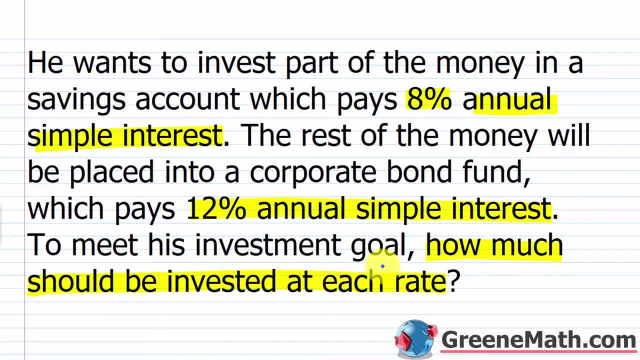 on seventy thousand dollars. how much should he put in the savings account and how much should he put in the corporate bond fund? all right, so we've read the problem. we understand what we need to do. let's let a variable like x be equal to the amount he invests in. one of these guys doesn't. 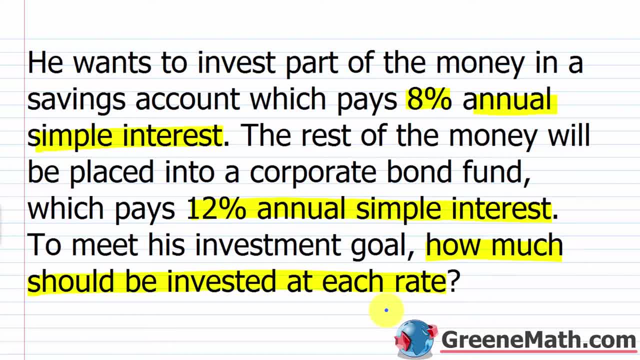 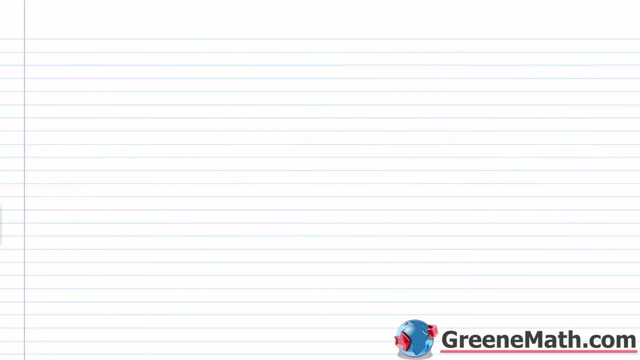 matter which one you choose. you can say x is the amount he invests in the savings account, or you can say x is the amount he invests in the corporate bond fund. it makes no difference. so i'm going to come down here and say we're going to let x be equal to the amount invested. 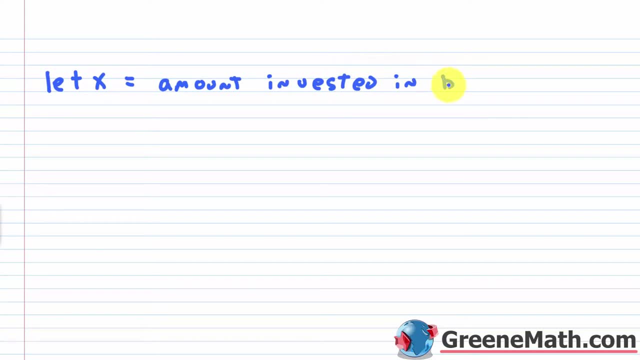 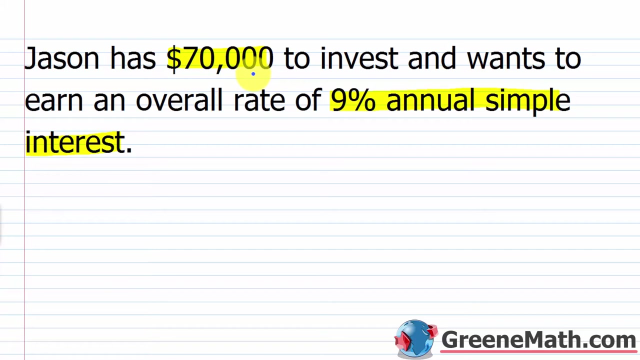 in the bond fund. let me put the in the bond fund, okay. so then, what can we say about the amount invested in the savings account? well, we're told that jason has a total of seventy thousand dollars to invest and he only puts it in either the savings account. 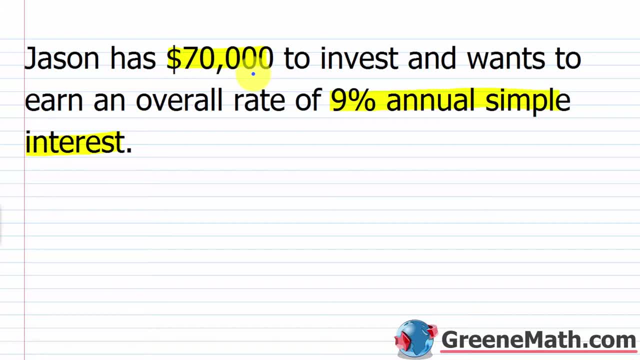 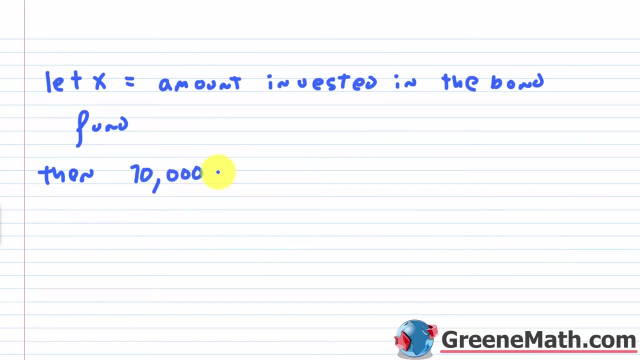 or the bond fund. so if x is representing the amount that's put in the bond fund, then seventy thousand minus x has to be the amount that he put in the savings account. so seventy thousand, which is the total amount minus x, which is the amount invested in the bond fund, is going to be equal to the amount. 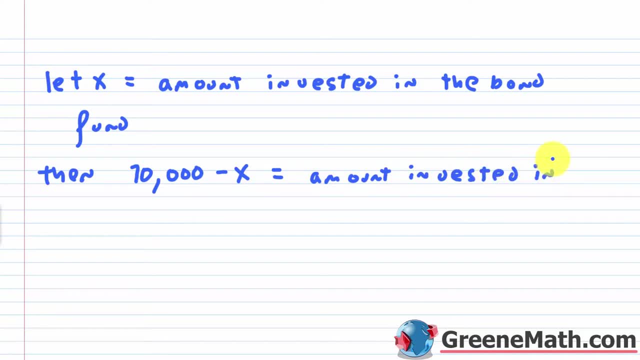 invested in the savings account. okay, nice and simple, let me make that better, okay? so now that we have kind of our variable set up and the other unknown is expressed in terms of that variable, we're going to move into a little bit more detail about how we're going to. 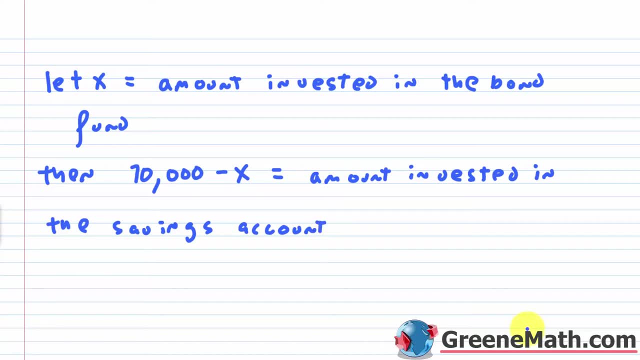 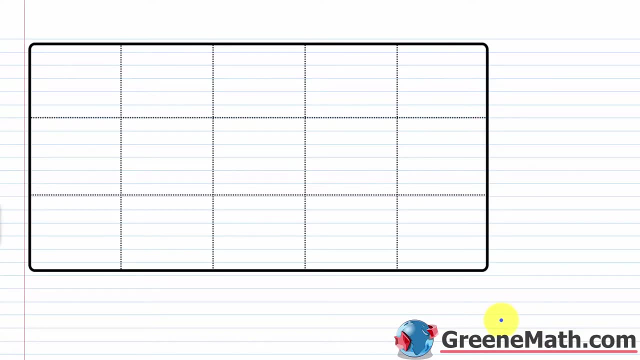 move into a little bit more detail about how we're going to move into a little bit more detail about how we're going to into our next step, which is to basically set up an equation. to do that, i'm going to make a little table a lot of times. i think it's a little bit helpful if you're unfamiliar with solving word. 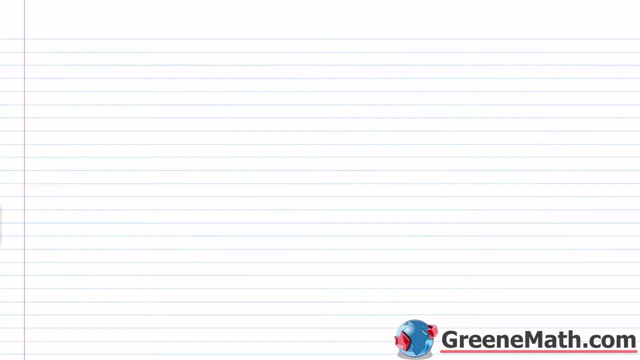 It makes no difference. So I'm going to come down here and say: we're going to let X be equal to the amount invested in the bond fund. Let me put the in the bond fund, Okay. So then what can we say about the amount invested in the savings account? 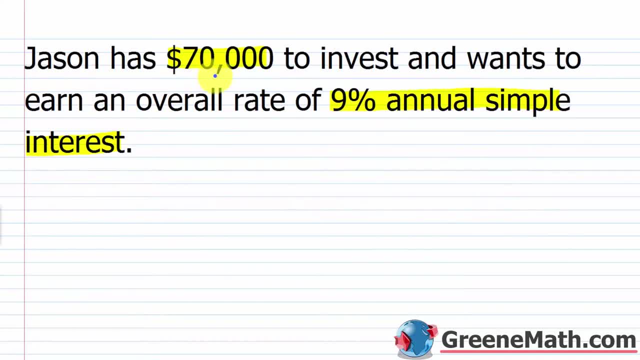 Well, we're told that Jason has a total of $70,000 to invest And he only puts it in either the savings account or the bond fund. So if X is representing the amount that's put in the bond fund, then 70,000 minus X has to be the amount that he put in the savings account. 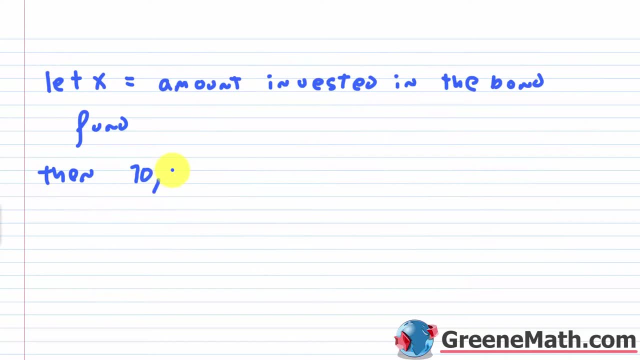 So 70,000, which is the total amount minus X, which is the amount invested in the bond fund, is going to be equal to the amount invested. So 70,000 minus X is equal to the amount that he put in the bond fund. 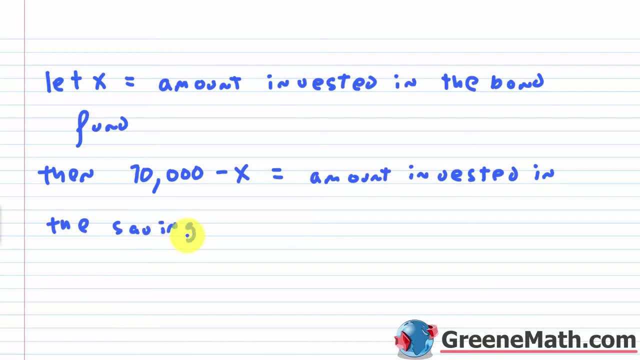 So that's going to be equal to the amount invested in the savings account. Okay, Nice and simple. Let me make that better. Okay, So now that we have kind of our variable set up and the other unknown is expressed in terms of that variable, 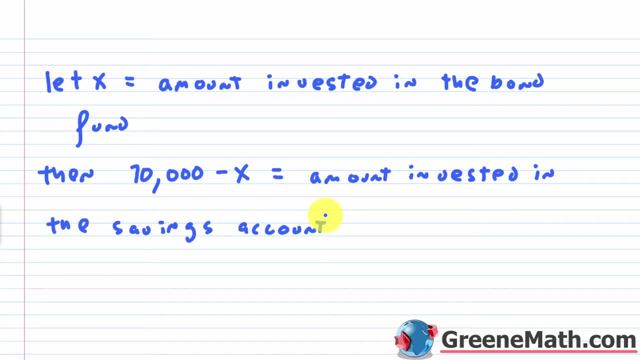 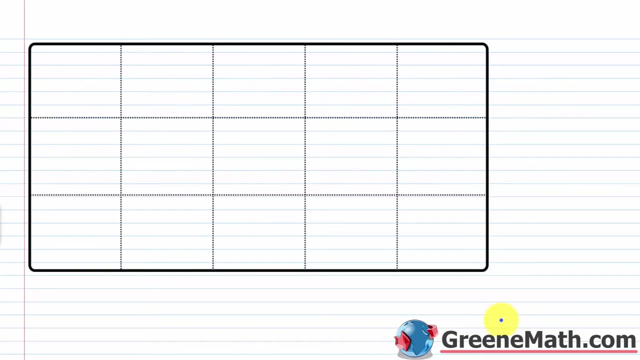 we're going to move into our next step, which is to basically set up an equation. To do that, I'm going to make a little table A lot of times. I think it's a little bit helpful, If you're unfamiliar with solving word problems, to set up a table. some people don't do it. 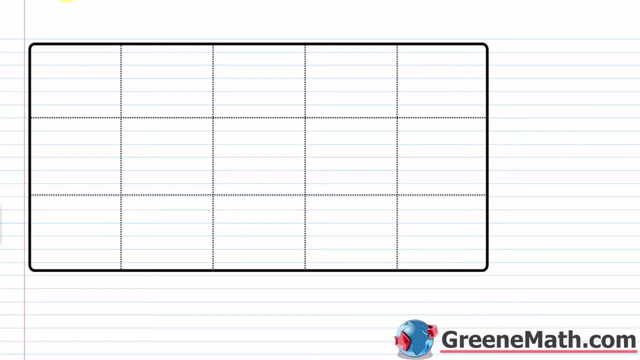 They feel like it's a waste of time but it can be helpful. So let's just go ahead and do it. So we're going to write our simple interest formula up here on the top. So I, the simple interest earned- is equal to P, the principal or amount invested. 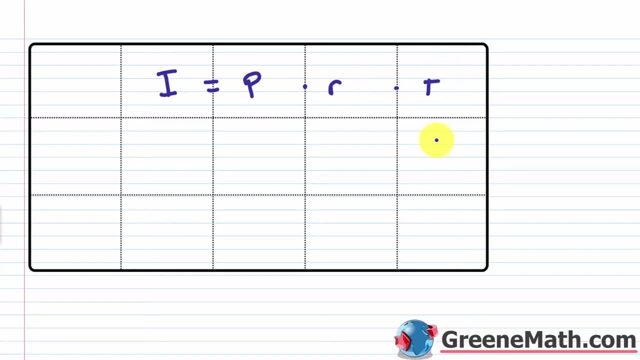 times R the rate as a decimal times T the time. Then, for this guy right here, this is going to be the investments. So I'll just put INV for investments. So you have the savings account and you have the corporate bond fund. 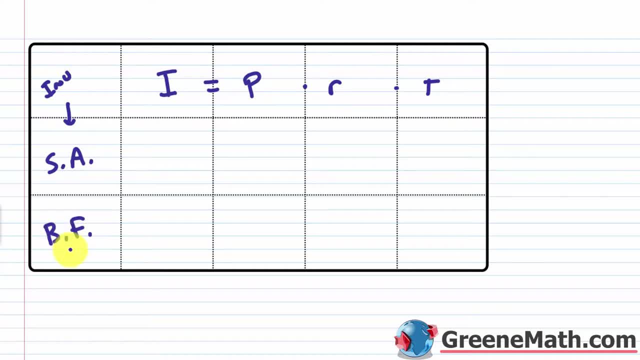 So I'll just kind of initial those. So we know that for the amount invested or the principal, the bond fund we said was X, So let's put an X here. For the savings account, we said it was $70,000 minus X. 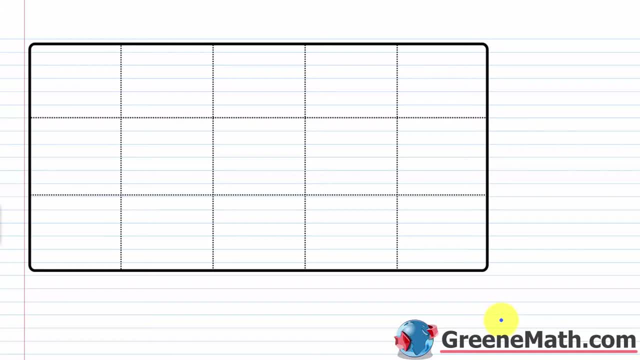 problems to set up a table. some people don't do it. they feel like it's a waste of time, but it can be helpful, so let's just go ahead and do it. so we're going to write our simple interest formula up here on the top. so i the simple interest earned is equal to p. the principle. 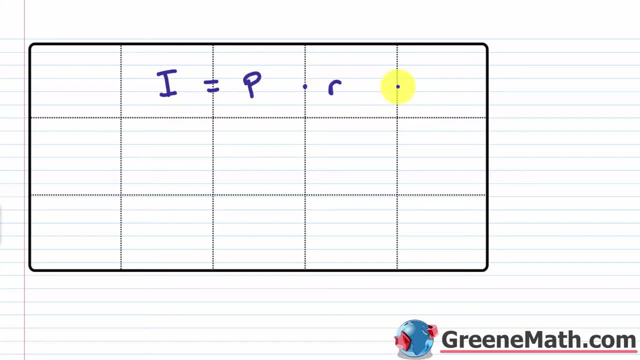 or amount invested. times r, the rate is a decimal times t the time. then for this guy right here, this is going to be plus or minus times r and minus i and minus x, all throughout this equation. so the to be the investments, So I'll just put INV for investments, So you have the savings account. 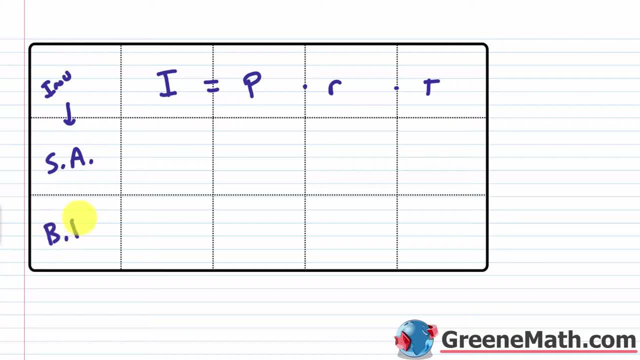 and you have the corporate bond fund. So I'll just kind of initial those. So we know that for the amount invested or the principal, the bond fund we said was X, So let's put an X here. For the savings account, we said it was 70,000 minus X. Now the rate is given to us in the 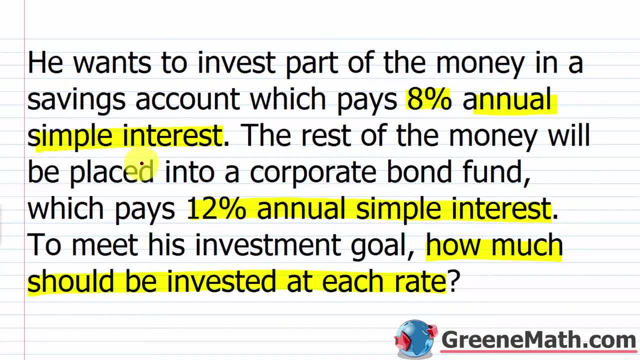 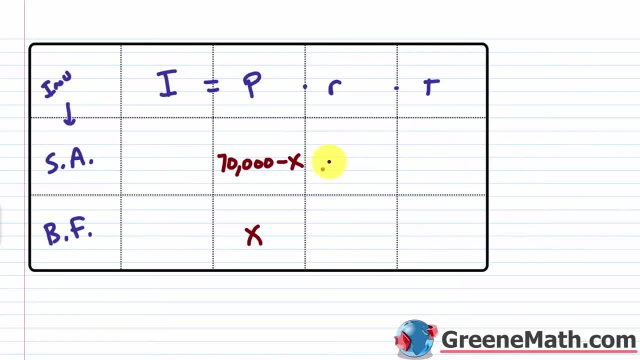 problem. It says the savings account pays 8% annual simple interest and it says the corporate bond fund pays 12% annual simple interest. So the savings account again is 8% or 0.08 as a decimal, The bond fund is 12% or 0.12 as a decimal. Now, what about the time? Well, basically we're dealing. 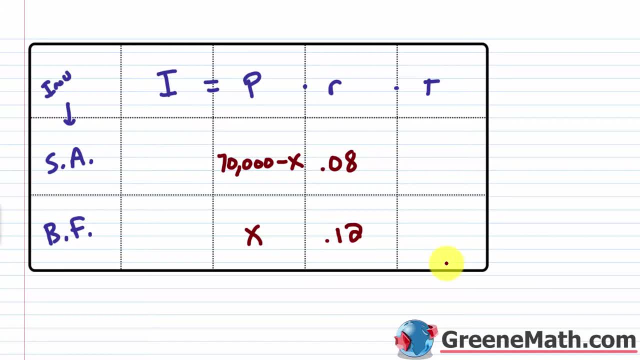 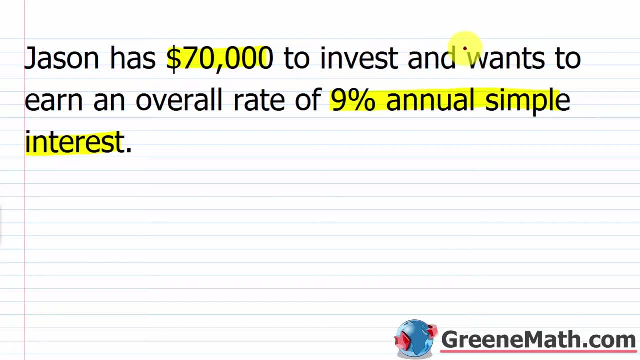 with a scenario where the time is just going to be one. So if we go back up, you can see that it basically says in the first part of the problem, Jason has $70,000 to invest and wants to earn an overall rate of $70,000. So we're going to go back up and we're going to go back and we're going to. 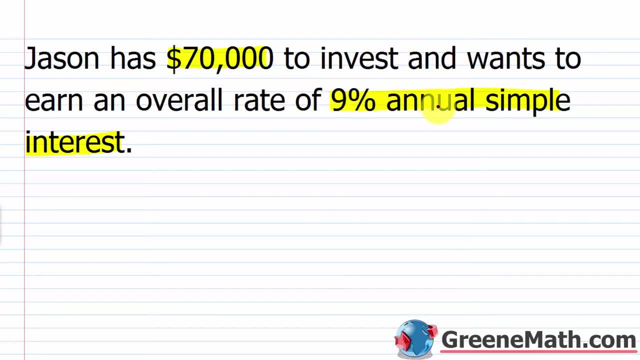 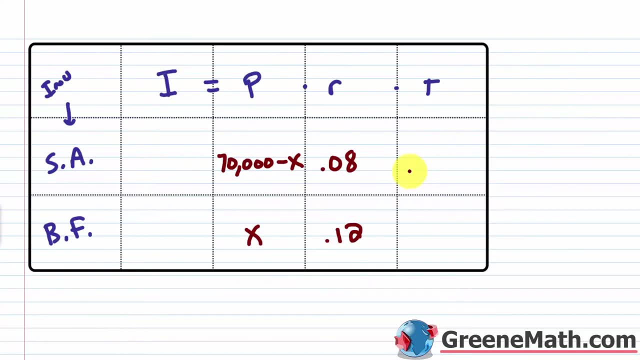 of 9% annual, which is yearly, simple interest. So what are we doing? for one year, right? One year period, So we can go back down and just put a one for each time period. You can basically get rid of it, because multiplying by one just leave something unchanged, right? But we'll just leave it there. 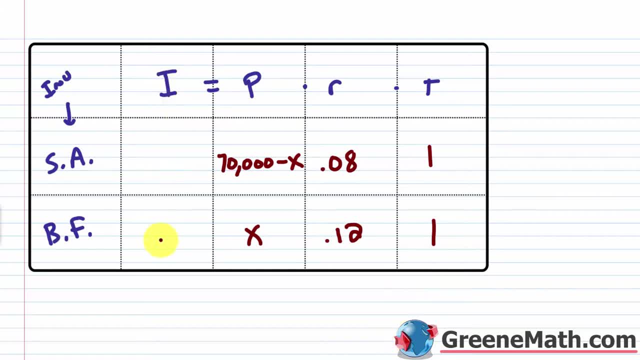 for kind of completeness. So we know that I, the simple interest earned, is the product of the principal times the rate, times the time. So at the bottom it's pretty easy. I would just have 0.12 X. for this guy right here It's kind of hard to fit this, but we're going to have 0.08 times the. 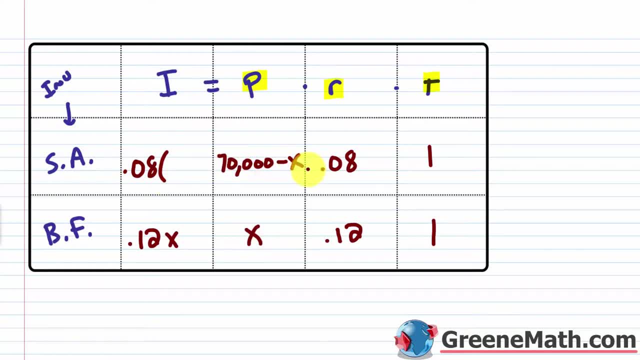 quantity: 70,000 minus X. So let me kind of scooch this part up So it's out of the way. So I'm going to put 70,000 minus X, just going to bleed into the next column. I can extend the column but it's. 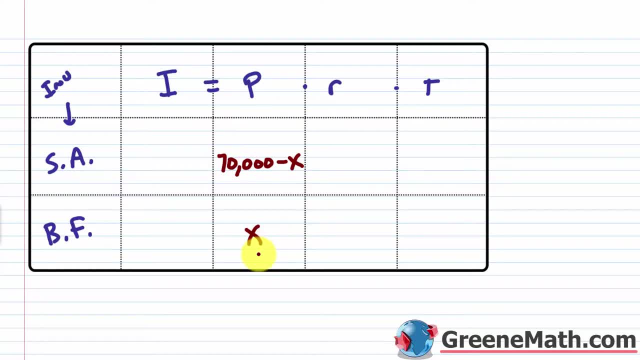 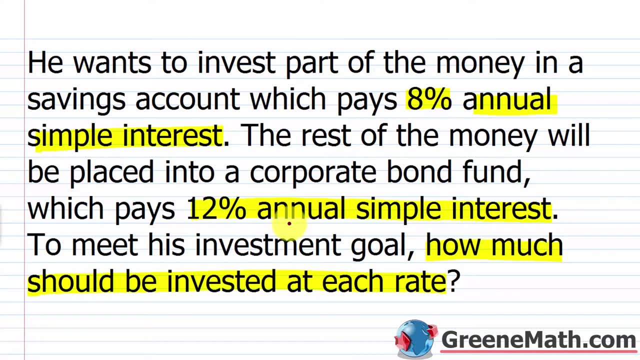 Now the rate is given to us in the problem. It says the savings account pays 8% annual simple interest And it says the corporate bond fund pays 12% annual simple interest. So the savings account again is 8% or 0.08 as a decimal. 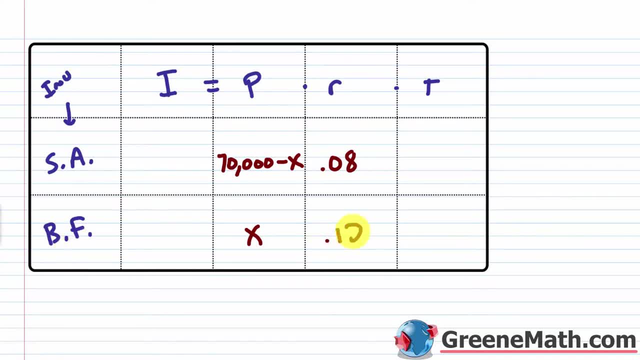 The bond fund is 12% or 0.12 as a decimal. Now what about the time? Well, basically, we're dealing with a scenario where the time is just going to be 1.. So if we go back up, you can see that it basically says in the first part of the problem. 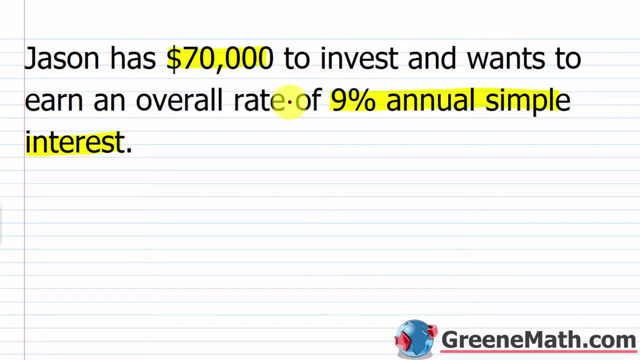 Jason has $70,000 to invest and wants to earn an overall rate of 9% annual, which is yearly, simple interest. So what are we doing for one year, right? One year period, So we can go back down and just put a 1 for each time period. 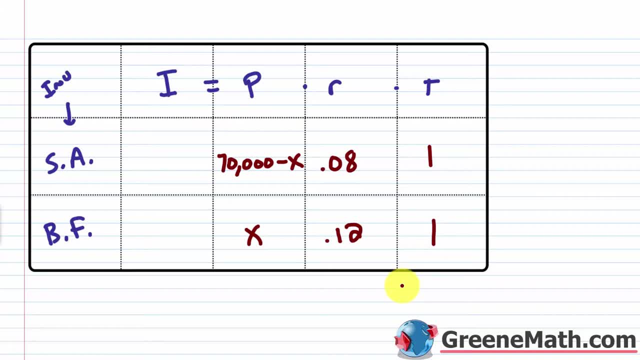 You can basically get rid of it, because multiplying by 1 just leaves something unchanged, right, But we'll just leave it there for kind of completeness. So we know that I, the simple interest earned, is the product of the principal times the rate times the time. 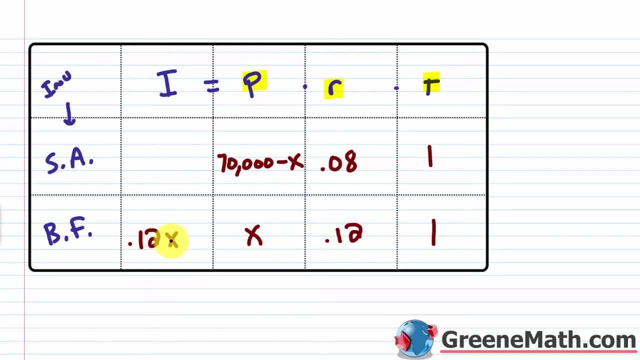 So at the bottom it's pretty easy. I would just have 0.12X For this guy right here. it's kind of hard to fit this, but we're going to have 0.08 times the quantity, 70,000 minus X. 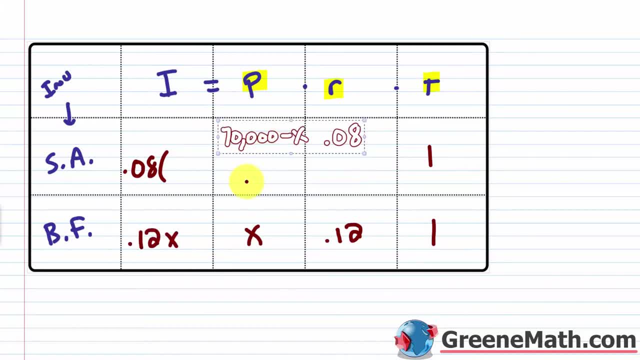 So let me kind of scooch this part up so it's out of the way. So I'm going to put 70,000 minus X, Just going to bleed into the next column. I can extend the column, but it's going to kind of make everything go crazy. 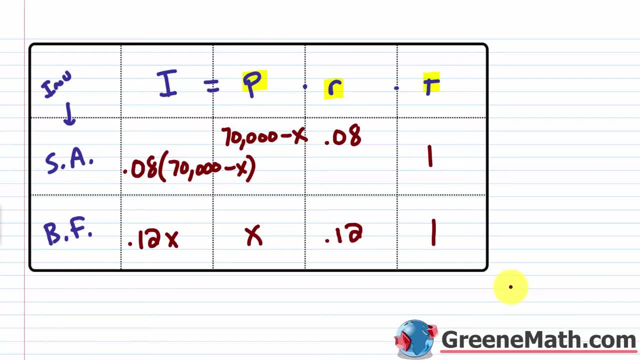 So let's just leave it like that And we can now kind of think about how we can use this information. So I have the simple interest earned from the savings account, which is 0.08 times the quantity 70,000 minus X. 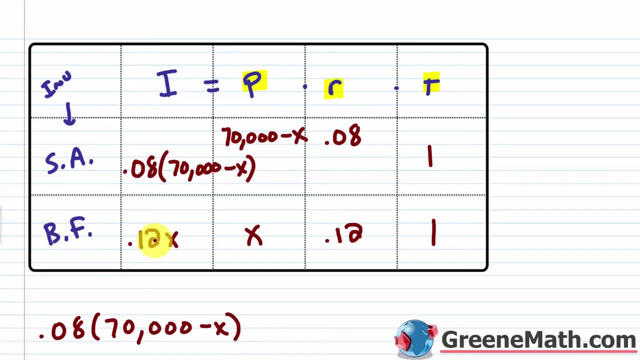 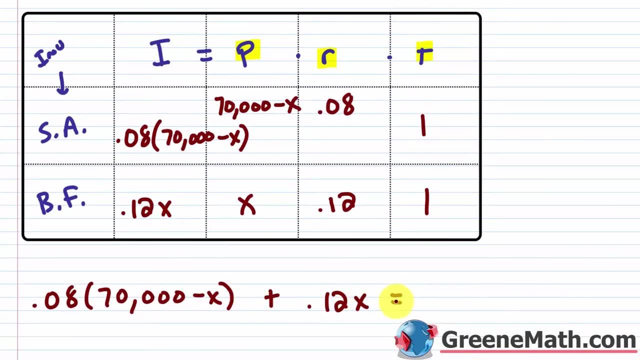 And then I have the simple interest earned from the corporate bond fund, which is 0.12X. So if I sum these amounts together, this needs to be equal to what? Well, again, it tells us that he has $70,000 to invest. 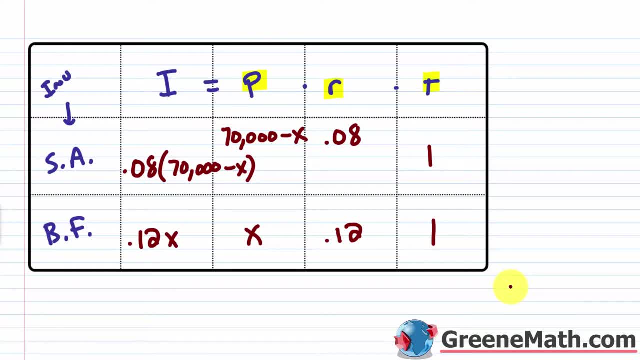 going to kind of make everything go crazy, So let's just leave it like that And we can now kind of think about how we can use this information. So I have the simple interest earned from the savings account, which is 0.08 times the quantity 70,000 minus X, And then I have the 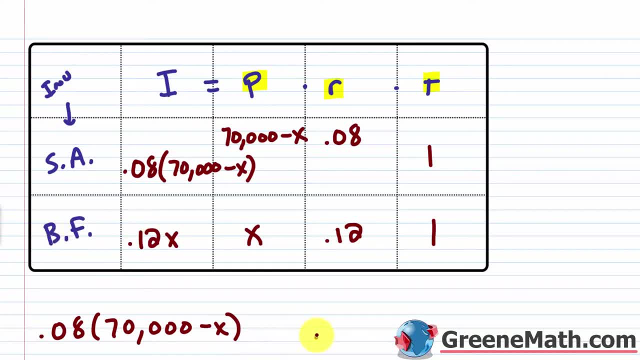 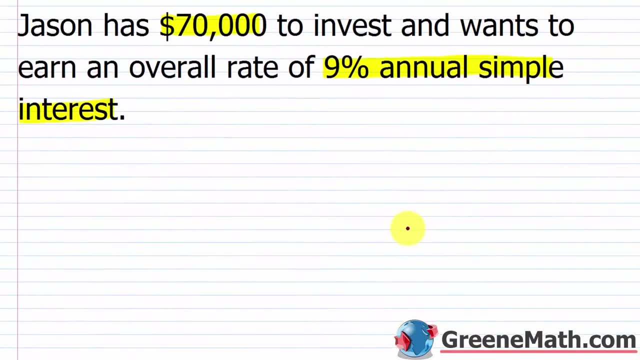 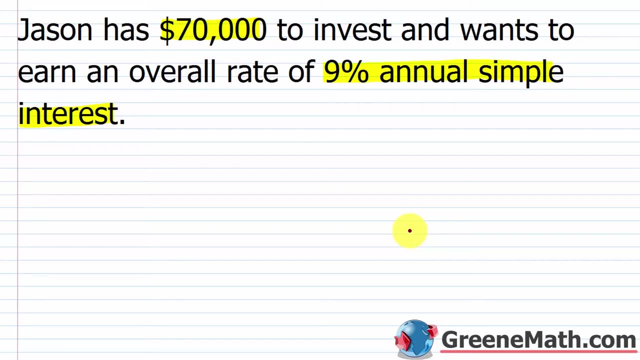 simple interest earned from the corporate bond fund, which is 0.12 X. So if I sum these amounts together, this needs to be equal to what? Well, again, it tells us that he has $70,000 to invest and he wants to earn an overall rate of return of 9%. So the sum of the simple interest from those two investments has got to be equal to 0.08.. And then I have the simple interest earned from the savings account, which is 0.08 times the quantity 70,000 minus X. And then I have the simple interest earned from the corporate bond fund, which is 0.12 X. And if I sum these aspects together, 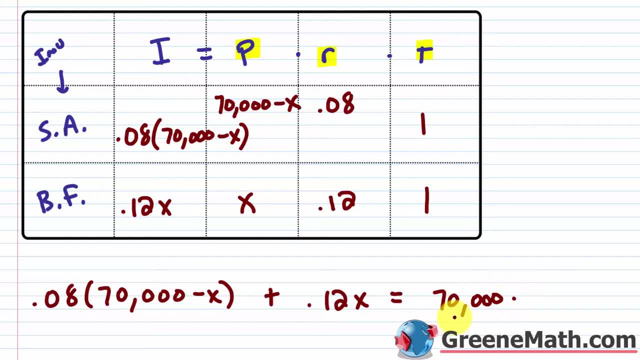 this needs to be equal to the 20,000 times the black money in the first turn. So if I sum these out again, let's just go back. And now I can just similar it all, keeping myself here in target. So 0.08 times the quantity 70,000.. And so here, in the current situation, 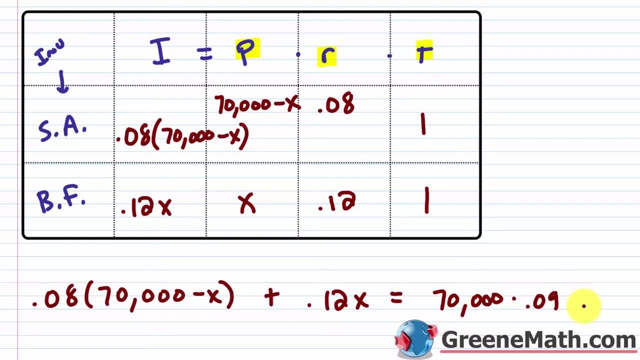 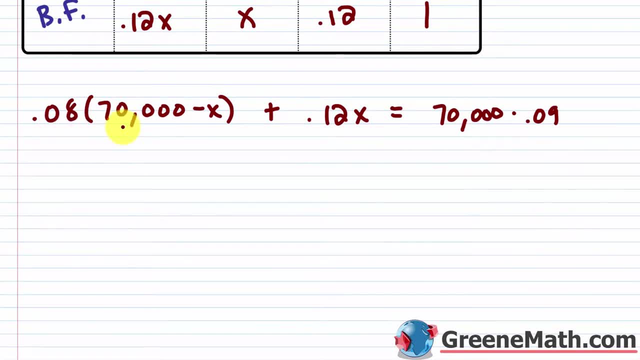 I changed it down with a period and I have a long term審uring And I'm just going to leave it as it is only just addition, but I'm going to leave this basis. with that, This becomes the mon masc. Well, I cut run-in. 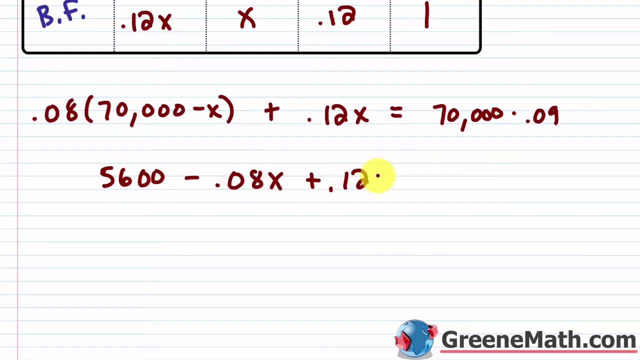 So here I can see how this works And I'm going to break it down And that structure here. I'm just going to leave it like that. This price here will be $1.2 and then $a$60. So 6,300.. So negative 0.08X plus 0.12X is going to be 0.04X. So you'd have 5,600 plus 0.04X. 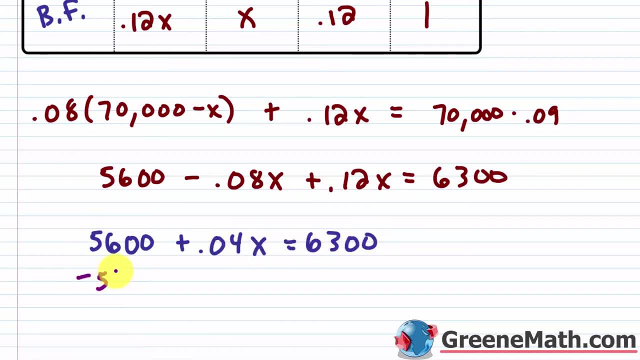 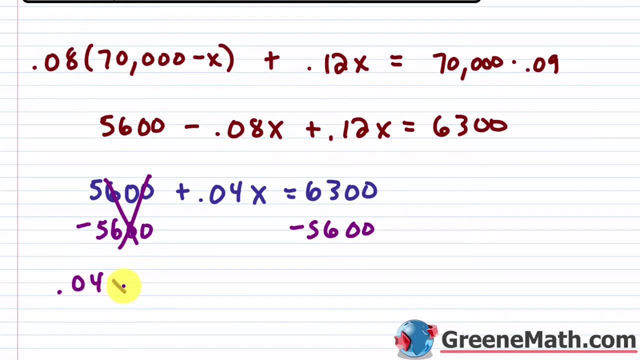 is equal to 6,300. Then I can subtract 5,600 away from each side of the equation. That'll cancel. If I have, 0.04X is equal to 6,300, minus 5,600 is 700. Okay. 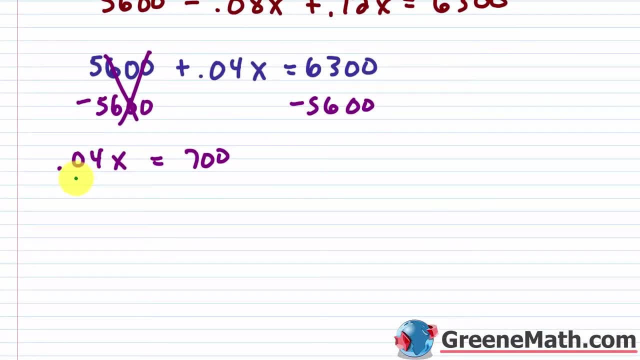 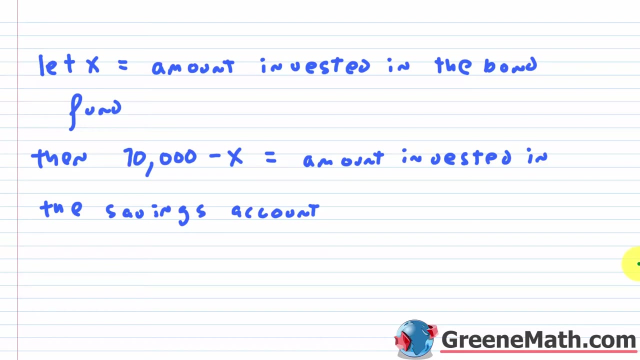 So the last step here to get X by itself is to divide both sides by 0.04.. I'll get: X is equal to 17,500.. Okay, So let's take this back up. So this is where you really need to again think about a sentence you can write, because you don't just put: X equals 17,500. 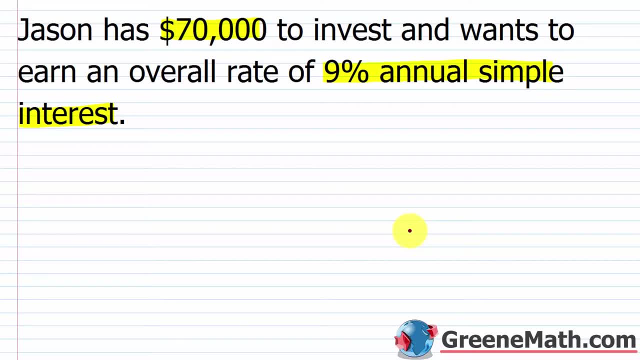 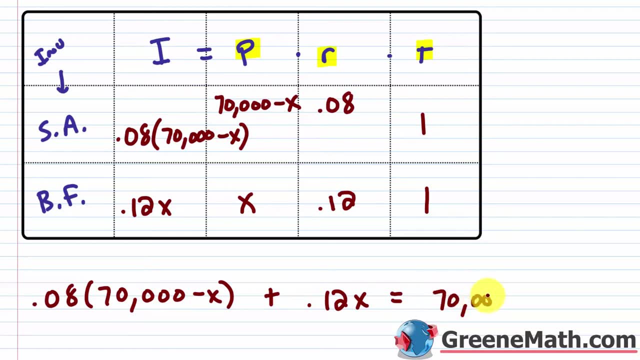 and he wants to earn an overall rate of return of 9%. So the sum of the simple interest from those two investments has got to be equal to 70,000, which is the principal times, the rate, which is 0.09,. 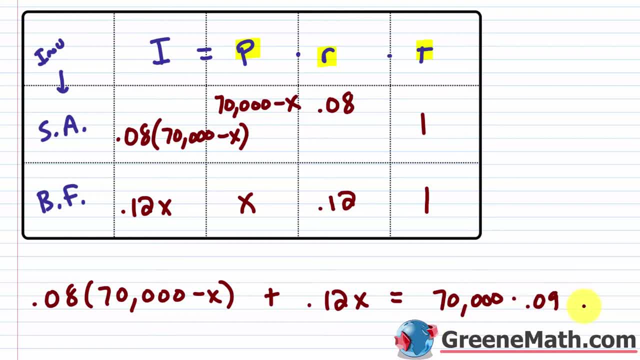 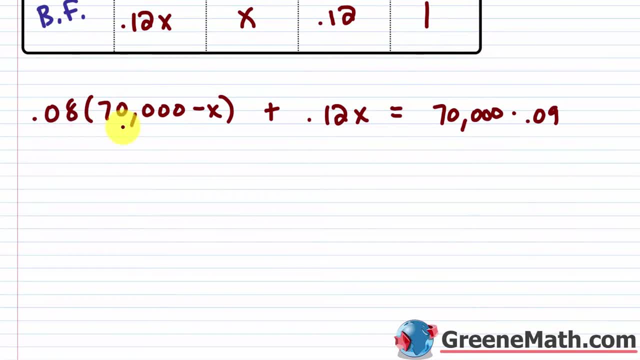 times the time, which is 1.. Okay, so you can just leave that off. So let's go through. We've set up our equation now and let's just solve this guy. So 0.08 times 70,000 is 5,600.. 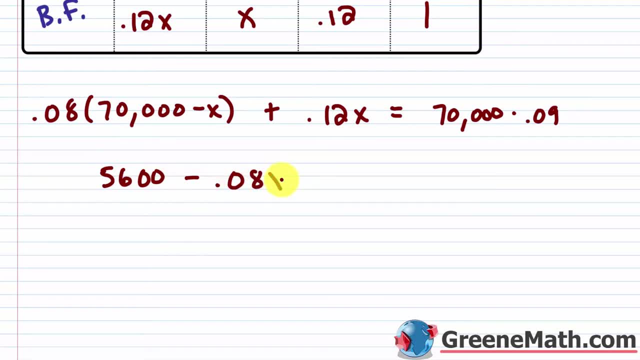 Then minus you'd have 0.08 times X, then plus 0.12X, And this equals 70,000 times 0.09, is 6,300.. So 6,300.. So negative 0.08X plus 0.12X. 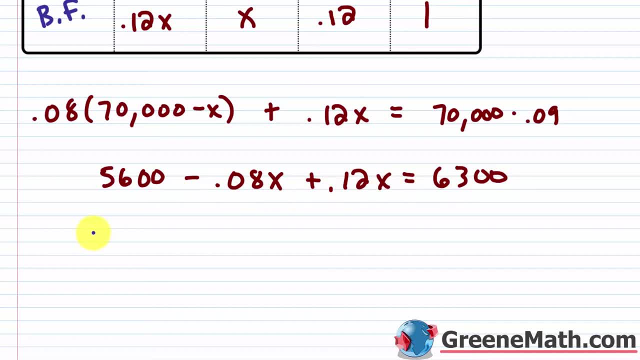 is going to be 0.04X, So you'd have 5,600 plus 0.04X is equal to 6,300.. Then I can subtract 5,600 away from each side of the equation. That'll cancel. 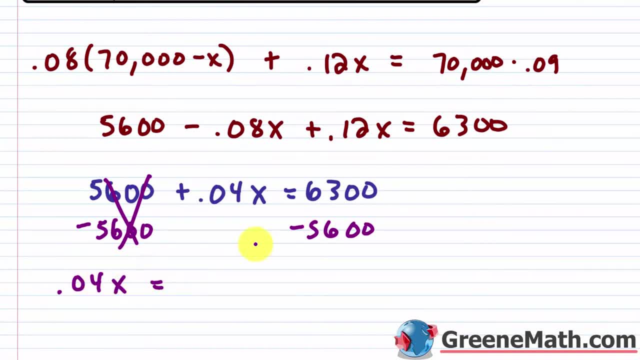 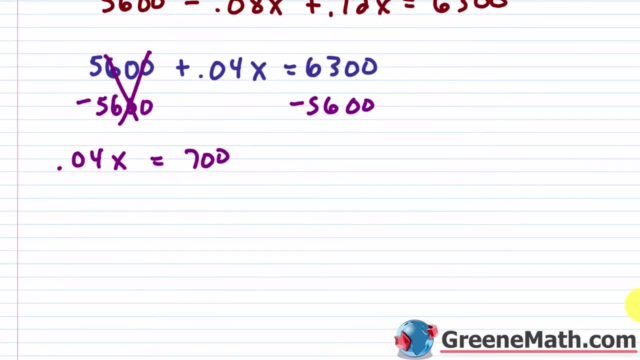 If I have, 0.04X is equal to 6,300, minus 5,600 is 700.. Okay, So the last step here to get X by itself is to divide both sides by 0.04.. I'll get: X is equal to 17,500. 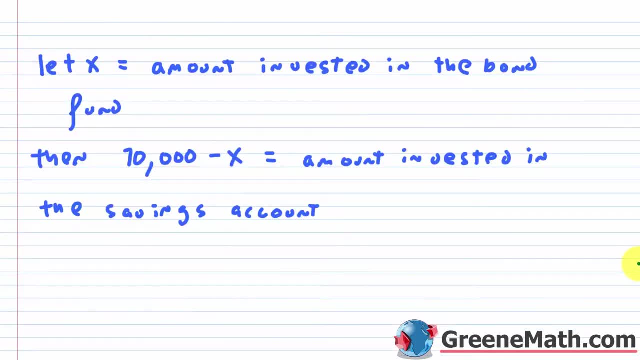 Okay, so let's take this back up. So this is where you really need to again think about a sentence you can write, because you don't just put X equals 17,500 and turn in the test. Okay, you've got to make sense of it in terms of the problem. 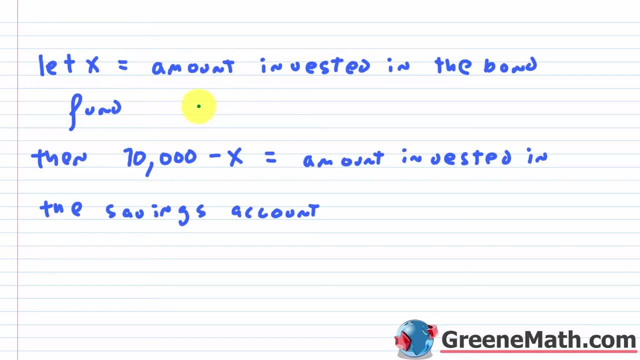 So X was the amount invested in the bond fund, So we know that's $17,500.. Then 70,000 minus X, so 70,000 minus 17,500, or 52,500.. 52,500 is the amount invested in the savings account. 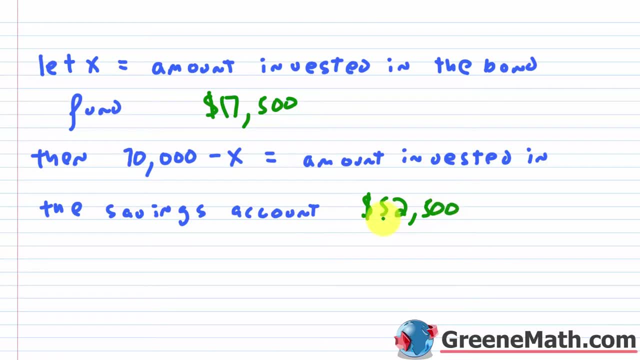 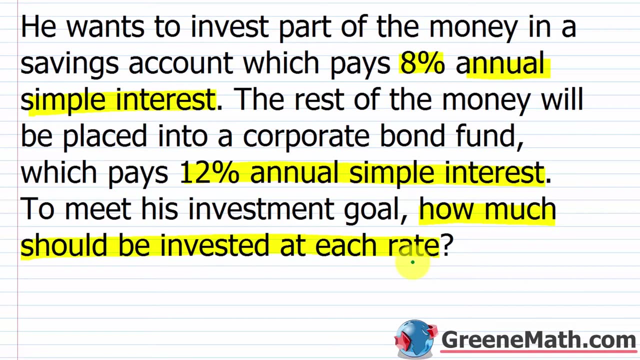 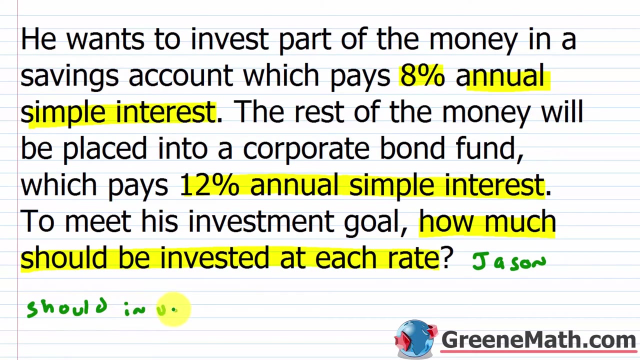 So this is 52,500.. So now we're ready to go back up and answer this in terms of the question being asked: How much should be invested at each rate? Well, we can say that Jason should invest $52,500 in the savings account. 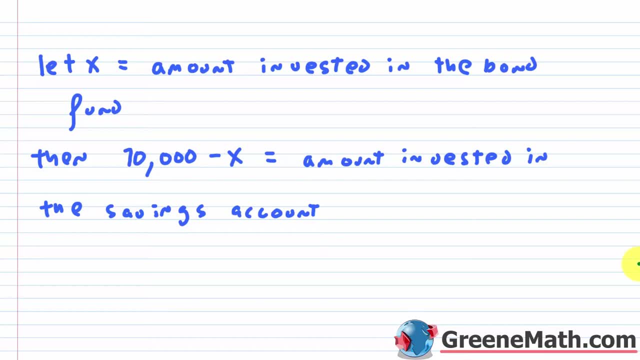 and turn in the test. Okay, You've got to make sense of it in terms of the problem. So X was the amount invested in the bond fund, So we know that's $17,500.. Okay Then, $70,000 minus X. so $70,000 minus $17,500, or $52,500, is the amount invested in the savings account. 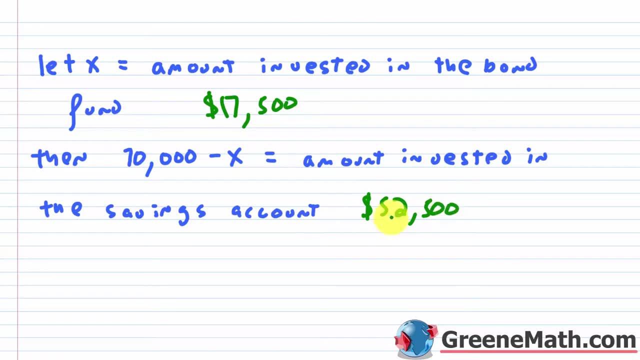 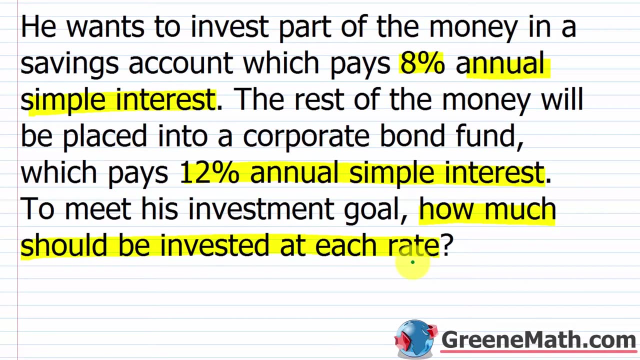 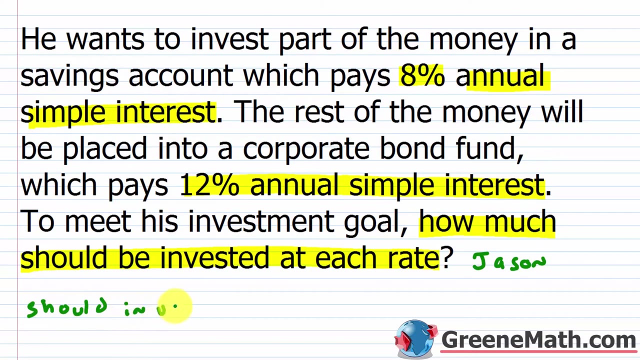 So this is $52,500.. So now we're ready to go back up and answer this in terms of the question being asked: How much should be invested at each rate? Well, we can say that Jason should invest $52,500 in the savings account and $17,500 in the bond fund. 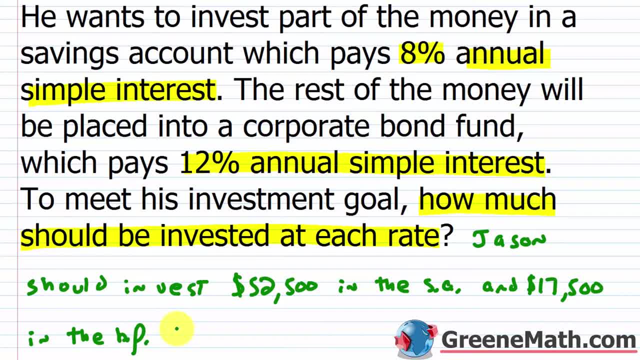 Okay, So Jason should invest $52,500 in the savings account and $17,500 in the bond fund. Okay, So how can we check this to make sure that it's accurate? Well, again, if we go back to the beginning of the problem, Jason has $70,000 to invest. 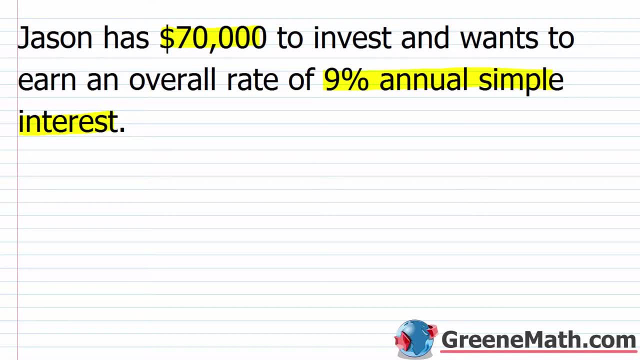 So let's check that first. Is the amount that he put in the bond fund plus the amount that he put in the savings account equal to $70,000?? $52,500 plus $17,500 does equal $70,000.. So that part is a check. 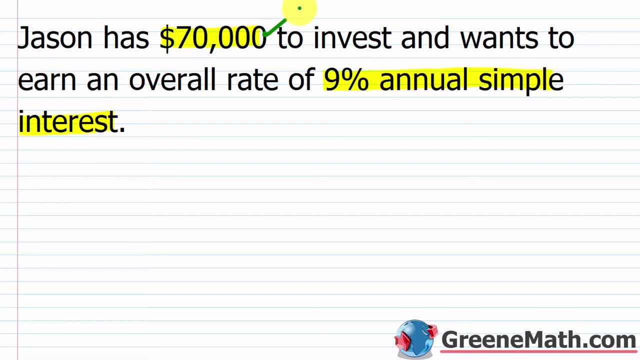 So this is a check. This is good to go. Now he wants to earn an overall rate of return of 9% annual simple interest. So $70,000 earning 9% annual simple interest would mean that he's earning $6,300 a year in annual simple interest. 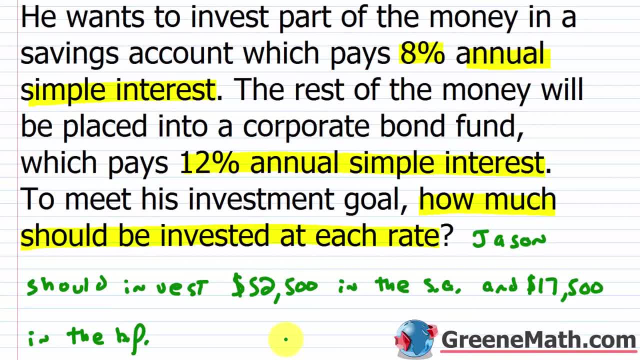 Okay. So let's check that against what he's going to earn with the two investments. So he's going to earn 8% with the savings account and he's going to earn 12% with the corporate bond fund. So let's go back up. 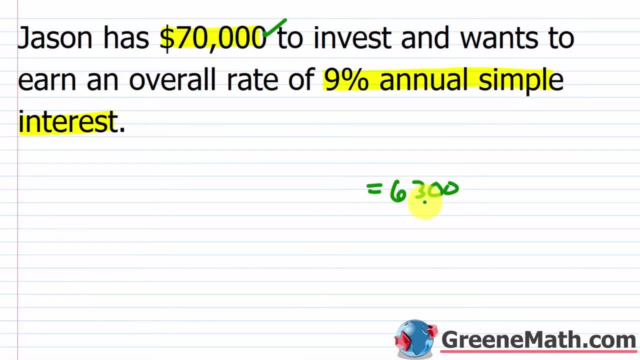 Again, we have $6,300.. We have $6,300 as the amount that he's earning and we're going to check. So we have $52,500 in the savings account, which is earning 8%. So that would give me $4,200 a year. 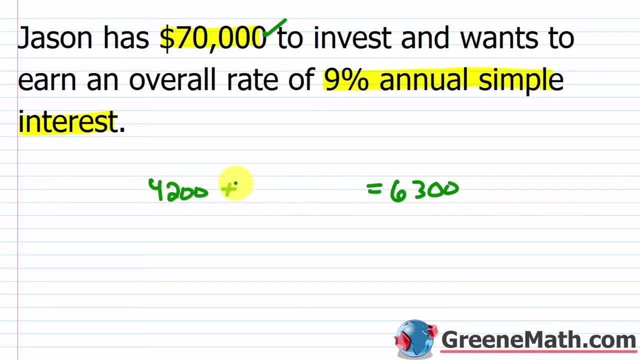 And then he put $17,500 in the bond fund, which is earning 12%, So that would give him $2,100.. Okay, So if you sum these two amounts together, the $4,200 he gets from the savings account and the $2,100 he gets from the bond fund- 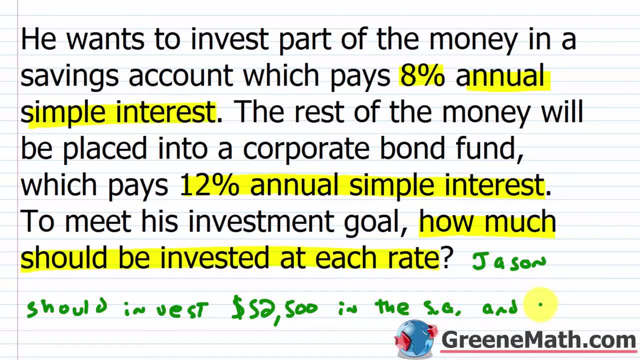 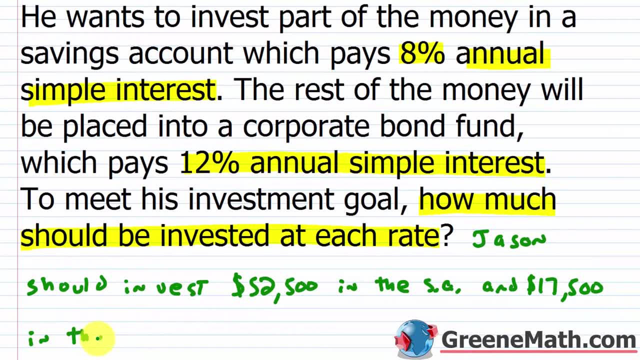 And $17,500 in the bond fund. Okay, So Jason should invest $52,500 in the savings account and $17,500 in the bond fund. Okay, So how can we check this to make sure that it's accurate? Well, again, if we go back to the beginning of the problem, Jason has $70,000 to invest. 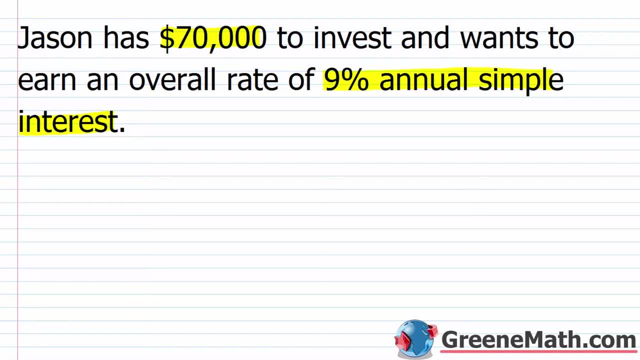 So let's check that first. Is the amount that he put in the bond fund plus the amount that he put in the savings account equal to 70,000?? 52,500 plus 17,500 does equal 70,000.. So that part is a check. 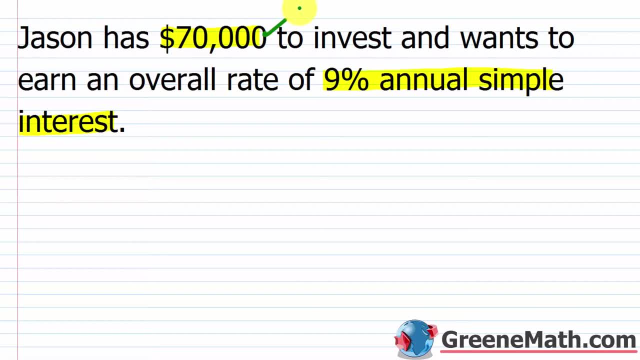 So this is good to go. Now he wants to earn an overall rate of return of 9% annual simple interest. So 70,000 earning 9% annual simple interest would mean that he's earning $6,300 a year in annual simple interest. 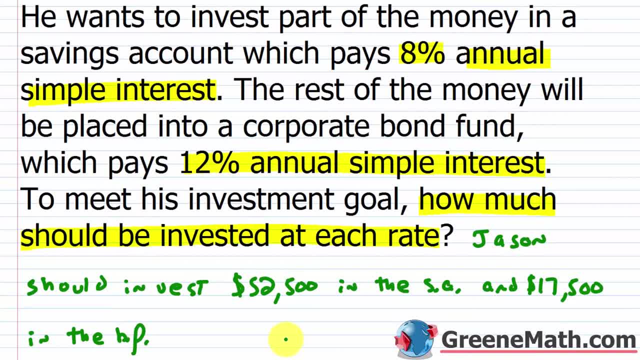 Okay. So let's check that against what he's going to earn with the two investments. So he's going to earn 8% with the savings account and he's going to earn 12% with the corporate bond fund. So let's go back up. 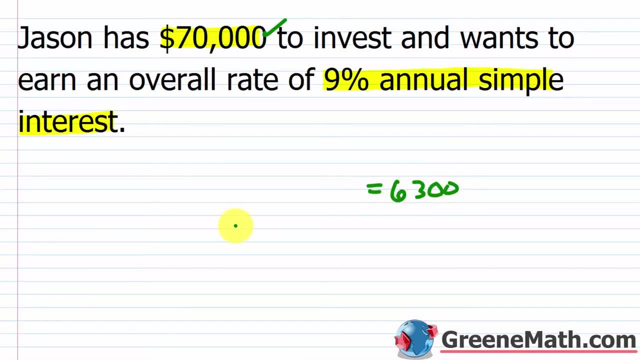 Again, we have 6,300 as the amount that he's earning And we're going to check. So we have 52,500 in the savings account, which is earning 8%. So that would give me $4,200 a year. 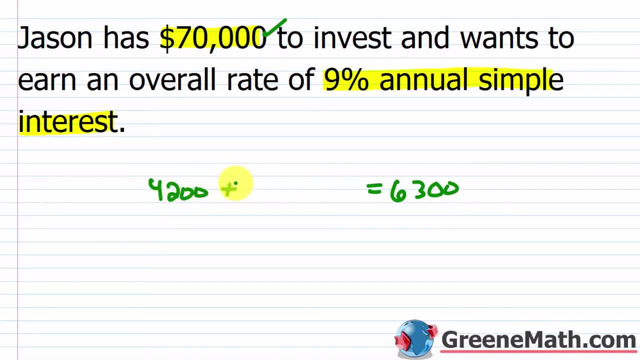 Okay, So we have 52,500 in the bond fund, which is earning 12%, So that would give him $2,100.. Okay, So if you sum these two amounts together- the 4,200 he gets from the savings account and the $2,100 he gets from the bond fund- he's going to get the $6,300 he's looking for in annual simple interest. 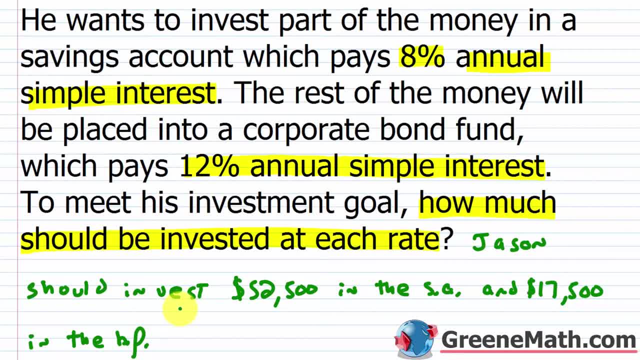 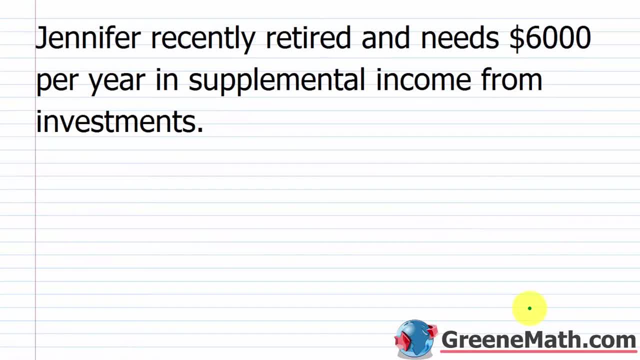 So we can say this problem does check out. And again, Jason should invest 52,500 in the savings account and $17,500 in the bond fund. All right, Let's take a look at one more of these. So Jennifer recently retired and needs $6,000 per year in supplemental income from investments. 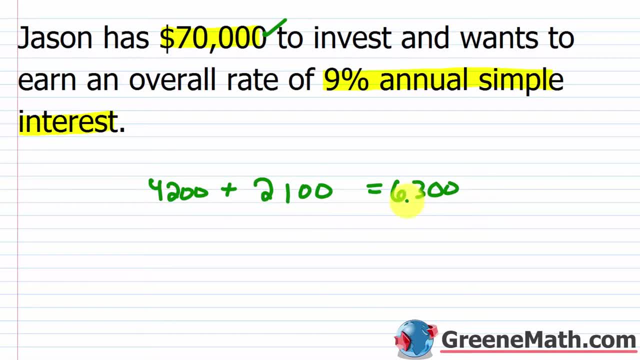 he's going to get the $6,300.. So he's going to earn 12% with the savings account and he's going to earn 12% with the bond fund. So he's going to earn 12% with the savings account and he's going to earn 12% with the bond fund. 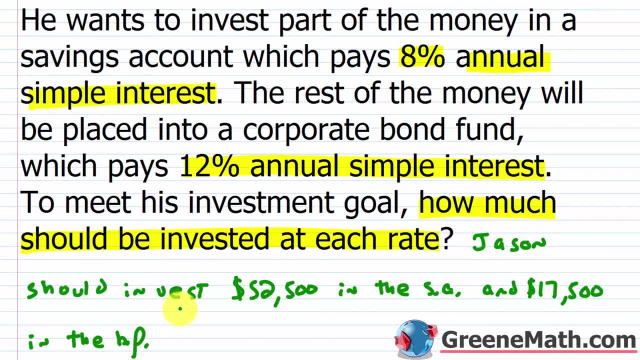 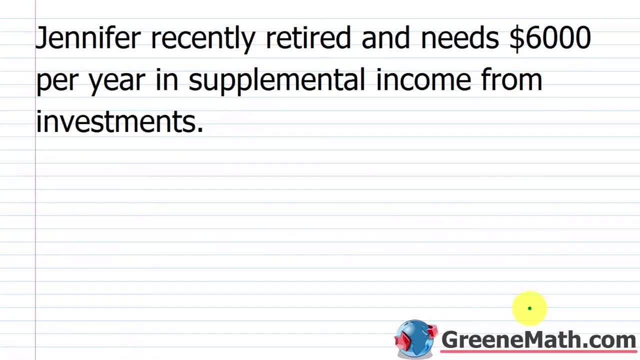 So we can say this problem does check out. And again, Jason should invest $52,500 in the savings account and $17,500 in the bond fund. All right, Let's take a look at one more of these. So Jennifer recently retired and needs $6,000 per year in supplemental income from investments. 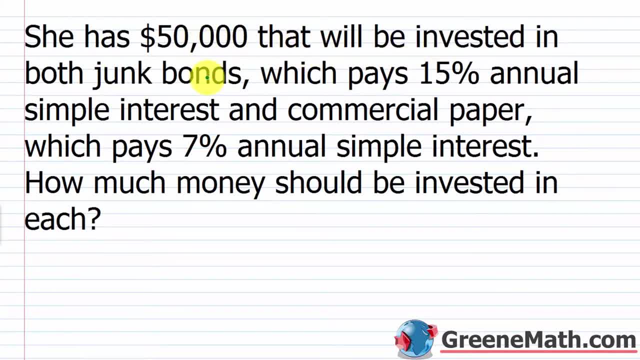 So she has $50,000 that will be invested in both junk bonds, which pays 15% annual simple interest, and commercial interest, And commercial paper, which pays 7% annual simple interest. How much money should be invested in each? 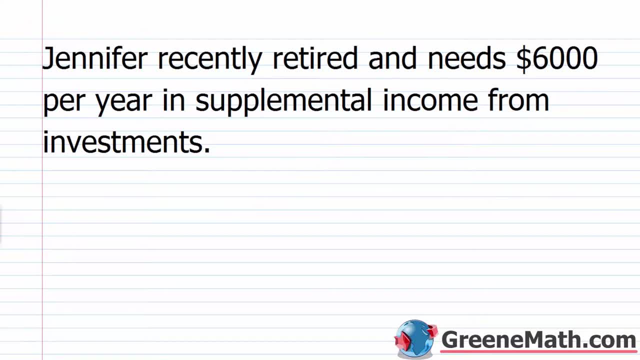 So again, let's go back up Again. she retired and needs $6,000.. $6,000 per year in supplemental income, So she needs $6,000.. She has $50,000.. So that's going to be her principal. 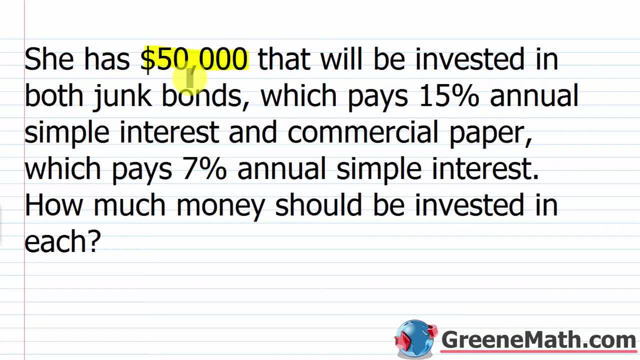 And that will be invested in again both junk bonds. The junk bonds are going to pay 15% annual simple interest And the commercial paper is It's going to pay 7% annual simple interest. So how much money should be invested in each? 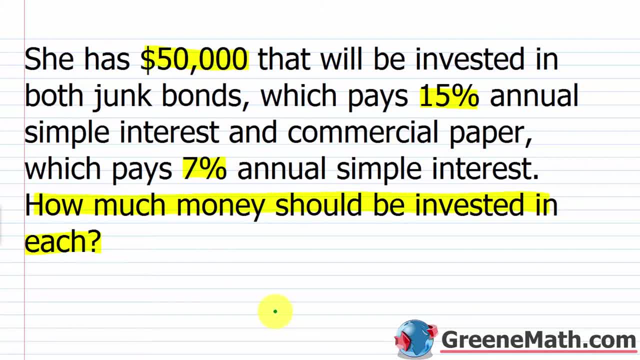 Okay, That's what we're trying to answer. So let's let a variable like X be the amount that she invests in. Let's just say the commercial paper. You can put it as either, but I'm just going to go with the commercial paper. 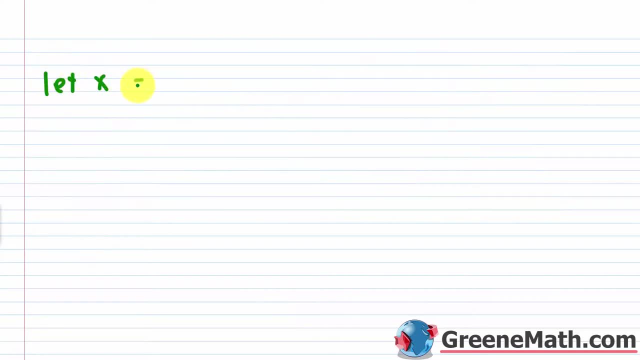 So let's go ahead and do that real quick. So let's let X be equal to the amount invested in commercial. And let me just abbreviate that because it's kind of hard to write all that, So I'm just going to put commercial paper: C period, P period. 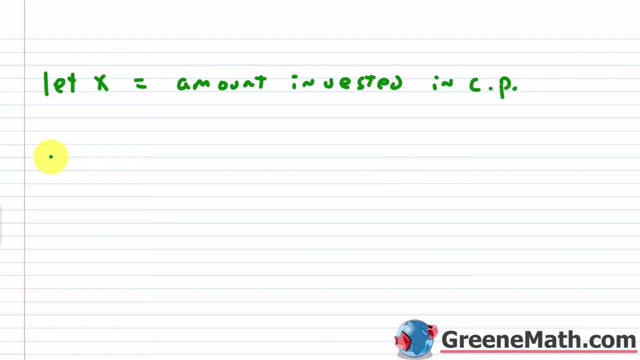 So then, what can we say about the amount that's put into junk bonds? Well, again, the total amount she's investing is $50,000.. So we can say then: $50,000 minus X is going to be the amount invested in junk bonds. 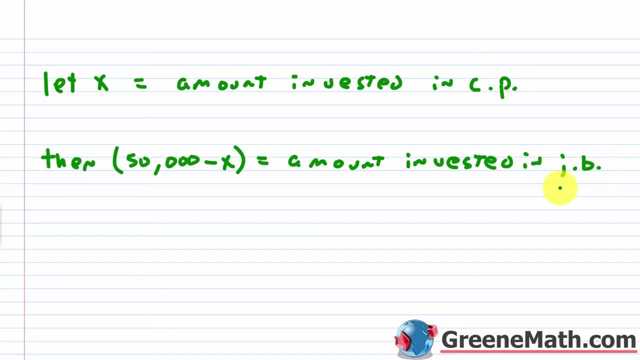 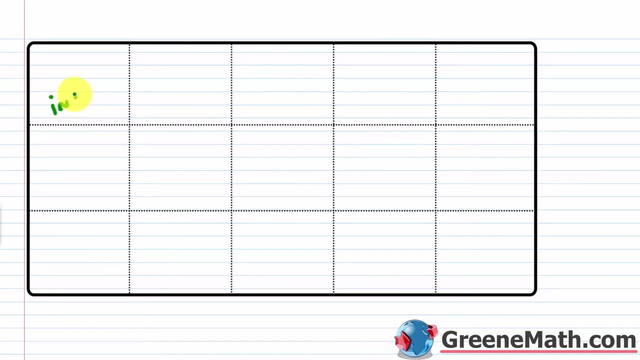 So I'll put J period, B period. Okay for junk bonds. So let's take this information to a table, just like we did in the last example. So for our investments, these are going to go down. You have your junk bonds and you have your 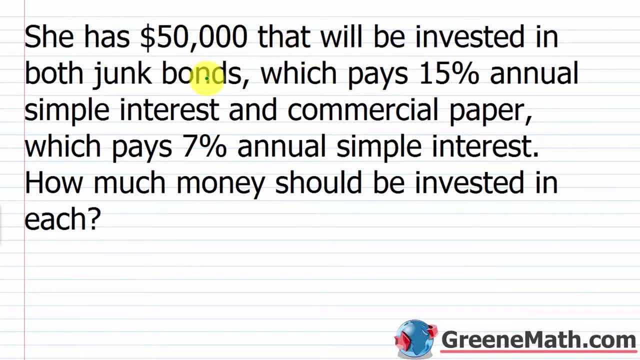 So she has $50,000 that will be invested in both junk bonds, which pays 15% annual simple interest, and commercial paper, which pays 7% annual simple interest. How much money should be invested in each? So again, let's go back up. 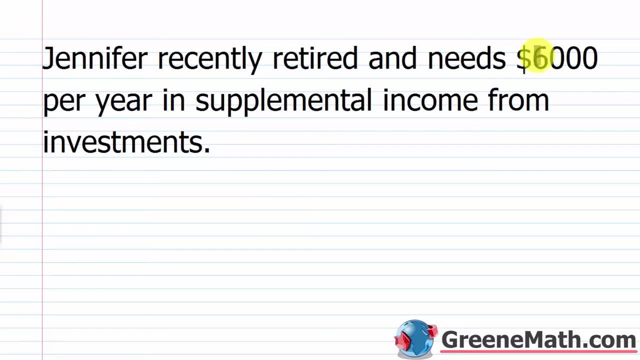 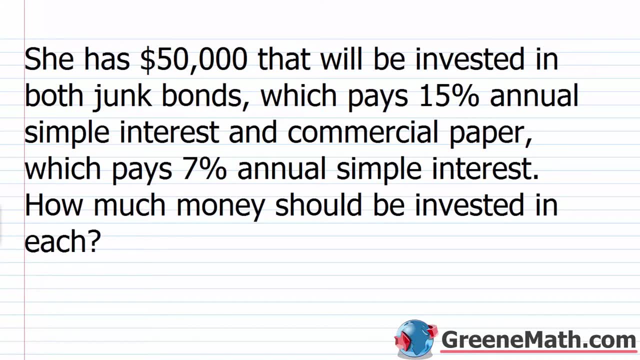 Again, she retired and needs $6,000.. $6,000.. $6,000 per year in supplemental income, So she needs $6,000.. She has $50,000.. So that's going to be her principal And that will be invested in again both junk bonds. 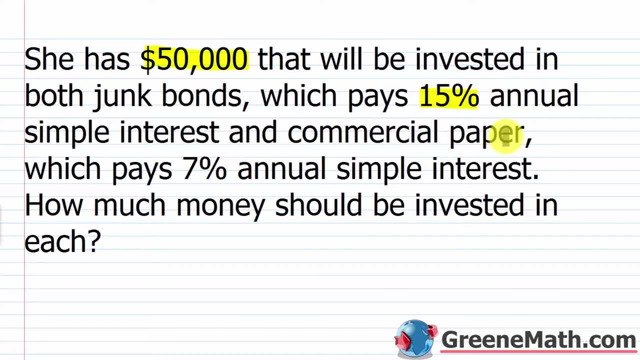 The junk bonds are going to pay 15% annual simple interest and the commercial paper is going to pay 7% annual simple interest. So how much money should be invested in each? Okay, That's what we're trying to answer. So let's let a variable like X be the amount that she invests in. 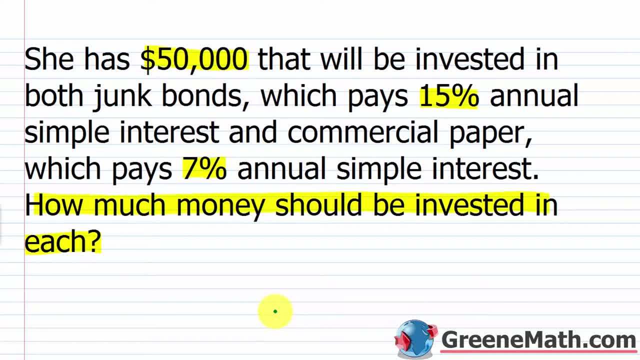 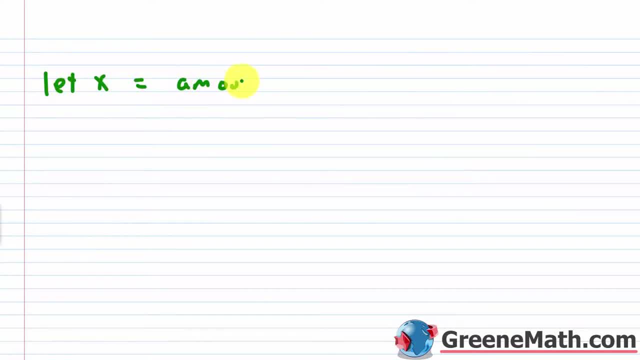 Let's just say the commercial paper. You can put it as either, but I'm just going to go with the commercial paper. So let's go ahead and do that real quick. So let's let X be equal to the amount invested in commercial. 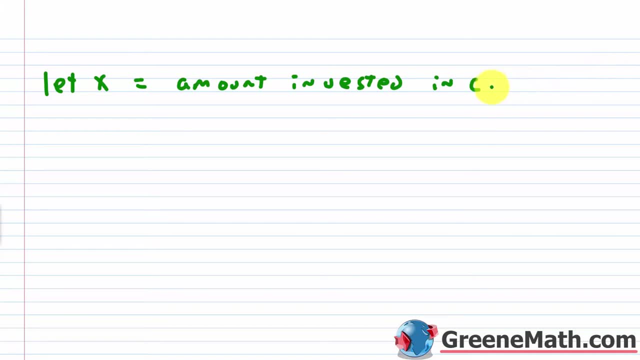 And let me just abbreviate that because it's kind of hard to write all that, So I'm just going to put commercial paper as CP. So then, what can we say about the amount that's put into junk bonds? So again, the total amount she's investing is $50,000.. 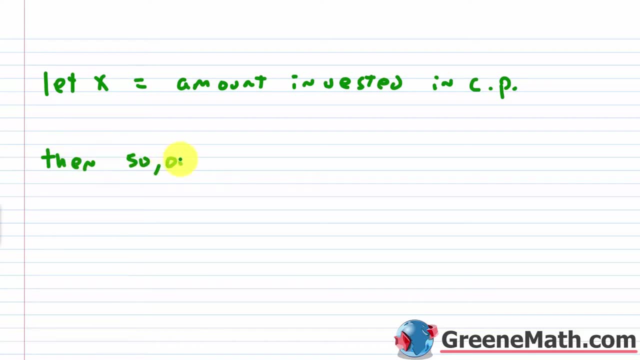 So we can say then $50,000 minus X is going to be the amount invested in junk bonds. So I'll put JB Okay For junk bonds. So let's take this information to a table, just like we did in the last example. 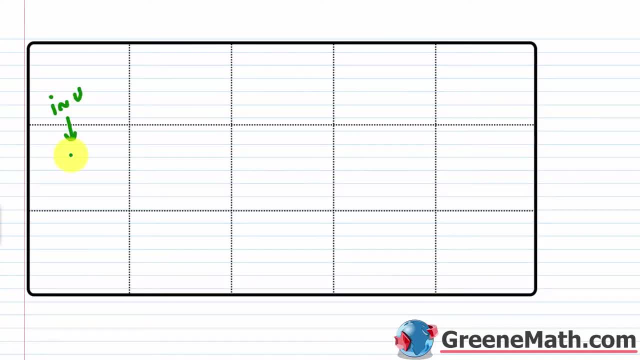 So for our investments, these are going to go down. You have your junk bonds and you have your commercial paper. Okay, And again we have our simple interest formula. I, the simple interest earned, is equal to P, the principal times R, the rate times T, the time. 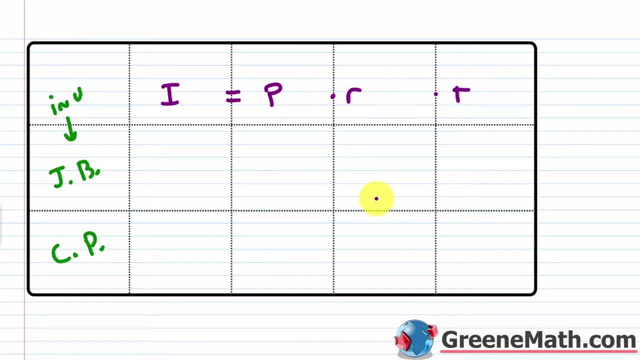 Okay, Now, in this case we're talking about an annual basis, So time is just going to be one for each of these, Okay, So very, very simple. For the rate, we know that for the junk bonds they pay 15%. 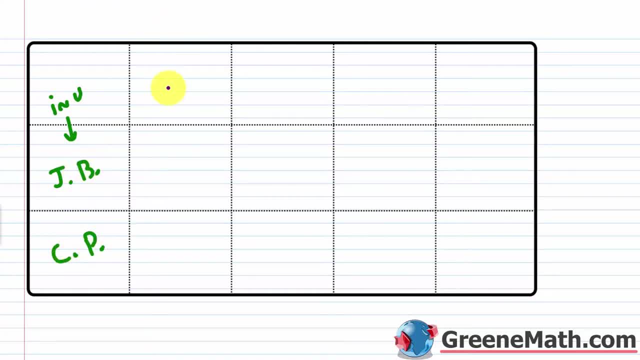 commercial paper. Okay, And again we have our simple interest formula I. the simple interest earned is equal to P, the principal, times R, the rate, times T, the time. Okay, Now, in this case we're talking about an annual basis, So time is just going to be one for each of these, Okay So? 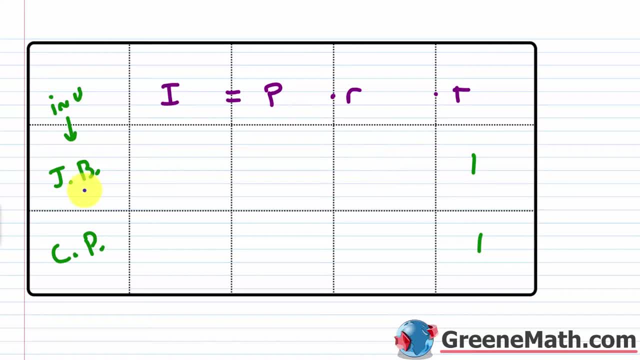 very, very simple For the rate. we know that for the junk bonds they pay 15%, So 0.15.. We know for the commercial paper it pays 7%, So 0.07.. Again, you've always got to express the rate as: 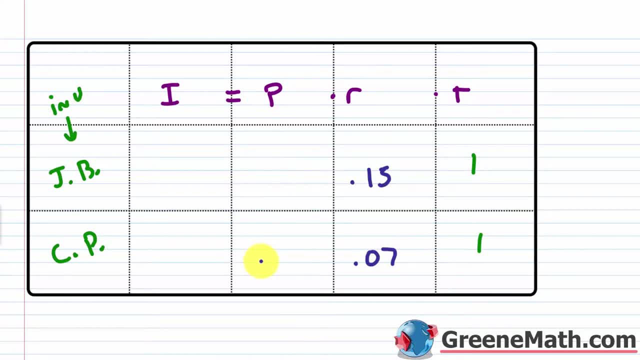 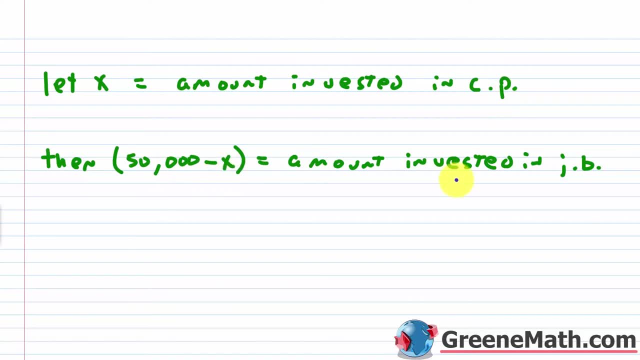 a decimal And then the principal or the amount invested in each of these. we just modeled that. We said X is the amount invested in the commercial paper and 50,000 minus X is the amount invested in the junk bonds. So the principal, or again the amount invested in the commercial paper. 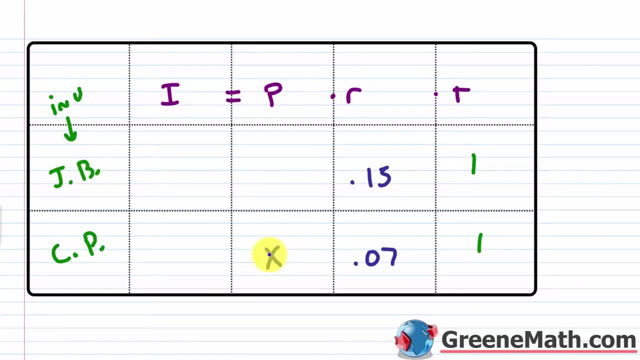 is X, And the amount invested in the junk bonds is going to be 50,000 minus X. Okay, So my simple interest earned again. all I've got to do is multiply in the rows. So I would have principal of 50,000 minus X times the rate of 0.15 times one, which really doesn't change anything. So 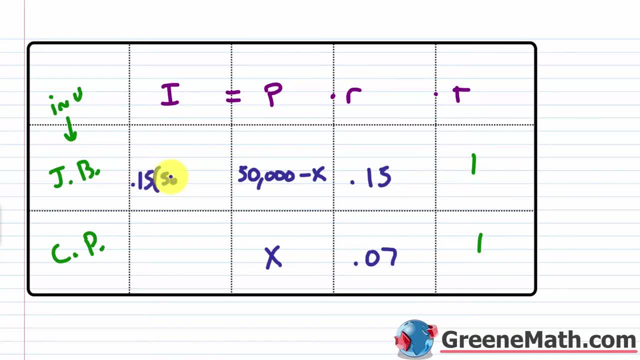 you basically have 0.15 times the quantity, 50,000 minus X. Again hard to kind of fit that in a And then over here. it's pretty easy for the commercial paper It's just going to be 0.07 times. 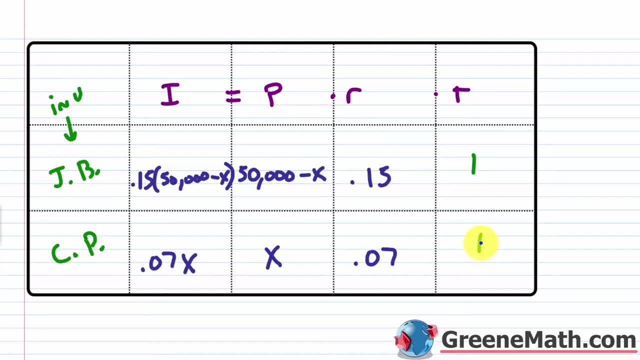 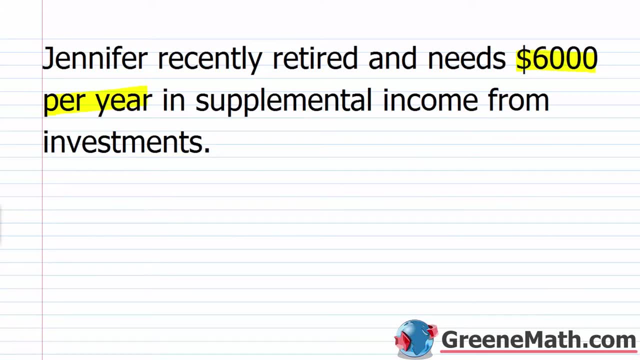 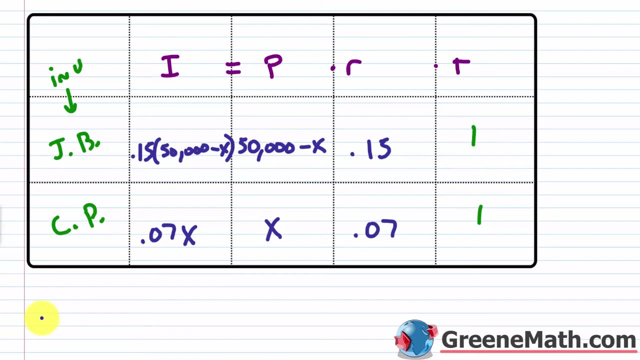 X. Again, you can multiply by one, but it doesn't really change anything. Now we are told that she wants to earn $6,000 per year in supplemental income from investments. Okay, So what do we know? We know that the interest she's going to earn from the junk bonds is 0.15 times the quantity. 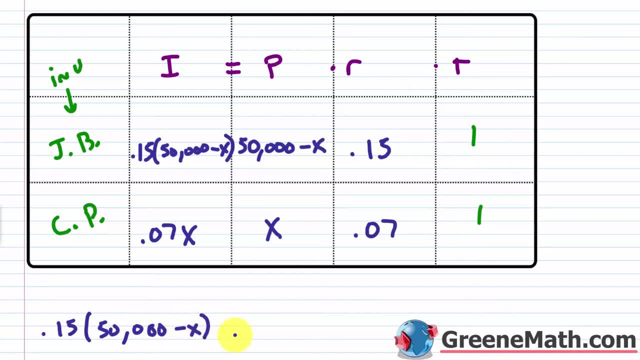 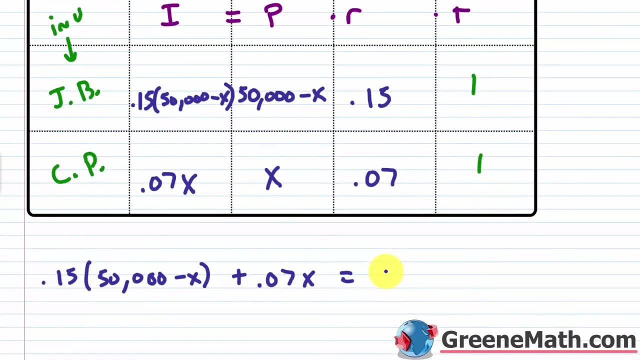 50,000 minus X, Then if we add that to the interest she's going to earn from the commercial paper, which is 0.07X, this has to be equal to 6,000.. Okay, Because that's what she needs to earn. 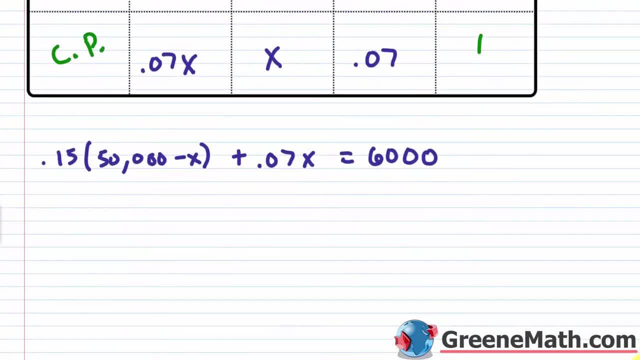 So let's go ahead and solve this equation Very, very easy: 0.15 times 50,000 is 7,500.. Then minus 0.15 times X is 0.15X. Then plus 0.07X again is equal to 6,000.. 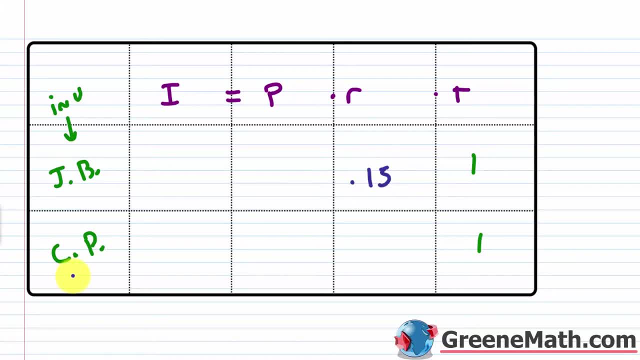 So 0.15.. We know for the commercial paper it pays 7%, So 0.07.. Again, you've always got to express the rate as a decimal And then the principal or the amount invested in each of these. we just modeled that. 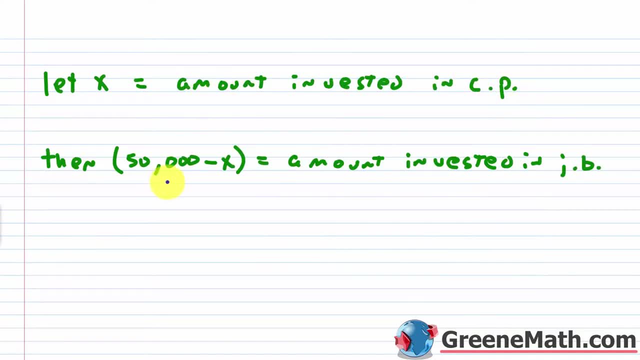 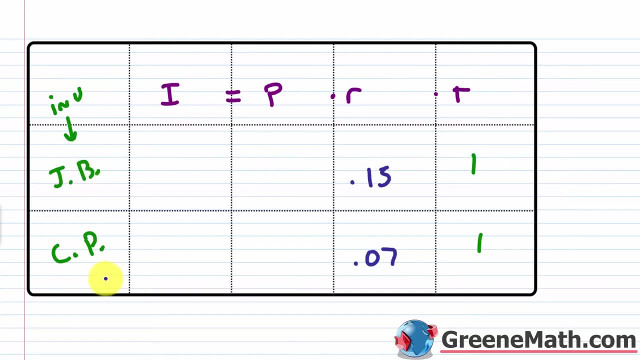 We said X is the amount invested in the commercial paper And $50,000 minus X is the amount invested in the junk bonds. So the principal, or again, the amount invested in the commercial paper is X And the amount invested in the junk bonds is going to be $50,000 minus X. 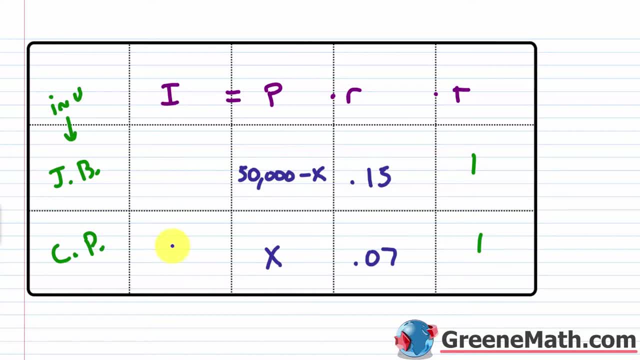 Okay, So my simple interest earned again. all I've got to do is multiply in the rows, So I would have principal of $50,000 minus X times the rate of 0.15 times 1,, which really doesn't change anything. 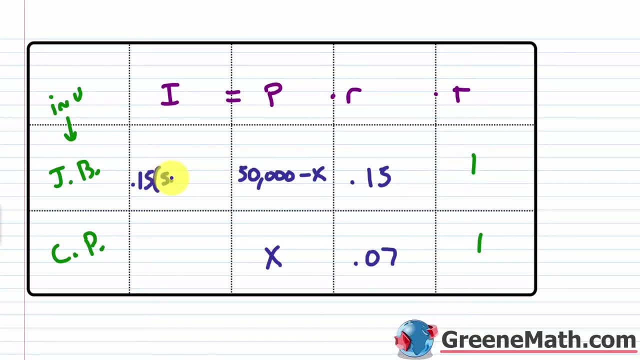 So you basically have 0.15 times the quantity, $50,000 minus X. Again, hard to kind of fit that in a column And then over here it's pretty easy for the commercial paper. It's just going to be 0.07 times X. 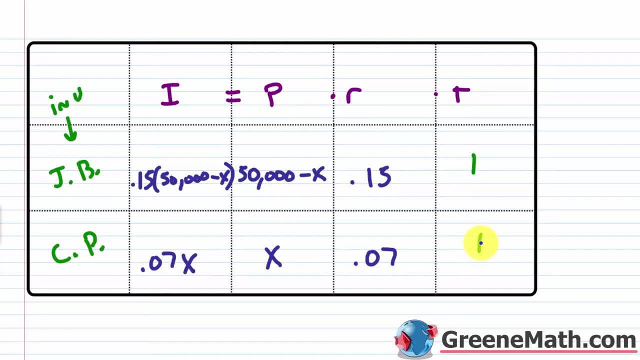 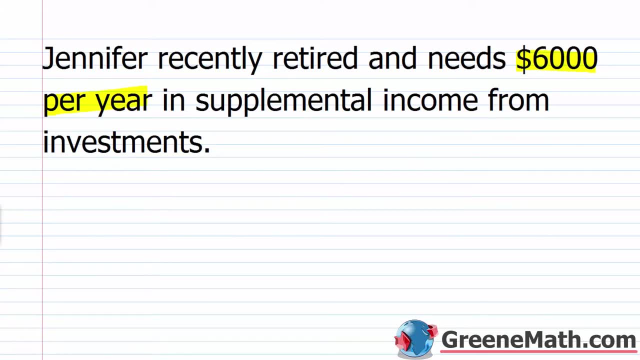 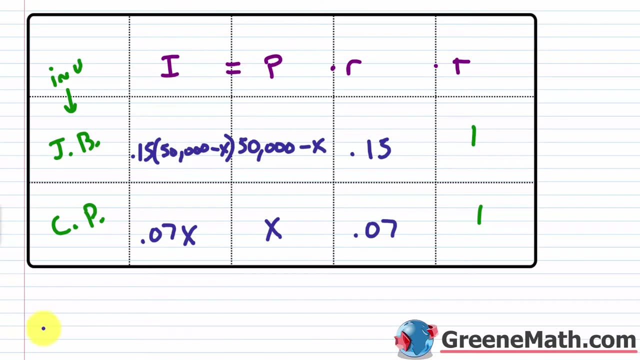 Again, you can multiply by 1,, but it doesn't really change anything. Now we are told that she wants to earn $6,000 per year in supplemental income from investments. Okay, So what do we know? We know that the interest she's going to earn from the junk bonds is 0.15 times the quantity: $50,000 minus X. 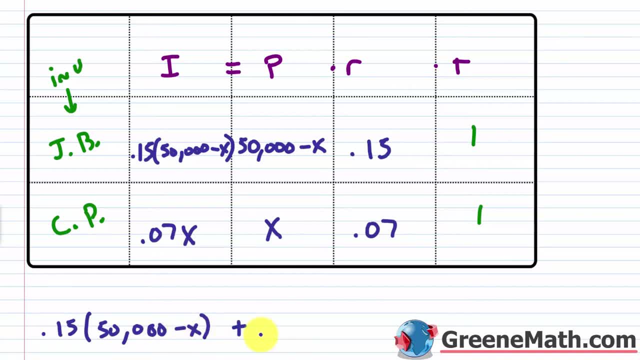 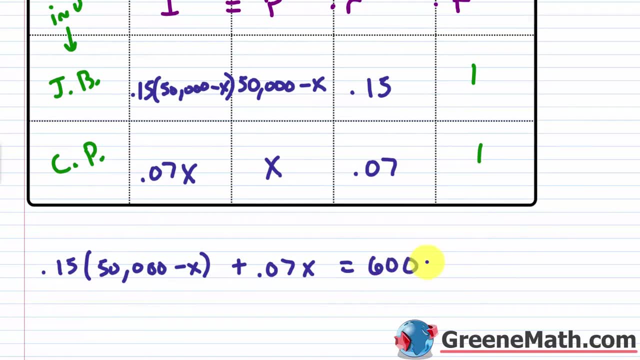 Then if we add that to the interest she's going to earn from the commercial paper, which is 0.07X, this has to be equal to $6,000.. Okay, Because that's what she needs to earn. So let's go ahead and solve this equation. 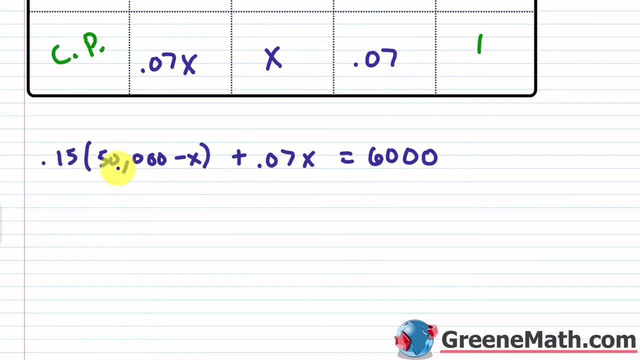 Very, very easy: 0.15 times $50,000 is $7,500.. Then minus 0.15 times X is 0.15X. Then plus 0.07X again is equal to $6,000.. 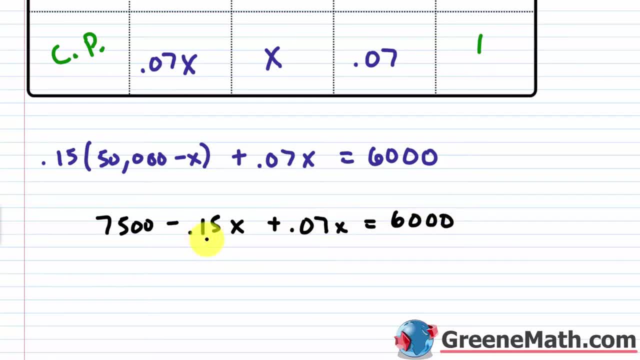 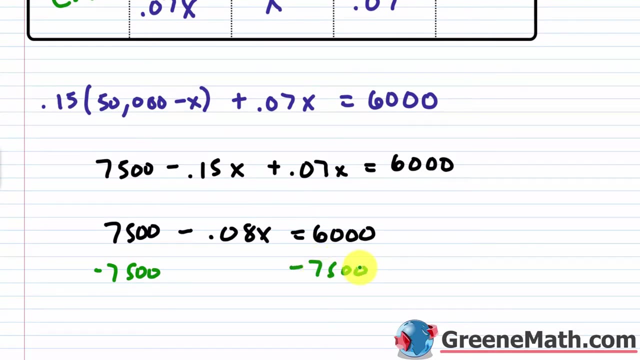 If we combine like terms here, you'd end up with negative 0.08X. So $7,500 minus 0.08X is equal to $6,000.. I'm going to subtract that. I'm going to subtract $7,500 away from each side of the equation. 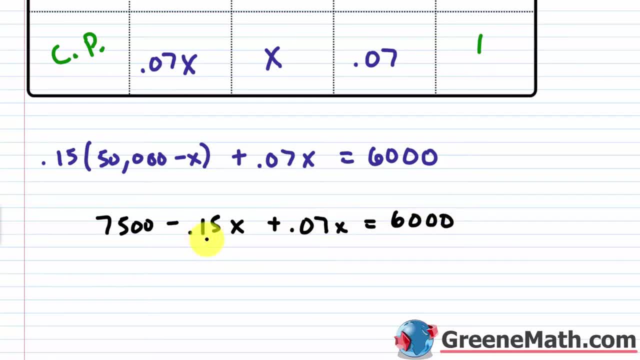 If we combine like terms here, you'd end up with negative 0.08X. so 7,500 minus 0.08X is equal to 6,000.. I'm going to subtract 7,500 away from each side of the. 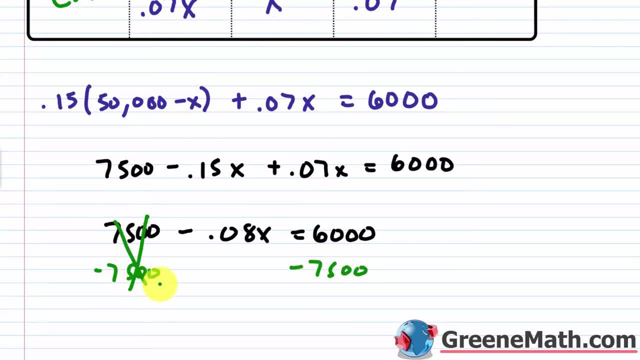 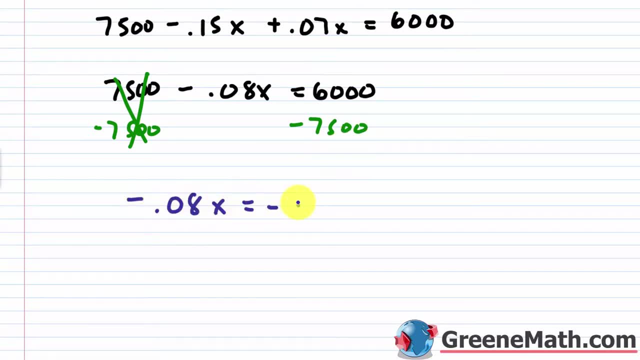 equation. That's going to cancel. You get some room going. So on the left, I'm just going to have my negative 0.08X. On the right, I'm going to have negative 1,500.. We'll finish this up by. 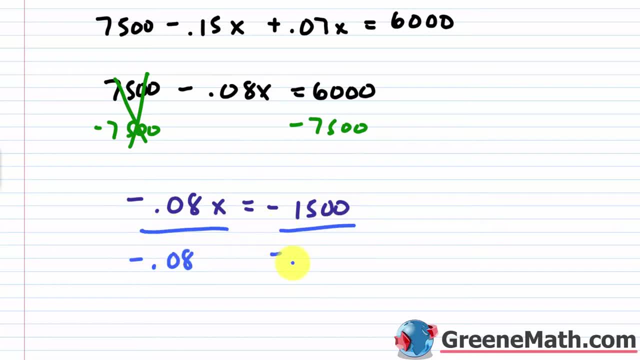 dividing both sides of the equation by negative 0.08.. So this is going to cancel with this And I'll have that X is equal to 18,750.. So 18,750.. Okay, So that's our answer for X, But again. 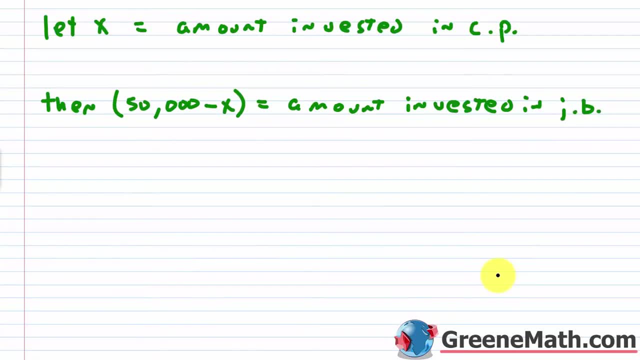 we're not done. We've got to make sense of that. So again, X was the amount invested in commercial paper, So we know that's $18,750.. And then we said that 50,000 minus X, which is $31,250,. 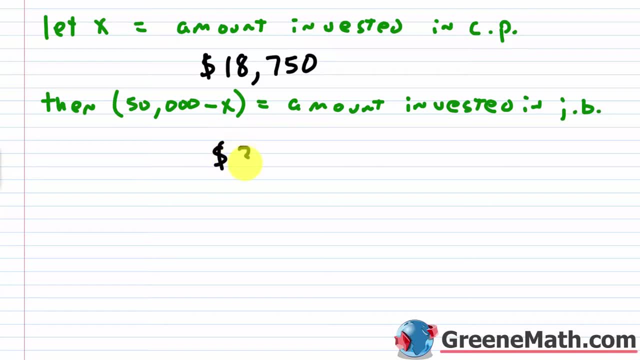 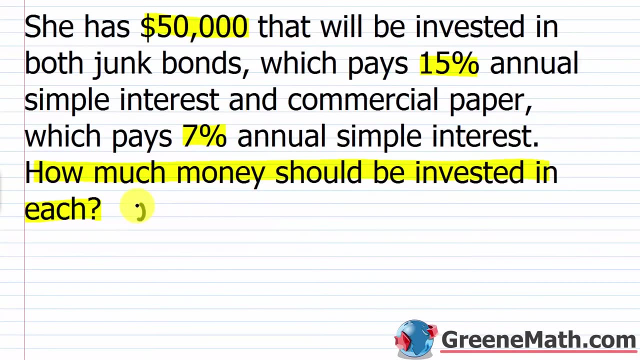 is going to be the amount invested in the junk bonds, So 31,250.. Okay, So let's go back up and make a nice little clean sentence. So Jennifer should invest $31,250 in junk bonds- Junk bonds, I'll just abbreviate it And $18,750. 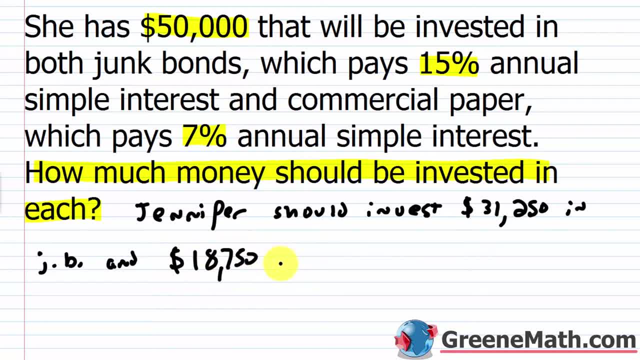 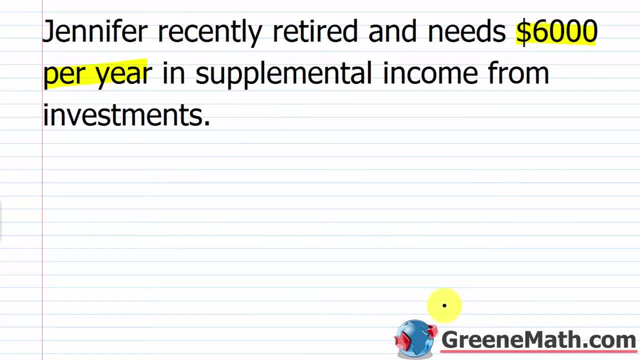 in commercial paper. Okay, So you can check this pretty easily by going back to the original statement, where it said: Jennifer recently retired and needs $6,000 per year. Okay, So that's what she has to earn. So just check the simple interest from the two investments. Again from the junk. 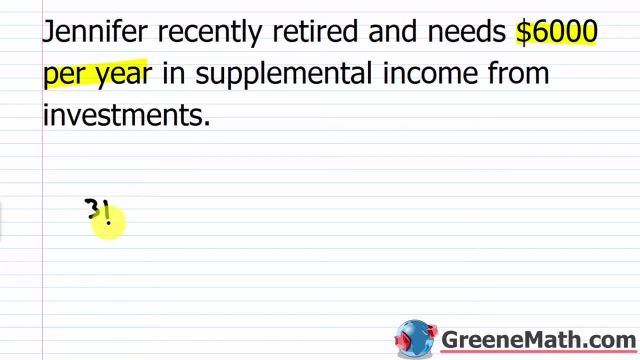 bonds. she's got $31,250 invested and she's getting 15% on that. So, times 0.15, that's going to give you what That's going to give you- $4,687.50.. Okay, So this is what she earns. 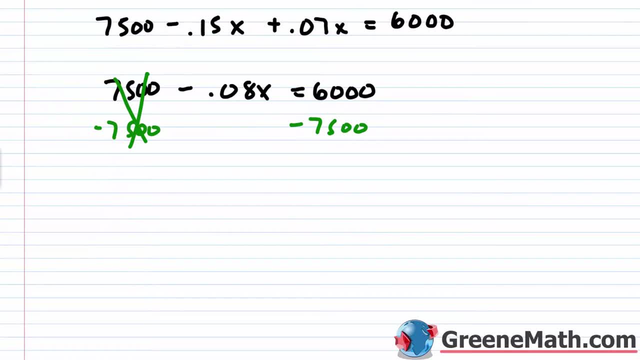 That's going to cancel. You get some room going. So on the left, I'm just going to have my negative 0.08X. On the right, I'm going to have negative $1,500.. We'll finish this up by dividing both sides of the equation by negative 0.08.. 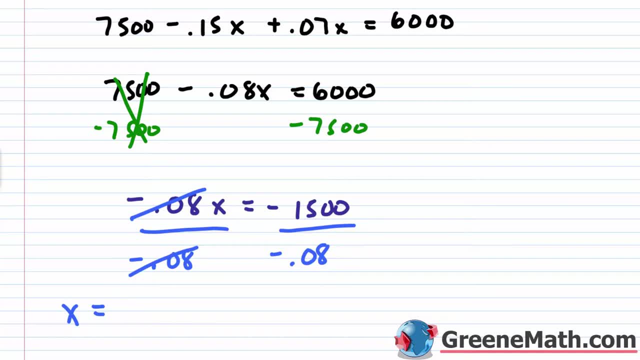 So this is going to cancel with this And I'll have that. X is equal to $18,750.. So that's our answer for X, But again we're not done. We've got to make sense of that. So again, X was the amount invested in commercial paper. 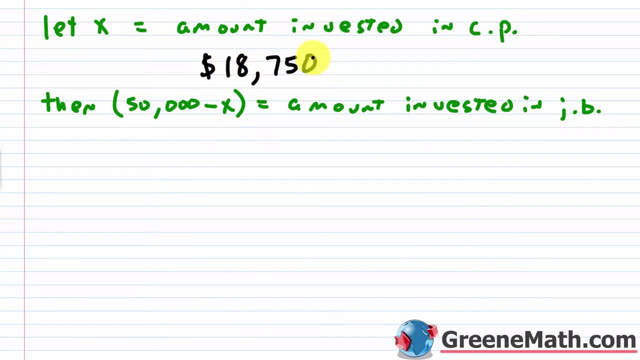 So we know that's $18,750.. And then we said that $50,000 minus X, which is $31,250, is going to be the amount invested in the junk bonds. So $31,250.. So let's go back up and make a nice little clean sentence. 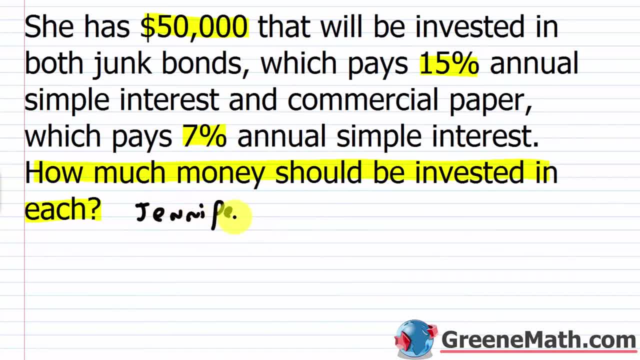 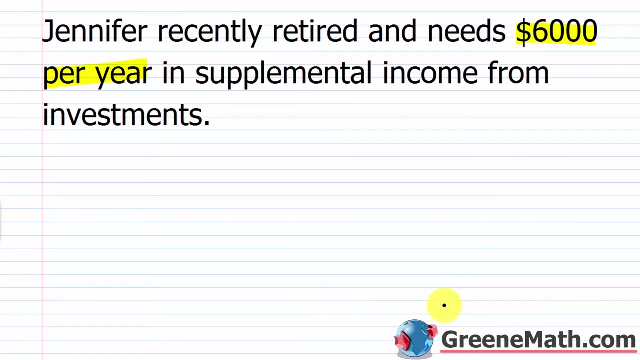 So Jennifer should invest $31,250 in junk bonds- Junk bonds, I'll just abbreviate it- And $18,750 in commercial paper. Okay, So you can check this pretty easily By going back to the original statement, where it said: Jennifer recently retired and needs $6,000 per year. 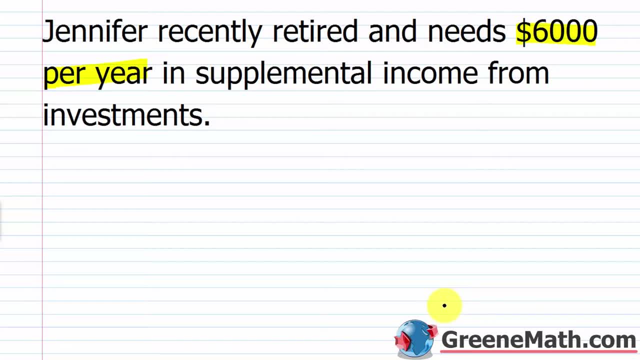 Okay, So that's what she has to earn. So just check the simple interest from the two investments. Again from the junk bonds, she's got $31,250 invested And she's getting 15% on that, So times 0.15.. 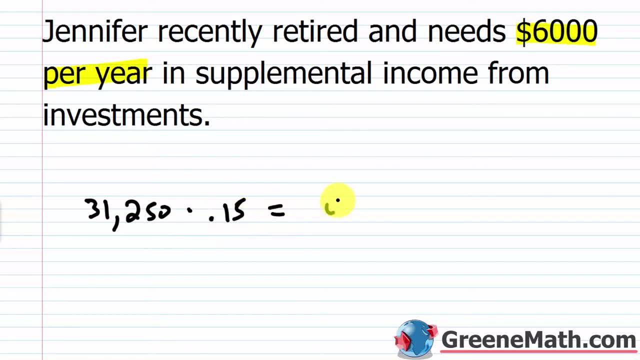 That's going to give you what That's going to give you: $4,687.50.. Okay, So this is what she earns from the junk bonds. I'm just going to put junk bonds. Okay, This is what she earns in yearly, simple interest. 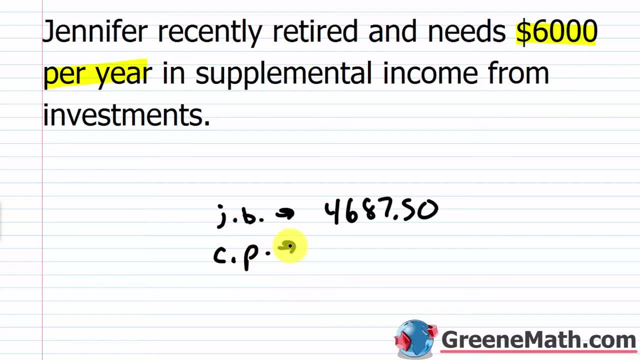 Then from the commercial paper she's going to earn 7% on $18,750.. So if I had $18,750 times 0.07, I would get $1,312.50.. So $1,312.50.. 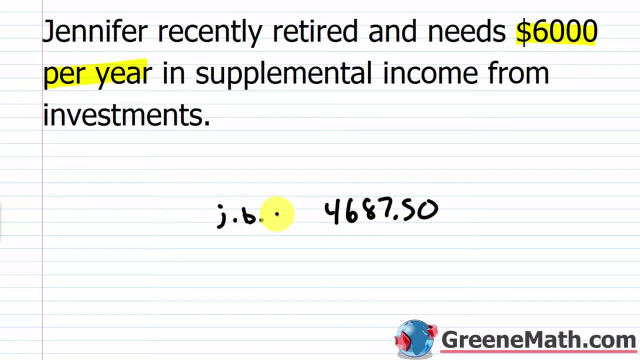 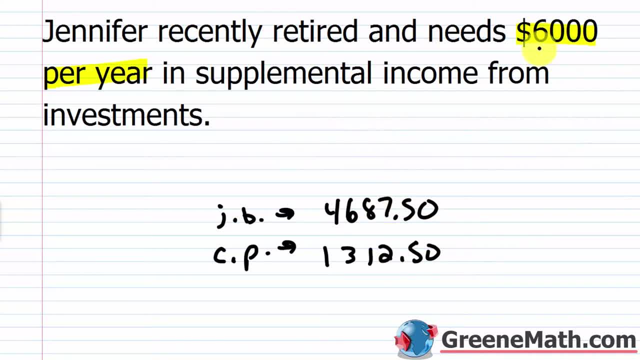 you have to do to check this problem is: sum these two amounts together. does it give you $6,000?? The answer to that is yes, right. If I add $4,687.50 to $1,312.50, I will get $6,000.. So that does tell me my solution is correct. 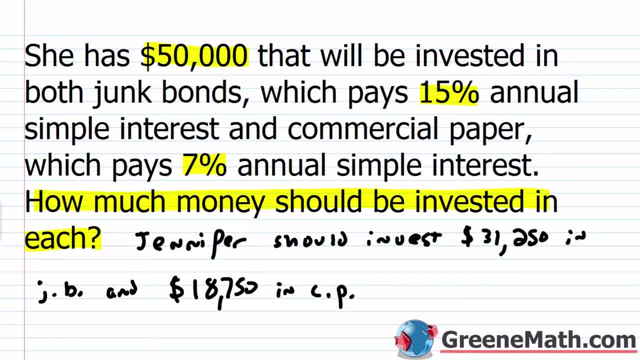 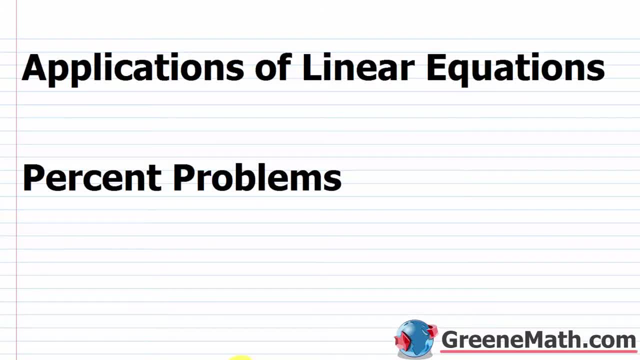 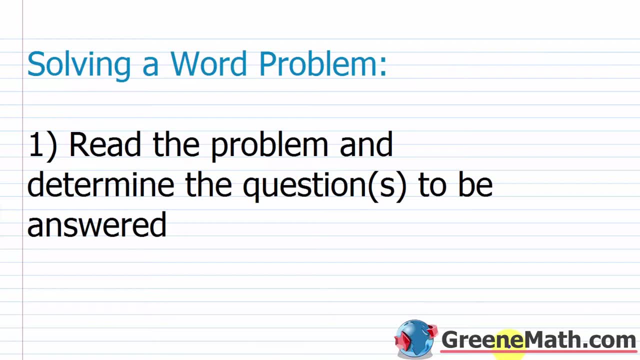 that Jennifer should invest $31,250 in the junk bonds and $18,750 in the commercial paper. In this lesson we want to review applications of linear equations and look at percent problems. So when we're in our section on applications of linear equations, again we can use a little. 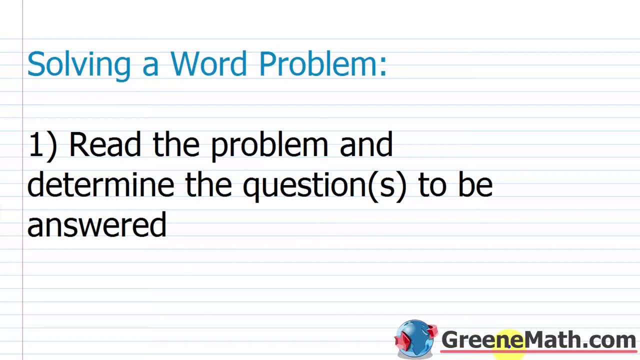 six-step procedure to get a solution for our word problem. So for solving a word problem again, the first step is just to read the problem and determine the question or questions to be answered. Then the next step is to assign a variable to represent the unknown Again. 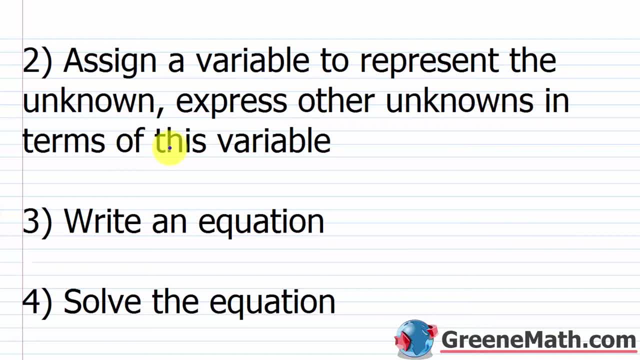 with these type of problems. you're going to express other unknowns in terms of this variable. Then we're going to write an equation that expresses the situation we're getting into. So we're going to write an equation that expresses the situation we're. 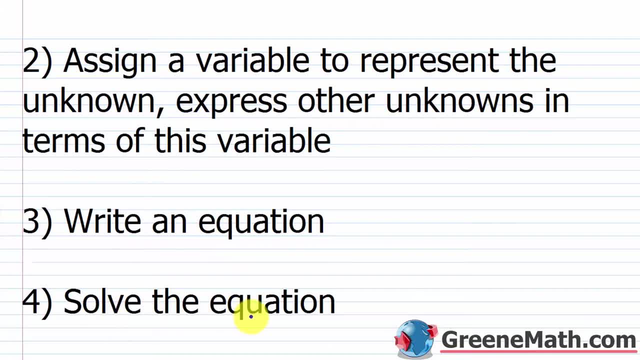 getting into And then we're going to write an equation that expresses the situation we're given right, based on the scenario and the problem. Then we're going to solve that equation, Then we're going to write the answer in terms of the question or again, questions asked. 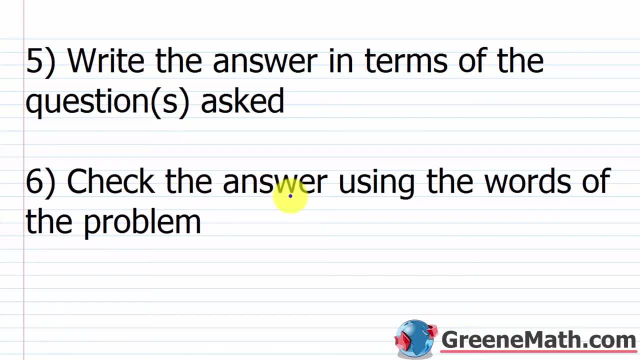 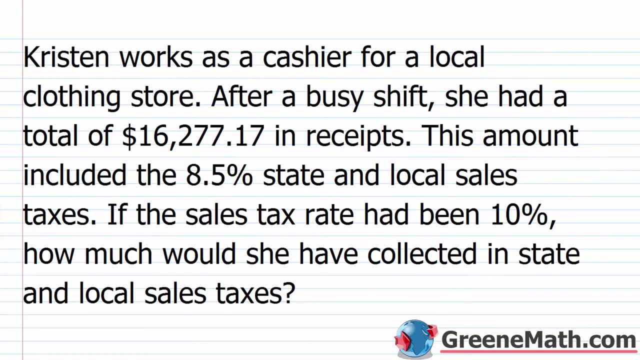 And then, lastly and most importantly, we're going to check the answer using the words of the problem. We always want to make sure that our answer is reasonable, All right, so for solving percent word problems, it's a very easy case scenario. It's one of the easiest types of 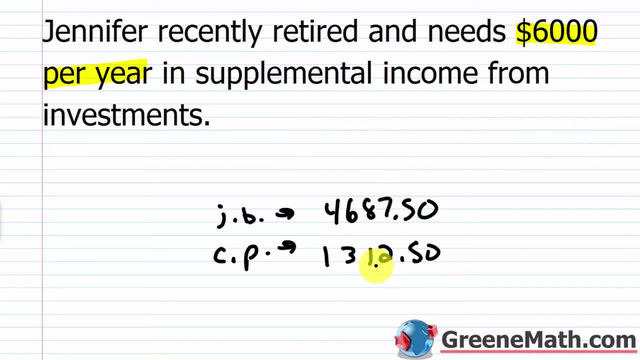 So all you have to do to check this problem is sum these two amounts together. Does it give you 6,000?? The answer to that is yes, Right. If I add $4,687.50 to $1,312.50, I will get $6,000.. 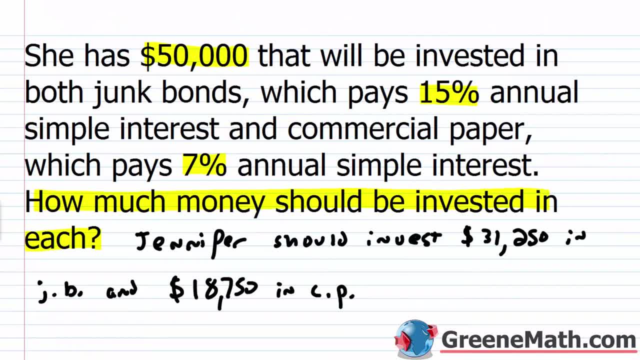 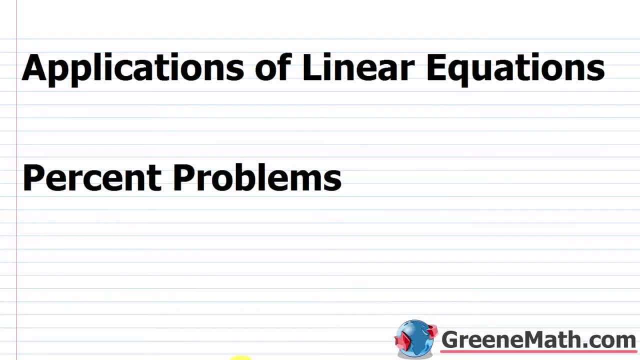 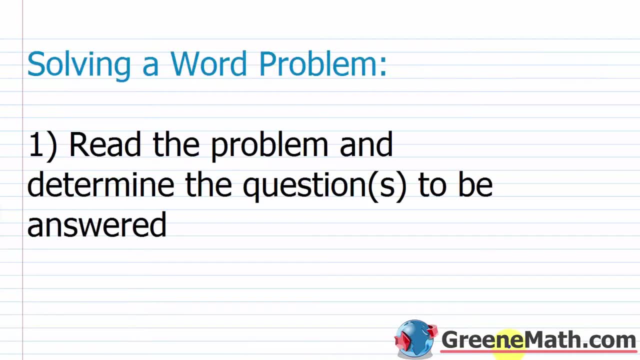 So that does tell me- my solution is correct- That Jennifer should invest $31,250 in the junk bonds and $18,750 in the commercial paper. In this lesson we want to review applications of linear equations and look at percent problems. So when we're in our section on applications of linear equations again we can use a little. 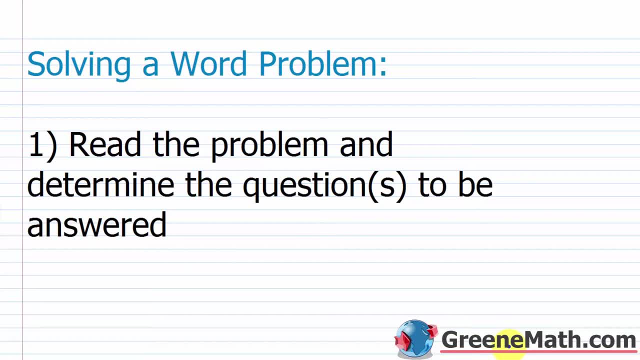 six-step procedure to get a solution for our word problem. So for solving a word problem again, the first step is just to read the problem and determine the question or questions to be answered. Then the next step is to assign a variable to represent the unknown. 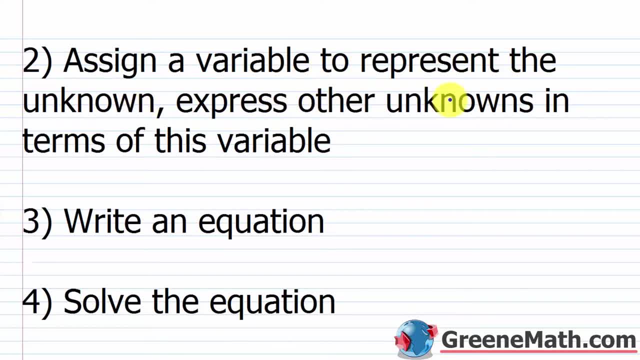 Again, with these type of problems, you're going to express other unknowns in terms of this variable. Then we're going to write an equation that expresses the situation we're given Right, Based on the scenario and the problem. Then we're going to solve that equation. 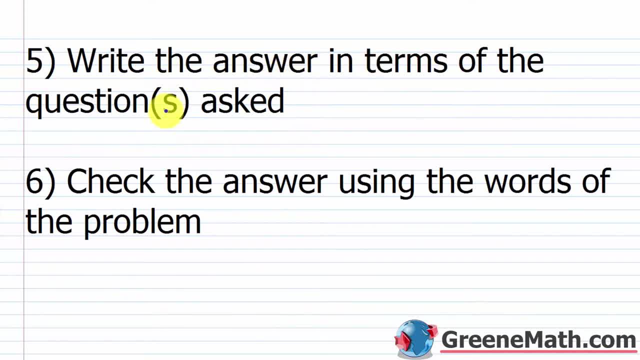 Then we're going to write the answer in terms of the question or again, questions asked, And then, lastly and most importantly, we're going to check the answer using the words of the problem. We always want to make sure that our answer is reasonable. 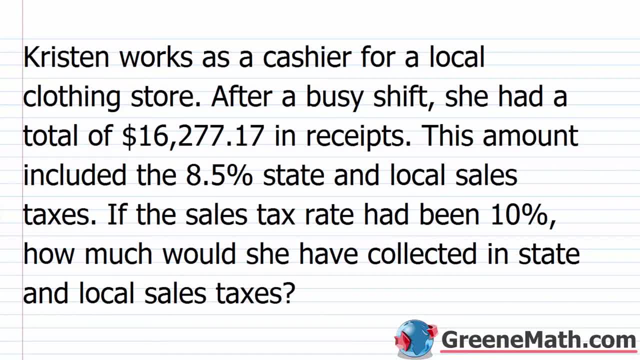 All right. So for solving percent word problems, it's a very easy case scenario. It's one of the easiest types of problems that you deal with when you're talking about applications of linear equations. Okay, Especially as long as you understand how to convert between a decimal and a percentage. 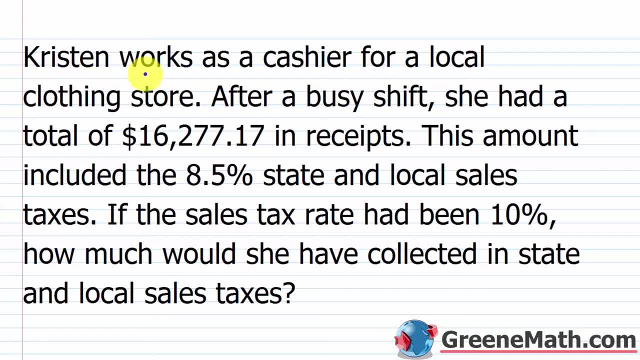 you're basically good to go. Okay, So we have that. Kristen works as a cashier for a local clothing store. After a busy shift she had a total of $16,277.17 in receipts. So this amount included the 8.5% state and local sales taxes. 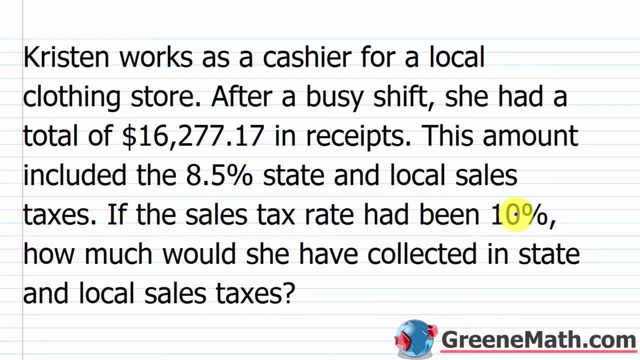 Now, if the sales tax rate had been 10%, how much would she have collected in state and local sales taxes? So this is what we need to figure out Again: if the sales tax rate had been 10% and this problem, it was 8.5.. 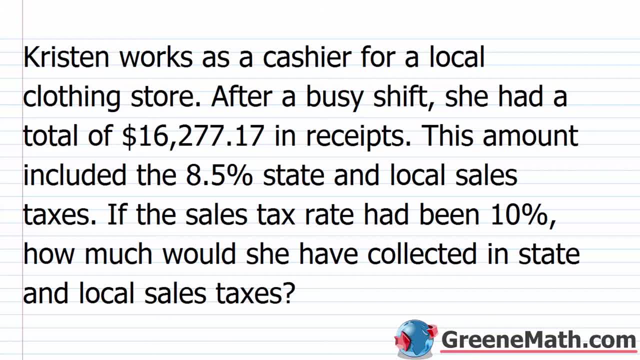 problems that you deal with when you're talking about applications of linear equations. okay. So, essentially, as long as you understand how to convert between a decimal and a percentage, you're basically good to go. okay, So we have that. Kristen works as a cashier for a local. 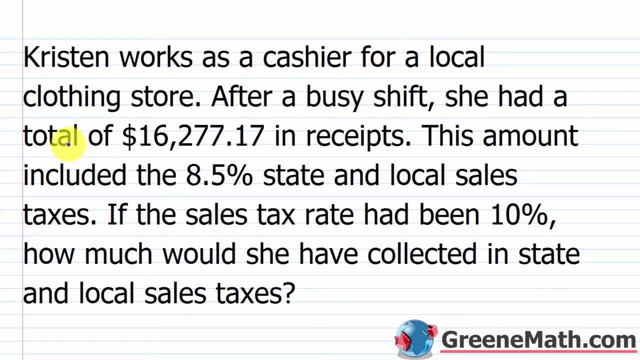 clothing store After a busy shift. she had a total of $16,277.17 in receipts, So this amount included the 8.5% state and local sales taxes. Now, if the sales tax rate had been 10%, how much would she have collected instead? 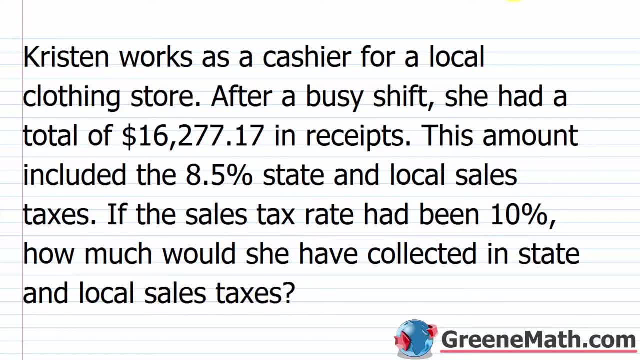 State and local sales taxes. So this is what we need to figure out Again: if the sales tax rate had been 10%- and this problem- it was 8.5.. So if it had been 10%, how much would she have collected? 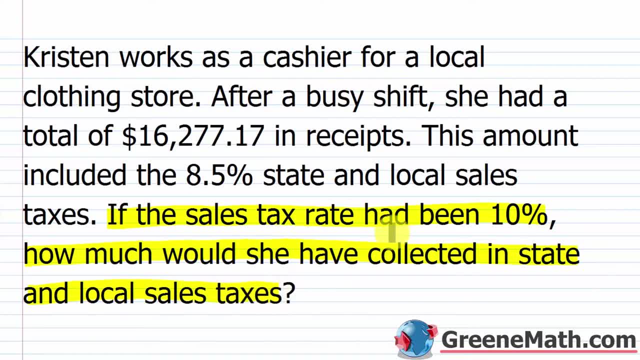 in state and local sales taxes. So that's what we need to find out. So, to attack this problem, it's very, very simple. You have two amounts that you're going to work with. The first amount is $16,277.17 in receipts And the second amount is $16,277.17 in receipts And the second amount is 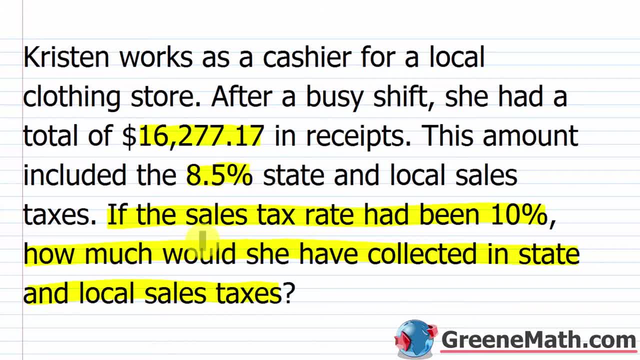 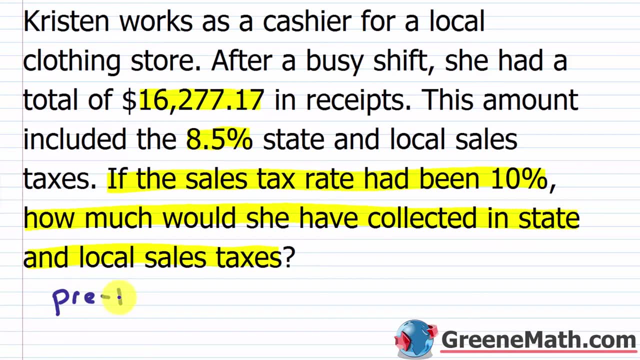 the 8.5% state and local sales taxes. So think about what this means. She's got this amount in total receipts, So it included the state and local sales tax, okay. So think about this. You have a pre-tax amount of goods sold, So you have some pre-tax amount of the goods sold. Plus you have 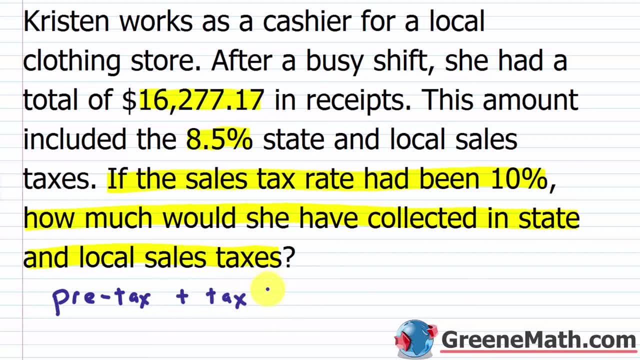 the taxes that are collected, And when we sum these two amounts together, we get this value here, this $16,277.17.. So what I'm going to do is I'm going to let a variable like x equal the pre-tax amount of all. 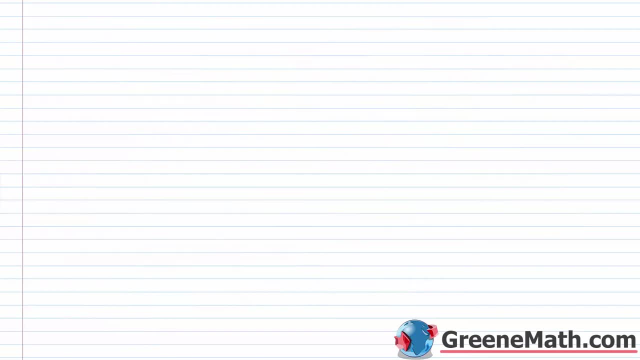 the goods sold. So let's go down And I'm just going to say we're going to let x be equal to the pre-tax amount of goods sold, okay? So again, if I go back to what I wrote there, I said that the pre-tax amount which we labeled as x 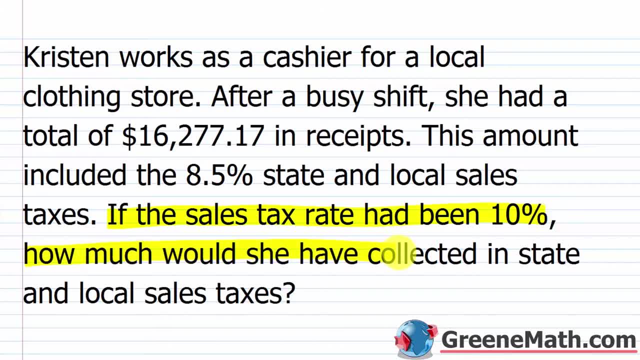 So if it had been 10%, how much would she have collected in state and local sales taxes? So that's what we need to find out. So to attack this problem, it's very, very simple. You have two amounts that you're going to work with. 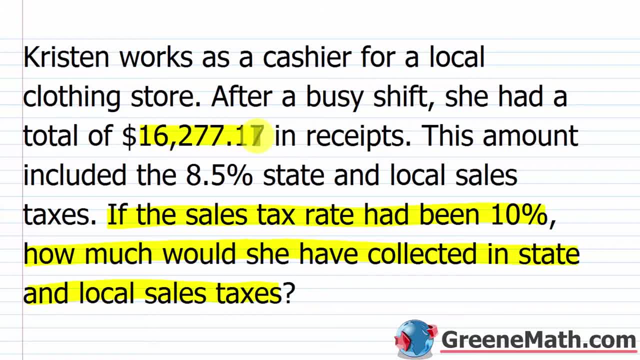 The first amount is a $16,277.17 in receipts And the second amount is the 8.5% state and local sales taxes. So think about what this means. She's got this amount in total receipts, So it included the state and local sales tax. 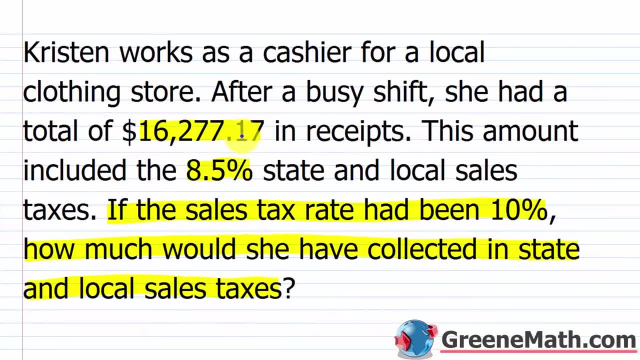 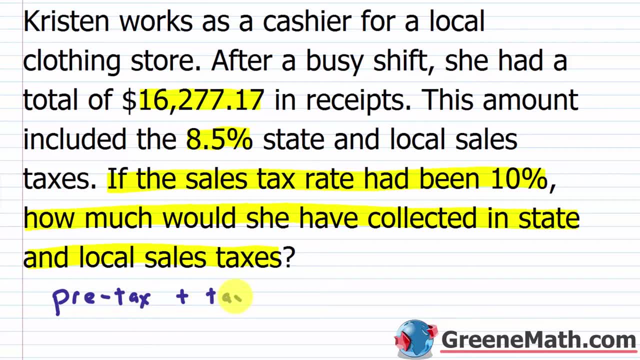 Okay. So think about this: You have a pre-tax amount of goods sold, So you have some pre-tax amount of the goods sold, Plus you have the taxes that are collected, And when we sum these two amounts together, we get this value here. 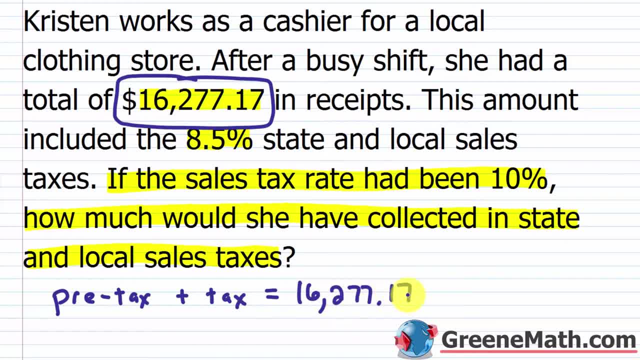 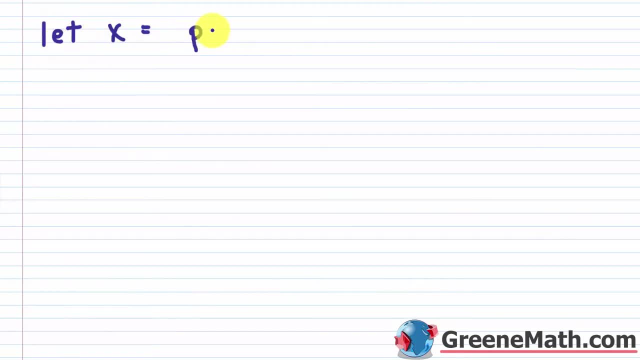 This $16,277.17.. So what I'm going to do is I'm going to let a variable like x equal the pre-tax amount of all the goods sold. So let's go down And I'm just going to say we're going to let x be equal to the pre-tax amount of goods sold. 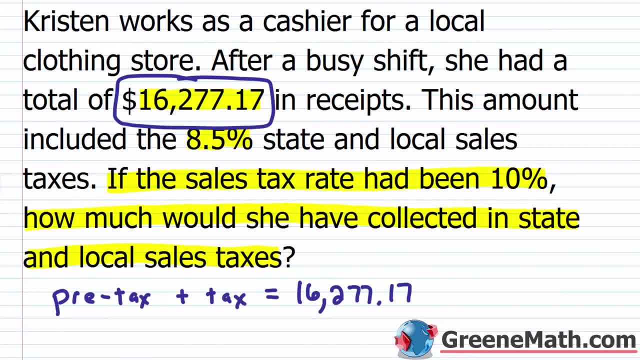 Okay. So again, if I go back to what I wrote there, I said that the pre-tax amount which we labeled as x- right, this will now be x plus the tax amount which. how can we get that? Well, if she sold x amount of goods and the tax is 8.5%, well then, all I have to do is multiply 8.5% times that pre-tax amount, right, which is x. 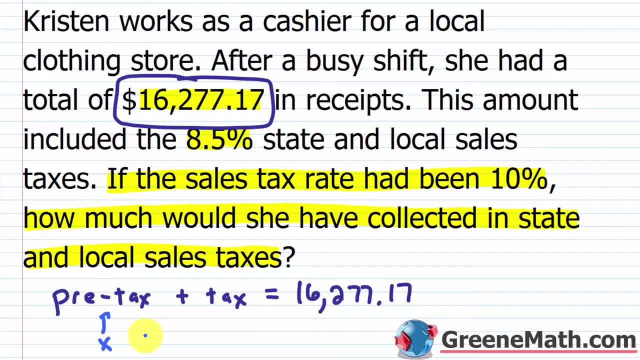 Now you do that as a decimal, So 8.5% as a decimal is .085.. Okay, So plus .085 times x, That would give me my 16,277.17.. So it's very easy to get our equation. 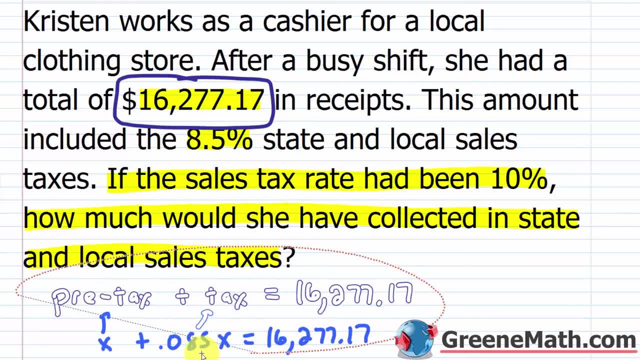 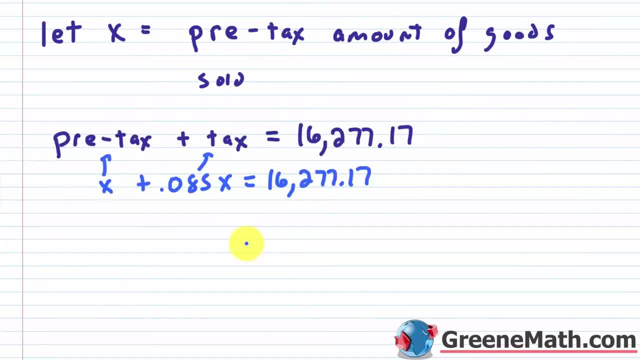 Let me kind of arrow that up there, And I'm just going to copy this because it's kind of busy here, So let me remove that from here. Let me just kind of throw that down here so we can just get some thought processes going. 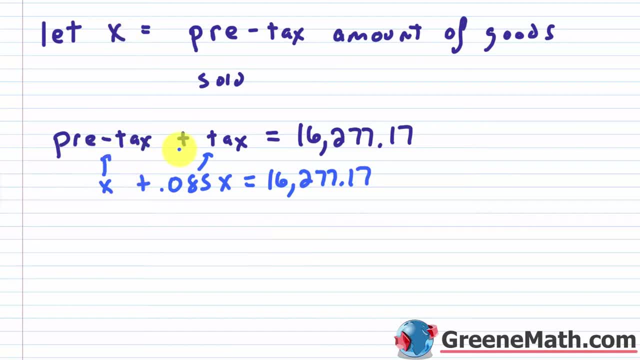 And we see that again the pre-tax amount is x plus the tax amount, which is .085,, which again is 8.5%. It's a decimal Times x, which is the pre-tax amount that gives me the tax. 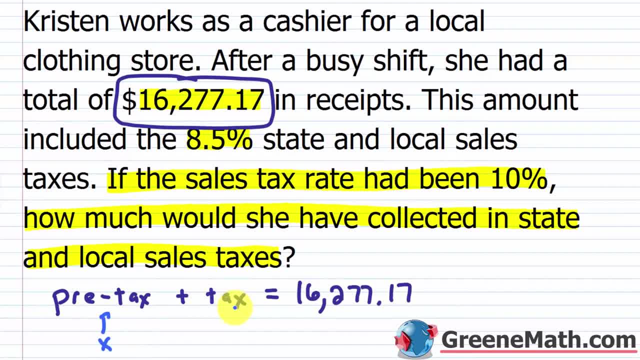 right, this will now be x plus the tax amount. which, how can we get that? Well, if she sold x amount of goods and the tax is 8.5%, well then, all I have to do is multiply 8.5% times that pre-tax. 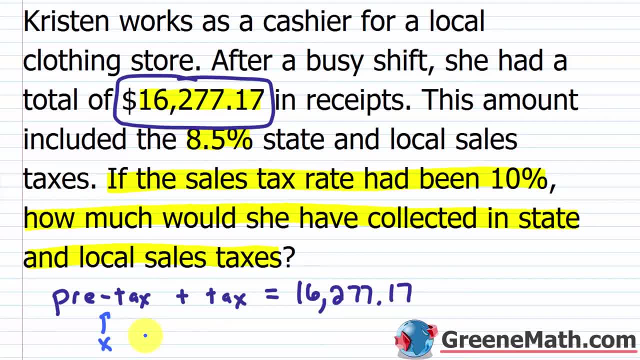 amount right, which is x. Now you do that as a decimal, So 8.5% as a decimal is 0.085.. So plus 0.085 times x, That would give me my $16,277.17.. So it's very easy to get our equation. Let me kind of arrow. 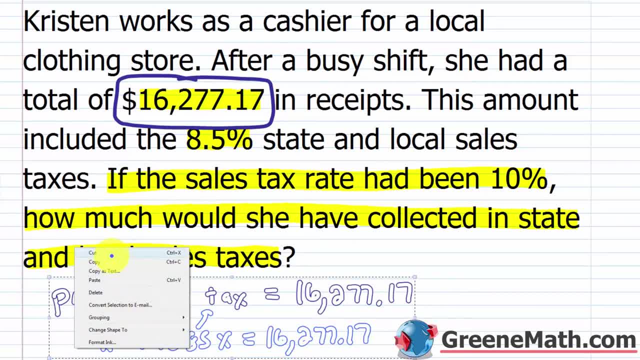 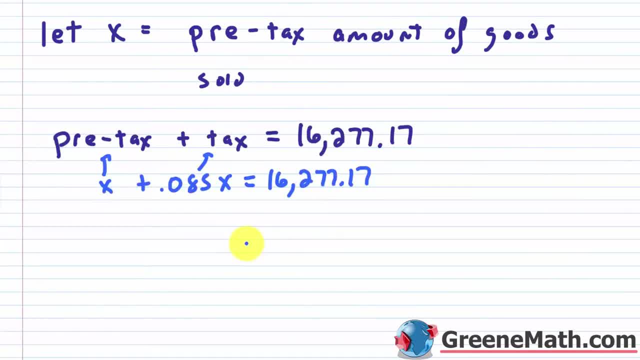 that up there And I'm just going to copy this because it's kind of busy here, So let me remove that from here And let me just kind of throw that down here, So we can just get some thought processes going. And we see that again, the pre-tax amount is x plus the tax amount, which is 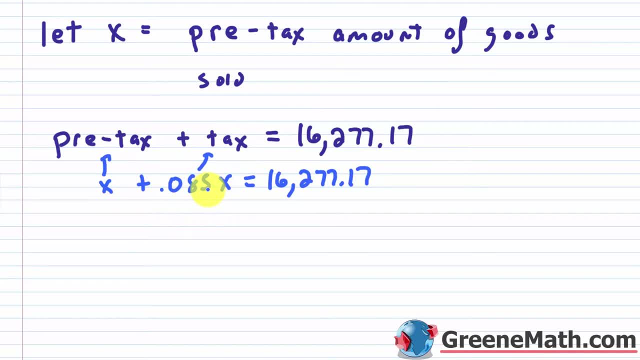 0.085, which again is 8.5% as a decimal times x, which is the pre-tax amount. that gives me the tax Sum. those two amounts together And again you get our total receipts, which is $16,277.17.. 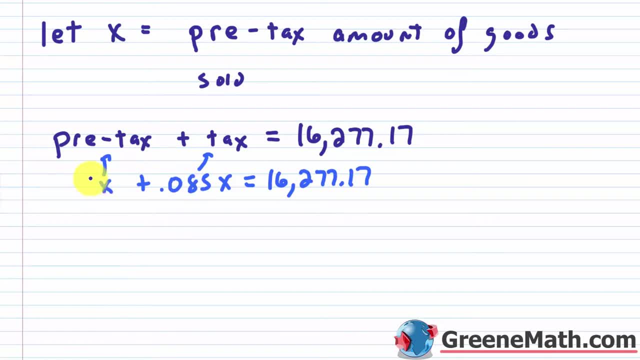 So on the left side I can just sum this right. So this is basically 1x plus 0.085x, So this would be 1.085x. Let me make that 8 a little better. And again this is equal to the. 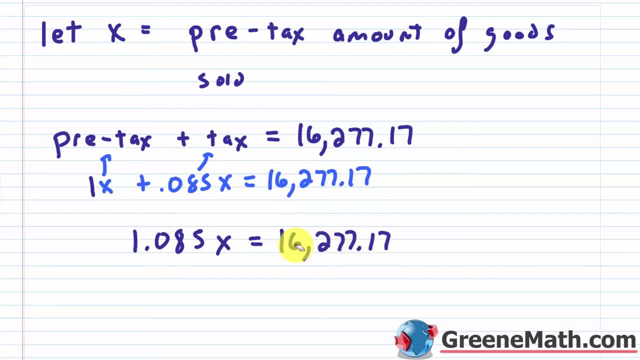 $16,277.17.. Now, if I want x by itself, just divide both sides by 1.085.. Again over here, 1.085.. I'm going to do that with a calculator And I'm going to end up with: 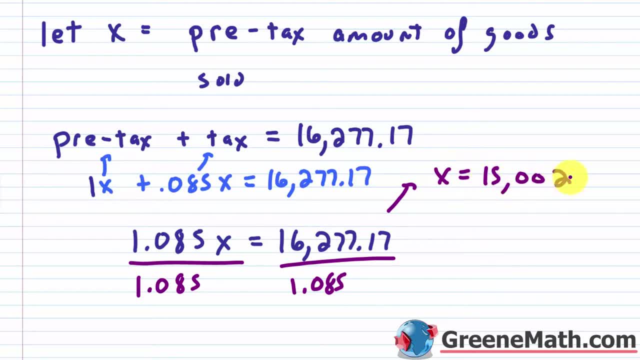 x is equal to 15,002.. So let me erase everything other than my x. I don't need any information anymore because I basically found what I need: the pre-tax amount of goods sold. So this is $15,002.. Okay, Now it doesn't ask us for this information in the problem. We go back up It specifically. says, if the sales tax rate had been 10%, how much would she have collected in stated local sales taxes? So they don't care that it's $15,002 in sales pre-tax right? They don't care about that at all. 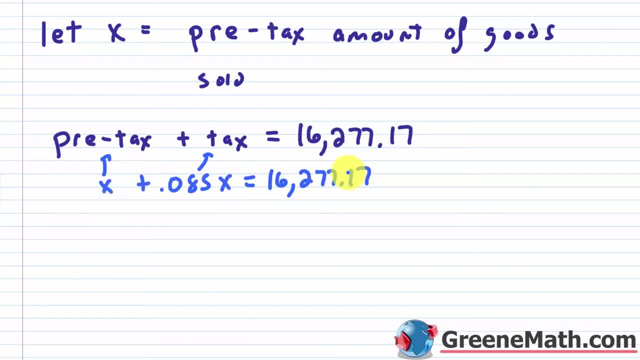 You sum those two amounts together And again you get our total receipts, which is $16,277.17.. So on the left side, I can just sum this right. So this is basically 1x plus .085x. 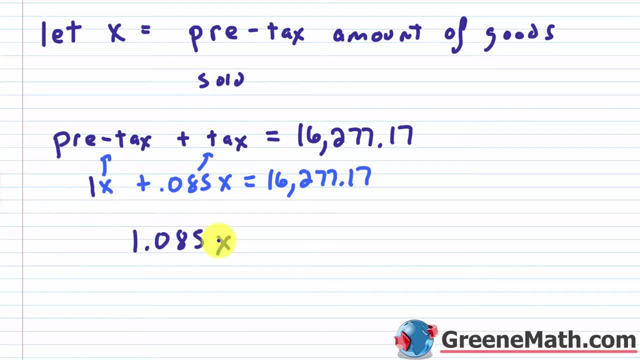 So this would be 1.085x. Let me make that 8 a little better- And again, this is equal to this $16,277.17.. Now, if I want x by itself, just divide both sides by 1.085.. 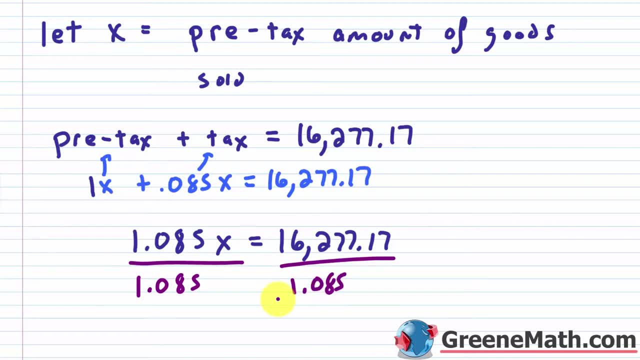 Again over here: 1.085.. I'm going to do that with a calculator And I'm going to end up with x is equal to 15,002.. So let me erase everything other than my x. I don't need any information anymore, because I basically found what I need: the pre-tax amount of goods sold. 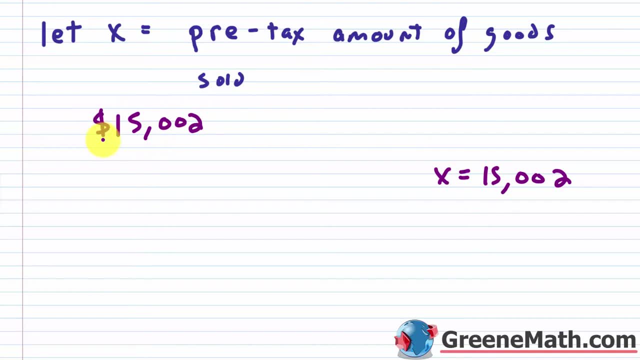 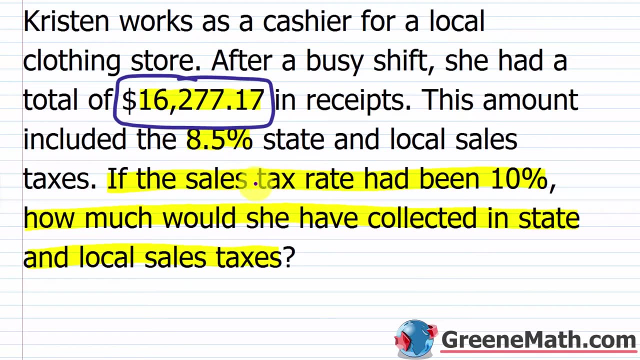 So this is $15,002.. Okay, Now it doesn't ask us for this information. in the problem We go back up, It specifically says: if the sales tax rate had been 10%, how much would she have collected in stated local sales taxes? 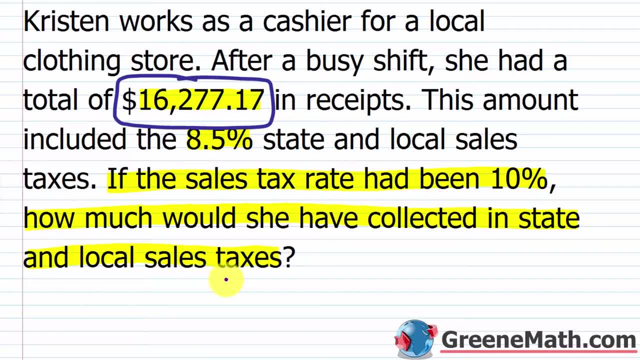 So they don't care that it's $15,002 in sales pre-tax right. They don't care about that at all. They want to know again: if the sales tax rate had been 10%, what would she have collected in stated local sales taxes? 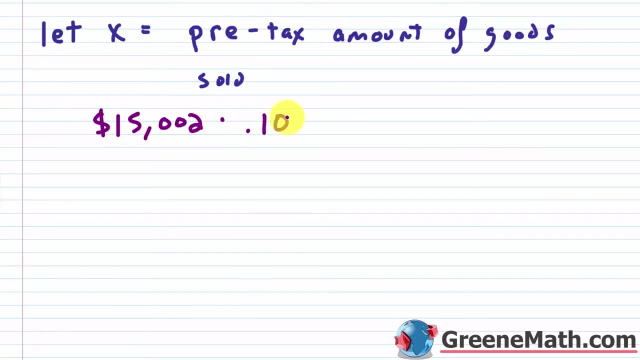 So I would just multiply that. So I would just multiply this by .10.. That's 10% as a decimal. That's very easy to do. I just move my decimal point one place to the left, So you would have $1,500.20.. 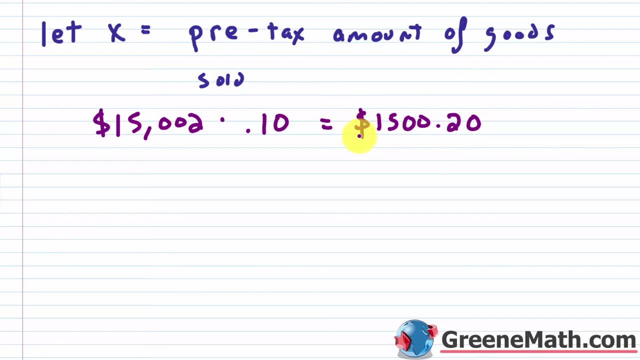 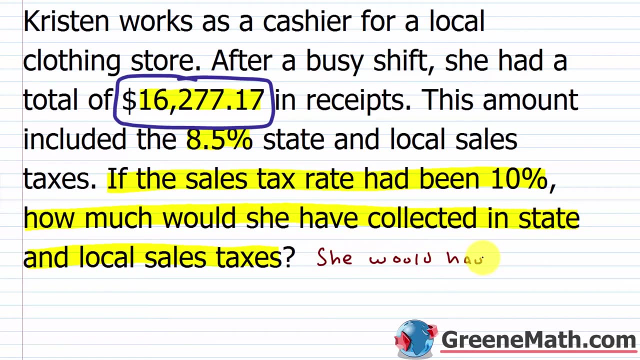 Okay, So $1,500.20.. That's going to be your answer. So I'll say she would have collected. So it's going to be $1,500.20.. Okay, So she would have collected $1,500.20. 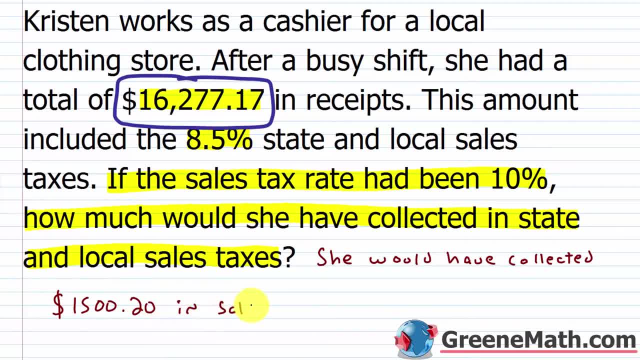 And you can put in. I'm just going to put sales taxes, So sales taxes. Okay. So to check this is pretty easy. If she had $16,277.17 in total receipts, And again this included the 8.5% stated local sales taxes. 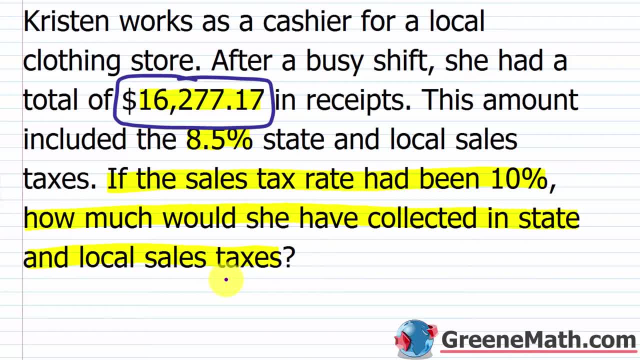 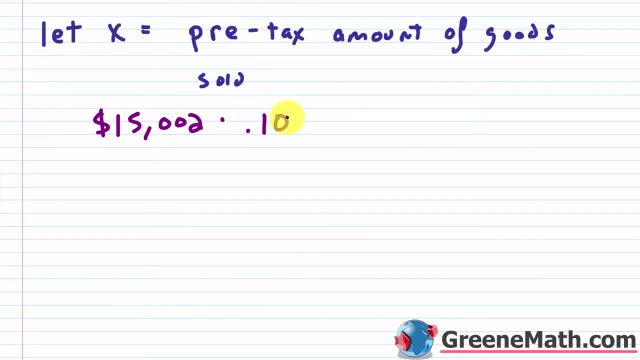 They want to know again: if the sales tax rate had been 10%, what would she have collected in stated local sales taxes? So I would just multiply this by 0.10.. That's 10% as a decimal. That's very easy to do. I just moved my decimal point one place to. 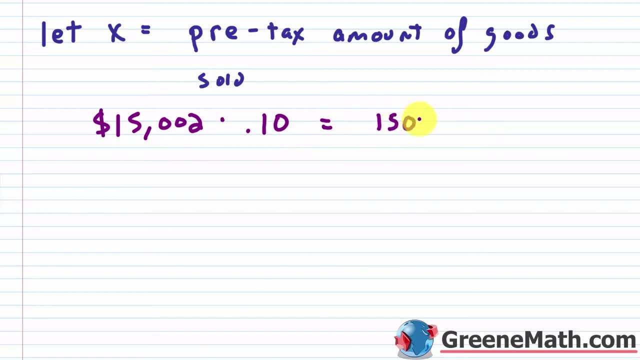 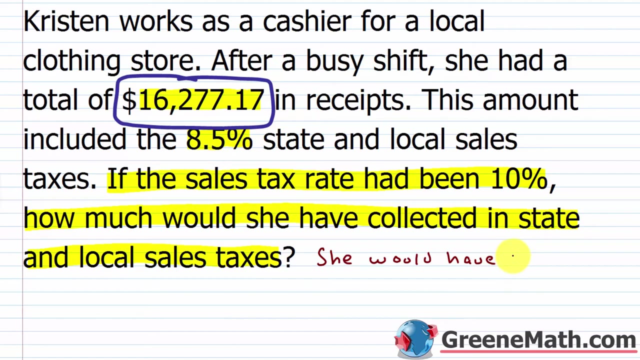 the left, So you would have $1,500.20.. Okay, So $1,500.20, that's going to be your answer. So I'll say she would have collected, So it's going to be $1,500 and then 20 cents. Okay, So she would have collected $1,500 and 20. 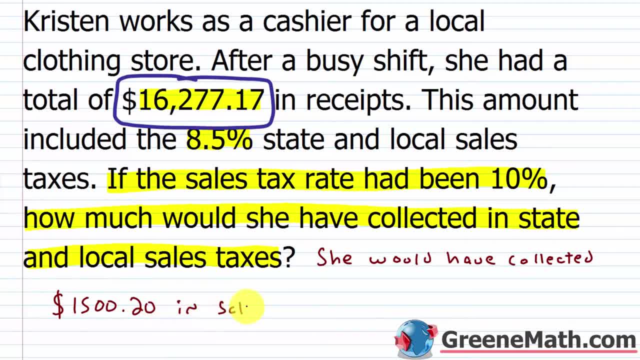 cents And you can put in- I'm just going to put sales tax. So she would have collected $1,500 and 20 taxes, So sales taxes, Okay. So to check this is pretty easy If she had $16,277 and 17 cents in. 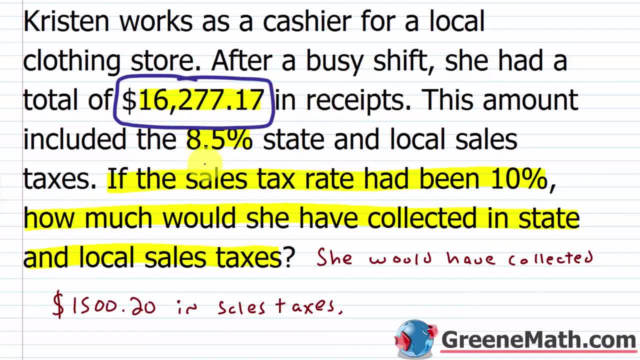 total receipts And again this included the 8.5% state and local sales taxes. Well, if I started with again the $15,002 in pre-tax goods sold, if I added in the 8.5% tax on that one way that 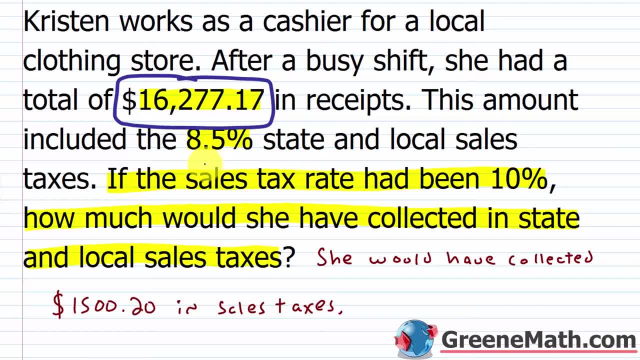 I could do, that is, I could multiply $15,002 by $1,500.20.. So that's going to be $1,500.20.. So 1.085.. Okay, And that would give me the 16,277.17.. So that part would check out. 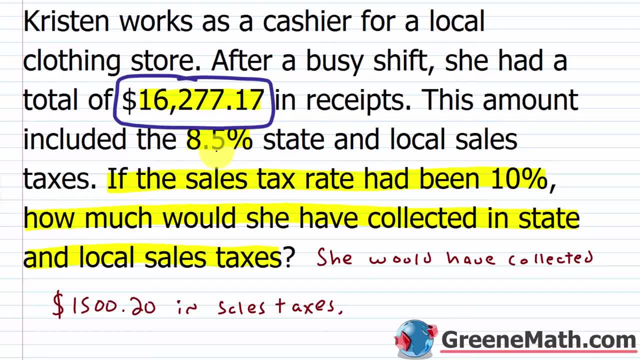 Now I know that it's $15,002.. Okay, That's pre-tax. goods sold Again. if the sales tax rate had been 10%, well, all you got to do is move the decimal point one place to the left. Okay To multiply by. 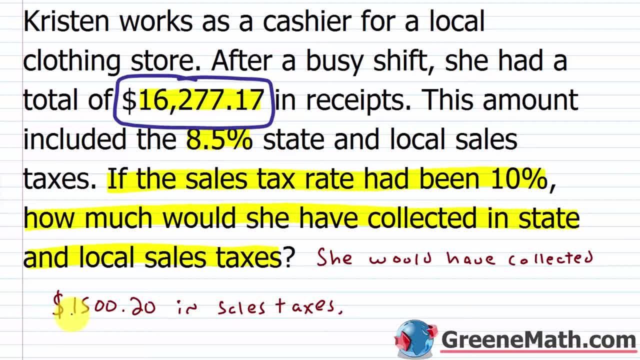 0.1, 10% as a decimal, And you would end up with this $1,500 and 20 cents again in sales taxes. Okay, So our answer here is correct. Again, she would have collected $1,500 and 20 cents in sales taxes. 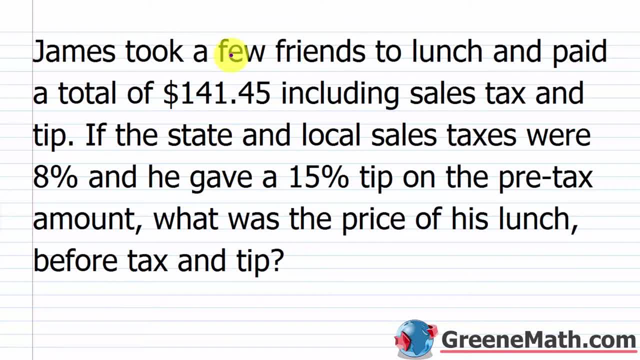 All right, Let's take a look at another one. So we have here that James took a few friends to lunch and paid a total of $141.45, including sales tax and tip. If the state and local sales taxes were 8% and he gave a 15% tip on the pre-tax amount, what was the price of his lunch before tax? and 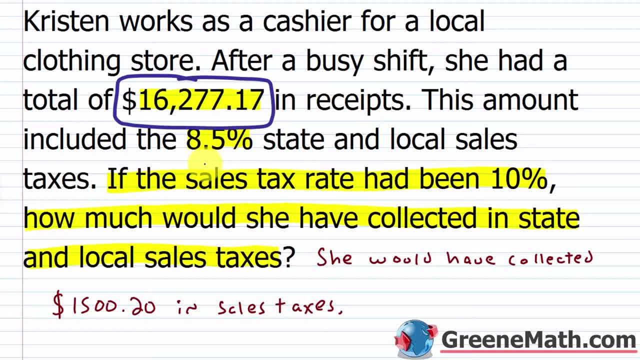 Well, if I started with again the $15,002.00.. And pre-tax goods sold, If I added in the 8.5% tax on that, One way that I could do that is I could multiply $15,002.00 by 1.085.. 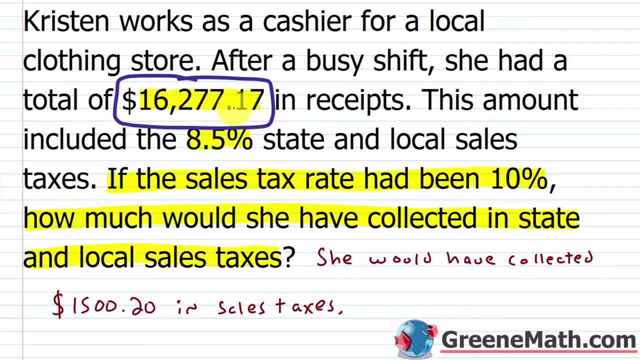 Okay, And that would give me the $16,277.17.. So that part would check out. Now I know that it's $15,002.00.. Okay, That's pre-tax goods sold. Again, if the sales tax rate had been 10%. 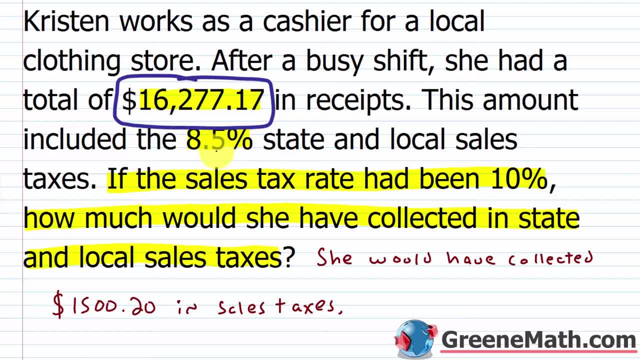 Well, all you got to do is move the decimal point one place to the left. Okay, To multiply by .1.. 10% is a decimal And you would end up with this $1,500.20.. Again in sales taxes. 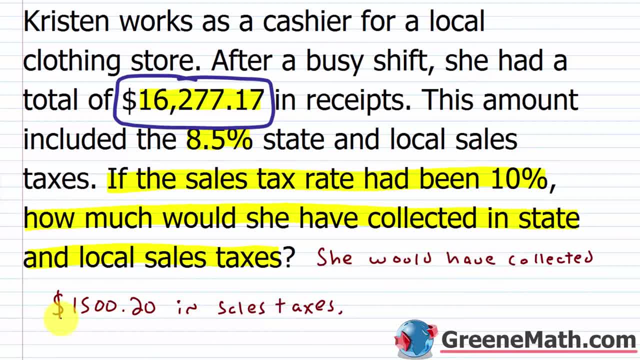 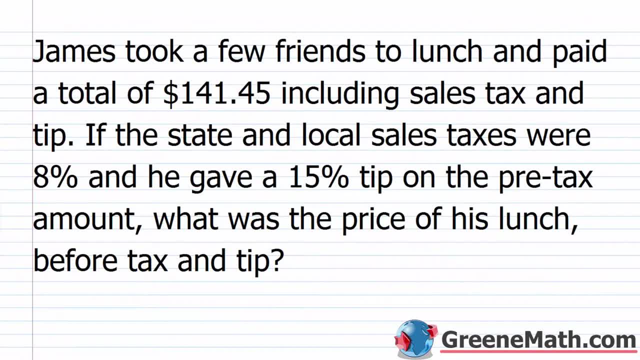 Okay, So our answer here is correct. Again, she would have collected $1,500.20 in sales taxes. All right, Let's take a look at another one. So we have here that James took a few friends to lunch and paid a total of $141.45. So the answer is according to the tax rate. So the answer is this: James took a total of $141.45 before food and drinks. Now he could have paid $141.45 prior to lunch and before food, So it's a pretty good choice. 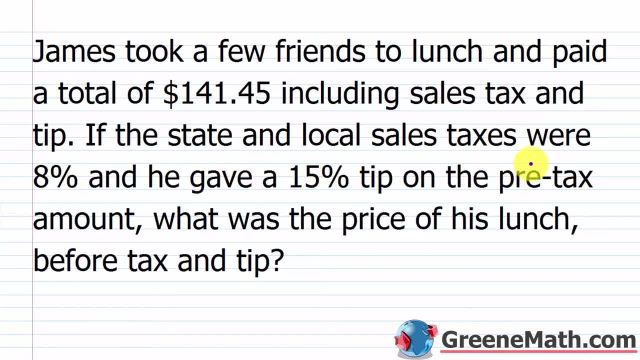 And I think you should know this. James is going to show you how to do this. He's going to show you how to do this. Let's do this. James is going to show you how to do this. Here we go. He's going to tell you how to do this. 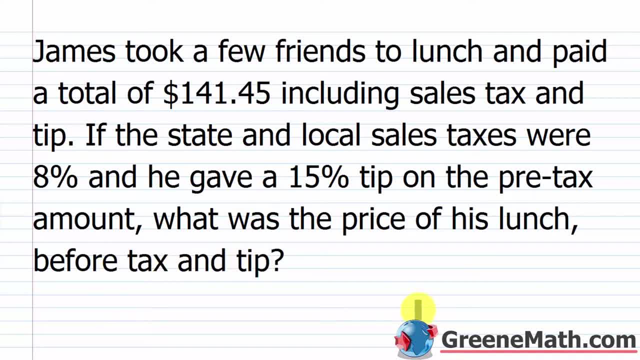 Okay, So let's go ahead and start. Here we go. One $1.002.00.. Okay, Here we go. He started this off Right, Let's go back. Let's see tax and the tip. what would the amount have been? so again, just like the last problem, we have a. 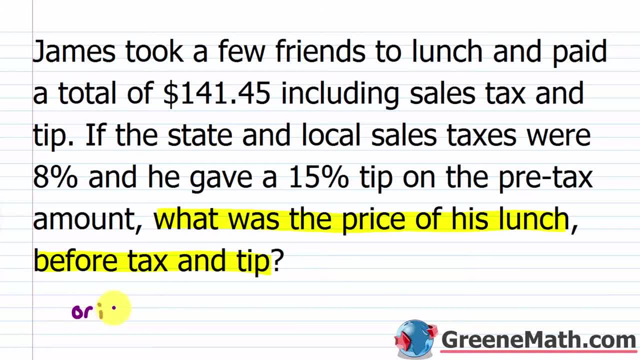 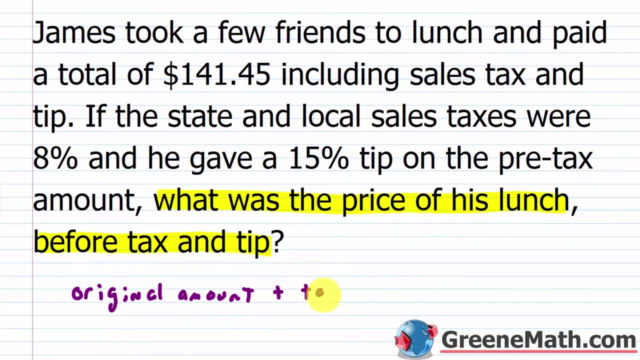 pre-tax, pre-tip amount, where we say the original amount of the food, so the original amount, then you have plus the tax and then plus the tip and this equals this 141.45. so let's bring this down to a fresh sheet. so the original amount, i'm just going to call that x. 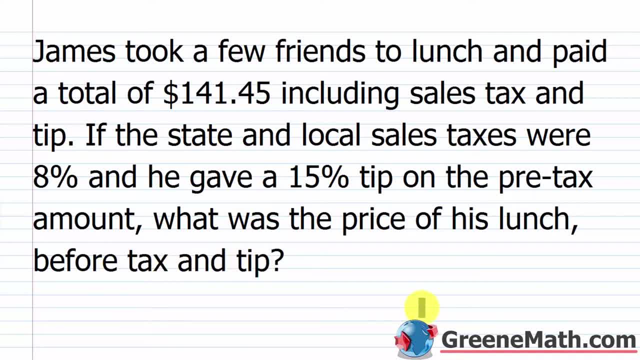 tip. Okay, So that would end up in a similar way. But what we want to find out is what was the price of his lunch before tax and tip? So before he gave the tax and the tip, what would the amount have been? 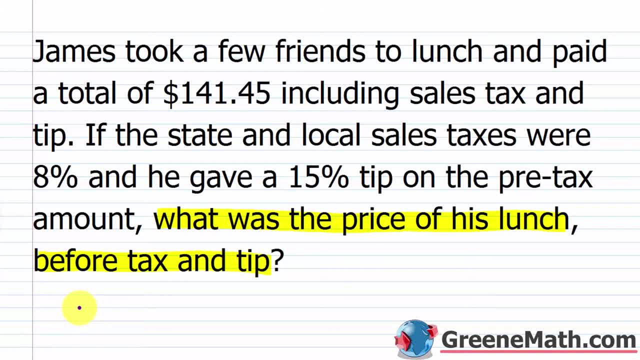 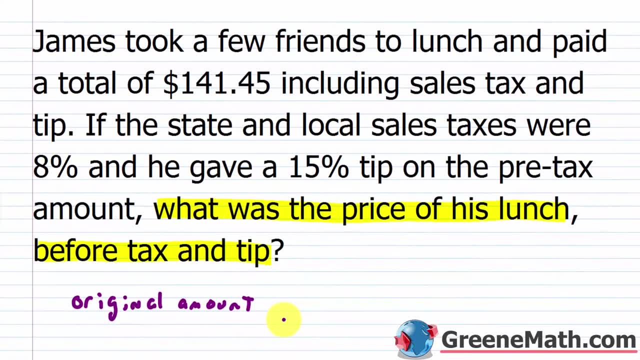 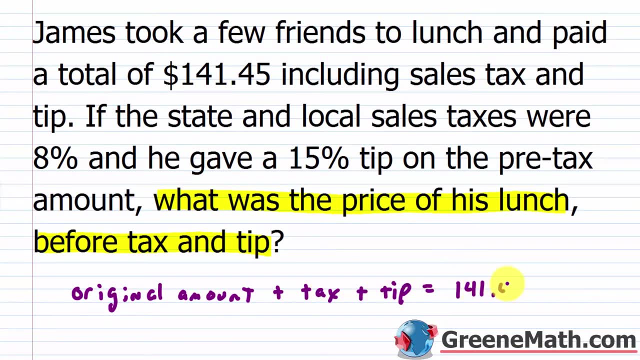 So again, just like the last problem, we have a pre-tax, pre-tip amount where we'd say the original amount of the food, So the original amount, Then you have plus the tax and then plus the tip, And this equals this $141.45.. 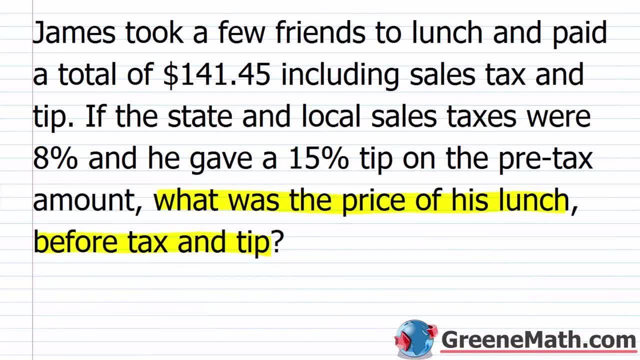 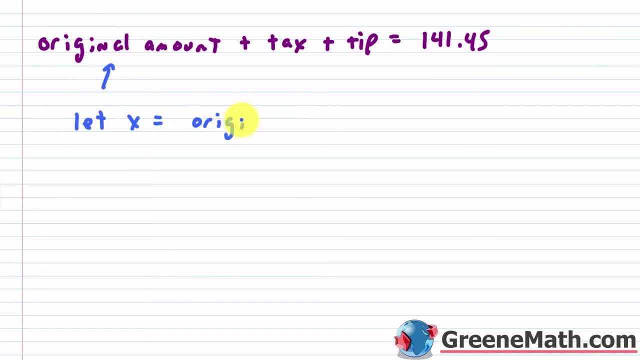 So let's bring this down to a fresh sheet. So the original amount- I'm just going to call that X. So let X be the original amount of the food. Okay, This is before tax or tip. So if I have X plus my tip and plus my tax, 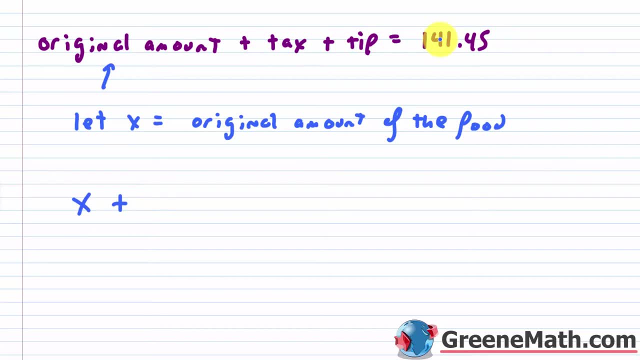 again, I'm going to get this $141.45.. So we said that the tax if we go back up was 8% and the tip is 15%. So the tax again is 8%. So that's 0.08 times X, right, That's 8%. 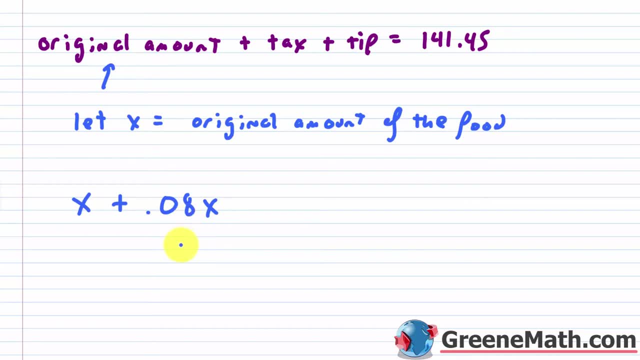 as a decimal, 0.08.. Again, multiply that by X. That's going to give you the tax. Okay, And again, this is the original amount. Or you could say pre-tax, pre-tip amount, whatever you want to do. 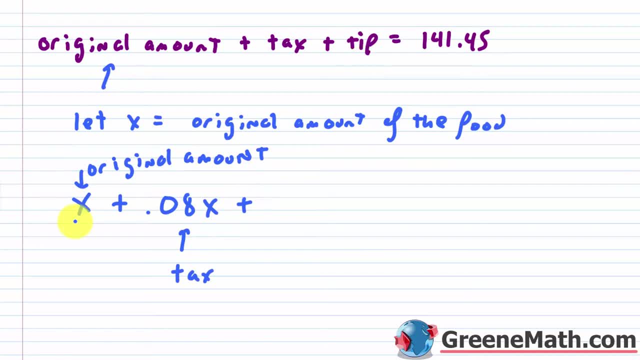 Then plus I've got to get my tip and the tip is 15% of the original amount. So that's 0.15, which is 15% as a decimal times X. So this is your tip. So this equals, you've got your $141.45.. If I sum everything on the left, just combine like terms. 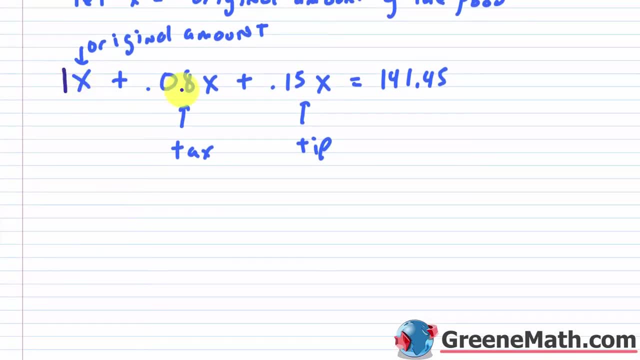 what's going to happen is I'll have 1X plus 0.08X plus 0.15X. So 1 plus 0.08 plus 0.15 is going to be 1.23, and then times X, And again this equals 0.15X plus 0.15X. 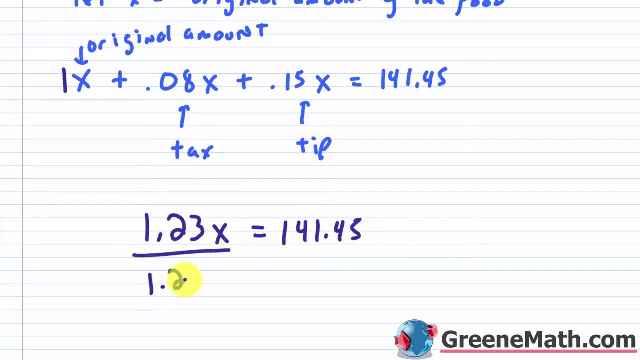 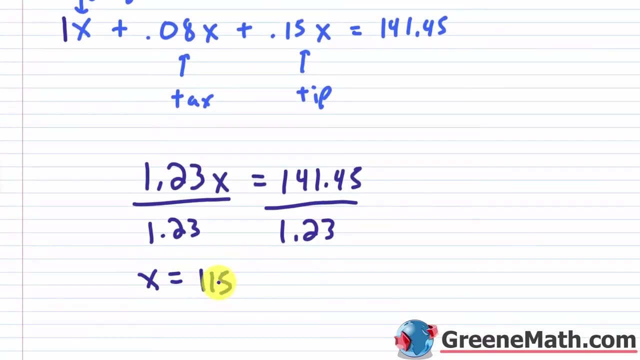 So that's 0.141.45.. Divide both sides of the equation by 1.23.. And what are we going to get? We're going to get that X is equal to 115.. Okay, So that was the price of his food before again. 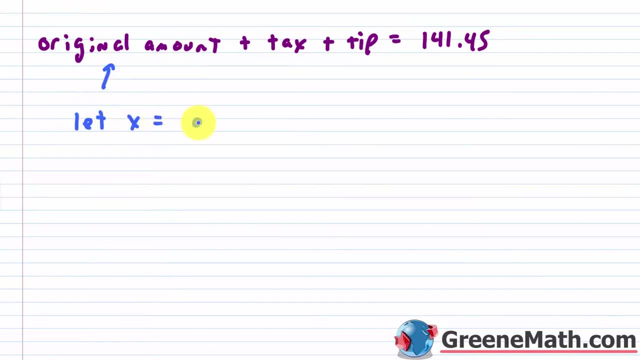 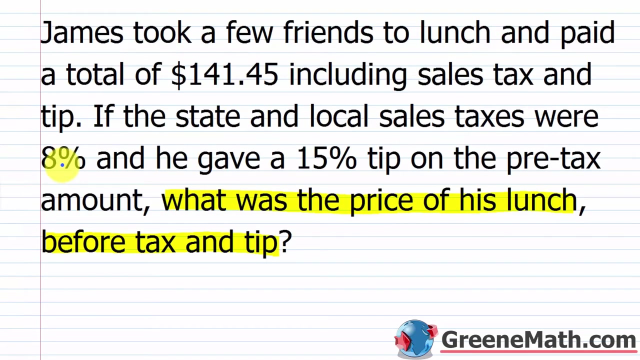 so let x be the original amount of the food. okay, this is before tax or tip. so if i have x plus my tip and plus my tax again, i'm going to get this 141.45. so we said that the tax, if we go back up, was eight percent and the tip is. 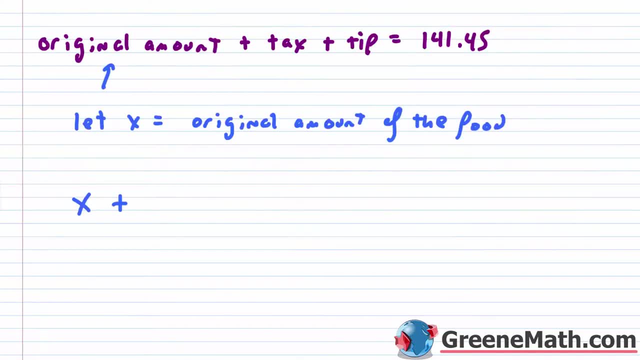 15. so the tax again is eight percent. so we're going to get this 141.45. so that's 0.08 times x. right, that's eight percent as a decimal, 0.08 again, multiply that by x, that's going to give you the tax. okay, and again, this is the original amount. 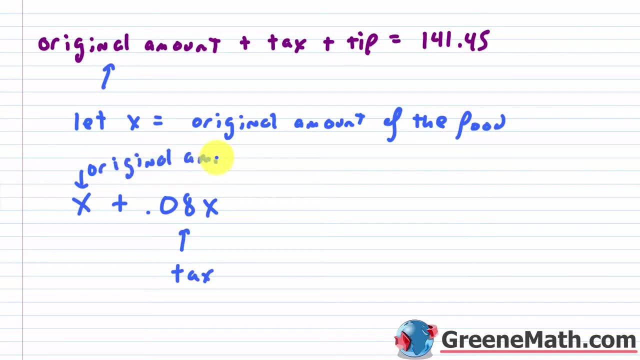 or you could say pre-tax, pre-tip amount, whatever you want to do, then plus, i've got to get my tip, and the tip is 15 of the original amount. so that's 0.15, which is 15 as a decimal times x. so this is your tip. 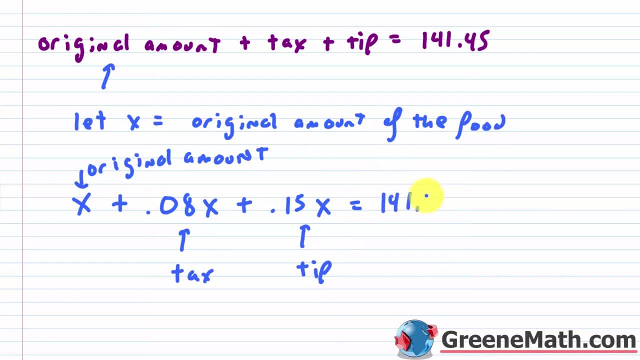 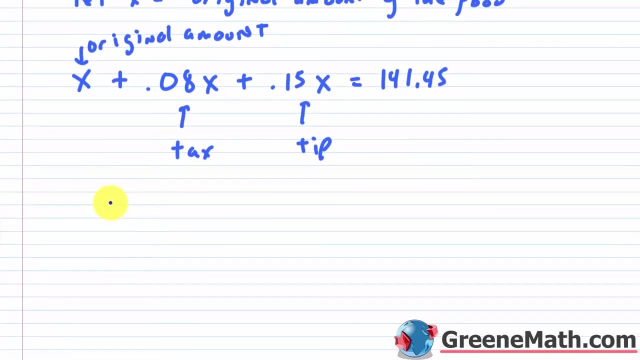 so this equals: you've got your 141.45 if i sum everything on the left. just combine like terms: what's going to happen is i'll have 1x plus 0.08x plus 0.15x, so 1 plus 0.08 plus 0.15. 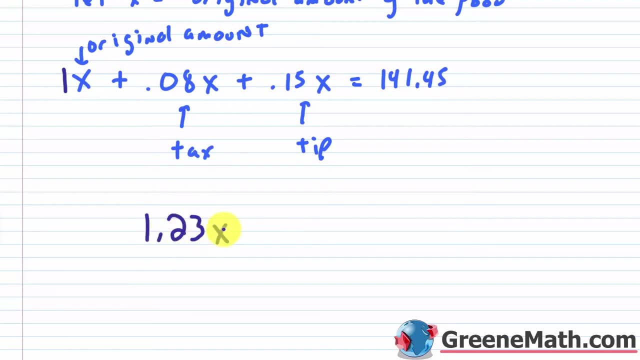 is going to be 1.23, and then times x, and again this equals 141.45. divide both sides the equation by 1.23 and what it represents is your total cost is your 141.43 times x. soiles in implication, i'll give mine. 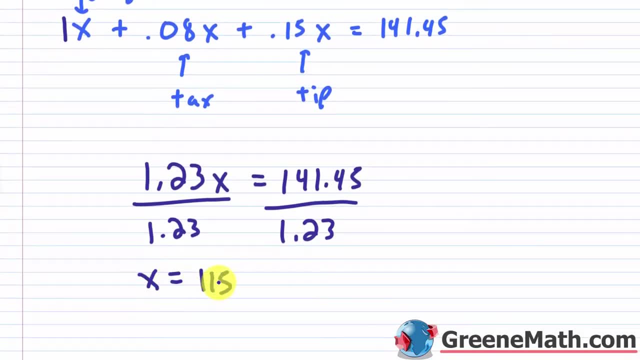 45 plus 15 plus 15 plus 1.15. so you calculate that and divide that into the equation and the total would be we going to get. We're going to get that X is equal to 115.. Okay, So that was the price of his. 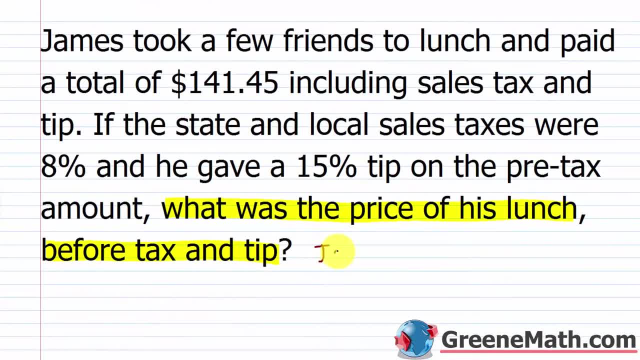 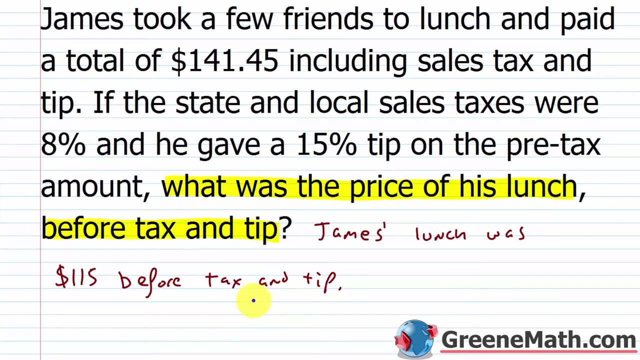 food before again the tax and the tip. So we'll say that James's lunch was $115 before tax and tip. Okay, And again, pretty easy to check this If you think about the $115 before tax and tip. So if he had $115, his tip would have been what? It would have been 15% of that. So 15% of 115 is. 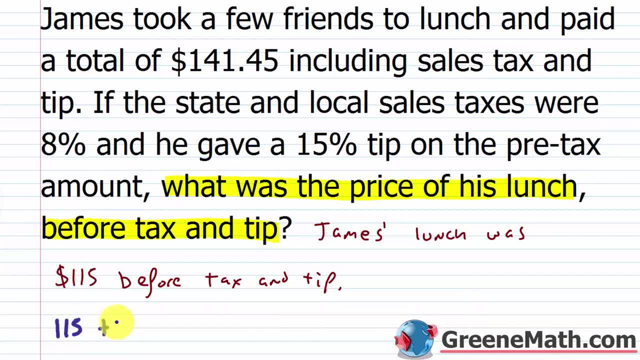 17.25.. So you'd have 115 plus 17.25.. That's your tip And then plus your sales tax, that's 8%. If you did 8% of 115, you would get 9.2.. 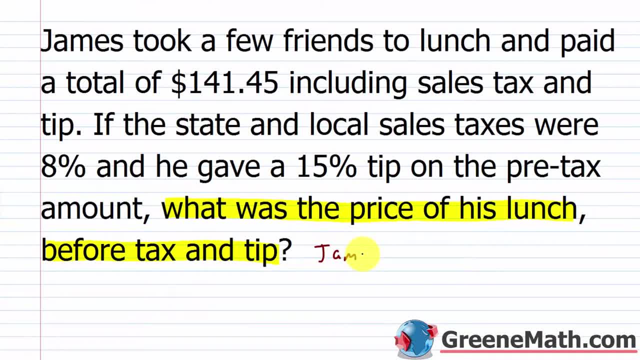 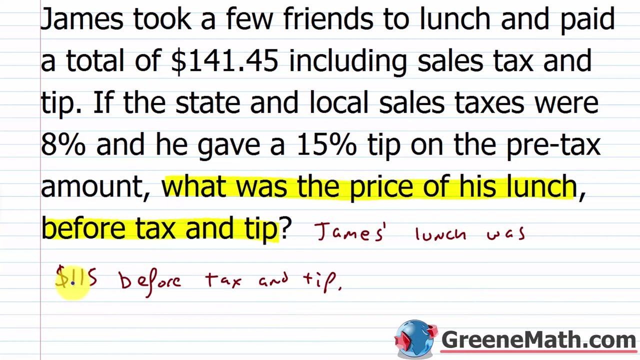 the tax and the tip. So we'll say that James's lunch was $115 before tax and tip. Okay, And again, pretty easy to check this If you think about the $115 before tax and tip. So if he had $115, his tip would have been what? It would have been 15% of that. So 15% of 115 is. 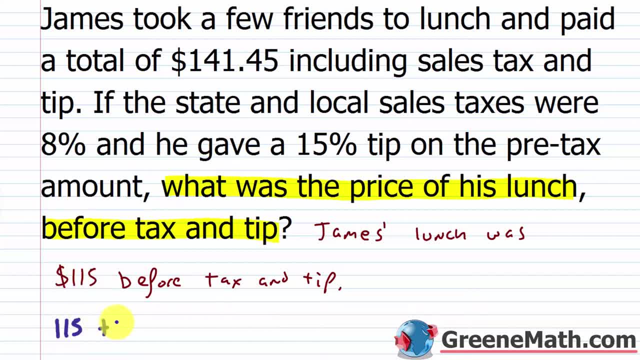 17.25.. So you'd have 115 plus 17.25.. That's your tip, And then plus your sales tax, that's 8%. If you did 8% of 115, you would get 9.2.. So if you add that up you get 9.2.. So if you add that up, 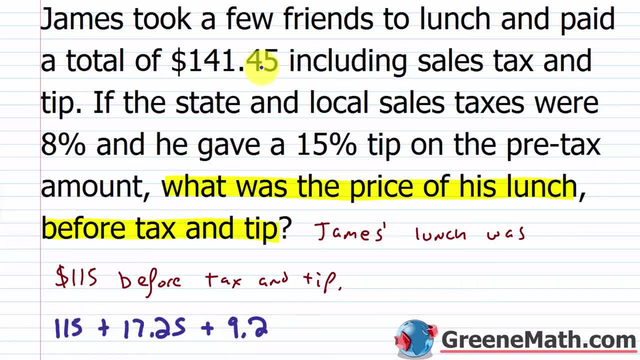 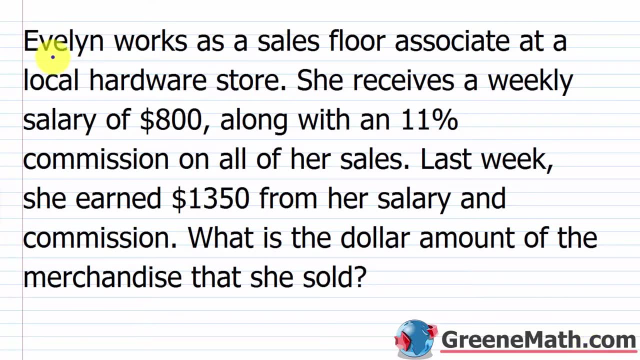 add those three amounts together you will get the 141.45.. Okay, So that tells us our solution here is correct. James's lunch, again, was $115 before tax and tip. All right, Let's take a look at one more problem. Again, these are very, very easy problems. So Evelyn works as a sales floor. 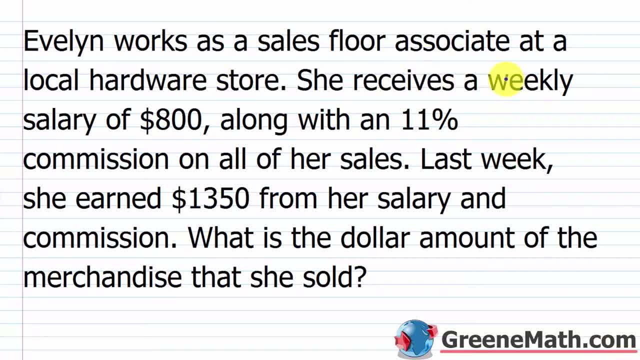 associate at a local hardware store. She receives a weekly salary of $800 along with an 11% commission on all of her sales. So last week she earned $1,350.. From her salary and commission, What is the dollar amount of the merchandise that she sold? 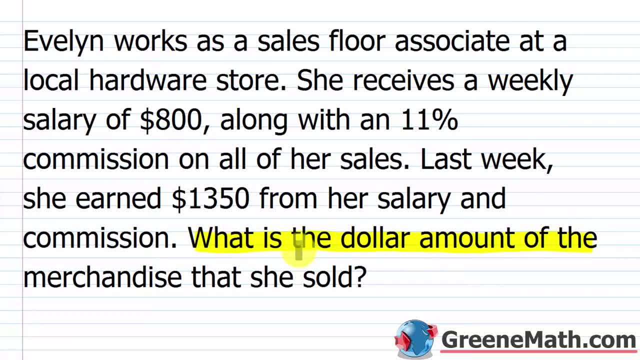 So this is what we're trying to find out: What is the dollar amount of the merchandise that she sold? Okay, Pretty easy. So again, she receives a weekly salary of $800 and she gets an 11% commission on all of her sales. Okay, Again, last week, this is what she earned. She earned $1,350.. 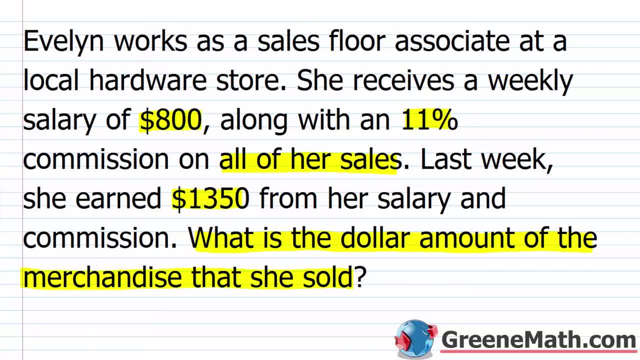 So the key to understanding this is that she's going to get that $800.. As a salary, no matter if she sells $0 or $1,000,000. Okay, It doesn't matter. She's getting a weekly salary plus commission. So if she got $1,350, I need to subtract the $800 away. 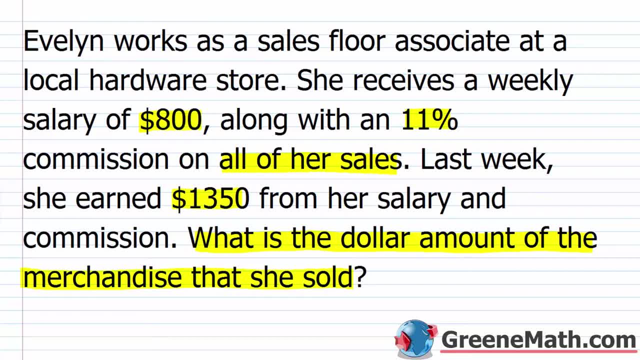 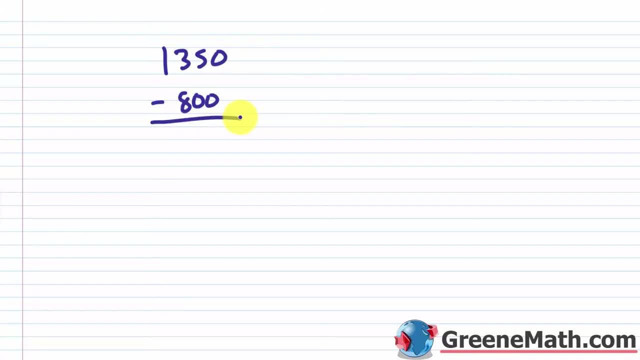 to find out what our commission was. So I would do 1,350.. Again, the total amount she got minus the $800, which is kind of the salary or the set amount she gets, no matter what. So if we subtract this away, this comes down five. 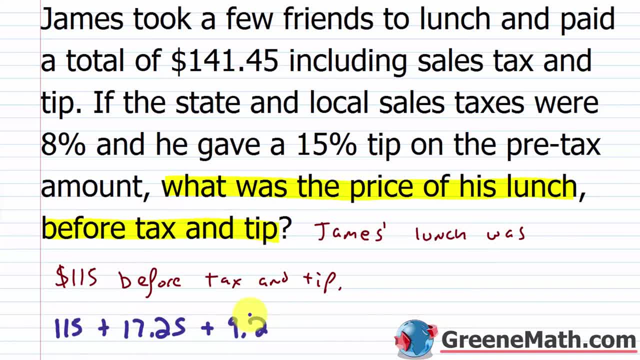 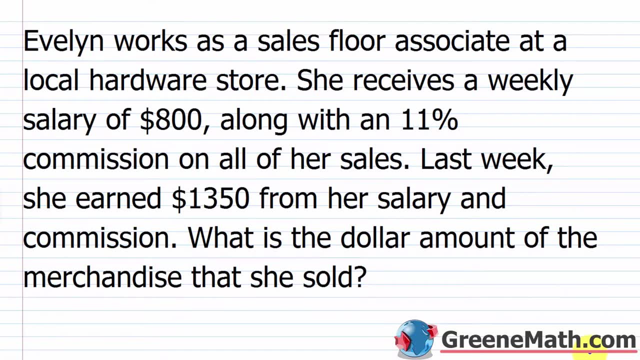 So if you add those three amounts together you will get the 141.45.. Okay, So that tells us our solution here is correct. James's lunch, again, was $115 before tax and tip. All right, Let's take a look at one more problem. Again, these are very, very easy problems. So Evelyn works as a sales. 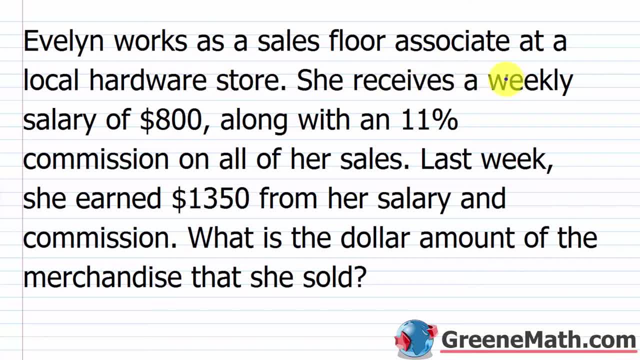 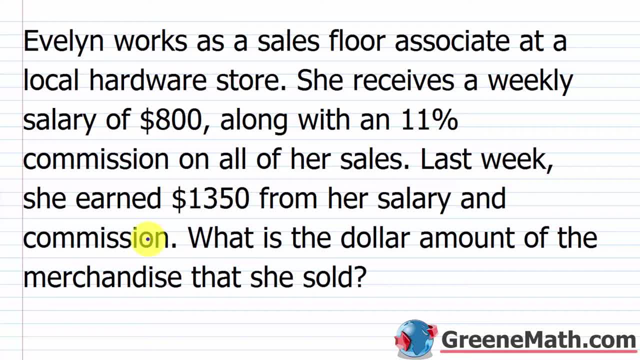 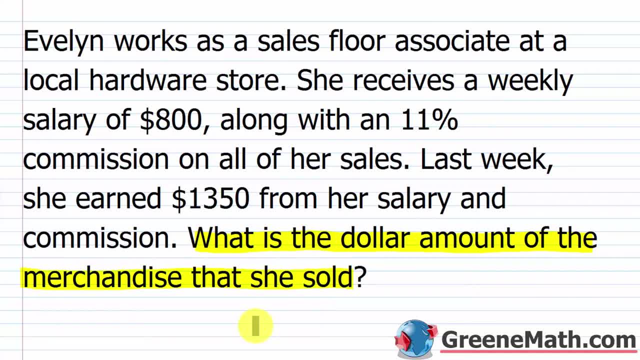 Pretty easy. So, again, she receives a weekly salary of $800 and she gets an 11% commission on all of her sales. Okay, Again, last week, this is what she earned. She earned $1,350.. So the key to understanding this is that she's going to get $115 before tax and tip, So she's 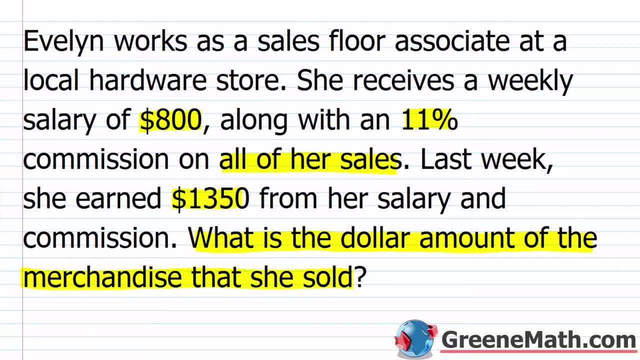 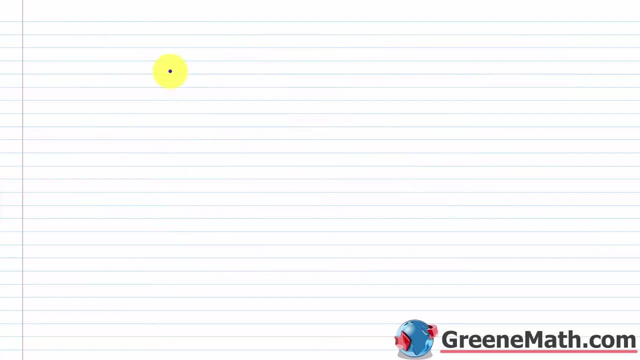 going to get that $800 as a salary, no matter if she sells $0 or a million dollars. Okay, It doesn't matter. She's getting a weekly salary plus commission. So she got $1,350.. I need to subtract the $800 away to find out what our commission was, So I would do $1,350. Again. 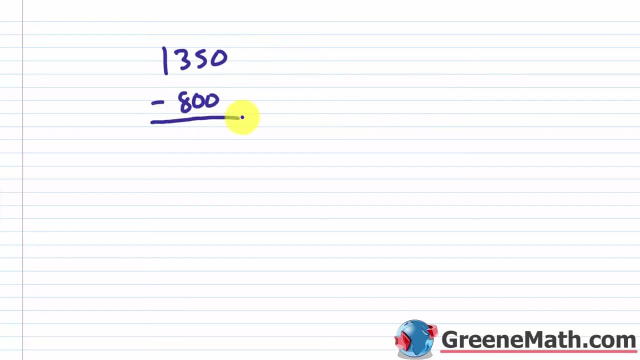 the total amount she got minus the $800, which is kind of the salary or the set amount she gets, no matter what. So if we subtract this away, this comes down Five. borrow here: 13 minus eight is five, So she's got $550 from commission. 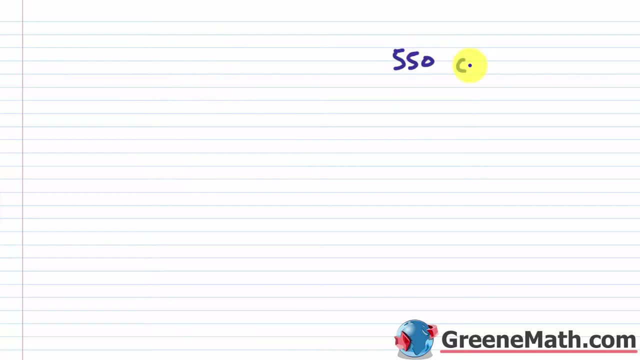 So $550 from commission. Okay. So how much was her commission rate? Again, it was 11%. Okay, So it's 11% for the commission rate. So what this means is that she has some amount of goods sold. Let's just say it's X, So let X be equal to the amount. 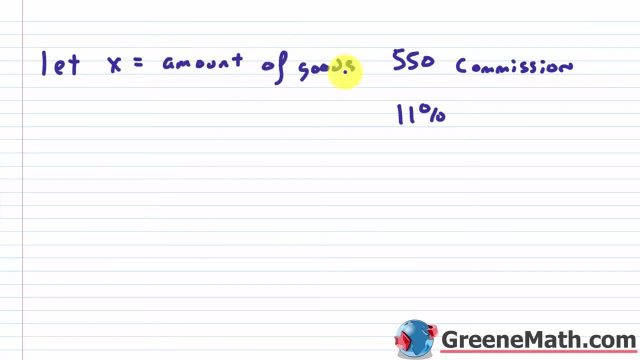 Of goods sold Okay By her. So if I take X and I multiply it by 11%, that would give me the amount of commission she made, which we know is $550.. So as a decimal, 11% is 0.11.. So 0.11,. 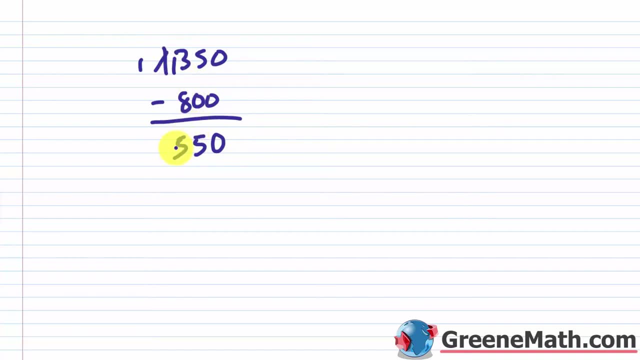 borrow here: 13 minus eight is five, So she's got $550 from commission. So $550 from commission, Okay. So how much was her commission rate? Again, it was 11%. Okay, So it's 11% for the commission rate. So what this means is that she has some amount. 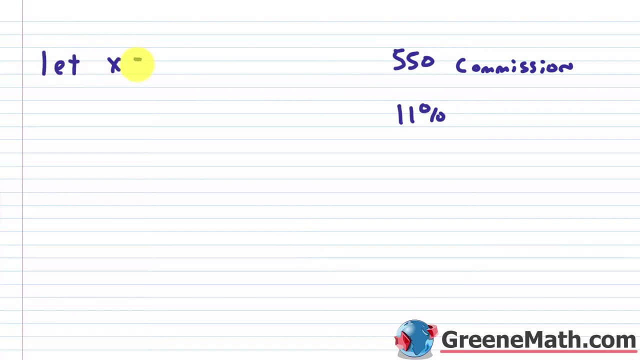 of goods sold. Let's just say it's X. So let X be equal to the amount of goods sold. Okay, By her. So if I take X and I multiply it by 11%, that would give me the amount of commission she made, which we know is $550.. So, as a decimal, 11% is 0.11.. So 0.11, then. 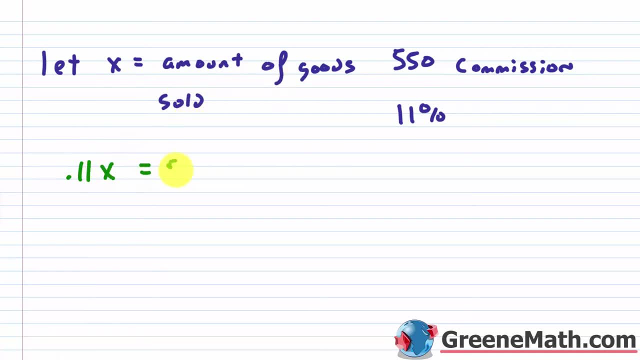 times X, again, the amount of goods she sold should be equal to $550.. Okay, That's again the amount of commission she received. If I divide both sides of the equation by 0.11, I'm going to get that X is equal to 5,000.. Okay, So this is what she sold in merchandise. Okay, 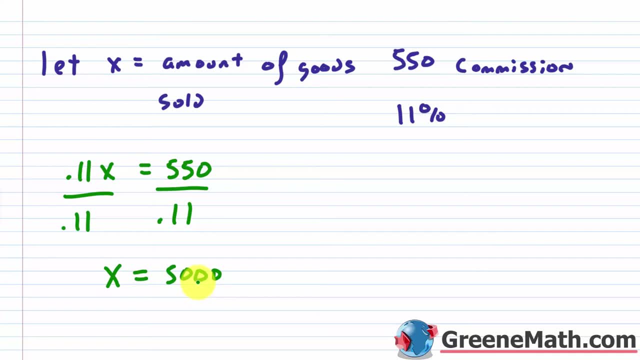 If she sold $5,000 worth of stuff and she got an 11% commission on it, she would get $550 in commission. You can check that in your head: 5,000 times 11% is 550.. Again, that's what we. 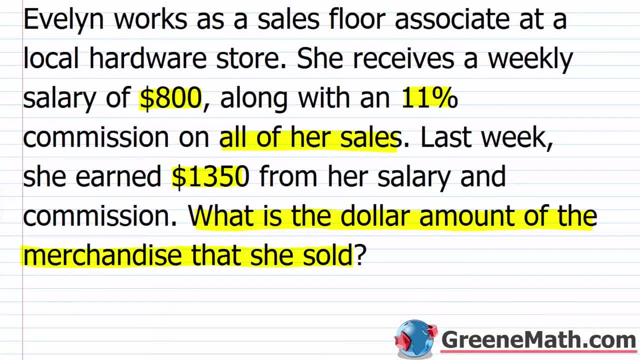 said she got in commission. So let's go ahead and write our solution as a sentence. Let's change my marker here And I'll say that she sold $5,000 worth of merchandise. If you want to check this, it's pretty easy. You can check it almost in your head if you wanted to. 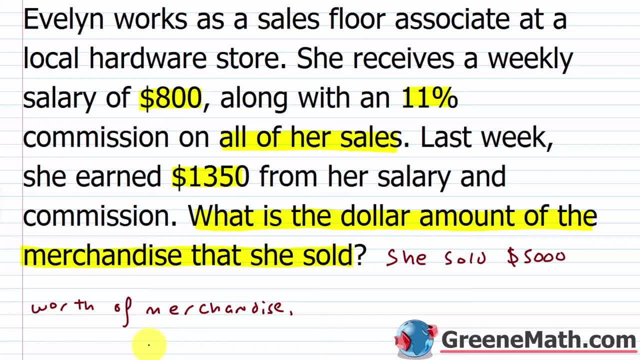 Again, she got a total of $1,350 from her salary and commission. It says right here that her salary was $800.. Okay, So again, take the salary out. That's going to give you $550 that she got from commission. Now, if she sold $5,000 worth of merchandise, that's going to give you $550. 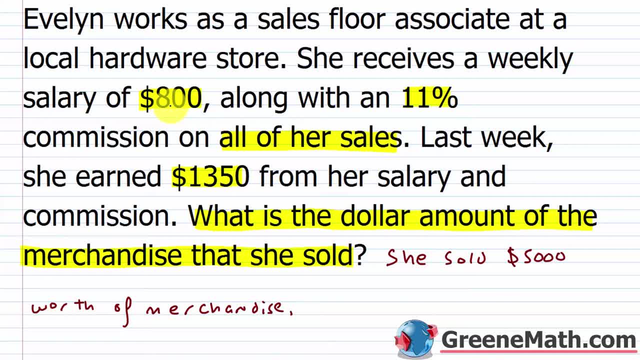 $5,000 worth of merchandise and she gets an 11% commission Again. you can check that really quickly and say, okay, well, 5,000 times 0.11 would give you 550.. So our answer here is correct. 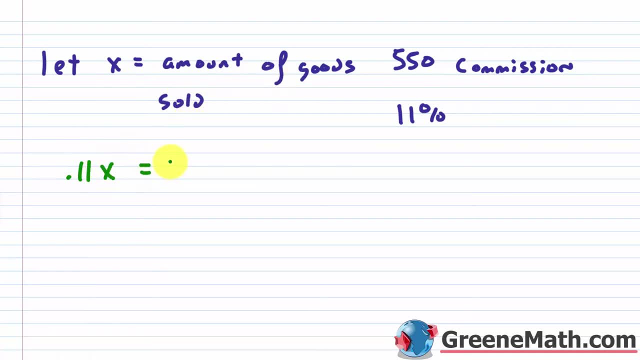 then times X again, the amount of goods she sold should be equal to $550.. Okay, That's again the amount of commission she received. If I divide both sides of the equation by 0.11, I'm going to get that X is equal to 5,000.. Okay, So this is what she sold in merchandise. Okay, 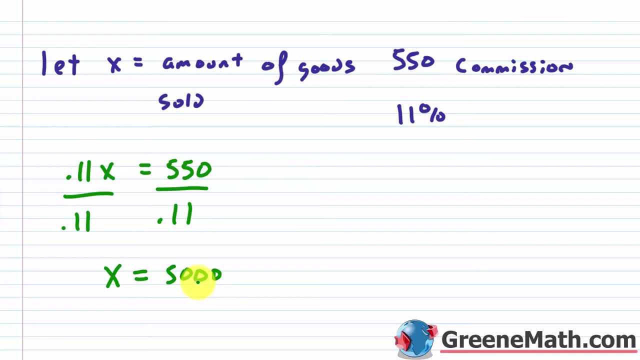 If she sold $5,000 worth of stuff and she got an 11% commission on it, she would get $550 in commission. You can check that in your head: 5,000 times 11% is 550.. Again, that's what we. 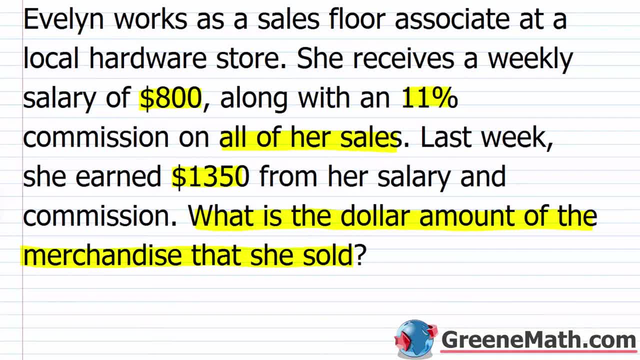 said she got in commission. So let's go ahead and write our solution as a sentence. Let's change my marker here And I'll say that she sold $5,000.. So let's go ahead and write our solution as a sentence. Let's change my marker here And I'll say that she sold $5,000.. And I'll say that she sold. 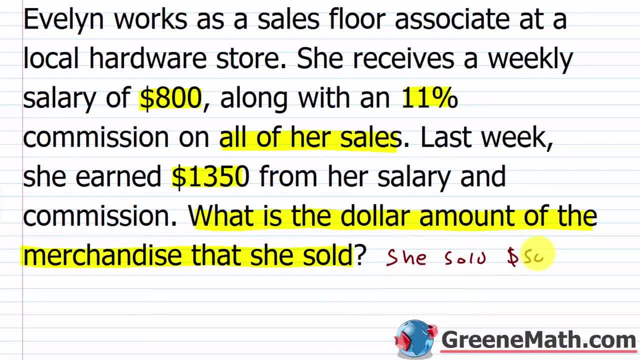 $5,000 worth of merchandise. If you want to check this, it's pretty easy. You can check it almost in your head if you wanted to. Again, she got a total of $1,350 from her salary and commission. It says right here that her salary was $800.. Okay, So again, take the salary out. 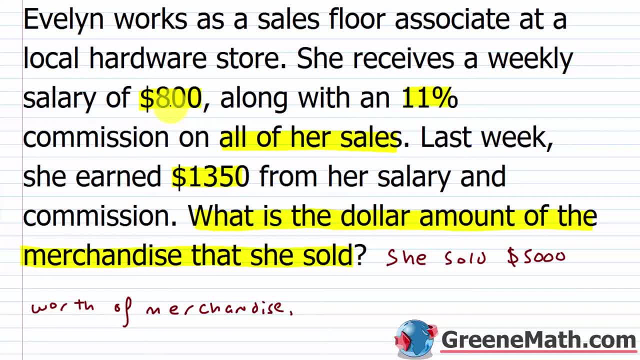 That's going to give you $550 that she got from commission. Now if she sold $5,000 worth of merchandise and she gets an 11% commission again, you can check that really quickly and say, okay, well, 5,000 times 0.11 would give you 550.. So our answer here: 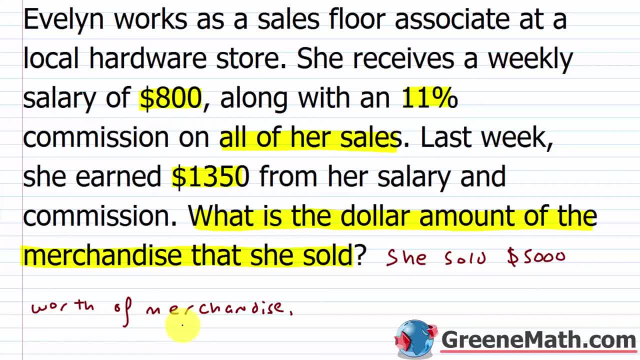 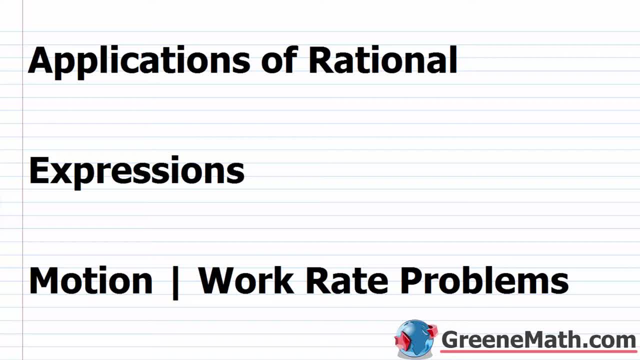 is correct. Again, she sold $5,000 worth of merchandise. In this lesson we want to review applications of rational expressions And specifically here we're going to look at some motion and some work rate problems. So at this point you should be pretty comfortable with. 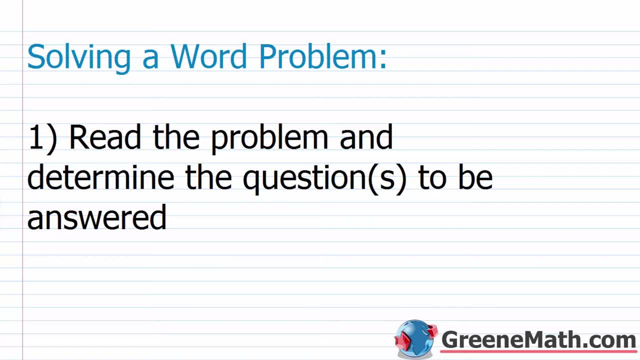 solving work problems, And although some problems are pretty easy to solve, you should be pretty comfortable with solving them. If we have some problems in the section that will not result in linear equations, we can still rely on our little six-step procedure that we used in our section on. 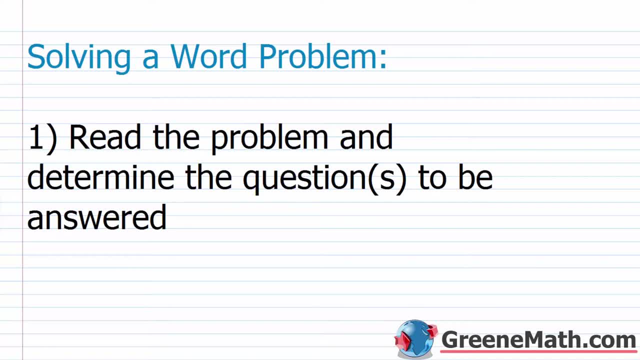 applications of linear equations. So again, for solving a word problem, the first thing we want to do is read the problem and determine the question or questions to be answered. Then the next thing we want to do is assign a variable to represent the unknown And for the scenarios we're 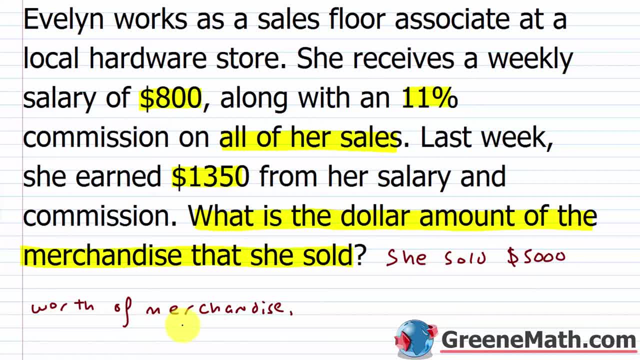 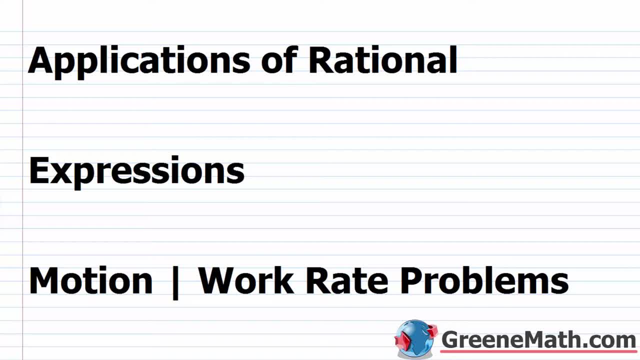 Again she sold $5,000 worth of merchandise. In this lesson we want to review applications of rational expressions And specifically here we're going to look at some motion and some work rate problems. So at this point you should be pretty comfortable with solving. 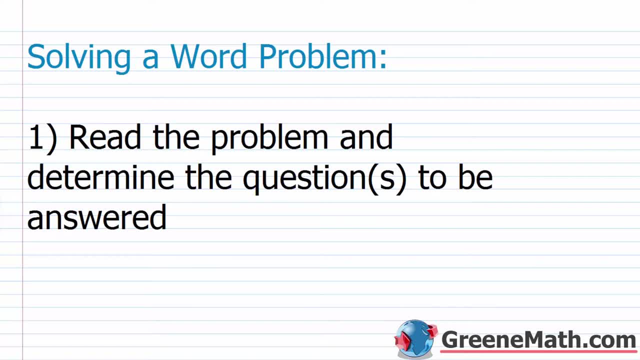 work problems, And although some problems in this section will not be solved, you should be able to solve them. So again, for solving a word problem, the first thing we want to do is read the problem and determine the question or questions to be answered. Then the next thing we want to do is: 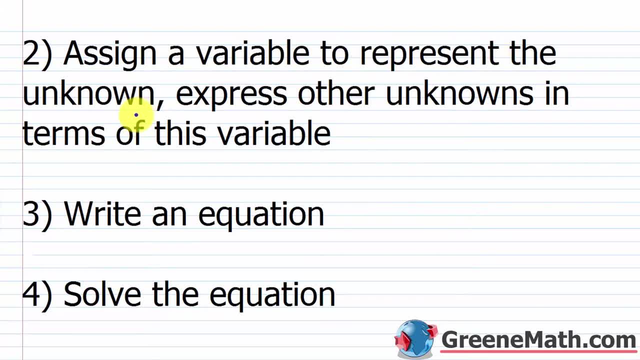 assign a variable to represent the unknown And for the scenarios we're going to have today, we can express other unknowns in terms of this variable. Then the next thing we want to do is write an equation, And this is based on the scenario we're given. Then we want to solve the 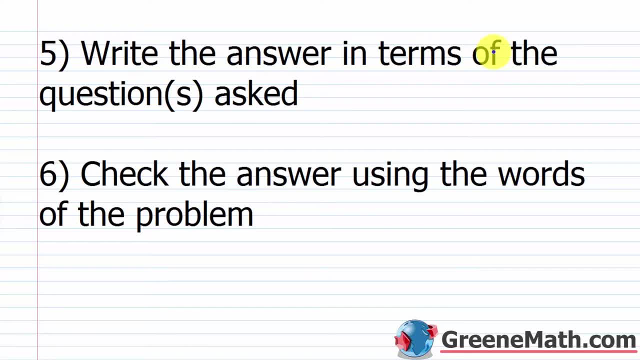 equation, Then we want to write the answer in terms of the question or again, questions asked. Then, lastly, we want to check the answer using the words of the problem. Just make sure that things are reasonable. So if you're in the section on applications of rational expressions, 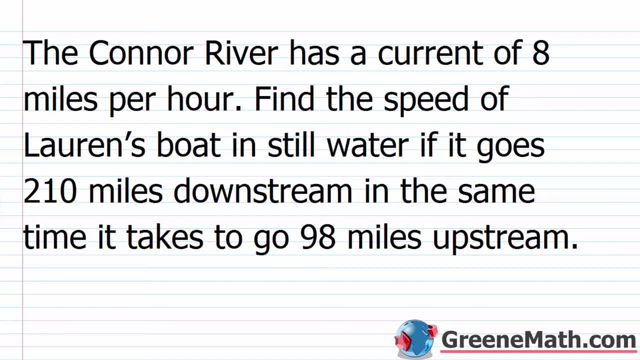 the most common problems you're going to see are going to be work rate problems, or some people call them rate of work problems. Or you're going to see motion word problems. right, These involve again the distance. This formula, distance, equals rate of speed, times, time, travel. So we talked about this formula when 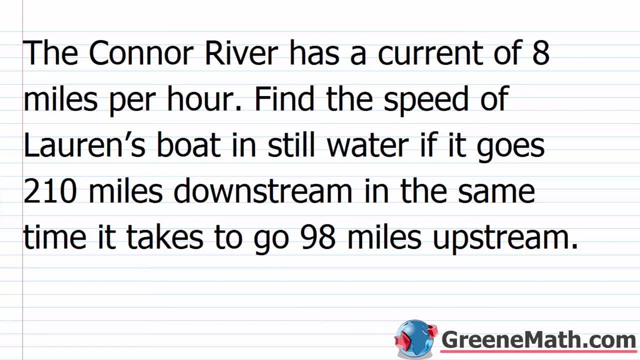 we looked at applications of linear equations. So we see it again And we'll see this throughout our course many times. So again, if you don't know, the formula d for distance is equal to r for rate times, t for time. So if I'm going 40 miles per hour and I do this for three hours, 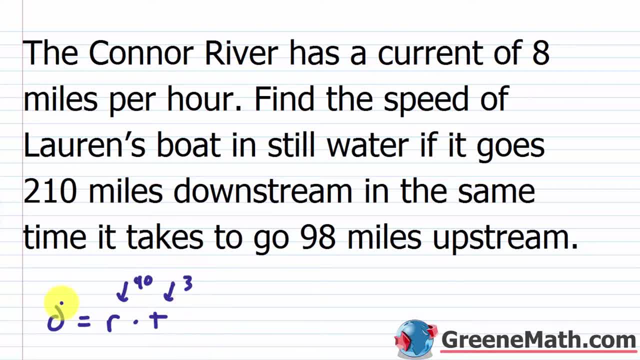 I multiply 40 times three, That gives me my distance of 120 miles. Okay, so this would be 120 in that case. So pretty easy formula to understand, Very, very intuitive, And we're just going to use it to kind of solve this first problem. 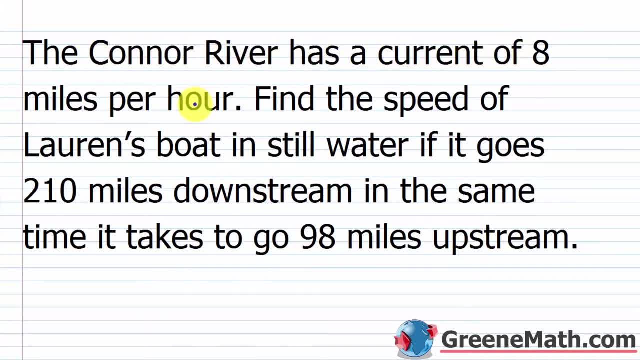 So the Connor River has a current of eight miles per hour. Find the speed of Lauren's boat in still water if it goes 210 miles downstream. in the same time it takes to go 98 miles upstream. Okay, so what are we being asked for? We're being asked to. 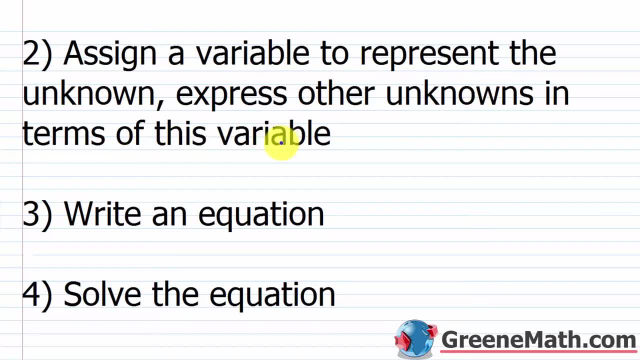 going to have today, we can express other unknowns in terms of this variable. Then the next thing we want to do is write an equation, And this is based on the scenario we're given. Then we want to solve the equation. Then we want to write the answer in terms of the question. 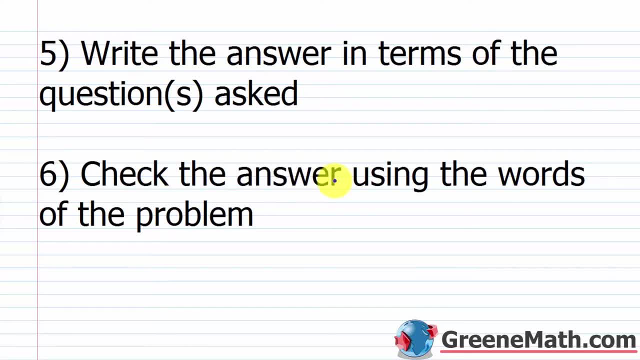 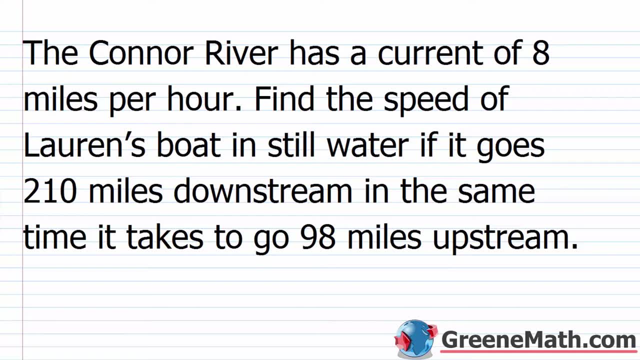 or again questions asked. Then, lastly, we want to check the answer using the words of the problem. Just make sure that things are reasonable. So if you're in the section on applications of rational expressions, the most common problems you're going to see are going to be work rate. 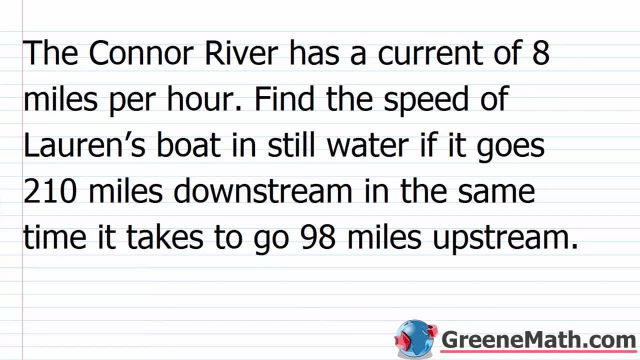 problems, or some people call them rate of work problems, or you're going to see motion word problems. These involve again the distance formula. Distance equals rate of speed, times, time travel. So we talked about this formula when we looked at applications of linear equations. So we see: 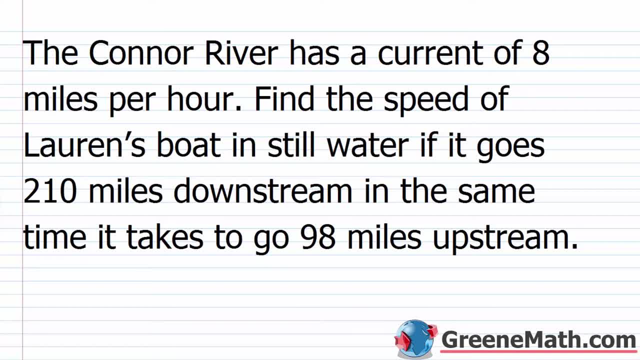 it again, And we'll see this throughout our course many times. So again, if you don't know, the formula d for distance is equal to r for rate times, t for time. So if I'm going 40 miles per hour and I do this for three hours, I multiply 40 times three. 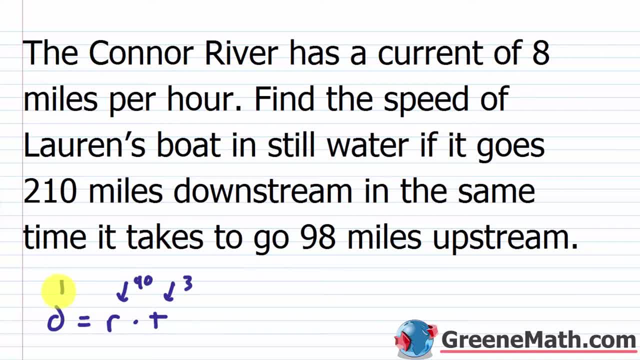 That gives me my distance of 120 miles. So this would be 120 in that case. So pretty easy formula to understand, Very, very intuitive, And we're just going to use it to kind of solve this first problem. So the Connor River has a current of eight miles per hour. Find the speed of Lauren's. 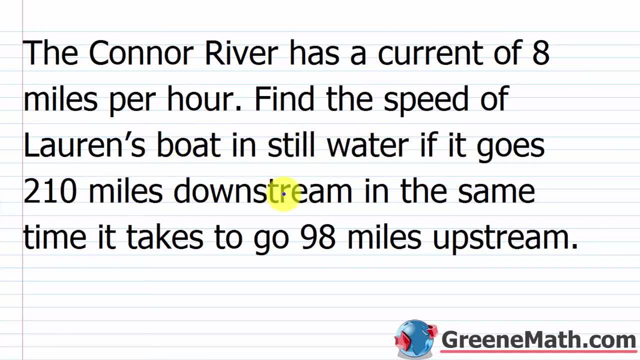 boat in still water if it goes 210 miles downstream, in the same time it takes to go 98 miles upstream. Okay, So what are we being asked for? We're being asked to find the speed of Lauren's boat in still water. Okay, This is what we need to. 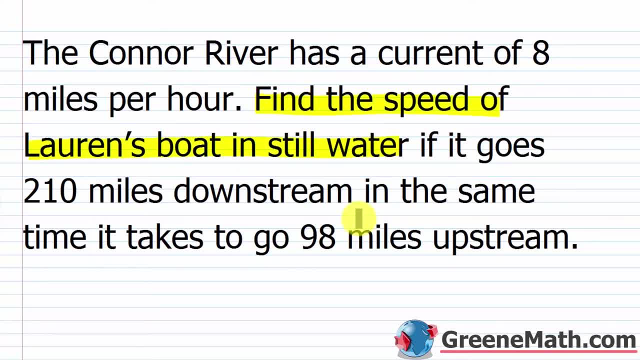 find. Now we're given a lot of information to help us find this. It tells us the Connor River has a current of eight miles per hour. It also tells us that her boat can go 210 miles downstream in the same time it takes to go 98 miles upstream. So when you get these type of problems, 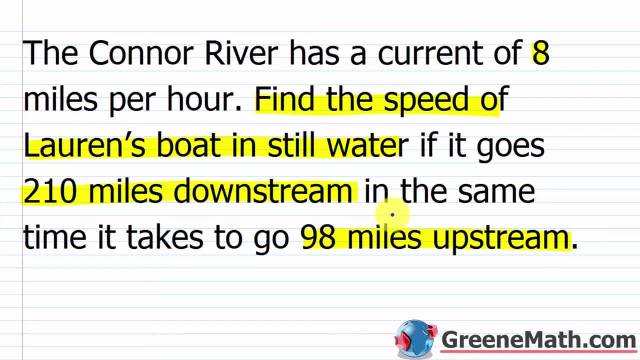 you need to understand the difference between still water upstream and downstream Okay. So the way these problems work: if you're in still water, basically there's no current Okay. If you're going upstream, you are fighting the current Okay, So you have to subtract the 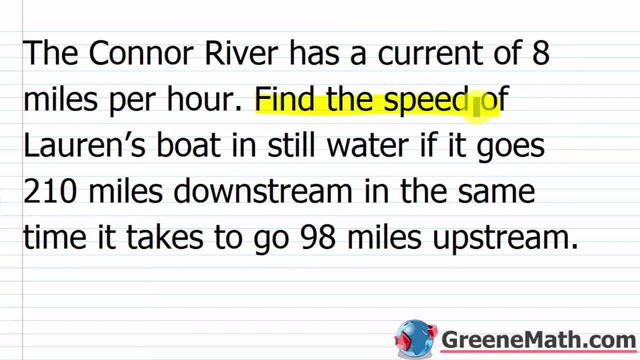 find the speed of Lauren's boat in still water. Okay, this is what we need to find Now. we're given a lot of information to help us find this. It tells us the Connor River has a current of eight miles per hour. It also tells us that her boat can go 210 miles downstream. 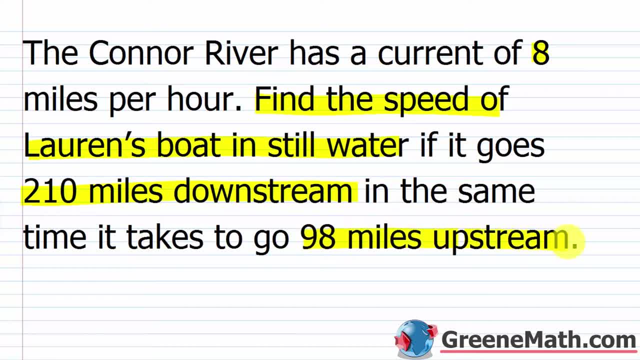 in the same time, it takes to go 98 miles upstream. So when you get these type of problems, you need to understand the difference between still water upstream and downstream. Okay, so the way these problems work is that we're going to find the speed of Lauren's boat in still water. 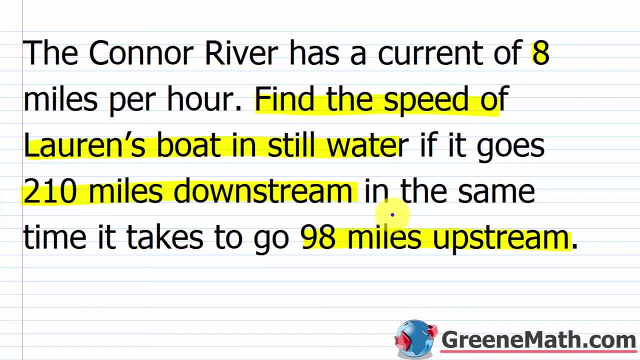 If you're in still water, basically there's no current. Okay, if you're going upstream, you are fighting the current. Okay, so you have to subtract the speed of the current away from the speed of the boat in still water. If you're going downstream, the current is pushing. 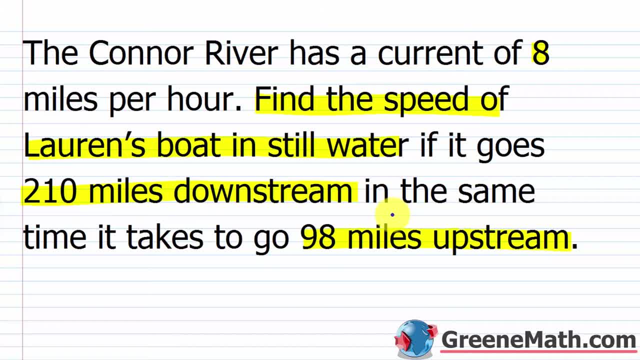 on you. Okay, so you're going with the current, And so now you need to add the speed of the current to the speed of the boat in still water. Okay, so we'll talk about that more in a second. For right now, our next step is to what It's to assign a variable to. 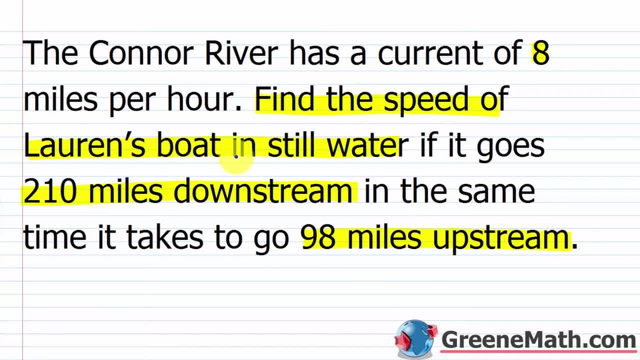 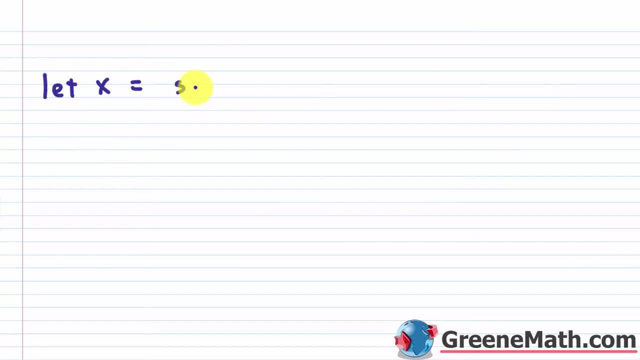 represent the unknown. Our unknown here is the speed of Lauren's boat in still water, So I'm just going to let x be equal to that. So let's let x be equal to the speed of Lauren's boat in still water. Okay, so that's water with no current, All right, so let's take this. 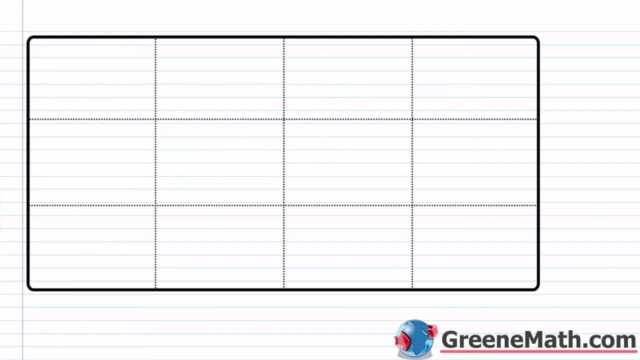 down to a little table so we can organize our information. So the first thing I'm going to do is put my distance formula up here Again. d stands for distance, And this is equal to r, which stands for rate of speed, multiplied by t, which stands for time travel. Okay, 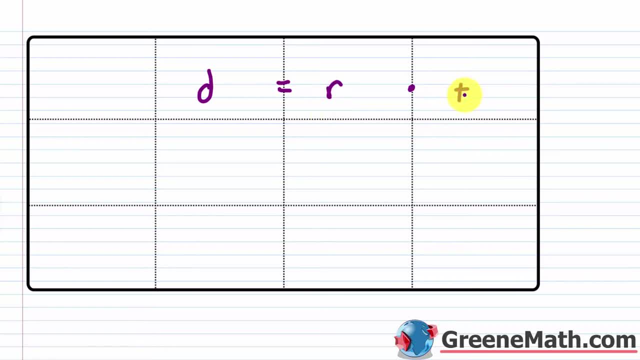 again, if I'm moving at 40 miles per hour and I do this for three hours, 40 times three is 120. So I know it would go 120 miles. Okay, it's a very intuitive form. So I'm just going to put my two scenarios over here on the left, So we have upstream. 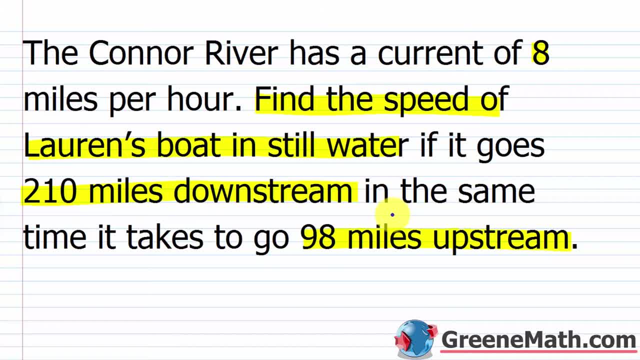 speed of the current away from the speed of the boat in still water. If you're going downstream, the current is pushing on you. Okay, So you're going with the current, And so now you need to add the speed of the current to the speed of the boat in still water. Okay, So we'll talk. 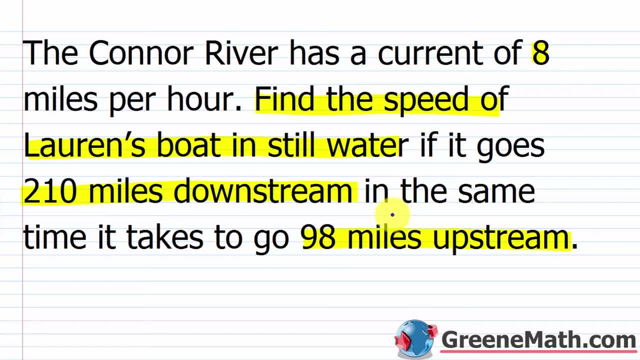 about that more in a second, For right now, our next step is to what It's to assign a variable to represent the unknown. Our unknown here is the speed of Lauren's boat in still water, So I'm just going to let X be equal to that. So let's let X be equal. 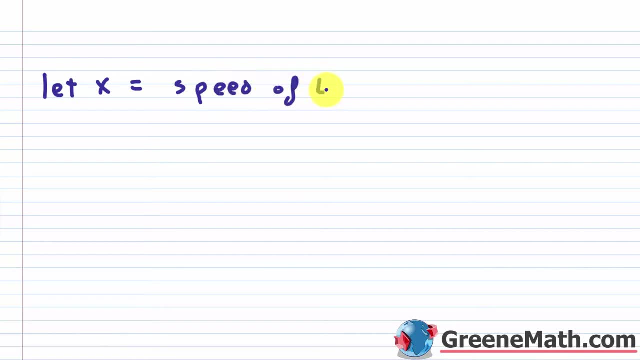 to the speed of Lauren's boat in still water. Okay, So that's water with no current, All right. So let's take this down to a little table so we can organize our information. So the first thing I'm going to do is put my distance formula up here Again. D stands for. 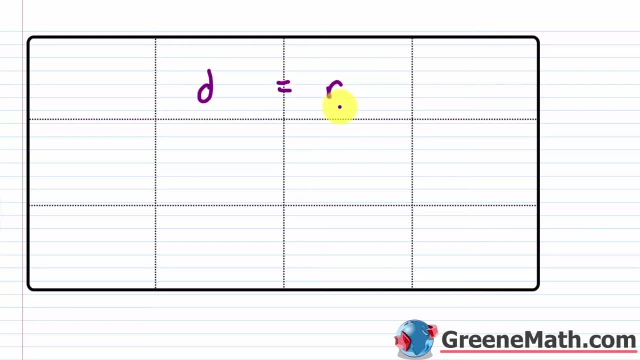 distance, And this is equal to R, which stands for rate of speed, multiplied by T, which stands for time travel. Okay, Again, if I'm moving at 40 miles per hour and I do this for three hours, 40 times three is 120.. So I know it would go 120 miles. Okay, It's a very intuitive formula. 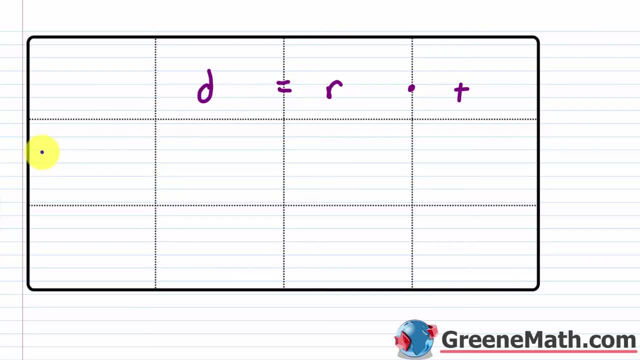 So I'm just going to put my two scenarios over here on the left. So we have upstream and we have downstream. Okay, So what am I told in the problem? Again, my rate in still water is unknown. That's what we're trying to find, But we expressed it as X, So I'm going to put X here and I'm going to put X. 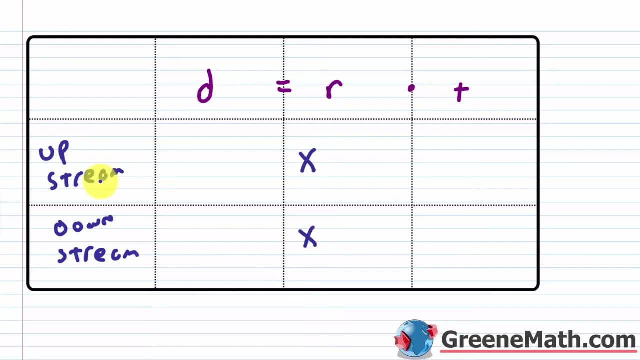 here. Now, in the case where I'm going upstream again, I'm fighting the current. The current is eight miles per hour, So I've got to subtract eight away from the speed of the boat in still water. So I subtract eight away from X. 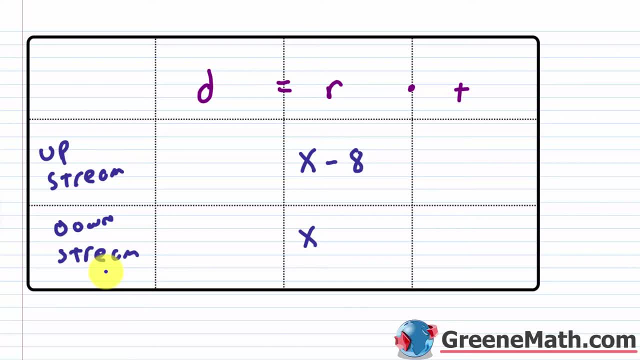 In the case of going downstream, it's the opposite right, The current's pushing on me, So I'm going to add eight or again the speed of the current to the speed of the boat in still water. So for upstream, my rate is X minus eight. For downstream, my rate is X plus eight. 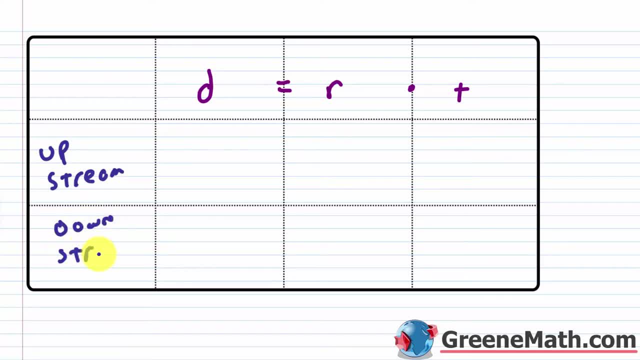 and we have downstream. Okay. So what am I told in the prop? Again, my rate in still water is unknown. That's what we're trying to find, But we expressed it as x, So I'm gonna put x here, and I'm going to put x here Now in the case where I'm going upstream. 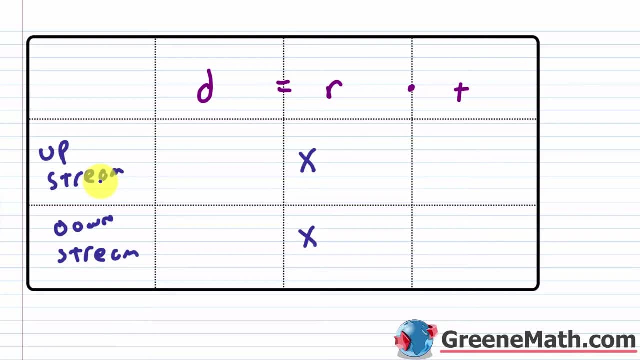 again, I'm fighting the current. the current was eight miles per hour, So I've got to subtract eight away from the speed of the boat. and still what? so I subtract eight away from x. In the case of going downstream, it's the opposite right: the current's pushing on me. so i'm going to add 8. 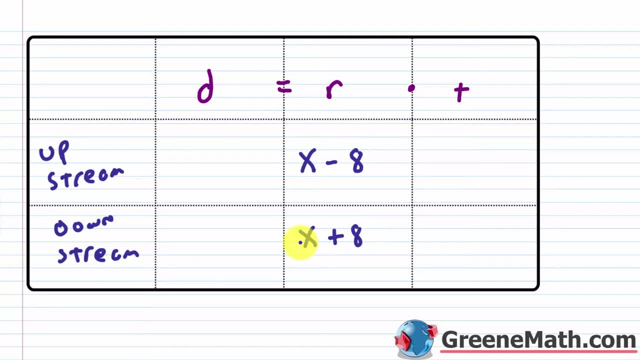 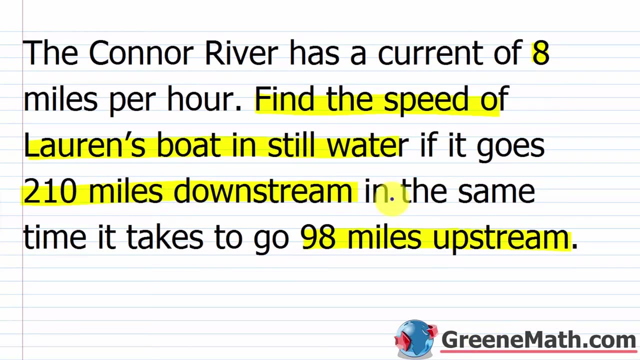 or again, the speed of the current to the speed of the boat, and still water. so for upstream, my rate is x minus 8. for downstream, my rate is x plus 8.. now, what about the distance? well, it specifically tells us that the boat goes 210 miles downstream. in the same time it takes to go 98 miles upstream. 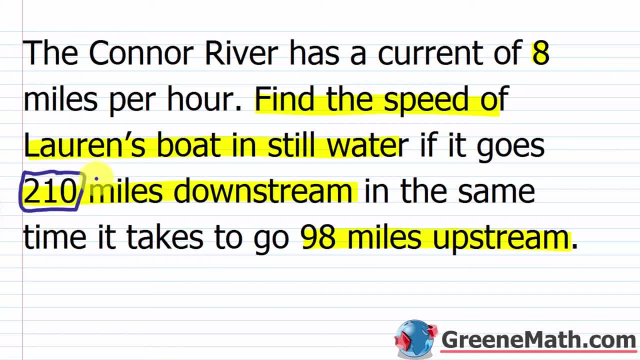 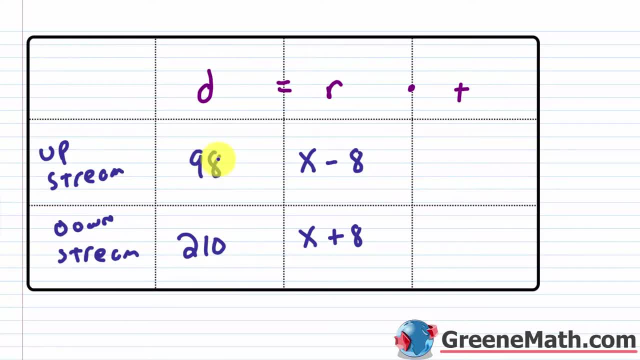 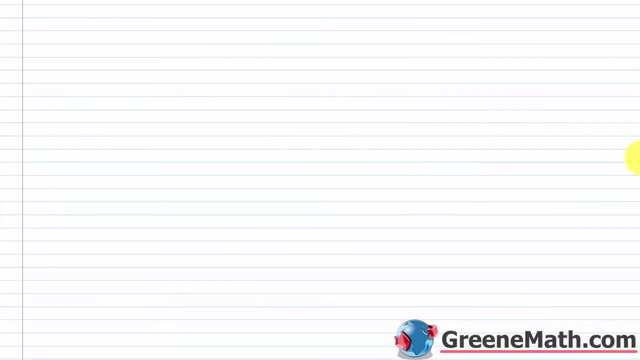 so my distance for downstream will be 210 and my distance for upstream will be 98.. so for downstream it's 210, for upstream it's 98.. okay, so now what about the time? well, to do the time, what we can do, we can solve the distance formula for time. so again, distance is equal to rate of speed times. 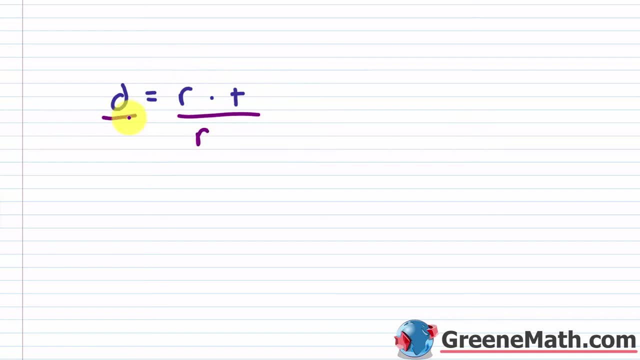 time travel. okay, so if i divide both sides by r, what's multiplying t there? we know that this would cancel. with this i basically have that time is equal to distance over rate. so right now i have a distance and i have a rate for each scenario. so if i divide my distance by my rate, i'm going to have my time. 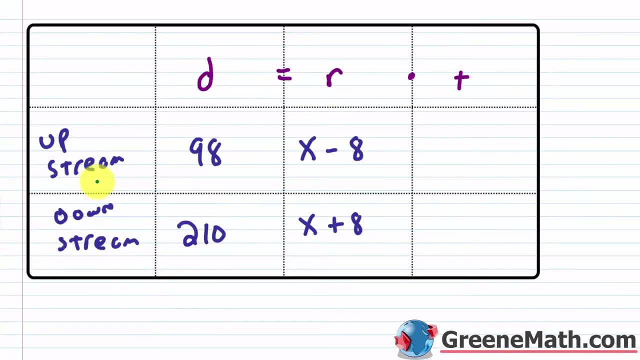 modeled okay, so let me erase this. so for upstream, my distance is 98 and my rate is x minus 8.. so the time again is distance divided by rate, so it's going to be 98 divided by x minus 8.. for downstream again, my distance is 210. 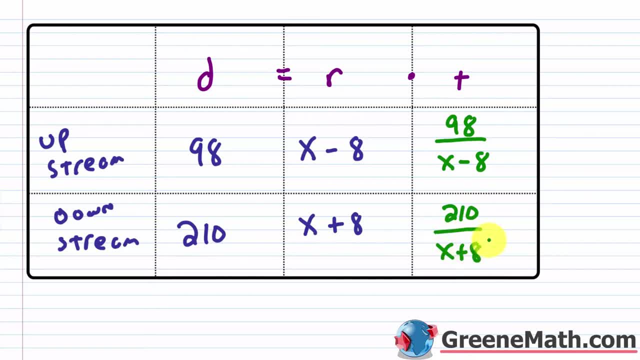 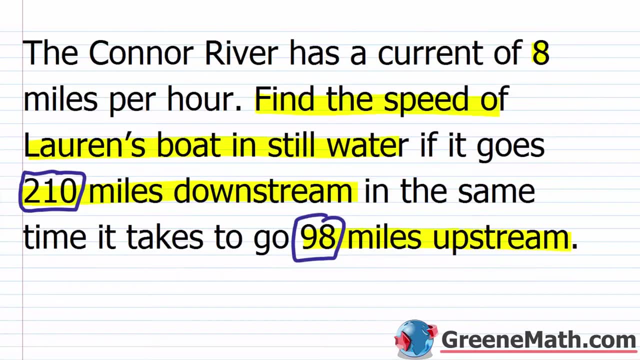 and my rate is x plus eight, so my time for downstream will be 210 over x plus eight. now it tells us in the problem- let me go back up- that the boat can go 210 miles downstream in the same time it takes to go 98 miles upstream. so all we have to do is set the two times equal to each other. 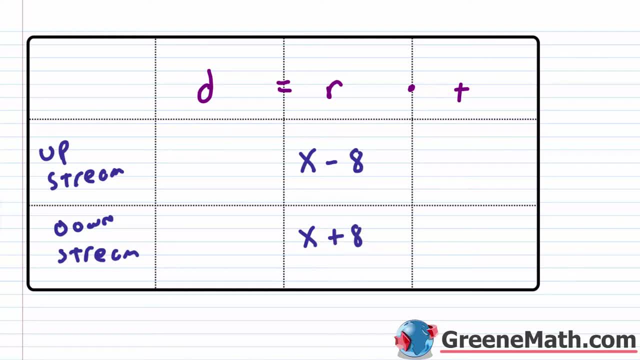 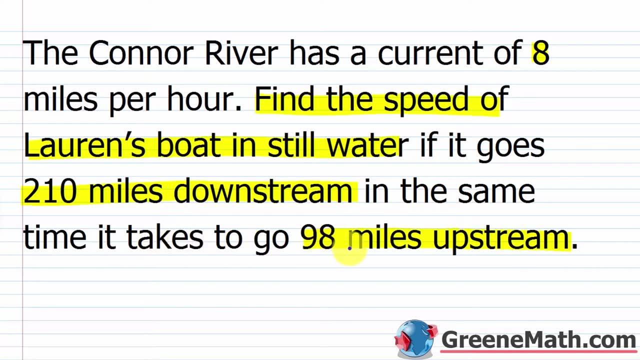 Now, what about the distance? Well, it specifically tells us that the boat goes 210 miles downstream in the same time it takes to go 98 miles upstream. So my distance for downstream will be 210.. And my distance for upstream will be 98. So for downstream it's 210.. For upstream it's 98.. 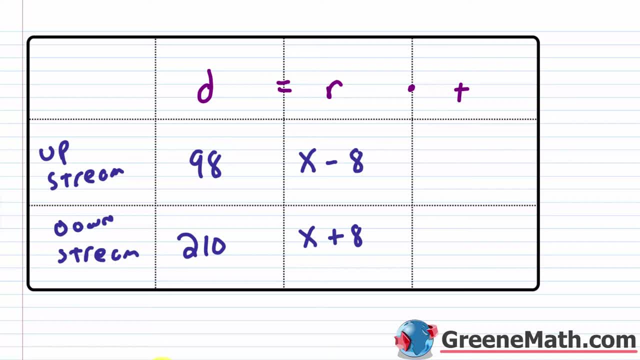 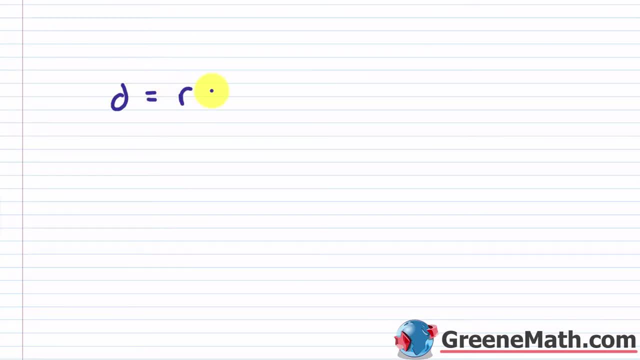 Okay. So now what about the time? Well, to do the time, what we can do, we can solve the distance formula for time. So again, distance is equal to rate of speed, times, time travel, Okay. So if I divide both sides by R, what's multiplying T? there we know that this would cancel with this. 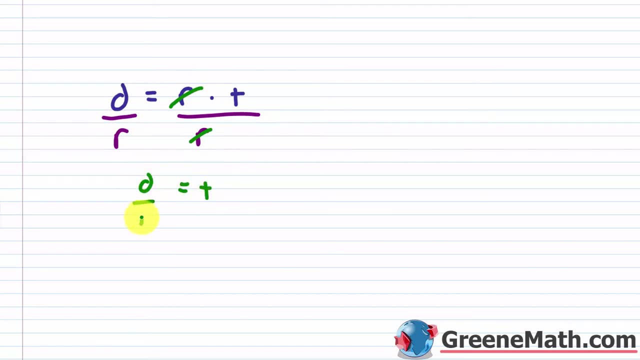 I basically have that time is equal to distance over rate. So right now I have a distance and I have a rate for each scenario. So if I divide my distance by my rate, I'm going to have my time modeled, Okay, So let me erase this. So for 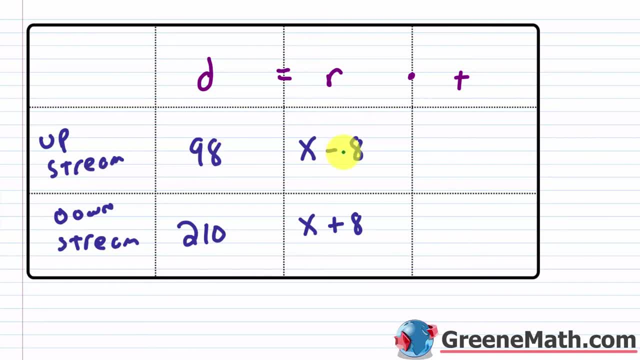 upstream, my distance is 98.. And my rate is X minus eight. So the time again is distance divided by rate. So it's going to be 98 divided by X minus eight. For downstream again, my distance is 210.. 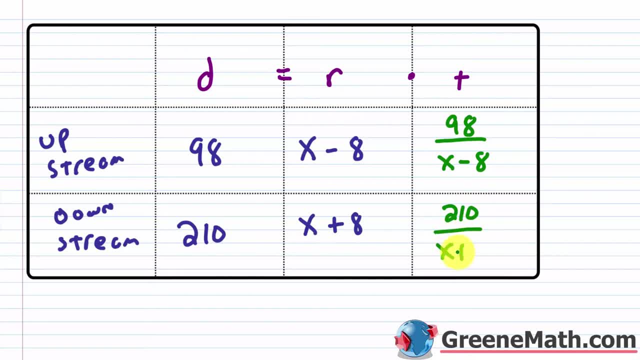 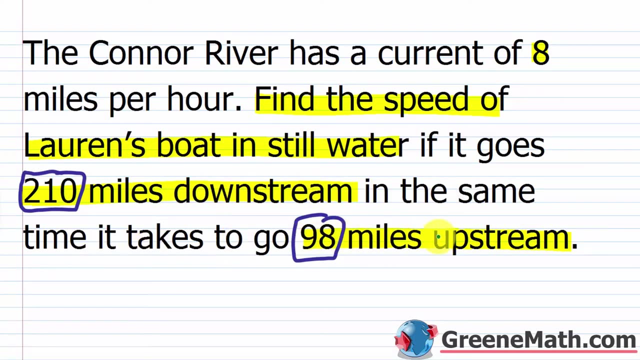 And my rate is X plus eight. So my time for downstream will be 210 over X plus eight. Now it tells us in the problem- let me go back up- that the boat can go 210 miles downstream in the same time it takes to go 98 miles upstream. So 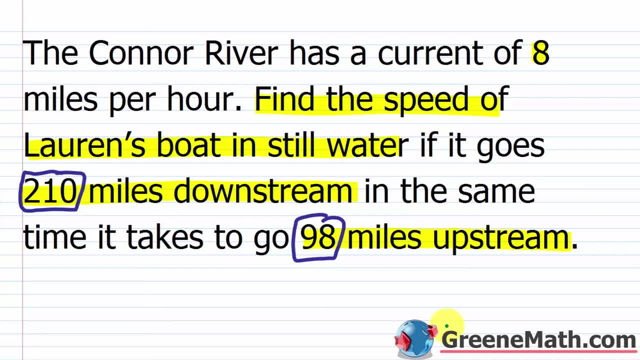 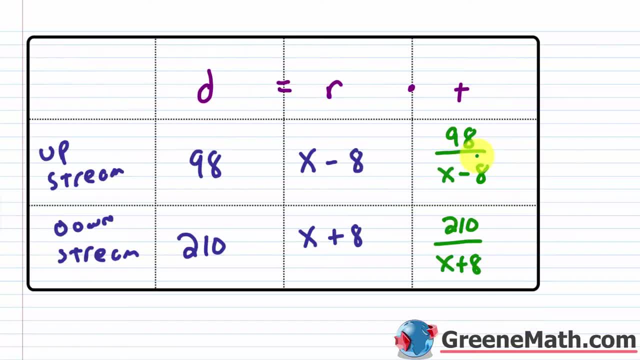 all we have to do is set the two times equal to each other, because again in the problem, it tells us that it's the same. It says in the same in the same time. Okay, So I can take 98 over X minus eight, So 98 over X minus eight. 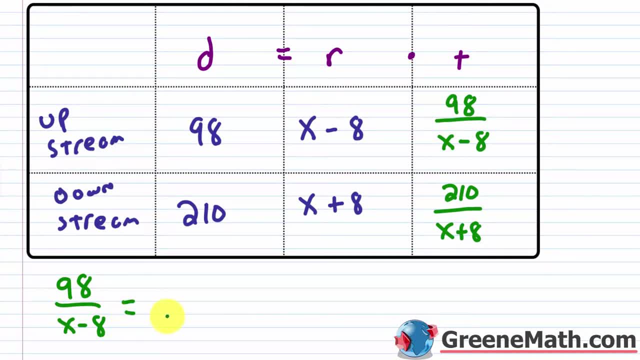 That's the time for going upstream, and set this equal to my time for going downstream, which is 210 over X plus eight. So let me just copy this. We'll go to a fresh sheet. So how can we solve this? We already know how to solve rational equations. It's very. 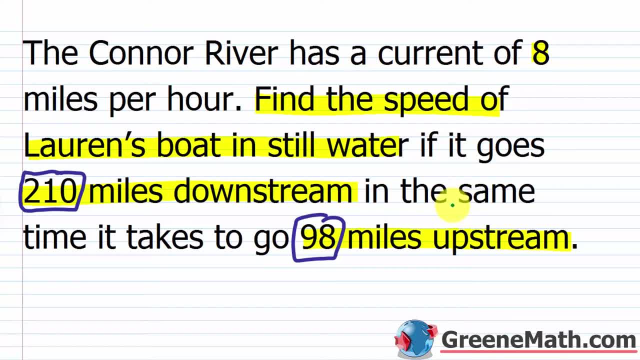 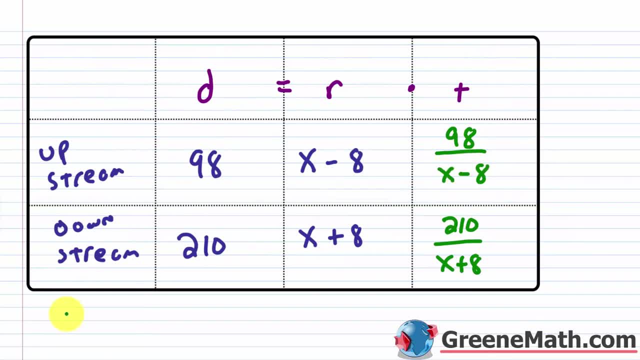 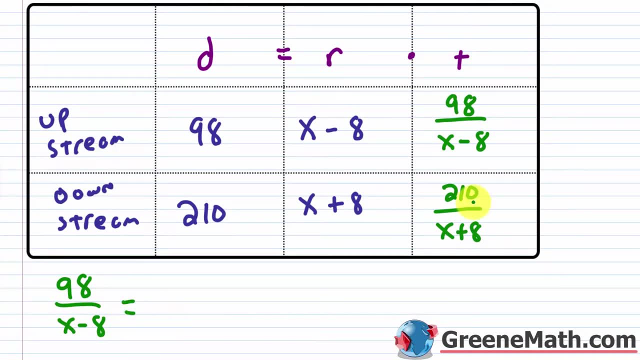 because again in the problem it tells us that it's the same. it says in the same in the same time. okay, so i can take 98 over x minus 8.. so 98 over x minus 8, that's the time for going upstream, and set this equal to my time for going. 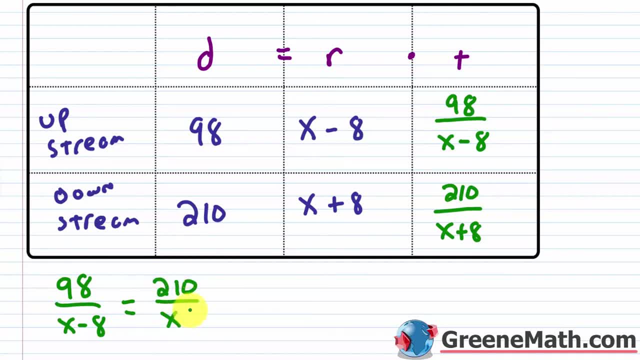 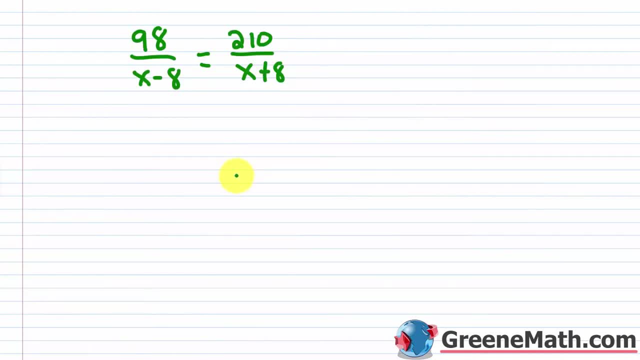 downstream, which is 210 over x plus 8.. so let me just copy this. we'll go to a fresh sheet. so how can we solve this? we already know how to solve rational equations. it's very, very easy. in this particular case, i don't need to multiply both sides by the lcd. 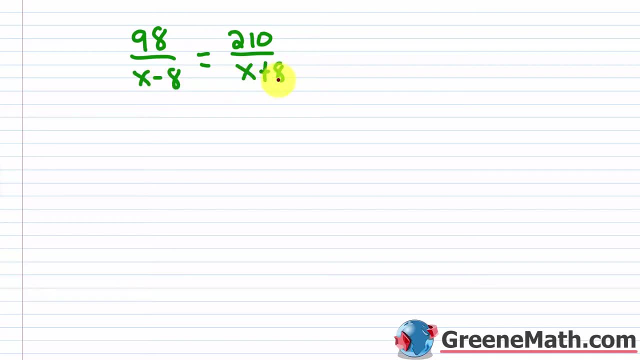 right, the lcd would be x minus 8 times x plus 8.. i could multiply both sides by that, but the trickier method here would be just to cross multiply. so you take this guy right here, multiply by this. you take this guy right here, multiply by that. so essentially what i'd have is: 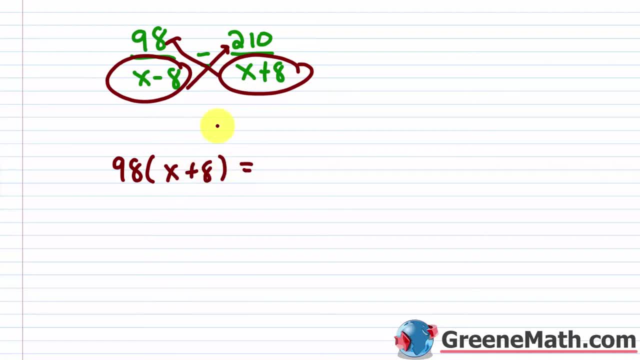 98 times the quantity x plus 8 is equal to: you'd have 210 times the quantity x minus 8.. so i could just start by using my distributive property on each side. but one thing you want to see here is that 98 and 210 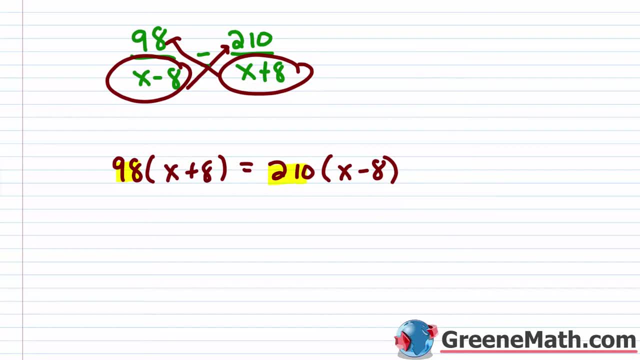 are each divisible by 14.. right, so this a little easier on myself. I'm gonna divide both sides of the equation by 14. remember, this is multiplication here, so this is legal to cancel. 98 divided by 14 is gonna give me 7, so I put a 7 here. then 210 divided by 14 is gonna give me. 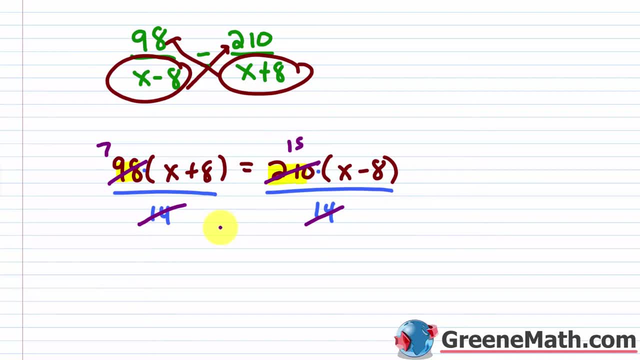 15, and now I have smaller numbers to work with, so it's just gonna make my life a lot easier. so 7 times X is 7 X, and then plus 7 times 8 is 56. this equals 15 times X is 15 X, and then minus 15 times 8 is 120. okay, so let me. 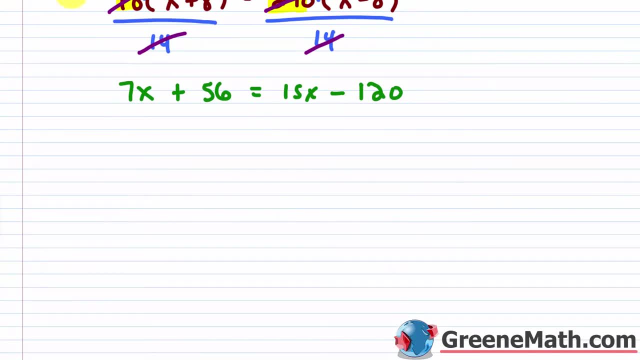 scroll down a little bit, get some room going. I can subtract 15 X away from each side of the equation and I can subtract 56 away from each side of the equation. so we know that this is gonna cancel and this is gonna cancel. 7 X minus 15 X is 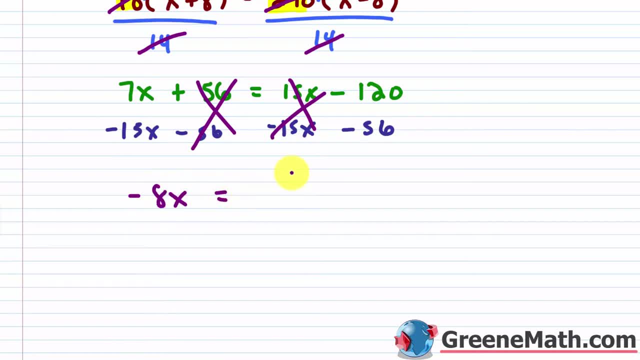 gonna give me negative 8 X and this will be equal to negative 120. minus 15 X is equal to minus 15 X. minus 15 X is equal to minus 15. X is equal to minus 56 is negative 176. if I finish this up by dividing both sides by: 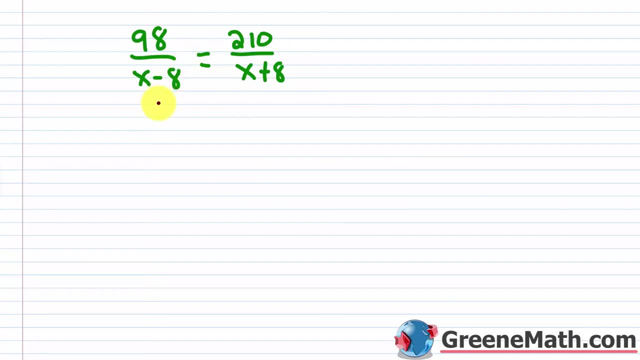 very easy. In this particular case. I don't need to multiply both sides by the LCD. right The LCD would be X minus eight times X plus eight. I can multiply both sides by that, but a quicker method here would be just to cross multiply. So you take this guy, you take this guy, you take this guy. 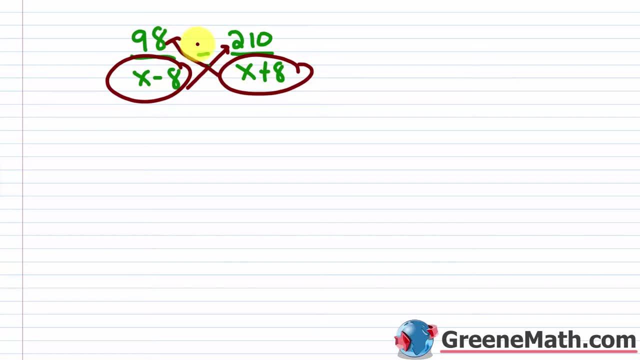 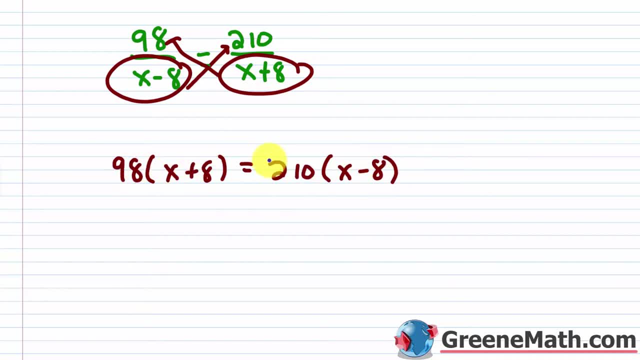 quantity X minus eight. So I could just start by using my distributive property on each side. But one thing you want to see here is that 98 and 210 are each divisible by 14, right? So to make this a little easier on myself, I'm going to divide both sides of the. 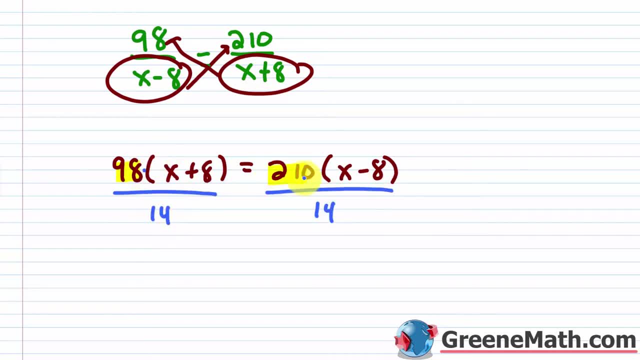 equation by 14.. Remember, this is multiplication here, So this is legal to cancel. 98 divided by 14 is going to give me seven, So I'd put a seven here. Then 210 divided by 14 is going to give me. 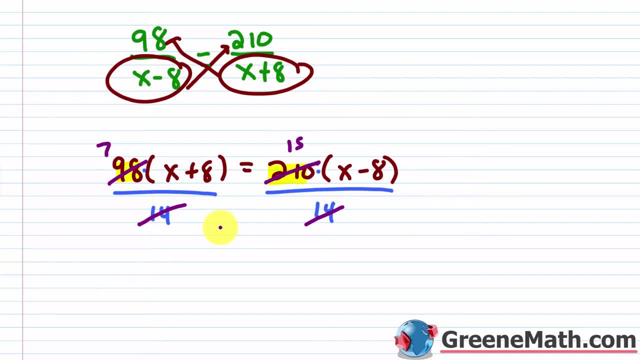 15.. And now I have smaller numbers to work with, So it's just going to make my life a lot easier. So seven times X is seven X, and then plus seven times eight is 56.. This equals 15 times X is 15 X. 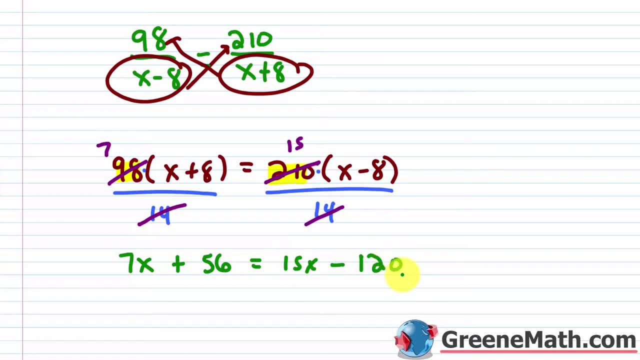 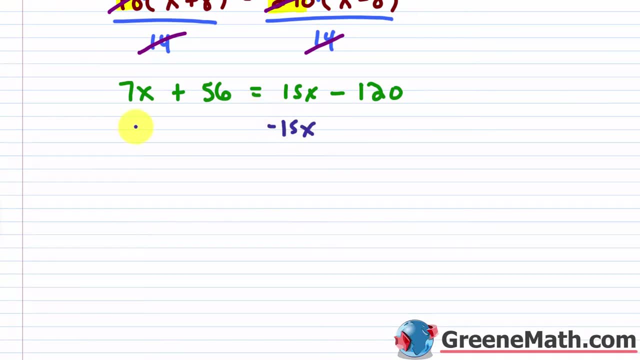 and then minus 15 times X is 15 X. So that's going to make my life a lot easier. So let me scroll down a little bit, get some room going. I can subtract 15- X away from each side of the equation And I can subtract 56 away from each side of the equation. So we know that. 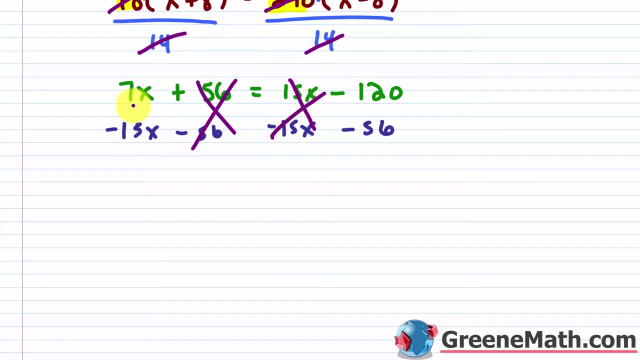 this is going to cancel, and this is going to cancel 7 X minus 15. X is going to give me negative eight X, And this will be equal to negative 120 minus 56 is negative 176.. If I finish this up by dividing both sides by negative eight, right the coefficient of X there. 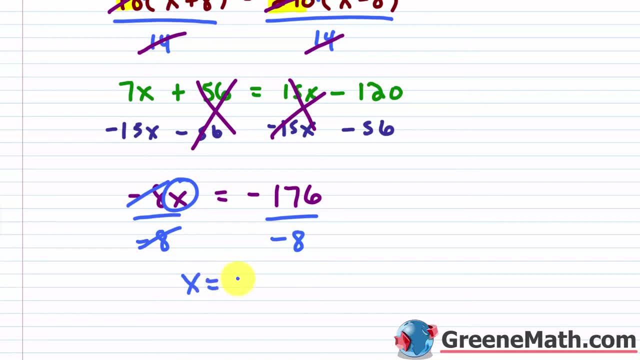 what I'm going to get is this: cancels with this I'll have: X is equal to 22.. So this is what we're looking for. I can't just put X equals 22.. Obviously, I've got to answer my question. 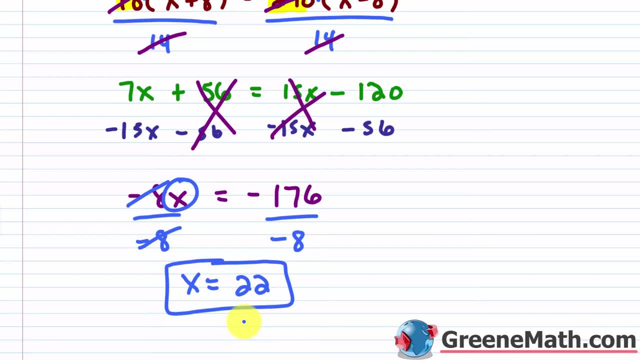 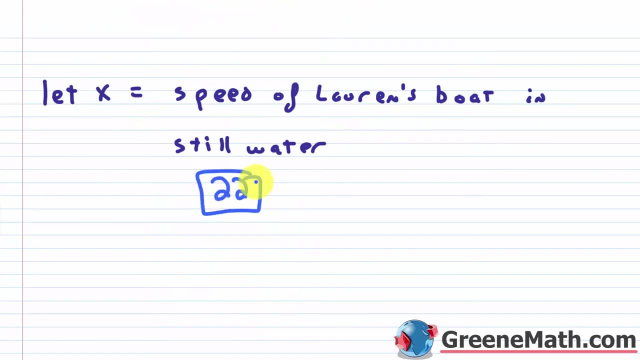 But X tells me the speed of Lauren's boat in Stillwater, which is exactly what we want to know, right? So it's going to be 22 miles an hour. So I can say this is 22 here, And let me go up. 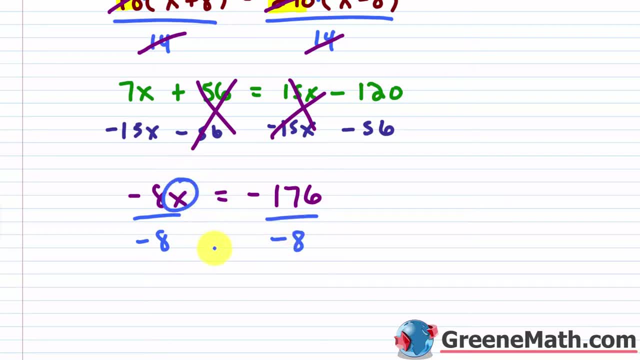 negative 8. right, the coefficient of X there. what I'm gonna get is this: cancels with this I'll have: X is equal to 22, so this is what we're looking for. I can't just put X equals 22. obviously I've got to answer my question. but X? 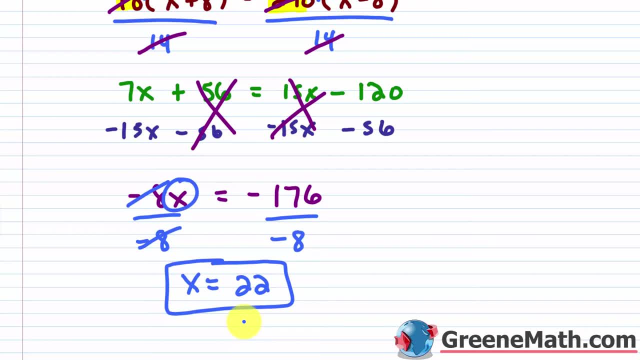 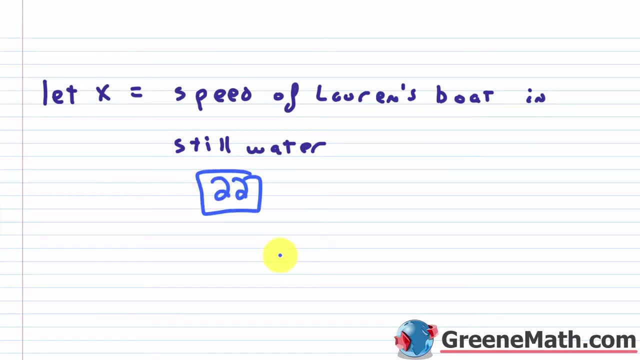 tells me the speed of Lauren's boat, and still water, which is exactly what we want to know, right? so it's gonna be 22 miles an hour, so I can say this is 22 here, and let me go up and just answer my question. so I can just say that Lauren's 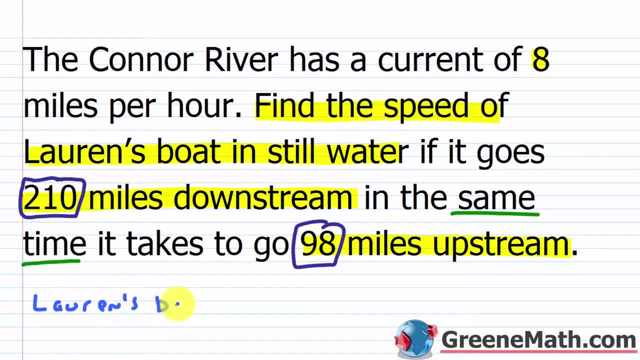 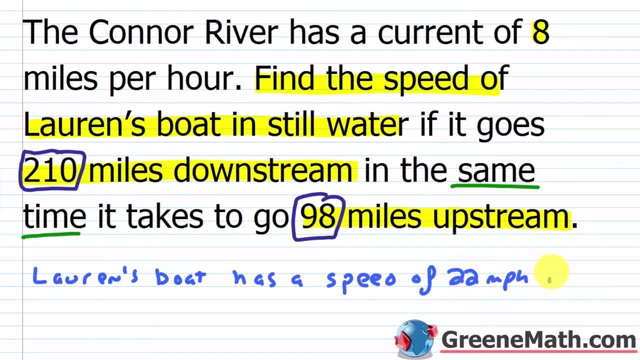 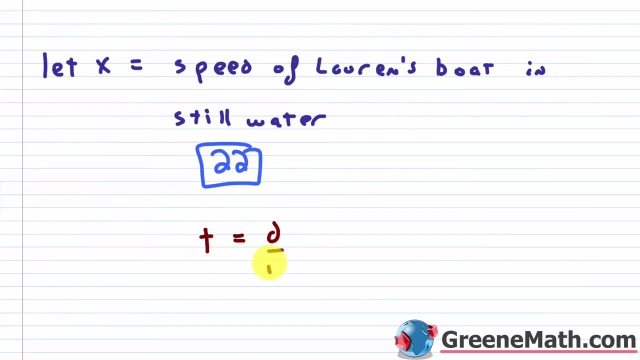 boat has a speed of 22 miles per hour and still water. so how can I get this right? how can we check to make sure we got the right answer? well, again, if we go back to the fact that time is equal to distance over rate, we can just kind of 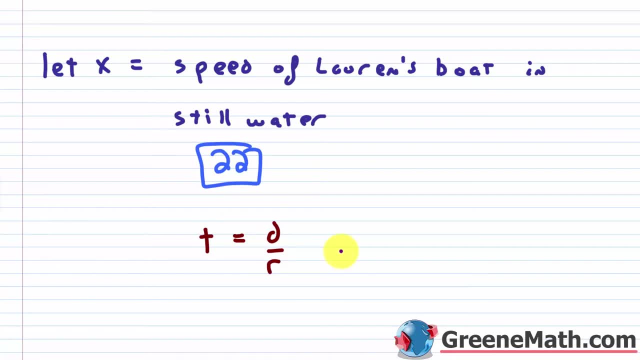 think about the scenario we're given for the downstream scenario. we know that her distance is 210 miles and we know that her rate of speed is the speed of the boat and still water, which is 22, plus the speed of the current, which is 8, so that's gonna be 30. so 210 divided by 30 would be 7. so this is her. 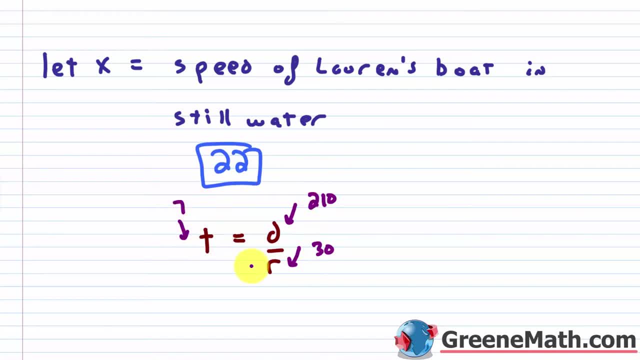 downstream scenario and she's gonna get that right here and now that she has the. it took her seven hours to go 210 miles. Now the other scenario. let me just set this up over here. We know that she goes 98 miles going at a rate of speed, Remember, if it's going upstream. 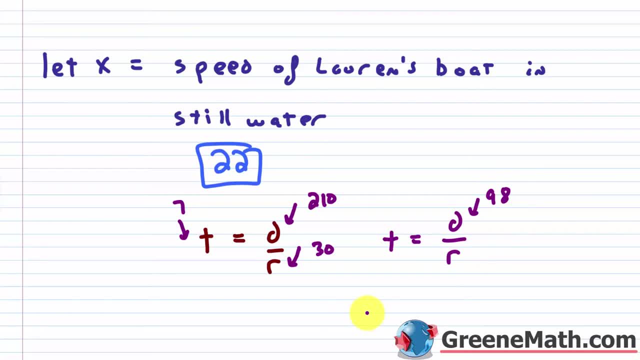 it's going to be 22,. the speed of the boat in still water, minus eight, okay, the speed of the current, which is going to be 14.. Okay, so this is 14.. And we know that 98 divided by 14 is 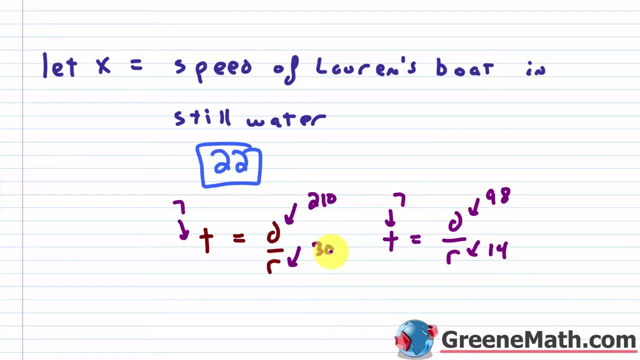 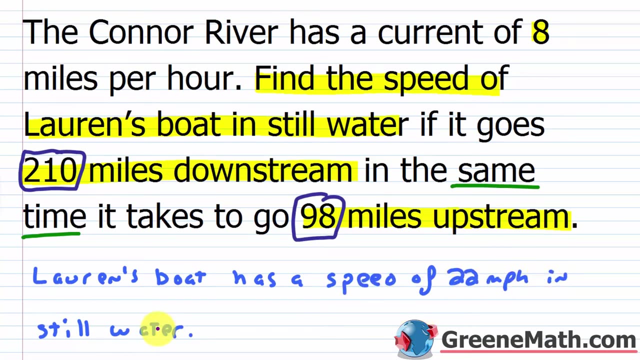 seven. So this is true, right, It took her the same amount of time to go 210 miles downstream- right seven hours- that it takes to go 98 miles upstream- again seven hours. So our answer here is correct. Again, we can say that Lauren's boat has a speed of 22 miles per hour in still water. 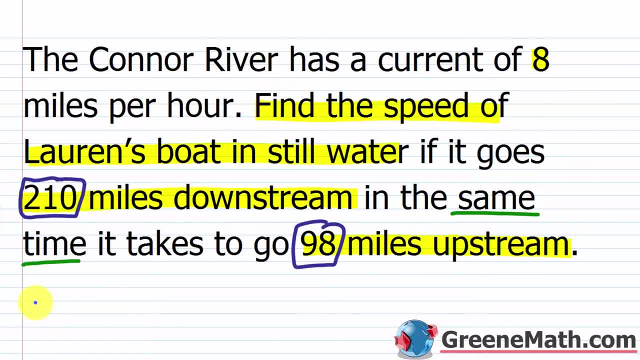 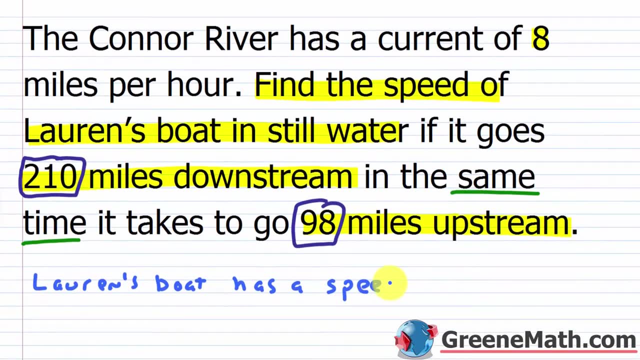 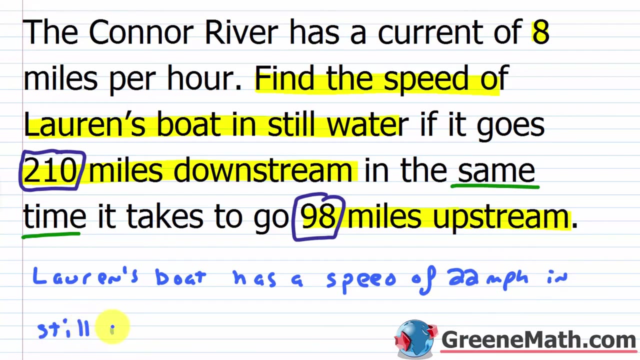 and just answer. So I can just say that Lauren's boat has a speed- and let me make this better- of 22 miles per hour in Stillwater. So how can we check to make sure we got the right answer? Well, again, if we go back to our previous equation, we're going to see that we have a speed of 22 miles per hour. 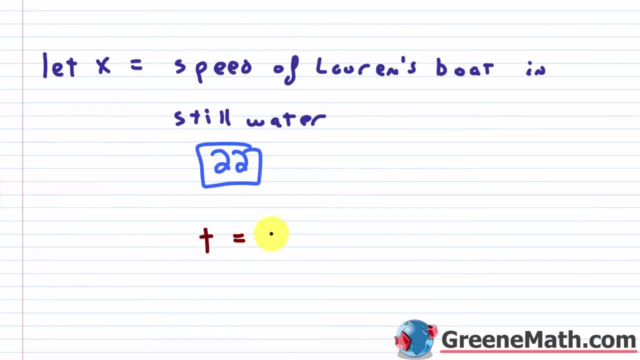 If we go back to the fact that time is equal to distance over rate, we can just kind of think about the scenario we're given For the downstream scenario. we know that her distance is 210 miles And we know that her rate of speed is the speed of the boat in Stillwater, which is 22,. 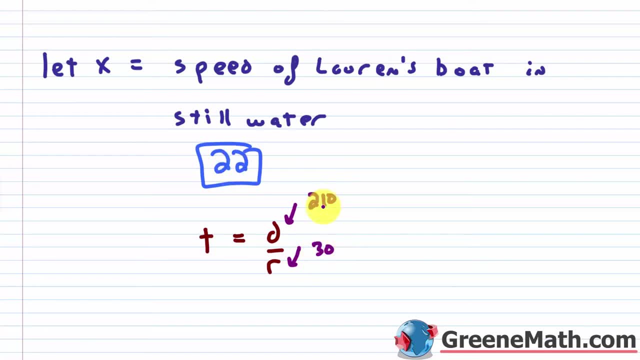 plus the speed of the current, which is eight, So that's going to be 30. So 210 divided by 30 would be seven. So this is her downstream scenario. It took her seven hours to go 210 miles Now. 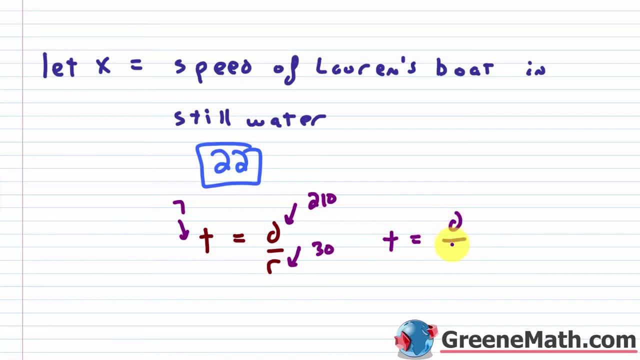 the other scenario. let me just set this up over here. We know that she goes 98 miles going at a rate of speed- Remember, if it's going upstream it's going to be 22,. the speed of the boat in Stillwater minus eight, okay, the speed of the current. 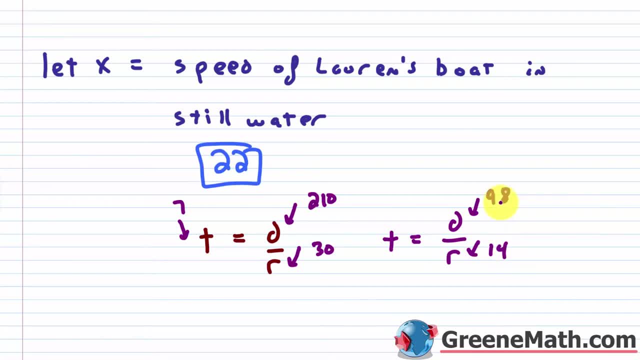 which is going to be 14.. Okay, so this is 14.. And we know that 98 divided by 14 is seven. So this is true, right, It took her the same amount of time to go 210 miles downstream. 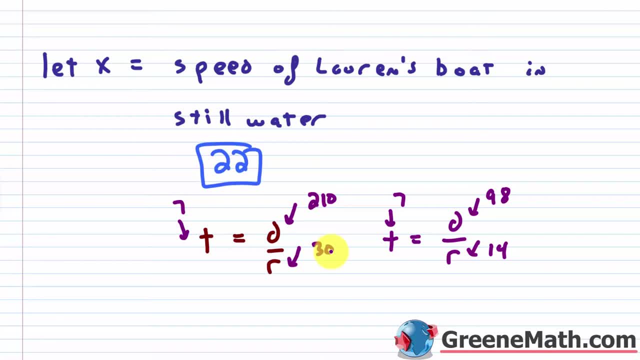 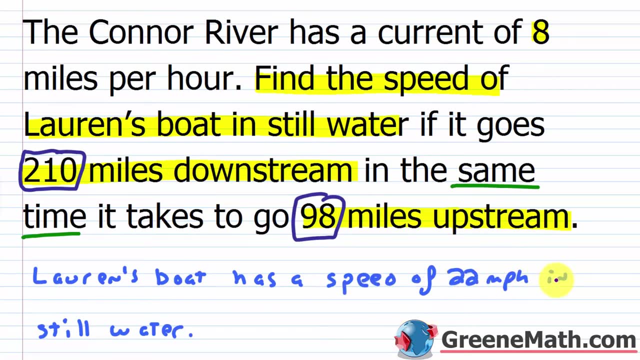 right Seven hours that it takes to go. So our answer here is correct. Again, we can say that Lauren's boat has a speed of 22 miles per hour in Stillwater. All right, now let's move on and talk about rate of work problems. 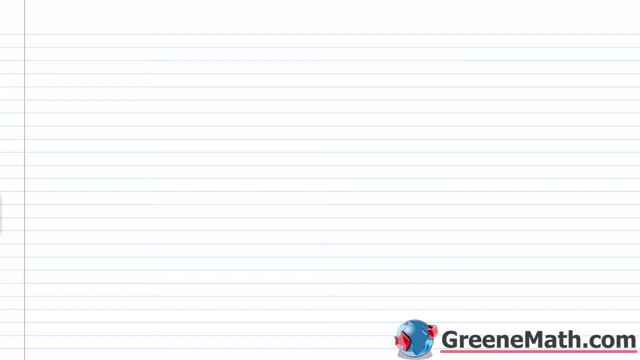 otherwise known as work rate problems. So essentially, these are very easy problems to solve once you understand how to kind of set them up, And they just deal with the rate of speed at which a job can be completed, given the individual work rates from the people performing the job. 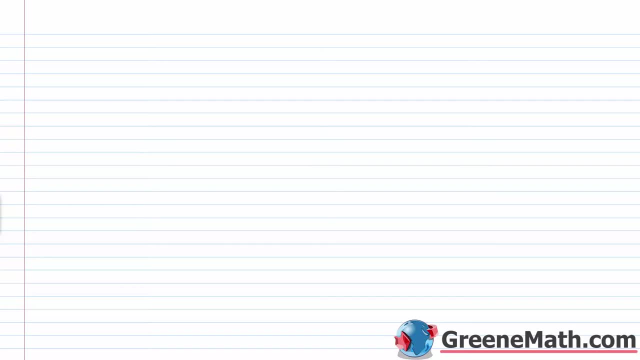 Okay, so again, very, very easy. If you understand the distance formula that we just used in the last problem, then you could understand this formula I'm going to give you here today. So the distance formula again is: D per distance is equal to the rate of speed, R times T for time travel. Okay, 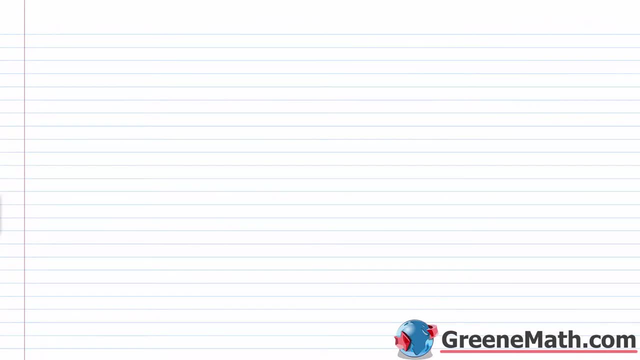 All right, now let's move on and talk about rate of work problems, otherwise known as work rate problems. So essentially, these are very easy problems to solve, once you understand how to kind of solve them. So let's go ahead and start with the first one. So let's go ahead and start. 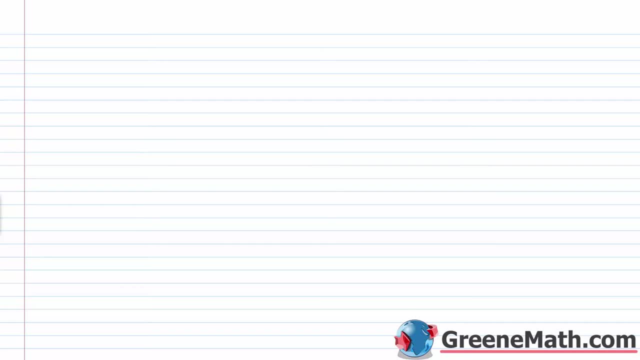 with the first one. So let's go ahead and start with the first one. So let's go ahead and start with the set them up. And they just deal with the rate of speed at which a job can be completed, given the individual work rates from the people performing the job. Okay, so again, very, very easy. 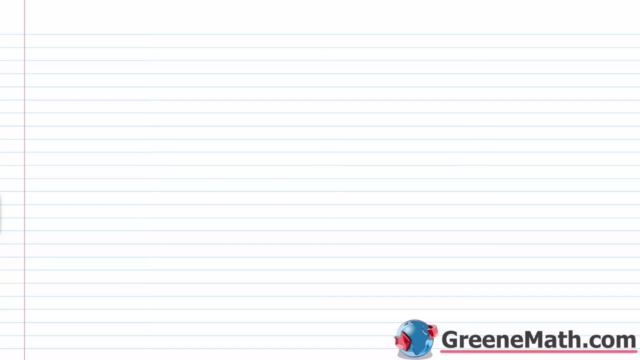 If you understand the distance formula that we just used in the last problem, then you could understand this formula I'm going to give you here today. So the distance formula again is: D per distance is equal to the rate of speed R times T for time travel. Okay, very intuitive Again if I go 40 miles per hour for three hours. 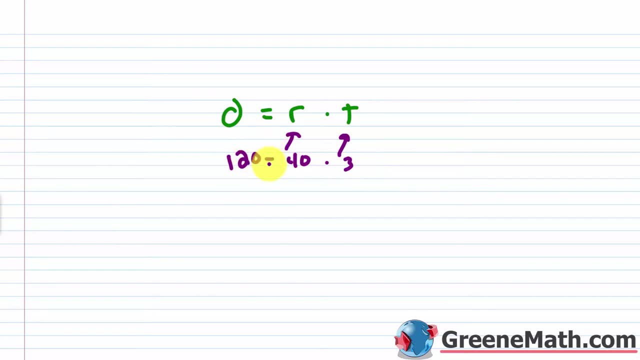 40 times three is what. it's 120. So I know I've gone 120 miles. okay, very intuitive, very easy to understand. The same thing goes when we work with work rate problems or rate of work problems. So instead of D you have a, which stands for the amount of work completed, And we think about this. 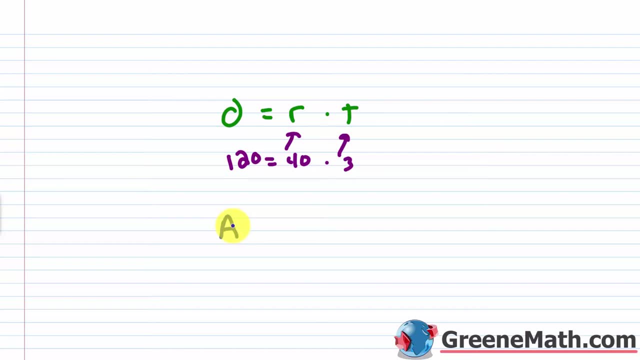 in terms of jobs completed. So it could be one jobs completed in pretty much every scenario that I've seen. But if you wanted to extend that and say, okay, we have two jobs completed, 11 jobs completed, 2 million jobs completed, whatever, that is okay, but a here stands for the amount of work. 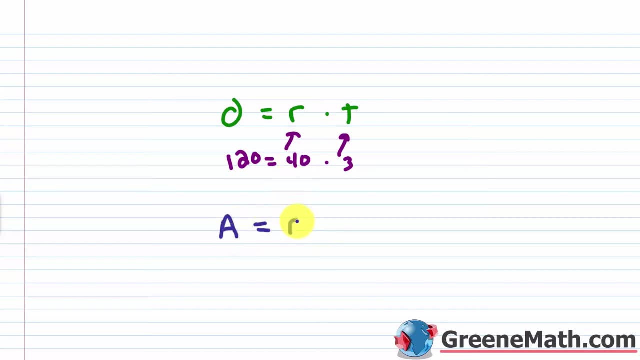 completed. This is equal to R, which is your rate at which the work is done. Okay, otherwise known as a work rate. That's how these problems get their name. Okay, then times T, which is our time, And that's the amount of time that you're working for. So let's say, for example, my rate of work. 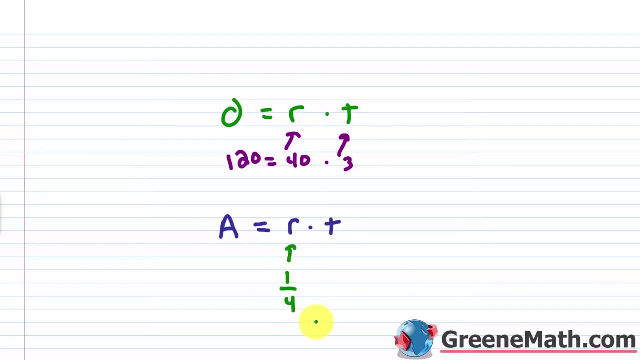 and this will make more sense when I explain in a minute- is one over four, Okay, And I multiply this by a time of eight. What does that give me? We know that eight times one, fourth is two. So what does that give me? We know that eight times one, fourth is two. So what does that give me? 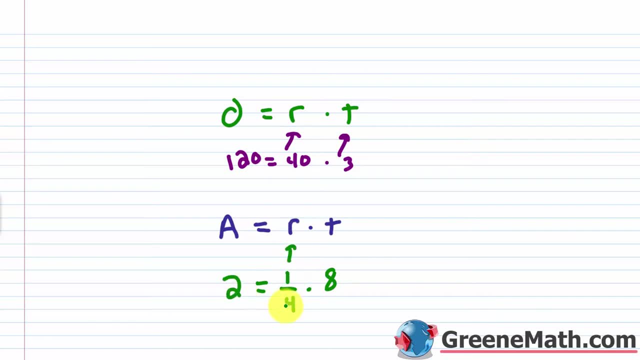 My work rate tells me how much of the job I can complete in one unit of time. So let's say, as an example, I'm working with hours. let's say I was painting a house, So it takes me four hours to paint the house. Well, in one hour, one unit of time, I'm done with one fourth of that job, If I 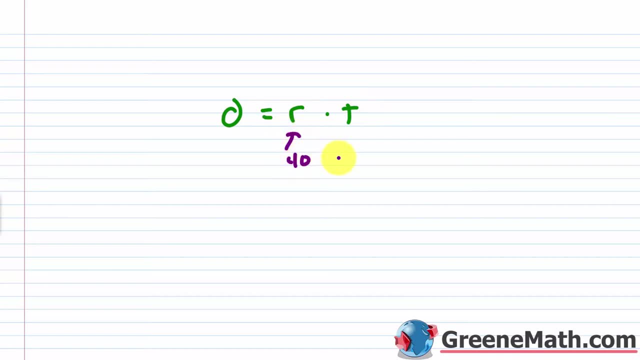 very intuitive Again, if I go 40 miles per hour for three hours, 40 times three is what it's 120.. So I know I've gone 120 miles. Okay, very intuitive, very easy to understand. The same thing goes when we do the distance formula. So if I go 40 miles per hour, 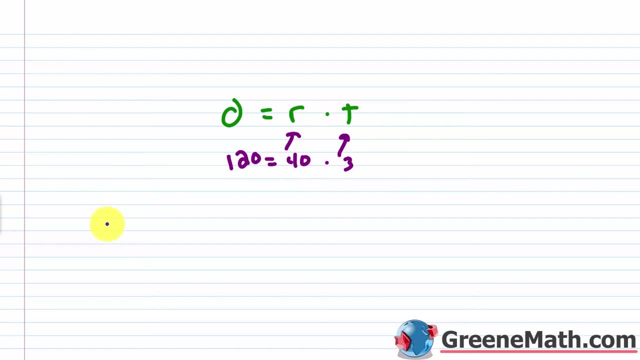 we work with work rate problems or rate of work problems. So instead of D you have a, which stands for the amount of work completed. When we think about this in terms of jobs completed, so it could be one jobs completed in pretty much every scenario that I've seen. But if you wanted to extend that, 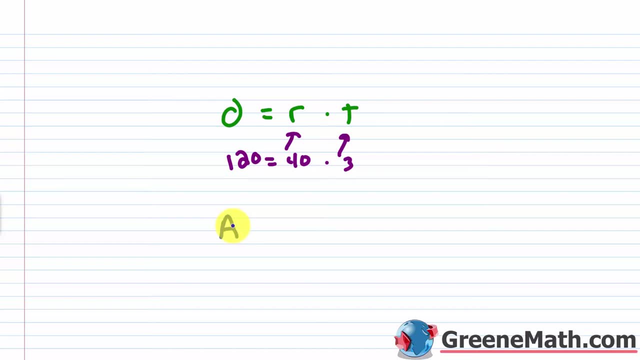 and say: okay, we have two jobs completed, 11 jobs completed, 2 million jobs completed, whatever. that is okay, but a here stands for the amount of work completed. This is equal to R, which is your rate at which the work is done. Okay, otherwise known as a work rate. That's how the work rate is done. 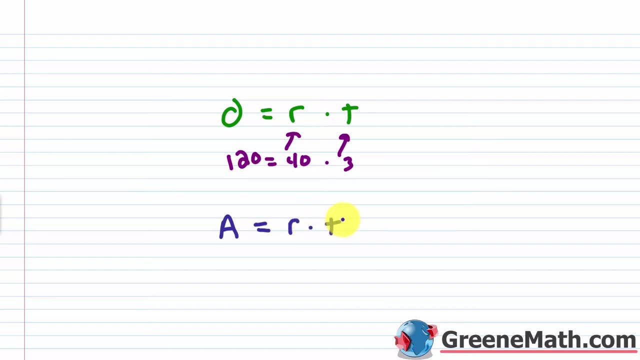 So let's say, for example, my rate of work- and this will make more sense when I explain in a minute- is one over four. Okay, And I multiply this by a time of eight. What does that give me? We know that eight times one, fourth is two. So what does this mean? My work rate tells me how much of the 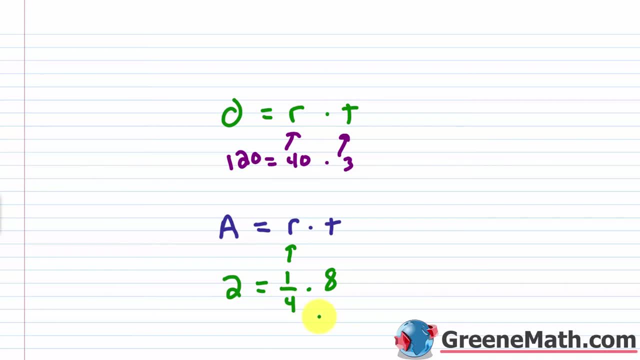 job I can complete in one unit of time. So let's say, as an example, I'm working with a job that's done with hours. Let's say I was painting a house, So it takes me four hours to paint the house. Well, in one hour, one unit of time, I'm done with one fourth of that job. If I work at this rate for 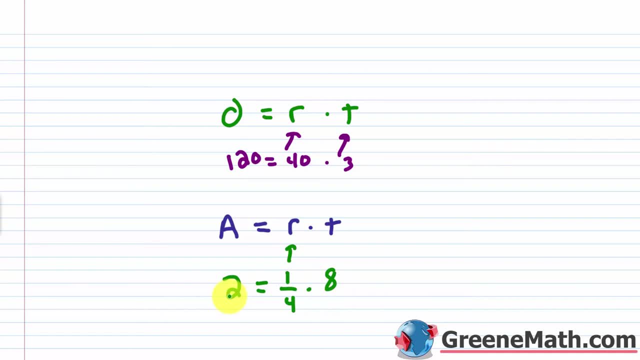 eight hours. okay, I continue at eight hours. I'm going to paint two houses, right? Okay, that's all that same. If I change this to four, then this just becomes one, right? So if I work at a work, 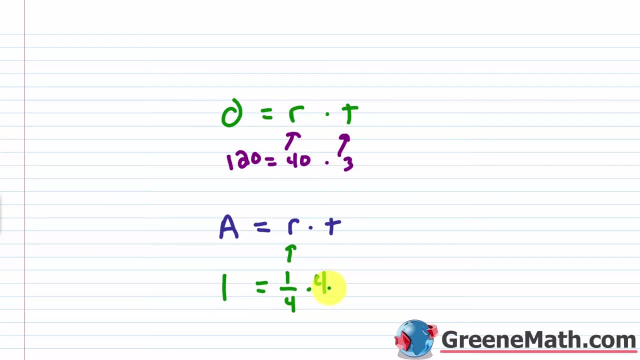 rate of one fourth of the job per hour, and I do this for four hours. well then, I've got one completed job. Now, in almost every case, or in every case, I'm going to be painting a house. in case that I've ever seen, A is going to be one. So basically what you want to focus on here. 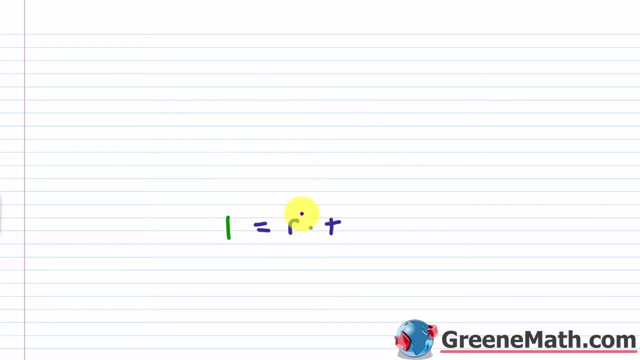 and let me erase this. we don't need this information anymore. This R here is your rate of work or your work rate. That's what you're focused on in the problem. So I'm going to divide both sides of the equation by T. That's what's multiplying R. So I can isolate And I'll say: 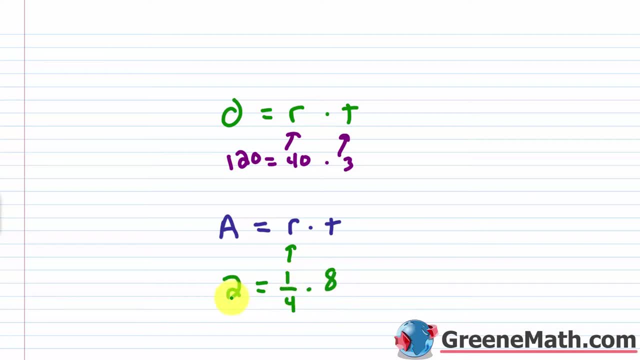 work at this rate for eight hours. okay, I continue at eight hours. I'm going to paint two houses, right? Okay, that's all that same. If I change this to four, then this just becomes one, right? So if I work at a work rate, I'm going to paint two houses, right? So if I change this to four, 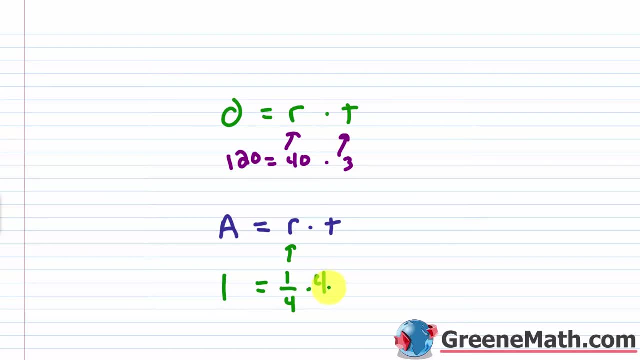 I'm going to paint two houses, right? So if I work at a work rate of one fourth of the job per hour and I do this for four hours, well then I've got one completed job. Now, in almost every case, or in every case that I've ever seen, A is going to be one. So basically what you want to. 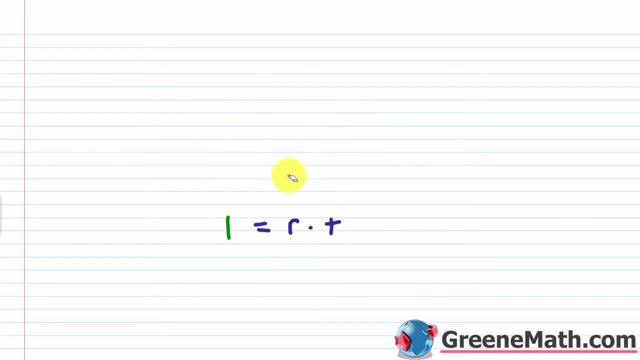 focus on here and let me erase this. we don't need this information anymore. This R here is your rate of work or your work rate. That's what you're focused on in the problem. So I'm going to divide both sides of the equation by T. That's what's multiplying R, So I can isolate And I'll say that R my work rate is one fourth of the job per hour. So I'm going to divide both sides of the equation by T. That's what's multiplying R. So I can isolate And I'll say that R- my work rate. 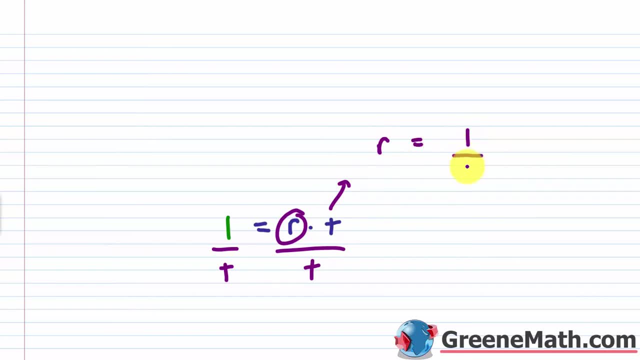 or rate of work is equal to one over T. So this is very important. You probably want to write that down in your notes. if you're taking notes, This is what we're going to use in almost every scenario to get an answer okay. So you've got to know that if you're working on a problem like this. 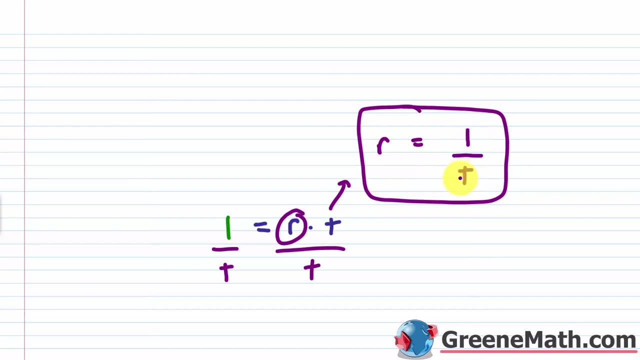 and you want your work rate. just take a one and divide it by the amount of time it takes to complete the job. So again, in the case where we could paint the house in four hours, while I would get a work rate, my R would be equal to one over T. So I'm going to divide both sides of the equation. 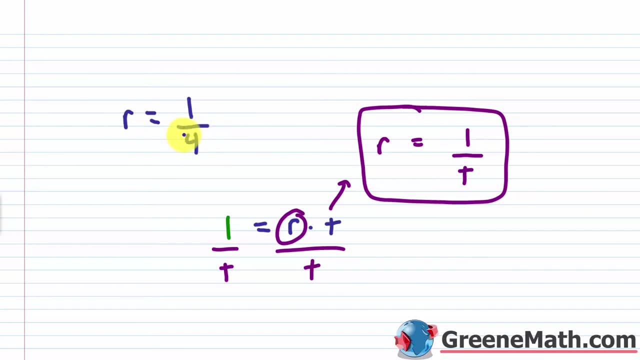 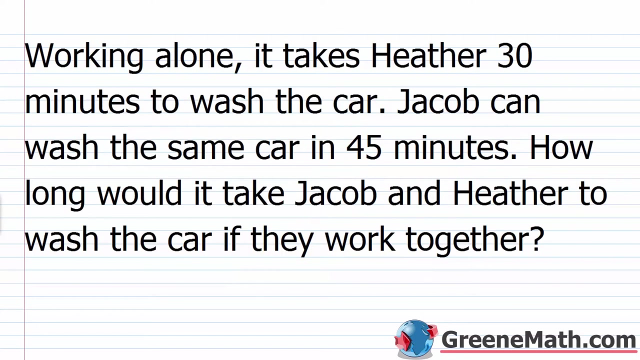 and the rest of the equation by equaling the number of times. I've completed this. So the other thing that we need up in and look at one. All right, So working alone, it takes Heather 30 minutes to wash the car. Jacob can wash the same car in 45 minutes. How long would it take Jacob and Heather to wash? 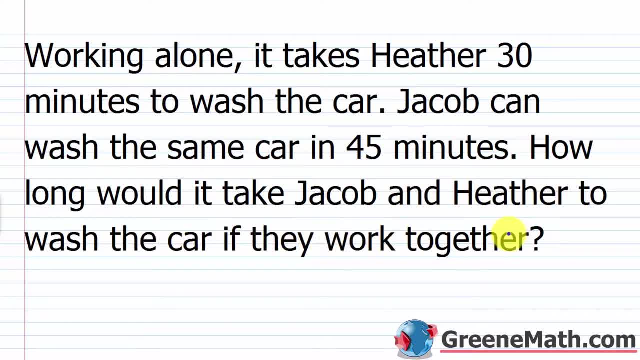 the car if they work together, All right. So the first thing I'm going to do here, just like we always do, is just find out. what are they asking us to find? Well, the question we need to answer here is: how long would it take Jacob and Heather to wash the car if they work together? This is a 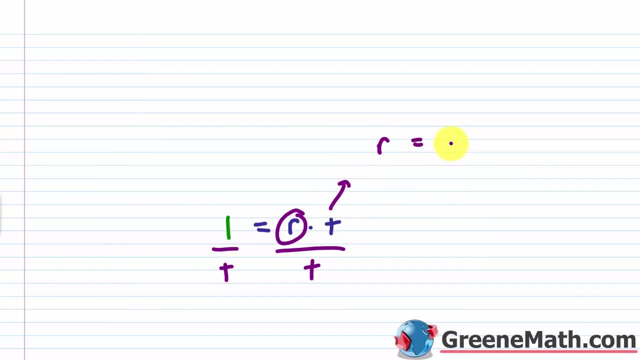 that R, my work rate, or rate of work, is equal to one over T, So this is very important. You probably want to write that down in your notes if you're taking notes, but this is what we're going to use in almost every scenario to get an answer. okay, So you've. 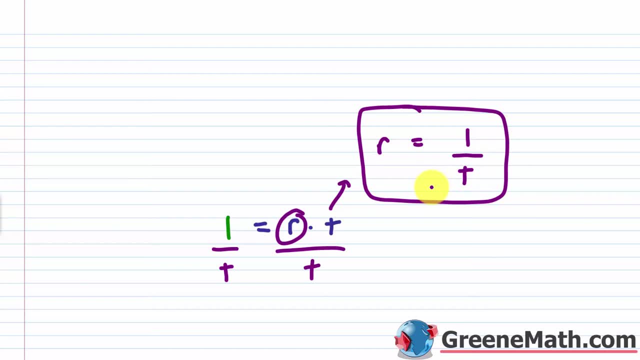 got to know that if you're working on a problem like this and you want your work rate, just take a one and divide it by the amount of time it takes to complete the job. So again, in the case where we could paint the house in four hours, while I would get a work rate, my R would be equal to one. 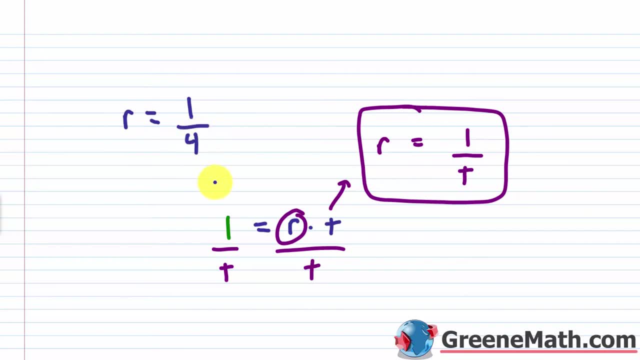 over, takes four hours to complete it. so one over four. And all this is telling me is that in one unit of time or one hour, I've completed one fourth of the job. So I'm going to divide that by one fourth of the job, okay. As another example, suppose it takes me 15 minutes to wash. 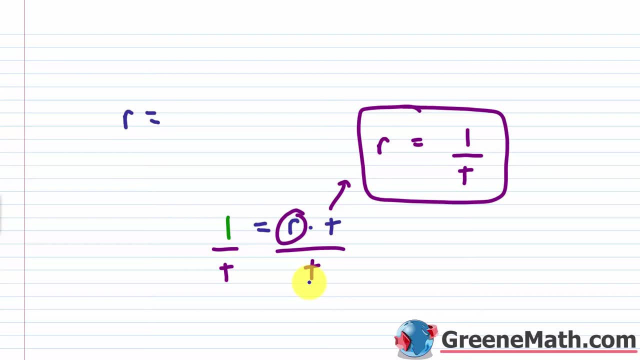 my car okay, In one unit of time, which is now one minute because we're working with minutes. then I've done one over again. it took me 15 minutes to complete it, so one over 15, or one-fifteenth of that job is complete okay. So that's the general idea behind these problems. 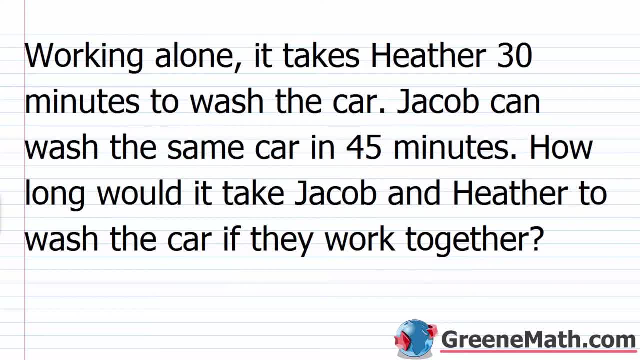 and now let's kind of jump in and look at one. All right, so working alone, it takes Heather 30 minutes to wash the car. Jacob can wash the same car in 45 minutes. How long would it take Jacob and Heather to wash the car if they work together? All right, 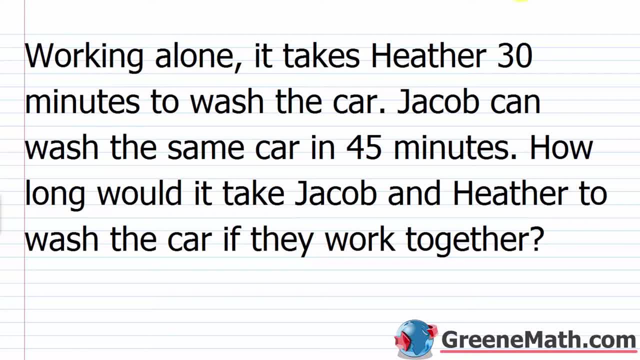 so the first thing I'm going to do here, just like we always do, is just find out. what are they asking us to find? Well, the question we need to answer here is: how long would it take Jacob and Heather to wash the car? if they work together, This is a pretty 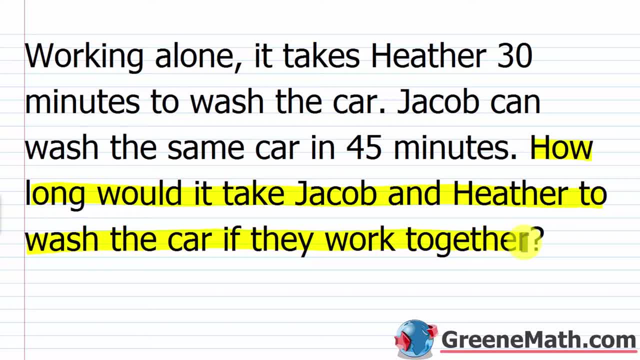 typical scenario. So you have their individual rates of work right. We know that Heather takes 30 minutes to wash the car. we know that Jacob takes 45 minutes to wash the car. but hey, if they work together same speed that they're working at when they do it individually, how long would it take for them? 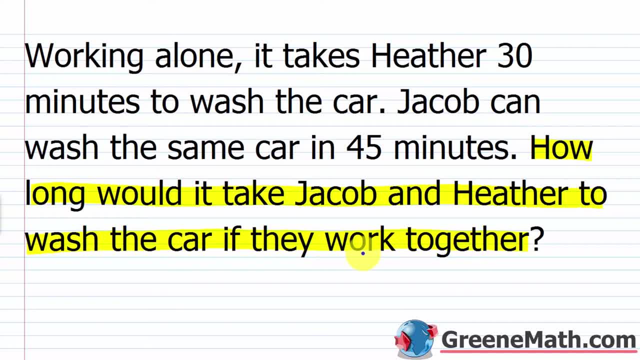 to wash the car. Okay, so that's what we're trying to figure out. So what I'm going to do is I'm going to let a variable like x be equal to that. So I'm going to go to the next page and I'm just going. 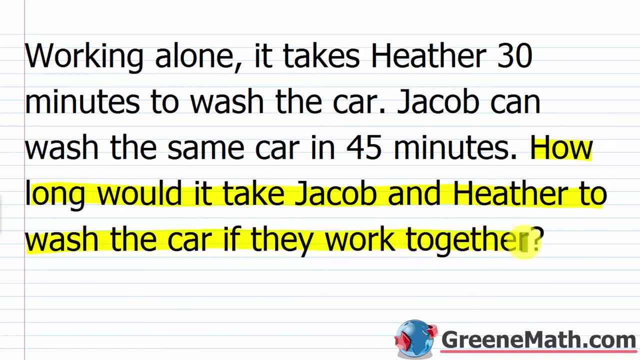 pretty typical scenario. So you have their individual rates of work right. We know that Heather takes 30 minutes to wash the car. We know that Jacob takes 45 minutes to wash the car. But hey, if they work together at the same speed that they're working at when they do it. 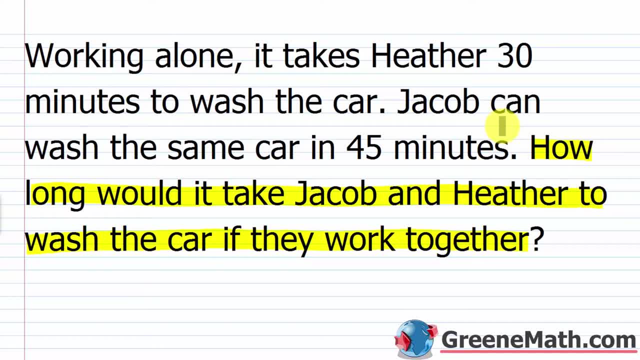 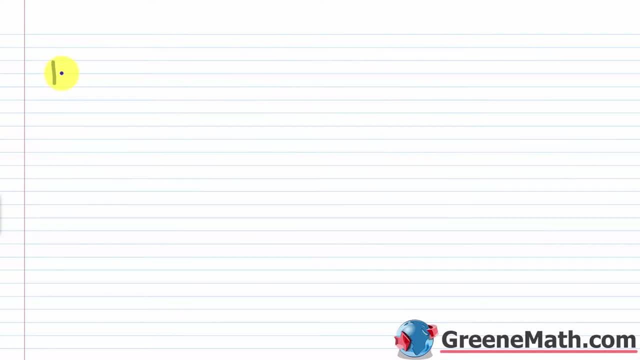 individually. how long would it take for them to wash the car? Okay, So that's what we're trying to figure out. So what I'm going to do is I'm going to let a variable like X be equal to that. So I'm going to go to the next page and I'm just going to say that we're going to let X. 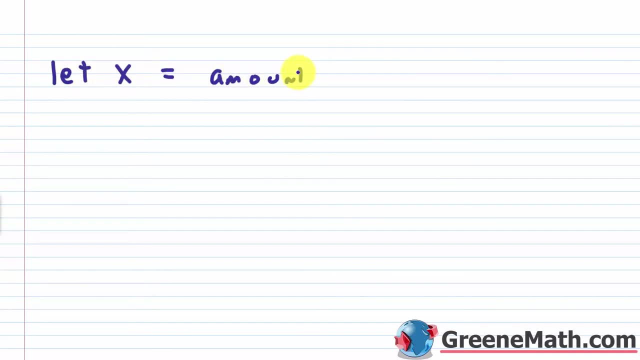 be equal to the amount of time- And I'm just going to say- to complete the job. to complete the job, right, But if you wanted to be more detailed, you could say the amount of time to complete the job when Jacob and Heather work together. Okay, And of course, since we're 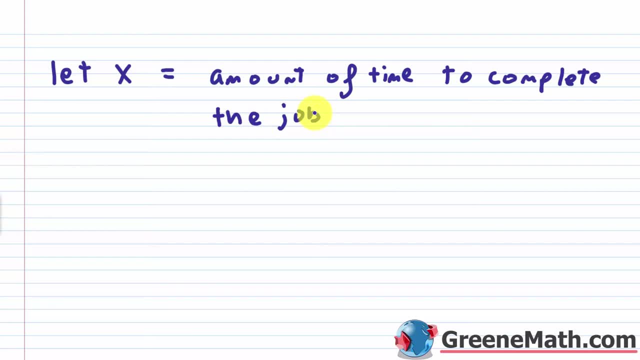 working with minutes. here the units are going to be minutes. Okay, So you got to make sure of that because, since some of these problems, you have crossovers between minutes and hours, you can have minutes and seconds, you know, so on and so forth, But for this one it's very easy. We're. 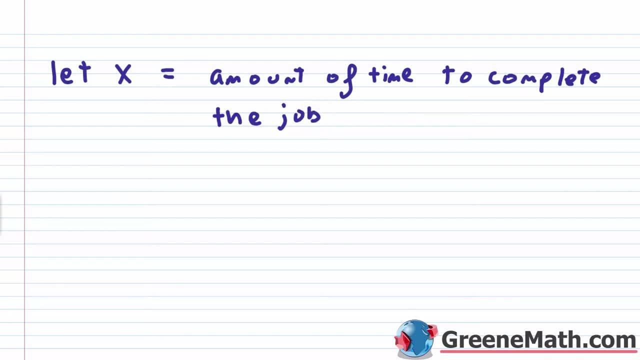 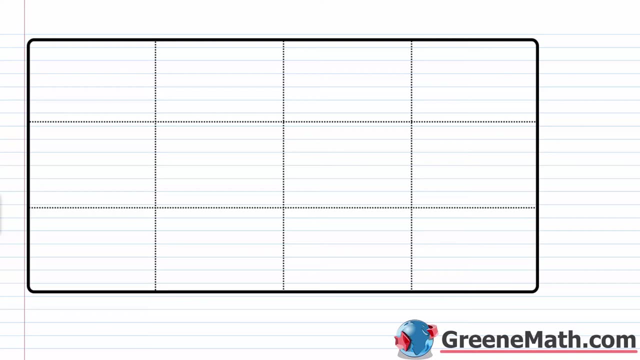 just working with minutes, All right. So let's go down to a little table and we're going to organize some information And then, once you see this in the next few problems, you're going to go right through it. Okay, Very, very simple. So of course we have Jacob and we have Heather. 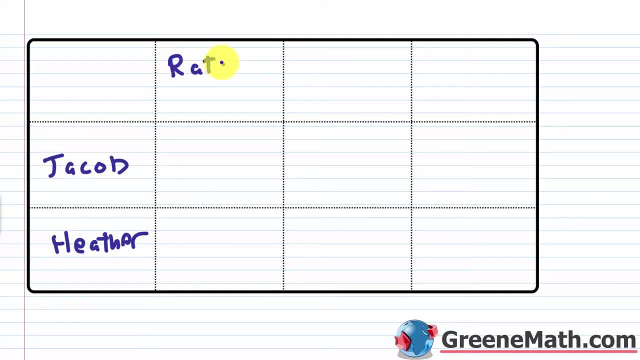 Now, the first thing I'm going to write is the rate of work. So the rate of work- And before we started this problem we talked about how to get it- It's one over the amount of time they take to complete the job. 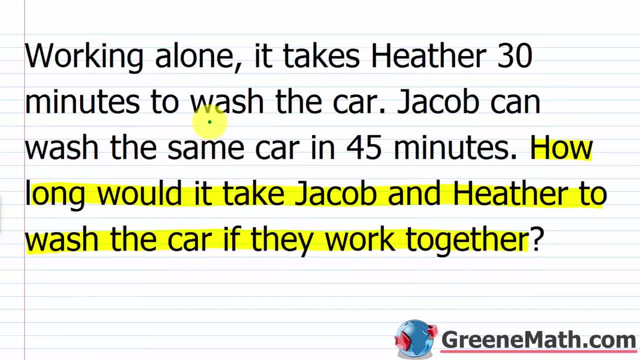 So I'm going to put a one over and then blank for each one. Let's go back up. So for Heather it takes 30 minutes to wash the car, So her rate of work would be one over 30.. Again for every. 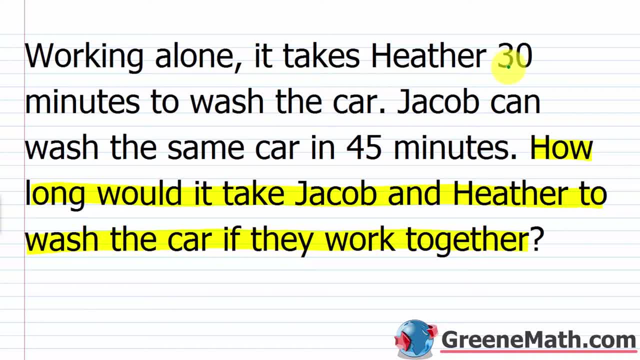 minute that passes she's done one 30th of that job For Jacob. his is going to be one. It takes him 45 minutes to wash the car, So it's going to be one over 45.. Every minute that passes. 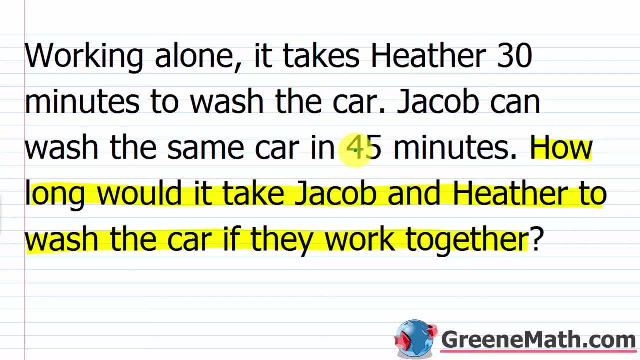 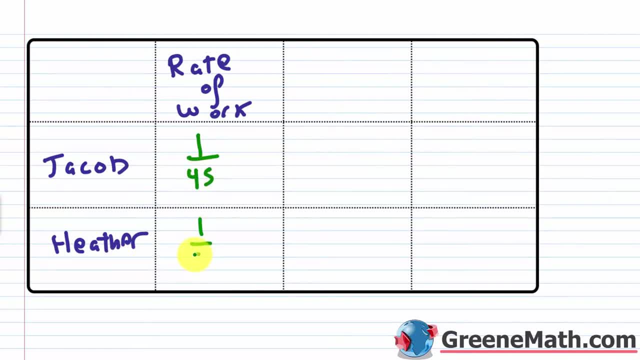 he's going to be done with one over 45 or one 45th of that job. So let's go down again. for Jacob, He's got a work rate of one over 45.. For Heather, she's got a work rate of one over 30.. 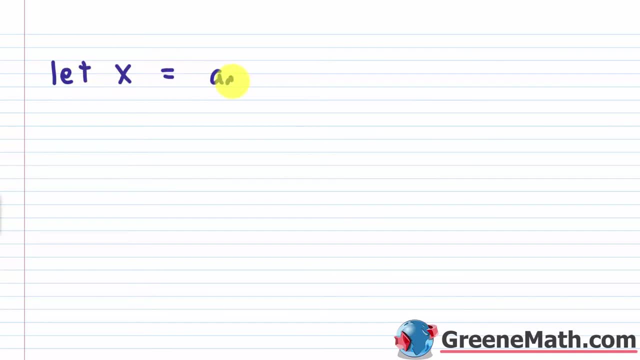 to say that we're going to let x be equal to the amount of time and I'm just going to say to complete the job, to complete the job, right. But if you wanted to be more detailed, you could say: complete the job when Jacob and Heather work together. Okay, and of course, since we're working, 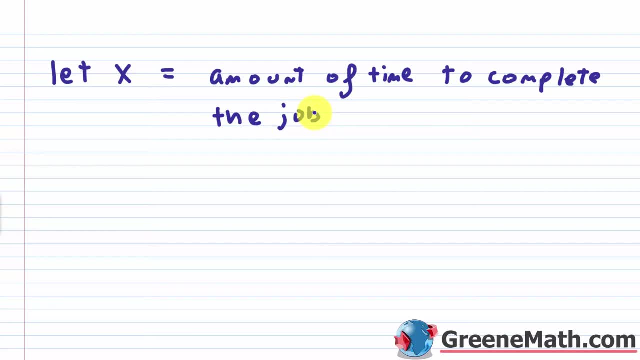 with minutes. here the units are going to be minutes. Okay, so you got to make sure of that because, since some of these problems, you have crossovers between minutes and hours, you can have minutes and seconds, you know, so on and so forth. But for this one it's very easy. we're just 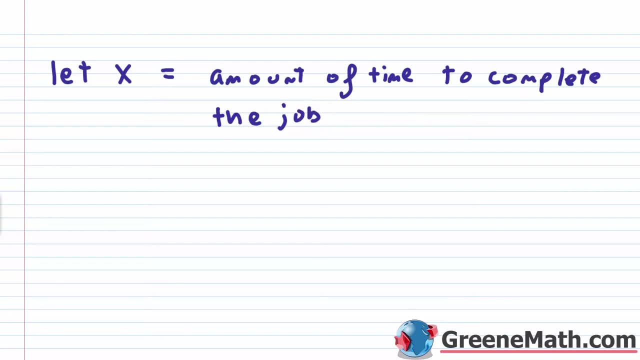 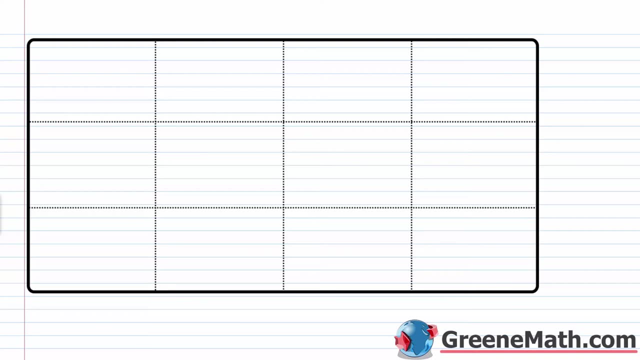 working with minutes, All right, so let's go down to a little table. We're going to organize some information And then, once you see this in the next few problems, you're going to go right through it. Okay, very, very simple. 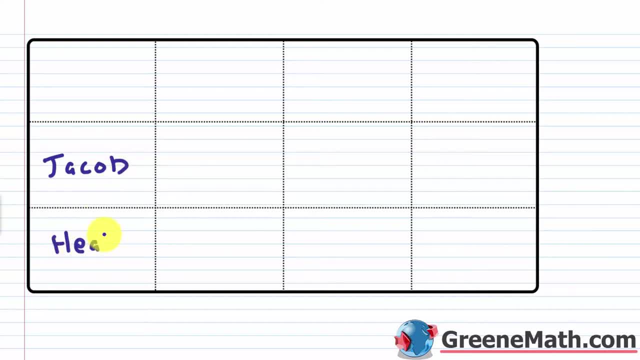 So we have Jacob and we have Heather. Now the first thing I'm going to write is the rate of work. So the rate of work- And before we started this problem we talked about how to get it- it's one over the amount of time they take to complete the job. So I'm going to put a one over. 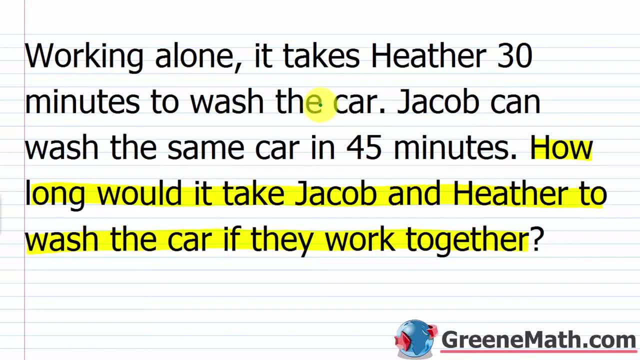 and then blank for each one. let's go back up. So for Heather it takes 30 minutes to wash the car, So her rate of work would be one over 30.. Again, for every minute that passes she's done 1 30th of. 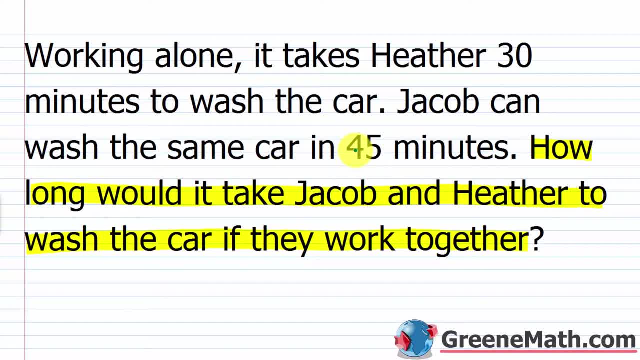 that job For Jacob, his is going to be one. it takes him 45 minutes to wash the car, So it's going to be one over 45. Every minute that passes he's going to be done with one over 45, or 1 45th of. 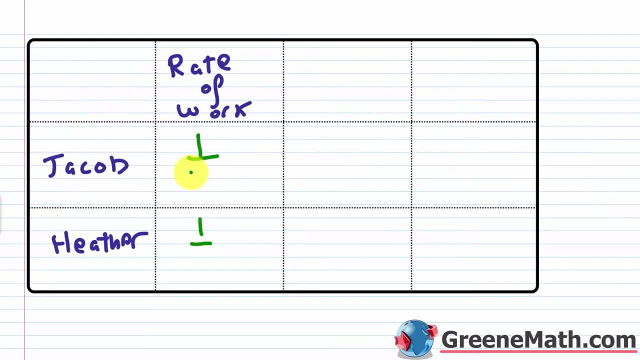 that job. So let's go down again. for Jacob, he's got a work rate of one over 45.. For Heather, she's got a work rate of one over 30.. Okay, so now I'm going to put time working together. So time. 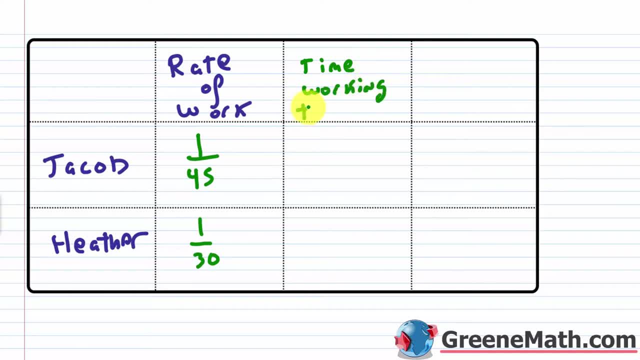 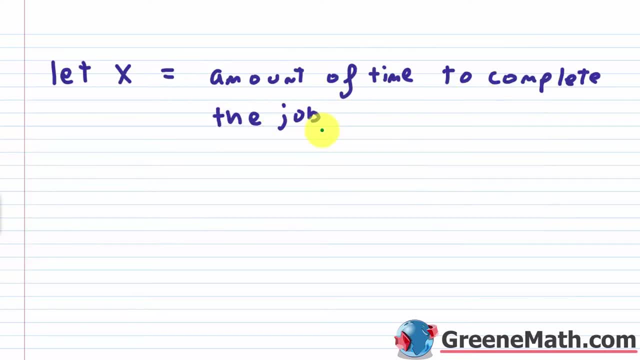 working, And then together. Now we modeled this on the page up as x, the amount of time to complete the job. Again, this is working together, So I'm just going to put this as x here and x here. Okay, it's the same in each case. Now 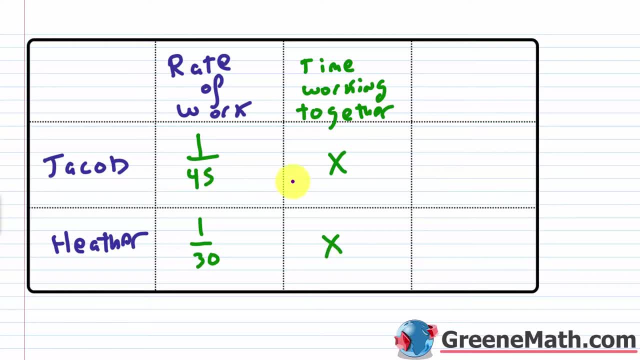 the next thing you need is the total contribution of each person. How much of the car does Jacob get done in this amount of time? How much of the car does Heather get done in this amount of time? So I'm just going to write this as total contribution. Okay, so to get this, we can just multiply. 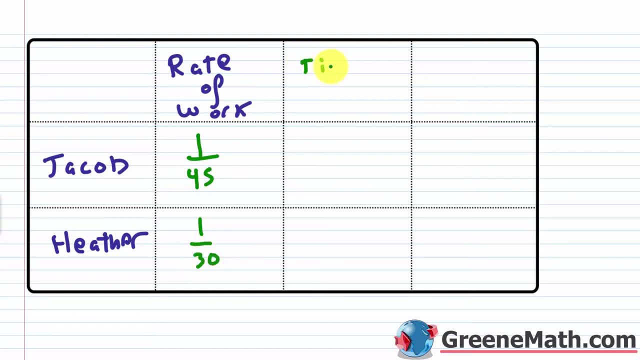 Okay, So now I'm going to put time working together. So time working and then together. Now we modeled this on the page, up as X, the amount of time to complete the job. Again, this is working together, So I'm just going to put this as X here and X here. Okay, It's the. 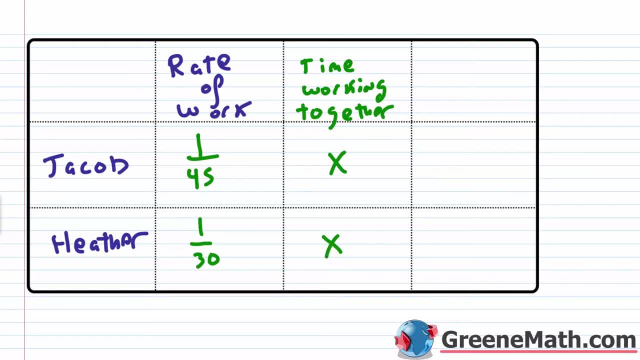 same in each case. Now, the next thing you need is the total contribution of each person. How much of the car does Jacob get done in this amount of time? How much of the car does Heather get done in time? So I'm just going to write this as total contribution. Okay, So to get this, we can just 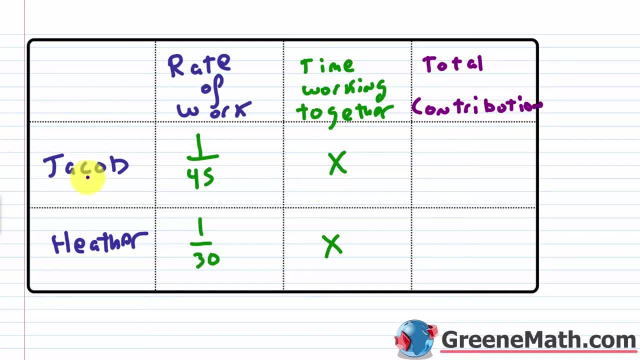 multiply, right, Because if you want to know the amount of work that Jacob performed, I just multiply my R times, my T, right, My A. the amount of work that's performed is R- the rate of work times, T- the time that you're doing that work for. Well, I've got my rate of work. I've got my time. 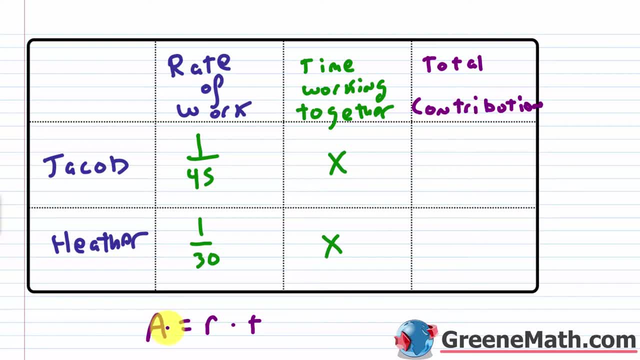 that I'm working for, So my contribution here, the amount of work that's being performed for Jacob- is 1 over 45 times X. You could write it as 1 over 45 times X, or you could write it as X over 45,, which is probably a little better. 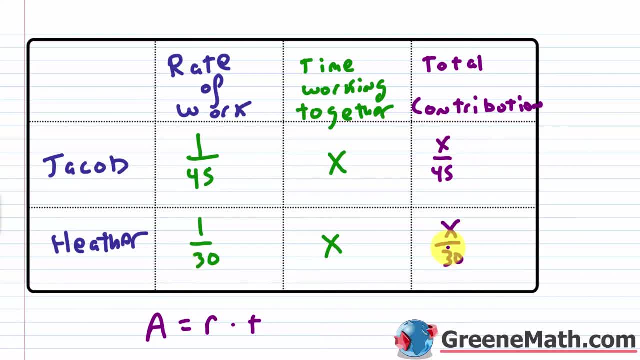 Same thing goes for Heather. It's going to be X over 30, right, Just multiply across Very, very easy. And now what we need to understand is that between Jacob and Heather, they're going to complete one job, Okay. So the equation here is very easy to set up. Jacob's contribution. 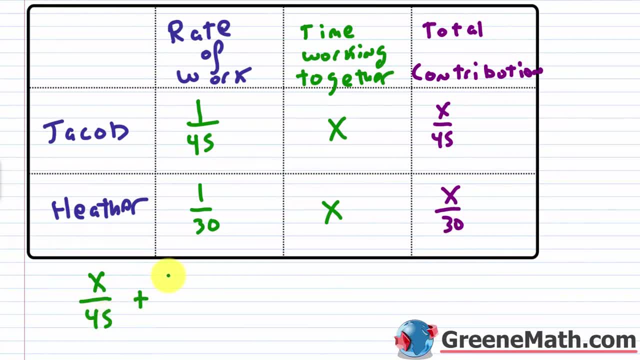 which is X over 45, plus Heather's contribution, which is X over 30, is going to be equal to 1.. Again, that's for one completed job. So the first time you see this it might not make a whole lot of sense. But again, after you solve like two or three of these, 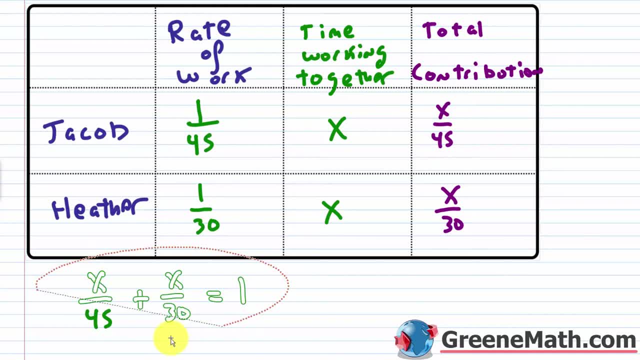 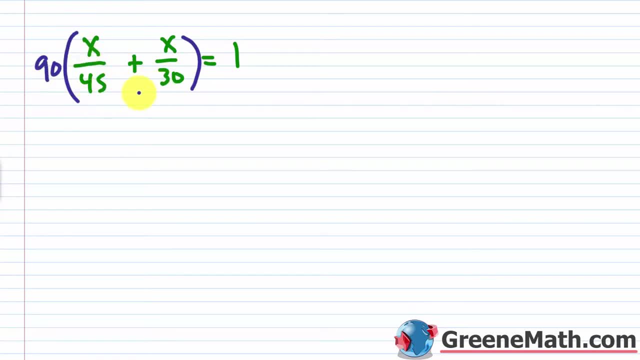 you're going to find that these are the easiest problems in the world to solve, So let's copy this. So what I'm going to do to clear these denominators, I'm going to multiply both sides of the equation by the LCD. The LCD. if I look at the denominators, I got 45 and 30, it's going to. 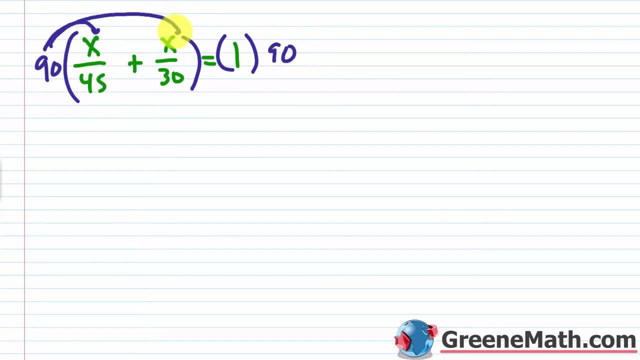 be 90.. So I'm going to use my distributive property here. 90 times X over 45,. 90 divided by 45 is 2, 2 times X is 2X. So I'm going to use my distributive property here. 90 times X over 45,. 90 divided by 45 is 2, 2 times X is 2X. 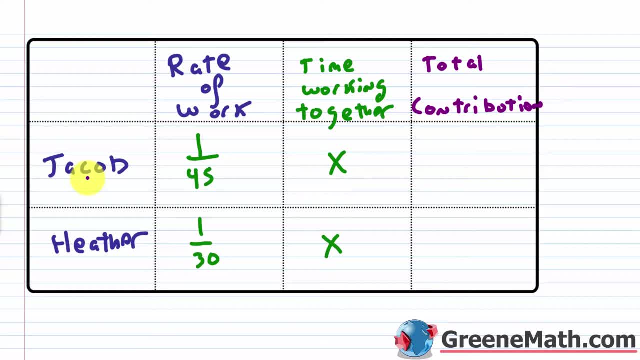 right, Because if you want to know the amount of work that Jacob performed, I just multiply my r times, my t right, My a. the amount of work that's performed is r the rate of work times, t- the time that. 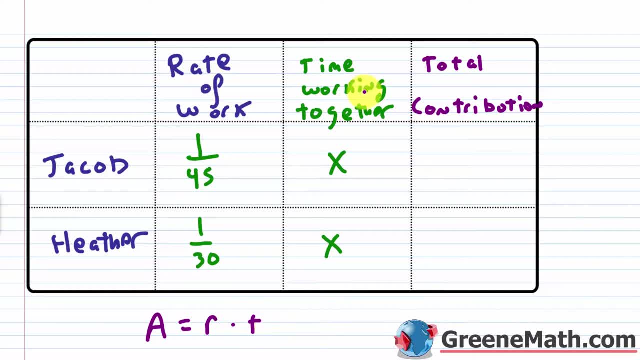 you're doing that work for. Well, I've got my rate of work, I've got my time that I'm working for. So my contribution here, or the amount of work that's being performed for Jacob, is one over 45 times x. you could write it as one over 45 times x, or you could write it as x over 45, which is 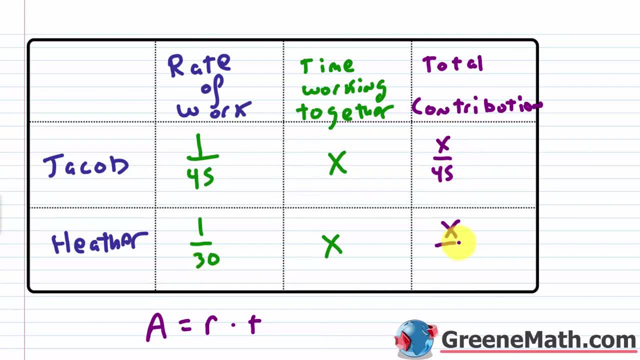 probably a little better. Same thing goes for Heather. it's going to be x over 30, right, Just multiply across very, very easy. And now what we need to understand is that between Jacob and Heather, they're going to complete one. 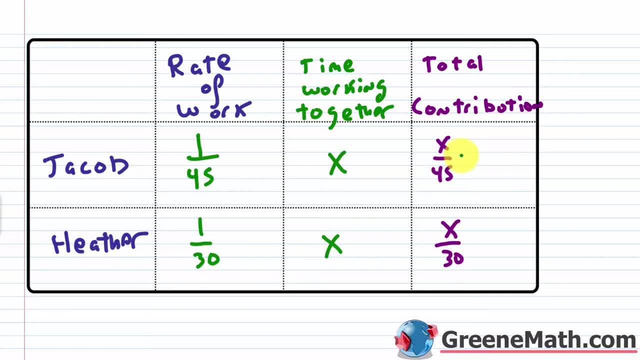 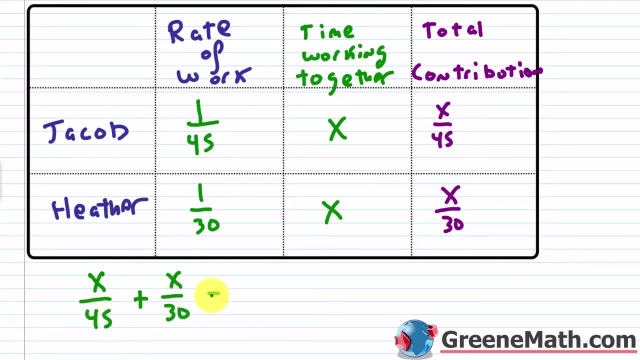 job okay. So the equation here is very easy to set up: Jacob's contribution, which is x over 45, plus Heather's contribution, which is x over 30, is going to be equal to one. again, that's for one. 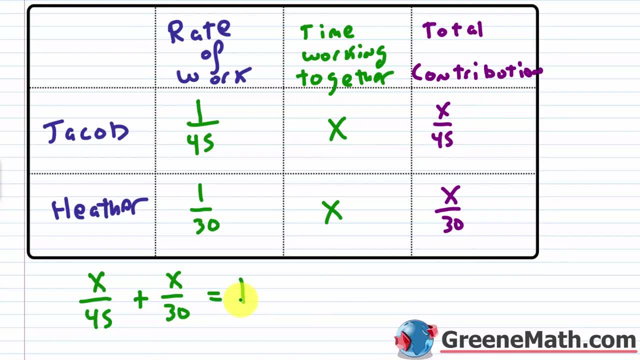 completed job. So the first time you see this it might not make a whole lot of sense. but again, after you solve like two or three of these, you're going to find that these are the easiest problems in the world to solve. 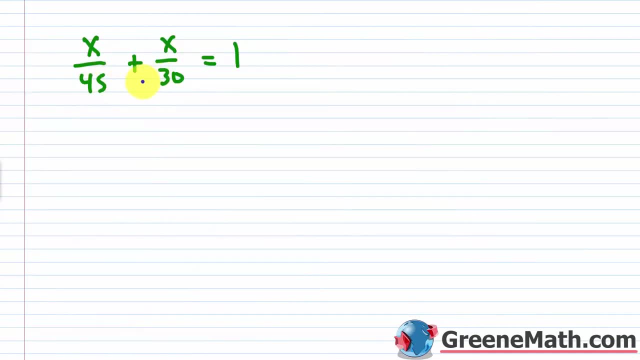 So let's copy this. So what I'm going to do to clear these denominators, I'm going to multiply both sides of the equation by the LCD, The LCD. if I look at the denominators, I've got 45 and 30,. 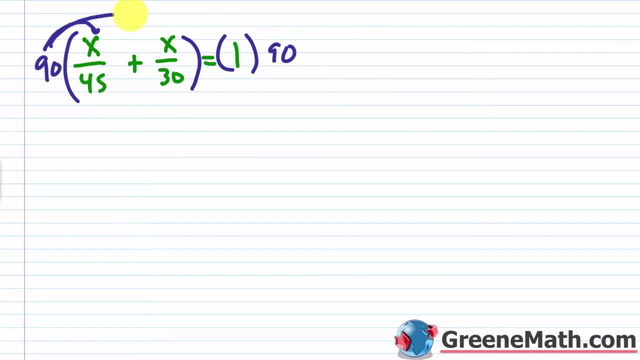 it's going to be 90. So I'm going to use my distributive property here: 90 times x over 45,. 90 divided by 45 is 2,. 2 times x is 2x. then plus 90 divided by 30 is going to be 3, then times x is: 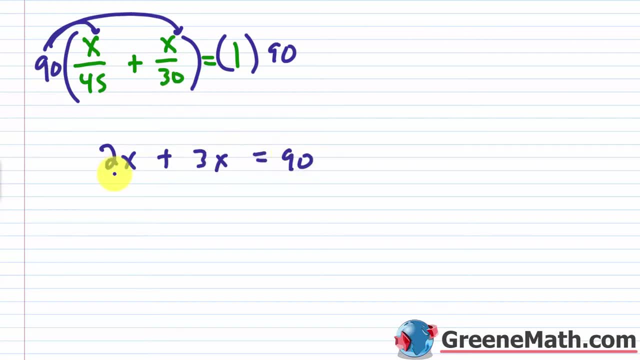 3x, and this equals 90. Sum on the left so 2x plus 3x- if I combine like terms there, I get 5x. this equals 90. Divide both sides of the equation by 5, and we're going to find that x is going to be equal to 18.. So 18 is the number of minutes that 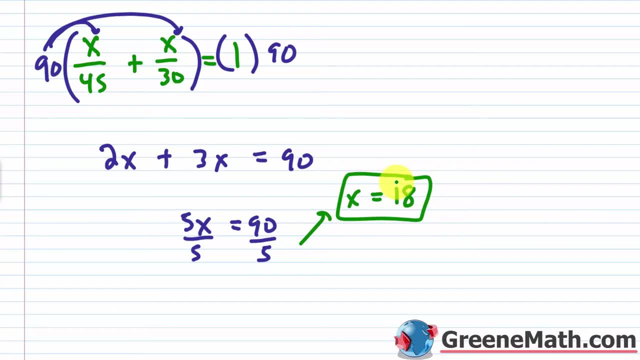 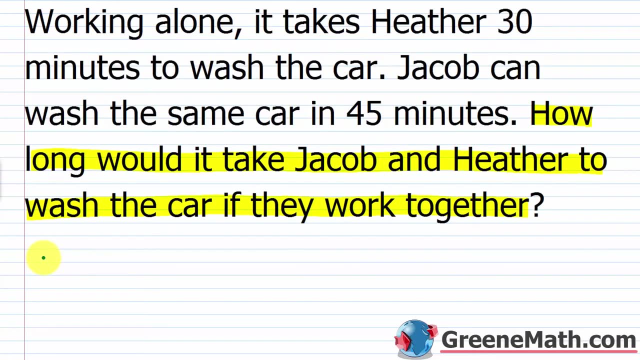 they each have to work when they're working together to complete the job, right? So if we go back up again, we said amount of time to complete the job, that's when they're working together And of course, this is in minutes. So let me just say that they work. 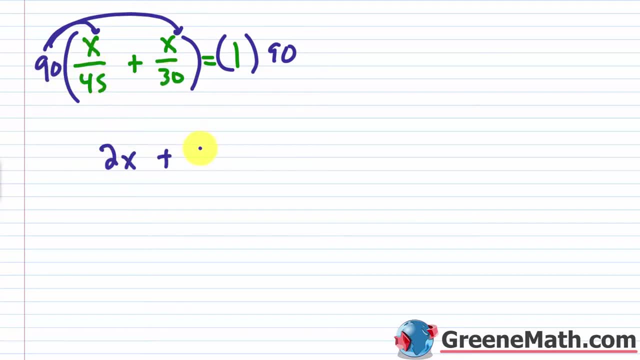 Then plus 90 divided by 30 is going to be 3.. Then times X is 3X. This equals 90. Sum on the left so 2X plus 3X. If I combine like terms there, I get 5X. This equals 90. Divide both sides of. 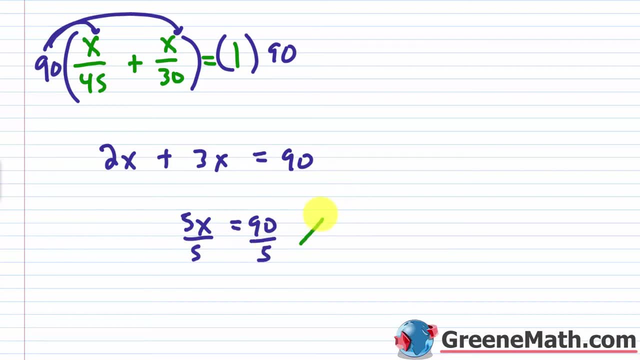 the equation by 5. And we're going to find that X is going to be equal to 18.. So 18 is the number of minutes that they each have to work when they're working together to complete the job, right? So if we go back up again, we said amount of time to complete. 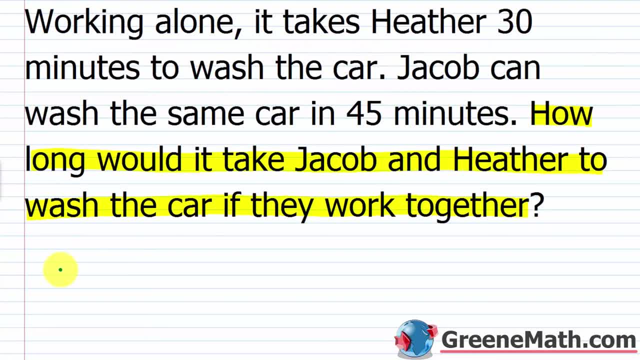 the job. that's when they're working together And of course this is in minutes. So let me just say that they work for 18 minutes to complete the job. Okay, You can answer a whole lot of different ways there. That's just a very simple sentence to say they work for 18 minutes to 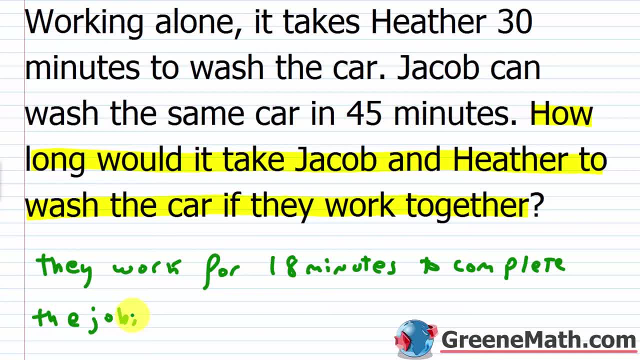 complete the job. Now, is it correct? How can we check this? Well, we can take the fraction amount that Heather does and the fraction amount that Jacob does and add those together and see if it equals 1.. So we know that, if we go back down, A is equal to R times T. I'm going to put two. 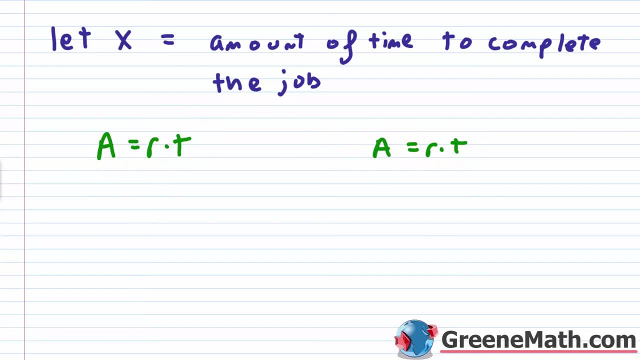 scenarios: A equals R times T. So how much or what amount of the job does Heather do? Well, remember her R. her rate of work is 1 over 30. And she works for T minutes. And again, we found that the time that they're going to work together, which we labeled as X, 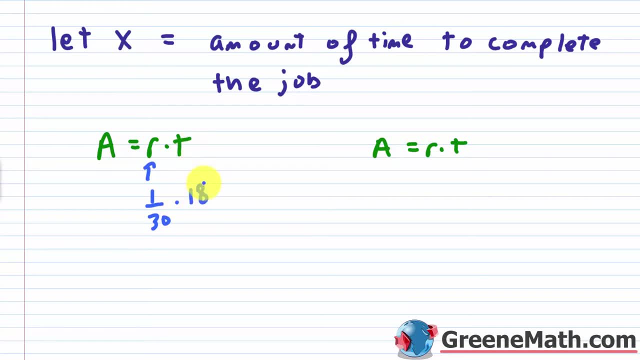 was going to be 18.. So essentially I'm going to put this as times 18.. That's going to give me the amount of work that she does. So between 18 and 30, I have a common factor of 6.. So if I divide 18 by 6,, 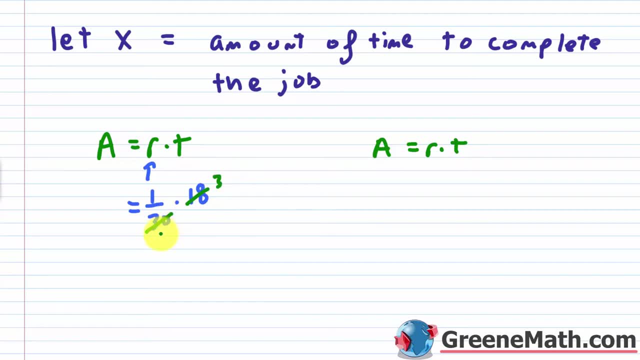 I get 3.. If I divide 30 by 6, I get 5.. So I get 3 fifths there. So this is going to be 3 fifths. That's the amount of work that she completes Now for Jacob. he's a little bit slower, So his rate. 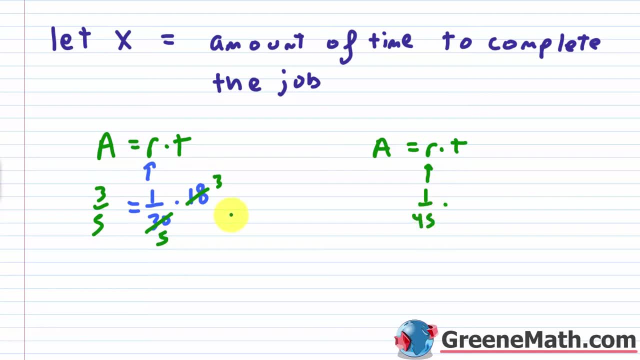 of work is 1 over 45. And the time is the same right, Because they work the same amount of time when they're working together. So this is 18.. Each here is divisible by 9.. 45 divided by 9 would be 5.. 18 divided by 9 would be. 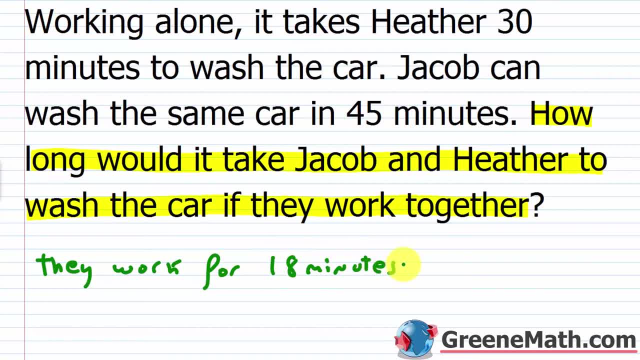 for 18 minutes to complete the job. Okay, you can answer a whole lot of different ways there. That's just a very simple sentence to say they work for 18 minutes to complete the job. Now is it correct? How can? 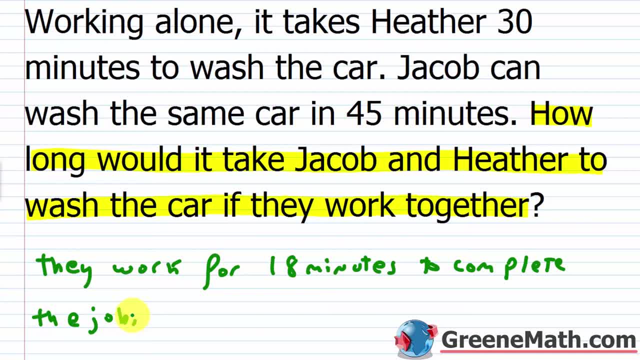 we check this? Well, we can take the fractional amount that Heather does and the fractional amount that Jacob does and add those together and see if it equals 1.. So we know that, if we go back down, a is equal to r times t. I'm going to put it here. I'm going to put it here. I'm going to put it. 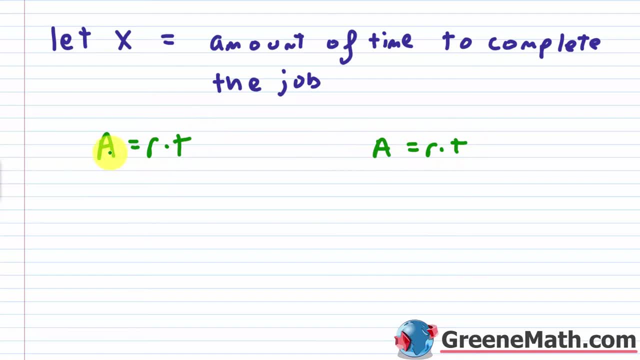 here I'm going to put two scenarios. a equals r times t. So how much or what amount of the job does Heather do? Well, remember her r. her rate of work is 1 over 30. And she works for t minutes. 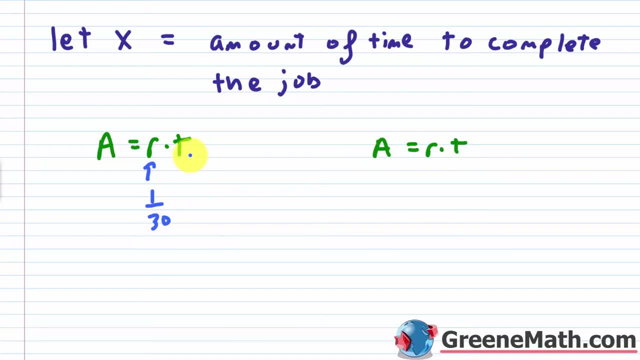 And again we found that the time that they're going to work together, which we labeled as x, was going to be 18.. So essentially I'm going to put this as times 18.. That's going to give me the amount of work that she does. So between 18 and 30,, I have a common factor of 6.. So if I divide 18, 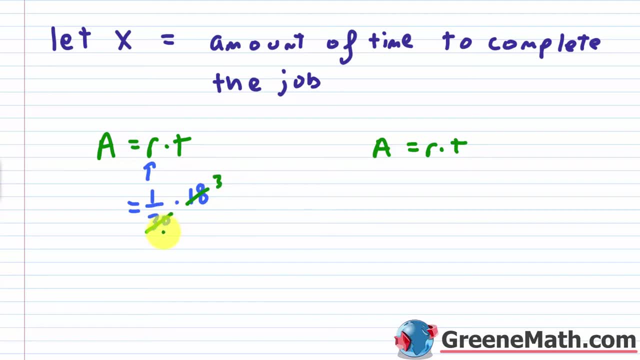 by 6, I get 3.. If I divide 30 by 6, I get 5.. So I get 3 fifths there. So this is going to be 3 fifths. That's the amount of work that she completes Now for Jacob. he's a little bit slower, So his rate of work is: 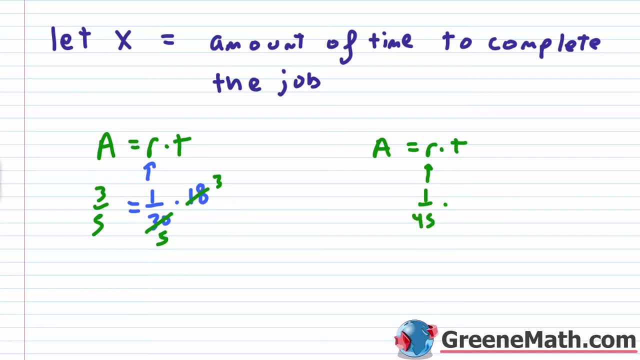 1 over 45. And the time is the same right, Because they work the same amount of time when they're working together. So this is 18.. Each here is divisible by 9.. 45 divided by 9 would be 5.. 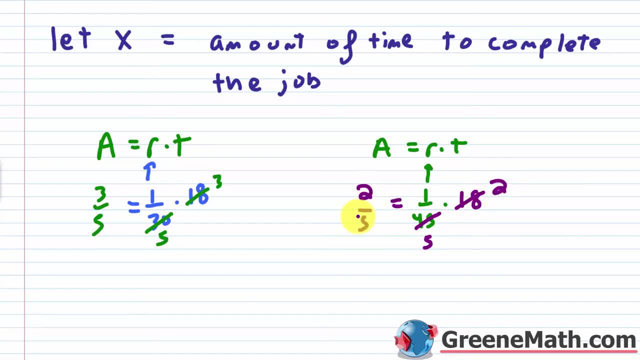 18 divided by 9 would be 2.. So this is 2 fifths. Now, if you go ahead and take the amount of work that Jacob completes, which is 2 fifths, that's what he does in 18 minutes and you add that to the amount of work that Heather completes. 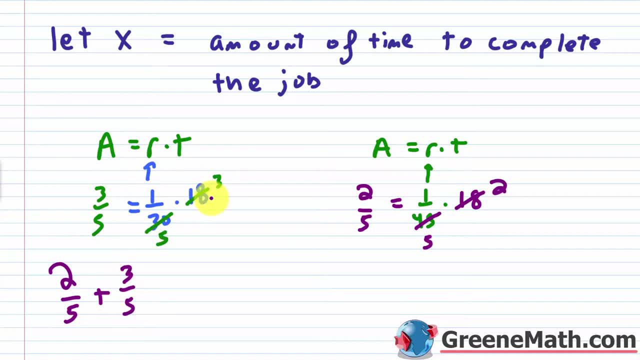 she's got 3 fifths of the job. that's completed And that's what she does. in 18 minutes. You do get 1, right: 2 fifths plus 3 fifths is 5 fifths, 5 fifths is 1.. So we can say: our answer here is: 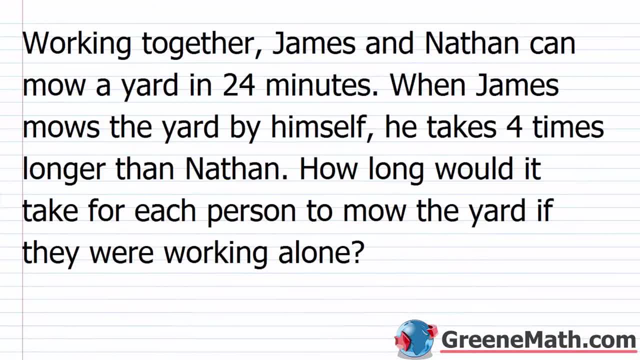 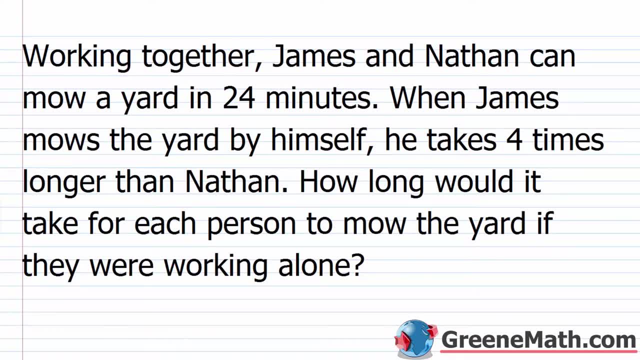 correct, They work for 18 minutes to complete the job. All right, Very easy overall. Let's take a look at another one. So, working together, James and Nathan can work for 18 minutes to complete the job. They can mow a yard in 24 minutes. When James mows the yard by himself, he takes four times. 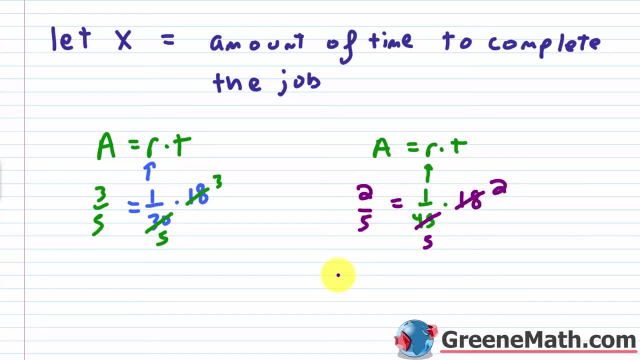 2. So this is 2 fifths. Now, if you go ahead and take the amount of work that Jacob completes, which is 2 fifths, that's what he does in 18 minutes and you add that to the amount of work. 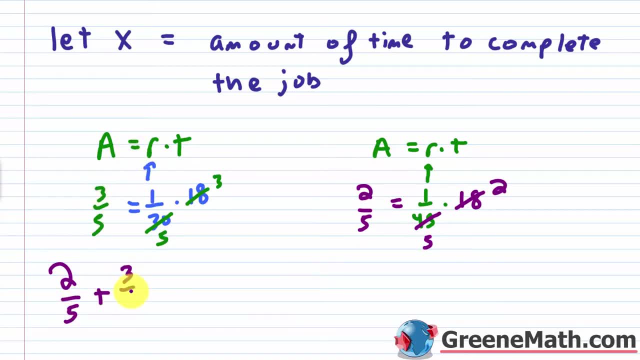 that Heather completes. she's got 3 fifths of the job. that's completed And that's what she does in 18 minutes. You do get 1, right: 2 fifths plus 3 fifths is 5 fifths, 5 fifths is 1.. So we can. 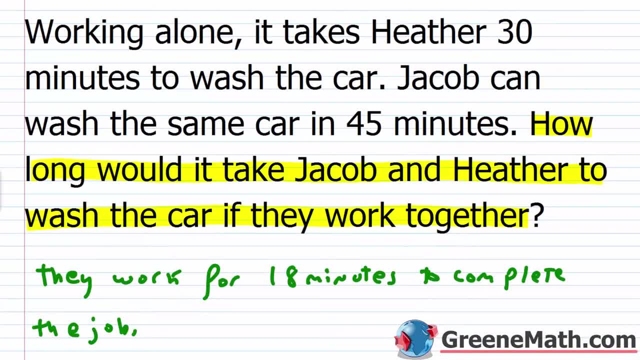 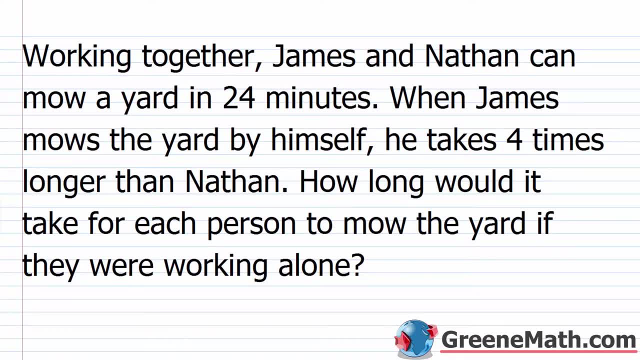 say, our answer here is 1.. So we're going to add that to the amount of work that Jacob completes. They work for 18 minutes to complete the job. All right, Very easy overall. Let's take a look at another one. So, working together, James and Nathan can mow a yard in 24 minutes. 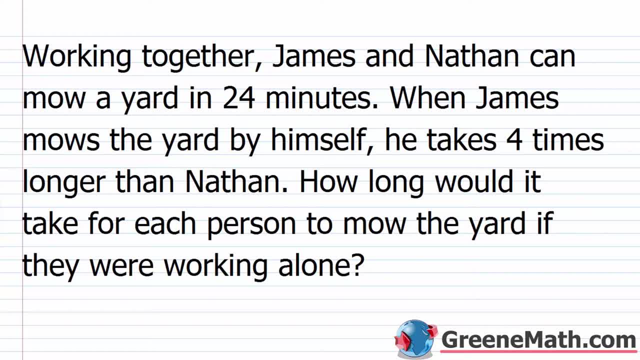 When James mows the yard by himself, he takes 4 times longer than Nathan. How long would it take for each person to mow the yard if they were working alone? So in the last problem, we knew their individual rates of work, right, We knew that. 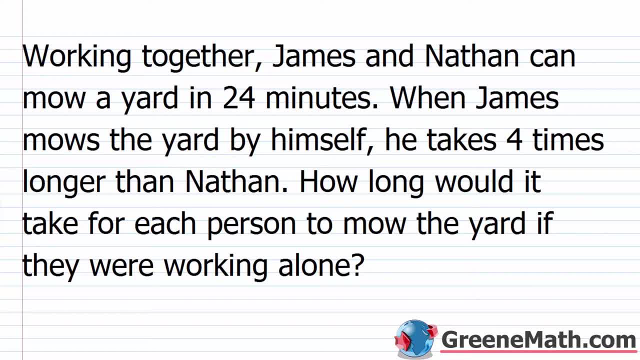 for Jacob, he could wash the car in 45 minutes. For Heather, she could wash the car in 30 minutes. But we didn't know, or we could say we had defined, how long it would take if they worked together In this case. we know how long it takes when they work together, right? It tells us, right? 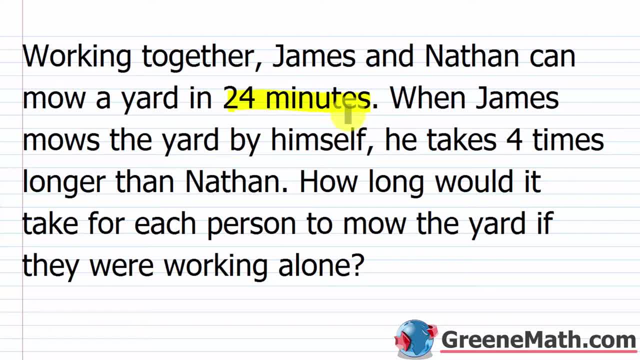 here it's 24 minutes, But we don't know how long it takes them individually, okay. So that's the question here: How long would it take for each person to mow the yard if they were working alone? So how long does it take for James? How long does it take for Nathan? So we're specifically told. 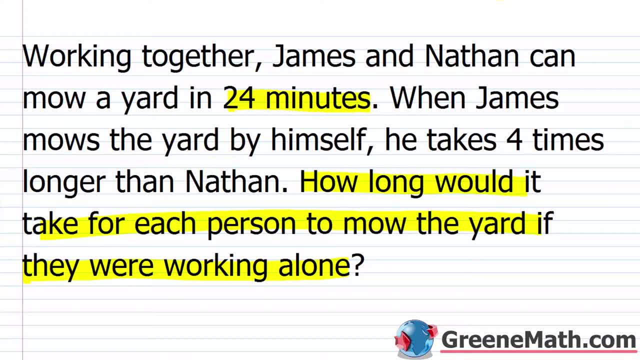 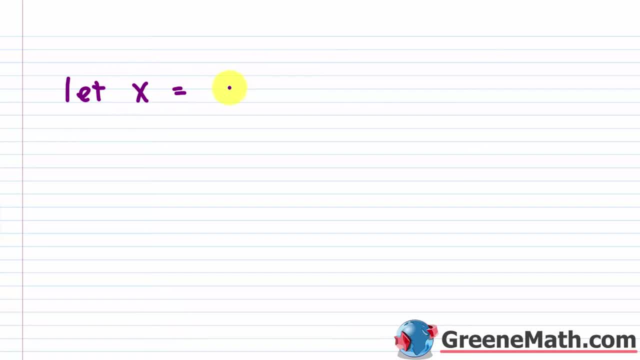 that James takes 4 times longer than Nathan. So let's let x be equal to the amount of time it takes for Nathan to mow the yard by himself. So the time for Nathan, and I'm not going to write the rest. you can write the rest if you want, but it's just the time for. 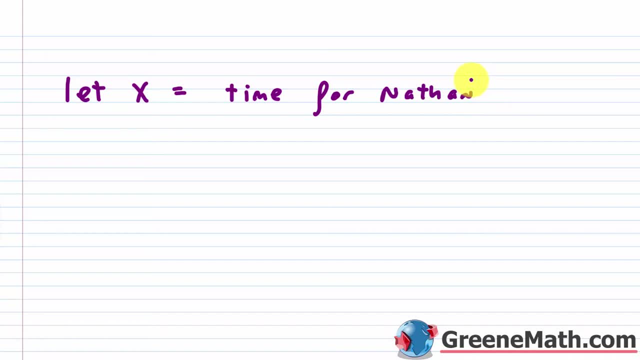 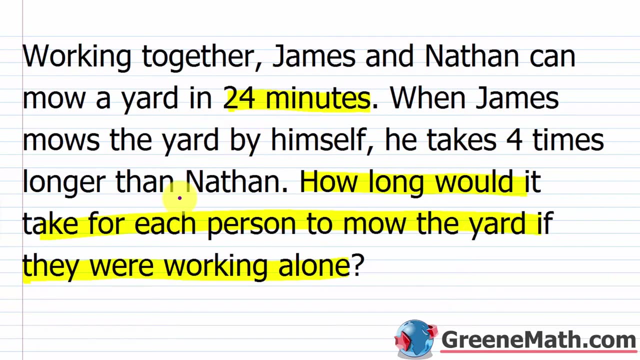 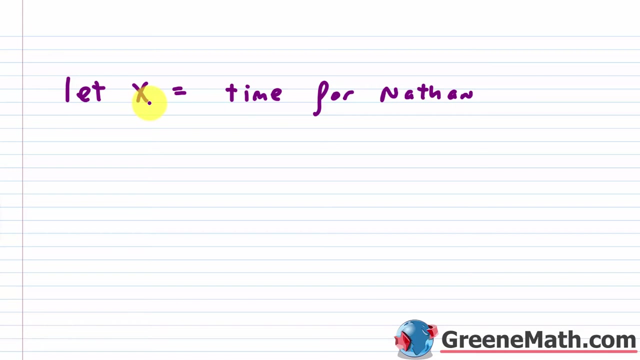 Nathan to again mow the yard by himself. So then, because James takes 4 times longer, again, it tells us that right here. when James mows the yard by himself, he takes 4 times longer than Nathan. What I can do is just multiply 4 times x to get the time for James. So I could say: 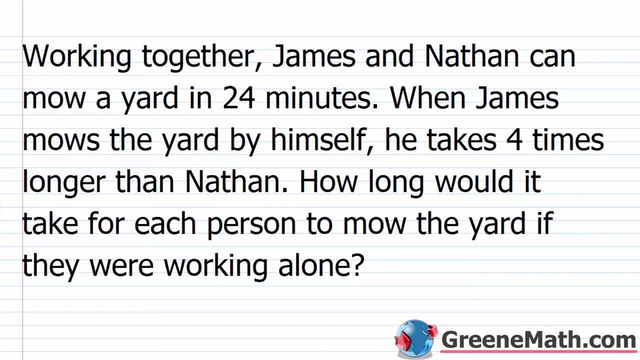 longer than Nathan. How long would it take for each person to mow the yard if they were working alone? So in the last problem we knew their individual rates of work right. We knew that for Jacob, he could wash the car in 45 minutes. For Heather, she could wash the car in 30 minutes. 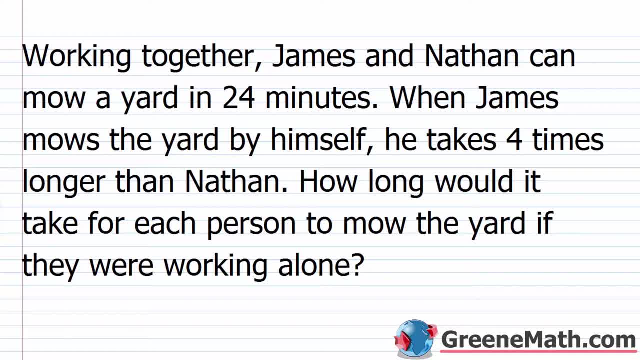 But we didn't know, or we could say we had defined, how long it would take if they worked together. In this case, we know how long it takes when they work together. right, It tells us right here it's 24 minutes. So we know how long it would take if they worked together And we know how long it. 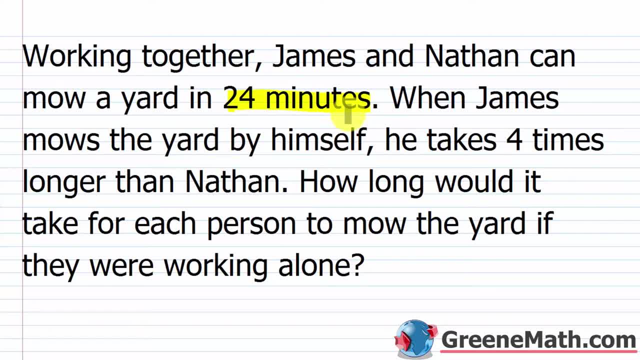 would take for each person to mow the yard if they were working alone. So how long does it take for James? How long does it take for Nathan? So we're specifically told that James takes four times longer than Nathan. So let's let X be equal to the amount of time it takes for Nathan to mow the yard. 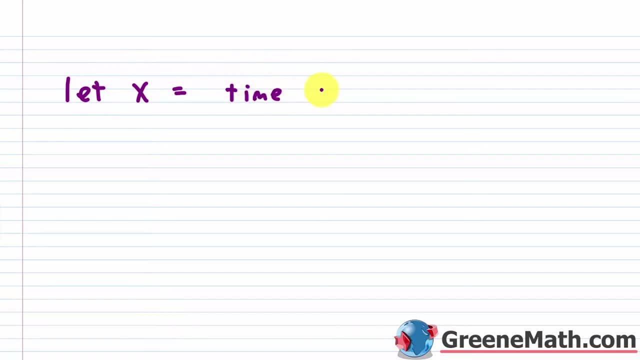 by himself. So the time for Nathan- and I'm not going to say how long it takes for Nathan, but I'm not going to write the rest. You can write the rest if you want, but it's just the time for Nathan to again mow the yard by himself. So then, because James takes four times longer? 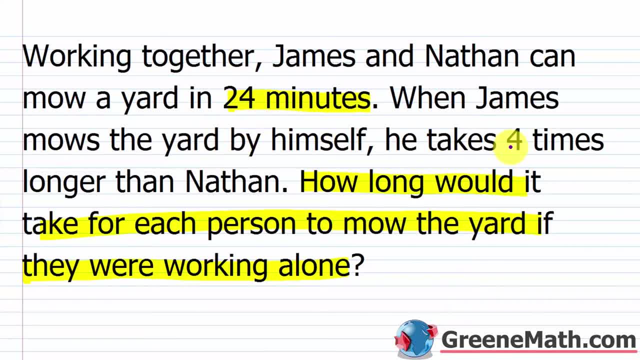 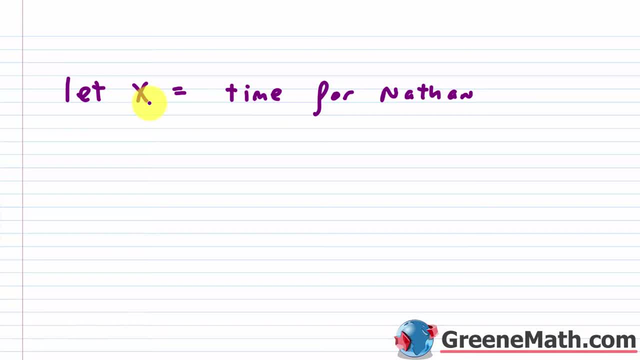 again. it tells us that right here. when James mows the yard by himself, he takes four times longer than Nathan. What I can do is just multiply four times X to get the time for James. So I could say then four X is equal to the time for James. Okay, 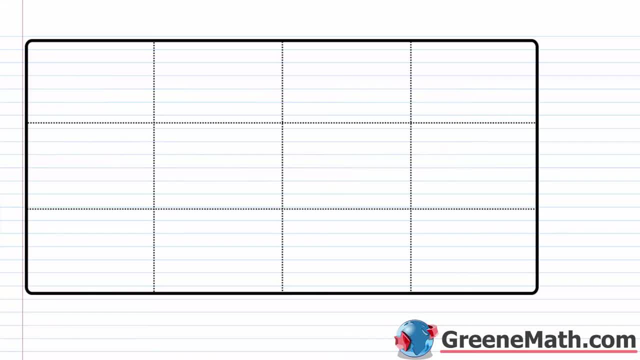 Okay, Let's go back to our table and kind of organize. So again we have Nathan and James, So we have Nathan and we have James, And again we have the rate of work. the rate of work and we have the time working together. 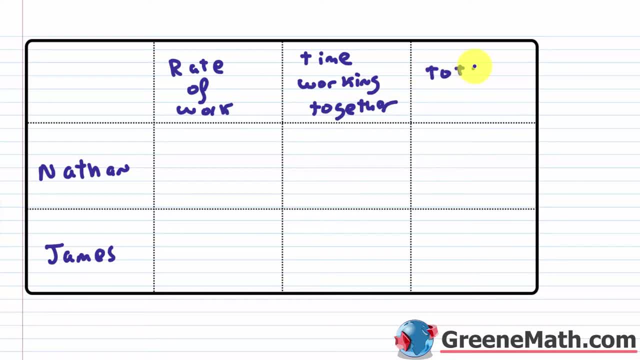 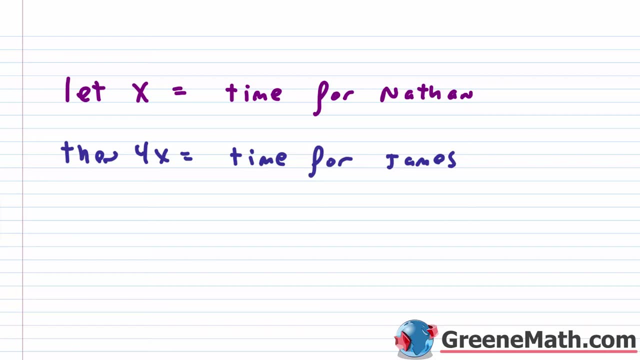 And then we have their total contribution. So for the rate of work, remember it's one over the amount of time it takes for that person to complete the job. So if it takes me four hours to paint a house, again the rate of work is 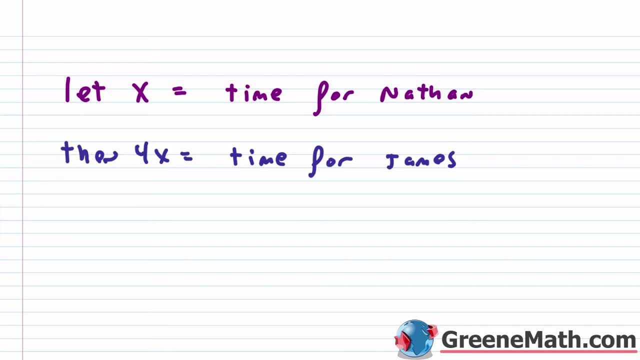 one over four. That's how much I'm going to do in one unit of time. So in an hour I'm going to do one fourth of the job. Here we know for Nathan this is in terms of minutes he can complete one over the amount of time it takes for that person to complete the job. 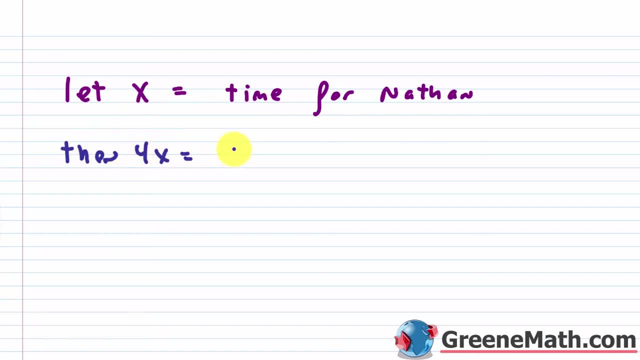 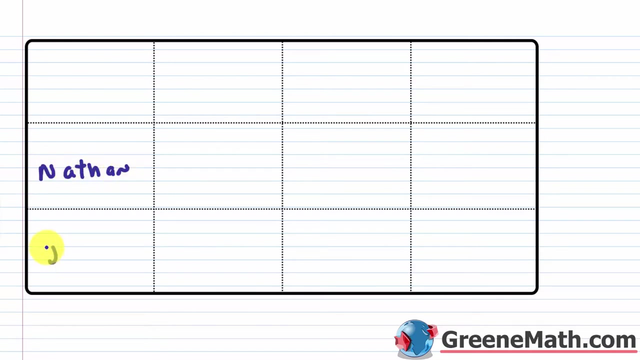 again, 4x is equal to the time for James. Okay, let's go back to our table and kind of organize. So again we have Nathan and James. So we have Nathan and we have James, And again we have the rate of work. the rate of work and we have the time working together. 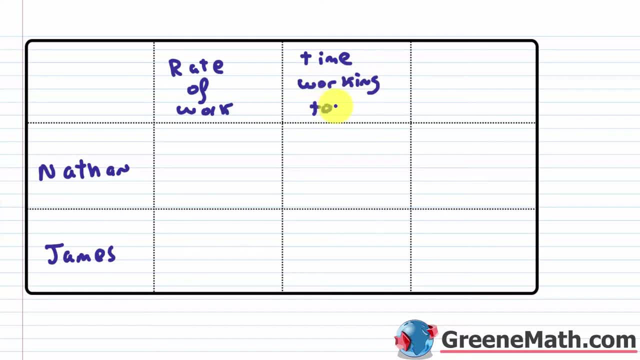 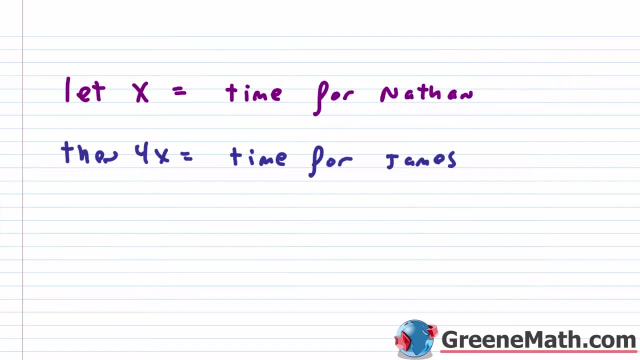 and then we have their total contribution. So for the rate of work, remember it's 1 over the amount of time it takes for that person to complete the job. So if it takes me 4 hours to paint a house, again the rate of work is 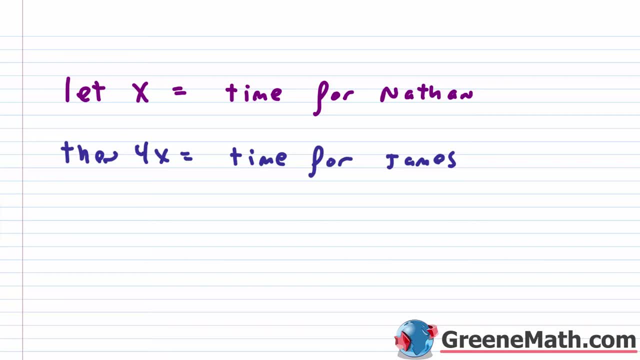 1 over 4.. That's how much I'm going to do in 1 unit of time. So in an hour I'm going to do one-fourth of the job Here we know. for Nathan this is in terms of minutes. 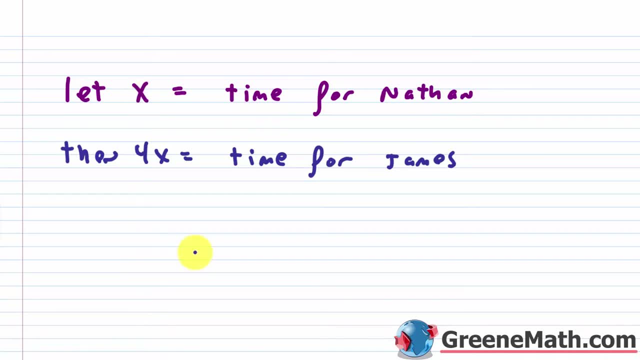 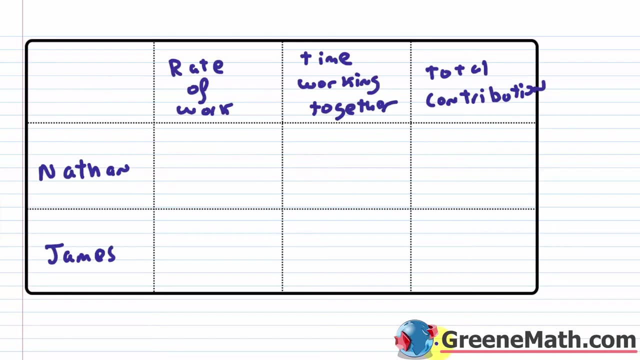 he can complete 1 over x amount of that job every minute. Okay, So for James it's going to be 1 over 4x every minute. So for Nathan it's 1 over x, For James it's 1 over 4x. 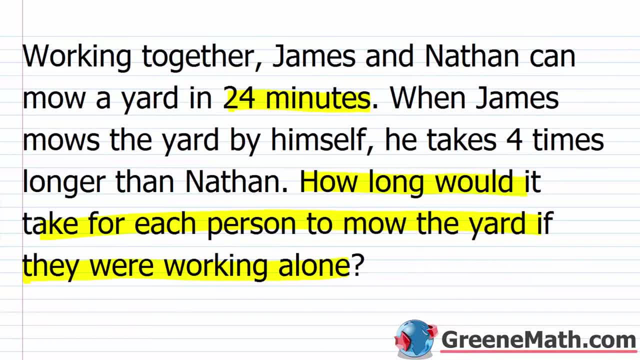 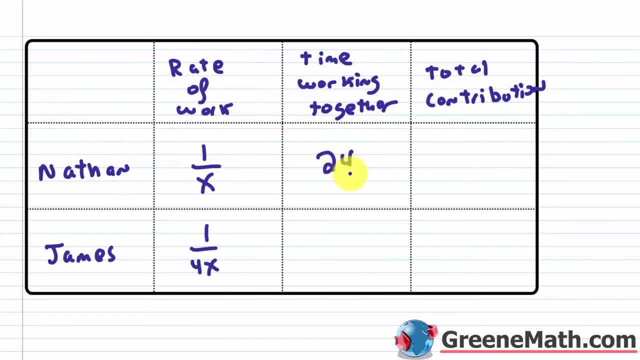 The time working together. It tells us that in the problem, It tells us specifically that James and Nathan can mow a yard in 24 minutes. That's again when they're working together. So each person is going to work for 24 minutes in this scenario. 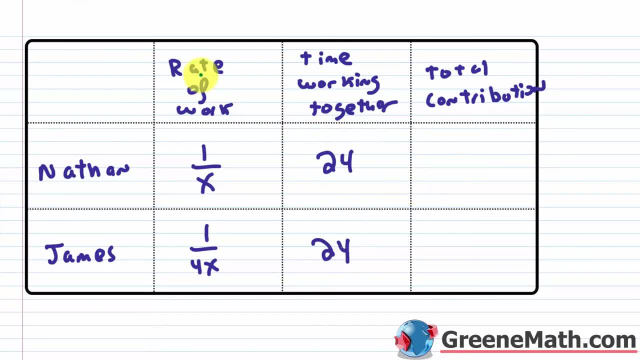 So what's their contribution? Again, you just multiply. This is the rate of work, This is the time working. So 24 times 1 over x. You can do just 24 over x to make it simpler. And then here it's 24 over 4x, which we could simplify. 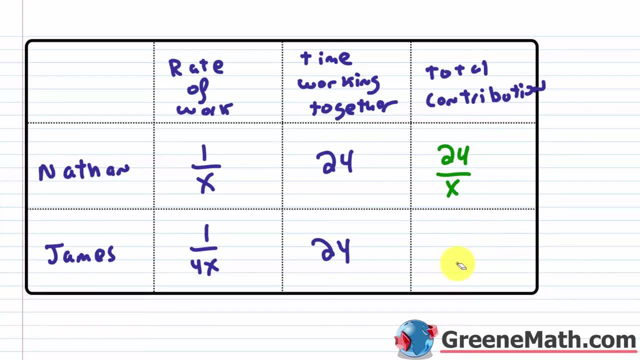 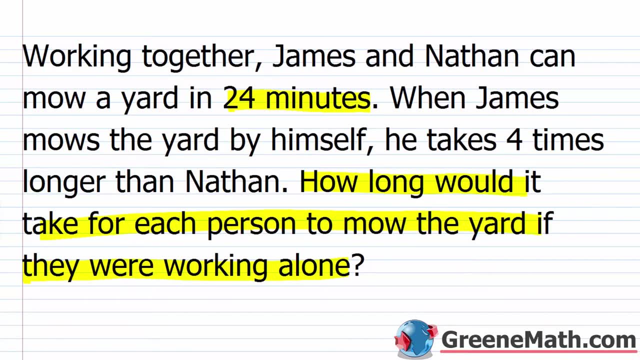 24 over 4 is 6.. So I could just say this is 6 over x. Now how do we get an equation going? Well, we know that When we sum the amount of work done from both of them over this again 24-minute period. 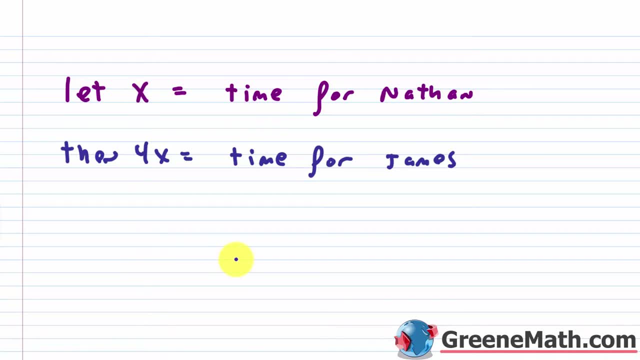 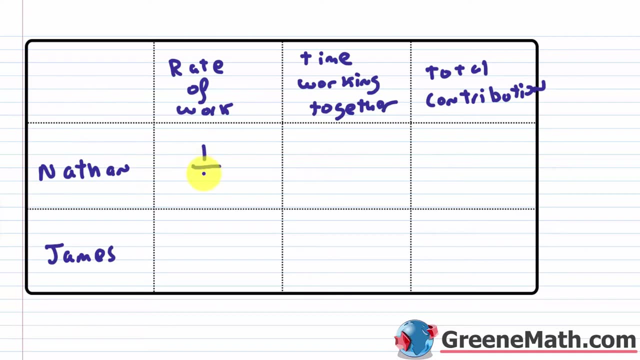 So for Nathan, it's one over X amount of that job every minute, Okay. So for James it's going to be one over four X every minute. So for Nathan, it's one over X. For James, it's one over four X. 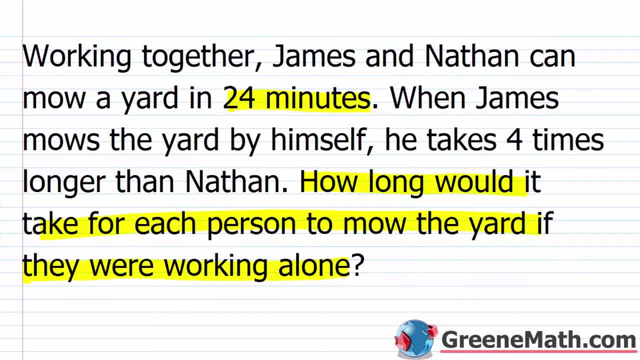 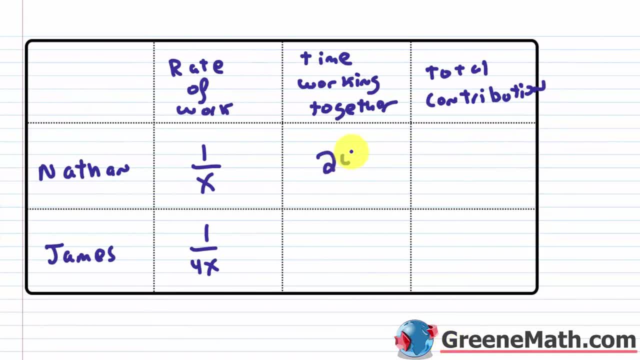 The time working together. it tells us that in the problem, It tells us specifically that James and Nathan can mow a yard in 24 minutes. That's again when they're working together. So each person is going to work for 24 minutes in this scenario. So what's their contribution? Again, 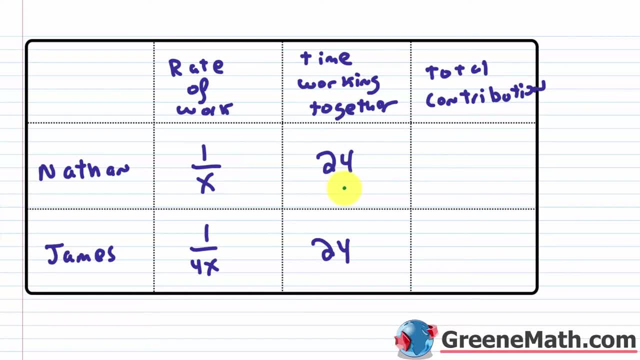 you just multiply, So the rate of work. this is the time working. So 24 times one over X, you can do just 24 over X to make it simpler. And then here it's 24 over four, X, which we could simplify. 24 over four is: 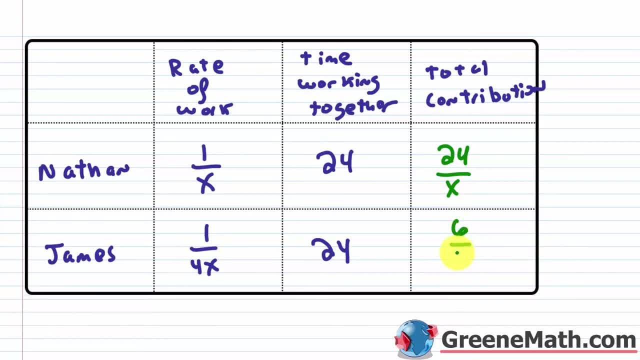 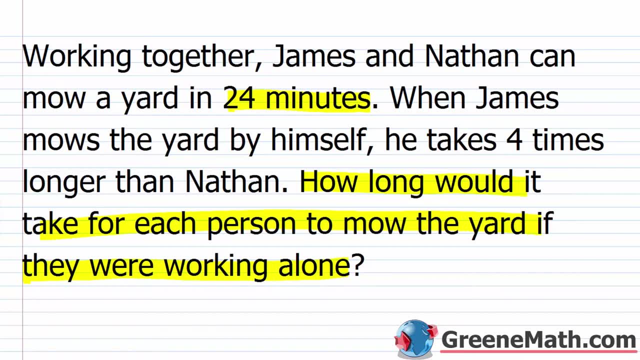 six. So I could just say this is six over X. Now how do we get an equation going? Well, we know that when we sum the amount of work done from both of them over this again 24 minute period, they've completed one job. So the amount of work that Nathan? 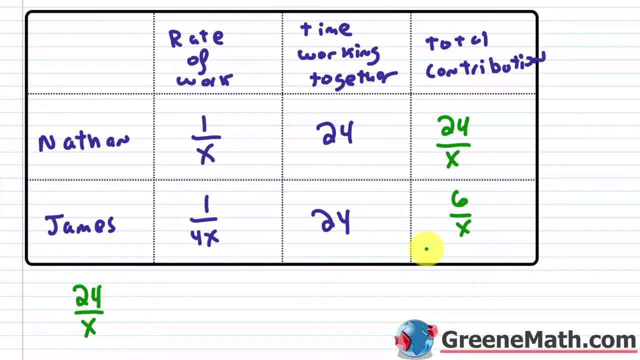 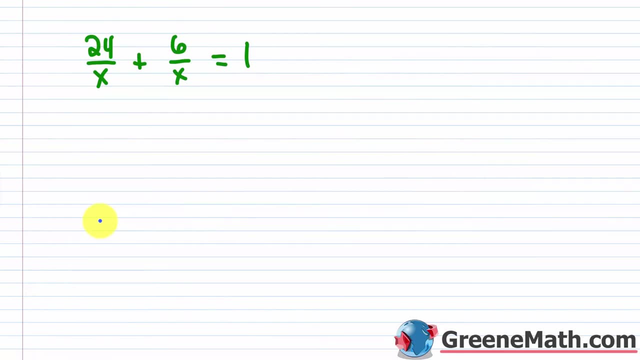 does is 24 over X. The amount of work that James does is six over X. If I add these two amounts together, I should get one completed job. So let's copy this, All right. So what can I do here? Well, I can multiply both sides of the equation by X. right, That would be the LCD. 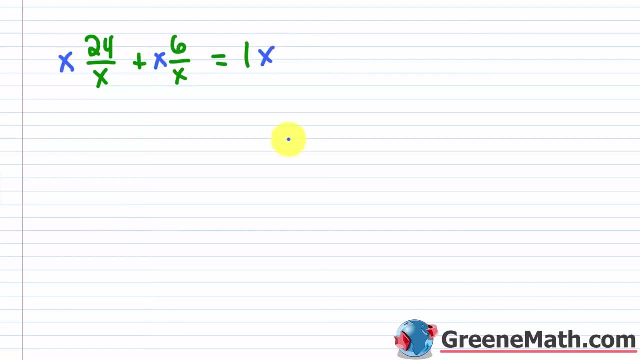 So I'll multiply this by X, this by X and this by X. So, essentially, this is going to cancel. This is going to cancel. You'll basically just have what: 24 plus six, which is 30, is equal to X. 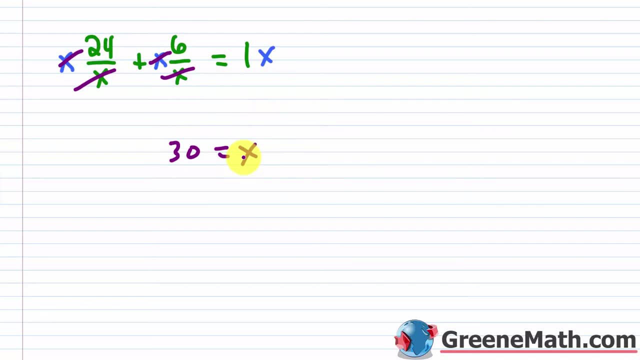 So that's really a piece of cake. We've immediately found that X is 30. And we know that X was the time for Nathan, So this is going to be 30 minutes, And then for James it's going to be four times that, or 120 minutes. If you wanted to put that in terms of hours, you could. that's two. 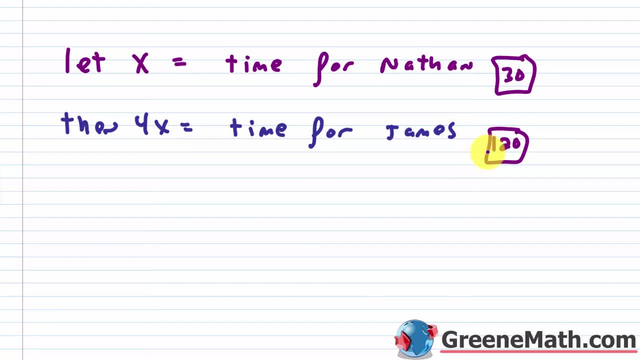 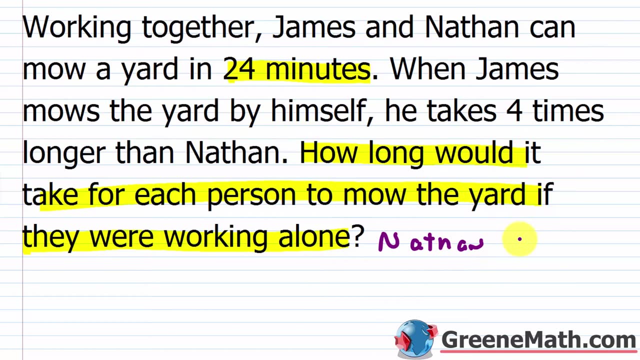 hours. If you didn't know that, it's okay. You can put it in terms of minutes, right, It doesn't matter. So I'm just going to say that Nathan can mow the yard in 30 minutes. So Nathan can mow. 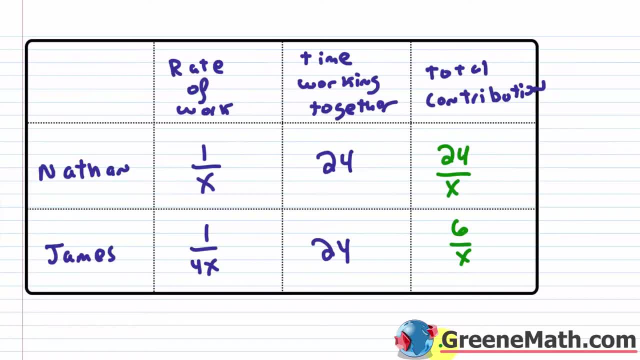 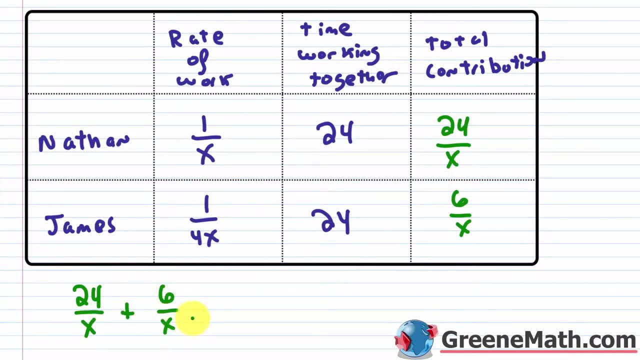 they've completed one job. So the amount of work that Nathan does is 24 over x. The amount of work that James does is 6 over x. If I add these two amounts together, I should get one completed job. So let's copy this: 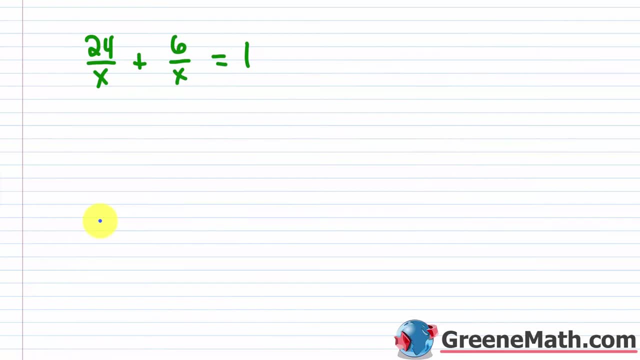 Alright. so what can I do here? Well, I can multiply both sides of the equation by x. right, That would be the LCD. So I'll multiply this by x, This by x And this by x. So essentially, this is going to cancel. 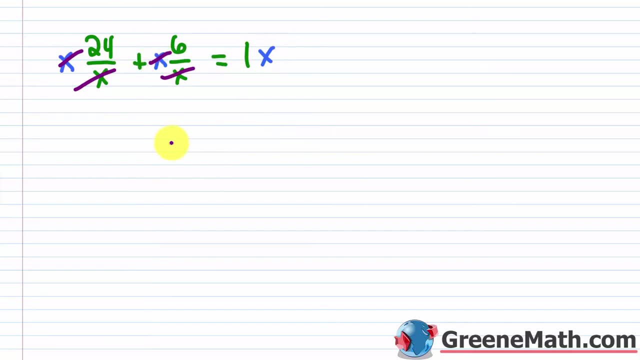 This is going to cancel. You'll basically just have what: 24 plus 6,, which is 30,, is equal to x. So that's really a piece of cake. We've immediately found that x is 30. And we know that x was the time for Nathan. 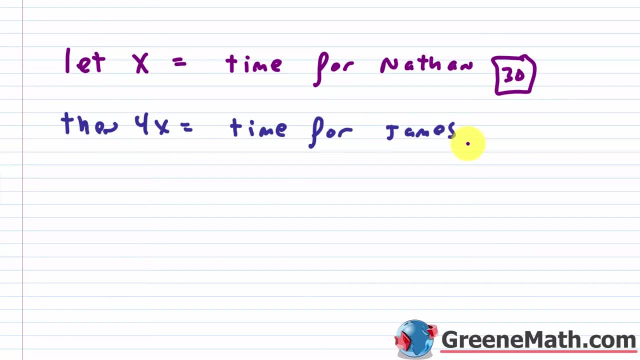 So this is going to be 30 minutes, And then for James it's going to be 4 times that, or 120 minutes. If you wanted to put that in terms of hours, you could. That's 2 hours. 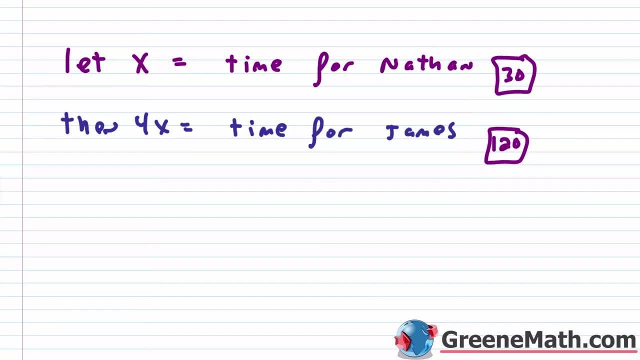 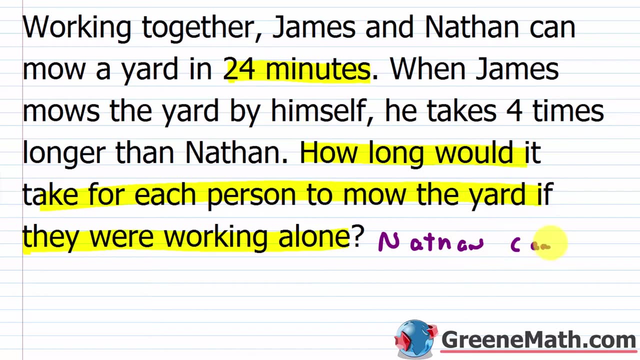 If you didn't know that, it's okay. You can put it in terms of minutes, Right, It doesn't matter. So I'm just going to say that Nathan can mow the yard in 30 minutes. So Nathan can mow the yard in 30 minutes. 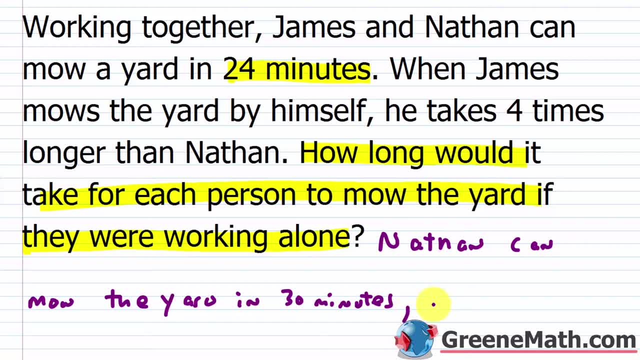 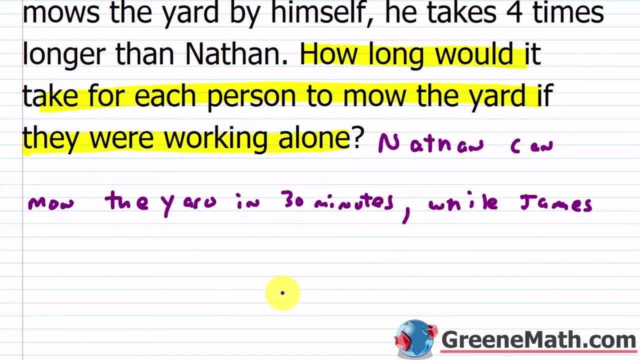 Then I'll say, while James can do it, Okay, And you can say 2 hours or 120 minutes. I'll just say 120 minutes because the problem was given in minutes. But again, you can put 2 hours, It's the same thing. 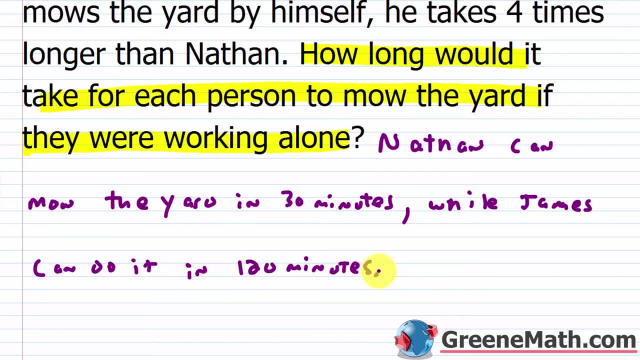 So does this make sense? Let's kind of scooch up just a little bit. So again, working together, James and Nathan can mow a yard in 24 minutes. So we know that When James mows the yard by himself, he takes 4 times longer than Nathan. 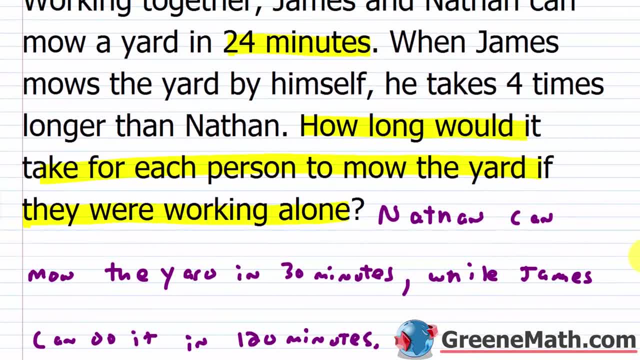 So, according to our answer, James does it in 120 minutes and Nathan does it in 30 minutes. So if this is correct, we're good to go. Okay, So we know that. So we know that. So we know that. 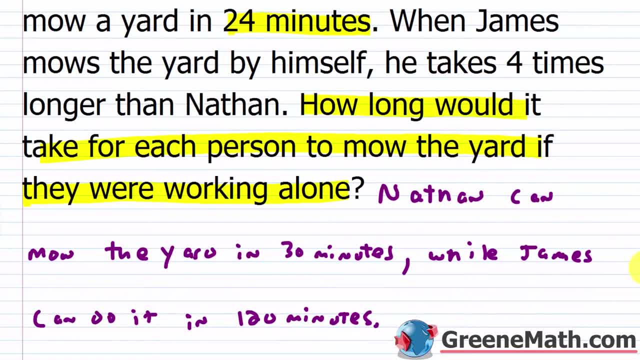 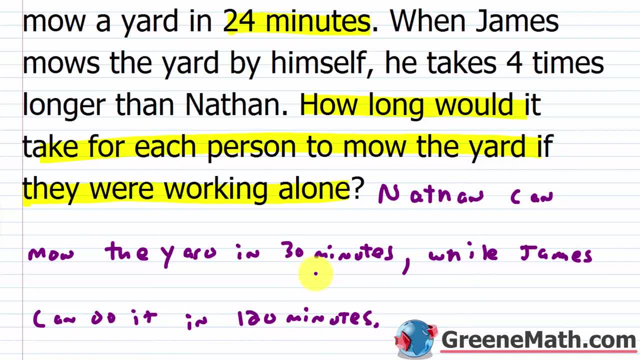 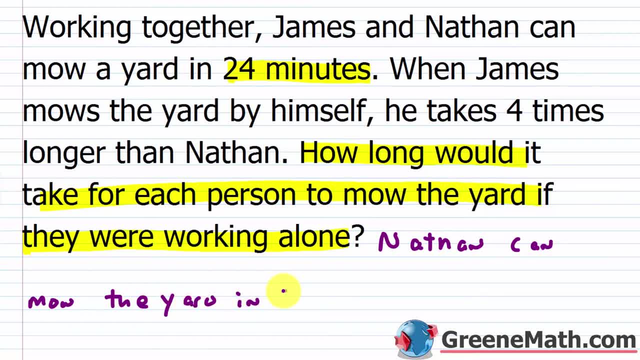 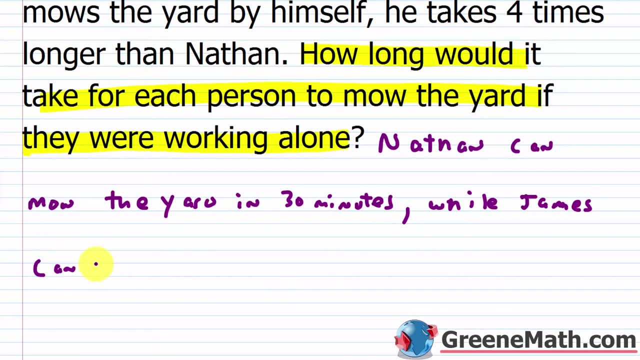 The yard in 30 minutes. Then I'll say: while James can do it And you can say two hours or 120 minutes, I'll just say 120 minutes because the problem was given in minutes, But again you can put two hours, It's the same thing. So does this make? 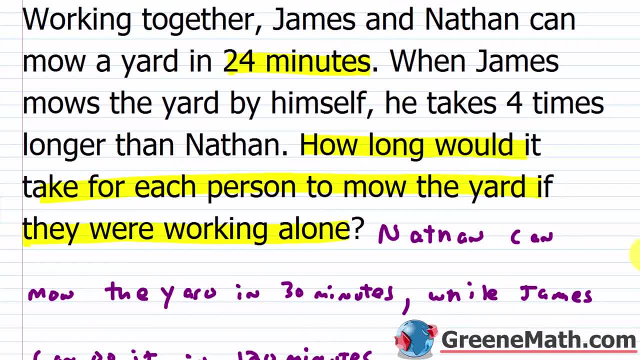 sense. It's kind of simple. I'm going to put two hours, I'm going to put two hours, I'm going to scooch up just a little bit. So again, working together. James and Nathan can mow a yard in 24. 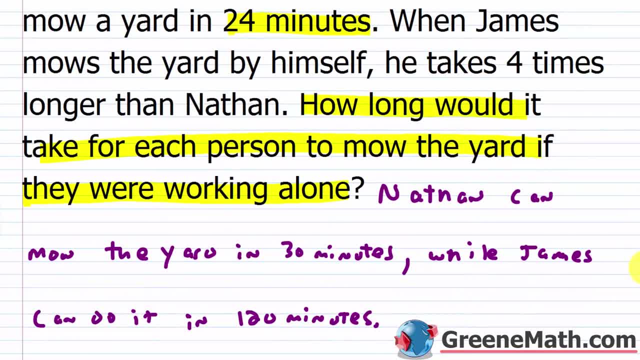 minutes. So we know that when James mows the yard by himself, he takes four times longer than Nathan. So, according to our answer, James does it in 120 minutes and Nathan does it in 30 minutes. So if this is correct, we're good to go right, Because it is four times 30 times four will give. 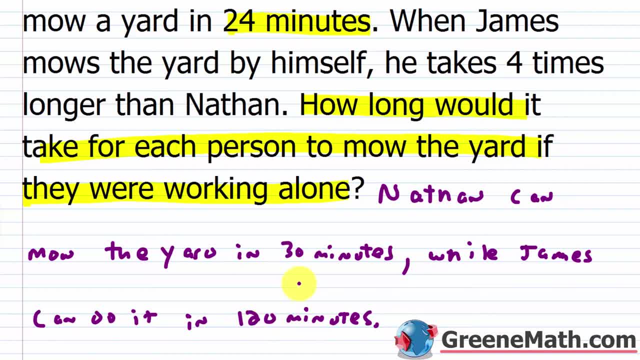 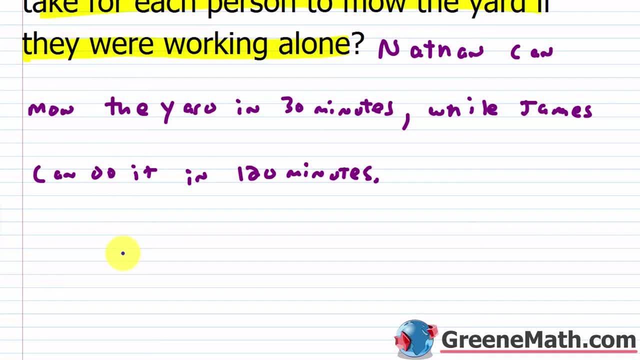 me 120.. So that part does check out. We just need to make sure that they can work together and get it in 24 minutes. So again, think about this: The amount of work that Nathan does is he's going to do one over 30 of that job every minute. 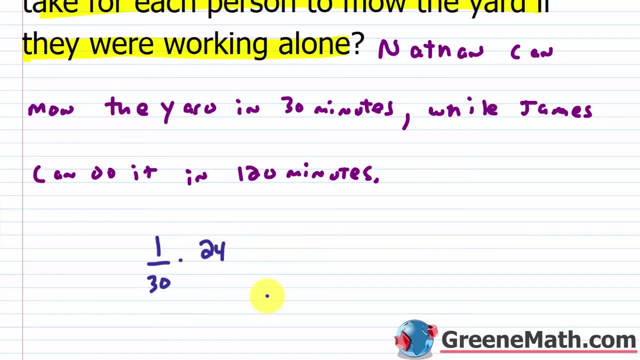 So he's going to do this again. if they work together for 24 minutes, Then if I add to this how much James does, So he's going to do one over 120 of that job for every minute And he's going to do that for 24 minutes. If I sum these amounts, I should get. 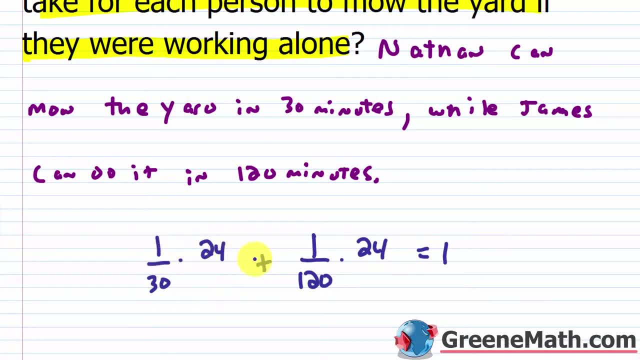 one. This is the amount that Nathan does all the way to the left. Then we have plus. Again we have the amount that kind of James does over here. Again, if I sum them, I should get one. So how can I reduce this here? Well, I can divide both by six. That would give me a four here and a. 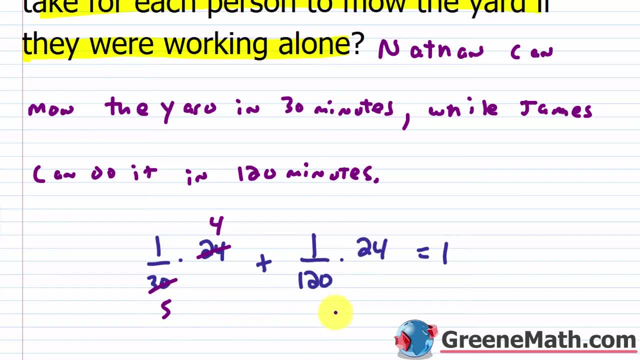 five here For this one. 120 divided by 24 is five, So I can cancel this with this and put a five here. So you've got four fifths of the job, which is what Nathan's going to do, plus one fifth of the. 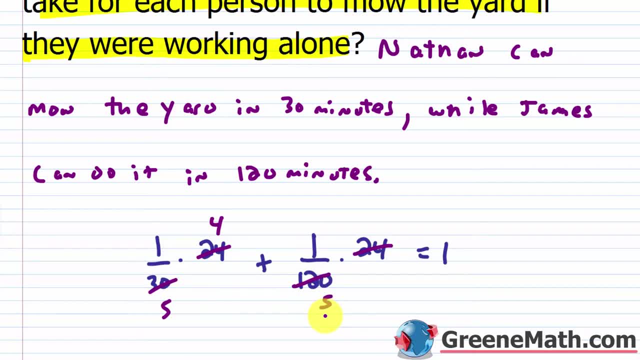 job, which is what James is going to do. You sum those two amounts together, you get five fifths, or one Again for one complete. So our answer here is correct: Nathan can mow the yard in 30 minutes, while James can do it in 120. 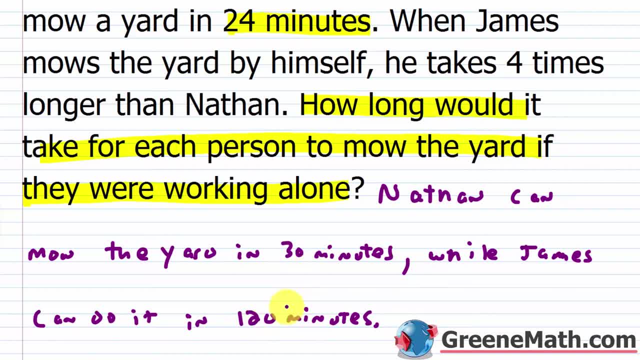 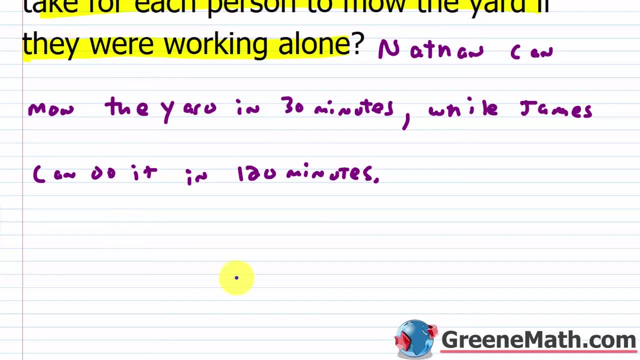 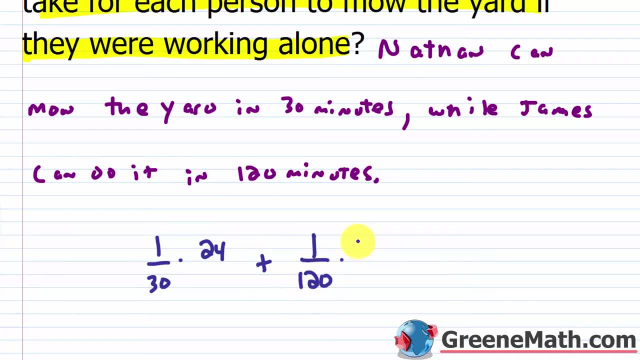 that job for every minute and he's going to do that for 24 minutes. if i sum these amounts, i should get one. this is the amount that nathan does all the way to the left. then we have plus again. we have the amount that kind of james does over here. again, if i sum them, i should get one. 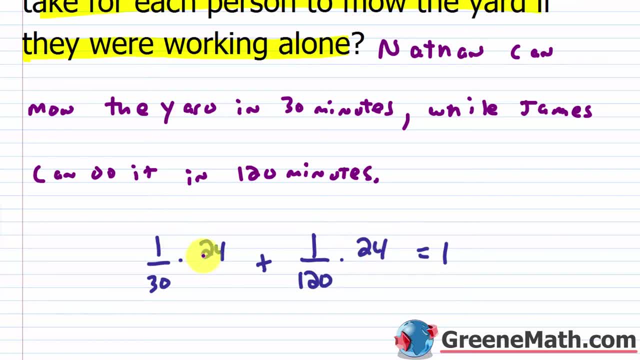 so how can i reduce this here? well, i can divide both by six. that would give me a four here and a five here. for this one, 120 divided by 24 is five, so i can cancel this with this and put a five here. so you've got four fifths of the job, which is what nathan's going to do, plus one fifth of the job. 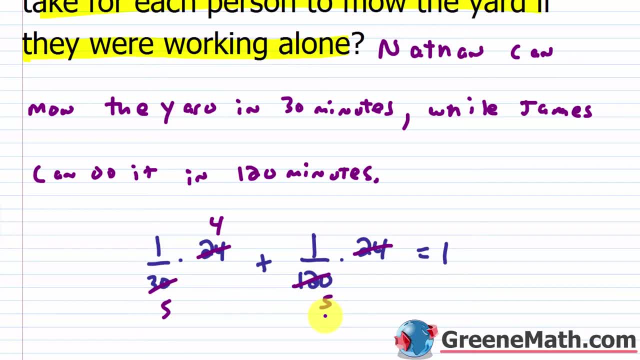 which is what james is going to do. you sum those two amounts together, you get five fifths, or one again for one completed job. so our answer here is correct: nathan can mow the yard in 30 minutes, while james can mow the yard in 30 minutes. 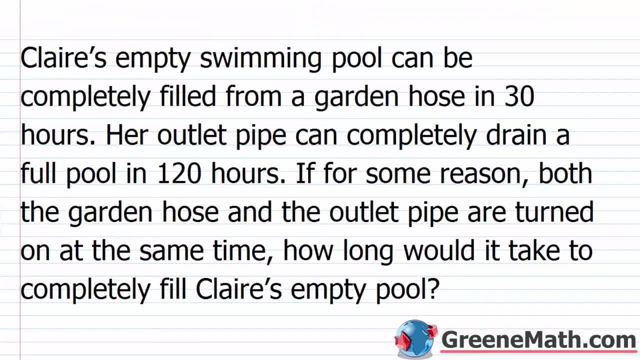 james can do it in 120 minutes or again two hours. okay, so pretty easy overall. let's look at one that's a little bit more challenging, but again it's not so much because these problems are really easy. so claire's empty swimming pool can be completely filled from a garden hose in 30 hours. 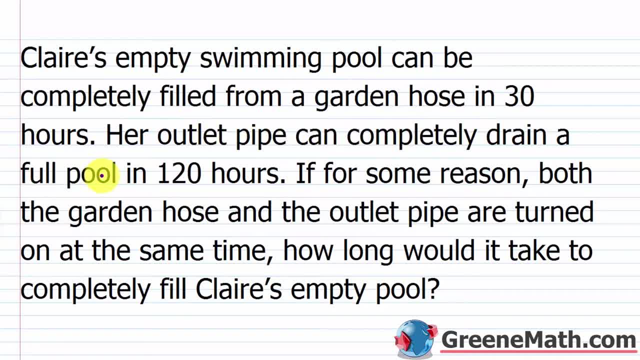 her outlet pipe can completely drain a full pool in 120 hours. if, for some reason, both the garden hose and the outlet pipe are turned on at the same time, how long would it take to completely fill claire's empty pool? so the question we need to answer here is: how long would it take to completely fill claire's empty? 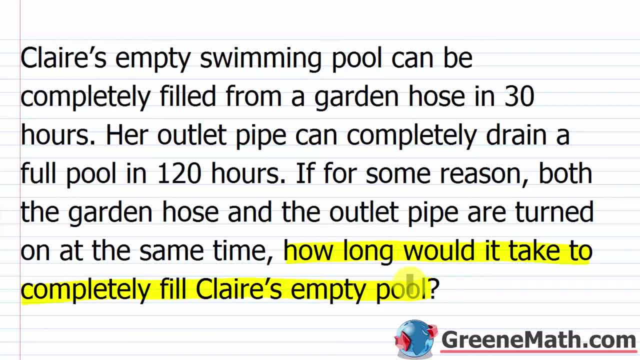 pool. given these two competing forces, you've got one kind of hose pipe that's filling the pool and then you've got an outlet pipe or you could say a drain pipe that's emptying the pool, so they're kind of working against each other. you can think about this as if you're filling your 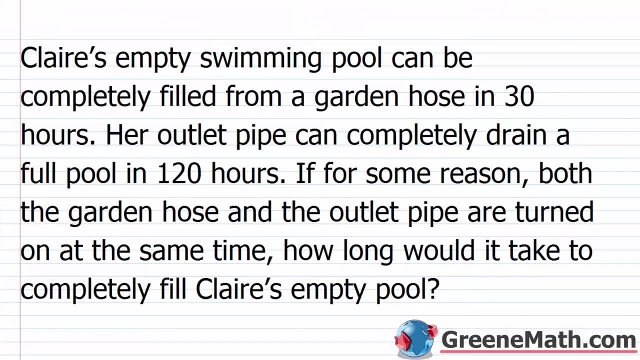 minutes, or again two hours. Okay, So pretty easy overall. Let's look at one that's a little bit more challenging, but again it's not so much because these problems are really easy. So Claire's empty swimming pool can be completely filled from a garden hose in 30 hours. Her outlet pipe can. 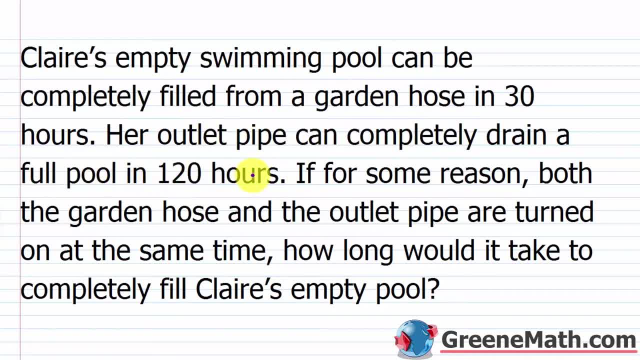 completely drain a full pool in 120 hours. If, for some reason, both the garden hose and the outlet pipe are on at the same time, how long would it take to completely fill Claire's empty pool? So the question we need to answer here is: how long would it take to completely fill Claire's empty? 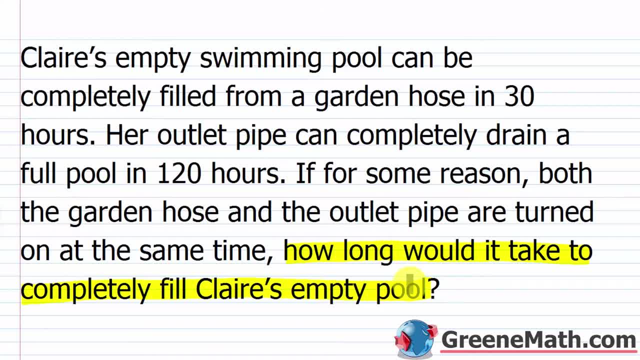 pool. Given these two competing forces, you've got one kind of hose pipe that's filling the pool and then you've got an outlet pipe or you can say a drain pipe that's emptying the pool, So they're kind of working against each other. You can think about this as if you're filling your kitchen sink. 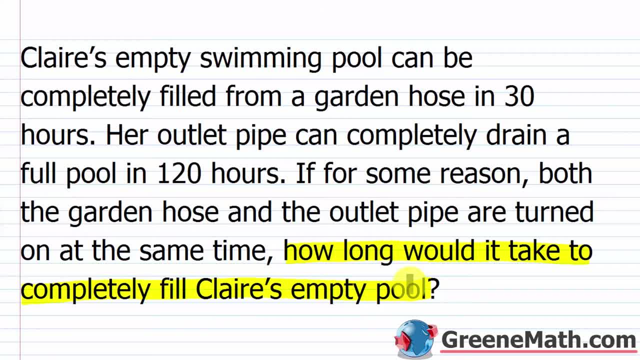 okay, And you kind of you've got the water on full blast, but you hold the stopper just up just a little bit, right? So some of the water can drain. So if the amount of water coming in is more than the amount of water going out, eventually you're going to fill your sink, right, But it's just. 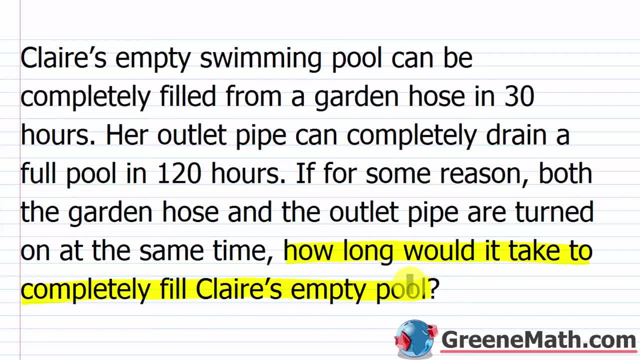 going to take longer than if you had the sink kind of all the way stopped up. Okay, So that's the idea of what's going on here. So how can we model this? Let's just say we're going to let X be equal. 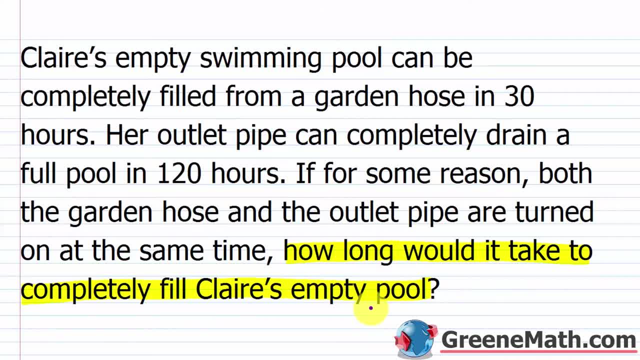 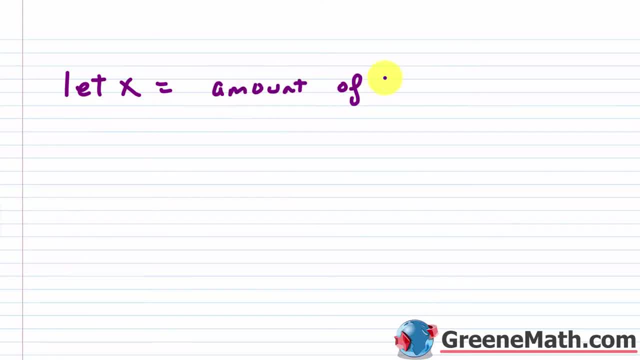 to the amount of time it would take To completely fill Claire's empty pool. So I'm just going to say: let X be equal to the amount of time to fill the pool. Okay, Let's go down to the kind of table. Let's organize some stuff. 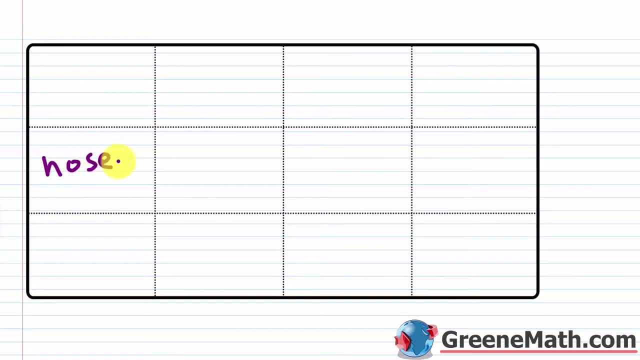 So we've got our hose that's filling the pool and then we've got our outlet pipe that's trying to drain it. So we've got our hose that's filling the pool and then we've got our outlet pipe. And let me be more specific here and just put garden hose. So garden hose because 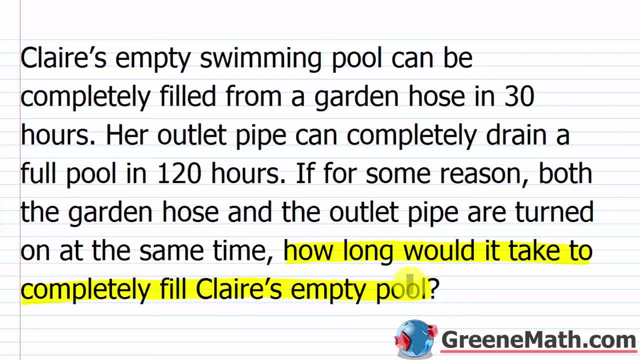 kitchen sink. okay, and you kind of you got the water on full blast, but you hold the stopper just up just a little bit, right? so some of the water can drain. so if the amount of water coming in is more than the amount of water going out, eventually you're going to fill your sink, right? 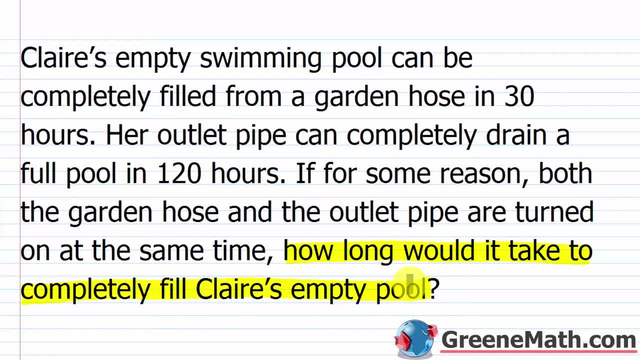 but it's just going to take longer than if you had the sink kind of all the way stopped up. okay, so that's the idea of what's going on here. so how can we model this? let's just say we're going to let x be equal to the amount of time it would take to completely fill claire's empty pool. so i'm just 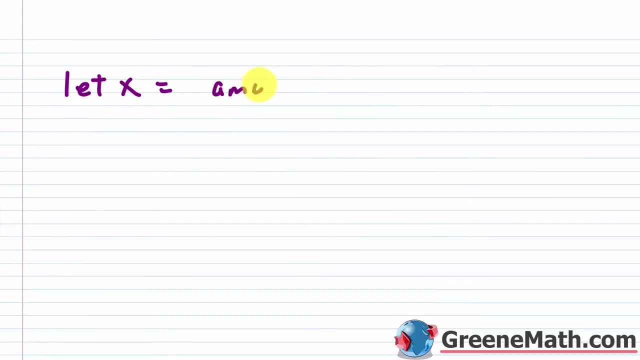 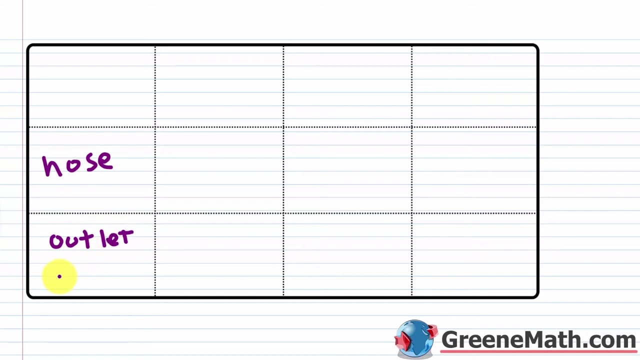 going to say: let x be equal to the amount of time to fill the pool. okay, let's go down to the kind of table, let's organize some stuff. so we've got our hose that's filling the pool and then we've got our outlet pipe that's trying to drain it- and let me be more specific here- and just put garden hose. 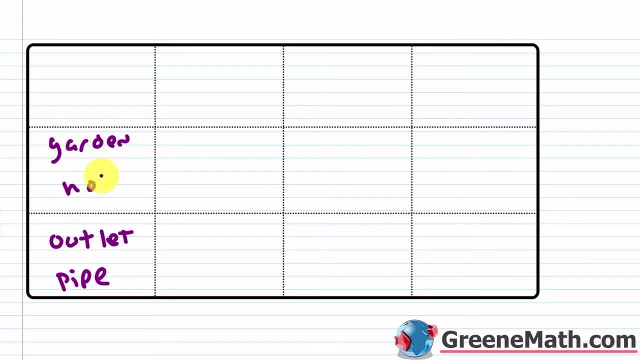 so garden hose, because that's what it says in the problem. now again, we're going to have our rate of work, we're going to have our time working together and then we're going to have our total contribution. so we know one thing so far: it's the time working together is x. 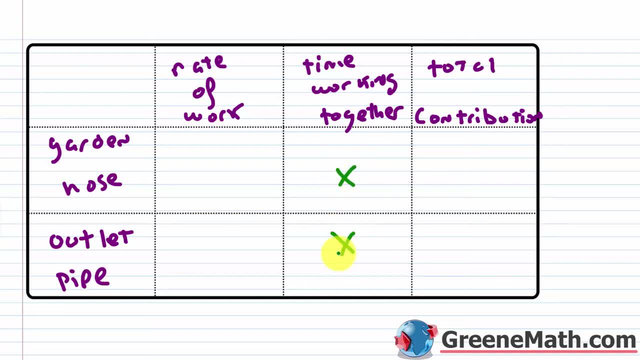 because we just like to have our time working together. and then we're going to have our total contribution and we're going to have our time working together. so i'm going to take this and bring this triple number per hour that was going to the plan, the same way we did last week. if this 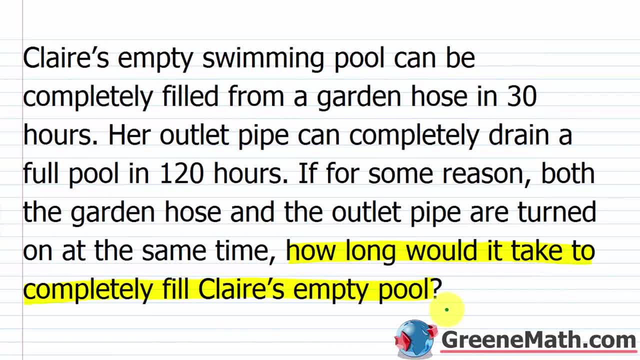 can consider the whole plan and prepare a little bit more than a year square right now. let's put here: that's my objectiveCchain. that should be equal to the amount of time that we need to fill our. there is still enough time left to fill our pool. there is still enough time missing in the 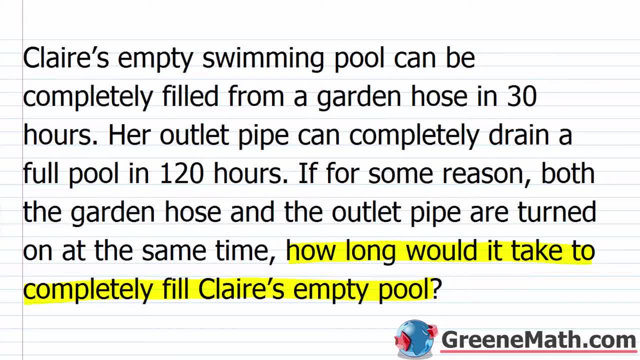 pool. for me, this is something i've very appreciate, because that was a mistake i made. i looked at this and i'm going to use bricks because the rules are all the problems i ground west in style is going to be done much faster. we're just going to go all the way to where the next part of the project is, and 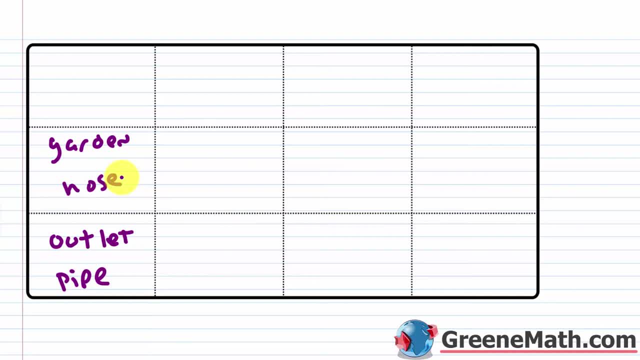 that's what it says in the problem. Now, again, we're going to have our rate of work, We're going to have our time working together And then we're going to have our total contribution. So we know one thing so far: it's the time working together is X, because we just let a variable. 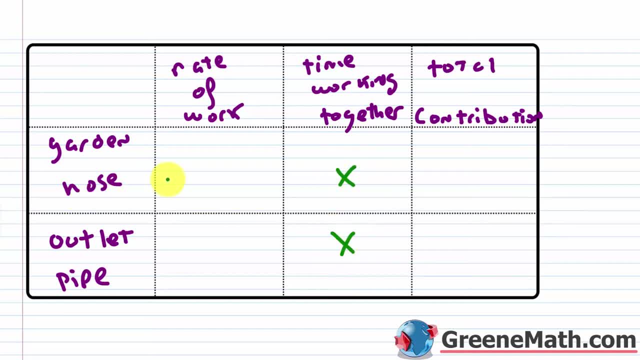 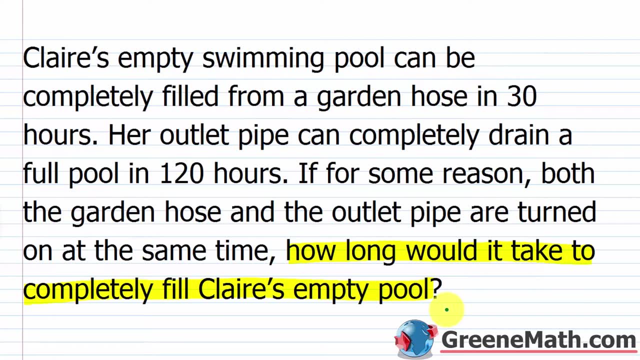 represent that. So this is X and this is X The rate of work. let's go back up. We've got to find the garden hose and the outlet pipe So the garden hose can fill the pool in 30 hours, So every hour. 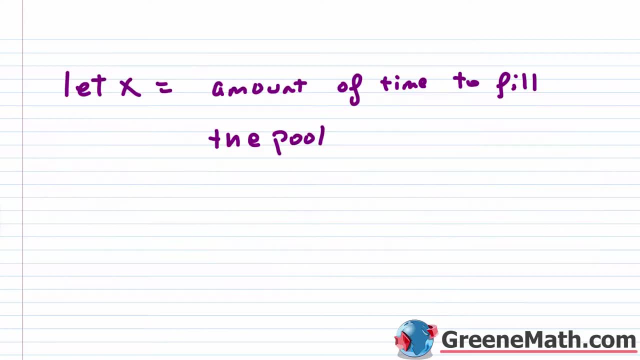 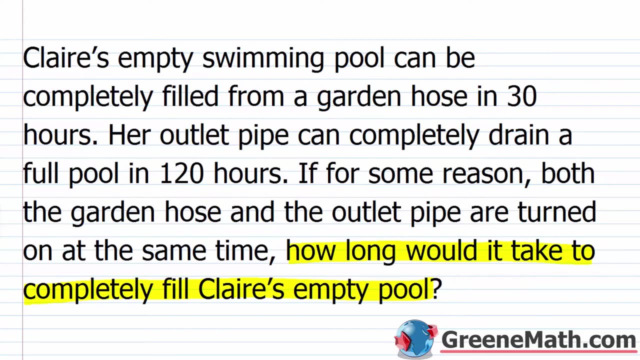 it's done one over 30 of that job, So the rate of work is one over 30. So I'll put one over 30.. Now the outlet pipe which is trying to drain the pool. that's its goal, Okay, So. 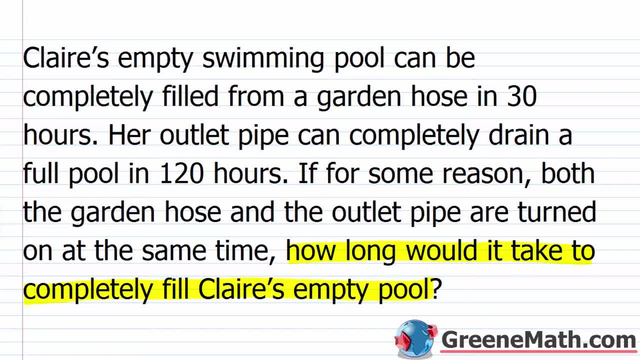 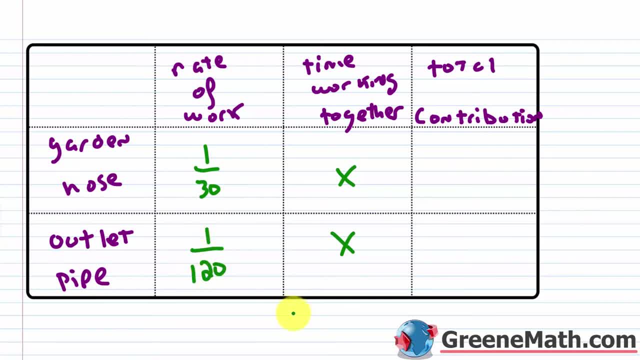 every hour. since it takes 120 hours to do this, it's done one over 120 of that, So I'll put one over 120.. So that's the rate of work. Now the contribution works a little bit differently here because they're competing forces, right? You can kind of think about the garden hose as filling it. 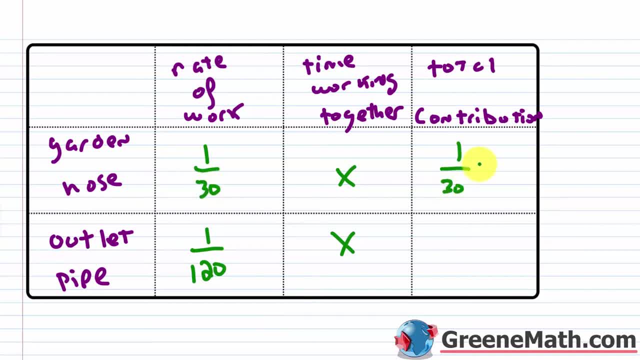 So I'm going to put a positive one over 30 times X, or you can just put X over 30.. Really, you can think about the outlet pipe as fighting against this right. You can think about what it's doing as subtracting away. So you can put this as a minus X times one over. 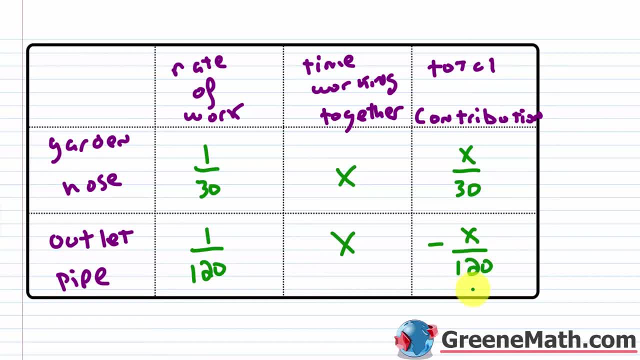 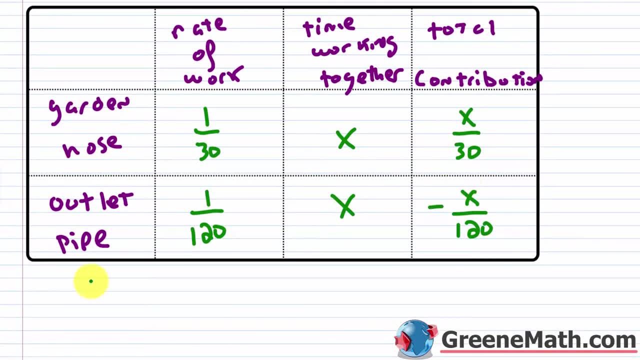 120, which would be X over 120.. So if you sum these two amounts together, you should set it equal to one and solve that equation. So I would have X over 30.. I'll just put minus, or you can put plus negative, doesn't matter, I'll put minus X over 120.. I'll set that equal. 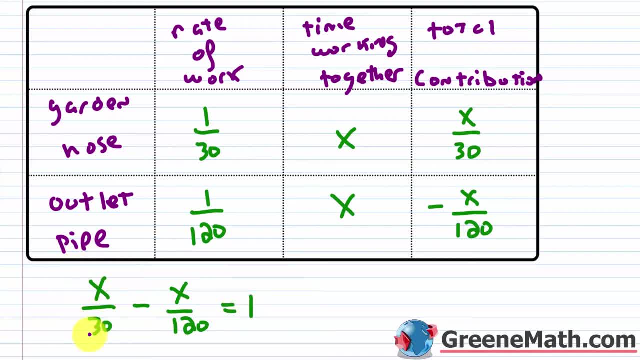 to one. So in other words, the total contribution or the total amount of water that goes in from the garden hose, minus the total contribution or the total amount of water that gets pulled out from the outlet pipe. when that's set equal to one, the value for X is going. 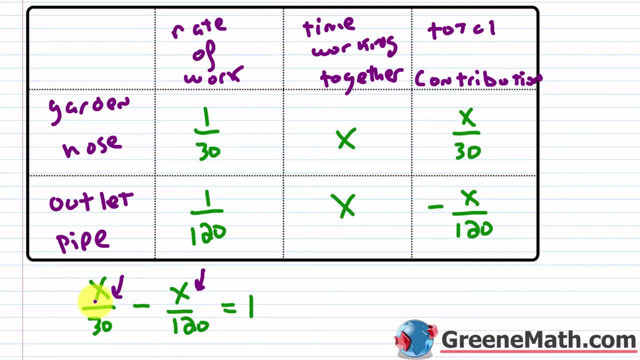 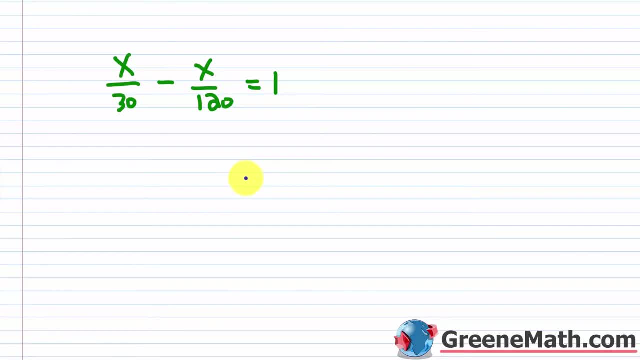 to tell me the amount of time it takes for them to complete that job again working together. So let me copy this. So what I want to do is just multiply both sides by the LCD, which is going to be 120.. Pretty easy to do, So I know that I'm going to distribute this to each. 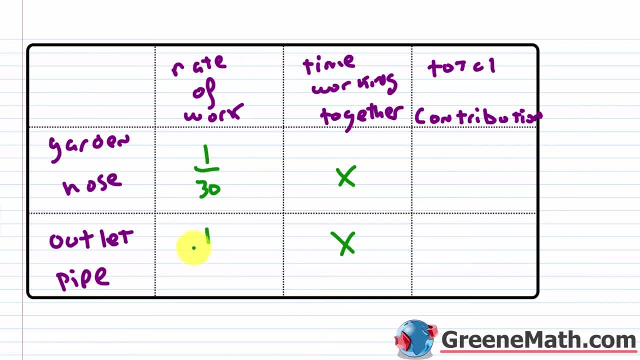 1 over 120 of that. so i'll put 1 over 120. so that's the rate of work. now the contribution works a little bit differently here because they're competing forces, right? you can kind of think about the garden hose as filling it. so i'm going to put a positive 1 over 30 times x, or you. 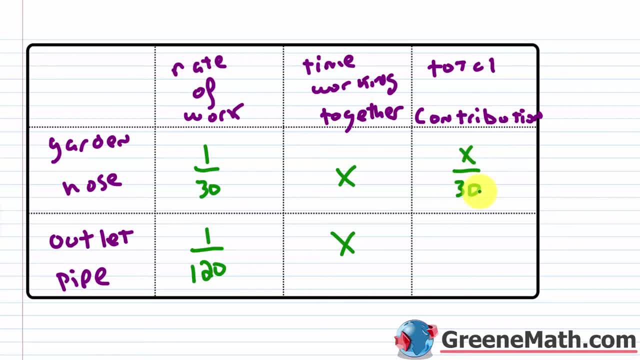 just put x over 30. really, you can think about the outlet pipe as fighting against this right. you can think about what it's doing as subtracting away. so you can put this as a minus x times 1 over 120, which would be x over 120. so if you sum these two amounts together, you should set it equal. 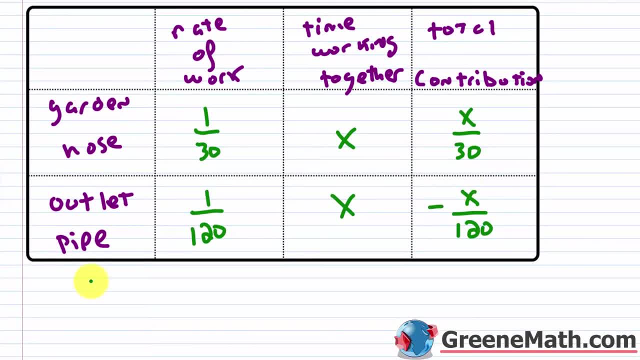 to 1 and solve that equation. so i would have x over 30. i'll just put minus, or you can put plus negative, doesn't matter, i'll put minus x over 120, i'll set that equal to 1. so, in other words, the total contribution or the total amount of water. 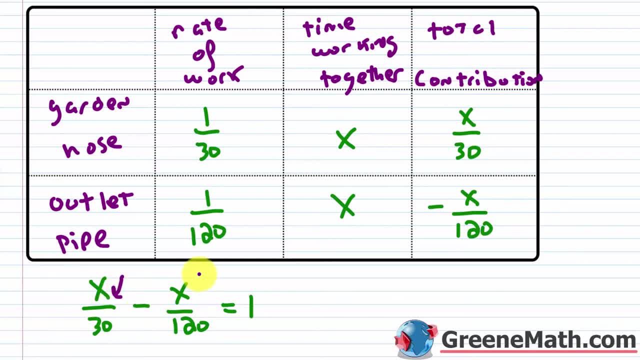 that goes in the water is the amount of water that goes in the water. so i'm going to put x over 120 from the garden hose, minus the total contribution or the total amount of water that gets pulled out from the outlet pipe. when that's set equal to 1, the value for x is going to tell me the amount. 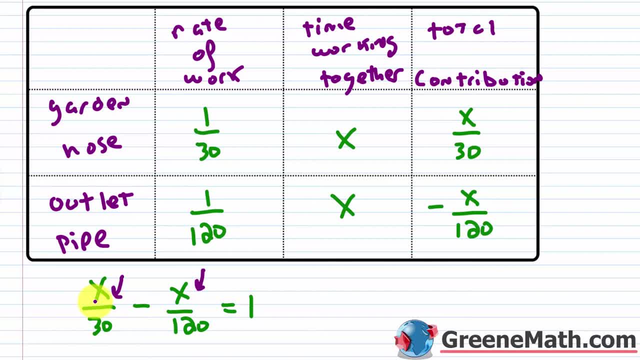 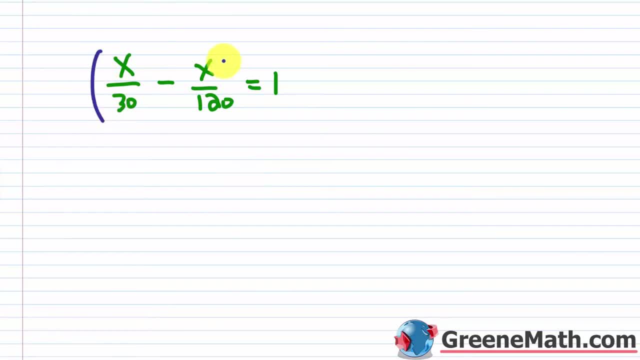 of time it takes for them to complete that job again working together. so let me copy this. so what i want to do is just multiply both sides by the lcd, which is going to be 120. pretty easy to do. so i know that i'm going to distribute this to each term, inside the parentheses: 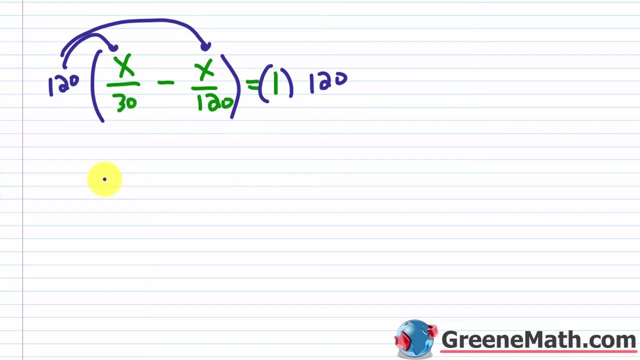 120 divided by 30 is 4, right, so i'd have 4x minus 120 divided by 120 is 1. so i just have x there. this equals 120. 4x minus x is 3x. this equals 120. divide both sides of the equation by 3. 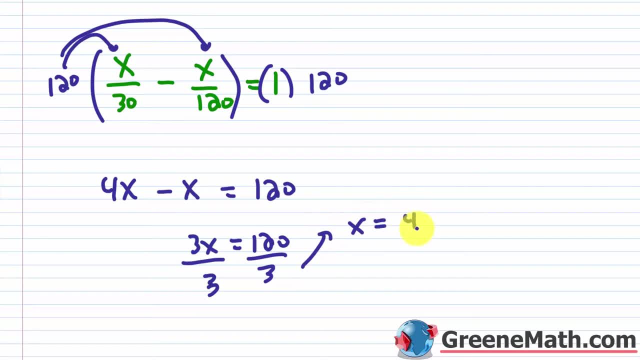 and you're going to find that x is equal to 40. so that tells us what. it tells us that the garden hose and the outlet pipe can both be left on and the pool is going to go from completely empty to completely full in 40 hours. let's go back up, so it would take. 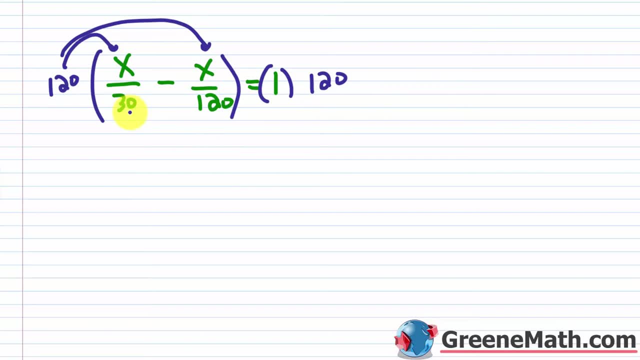 term inside the parentheses. 120 divided by 30 is four, right, So I'd have 4X minus 120 divided by 120 is one, So I just have X there. This equals 120.. 4X minus X is 3X. This equals 120.. Divide both sides of the equation by: 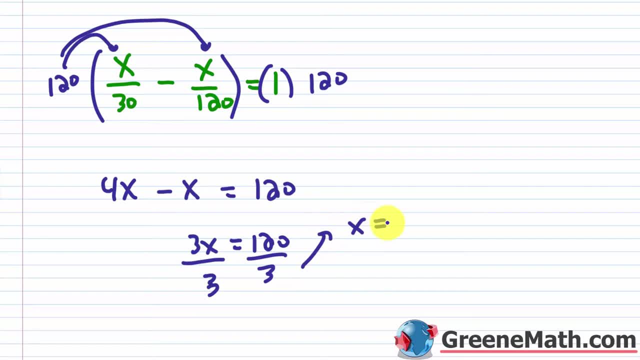 three, and you're going to find that X is equal to 40. So that tells us what. It tells us that the garden hose and the outlet pipe can both be left on and the pool is going to go from completely empty to completely full. 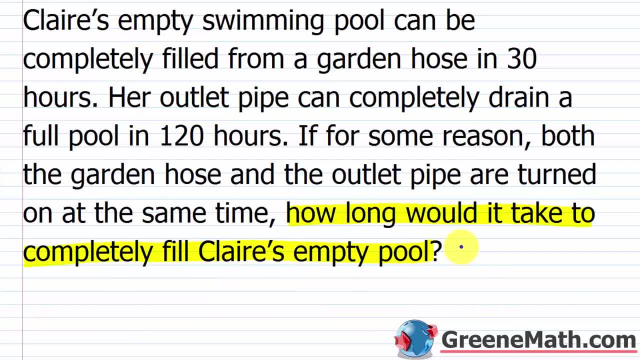 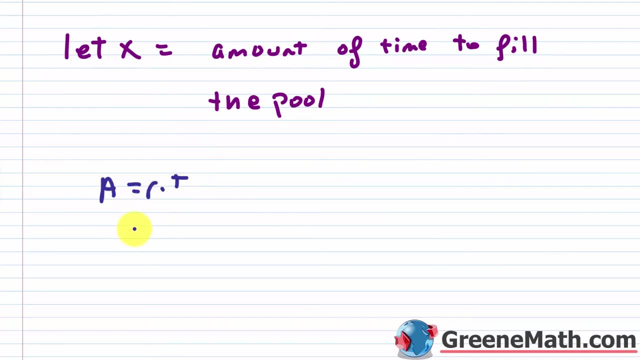 In 40 hours. Let's go back up. So it would take 40 hours to fill the pool. Okay, So let's check this. So again I go back to my formula of A equals R times T. So think about this. for each scenario, You have another one over here, So what? 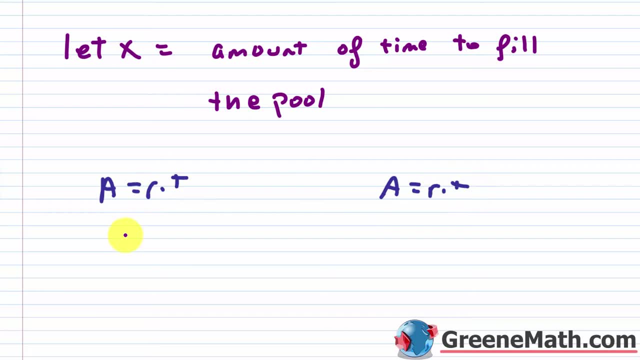 I'm going to do is I'm going to say the garden hose, how much water does it put in? So we think about the rate Again. it does a full job in 30 hours, So the rate is one over 30. When they work together, again, they're going to work for 40. 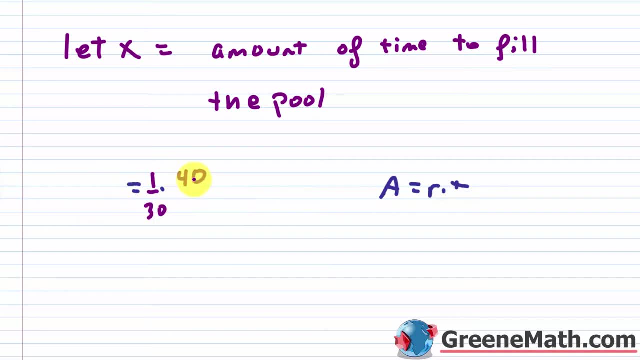 hours. So the amount that's going to be done is what I can divide both of these by 10.. This will be three and this will be four, So it's going to be four thirds. that's going to be completed So. 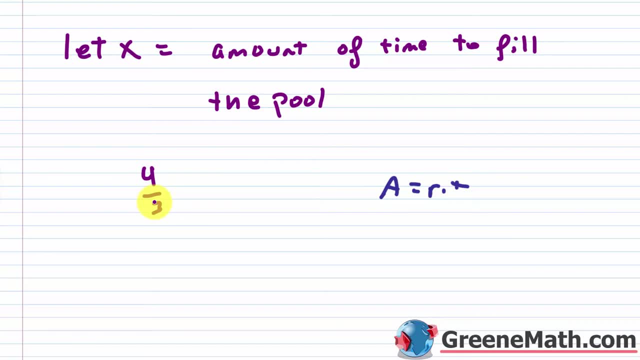 four thirds of the job is completed. Now I'm subtracting away what gets completed, but the outlet pipe what's going to get drained away here. So the rate there again it accomplishes the whole thing: 120 hours, So it's one over 120.. 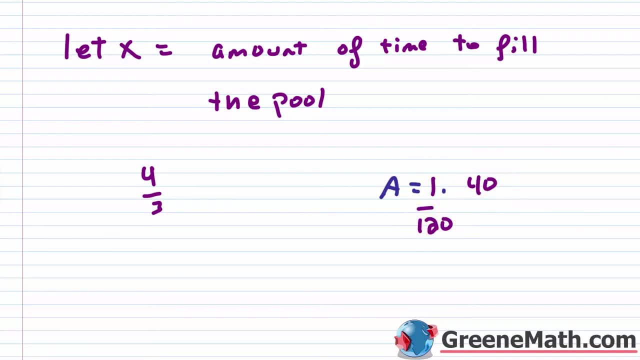 And then the time again it's going to go for 40 hours. So 120 divided by 40 is three. So this would be a three and this would be a one. So basically this is one third. So does this make? 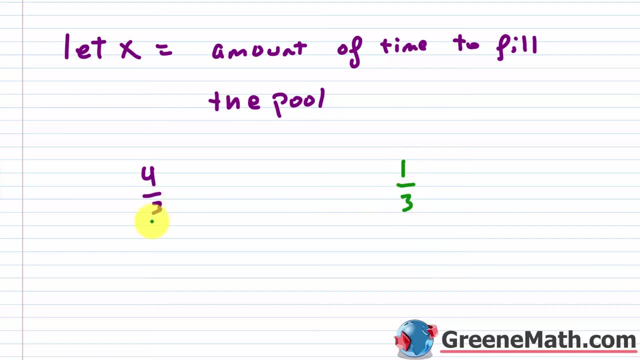 sense? Yes, it does. If the garden hose completes four thirds of the job in 40 hours and the outlet pipe completes one third of the job in 40 hours, well, four thirds minus one third gives me three thirds or one again. what's happening here is the garden hose is filling a pool and then another. 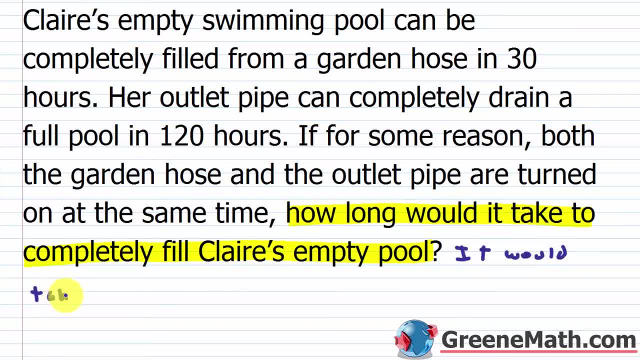 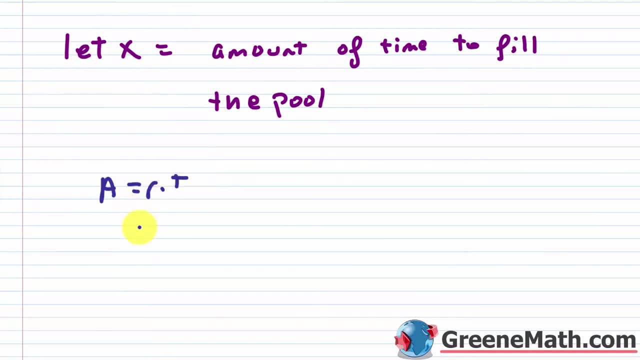 40 hours to fill the pool, okay, so let's check this. so again, i go back to my formula of a equals r times t. so think about this. for each scenario you have another one over here. so what i'm going to do is i'm going to say the garden hose. 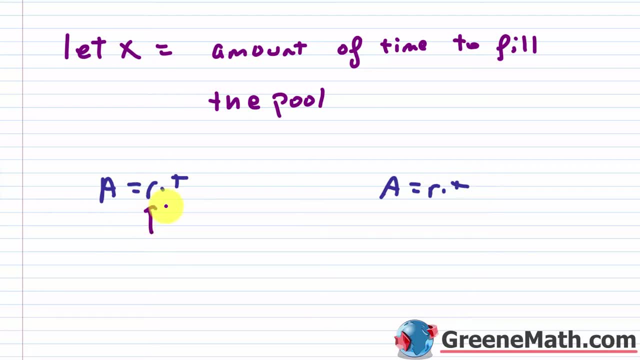 is required in order to cause a full flavor to your garden window- i'm going to say sorry- but also in order to alight the kokara in the garden window. so you have toimt out the villas that are associated with the garden. perfect, if anything. i'm going to sad, mmm. 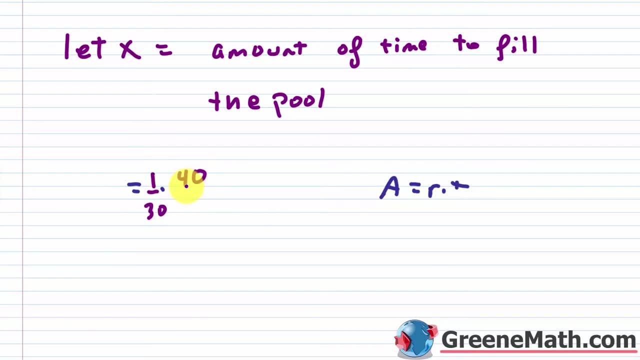 it's thegueether, and so now i'm going to say here this standard written bag. so we'll say that this is this culé台, And i'm going to convert that in a果 and see if we get a culé in the middle of these. easier about it. how much water does it put in? so we think about the rate again. it days a full job and 30 hours, so the rate is 1 over 30 when they worked together. again, if they're going to works for 40 hours, so the amount that's going to be done is WHAT. 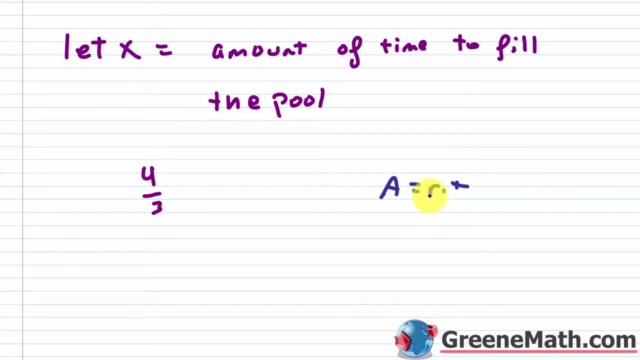 by the outlet pipe, what's going to get drained away here. so the rate there again it accomplishes the whole thing: 120 hours, so it's 1 over 120, and then the time again it's going to go for 40 hours. so 120 divided by 40 is 3. so this would be a 3 and this would be a 1. so basically, this is one third. 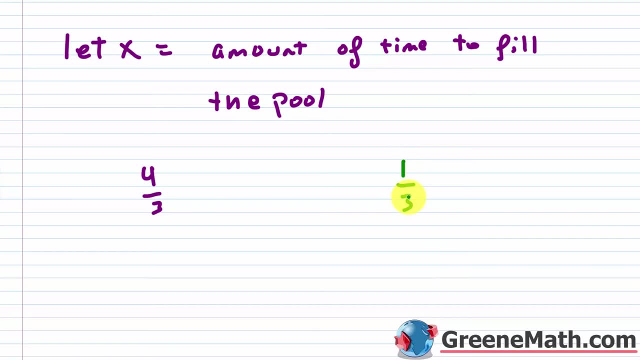 so does this make sense? yes, it does. if the garden hose completes four thirds of the job in 40 hours and the outlet pipe completes one third of the job in 40 hours, well, four thirds minus one third gives me three thirds, or one again. what's happening here is the garden hose is 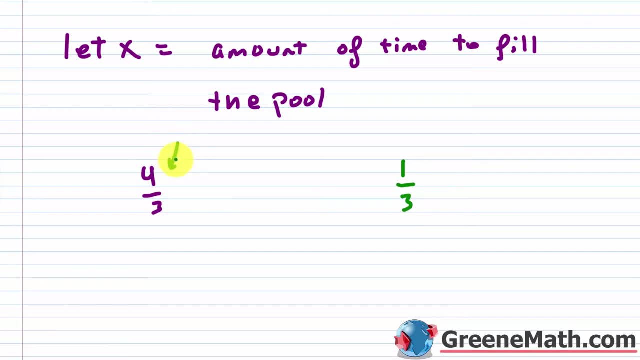 filling a pool and then another third of a pool. okay, so four thirds. then the outlet pipe is taking a third away. right, it's taking that extra third away, so you're left with three thirds or just one full pool. okay, so we can say our answer here is correct. 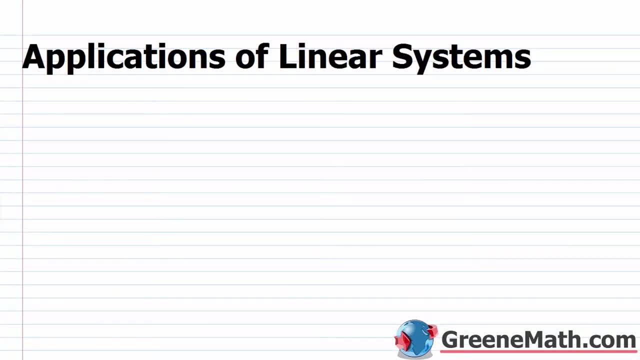 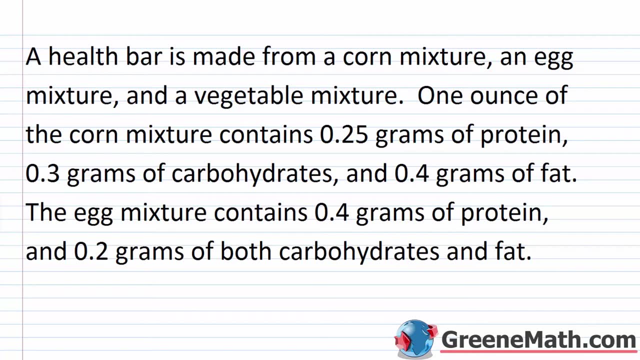 it would take 40 hours to fill the pool. in this lesson we want to review applications of linear systems. all right, so over the course of the last few lessons we've kind of talked about systems of linear equations in two and three variables. now we're just going to look at some. 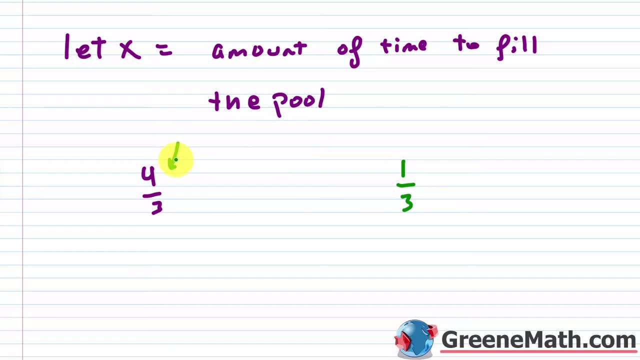 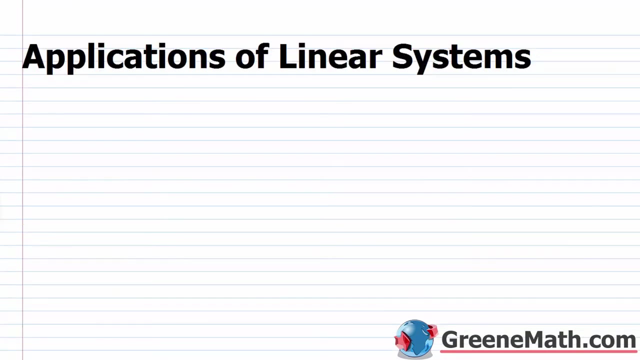 third of a pool. okay, so four thirds. then the outlet pipe is taking a third away. right, it's taking that extra third away. so you're left with three thirds or just one full pool. okay, so we can say our answer here is correct: it would take 40 hours to fill the pool. in this lesson we want to 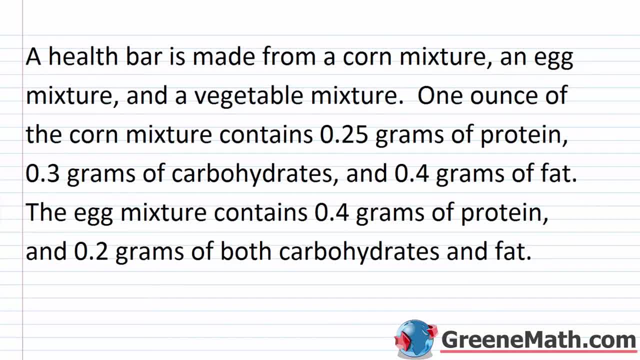 review: applications of linear systems. all right, so over the course of the last few lessons we've kind of talked about systems of linear equations in two and three variables. now we're just going to look at some kind of application problems or some word problems that come up in the section. 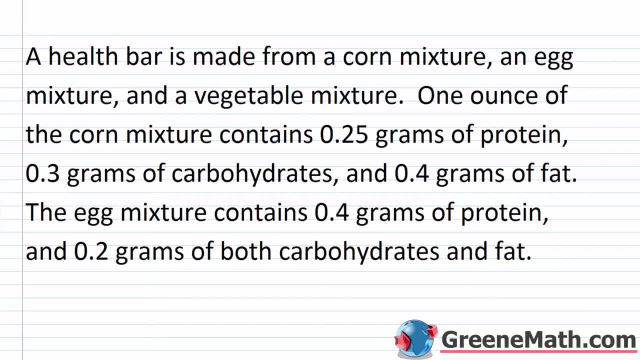 and then from here we're just going to be dealing with kind of matrices, all right. so let's start out with the first problem. so we have that- a health bar. you're going to want to make sure that you've got a health bar and you're going to want to. 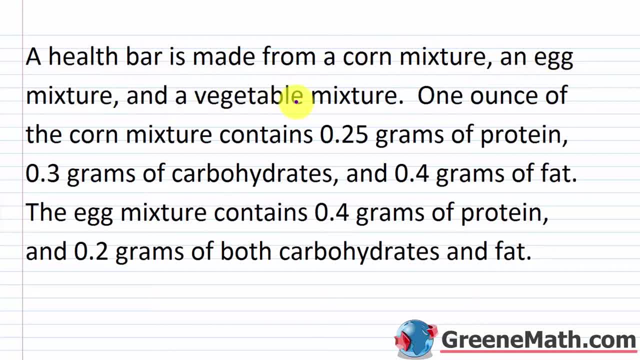 is made from a corn mixture, an egg mixture and a vegetable mixture. One ounce of the corn mixture contains 0.25 grams of protein, 0.3 grams of carbohydrates and 0.4 grams of fat. The egg mixture contains 0.4 grams of protein. 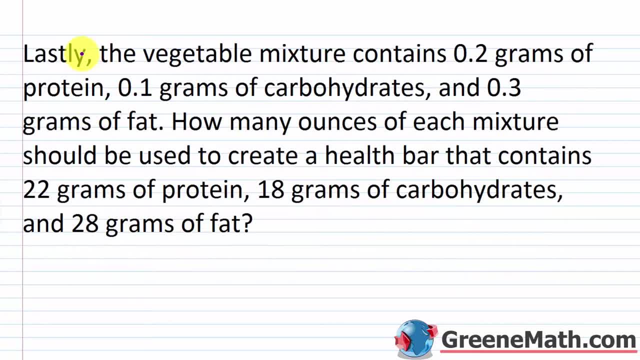 and 0.2 grams of both carbohydrates and fat. Lastly, the vegetable mixture contains 0.2 grams of protein, 0.1 grams of carbohydrates and 0.3 grams of fat. How many ounces of each mixture should be used? 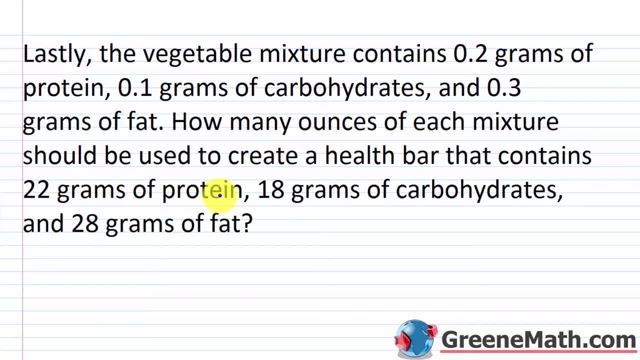 to create a health bar that contains 22 grams of protein, 18 grams of carbohydrates and 28 grams of fat. So, just like any other word problem that we've kind of worked on before, the very first thing you always wanna do is figure out: what are you being asked to find? 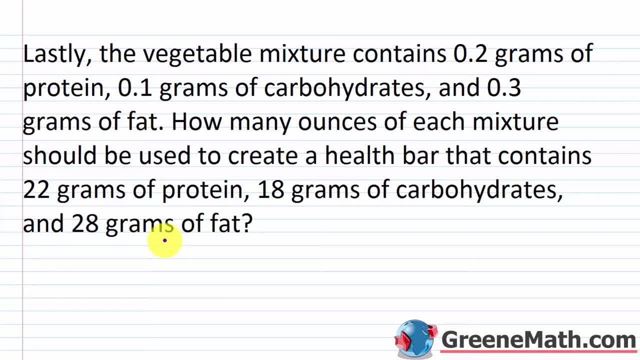 A lot of times you'll struggle because you're kind of flopping around through information. you're not specific on what you need to find. So you need to key in on that and you need to say: okay, I wanna find how many ounces. 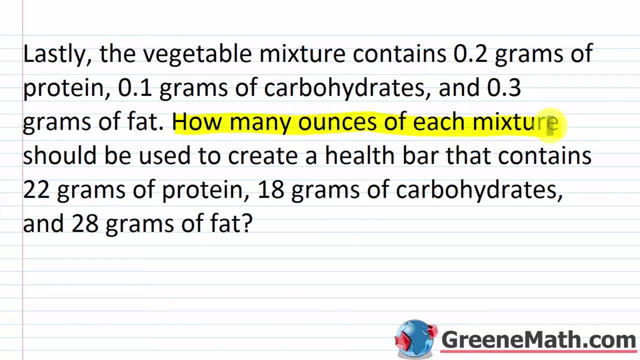 of each mixture- okay, So remember, we had the corn mixture, the egg mixture and the vegetable mixture- and should be used to create a health bar that contains 22 grams of protein, 18 grams of carbohydrates and 28 grams of fat. okay, 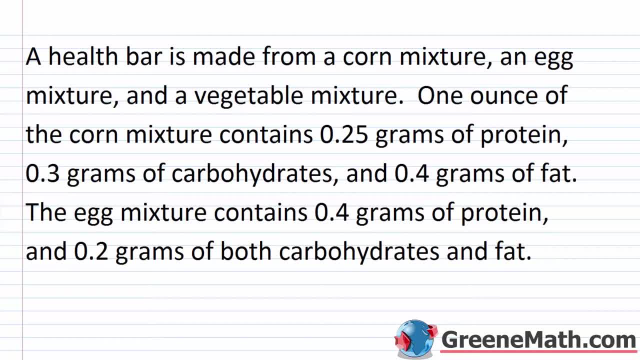 kind of application problems or some word problems that come up in the section and then from here we're just going to be dealing with kind of matrices. all right, so let's start out with the first problem. so we have that a health bar is made from a corn. 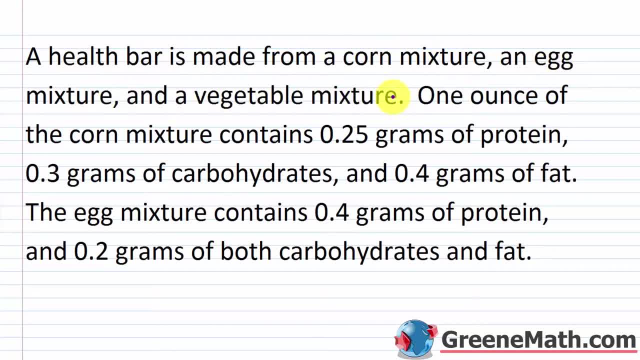 mixture, an egg mixture and a vegetable mixture. one ounce of the corn mixture contains 0.25 grams of protein, 0.3 grams of carbohydrates and 0.4 grams of fat. the egg mixture contains 0.4 grams of protein and 0.2 grams of both carbohydrates and fat. lastly, the vegetable mixture contains: 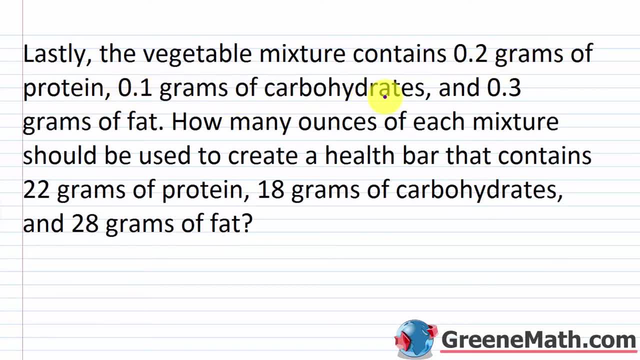 0.2 grams of protein, 0.1 grams of carbohydrates and 0.3 grams of fat. how many ounces of each mixture should be in a vegetable mixture and how many ounces of each vegetable mixture should be should be used to create a health bar that contains 22 grams of protein, 18 grams of. 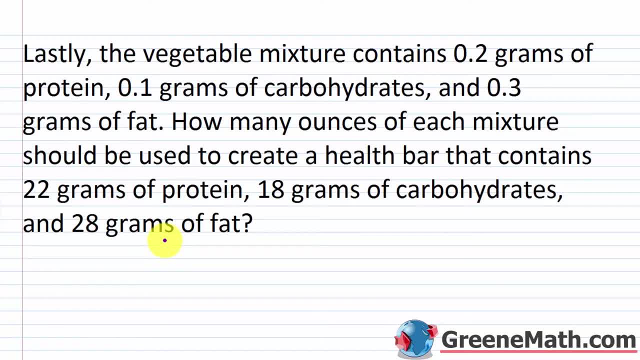 carbohydrates and 28 grams of fat. So, just like any other word problem that we've kind of worked on before, the very first thing you always want to do is figure out: what are you being asked to find. A lot of times you'll struggle because you're kind of flopping around through information. 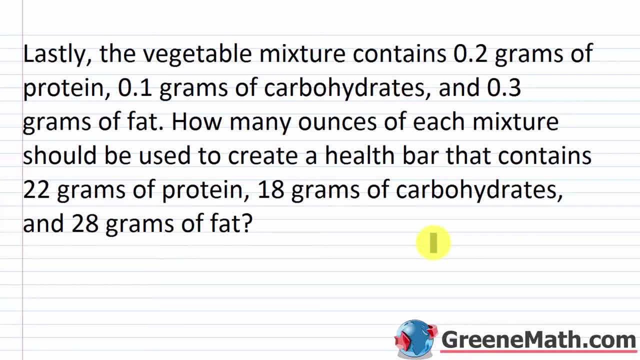 you're not specific on what you need to find, So you need to key in on that and you need to say: I want to find how many ounces of each mixture. so remember we had the corn mixture, the egg mixture and the vegetable mixture and should be used to create a health bar. that. 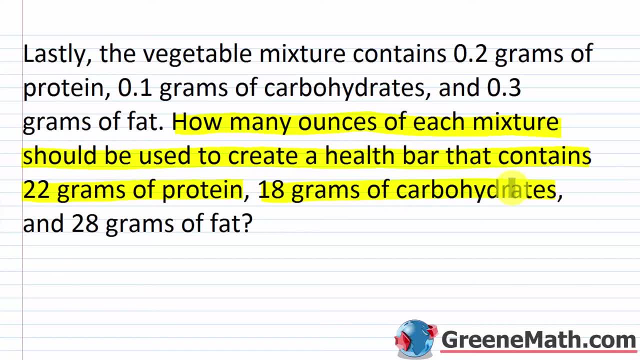 contains 22 grams of protein, 18 grams of carbohydrates and 28 grams of fat. So we have three unknowns. We need to know again how many ounces of the corn mixture we're going to use, how many ounces of the egg mixture we're going to use and how many ounces of the 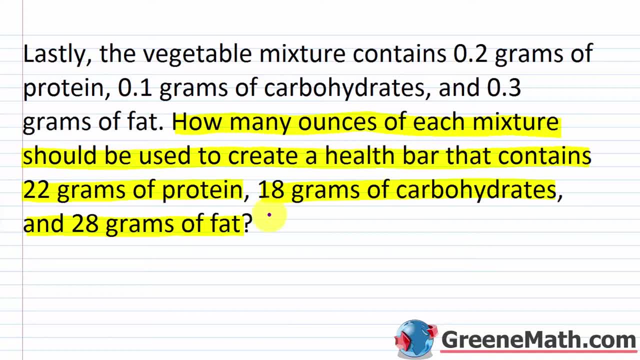 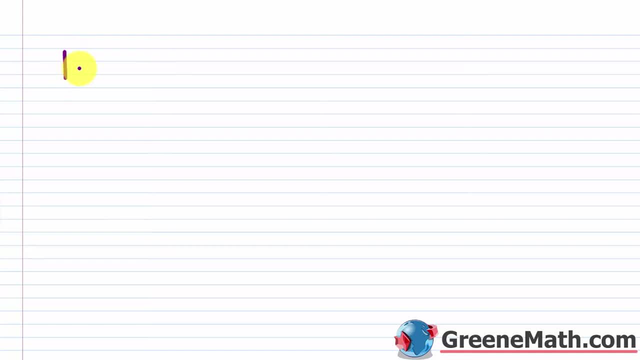 vegetable mixture we're going to use to kind of create this health bar with these specifications. So let's go ahead and label these three as x, y and z. So let's let x be equal to the amount in ounces for the corn mixture, and then we'll say y can be equal to the amount in ounces for the. 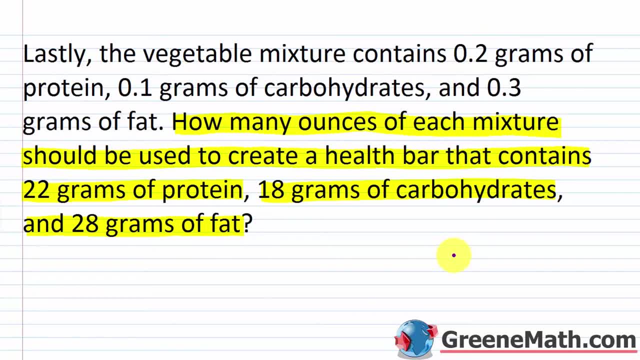 So we have three unknowns right. We need to know again how many ounces of the corn mixture we're gonna use, how many ounces of the egg mixture we're gonna use and how many ounces of the vegetable mixture we're gonna use to kind of create this health bar. 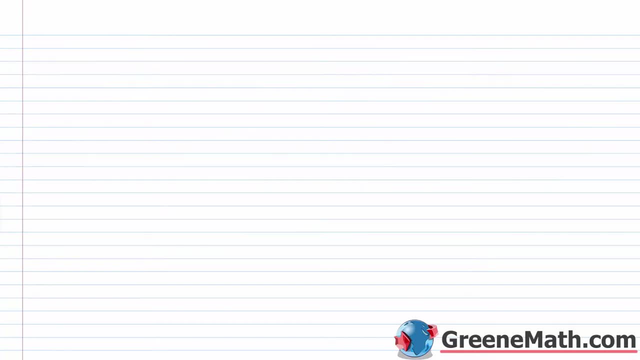 with these specifications. So Let's go ahead and label these three as X, Y and Z. So let's let X be equal to the amount in ounces for the corn mixture, And then we'll say Y can be equal to the amount in ounces. 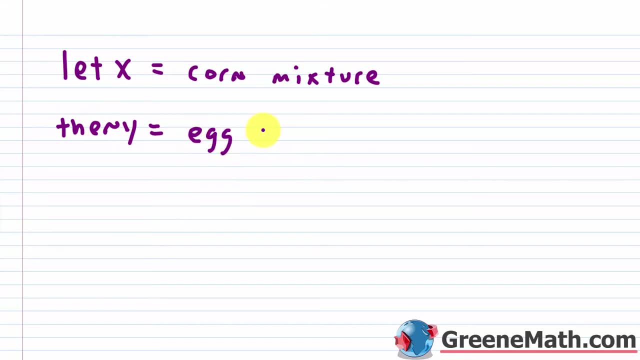 for the egg mixture. And just to keep this short, I'm just gonna leave mixture off And then we'll also say: then for Z, we're gonna say the amount in ounces for the vegetable mixture. So I'm just gonna put V-E-G to kind of abbreviate that. 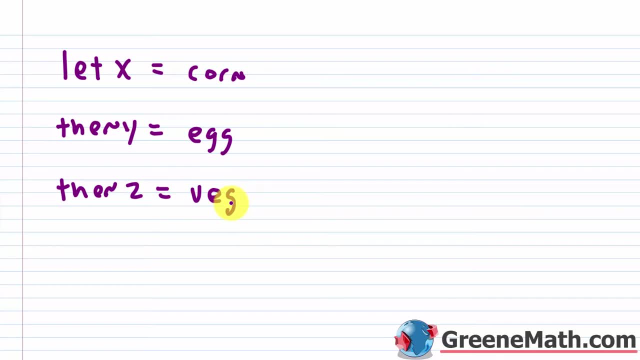 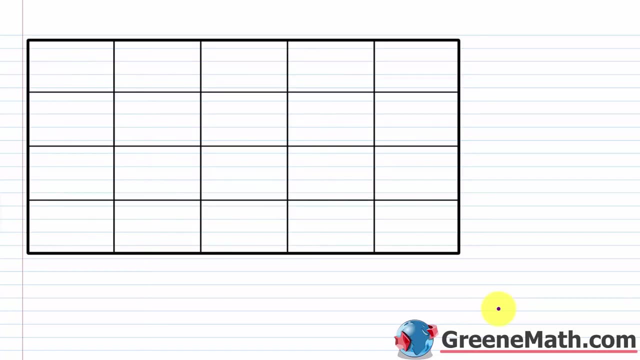 Okay, So the best way to kind of look at this type of problem is with a table. You don't need one, but it definitely helps. So I've already kind of pre-drawn one for us, So I'm gonna show you how you can fill out. 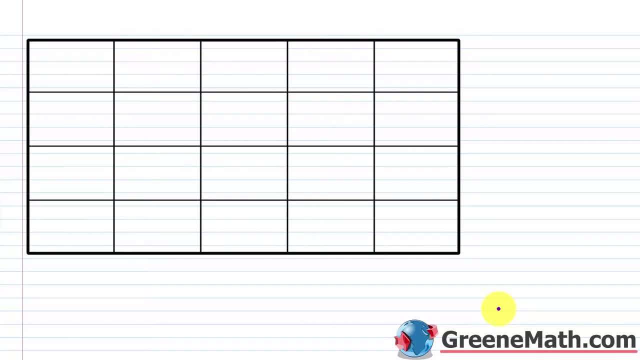 the information here and then get some equations going and get a solution. So the first thing is let's talk about the different kind of mixtures you have. You have the corn mixture, you have the egg mixture and you have the vegetable mixture. 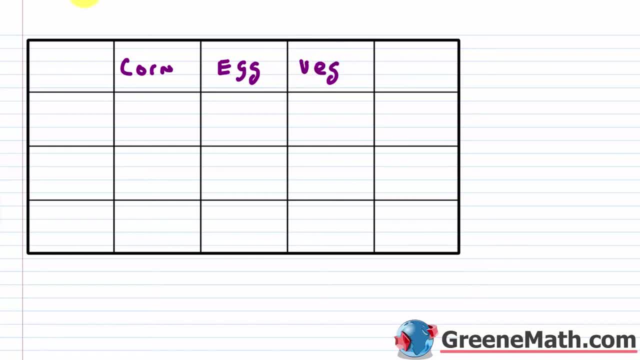 Okay, which I'm gonna abbreviate V-E-G. Then we're given the amounts of protein, carbohydrates and fat. So I'm just gonna put protein just P-R-O, carbohydrates C-A-R, and then for fat just F-A-T. 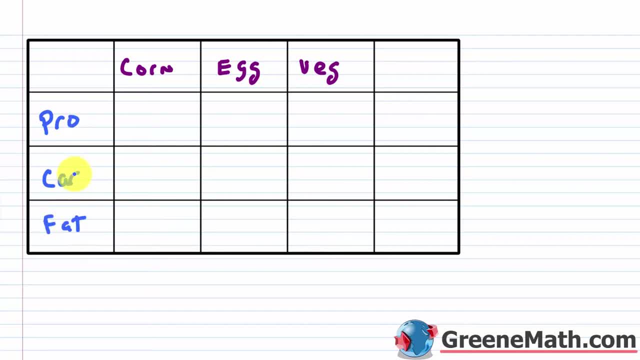 Of course that spells fat, but for the other ones they're abbreviated. Okay, then we also wanna put in a total here, and this will make sense once we kinda have the information going. So what I can do is I can look up back in the problem. 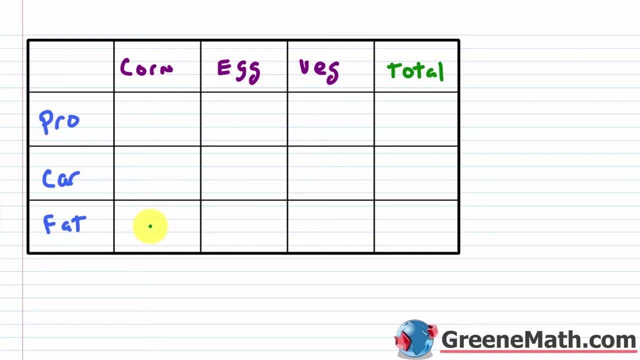 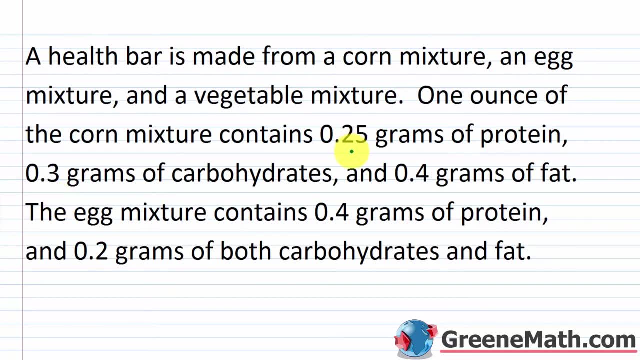 the statistics for how much protein, carbohydrate and fat each one of these guys have. I'm just gonna fill in my table, So let's go back up. So for the corn, for every ounce it's got 0.25 grams of protein. 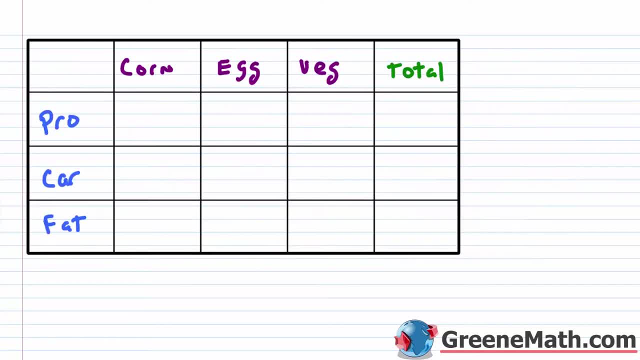 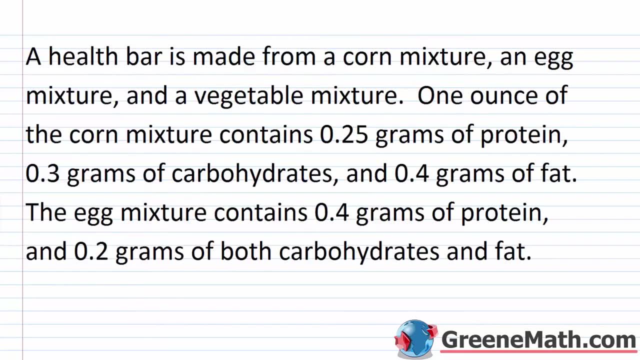 0.3 grams of carbohydrates, 0.4 grams of fat. So we've got 0.25 for protein, 0.3 for carbs and 0.4 for fat. All right, for the egg mixture we have 0.4 grams of protein. 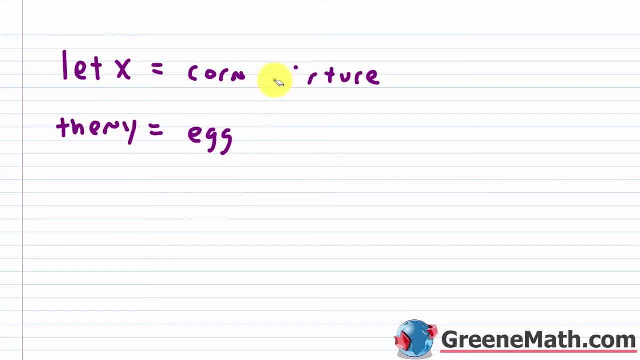 egg mixture. And just to keep this short, I'm just going to leave mixture off and then we'll also say: then for z, we're going to say the amount in ounces for the vegetable mixture. So I'm just going to put veg to kind of abbreviate that. Okay, so the best way to kind of look at this type of problem, 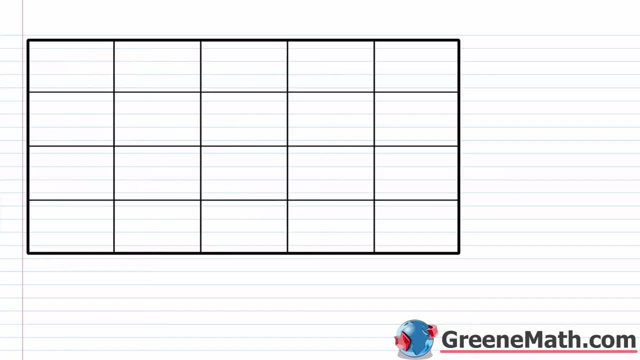 is with a table. You don't need one, but it definitely helps. So I've already kind of pre-drawn one for us. So I'm going to show you how you can fill out the information here and then get some equations going and get a solution. So the first thing is let's talk. 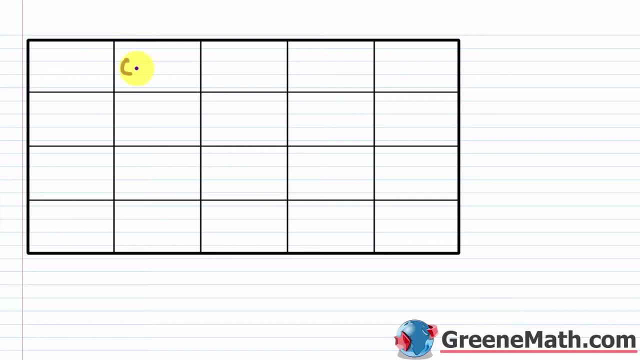 about the different kind of mixtures you have. You have the corn mixture, you have the egg, you have the egg mixture and you have the vegetable mixture- okay- which I'm going to abbreviate veg. Then we're given the amounts of protein, carbohydrates and fat, So I'm just going 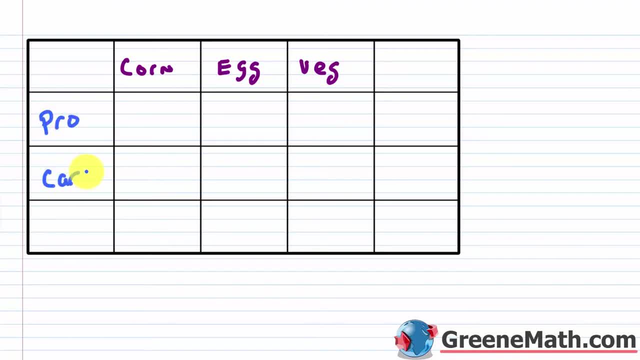 to put protein just pro carbohydrates car, and then for fat, just fat. Of course that spells fat, but for the other ones they're abbreviated. Okay, then we also want to put in a total here, and this will make sense once we kind of have the information going. So what I can do is I can look. 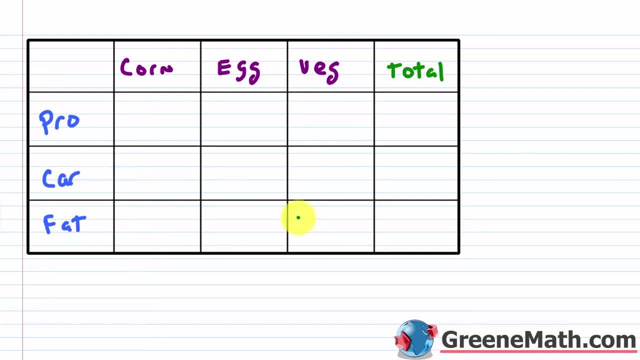 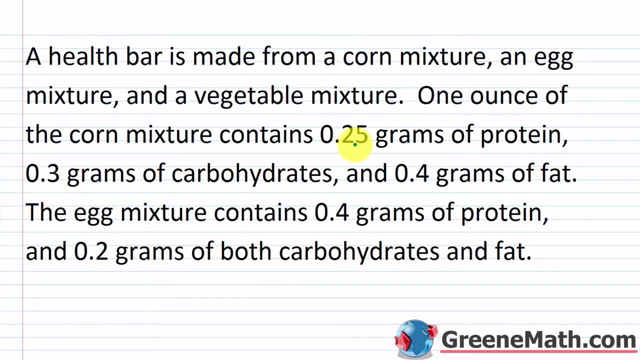 for how much protein, carbohydrates and fat each one of these guys have. I'm just going to fill in my table, So let's go back up. So for the corn, for every ounce it's got 0.25 grams of protein. 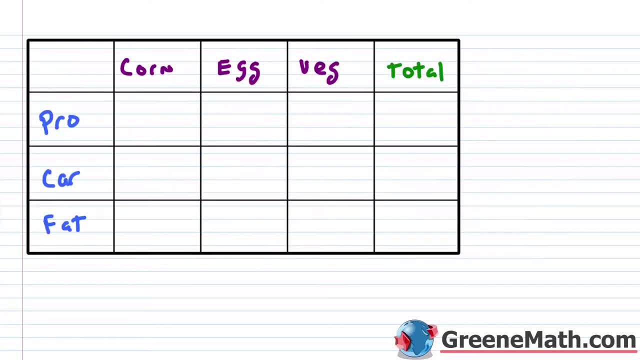 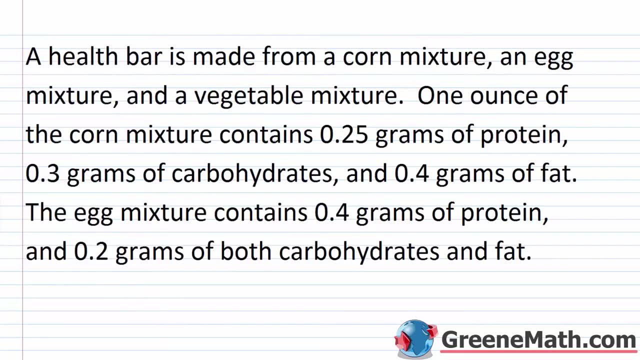 0.3 grams of carbohydrates, 0.4 grams of fat. So we've got 0.25 for protein, 0.3 for carbs and 0.4 for fat. All right, for the egg mixture we have 0.4 grams of protein and then 0.2 grams. 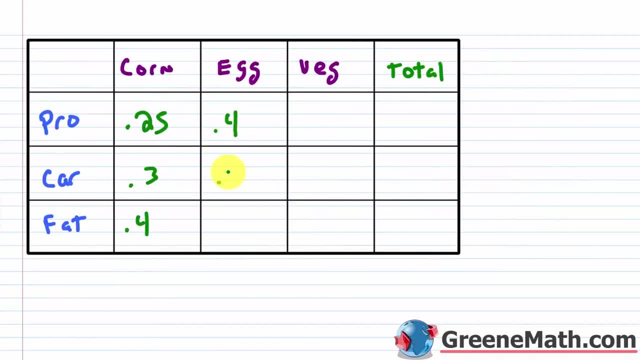 for both carbohydrates and fat. So we've got 0.4 and then 0.4 grams of protein. So we've got 0.4 and then 0.2 and then 0.2 again. Then, lastly, for our vegetable mixture, we've got 0.2 grams of. 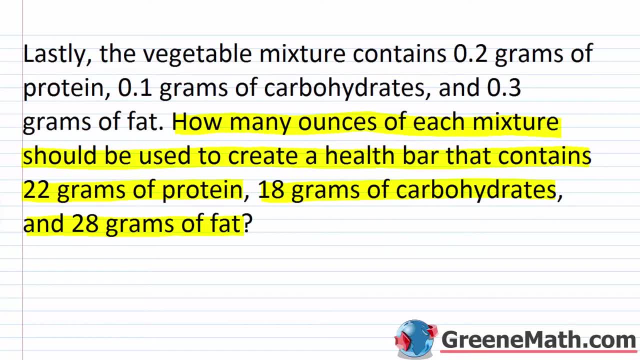 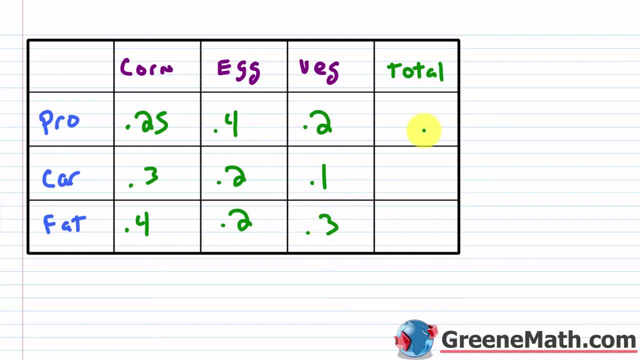 protein, 0.1 grams of carbohydrates and 0.3 grams of fat. So we've got 0.2 for the protein, 0.1 for the carbohydrates and 0.3 for the fat. Now I have a column here for the total. 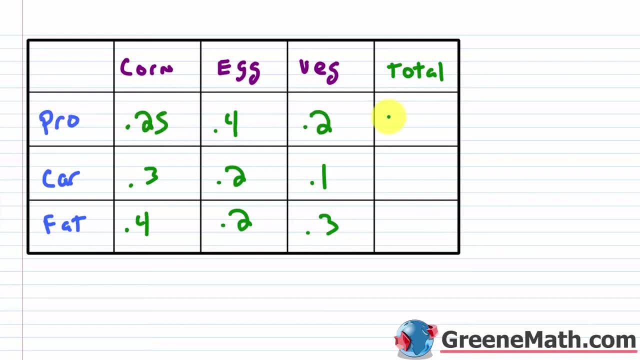 and what I'm going to do here. notice how, going across, it's all protein. right, It's the protein for the corn, the eggs and the vegetable. We want to know what the protein total is going to be from these three sources. 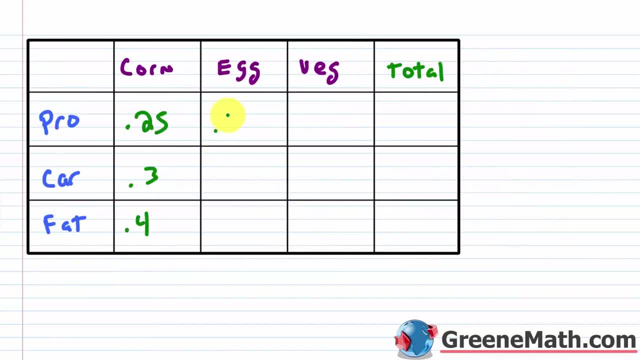 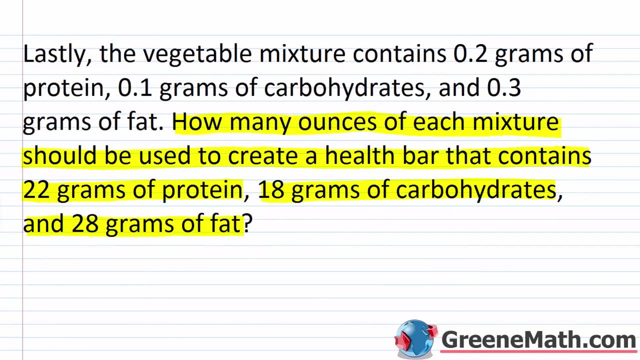 and then 0.2 grams, for both carbohydrates and fat. So we've got 0.4, and then 0.2, and then 0.2 again. Then, lastly, for our vegetable mixture, we've got 0.2 grams of protein. 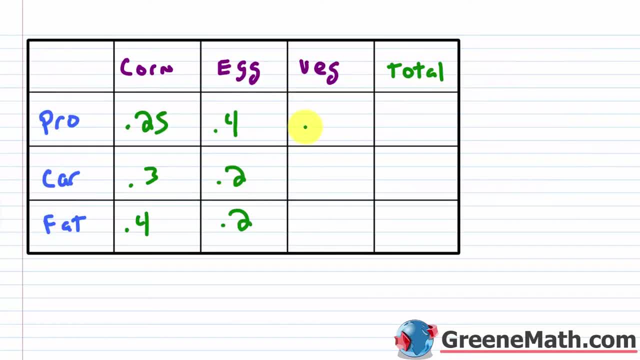 0.1 grams of carbohydrates and 0.3 grams of fat. So we've got 0.2 for the protein, 0.1 for the carbohydrates and 0.3 for the fat. Now I have a column here for the total. 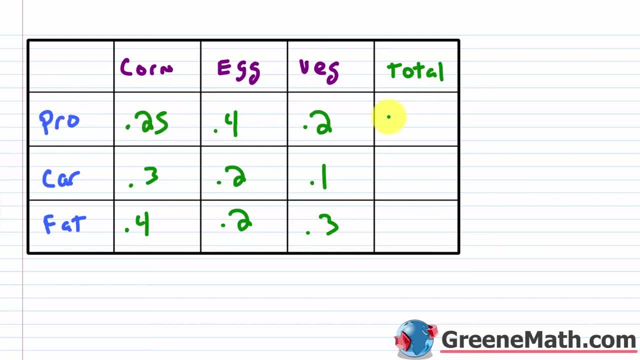 and what I'm gonna do here. notice how, going across, it's all protein. right, It's the protein for the corn, the eggs and the vegetable. We wanna know what the protein total's going to be from these three sources. 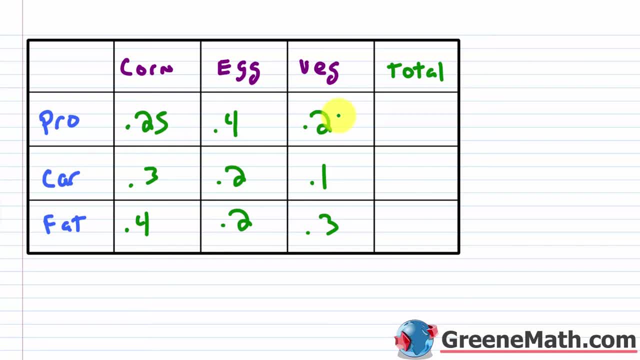 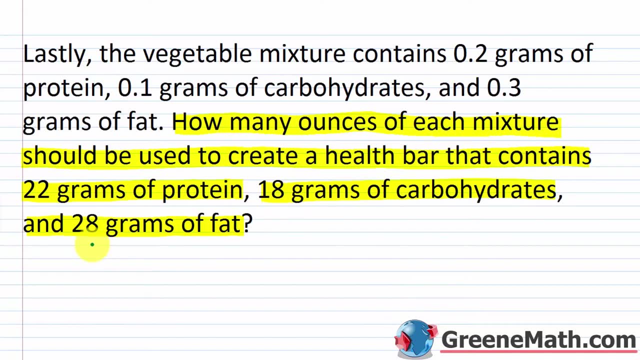 and again, it's based on the requirement that's given to us when we're building this health bar. If we go back, we see that it needs to be 22 grams of protein, 18 grams of carbohydrates and 28 grams of fat. 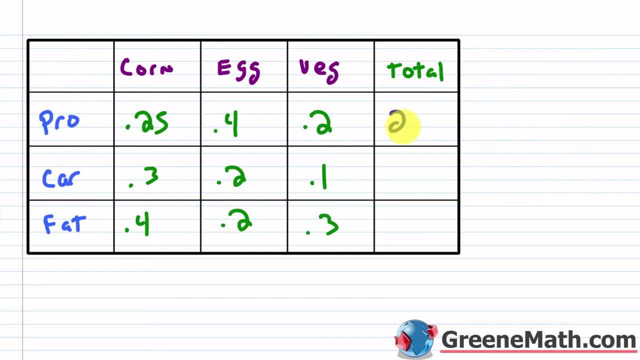 So for the total there for protein it's gonna be 22,. right, just going across. For carbohydrates going across, the total needs to be 18.. And for fat going across, the total needs to be 28,. okay. 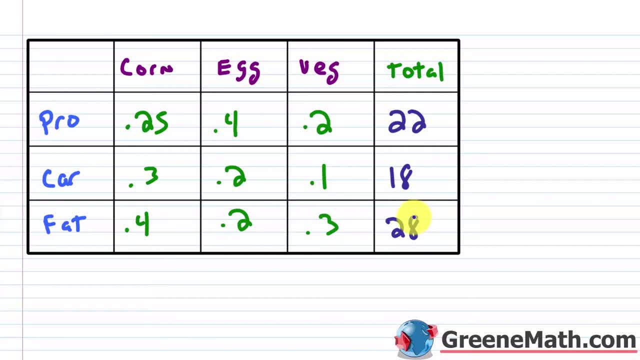 So this is how we're gonna get our equations, because what we know is that the protein's gonna have to be, you know, it's gonna have to be a certain amount of protein. okay, So this is how we're gonna get our equations, because what we know is that the protein needs to be 18.. 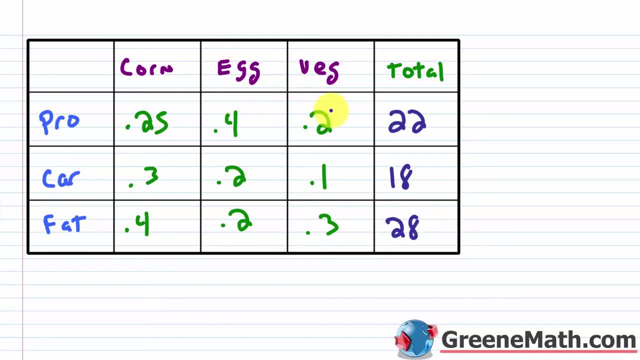 only comes from three sources. right, It comes from corn, eggs and vegetables. The number of ounces of this corn mixture I use, so that's going to be x times this kind of 0.25, which is the number of grams- okay, of protein per one ounce. So this amount here would tell me the amount of 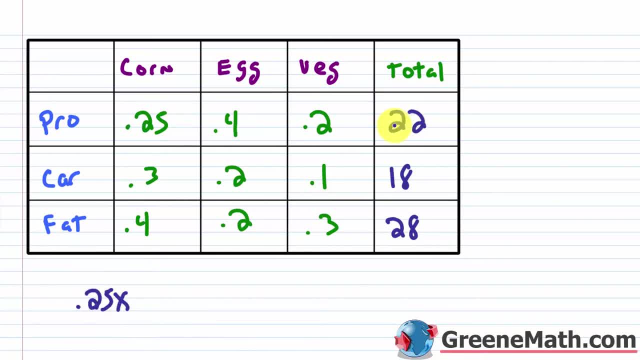 protein I'm getting from just the corn, okay, But I need to reach this amount, so I'm going to add to this the amount of protein I get from the egg, so that's 0.4 times y. okay, Then plus additionally. 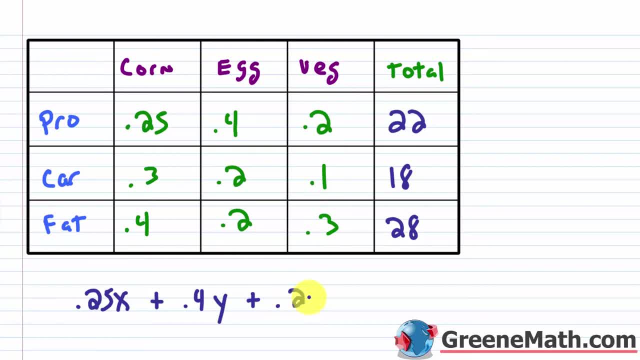 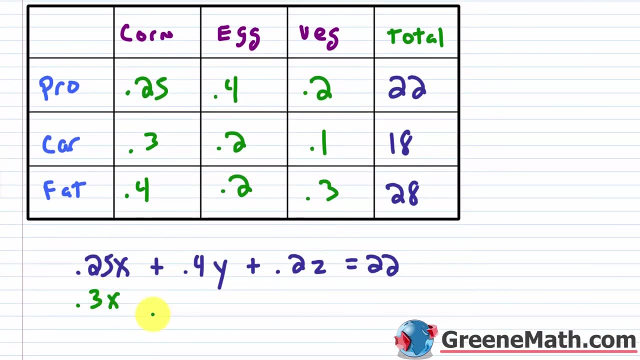 the amount of protein I'm getting from the vegetables. so 0.2 times z, This has to be equal to 22,. okay, Because that's the only place the protein's coming from. The same thing's going to happen with the carbohydrates and the fat. We can just go across. So I can say that 0.3 times x. 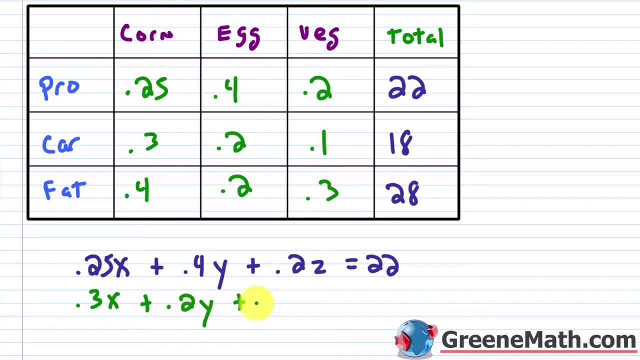 plus 0.2 times y, plus 0.1 times z is the amount of protein I get from the egg, So that's 0.4 times y. okay, Then plus additionally is equal to 18.. And I'm going to run out of space here, so let me scroll down. I'm going to cut this. 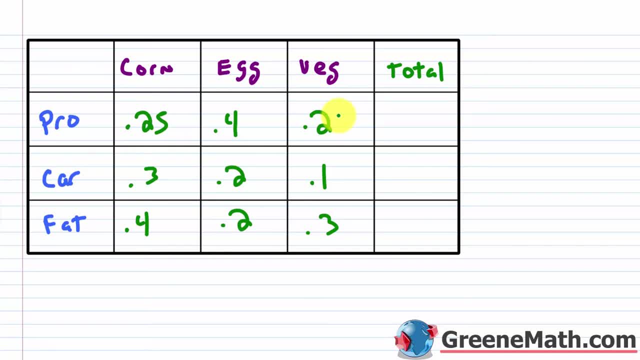 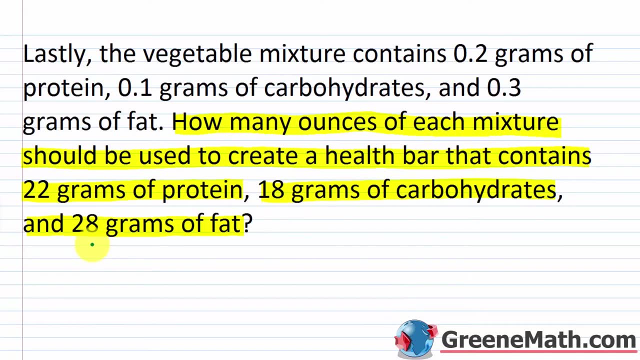 And again, it's based on the requirement that's given to us when we're building this health bar. If we go back, we see that it needs to be 22 grams of protein, 18 grams of carbohydrates and 28 grams of fat. So for the total there, for protein, it's going to be 22,. right, Just going. 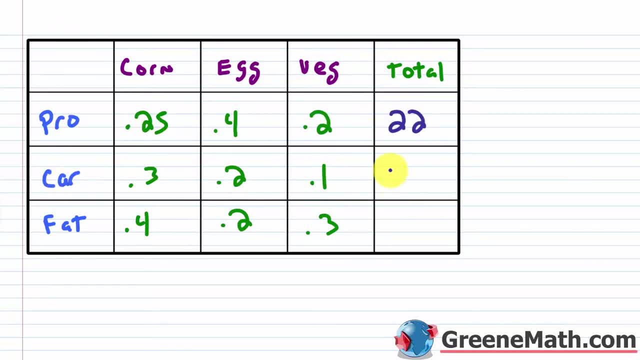 across. For carbohydrates going across, the total needs to be 18.. And for fat going across, the total needs to be 28,. okay, So this is how we're going to get our equations, because what we know is that the protein only. 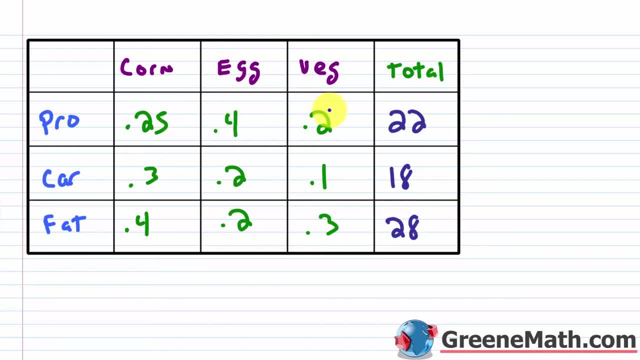 what we know is that the protein only comes from three sources. right, It comes from corn, eggs and vegetables. The number of ounces of this corn mixture I use, so that's going to be x times this kind of 0.25, which is the number of grams, okay, of protein per one ounce. So this amount. 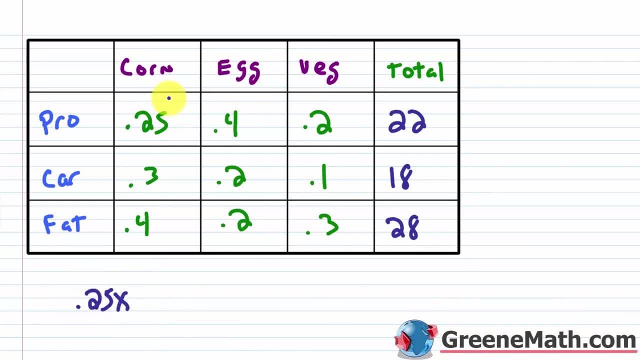 here would tell me the amount of protein I'm getting from just the corn. okay, But I need to reach this amount, so I'm going to add to this the amount of protein I get from the egg, so that's 0.4 times y okay. 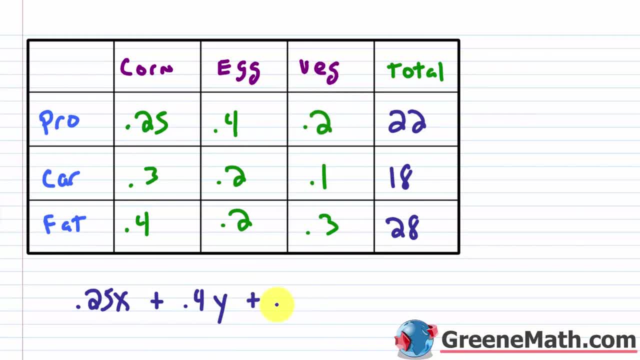 Plus, additionally, the amount of protein I'm getting from the vegetables. so 0.2 times z, This has to be equal to 22,. okay, Because that's the only place the protein's coming from. The same thing's going to happen with the carbohydrates and the fat. We can just go. 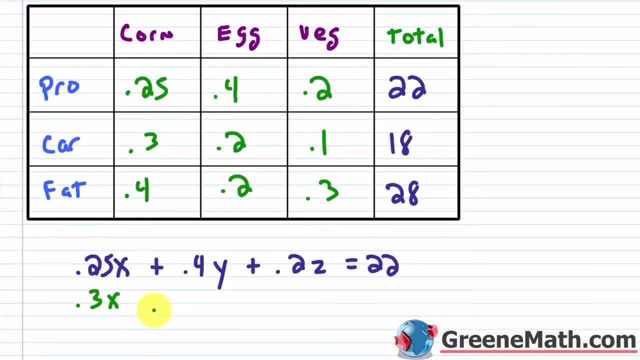 across. So I can say that 0.3 times x plus 0.2 times y plus 0.1 times z is equal to 18.. And I'm going to run out of space here, so let me scroll down. I'm going to cut this off. 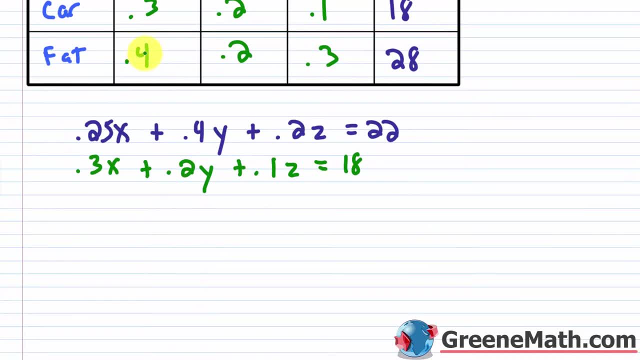 but we're going to remember that 0.3 times x plus 0.2 times y is equal to 18.. So that the kind of column here is for corn, then this guy is for egg and this guy is for vegetables. So we're just going to copy: We have 0.4x plus 0.2y plus 0.3z equals 28,. okay, So that's. 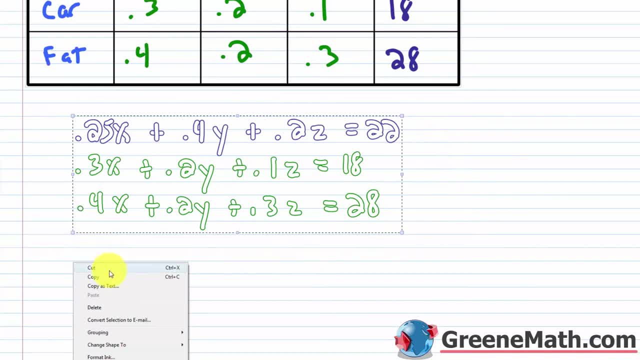 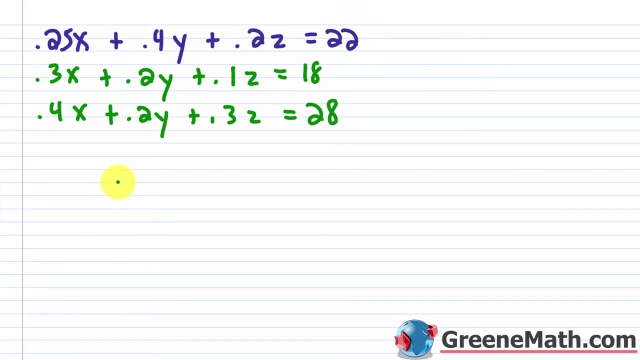 all we really need to do. So let's just cut this away from here. We're going to take a fresh sheet and let's solve this system real quick and get our solution for our problem. Now you can work with decimals if you want. If you have a calculator, it's fine. 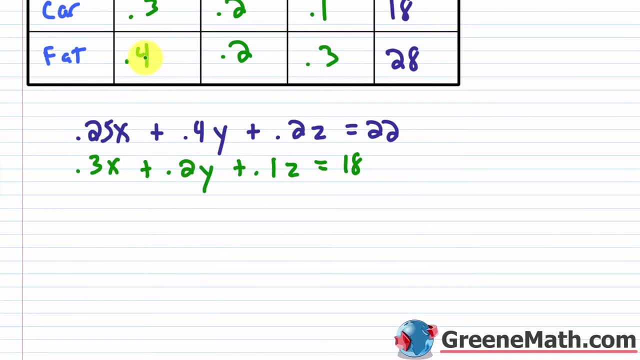 off. but we remember that the kind of column here is for corn, then this guy is for egg and this guy is for vegetables. So we're just going to copy: We have 0.4x plus 0.2y plus 0.3z equals 28,. okay. 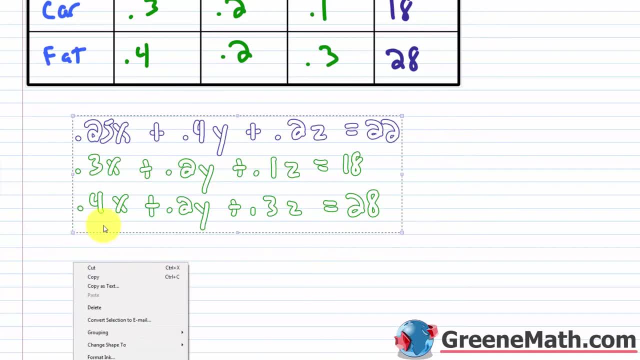 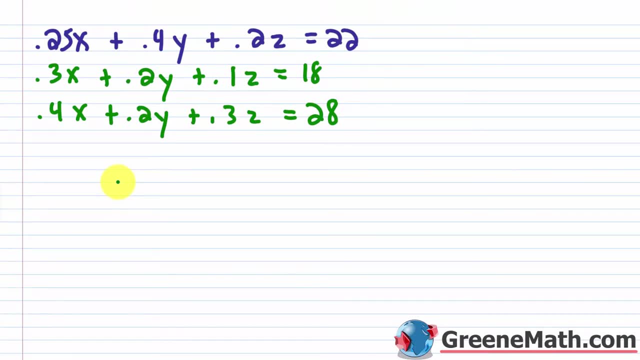 So that's all we really need to do. So let's just cut this away from here. We're going to take a sheet and let's solve this system real quick and get our solution for our problem. Now you can work with decimals if you want. If you have a calculator, it's fine. A lot of people don't like. 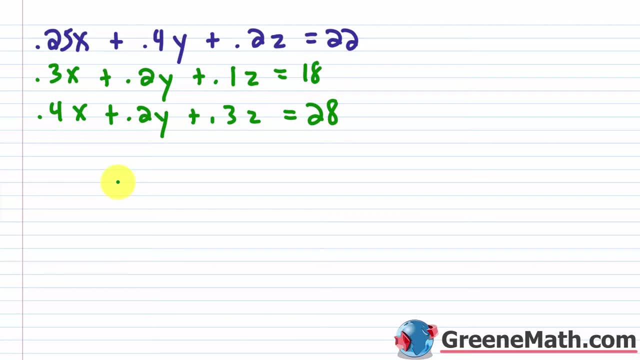 working with fractions or decimals, So I'm just going to transform this into a kind of decimal-free equation. in each case, I'm just going to go ahead and multiply kind of everything by 100.. So what I'd have is 25x plus 40y plus 20z equals 2,200,. okay, I just multiplied everything there by 100. 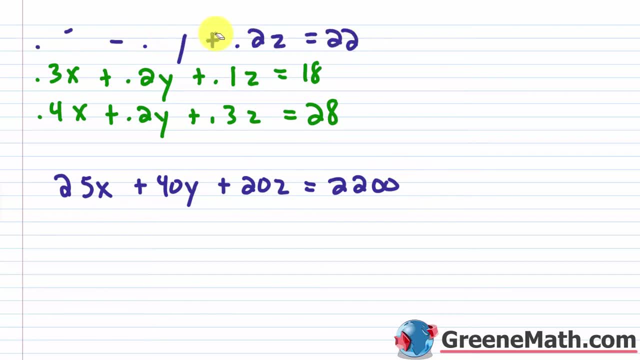 so that I could clear all the decimals. okay, So this one's gone now. And then for this one, I'm going to do multiplying everything by just 10, because that's all you need. So this would be: 3x plus 2y plus 1z equals 180.. So let's erase that. And then for this one, 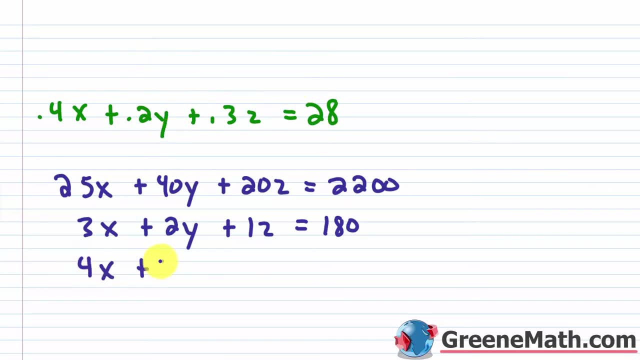 I only need 10 as well. So I'm going to have 4x plus 2y plus 3z equals 280.. Okay, so let's erase this and let's scooch this up. So again, when you work with a linear system, you're going to have: 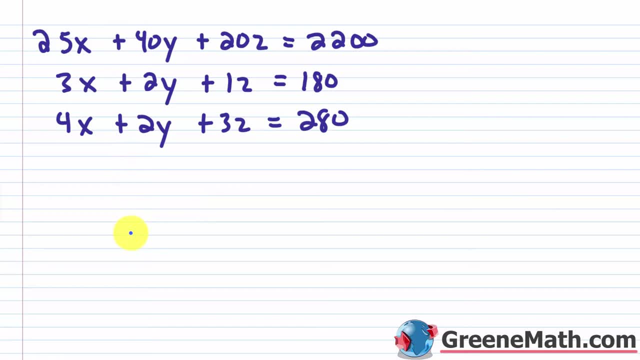 a linear system with three variables and you're not using a matrix. The first thing you want to do is kind of look at these equations. So I'm just going to label this as 1,, 2, and 3.. You just want. 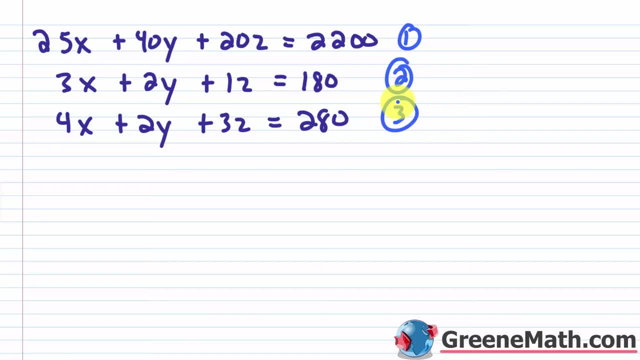 to pick two of them and then from the two you want to eliminate one of the variables. So if I look at these equations it looks like it's pretty easy to eliminate the variable y. okay, Because I have 2y here and 2y here. So from 2 and 3, I can really quickly eliminate y by just. 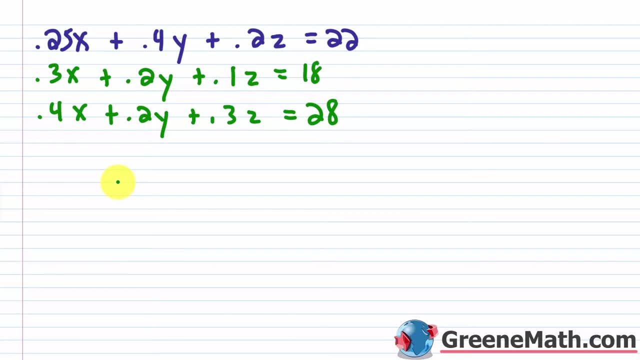 A lot of people don't like working with fractions or decimals, so I'm just going to transform this into a kind of decimal-free equation. in each case, I'm just going to go ahead and multiply kind of everything by 100.. So what I'd have is 25x. 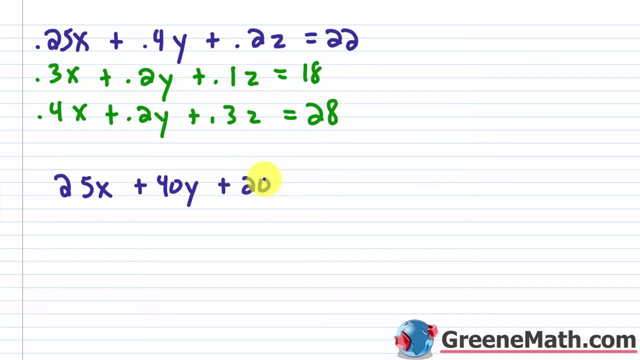 plus 40y plus 20z equals 2,200,. okay, I just multiplied everything there by 100 so that I could clear all the decimals. okay, So this one's gone now, And then for this one, I'm going to do multiplying everything by just. 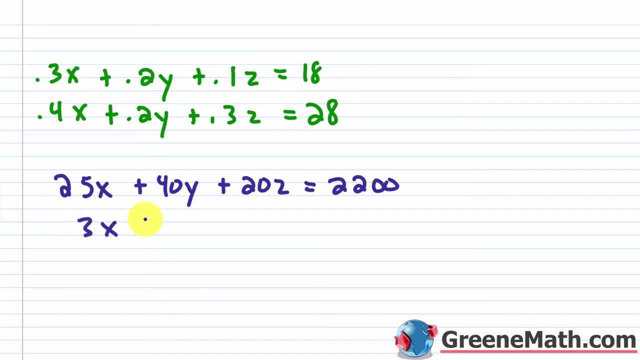 10, because that's all you need. So this would be: 3x plus 2y plus 1z equals 180.. So let's erase that. And then for this one, I only need 10 as well. So I'm going to have 4x. 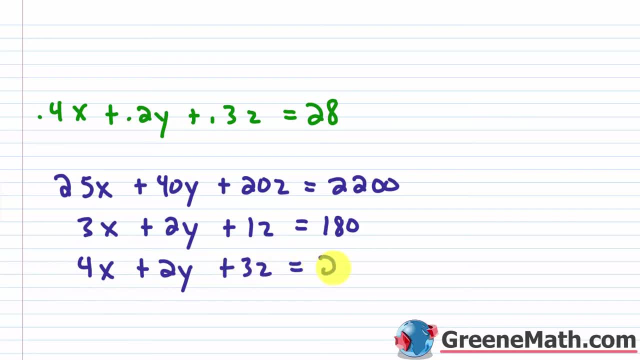 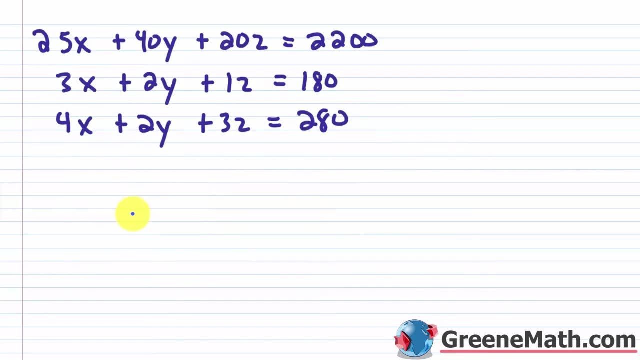 plus 2y plus 3z equals 280, okay, So let's erase this and let's scooch this up. So again, when you work with a linear system with three variables and you're not using a matrix, the first thing you want to do is: 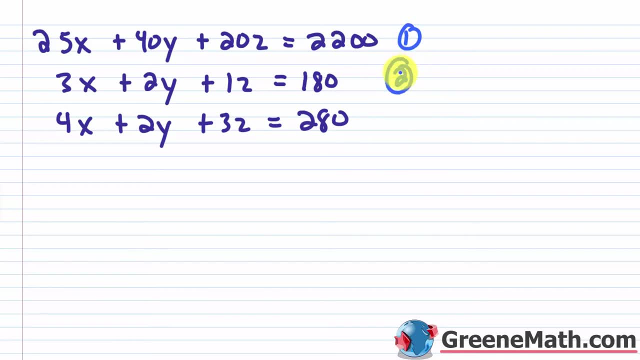 kind of look at these equations, So I'm just going to label this as 1,, 2, and 3. You just want to pick two of them and then from the two you want to eliminate one of the variables. So if I look at these equations, it looks like it's pretty easy to eliminate. 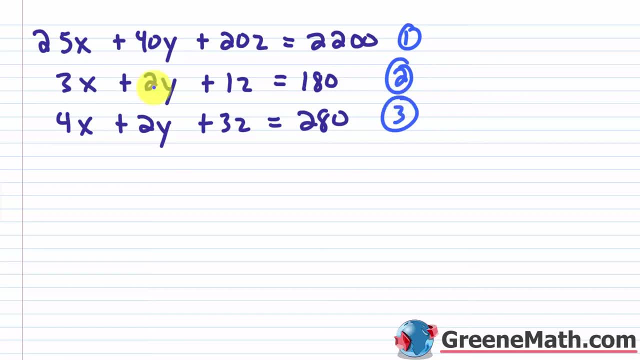 the variable y. okay, Because I have 2y here and 2y here. So from 2 and 3, I can really quickly eliminate y by just multiplying one of the equations by negative 1.. And I'm going to start with 1 and 2 and just multiply equation 2 by negative. 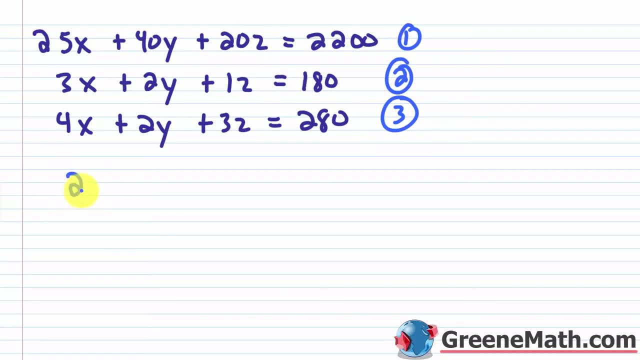 20.. So I'm going to keep equation 1 as it is. So 25x plus 40y plus 20z, and this equals 2,200.. And again for equation 2, I'm going to multiply both sides by negative 20.. 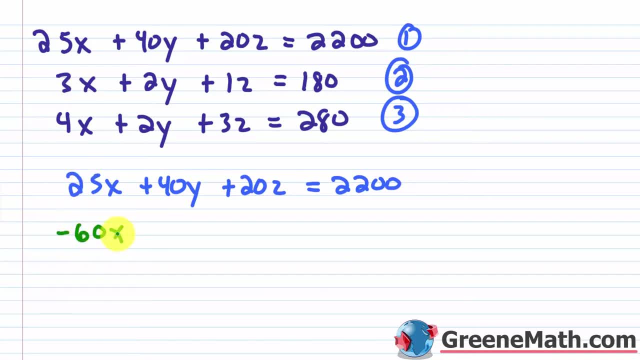 So negative 20 times 3x would be negative 60x. Negative 20 times 2y would be minus 40y. And you see that now I have opposite coefficients on y. The negative 20 times z is going to be: 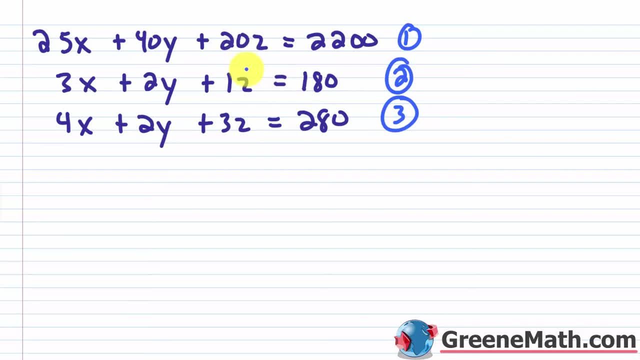 multiplying one of the equations by negative 1.. And I'm going to start with 1 and 2 and just multiply equation 2 by negative 20.. So I'm going to keep equation 1 as it is, So 25x plus 40y plus 20z, and this equals 2,200.. And again, 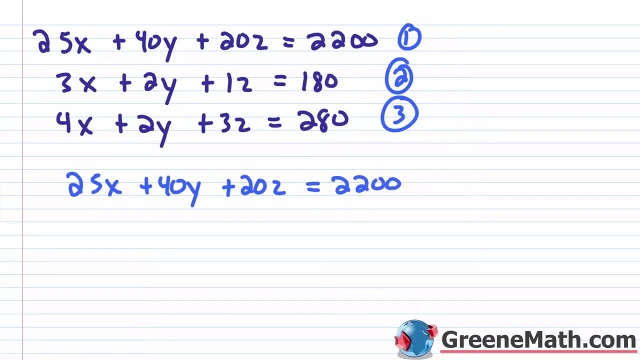 for equation 2, I'm going to multiply both sides by negative 20.. So negative 20 times 3x would be negative 60x. Negative 20 times 2y would be minus 40y. And you see that now I have opposite. 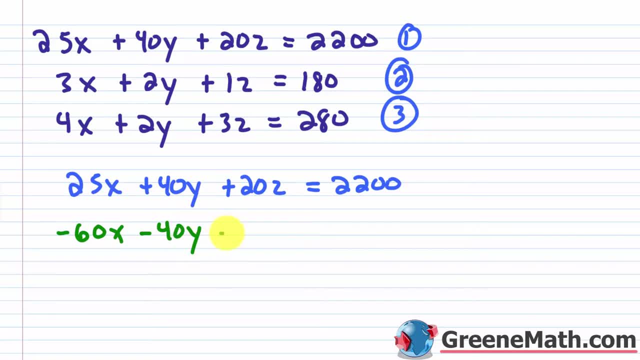 coefficients on y, The negative 20 times z is going to be minus 20z, And this equals negative 20 times 180 is going to be negative 3,600,. okay, Now again for this process to work. you want to have this kind of. 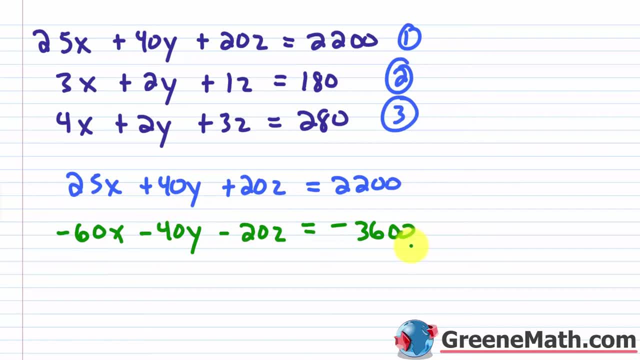 in the format where all the variable terms are on one side and your constants on the other. That way when you add the two left sides and you set it equal to the two right sides, you're adding like terms. So 25x minus 60x is going to be negative 35x. 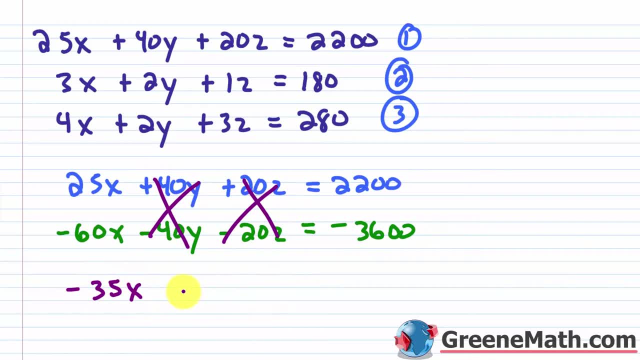 Then this is going to cancel, and so is this. So this would be equal to: I've got 2,200 minus 3,600, which is negative 1,400, okay, So let me erase this information. I don't need it anymore. 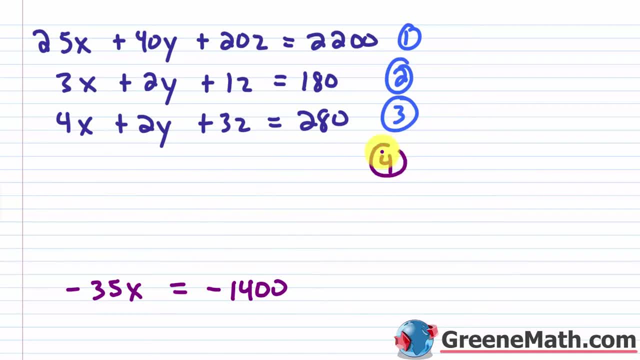 You could really call this equation 4 if you wanted to. So I can say this is equation 4.. Negative 35x is equal to negative 1,400.. So from this I can just solve for x right away. We kind of got lucky because two things dropped out, So I'm going to divide both sides by negative. 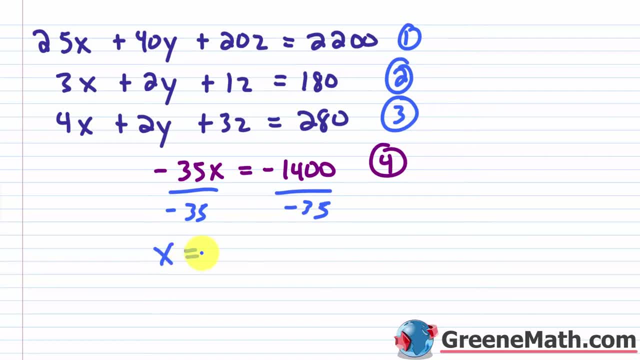 35. And I'm going to find that x is equal to negative 1,400.. So I'm going to divide both sides is equal to 40,. okay, So at this point I know that x is 40. So let me erase this and just put. 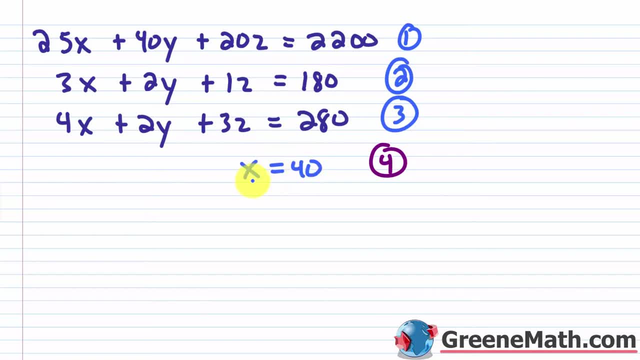 equation 4 as saying that x is equal to 40, okay, So that's one of my equations. Now I can't really do anything with x equals 40 because I still have two unknowns, So I'm still going to eliminate the 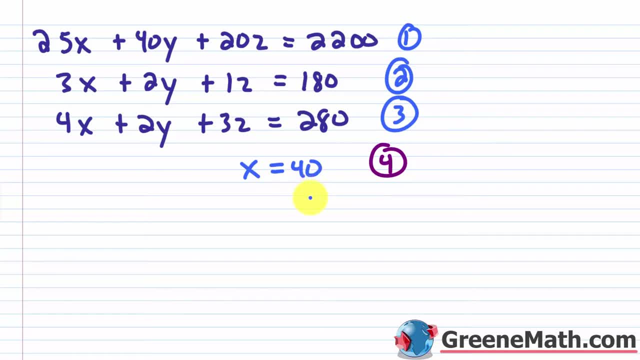 same variable. but it's worth noting that when you have this situation, I can eliminate either z or I can eliminate y- okay- from equation 2 and 3 or from equation 1 and 3.. And what that's going to do is it's going to give me a linear system with kind of two variables. 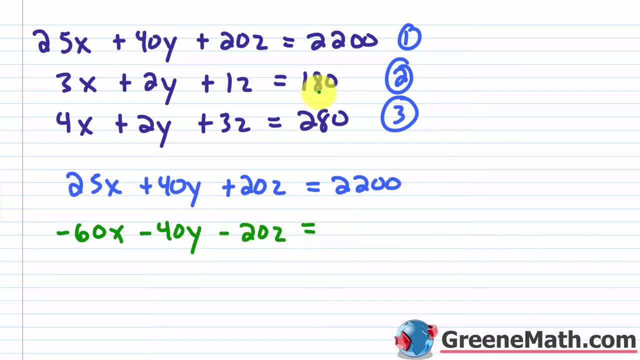 minus 20z, And this equals negative 20 times 180, is going to be negative 3,600,. okay, Now again for this process to work. you want to have this kind of in the format where all the variable terms are on one side and your constants on the other. That way, when you add the two left. 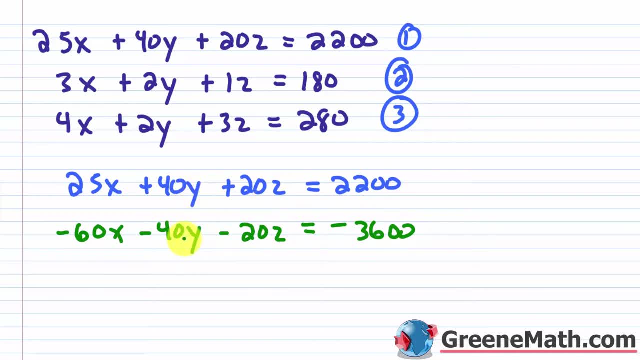 sides and you set it equal to the two right sides, you're adding like terms. So 25x minus 60x is going to be negative 35x. Then this is going to cancel, and so is this. So this would be equal to: 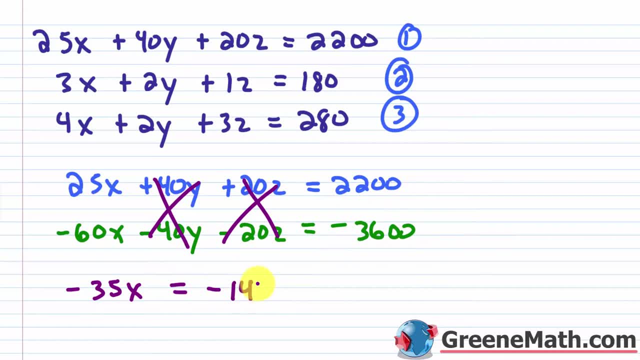 I've got 2,200 minus 3,600, which is negative 1,400,. okay, So let me erase this information. I don't need it anymore. You could really call this equation 4 if you wanted to, So I can say: this is equation 4.. 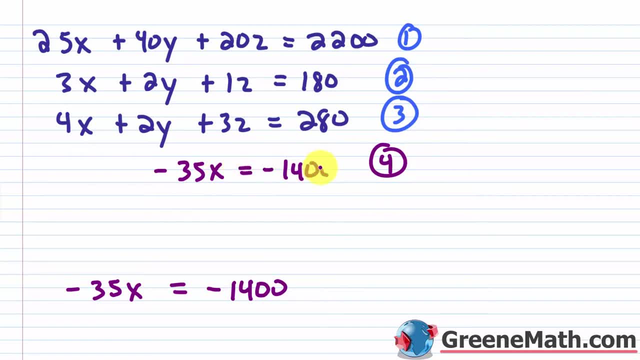 Negative 35x is equal to negative 1,400.. So from this I can just solve for x right away. We kind of got lucky because two things dropped out. So I'm going to divide both sides by negative 35, and I'm going to find that x is equal to 40,. okay, So at this point I know that x is 40. 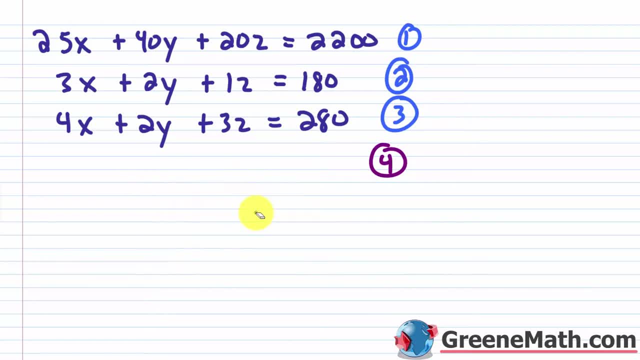 So let me erase this information. I don't need it anymore. So I'm going to divide both sides by negative 35, erase this and just put equation four as saying that x is equal to 40. okay, so that's one of my equations. now i can't really do anything with x equals 40 because i still have two unknowns. so 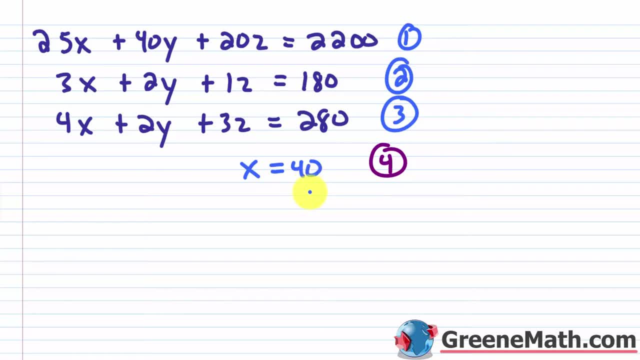 i'm still going to eliminate the same variable, but it's worth noting that when you have this situation, i can eliminate either z, or i can eliminate y- okay- from equation two and three, or from equation one and three, and what that's going to do is it's going to give me a linear system with kind of 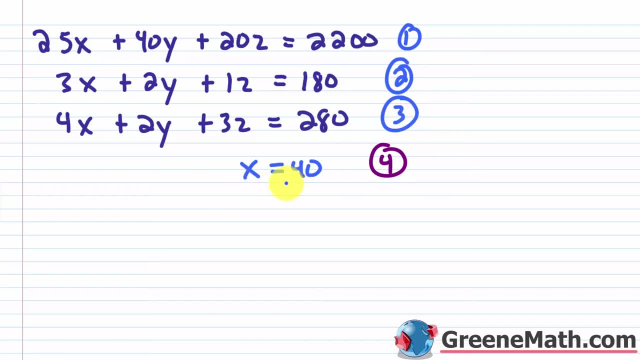 two variables. i already know that x is 40, so i can immediately just plug in and figure out what y is or what z is, again based on what i choose to eliminate. what i'm going to do is i'm just going to stay consistent and i'm going to eliminate y again, and i'm going to do that from two and three. 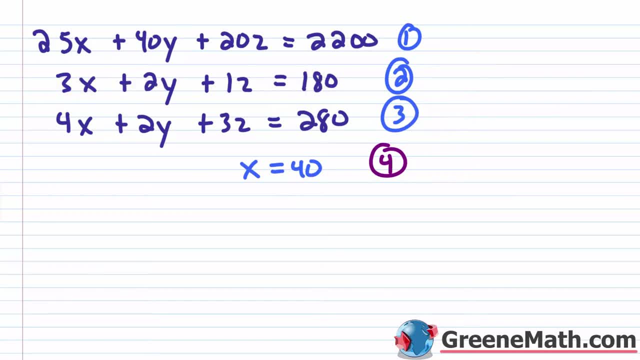 so what i'm going to do is i'm going to multiply equation two by negative one, so i'm going to have negative three x minus two. y minus z equals negative 180. again. i just multiplied everything by negative one. i'm going to keep equation three as it is, so four x plus two y. 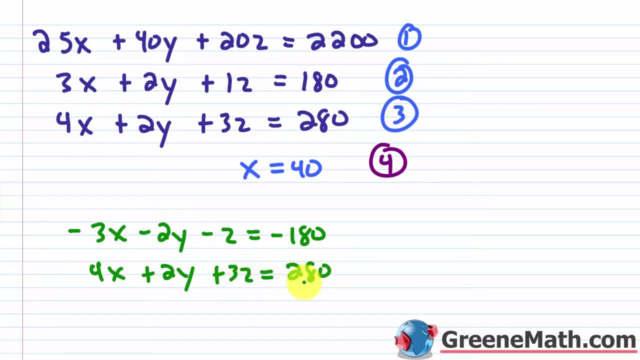 minus two, y minus z equals negative 180. again i just multiplied everything by negative one minus two y minus z equals negative 180. again i just multiplied everything by negative one plus 3z, And this equals 280.. And again I have opposite coefficients. on my variable y I have: 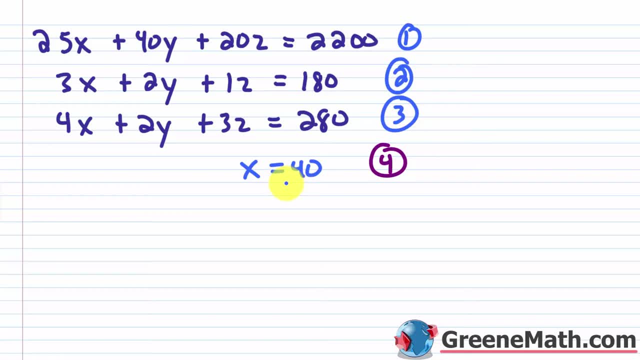 I already know that x is 40, so I can immediately just plug in and figure out what y is or what z is, again based on what I choose to eliminate. What I'm going to do is: I'm just going to stay consistent and I'm going to eliminate y again, And I'm going to do that from 2 and 3.. So what? 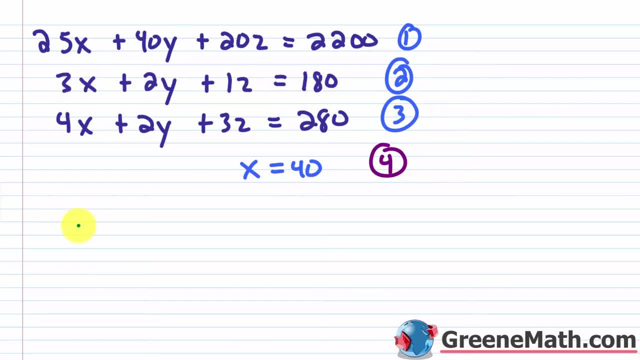 I'm going to do is I'm going to multiply equation 2 by negative 1.. So I'm going to have negative 3x minus 2y minus z equals negative 180.. Again, I just multiplied everything by negative 1.. 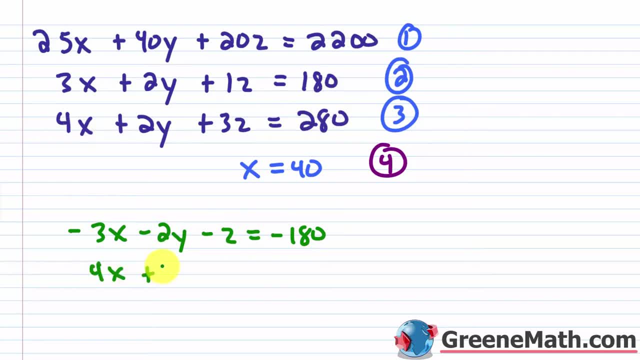 I'm going to keep equation 3 as negative 3.. So I'm going to keep equation 3 as negative 3.. So 4x plus 2y plus 3z, and this equals 280.. And again I have opposite coefficients on my. 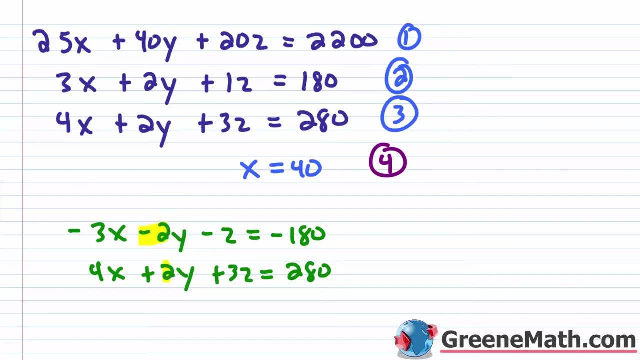 variable y, I have negative 2 and positive 2.. So when I add the left sides, this is going to cancel right. So negative 3x plus 4x is going to be x, And then we have negative z plus 3z. 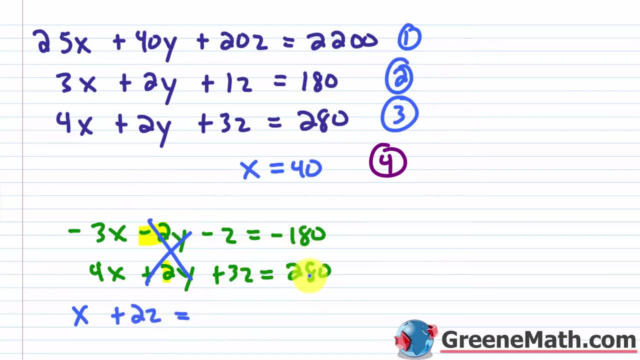 which is plus 2z. This equals negative 180 plus 280 is 100.. So let's erase this. And again, we already know from our equation: we're going to have negative 3x plus 3z plus 3z. 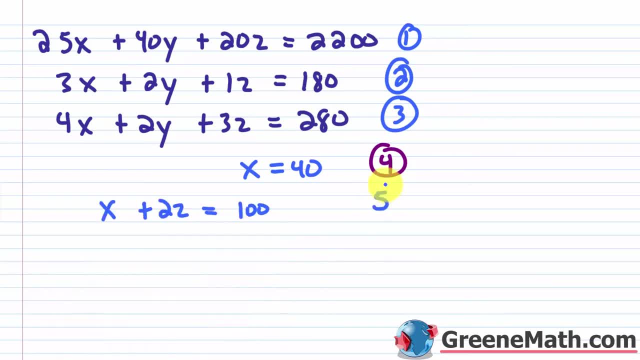 So I'm going to call this equation 5 now And I'm going to plug a 40 in for x there. So I have: 40 plus 2z equals 100.. And let me subtract 40 away from each side of the equation. 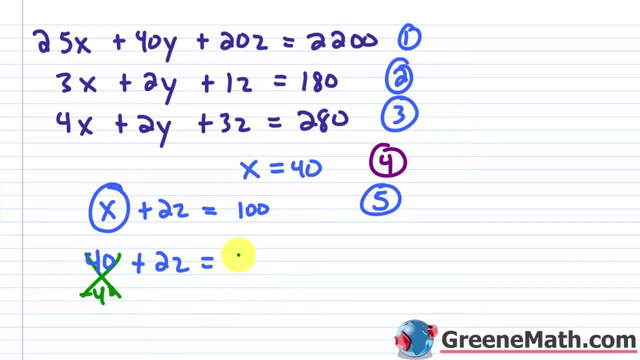 This cancels And this will become 60. So let me kind of clean this up a little bit. We essentially just have: 2z equals 60. Divide both sides by 2. And of course we find that z is equal to 30.. Okay, So let me erase all of this now. We don't need any of this information anymore. 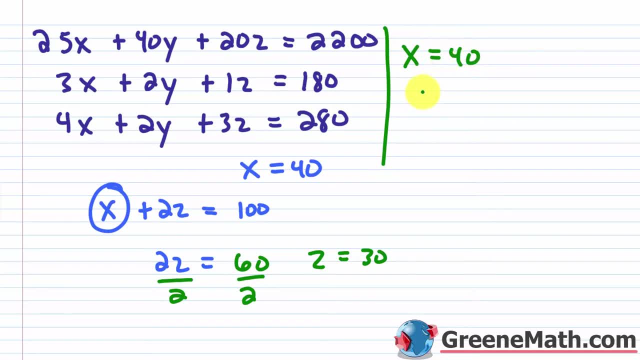 I'm just going to do that And I'm going to call this equation 5 now, And I'm going to plug a 40 in for x there And I'm going to put over here that x equals 40 and z equals 30. And now we just need: 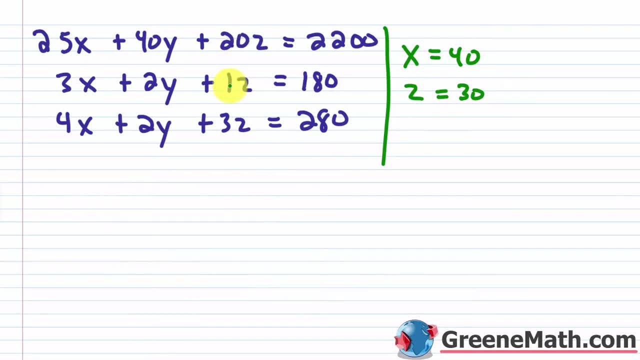 to find y. Okay, And that's pretty easy to do: Just plug into any of the original equations- a 40 for x and a 30 for z- and figure out what y is. So it looks like it's pretty easy to work. 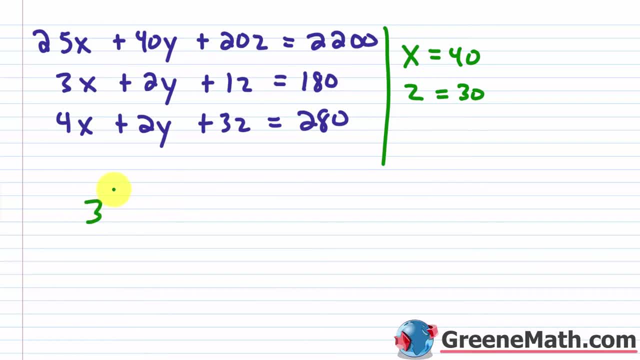 with this second equation or this middle equation. So 3 times x, 3 times 40, plus 2y plus 1 times z, z is 30, so just plus 30, equals 180.. Okay Well, 3 times 40 is 120.. 120 plus 30,. 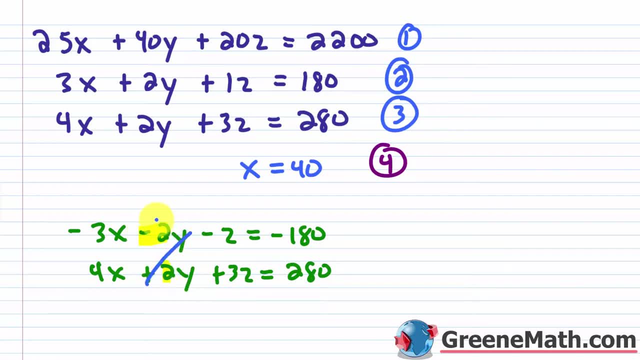 negative 2 and positive 2.. So when I add the left sides, this is going to cancel right. So negative 3x plus 4x is going to be x, And then we have negative z plus 3z, which is plus 2z. This equals. 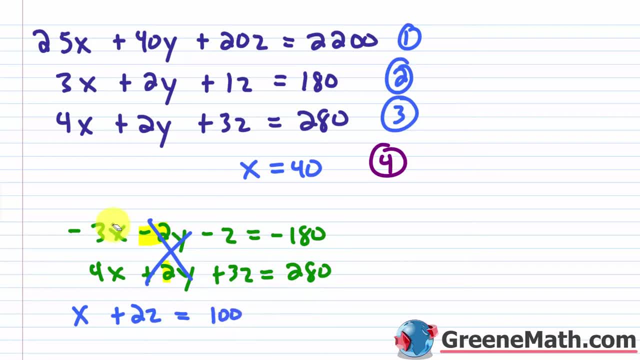 negative. 180 plus 280 is 100. So let's erase this. And again, we already know from our equation 4 that x is going to be 40. So I'm going to call this equation 5 now And I'm going to plug a 40. 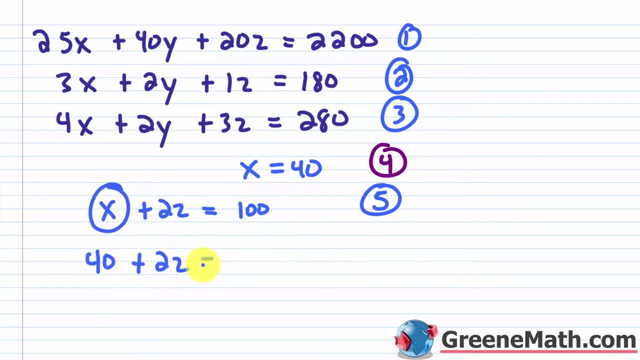 in for x there. So I have 40 plus 2z equals 100. And let me subtract 40 away from each side of the equation. This cancels And this will become 60. So let me kind of clean this up a little bit. 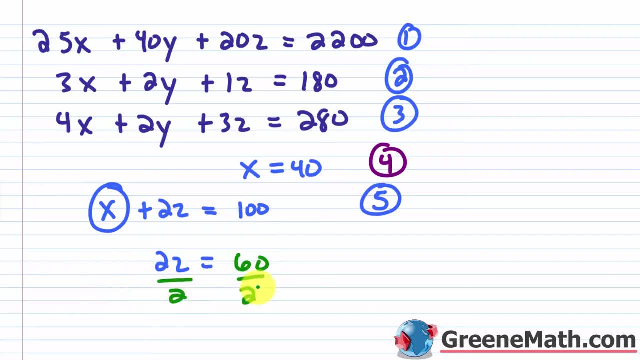 We essentially just have: 2z equals 60. Divide both sides by 2. And, of course, we find that z is equal to 30, okay, So let me erase all of this now. We don't need any of this information anymore. 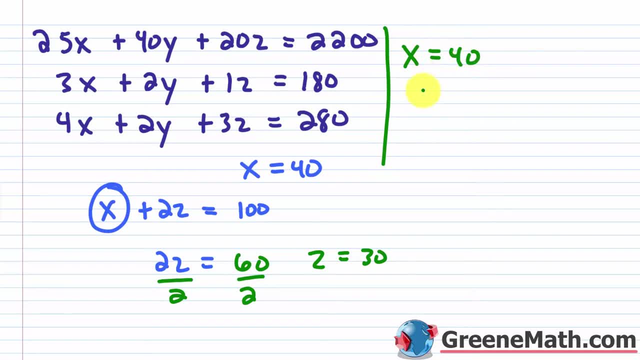 I'm just going to put over here that x equals 40 and z equals 30. And now we just need to find y. okay, And that's pretty easy to do, Just plug into any of the original equations a 40 for x and a 30 for z and figure. 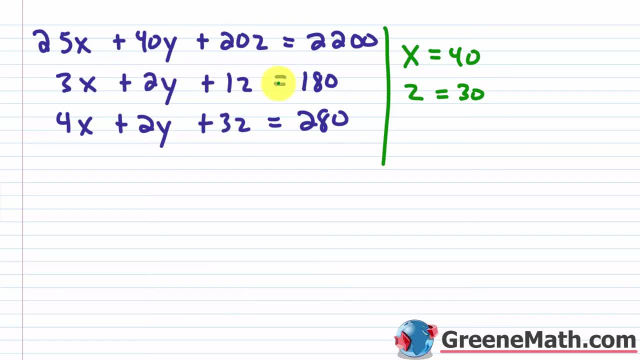 out what y is. So it looks like it's pretty easy to work with this second equation or this middle equation. So 3 times x, 3 times 40, plus 2y plus 1 times z, z is 30, so just plus 30, equals 180. 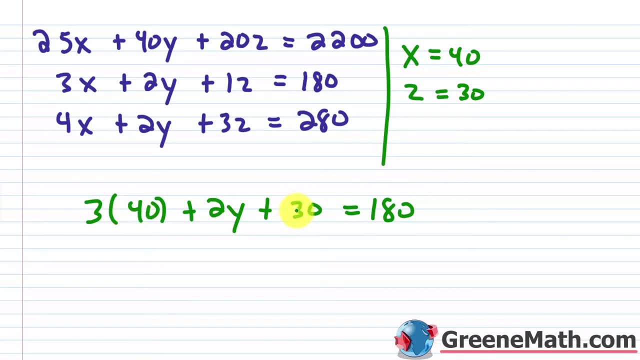 Okay, Well, 3 times 40 is 120.. 120 plus 30 is 150.. So let's erase this and put 150.. Then if I subtract that away from each side, this cancels. You'll have 2y is equal to 30.. Divide both sides by 2.. You get y equals 15,. 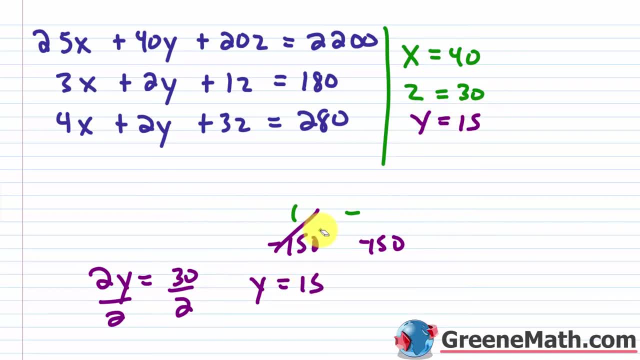 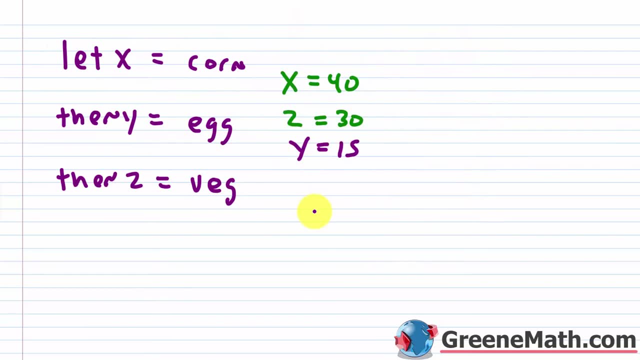 okay, So y equals 15.. All right, So let's erase everything and we can state our answer. So let me copy this real quick And let me just paste that here So we remember that x is the amount in ounces of the corn mixture we're going to use. 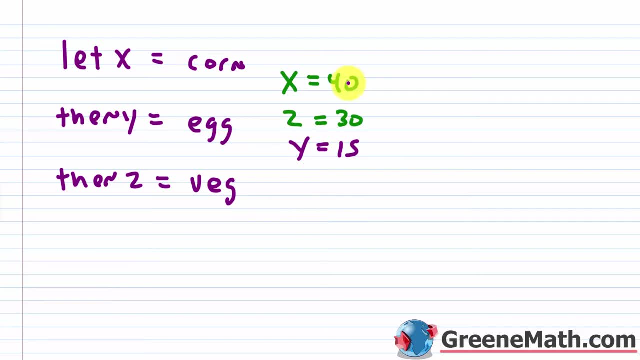 And that's going to be 40,. okay, So we're going to use 40 ounces of the corn mixture And then we know that y was the amount of the egg mixture we're going to use. That's going to be 15. 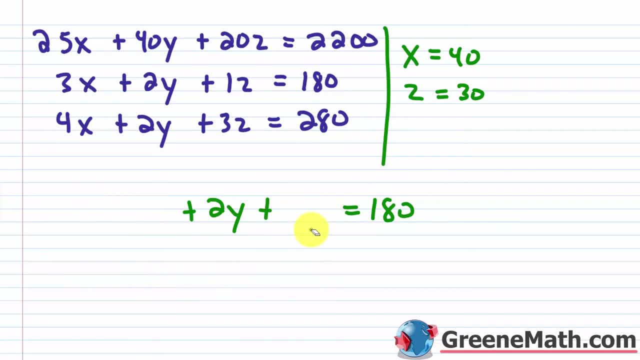 is 150.. So let's erase this and put 150.. Then if I subtract that away from each side, this cancels. You'll have 2y is equal to 30.. Divide both sides by 2.. You get y equals 15.. Okay. 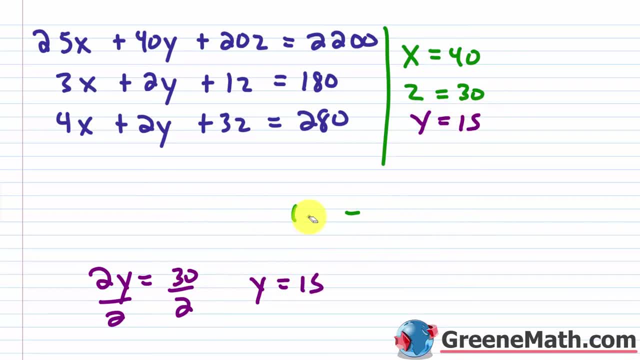 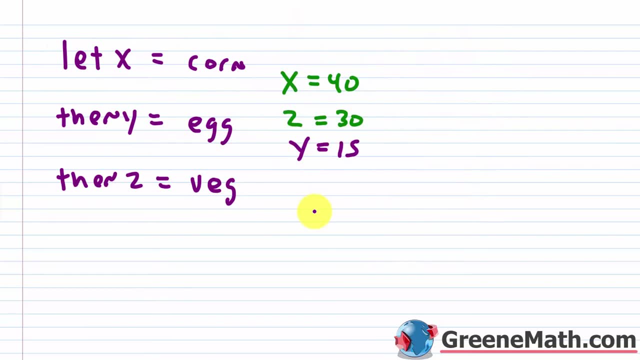 So y equals 15.. All right, So let's erase everything and we can state our answer. So let me copy this real quick And let me just paste that here So we remember that x is the amount in ounces of the corn. Make sure, we're going to paste that here. So we're going to paste that here. 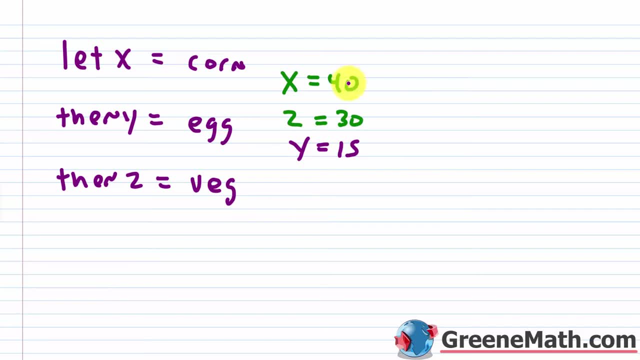 We're going to use, and that's going to be 40.. Okay, So we're going to use 40 ounces of the corn mixture, And then we know that y was the amount of the egg mixture we're going to use. That's. 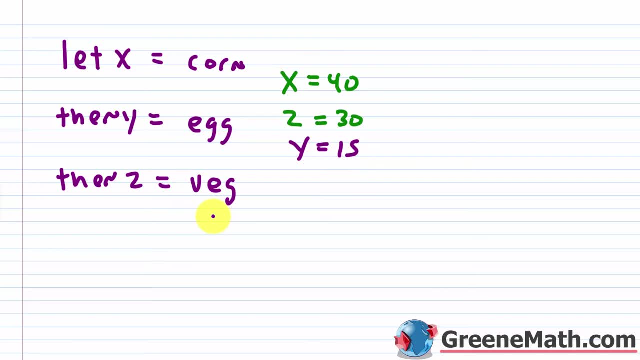 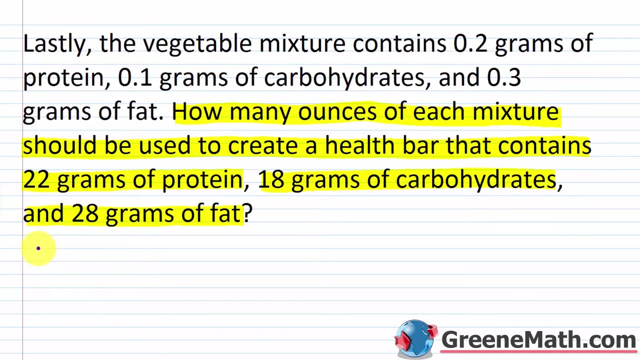 going to be 15 ounces And we know that z is the amount in ounces of the vegetable mixture. That's going to be 30.. Okay, So let's write this as a nice little sentence, So we will say that they should use Again: the corn mixture was x and x was 40. So 40 ounces. 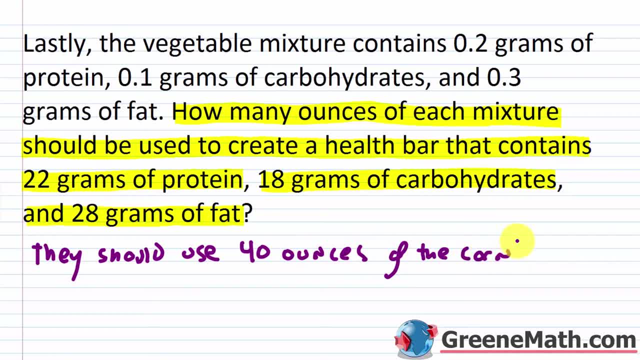 Of the corn mixture With, you're going to have again 15 ounces. Remember y was the amount of kind of egg mixture and we had y equals 15.. So 15 ounces of the egg mixture And then and 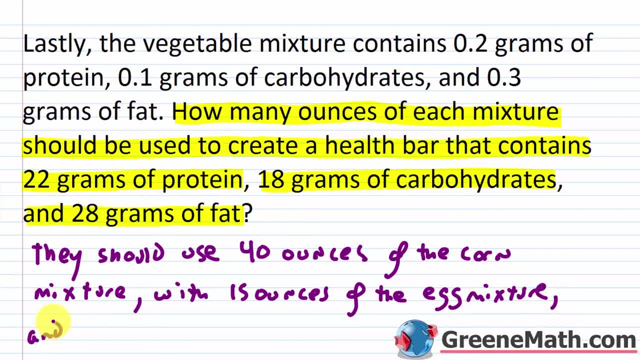 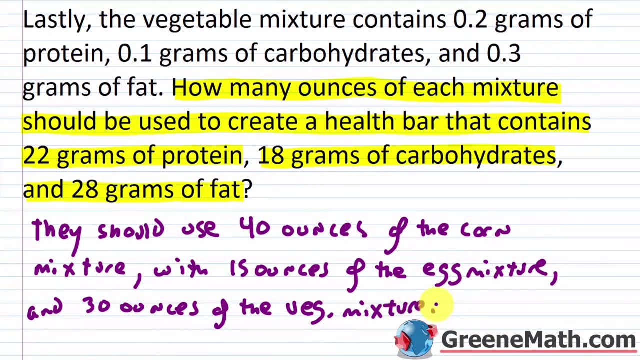 Z was the amount of the vegetable mixture they used and that was 30.. So and 30 ounces of the vegetable mixture. So they should use 40 ounces of the corn mixture with 15 ounces of the egg mixture and 30 ounces of the vegetable mixture. 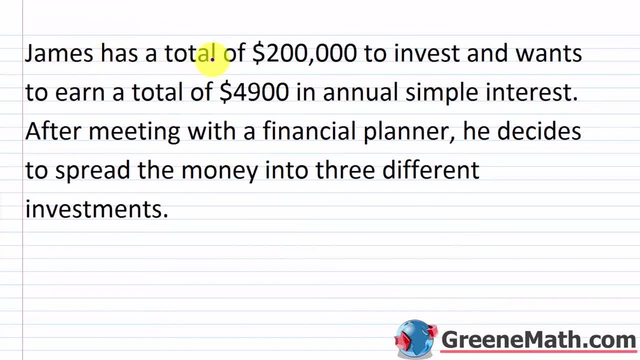 All right, let's look at a simple interest problem. So James has a total of $200,000 to invest and wants to earn a total of $4,900 in annual simple interest. After meeting with a financial planner, he decides to spread the money into three different 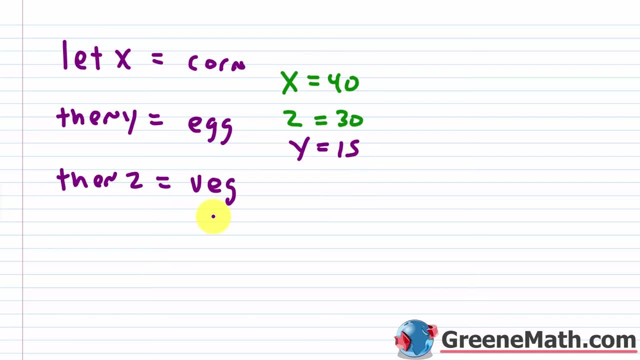 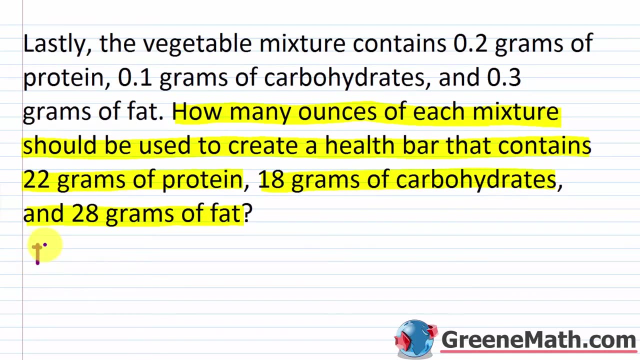 ounces And we know that z is the amount in ounces of the vegetable mixture. That's going to be 30, okay, So let's write this as a nice little sentence. So we will say that they should use again. the corn mixture was x and x was 40. So 40 ounces. 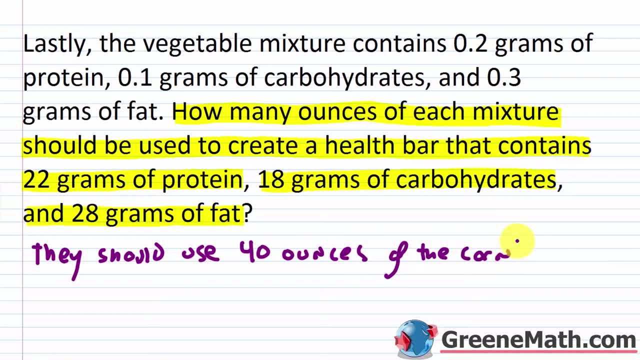 Of the corn mixture With, you're going to have again 15 ounces. Remember y was the amount of kind of egg mixture And we had y equals 15.. So 15 ounces of the egg mixture And then and 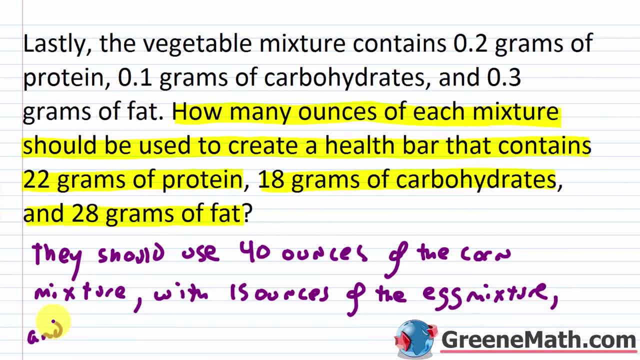 or y was the amount of corn mixture we type. So that's going to be 30.. So it's the corn mixture with the egg mixture. So x is 40 and the corn mixture with 25.. So it's going to be 40 and 50 is the amount of the. 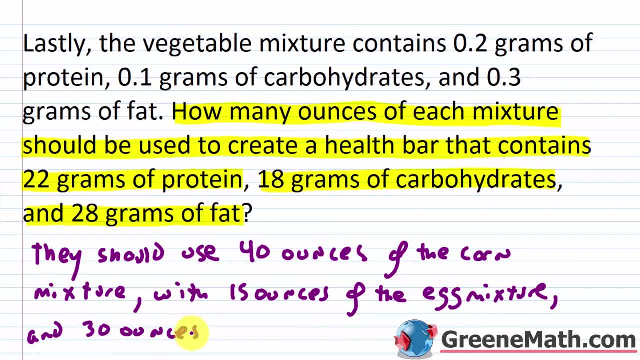 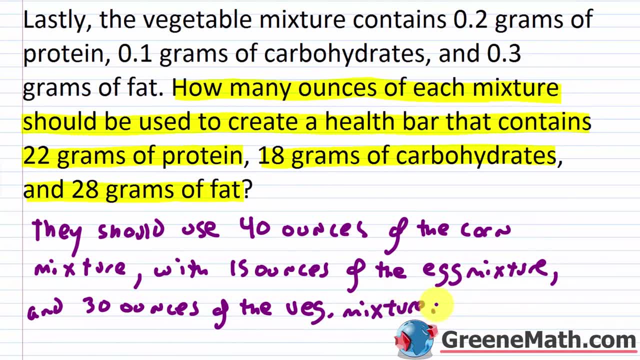 And now we know that' I'm going to say z, about 1 ounce of the corn mixture. um, z was the amount of the vegetable mixture they used And that was 30.. So, and 30 ounces of the vegetable mixture. Okay, So they should use 40 ounces of the corn mixture with new. 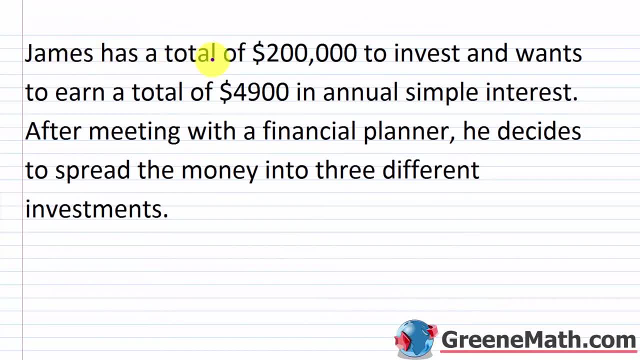 ounces of the egg mixture and 30 ounces of the vegetable mixture. All right, Let's look at a simple interest problem. So James has a total of $200,000 to invest- $4,900 in annual simple interest After meeting with a financial planner. 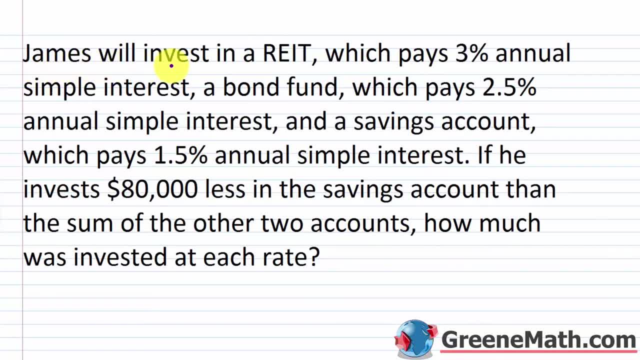 he decides to spread the money into three different investments. So James will invest in a REIT, which is a real estate investment trust, which pays 3% annual simple interest, a bond fund which pays 2.5% annual simple interest. 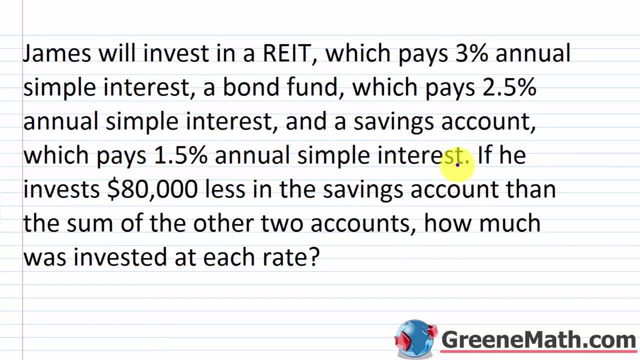 and a savings account which pays 1.5% annual simple interest. If he invests $80,000 less in the savings account, then the sum of the other two accounts how much was invested at each rate. So pretty easy problem overall. 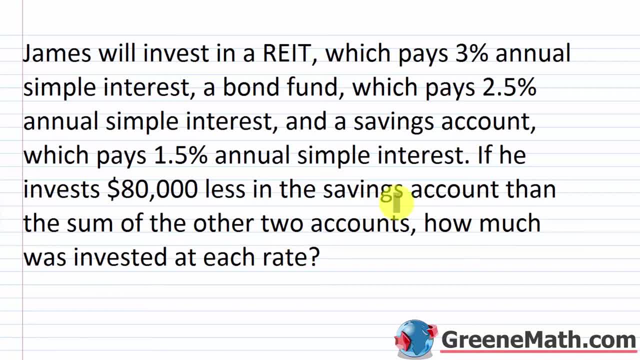 Again, when you start these, you wanna figure out what you're being asked to find. So we just need to find how much was invested at each rate. Remember he had a total- if we go back up- of $200,000, that's invested. 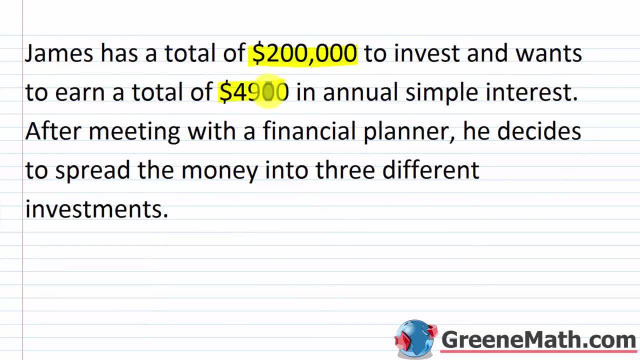 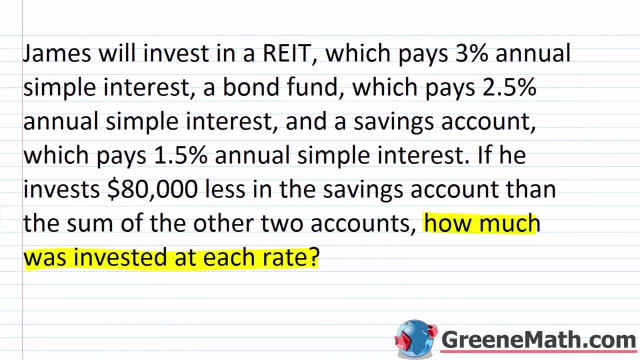 and he wants to earn this amount right here. So we wanna set up kind of three variables to represent the three unknowns. We need to know how much he's going to invest in the REIT. We're getting the real estate investment trust. 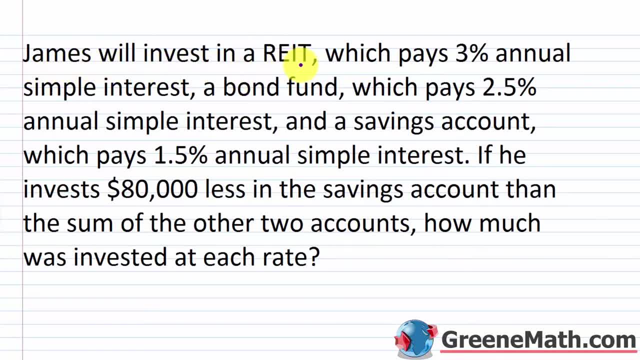 investments. So James will invest in a REIT, which is a real estate investment trust which pays 3% annual simple interest, a bond fund which pays 2.5% annual simple interest, and a savings account which pays 1.5% annual simple interest. 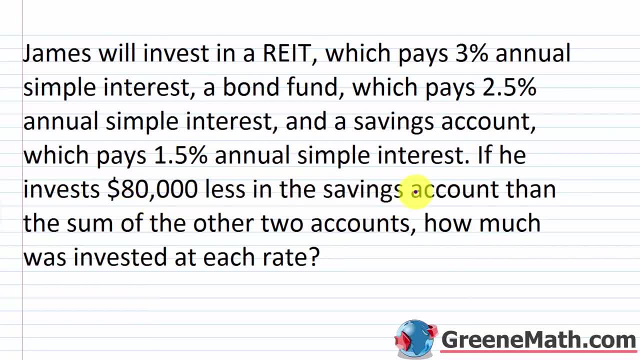 If he invests $80,000 less in the savings account, Then the sum of the other two accounts how much was invested at each REIT. So pretty easy problem overall. again, when you start these, you want to figure out what. 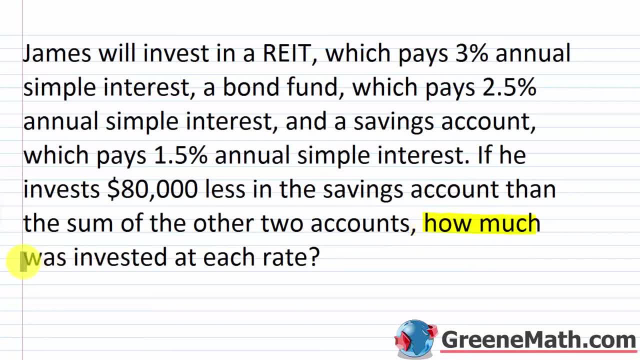 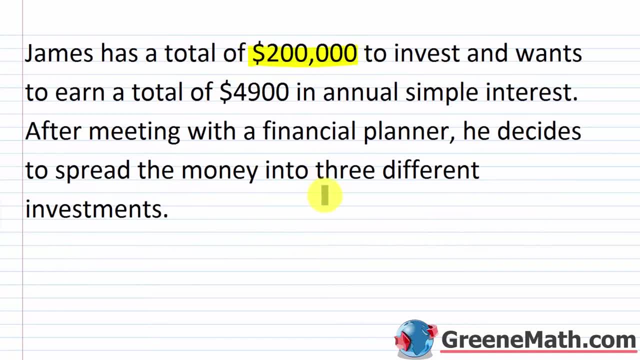 you're being asked to find. So we just need to find how much was invested at each rate. Remember he had a total, if we go back up, of $200,000 that's invested, and he wants to earn this amount right here. 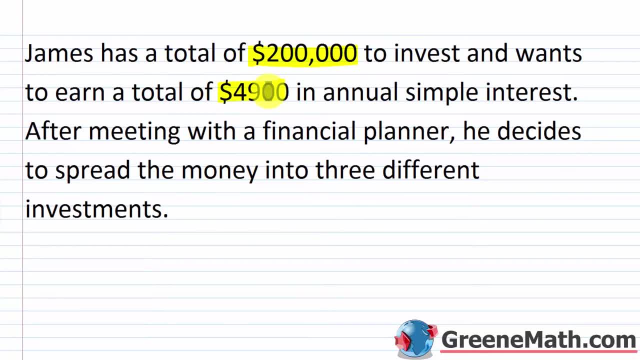 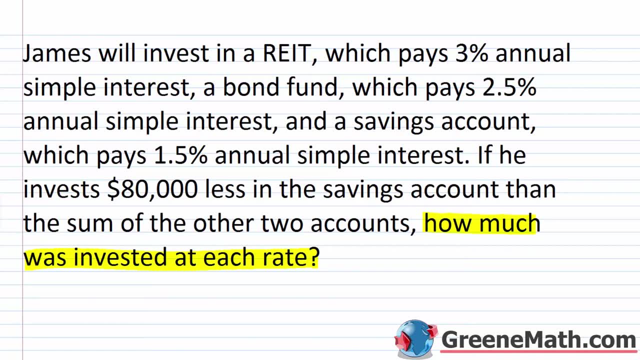 So we want to set up kind of three variables to represent the three unknowns. we need to know how much he's going to invest in the REIT, or again the real estate investment trust, the bond fund and then also the savings account. 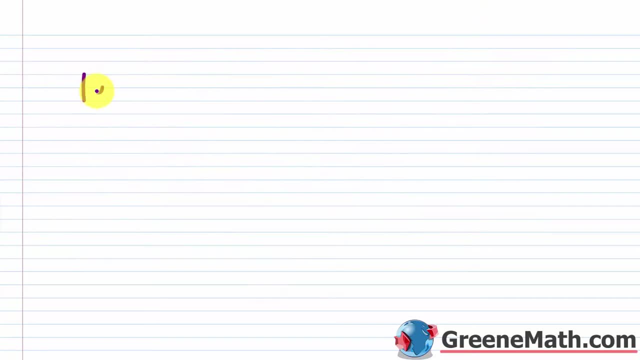 So let's go ahead and let our variables like X, Y and Z represent those. So X can be the REIT, that's the amount he invests in that, And then we can say Y will be equal to the bond fund, the bond fund, and then Z can be. 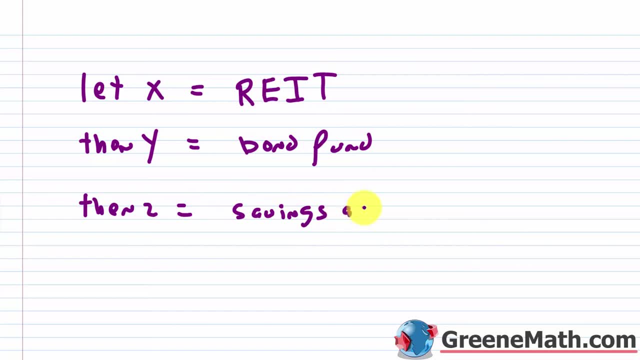 equal to the savings. Okay, so we need to get three equations to solve for this kind of three unknowns that we have here. So let me go down and let's think about the first equation. Okay, the first equation is pretty easy. 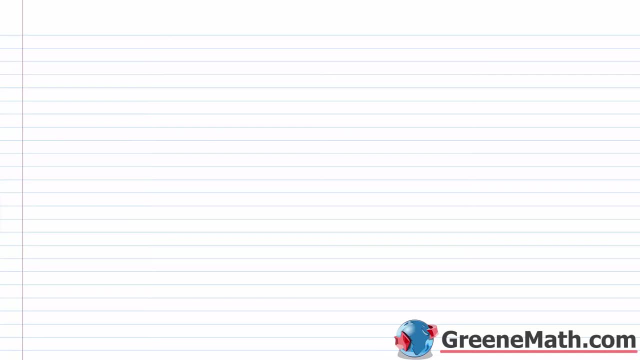 You know that the amount that he invests is $200,000,. okay, and he invests this with three different kind of investment vehicles. So it must be true that X plus Y plus Z equals $200,000.. So that can be my first equation. 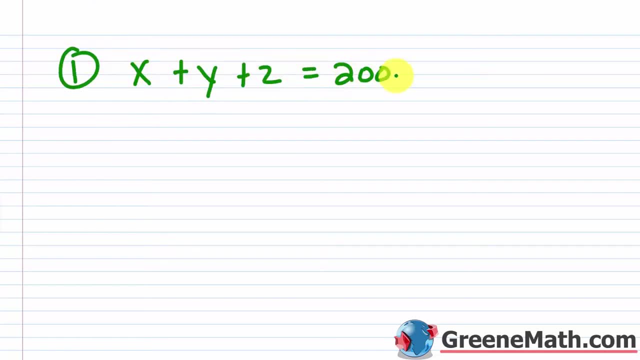 X plus Y plus Z equals $200,000.. That's an easy one because, again, the amount he invests in the REIT, which is X, plus the amount he invests in the bond fund, which is Y, plus the amount he invests in the savings, 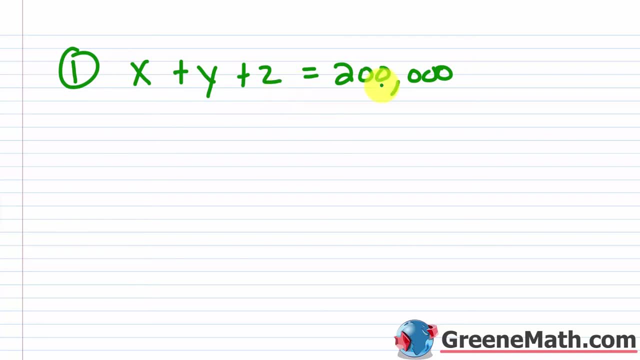 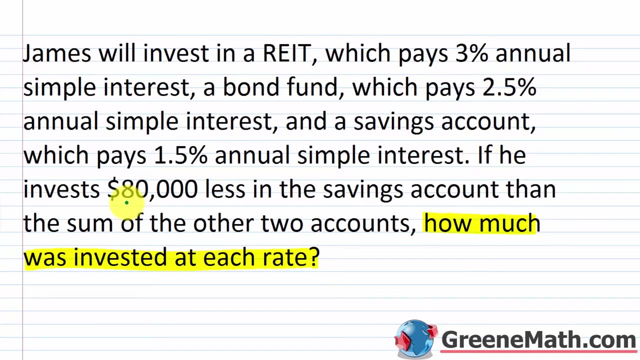 account, which is Z, has to be equal to $200,000, because that's what he puts in to all three. Now for the next one. we can read the problem and it tells us specifically that he invests $80,000 less in the savings account. 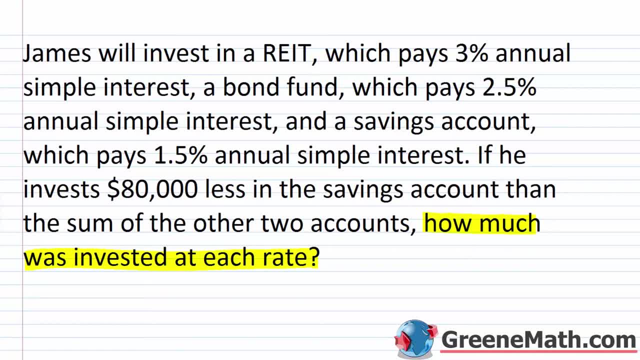 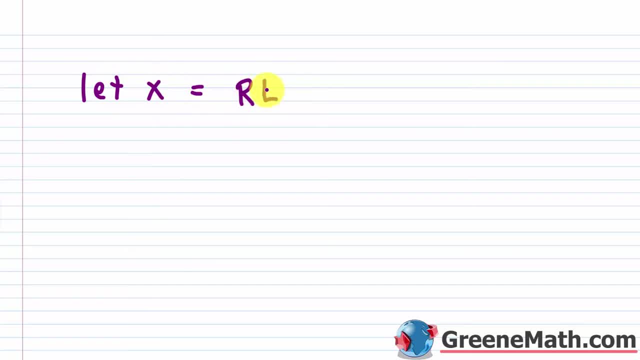 the bond fund and then also the savings account. So let's go ahead and let our variables like X, Y and Z represent those. So X can be the REIT- okay, that's the amount he invests in that- And then we can say Y will be equal to the bond fund. 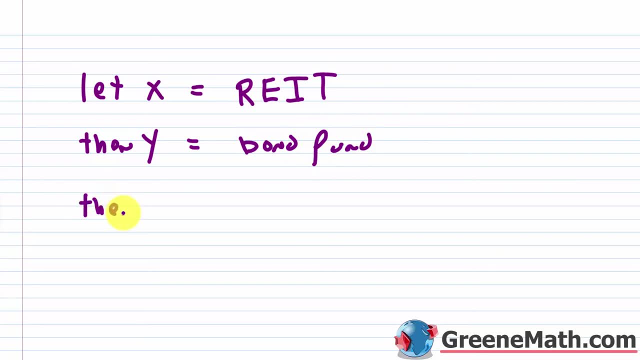 okay, the bond fund, And then Z can be equal to the savings, the savings account, okay. So we need to get three equations to solve for this kind of three unknowns that we have here. So let me go down and let's think about the first equation, okay. 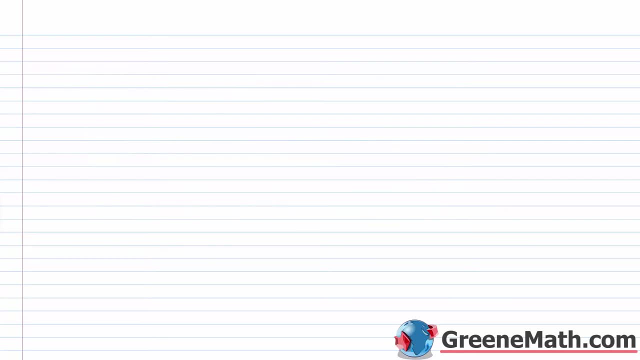 The first equation is pretty easy. You know that the amount that he invests is 200,000, okay, And he invests this with three different kind of investment vehicles, So it must be true that X plus Y plus Z equals 200,000. 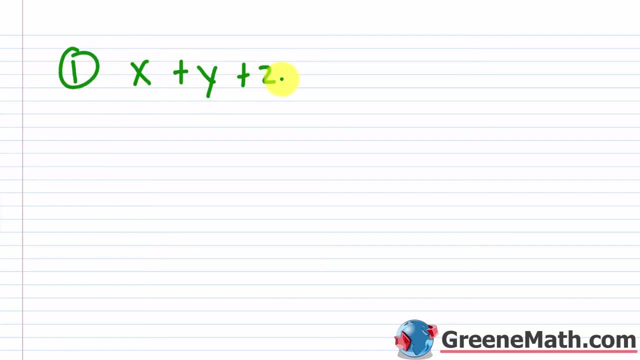 So that can be my first equation: X plus Y plus Z equals 200,000,. okay, And that's an easy one because, again, the amount he invests in the REIT, which is X plus the amount he invests in the bond fund, 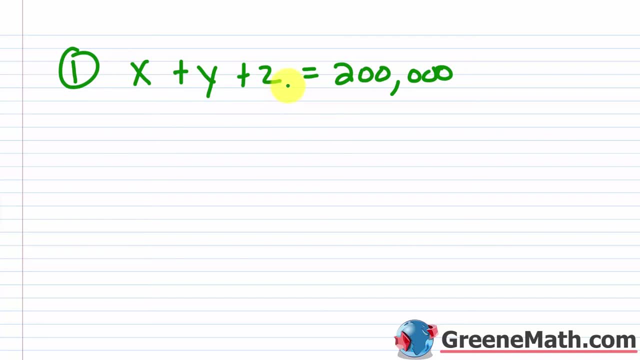 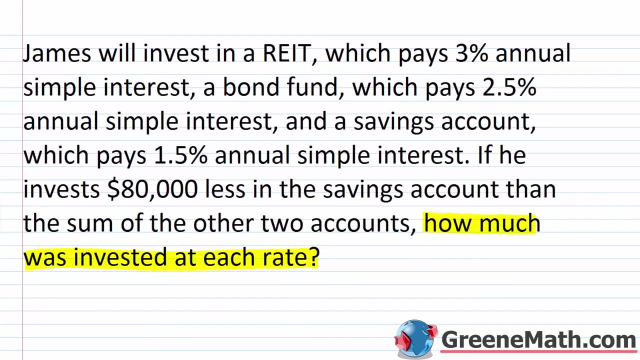 which is Y, plus the amount he invests in the savings account, which is Z, has to be equal to 200,000, because that's what he puts into all three. Now for the next one. we can read the problem and it tells us specifically that he invest $80,000. 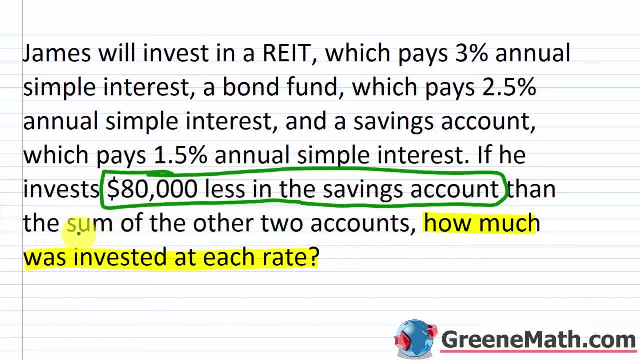 less in the savings account okay than the sum of the other two accounts. Okay account with Z and the sum of the other two accounts. the other two accounts were X and Y. so if I sum that that's X plus Y. so it's 80,000 less than X plus Y. so for 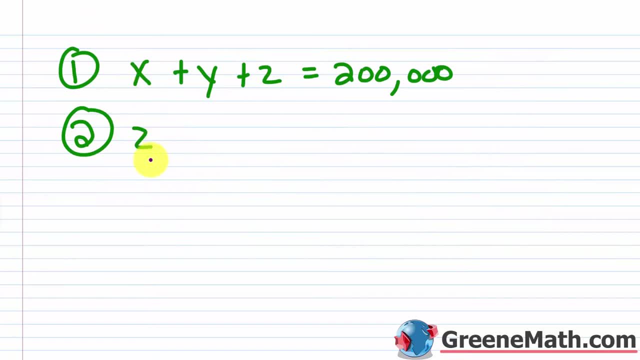 equation 2, Z again, the amount he invests in the savings account is equal to the sum of X plus Y. this is the amount he invests in the other two, so the REIT and the bond fund, minus 80,000. right, because it's $80,000 less than this amount here. 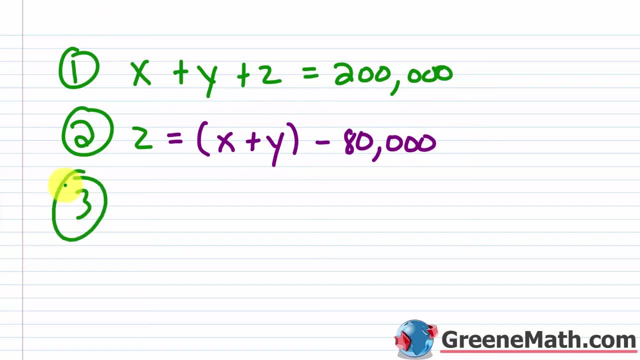 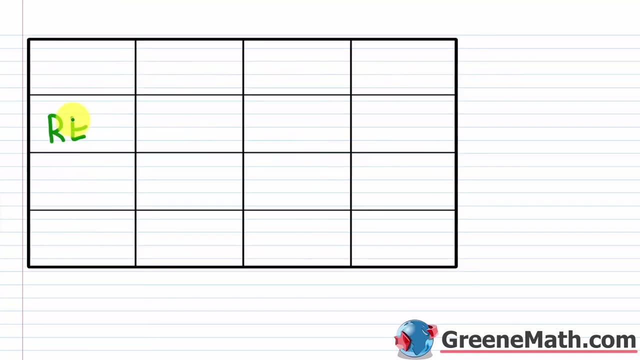 now for the third equation. we need to think about the interest. okay, the interest. so to do that, let's set up a little table. so what we're gonna have is our REIT, we're gonna have our bond fund and we're gonna have our savings account. 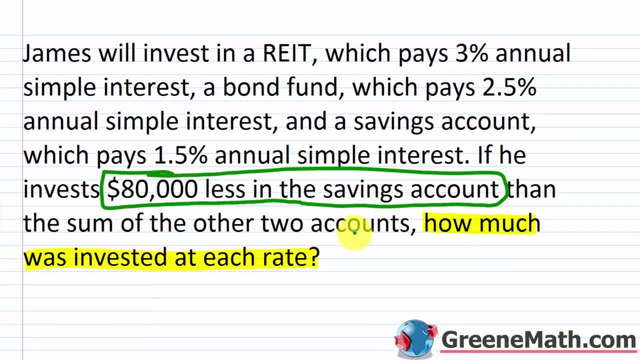 Okay, So the savings account was Z and the sum of the other two accounts. the other two accounts were X and Y, so if I sum that, that's X plus Y, So it's $80,000 less than X plus Y. 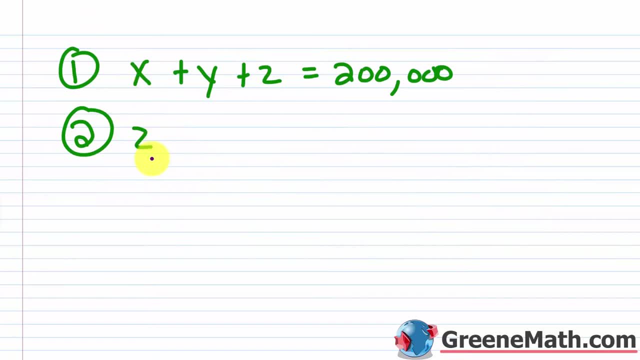 So for equation two, Z again, the amount he invests in the savings account is equal to the sum of X plus Y. This is the amount he invests in the other two, so the REIT and the bond fund minus. 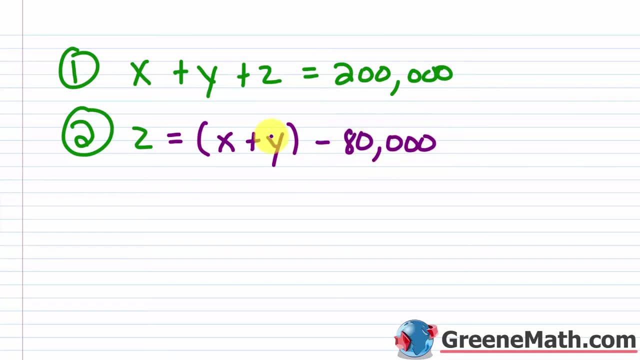 $80,000, right, Because it's $80,000.. So it's $80,000 less than this amount here. Now for the third equation. we need to think about the interest. okay, the interest. So to do that, let's set up a little table. 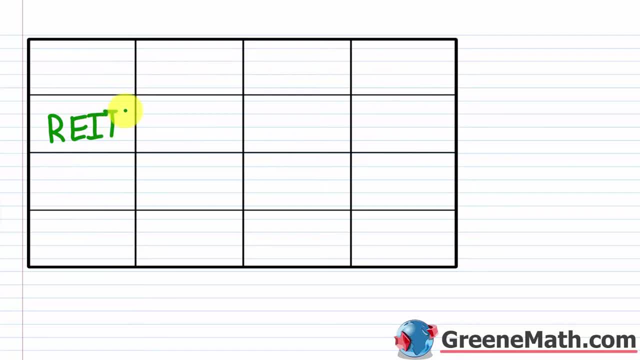 So what we're going to have is our REIT. we're going to have our bond fund and we're going to have our savings account, and then we're going to have the amount invested, or you could say the principal. We're going to have our rate, and this is as a decimal. 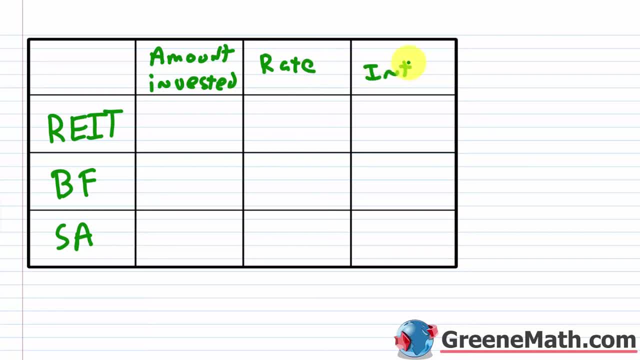 Okay, And then we're going to have our interest. okay. Now we're working with simple interest. it's not compounding, okay? So most of you already know, because we talked about this earlier in the course, the simple interest formula is I, which stands for the amount of simple interest earned, is equal. 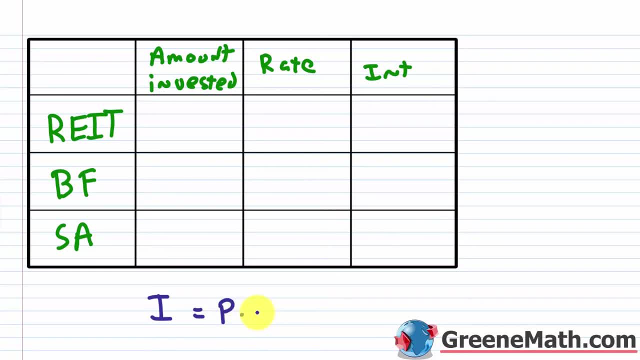 to P, which is the principal, okay, the amount invested times R, which is the rate as a decimal times the time In. generally speaking, this is going to be in years, okay, unless they tell you it's in months or something like that, but most of these problems it's going to be years. 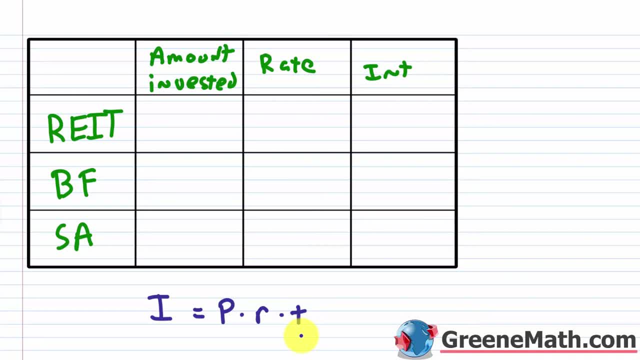 okay, We're talking about on an annual basis, so it's one year. So, because T would be a one, you can just drop it out and you could say that the interest earned- which is this column right here, okay, is going to be equal to the product of these. 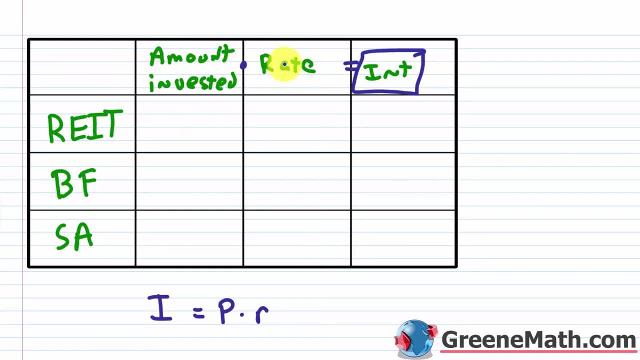 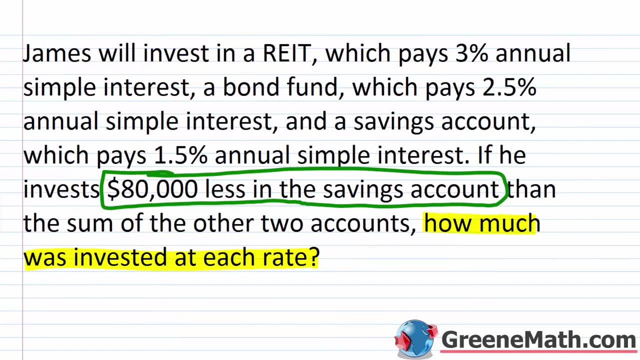 two, The amount invested, or the principal, multiplied by the rate. okay, as a decimal, okay. So let's erase this real quick and let's see if we can get this information. So specifically, it tells us the REIT pays 3% annual simple interest. 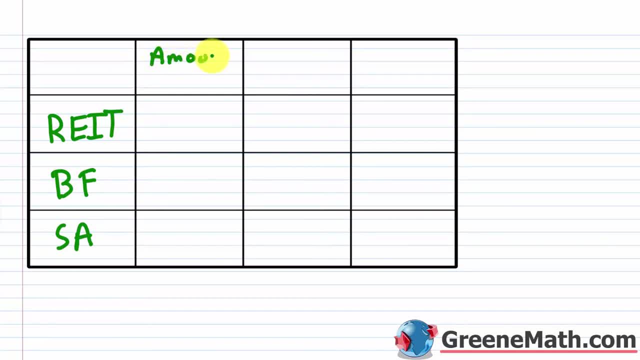 and then we're gonna have the amount invested, or you could say the principal. we're gonna have our rate, and this is as a decimal, and then we're gonna have our interest. okay, okay. so we're gonna have our interest and then we're gonna have our interest. 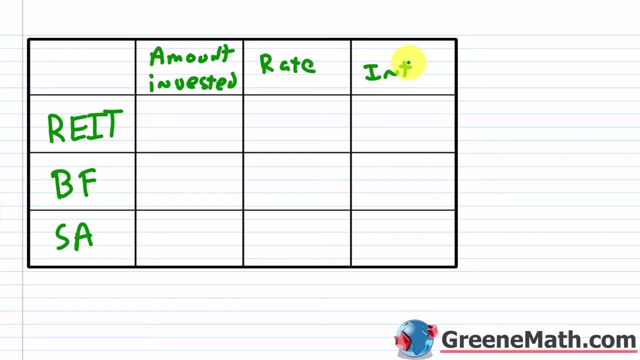 now we're working with simple interest. it's not compounding, okay. so most of you already know, because we talked about this earlier in the course, the simple interest formula is I, which stands for the amount of simple interest earned, is equal to P, which is the principal okay, the amount invested times R, which is the. 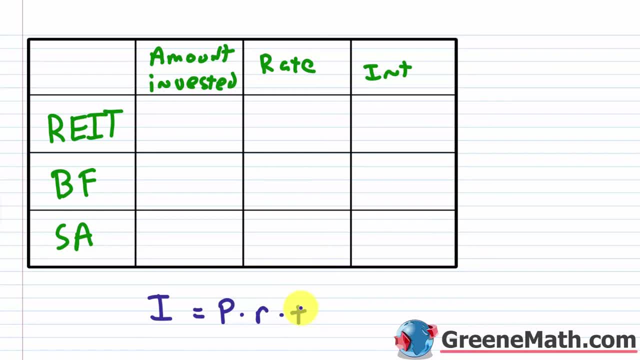 rate as a decimal times the time in. generally speaking, this is gonna be in years, okay, unless they tell you it's in months or something like that. but most of these problems it's gonna be years, okay. now, in this case we're talking about on an annual basis, so it's. 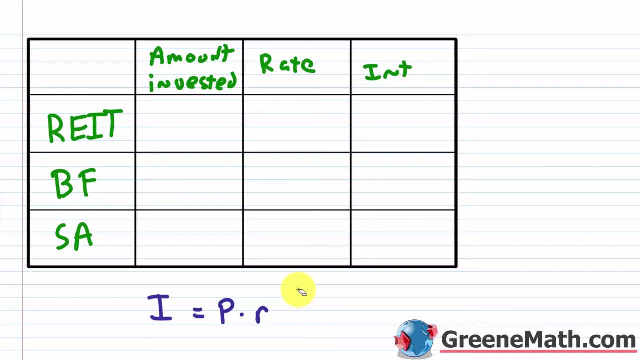 one year. so, because T would be a 1, you can just drop it out and you could say that the interest earned- which is this column right here, okay- is going to be equal to the product of these two, the amount invested, or the principal, multiplied by the rate. okay, as a decimal, okay. so let's erase this real quick and 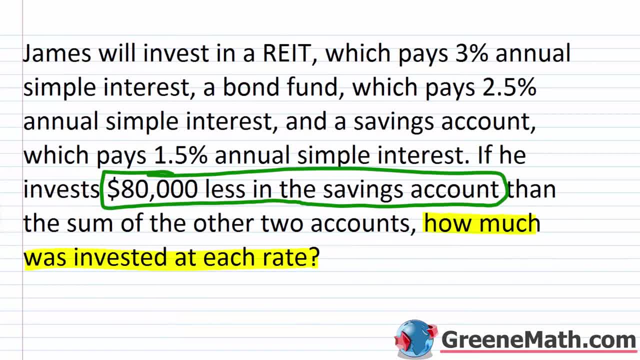 let's see if we can get this information so specifically. it tells us the REIT pays 3% annual simple interest, the bond fund pays 2.5% annual simple interest in and the savings account pays 1.5 annual simple interest. so for the rate for the REIT it's going. 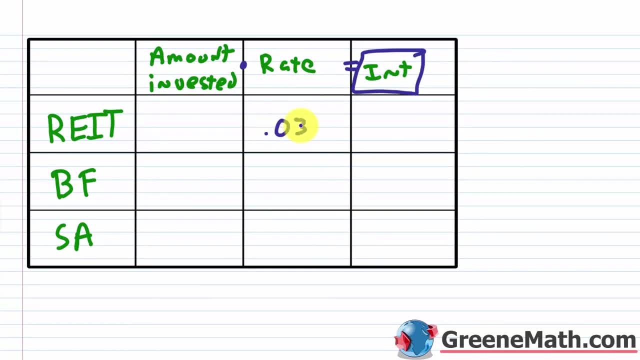 to be 3 or 0.03 as a decimal, and then for the bond fund it's going to be 2.5 or 0.025 as a decimal, and then for the savings account is 1.5 or 0.015 as a decimal. now for the amount invested. remember. 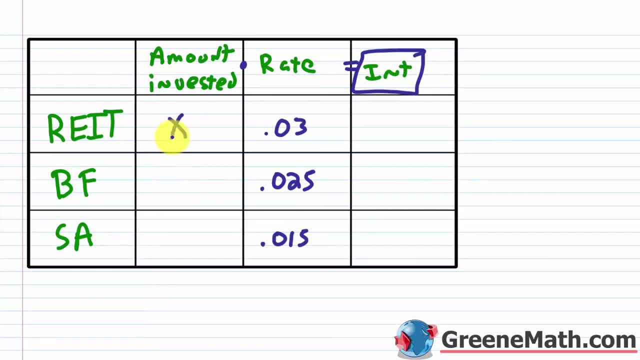 this is unknown. x is used to represent the amount invested in the REIT, y is used to represent the amount invested in the bond fund and z is used to represent the amount invested in the savings account. so, again, the product of these two would give me the simple interest earned over the course. 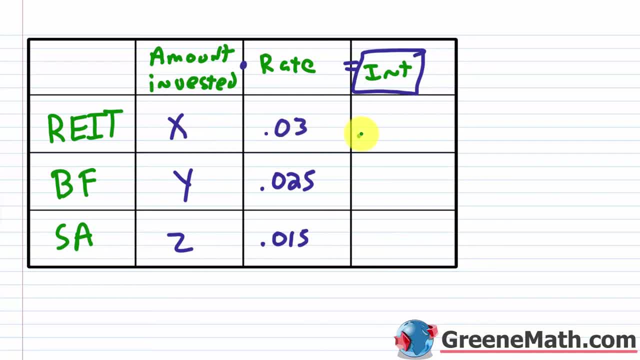 of a year. so point zero three times x. point zero three times x is the simple interest earned from the REIT. point zero two five times y- okay- is the simple interest earned from the bond fund. and point zero one five times z is the amount of simple interest earned from the savings account. 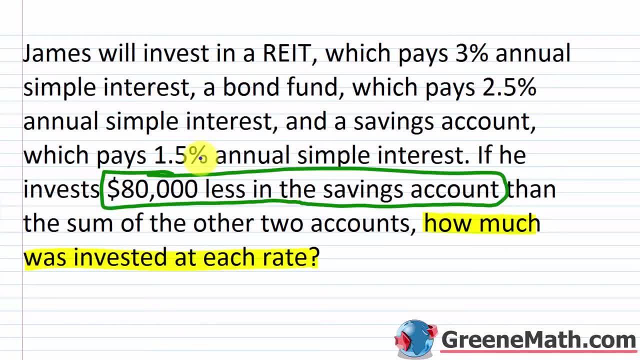 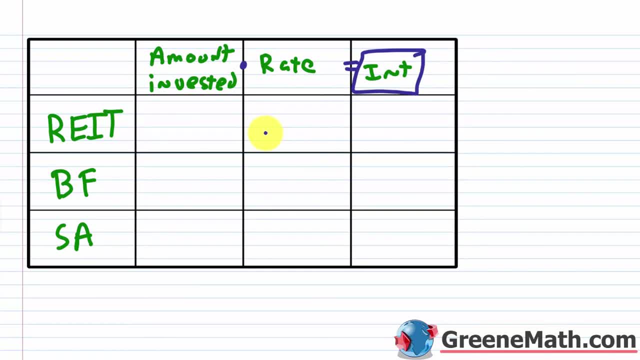 The bond fund pays 2.5% annual simple interest And the savings account pays 1.5% annual simple interest. So for the rate for the REIT it's going to be 3% or .03 as a decimal. 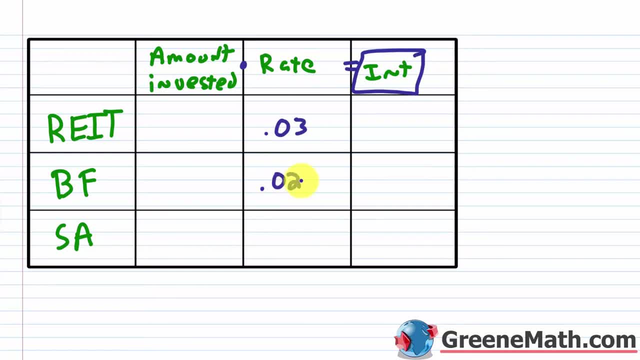 And then for the bond fund, it's going to be 2.5% or .025 as a decimal, And then for the savings account, it's 1.5% or .015 as a decimal. Now for the amount invested. remember, this is unknown. 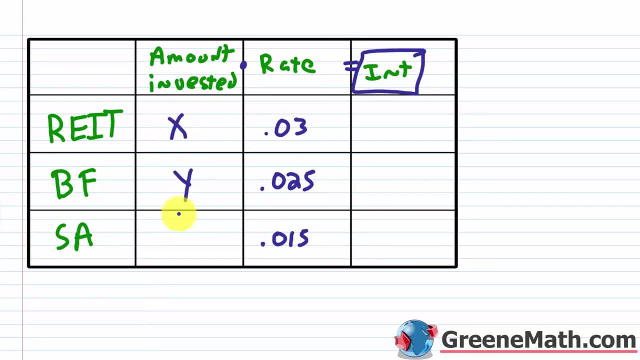 X is used to represent the amount invested in the REIT, Y is used to represent the amount invested in the bond fund And Z is used to represent the amount invested in the savings account. So again, the product of these two would give me the simple interest earned over the course. 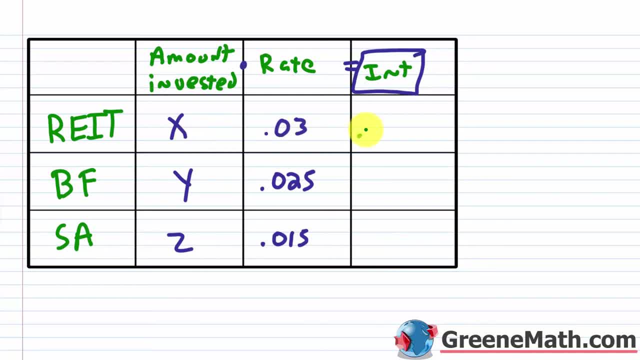 of a year, So .03 times X. .03 times X is the simple interest earned from the REIT, .025 times Y- okay- is the simple interest earned from the bond fund, And .015 times Z is the amount of simple interest earned from the savings account. 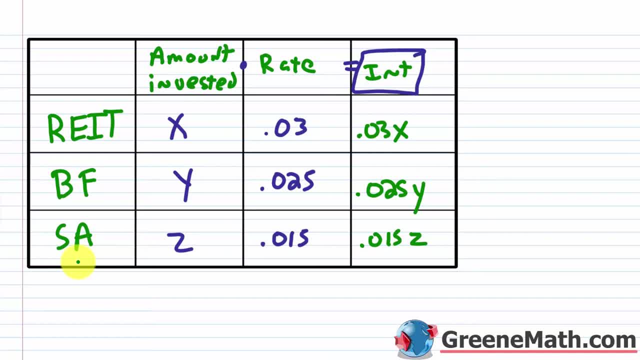 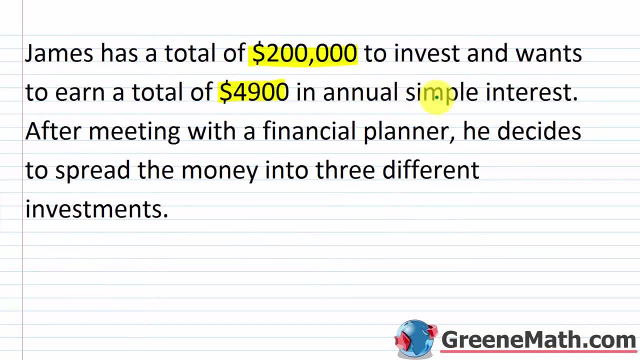 Now, what do we do with this information? How do we make an equation? Well, if you were paying attention to the first part of the problem, it tells us specifically: he wants to earn $4,900 in annual simple interest. Now the $4,900 can only come from these kind of three sources. 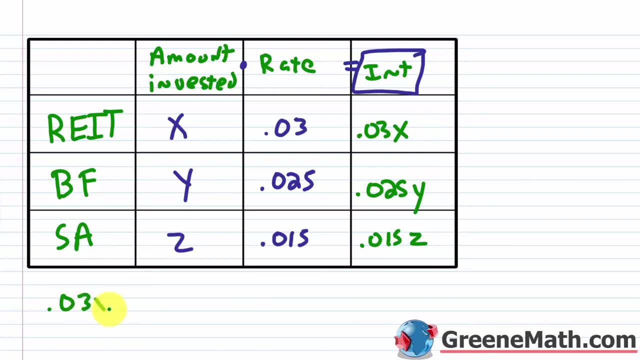 So I know that the interest from the REIT, which is .03X, plus the interest from the bond fund, which is .025Y, plus the interest from the savings account, which is .015Y, plus the interest from the bond fund, which is .025Y, plus the interest from the savings. 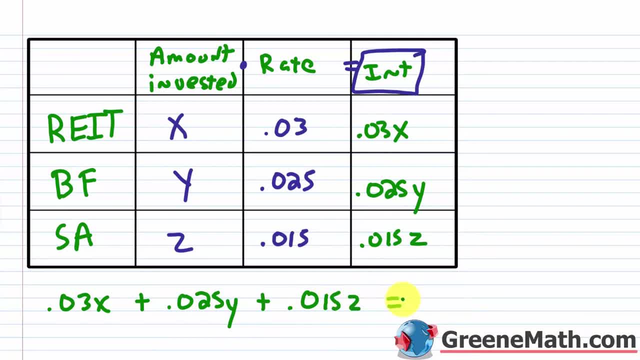 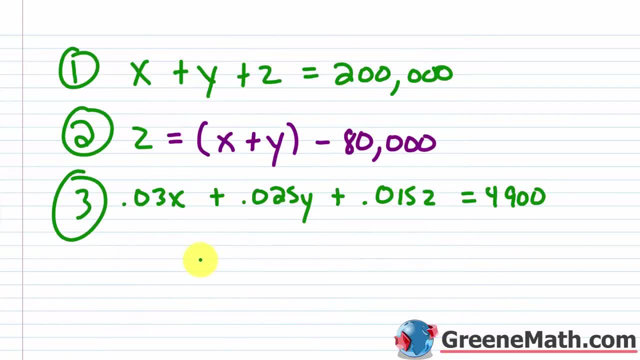 account, which is .015Z, has to be equal to that amount. okay, that $4,900.. So let's copy this. This is going to be our third equation. So, again, if you don't like working with decimals, you can clear them. 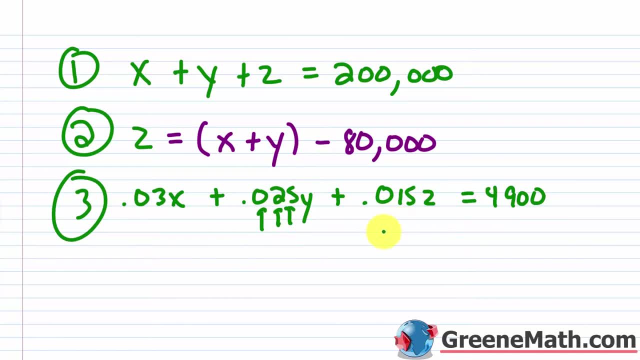 For this one you've got three decimal places here and here, so you've got to multiply everything by 1,000, okay, by 1,000.. So this guy would move three places to the right, so it would be 30X. 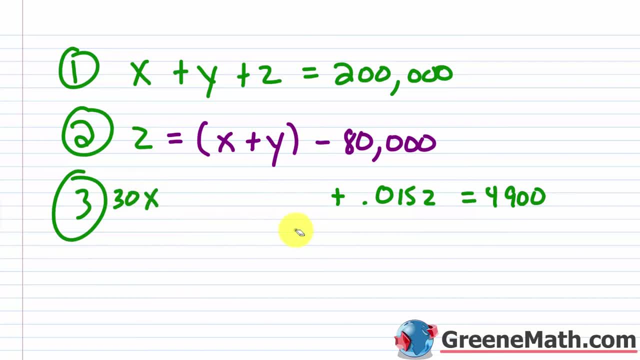 So it would be 30X. This guy would be 25Y, so plus 25Y. Then this guy would be 15Z, so plus 15Z, And then this guy again, if this is right here- let me kind of scooch this down- so we: 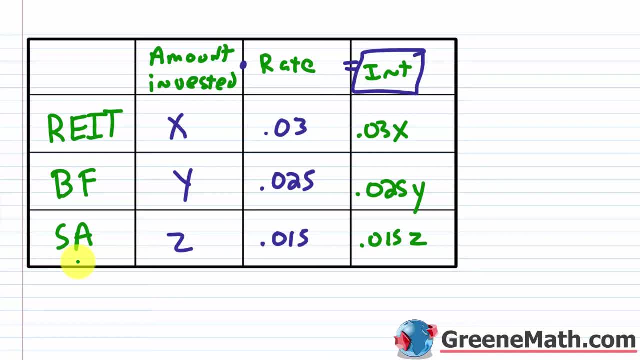 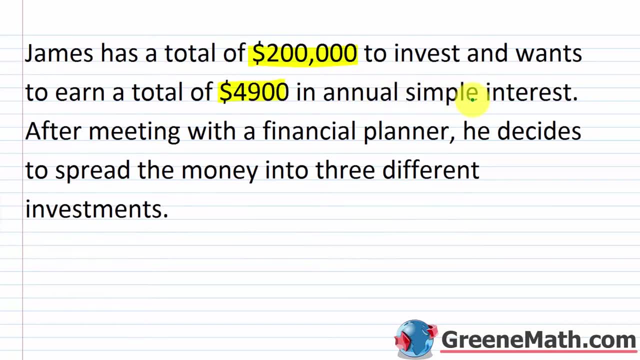 now, what do we do with this? for information, how do we make an equation? well, if you were paying attention to the first part of the problem, it tells us specifically: he wants to earn forty nine hundred dollars in annual simple interest. now, the forty nine hundred dollars can only come from these kind. 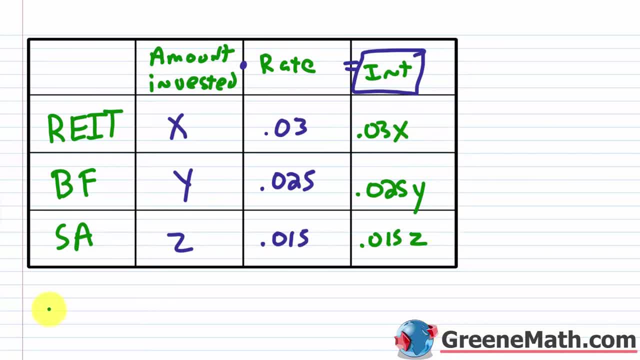 of three sources. so i know that the interest from the REIT, which is point zero, three x, plus the interest from the bond fund, which is point zero, two, five, y, plus the interest from the savings account, which is point zero, one, five z, has to be equal to that amount. okay, that four thousand nine hundred dollars. so let's copy this. 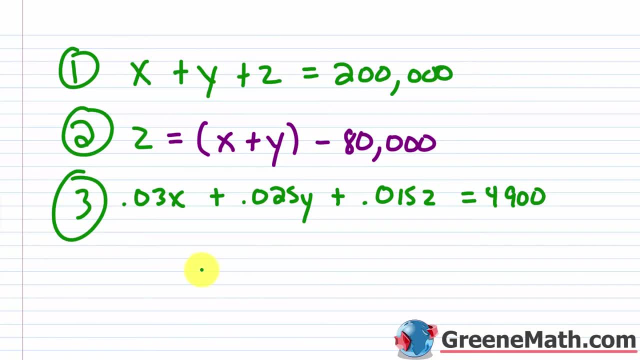 this is going to be our third equation. so again, if you don't like working with decimals, you can clear them. for this one you've got three decimal places here and here, so you've got to multiply everything by a thousand. okay, by a thousand. so this guy would move three places to the right, so it would be 30x. 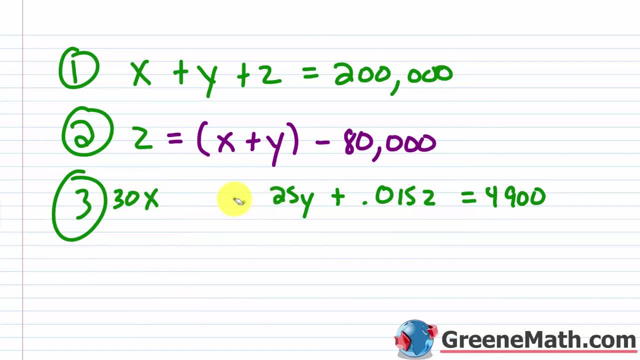 so it would be 30x. this guy would be 25y, so plus 25 y. then this guy would be 15 z, so plus 15 z, and then this guy again. if this is right here, let me kind of scooch this down so we have room. i'm moving everything three places to the right, so 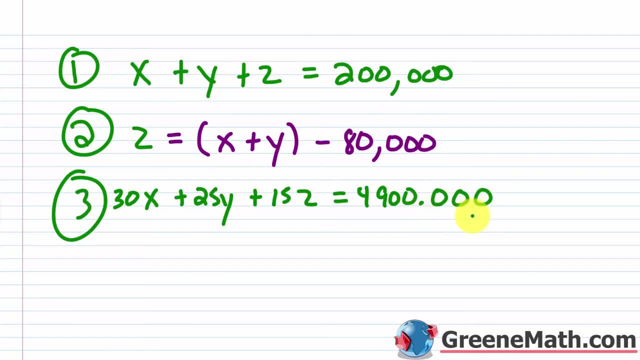 i put a zero here, a zero here and a zero here, this would go one, two, three places to the right, so it would end up with four million nine hundred thousand. okay, so now that we have our three equations, we can solve the system and figure out the answer now. 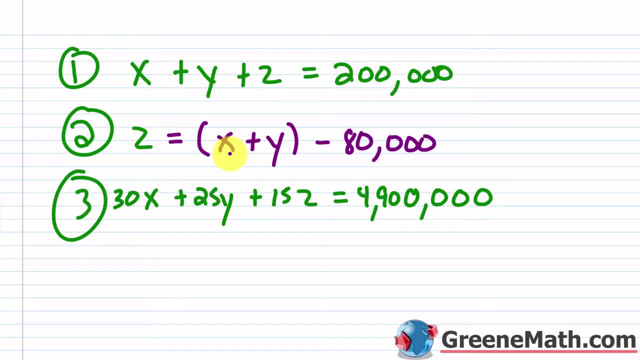 for equation two, you really want to set this up into the format of: you know, ax plus by plus cz equals d. okay, all the variables on one side, the number, the constant on the other. so i can really just drop the parentheses from here and essentially what i'd have is if i move each of 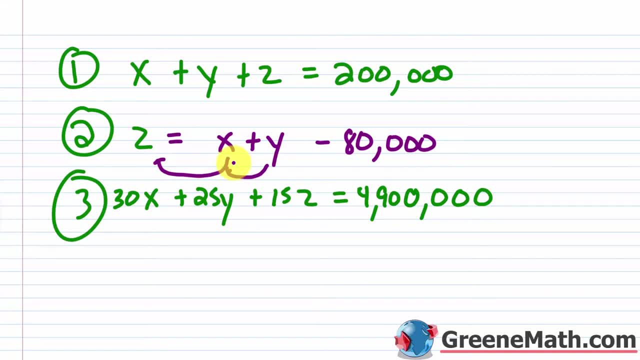 these over here. i would just subtract them away. i would have negative x minus y plus c. okay, so negative x, negative x minus y plus z is equal to- and it's going to be- negative eighty thousand. okay. so it's really easy to use elimination to get rid of either x or y from the kind of first. 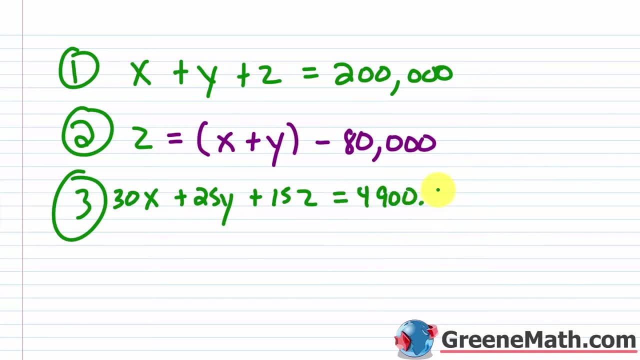 have room. I'm moving everything three places to the right, So I put a zero here, a zero here and a zero here. This would go one, two, three places to the right, So it would end up with $4,900,000, okay. 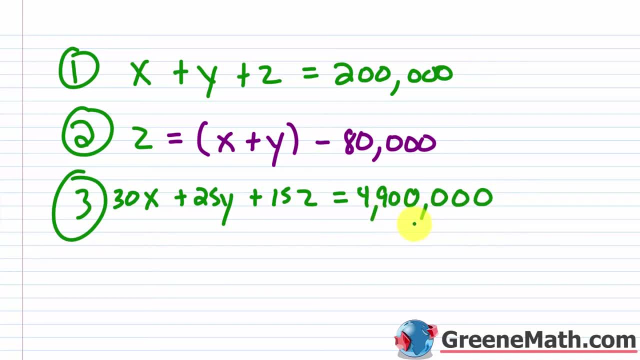 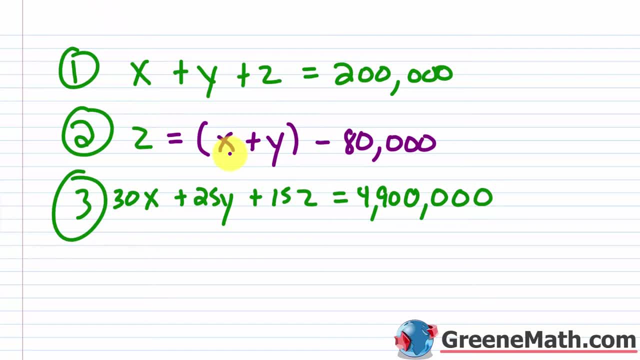 answer. Now for equation two. you really want to set this up into the format of: you know, AX plus BY, plus CZ equals D. okay, All the variables on one side, the number, the constant on the other. So I can really just drop the parentheses from here and essentially what I'd have is: 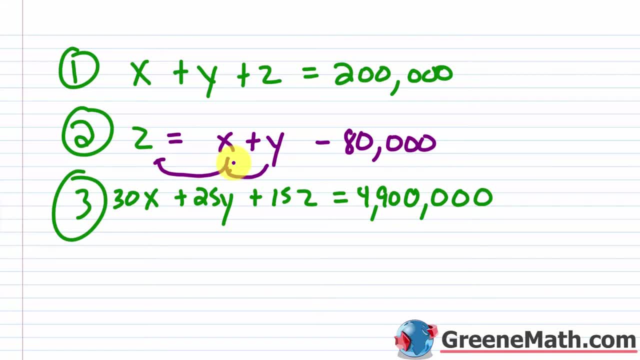 if I move each of these over here, I would just subtract them away. I would have negative X minus Y plus C. okay, So negative X, Negative X Minus Y Plus Z is equal to- and it's going to be negative- 80,000, okay. 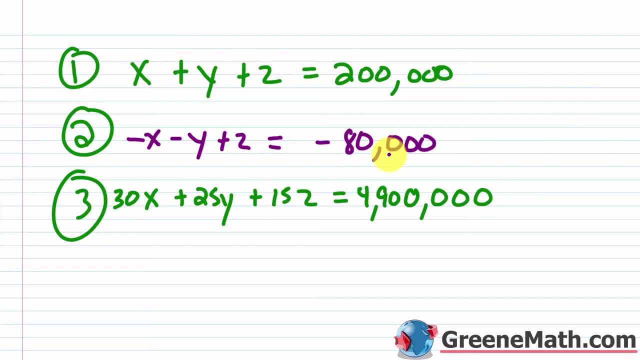 So it's really easy to use elimination to get rid of either X or Y from the kind of first two equations. So let's just choose to get rid of X. You'll notice that both of these are going to drop out. so it's going to be a nice easy. 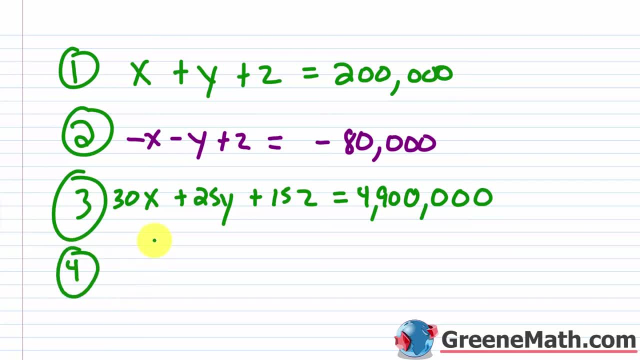 scenario for us. So for equation four, what I'm going to do is I'm going to add equation one and equation two together, So X plus negative X that's gone, Y plus negative Y that's gone, Z plus Z is 2Z. 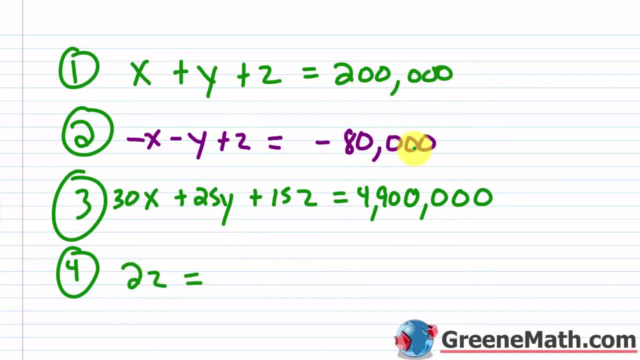 And this will be equal to 200,000 minus 80,000 is 120,000.. And, of course, if we divide both sides by two, we'd find that Z is equal to 60,000.. So we already know what Z is right, or the amount that he invests in the savings account. 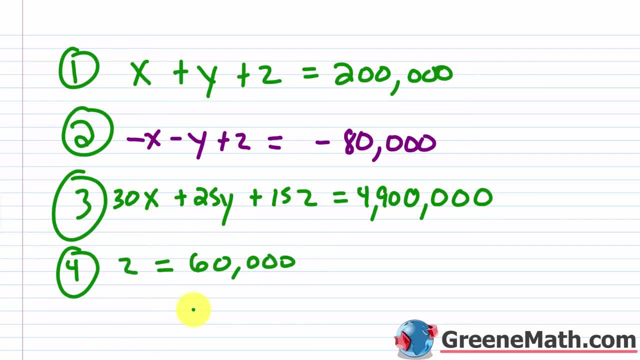 What about Y and X? So we're going to pick another two equations. So again, we can do one and three, or two and three, and we're going to eliminate. You can do either X or Y, It doesn't matter, You just eliminate either X or Y. 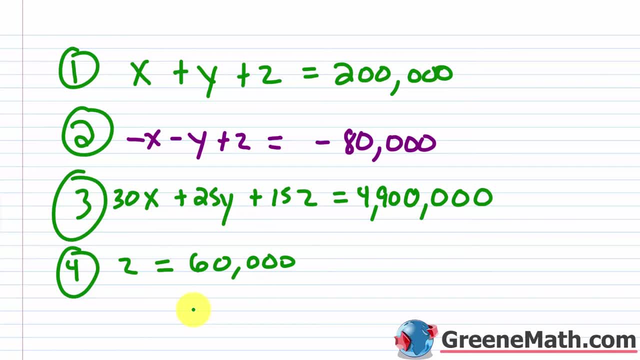 So that you can plug in for Z and figure out what the other one is and then back substitute again. So from two and three let me just go ahead and eliminate X. So let me scroll down and get some room going. So equation two: it's already negative, but let me multiply it by 30.. 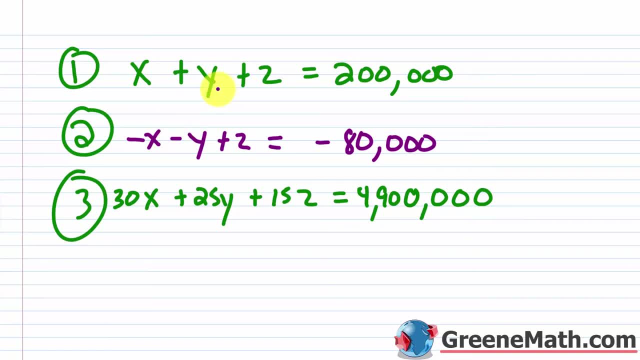 two equations. so let's just choose to get rid of x. you'll notice that both of these are gonna drop out, so it's gonna be a nice easy scenario for us. so for equation four, what i'm gonna do is i'm gonna add equation one and equation two together, so x plus negative x- that's gone, y plus negative y. 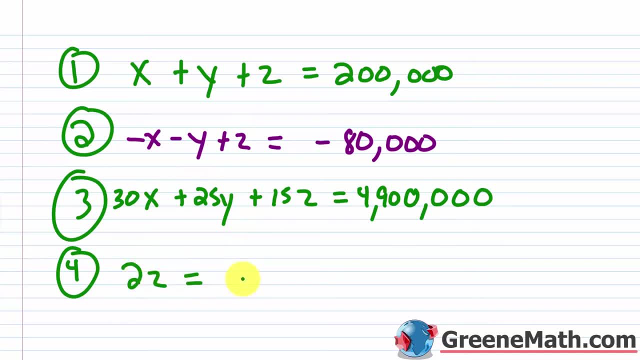 that's gone. z plus z is two z, and this will be equal to two hundred thousand minus eighty. 80,000 is 120,000. And, of course, if we divide both sides by two, we'd find that Z is equal to 60,000.. So we already know what Z is right, Or the amount that he invests in the savings account. 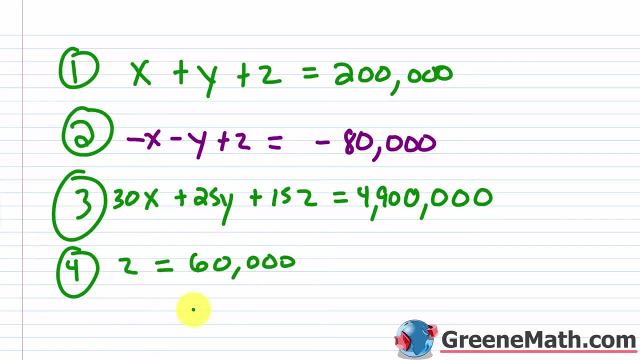 What about Y and X? So we're going to pick another two equations. So again, we can do one and three, or two and three, and we're going to eliminate. you can do either X or Y, It doesn't matter, You just eliminate either X or Y so that you can plug in for Z and figure out what the 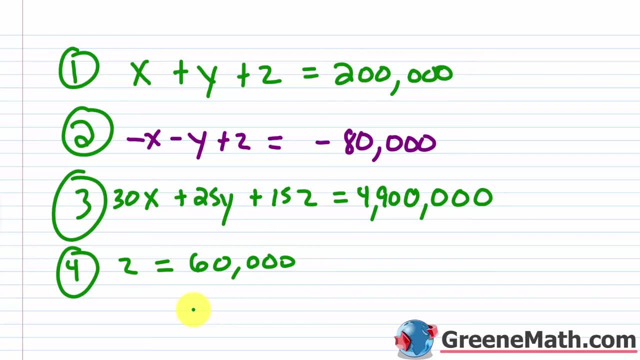 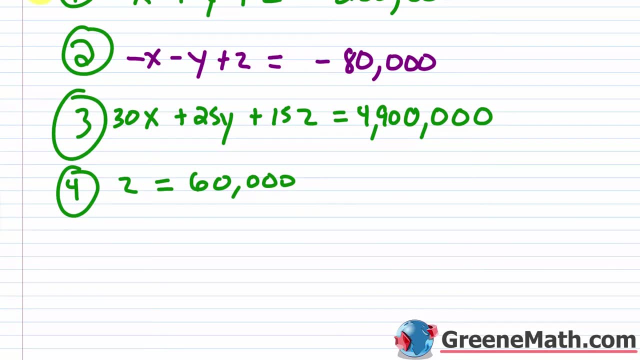 other one is, and then back substitute again. So from two and three let me just go ahead and eliminate X. So let me scroll down and get some room going. So equation two: it's already negative, but let me multiply it by 30. So I would have negative 30X minus 30Y plus 30Z, And this equals. 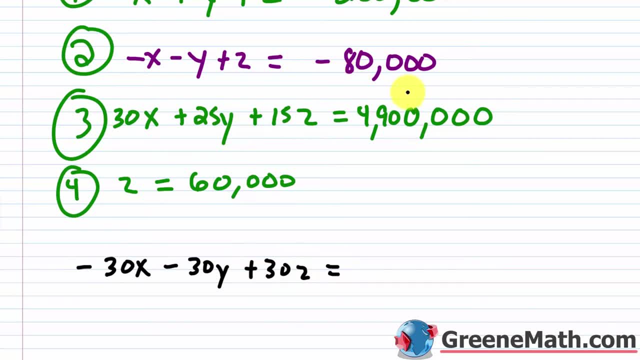 if I took negative 80,000 and multiplied it by 30,, negative eight times three is negative 24. And then I have this many zeros, So one, two, three, four, and then I'd add one more zero, So this would end up. 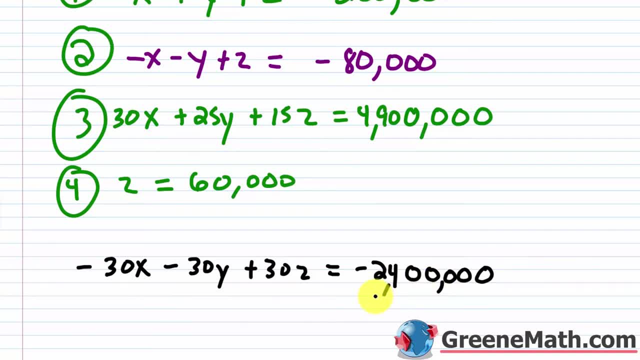 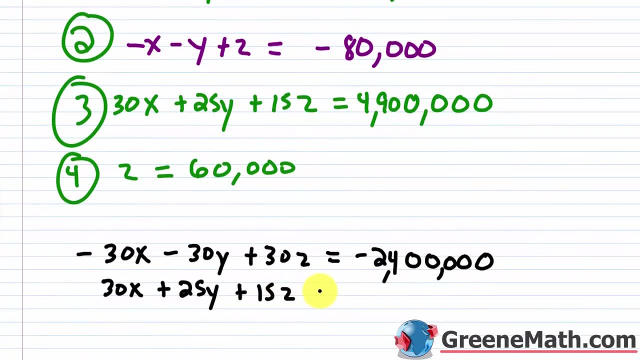 being negative 2,400,000.. Okay, So then I'm just going to copy equation three as it is. So 30X plus 25Y plus 15Z equals 4,900,000.. Okay, So let me scroll down and get some room going. 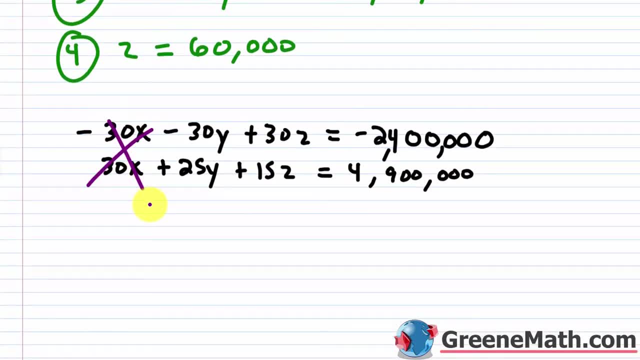 And we know that this is going to go away. Negative 30Y plus 25Y is going to be negative 5Y, And then plus 25Y is going to be negative 5Y, And then plus 25Y is going to be negative 5Y. 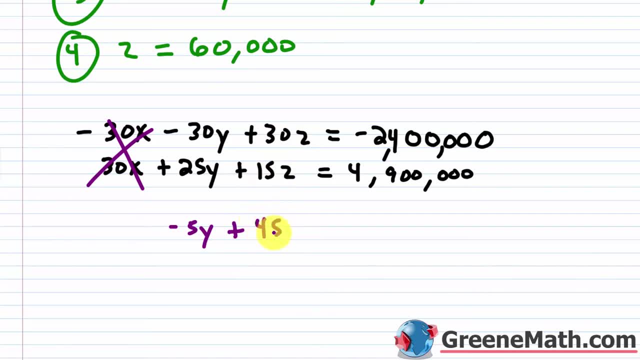 And then plus 30Z, plus 15Z is going to be 45Z, And this equals: if I take negative 2,400,000 and add that to 4,900,000, I'm going to get 2,500,000.. Okay, And we'll call this equation five. 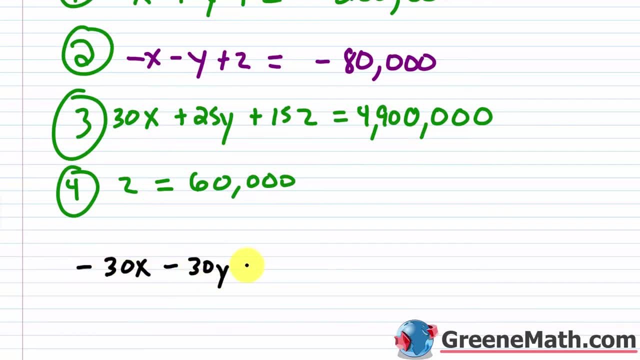 So I would have negative 30 X minus 30 Y plus 30 Z, And this equals, if I took negative 80,000 and multiply it by 30.. Negative eight times 30.. Negative three is negative 24.. And then I have this many zeros. 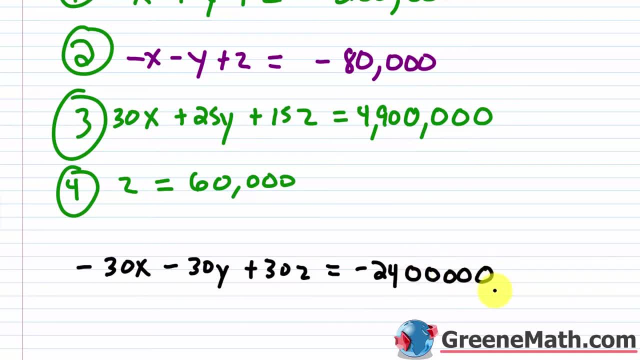 So one, two, three, four, and then I add one more zero, So this would end up being negative 2,400,000.. So then I'm just going to copy equation three as it is. So 30 X plus 25 Y plus 15 Z equals 4,900,000. 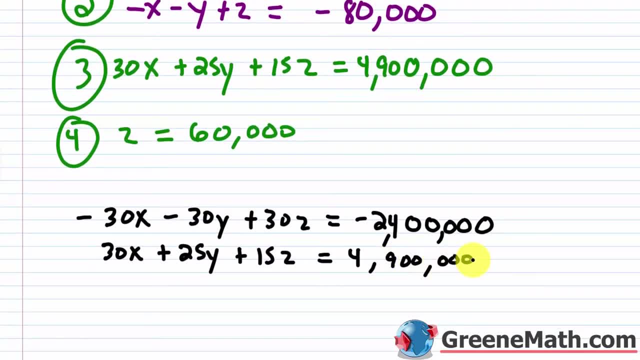 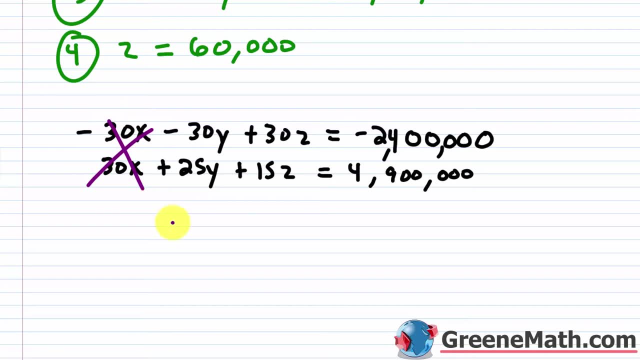 Let me scroll down and get some room going, and we know that this is going to go away. Negative 30. plus 25Y is going to be negative 5Y, And then plus 30Z, plus 15Z is going to be 45Z, And this: 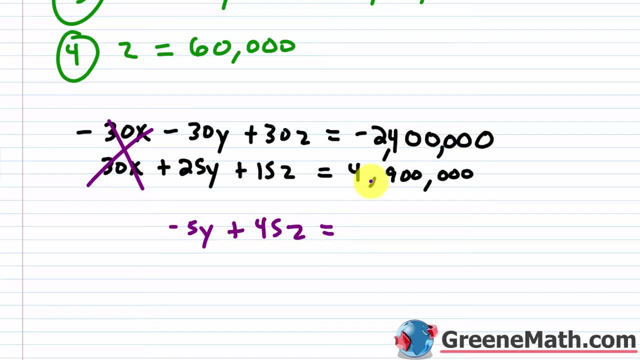 equals. if I take negative 2,400,000 and add that to 4,900,000, I'm going to get 2,500,000.. Okay, And we'll call this equation five. Again, I already know what Z is, So what I'm going to do. 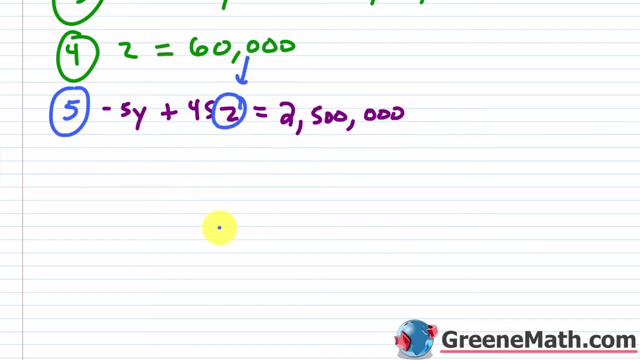 is. I'm going to plug in for Z here. It's going to plug that in and I'm going to find out what Y is. So I have negative 5Y plus 45 times 60,000.. Okay Is equal to 2,500,000.. Okay, So 45 times 60,000. 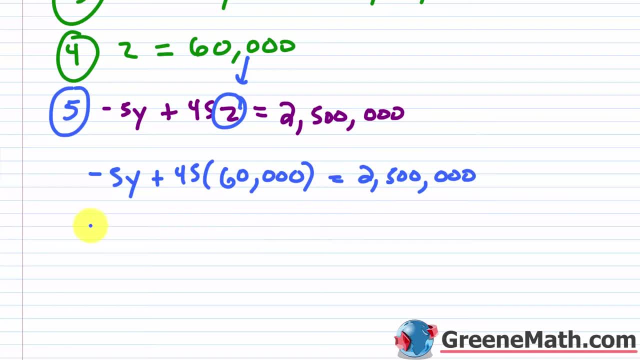 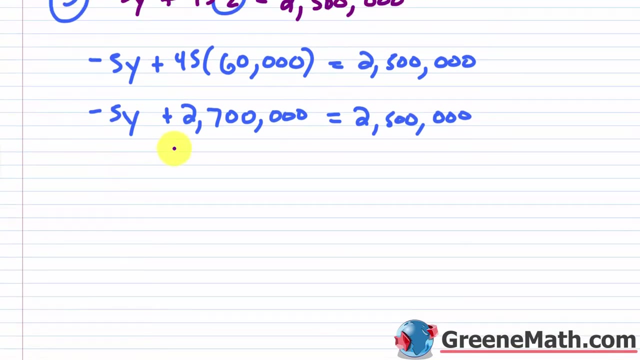 is 2,700,000.. So I would have negative 5Y plus 2,700,000.. Okay, And this equals 2,500,000.. Okay, Let me scroll down a little bit So we already know. if I said, 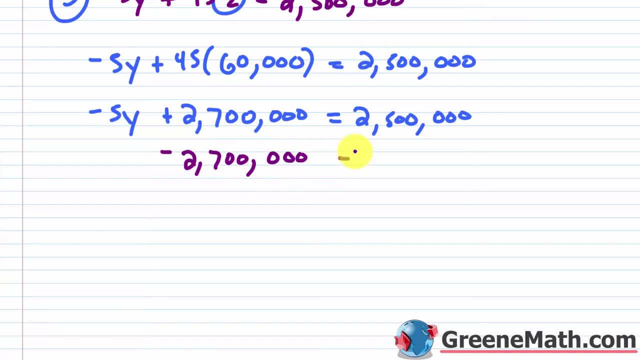 subtract 2,700,000 away from each side, this is going to cancel. I'll have negative. 5Y is equal to 2,500,000, minus 2,700,000 is going to give me negative 200,000.. So negative 200,000.. If we then divide both sides by negative. 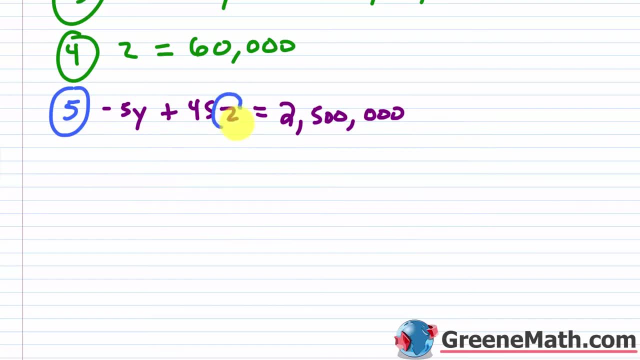 Again, I already know what Z is. So what I'm going to do is I'm going to plug in for Z here. It's going to plug that in and I'm going to find out what Y is. So I have negative 5Y plus 45 times. 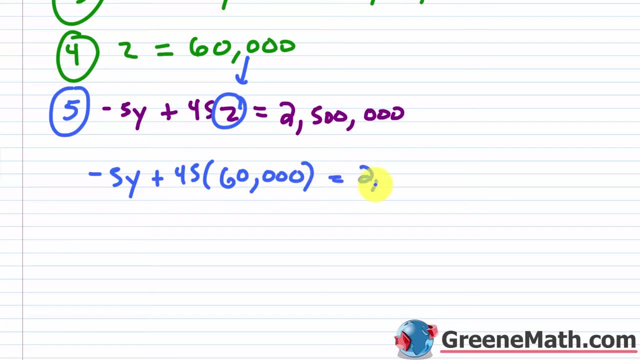 60,000.. Okay, Is equal to 2,500,000.. Okay, So I'm going to plug that in and I'm going to plug that in 2,500,000.. Okay, So 45 times 60,000 is 2,700,000.. So I would have negative 5Y. 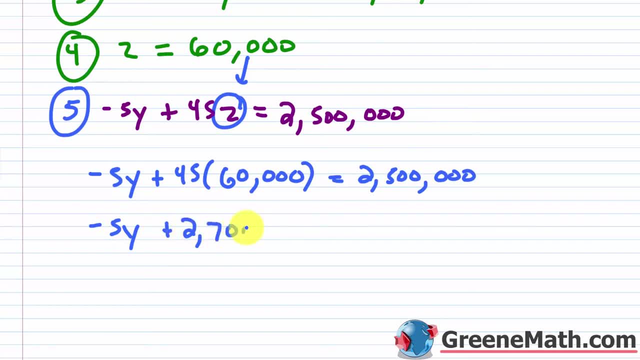 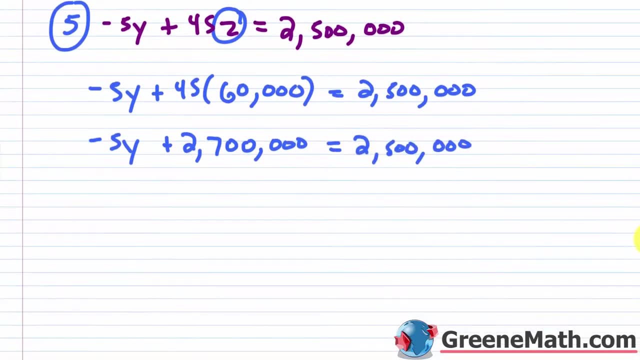 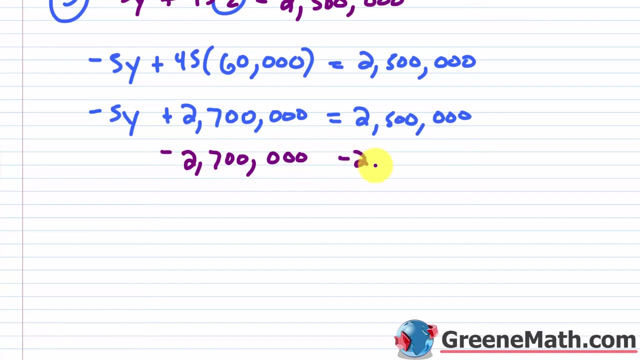 plus 2,700,000.. Okay, And this equals 2,500,000.. Let me scroll down a little bit So we already know. if I subtract 2,700,000 away from each side, this is going to cancel. I'll have negative. 5Y is equal to 2,500,000 minus 2,700,000. 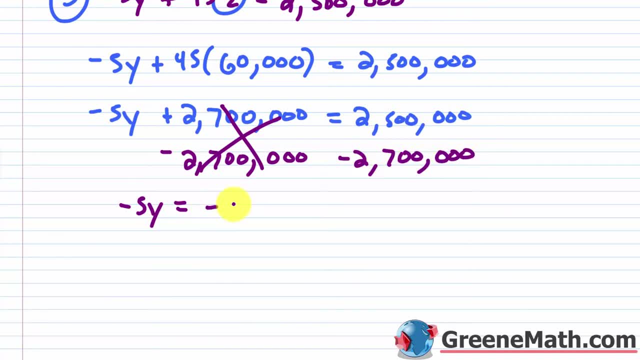 is going to give me negative 200,000.. So, negative 200,000.. If we then divide both sides by negative five, I'm going to find that Y is equal to 40,000.. Okay, 40,000.. So what's X going to be? Well, 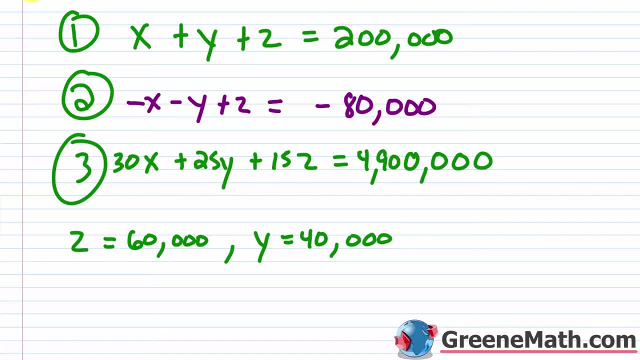 if I just plug into this first equation, which is pretty easy to work with, I can easily find out that X is going to be 40,000.. So what's Y going to be? Well, if I just plug into this first equation, 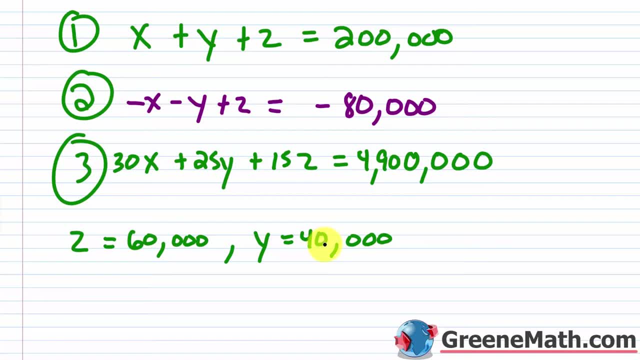 it's going to be 100,000, right. And you can eyeball that and see 60 plus 40 is 100, right. So it's going to be a hundred grand. And then if you had 200 there while missing a hundred right. 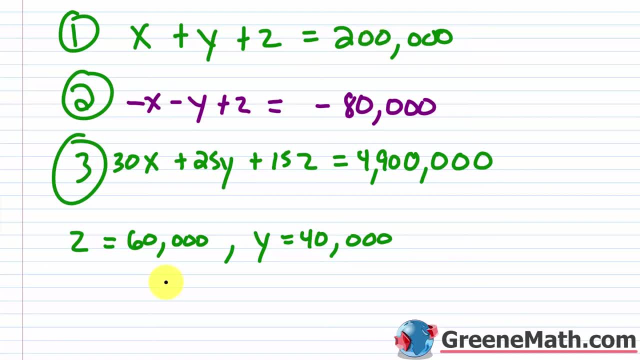 That's how I did it in my head, But again, you can plug it in, It doesn't matter. So X plus Y is 40,000, plus you have your Z, which is 60,000.. This equals 200,000.. And again, you know that. 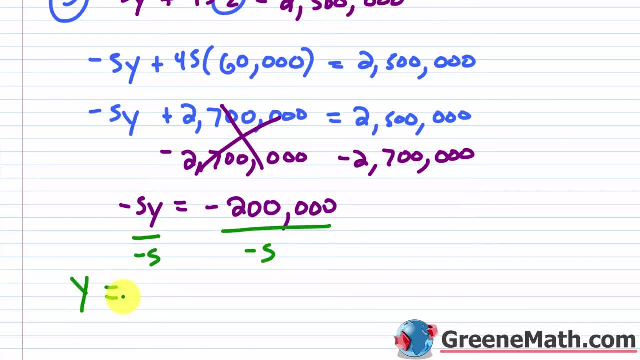 five, I'm going to find that Y is equal to 40,000.. Okay, 40,000.. So what's the difference between negative 5Y and negative 5Y? Well, I'm going to find that Y is equal to 2,700,000.. Okay, So what's X going to be? Well, if I just plug into this first, 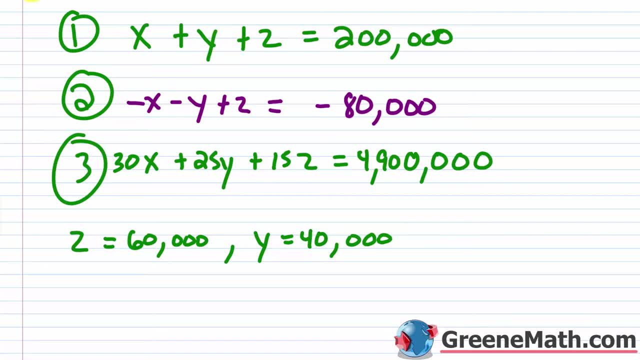 equation which is pretty easy to work with. I can easily find out that X is going to be a hundred thousand, right? And you can eyeball that and see: 60 plus 40 is a hundred, right, So it's going to be a hundred grand. And then if you had 200 there while missing a hundred right? 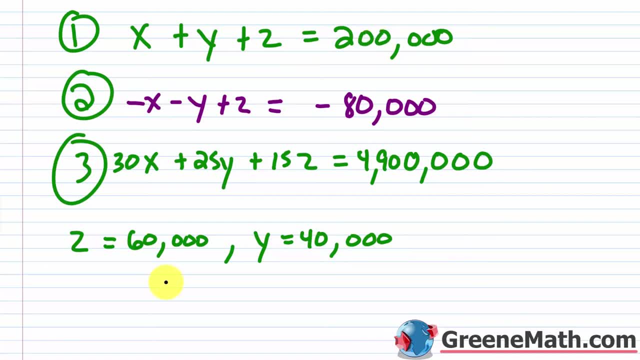 That's how I did it in my head, But again, you can plug it in, It doesn't matter. So X plus Y is 40,000, plus you have your Z, which is 60,000.. This equals 200,000.. 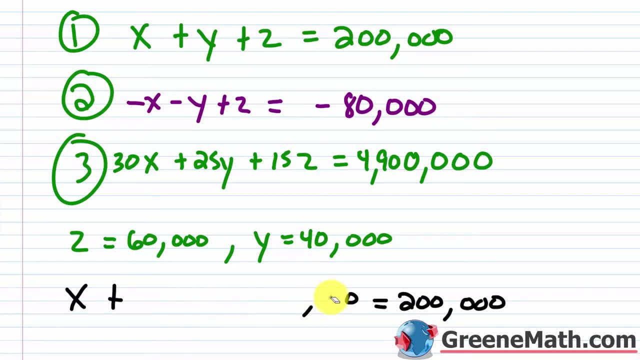 And again, you know that this sum here, 40,000 plus 60,000- is a hundred thousand. So this is a hundred thousand here, And if I subtract a hundred thousand away from each side, this goes away from here, and over here on the right it's going to be a hundred thousand. Okay. 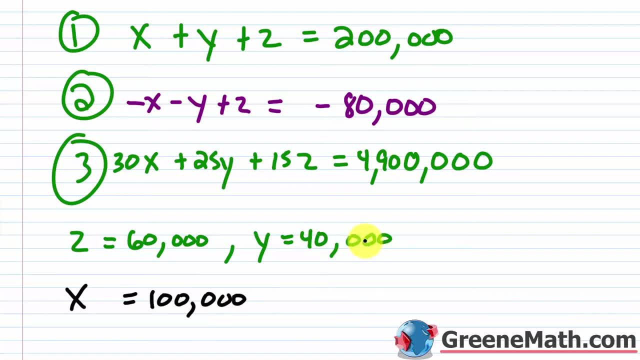 So we get that X is a hundred thousand, Y is 40,000.. Z is 60,000.. So that means that he invests a hundred thousand in the REIT, He invests 40,000 in the bond fund and then 60,000. 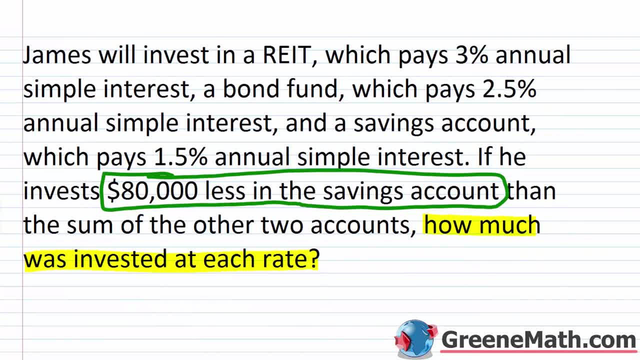 in the savings account, All right, So let's write that real quick. I'm going to make a nice little concise answer and just say that he invests $100,000 in the REIT, or again the real estate investment trust. 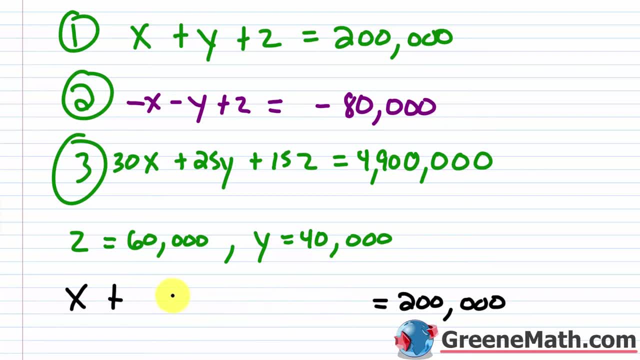 this sum here, 40,000 plus 60,000, is a hundred thousand. So this is a hundred thousand here, And if I subtract a hundred thousand away from each side, this goes away from here and over here on the right, it's going to be a hundred thousand. Okay, So we get that. X is a hundred thousand. 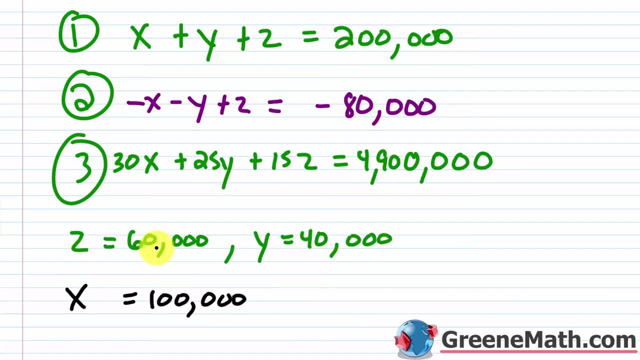 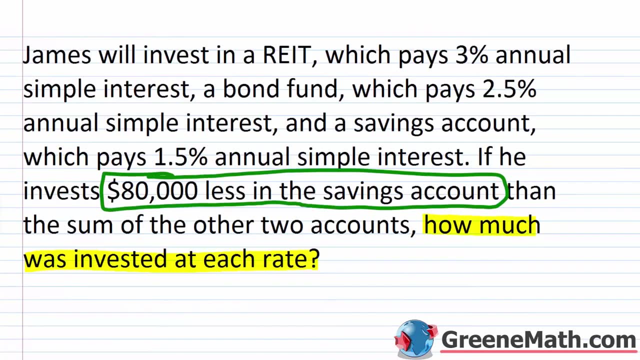 Y is 40,000.. Z is 60,000.. So that means that he invests a hundred thousand in the REIT, He invests 40,000 in the bond fund and then 60,000 in the savings account. All right, So let's write that. 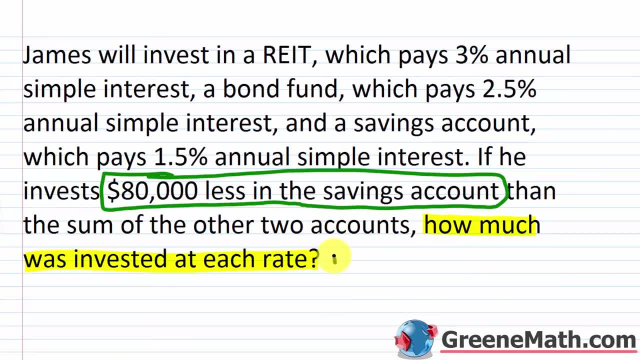 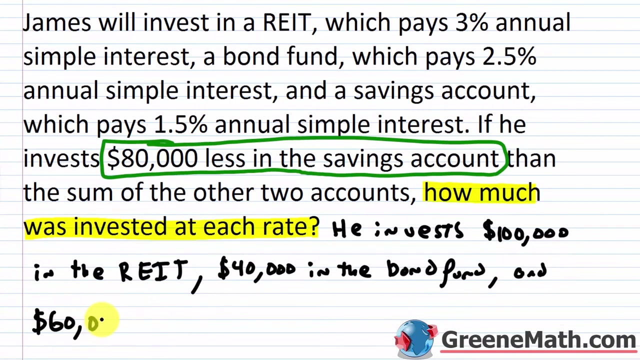 real quick And I'm going to make a nice little concise answer and just say that he invests $100,000 in the REIT or again the real estate investment trust, And then he put $40,000 in the bond fund And he put $60,000 in the savings account. 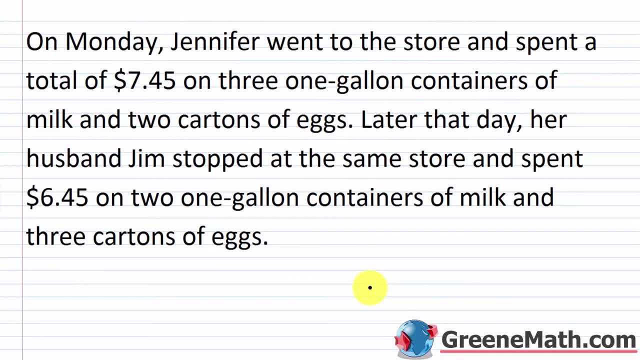 All right For the last problem. we have that on Monday, Jennifer went to the store and spent a total of $7 and 45 cents on three one gallon containers of milk and two cartons of eggs. Later that day, her husband, Jim, stopped at the same store and spent $6 and 45 cents. 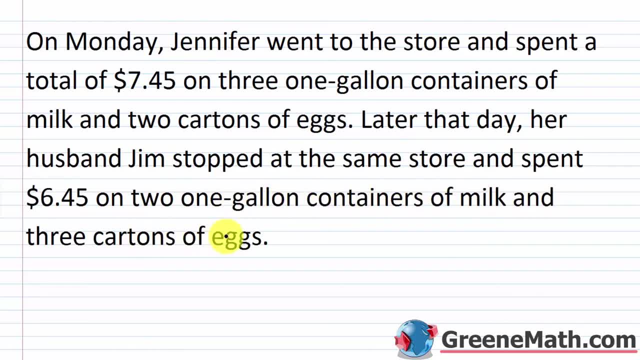 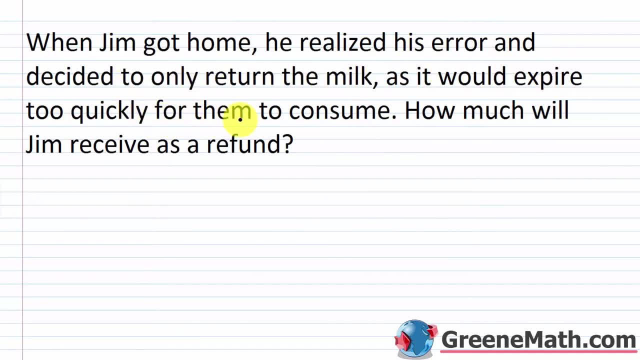 on two one gallon containers of milk and three cartons of eggs. When Jim got home, he realized his error and decided to only return the milk, as it would expire too quickly for them to consume. How much will Jim receive as a refund? Okay, So this is what we're trying to. 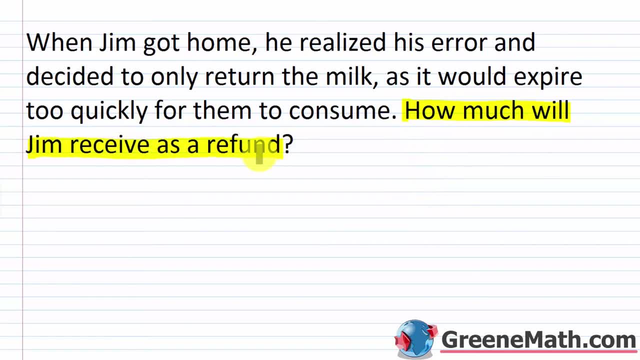 figure out How much will Jim receive as a refund? Now, this is given the fact that he's only going to return the milk. Okay, He's not returning the eggs, He's just returning the milk, And we don't know the individual prices for anything. We're only told that. you know, Jennifer goes to the. 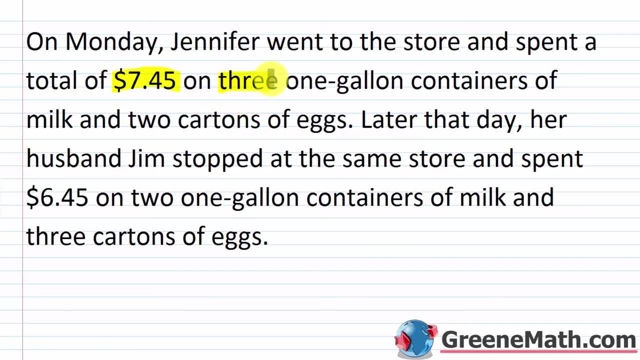 store and she spends $7 and 45 cents on three one gallon containers of milk and two cartons of eggs, And then later on Jim goes to the same store. Okay, So we're going to assume it's the same price for the milk and the. 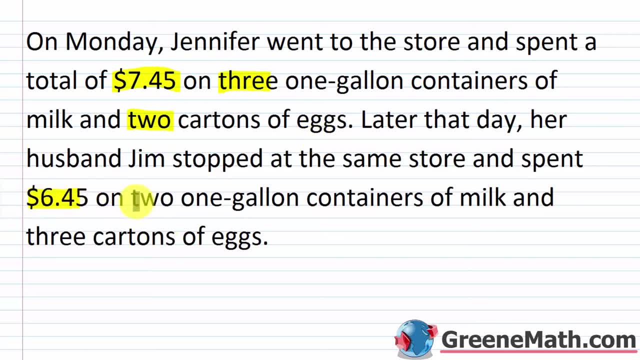 eggs And he spends $6 and 45 cents. He only buys two one gallon containers of milk and three cartons of eggs. Okay, So we've got to figure this out with a system of equations. The unknowns here are going to be the cost for a one gallon container of milk and the cost for one carton of eggs. 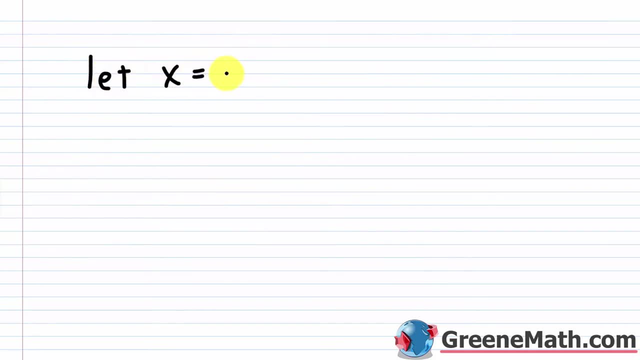 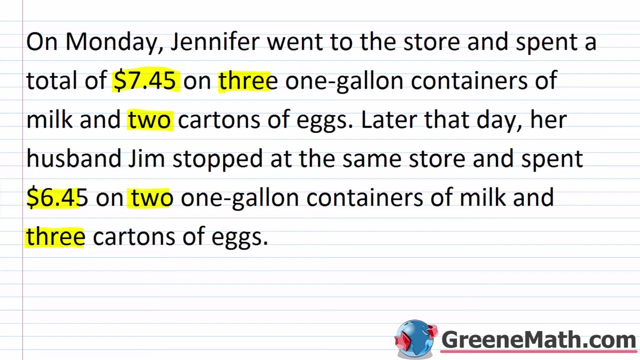 So let's let X be equal to the cost for one gallon, and this is a one gallon container of milk, And then Y can be the cost in each of these. 1 gallon pads has a cost of the first eggs, And then what does the cost of? 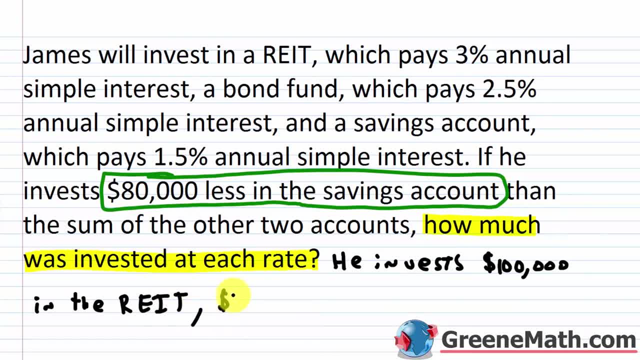 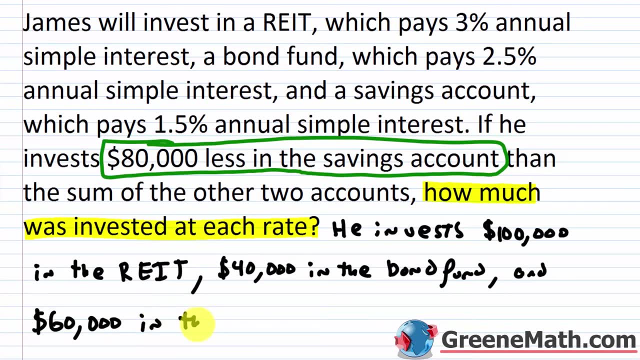 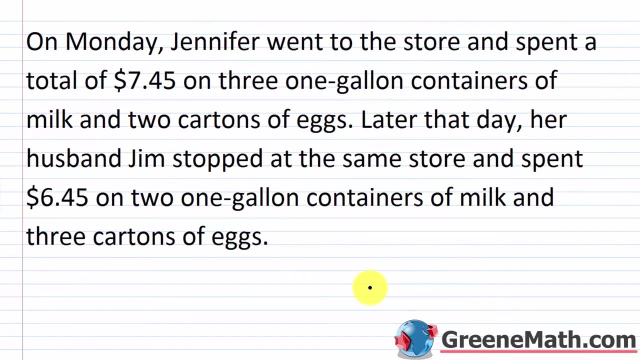 And then he put $40,000 in the bond fund And he put $60,000. in the savings account. All right, for the last problem, we have that on Monday Jennifer went to the store and spent a total of $7.45. 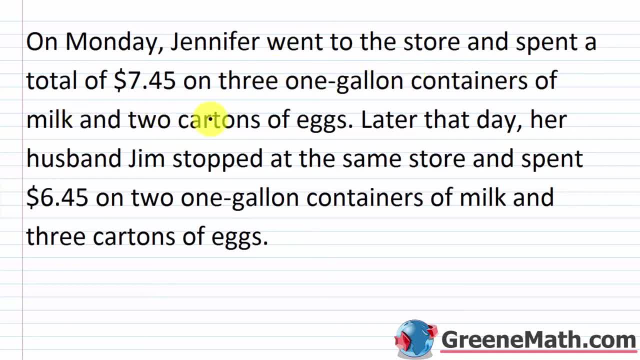 on three one-gallon containers of milk and two cartons of eggs. Later that day, her husband, Jim, stopped at the same store and spent $6.45 on two one-gallon containers of milk and three cartons of eggs. When Jim got home, he realized his error. 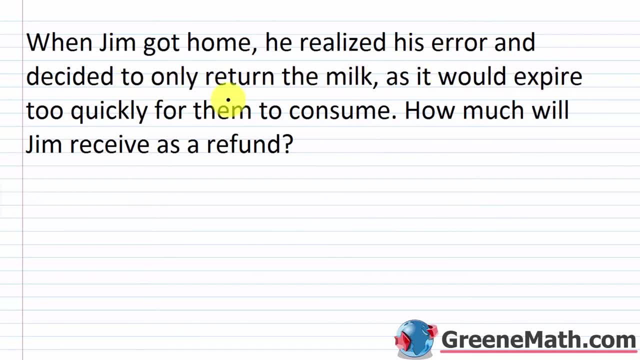 and decided to only return the milk as it would expire too quickly for them to consume. How much will Jim receive as a refund? okay, So this is what we're trying to figure out: How much will Jim receive as a refund Now? this is given the fact. 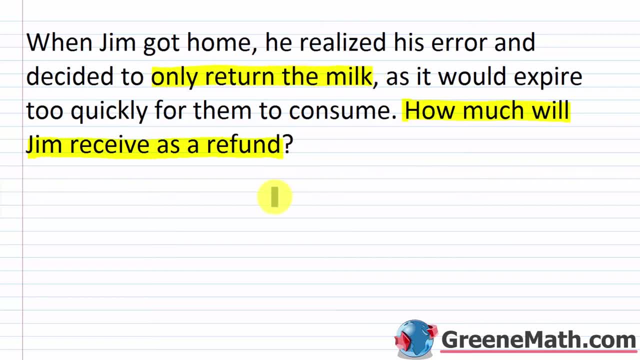 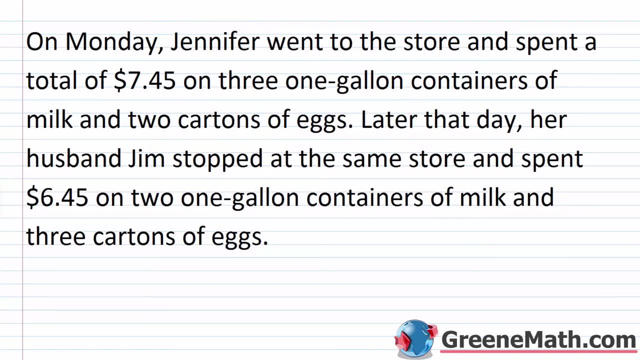 that he's only going to return the milk. okay, He's not returning the eggs, he's just returning the milk. And we don't know the individual prices for anything. We're only told that. you know, Jennifer goes to the store. 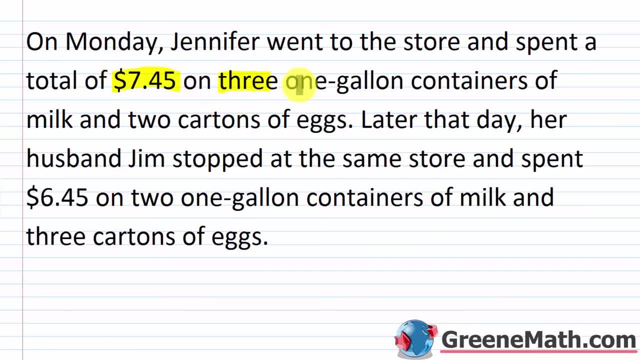 and she spends $7.45,- $7.45 on three one-gallon containers of milk and two cartons of eggs, And then later on Jim goes to the same store. okay, So we're going to assume it's the same price. 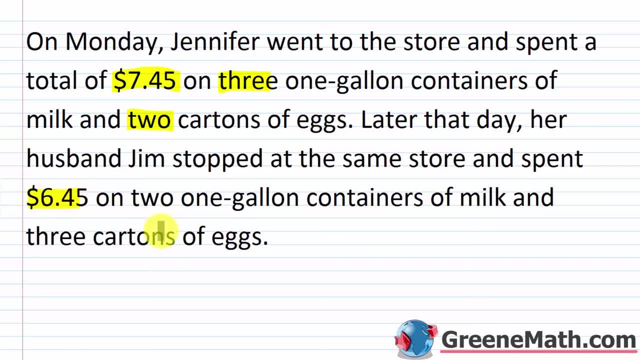 for the milk and the eggs, And he spends $6.45.. He only buys two one-gallon containers of milk and three cartons of eggs. okay, So we've got to figure this out with a system of equations. The unknowns here are going to be: 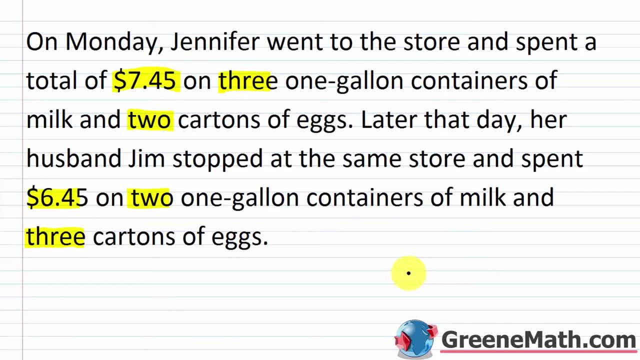 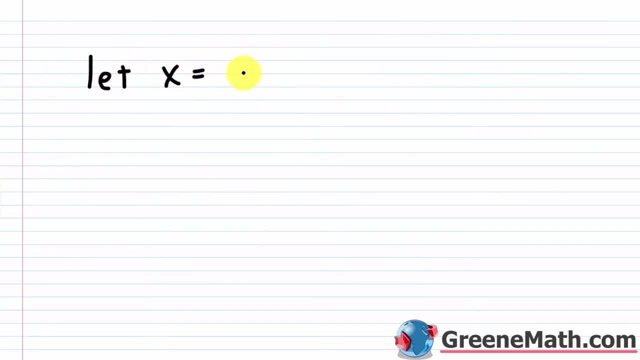 the cost for a one-gallon container of milk and the cost for one carton of eggs. So let's let X be equal to the cost for one gallon, okay, And this is a one-gallon container of milk, And then Y can be the cost for one carton of eggs, okay. 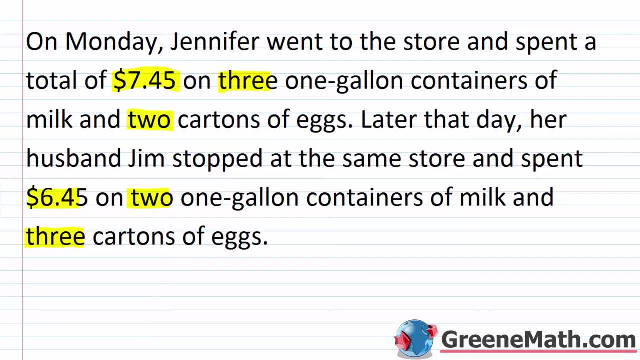 So what can we do with this? Let's go back up So we know that Jennifer spent $7.45 on three one-gallon containers of milk and two cartons of eggs. So the way we can model this, since X is the cost of one gallon of milk. 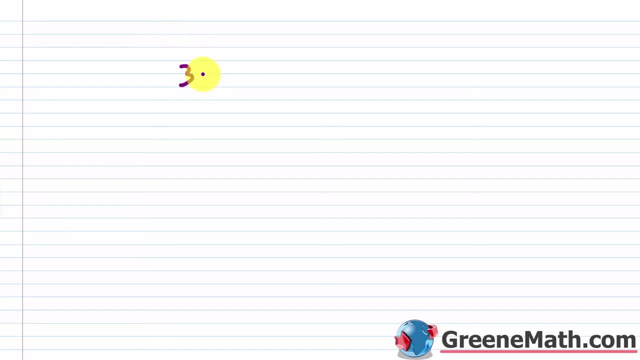 and she bought three of them, then three times X would be the amount she spent on milk. Then, plus, you have the fact that she buys two cartons of eggs. okay, so two cartons of eggs. Why is the cost of one carton of eggs? 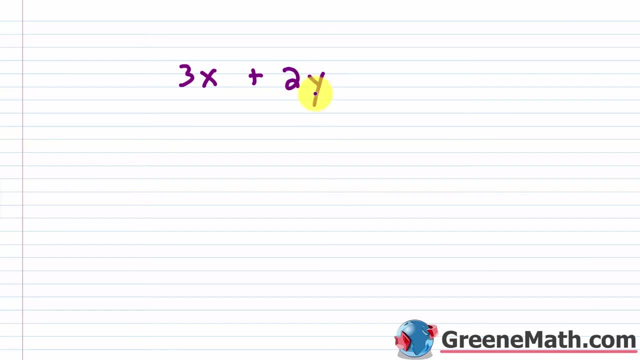 So two times Y would give me the cost for eggs in that kind of transaction. And again, if I sum these two amounts together, I get the amount she spent, which is $7.45,. okay, Again, you can clear the decimal if you want. 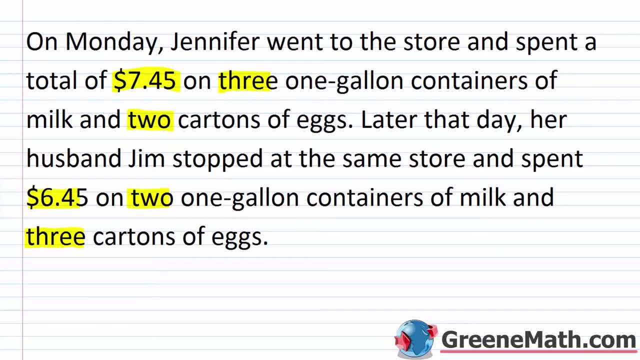 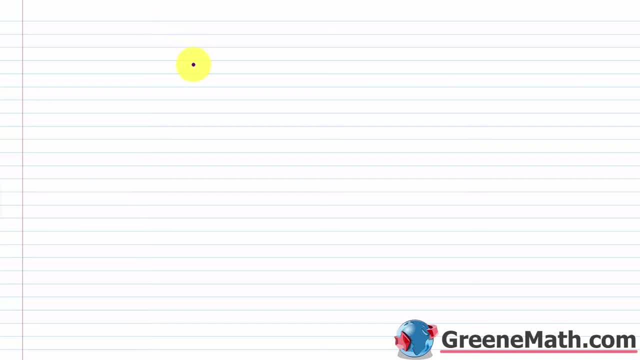 share be for Arizona: gallon containers of milk and two cartons of eggs. So the way we can model this, since X is the cost of one gallon of milk and she bought three of them, then three times X would be the amount she. 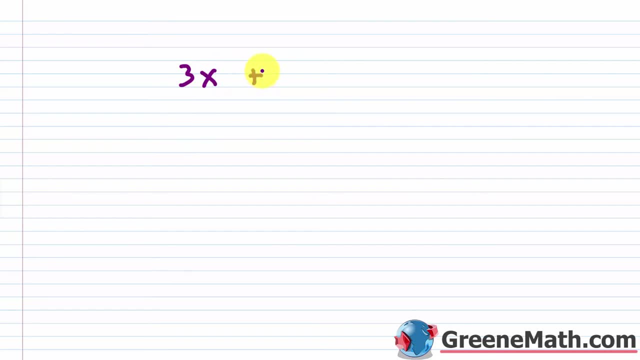 spent on milk. Then, plus, you have the fact that she buys two cartons of eggs. Okay, so two cartons of eggs Y is the cost of one carton of eggs. So two times Y would give me the cost for eggs in. 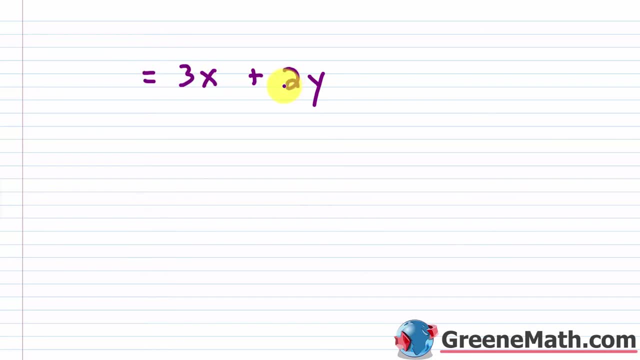 that kind of transaction. And again, if I sum these two amounts together, I get the amount she spent, which is $7.45.. Okay, Again, you can clear the decimal. if you want, You can multiply everything by 100.. So we could say this is: 745 is equal to 300X plus 200Y- Not necessary if you're working. 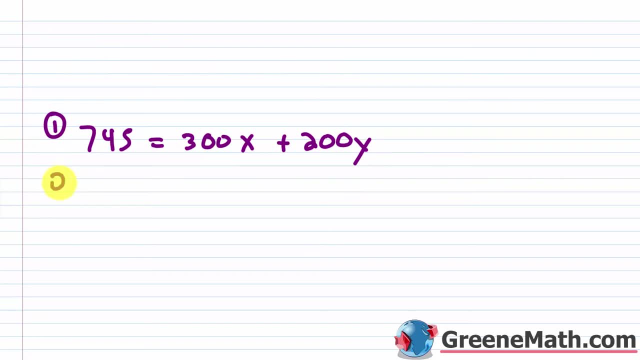 with a calculator, but I'll just do it because your book would probably do it. Then for equation two, I'm going to do the same thing with Jim. So if we go back up, So for Jim, he spent $6.45. 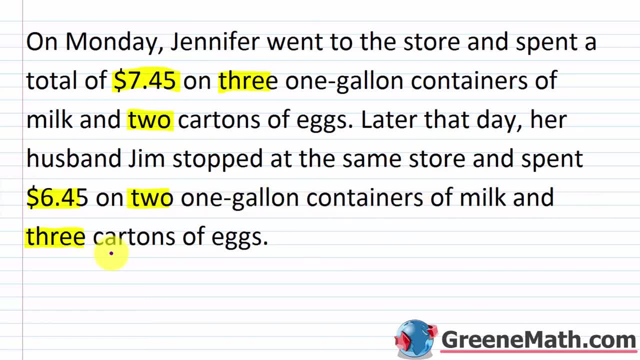 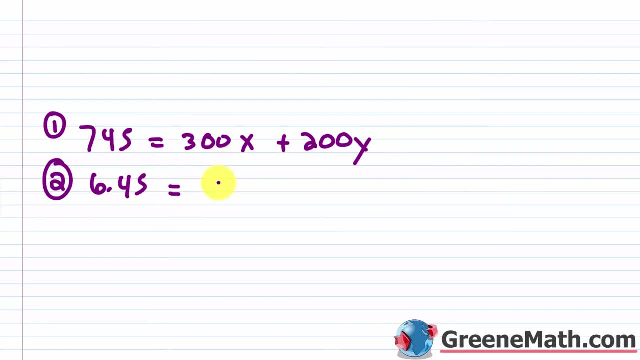 again on two one-gallon containers of milk and three cartons of eggs. So we would have that $6.45, or $6.45 is equal to again. he only bought two gallons of milk, so 2X plus. he bought three. 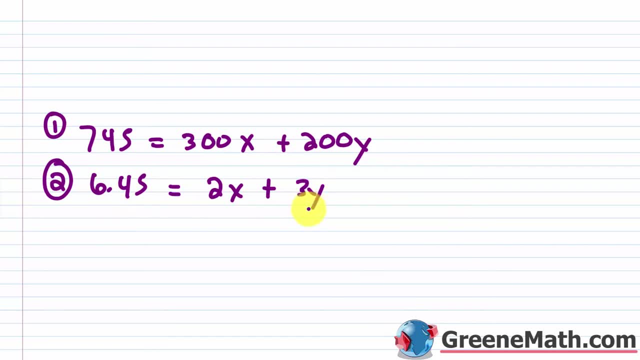 cartons of eggs, so 3Y. Again, you can multiply everything by 100 and say this is: 645 is equal to 200X plus 300Y. Okay. So let's erase this and let's drag this up, So we only have a linear. 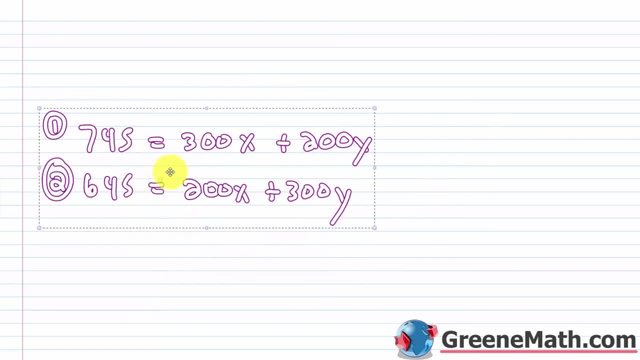 system with two variables. So we only have a linear system with two variables. So we only have a pretty easy to work with this at this point after we've been dealing with three. All right, So we can solve this with substitution if we want, or we can solve it with elimination. I think it's. 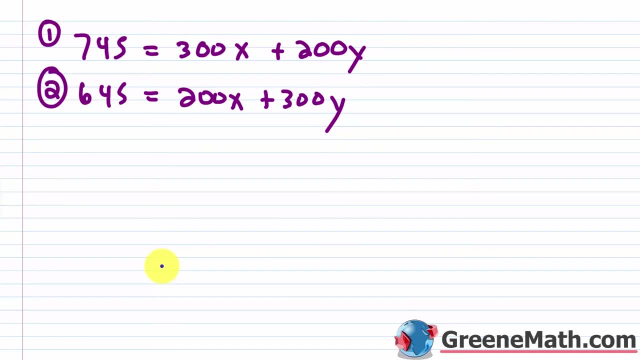 probably better to solve it with elimination, although substitution would probably be just as fast, but let's just use elimination. So what I'm going to do is I'm going to eliminate the variable X, And the way I'm going to do that is I'm going to think about the least common multiple between: 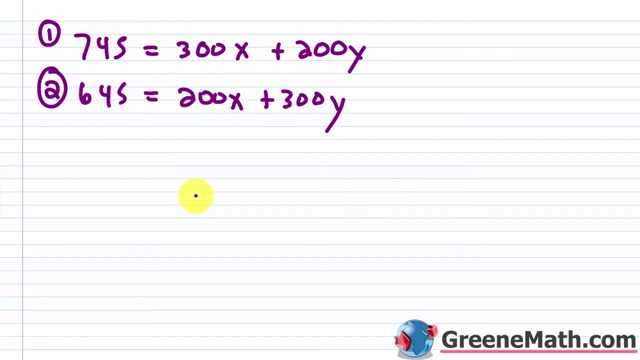 300 and 200. So that would be 600, right, If I think about three and two. okay, three and two, the least common multiple would be six, just because it's 300 and 200. Now it would be 600. 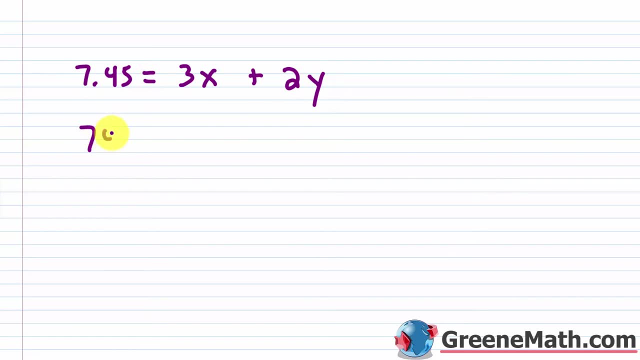 You can multiply everything by 100. So we could say this is: 745, is equal to 300X plus 200Y. Not necessary if you're working with a calculator, but I'll just do it because your book would probably do it. 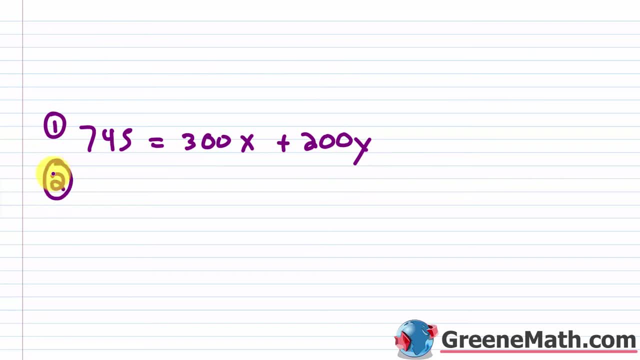 Then for equation two, I'm going to do the same thing with Jim. So if we go back up, So for Jim he spent $6.45, again on two one-gallon containers of milk and three cartons of eggs. 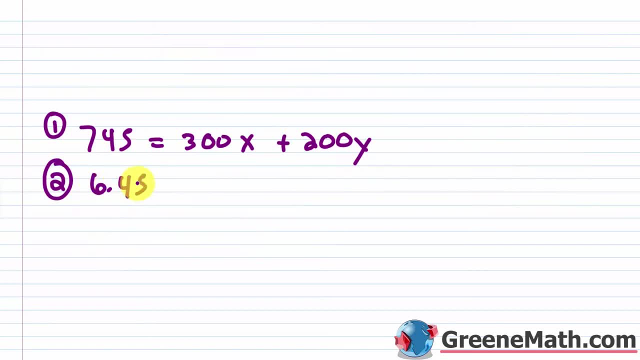 So we would have that 6.45, or $6.45 is equal to again. he only bought two gallons of milk, so 2X plus. he bought three cartons of eggs, so 3Y Again. you can multiply everything by 100. 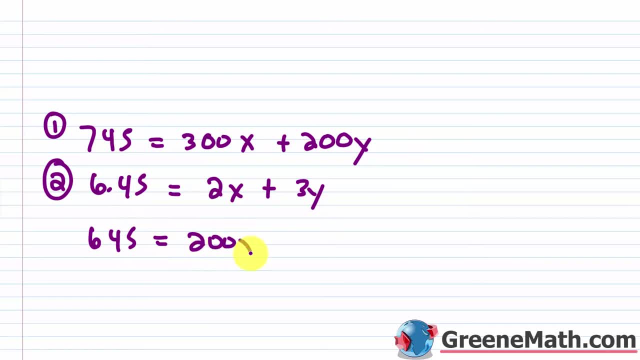 and say: this is 645 is equal to 200X plus 300Y. okay, So let's erase this and let's drag this up So we only have a linear system with two variables, so pretty easy to work with this at this point. 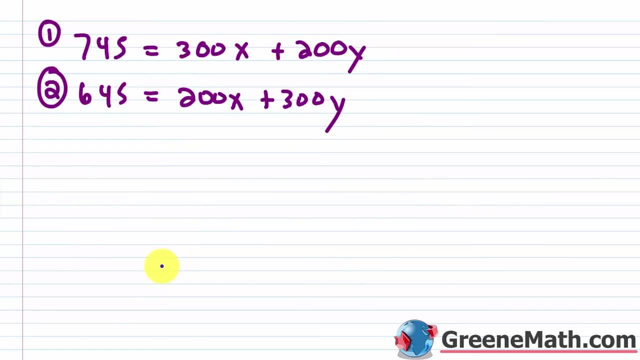 after we've been dealing with three. All right, so we can solve this with substitution, if we want, or we can solve it with elimination. I think it's probably better to solve it with elimination, although substitution would probably be just as fast. 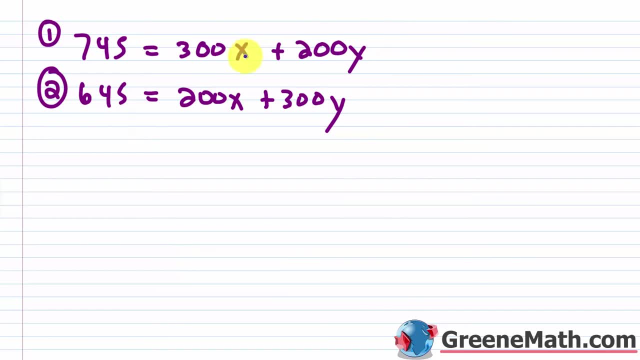 but let's just use elimination. So what I'm going to do is I'm going to eliminate the variable X, and the way I'm going to do that is I'm going to think about the least common multiple between 300 and 200, so that would be 600, right? 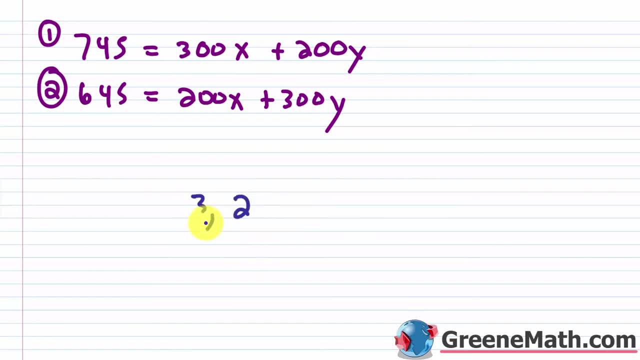 If I think about three and two. okay, three and two, the least common multiple would be six, Just because it's 300 and 200, now it would be 600, okay, So what I'm going to do is I'm going to multiply. 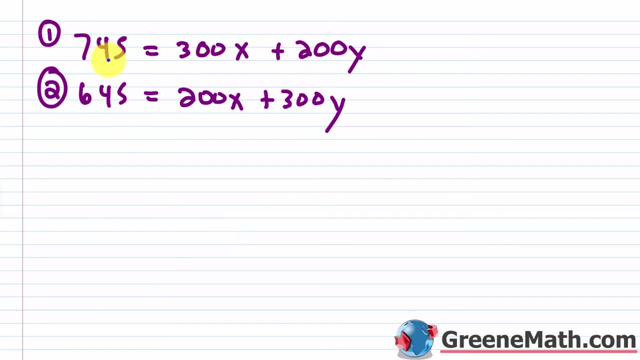 equation one by, let's say, negative two. So 745 times negative two would be negative 1,490, and this equals 300 times negative two is negative 600, then of course, times X and then 200 times negative two. 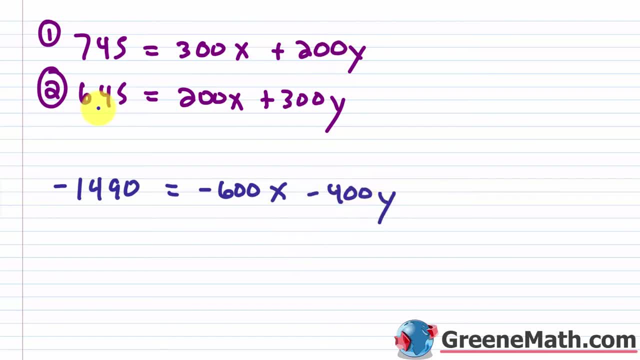 would be minus 400, and then times Y, Then for this guy right here, I'm going to multiply it by positive three. okay, So three times 645 is going to be 1,935, and this equals three times 200 is 600,. 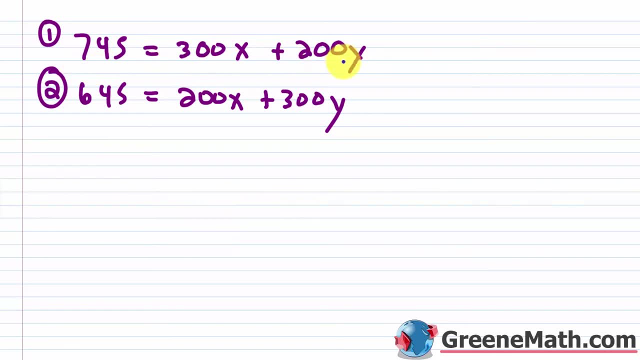 Okay. So what I'm going to do is I'm going to multiply equation one by, let's say, negative two. So 745 times negative two would be negative 1,490. And this equals 300 times negative two is negative 600. Then, of course, times X, and then 200 times negative two would be minus 400. And then times Y. 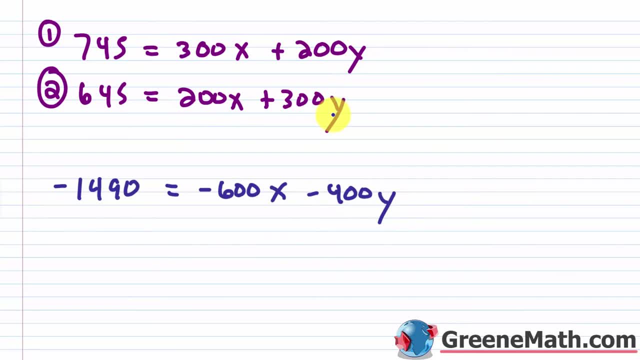 Then for this guy right here, I'm going to multiply it by positive three. Okay, So three times 645 is going to be 1,935.. And this equals three times 200, is 600, then times X, then plus three times. 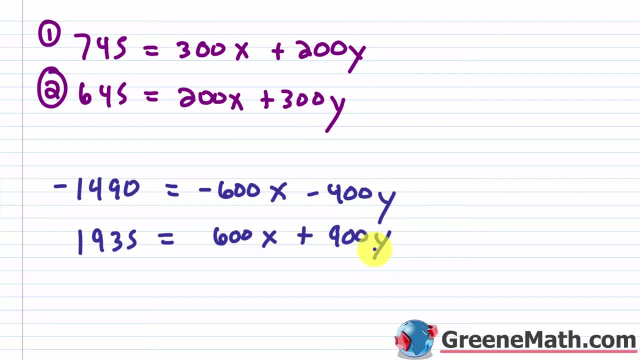 300 is 900, then times Y: Okay. So if we sum the left sides together we're going to get 445, right. So 1,935 plus negative 1,490 would be 445.. On the right sides, this would cancel. 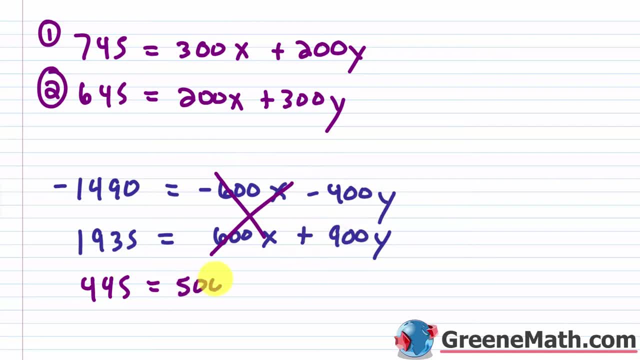 negative: 400 Y plus 900 Y is 500 Y, So we're going to get 445.. So we're going to get 445.. So let me erase this. We don't need this anymore. And let me just kind of slide this up. 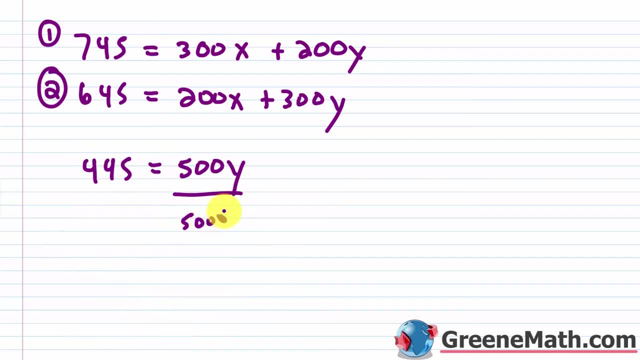 So let me bring this up. Let me divide both sides by 500.. So divide by 500.. So I can just erase this and say: Y equals this. Now, this is a fraction. If you want to simplify this quickly, here's how I would do it. I would break this up into: 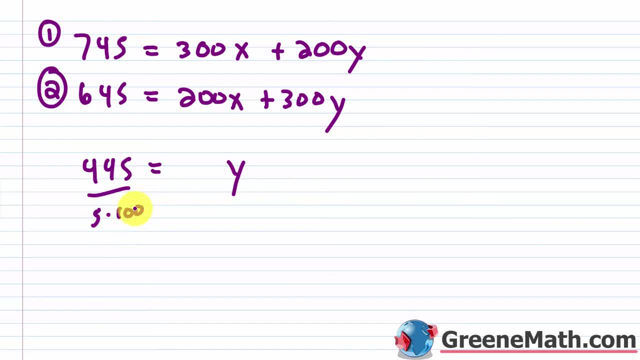 five times 100.. Okay, Cause it's easy to divide by 100.. 445 divided by five would be 89. So if I cancel this with this, I would get 445.. So I'm going to get 445 divided by 100.. 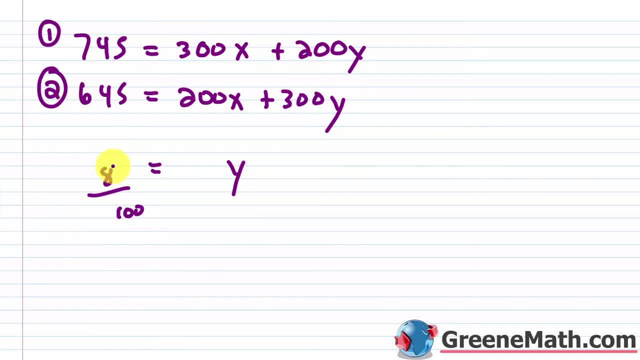 I would have 89.. Okay, So I have 89 over a hundred now. So we know, if we divide by a hundred, just moving my decimal point two places to the left, So this would be 89 here. This would go one, two places to the left, So 0.89.. Okay, So that's my Y. So Y is equal to 0.89.. So that's. 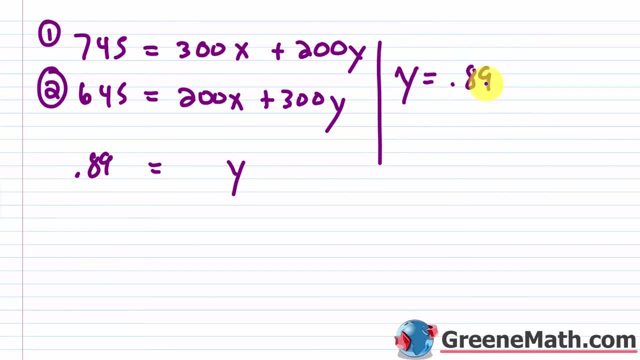 the cost of one carton of eggs. So apparently, where they live it's super cheap for eggs. Okay, So then now we need to find out X, And of course I could just plug into either equation one or two, So I'm just going to use equation. 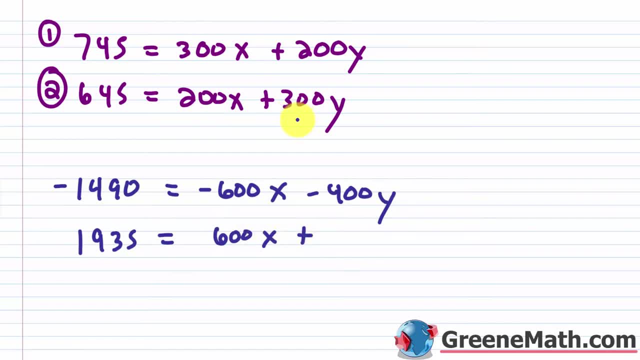 then times X, then plus three times 300 is 900, then times Y. okay, So if we sum the left sides together we're going to get 445, right. So 1,935 plus negative 1,490 would be 445.. 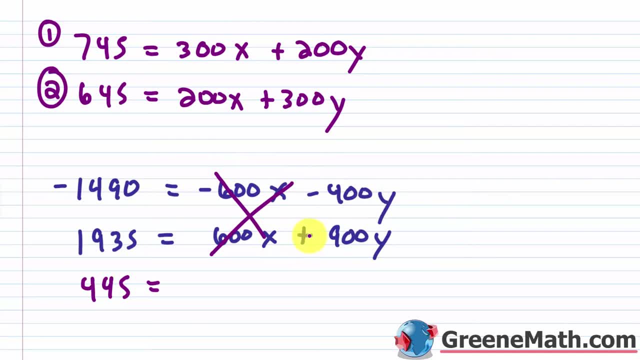 On the right sides. this would cancel negative. 400Y plus 900Y is 500Y. So let me erase this. We don't need this anymore And let me just kind of slide this up. So let me bring this up. 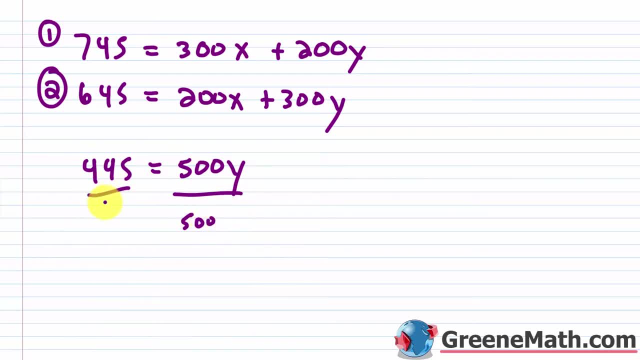 Let me divide both sides by 500.. So divide by 500.. So I can just erase this and say Y equals this. Now, this is a fraction. If you want to simplify this quickly, here's how I would do it. I would break this up into five times 100, okay. 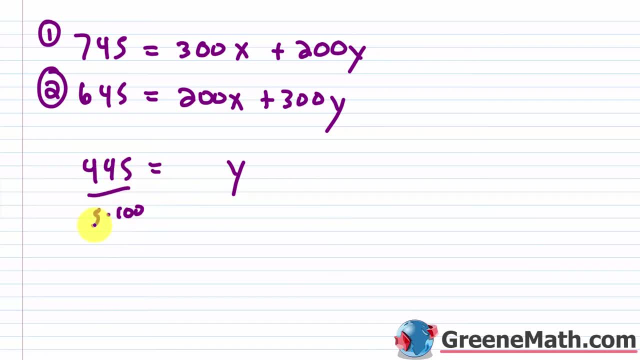 Because it's easy to divide by 100.. 445 divided by five would be 89. So if I canceled this with this, I would have 89.. Okay, so I have 89 over 100 now. So we know if we divide by 100,. 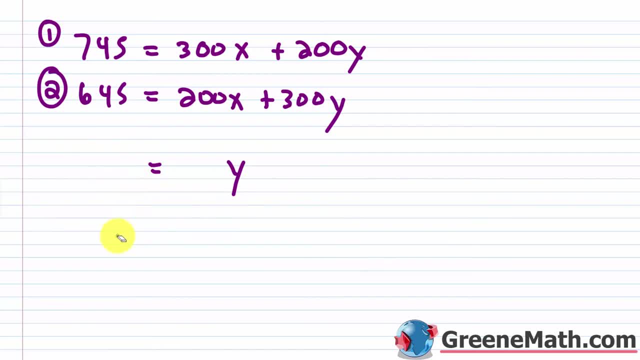 just moving my decimal point. two places to the left, So this would be eight, nine here. This would go one, two places to the left, so 0.89.. Okay, so that's my Y. So Y is equal to 0.89. 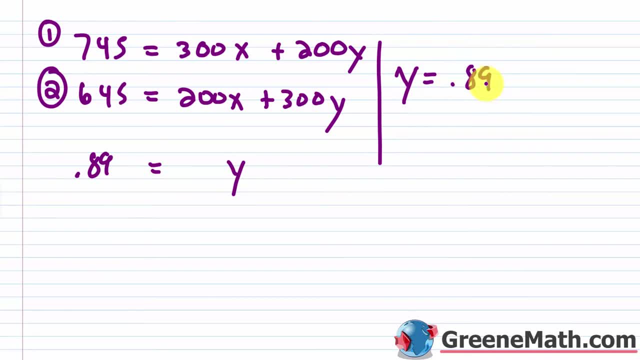 So that's the cost of one carton of eggs. So apparently, where they live, it's super cheap for eggs. Okay, so then now we need to find out X, And of course I could just plug into either equation one or two. 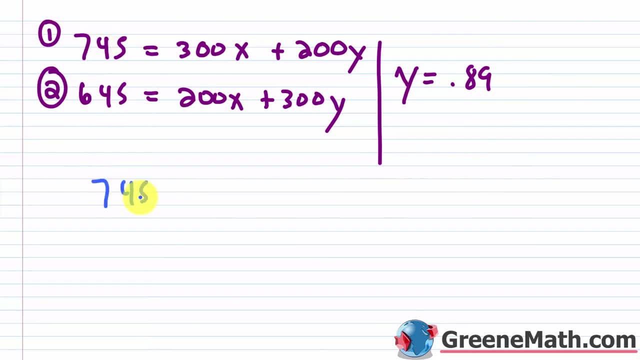 So I'm just gonna use equation one. So 745 is equal to 300 times X, plus 200 times, you've got your 0.89.. Where again, you can do this in fractional form if you want. Remember this was 89 over 100, okay. 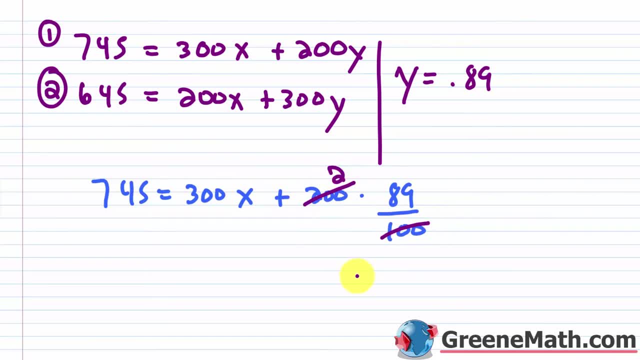 So that allows me to just cancel this with this and get a two. And then two times 89 is 178.. Okay, so 178.. Let me subtract that away from each side of the equation That will cancel. 745 minus 178 is gonna be 567.. 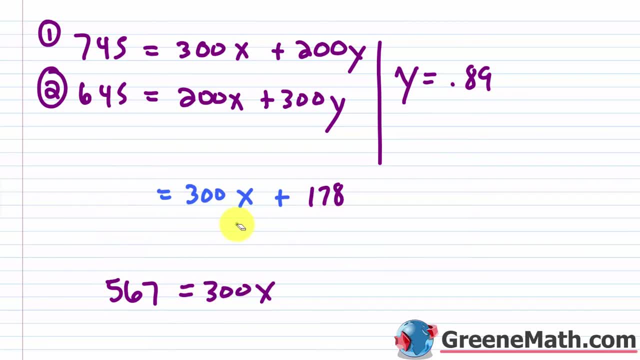 So this equals 300X. Let me erase this And we can use a similar trick again. This will help you if you don't have a calculator, right? So this guy right here. if I divide both sides by 300, I can think about three times 100, okay. 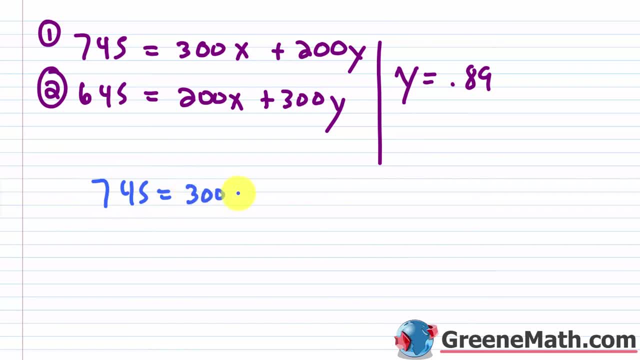 One. So 745 is equal to 300 times X plus 200 times. You've got your 0.89 where again you can do this in in fractional form If you want. remember this was 89 over a hundred, Okay. 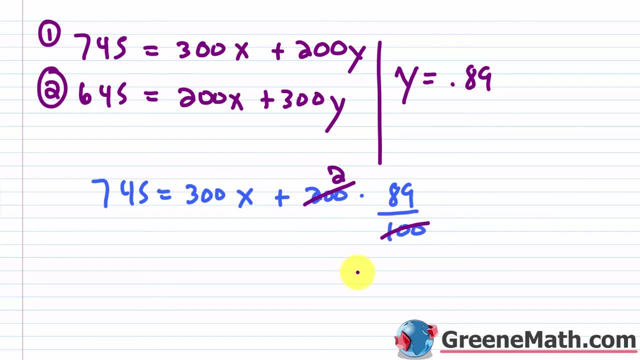 So that allows me to just cancel this with this and get a two, and then two times 89 is 178.. Okay, So 178, let me subtract that away from each side of the equation. that will cancel. 745 minus 178 is going to be 567.. So this equals 300 X. Let me erase this And we can use a similar trick. 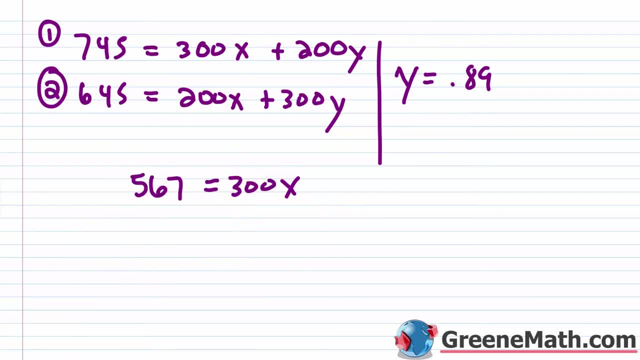 again, This will help you if you don't have a calculator, right? So this guy right here. if I divide both sides by 300, I can think about three times a hundred. Okay, So what's 567 divided by three? Well, that's going to be 189.. So this would be 189. And I'm going to cancel this out. 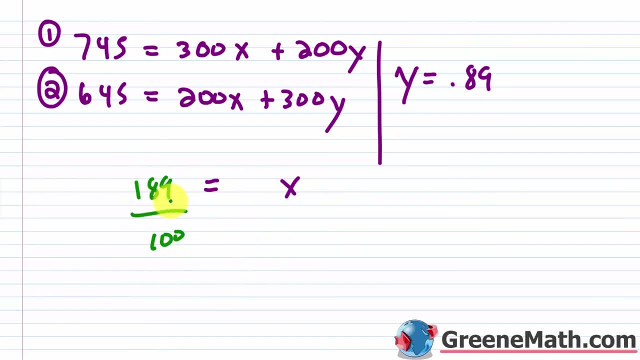 here over a hundred, right? So let me erase this. So X is 189 over a hundred, So this is a hundred. or again, this moves two places to the left, So X is equal to 189.. Move this one two places to the left, So 1.89, or a dollar and 89 cents, So that's the cost per one gallon of milk. 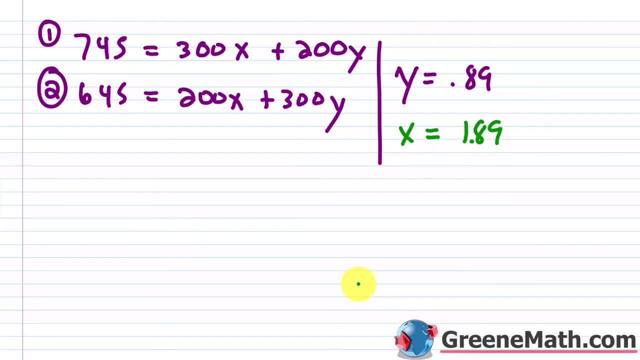 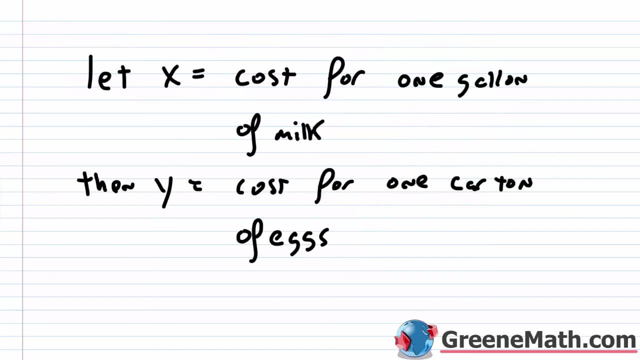 So apparently, wherever they live, they have really cheap milk and really cheap eggs. Okay, So this does not actually answer our question. Okay, So this is where a lot of students mess up. They say their answer is: it's a dollar 89 for one gallon of milk, and it's 89. 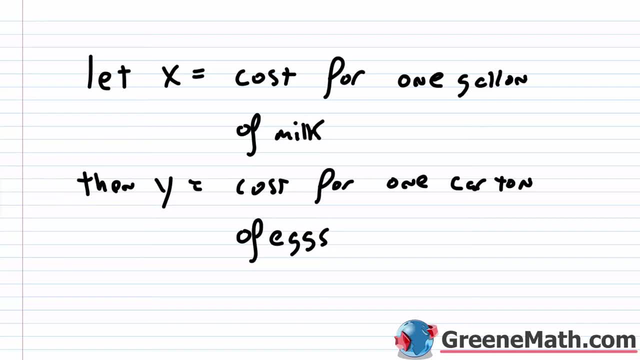 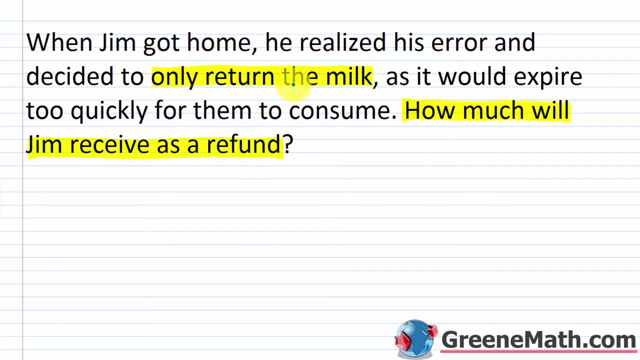 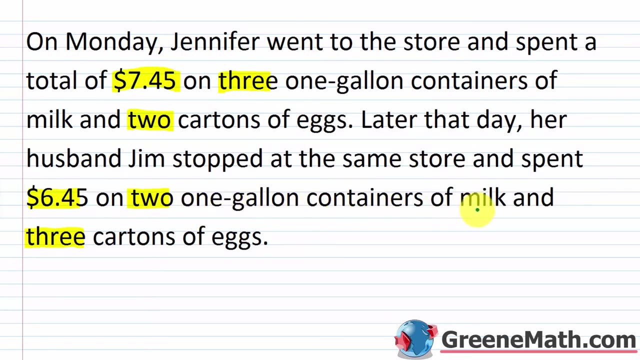 carton of eggs And the teacher marks it wrong And they wonder why. the reason is. you have to read the problem. Okay, How much will Jim receive as a refund? He only returns the milk. Okay, So how much? how much milk did Jim get? Jim got two one gallon containers of milk. Again, the milk is. 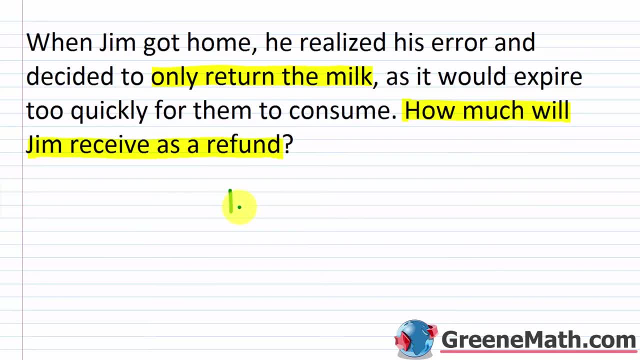 a dollar 89 a piece. So all I need to do is take the 1.89.. Again, that was X. That was the cost per one gallon of milk, and multiply it by two. So multiply it by two Again. all you have to do. 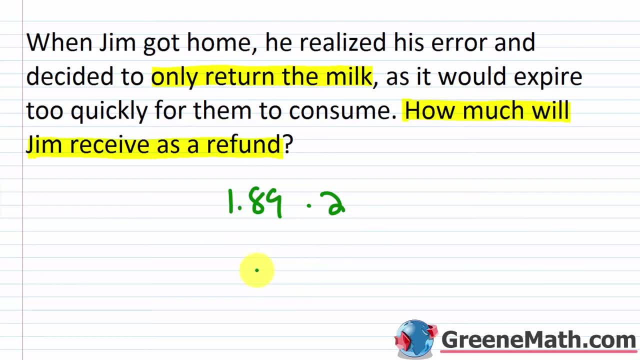 is 189 times two. and then move the decimal point two places to the left, So 189 times two is 378.. So it's 378.. Again, move the decimal point two places to the left, You get $3 and 78 cents. 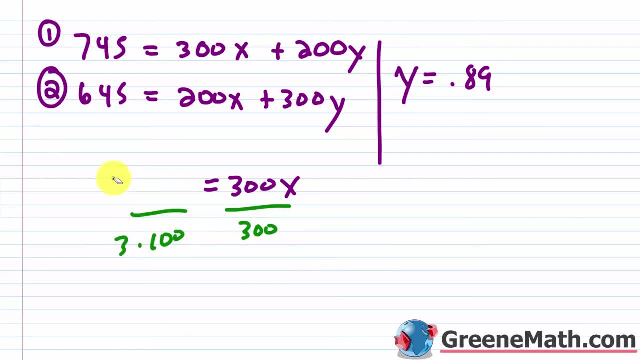 So what's 567 divided by three? Well, that's gonna be 189.. So this would be 189. And I'm gonna cancel this out here- over 100, right? So let me erase this. So X is 189 over 100.. 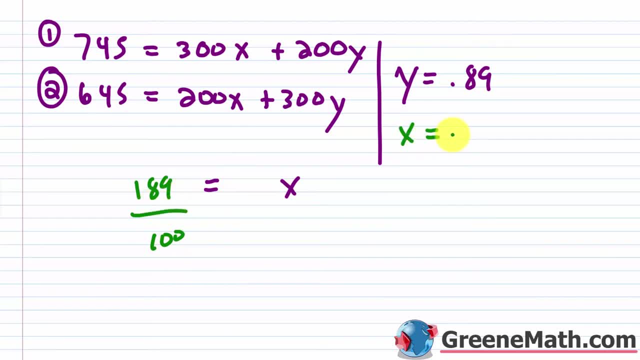 Or again, this moves two places to the left, So X is equal to 189.. Move this one two places to the left, So 1.89 or $1.89.. So that's the cost per one gallon of milk. So apparently, wherever they live, 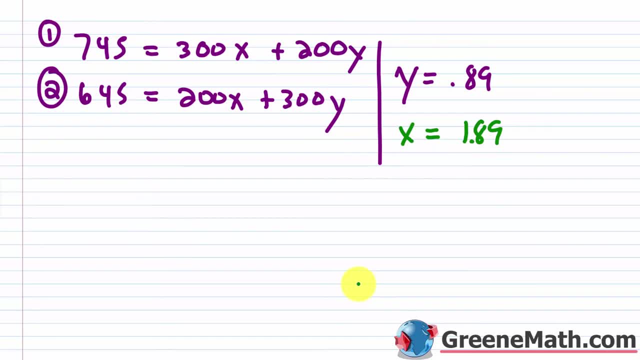 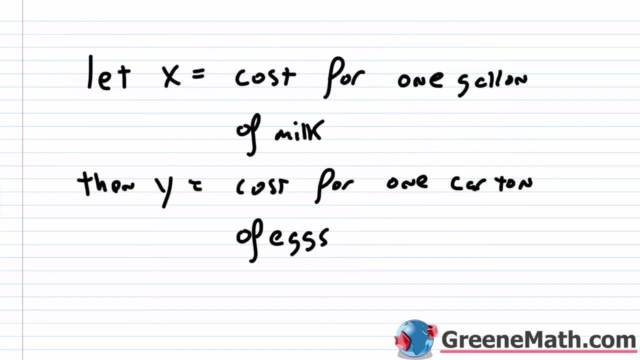 they have really cheap milk and really cheap eggs. Okay, so this does not actually answer our question, okay? So this is where a lot of students mess up. They say their answer is it's $1.89 for one gallon of milk. 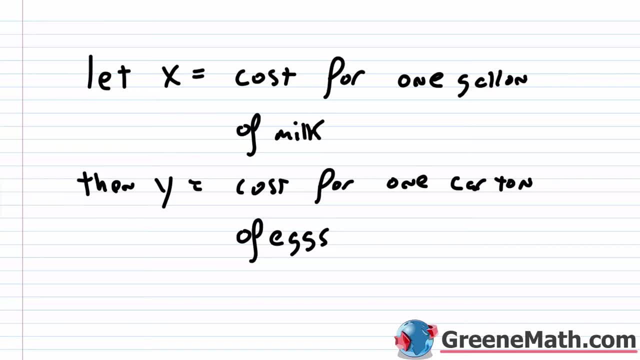 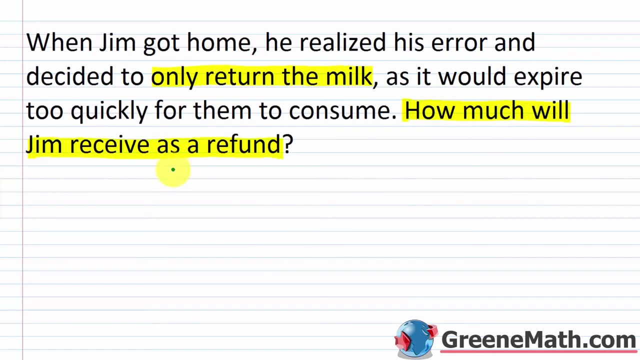 And it's 89 cents for one carton of eggs. And the teacher marks it wrong and they wonder why The reason is. you have to read the problem, okay. How much will Jim receive as a refund? He only returns the milk, okay. 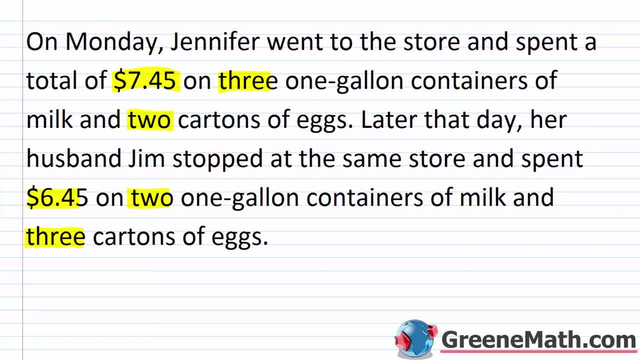 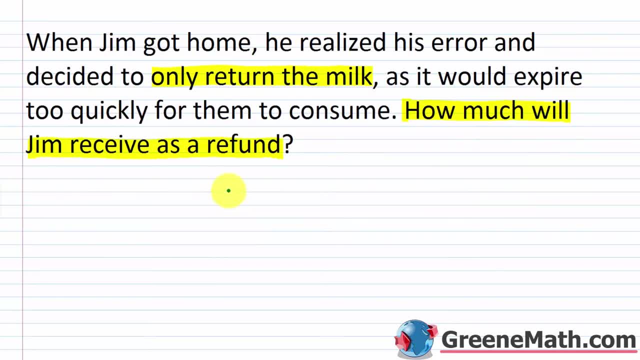 So how much milk did Jim get? Jim got two one-gallon containers of milk. Again, the milk is $1.89 a piece. So all I need to do is take the 1.89.. Again, that was X. that was the cost per one gallon of milk. 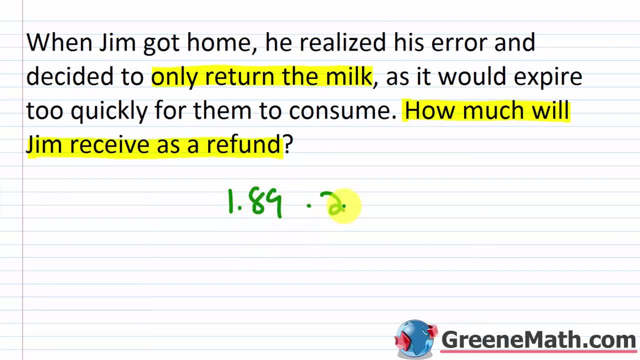 And multiply it by two. so multiply it by two again. all you have to do is 189 times two and then move the decimal point two places to the left. so 189 times two is 378. so it's 378 again. move the decimal point two places. 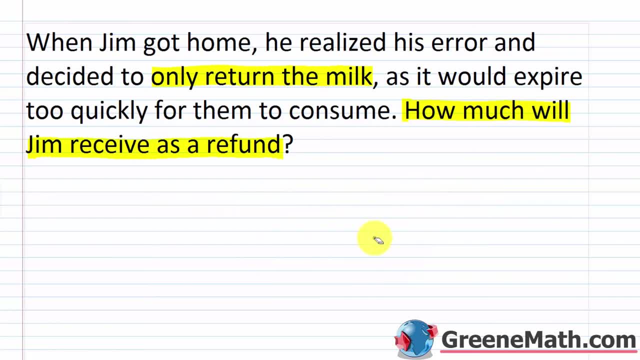 to the left, you get three dollars and 78 cents. so he will get or he will receive. if you want to say that, three dollars and 78 cents for his refund again just for the milk, make sure you read these problems because they throw kind of curveballs at you to make sure you're paying attention in this. 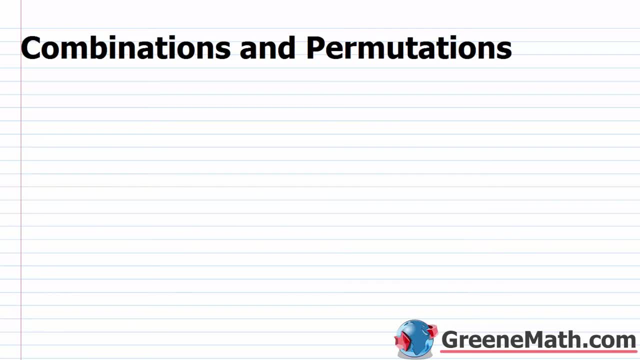 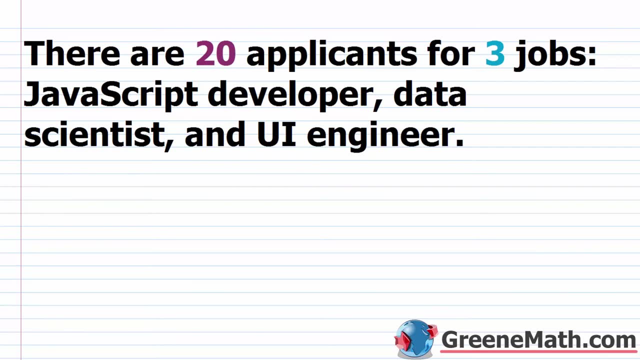 lesson. we want to talk about combinations and permutations. all right, so when we get to this section, a lot of students are going to have difficulty determining whether to use our formula for multiplication, or to use our formula for multiplication, or to use our formula for permutations, or whether to use our formula for combinations. basically, we're going to start out. 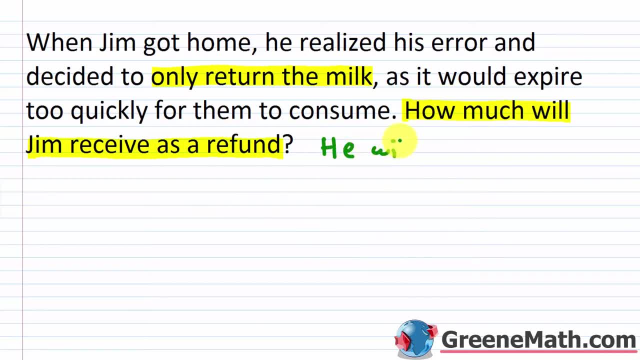 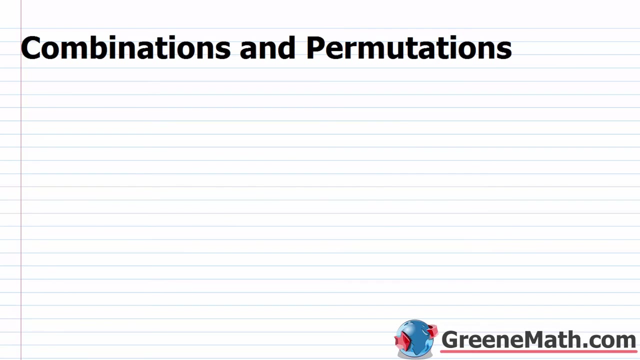 So he will get, or he will receive, if you want to say that, $3 and 78 cents for his refund. Again, just for the milk. Make sure you read these problems because they throw kind of curve balls at you to make sure you're paying attention. In this lesson we want to talk about combinations. 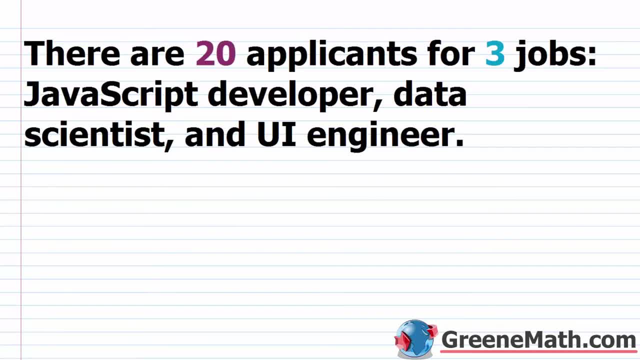 and permutations, All right. So when we get to this section, a lot of students are going to have difficulty determining whether to use our formula for permutations or whether to use our formula for combinations. Basically, we're going to start out with one here where we say that there 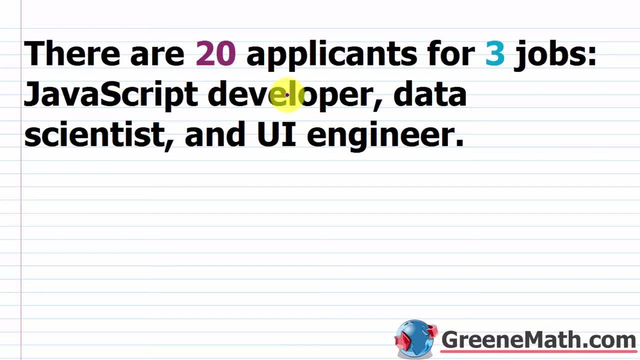 are 20 applicants for three jobs: a JavaScript developer, a data scientist and a data scientist And a UI engineer. Well, basically, the way that you decide here, you're going to be selecting three people out of the 20.. So, if you have the number of ways of selecting R items out of N, 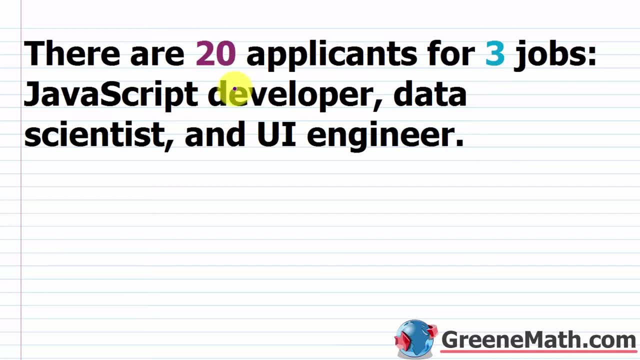 items. in this case, it's three out of 20.. And repetition is not allowed, because the same person can't get the JavaScript developer job, the data scientist job and the UI engineer job. It's got to be three separate people. Well, you want to consider the fact that, if the order is important, 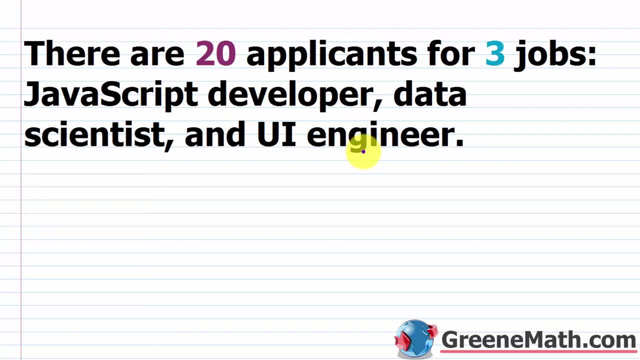 you want to use three people. So if you have three people, you want to use three people. So if you have three people, you want to use a permutation. If the order is not important, you want to use a combination. So here the order is very important to us because it's a different result if I get a 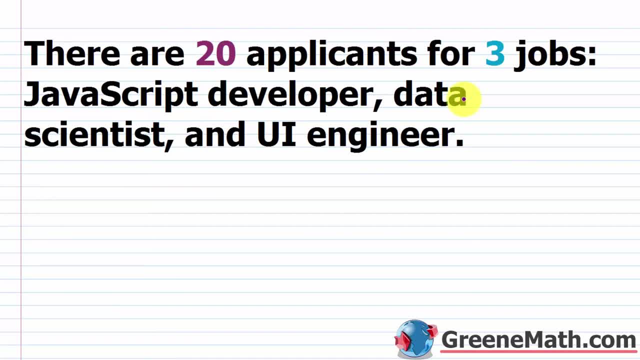 job as a JavaScript developer versus if I get a job as a data scientist. So, because the order is important, we want to use our formula for permutations, And that's a real easy formula. It's going to be P, like this, And then I'm going to put some parentheses. It's going to be N. 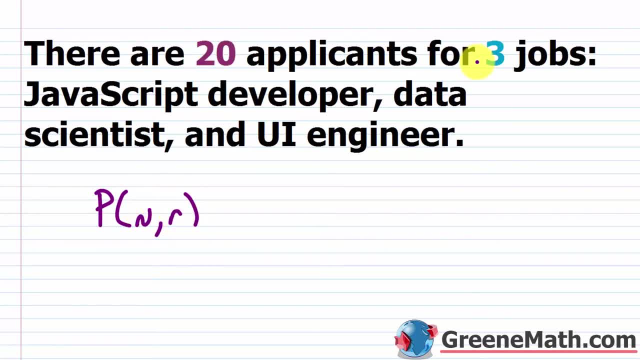 R. The N here is going to be the 20. R, here is going to be the 3.. We'll fill that in in a minute. This equals: you've got your N factorial over. you've got your N minus R factorial. Okay. so in this case, we're going to 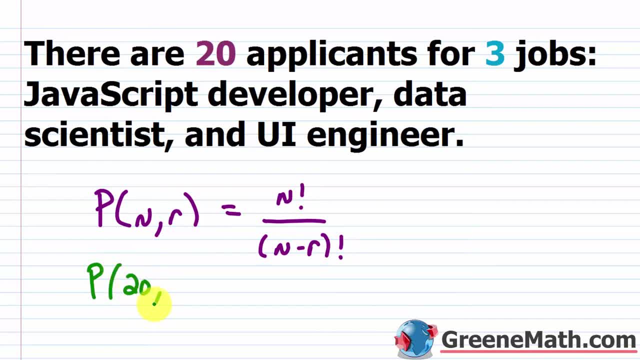 have P and we would say 20 pick 3.. Okay, that's how you can read that if you want. And this is going to be equal to 20 factorial over and I made that a little bit long, so let's fix that. 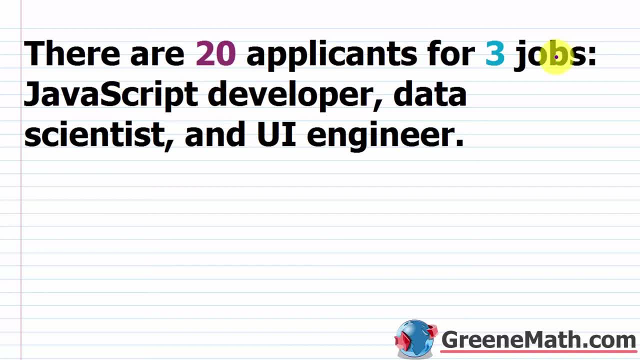 with one here where we say that there are 20 applicants for three jobs: a javascript developer, a data scientist and a ui engineer. well, basically, the way that you decide here, you're going to be selecting three people out of the 20.. so, if you have the number of ways of selecting r items out, 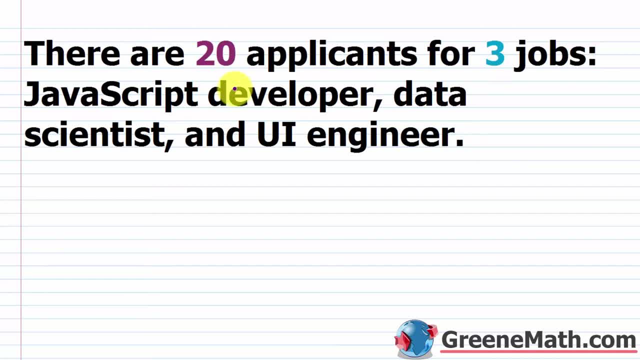 of n items. in this case it's three out of twenty, and repetition is not allowed, because the same person can't get the javascript developer job, the data scientist job and the ui engineer job. it's got to be three separate people. well, you want to consider the fact that if the 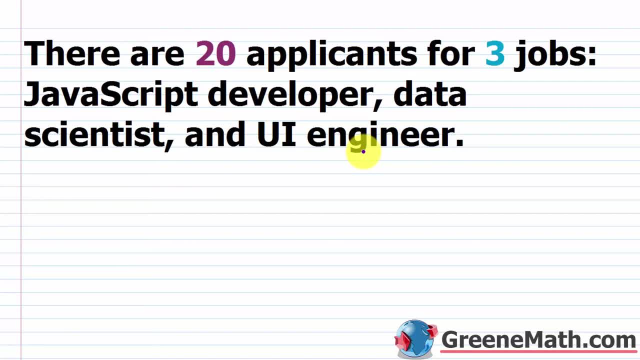 order is important, you want to use a permutation. if the order is not important, okay, you want to use a combination. so here the order is very important to us because it's a different result if i get a job as a javascript developer versus if i get a job as a data scientist, okay. so, because the order is 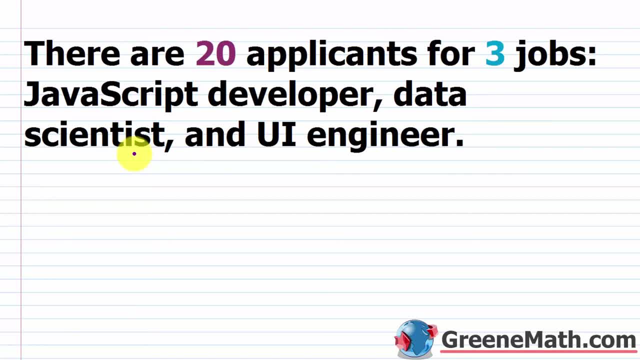 important. we want to use our formula for permutations and that's a real easy formula. it's going to be p, like this, and then i'm going to put some parentheses. it's going to be n comma r. okay, the n here is going to be the 20, the r here is going to be the three. we'll fill that in a. 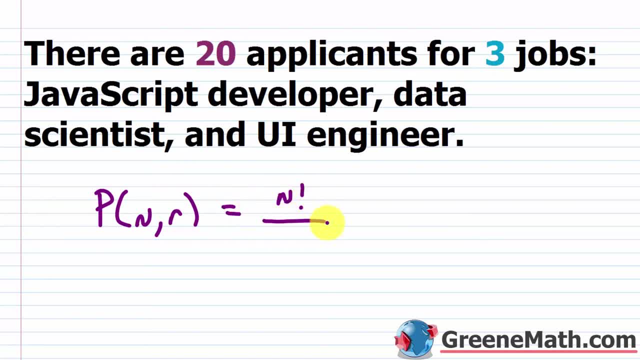 minute. this equals: you've got your n factorial over, you've got your n minus r factorial. okay. so in this case we're going to have p and we would say: 20 pick three. okay, that's how you can read that, if you want. and this is going to be equal to 20 factorial. 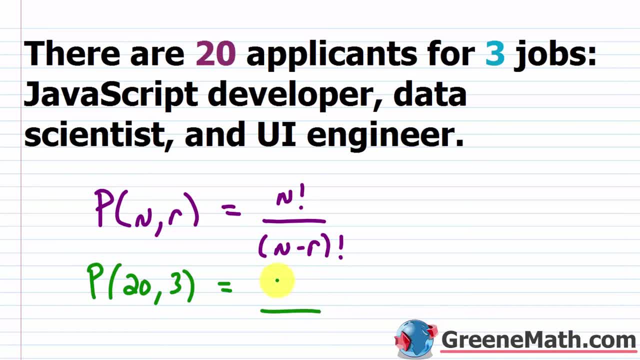 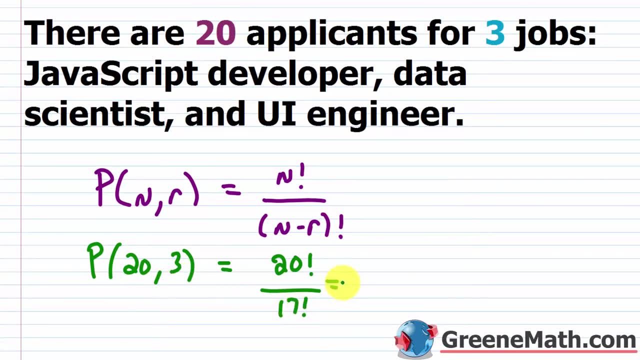 over and i made that a little bit long, so let's fix that. so 20 factorial over. in this case you'd have 20 minus 3 or 17 factorial. okay, if you want to simplify this, you can. of course, this key is on your calculator if you're using a ti 83 or 84 or whatever the version is you're using, but let's 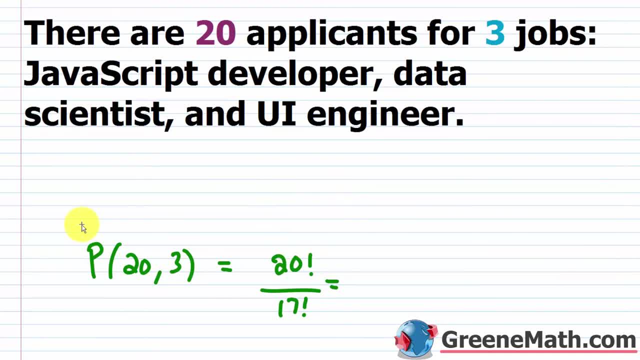 just go through this one in the future ones. i'm just going to punch it into the calculator and make it a lot quicker. let's move this up here. this would be what it would be: 20 times 19 times, 18 times 17. you know so on and so forth. but this part here because the 17 factorial 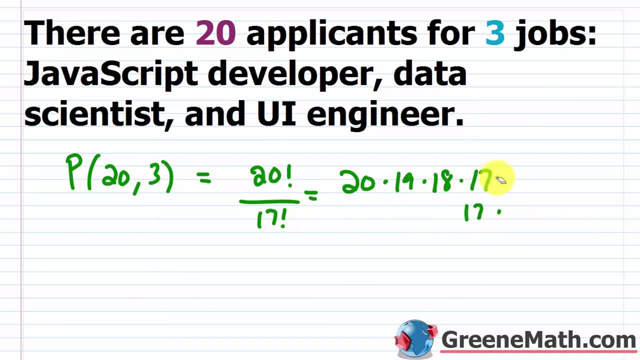 is going to keep going down to one. you can get rid of that part and just erase this and say it's 20 times 19, times 18, which is going to be what? well, 20 times 19 is 380, then times 18 is going to be. 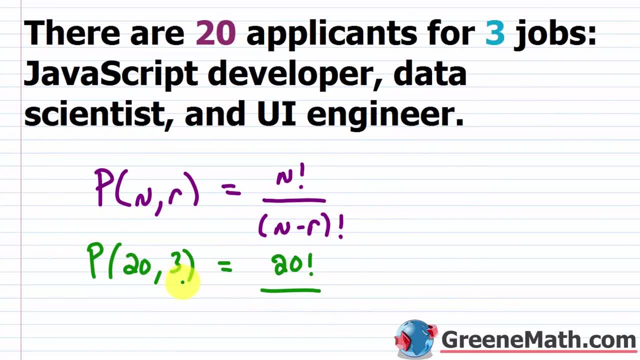 So 20 factorial over. in this case you'd have 20 minus 3 or 17. Factorial- Okay, if you want to simplify this, you can. Of course, this key is on your calculator if you're using a TI-83 or 84 or whatever the version is you're using. But let's just go through. 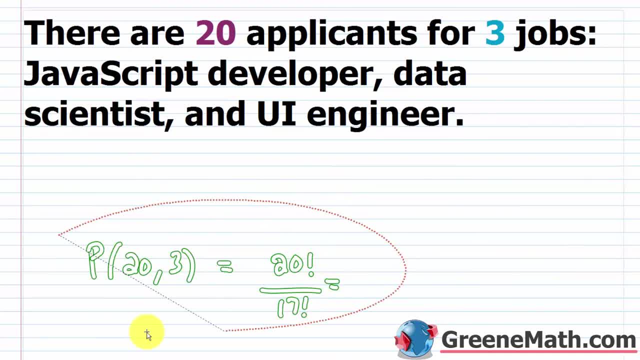 this one in the future ones. I'm just going to punch it into the calculator and make it a lot quicker. Let's move this up here. This would be what It would be: 20 times 19 times, 18 times 17,. 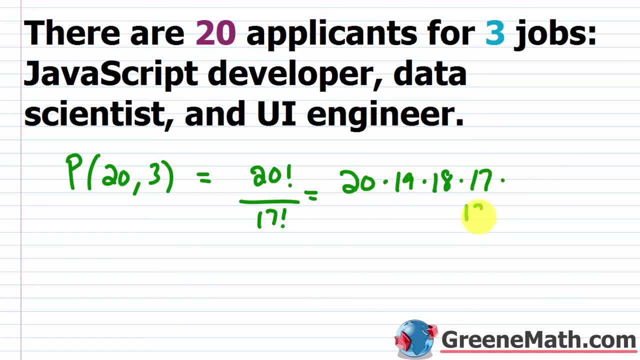 you know, so on and so forth, But this part here, because the 17 factorial is going to keep going down to one, you can get rid of that part and just erase this and say it's 20.. 20 times 19, times 18, which is going to be what? Well, 20 times 19 is 380, then times 18 is going. 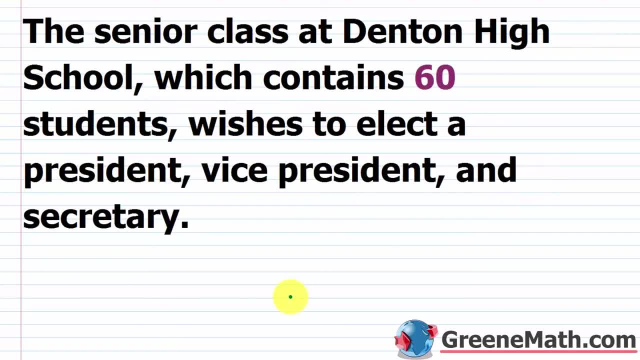 to be 6,840.. All right, let's look at the next one. So we have the senior class at Denton High School, which contains 60 students. wishes to elect a president, vice president and secretary. So we're choosing three students out of the 60 for these three positions. The order is going to. 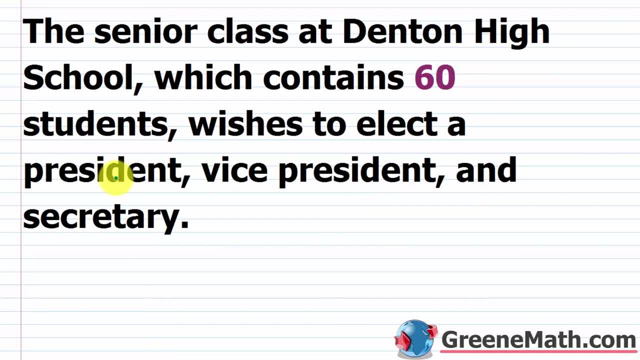 matter here, right? If someone gets selected as a president, it's a different result as if they got selected as a secretary. So, in other words, let's say that John got picked to be the president. Let's say Larry got picked to be the vice president, for example, And let's 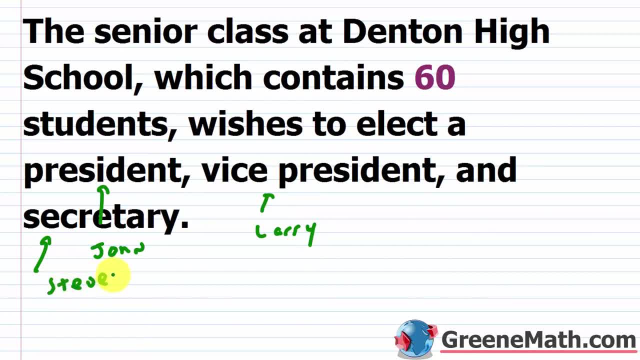 say that Steve, okay, Steve got picked to be the secretary. Well, if I switch things up, I can have the same three students. okay, but they got different positions. That's a completely different result, okay, So in this case we want to use a permutation And we remember the formula. 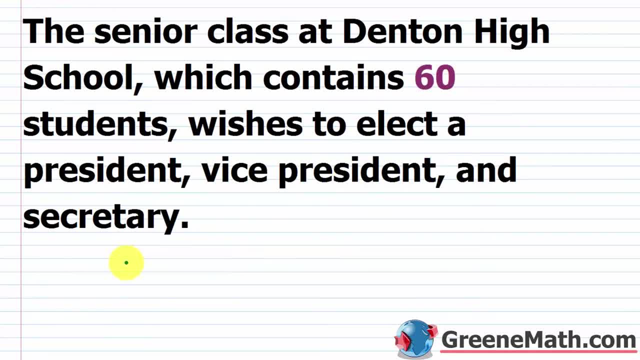 so I'm just going to type this into my calculator. I'm going to do 60,, okay, 60. And then you're going to have that key that says n, pick r. So it looks like this: a lowercase n, an uppercase p and a. 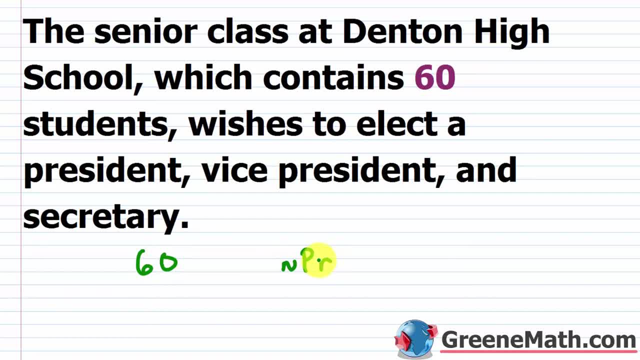 lowercase r, But I'm going to hit 60,, this key right here, and then three right, Because there's going to be three students selected: president, vice president and secretary- And if you run that calculation you're going to get 205,320.. So 205,320. 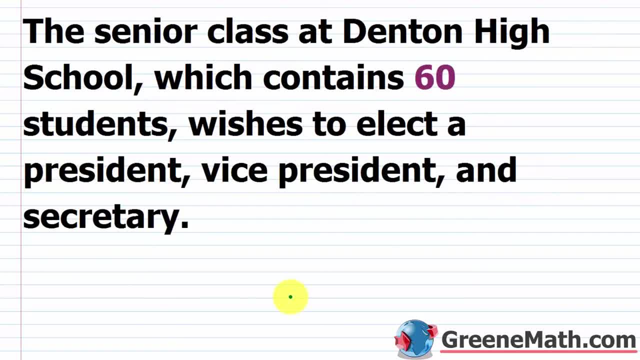 6840. all right, let's look at the next one. so we have the senior class at denton high school, which contains 60 students, wishes to elect a president, vice president and secretary. so we're choosing three students out of the 60 for these three positions. the order is going to matter here, right, if someone gets selected as a president. 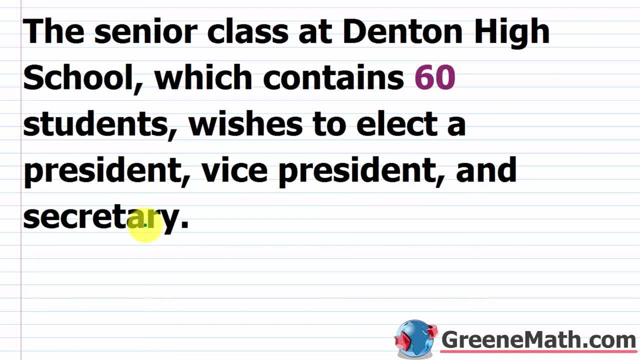 it's a different result, as if they got selected as a secretary. so, in other words, let's say that john got picked to be the president and let's say larry got picked to be the vice president, for example, and let's say that steve- okay, steve got picked to be the secretary. 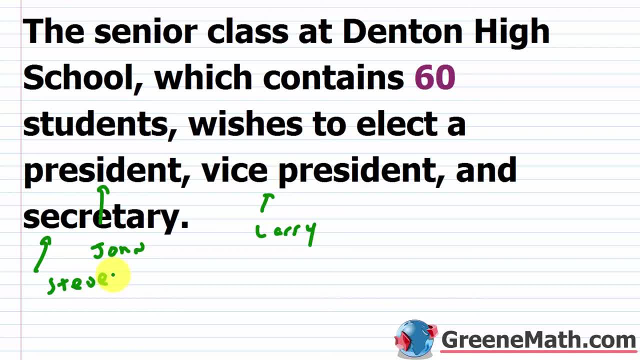 well, if i switch things up, i can have the same three students. okay, but they got different positions. that's a completely different result, okay? so in this case we want to use a permutation and we remember the formula for that. so i'm just going to type this into my calculator. 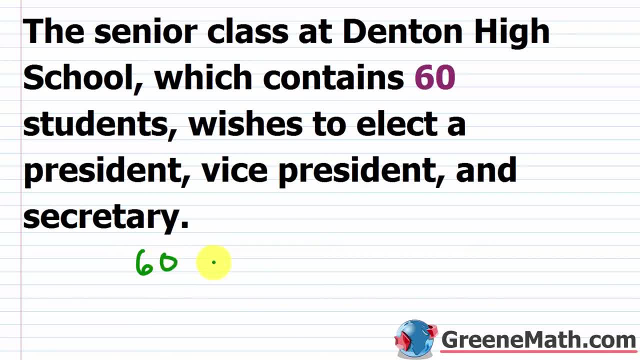 i'm going to do 60, okay 60, and then you're going to have that key that says n, pick r. so it looks like this: a lowercase n, an uppercase p and a lowercase r, but i'm going to hit 60, this key right here, and then three right, because it's going to be 60, and then 60, and then 60, and then 60, and 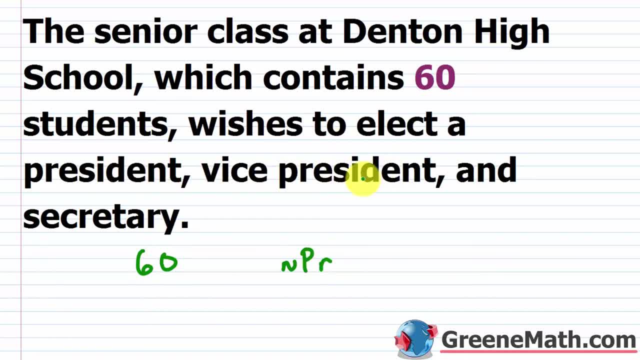 there's going to be three students selected: president, vice president and secretary, and if you run that calculation you're going to get 205, 320. so 205 320 and again, if you want to use the proper notation there, you've got this p and then you've got the first number, that's 60, and then 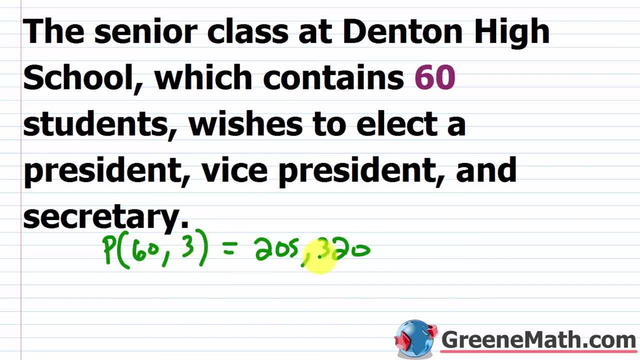 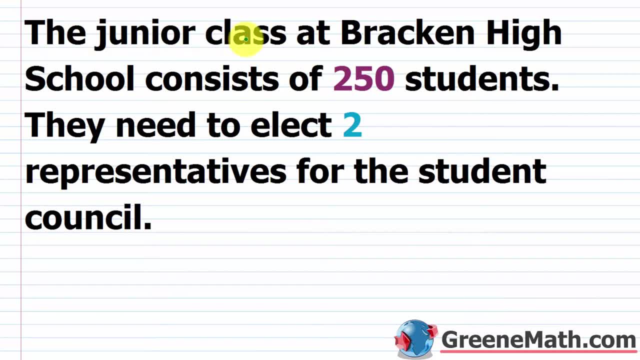 comma 30. okay, so this is what this is equal to. again, if you go on your calculator, it's the n p r key. okay, let's look at another example. so we have the junior class at bracken high school consists of 250 students. they need to. 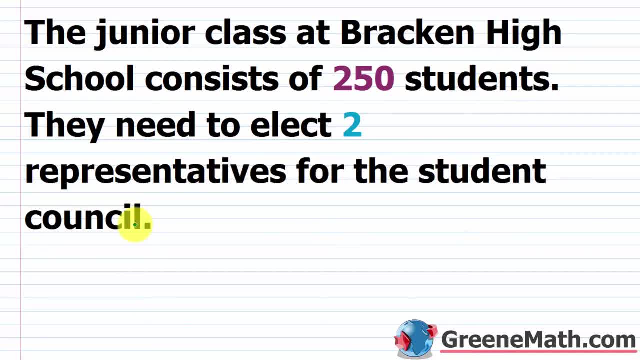 elect two representatives for the student council. okay, well, this is a little bit similar to the last question, but we're going to end up using a different formula here, because now the order doesn't matter anymore. okay, repetition's still not allowed, but the order doesn't matter anymore. 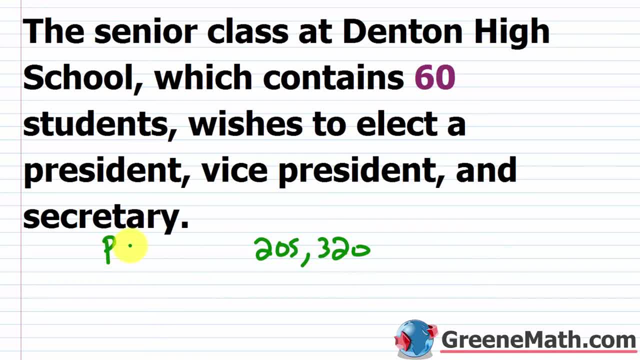 And again, if you want to use the proper notation there, you've got this p, and then you've got the first number, that's 60, and then comma 30.. Okay, so this is what this is equal to Again. 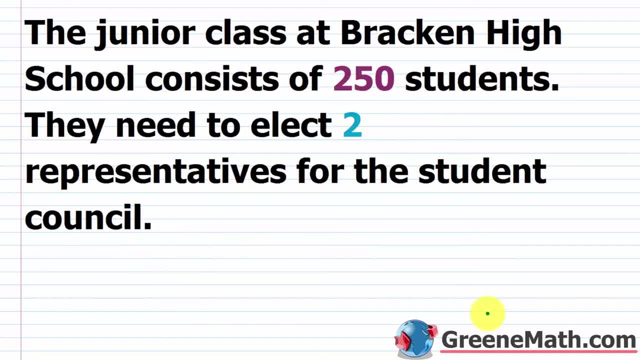 if you go on your calculator, it's the n p r key. Okay, let's look at another example. So we have the junior class at Bracken High School consists of 250 students. They need to elect two representatives for the student council. Okay, well, this is a little bit similar to the last. 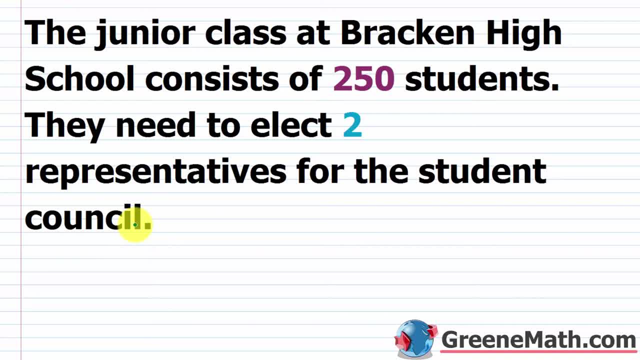 we're going to end up using a different formula here, because now the order doesn't matter anymore. Okay, repetition is still not allowed, But the order doesn't matter anymore, Because, let's say, John gets the first representative position and Steve gets the second one. 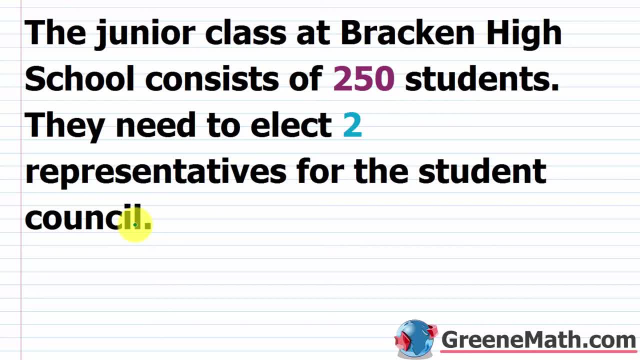 Well, it doesn't matter if we reverse that, and Steve got chosen first and then John did, because they're both going to just be representatives. Okay, so the order doesn't matter here. So we want to use the formula for combinations, And we learned this in the last. 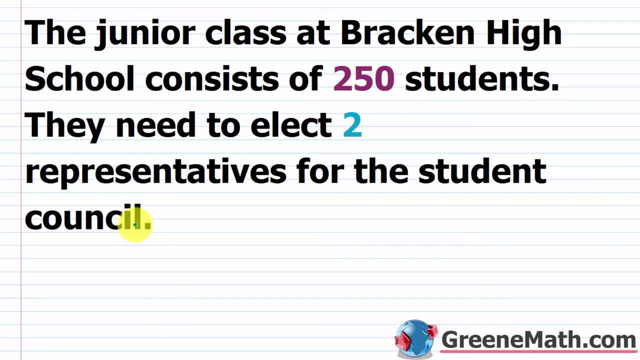 about the binomial theorem, right? so we have this formula: it's n choose r, so we have this c and then n comma r here, and this equals your n factorial over your n minus r factorial, and then times your r factorial. okay, so what ends up happening is we're dividing out the duplicates. 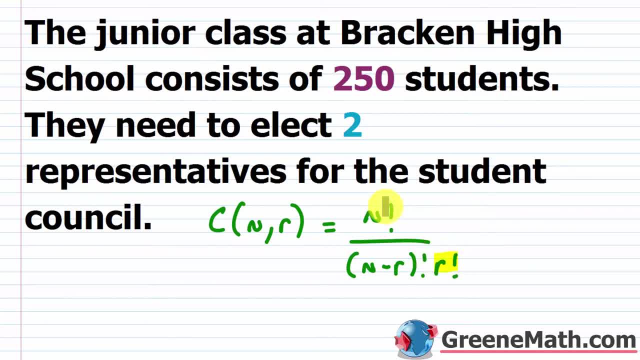 with this extra part here. okay, this is all you have to remember, because if you've got this part down from the permutations formula, you're just throwing that extra little bit there in the denominator to divide out the duplicates, and that's how you get your combination formula. 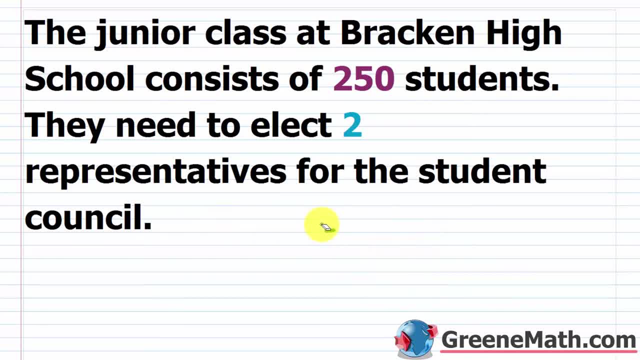 okay. so let's erase this real quick. let's actually plug in the numbers. i'm going to again use my calculator here, because you would basically be doing this c here with 250 comma 2, and i'm not going to set this up. you're just going to hit 250 and then go to ncr and i'm going to get a result. 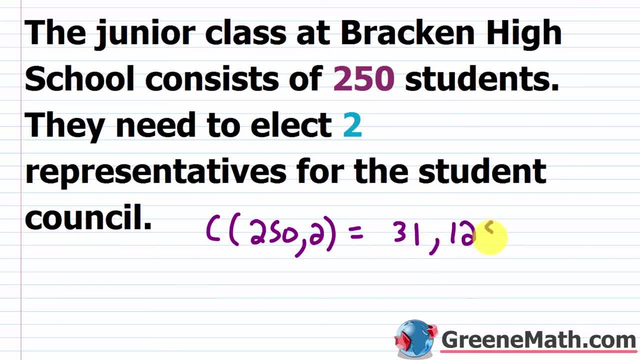 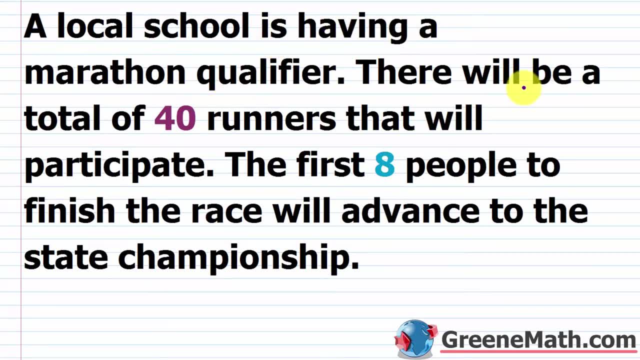 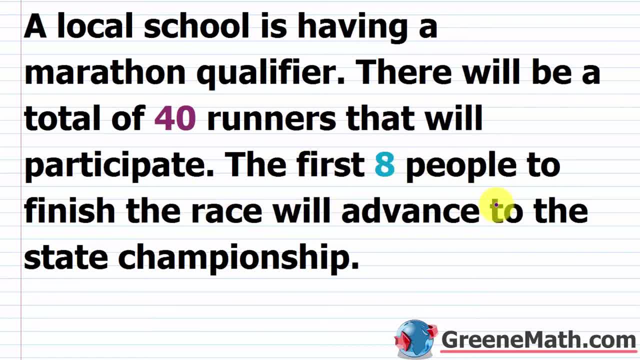 the first eight people to finish the race will advance to the state championship. okay, so do i want a permutation or a combination? does the order matter here? we know that repetition is not allowed, right, because if i'm in the first position, i can't also be in the third position. but does the order? 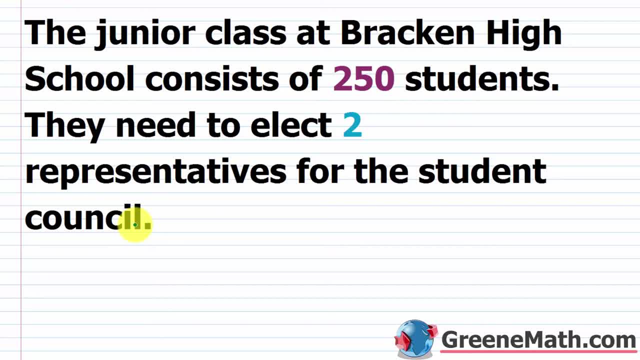 because, let's say, john gets the first representative position and steve gets the second one. well, it doesn't matter anymore, because he's going to be the second representative position. so it doesn't matter if we reverse that and steve got chosen first and then john did, because they're 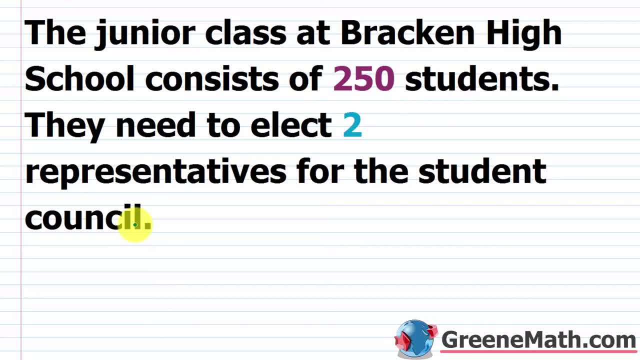 both going to just be representatives. okay, so the order doesn't matter here. so we want to use the formula for combinations, and we learned this in the last lesson when we talked about the binomial theorem. right, so we have this formula. it's n choose r, so we have this c and then n comma r. 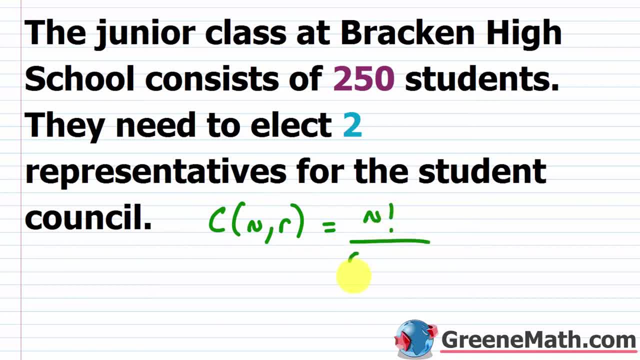 here, and this equals your n factorial over your n minus r factorial, and then times your r factorial. okay, so what ends up happening is we're dividing out the duplicates with this extra part here. okay, this is all you have to remember, because if you've got this part down from the permutations, 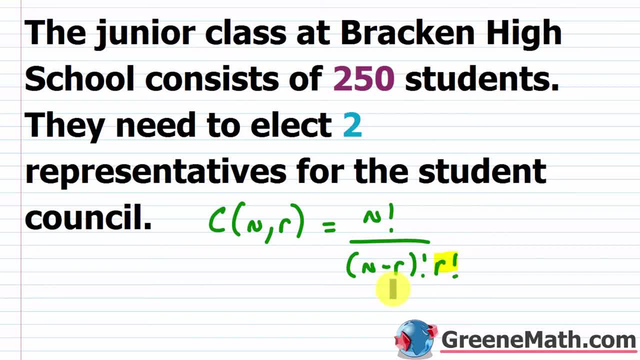 formula. you're just throwing that extra little bit there in the denominator to divide out the duplicates, and that's how you get your combination formula. okay, so let's erase this real quick. let's actually plug in the numbers. i'm going to again use my calculator here, because you would basically 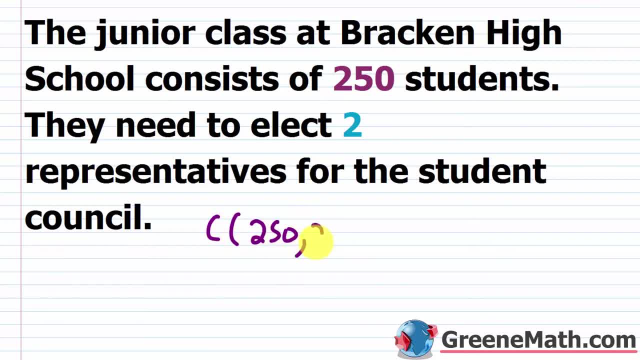 be doing this c here with 250, comma 2, and then i'm going to use my calculator here and i'm going to, and i'm not going to set this up, you're just going to hit 250 and then go to ncr and i'm going. 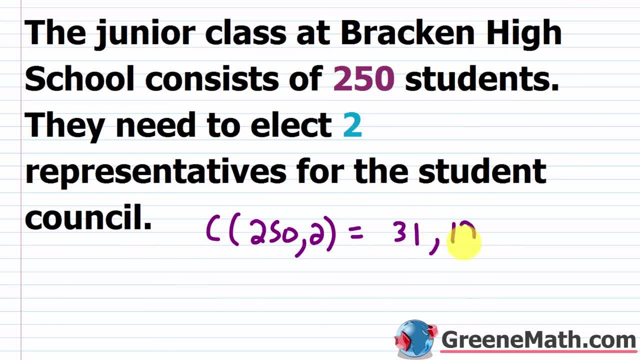 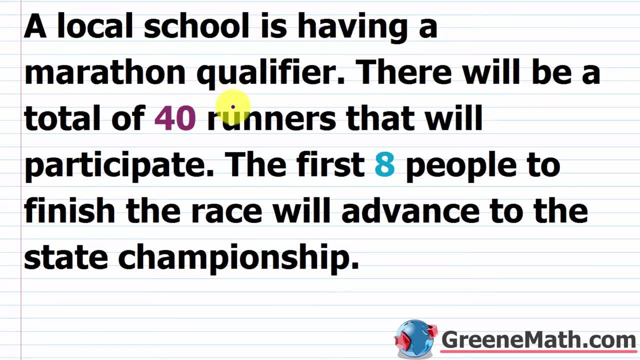 to get a result of 31 125. okay, let's look at another example. so a local high school is having a marathon qualifier. there will be a total of 40 runners that will participate. the first eight people to finish the race will advance to the state championship. okay, so do i want a permutation? 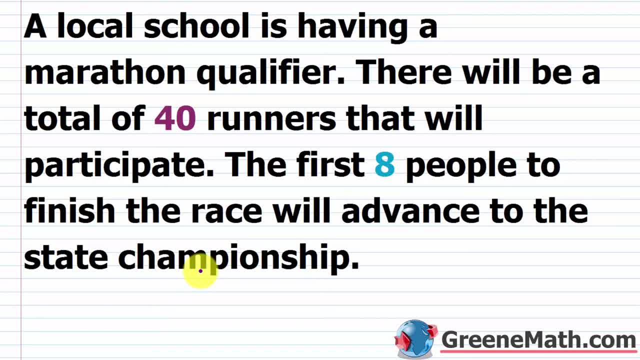 or a combination. does the order matter here? we know that repetition is not going to matter, right, because if i'm in the first position i can't also be in the third position. but does the order matter? well, no, not for our result, because it just says the first eight people, so it doesn't. 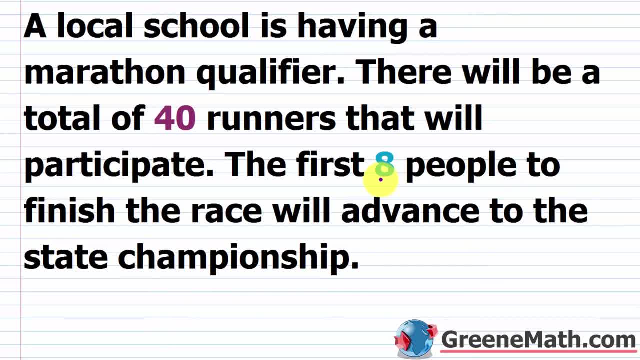 matter if i finished first or seventh, okay, as long as i'm in that top eight, okay, i'm going to advance to the state championship. so we would use a combination. here and again i would just do c and then i'm going to put 40 comma 8 again. just punch this into your calculator. you're going to do. 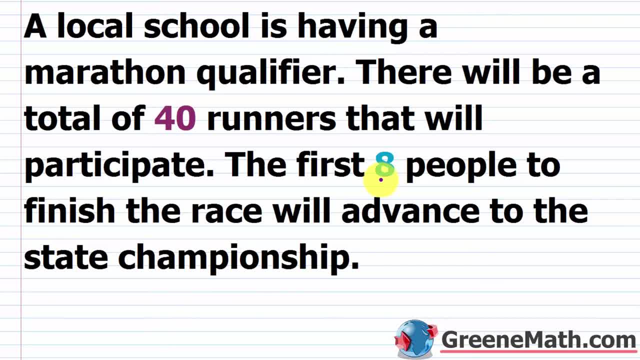 matter? well, no, not for our result, because it just says the first eight people. so it doesn't matter if i finished first or seventh. okay, so i'm going to go to the first eight people and i'm going to do that. okay, as long as i'm in that top eight, okay, i'm going to advance to the state championship. 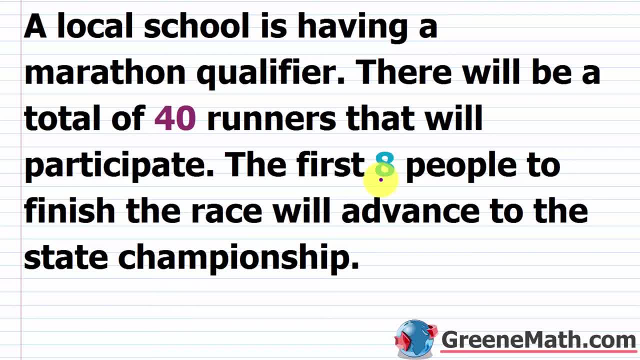 so we would use a combination here and again. i would just do c and then i'm going to put 40 comma eight again. just punch this into your calculator. you're going to do 40, choose eight and that gives us a pretty big number. it's going to be 76 million. and then you're going to have 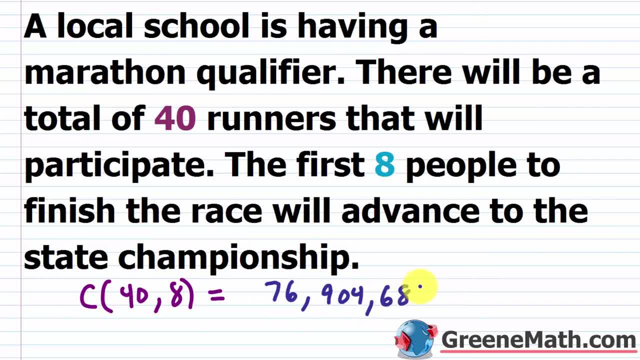 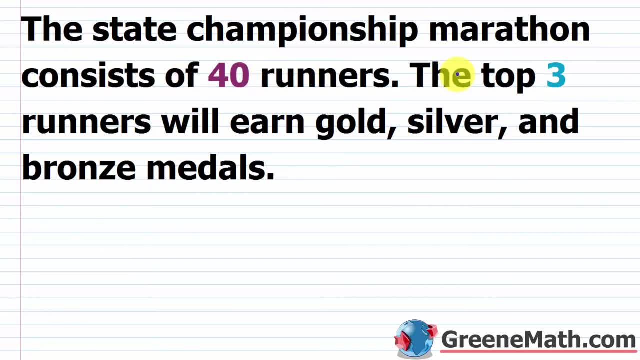 904 685. all right, let's just look at one more. so the state championship marathon consists of 40 runners. the top three runners will earn gold, silver and bronze medals. so can we have repetition here? no right, because if i finished first, i can't also finish second or third. okay, and then does the order. 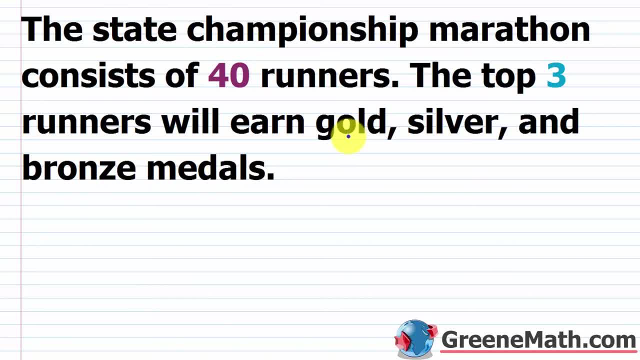 matter. well, yeah, it definitely matters. right, if i finish in first place, that's a different result than if i finish in second place. in one case i'm getting gold, in the other case i'm getting silver. so the order does matter. so i want to use the permutations formula. 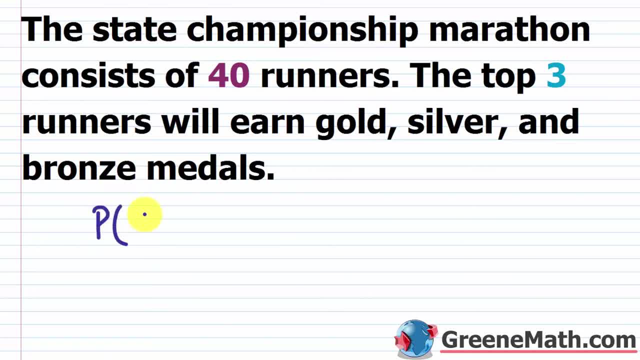 i would just use my calculator. or again, you've got this p with this 40 comma 3. if you want to say it's equal to, you can punch this into your calculator. or again, you can use your little formula. i just think it's easier to punch it in on a calculator because a lot of these, the numbers, 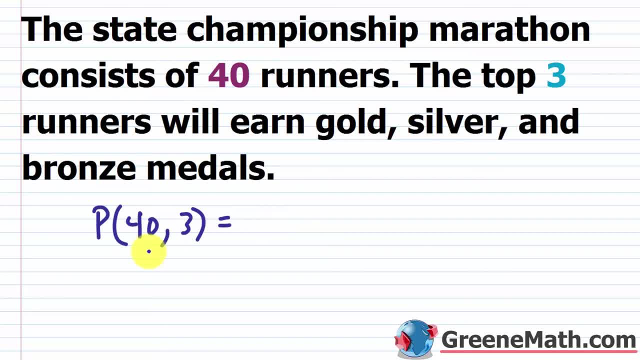 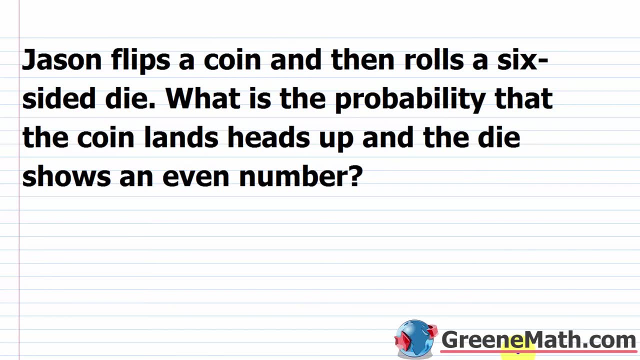 are just going to be astronomically big. so if we go ahead and punch up 40 and then you do your npr key and then three, you're going to get 59 280 as a result. in this lesson we want to look at some problems. so at some point in your algebra course or your pre-calculus course you're going to come. 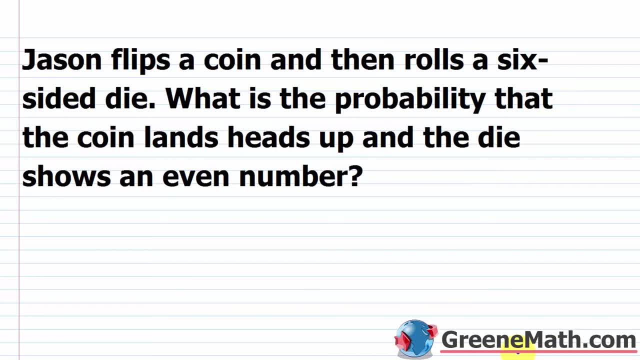 across a small section on probability and i just want to go through some basic word problems that you're going to see and talk about how we can solve these guys. so i'm just going to jump right in. i'll just kind of explain things as we go. it's a very, very easy topic overall. so jason flips a. 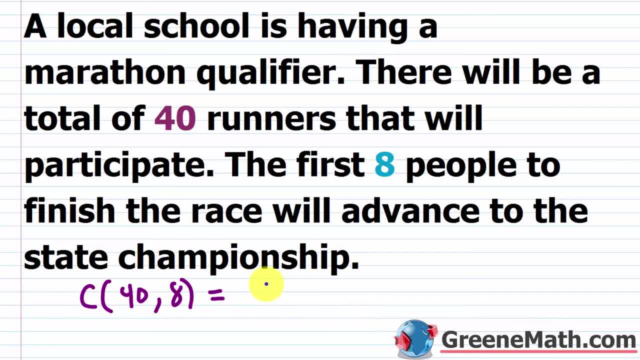 40, choose 8, and that gives us a pretty big number. it's going to be 76 million, and then you're going to have 904 685.. all right, let's just look at one more. so the state championship marathon consists of 40 runners. 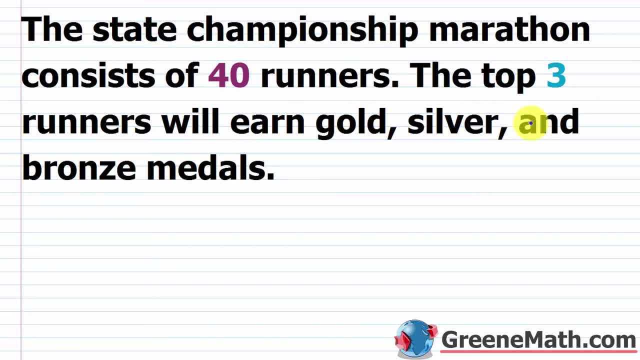 the top three runners will earn gold, silver and bronze medals. so can we have repetition here? no, right, because if i finished first, i can't also finish second or third. okay, and then does the order matter? well, yeah, it definitely matters, right? If I finish in first place, that's a different result than if I finish in second place. 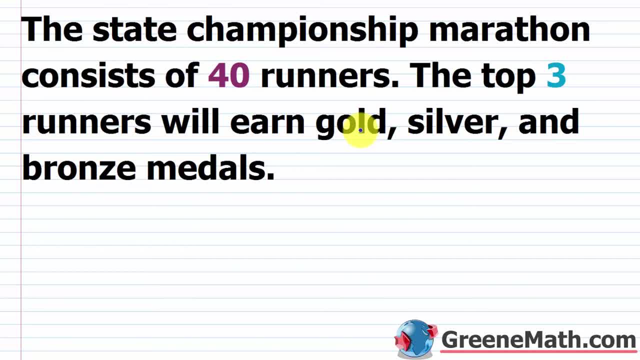 In one case I'm getting gold, In the other case I'm getting silver. So the order does matter. So I want to use the permutations formula, So I would just use my calculator. Or again, you've got this P with this 40,3, if you want to say it's equal to. 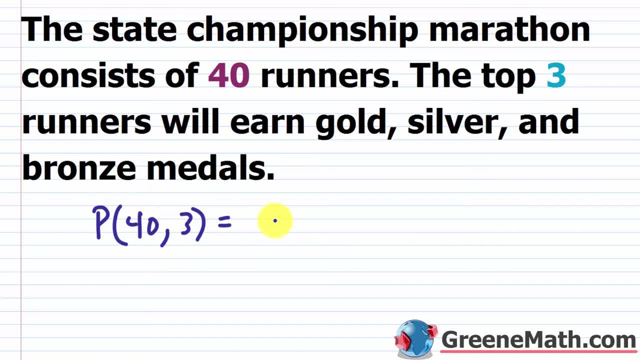 You can punch this into your calculator, Or again, you can use your little formula. I just think it's easier to punch it into my calculator because a lot of these the numbers are just going to be astronomically big. So if we go ahead and punch up 40, and then you do your NPR key and then three, you're. 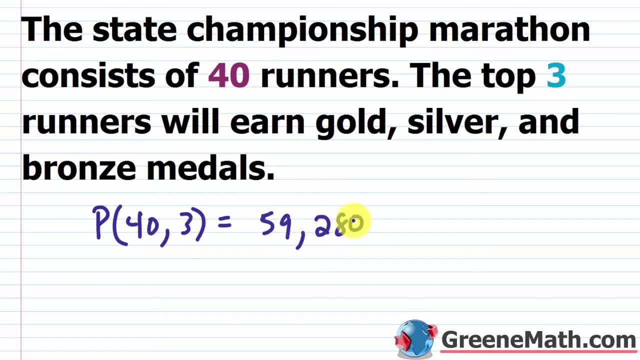 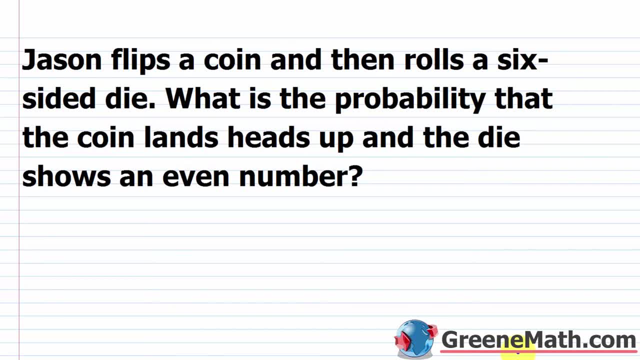 going to get 59,280 as a result. In this lesson we want to look at some probability word problems. So at some point in your algebra course or your pre-calculus course you're going to come across a small section on probability. 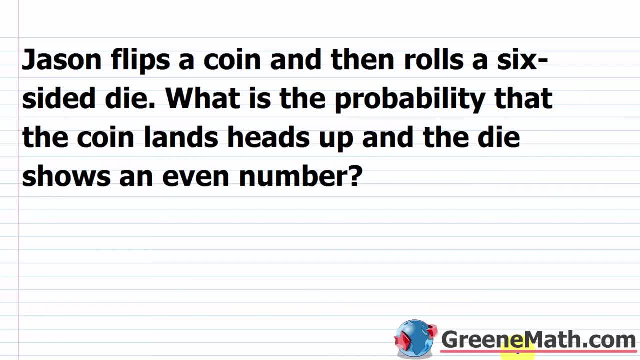 And I just want to go through some basic word problems that you're going to see and talk about how we can solve these guys. So I'm just going to jump right in. I'll just kind of explain things as we go. It's a very, very easy topic overall. 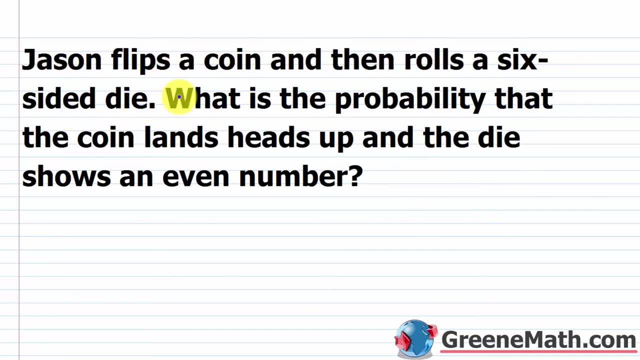 So Jason flips a coin and then rolls a six-sided die, What is the probability that the coin lands heads up- and okay, I'm going to highlight that- and the die shows an even number. Okay. So when you deal with these problems, you're going to have problems that say, and: 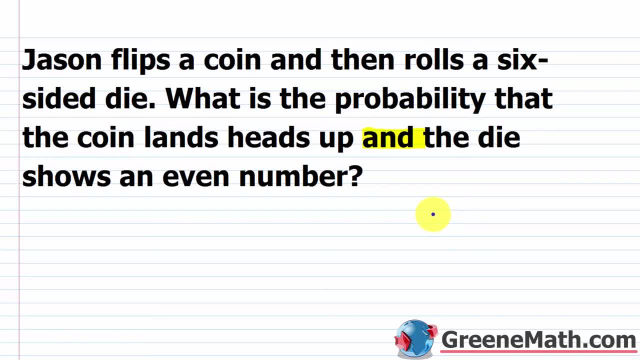 So some event occurs and some other event occurs. In this case, one event is flipping a coin and him getting a heads up, And the other event is rolling a die And getting an even number. So a two, a four or six. 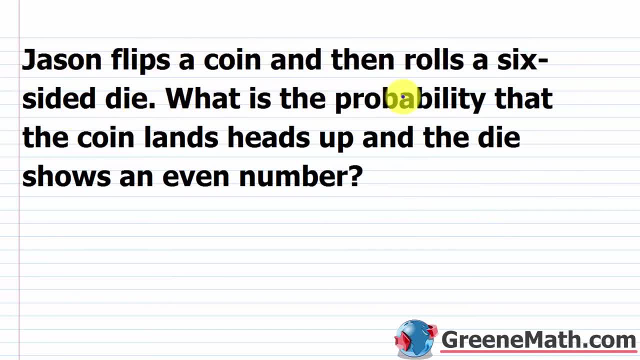 coin and then rolls a six-sided die, what is the probability that the coin lands heads up and okay, i'm going to highlight that, and the die shows an equal number of points. so i'm going to go ahead and then i'm going to say an even number, okay, so when you deal with these problems, you're going to have 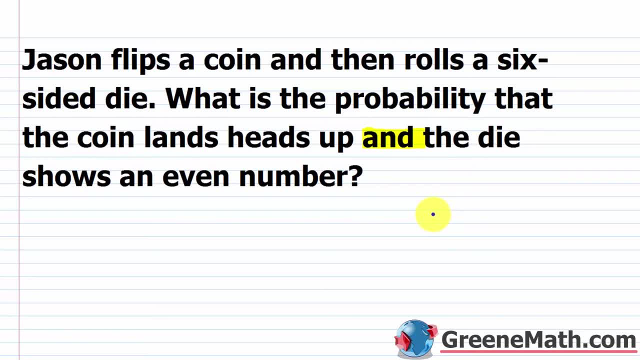 problems that say: and so some event occurs and some other event occurs. in this case, one event is flipping a coin and i'm getting a heads up, and the other event is rolling a die and getting an even number. so a two, a four or six- okay, when you hear the word and you need to be thinking about. 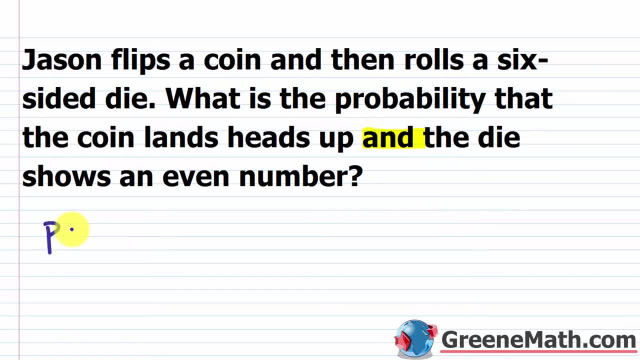 multiplication. so i would take and use this formula, the probability of some event a and some event B happening. Okay, In this case we'd say that coin landing heads up and also the die showing an even number is equal to the probability of this event A happening times. 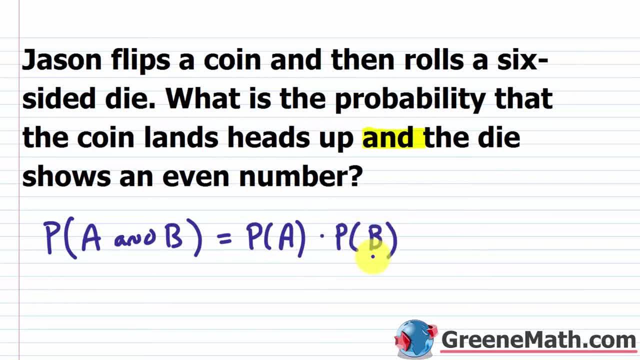 the probability of this event B happening. Okay, Now, this is given the fact that they are independent events, meaning the first event does not impact the result of the second event in any way, shape or form. Okay, If he flips a coin, that does not impact the result of rolling a six-sided die. 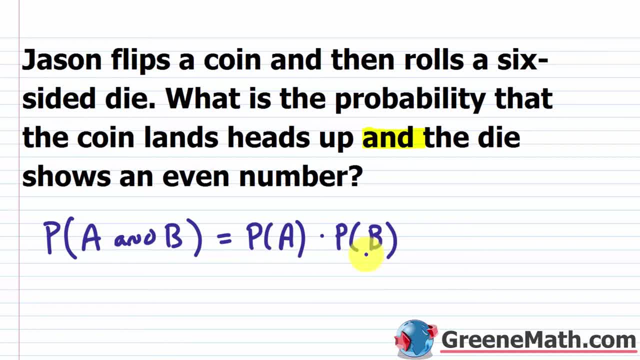 Okay, So these are independent events. We can just use this formula as it's given. So what we want to do here is just think about the fact that the probability for flipping a coin and getting a heads up is going to be what It's going to be- a half or 50%. We all know this because we've thought. 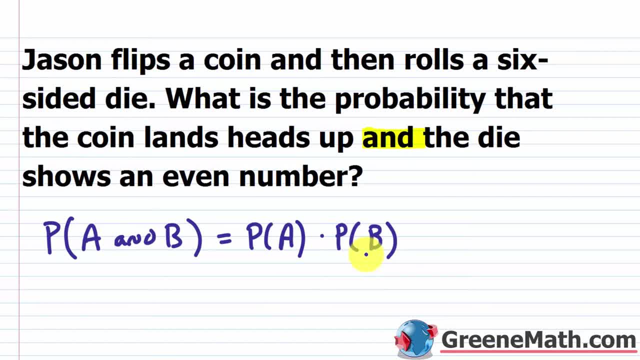 about that throughout life, at some point, flipping a coin, saying, hey, my odds are 50-50.. Well, how do we know that? Well, we know that because we've thought about that throughout life at some point. How do we show this mathematically? Where does that 50-50 or the 50% come from? Well, essentially, 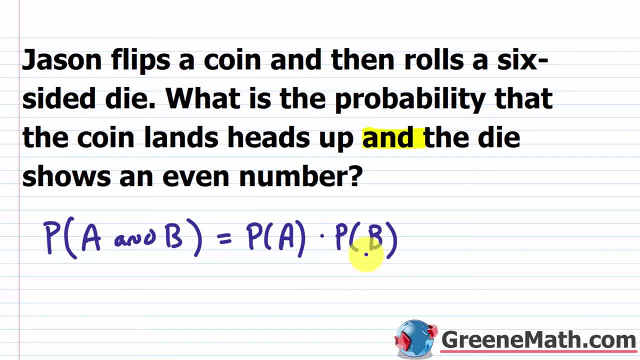 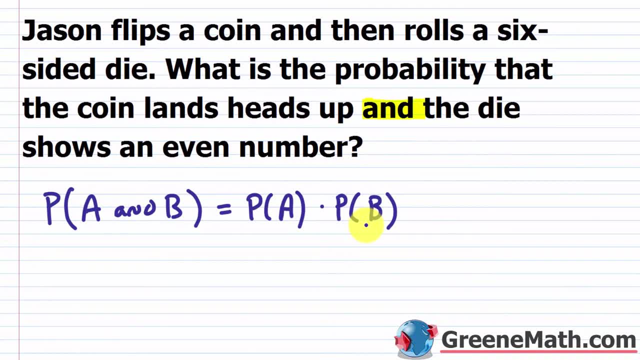 what you do is you think about the number of different ways that you can get an outcome from flipping a coin. Well, you can basically get a heads up or tails up, right? So there's two possibilities. So I'll put that in the denominator and then think about what you're looking for. 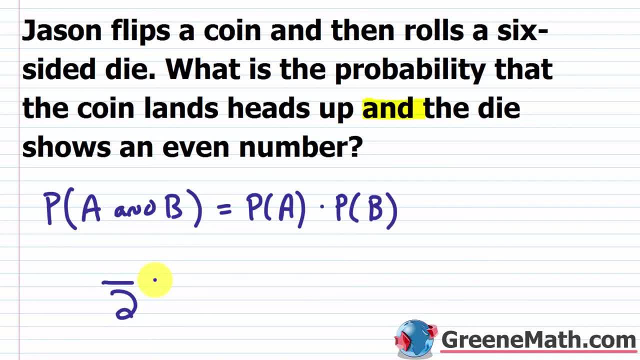 What's the result? Well, I want a heads up, and that can only happen one way, right, So I would put that number in the numerator, Okay, And as we do more of these, this will make more sense. But essentially, this is the number of ways that you can get an outcome from flipping a coin. 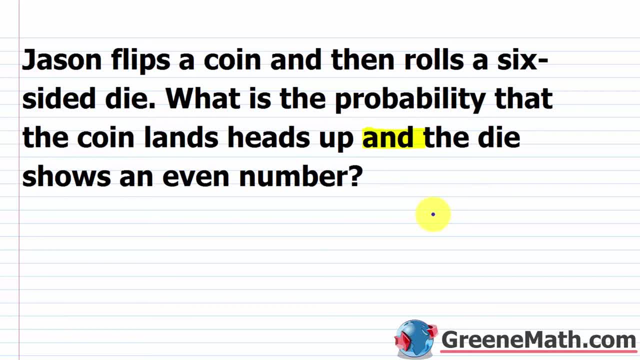 Okay When you hear the word and you need to be thinking about multiplication. So I would take and use this formula: The probability of some event A and some event B happening- okay, in this case we'd say the coin landing heads up and also the die showing an even number is equal to the probability. 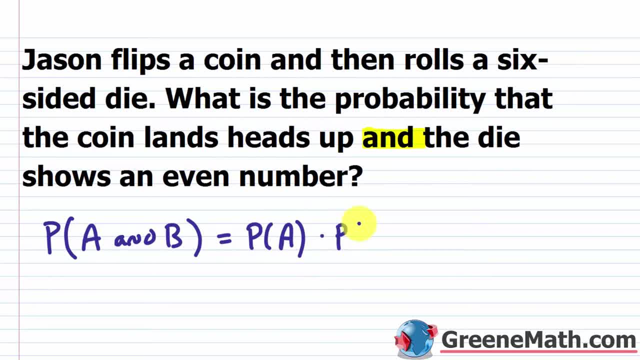 of this event A happening times. the probability of this event B happening: Okay, Now, this is good, Okay. Okay, Given the fact that they are independent events, meaning the first event does not impact the result of the second event in any way, shape or form. 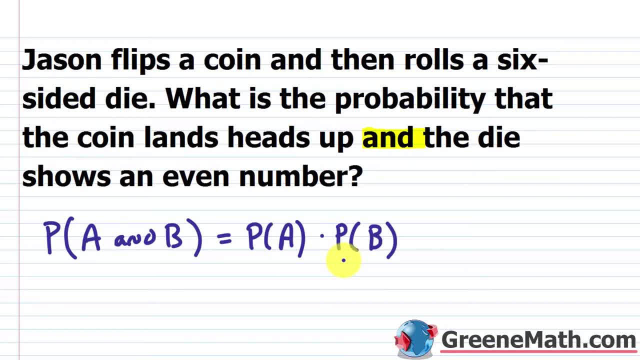 Okay, If he flips a coin, that does not impact the result of rolling a six sided die. Okay. So these are independent events. We can just use this formula as it's given. So what we want to do here is just think about the fact that the probability for flipping 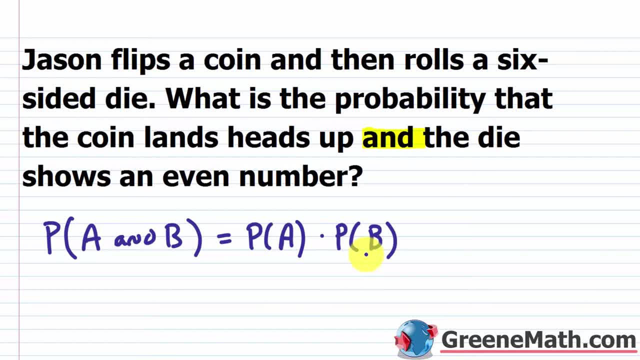 a coin and getting a heads up is going to be what It's going to be: a half or 50%. We all know this because we've thought about that throughout life at some point flipping a coin saying Hey, my odds are 50, 50.. 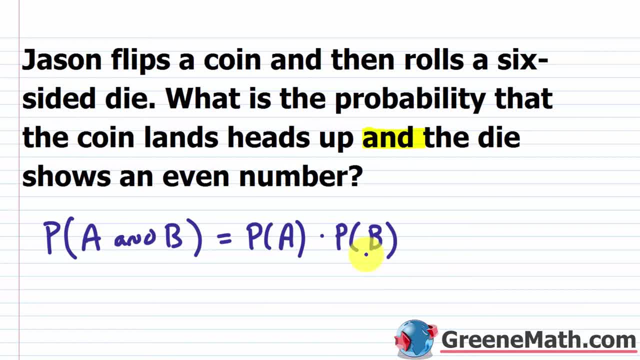 Well, how do we show this mathematically? Where does that 50, 50 or the 50% come from? Well, essentially, what you do is you think about the number of different ways that you can get an outcome from flipping a coin. 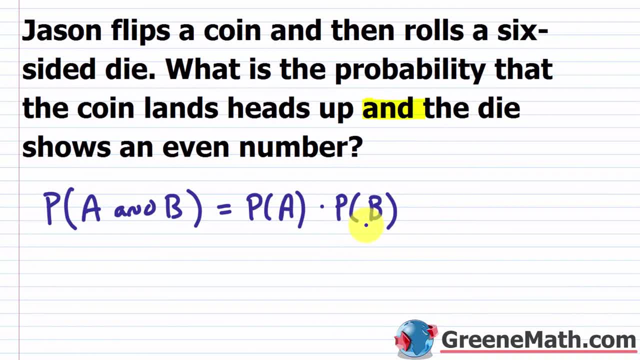 Well, you can basically get a heads up or tails up, right? So there's two possibilities. So I'll put that in the denominator and then think about what you're looking for. What's the result? Well, I want a heads up, and that can only happen one way, right? 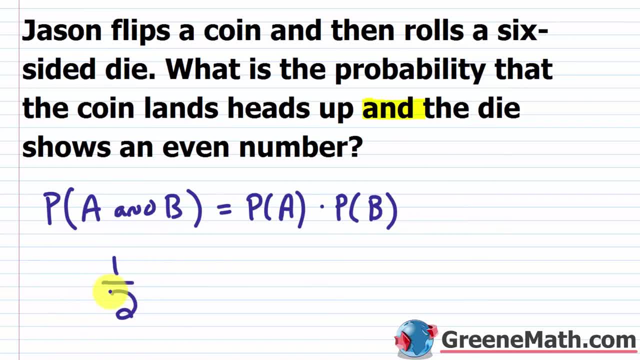 So I would put that number in the numerator, Okay, And as we do more of these, this will make more sense, But essentially, this is the formula you want to use. That's where one half comes from. This is basically the number of favorable outcomes. 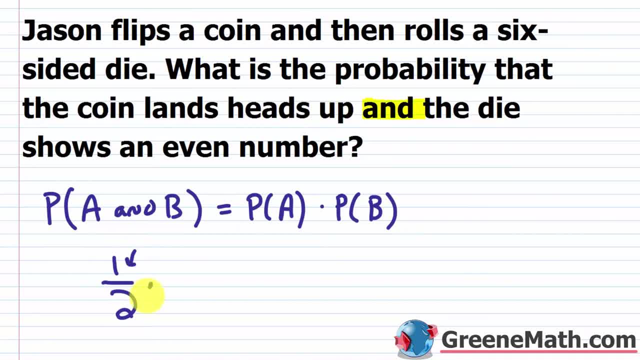 In this case, a favorable outcome would be landing heads up over the total number of possible outcomes, And the possible outcomes here would be landing heads up or landing tails up. Okay, So I know that's one half, So let's just say that this satisfies. 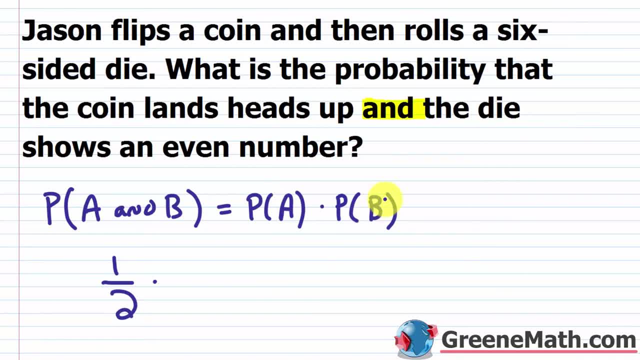 The probability of event a. now what about the probability of event B? Let's say, that's the die showing an even number. Well, with a die, if it's six sided, it can land on a one. Let me just kind of write this down here in a different color: a one, a two, a three. 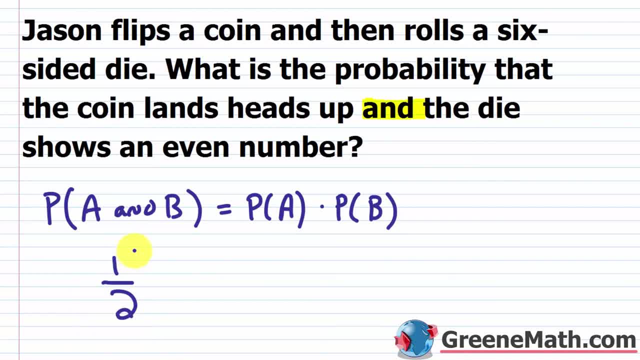 This is the formula you want to use. That's where one half comes from. This is basically the number of favorable outcomes. In this case, a favorable outcome would be landing heads up over the total number of possible outcomes, And the possible outcomes here would be: 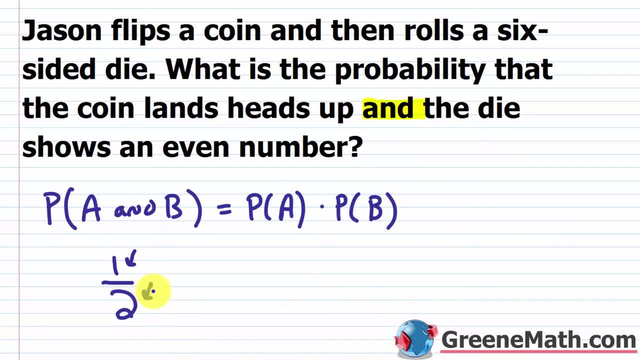 landing heads up or landing tails up. Okay, So I know that's one half. So let's just say that this satisfies the probability of event A. Now, what about the probability of event B? Let's say that's the die showing an even number. Well, with a die, if it's six-sided, it can land on. 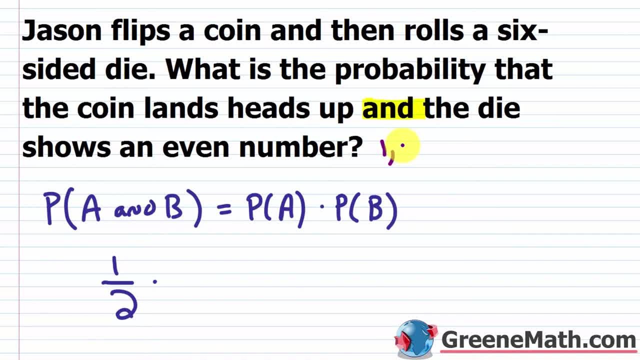 a one- Let me just kind of write this down here in a different color: A one, a two, a three, a four, a five or six. So we know that the two is an even number, the four and the six. Okay So. 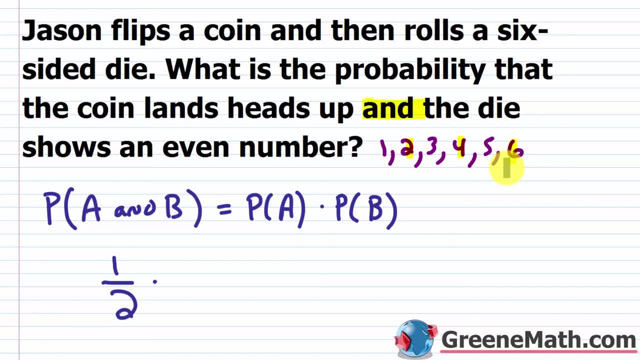 two, four and six. those are even numbers. So how many different favorable outcomes can I have? Well, I have one, two, three favorable outcomes that are possible out of a total of six. So I would put three over six, which you can simplify to one half, Okay. 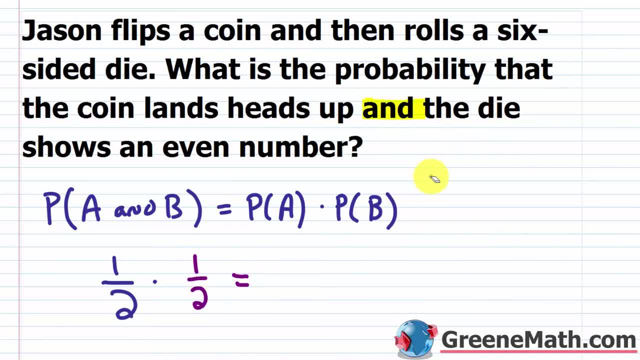 And then you just multiply the two together, And let me just kind of erase this. You multiply the two together and you get one fourth. Okay, Now you can leave it as a fraction and say it's one fourth of the probability, or you can convert it to a decimal, which is 0.25,. 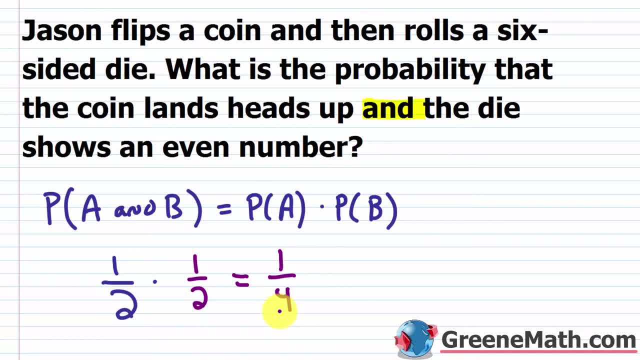 and then to a percentage and say it's 25%. Okay, So essentially, the probability of this Jason guy flipping a coin and getting a heads up and also taking a die and rolling it and getting an even number is 25%. Okay, Let's look at: 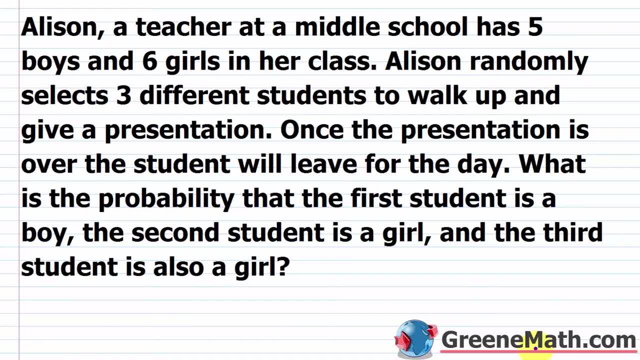 a slightly more challenging problem And in this case we're going to have dependent events. So Allison, a teacher out of middle school, has five boys and six girls in her class. Allison randomly selects three different students to walk up and give a presentation. 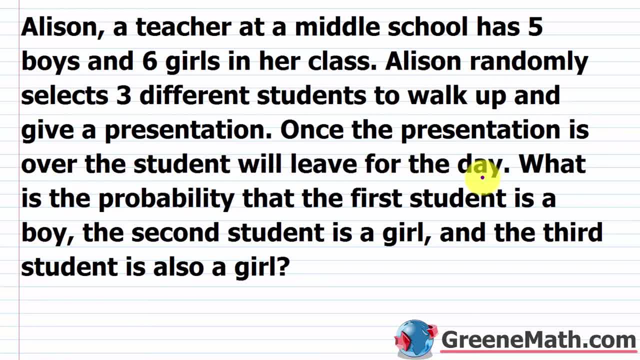 Once the presentation is over, the student will leave for the day. What is the probability that the first student is a boy, the second student is a girl and the third student is also a girl? So you see, the problem here is that these events are not independent. okay, Once she picks a. 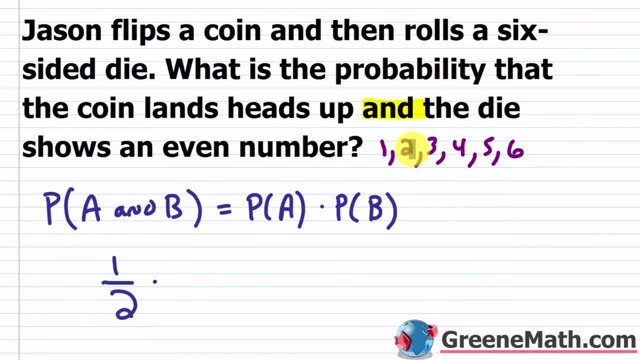 a four, a five or six. So we know that the two is an even number, the four and the six. Okay, So two, four and six, those are even numbers. So how many different favorable outcomes can I have? Well, I have one, two. 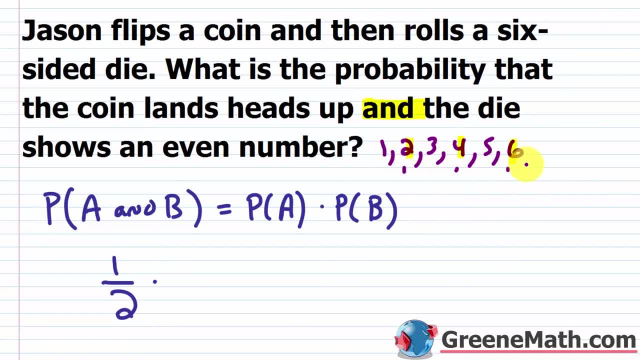 Three favorable outcomes that are possible out of a total of six. So I would put three over six, which you can simplify to one half, Okay, And then you just multiply the two together, And let me just kind of erase this. You multiply the two together and you get one four. 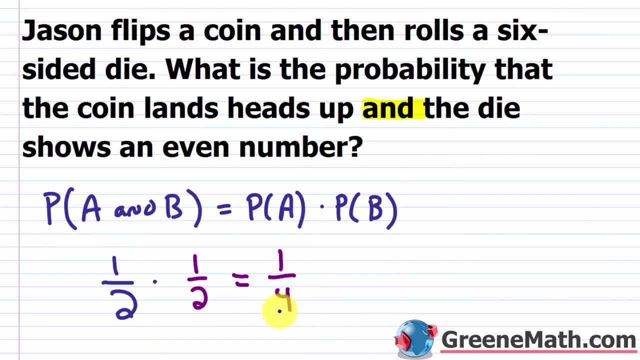 Okay, Now you can leave it as a fraction, say it's one fourth of the probability, where you can convert it to a decimal, which is 0.25, and then to a percentage and say it's 25%. Okay, So essentially the probability of this, Jason guy. 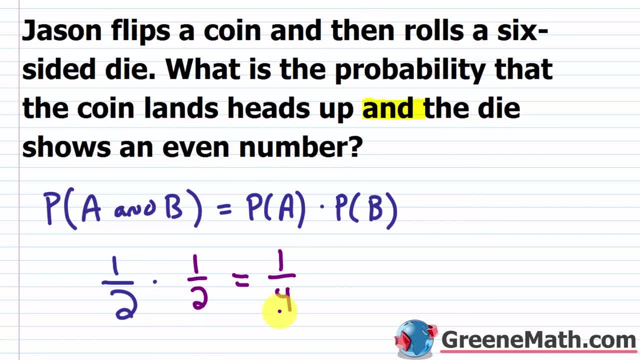 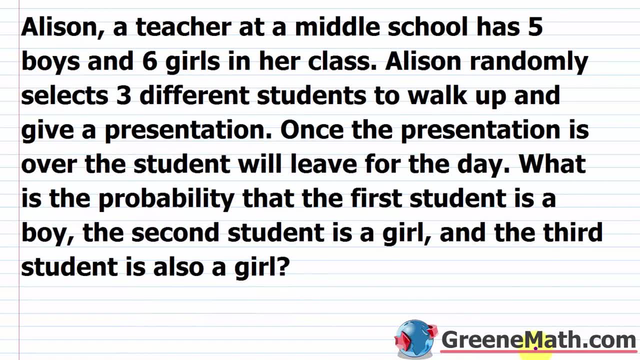 Okay, Flipping a coin and getting a heads up and also taking a die and rolling it and getting an even number is 25%. Okay, Let's look at a slightly more challenging problem And in this case we're going to have dependent events. 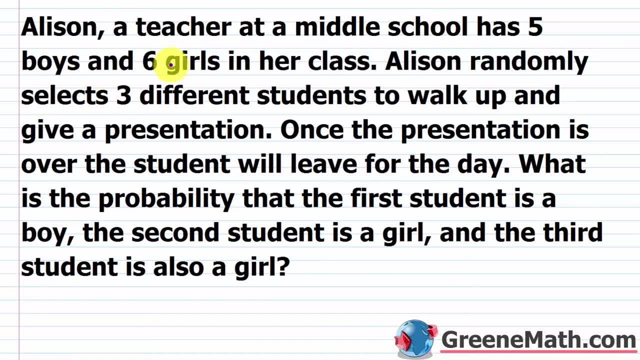 So Alison, a teacher out of middle school, has five boys and six girls in our class. Alison randomly selects three different students to walk up and give a presentation. Once the presentation is over, the student will leave for the day. What is the probability? that the first student is a boy, the second student is a girl and 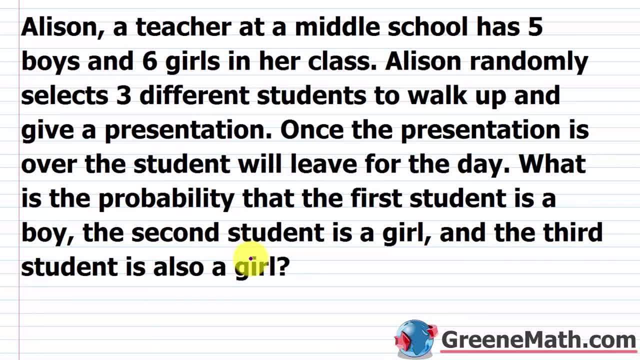 the third student is also a girl. So you see, the problem here is that these events are not independent. Okay, Once she picks a student and we're looking for her to pick a boy first, Okay. Then the next time we want her to pick a girl. 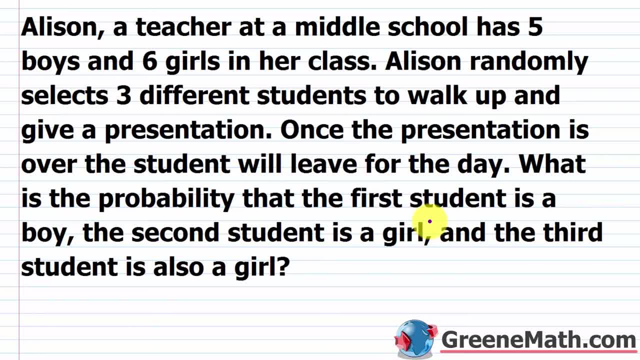 And then the next time we want her to pick a girl. But each time she's picking, the class size is changing, Right? So the number of boys is changing, Number of girls is changing, Whatever it is in that, In that scenario, but the class size is constantly changing. 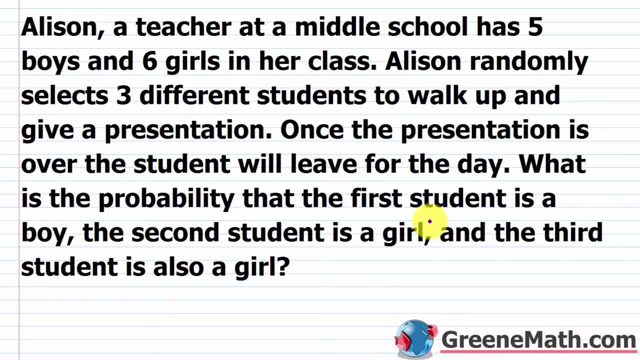 So we have to readjust our probability. Okay, So we're still going to think about multiplying the probabilities together, But you use a different formula for this. If it was just two things, here it's three, but let's say it was two things. 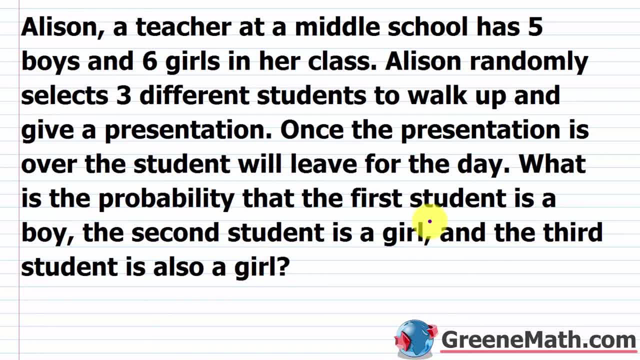 student and we're looking for her to pick a boy first, okay. Then the next time we want her to pick a girl, and then the next time we want her to pick a girl. but each time she's picking, the class size is changing right? So the number of boys is changing, the number of girls is. 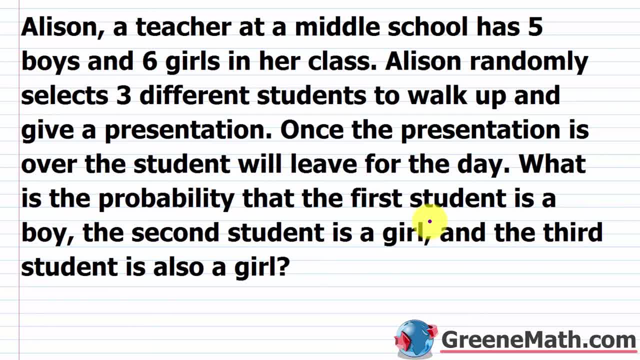 changing, whatever it is in that scenario. but the class size is constantly changing, so we have to readjust our probability. okay? So we're still going to think about multiple choice, right? So we're still going to think about multiple choice, right? So we're still. 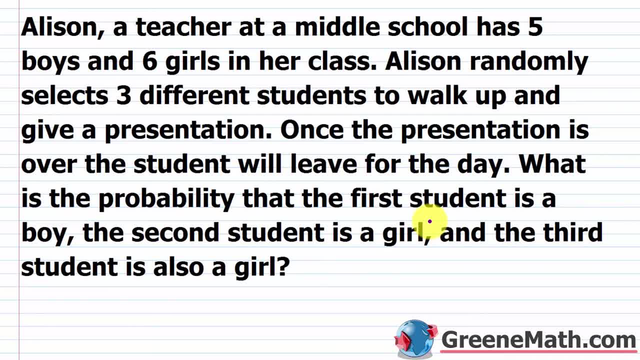 multiplying the probabilities together. but you use a different formula for this. If it was just two things here, it's three, but let's say it was two things. So the probability of A and B- okay, If these guys are dependent, it's just two. it would be the probability of A times the 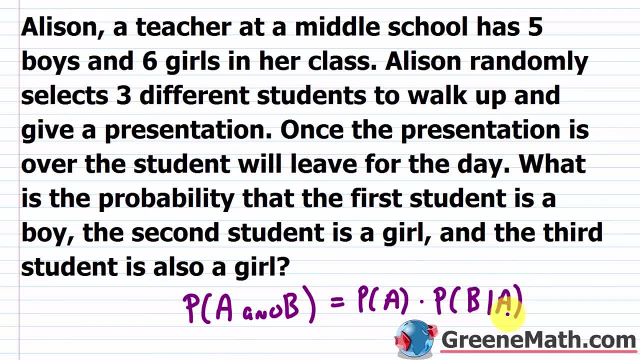 probability of B, given that A has happened. okay, So, given that A has happened, what's the probability of B happening? okay, And in this case we're going to adjust it because we have one more thing to consider, because now we're thinking about the probability that the first student is a. 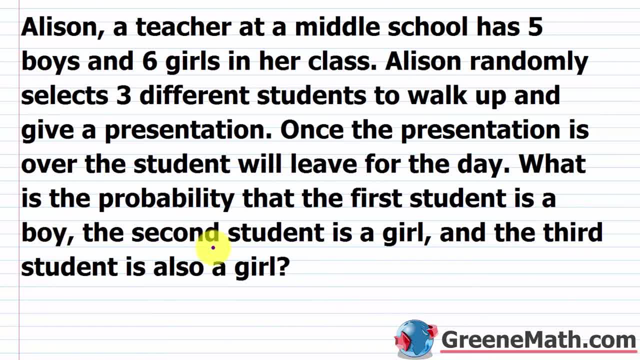 boy: okay, So that happens. Then the probability that the next student is a girl: okay, And then the probability that the third student is also a girl. So again you have. and so you're thinking about multiplication. okay, So what is the probability on the first graph that that student? 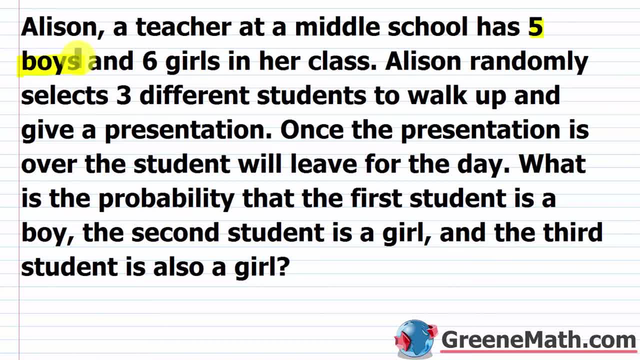 is a boy. Well, there's going to be five boys, okay. So there's five possible choices in there. that's going to be boys. Out of a total of five possible choices, there's going to be five boys. plus six is 11, 11 total students. So the first number we're looking at is- I'm just going to write- 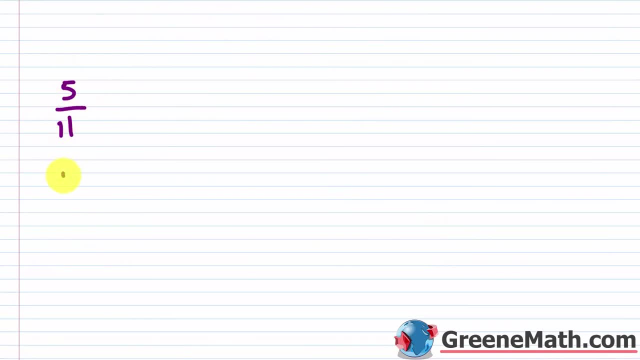 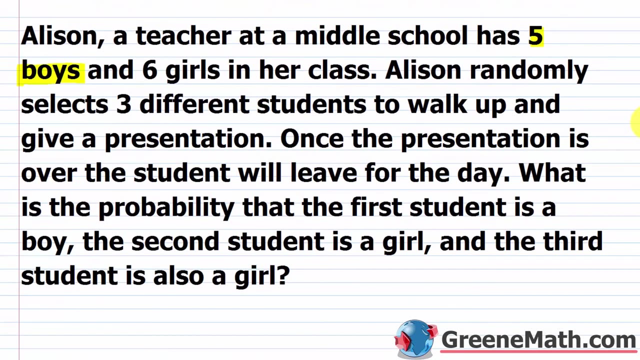 this down here, five over 11.. I'm just going to put this as the first, okay, So the second is going to be what? Well, if I go back up, I know that the student leaves. he can't be rechosen now. 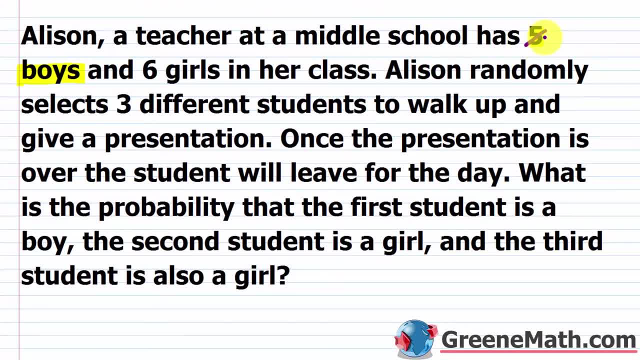 and there's going to now be what? Well, there's one less boy, so there's four boys and there's the same number of girls, but the total number in the class now is four plus six or 10, okay. So the total number in the class now is four plus six or 10, okay. So the total number 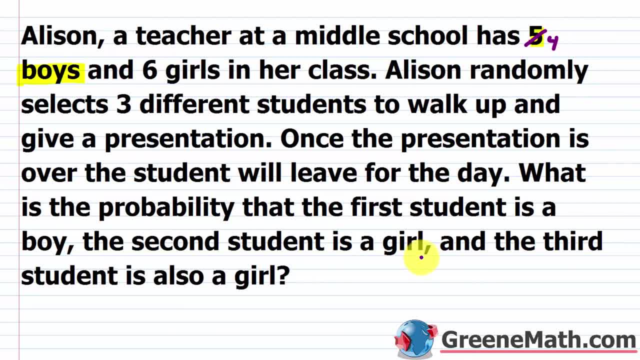 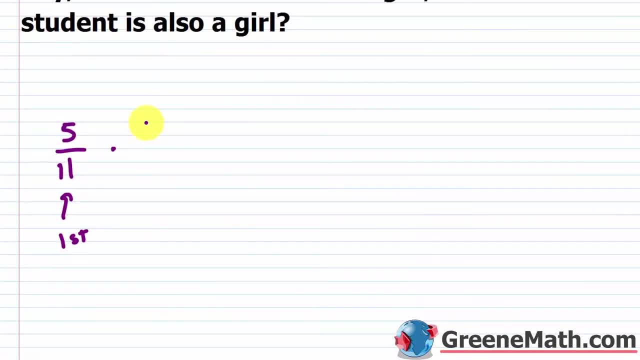 if I think about picking a girl now, it's going to be six girls out of a 10-student classroom. okay, Let me just erase this. So let's go down here and put that now it's six over 10, okay, So. 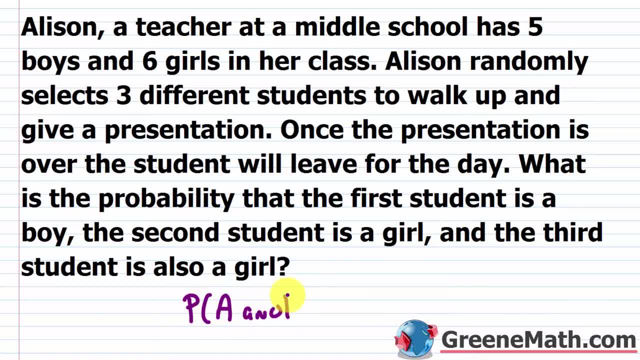 So the probability of A and B? Okay, If these guys are dependent, it's just two. It would be the probability of A times the probability of B, given that A has happened. Okay, So, given that A has happened, what's the probability of B happening? 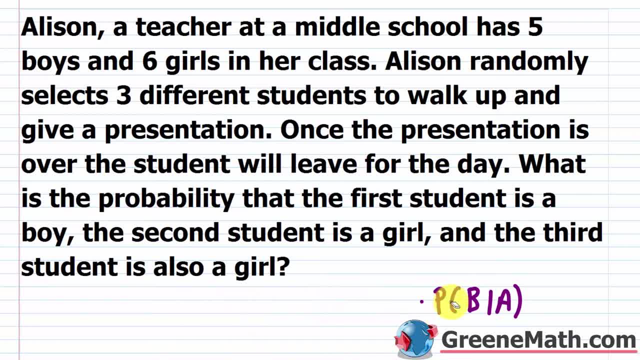 Okay, And in this case we're going to adjust it because we have one more thing to consider, because now we're thinking about the probability that the first student is a boy- Okay, So that happens. Then the probability that the next student is a girl. 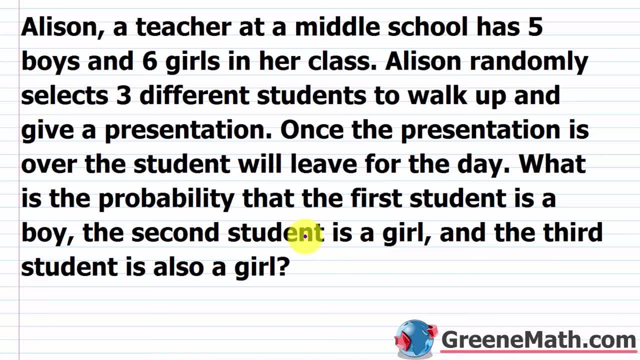 Okay. And then the probability that the third student is also a girl. So again, you have, and so you're thinking about multiplication, Okay. So what is the probability on the first graph that that student is a boy? Well, there's going to be five boys. 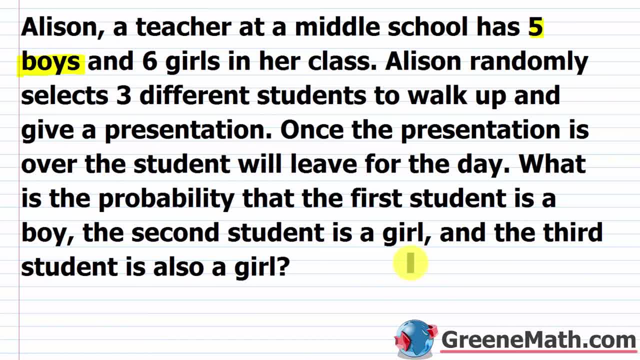 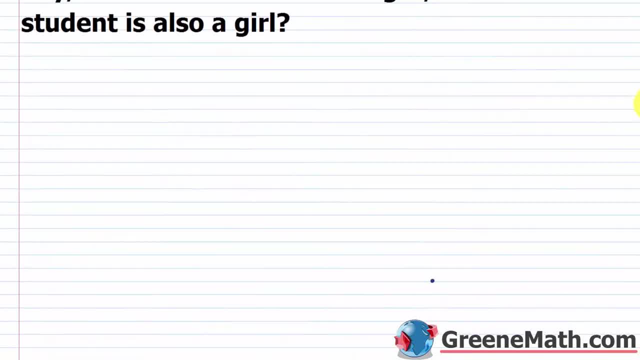 Okay, So there's five possible choices in there. That's going to be boys. out of a total of five plus six is 11, 11 total students. So the first number we're looking at is- I'm just going to write this down here: 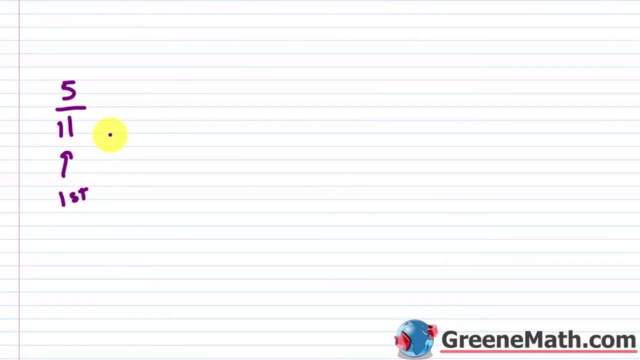 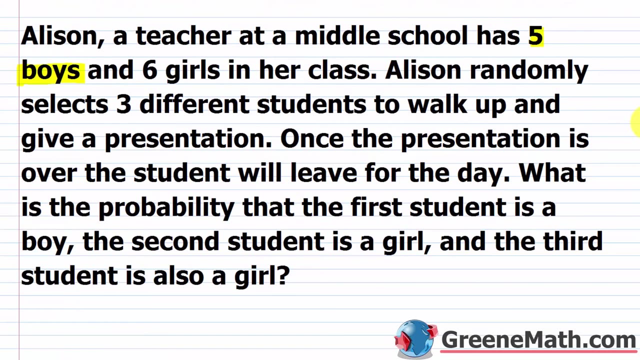 Five over 11.. I'm just going to put this as the first. Okay, So the second is going to be what? Well, if I go back up, I know that the student leaves, he can't be rechosen now, And there's going to now be what. 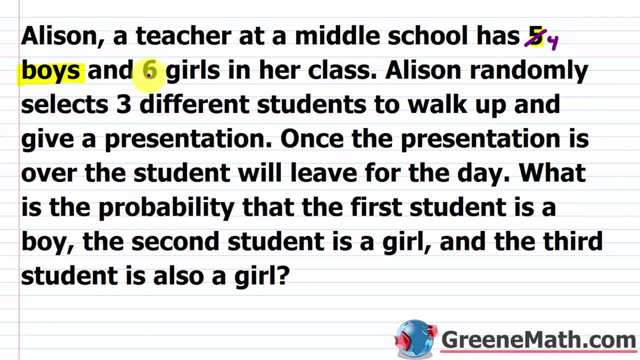 Well, there's one left, So there's four boys and there's the same number of girls, But the total number in the class now is four plus six or 10.. Okay, So if I think about picking a girl now, it's going to be six girls out of a 10 student classroom. 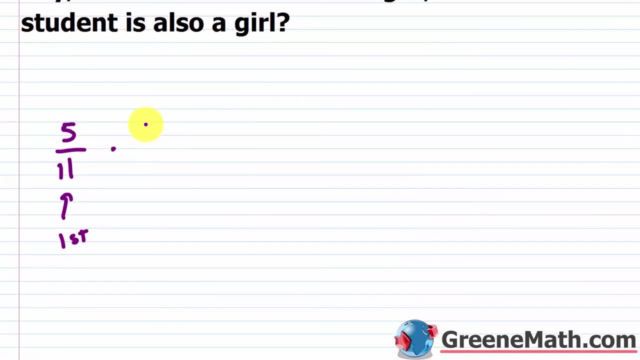 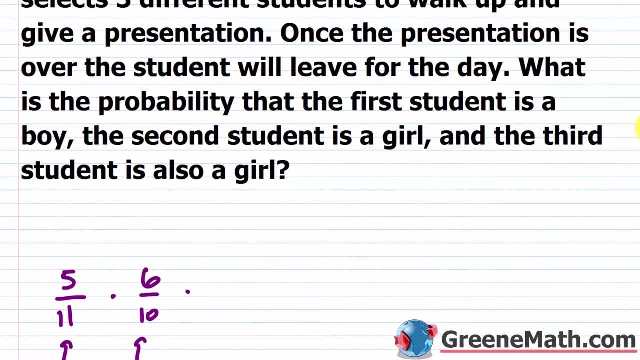 Okay, Let me just erase this. So let's go down here and put that now it's six over 10.. Okay, So this is second, you'd say. And now what's going to happen for the third choice when we go back up? 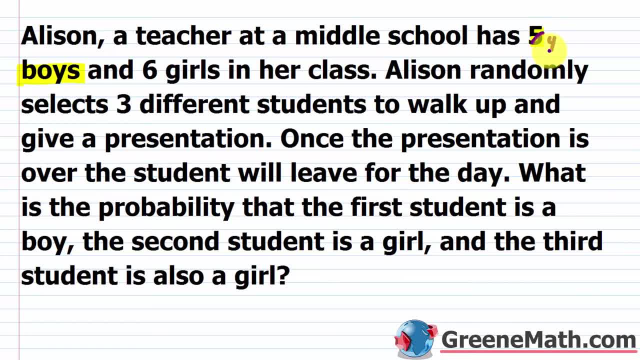 Well, now there's- let me just kind of scratch this out Again. say, this is four, This is going to go down to five. There's a total of nine students and there's five girls, So there's five over nine. 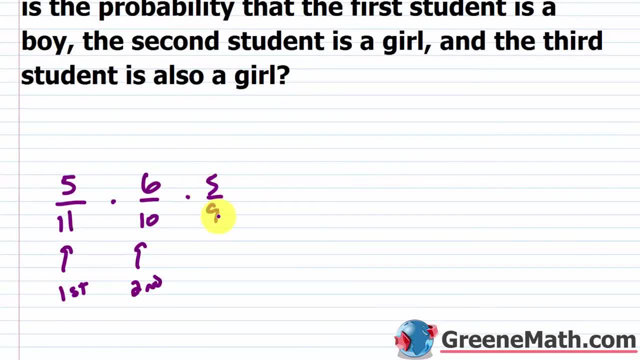 Okay, Let me just erase this again. And now I'll say: this is five over nine And this is going to be the third pick. Okay, So the probability of picking a boy on the first run is five over 11.. Then, given the fact that that event has already happened, 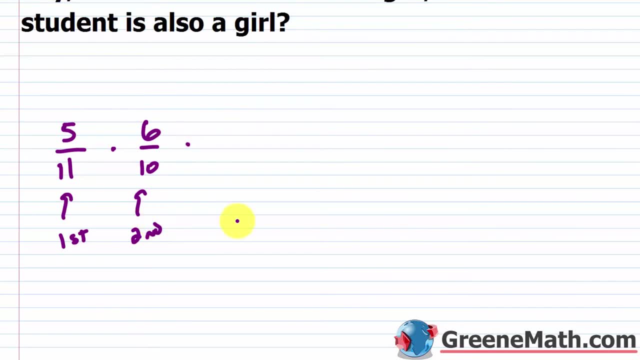 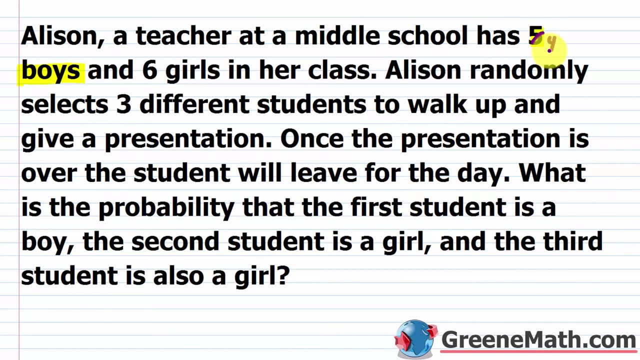 this is second, you'd say. And now what's going to happen for the third choice when we go back up? Well, now there's- let me just kind of scratch this out again- say: this is four, this is going to go down to five. There's a total of nine students and there's five girls, So there's. 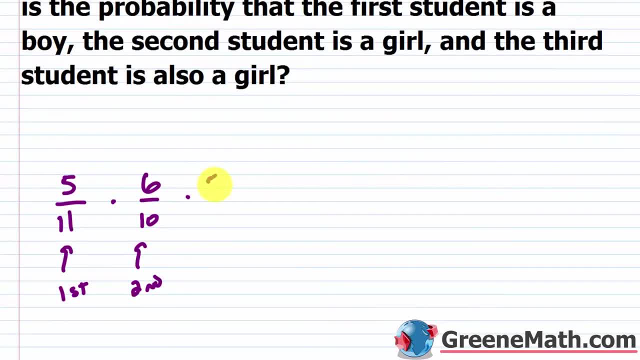 five over nine. okay, So there's a total of nine students and there's five girls, So there's five. Okay, let me just erase this again. And now I'll say: this is five over nine and this is going to be the third pick. okay, So the probability of picking a boy on the first run is five over 11.. 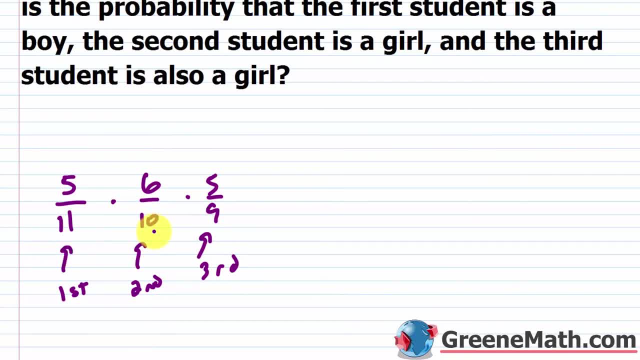 Then, given the fact that that event has already happened, now, there's a six over 10 probability of picking a girl. Now, given the fact that both of those events happened, the probability on the third pick that it's a girl is five over nine. okay, So again to get the final probability, or 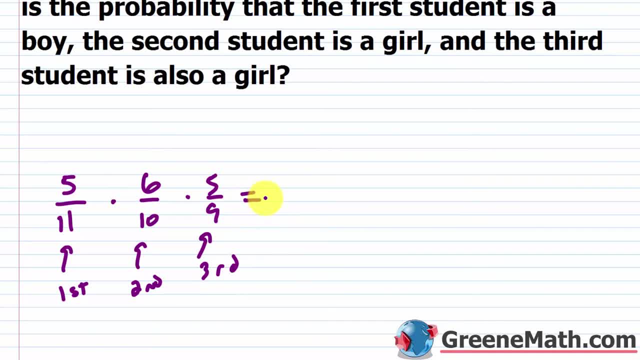 the probability that all these events are going to happen, you're going to have to pick a girl. So this: and she picks the first student as a boy, and she picks the second student as a girl, and she picks the third student as a girl, it's going to be the product of these probabilities. 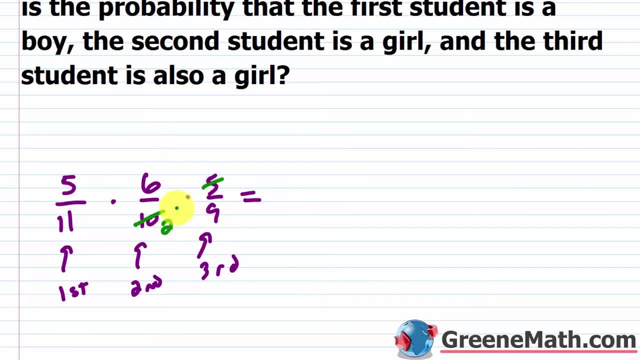 So, before we multiply, notice, you can cancel this with this and get a two here, And then six divided by two would be three, and then nine divided by three would be three. Okay, so I'm going to put a one here, And basically what you'd have is five times one or five over. 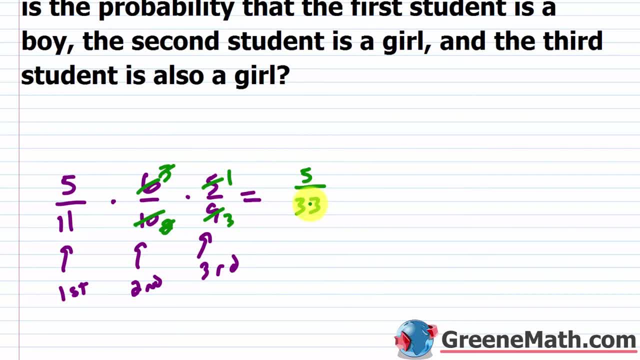 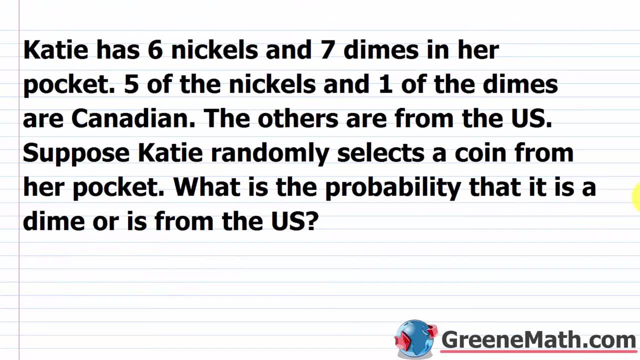 11 times three, which is 33.. So you have five over 33, which is the probability of picking a boy, then a girl, then a girl. All right, so now let's talk about some word problems that involve this or So, when event A 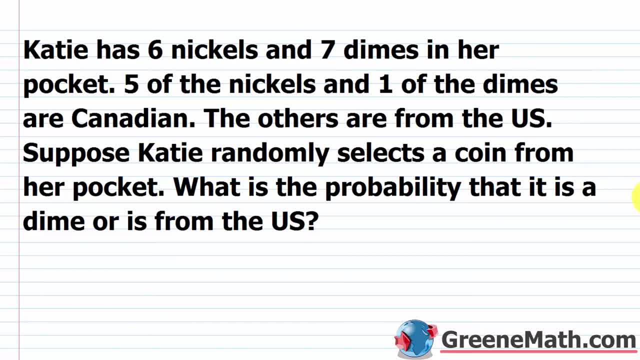 happens or an event B happens. So with this we're going to be adding now. So when you hear and you got to be thinking about multiplication, When you hear or you've got to be thinking about adding, okay, But there's a trick to this. And let me just kind of go through this with this. 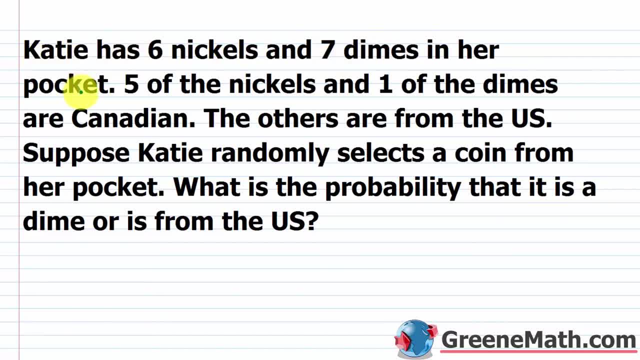 problem. So Katie has six nickels and seven nickels. So Katie has six nickels and seven dimes in her pocket. Five of the nickels and one of the dimes are Canadian. The others are from the US. Suppose Katie randomly selects a coin from her pocket. What is the probability that it is a? 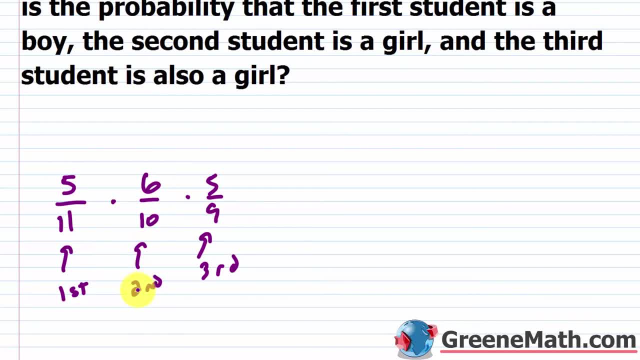 now, there's a six over 10 probability of picking a girl. Now, given the fact that both of those events happened, the probability on the third pick that it's a girl is five over nine. Okay, So again to get the final probability, or the probability that all these events happen. 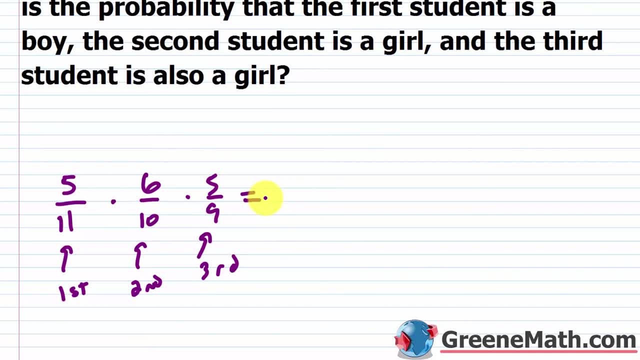 So this: and she picks the first student as a boy, and she picks the second student as a girl and she picks the third student as a girl. It's going to be the product of these probabilities. So before we multiply, notice you can cancel this with this and get a two here. 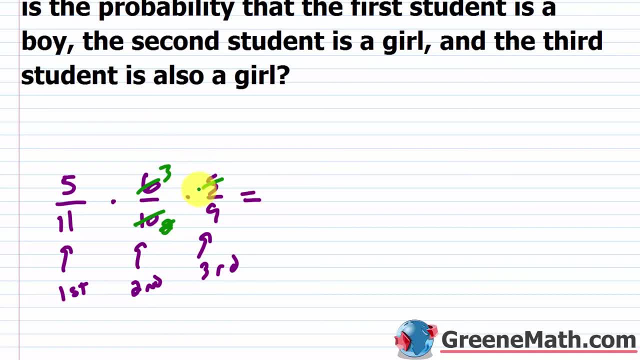 And then six divided by two would be three, And then nine divided by three would be three. Okay, So I'm going to put a one here And basically what you'd have is five times one, or five over 11 times three, which is 33.. 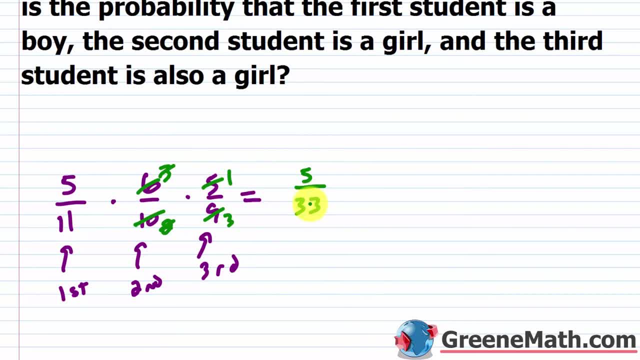 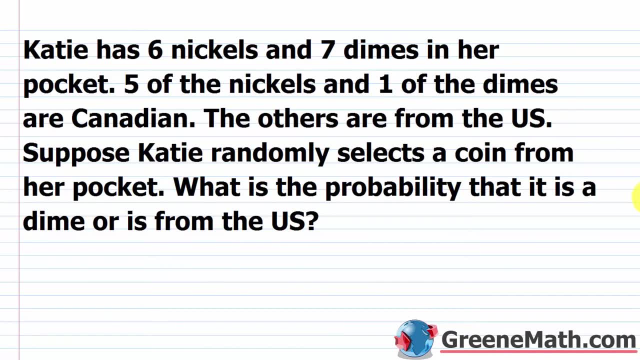 So you have five over 33,, which is the probability of picking a boy, then a girl, then a girl. All right, So now let's talk about some word problems that involve this Or so, when event a happens or an event B happens, 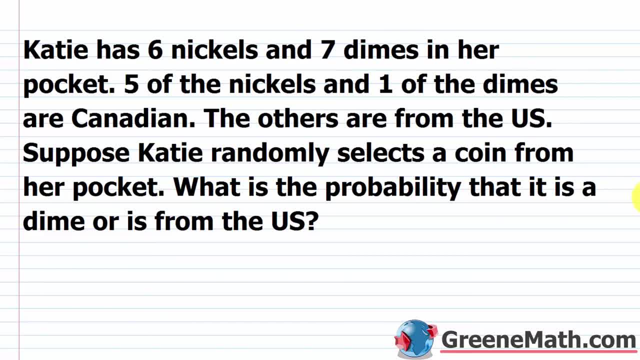 So with this, we're going to be adding now. So when you hear, and you got to be thinking about multiplication, when you hear, or you've got to be thinking about adding, okay, but there's a trick to this, And let me just kind of go through this with this problem. 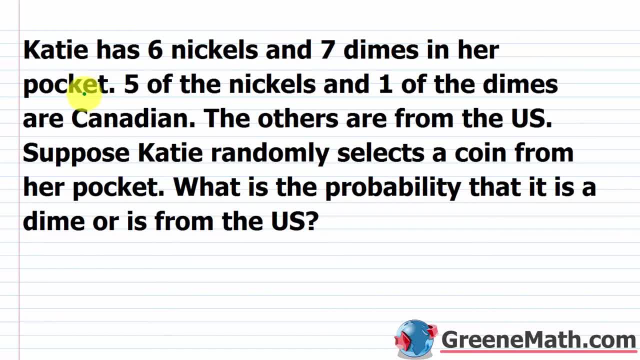 So Katie has six nickels and seven dimes in her pocket. five of the nickels and one of the dimes are Canadian. The others are from the U? S. suppose Katie randomly selects a coin from her pocket, What is the probability that it is a dime or is from the 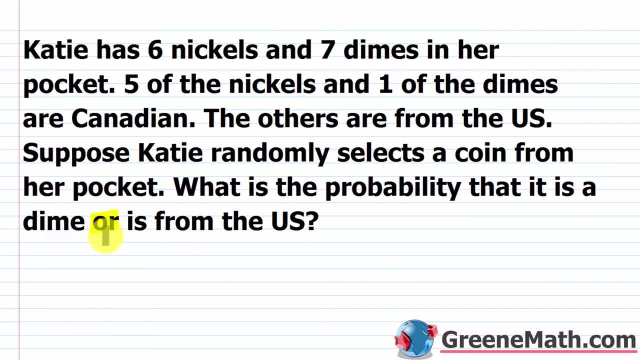 U S- this is the key word here- the or. okay. So what you want to be thinking about is the, the probability of some event a happening or some event B happening is the probability of the event a happening plus the probability of the event B happening minus. 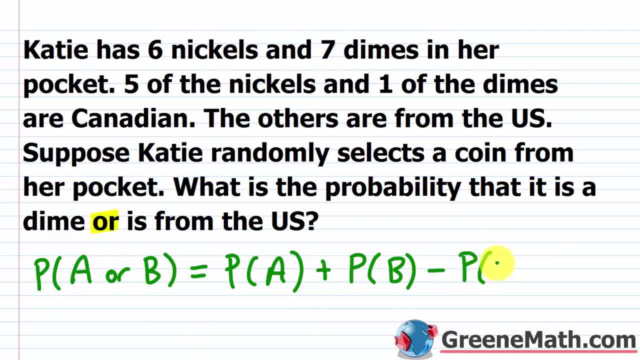 Okay, This is important, minus the probability of a and B happening. Okay, And I know a lot of people use set notation there, so you might see this as well. Okay, So the intersection of a and B, however you want to write it. 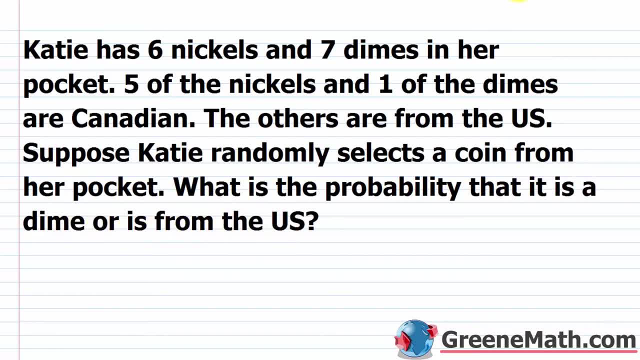 dime, or is from the US. This is the key word here- the or, okay. So what you want to be thinking about is the probability of some event A happening or some event B happening. is the probability of some event B happening plus the probability of the event B happening minus? okay, this is. 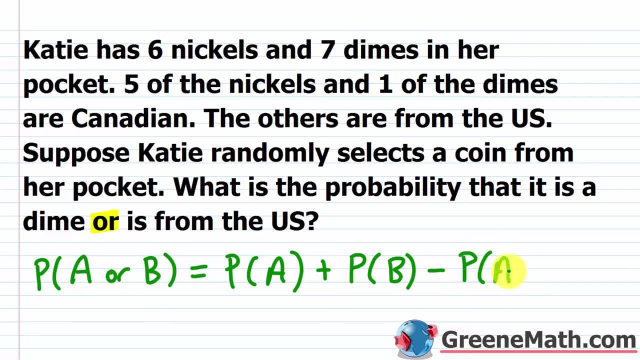 important, minus the probability of A and B happening. okay, And I know a lot of people use set notation there, so you might see this as well. okay, So the intersection of A and B. However you want to write it, it doesn't really matter. I'm just going to stick to writing and I think that's. 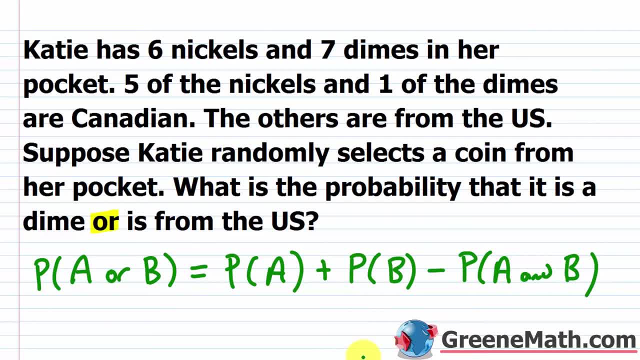 a little bit easier for us to understand. Okay, in this particular case we don't have something known as mutually exclusive. Mutually exclusive events are two events that can never occur simultaneously. So in this particular case we don't have that, because it says: what is the probability that it is a dime or is from? 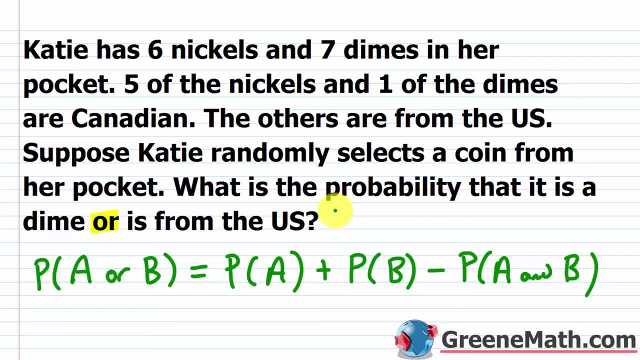 the US. Well, we have dimes that are also from the US, so we have to use this full formula. okay, If we didn't have dimes from the US, we could knock this part out. okay, This is going to take. 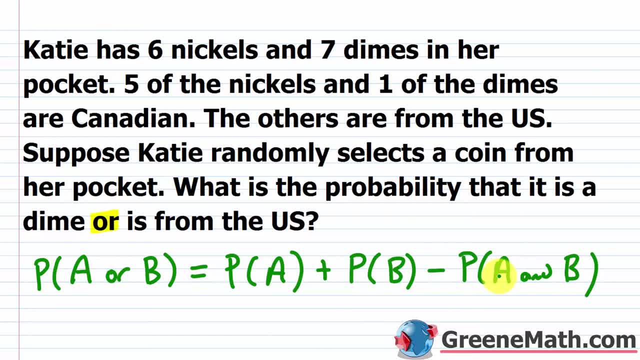 out the double counting. So let's go through real quick and think about what's the probability that it's a dime. Well, we know that she has six nickels and seven dimes. okay, Well, six plus seven is 13.. So 13 coins overall. seven of them are dimes. So the probability of having 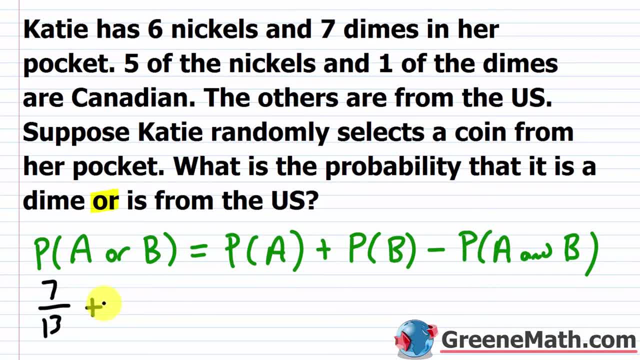 a dime is seven over 13,. then, plus What's the probability? okay, that the coin is from the US, meaning it's not Canadian. Well, it tells you that five of the nickels and one of the dimes are Canadian, So six out of the 13 coins are Canadian. So seven out of the 13 are 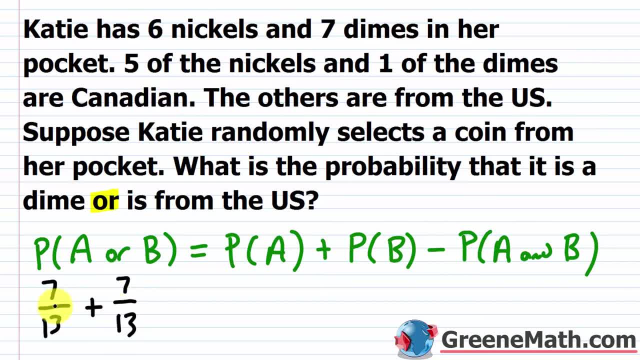 American or US currency. So seven over 13.. Seven plus seven is 14.. 14 over 13 is a number larger than one. When we deal with probabilities, it's either zero, okay, meaning it's not going to happen, up to and including one One means it's certain to happen. Anything in between means it. 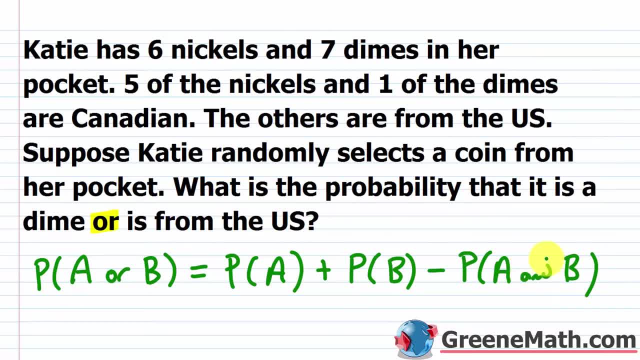 doesn't really matter, I'm just going to stick to writing, And I think that's a little bit easier for us to understand. Okay, In this particular case, we don't have something known as mutually exclusive events. Mutually exclusive events are two events that can never occur simultaneously. 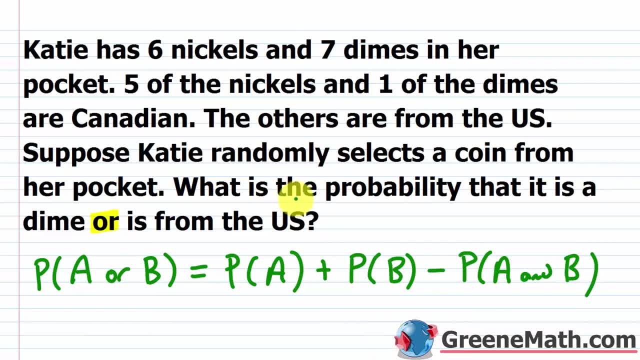 So in this particular case, we don't have that, because it says: what is the probability that it is a dime or is from the U S? well, we have dimes that are also from the U? S, so we have to use this full formula. 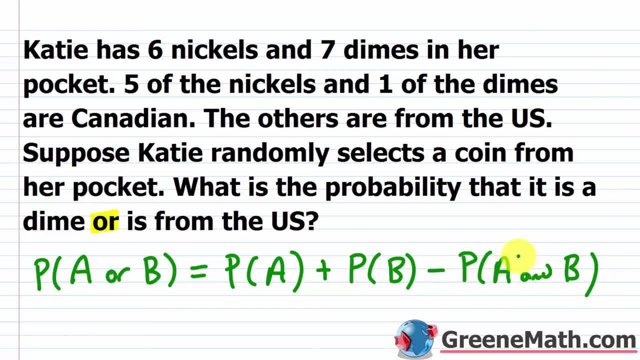 Okay, If we didn't have dimes from the U S, we could knock this part out. Okay, This is going to take out the double count, So let's go through real quick and think about what's the probability that it's a dime. 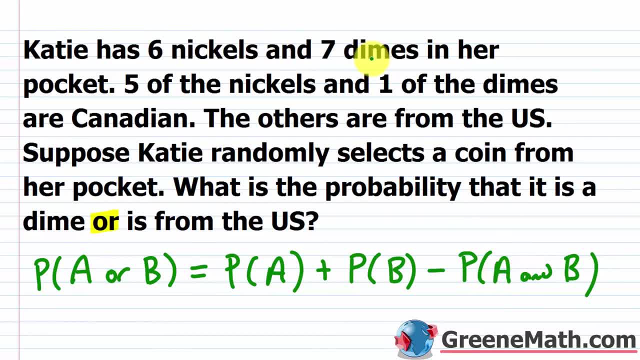 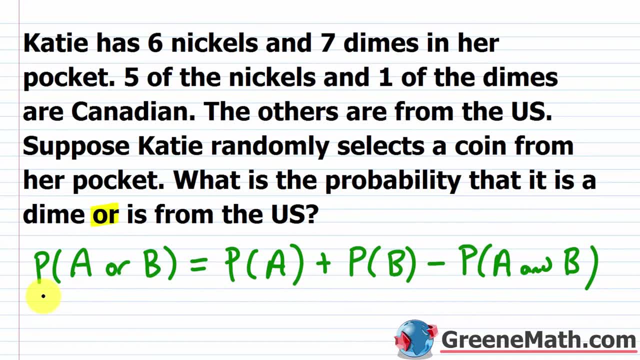 Well, we know that she has six nickels and seven dimes. Okay, Well, six plus seven is 13.. So 13 coins overall. seven of them were dimes. So the probability of having a dime is seven over 13.. 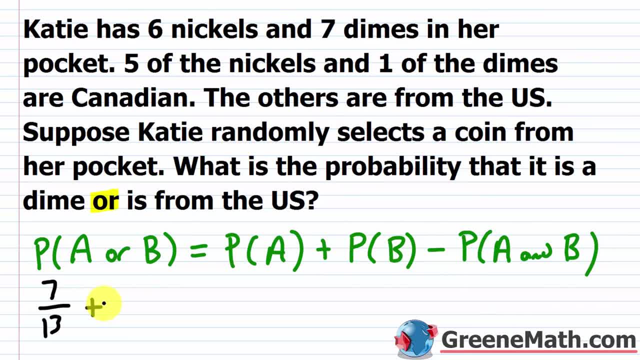 Then, plus what's the probability? Okay, That the coin is from the U S, meaning it's not Canadian. Well, it tells you that five of the nickels and one of the dimes are Canadian, So six out of the 13 coins are Canadian. 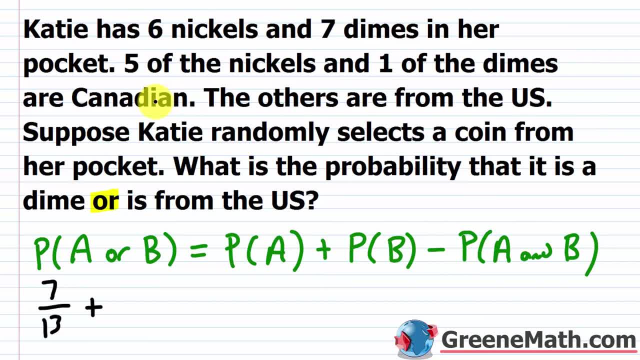 So seven out of the 13 are American or U S currency. So seven over 13,. seven plus seven is 14,. 14 over 13 is a number larger than one. When we deal with probabilities, it's either zero, Okay. 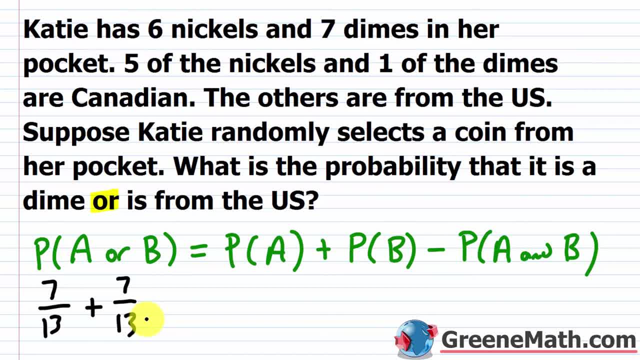 Meaning it's not going to happen up to an including one. one means it's certain to happen. Anything in between means it may or may not happen. Okay, But you can't get a probability Less than zero or greater than one. 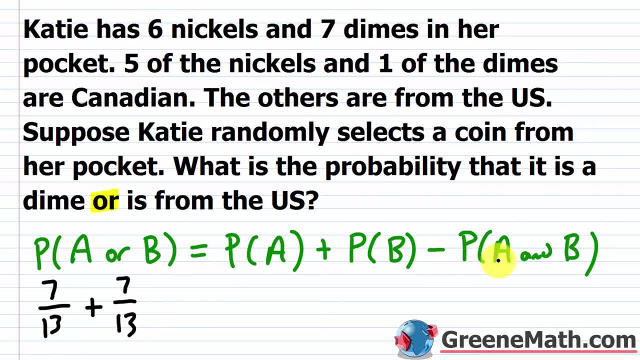 That doesn't make any sense. Okay, So that would be a red flag if you forgot to subtract this out. So all we need to do to fix this is subtract out the probability of a and B occurring. Okay, So how many dimes that we have that are also from the U S? well, 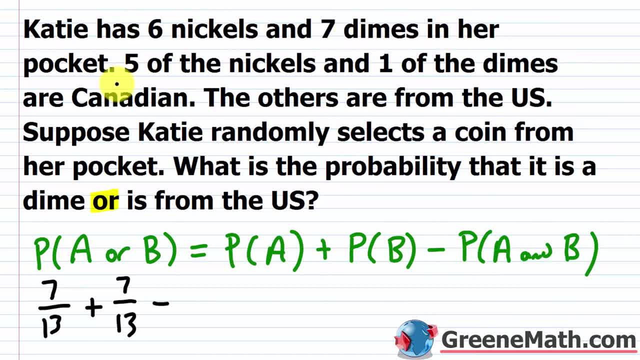 let's think about that. We know that there are seven dimes in her pocket. Okay, Total of seven, And it says that five of the nickels and one of the dimes are Canadian. So that means that six of the dimes. 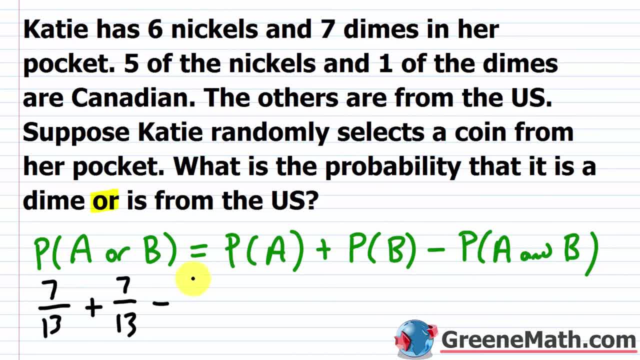 or from the U S. okay, So that tells me that I need to subtract away six over 13,. right, Because six of the dimes are from the U? S. So if I crank this out now, I get seven plus seven, which is 14, and then 14 minus six. 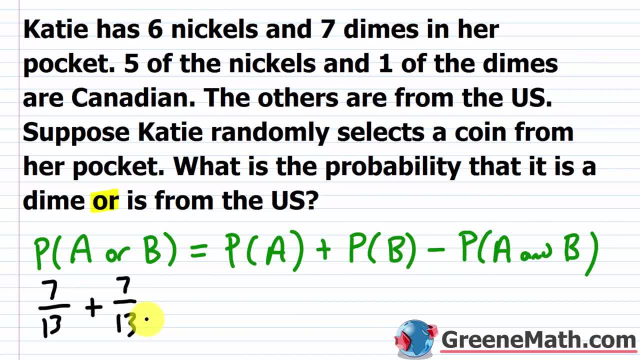 may or may not happen, okay, But you can't get a probability less than zero or greater than one. That doesn't make any sense, okay. So that would be a red flag if you forgot to subtract this out. So all we need to do to fix this is: 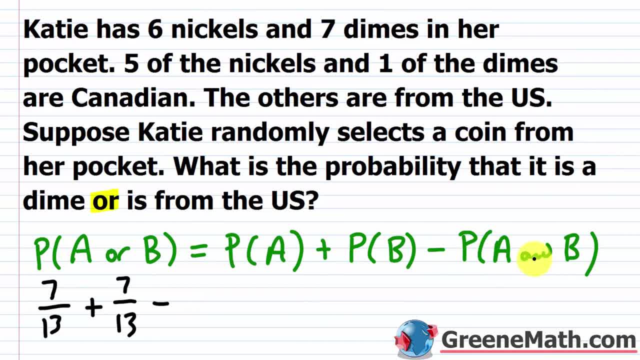 subtract out the probability of A and B occurring, okay. So how many dimes do we have that are also from the US? Well, let's think about that. We know that there are seven dimes in her pocket. okay, total of seven. And it says that five of the nickels and one of the dimes are 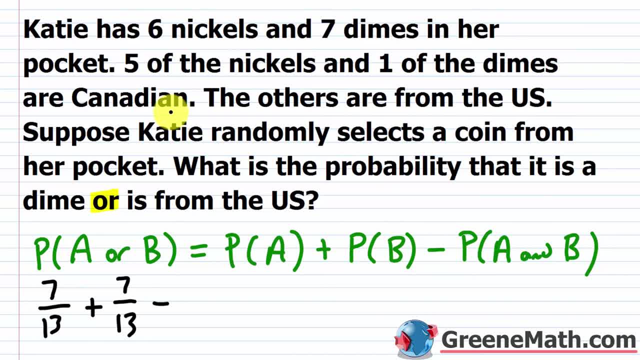 Canadian. So that means that six of the dimes are from the US. okay, So that tells me that I need to subtract away six over 13,. right, Because six of the dimes are from the US. So if I crank this out now, I get seven plus seven, which is 14.. And then 14 minus six. 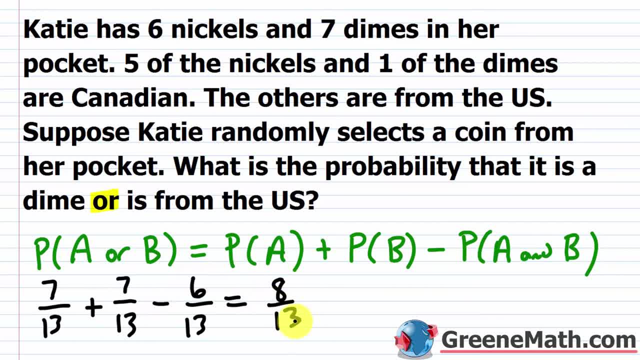 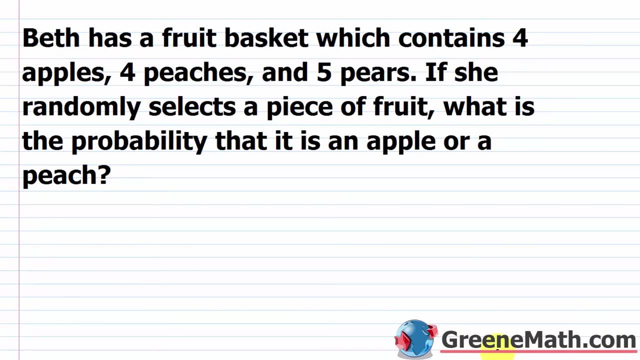 which is eight. So I get a result of eight over 13.. So that's going to be the probability that she picks a coin. that's going to be a dime or it's from the US. Okay, let's look at another example of this, And now we're going to see mutually exclusive events. So Beth has a fruit. 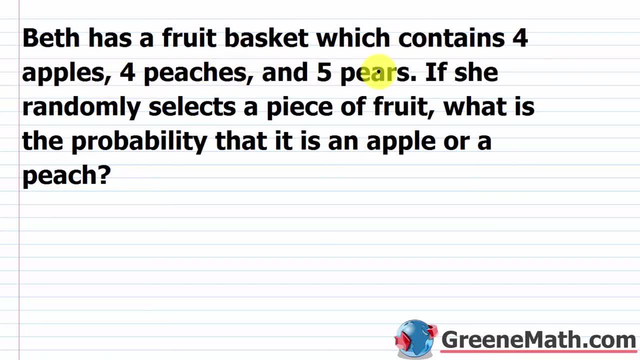 basket which contains four apples, four peaches and five pears. If she randomly selects a peach, what is the probability that it is an apple or a peach? Again, when you see this keyword, or you're thinking about addition? okay, But in this particular case you don't need that full. 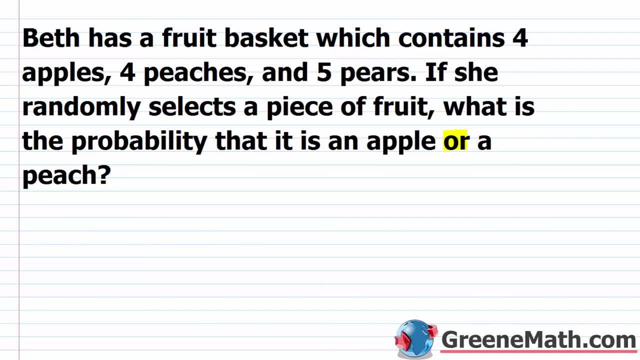 formula okay, Because it's not possible for her to select something that's an apple and a peach at the same time. So again, when you think about the probability of some event A happening or some event B happening, it's the probability of A plus the probability of B. So if you're thinking about 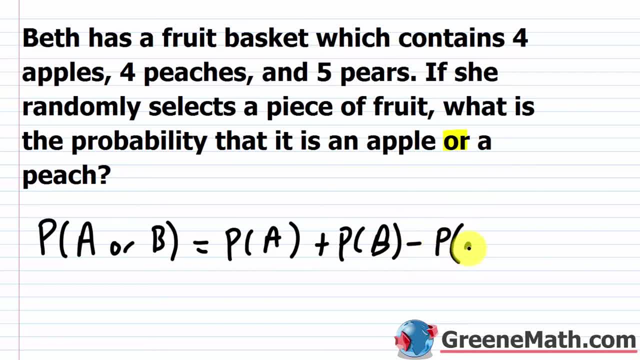 the probability of A and B occurring, and I didn't write my A there, so A and B. Well, in this particular case, you can get rid of this, because it's going to be zero Again. you cannot have a piece of fruit- that's an apple- and a peach at the same time. Maybe they're working on that, I'm not. 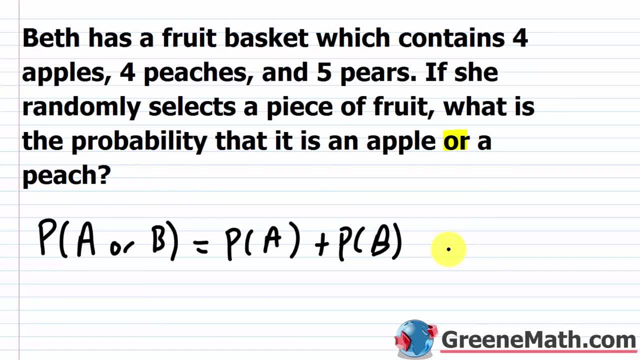 sure, But in this scenario it's not possible. So we just think about the probability of A. Let's say that's where she selects an apple. Well, there's four apples out of a total of four plus four plus five, So that's going to be a piece of fruit that's an apple and a peach at the same time. 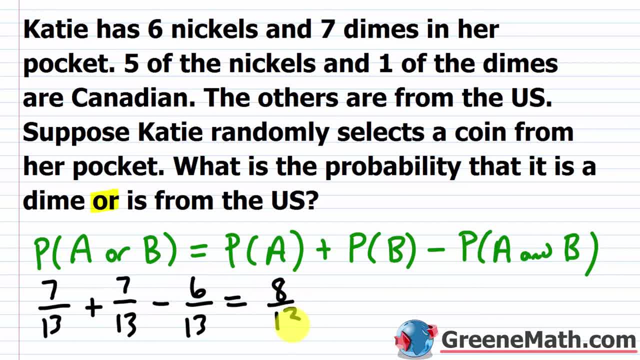 which is eight. So I get a result of eight over 13.. So that's going to be the probability that she picks a coin. That's going to be a dime or it's from the U S. okay, Let's look at another example of this. 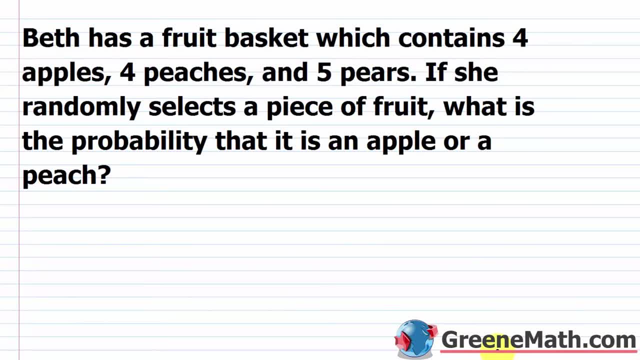 And now we're going to see mutually exclusively exclusive events. So Beth has a fruit basket which contains four apples, four peaches and five payers. If she randomly selects a piece of fruit, what is the probability that it is an apple or a peach? 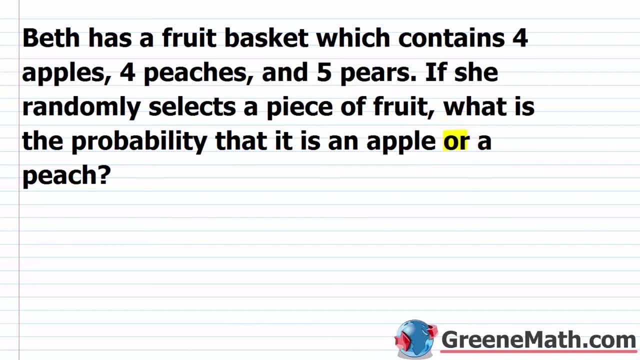 Again, when you see this keyword or you're thinking about addition, Okay, But in this particular case you don't need that full formula. Okay, Because it's not possible for her to select something That's an apple and a peach at the same time. 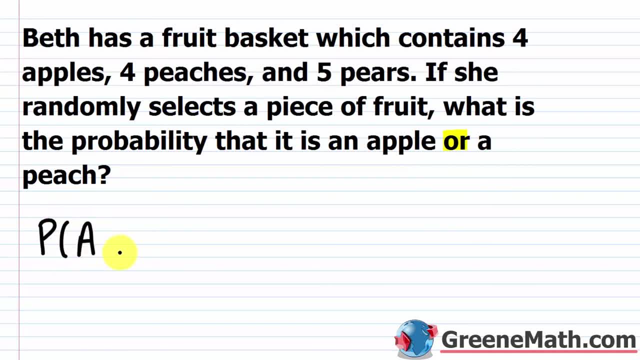 So, again, when you think about the, the probability of some event a happening or some event B happening, it's the probability of a plus the probability of B and then minus the probability of a and B occurring, And I didn't write my a there. 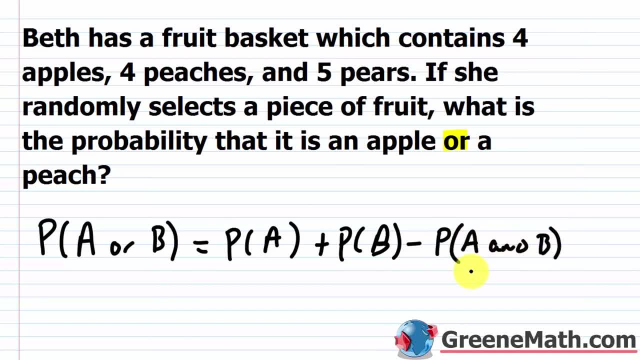 So a and B. well, in this particular case, you can get rid of this, because it's going to be zero Again. you cannot have a piece of fruit, That's an apple and a peach at the same time. Maybe they're working on that. 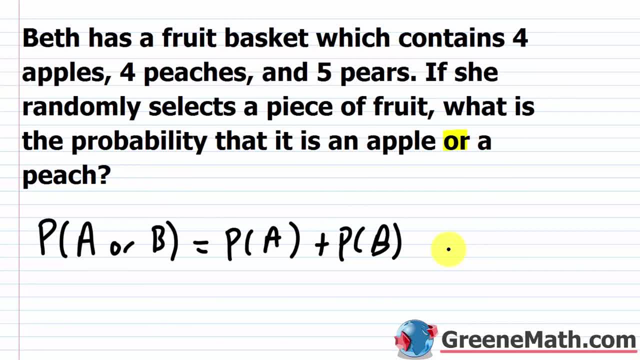 I'm not sure, but in this scenario it's not possible. So we just think about the probability of a- let's say that's where she selects an apple. Well, there's four apples out of a total of four plus four plus five. 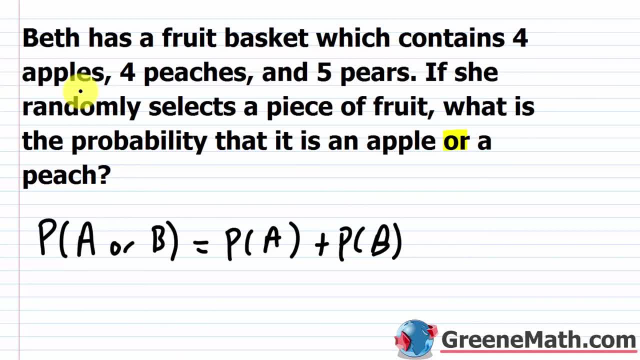 four plus four is eight. eight plus five is 13.. So the total of four over 13.. Okay, That's going to be your probability of picking an apple. then, Plus what's the probability of picking a peach? Well, again, 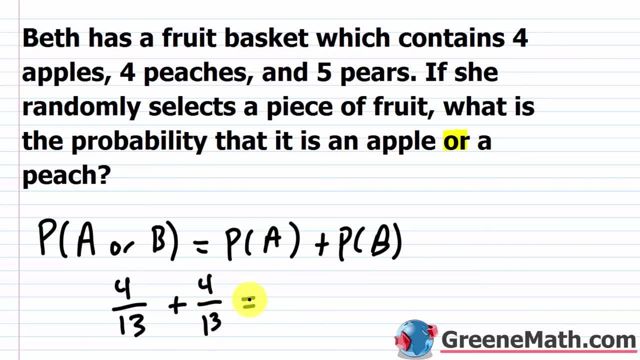 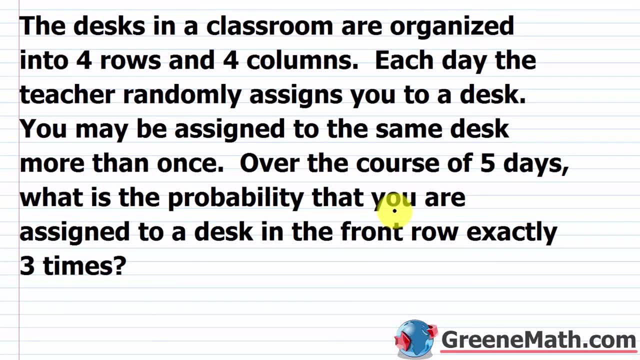 it's four over 13.. So all I have to do is just sum these and I get eight over 13.. All right, So let's wrap up the lesson by looking at an example where we use our our binomial probability formula. 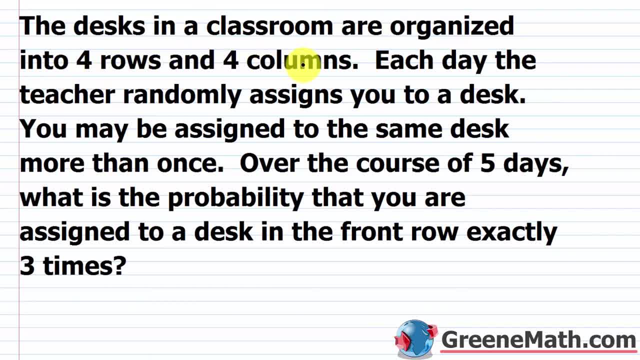 So the desks in a classroom are organized into four rows and four columns. Each day, the teacher randomly assigned you to a desk. You may be assigned to the same desk more than once over the course of five days. What is the probability that you are assigned to a desk in? 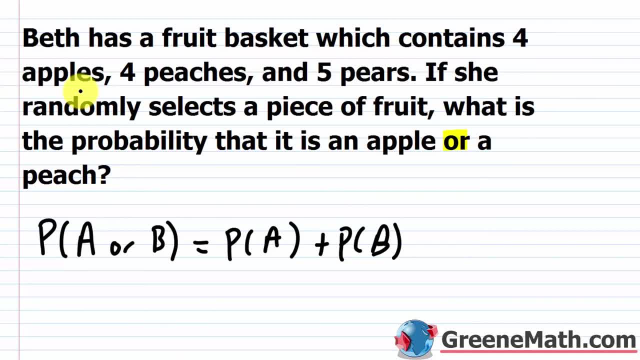 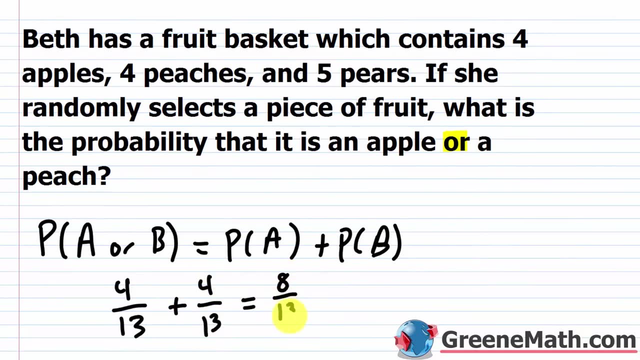 Four plus four is eight. Eight plus five is 13.. So the total of four over 13,. okay, that's going to be your probability of picking an apple. Then, plus, What's the probability of picking a peach? Well, again, it's four over 13.. So all I have to do is just sum these and I get eight over 13.. 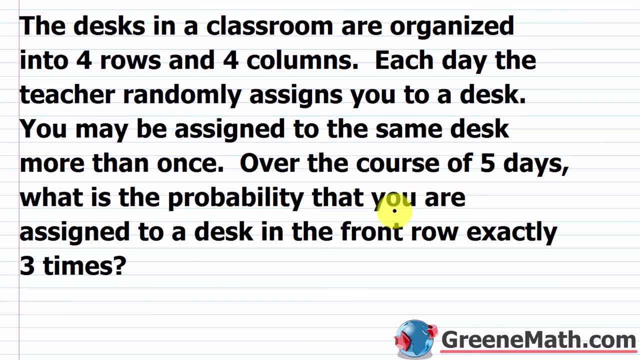 All right, so let's wrap up the lesson by looking at an example where we use our binomial probability formula. So the desks in a classroom are organized into four rows and four columns. Each day, the teacher randomly assigns you to a desk. 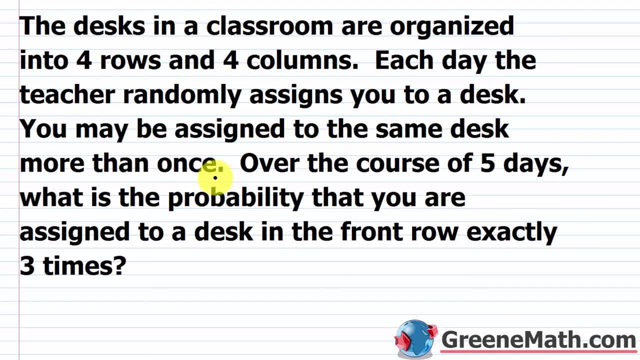 You may be assigned to the same desk more than once Over the course of five days. what is the probability that you are assigned to a desk in the front row- exactly three times? Okay. so if you are dealing with a scenario such as this where you have repeated independent trials, okay, so this: 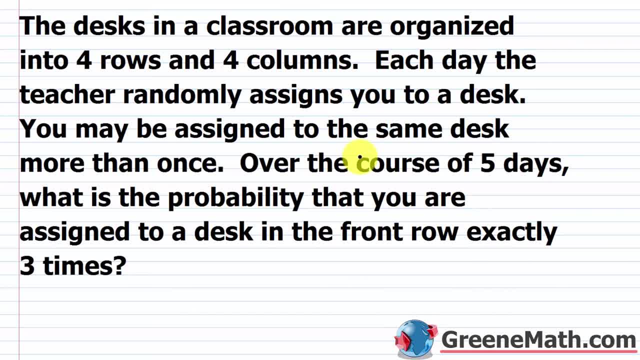 is independent because every day you're randomly assigned to a desk and you can sit where you've sat before, And the outcome in each trial is either a success- meaning in this case you will get assigned to the front row- or a failure. okay, So if you want to find the probability of our 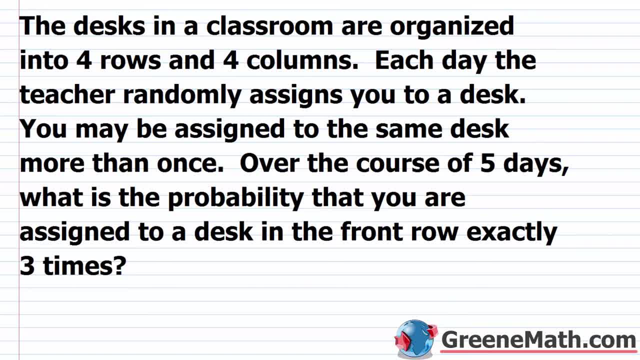 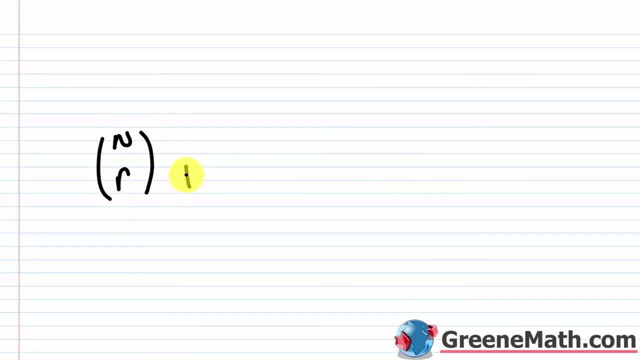 successes in n trials. you can use this formula. So let me write this down here And we'll come back up in a minute. So n choose r. okay, we remember that. And then times p raised to the power of r. 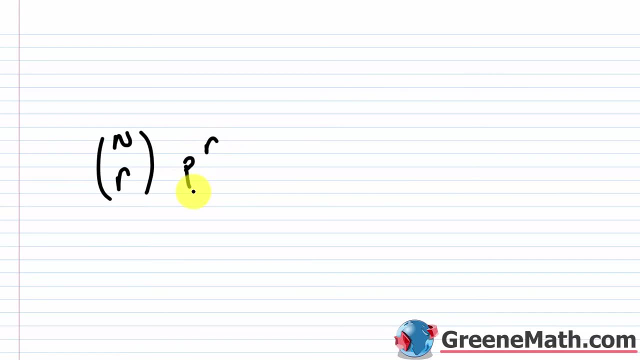 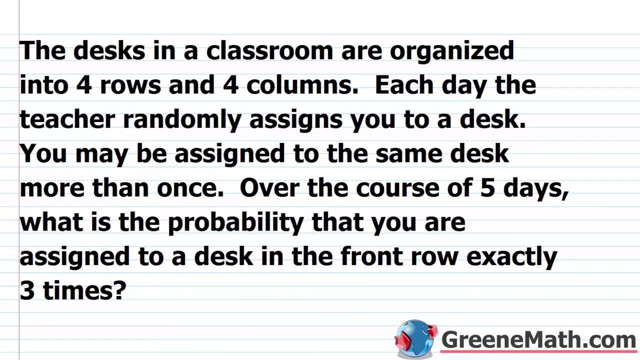 p is the probability of a success. So on a single day, what's the probability of you getting seated in the front row? I'll get to that in a second. Then times one minus this p, raised to the power of r, p, raised to the power of n minus r, So n is the number of trials. So if we go back up, we know that. 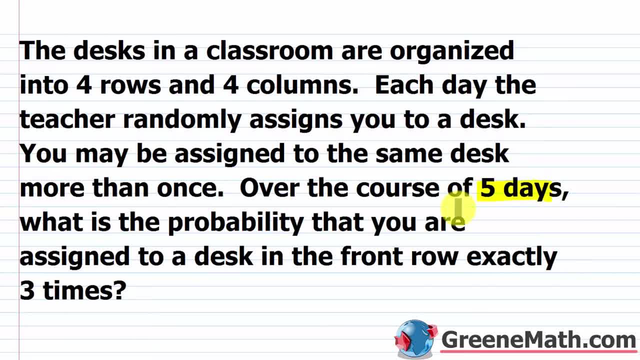 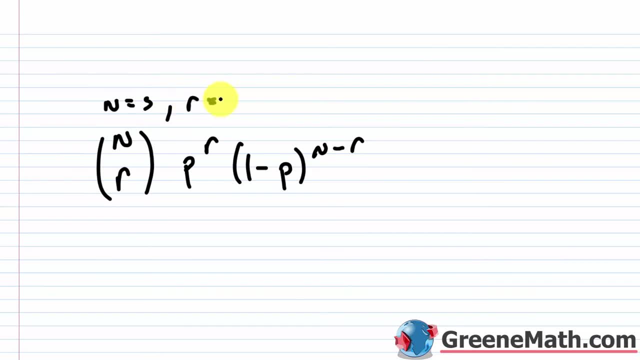 this is going to happen for five days, So over the course of five days. so n is five And the number of successes we're looking for is r, right, So three times is we're looking for that number to happen. So n is five, n is five And r is three. Okay, so you're just plugging things in, So you 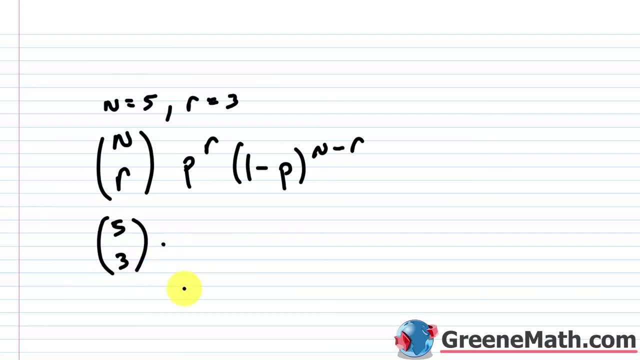 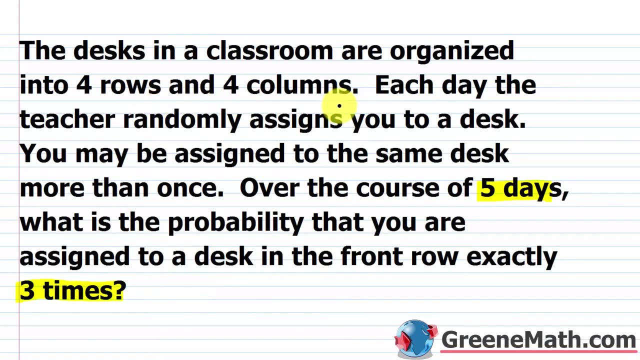 have five and three. okay, Then p is the probability of you getting seated in the front row, So n is the probability of a success on any given day. Well, if we go back, we know that there's a total of 16 desks right, Four rows and four columns. four times four is 16.. So in the front row, 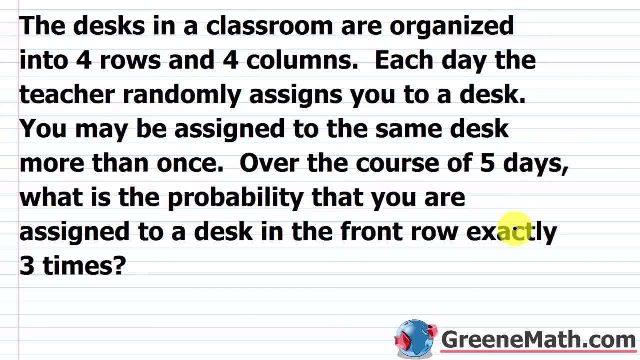 the front row Exactly three times. Okay. So, if you are dealing with a scenario such as this, where you have repeated independent trials, okay so this is independent because every day you're randomly assigned to a desk and you can sit where you've sat before. 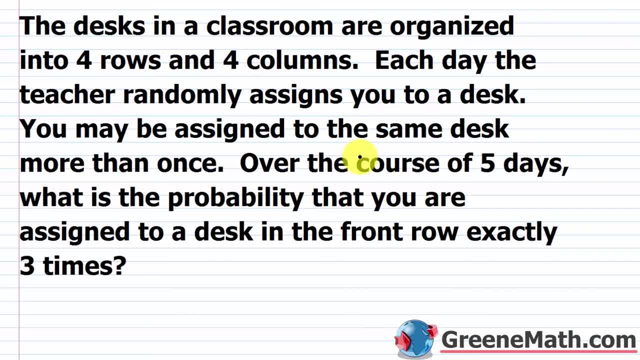 And the outcome in each trial is either a success- meaning in this case you will get assigned to the front row- or a failure. Okay, So if you want to find the probability of our successes in end trials, you can use this formula. 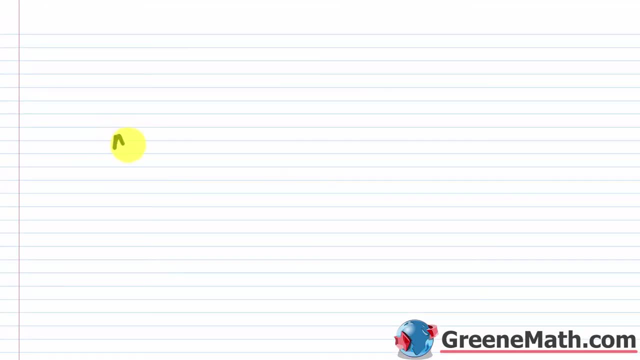 So let me write this down here and we'll come back up in a minute. So N choose R. Okay, We remember that. and then times P raised to the power of R, P is the probability of a success. So on a single day, 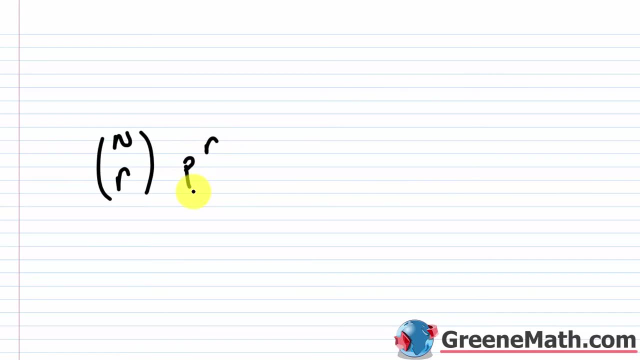 what's the probability of you getting success? Okay, So if you're seated in the front row, I'll get to that in a second. then times one minus this, P, raised to the power of N minus R, So N is the number of trials. 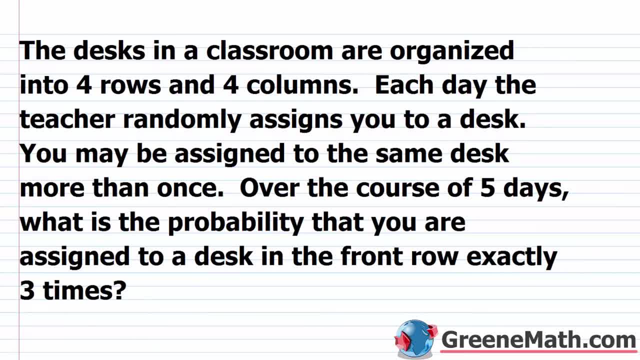 So if we go back up, we know that this is going to happen for five days, So over the course of five days. so N is five and the number of successes we're looking for is R, right, So three times is we're looking for that number to happen. 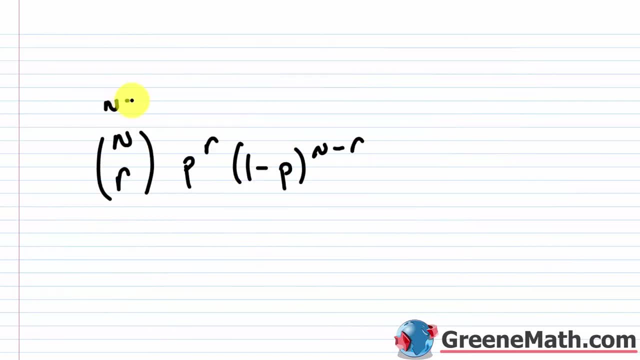 So N is five, N is five And R is three. Okay, So you're just plugging things in, So you have five and three. Okay, Then P is the probability of a success on any given day. Well, if we go back, 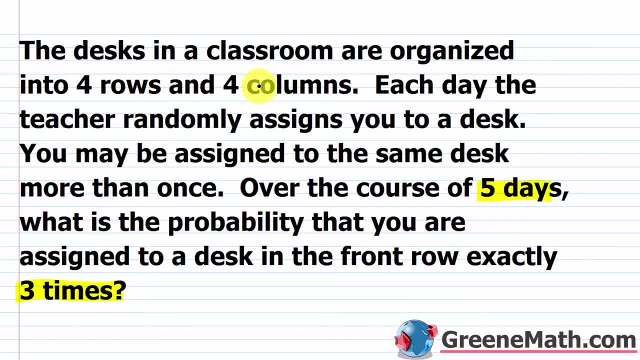 we know that there's a total of 16 deaths right, Four rows and four columns. four times four is 16.. So in the front row you're going to have four deaths. So that means you have a four over 16 or one fourth or 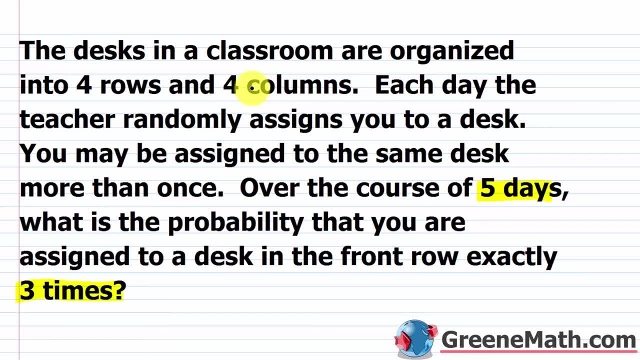 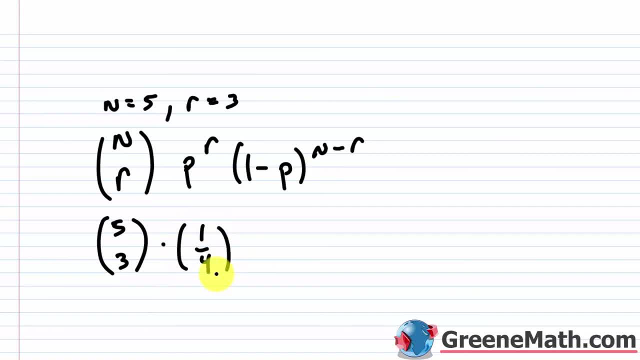 25% probability of getting seated in the front row on any given day. So we're going to put a one fourth here. You could use a decimal if you want. It doesn't matter, It's going to be the same result in the end. 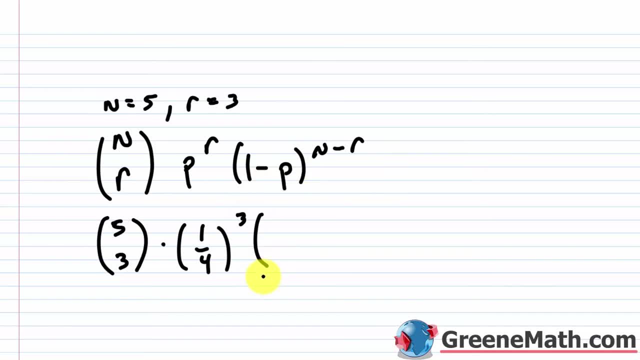 R again is three, and then one minus one fourth. If you're using a fraction, you would do four fourths minus one fourth, which is three fourths, and then raise the power of N, which is five, minus R, which is three. 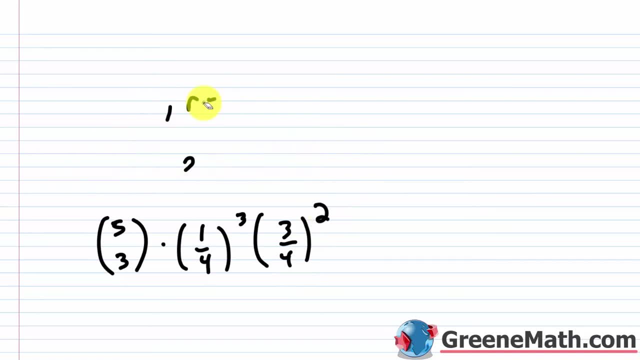 So this is going to be squared, Okay. So once you have this set up, you can just erase this and crank this out. So, on a calculator, five choose three is going to be 10.. Then, if we think about one fourth cubed. 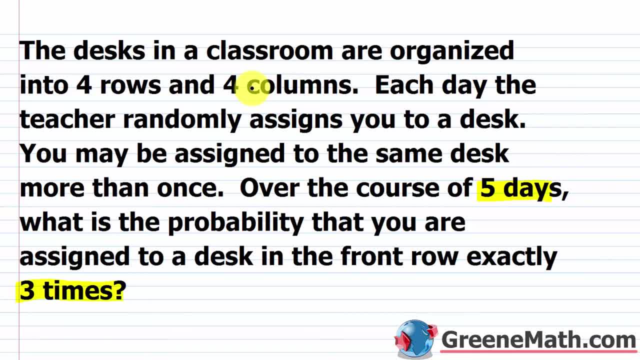 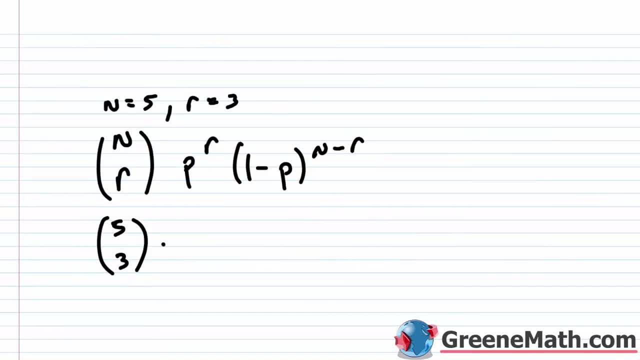 you're going to have four desks. So that means you have a four over 16, or one fourth or 25% probability of getting seated in the front row on any given day. So we're going to put a one fourth here. You could use a decimal if you want. it doesn't matter, It's going to be the same result. 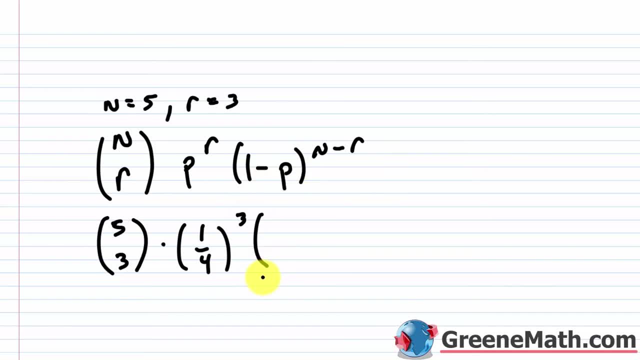 in the end, r again is three And then one fourth. it doesn't matter, It's going to be the same one minus one fourth. If you're using a fraction, you would do four fourths minus one fourth, which is three fourths, And then raise the power of n, which is five, minus r, which is three. So 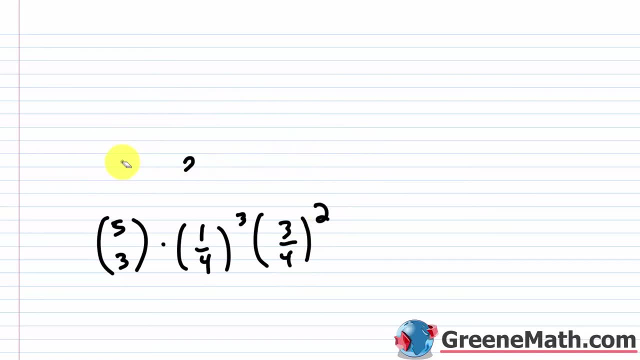 this is going to be squared, Okay. So once you have this set up, you can just erase this and crank this out. So, on a calculator, five choose three is going to be 10.. Then if we think about one fourth cubed, that's going to be one over four cubed is 64.. Then if we think about three, 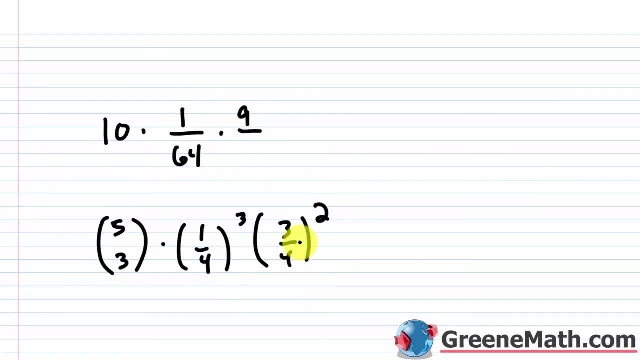 fourths squared, three squared is nine. Four squared is nine, So that's going to be three squared is 16.. Can I cancel anything before I multiply? I can just get rid of this. I don't need it anymore. Can I cancel anything? Well, yeah, I can cancel a factor of two here and here. 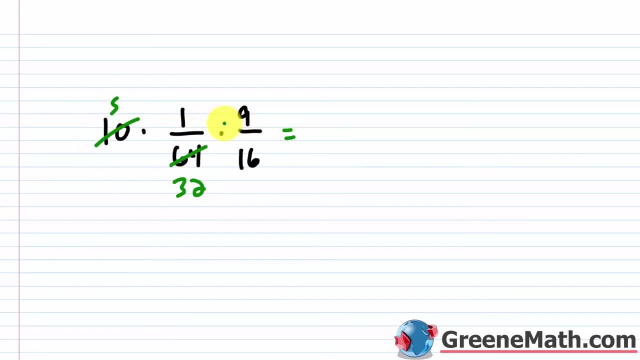 So this would be 32.. This would be five. So five times nine is 45 over what is 32 times 16.. That's going to be 512.. So 45 over 512, that's going to be your probability of getting seated in the front. 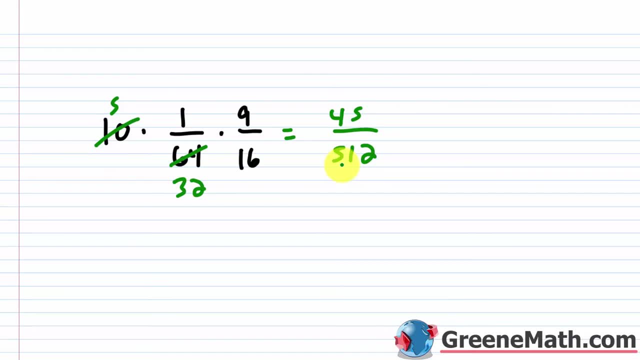 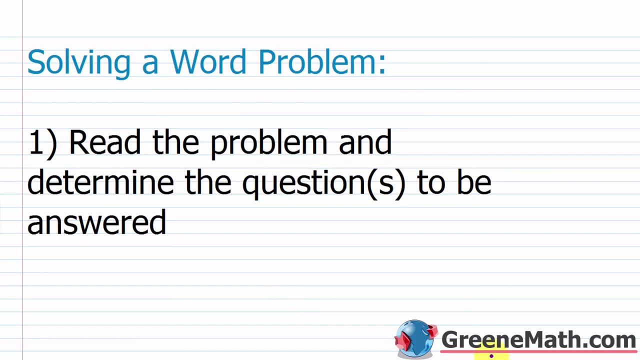 row exactly three days out of a total of five days. In this lesson we want to think about applications of quadratic equations. So throughout our study of algebra we often come across word problems or application problems. So so far in our course we've only discussed word problems. 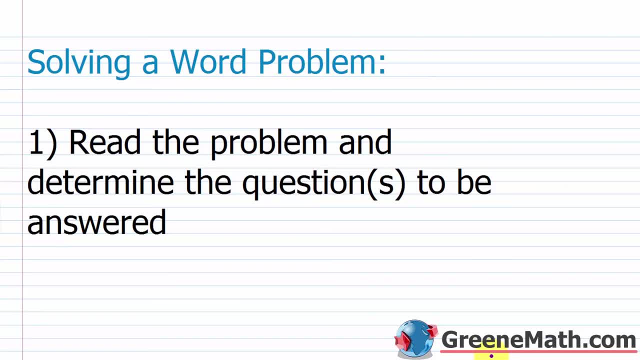 that involve solving a linear equation in one variable. Now we're going to go one step further and take a look at some word problems that involve quadratic equations. So I want you to recall that we have a little six step procedure that we can use for solving word problems, And although we've 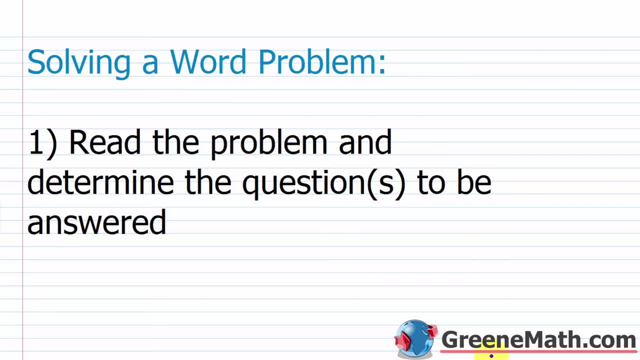 introduced this method for you to do. we're not going to do it. We're going to do it in a different way. We're going to use it with applications of linear equations. We can also use it in this section as well. So let's just kind of recap this six step procedure. I think you'll find it useful. 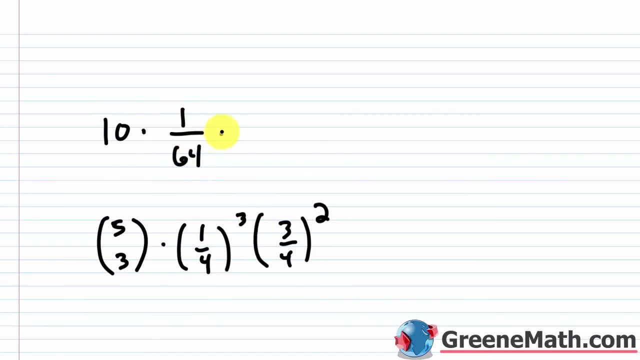 that's going to be one over four cubed is 64.. Then if we think about three fourths squared, three squared is nine, four squared is 16.. Can I cancel anything before I multiply? I can just get rid of this. 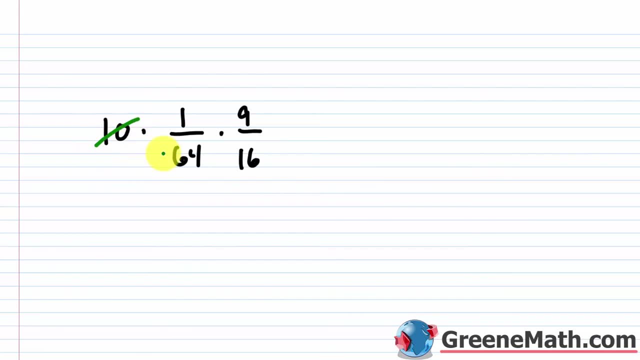 I don't need it anymore. Can I cancel anything? Well, yeah, I can cancel a factor of two here and here. So this would be 32.. This would be five. So five times nine is 45 over what is 32 times 16.. 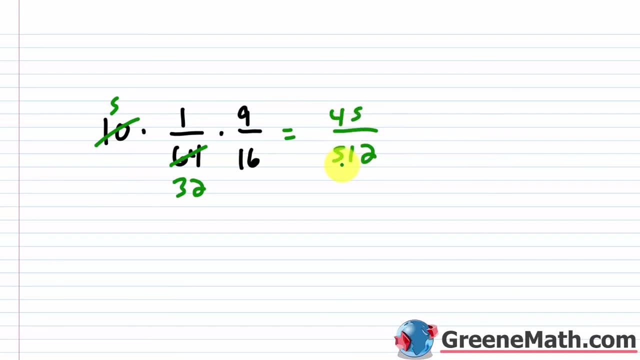 That's going to be 512.. So 45 or 512.. That's going to be your probability of getting seated in the front row exactly three days out of a total of five days. In this lesson we want to think about applications of quadratic equations. 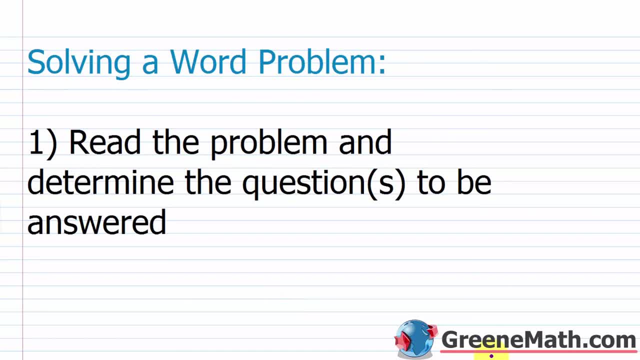 So throughout our study of algebra, we often come across word problems or application problems. So so far, our course, we've only discussed word problems that involve solving a linear equation in one variable. Now we're going to go one step further and take a look at some word problems. 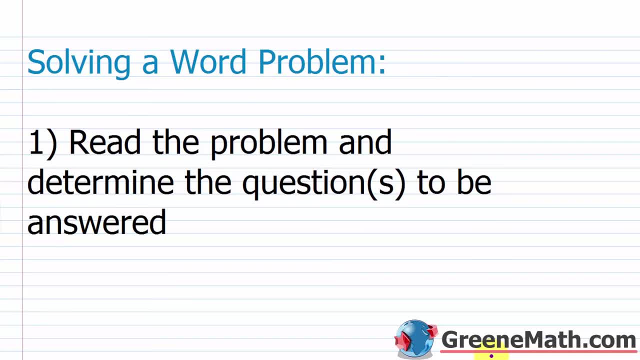 that involve quadratic equations. So I want you to recall that we have a little six step procedure that we can use for solving word problems, And although we've introduced this method for use with applications of linear equations, we can also use it in this section as well. 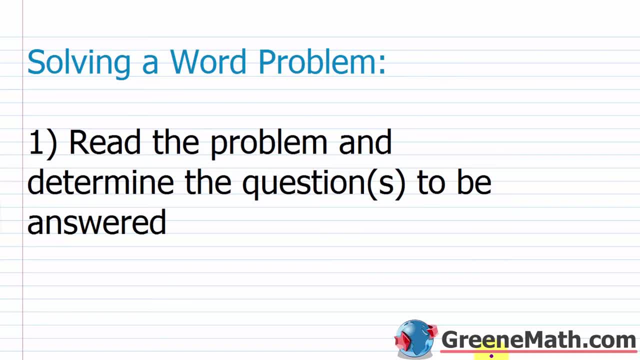 So let's just kind of recap this six step procedure. I think you'll find it useful if you write it down and kind of go through the steps when you're solving the problem. So, solving a word problem, we have that our first step is to read the problem and determine the question or 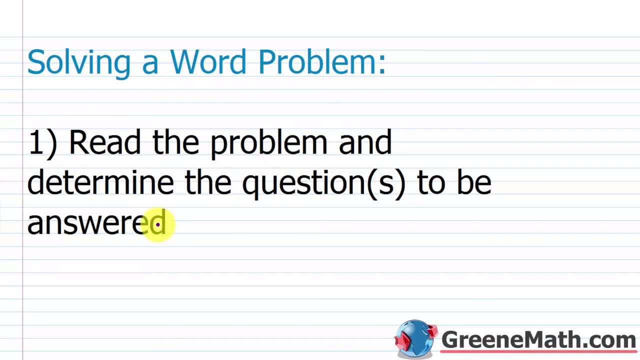 perhaps questions to be answered. You always want to make sure that you understand the question, or again, the question that you're being asked to kind of answer. It helps you kind of format things in a way. Well, what am I trying to find? 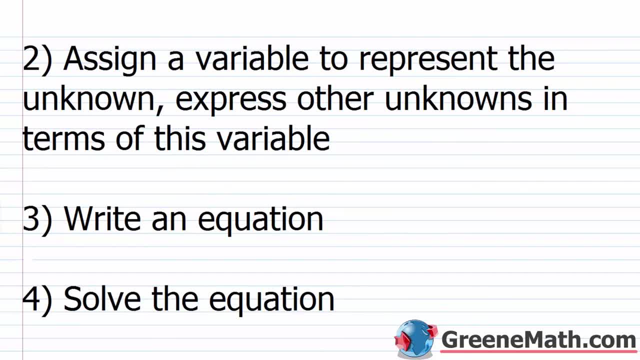 Then the second step is to assign a variable to represent the unknown, And in some cases we're going to have to express other unknowns in terms of this variable. Then, third, we want to write an equation that describes the scenario we're given. 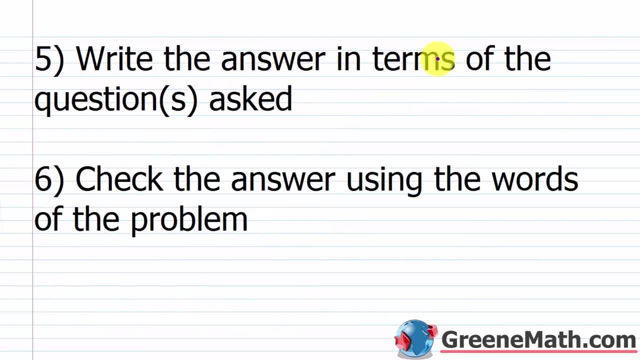 And then fourth, we're just going to solve that equation. Then, fifth, we want to write the answer in terms of the question, or again, perhaps, questions asked. And then the sixth thing, probably the most important, we want to check the answer using the words. 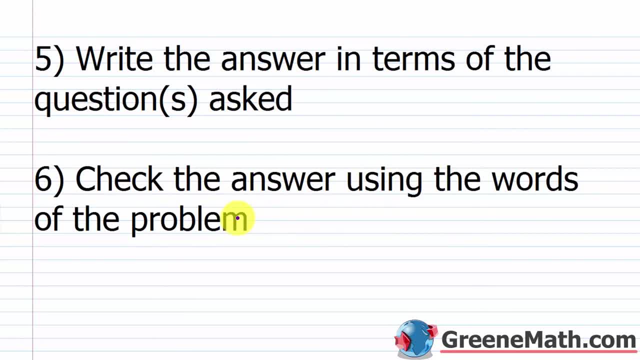 the problem. We want to make sure that the answer is reasonable. Okay, You're going to see, in some of the examples we get today, we're going to have some solutions to our equation that we set up that don't quite work in the context of the problem we're given. 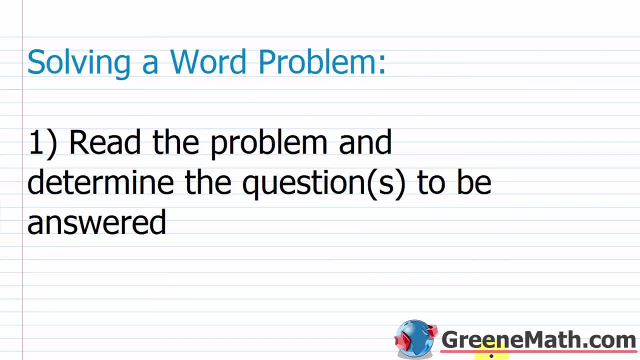 if you write it down and kind of go through the steps when you're solving the problem. So solving a word problem, we have that. our first step is to read the problem and determine the question or perhaps questions to be answered. You always want to make sure that you understand. 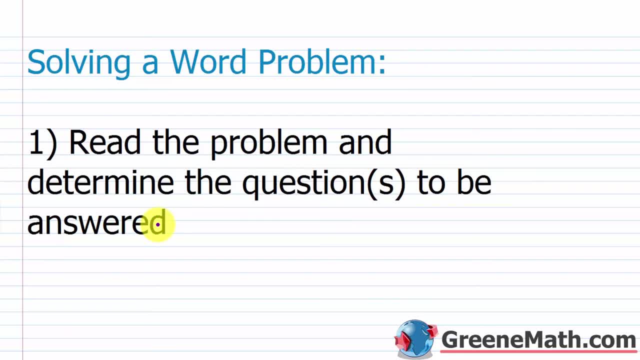 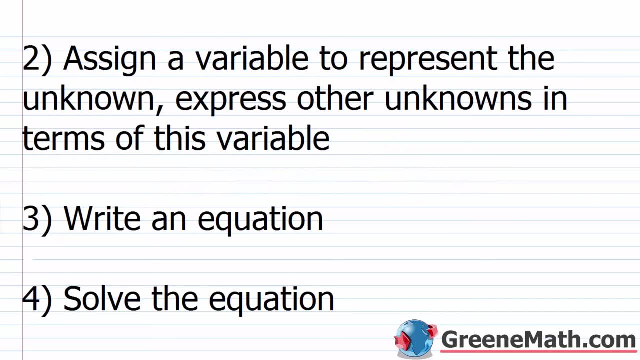 the question, or again the question that you're being asked to kind of answer. It helps you kind of format things in a way. well, what am I trying to find Then? the second step is to assign a variable to represent the unknown And, in some cases, 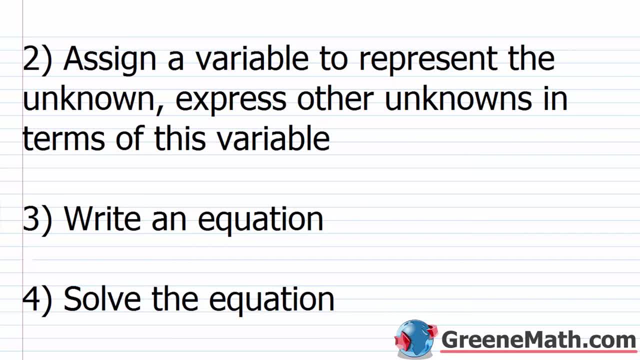 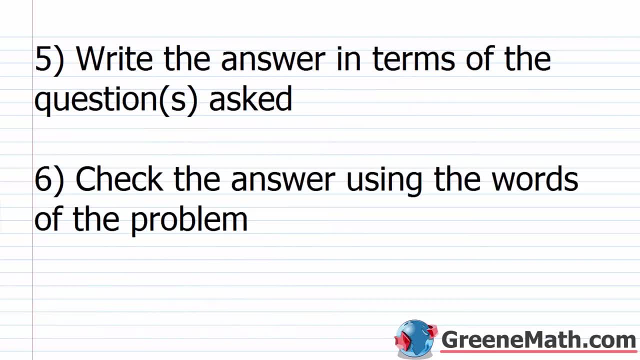 we're going to have to express other unknowns in terms of this variable. Then, third, we want to write an equation that describes the scenario we're given. And then, fourth, we're just going to solve that equation. Then, fifth, we want to write the answer in terms of the question, or again perhaps, 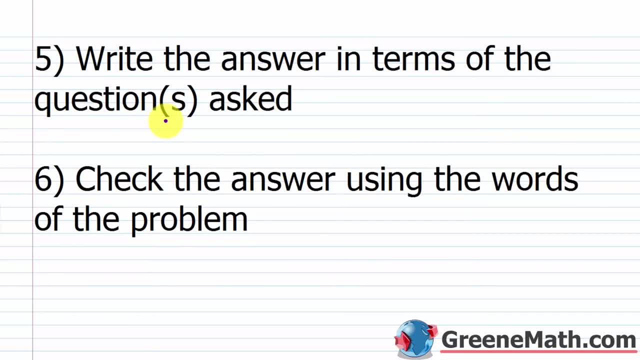 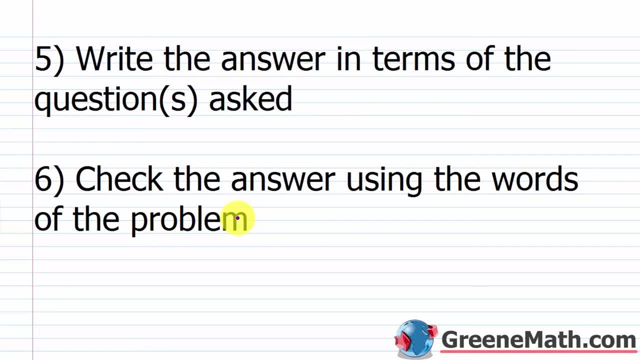 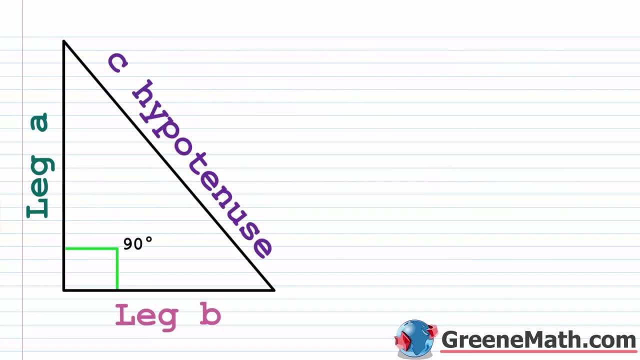 answer. We're going to have some solutions to our equation that we set up that don't quite work in the context of the problem we're given. Okay, and we'll get to that later on. All right, so the first few problems we're going to look at are going to involve the Pythagorean formula, I know. 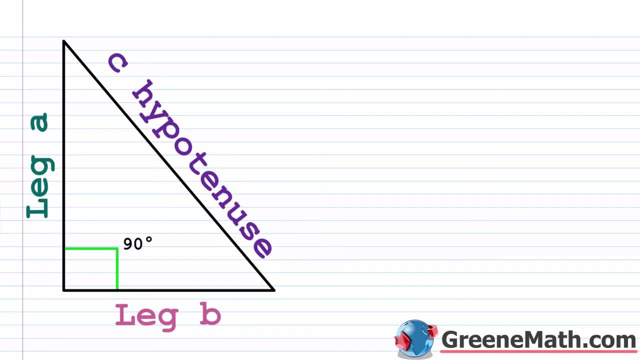 that most of you already know about the Pythagorean formula, but just in case you don't, it doesn't hurt for a little bit of a review. So the Pythagorean formula basically shows the relationship between the lengths of the sides of a right triangle. So again we know, we have a right. 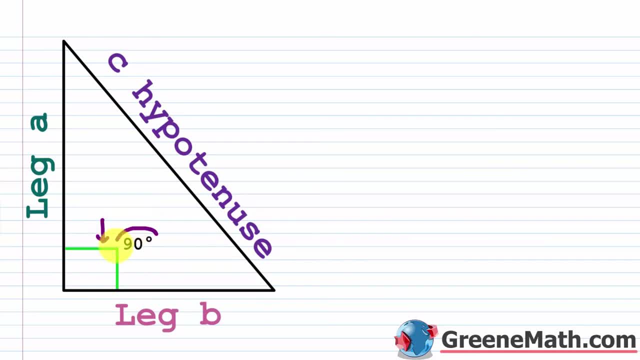 triangle because of this signature mark here. This is telling us that the right triangle is telling us we have a 90-degree angle or a right angle, Okay. so if you have a right angle in a triangle, it's known as a right triangle. Now, with a right triangle, we have this special 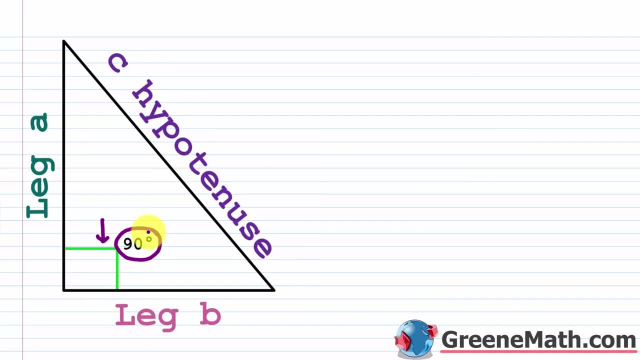 relationship between the sides. Okay. so you have these two shorter sides, known as legs. You have this here, leg A, which is this kind of vertical measure here, And then you have this leg B, which is this horizontal measure here, Okay. and then you have C, which is the hypotenuse. 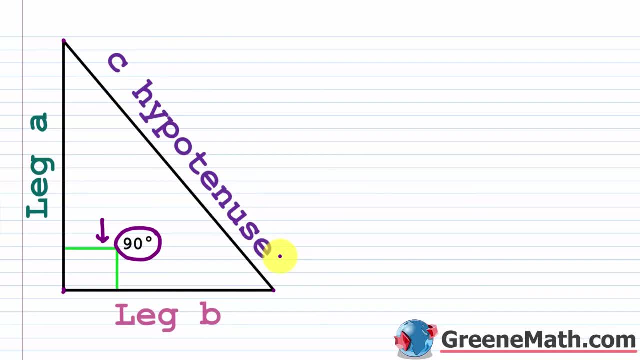 Okay, the hypotenuse is always going to be opposite of the right angle, so opposite of this, and it's the longest side. So most of you already know this. The Pythagorean formula tells you that A squared right, which is basically the measure of leg A, 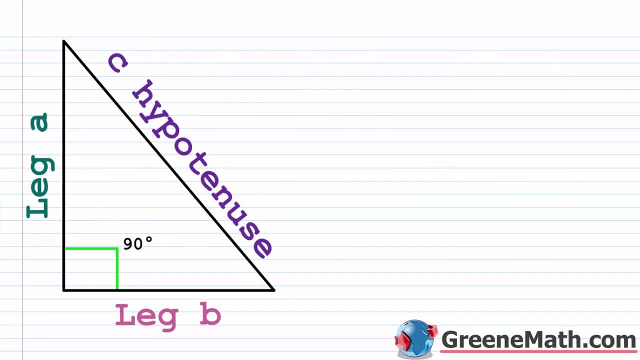 Okay, And we'll get to that later on. All right, So the first few problems we're going to look at are going to involve the Pythagorean formula. I know that most of you already know about the Pythagorean formula, but just in case you don't, 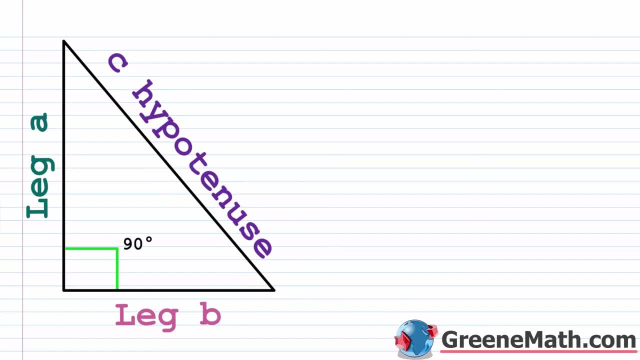 it doesn't hurt for a little bit of a review. So the Pythagorean Pythagorean formula basically shows the relationship between the lengths of the sides of a right triangle. So again we know we have a right triangle because of this signature mark here. 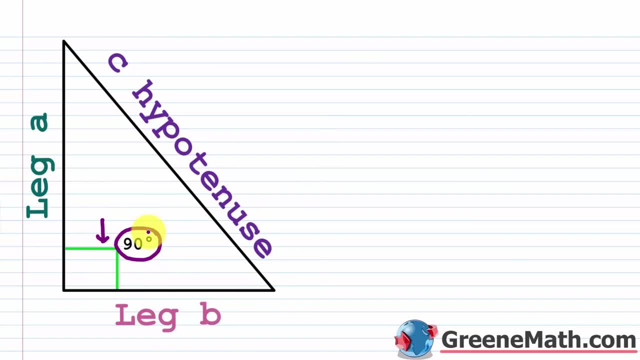 This is telling us we have a 90 degree angle or a right angle. Okay, So if you have a right angle in a triangle, it's known as a right triangle. Now, with a right triangle, we have this special relationship between the sides. 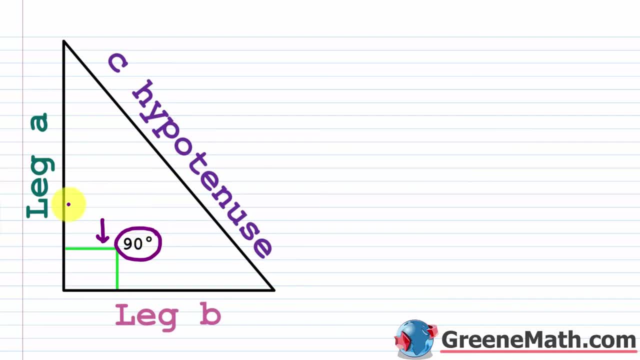 Okay, So you have these two shorter sides known as legs. You have this here, leg a, which is this kind of vertical measure here, And then you have this leg b, which is this horizontal measure here. Okay, And then you have c. 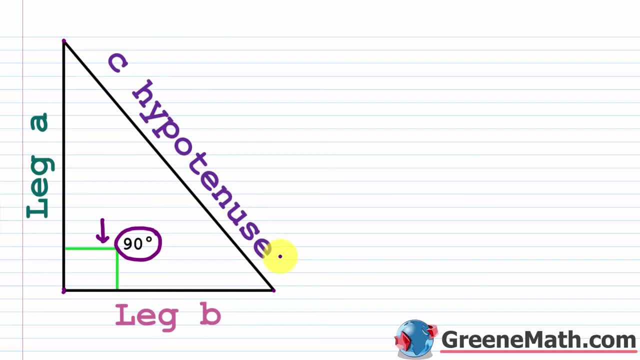 which is the hypotenuse. Okay, The hypotenuse is always going to be opposite of the right angle, So opposite of this, and it's the longest side. So most of you already know this. The Pythagorean formula tells you that a squared 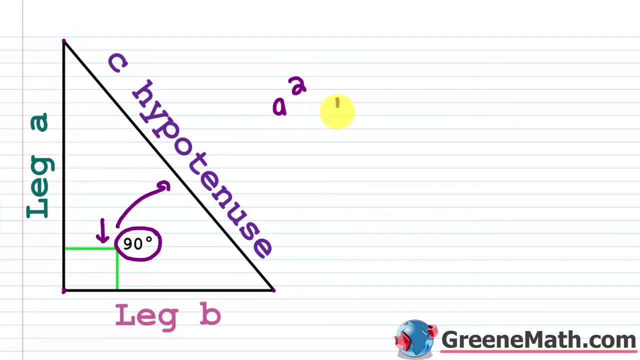 right, which is basically the measure of leg a that guy squared, plus b squared Again, the measure of b, leg b squared. If I sum those two amounts together, it's equal to c, which is the hypotenuse that measure squared. 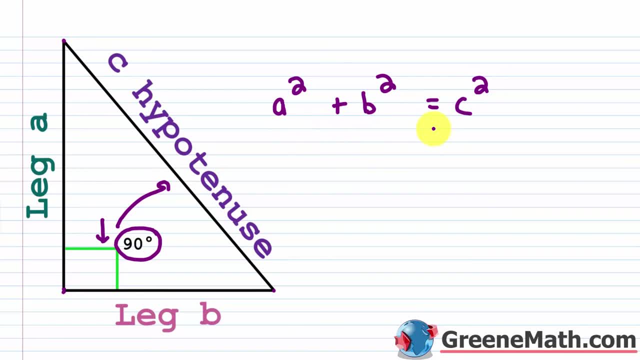 Okay, This is your Pythagorean formula And it's true for any right triangle that you come across. So, using this Pythagorean formula, basically, if we don't know one of the sides of a right triangle, but we know the other two, 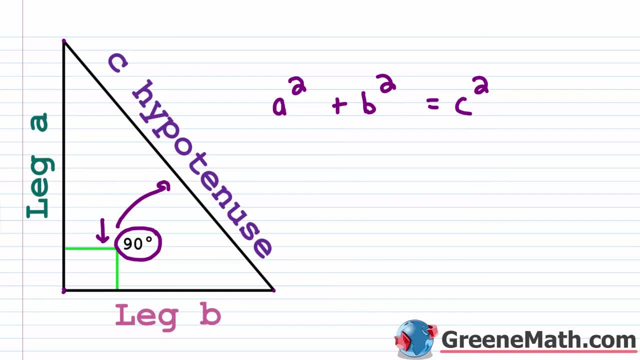 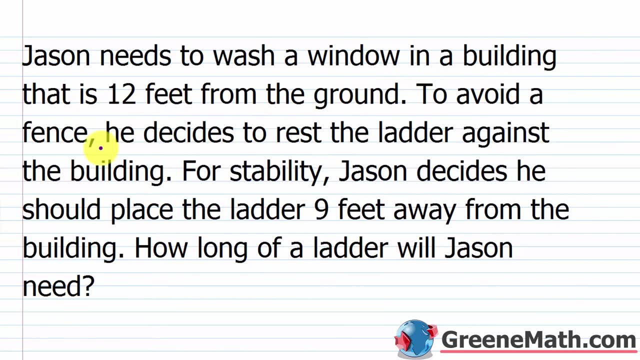 we can solve for the unknown. Okay, So let's take a look at our first sample problem. All right, So Jason needs to wash a window in a building that is 12 feet from the ground. To avoid a fence, he decides to rest the ladder against the building. 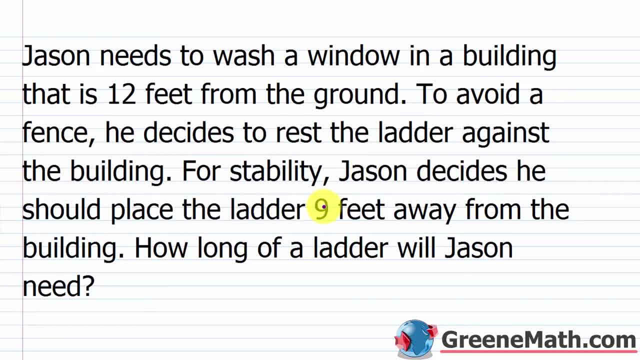 For stability, Jason decides he should place the ladder nine feet away from the building. How long of a ladder will Jason need? Okay, So the first thing we need to understand again is: what am I being asked to find? And in this case, 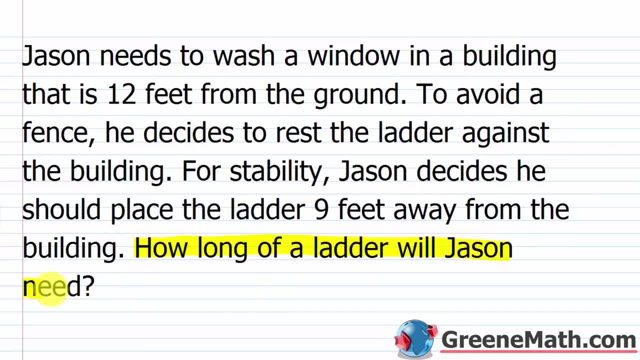 it's this little question here, right? So how long of a ladder will Jason need? So we'll just highlight that That's what we're trying to find. So when we go to assigning a variable, we're just going to let x represent exactly what we're trying to find. 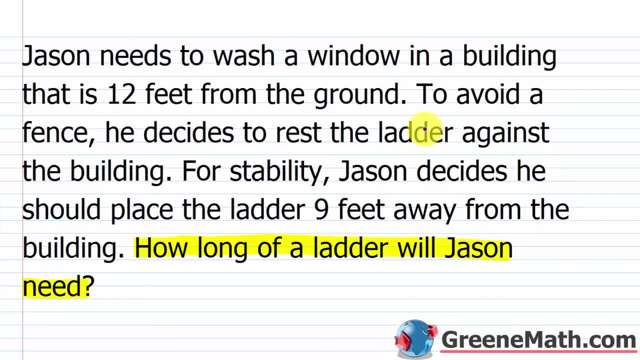 which is the measure of Jason's ladder, And this is going to be the measure of the ladder, And this is going to be the measure of the ladder, And this is going to be in feet, because we're working with feet in the problem. 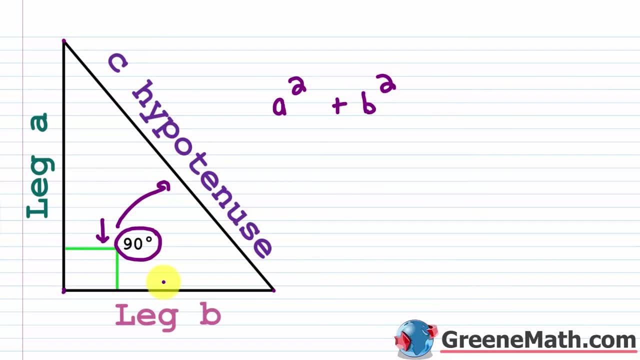 that guy squared plus B squared again the measure of B leg B squared. If I sum those two amounts together, it's equal to C, which is the hypotenuse that measure squared. Okay, this is your Pythagorean formula and it's true for any right triangle that you come across. 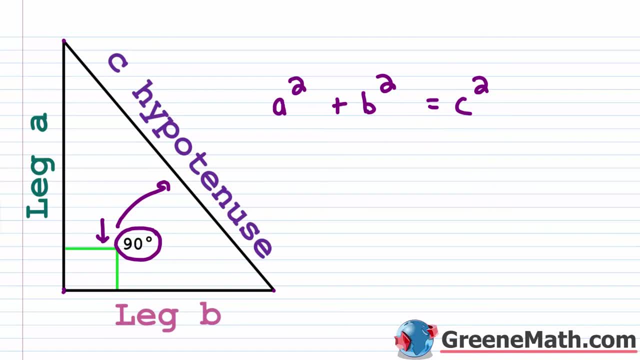 So using this Pythagorean formula- basically, if we don't know one of the sides of a right triangle but we know the other two, we can solve for the unknown. Okay, so let's take a look at our first sample problem. All right, so Jason needs to wash a window in a building that is 12 feet from the. 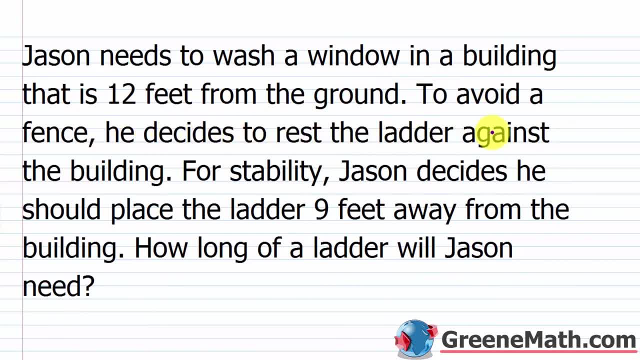 ground To avoid offense. he decides to rest the ladder against the building For stability. Jason decides he should place the ladder nine feet away from the building. How long of a ladder will Jason need? Okay, so the first thing we need to do is to find the right triangle. So we're going to do a little bit of 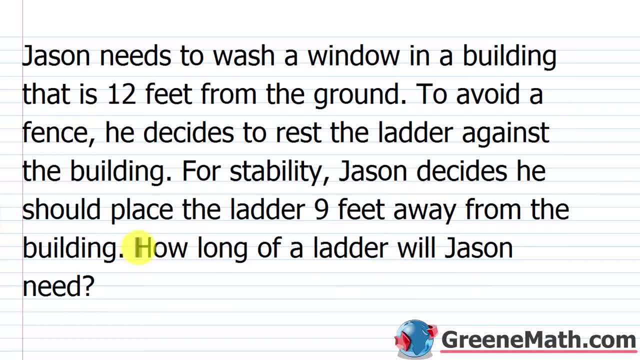 math here. So what we need to understand again is: what am I being asked to find? And in this case it's this little question here, right? So how long of a ladder will Jason need? So we just highlight that That's what we're trying to find. So when we go to assigning a variable, 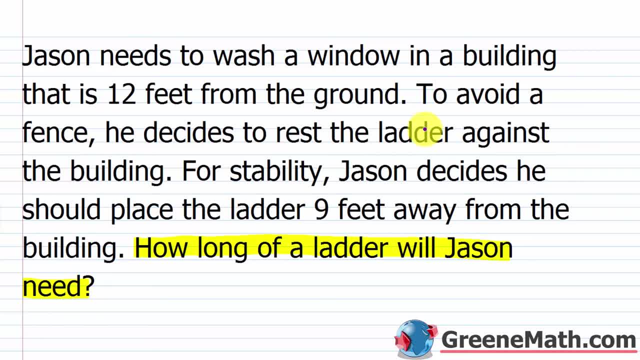 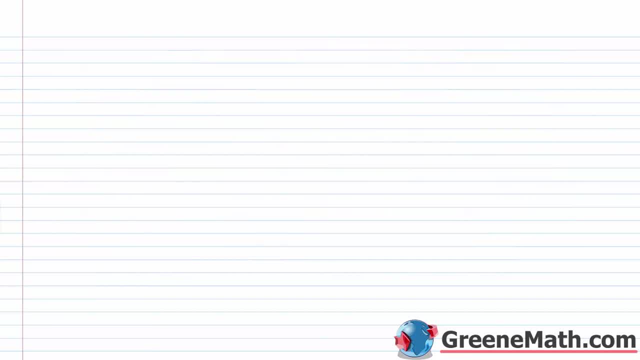 we're just going to let x represent exactly what we're trying to find, which is the measure of Jason's ladder, And this is going to be in feet, because we're working with feet in the problem. So let's go down here to a fresh sheet. We're going to say that we're going to let x be equal. 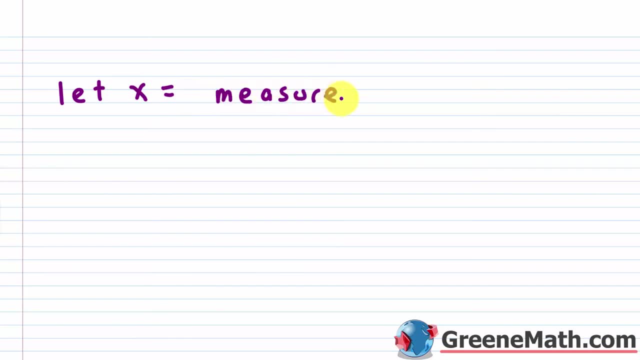 to the measure. So let's go down here to a fresh sheet. We're going to let x be equal to the measure of Jason's ladder, And of course this is going to be in feet. Okay, so in feet. All right, so I'm not going to write. 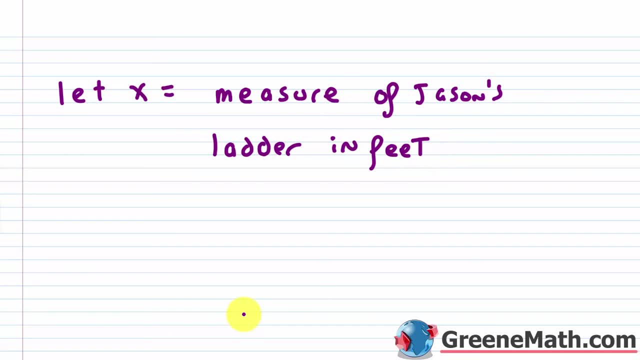 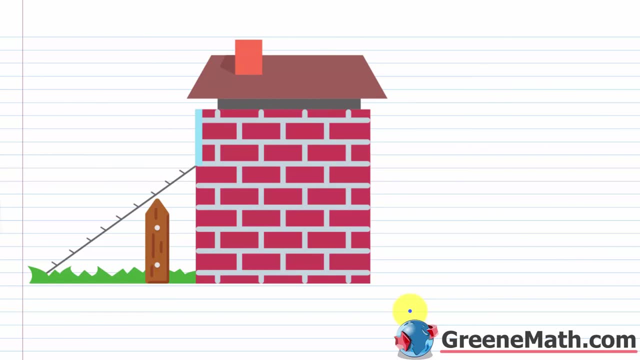 feet every time. I'm just going to work with the number parts. We're just going to understand that we're working with feet, All right. so to help us understand what's going on, we have this little illustration here. It's not perfect, but it'll just give you an idea of what's kind of happening. 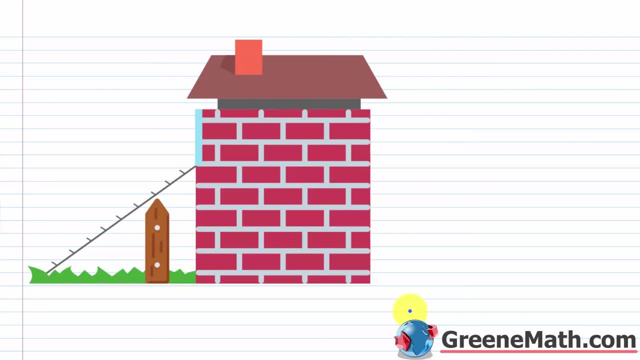 in our problem. So when we started out with the number part- we were just going to write feet out- we said that Jason wanted to wash a window in a building that is 12 feet from the ground. so this guy right here, this represents our window. okay, that's. 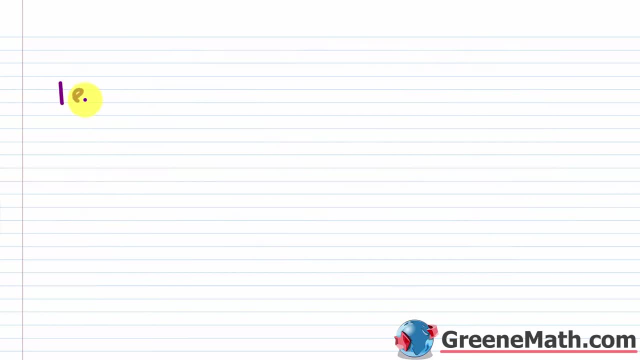 So let's go down here to a fresh sheet. We're going to say that we're going to let x be equal to the measure of Jason's ladder, And of course this is going to be in feet. Okay, So in feet. 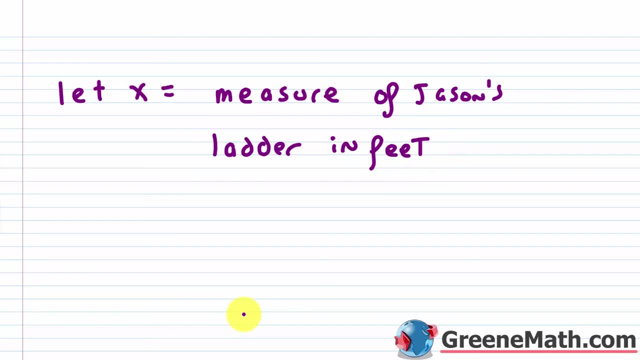 All right. So I'm not going to write feet every time, I'm just going to work with the number parts. We're just going to understand that we're working With feet, All right. So to help us understand what's going on, 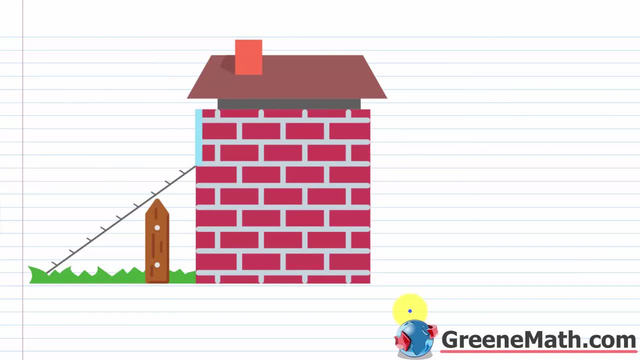 we have this little illustration here. It's not perfect, but it'll just give you an idea of what's kind of happening in our problem. So when we started out, we said that Jason wanted to wash a window in a building that is 12 feet. 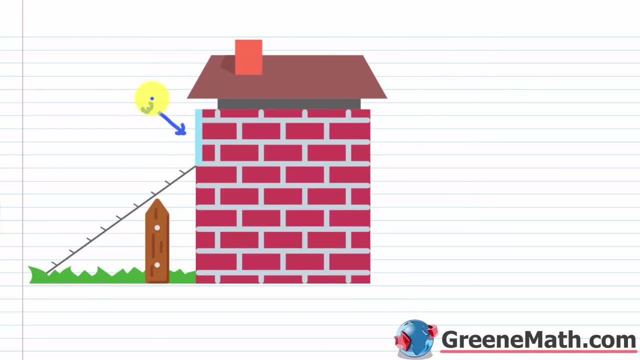 from the ground. So this guy right here, this represents our window. Okay, That's in our drawing And basically you could say that it's 12 feet from the ground. So from right here to right here, that measurement, let me kind of draw a little vertical. 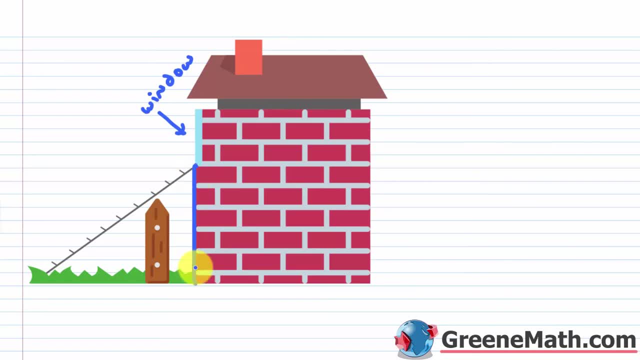 Okay, Vertical line: Okay, Not perfect, but it'll have to do So. this guy's going to be 12 feet. Again, I'm just going to put 12. and then also it tells us that for stability, Jason decides he should place the ladder nine feet away from the. 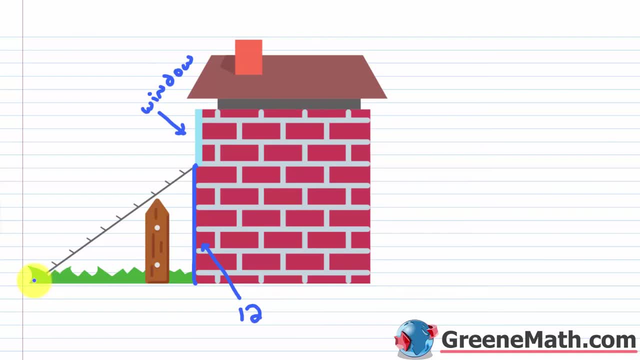 building. So the ladder: we can't see it cause it's hidden in the grass. but let's just say it's about right there. So from right there to right here, let me use a different color. So from right there to right here. 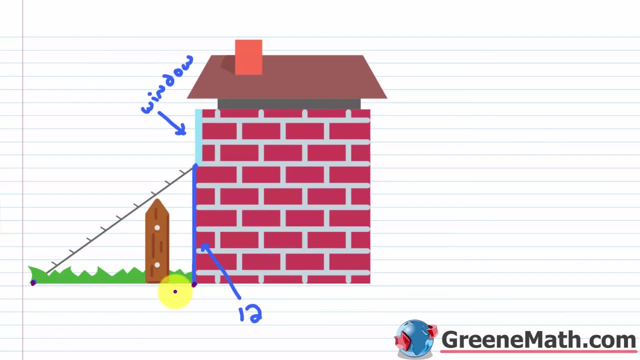 that horizontal measure is going to be nine feet, So let me again just draw a little horizontal line. Okay, Again, not perfect, but you get the idea. So this guy is nine feet, I'm just going to put nine and I can put my little symbol here. 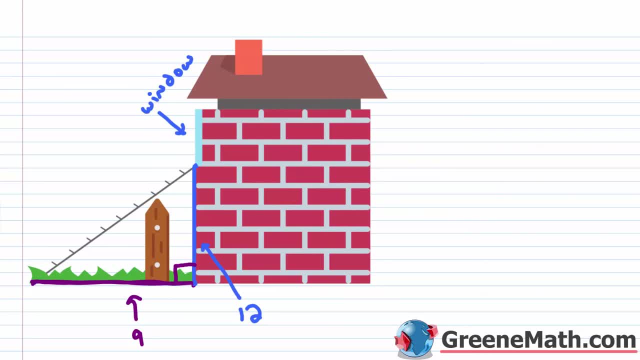 This is going to be a right angle, So I've got that symbol there. So we have a right triangle, right. We have that. this guy here: this horizontal leg is nine. This guy right here: this vertical leg is 12. and I'm solving for this guy right here. 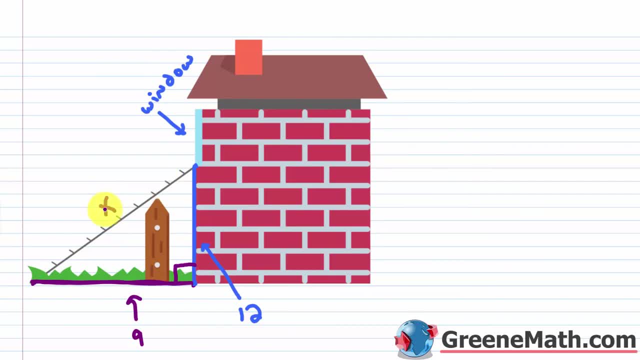 which is the length of his ladder. This is exactly what I need to find. I could just put this as X, right here. This guy is going to be the height I put news Okay, So essentially I can say that again for my Pythagorean formula. 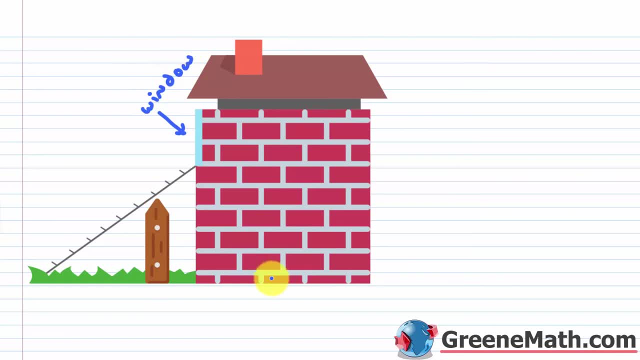 in our drawing and basically you could say that it's 12 feet from the ground. so from right here to right here- that measurement- let me kind of draw a little vertical line. okay, not perfect, but it'll have to do so. this guy's gonna be 12. 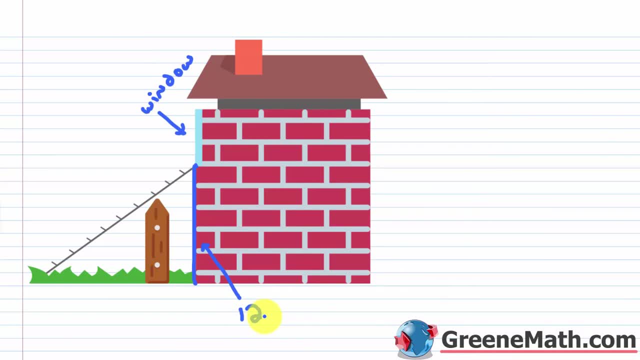 feet. again, I'm just gonna put 12. and then also it tells us that for stability Jason decides he should place the ladder nine feet away from the building. so the ladder we can't see because it's hidden in the grass. but let's just say it's. 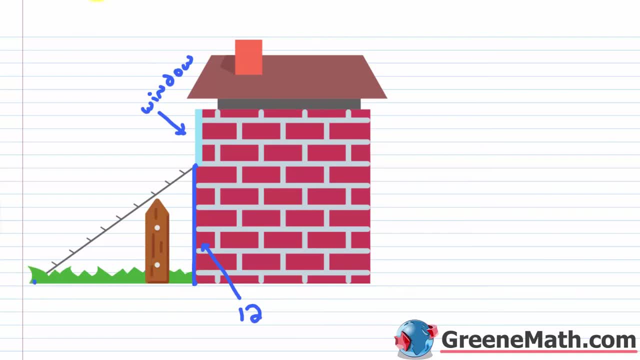 about right there. so from right there to right here, let me use a different color. so from right there to right here, that horizontal measure is going to be nine feet. so let me again just draw a little horizontal line. okay, again, not perfect. okay, so let me again just draw a little horizontal line. okay, again, not perfect. 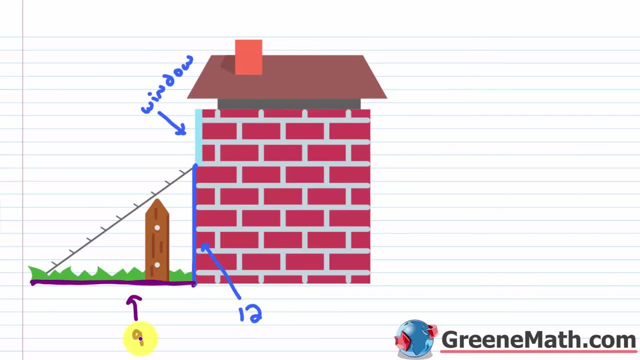 but you get the idea. so this guy is nine feet. I'm just gonna put nine and I can put my little symbol here. this is gonna be a right angle, so I've got that symbol there. so we have a right triangle, right, we have that. this guy here, this. 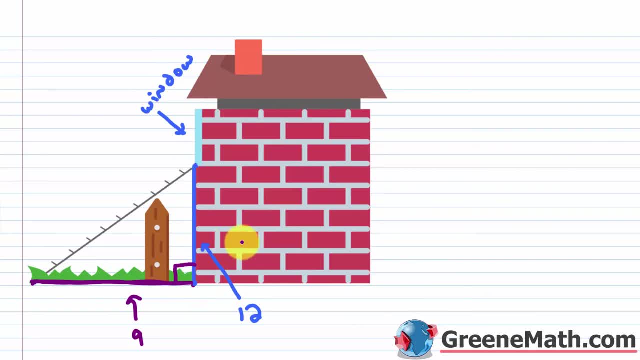 horizontal leg is nine. this guy right here. this vertical leg is 12, and I'm solving for this guy right here, which is the length of his ladder. this is exactly what I need to find. I could just put this as X. right here this guy is going to be. 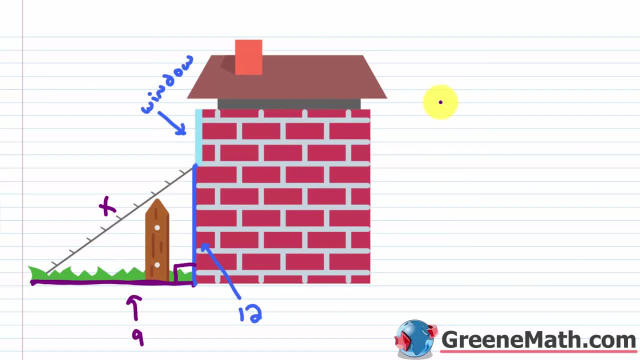 the hypotenuse okay. so essentially I can say that again for my Pythagorean formula, a squared plus B squared equals C squared, where a and B are the lengths of the two shorter sides or the legs right. so we know that's 9 and 12, so we just plug in and say that: 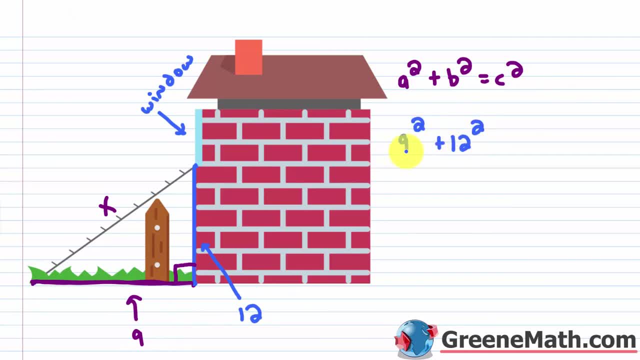 we have 9 squared plus 12 squared, and it doesn't matter the order that you do that in is equal to: instead of C, I just have X, so I'm gonna say this is X squared. okay. so 9 squared, we know, is 81, plus we know, 12 squares, 144. this equals. 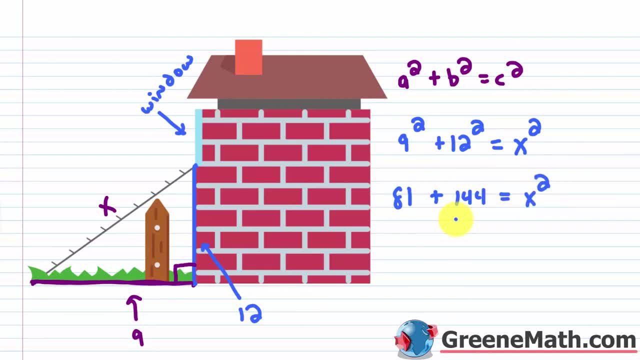 X squared, and 81 plus 144 equals C squared, so that's nine, and 12 squared is 144, is of course 225. So we get that x squared. okay, x squared is equal to 225. So we can solve this with our square root property. We know that x would be 15 or negative 15, right? Take the. 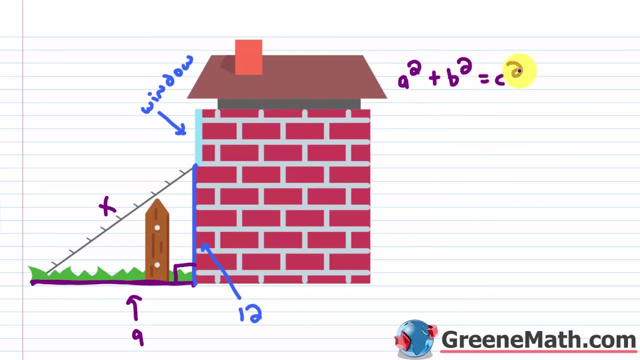 a squared plus B squared equals C squared, where a and B are the lengths of the two shorter sides or the lakes right. So we know that's nine and 12.. So we can just plug in and say that we have nine squared plus 12 squared. 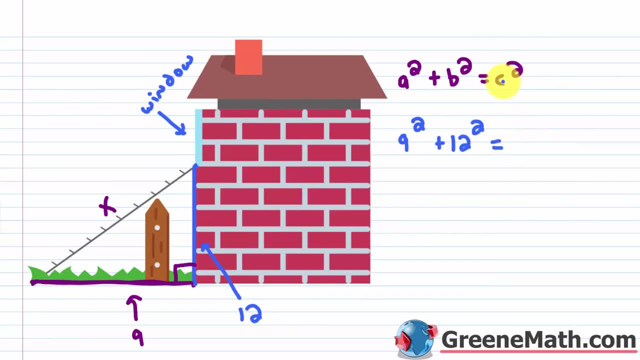 And it doesn't matter, The order that you do that in is equal to. instead of C, I just have X, So I'm going to say this is X square. Okay, So nine squared, we know, is 81.. Plus, we know, 12 squared is 144.. 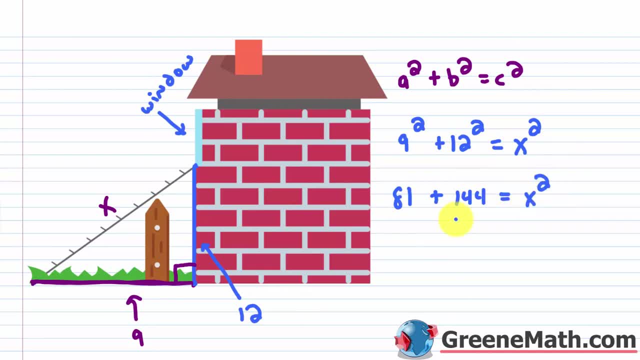 This equals X squared, and 81 plus 144 is, of course, 225. So we get that X squared. Okay, X squared is equal to 225. So we can solve this with our square root property. We know that X would be 15 or negative 15,. 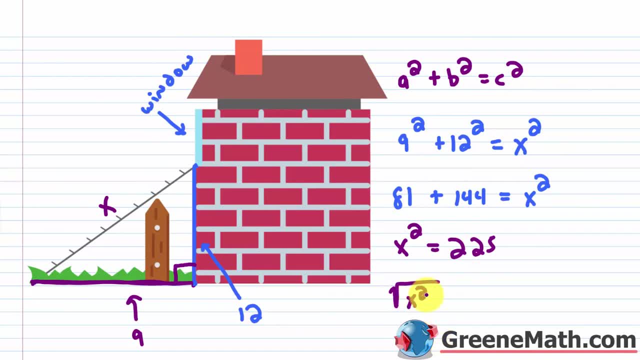 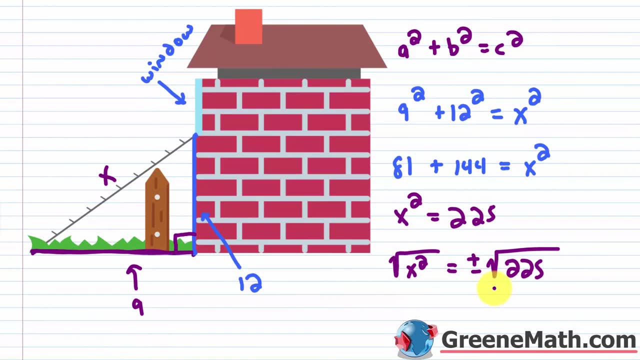 right, Take the square root of each side. So square root of this side is equal to plus or minus the square root of this side, And let me kind of scroll down and get a little bit of room going And we can basically say again: 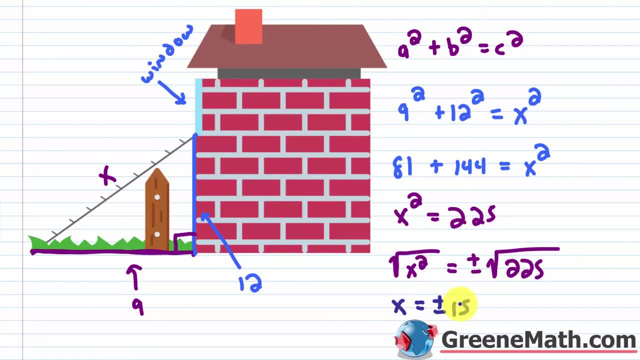 that X is equal to plus or minus 15.. Now does it make sense? Okay, Does it make sense for the measure of this ladder to be negative 15?? No, it's nonsense. Okay, So that's where you know. 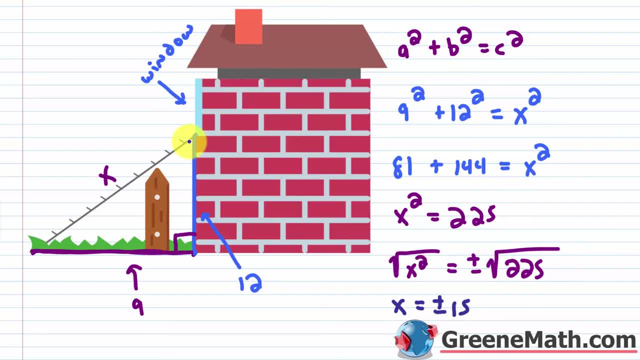 checking your answer When you think about kind of the steps we gave makes a lot of sense. So if you incorrectly said that the ladder could be 15 feet or negative 15 feet, when you go to check that you can say okay. 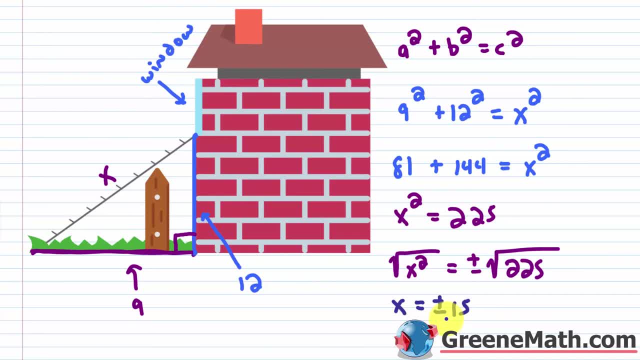 that doesn't make sense, right? A ladder can't measure Negative 15 feet. That that's complete nonsense. So you just have to throw that solution out and say that X or the kind of length of the measurement of that ladder, is going to be 15 feet. 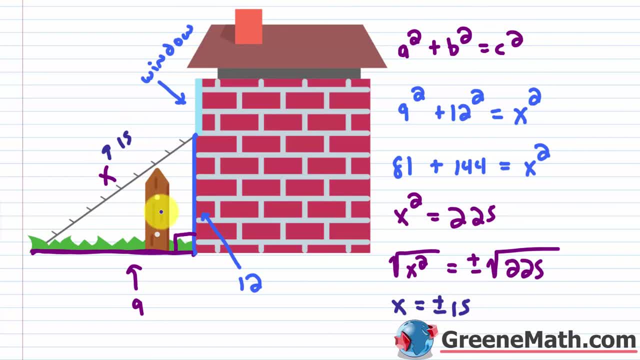 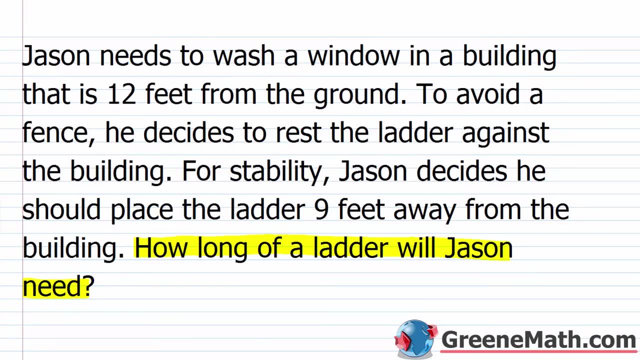 Okay, So I'm just going to write that in there and say this is 15, or again 15 feet, So let's go back up And again we can just kind of write a little sentence to describe our answer. So how long of a ladder will Jason need? 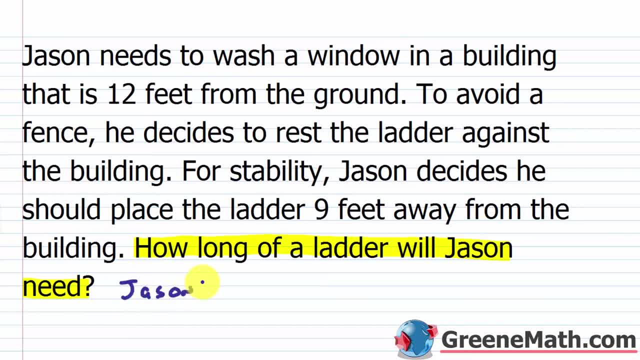 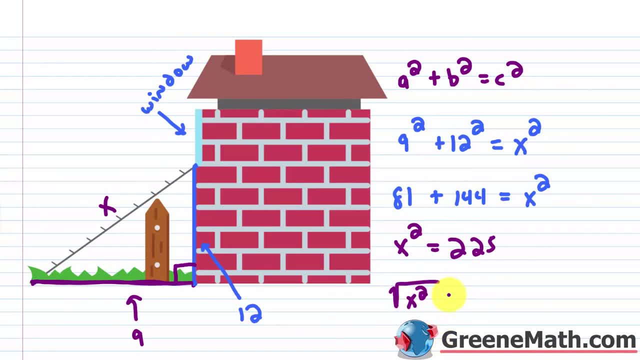 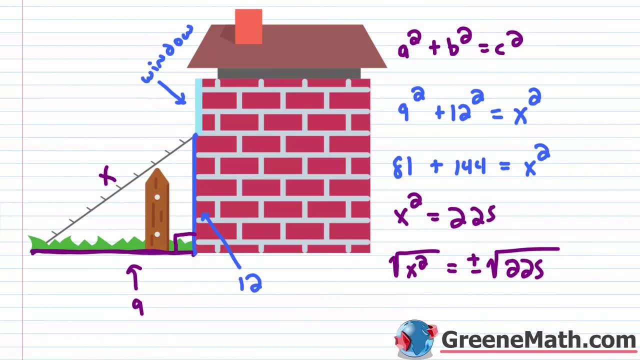 square root of each side. So square root of this side is equal to plus or minus the square root of this side. And let me kind of scroll down and get a little bit of room going And we can basically say again that x is equal to plus or minus 15.. Now does it make sense? Okay, does it make sense? 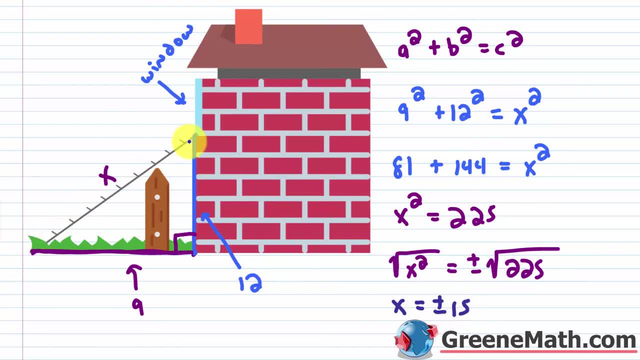 for the measure of this ladder to be negative 15?? No, it's nonsense. Okay, so that's where you know. checking your answer when you think about kind of the steps we gave makes a lot of sense. So if you incorrectly said that the ladder could be 15 feet or negative 15 feet when you go, 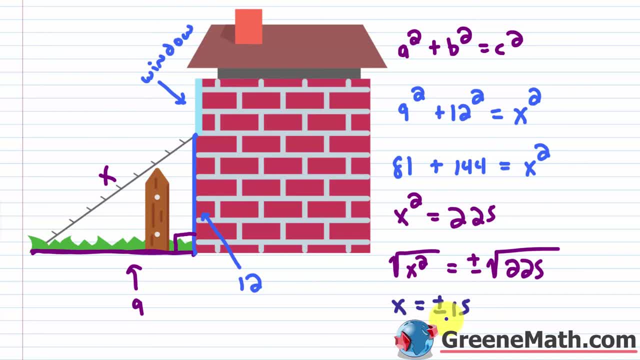 to check that. you can say: okay, that doesn't make sense, right, A ladder can't measure negative 15 feet. That's complete nonsense. So you just have to throw that solution out and say that x or the kind of length. 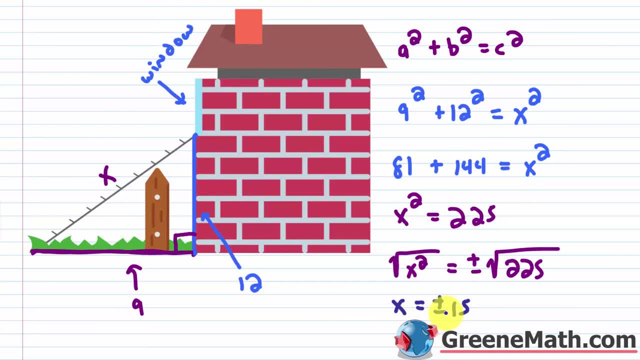 of the measurement of that ladder is going to be 15 feet. Okay, so I'm just going to write that in there and say: this is 15, or again 15 feet. So let's go back up And again we can just kind of 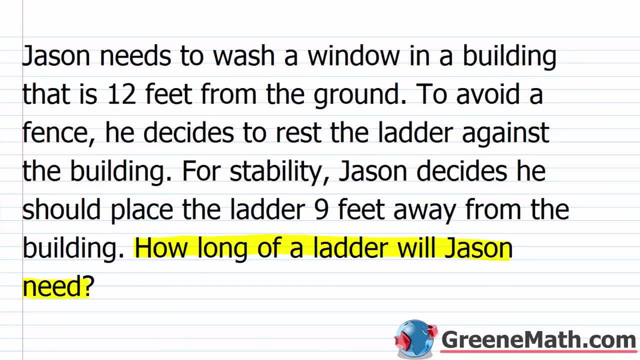 write a little sentence to describe our answer. So, how long of a ladder will Jason need? Well, we'll say that Jason needs a ladder. Jason needs a ladder that is 15 feet long. Okay, So checking this is really really easy. Again, we just go through our 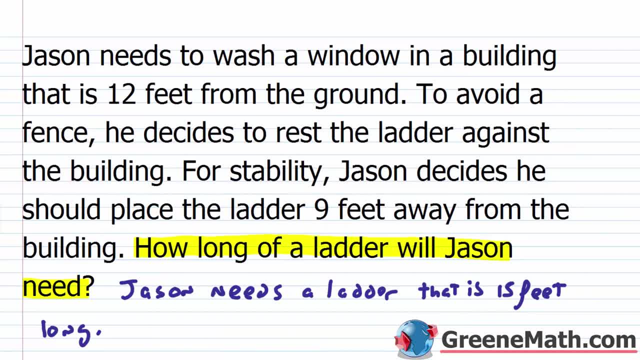 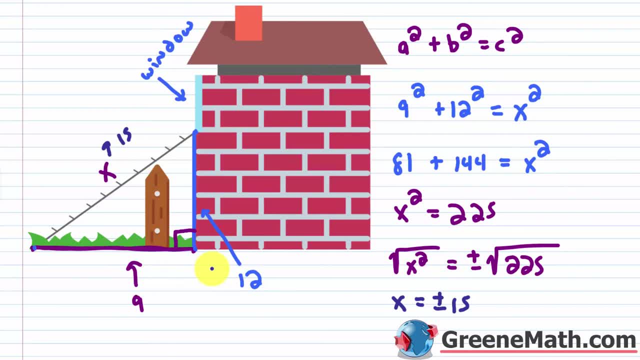 Pythagorean formula, And it's easier to check something like this by looking at the picture again, just so you get an idea what's going on. Again, we said that with Jason: he needs to wash a window in a building that's 12 feet from the ground, So this is where the window is And this 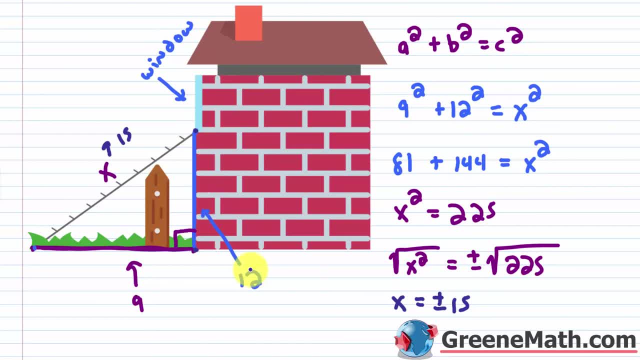 is where the ground is. So the distance from here to here, that's 12 feet. Okay, so that's where we got the 12 from, And then to avoid a fence, we're going to go through our Pythagorean formula. So 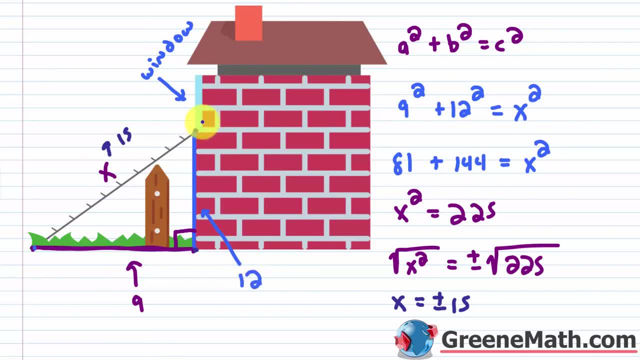 again, we see that we have a right triangle And so we can use our Pythagorean formula. We plugged in, we got nine squared plus 12 squared equals x. squared x was the length of the building, So the left side of this, which is 225.. So we ended up with x squared equals 225.. We took the square. 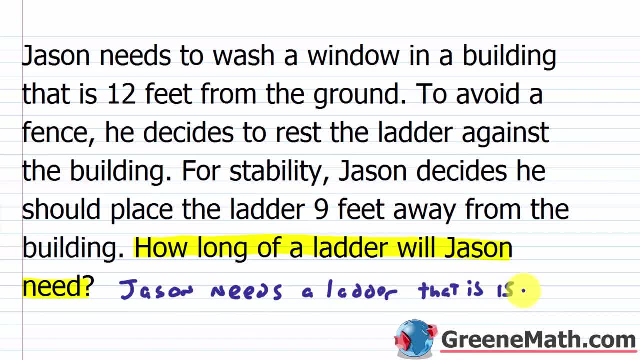 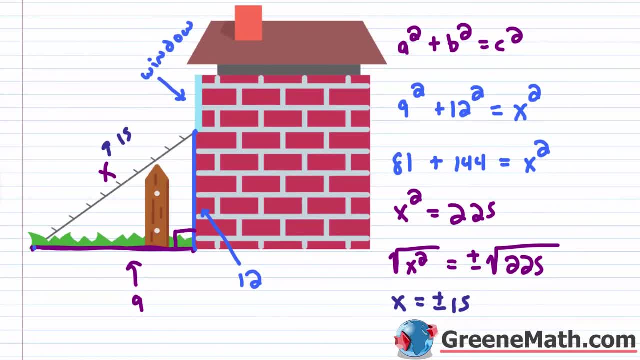 something like this: by looking at the picture- Again- this is- you get an idea of what's going on. Again, we said that with Jason: he needs to wash a window on a building that's 12 feet from the ground, So this is where the window is. 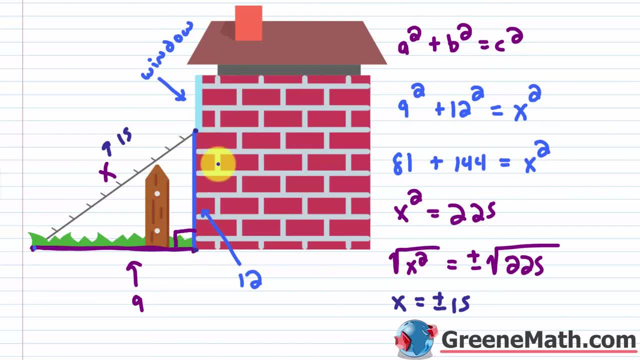 and this is where the ground is. So the distance from here to here, that's 12 feet. Okay, that's where we got the 12 from. And then, to avoid offense, he decides to rest the ladder against the building. So that's why this ladder is drawn in this manner. Okay, And then basically, 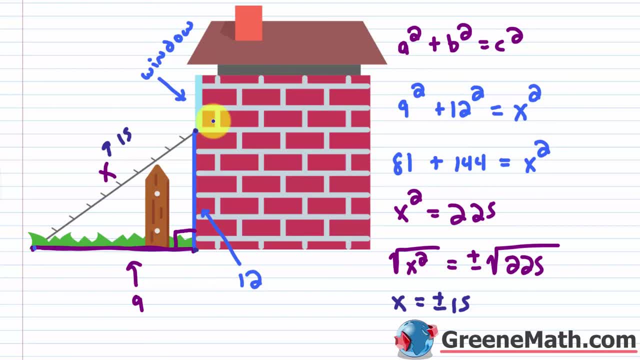 it says that, for stability, Jason decides he should place the ladder nine feet away from the building. So from here to here is nine feet. That's where we got that nine from. Okay, So this part all checks out. So then we're asked: how long of a ladder will he need? Well, again, we see that we. 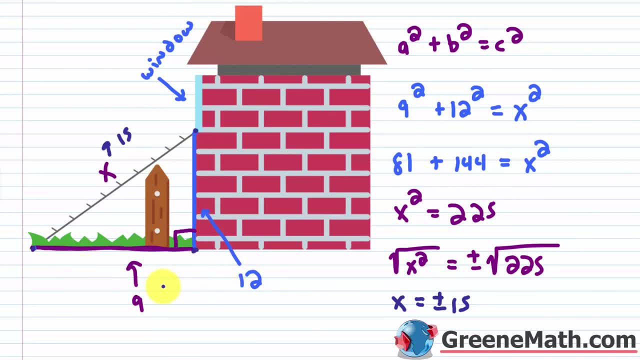 have a right triangle, And so we can use our Pythagorean formula. We plugged in, we got nine squared plus 12. squared equals X squared. X was the length of the ladder, And so we got 81 plus 144 on the left side of this, which is 225. So we ended up with X squared equals 225.. We took the. 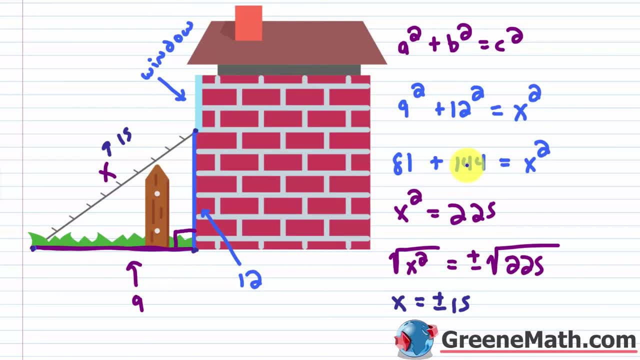 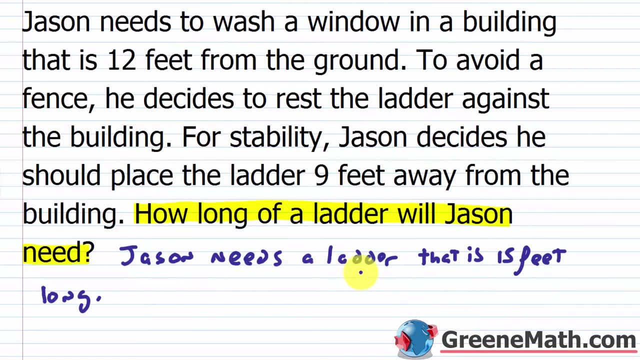 square root of each side right, And we found that we had X equals plus or minus 15.. We threw out negative 15 because it didn't make any sense. So that's how we got our solution, where we said that Jason needs a ladder that is 15 feet long. Okay, So this solution is correct. All right, Let's go. 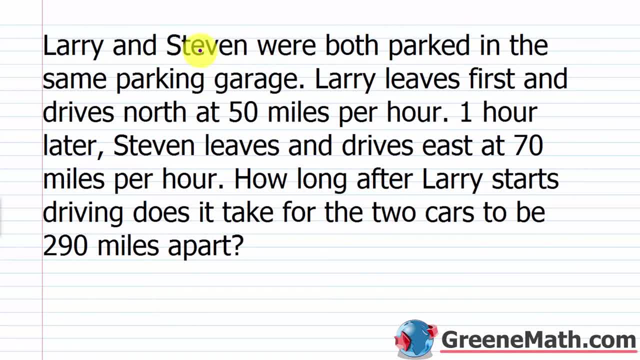 ahead and take a look at another one. So we have that. Larry and Steven were both parked in the same parking garage. Larry leaves first and drives north at 50 miles per hour. One hour later, Steven leaves and drives east at 70 miles per hour. 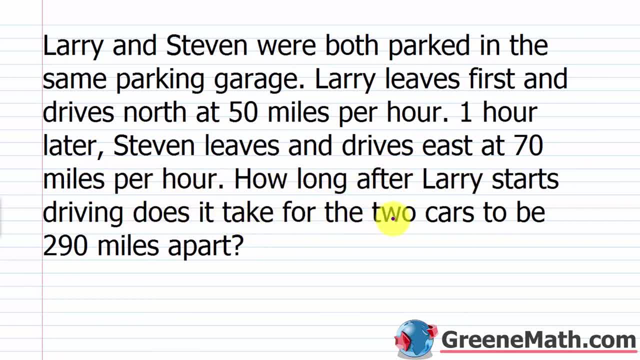 How long after Larry starts driving does it take for the two cars to be 290 miles apart? So again, we want to understand the main question and here it's just to find how long after Larry 90 miles apart. So for this problem we're going to end up using our Pythagorean formula And we're 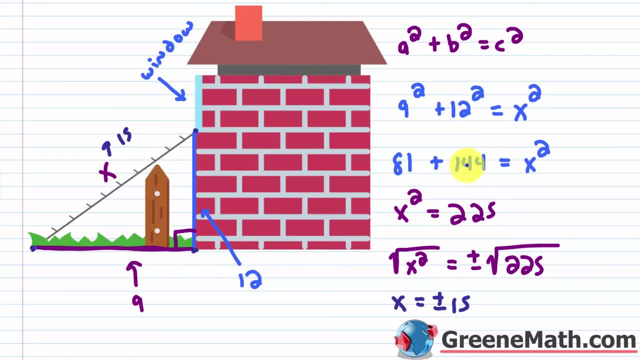 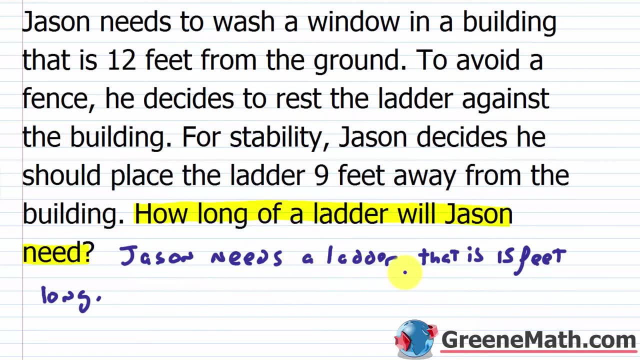 root of each side right, And we found that we had x equals plus or minus 15.. We threw out negative 15 because it didn't make any sense. So that's how we got our solution, where we said that Jason needs a ladder that is 15 feet long. Okay, so this solution is correct. All right, let's go ahead and 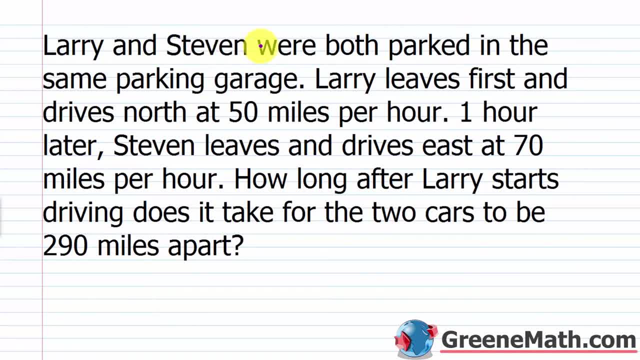 take a look at another one. So we have that Larry and Steven were both parked in the same parking garage. Larry leaves first and drives north at 50 miles per hour. One hour later, Steven leaves and drives east at 70 miles per hour. How long after Larry starts driving does it take for the two cars? 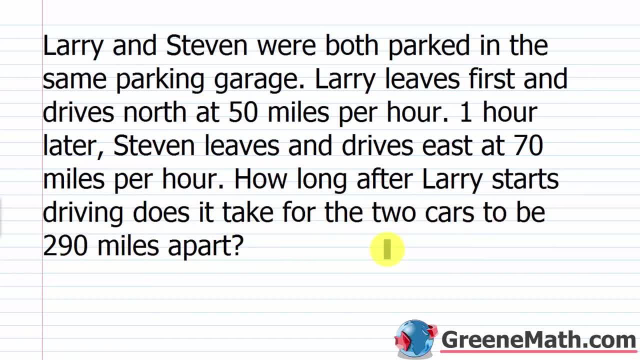 to be 290 miles apart. So again, we want to understand the main question, And here it's just to find: how long after Larry starts driving does it take for the two cars to be 290 miles apart? So for this problem we're going to end up using our Pythagorean formula And we're also going to use the 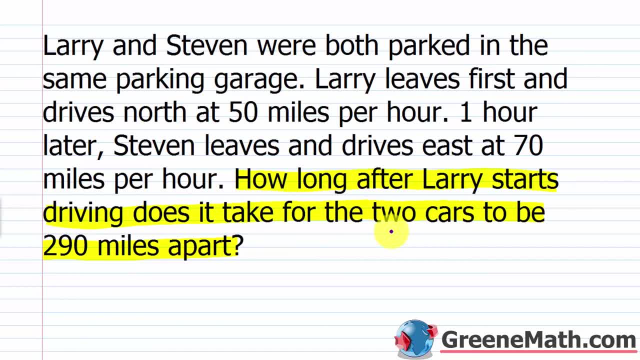 distance formula that we see with motion word problems. right, The distance equals the rate of speed, times the amount of time traveled. All right, so before we kind of get into that, though, we need to assign a variable to represent the unknown. In this case, we're going to end up. 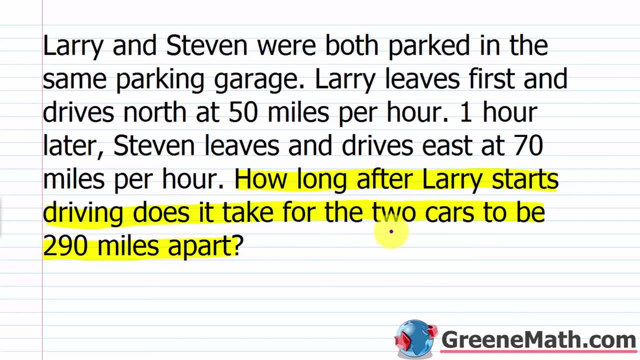 having kind of two unknowns, because we don't know how long Larry's going to drive for, We also don't know how long Steven's going to drive for. Okay, so what we're going to do is, since Larry leaves first, we're going to say that X is going to be 290 miles apart, So we're going to assign a variable. 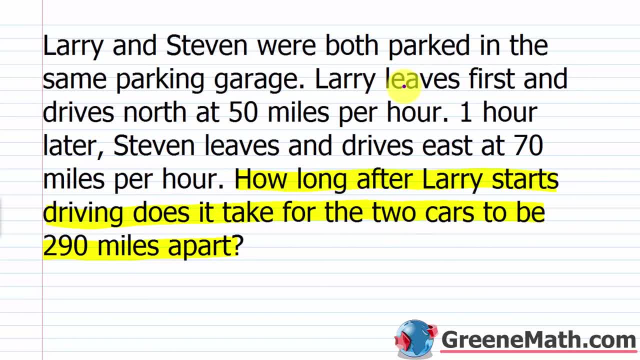 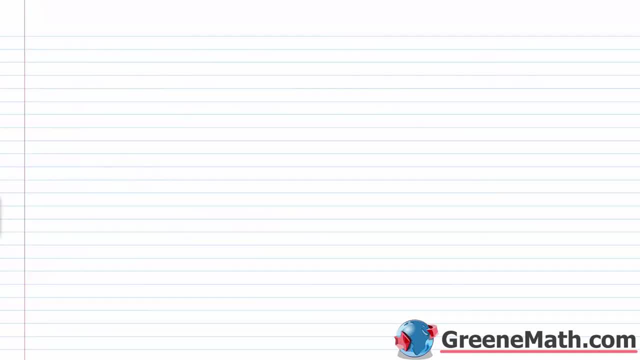 X is the amount of time that Larry drives for before. the two are 290 miles apart. Okay, so let's go down here to a fresh sheet And I'm just going to say we're going to let X be equal to the amount of time And I'm just going to put for Larry: Okay, and we know what that means It's going to. 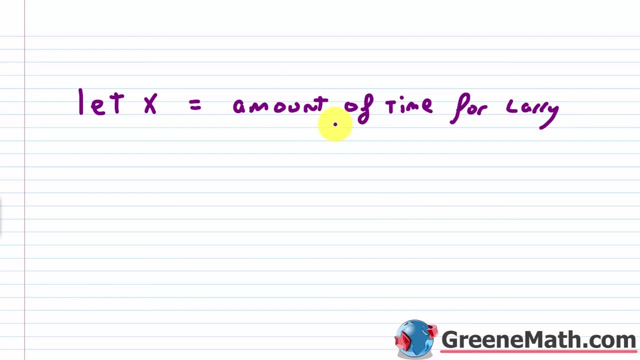 be specifically in hours And it's going to be the amount of time that Larry drives for before. again, the two cars are 290 miles apart, So we're going to let X be equal to the amount of time that Larry drives for before. the two are 290 miles apart. 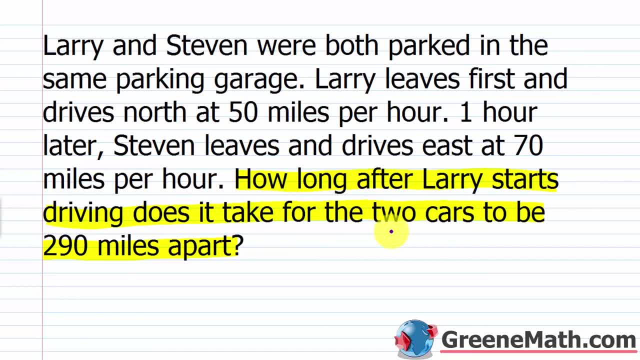 also going to use the distance formula that we see with motion word problems. right, The distance equals the rate of speed times, the amount of time traveled. All right, so before we kind of get into that, though, we need to assign a variable to represent the unknown. In this case, we're going. 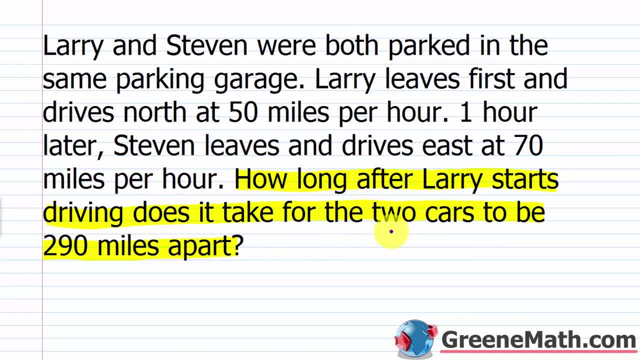 to end up having kind of two unknowns, because we don't know how long Larry's going to drive for, We also don't know how long Stephen's going to drive for. Okay, so what we're going to do is, since Larry leaves first, we're going to say that x is the amount of time that Larry drives for before. 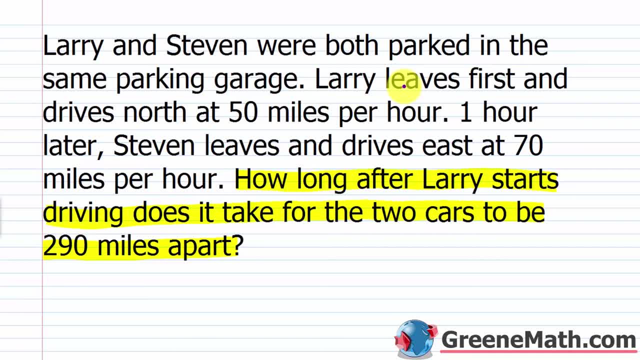 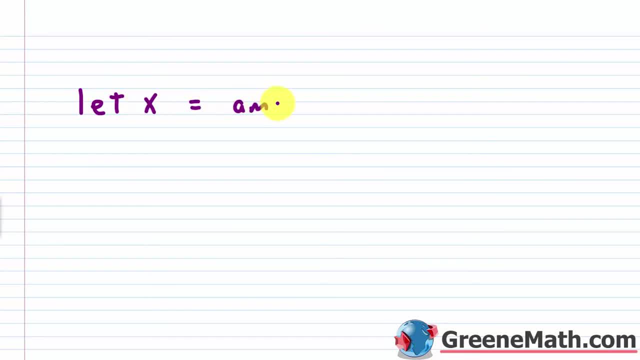 the two are 290 miles apart. Okay, so let's go down here to a fresh sheet And I'm just going to say we're going to let x be equal to the amount of time, And I'm just going to put for Larry: Okay. 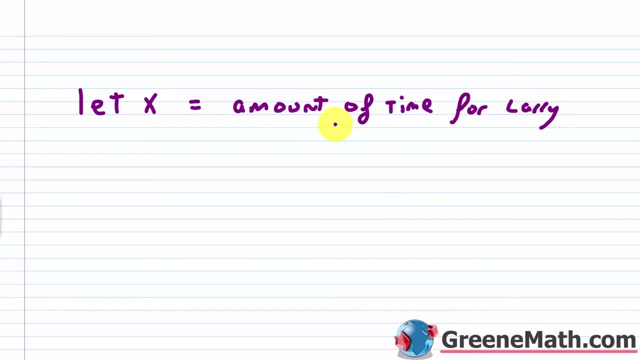 and we know what that means. It's going to be be specifically in hours and it's going to be the amount of time that larry drives for. before again, the two cars are 290 miles apart. now for steven, we can kind of base his time on larry's right. 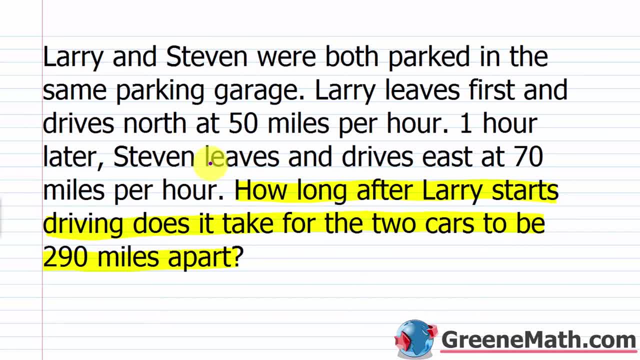 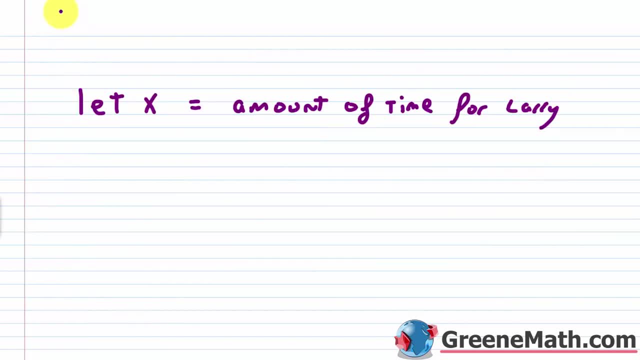 we know larry's time is x. well, for steven, we know that one hour later steven leaves, so he's been driving for an hour less at this point, when they are 290 miles apart. so i can just go x minus one to represent steven's time. okay, so we're going to say then i'll do that in a different color. so 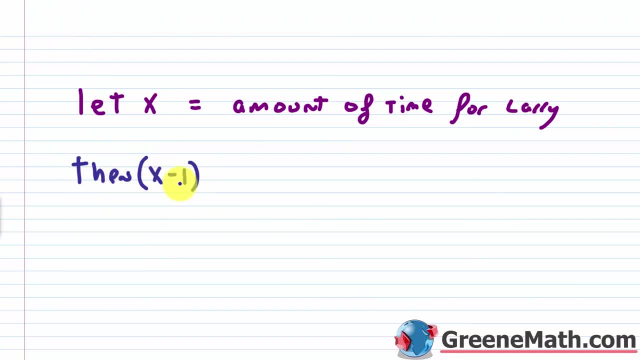 we'll say then: x minus one, this quantity is the amount, again, of time for steven. okay, we'll just make it nice and simple. like that you could write out something that's really long and say it's the amount of time for steven. you know, in hours before they're 290 miles apart, but you kind of get the 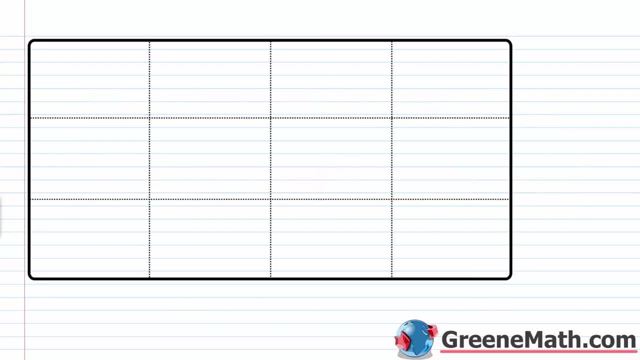 idea and we want to make it as short as possible. so we're going to make it as short as possible, all right. so the next thing we want to do is just come down to a little table, just organize our information so that we know what's going on. so our distance formula, in case you forgot the distance. 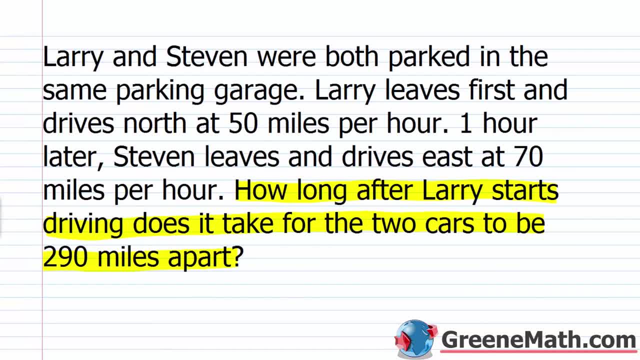 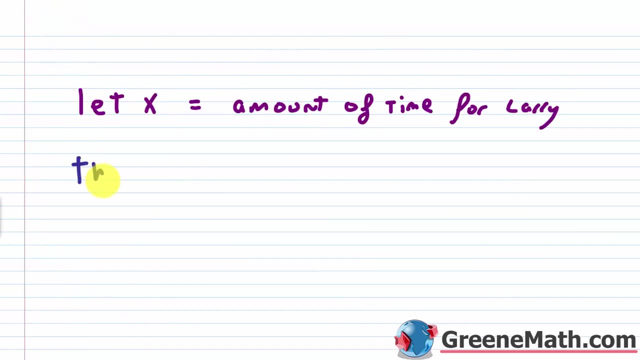 Now for Steven. we can kind of base his time on Larry's right. We know Larry's time is X. Well, for Steven, we know that one hour later Steven leaves. So he's been driving for an hour less at this point, when they are 290 miles apart. So I can just go X minus one to represent Steven's time. Okay, so we're going to say then I'll do that in a different color. So we'll say then, X minus one, this quantity is the amount. 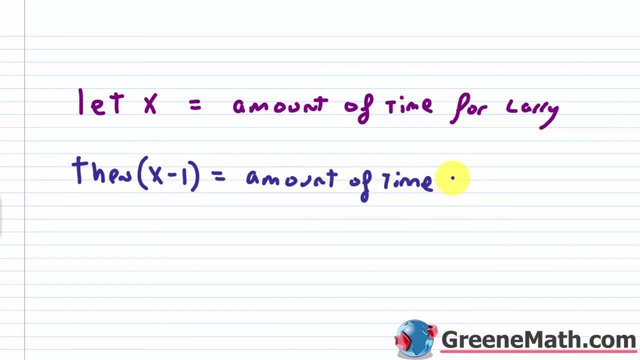 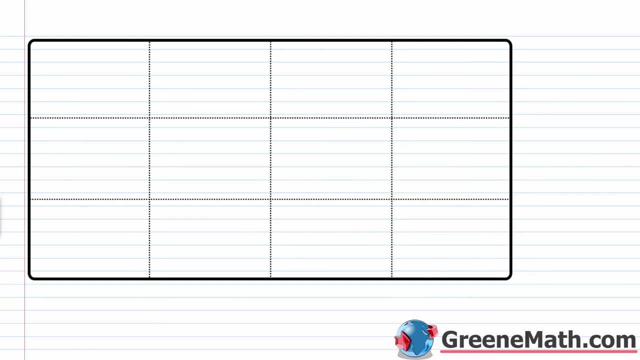 of time for Steven. Okay, we'll just make it nice and simple. like that You could write out something that's really long and say it's the amount of time for Steven. you know, in hours before they're 290 miles apart, But you kind of get the idea. and we want to make it as short as possible, All right, so the next thing we want to do is just come down to a little table, just organize our information so that we know what's going on. So our distance formula, in case you forgot the distance. 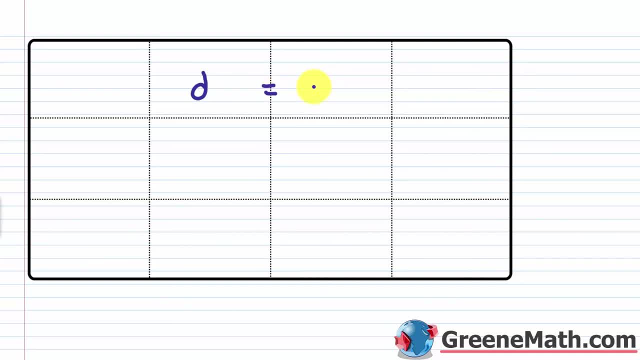 traveled, which I'm going to say is D, is equal to the rate of speed, which is R multiplied by the amount of time traveled, which is T. Okay, so the rate of speed is in miles per hour, the time is in hours and the distance is going to be in miles, Okay. And then we have two participants here: we have Larry, And then we have Steve, Okay, so those two guys are involved in the problem. So what information do we have? Well, we know the time, because we said that Larry is going to be driving for X hours. 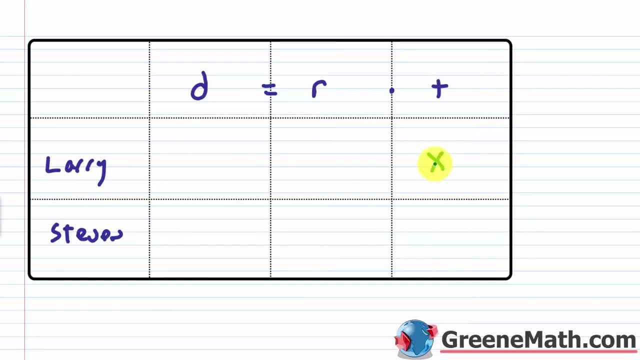 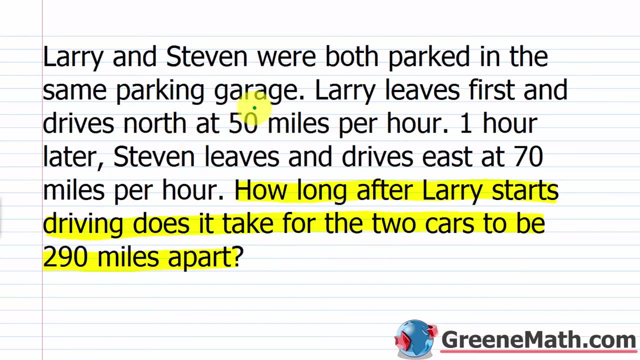 When the two are 290 miles apart. And we said that Steven, since he drives an hour less, is going to be driving for X minus one hours again when they're 290 miles apart. Now the rate we can get directly from the problem, it tells us specifically that Larry leaves first and drives north at 50 miles per hour, So this 50 miles per hour is going to be his rate of speed. And then for Steven, he leaves and drives east at 70 miles per hour, So 70 is going to be his rate of speed, again in terms of miles per hour. So let's just fill this in. 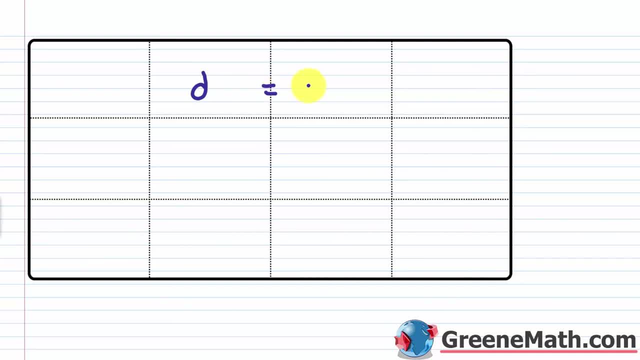 traveled, which i'm going to say is d, is equal to the rate of speed, which is r multiplied by the amount of time traveled, which is t. okay, so the rate of speed is in miles per hour, the time is in hours and the distance is going to be in miles. okay, and then we have two participants here. we 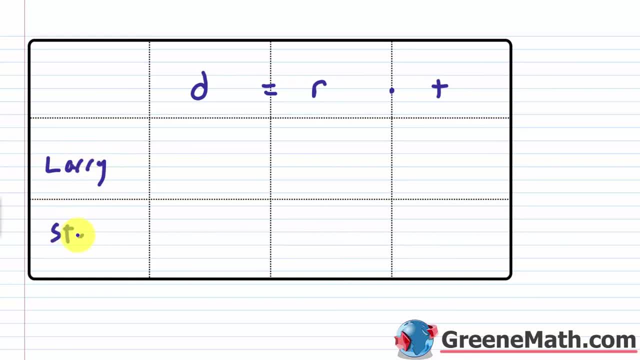 have larry and then we have steve. okay, so those two guys are involved in the problem. so what information do we have? well, we know the time because we said that larry's going to be driving for x hours when the two are 290 miles apart, and we said that steven, since he drives an hour less, is going to be. 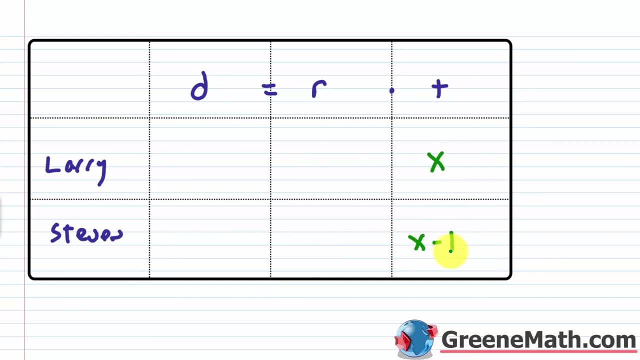 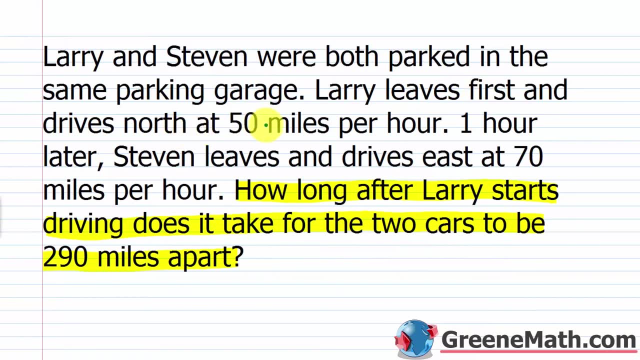 driving for x minus one hours again when they're 290 miles apart. now the rate we can get directly from the problem. it tells us specifically that larry leaves first and drives north at 50 miles per hour. so this is going to be the time that we're going to be driving for x hours, and then we have 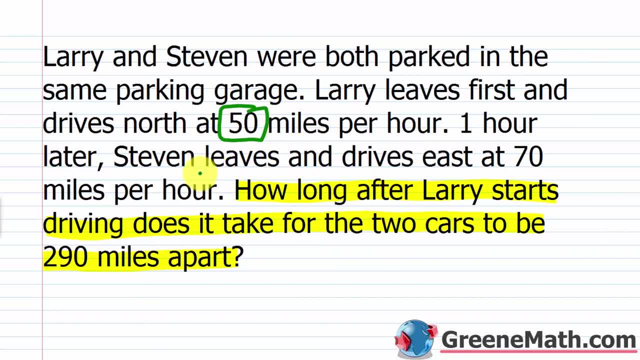 50 miles per hour is going to be his rate of speed. and then for steven he leaves and drives east at 70 miles per hour. so 70 is going to be his rate of speed, again in terms of miles per hour. so let's just fill this in: for larry it's going to be 50 miles per hour, for steven it's going to be 70. now, 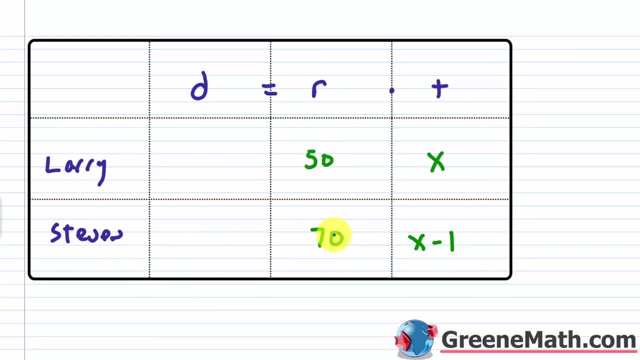 if i have a rate of speed and i have a time, i have a distance right, because i can just multiply r times t gives me d. so 50 times x is 50x and that's my distance. that's larry's going to travel when they're 290 miles apart. so for steven, he's going to have traveled 70 times the quantity. 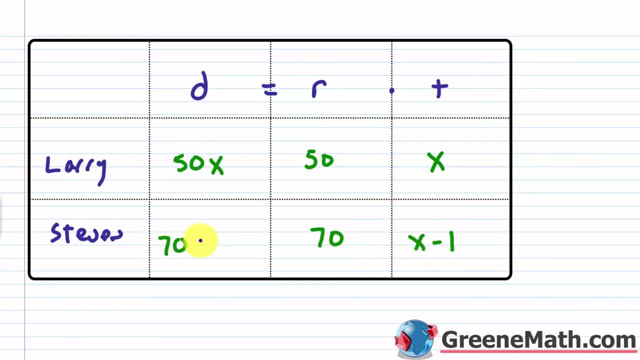 remember this is a quantity and this is multiplication, so put parentheses. so times the quantity x minus one, and you can go ahead and simplify this now, because you're going to have to later. you can just say: this is 70x minus 70, so we'll write this as 70x minus 70, just so that we 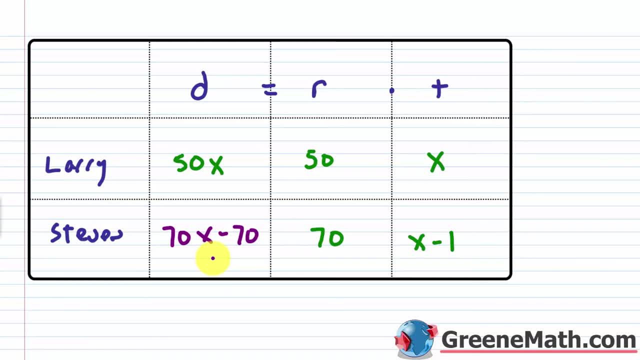 have it ready to go, okay. so before we kind of set up our equation, i want you to think about something, because usually at the end of the day, you're going to have a rate of speed and you're going to have this point. people make a drastic mistake. they're used to kind of solving these in another scenario. 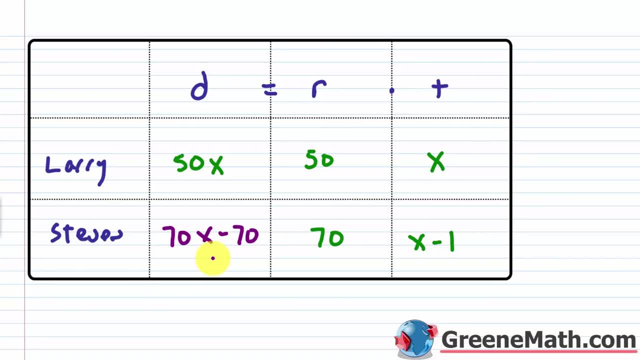 kind of with the opposite direction, travel with that one. they end up saying, okay, well, the distance larry travels, which is 50x, plus the distance steven travels, which is 70x minus 70. they sum those two amounts and they say, okay, well, that's got to be equal to 290. okay, this is wrong, this. 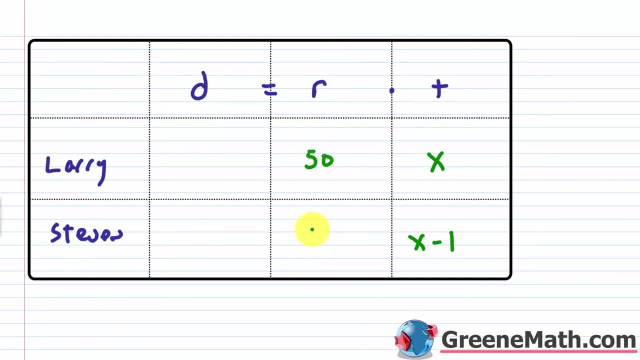 For Larry it's going to be 50 miles per hour, For Steven it's going to be 70.. Now if I have a rate of speed and I have a time, I have a distance right, Because I can just multiply R times T gives me D. So 50 times X is 50X And that's my distance, as Larry's going to travel again when they're 290 miles apart. So for Steven he's going to have traveled 70 times the quantity. Remember this is a quantity and this is multiplication, So put parentheses. So times the quantity X minus one. 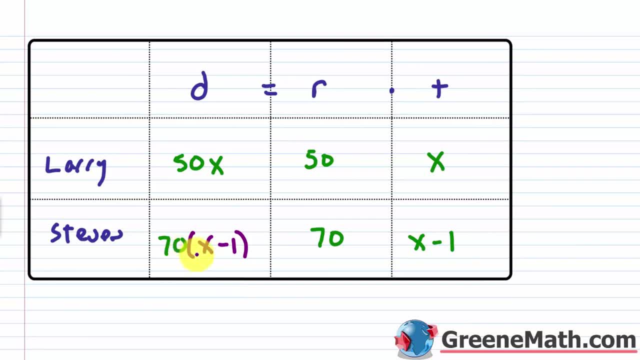 And you can go ahead and simplify this now, because you're going to have to later. You can just say: this is 70X minus 70. So we'll write this as 70X minus 70, just so that we have it ready to go. 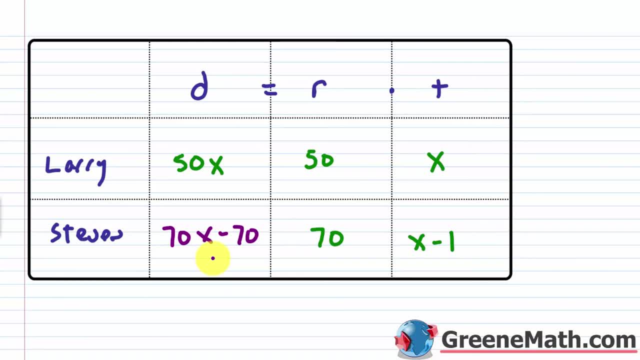 Okay, so before we kind of set up our equation, I want you to think about something, because usually at this point people make a drastic mistake. They're used to kind of solving these in another scenario, kind of with the opposite direction travel. 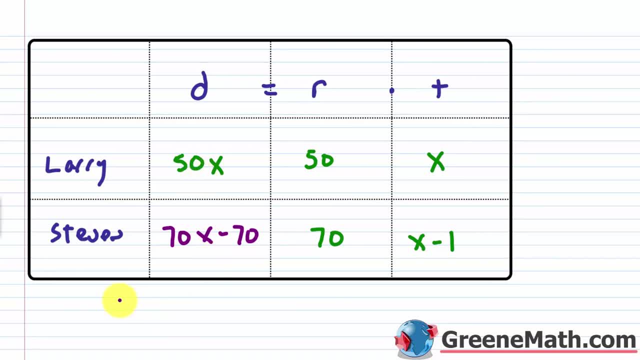 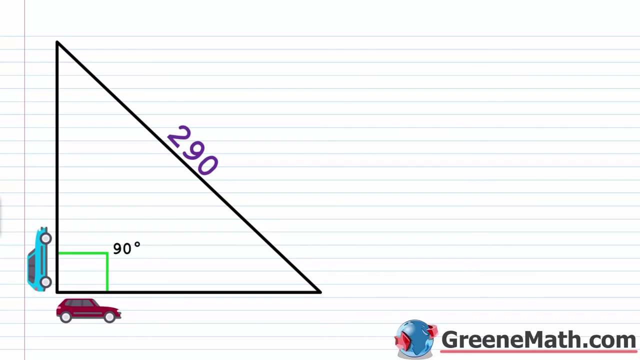 With that one, they end up saying, okay, well, the distance Larry travels, which is 50X, So 50X plus the distance Steven travels, which is 70X minus 70. They sum those two amounts and they say, okay, well, that's got to be equal to 290. Okay, this is wrong. This is what we saw kind of earlier in the course. This is not the current setup. Okay, what we have here- and just to kind of illustrate what's going on, I drew a little picture, a little illustration, And basically what we have again is another application of the Pythagorean formula, because we end up with something that is a right triangle, Okay. 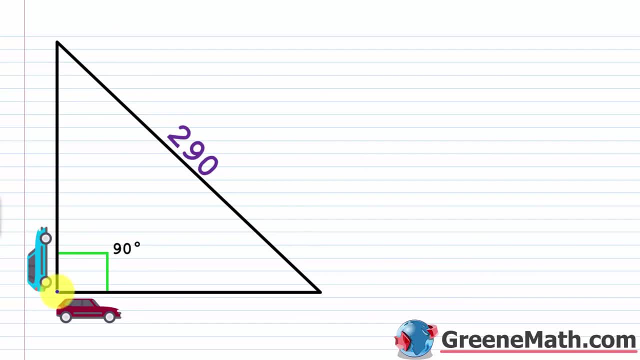 So we have that Larry is driving north. So you can picture him starting from here. Let's just say that's the parking garage And he drives north, which on every map that you look at, that's basically going up. Okay, so this is going to be a vertical leg for the right triangle And we know that measure the distance, if I go back, is going to be what? It's 50X. So let's go back here And I'm just going to write this in as 50X And we know that's for Larry. So I'm just going to put a little arrow here and say that's L for Larry. Okay, that's his distance. 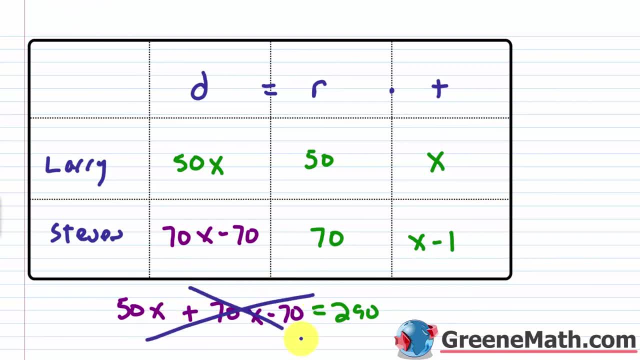 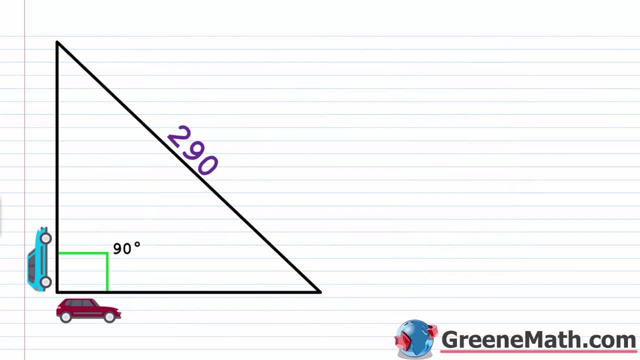 is what we saw kind of earlier in the course. this is not the current setup. okay, what we have here, and just to kind of illustrate what's going on here, is that we have a rate of speed and we have. i drew a little picture, a little illustration and basically what we have again is another. 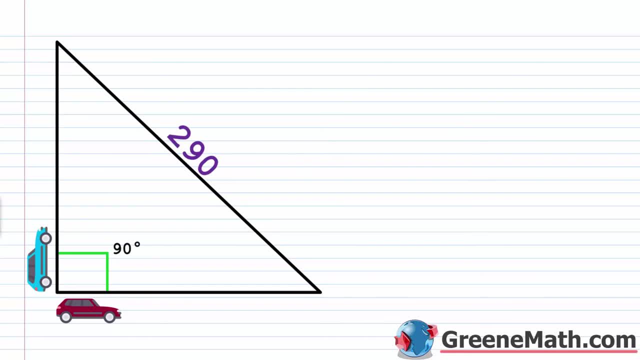 application of the pythagorean formula, because we end up with something that is a right triangle. okay, so we have that. larry is driving north, so you can picture him starting from here. let's just say that's the parking garage and he drives north, which on every map that you look at, that's. 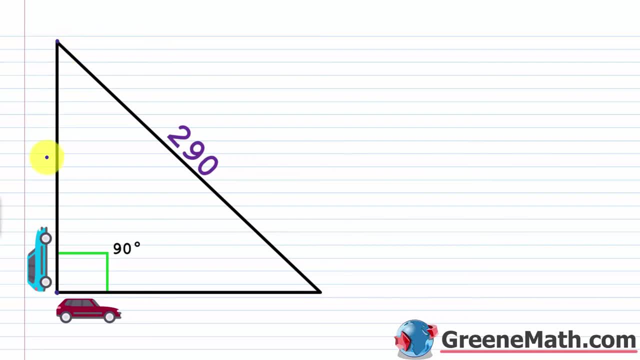 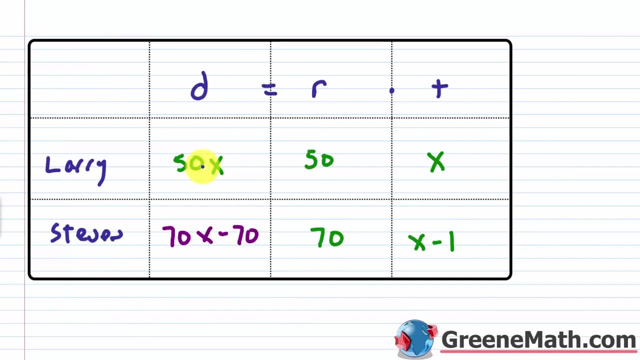 basically going up. okay, so this is going to be a vertical leg for the right triangle and we know that measure the distance, if i go back, is going to be what it's: 50x. so let's go back here and i'm just going to write this in as 50x. 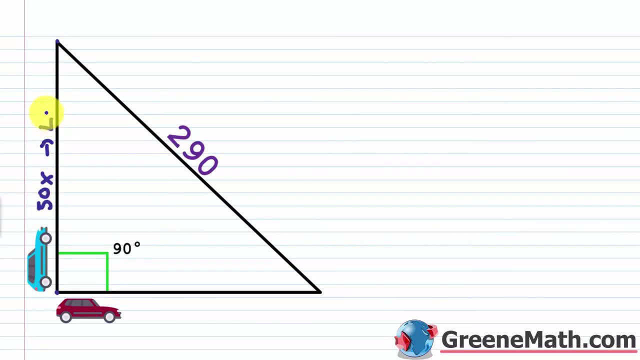 and we know that's for larry. so i'm just going to put a little arrow here and say that's l for larry. okay, that's his distance. that's again from here to here. that's the point he's going to be at when these two guys are 290 miles apart from each other. now for steven, let me put a little s. 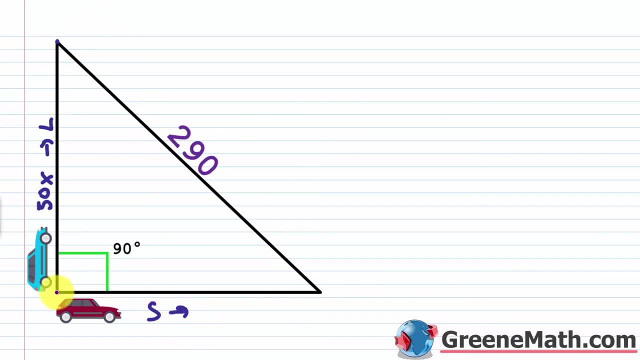 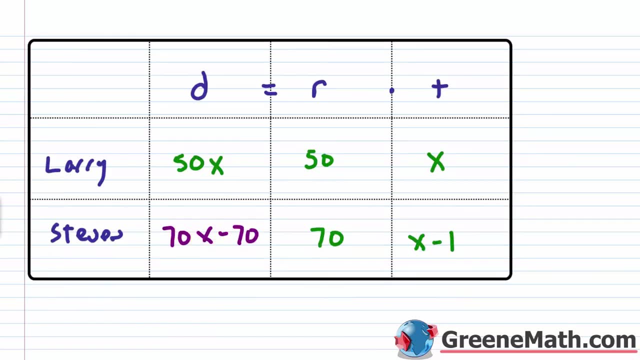 here and go this way, he's got this horizontal leg. so this guy to this guy, that distance. there again, if we go back up, that's 70x minus 70. so let me put this here as 70x minus 70. okay, so you can. 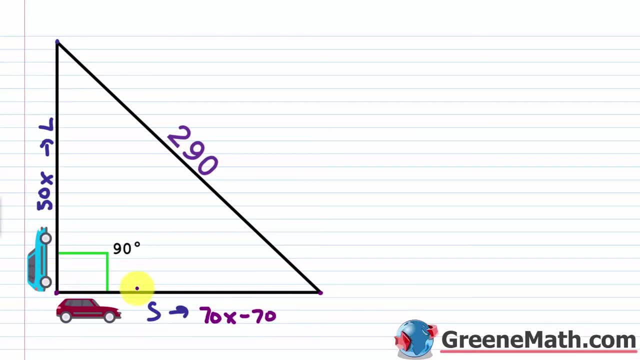 obviously see what's going on here. we've got our two legs for this right triangle and again the formula is that a squared plus b squared. okay, we square each of the legs and we sum those amounts together. this is equal to the hypotenuse squared, so c squared again. normally this is c, but in this 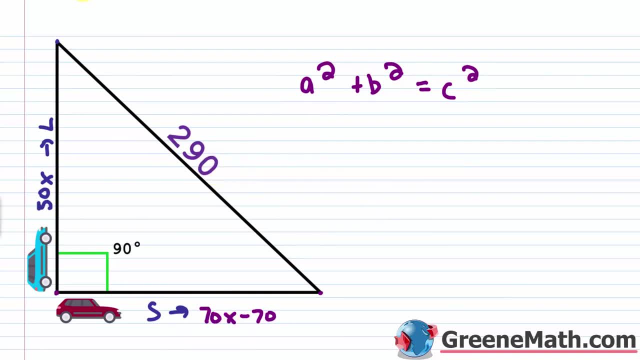 case. we have kind of expressions involved, so we're just going to put a little s here and go ahead and just kind of plug those in and work with those. so we end up with, let's just say, 50x, that quantity squared. then plus this guy is the quantity 70x. minus 70, the whole thing is squared. 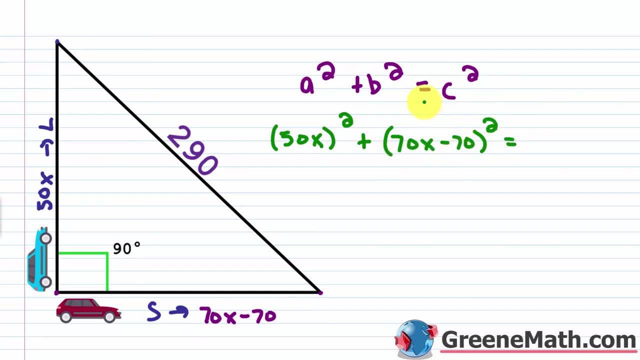 so make sure you wrap it in parentheses. and this equals our c, our hypotenuse is going to be 290, so that amount that's going to be squared, okay. so we're going to just copy this and go to a fresh sheet, because we'd run out of room here, because this is going to be quite tedious, so let's just 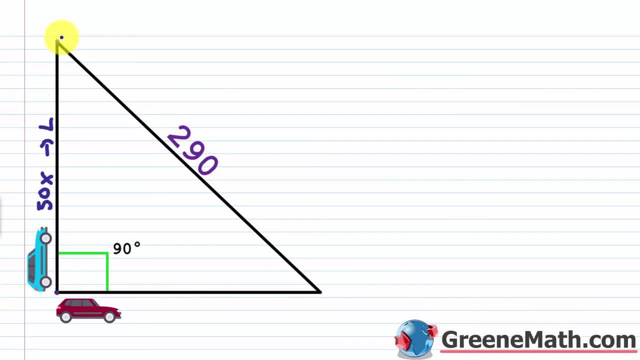 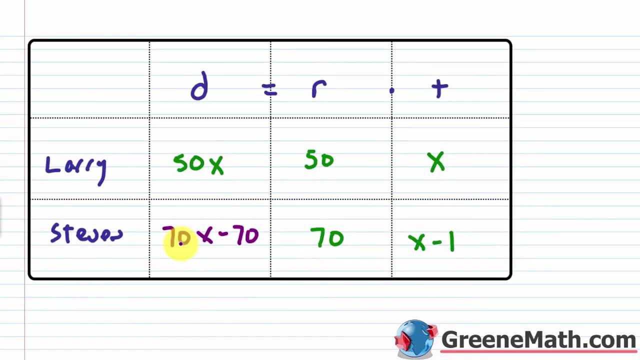 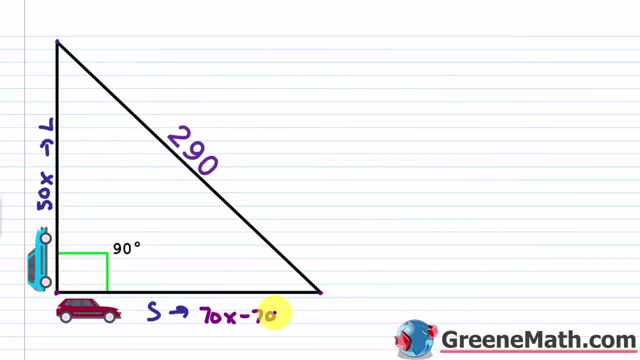 That's again from here to here. That's the point he's going to be at, when these two guys are 290 miles apart from each other. Now for Steven. let me put a little S here and go this way: He's got this horizontal leg. So this guy to this guy, that distance there. Again, if we go back up, that's 70X minus 70. So let me put this here as 70X minus 70.. Okay, so you can obviously see what's going on here. We've got our two legs for this right triangle. 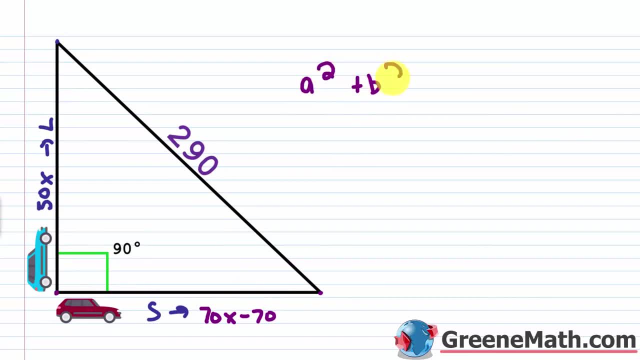 And again the formula is that A squared plus B squared, Okay, we square each of the legs and we sum those amounts together. This is equal to the hypotenuse squared. So C squared Again, normally this is C, But in this case we have kind of expressions involved, So we just kind of plug those in and work with those. So we end up with, let's just say, 50X. that quantity squared then plus this guy, is the quantity 70X minus 70.. The whole thing is squared. So make sure you wrap it in parentheses. 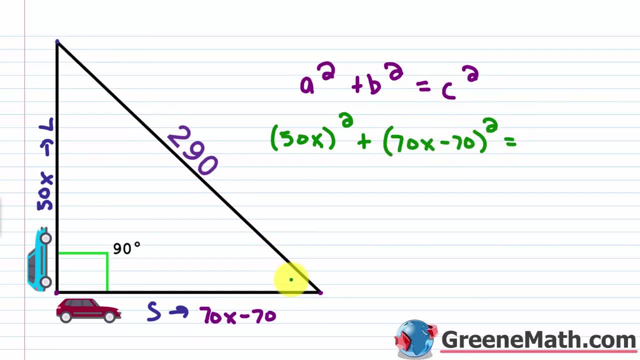 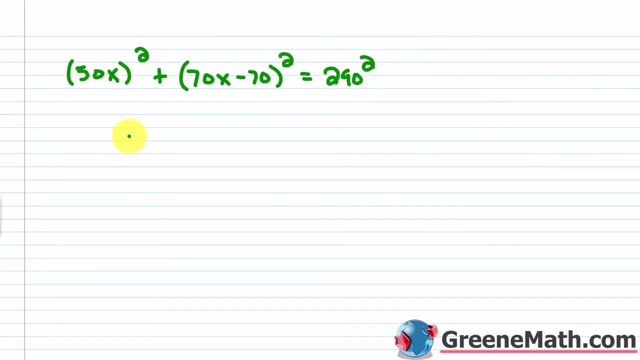 And this equals our 70X. So we're going to just copy this and go to a fresh sheet, because we'd run out of room here, because this is going to be quite tedious, So let's just paste this in here And let's get started. All right, so for 50X squared, if we wanted to simplify that, I would need a square 50 and also X, So that would give me 50 squared times X squared. Now, 50 squared is 2500.. So let me just replace that and say it's 2500.. Okay, so then we're going to have 50 squared times X squared. 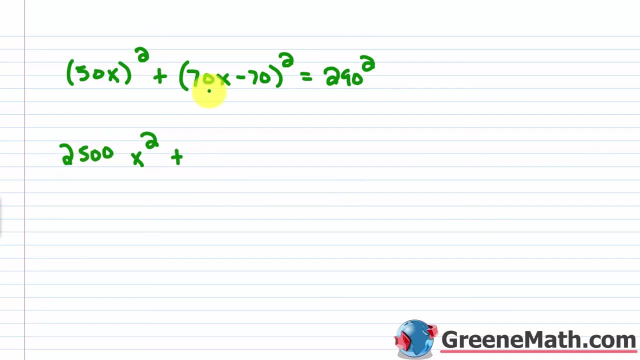 Now, don't make the mistake of doing this. A lot of students- again I've said this throughout the course- they do what they say. this is 70X squared minus 70 squared. Okay, that is wrong. This is wrong. Don't do that. Remember, if you have something in here with addition or subtraction, you've got to expand it. Okay, remember our special products formula. you can use that here to do this pretty quickly. You're going to square the first guy, which is 70X. that whole thing squared right. So the whole thing is squared. So it's 70 squared. 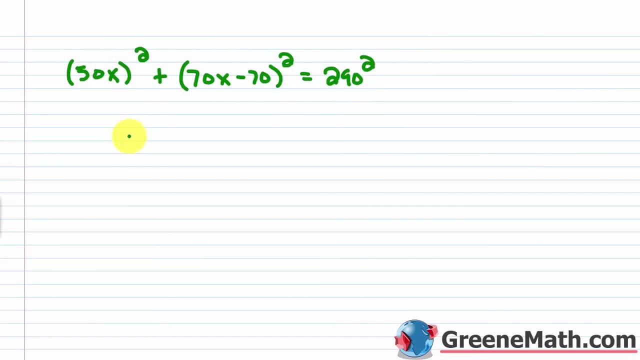 paste this in here and let's get started. all right, so for 50x we're going to put a little s, so 50x squared. if we wanted to simplify that, i would need to square 50 and also x, so that would give me 50 squared times x squared. now, 50 squared is 2500, so let me just replace that and say it's. 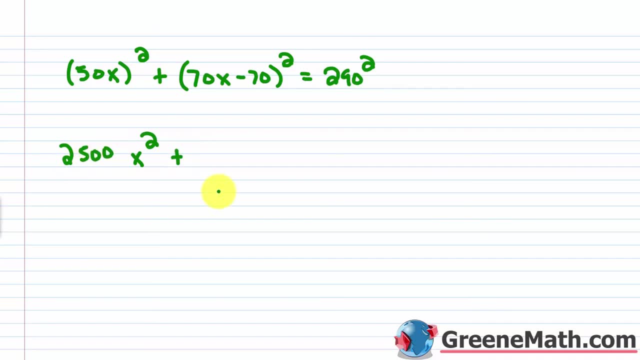 2500. okay, so then plus now, don't make the mistake of doing this. a lot of students again- i've said this throughout the course- they do what they say: this is 70x squared minus 70 squared. okay, that is wrong, this is wrong. don't do that. remember, if you have something in here. 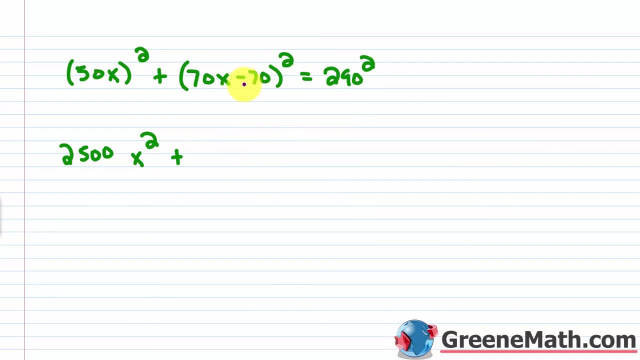 with addition or subtraction, you've got to expand it. okay, remember our special products formula. you can use that here to do this pretty quickly. you're going to square the first guy, which is 70x. that whole thing squared right, so the whole thing is squared. so it's 70 squared, which is 4900. 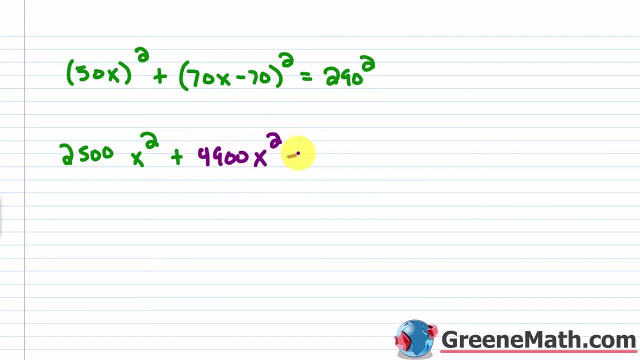 times x squared. okay, then you're going to have minus. you're going to have two times: this guy times this guy. so it's two times 70x times 70. okay, we'll just go ahead and crank that out real quick. two times 70 is 140. then times 70, again would be 9800. so basically, what you'd have is: 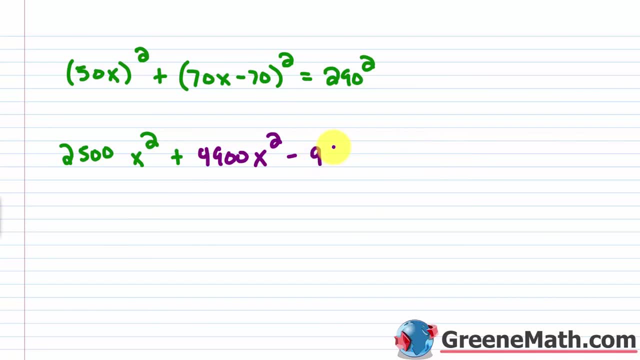 minus 9800x here. so minus 9800x, you could say 9800x, whatever you want to say. and then, lastly, you need to take this 70, the last term there, and square it. so we're going to go plus 70, squared. 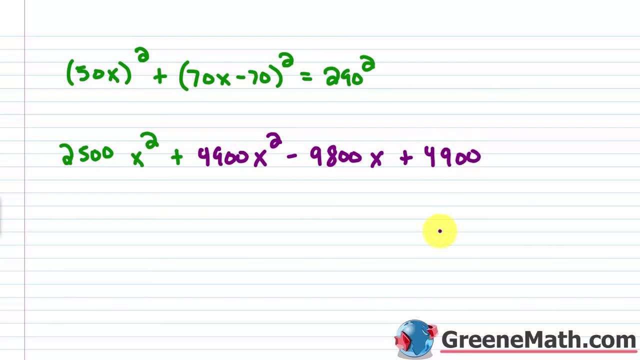 we already know is 4900, so this is 4900. okay, so that's this side right here. and this equals 290. squared is 84000, 100. let me slide this down so i can fit this all in one one line. so 84100, okay, so we have kind of. 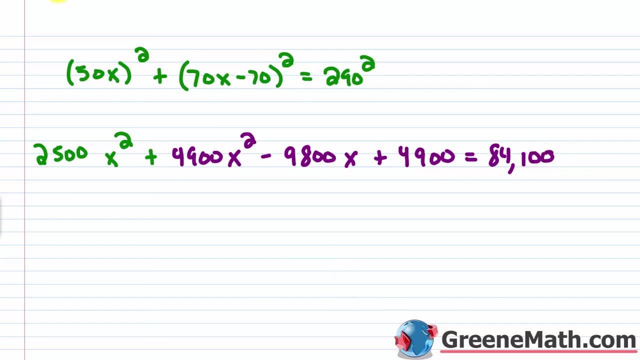 some big numbers involved here. so let's do some simplifying and then i'll show you what we can do to kind of make this as easy as possible. all right, so 2500x squared plus 4900x squared- those are like terms, so we can combine them. so if i had 2500 and 4900, i get 7400, so this is 7400x squared. 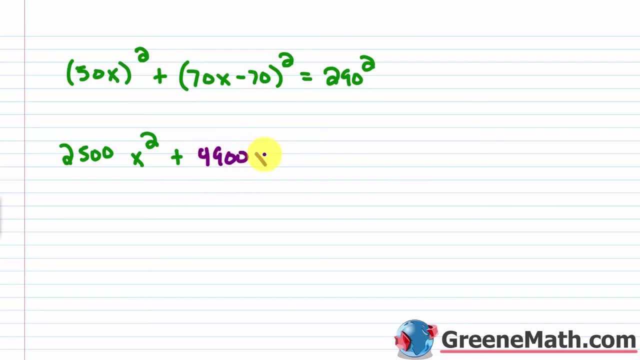 So it's 70 squared, which is 4900 times X squared. Okay, then you're going to have minus. you're going to have two times this guy times this guy. So it's two times 70X times 70. Okay, we'll just go ahead and crank that out real quick. Two times 70 is 140. Then times 70, again would be 9800. So basically, what you'd have is minus 9800 X here. So minus 9800 X. you could say 9800 X, whatever you want to say. And then, lastly, 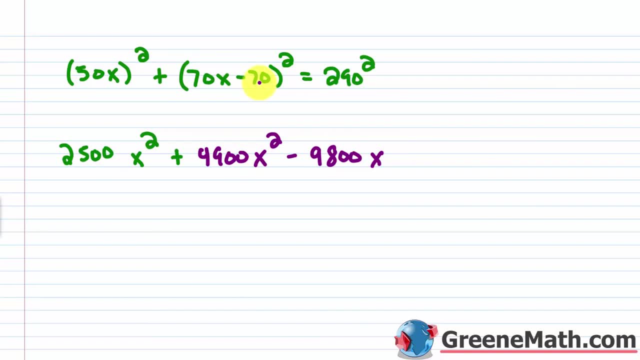 you need to take this 70, the last term there- and square it. So we're going to go plus 70. squared, we already know, is 4900.. So this is 4900.. Okay, so that's this side right here, And this equals: 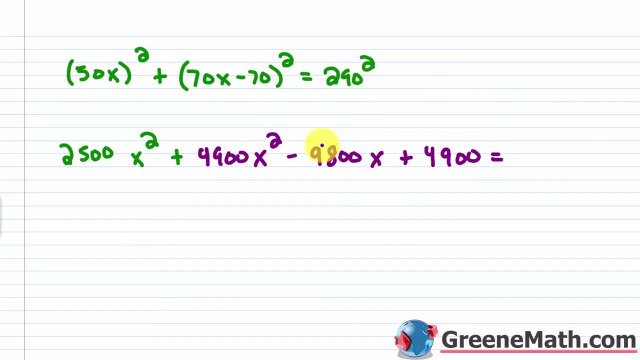 290 squared is 84,100.. Let me slide this down so I can fit this all in one line. So 84,100.. Okay, so we have kind of some big numbers involved here, So let's do some simplifying And then 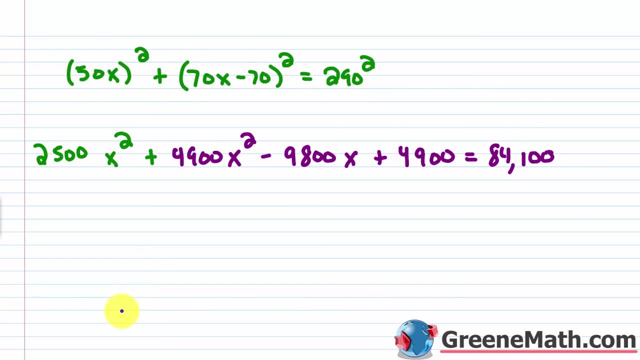 I'll show you what we can do to kind of make this as easy as possible. All right, so 2500 X squared plus 4900 X squared- those are like terms so we can combine them. So if I had 2500 and 4900, I get 7400.. So this is 7400 X squared, then minus 9800 X. I can't do. 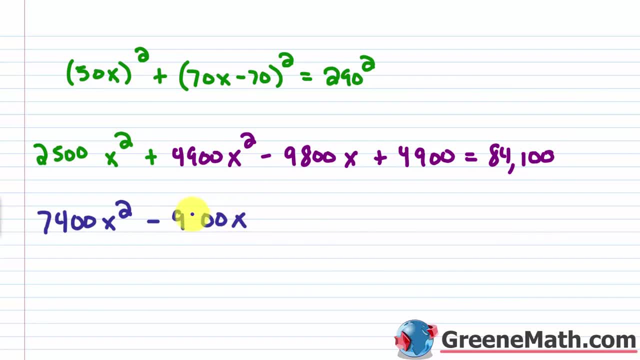 anything with that as of yet, So we'll just leave that as it is. And then what I can do over here, I'm going to subtract 84,100 away from each side of the equation, Okay, and what that's going to do is that's going to give me zero over here on the right side. 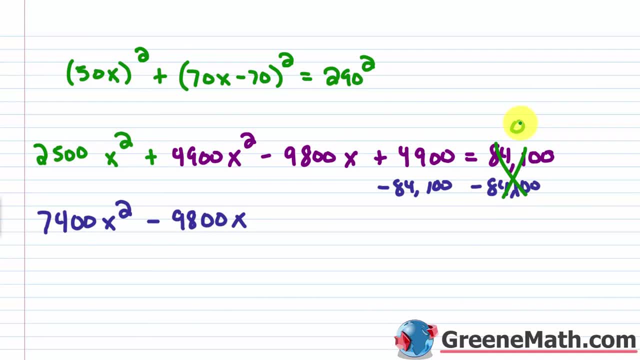 okay, because I'm solving a quadratic and I want it in the format of ax squared plus bx plus c equals zero, So I can use my quadratic form. Okay, so 4900 minus 84,100 is going to give me minus or negative 79,200.. Again, this equals zero. Now, if you want to plug these into the quadratic, 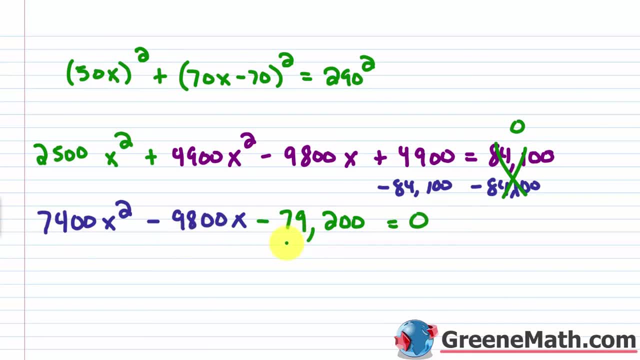 formula as they are. you can. You can plug them into the quadratic formula as they are. You can plug them into the quadratic formula as they are. You can plug them into the quadratic formula as they are. Most of you- I know pretty much all of you- are going to be using a calculator. I'm using a. 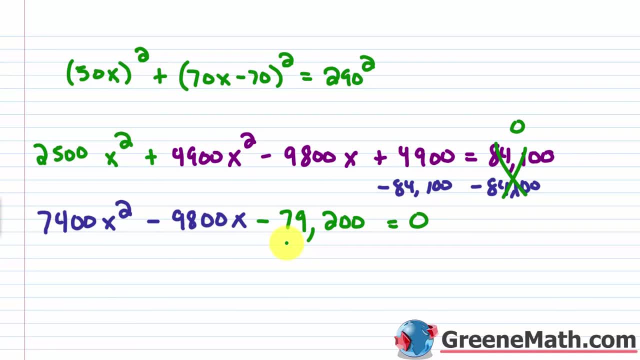 calculator. If you're working with bigger numbers or smaller numbers with calculator, it doesn't matter right, It does the calculation for you. But just to make this a little easier, a little simpler. So what we'll notice here is that each of these numbers ends with two zeros. This guy over. 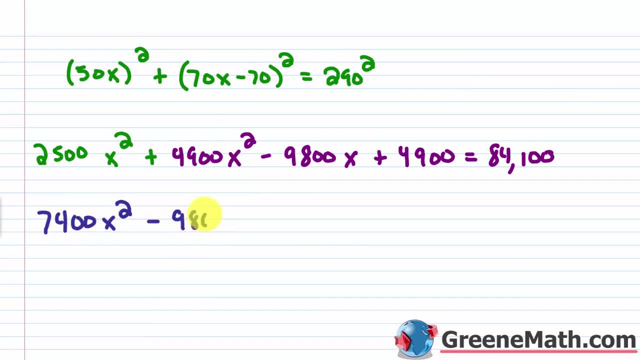 then minus 9800x. i can't do that, so i'm going to go minus 9800x squared, and then i'm going to continue to do that until i hear the maximum. so here it is about this much power. so what i'm going to do again is divide my cuadרת by the Material Factor. i'm going to 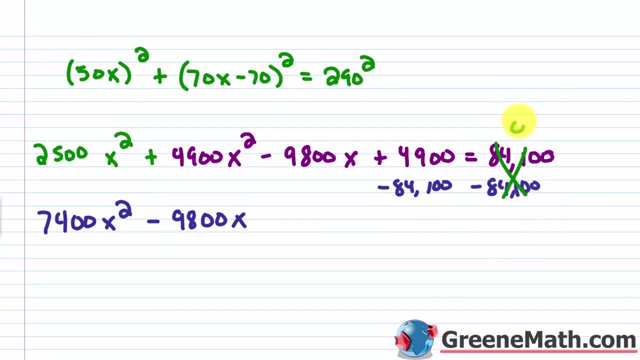 subtract 84100 from my expert type. i'm going to do this with the Yazda and this is so that if i analyze, and all i see here for my distribution, which is the model as you can see here, is that i have 4100, which is a negative because 1 raise half has to be. 10. they automatically fazla is going to be zero. so 44000 is going to give me this吉ar minus 4200 of value. all right, so this is going to give me 10 to the power from f4 there gonna be up at. 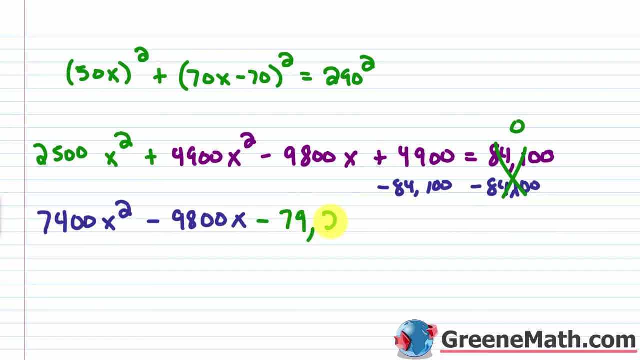 me minus or negative 79,200.. Again, this equals zero. Now, if you want to plug these into the quadratic formula as they are, you can. Most of you- I know pretty much all of you- are going to be using a calculator. I'm using a calculator If you're working with bigger numbers or smaller. 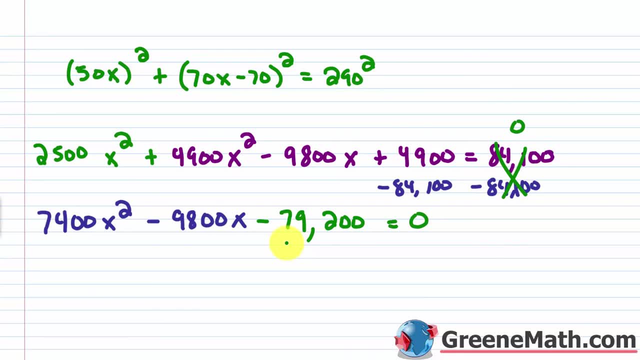 numbers with calculator. it doesn't really matter, right? It does the calculation for you. But just to make this a little easier, a little simpler. So what we'll notice here is that each of these numbers ends with two zeros. This guy over here is a zero, so it's not going to matter. 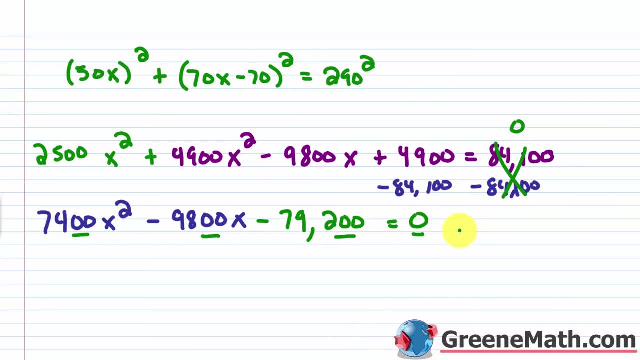 But if they all ended two zeros, they're divisible by 100,, right? So if I divided every part of this equation by 100, on the right, zero divided by 100 is still zero. So that's fine. Basically, I would just knock two zeros off from everything, right? So that makes it a lot simpler, right You? 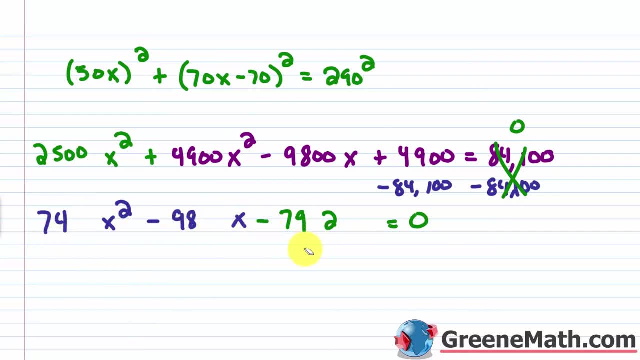 have 74x squared minus 98x minus, and this comma would disappear. You'd have 792, and this equals zero. okay, Perfectly mathematically legal to do that, And you would notice that you could also still divide each part by two. So if you wanted to make it even, 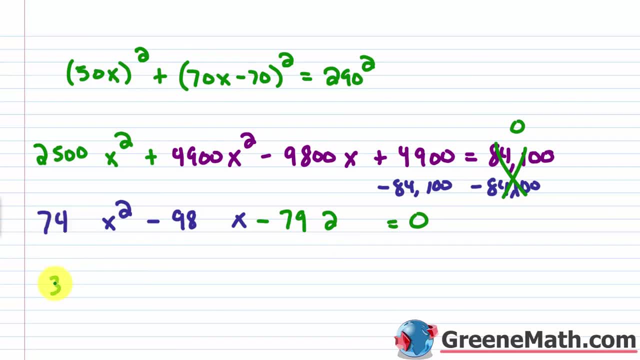 simpler. you could say that 74 divided by two is 37.. So 37x squared, and then 98 divided by two is 49. So minus 49x and then minus. if you take 792 and divide by two, you would get 396.. 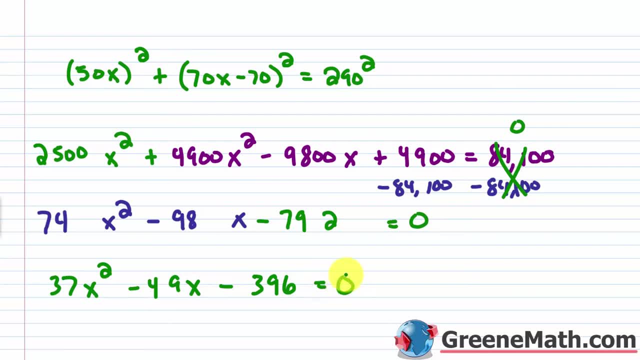 And we can say this is equal to zero. okay, So this is a lot simpler, a lot easier to work with. So let's kind of drag this up here and see what we got now. So we're going to use our quadratic formula. So, again, this is a lot simpler, a lot easier to work with, So we're going to use our. 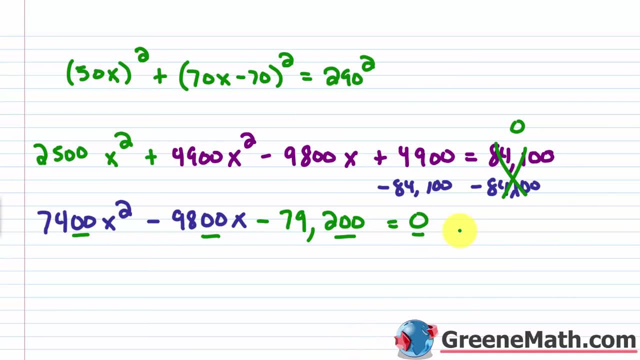 here is a zero, so it's not going to matter. But if they all ended two zeros, they're divisible by 100, right? So if I divided every part of this equation by 100, on the right, zero divided by 100 is still zero. So that's fine, Basically, I would just not divide by 100, but I would divide by. 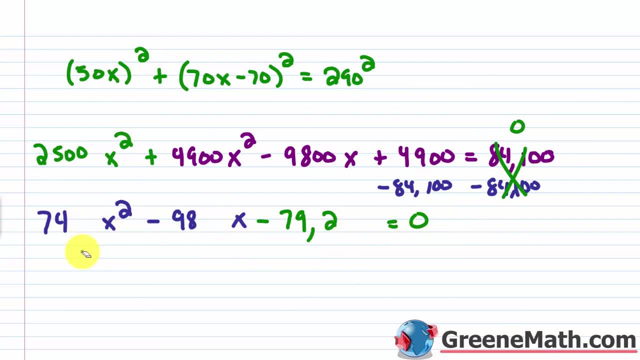 100,. right, So that makes it a lot simpler. right, You have 74x squared minus 98x minus, and this comma would disappear. You'd have 792, and this equals zero. okay, Perfectly, mathematically legal to do that, And you would notice that you could also still divide each. 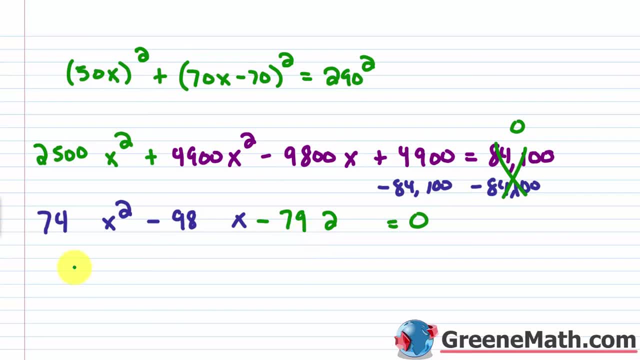 part by two. So if you wanted to make it even simpler, you could say that 74 divided by two is 37. So 37x squared, and then 98 divided by two is 49. So minus 49x and then minus. 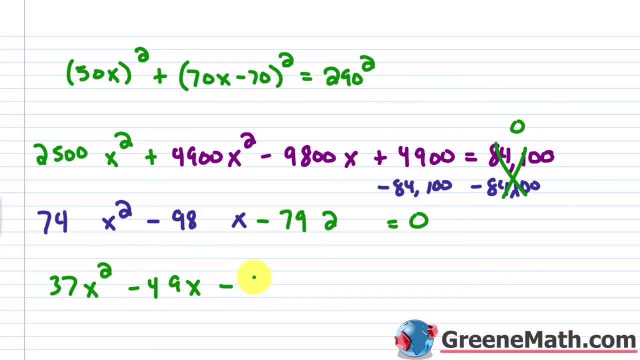 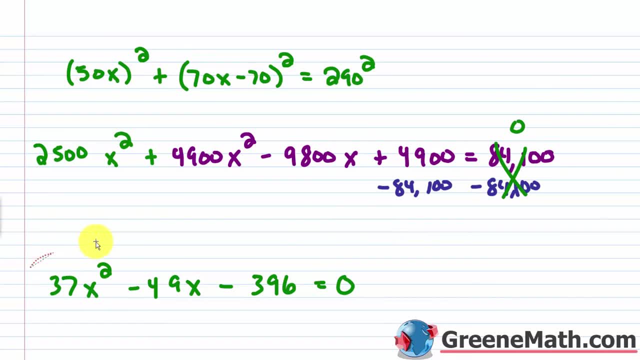 this is a lot simpler, a lot easier to work with. So let's kind of drag this up here and see what we got now. So we're going to use our quadratic formula. So, again, this is going to be A, this is going to be B. okay, It's the whole negative 49. And this is going to be C again. 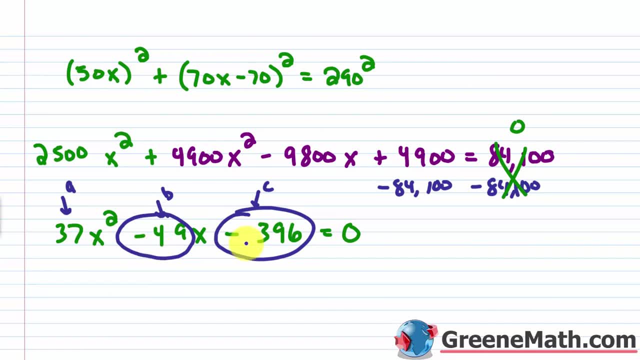 the negative: 396,. okay, And I circled the negative ones because sometimes you get confused and you try to just do it the other way around. So I'm going to do it the other way around. So I'm going to just take the number part without the sign When it's positive. obviously it doesn't matter. 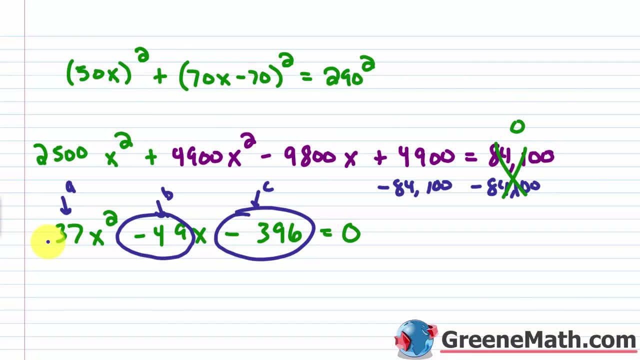 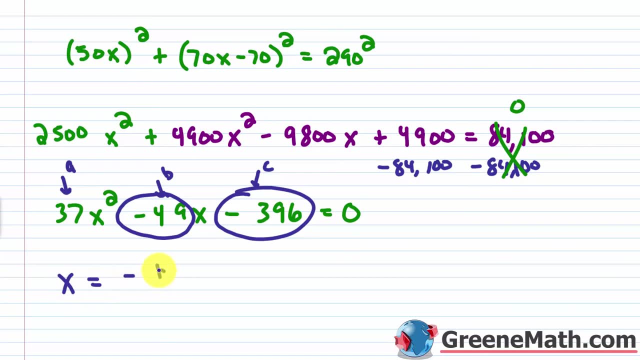 right, You're not bringing a sign with you, It's just positive. so it doesn't have a sign in front of it. All right, So with the quadratic formula, again in case you have forgotten it, x is going to be equal to the negative of B, plus or minus the square root of. you've got B squared. 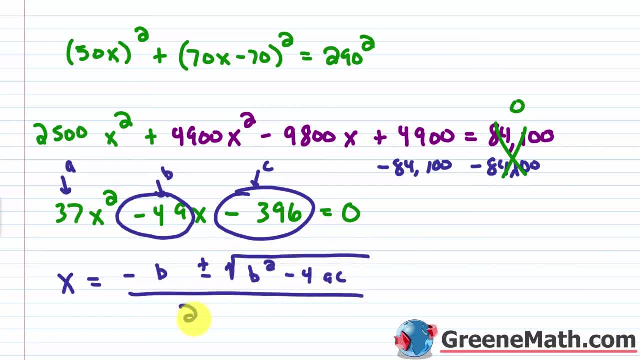 minus four times A, times C, This whole thing is over 2A. So all I'm going to do is just plug in: okay, Very, very easy. So for negative B again, B is negative 49.. The negative of: 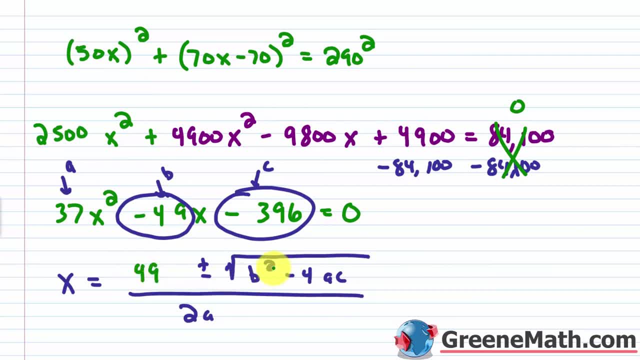 negative 49 is 49.. Plus or minus you've got B squared, so you'd have negative 49 squared. So let's just go ahead and do that real quick. If I square negative 49, I get 2,401.. So let me. 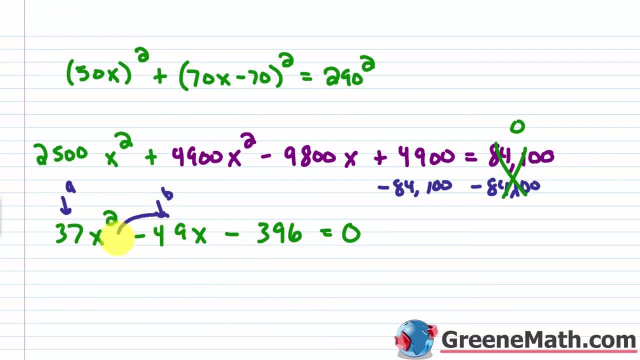 quadratic formula. So, again, this is going to be a, this is going to be b- okay, It's the whole negative 49, and this is going to be c. again the negative 396,. okay, And I circled the negative. 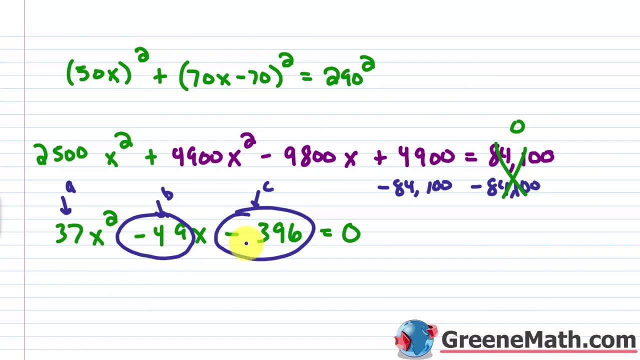 ones, because sometimes you get confused and you try to just take the number part without the sign. When it's positive, obviously it doesn't matter, right? You're not bringing a sign with you, It's just positive, so it doesn't have a sign in front of it. All right, So with the quadratic formula, 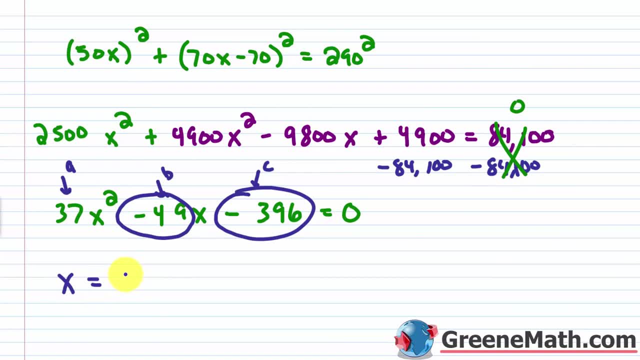 again in case you have forgotten it: x is going to be equal to the negative of b, plus or minus the square root of b. So we're going to use our quadratic formula and we're going to use our square root of. you've got b squared minus 4 times a times c. This whole thing is over 2a. 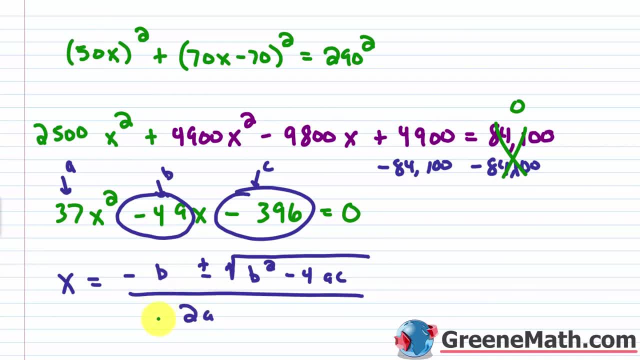 So all I'm going to do is just plug in: okay, Very, very easy. So for negative b again, b is negative 49. The negative of negative 49 is 49.. Plus or minus, you've got b squared. 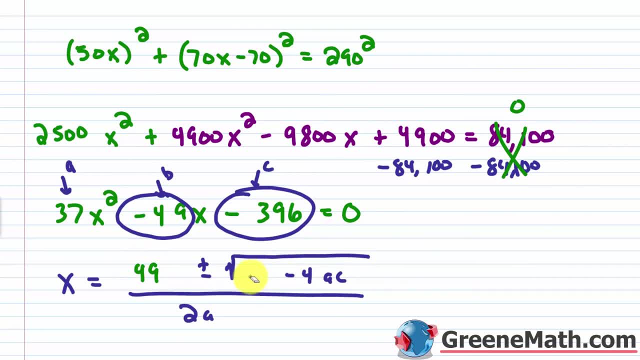 so you'd have negative 49 squared. So let's just go ahead and do that real quick. If I square negative 49, I get 2,401.. So let me write that in 2,401.. That's kind of hard to fit in there. 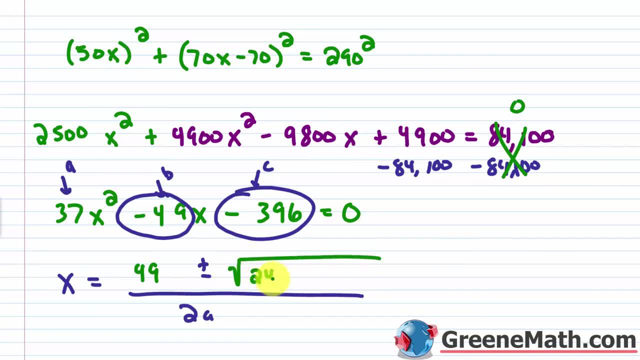 so let me redo this. So square root of 2,401, again minus 4 times for a, I have 37.. And then for c, I have my negative 396.. And we can crank this out now or come back in a minute. Let's just come back in a minute For a. 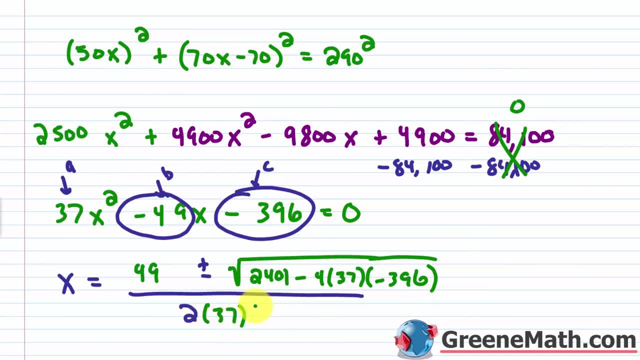 we have what We have: 37, so let's plug that in there. All right, let's do our calculation. So negative 4 times 37 is negative 148.. Then, times negative 396 is going to give me 58,608.. 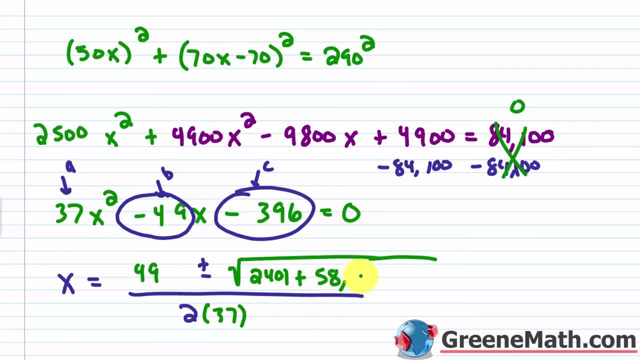 So let's just put plus 58,000. Again 608.. If we sum 2,401 and 58,608, we get 61,000, non. Okay, so let's write that there. So 61,000, non. Then down here 2 times 37,- we know from earlier- is 74.. Okay, All right. So what is? 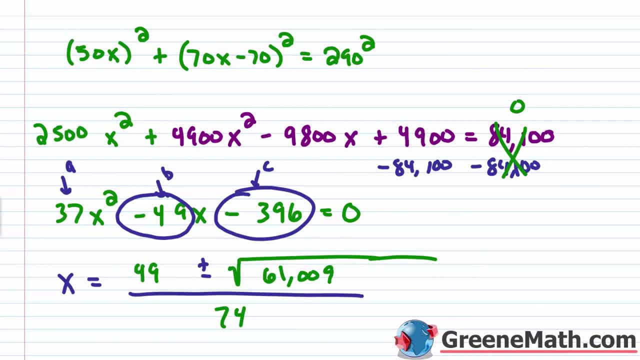 the square root of 61,009?? Well, if you punch that up on a calculator, you get 247.. So let's erase this and put 247.. Now we have two cases here, but you're going to see that we're going to. 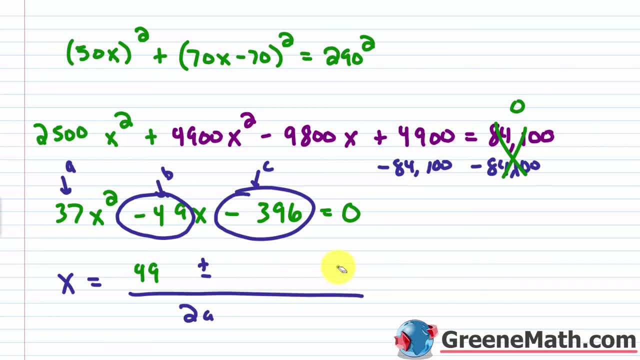 write that in 2,401.. That's kind of hard to fit in there, So let me redo this So: square root of 2,401, again minus four times, For A, I have 37.. And then for C, I have my negative 396.. 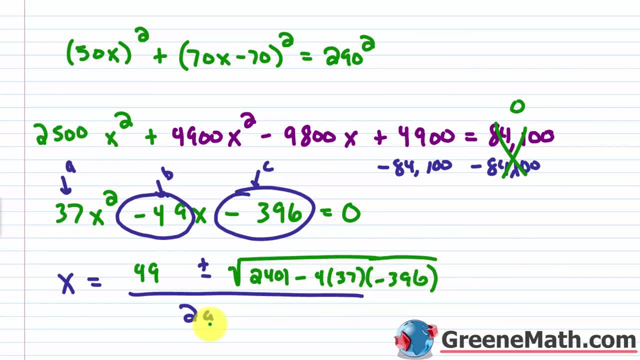 And we can crank this out now or come back in a minute. Let's just come back in a minute. For A, we have what We have: 37.. So let's plug that in there. All right, let's do our calculation. So: negative four times 37 is negative 148.. Then times negative. 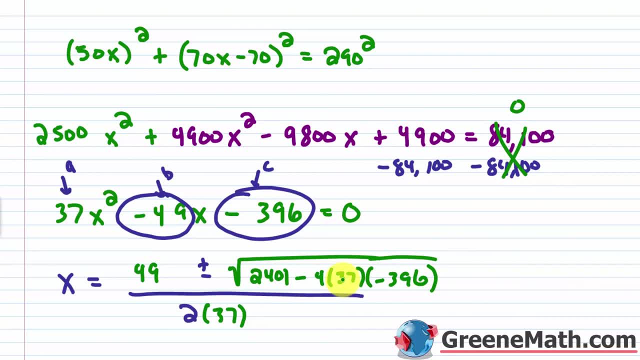 396 is going to give me 58,608.. So let's just put plus 58,000. Again 608.. If we sum 2,401 and 58,608, we get 61,000 non. Okay, So let's write that there. So 61,000 non. 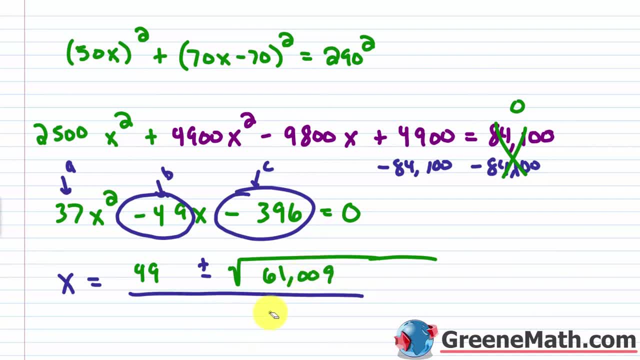 Then down here 2 times 37,- we know from earlier- is 74.. Okay, All right. So what is the square root of 61,009?? Well, if you point that up on a calculator, you get 247.. So let's erase this. 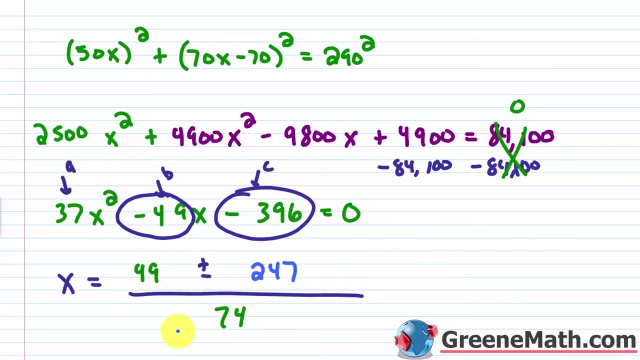 and put 247.. Now we have two cases here, but you're going to see that one of the cases ends up being nonsense, right? Remember, we're solving for x, which is the amount of time that, in this particular case, Larry's going to travel for or drive for before the 24,000.. So that's. 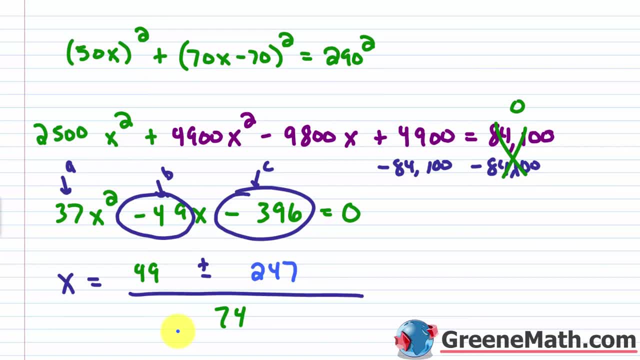 going to be the number of cars that he's going to drive. So that's going to be the number of cars that he's going to drive. So that's going to be the number of cars that he's going to drive. So you know that you can't have a negative amount of time. That wouldn't make sense in this scenario. 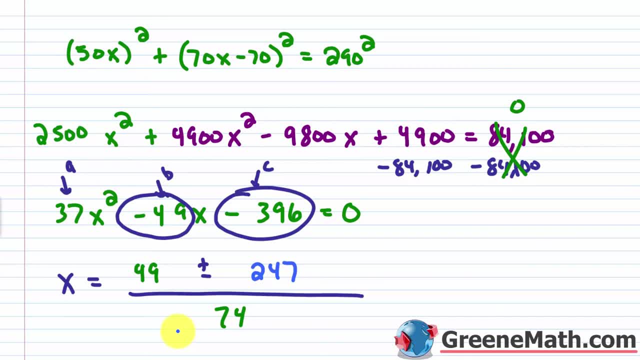 I can't say. well, he drove for negative 18 hours as an example. Okay, What does that mean? It doesn't mean anything, It's nonsense. So you have to throw it out. So the one of these guys that's going to. 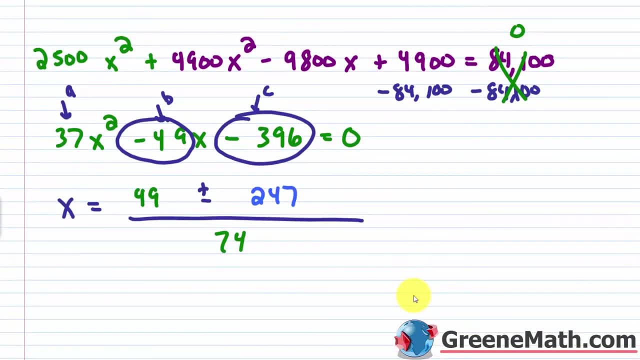 make it negative. we would just immediately exclude that. Okay, So the first scenario would be that x is equal to 49 plus 247 over 74. So we keep that one. The other one is going to be. the other scenario is what It's: x is equal to 49 minus 247 over 74. This is going to end up being 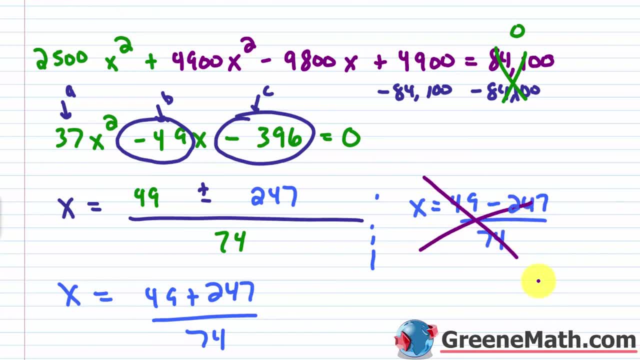 negative, So you can just throw this out. Okay, You don't need to worry about that solution at all. So, focusing on this one: 49 plus 247 is 296.. So if you had 296 over 74,, you would have four, Okay. 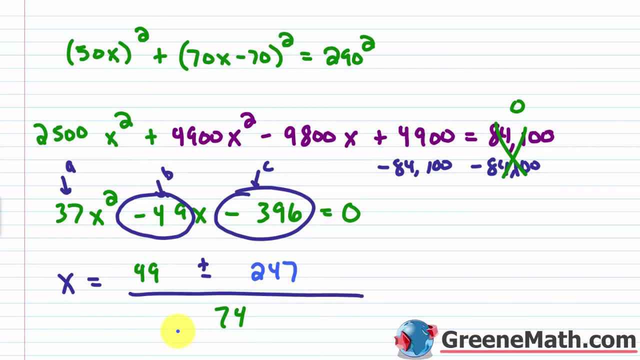 one of the cases ends up being nonsense, right? Remember, we're solving for x, which is the amount of time that, in this particular case, Larry's going to travel for or drive for before the two cars are 290 miles apart, So you know that you can't have a negative amount of time. That wouldn't. 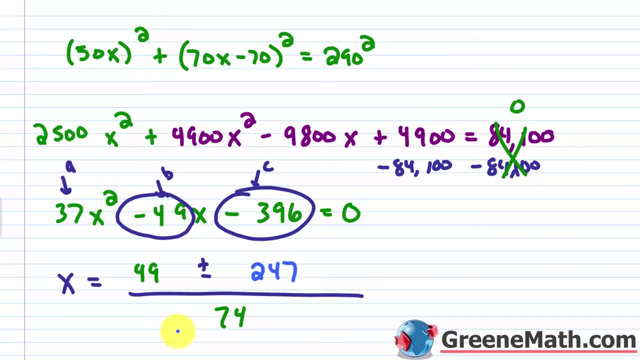 make sense in this scenario I can't say: well, he drove for negative 18 hours as an example. Okay, what does that mean? It doesn't mean, it's nonsense, You have to throw it out. So the one of 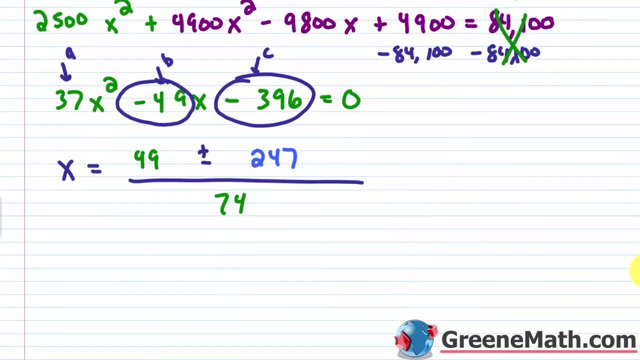 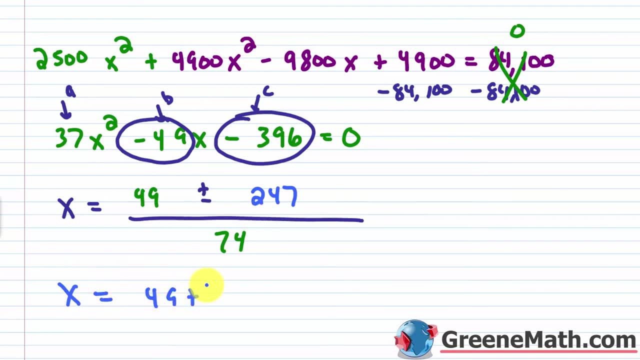 these guys. that's going to make it negative. we would just say: well, he drove for negative 18 hours. You can immediately exclude that, Okay? So the first scenario would be that x is equal to 49 plus 247 over 74. So we keep that one. The other scenario is what It's: x is equal to 49 minus. 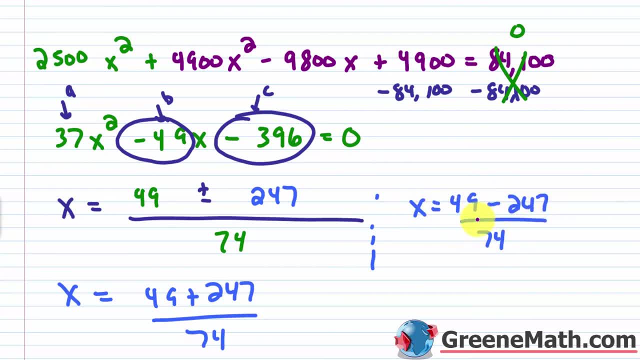 247 over 74.. This is going to end up being negative, So you can just throw this out. Okay, You don't need to worry about that solution at all. So focusing on this one: 49 plus 247 is 296.. 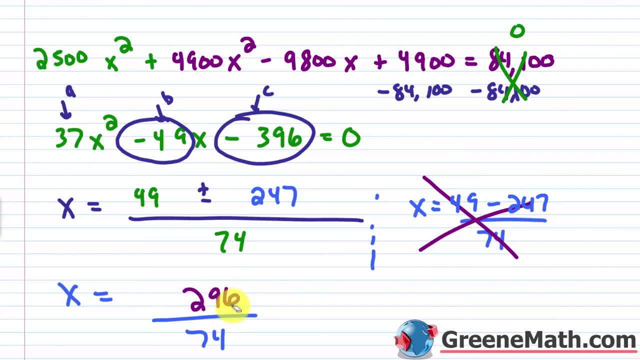 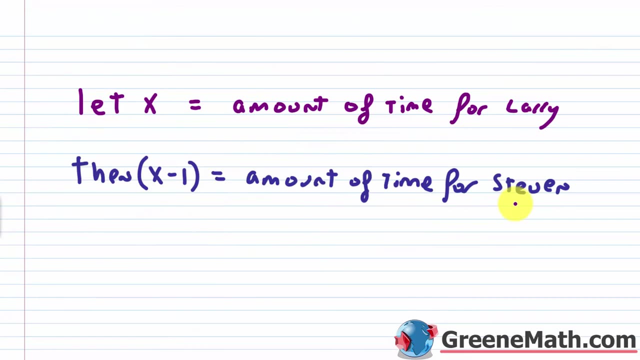 If you had 296 over 74, you would have four. Okay, So nice and simple. So x equals four. Again, that tells me that Larry drove for four hours before the two cars were 290 miles apart. Again, x was the amount of time for Larry, x minus one was the amount of time for Steven. So this guy is 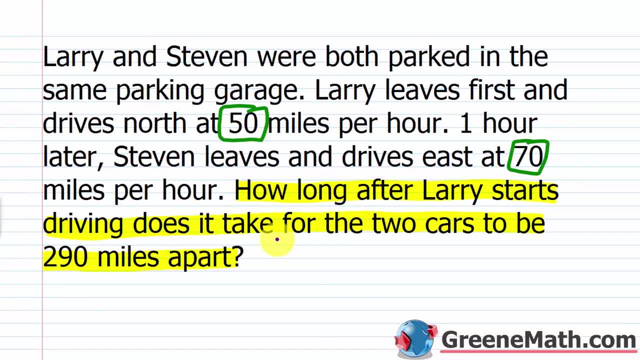 four and this guy is three right, Because four minus one is three. So again to officially answer this: how long after Larry starts driving does it take for the two cars to be 290 miles apart? We'll say Larry drives for four hours before the two cars. 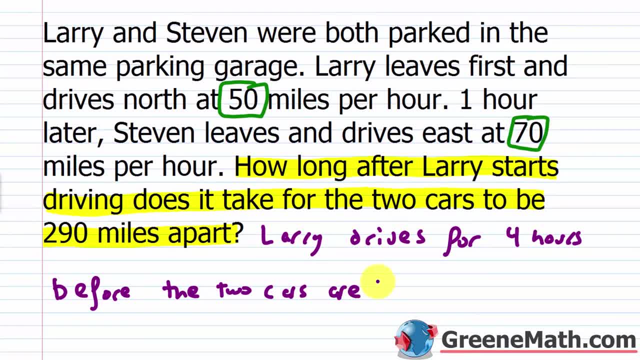 are 290 miles apart. Okay, And if you want to check this again, it's easy to go to the diagram and kind of visually see what's going on. You want to mark down some information: that Larry's going at 50 miles per hour and Steven's going at 70 miles per hour. So let's go to the diagram. 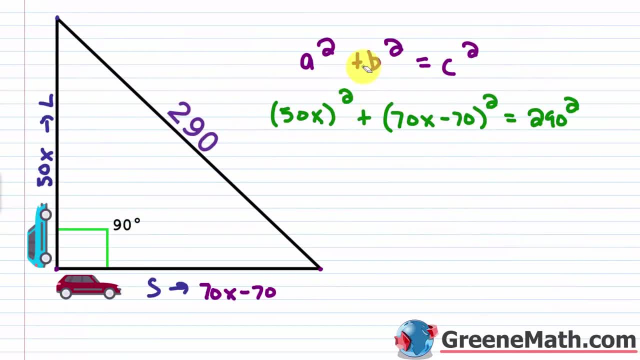 and let's go to the little drawing we have And let's see if we can make sense of this. We can erase all this. We can actually leave the a squared plus b squared equals c squared. We'll actually use that. So if I plug in a four for x, I'd have 200.. So that's for Larry. We know that. 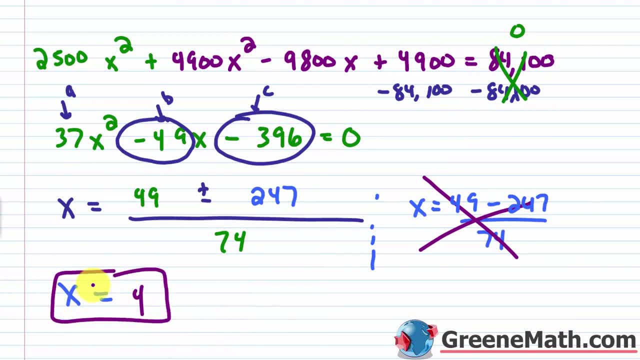 So nice and simple. So x equals four. Again, that tells me that Larry drove for four hours before the two cars were 247.. So that's going to make sense in this scenario. So that's going to make sense in this scenario. So that's going to make sense in this scenario. So that's going to make sense. 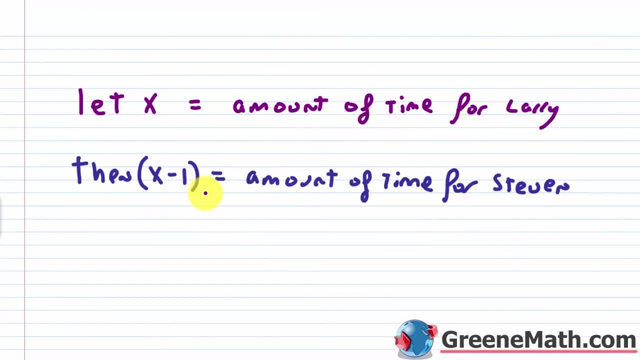 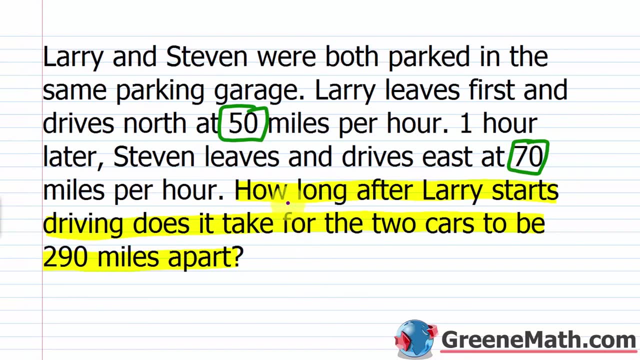 apart Again, x was the amount of time for Larry, x minus one was the amount of time for Stephen. So this guy is four and this guy is three, right, Because four minus one is three. So again now officially answer this: How long after Larry starts driving does it take for the two cars to 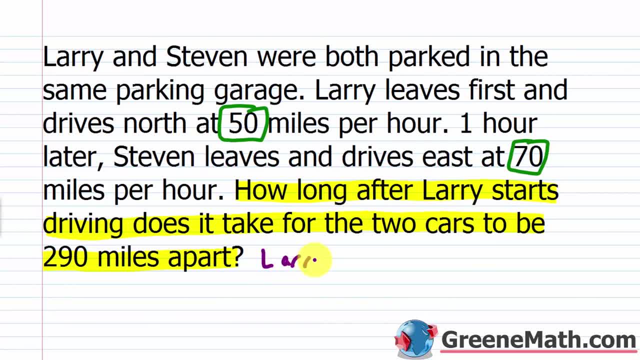 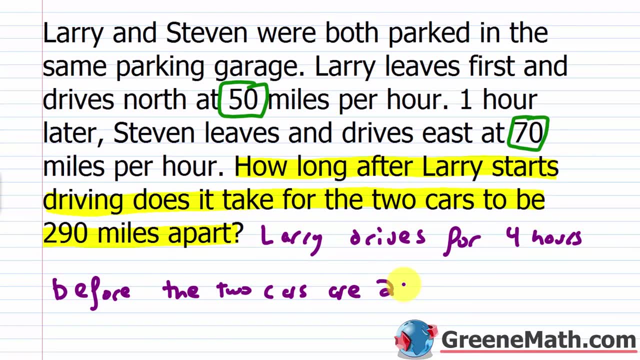 be 290 miles apart. We'll say Larry drives for four hours before. the two cars are 290 miles apart. Okay, And if you want to check this again, it's easy to go to the diagram and kind of visually see what's going on. You want to mark down some information that Larry's 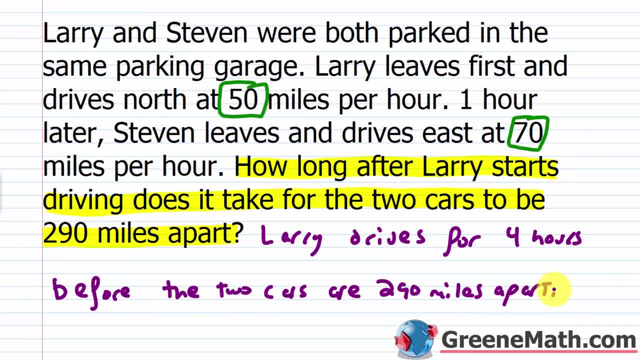 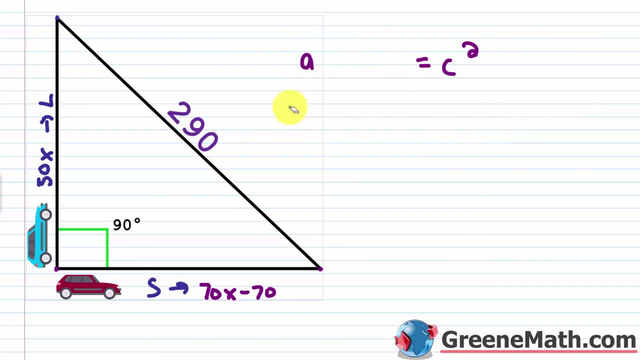 going at 50 miles per hour and Steven's going at 70 miles per hour. So let's go to the little drawing we have and let's see if we can make sense of this. We can erase all this. We can actually leave the a squared plus b squared equals c squared. We'll actually use that So. 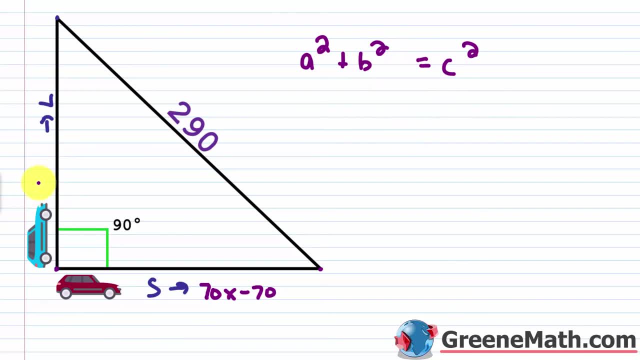 if I plug in a four for x, I'd have 200.. So that's for Larry. We know that he drives 200 miles from here to here And that's basically over the span of four hours, And that's how far he's going. 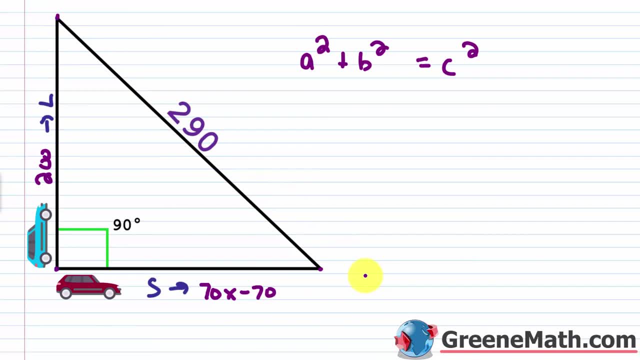 to have traveled when he gets to this point here, when they're 290 miles apart. And then for Steven you can plug in a four, which is what x is. You get 70 times four is 280.. 280 minus 70 is 210. 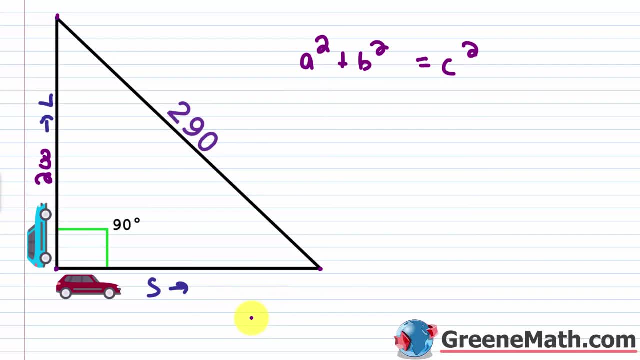 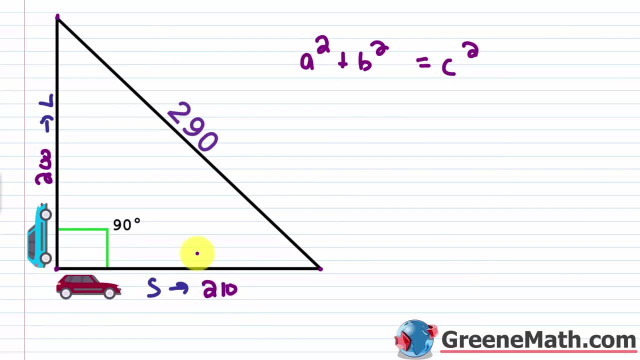 So either way, you get 210 as his distance from here to here. Okay, So again, we know about the right triangle: If this is 200 and this is 210, plugging in if one is 200 and the other is 210,. 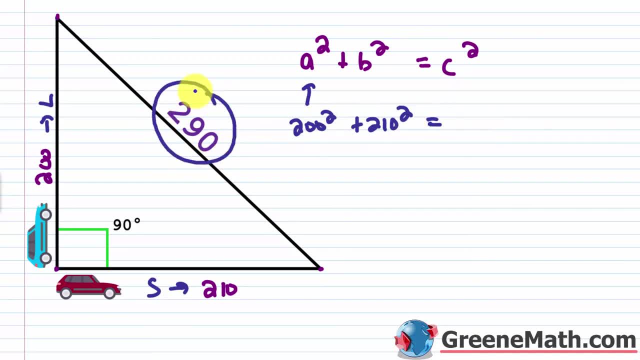 if we sum those two squares, it should be this guy right here squared. So is that true? 200 squared is what? Well, punch that up on a calculator, You're going to get 40,000.. Okay, 210 squared. punch that up on a calculator, You're going to get. 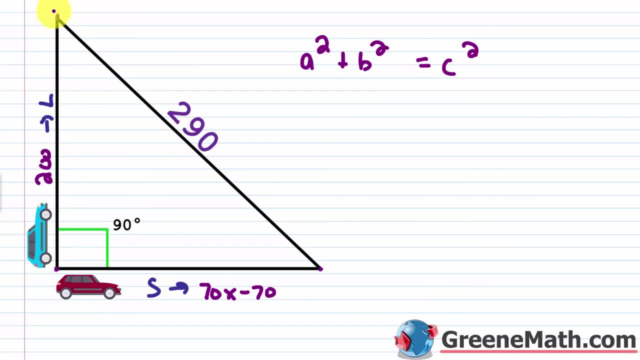 he drives 200 miles from here to here, And that's basically over the span of four hours, And that's how far he's going to have traveled when he gets to this point here, when they're 290 miles apart. And then, for Steven, you can plug in a four. 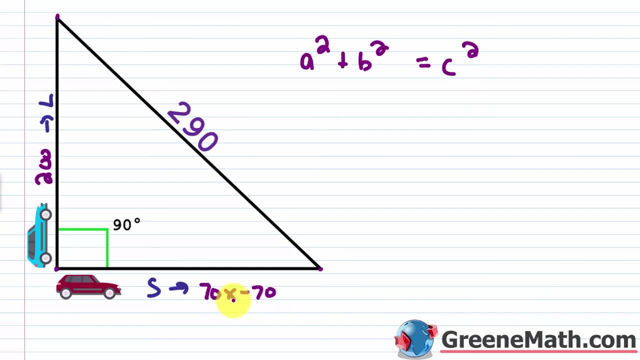 which is what x is You get. 70 times four is 280.. 280 minus 70 is 210.. Or you could again do it kind of manually and say, okay, well, he was going 70 miles per hour, He only drove for. 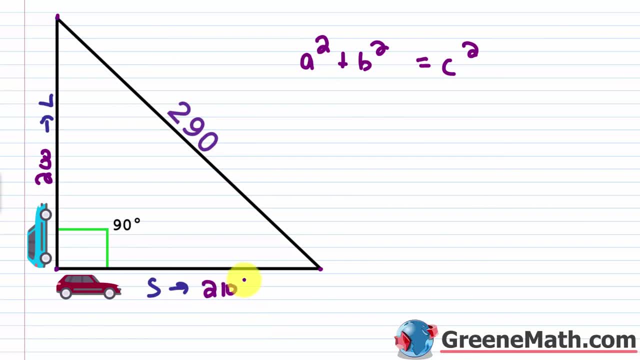 three hours. 70 times three is 210. So either way, you get 210 as his distance from here to here. Okay, So again we know about the right triangle: If this is 200 and this is 210, plugging in. 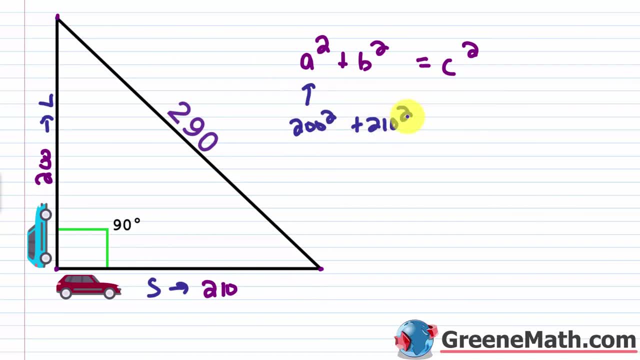 if one is 200 and the other is 210, if we sum those two squares, it should be this guy right here squared. So is that true? 200 squared is what? Well, punch that up on a calculator, you're going to get 40,000.. 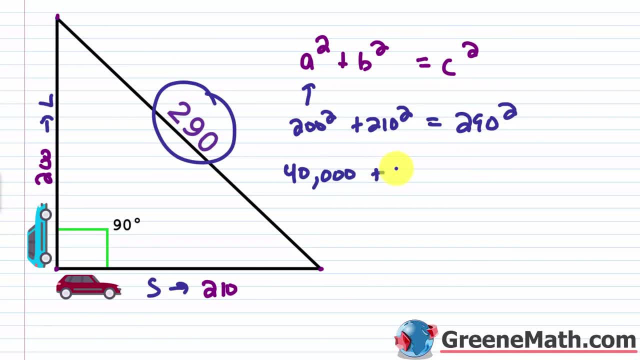 Okay, 210 squared. punch that up on a calculator. you're going to get 44,100.. And if you sum those two amounts together, you are going to get 290 squared, because that's going to be 84,100.. Okay. 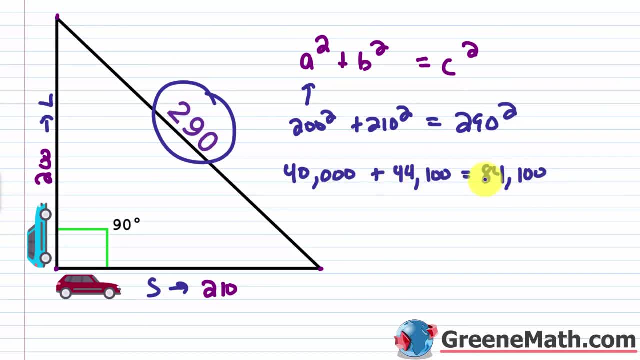 You can easily see that 40,000 plus 44,100 is 84,100.. So we can say here: our answer is correct. Larry drove for four hours, So that's why he's going to get 240 miles per hour. 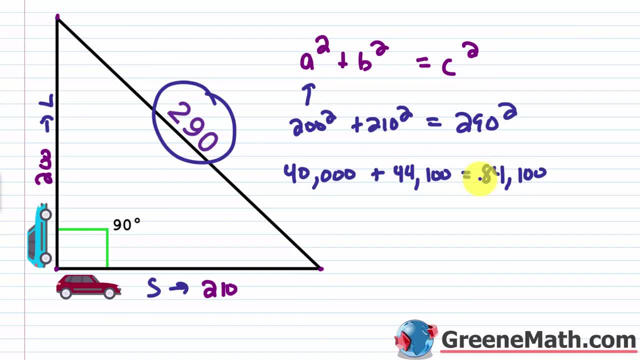 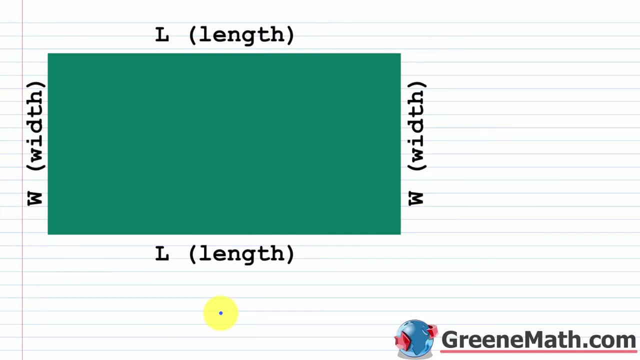 Before the two cars were 290 miles apart, All right. So another common type of problem in this section involves finding an unknown area. So, generally speaking, these problems are going to deal with some type of rectangular shape. This could be a pool, it could be a garden. 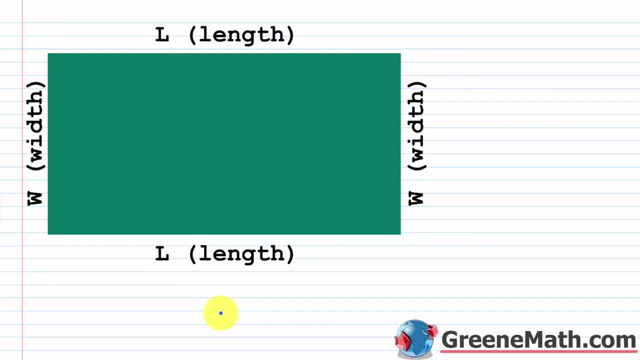 it could be a quilt. The example we're going to see next is going to be a rug, Okay, So something rectangular in nature. So what I want to cover really quickly is just the formula for the area of a rectangle. So we have a rectangle on our screen, We have our length, we have our 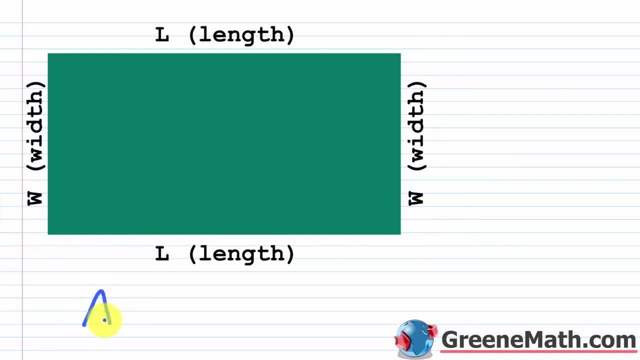 width and we have our width, Okay, So the area of a rectangle- we'll put A here- is equal to the length, which I'm going to put capital L times the width, which is capital W. Okay, So that's. 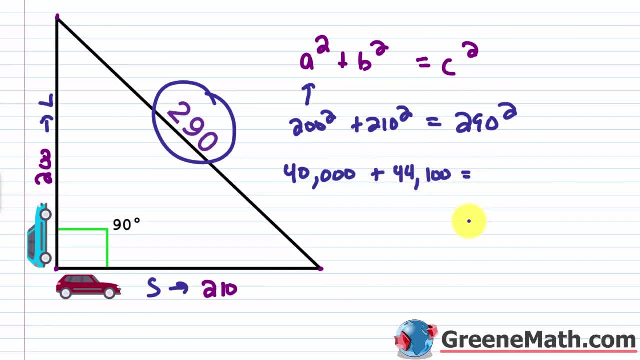 44,100.. And if you sum those two amounts together, you are going to get 290 squared, because that's going to be 84,100.. Okay, You can easily see that 40,000 plus 44,100 is 84,100.. 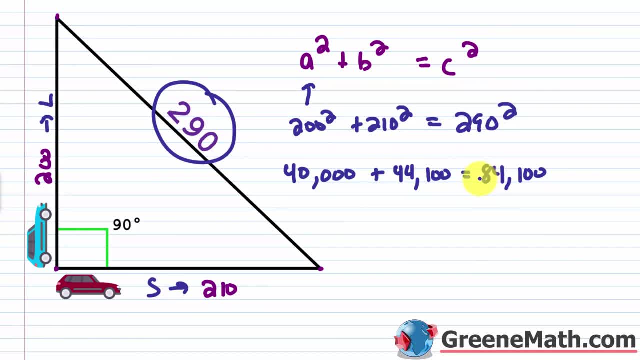 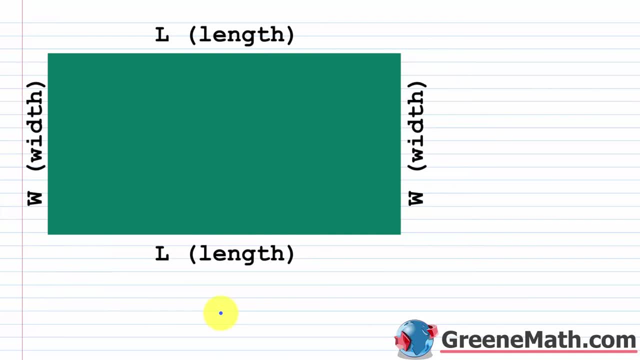 So we can say here: our answer is correct. Larry drove for four hours before. the two cars were 290 miles apart. All right, So another common type of problem in this section involves finding an unknown area. So, generally speaking, if you're driving a car, you're going to have to find an. 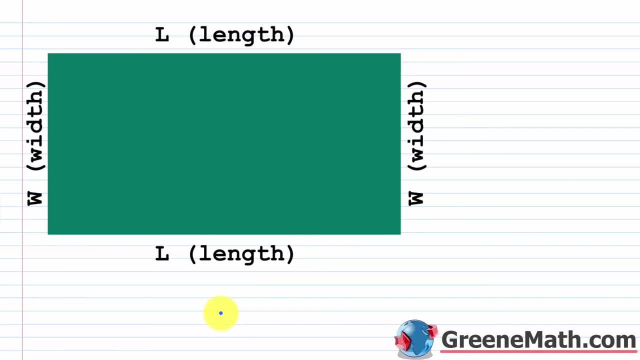 unknown area. Generally speaking, these problems are going to deal with some type of rectangular shape. This could be a pool, It could be a garden, It could be a quilt. The example we're going to see next is going to be a rug. Okay, So something rectangular in nature. So what I want to cover? 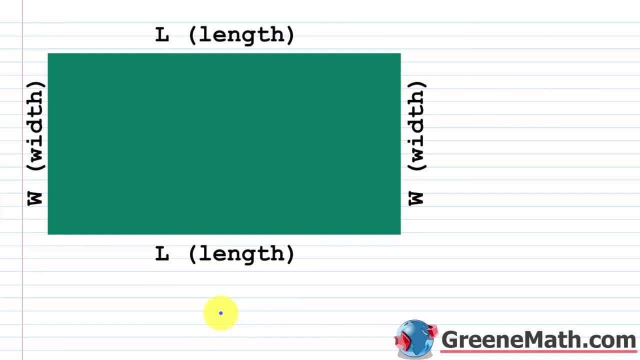 really quickly is just the formula for the area of a rectangle. So we have a rectangle on our screen, We have our length and we have our width. Okay, So the area of a rectangle- we'll put A here- is equal to the length, which I'm going to put capital L, times the width, which is capital W. 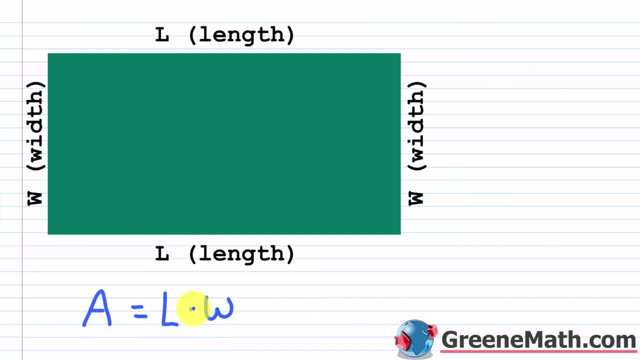 So that's the formula for the area of a rectangle. You might want to write that down because we're going to use it immediately in the next problem. So just as a quick example, suppose I said that the length here was eight inches And suppose I said the width here was six inches. Okay, And I 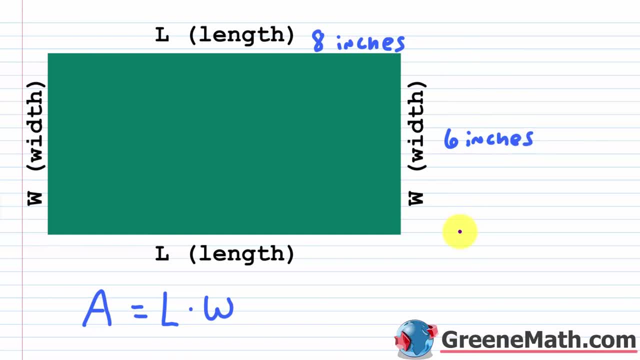 said: well, what's the area of this rectangle, given this information? Well, the area, I'll just put: capital A is equal to what It's eight times six, which is 48. You're just multiplying And then, inches times inches, you multiply your units. 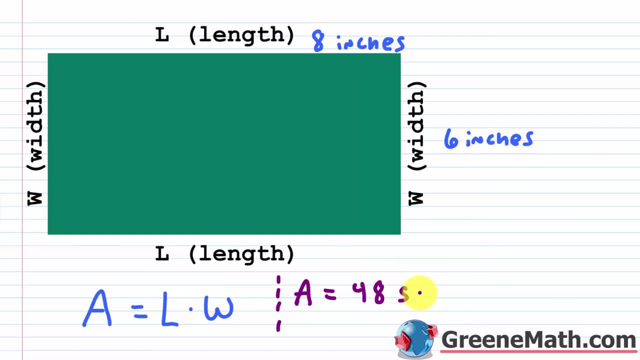 That's going to be inches squared, You could say square inches. So we're going to say this is 48 square inches. Okay, And let me make this Q a little bit better. Okay, So again, 48 square inches when we have a length of eight inches and a width of six inches, All right, So again, let's put this: 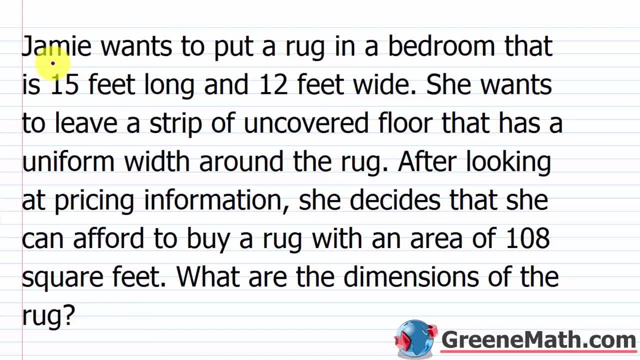 formula to immediate use. So we have here for our sample problem that Jamie wants to put a rug in a bedroom that is 15 feet long and 12 feet wide. She wants to leave a strip of uncovered floor that has a uniform width around the rug. After looking at pricing information she decides that she can. 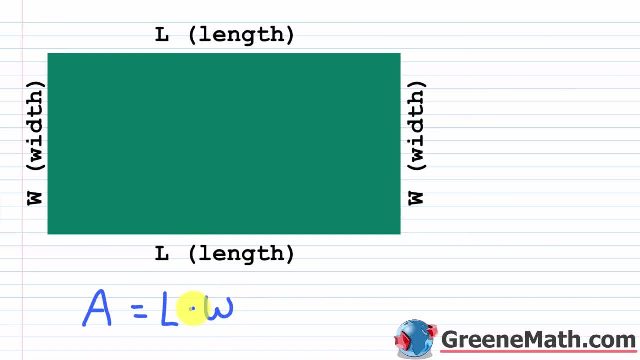 the formula for the area of a rectangle. Might want to write that down because we're going to use it immediately in the next problem. So just as a quick example, suppose I said that the length here was eight inches, And suppose I said the width here was six inches, Okay, And I said: 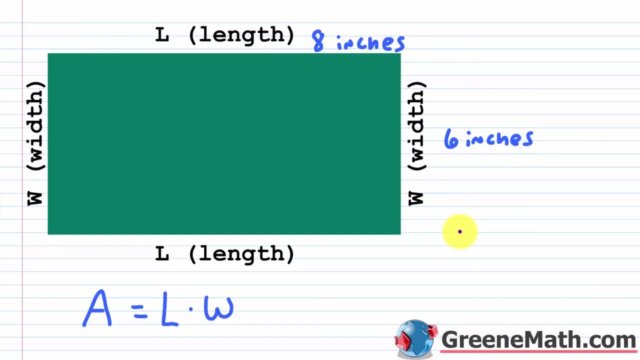 what's the area of this rectangle? Well, the area. I'll just put. capital A is equal to what It's eight times six, which is 48. You're just multiplying And then, inches times inches, you multiply your units. that's going to be: 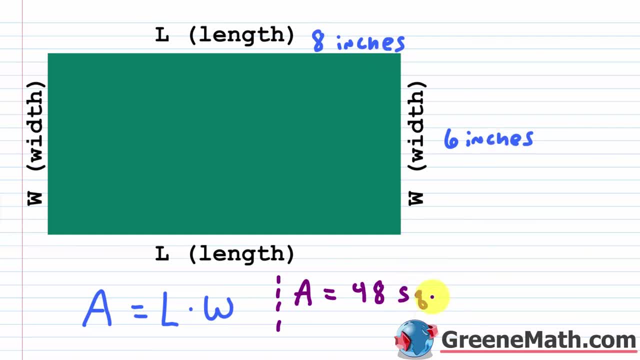 inches squared you could say square inches. So we're going to say this is 48 square inches. Okay, And let me make this Q a little bit better. Okay, So again, 48 square inches when we have a length of eight inches and a width of six inches. All right, So again, let's put this formula to. 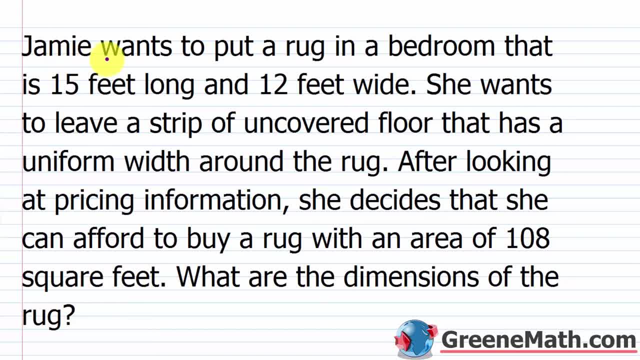 immediate use. So let's say we have a length of eight inches and a width of six inches. So we have here for our sample problem that Jamie wants to put a rug in a bedroom that is 15 feet long and 12 feet wide. She wants to leave a strip of uncovered floor that has a uniform width around. 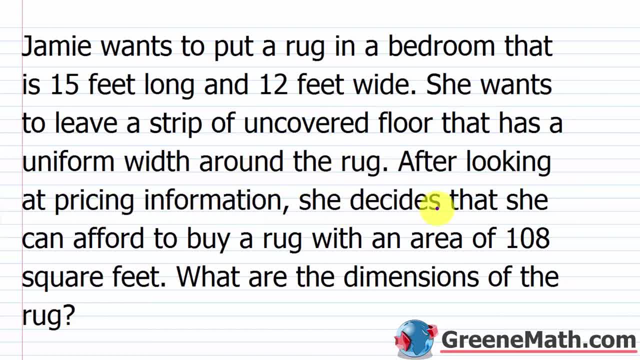 the rug. After looking at pricing information, she decides that she can afford to buy a rug with an area of 108 square feet. Okay, So what are the dimensions of the rug? So, again, what are we being asked to find? Well, given the fact that she can afford to buy a rug that has a length of six inches, 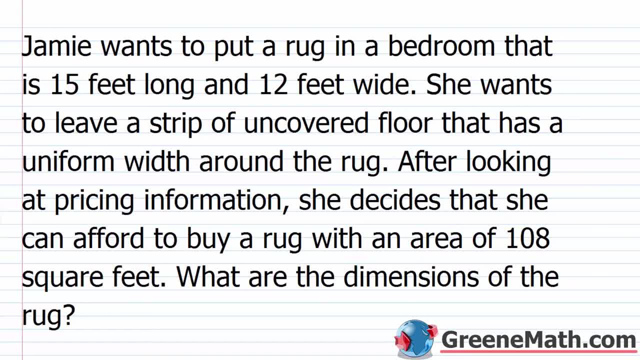 that has a maximum area of 108 square feet. we want to know what are the dimensions of the rug. Okay, Well, to solve this problem, if you haven't seen it before, it might be a little challenging for you to kind of set it up. Okay, So usually what you do with this is you draw a little diagram. 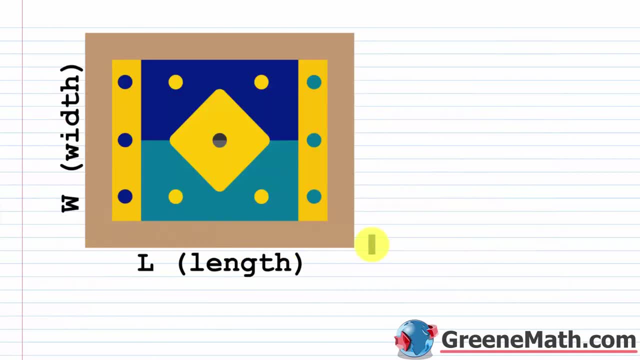 and I have that already set up, And what you'll see here is that the entire rectangle is meant to represent the bedroom, Okay, And then you have this kind of smaller rectangle which represents your rug, And then the brown. you see, that's a strip of uncovered floor, Okay, That's around the rug, Okay, And that's actually the. 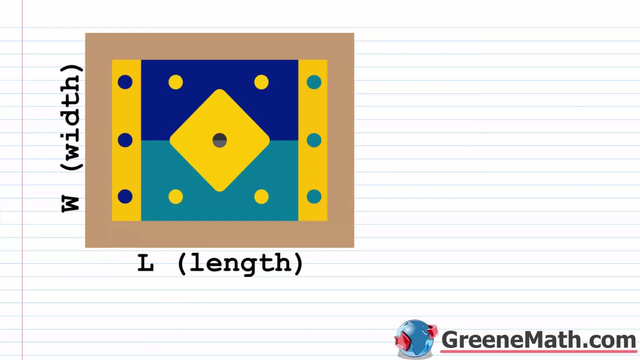 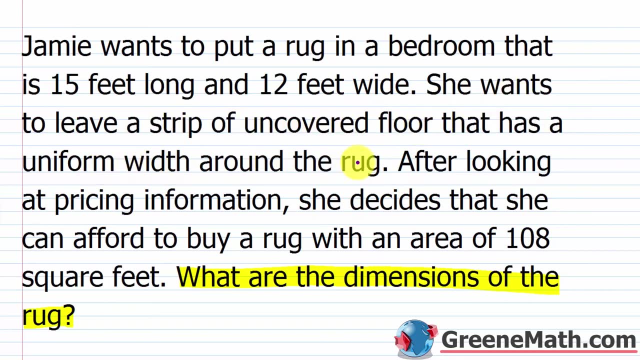 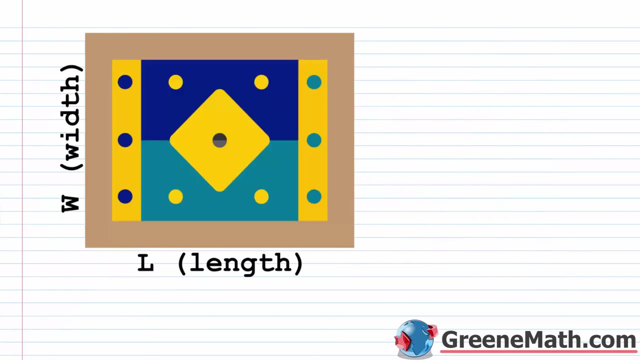 key to understanding this problem. So when we go back up- I just want to read this part one more time- She wants to leave a strip of uncovered floor that has a uniform width around the rug. This is very important. So this uniform width around the rug. Okay, Let me go back down and 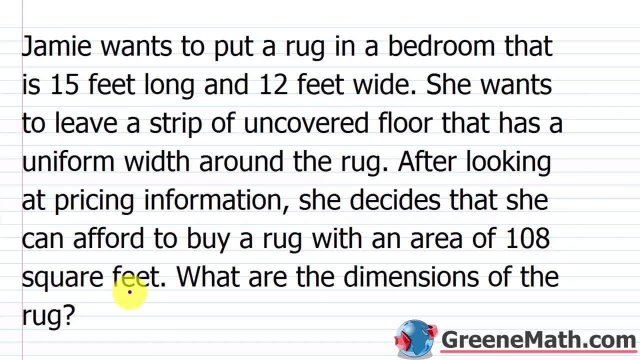 afford to buy a rug with an area of 108 square feet. Okay, So what are the dimensions of the rug? So, again, what are we being asked to find? Well, given the fact that she can afford to buy a rug that has a maximum area of 108 square feet, we want to know what are the dimensions of the rug. 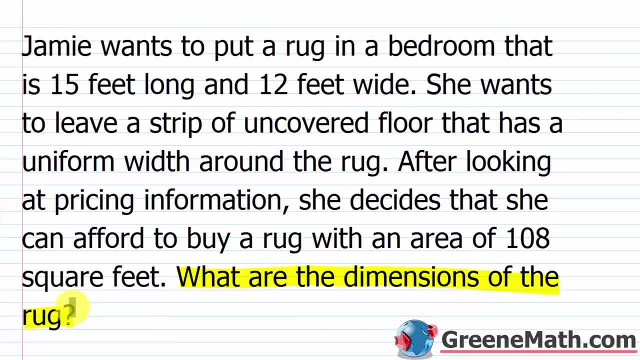 Okay, Well, to solve this problem. you haven't seen it before. It might be a little challenging for you to kind of set it up, Okay, So usually what you do with this is you draw a little diagram and I have that already set up. 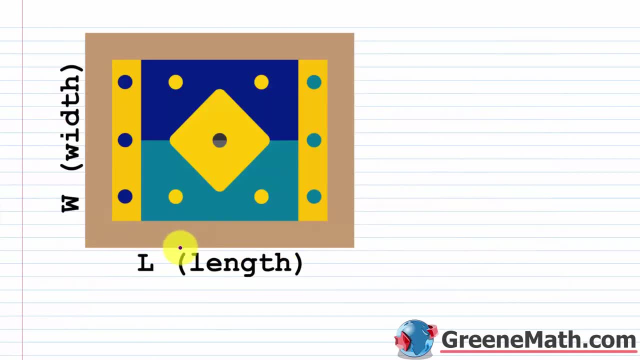 And what you'll see here is that the entire rectangle is meant to represent the bedroom, Okay, And then you have this kind of smaller rectangle which represents your rug, And then the brown. you see, that's the strip of uncovered floor. Okay, That's around the rug, Okay, And 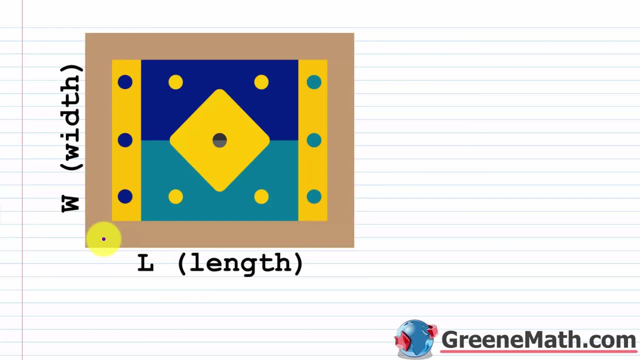 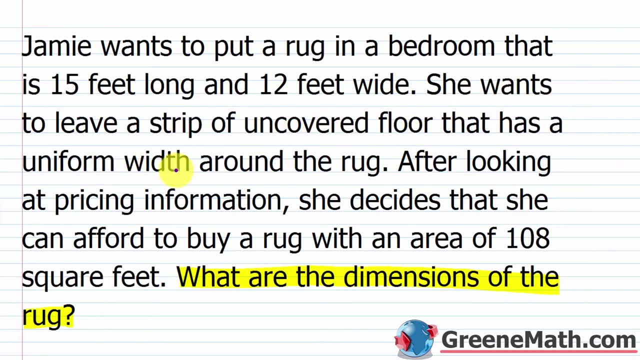 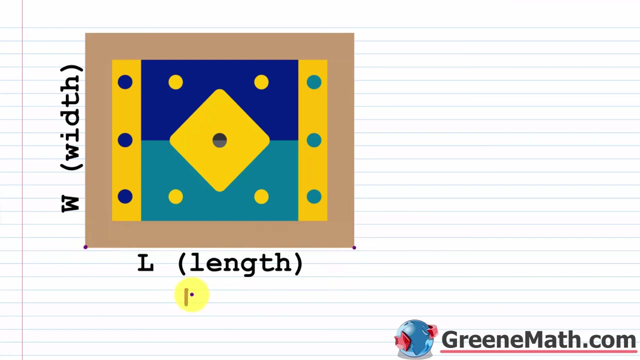 that's actually the key to understanding this problem. So when we go back up, I just want to read this part one more time. So what do we know? We know the length of the bedroom, or the measurement from here to here, is 15 feet. Okay, That's given in the problem. We know the width, the measurement from here to here. 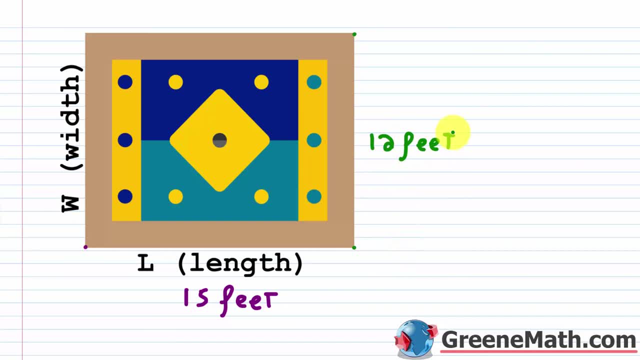 is 12 feet. That's given to us in the problem. We also know that this kind of strip of uncovered floor has a uniform width. So in other words, I know from here to here, and then from here to here, and from here to here and from here to here. this is all going to be the same all the way around. 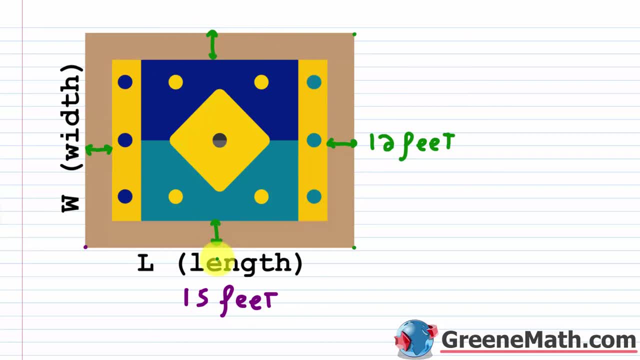 The width is all the same. Okay, So the key to this problem is letting a variable like X, or whatever you want to use, represent that uniform width for that strip of uncovered floor. Okay, So I'm just going to say: this is X, this is X, this is X. 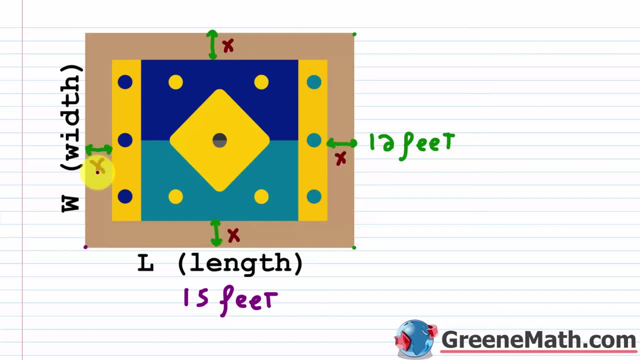 and this is X. Okay, So, given the information that we have now, can you see how you would set up and find the dimensions of the rug? Okay, So, for the rug, we want to know what's the length and what's the width. Well, for the length, I know the length of the bedroom It's given to. 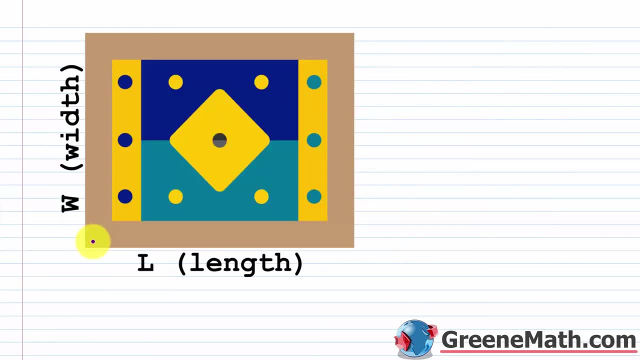 we're just going to label a few things. So what do we know? We know the length of the bedroom, or the measurement from here to here is 15 feet. Okay, That's given in the price. So we're going to go back to the problem. We know the width: the measurement from here to here is 12 feet, That's. 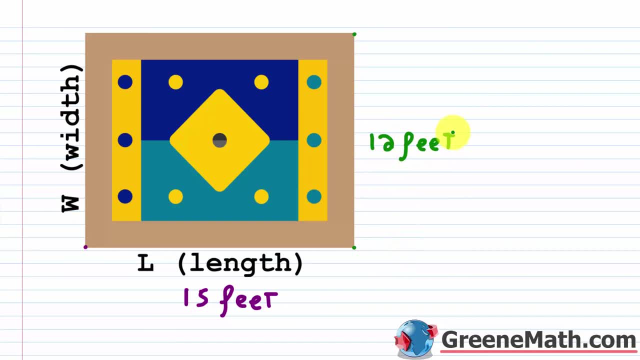 given to us in the problem. We also know that this kind of strip of uncovered floor has a uniform width. So, in other words, I know from here to here, and then from here to here, and from here to here, and from here to here, this is all going to be the same all the way around. The width is. 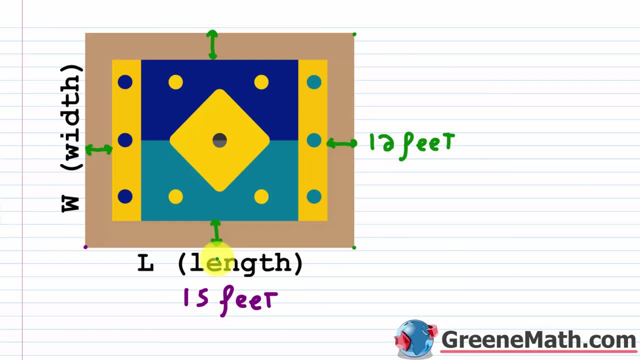 all the same. Okay. So the key to this problem is letting a variable like X, or whatever you want to use, represent that uniform width for that strip of uncovered floor. Okay, So I'm just going to say: this is X, this is X, this is X and this is X. Okay. So, given the 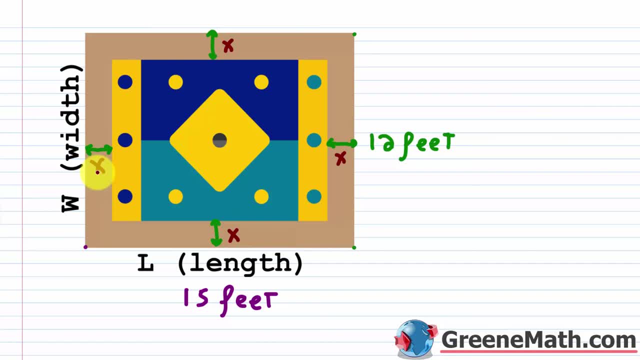 information that we have now, can you see how you would set up and find the dimensions of the rug? Okay, So for the rug, we want to know what's the length and what's the width. Well, for the length, I know the length of the bedroom. I know the length of the bedroom. I know the length of the bedroom. 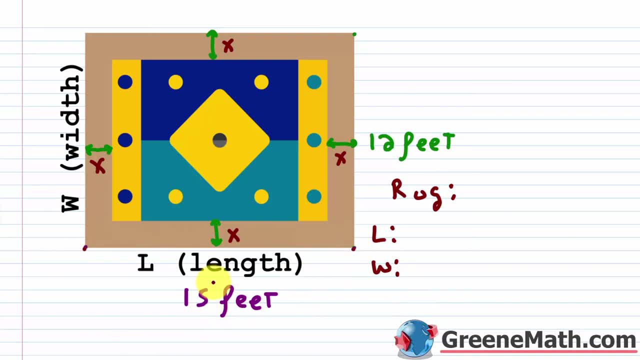 It's given to me it's 15 feet, So that's from here to here. If I want the length of the rug, well, I need to subtract out, kind of from here to here and from here to here, Okay, So what's? 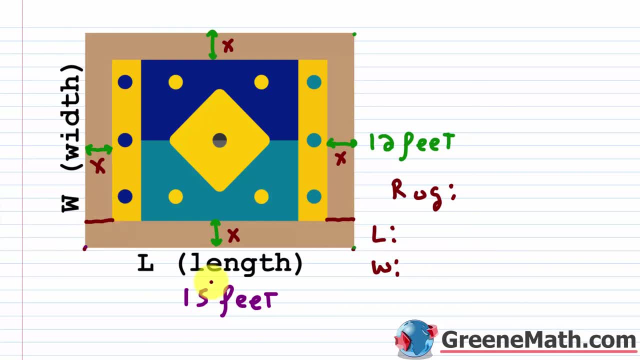 that measure And I kind of went over there. So let me draw that a little bit better. So what's that measure? Well, it's going to be 15, the total amount minus this, which is X- Okay, This is X, and then minus this, which is X. So 15 minus X, minus X, which is going to be 15 minus. 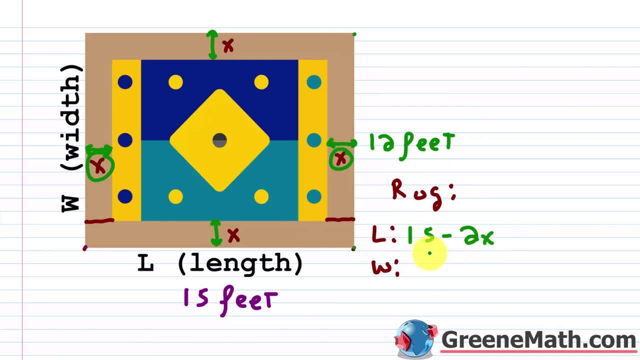 two X, Okay, So that's going to be my length of the rug, So I'm going to draw that measure. I'm going Now for the width. it's a similar thought process. Okay, The width is going to be from here to here. 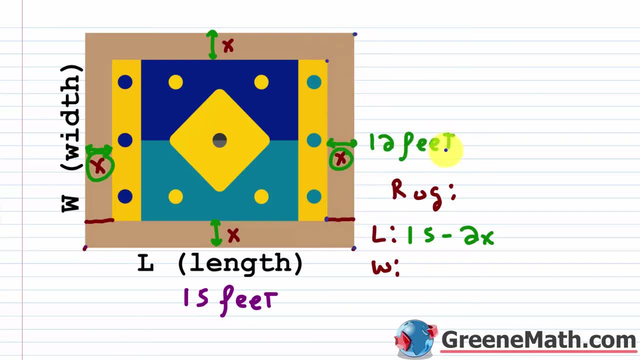 And again, I just want to think about the width of the whole room, which is 12 feet, So I'm just going to put 12 there and I want to subtract out this guy right here, which is X, And I want to. 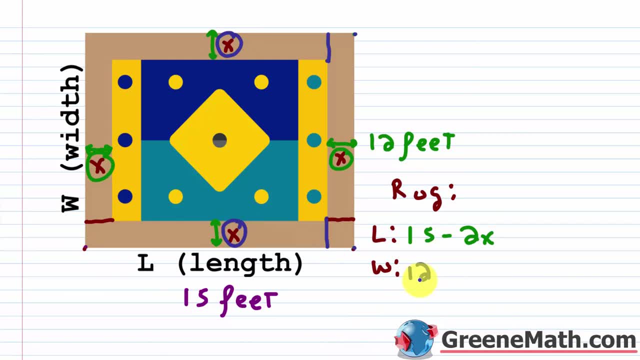 subtract out this guy right here, which is also X. So 12 minus X minus X is 12 minus two X. Okay, So now I have a length as an expression- 15 minus two X- and I have a width as an expression. 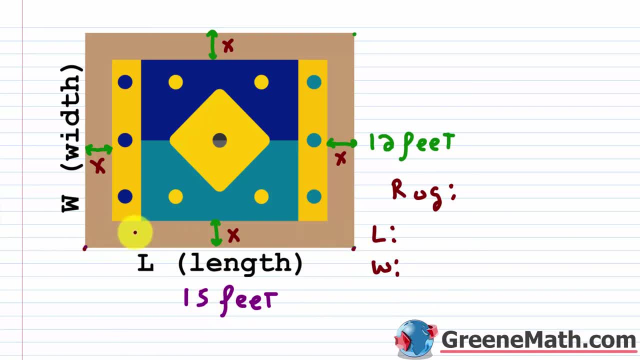 me It's 15 feet, So that's from here to here. If I want the length of the rug, well I need to subtract out, kind of from here to here and from here to here, Okay, So what's the length of the? 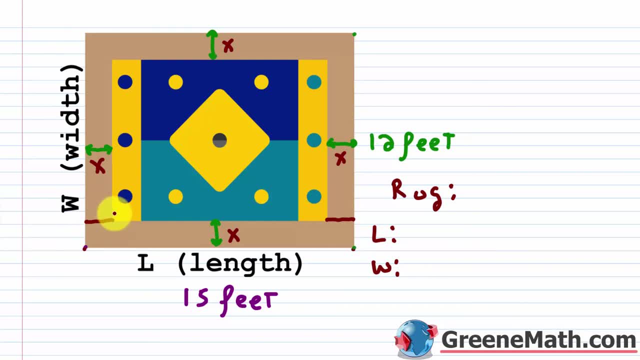 rug. What's that measure? And I kind of went over there, So let me draw that a little bit better. So what's that measure? Well, it's going to be 15, the total amount minus this, which is X. Okay. 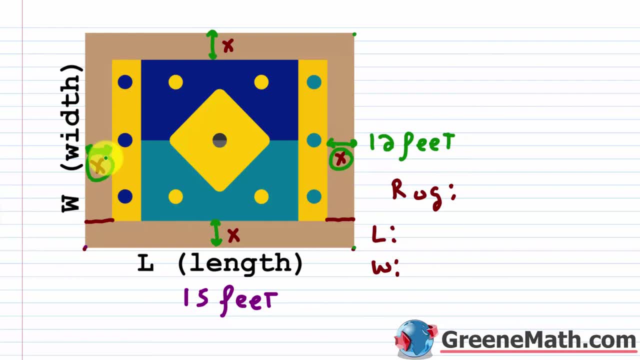 This is X, and then minus this, which is X, So 15 minus X minus X, which is going to be 15 minus two X. Okay, So that's going to be my length of the rug. Now for the width: it's a similar. 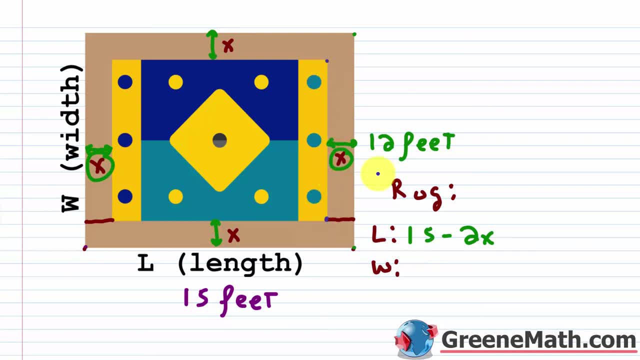 thought process: Okay, The width is going to be from here to here, And again I just want to think about the width of the whole room, which is 12 feet. So I'm just going to put 12, and I want to subtract out this guy right here, which is X, And I want to subtract out this guy. 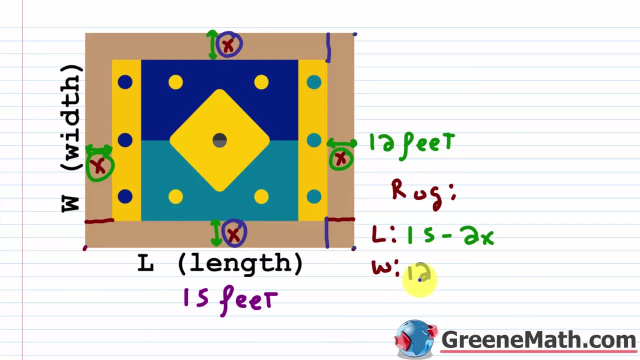 right here, which is also X. So 12 minus X minus X is 12 minus two X. Okay, So now I have a length as an expression- 15 minus two X- and I have a width as an expression- 12 minus two X. So let's. 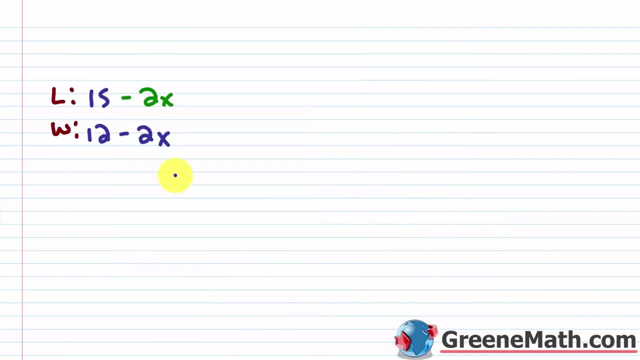 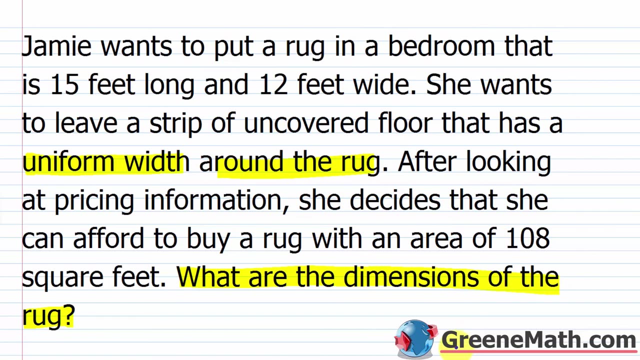 copy that real quick And I'm just going to paste that there And what we know from our problem. it tells us that she can afford to buy a rug with an area of 108 square feet, So we're going to assume that that's what she buys. 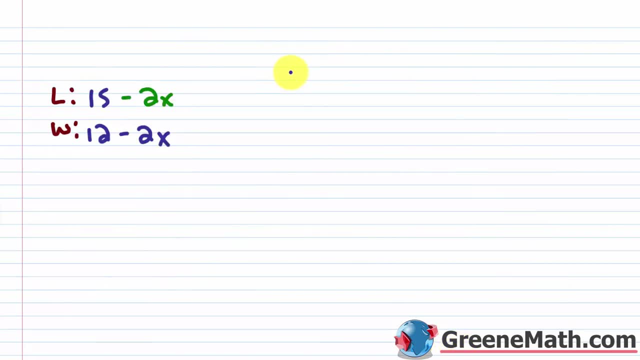 So my length times my width gives me my area. So what I'm going to do is I'm going to say 15 minus two X. that quantity, that's my length, multiplied by the quantity 12 minus two X, that's my width, This should equal my area, And we're told that the area is 108 square feet. 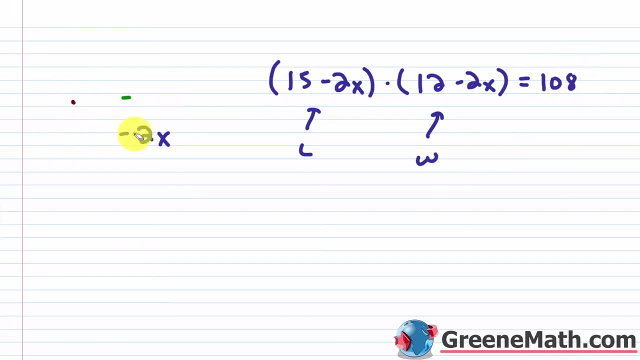 So I'm just going to put 108.. Okay, So I'm going to solve this equation for X and that's going to allow me to find out what is the length and what is the width for my rug that Jamie has. Okay, 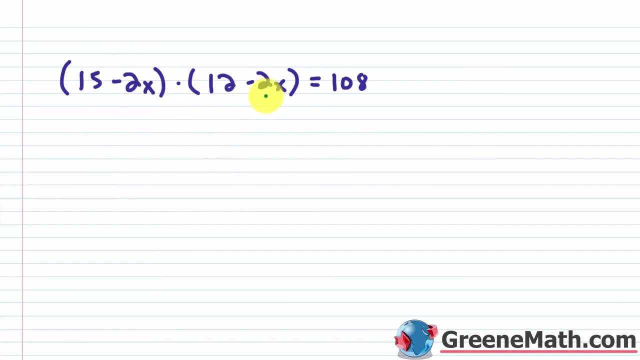 So 15 minus two X times 12 minus two X. we're going to use four for that. So 15 times 12 is 180.. And then 15 times negative: two X is minus 30 X. Negative: two X times 12 is minus 24 X. 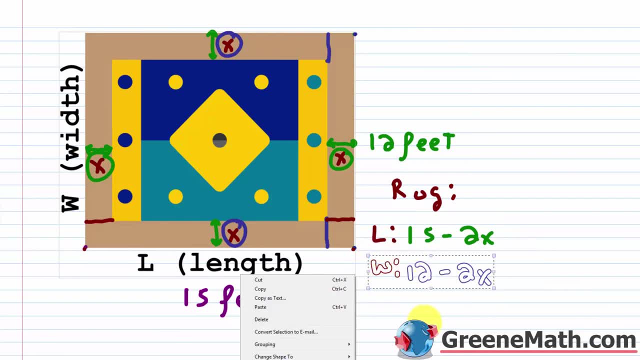 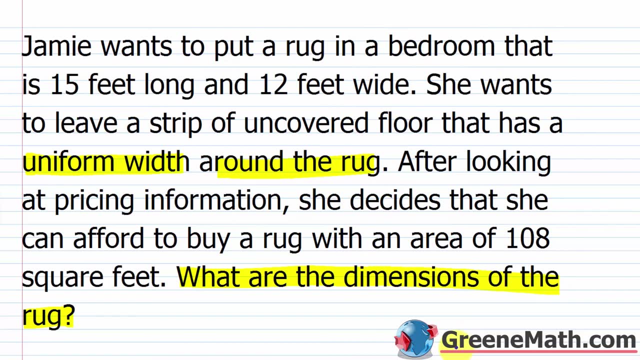 12 minus two X. So let's copy that real quick And I'm just going to paste that there. And what we know from our problem. it tells us that she can afford to buy a rug with an area of 108 square feet. So we're going to. 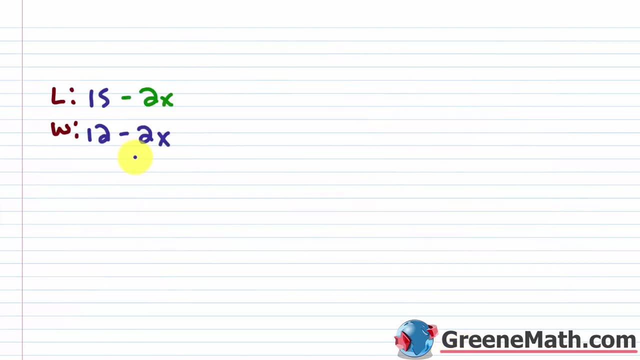 assume that that's what she buys. So my length times my width gives me my area. So what I'm going to do is I'm going to say 15 minus two X. that quantity- that's my length- multiplied by the quantity 12 minus two X- That's my width, This should equal my area And we're told that. 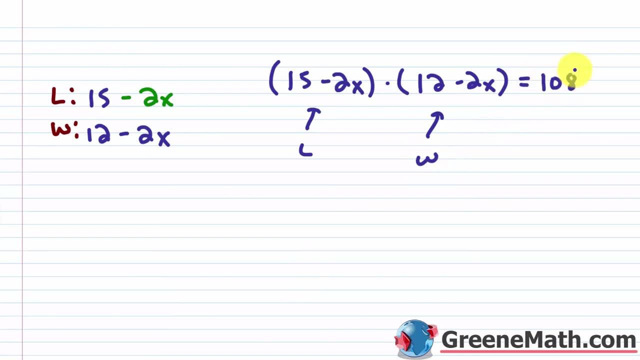 the area is 108 square feet, So I'm just going to put 108.. Okay, So I'm going to solve this equation for X And that's going to allow me to find out what is the length and what is the width for my rug that Jamie has. Okay, So 15 minus two X times 12 minus. 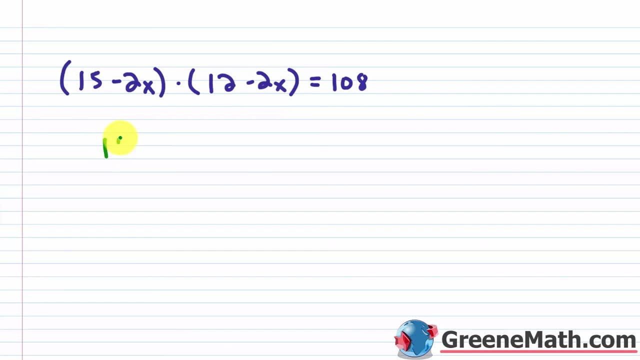 two X, we're going to use four for that. So 15 times 12 is 180.. And then 15 times negative: two X is minus 30 X. negative two X times 12 is minus 24 X. If I combine like terms I'm going to have: 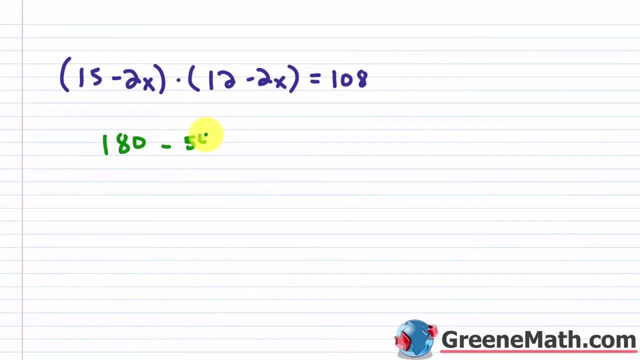 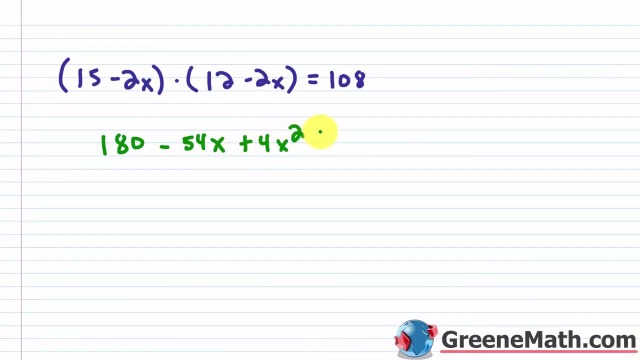 negative 54 X, So minus 54 X. All right, So then we have negative two X times negative two X, which is going to be plus four X squared, And then this is just equal to 108.. Okay, So let me kind of rearrange things here. 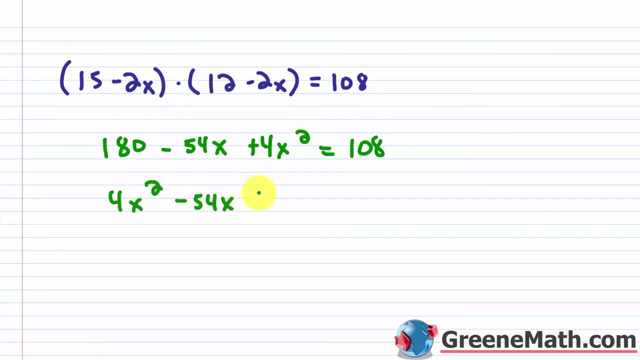 Let me put this as: four X squared minus 54, X plus 180 is equal to 108.. Now what I want to do is subtract 108 away from each side of the equation so that I can have zero on the right side, And I 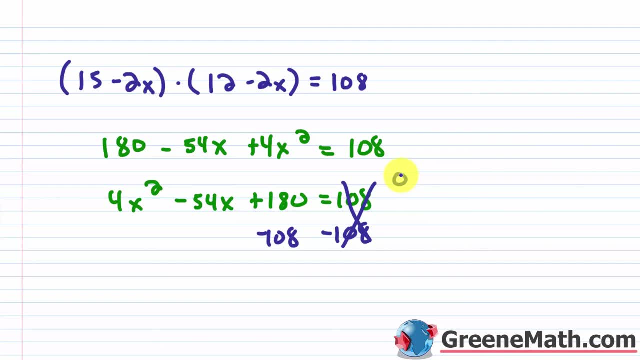 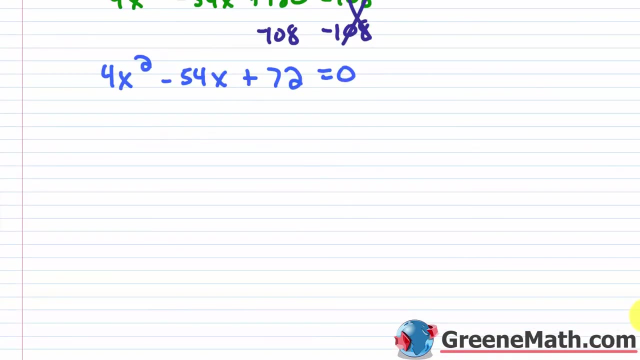 can go ahead and use my quadratic formula, or you could find out what that is. So I'm going to subtract the four X squared minus 54. X plus 180 minus 108 is going to be 72. This equals zero. Now, if you want to do this, this is an optional step. You don't need to. You can divide each part. 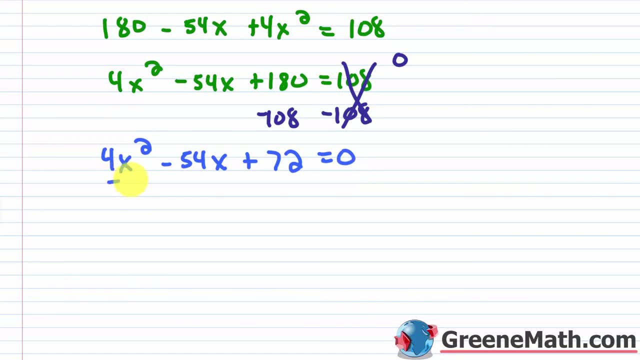 here by two. Okay, That's going to give you smaller numbers to work with. So if I divide this by two, this by two, this by two and this by two, I'm going to get two X squared minus 27 X plus. 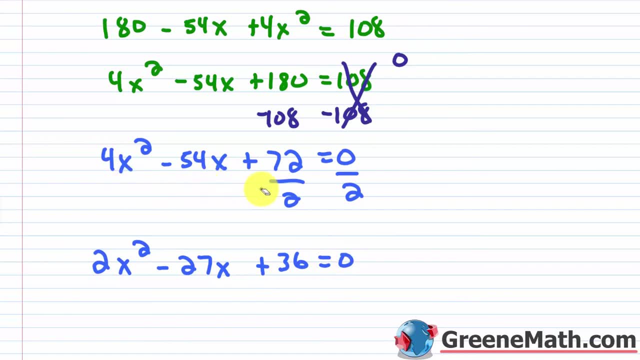 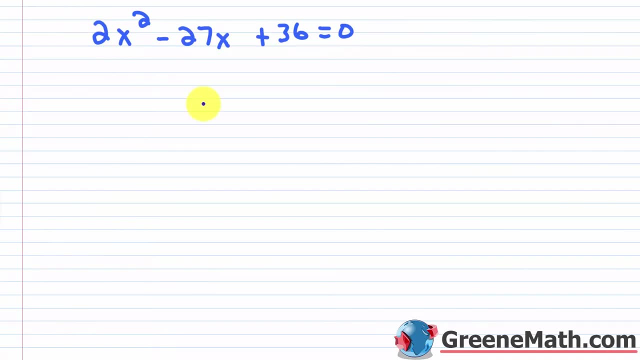 36 equals zero. Okay, That's just something I did to give us smaller numbers to work with, Again, completely optional. All right, So now let's use our quadratic formula Again. you can solve this one with factoring, but I'm going to use the quadratic formula, So this guy. 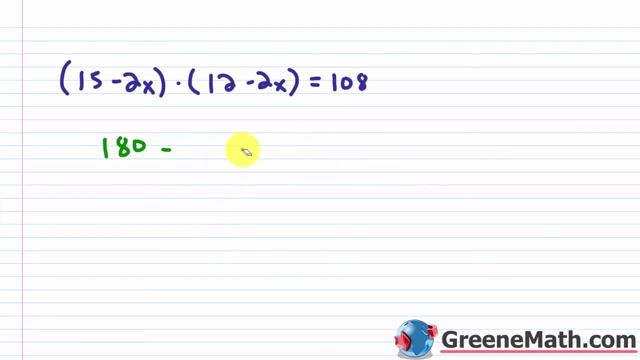 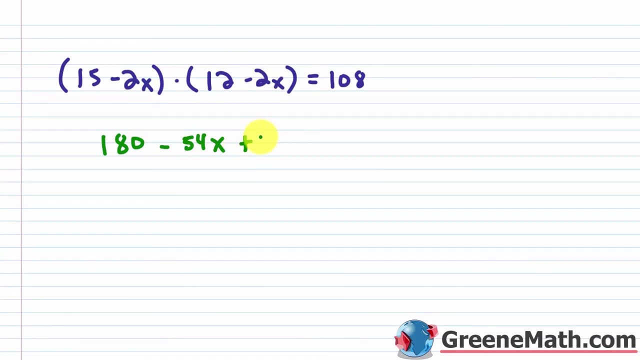 If I combine like terms, I'm going to have negative 54 X, So minus 54 X, All right. So then we have negative two X times negative two X, which is going to be plus four X squared, And then this is just equal to 108.. Okay. 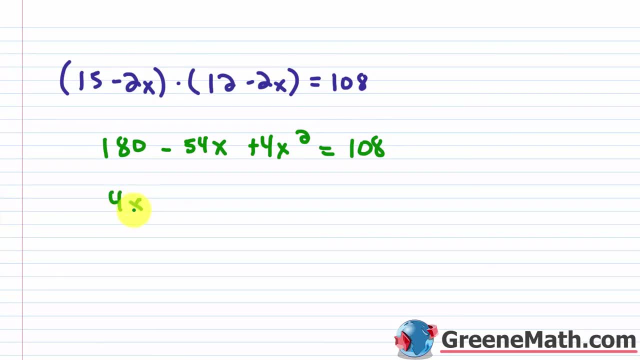 So let me kind of rearrange things here. Let me put this as: four X squared minus 54, X plus 180 is equal to 108.. Now what I want to do is subtract 108 away from each side of the equation so that I can have zero on the right side And I can go ahead and use my quadratic formula. 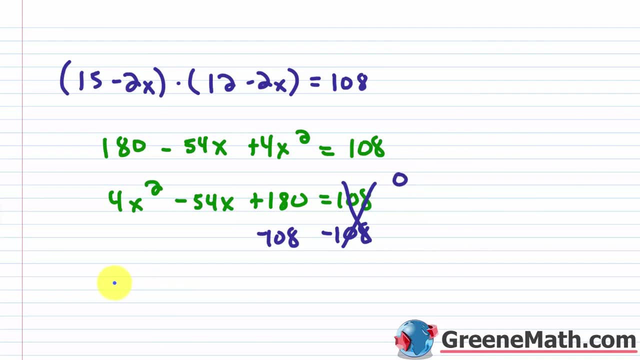 or you could factor whatever you want to do. Okay, So in this case, I'm going to have four X squared minus 54 X, and then plus 180 minus 108 is going to be 72. This equals zero. Now, if you want to do this, this is an optional step. You don't need to. 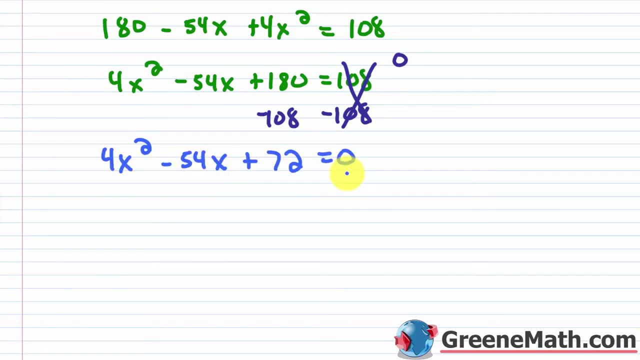 You can divide each part here by two. Okay, That's going to give you smaller numbers to work with. So if I divide this by two, this by two, this by two and this by two, I'm going to get two X. 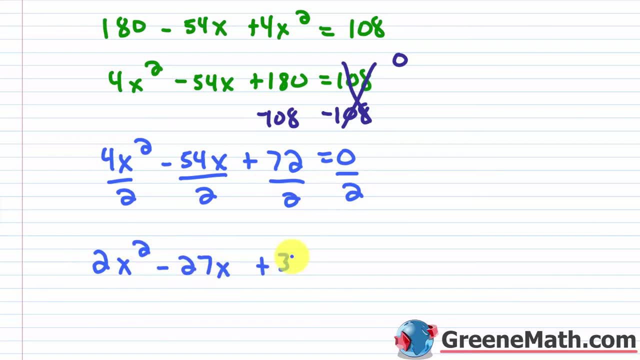 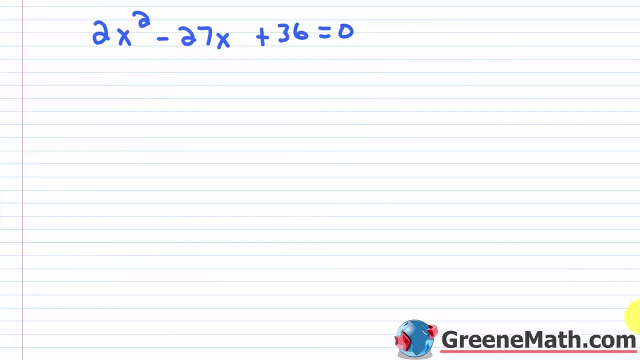 squared minus 27, X plus 36 equals zero. Okay, That's just something I did to give us smaller numbers to work with, Again, completely optional, All right. So now let's use our quadratic formula Again. you can solve this one with factors. 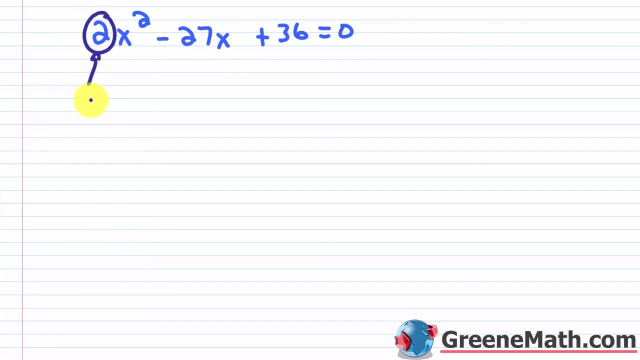 But I'm going to use the quadratic formula. So this guy right here, this is going to be A. This guy right here, this is going to be B. This guy right here is going to be C. Okay, So I'm going to plug into: X equals the negative of B plus or minus the square root of. you've got B squared. 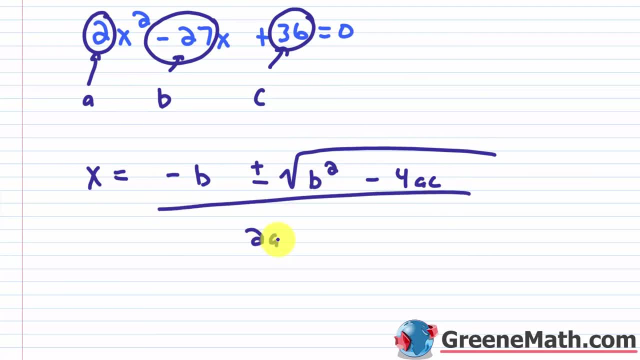 minus 4AC, The whole thing's over 2A. Okay, So the negative of B: B is negative 27.. So just plug that in there. Then B squared, you've got negative 27 squared four times A times C. A is. 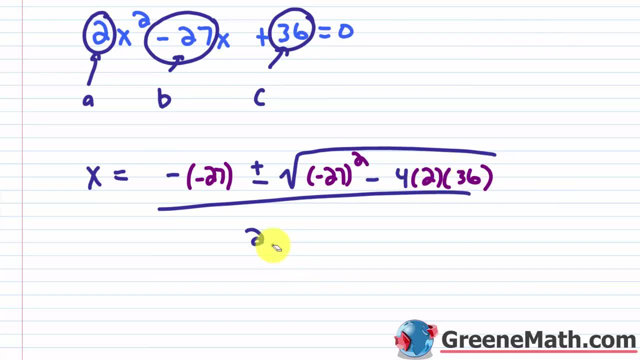 2.. C is 36.. And then A again is 2.. Okay, So we filled all of this in. Now we can just kind of crank it out. The negative of negative 27 is 27.. Okay, So that's easy enough. Negative 27 squared. 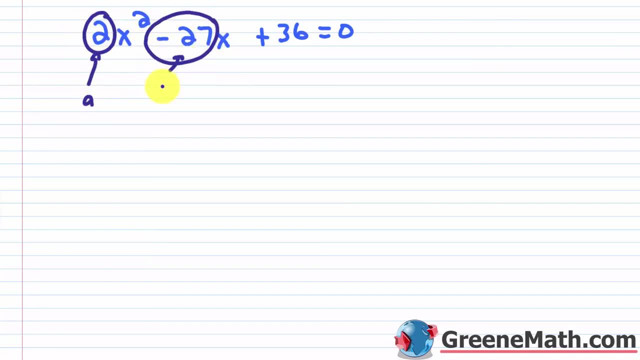 right here, this is going to be A. This guy right here, this is going to be B. This guy right here is going to be C. Okay, So I'm going to plug into: X equals the negative of B, plus or minus the square. 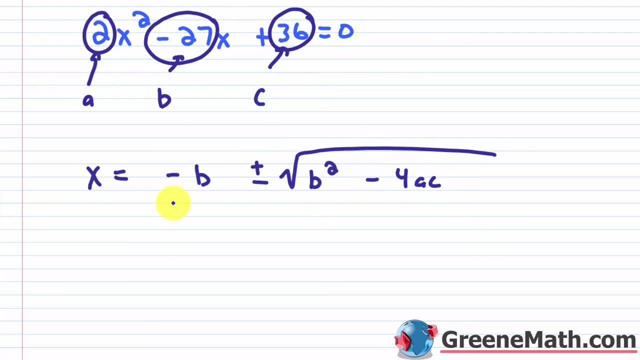 root of. you've got B squared minus four AC. The whole thing's over, Okay. So the negative of B, B is negative 27.. So just plug that in there, Then B squared. you've got negative 27 squared four times, eight times C. A is two, C is 36, and then A again is: 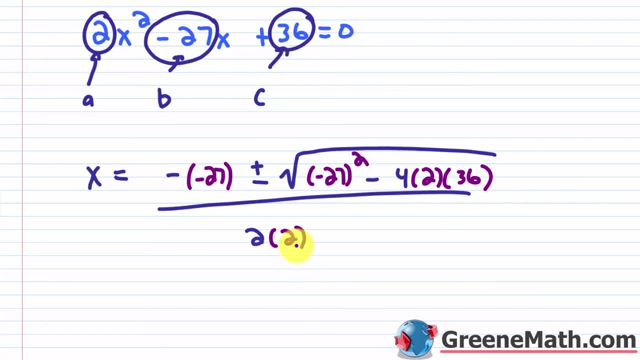 two. Okay, So we filled all this in. Now we can just kind of crank it out. The negative of negative 27 is 27.. Okay, So that's easy enough. Negative 27 squared is 729.. So this would be 729.. Negative. 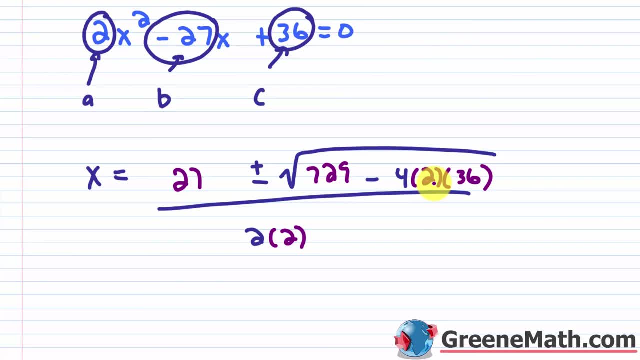 four times two is negative eight, And then negative eight times two is negative eight. Negative eight times 36 is negative 288.. So this is basically minus 288.. If I do that calculation real quick, I'm going to get 441, right. 729 minus 288 is 441.. If I took the square root of 441,, 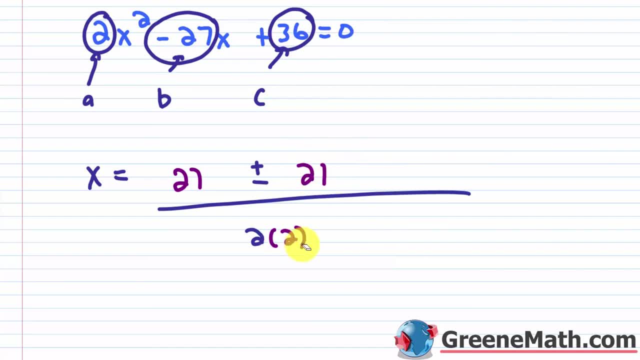 I would get 21.. Okay, So this is 21 here, And then two times two is four. Okay, So we're going to get two answers. You're going to find that one of them doesn't work, but we'll get to that in a minute. 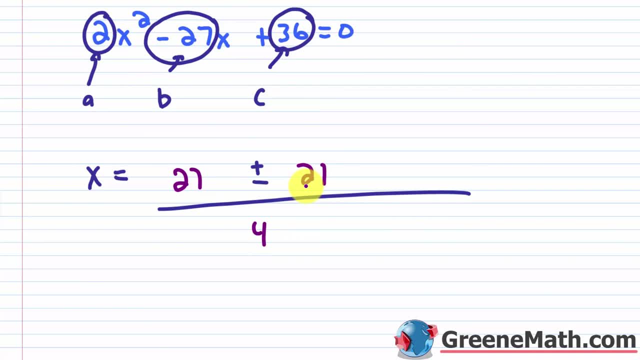 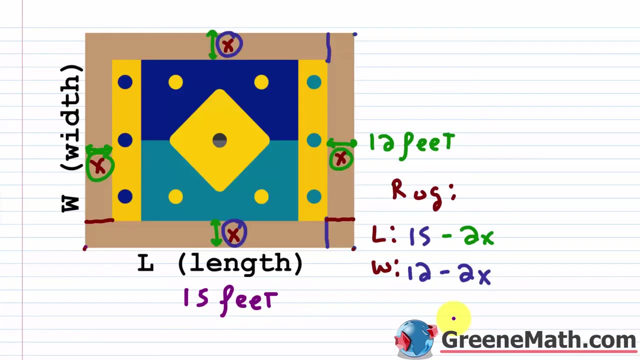 So 27 plus 21 is going to be 48.. 48 divided by four is 12.. So X equals 12.. And then also, 27 minus 21 is six. Six over four you can say that's three halves or 1.5.. So let's take these back to our illustration and we're going to see if they 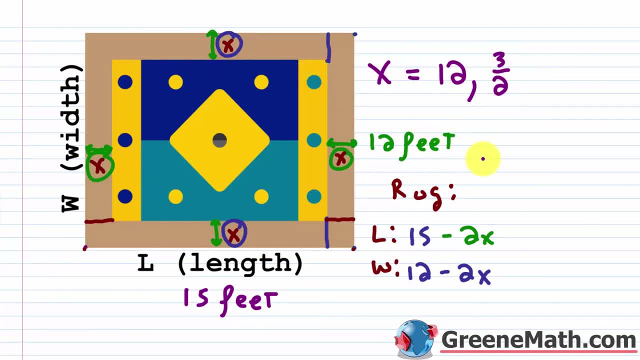 make sense. Okay, So let me paste this up here. So can X be 12?? Remember, I'm plugging in for X in each case, So I'm plugging in here and here. Well, two times 12 is 24.. 15 minus 24 is negative. 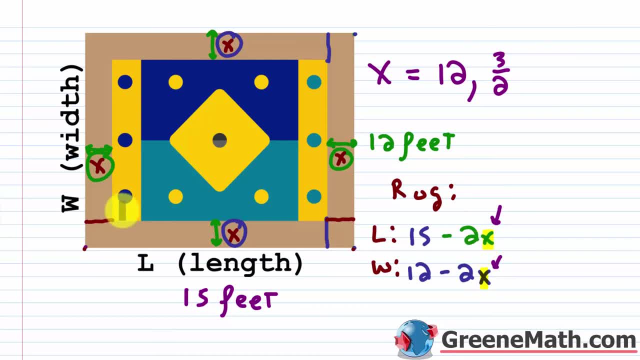 Okay, It's going to be negative nine. Does it make sense for this rug to have a length of 24?? No, it doesn't. It doesn't make sense for this rug to have a length of 24.. So it doesn't make sense for this rug to have a length of negative nine. Okay, No, it can't be. 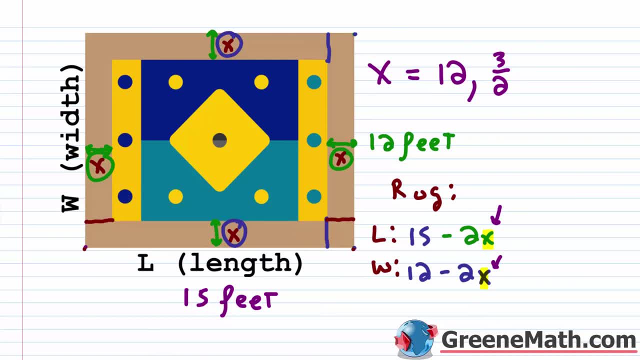 negative nine feet. That doesn't make any sense. It's nonsense. So you get that when you solve these problems, you just have to reject one of the solutions, So go ahead and throw that out. Okay, You can't use that. Can we use three halves? Yes, we can. Three halves is 1.5.. If you multiply two, 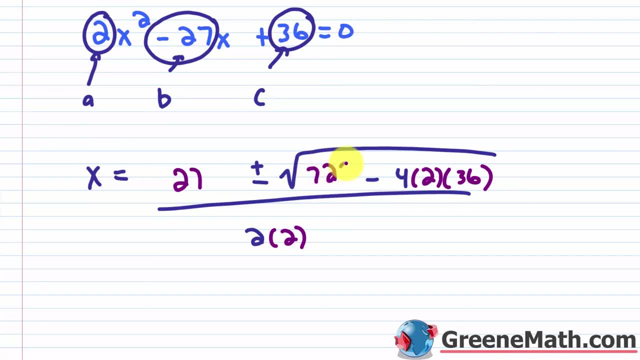 is 729.. So this would be 729.. Negative 4 times 2 is negative 8.. And then negative 8 times 36 is negative 288.. So this is basically minus 288.. If I do that calculation real quick. 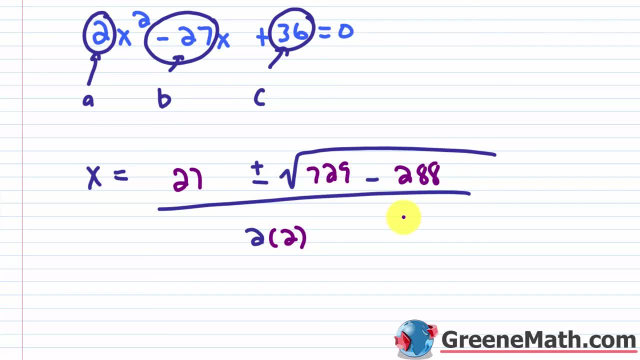 I'm going to get 441, right? 729 minus 288 is 488.. 441.. If I took the square root of 441, I would get 21.. Okay, So this is 21 here, And then two times two is four. Okay, So we're going to get two answers. You're going to find that one of. 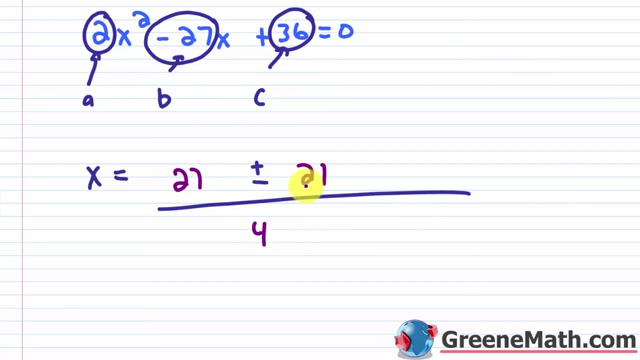 them doesn't work, but we'll get to that in a minute. So 27 plus 21 is going to be 48.. 48 divided by four is 12.. So X equals 12.. And then also 27 minus 21 is six. six over four, You can. 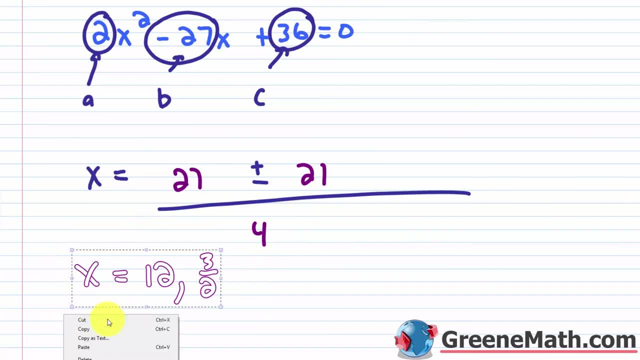 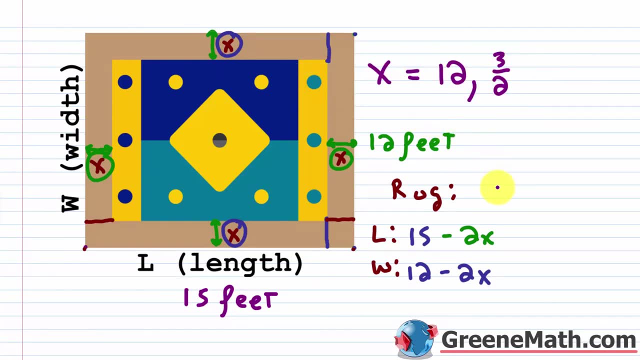 say that's three halves or 1.5.. So let's take these back to our illustration and we're going to see if they make sense. Okay, So let me paste this up here. So can X be 12?? Remember, I'm plugging. 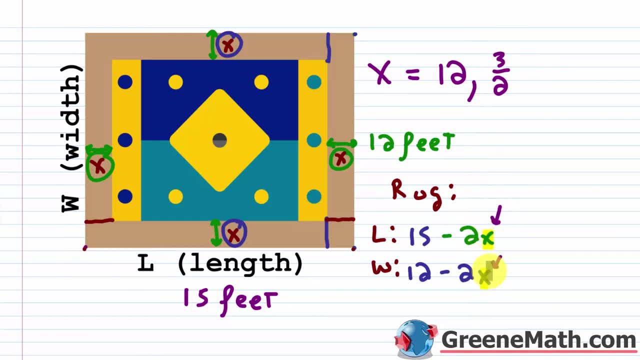 in for X in each case. So I'm plugging in here and here. Well, two times 12 is 24.. 15 minus 24 is negative. Okay, It's going to be negative nine. Does it make sense for this rug to have? 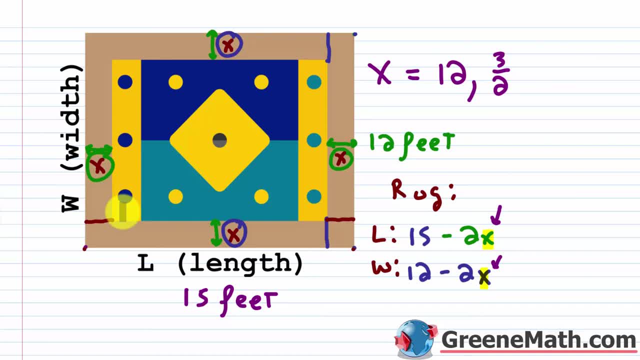 a length of negative nine. Okay, No, it can't be negative nine feet. That doesn't make any sense, It's nonsense. So you get that when you solve these problems, you just have to reject one of the solutions. So go ahead and throw that out. Okay, You can't use that. Can we use three halves? Yes, we can. 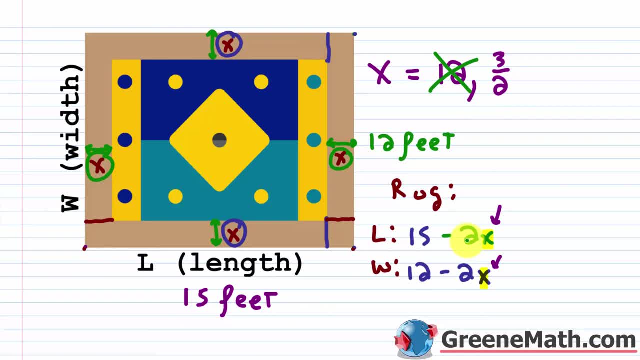 Three halves is 1.5.. If you multiply two by 1.5, you get three. Okay, So what you'd have in each case? you could just replace this with three and this with three. 15 minus three is 12.. So that's. 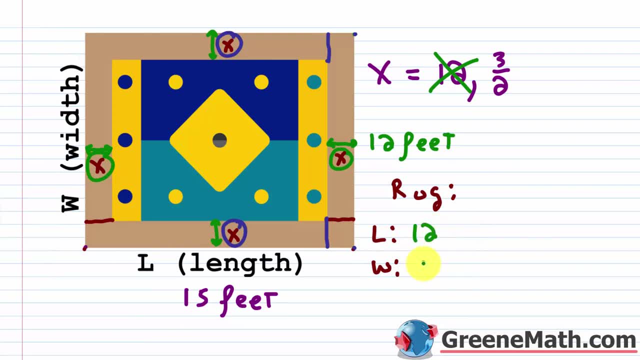 the length of the rug, And 12 minus three is nine, So that's the width of the rug. Okay, So we've found our answer for our problem. So what are the dimensions of the rug? We'll say that Jamie's rug. 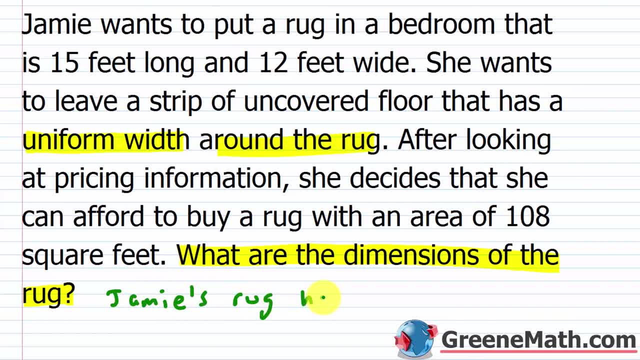 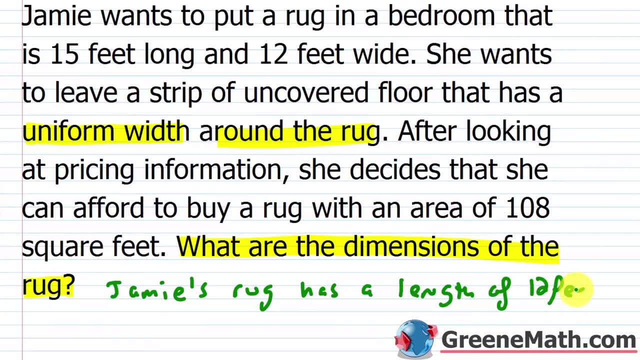 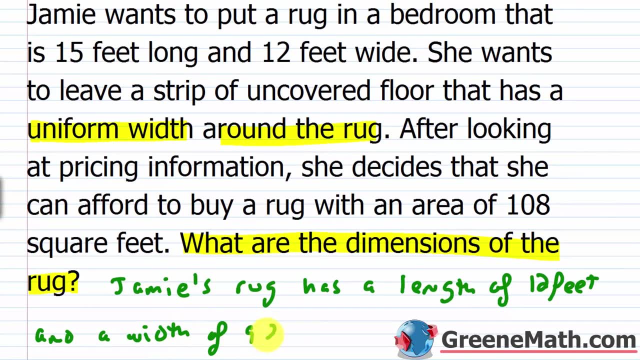 is Okay. Jamie's rug has a length of 12 feet and a width of nine feet. Okay. Is that consistent with what we're told in the problem? Well, 12 times nine is 108.. Feet times feet is feet squared or square feet. So that does match. 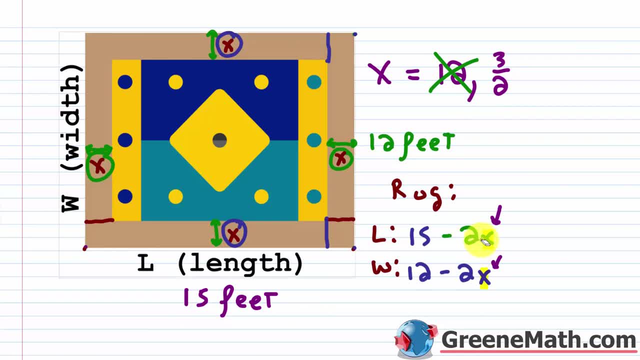 by 1.5, you get three. Okay, So what you'd have in each case? you could just replace this with three and this with three. 15 minus three is 12.. So that's the length of the rug And 12 minus three. 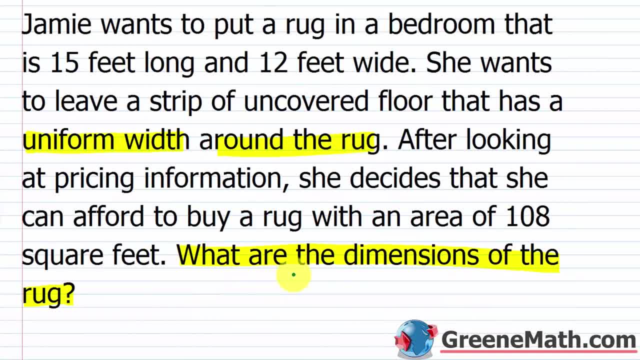 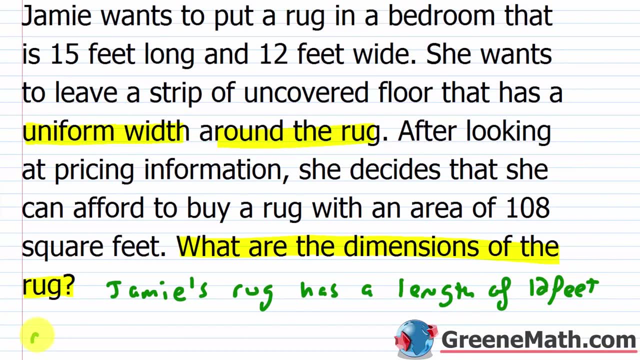 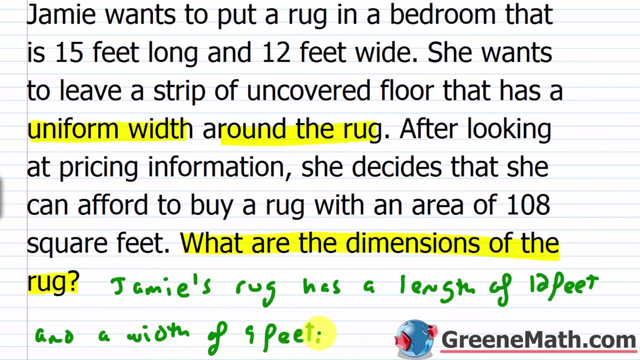 is one. Okay, So we basically found our answer for our problem. So what are the dimensions of the rug? We'll say that Jamie's rug has a length of 12 feet and a width of nine feet. Okay, Is that consistent with what we're told in the problem? Well, 12 times nine is 108.. Feet times feet is. 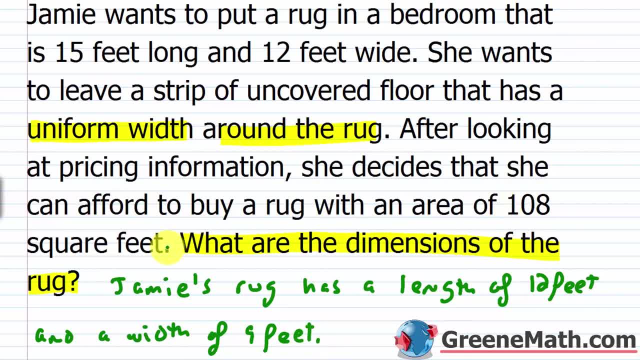 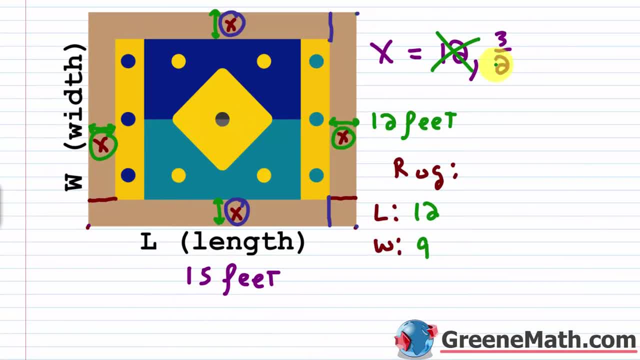 feet, squared or square feet. So that does match up with this. Okay, But you can also check to make sure that it is consistent with the rest of the problem. So when we come back to our little illustration again, we just want to check that this 1.5, this figure matches up with what we got right. So this 1.5 is the. 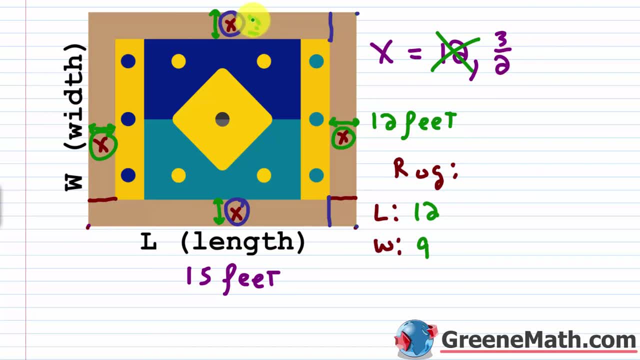 width of this strip of uncovered floor which has a uniform width. It's supposed to be the same all the way around, So it's 1.5 all the way around. Let me write that like this. Okay, So does that make sense? Well, if the length or the measurement from here to here 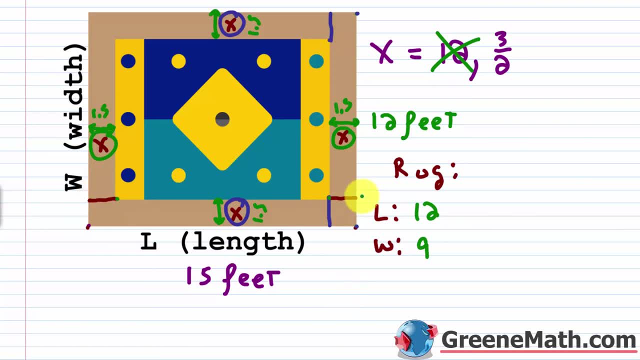 is 12 and I add 1.5 for this and 1.5 for this. well, yeah, 12 plus 1.5 plus 1.5 is 12 plus three, That's 15.. That's this guy right here, the length of the bedroom. Okay, So that makes sense Same. 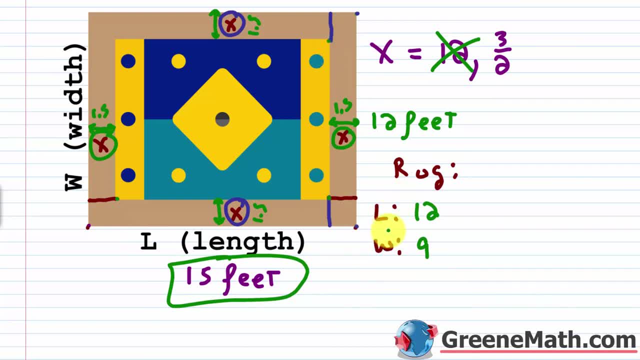 thing is going to happen for the width. So the measurement from here to here. we know that's nine. then plus another 1.5, plus another 1.5, nine plus three is 12.. Again, that's given to us in the 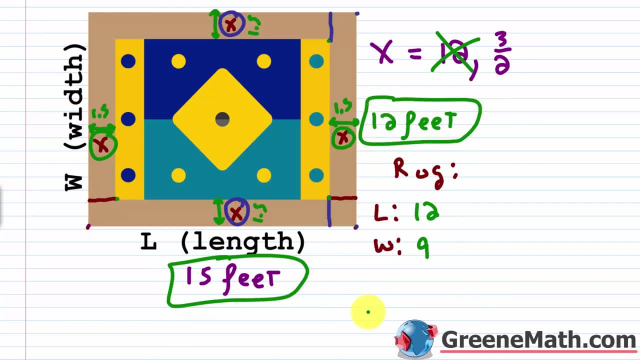 problem. So that checks out, And we also want to make sure that the measurement from here to here matches up, and it gives us 108 square feet, So we can basically say we're good to go. This rug has a measurement of 12 feet for the length and nine feet for the width. All right, So let's wrap up. 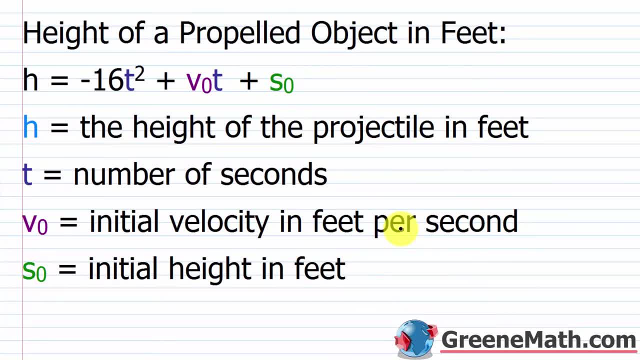 the lesson and talk about another common problem. you see, in this section We're going to be dealing with the height of a propelled object in feet. So when we get to this section we basically have a formula that we work with If air resistance is. 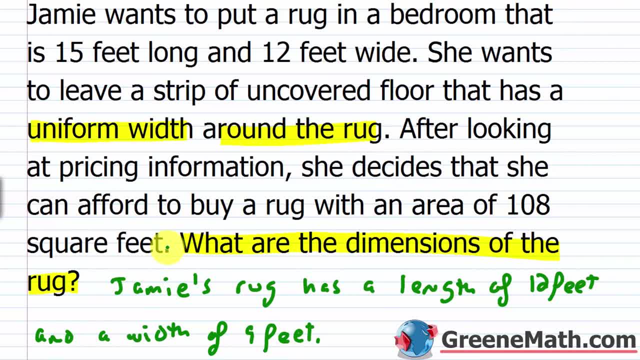 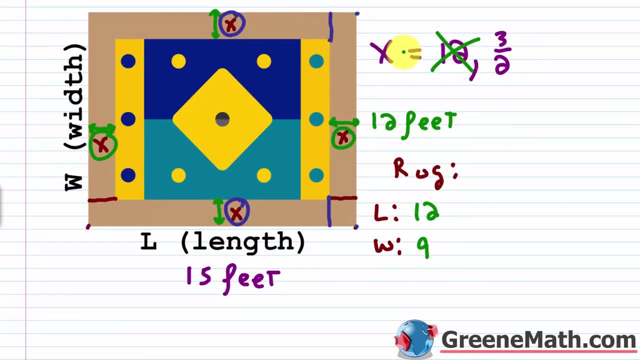 up with this. Okay, But you can also check to make sure that it is consistent with the rest of the problem. So when we come back to our little illustration again, we just want to check that this 1.5, this figure matches up with what we got right. So this 1.5 is the width of this. 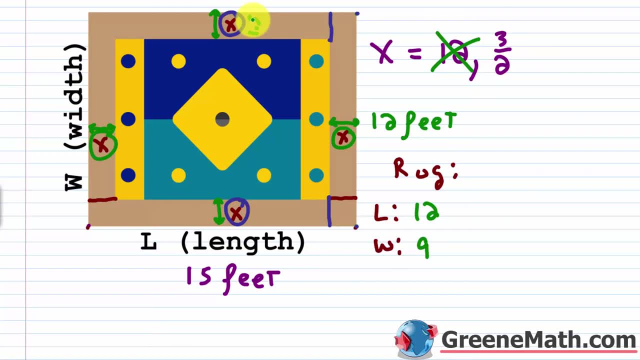 strip of uncovered floor which has a uniform width. It's supposed to be the same all the way around, So it's 1.5 all the way around. Let me write that like this: Okay, So does that make sense? Well, if the length, or the measurement from here to here gets equal to the length of this rug, 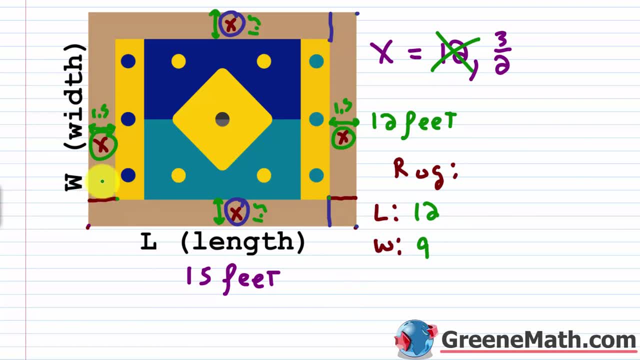 here is 12, and I add 1.5 for this and 1.5 for this. well, yeah, 12 plus 1.5 plus 1.5 is 12 plus 3, that's 15. that's this guy right here, the length of the bedroom. okay, so that makes sense. same thing. 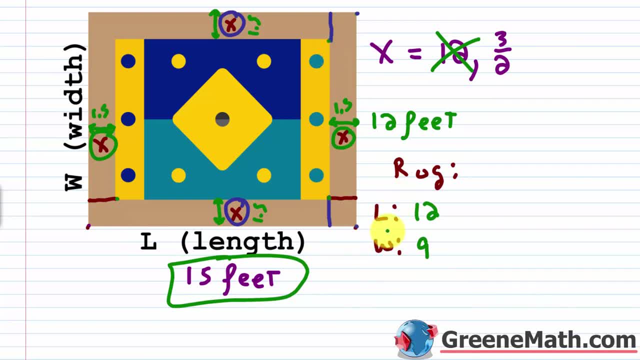 is going to happen for the width. so the measurement from here to here we know that's 9. then plus another 1.5 plus another 1.5. 9 plus 3 is 12. again, that's given to us in the problem. so that checks. 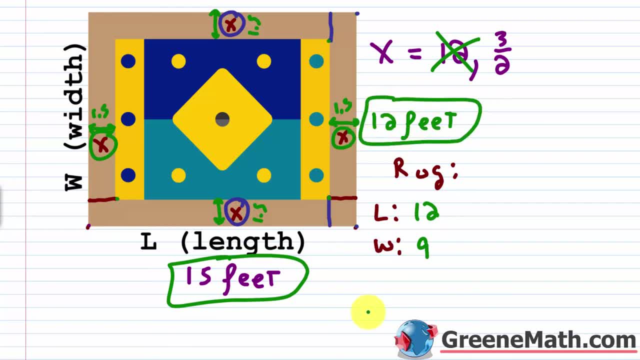 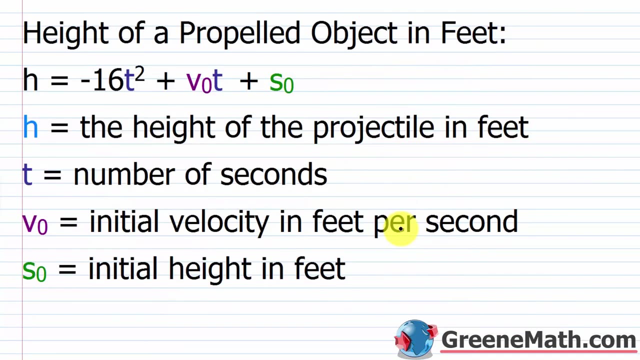 out, and we already checked the fact that the rug matches up and it gives us 108 square feet, so we can basically say we're good to go. this rug has a measurement of 12 feet for the length and 9 feet for the width. all right, so let's wrap up the lesson and talk about another common problem. 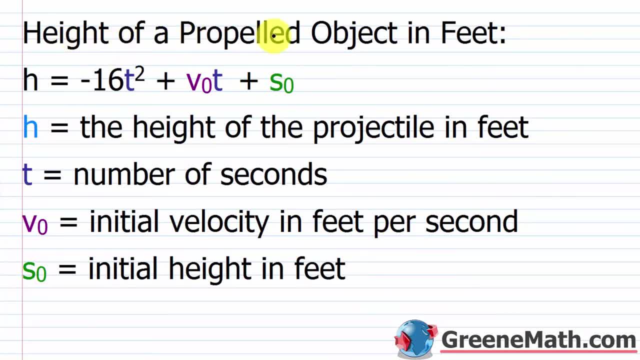 you see, in this section we're going to be dealing with the height of a propelled object in feet. so when we get to this section, we basically have a little formula that we work with. if air is hot, we're going to be dealing with the height of a propelled object in feet. 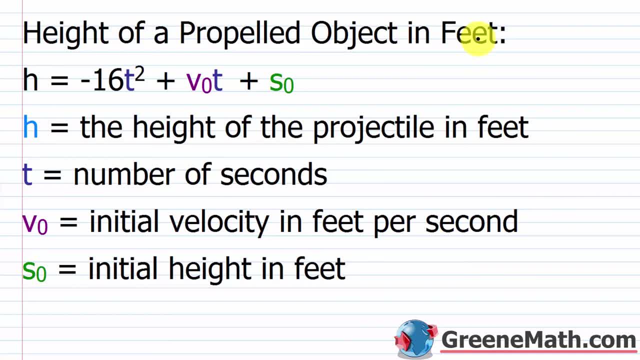 resistance is disregarded, the height of an object that's propelled directly upward can be thought about with this formula. so we have: h is equal to negative 16 t squared plus v sub 0 times t plus s sub 0. so when you're in this section in your algebra course you're going to be given this: 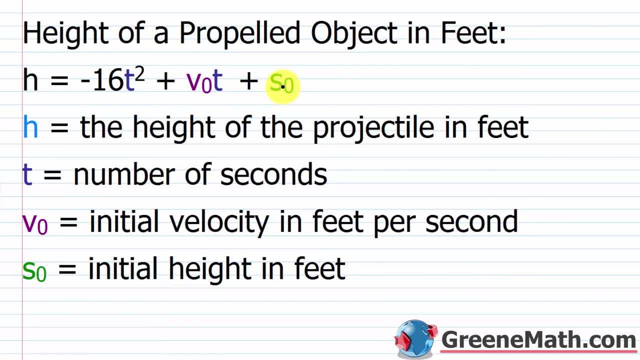 formula. they're going to give you stuff to plug in and then you're going to have to solve for something, okay? so h is the height of the projectile in feet, t is the number of seconds, v sub 0 is the initial velocity in feet per second and s sub zero is the initial height in feet. so when we're talking about height, 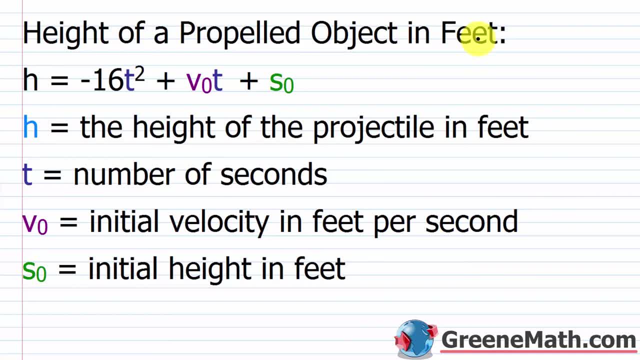 disregarded, the height of an object that's propelled directly upward can be thought about with this formula. So we have: H is equal to negative 16 T squared plus V sub zero times T plus S sub zero. So when you're in this section in your algebra course you're going to be given 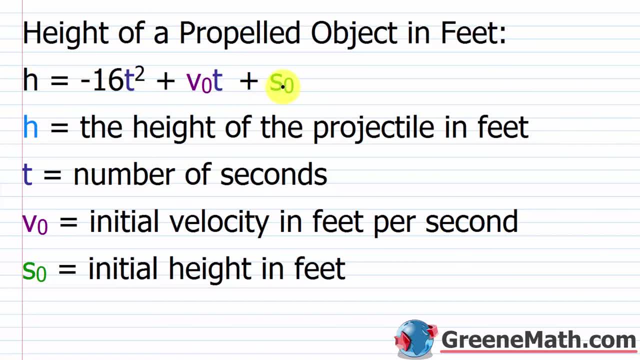 this formula. They're going to give you stuff to plug in and then you're going to have to solve for something. Okay, So H is the height of the projectile in feet, T is the number of seconds, V sub zero is the initial velocity in feet per second. 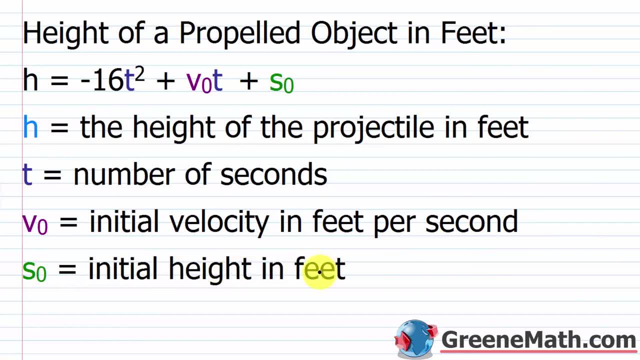 And S sub zero is the initial height in feet. So when we're talking about height, if I get a height of zero, that means I'm on the ground. Okay, If I get a height that's positive, let's say it's 50.. 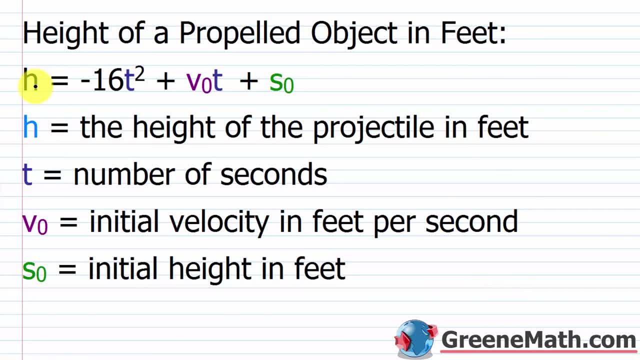 Let's say for H, again it's 50. That means I'm at a height of 50 feet in the air. Okay, If I get an initial height in feet, it's the same thing If I got 50, that means I'm launching from 50 feet. 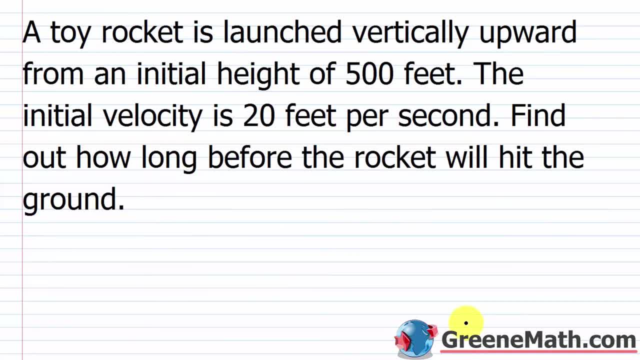 All right, Let's look at a sample problem. I think you'll find this to be very, very straightforward. A toy rocket is launched vertically upward from an initial height of 500 feet. The initial velocity is 20 feet per second. Find out how. 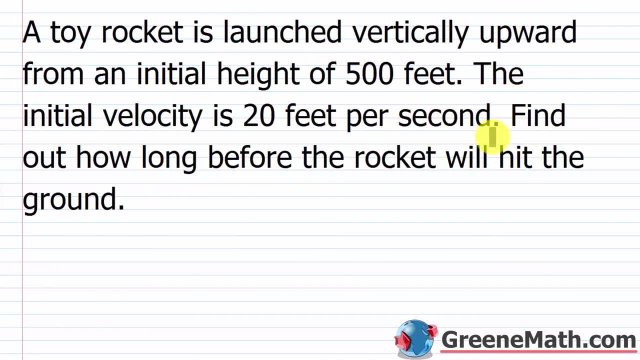 long before the rocket will hit the ground. Okay, So obviously we're just answering this part right here where it says to find out how long before the rocket will hit the ground. We're just going to take the formula: Let's go back for a second And we're going to grab this guy and I'm just 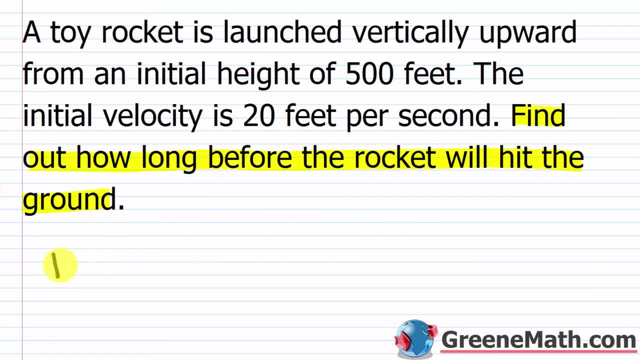 going to rewrite it right here real quick. So H is equal to: you've got negative 16 T squared. You got to be careful here because the T gets confused with a plus, So I'm going to put that in a different color. So plus: you've got your V sub zero times T. 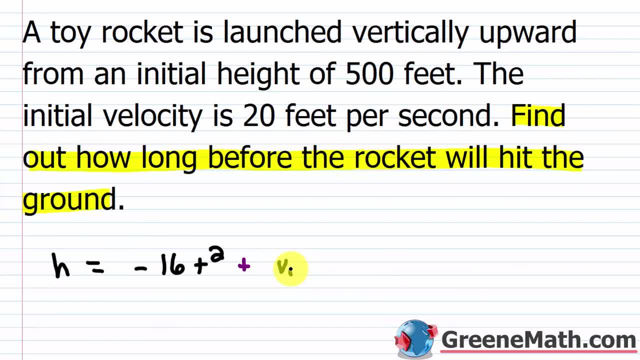 or you could say T times V sub zero. So let's put V sub zero times T, And again you've got another plus sign. So let's do that in a different color, And then you have your S sub zero. Okay, So this is your formula that you're working with. Now we can plug in a lot. 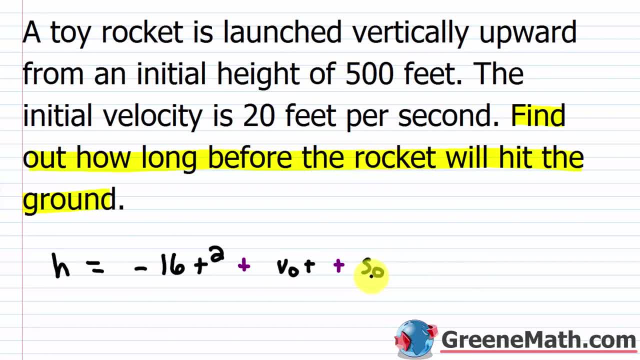 of information. here It says that the initial height is 500 feet S sub zero is your initial height, So you can just go ahead and erase this and put 500 there. And then it says: the initial velocity is 20 feet per second. So that's this V sub zero here. So I'll erase that and put a 20 there, Okay, 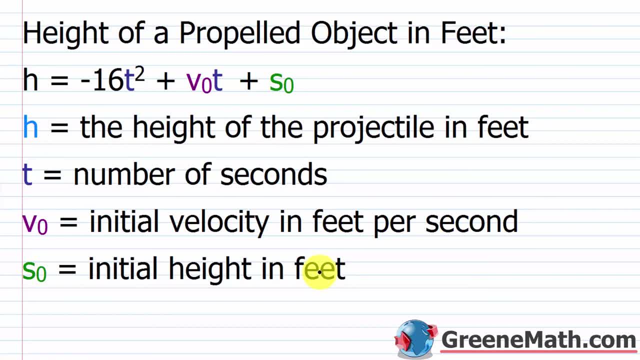 if i get a height of zero, that means i'm on the ground. okay, if i get a height that's positive, let's say it's 50. let's say for h, again it's 50. that means i'm at a height of 50 feet in the air. 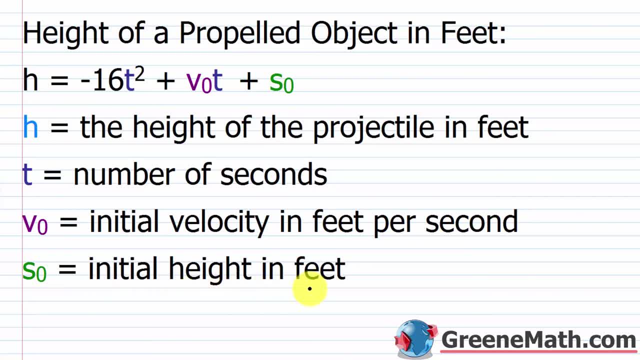 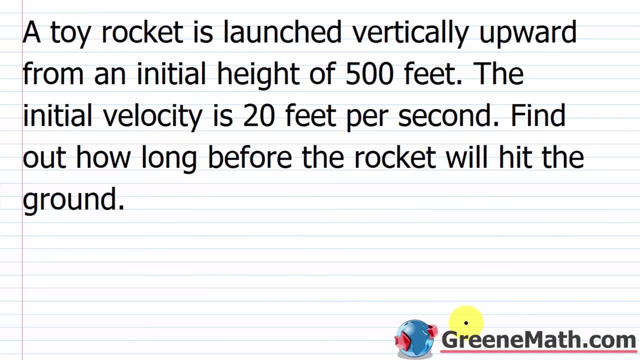 okay, if i get an initial height in feet, it's the same thing if i got 50. that means i'm launching from 50 feet. all right, let's look at a sample problem. i think you'll find this to be very, very straightforward. a toy rocket is launched vertically upward from an initial height of 500. 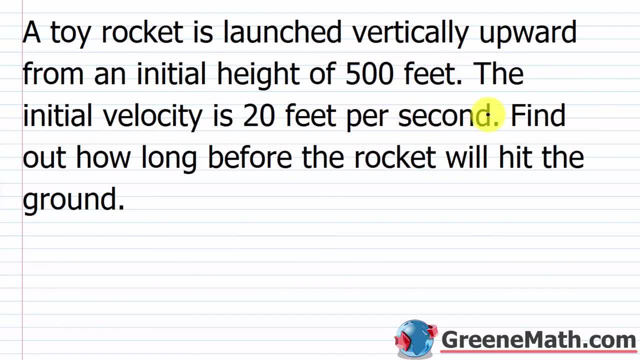 feet. the initial velocity is 20 feet per second. find out how long before the rocket will hit the ground. okay, so obviously we're just answering this part right here where it says to find out how long before the rocket will hit the ground. we're just going to take the formula. let's go back for a. 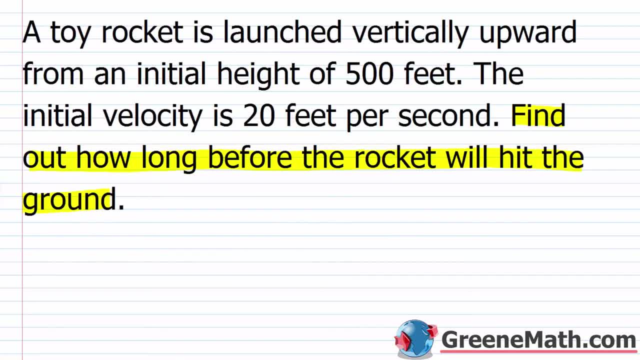 second, and we're going to grab this guy and i'm just going to rewrite it right here real quick. so h is equal to you've got negative 16 t squared. you got to be careful here, because the t gets confused with a plus sign. so i'm going to put 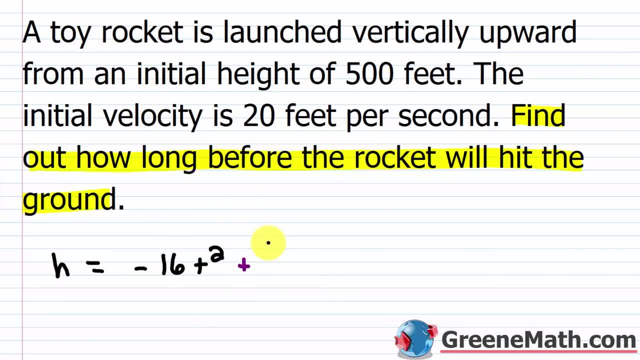 that in a different color. so, plus, you've got your v sub zero times t, or you could say t times v sub zero. so let's put v sub zero times t, and again you've got another plus sign. so let's do that in a different color, and then you have your s sub zero. okay, so this is your formula, that you're. 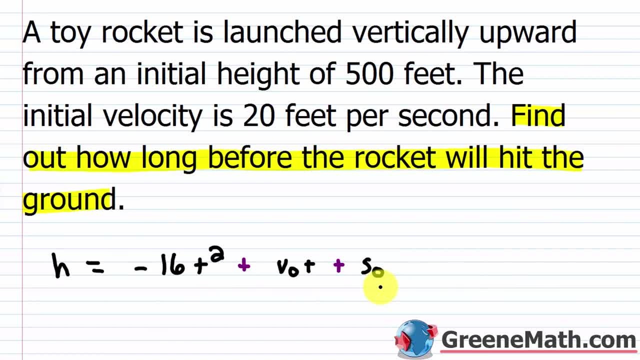 working with. now we can plug in a lot of information here. it says that the initial height is 500 feet s sub zero is your initial height, so you can just go ahead and erase this and put 500 there. and then it says the initial velocity is 20 feet per second. 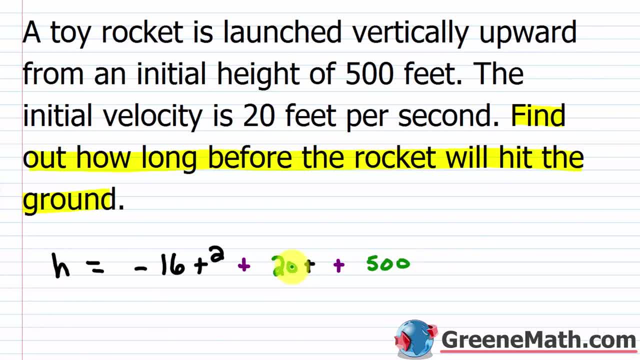 so that's this v sub zero here. so i'll erase that and put a 20 in. okay, so now we have two variables involved. i have h and i have t, but it says: find out how long before the rocket will hit the ground. we already said that when the rocket hits the ground, h is zero. right, that's the height, so i can. 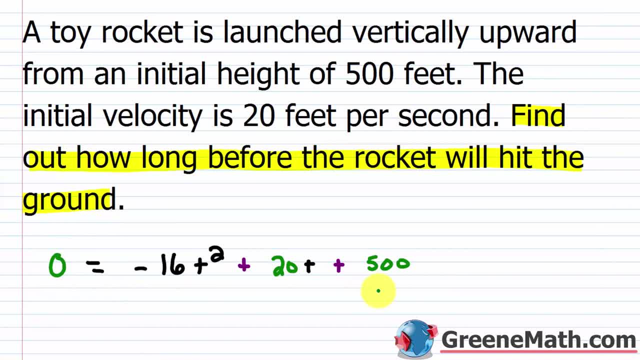 just replace it with h and i have t, so that's the initial height of the rocket. so i'm going to put the h with zero and all I have here is a standard quadratic equation, right? so I have negative 16 t squared plus 20 t plus 500. if I replace t with x, it's going to look very familiar for you, okay. 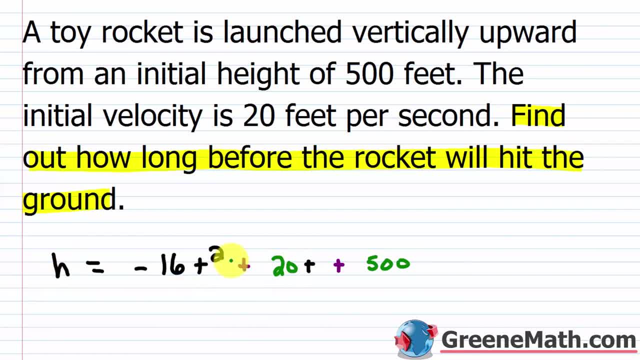 So now we have two variables involved. I have H and I have T, but it says: find out how long before the rocket will hit the ground. We already said that when the rocket hits the ground, H is zero. right, That's the height. So I can just replace H with zero, And all I have here is a. 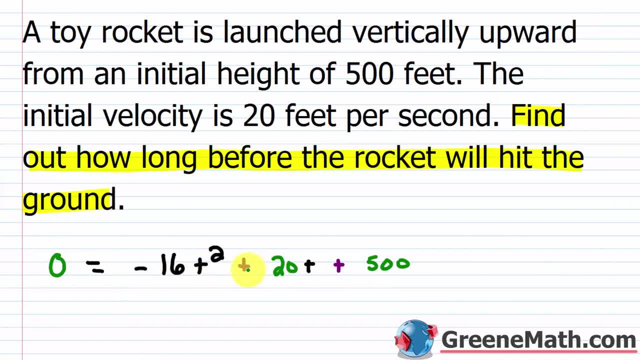 standard quadratic equation. So I have negative 16 T squared plus 20 T plus 500.. If I replace T with X, it's going to look very familiar for you. Okay, And I'm not going to keep it this way. I'm going to keep it with T. 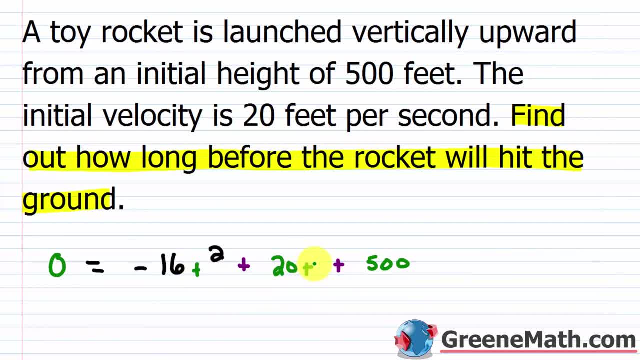 because that's consistent with our formula. But if you were struggling and you couldn't kind of grasp what's going on, just replace it with X, solve it, and then go back and replace that for T. Okay, Not a big deal. So I can solve this using the quadratic formula. I can also solve. 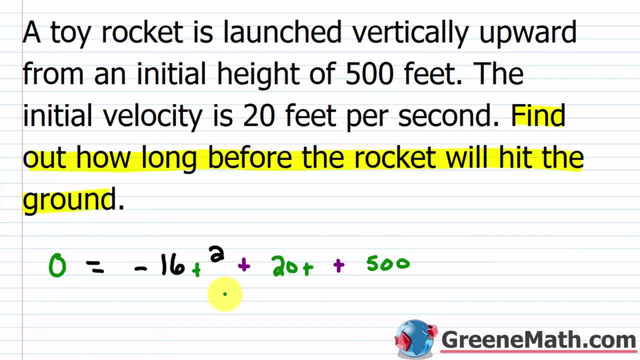 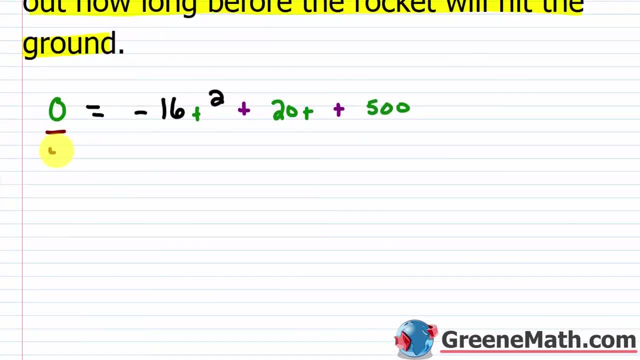 this particular one by factoring What I'm going to do. to make this a little bit simpler, I'm going to divide everything by four, just so we have smaller numbers to work with. So divide this by four, this by four, this by four and this by four. I'm going to get, and I'm also going to kind. 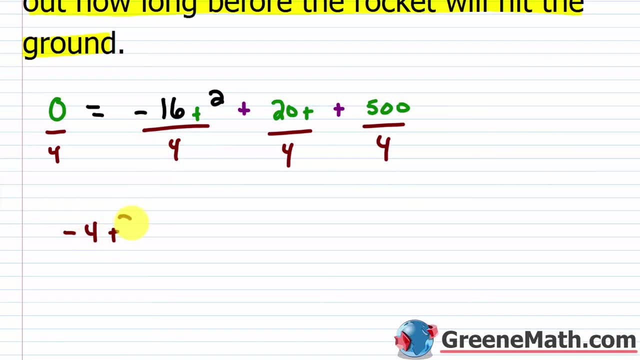 of rearrange things. So I'm going to get negative four T squared, then plus I'm going to have 20 over four is five, So five T, and then plus 500 divided by four is 125.. This equals zero, Okay. 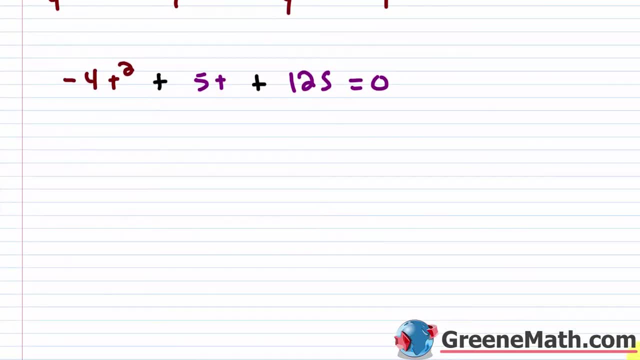 Let's go ahead and plug into the quadratic formula. So we know that, what We know, that this guy right here, this negative four, would be A. We know this guy right here, this five would be B and this guy would be C. Okay, This 125.. 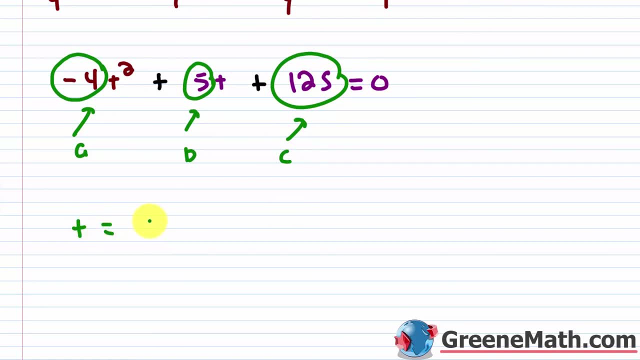 So instead of X we have T. So we're going to say T is equal to. you've got the negative of B: B is five. So negative five plus or minus the square root of you've got B squared Again: B is five. 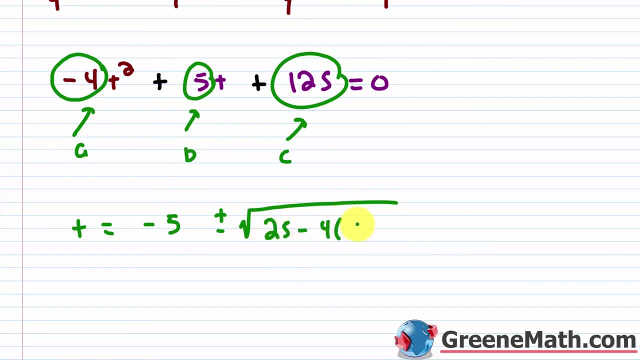 five squared is 25 minus four times A. A is negative four times C, C is 125.. And I'll do this in a minute. This is over 2A. A is negative four, So two times negative. four is negative eight. Okay, So negative four times negative four is plus 16.. So let's just put. 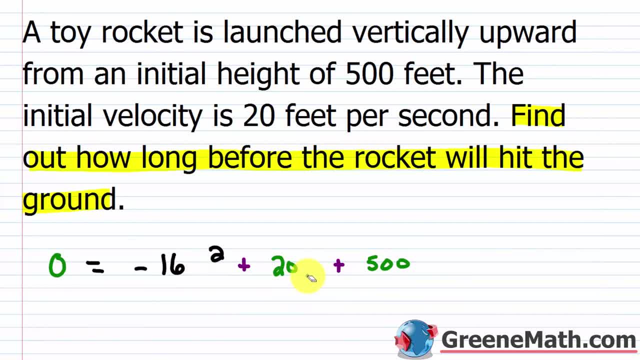 and I'm not going to keep it this way. I'm going to keep it with t because that's consistent with our formula. but if you were struggling and you couldn't, couldn't kind of grasp what's going on, just replace it with x, solve it and then go back and replace that for t. okay, not a big deal. so I 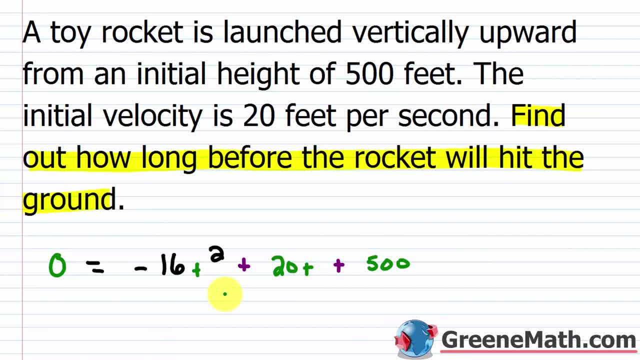 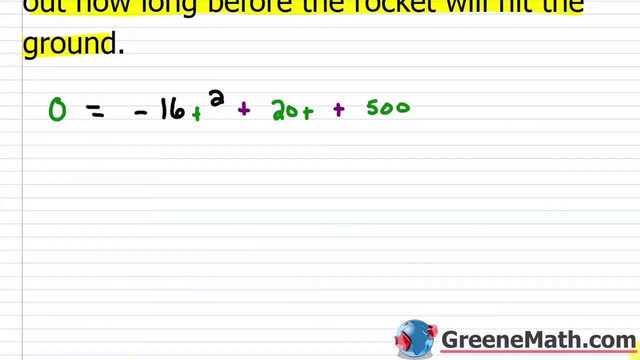 can solve this using the quadratic formula. I can also solve this particular one by factoring. what I'm going to do to make this a little bit simpler? I'm going to divide everything by 4, just so we have smaller numbers to work with. so divide this by 4, this by 4, this by 4 and this by 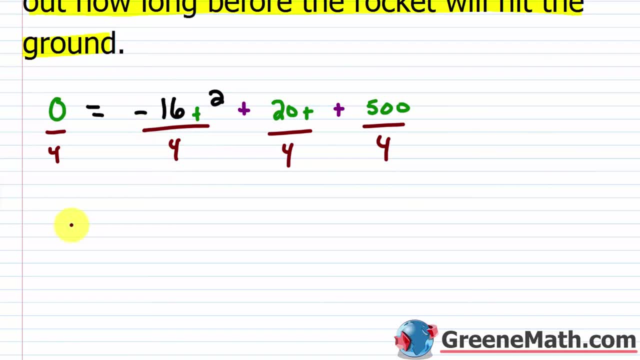 4 I'm going to get, and I'm also going to kind of rearrange things, so I'm going to get negative 4 t squared, then plus I'm going to have 20 over 4 is 5, so 5 t, and And then plus 500 divided by 4 is 125.. 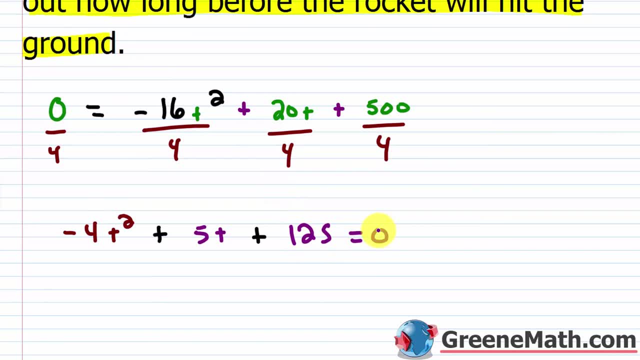 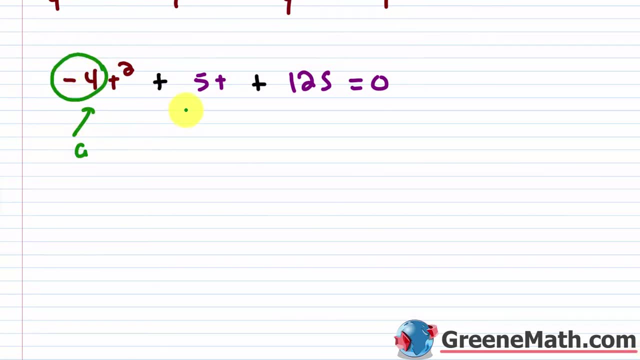 This equals 0.. Okay, let's go ahead and plug into the quadratic formula. So we know that what We know, that this guy right here, this negative 4 would be a. We know this guy right here: this 5 would be b. 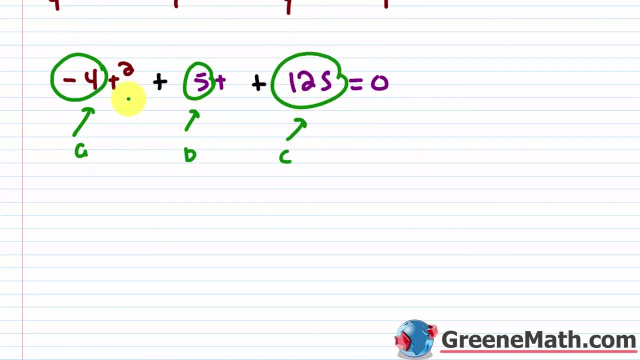 And this guy would be c. Okay, this 125.. So instead of x we have t. So we're going to say t is equal to: you've got the negative of b. b is 5, so negative 5, plus or minus the square root of. 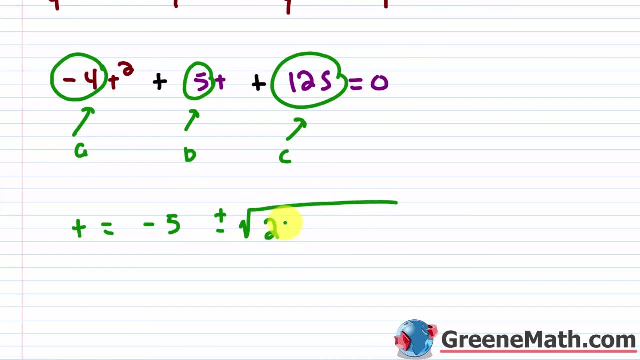 you've got b squared Again. b is 5,, 5 squared is 25.. Minus 4 times a, a is negative 4, times c c is 125.. And I'll do this in a minute. This is over. 2a. a is negative 4, so 2 times negative, 4 is negative 8.. 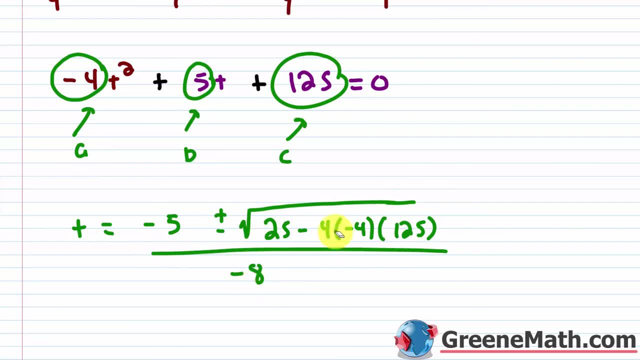 Okay so negative 4 times negative. 4 is plus 16.. So let's just put plus, you'd have 16 times 125.. That's going to be 2,000.. Okay so, 25 plus 2,000, you do this all in one shot. 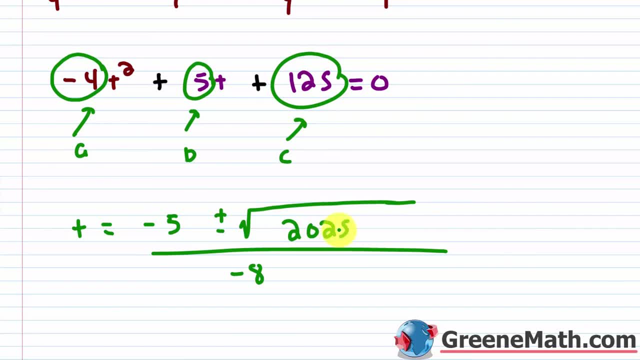 This is 2,025.. If you punch up square root of 2,025 on a calculator, you're going to get 45.. Okay, so this guy is 45.. Now one of these solutions you're going to throw out. okay. 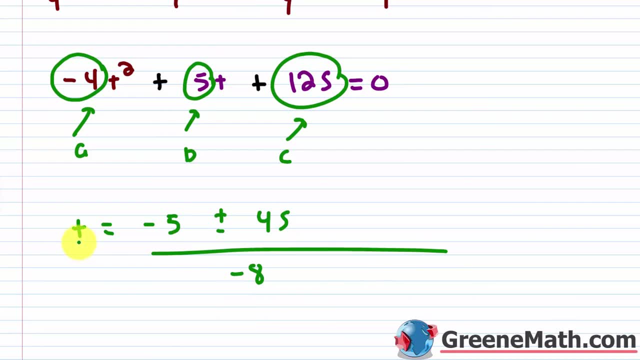 because we're solving for t, which is time, So it's got to be a positive value or zero. Okay, it's basically got to be non-negative. If you end up with something like negative 800 seconds, what does that mean? 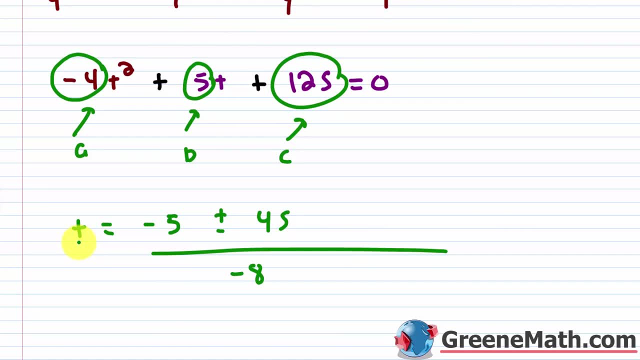 Right, it doesn't mean anything. Again, it's nonsense. We've seen that throughout this kind of lesson: If you get something that doesn't make sense, just reject it, throw it out. Okay, so the first one would be negative 5 plus 45.. 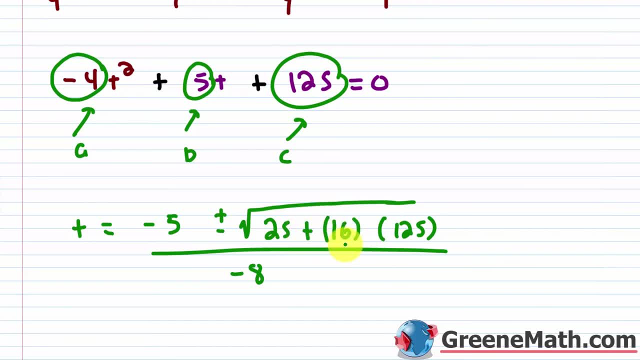 plus, you'd have 16 times 125.. That's going to be 2000.. Okay So, 25 plus 2000,. you do this all in one shot. This is 2025. If you punch up square root of 2025 on a calculator, 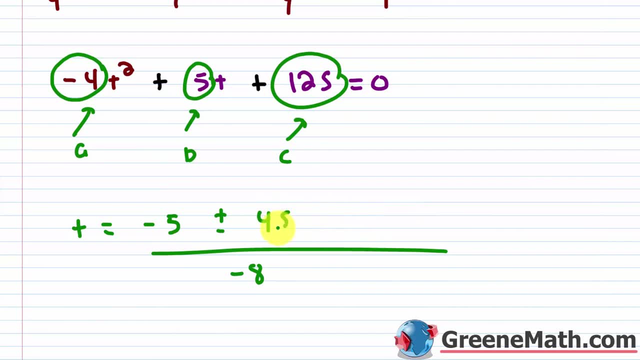 you're going to get 45. Okay, So this guy's 45.. Now, one of these solutions you're going to throw out. Okay, Because we're solving for T, which is time. So it's got to be a positive value or zero. 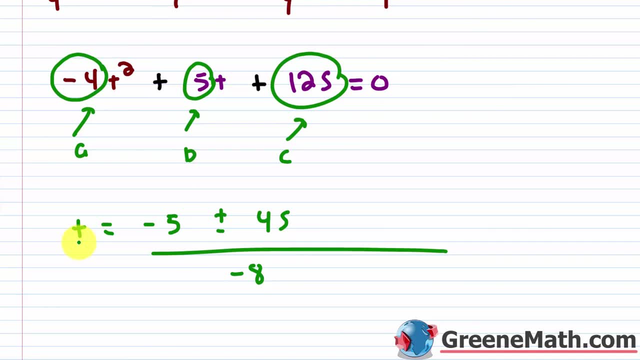 Okay, It's basically got to be non-negative. If you end up with something like negative 800 seconds, what does that mean? Right, It doesn't mean anything. Again, it's nonsense. We've seen that throughout this kind of lesson: If you get something that doesn't make sense, just reject. 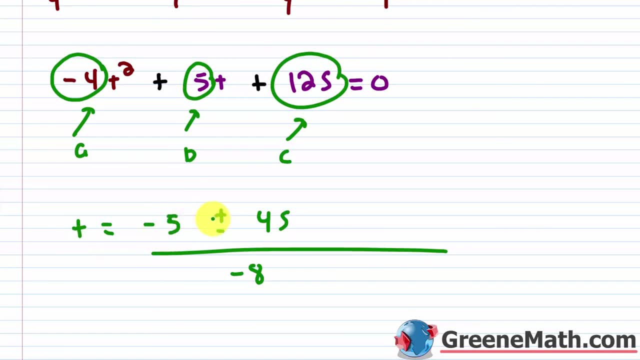 it throw it out. Okay, So the first one would be negative five plus 45. So let me kind of do that over here. So T equals so negative five plus 45,, which would be positive 40 over negative eight. This would end up giving me negative five seconds, which again doesn't. 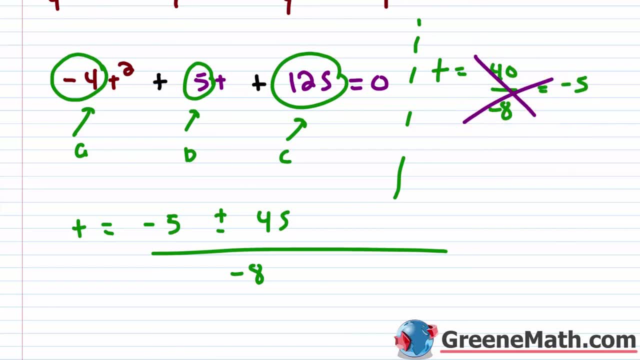 make sense. So we're just going to throw that solution out. Okay, We don't need it. Then T is equal to the other. one is negative five minus 45,, which would be negative 50. And then, divided by negative, eight- negative over negative is positive. I can also simplify by dividing each: 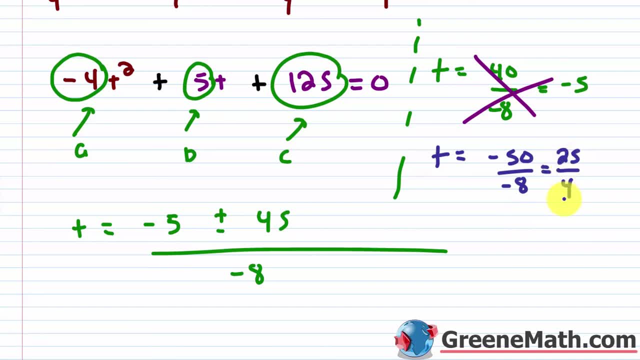 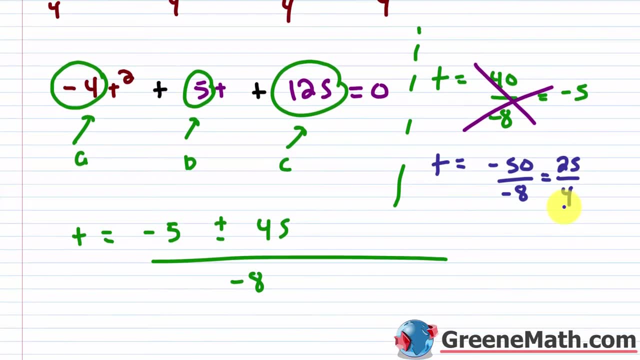 by two, So this would end up being 25 fourths. Now, in decimal form, that's 6.25.. And that's what we're going to use. So let me erase all this. We don't need any of it anymore. So find out. 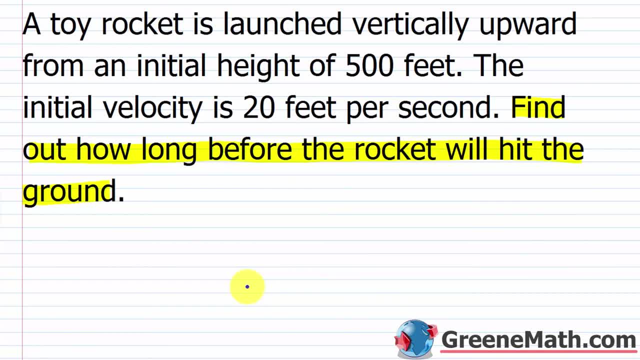 how long before the rocket will hit the ground. Well, we found that it's going to happen at 6.25 seconds, right? So we'll say that the rocket will hit the ground at 6.25 seconds. Okay, And again. 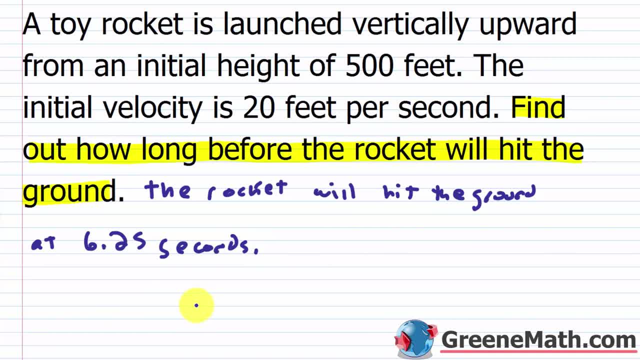 a very, very easy problem, Very, very easy. If you get this question on homework or tests, you just plug into the formula and you're basically just have to set up your quadratic equation and solve. Okay, So how about checking something like this? What would we do? Well, again, we just go through. 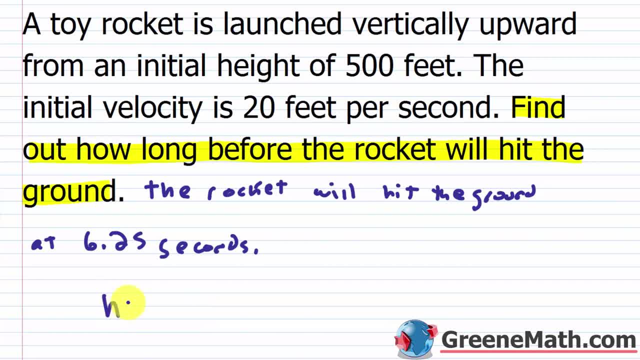 the formula again. It's H is equal to: we have your negative 16 times T. squared For T, I've got 6.25.. Again, I can plug in a fractional form here to make it a little simpler. So I'm going to put: 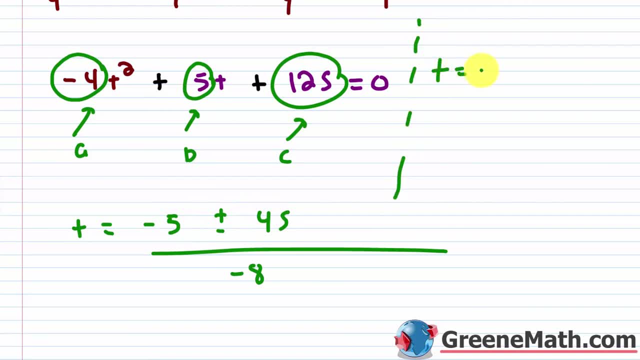 So let me kind of do that over here. So t equals so negative 5 plus 45,, which would be positive 40 over negative 8. This would end up giving me negative 5 seconds, which again doesn't make sense. 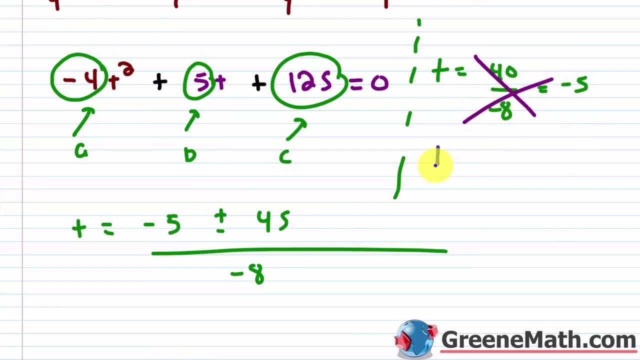 So we're just going to throw that solution out. Okay, we don't need it. Then t is equal to the other. one is negative 5 minus 45,, which would be negative 50. And then, divided by negative, 8, negative over negative is positive. 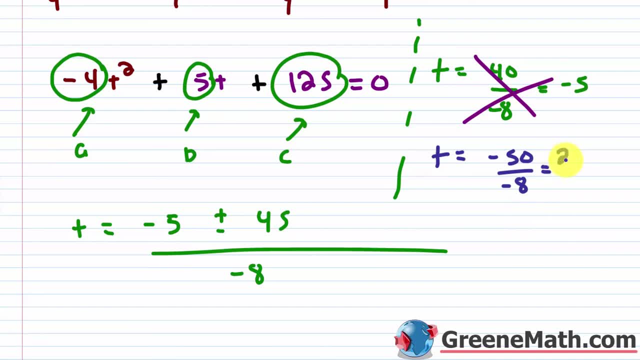 I can also simplify by dividing each by 2.. So this would end up being 25.. Now, in decimal form, that's 6.25, and that's what we're going to use. So let me erase all this. We don't need any of it anymore. 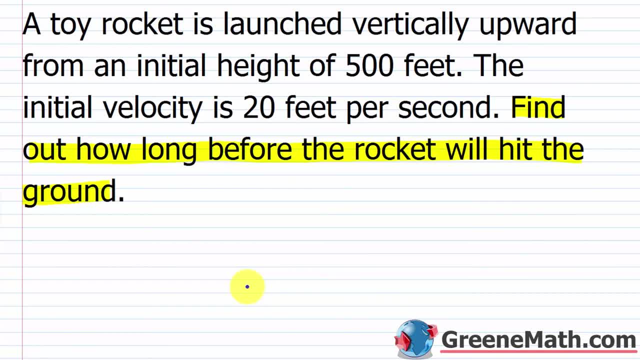 So find out how long before the rocket will hit the ground. Well, we found that it's going to happen at 6.25 seconds, right? So we'll say that the rocket will hit the ground at 6.25 seconds, okay? 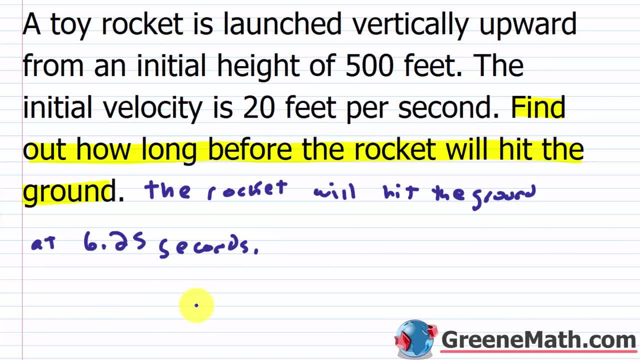 And again, a very, very easy, Very, very easy. if you get this question on homework or tests, You just plug into the formula and you basically just have to set up your quadratic equation and solve. Okay, so how about checking something like this? 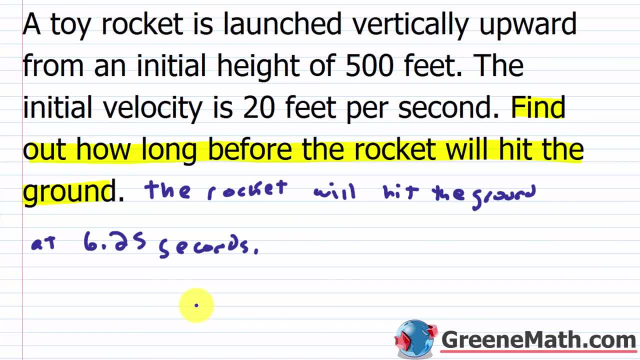 What would we do? Well, again, we just go through the formula. again, It's h is equal to. we have your negative 16 times t. squared For t, I've got 6.25.. Again, I can plug in a fractional form here to make it a little simpler. 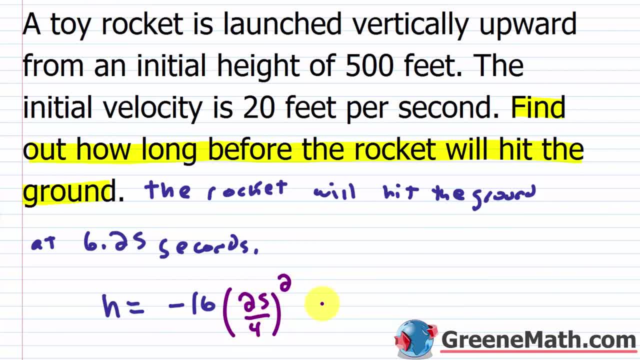 So I'm going to put 25 fourths. this guy squared. Then, plus v sub zero, the initial velocity was 20.. So we're going to put 20 times. You've got your t, which, again, I'm going to put 25 fourths for that. 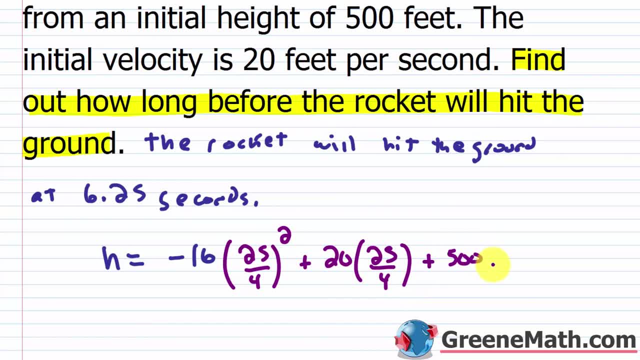 And then you've got plus your s sub zero, which is 500.. That was the initial height in feet, So that's 500 feet. Okay, so h is supposed to be zero. So we just check this, make sure we got the right answer. 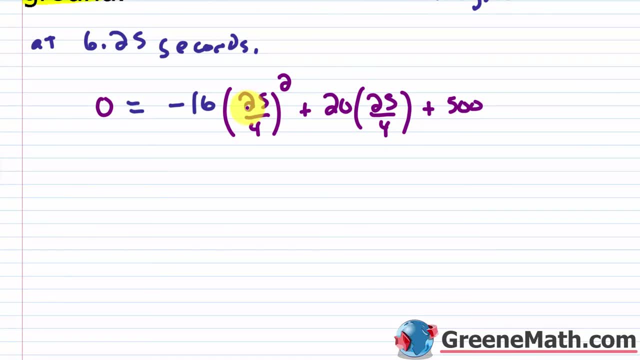 So let's go back down. So 25 squared is 625, 4 squared is 16.. So this would be 625.. I'm going to write that A little better. So 625 over 16.. This guy is going to cancel with this guy and give me a negative one.